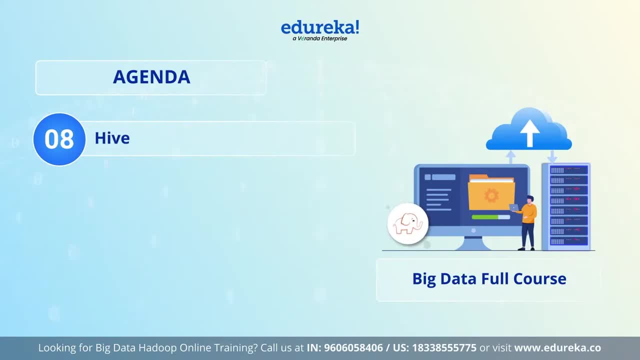 with Hadoop. Then we have hive, a data warehousing and SQL like query language for Hadoop. After that we have HB, A NoSQL database that runs on top of Hadoop and it is used for real-time data accessing and analysis. 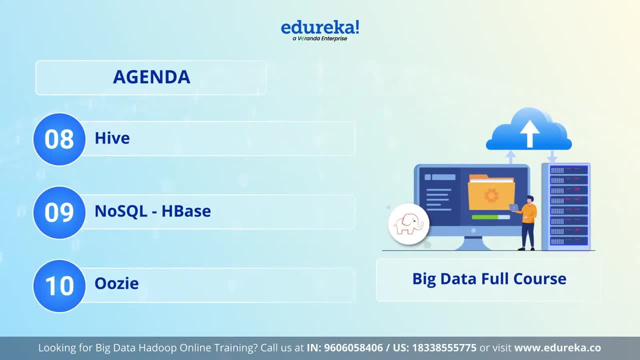 And after that we will learn about Uzi, which is used to manage and coordinate Hadoop jobs. After that, we will dive into some of the popular Hadoop projects, which will give you an understanding of how these technologies are being used in these industries. We will also cover the career. 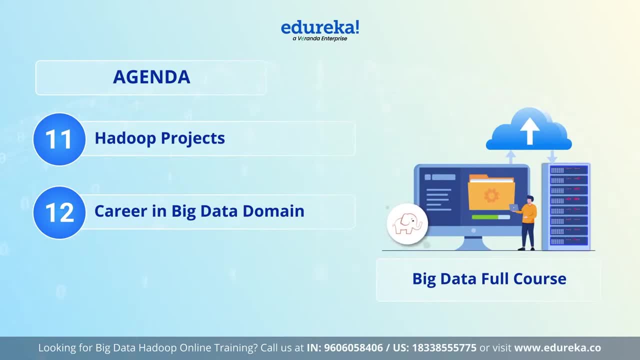 opportunities in the big data domain and tips to prepare for big data Hadoop interview questions. By the end of this full course, you will have a plenty of opportunities for hands-on practice and you will have a solid understanding of Hadoop ecosystem and be well prepared to work with the. 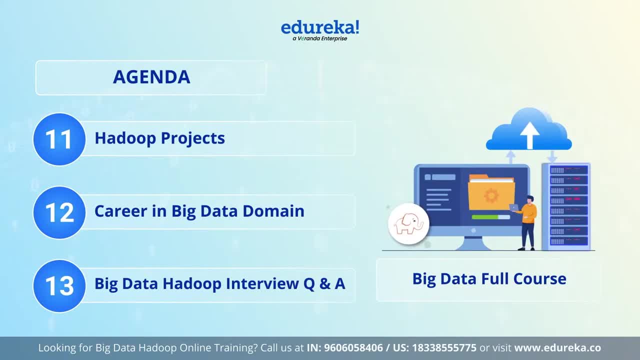 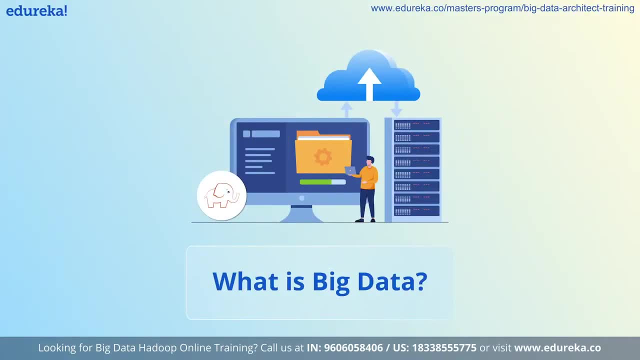 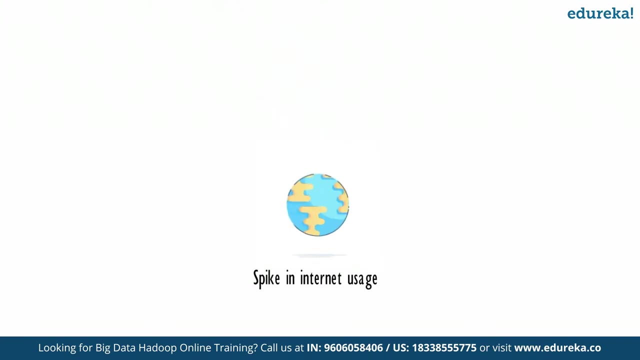 big data in professional setting. So let us get started with our first topic, that is, what is big data? What is big data With the spike in internet usage and other technologies such as IoT devices, mobile phones, autonomous devices like robotics, drones, vehicles, appliances? 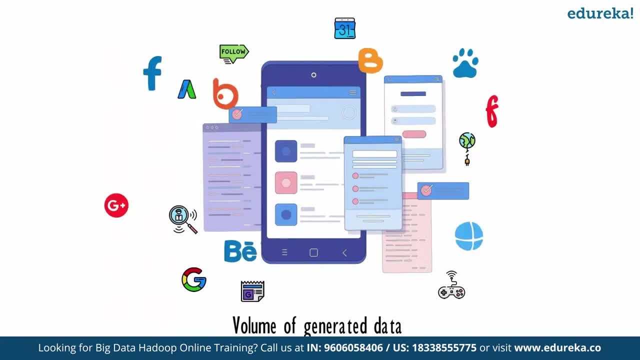 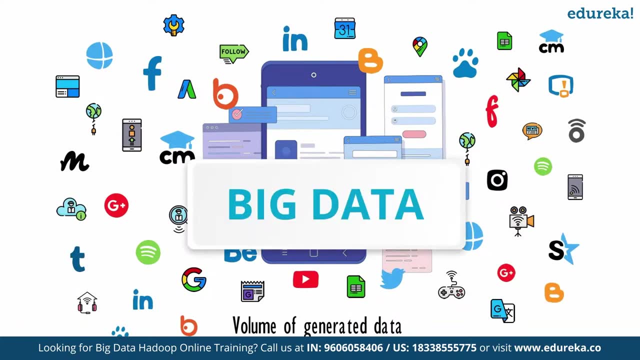 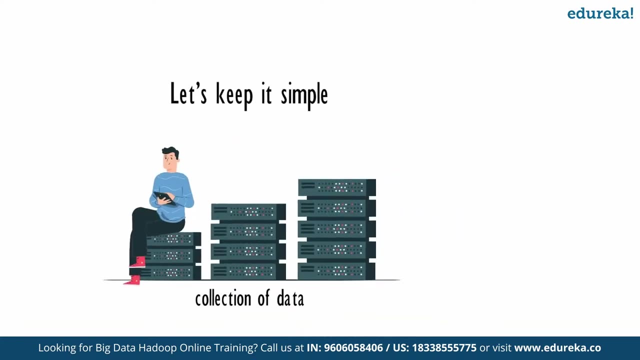 the volume of generated data is growing exponentially at an unprecedented rate. This constant increase in the amount of data generated has led to the emergence of big data. So what is big data? Let's keep it simple. Big data refers to a collection of data that is so huge and complex that none of the traditional 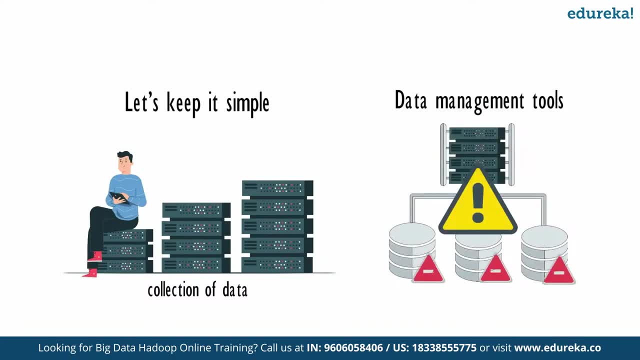 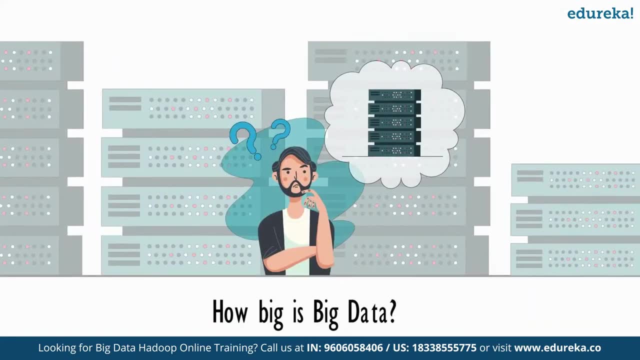 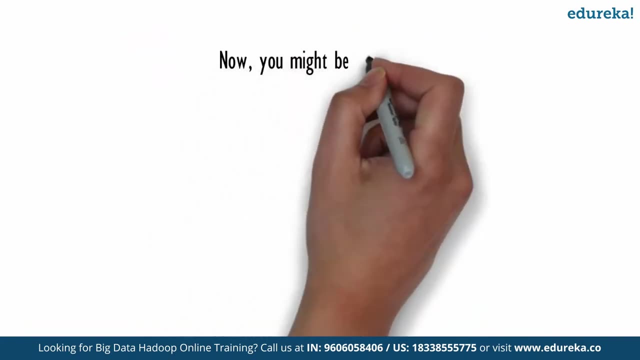 data management tools are able to store it or process it efficiently. Now you know that big data involves lots of data, but have you ever stopped to think about just how big is big data? According to Forbes, there are 2.5 quintillion bytes of data created every day. Now you might. 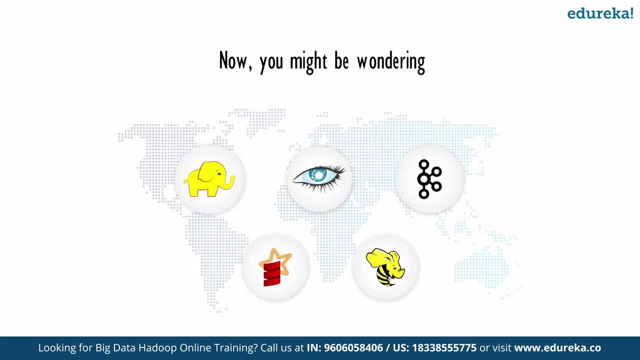 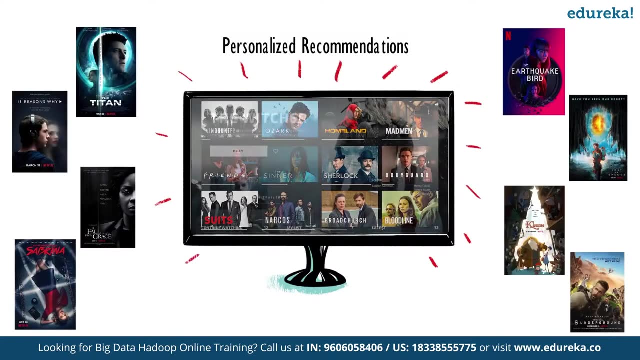 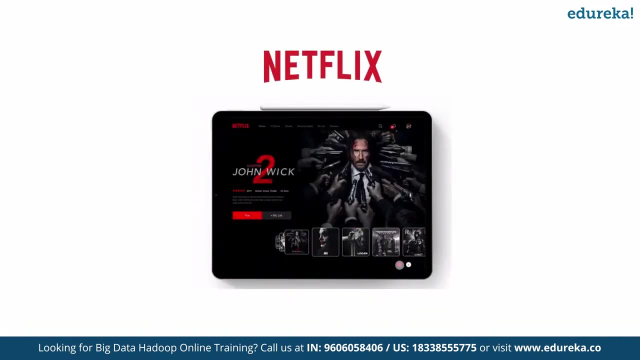 be wondering how big data tools manage to handle such a huge amount of data. When Netflix offers you personalized recommendations from its library of thousands of movies & tv shows, that's big data at work. Big data helps Netflix determine which programs may be of interest to you and the recommendation. 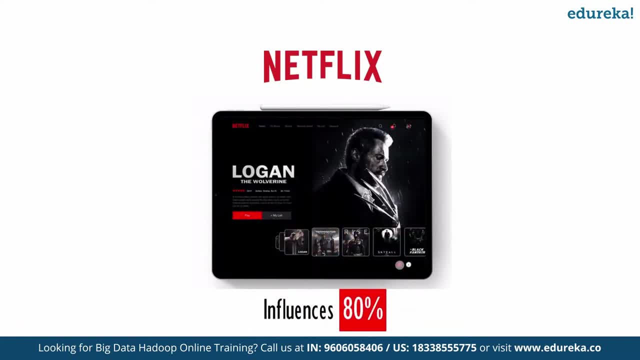 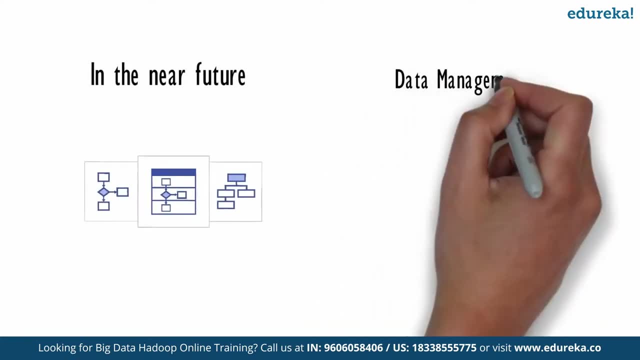 system actually influences 80% of the content we watch on Netflix. In the near future, with the growing increase in the volume of data, big data will grow bigger and the demand for data management experts will shootup The gap between the demand for data professionals and their availability for thearker. Nazi AI isپeoolifty 58 00. 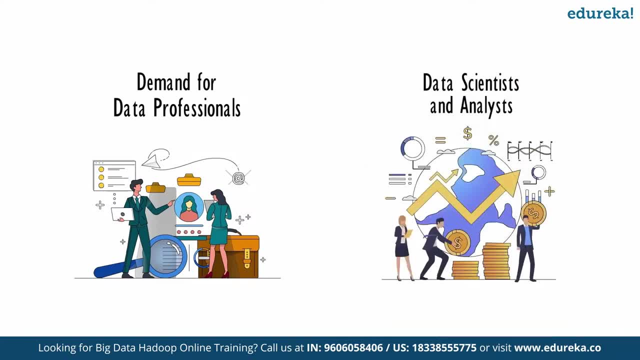 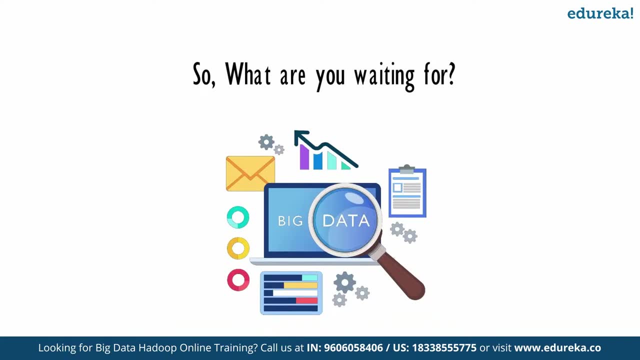 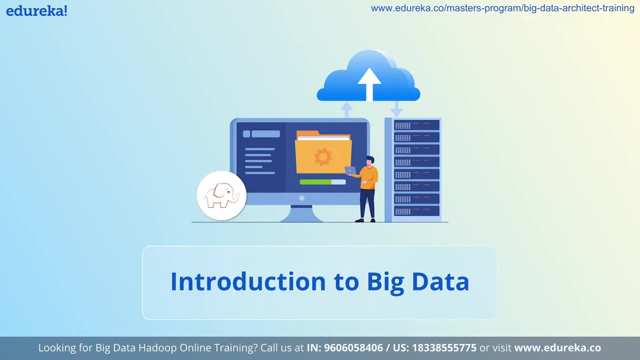 Bill Wieden. This will help data scientists and analysts draw higher salaries. So what are you waiting for? Drive into the world of big data and towards a brighter future. Now, I feel, Saurabh, it's the best time to tell the story about how data evolved and how big data. 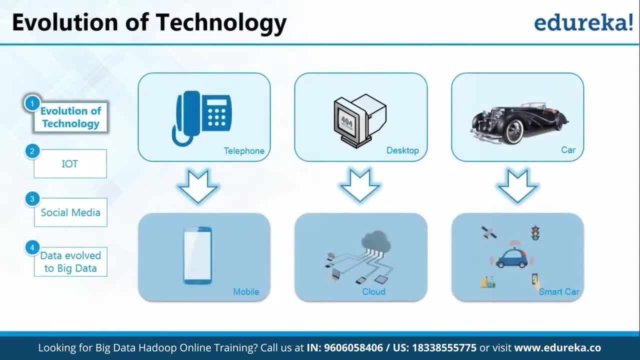 came Fine, Reshma, so we'll move forward. So, Saurabh, what can you notice here, Reshma? I see how technology has evolved. Earlier we had landline phones, but now we have smartphones, We have Android, we have iOS that are making our lives smarter, as well as our phones smarter, Apart from 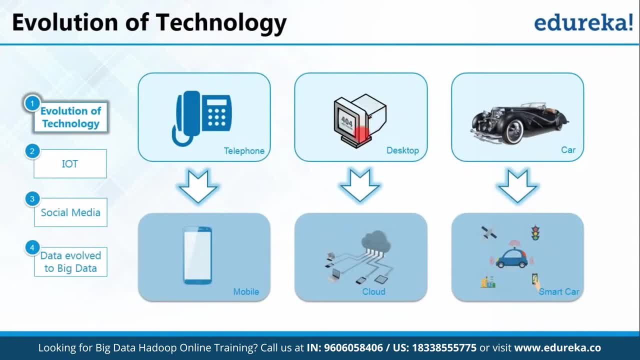 that we were also using bulky desktops for processing MBs of data. Now, if you can remember, we were using floppies and you know how much data it can store, right. Then came hard disk for storing TBs of data, and now we can store data on cloud as well, And similarly, nowadays even. 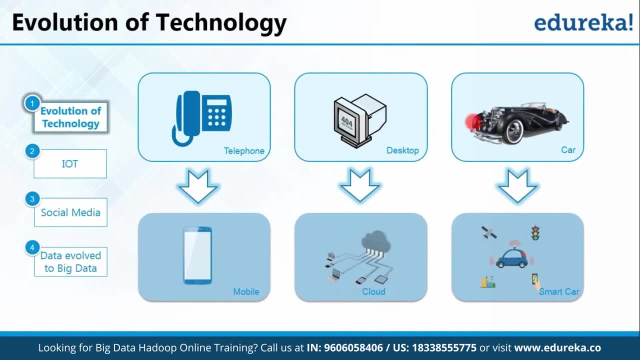 self-driving cars have come up. I know you must be thinking: why are we telling you this? I know you must be thinking: why are we telling you this Now? if you notice, due to this enhancement of technology, we're generating a lot of data, So 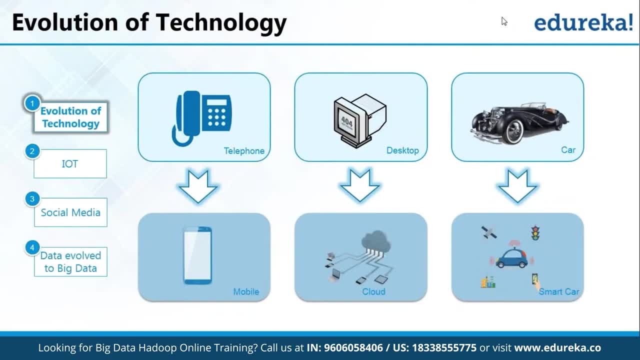 let's take the example of your phones. Have you ever noticed how much data is generated due to your fancy smartphones, Your every action, even one video that is sent through WhatsApp or any other messenger app that generates data. Now, this is just an example. You have no idea how much data. 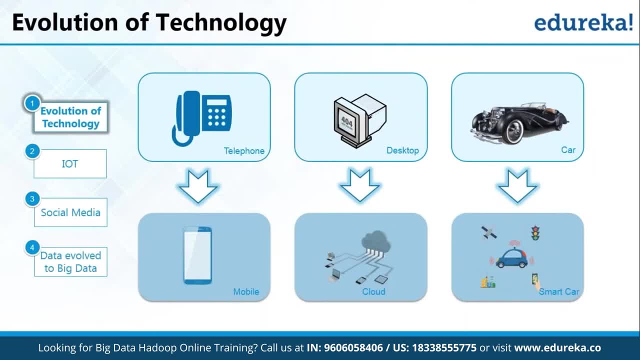 you're generating because of every action you do. Now the deal is this: data is not in a format that our relational data can store. It's not in a format that our relational data can store. It's not in a format that our relational data can store. It's not in a format that our relational data can. 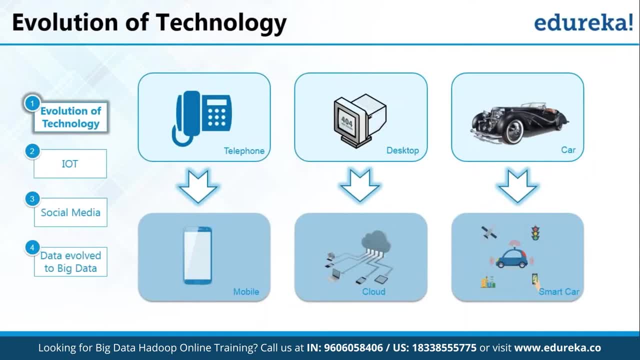 handle, And, apart from that, even the volume of data has also increased exponentially. Now I was talking about self-driving cars, So basically these cars have sensors that records every minute details like the size of the obstacle, the distance from the obstacle and many more, And 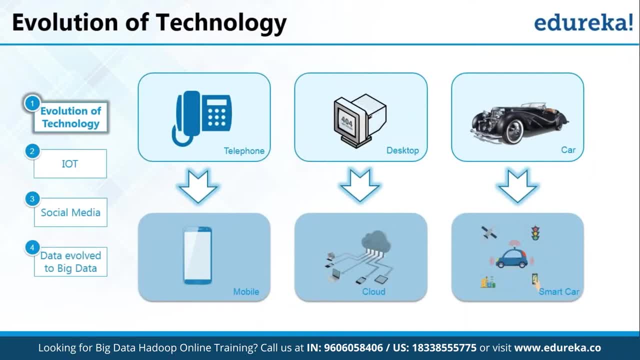 then it decides how to react. Now you can imagine how much data is generated for each kilometer that you drive on that car. I completely agree with you, Reshma. So let's move forward and focus on various other factors behind the evolution. 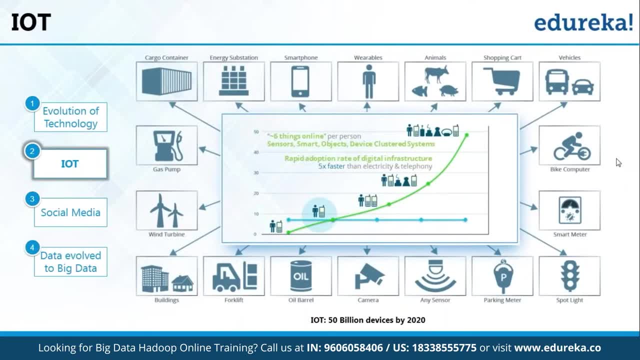 I think you guys must have heard about IoT. If you can recall the previous slide, we were discussing about self-driving cars. It is nothing but an example of IoT. Let me tell you what exactly it is. IoT connects your physical device with internet and makes the device smarter. So nowadays, if you have noticed, we have 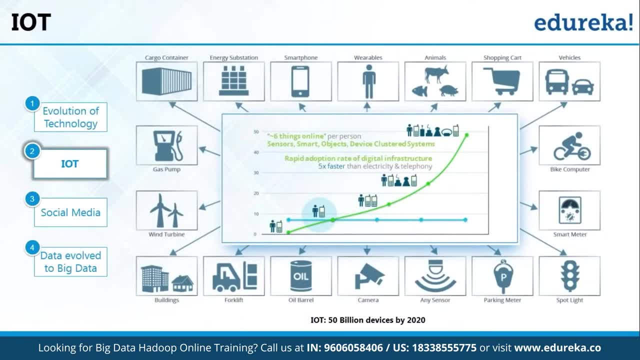 smart ACs, TVs, etc. So we'll take the example of smart air conditioners. So this device actually monitors your body temperature and the outside temperature and accordingly decides what should be the temperature of the room. Now, in order to do this, it has to first accumulate data From where It can. 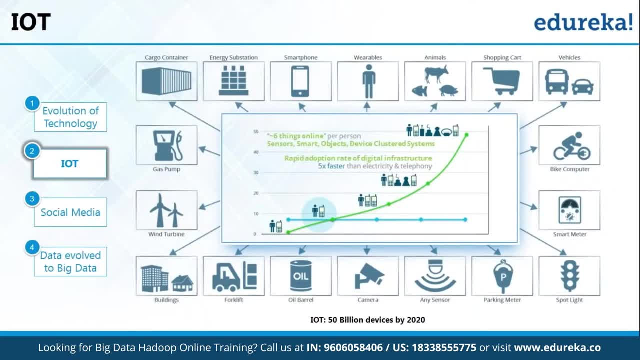 accumulate data from internet through sensors that are monitoring your body temperature and the surroundings, So basically, from various sources that you might not even know about. it is actually fetching that data and accordingly it decides what should be the temperature of your room. Now we can. 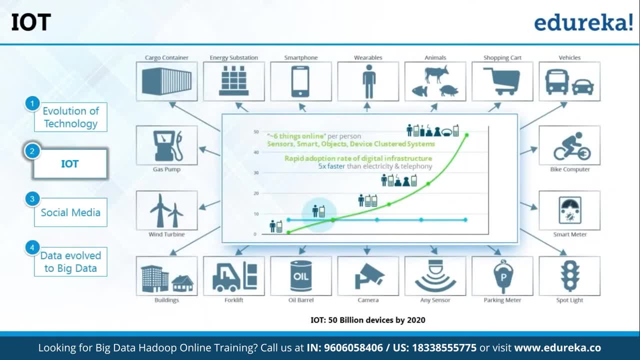 actually see that because of IoT we are generating a huge amount of data. Now there is one stat also that is there in front of your screen. So if you notice, by 20 years you can actually see the 20- will have 50 billion IoT devices. So I don't think so I need to explain much that how IoT is. 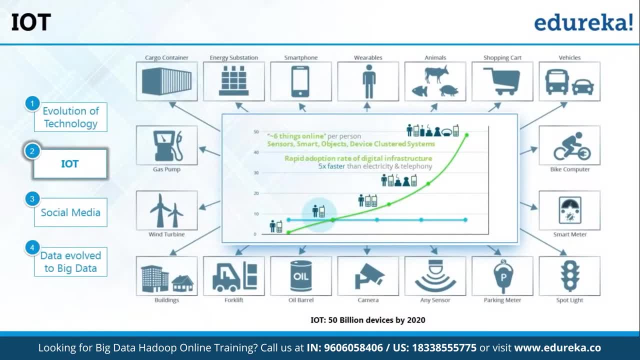 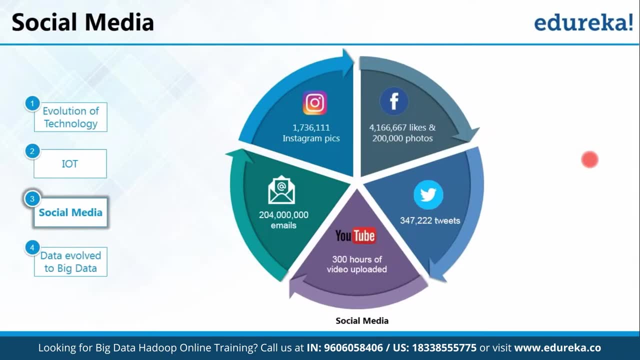 generating huge amount of data. So we'll move forward and focus on one more factor, that is, social media. Now, when we talk about social media, I think Reshma can explain this better. right, Reshma? Yes, Aurob, but I'm pretty sure that even you use it. So let me tell you that social media is actually 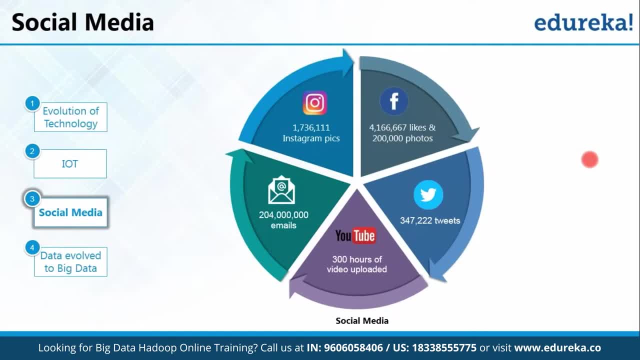 one of the most important factor in the evolution of big data. So nowadays everyone is using Facebook, Instagram, YouTube and a lot of other social media websites, So these social media sites have so much data. For example, it will have your personal details like your name, age and apart from that. 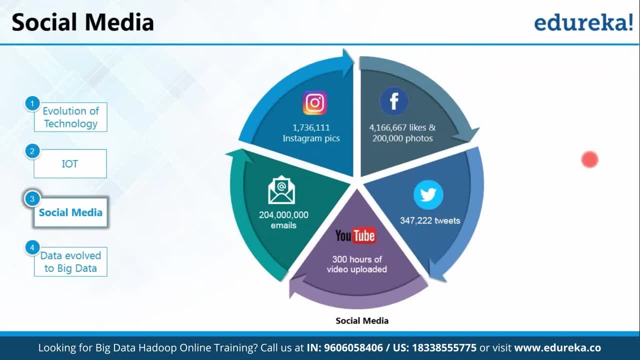 even each picture that you like or react to also generates data, And even the Facebook pages that you go around liking. that is also generating data, And nowadays you can see that most people are sharing videos on Facebook, So that is also generating huge amount of data And the 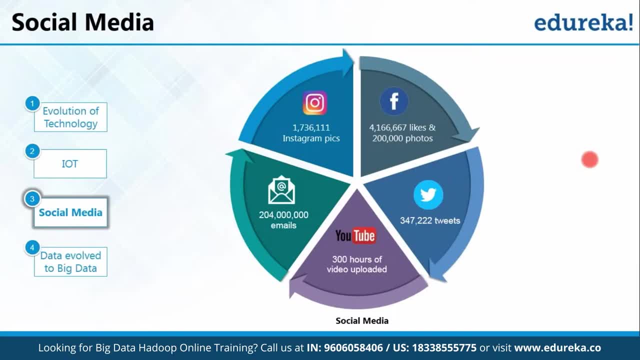 most challenging part here is that the data is not present in a structured manner and, at the same time, it is huge in size. Isn't that right, Aurob? Can't agree more. The point you made about the form of data is actually one of the biggest factor for the evolution of big data. So, due to all these reasons that we 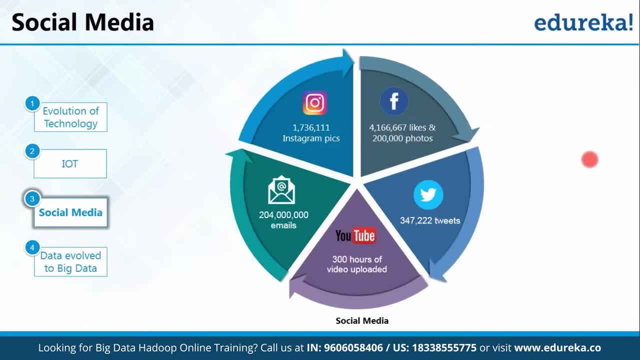 have discussed have not only increased the amount of data, but it has also shown us that data is actually getting generated in various formats. For example, data is generated with videos. that is well, So there are numerous- or you could say millions- of ways in which data is getting generated. 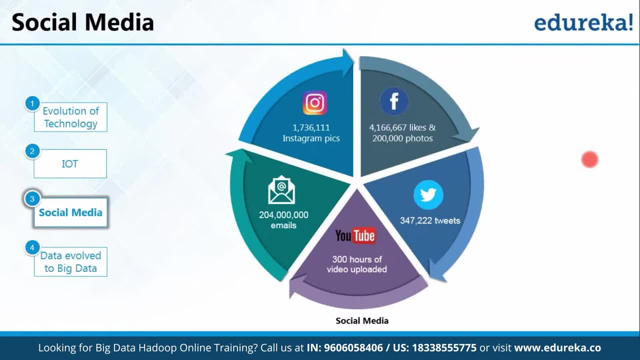 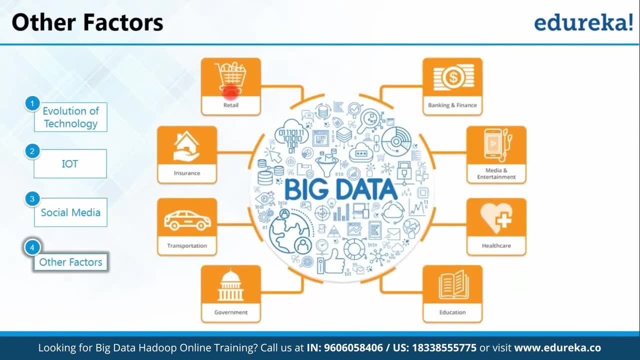 nowadays? Absolutely, And these are just a few examples that we have given you. There are many other driving factors for the evolution of data, So these are a few more examples because of which data is evolving and converting to big data. We'll discuss about the retail part. I'm pretty sure that 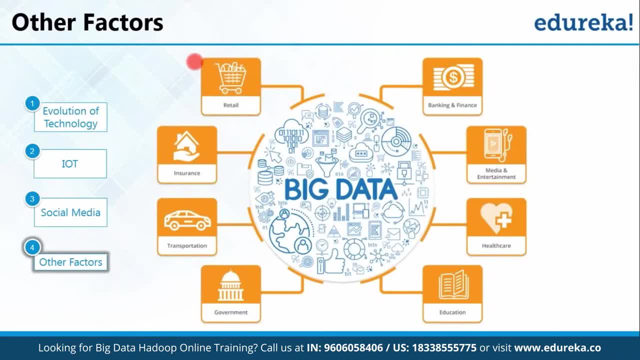 all of you must have visited websites like Amazon, Flipkart, etc. And Reshma, I know you visited a lot of times. Yeah, I do, And suppose Reshma wants to buy shoes, So she won't just directly go buy shoes, She'll search for a lot. 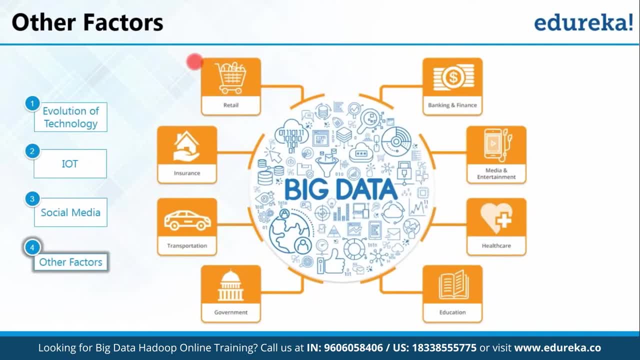 of shoes. So somewhere her search history will be stored, And I know for sure that this won't be the first time that she's buying something. So there will be her purchase history as well, along with her personal details, And there are numerous ways in which she might not even know that she's. 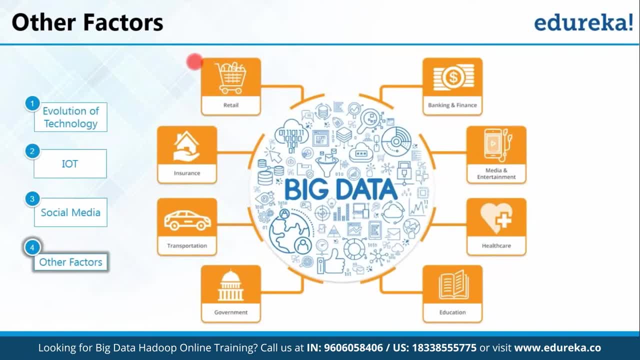 generating data, And obviously Amazon was not present earlier, So at that time there is no way that such huge amount of data was generated. Similarly, the data has evolved due to other reasons as well, like banking and finance, Media and entertainment, etc. etc. So now the deal is: what exactly is big data? How do we consider? 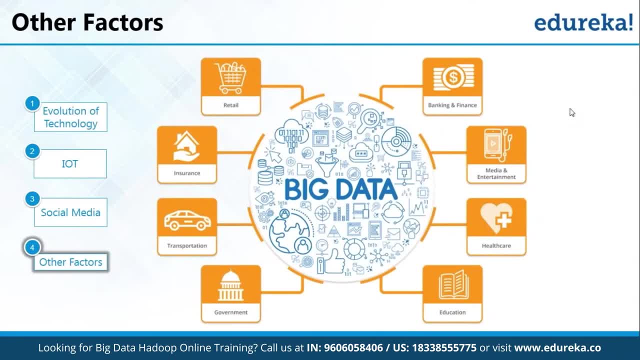 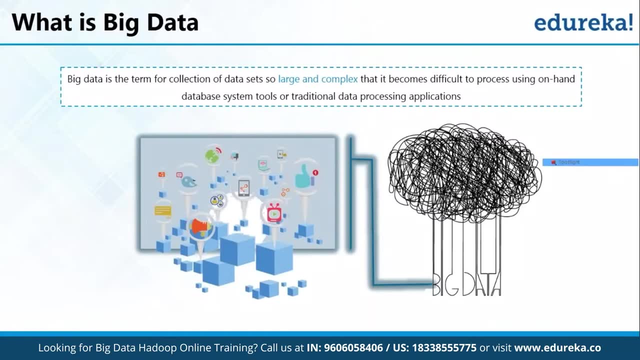 data as big data, So let's move forward and understand what exactly it is. OK, Now let us look at the proper definition of big data, even though we've put forward our own definitions already, So sort of why don't you take us through it? 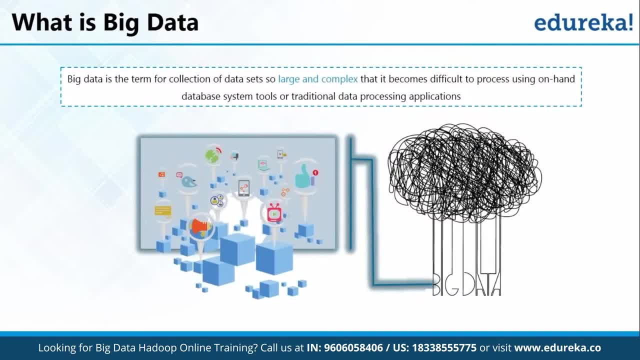 Yes, Reshma Sure. So big data is a term for collection of data sets so large and complex that it becomes difficult to process Using on hand database system tools or traditional data processing applications. OK, So what I understand from this is that our traditional systems are a problem because they're too. 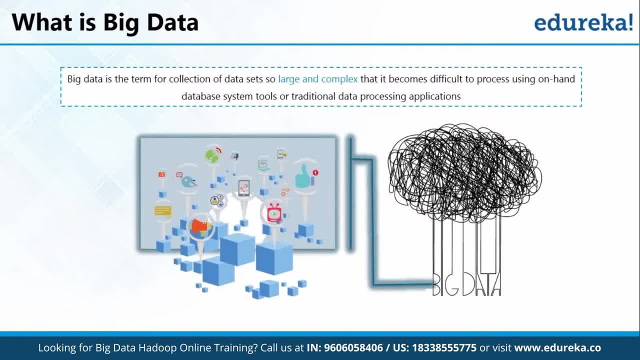 old fashioned to process this data or something? No, Reshma. The real problem is there is too much data to process. When the traditional systems were invented in the beginning, we never anticipated that we would have to deal with such enormous amount of the data. It's like a disease infected on you. 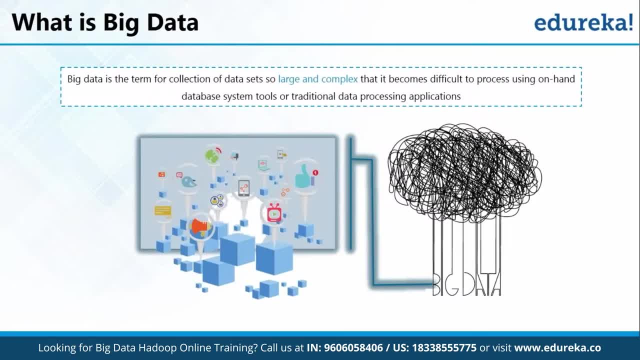 You don't change your body orientation when you get infected with the disease. Right, Reshma, You cure it with medicines. Couldn't agree more sort of. Now the question is: how do we consider some data as big data? How do we classify some data as big data? 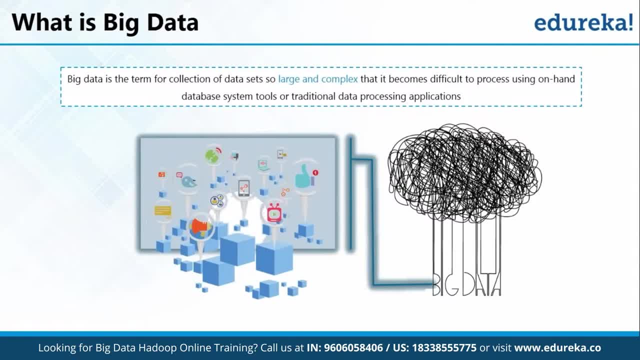 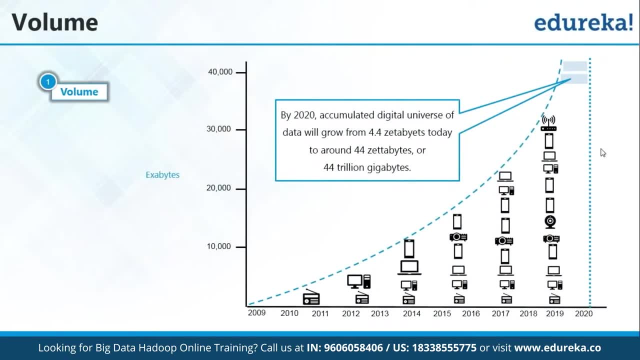 How do we know which kind of data is going to be hard for us to process? Well, sort of. we have the five V's to tell us that. So let's take a closer look at what are those. So, starting with the first V, it's the volume of data. 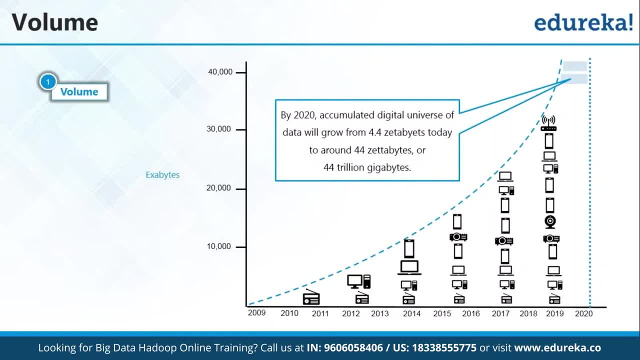 It's tremendously large. So if you look at the stats here, you can see the volume of data is rising exponentially. So now we are dealing with just 4.4 zettabytes of data and by 2020- just in three years- it's expected that the data will rise up to 44 zettabytes, which is like equal to 44 trillion gigabytes. 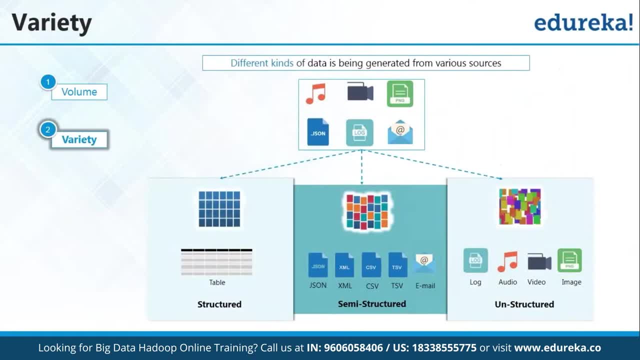 So that's really, really huge. It is because all these humongous, all this humongous data is coming from multiple sources, and that is the second V, which is nothing but variety. We deal with so many different kinds of files at all once. 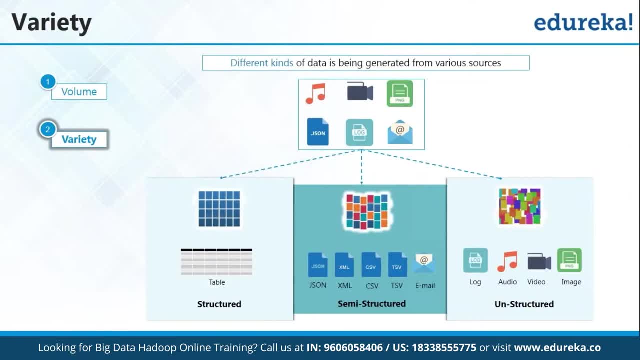 There are MP3 files, videos, JSON, CSV, TSV and many more. Now these are all structured, unstructured and semi structured altogether. Now let me explain this with the diagram that is there on your screen. So over here we have audio, we have video files, we have PNG files, we have JSON log files, e-mails, various. 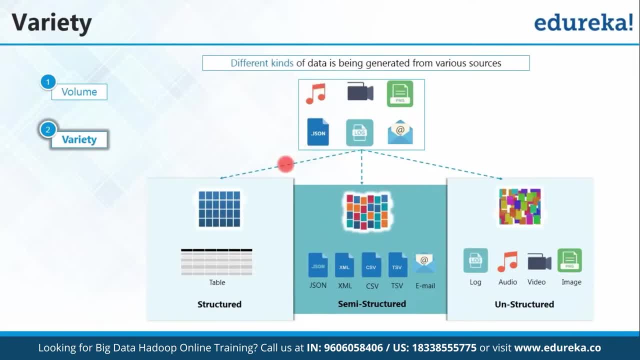 formats of data. Now this data is classified into three forms. One is structured format. Now, in structure format you have a proper schema for your data, So you know what all columns will be there and basically you know the schema about your data. So it is structured, it is in a structured format, or you can say in a tabular format. 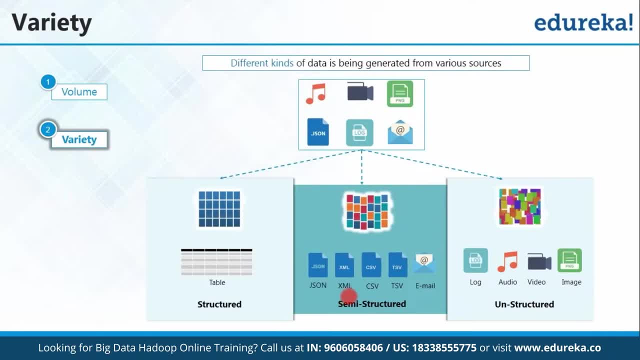 Now, when we talk about semi structured files, these are nothing but JSON, XML and CSV files where schema is not defined properly. Now, when I go to unstructured format, we have log files here, audio files, videos and images, So these are all considered as unstructured files. 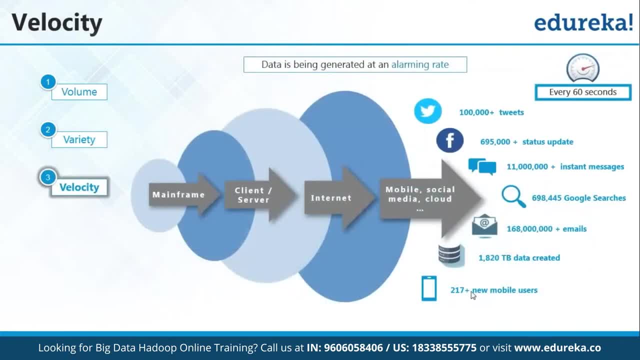 And Saurabh. it is also because of the speed of accumulation of all this variety of data altogether which brings us to our third V, which is velocity. So if you look here, earlier we were using mainframe systems: huge computers but less data, because there were less people working with computers at that time. 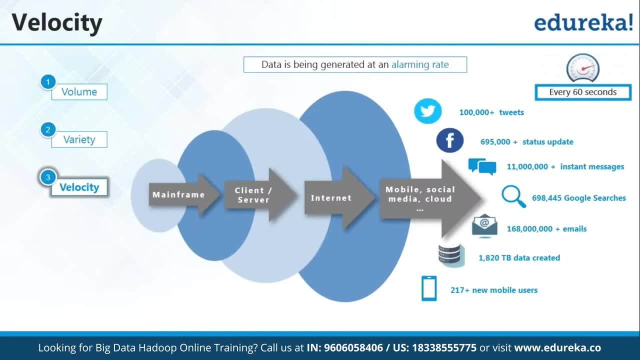 But as computers evolved and we came to the client server model, the time came for the web applications and the Internet boomed. and as it grew among the masses, the web applications got increased over the Internet and everyone started using all these applications, and not only from their computers and also from mobile devices. 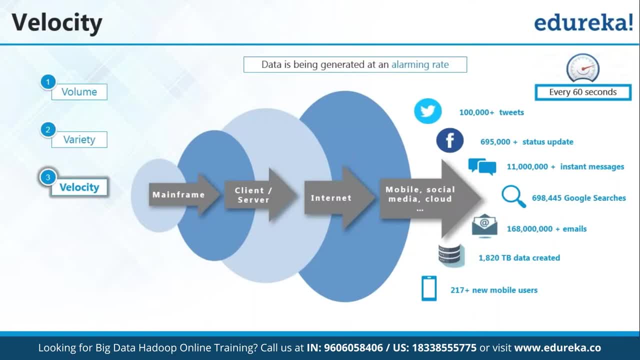 So more users, more appliances, more apps and hence a lot of data. And when you talk about people generating data, or Internet Reshma, the one kind of application that strikes first in the mind is social media. So you tell me how much data you generate alone with your Instagram posts and stories. 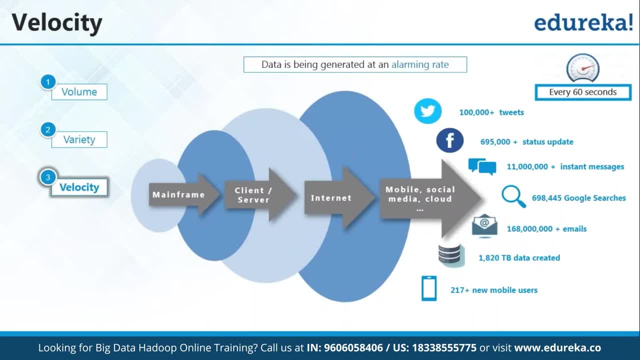 It will be quite a boast if I only talk about myself here. So let's talk, including every social media user. So if you see the stats In front of your screen, you can see that for every 60 seconds there are one hundred thousand tweets- actually more than one hundred thousand tweets- generated in Twitter every minute. 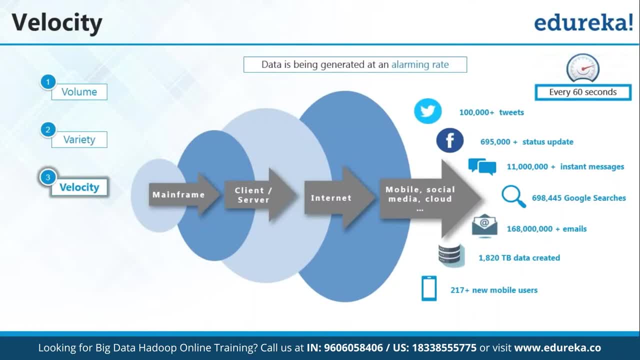 Similarly, there are six hundred ninety five thousand status updates on Facebook. We talk about messaging. There are eleven million messages generated every minute And similarly, there are six hundred and ninety eight thousand four hundred forty five Google searches. one sixty eight million e-mails And that. 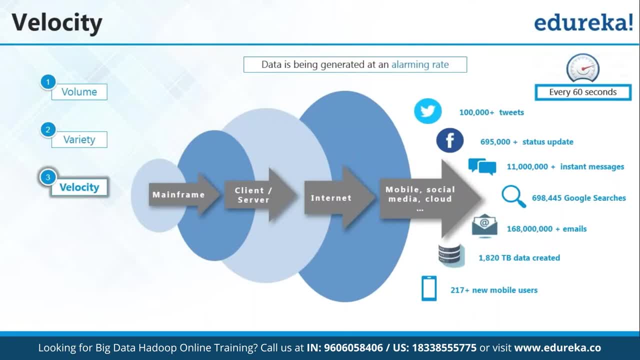 Goes to almost one thousand eight hundred twenty terabytes of data, And obviously the number of mobile users are also increasing every minute And there are two hundred and seventeen plus new mobile users every 60 seconds. Geez, that's a lot of data. 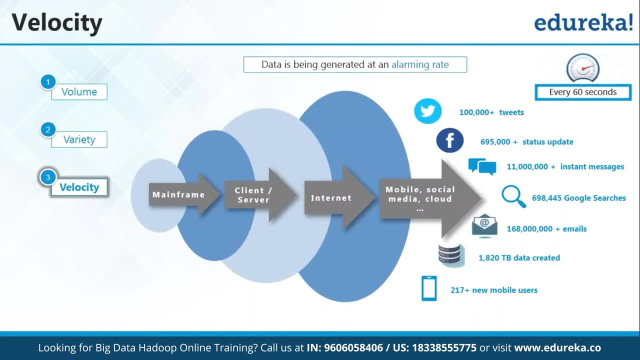 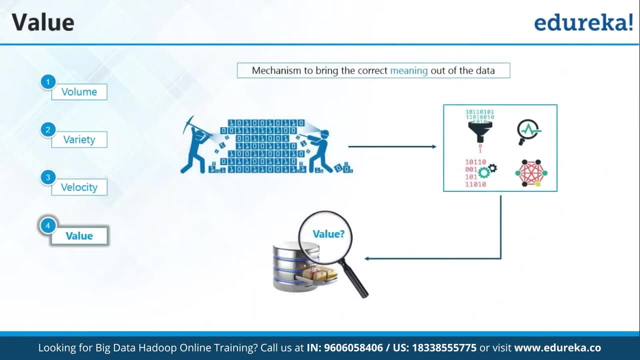 I don't even want to go ahead and calculate the total. it would actually scare me. Yeah, that's a lot. Now the bigger problem is how to extract the useful data from here, And that's when we come to our next tweet. that is value. 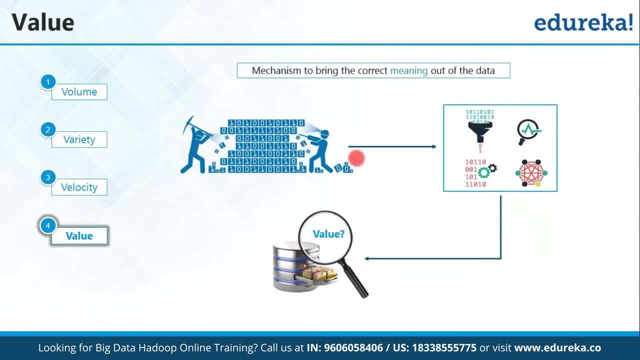 So over here what happens? first you need to mine the useful content from your data. Basically, you need to make sure that you have only useful fields in your data set. After that you perform certain analytics or you say you perform certain analysis on that data that you have clean and you need to make sure that, whatever analysis you have done, 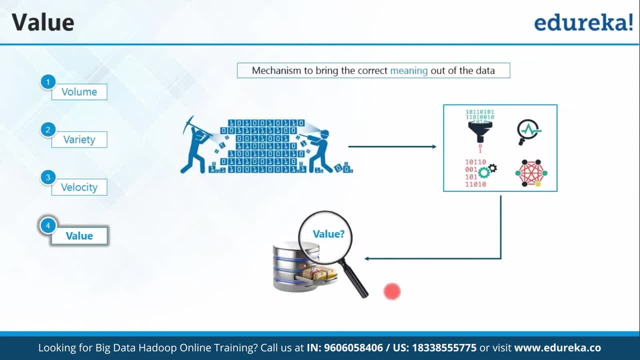 it is of some value, that is, it will help you in your business to grow. It can basically find out certain insights which were not possible earlier. So you need to make sure that whatever big data that has been generated, or whatever data that has been generated, it makes sense. 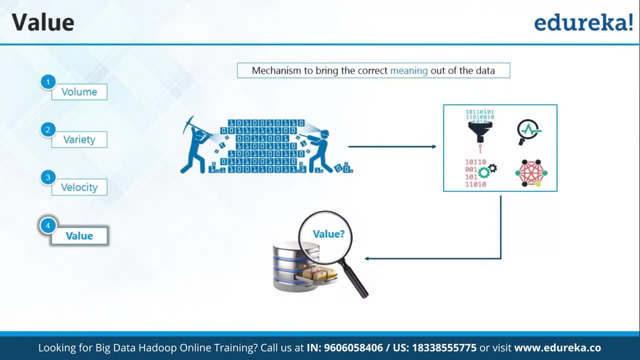 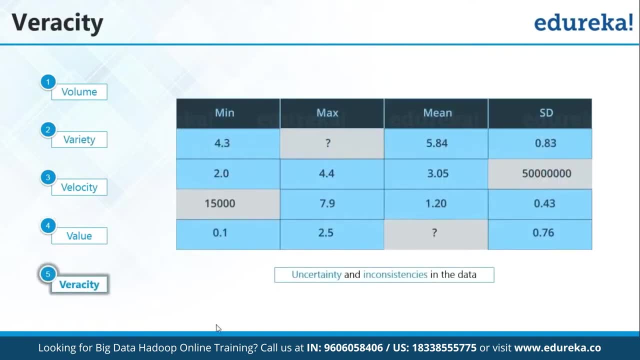 It will actually help your business to grow and it has some value to it. Now, getting the value out of this data is one big challenge. Let me tell you why, And that brings us to our next tweet, which is veracity. Now, this big data has a lot of inconsistencies. obviously, when you're dumping such huge amount, 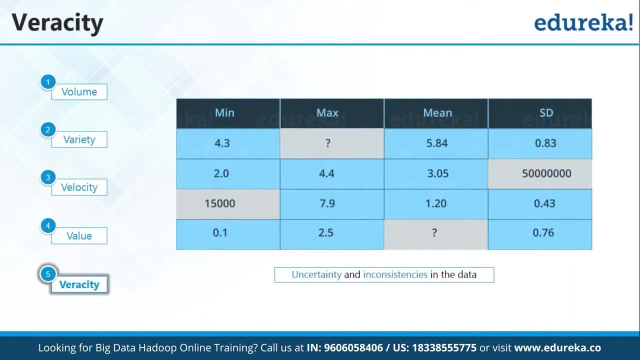 of data. some data packets are bound to lose in the process. Now what we need to do, we need to fill up these missing data and then start mining again and then process it. And then Let's start with a good insight, if possible. So, if you can notice, there's a diagram in front of your screen. 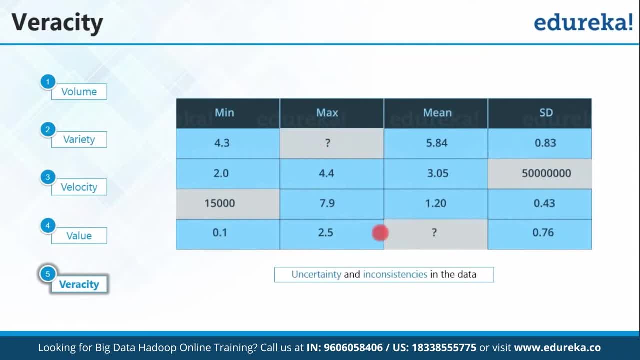 So over here we have this field which is not defined Similarly. this field- And if you can notice, here when we talk about this minimum value, you see the other minimum values and when you talk about this it is- it is way more than the other fields present. 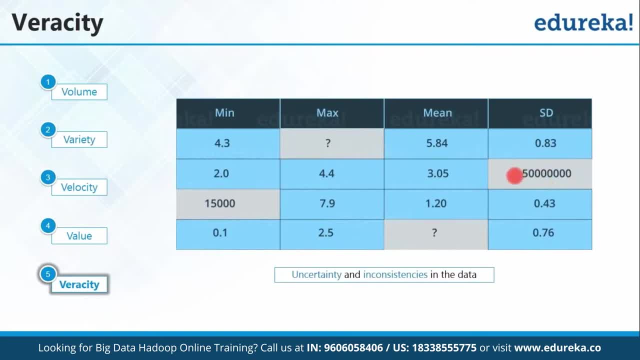 in this particular column. similarly goes for this particular element as well. OK, so obviously processing data like this is one problematic thing. and now I get it why big data is a problem. Well, we have only five V's now, but maybe later on we'll have more. 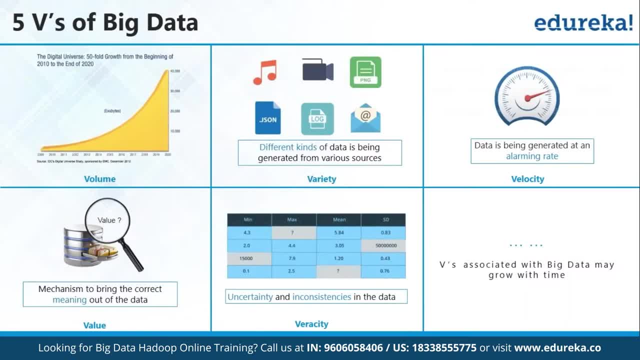 So there are good chances that big data might be even more big. OK, so there are a lot of problems in dealing with big data, but there are always different ways to look at some things. So let us get some positivity in the environment now and let us understand how can we use big. 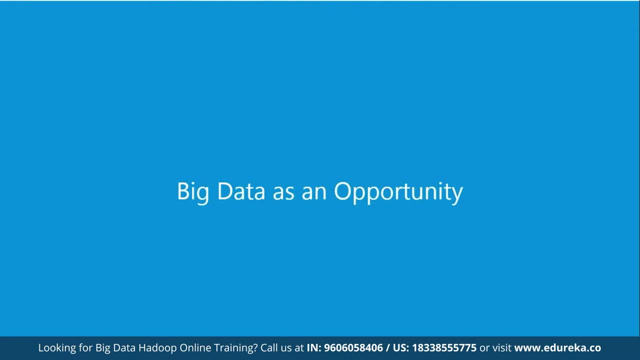 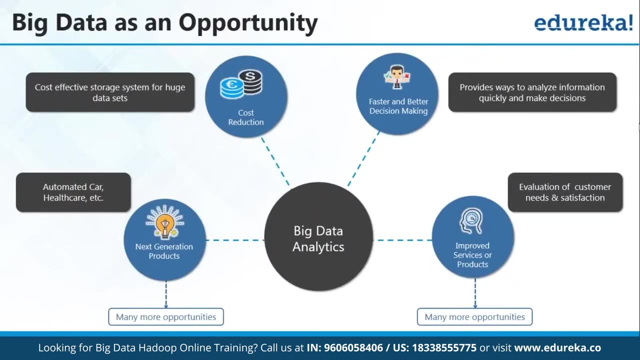 data as an opportunity. Yes, Reshma, and I would say the situation is similar to the proverb: when life throws you lemons, make lemonade. OK, Yeah, so let us go through the fields where we can use big data as a boon, And there are certain unknown problems solved only because we started dealing with big data. 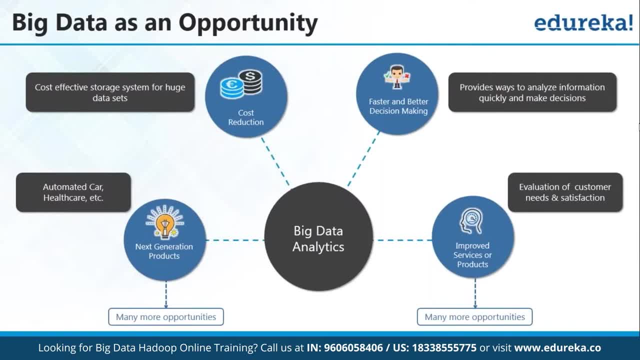 And the boon that you're talking about, Reshma, is big data analytics. First thing: with big data, we figured out how to store our data cost effectively. We were spending too much money on storage before. until big data came into the picture, We never thought of using commodity hardware to store and manage the data, which is both. 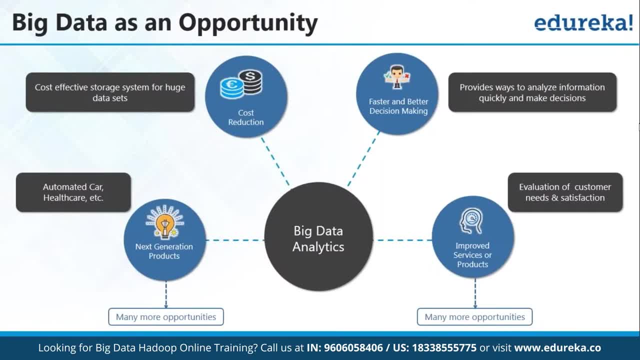 reliable And feasible as compared to the costly servers. Now let me give you a few examples in order to show you how important big data analytics is nowadays. So when you go to a website like Amazon or YouTube or Pandora, Netflix, any other website, So they'll actually provide you certain fields in which they'll recommend some products or 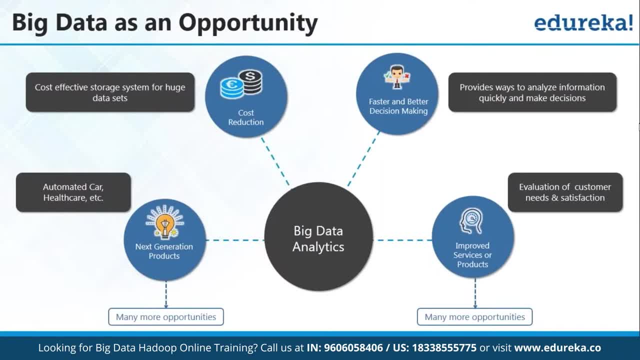 some videos or some movies or some songs for you, Right? So how do you think they do that? So, basically, whatever data that you are generating on these kind of websites, they make sure that they analyze it properly. Let me tell you, guys, That data is not small. 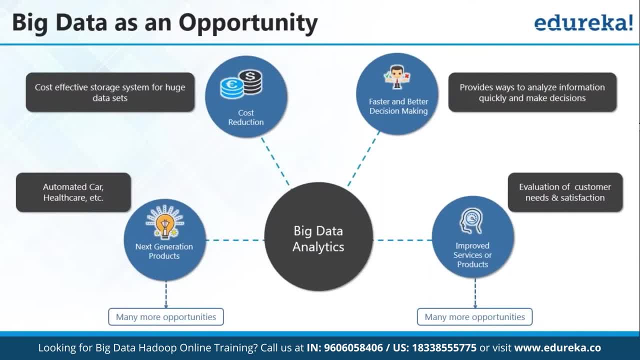 It is actually big data. Now they analyze that big data and they make sure that whatever you like or whatever your preferences are, accordingly, they'll generate recommendations for you. And when I go to YouTube- I don't know if you guys have noticed it, but I'm pretty sure you. 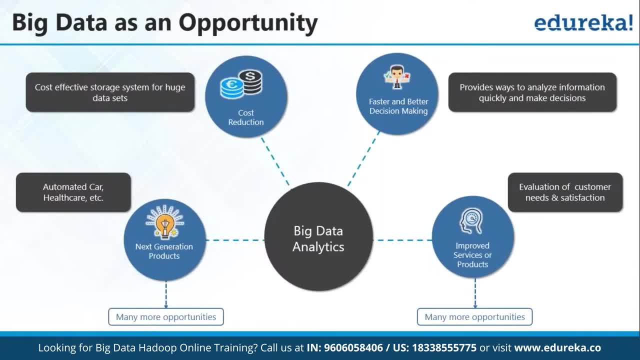 must have done that. So when I go to YouTube, YouTube knows what song or what video that I want to watch next. Similarly, Netflix knows what kind of movies are like, And when I go to Amazon, it actually shows me what all products that I would prefer to buy. 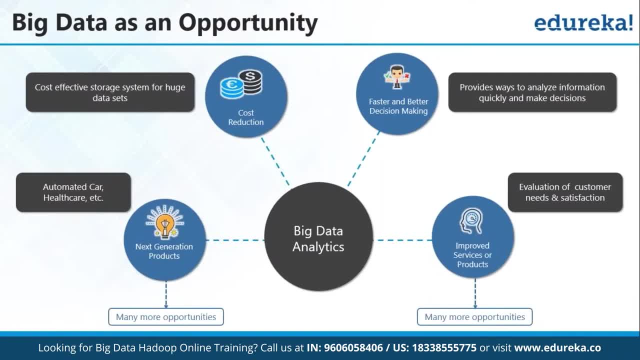 So how do you think it happens? It happens only because of big data analytics. OK, so there is one more example that just popped into my mind I'll share with you guys. So there is this time, when the Hurricane Sandy was about to hit on New Jersey in the United. 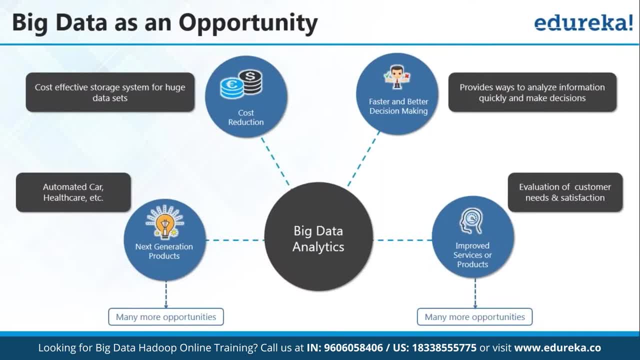 States. So what happened then? the Wal-Mart used big data analytics to profit from it. Now I'll tell you how they did it. So what Wal-Mart did is that they studied the purchase patterns of different customers when a hurricane is about to strike or any kind of natural calamity is about to strike on. 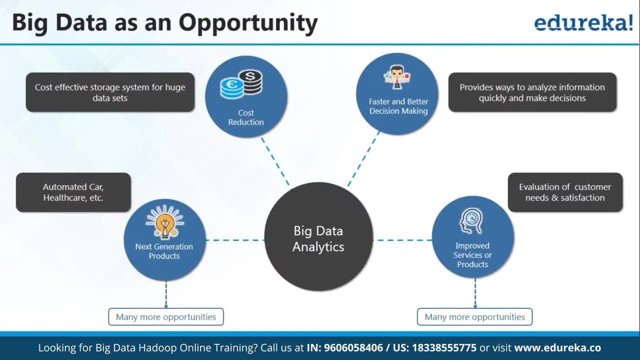 a particular area And when they made an analysis of it, so they found out that people tend to buy emergency stuff like flashlight life jackets and a little bit of other stuff And, interestingly, people also buy a lot of strawberry Pop-Tarts- Strawberry Pop-Tarts. 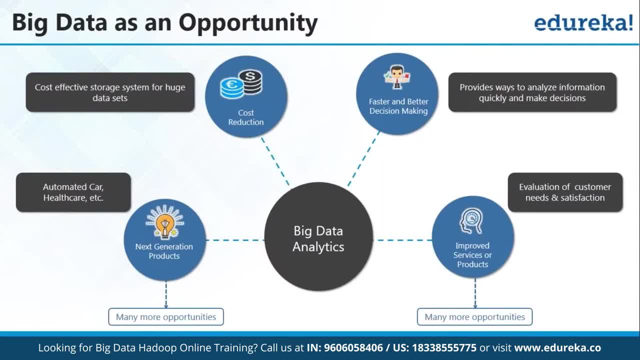 Are you serious? Yeah, And now I didn't do that analysis. I, Wal-Mart did that and apparently it is true. So what they did is they stuffed all their stores with a lot of strawberry Pop-Tarts and emergency stuff and obviously it was sold out and they earned a lot of money during. 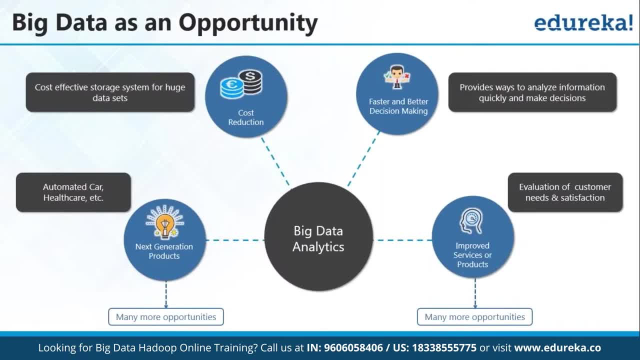 that time. But my question here, Reshma, is: people want to die eating strawberry Pop-Tarts, like? what was the idea behind strawberry Pop-Tarts? I'm pretty unsure about it. but yeah, since you have given us a very interesting example and Wal-Mart did that analysis, we didn't do it. 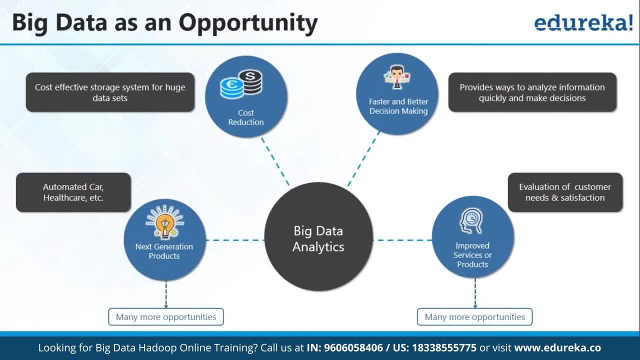 So, yeah, so it is a very good example in order to understand how big data analytics can help your business to grow and find better insights from the data that you have. Yeah, and also, if you want to know why, strawberry Pop-Tarts- maybe later on we can start making. 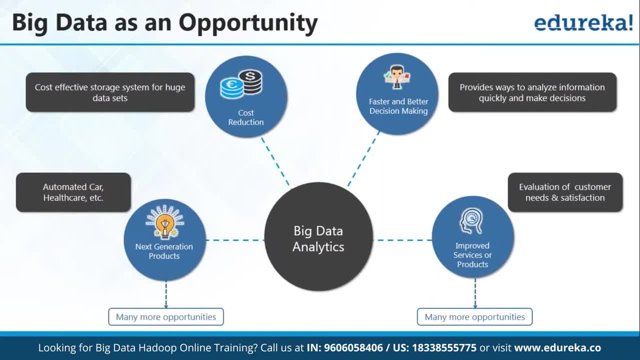 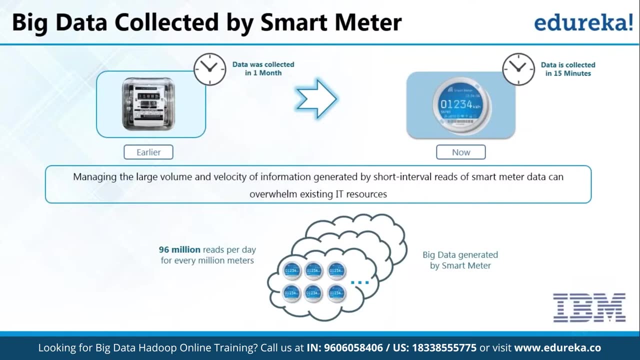 an analysis by gathering some more data also. Yeah, that can be possible. Okay, so now let's move ahead and take a look at a case study by IBM: how they have used big data analytics to profit their company. So if you have noticed that earlier, the data that was collected from the meters that you 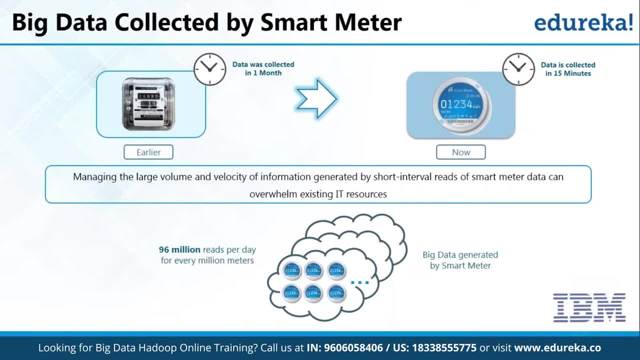 have in your home Electricity consumed, it is actually sending data after one month. But nowadays, what IBM did? they came up with this thing called smart meter and that smart meter used to collect data after every 15 minutes. So whatever energy that you have consumed, after every 15 minutes it will send that data. 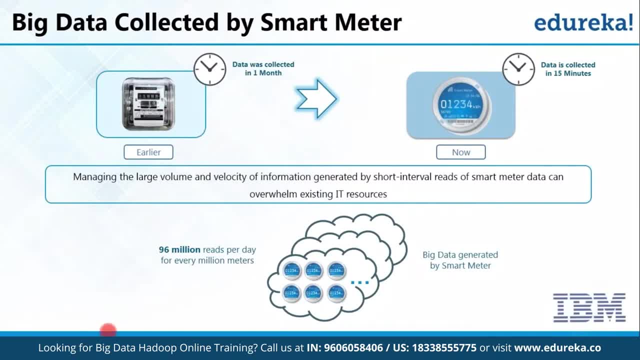 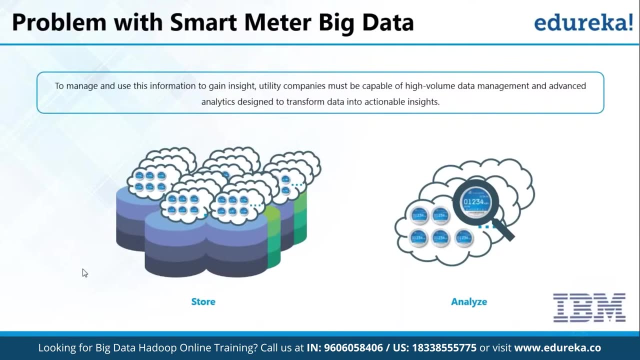 and because of it, big data was generated. So we have some stats here which says that we have 96 million reads per day for every million meters, which is pretty huge. this data, the amount of data that is generated, is pretty huge. Now IBM actually realized the data that they are generating. it is very important for them. 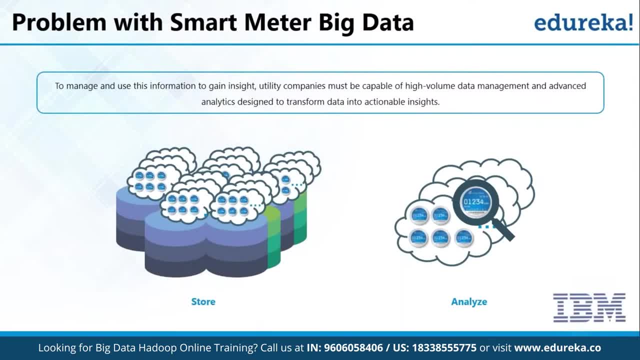 to gain something from that data. So, for that what they need to do, for that what they need to do, they need to make sure that they analyze this data, So they realize that big data analytics can solve a lot of problems and they can get better. 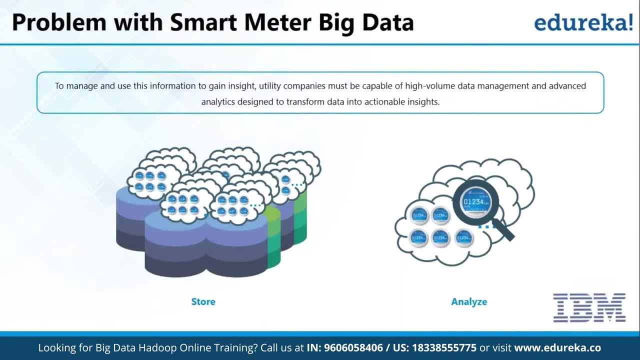 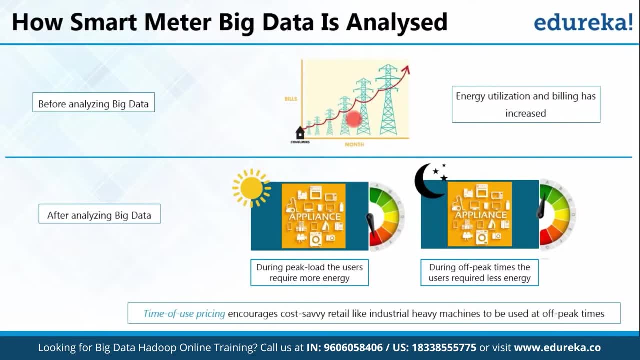 business insight through that. So let us move forward and see what type of analysis they did on that data. So, before analyzing that data, they came to know that energy utilization and billing was only increasing. After analyzing big data, they came to know that during peak load, the users require more. 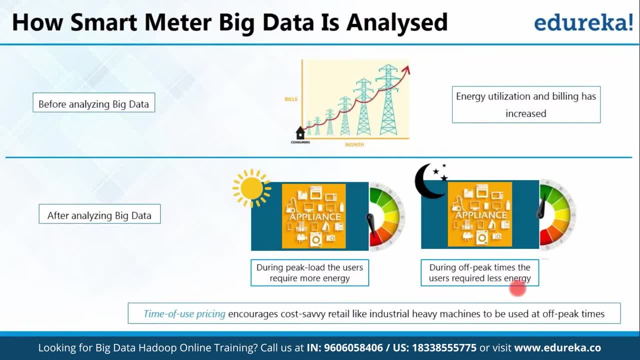 energy and during off peak times that users require less energy. So what advantage they must have got from this analysis. One thing that I can think of right now is they can tell the industries to use their machinery only during the off peak times, so that the load will be pretty much balanced. 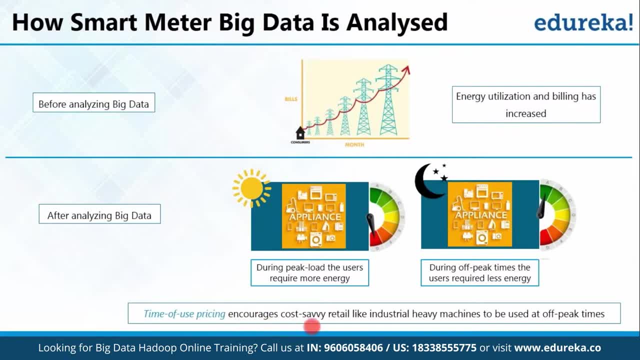 and you can even say that time of use pricing encourages cost savvy retail like industrial heavy machines to be used off peak time. So, yeah, They can save money As well, because off peak times pricing will be less than the peak time prices, right? So this is just one analysis. 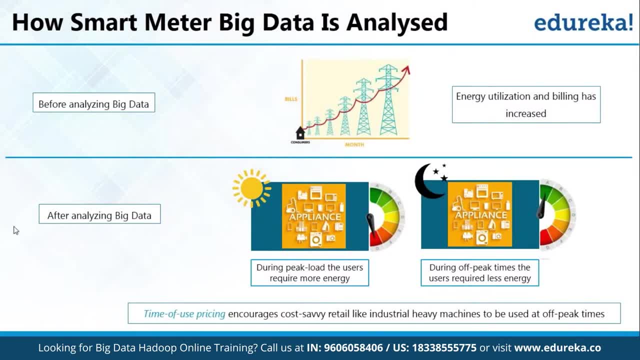 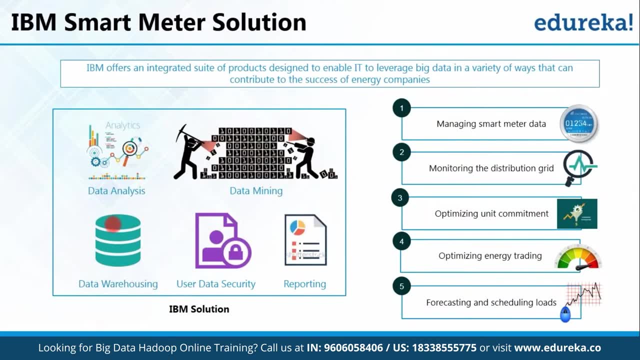 Now let us move forward and see the IBM suite that they developed. So over here, what happens? you first dump all your data that you get in this data warehouse. After that, it is very important to make sure that your user data is secure. Then what happens? you need to clean that data, as I've told you earlier as well, there might 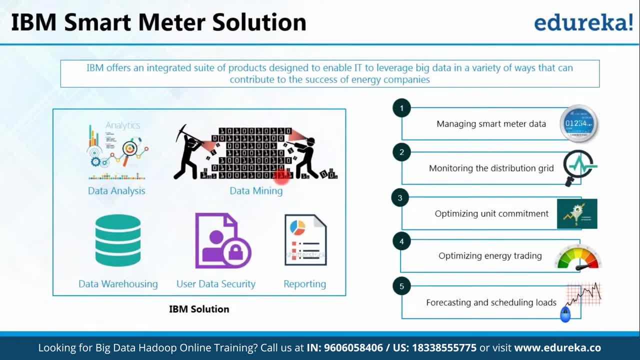 be many fields that you don't require, so you need to make sure that you have only useful material or useful data in your data set, and then you perform certain analysis, And in order to use this suite that IBM offered you efficiently, you have to take care of a 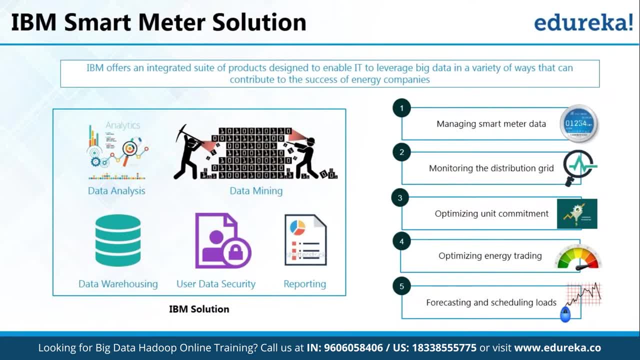 few things. The first thing is that you have to be able to manage the smart meter data. Now there is a lot of data coming from all this million smart meters, so you have to be able to manage that large volume of data and also be able to retain it, because maybe later 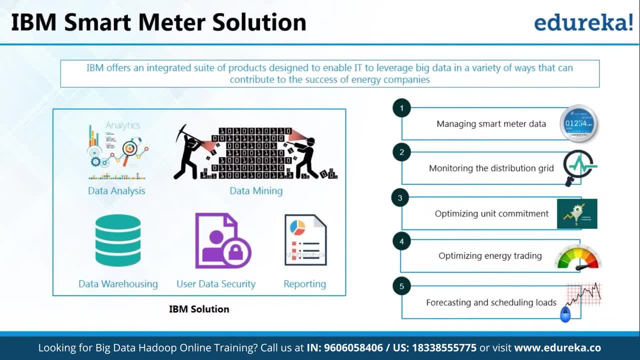 on. you might need it for some kind of regulatory requirements or something. The next thing you should keep in mind is to monitor the distribution grid so that you can improve and optimize the overall grid reliability so that you can identify the abnormal conditions which are causing any kind of problem, and then you also have to take care of optimizing. 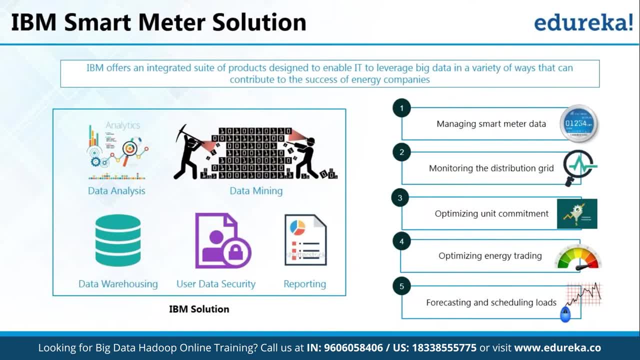 the unit commitment. So by optimizing the unit commitment the companies can satisfy their customers even more. they can reduce the power outages. that is, they can reduce the power outages so that their customers don't get angry more, Identify problems And then reduce it. obviously, 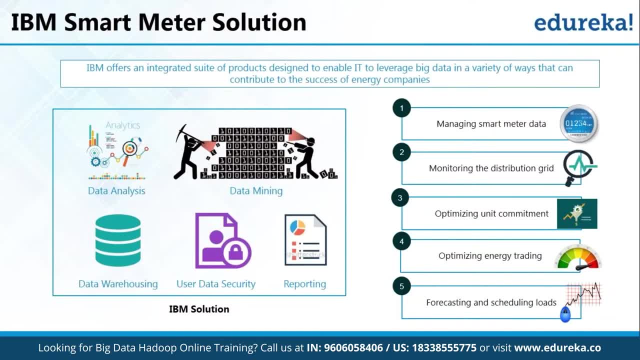 And then you have also to optimize the energy trading, So it means that you can advise your customers when they should use their appliances in order to maintain that balance in the power load. And then you also have to forecast and schedule loads, So companies must be able to predict when they can profitably sell the excess power. 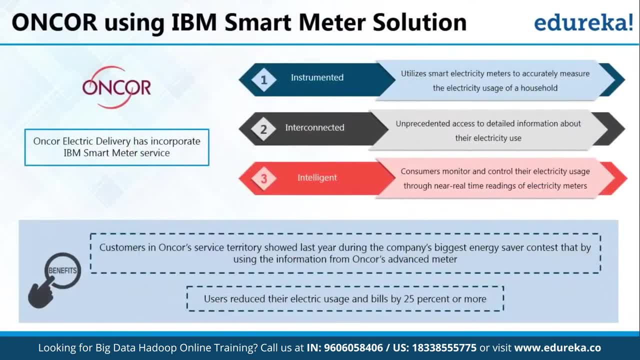 and when they need to hedge the supply. And continuing from this, Now let's talk about how Encore have made use of them. So Encore is an electric delivery company and it is the largest electrical distribution and transmission company in Texas And it is one of the six largest in the United States. 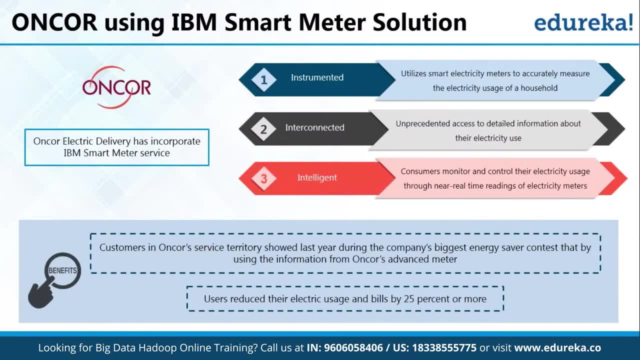 They have more than three million customers and their service area covers almost one hundred and seventeen thousand square miles, And they begin the advanced meter program in 2008, and they have deployed almost 3.25 million meters, So Serving customers of North and Central Texas. 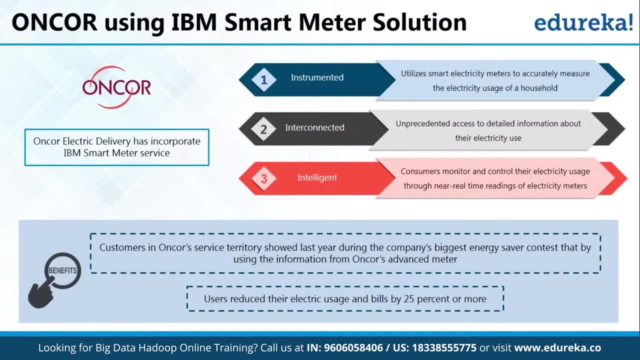 So, when they were implementing it, they kept three things in mind. The first thing was that it should be instrumented. So this solution utilizes the smart electricity meters so that they can accurately measure the electricity usage of a household in every 15 minutes. because, like we discussed, that, 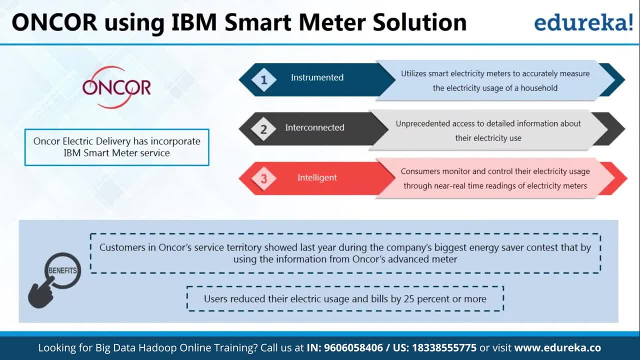 the smart meters were sending out data every 15 minutes and it provided data inputs. that is essential for consumption insights. Next thing is that it should be interconnected, So now the customers have access to the detailed information about the electricity they are consuming, and it creates a very enterprise wide view of all the meter assets, and it helped. 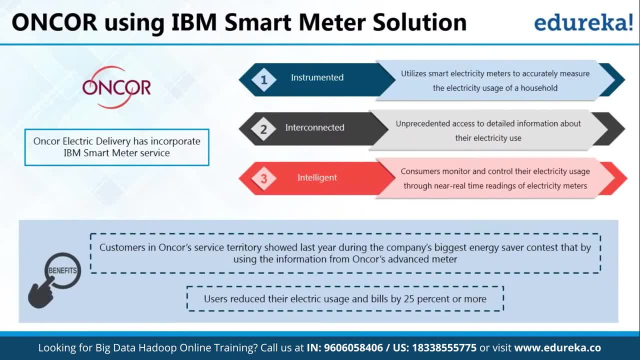 them to improve the service delivery. The next thing is to make your customers intelligent Now, since it is getting monitored already about how each of the household or each customer is consuming the power. so now they are able to advise the customers about, maybe to tell them to wash their clothes at night, because they are using a lot of appliances during. 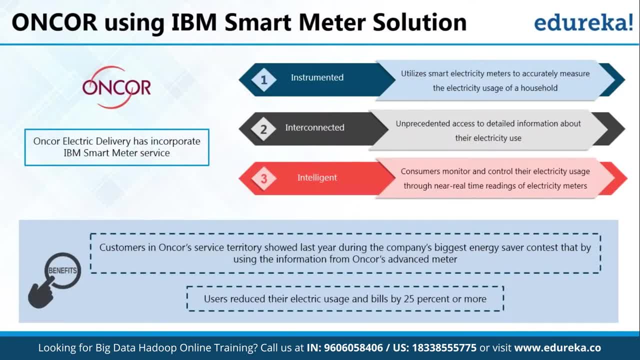 the daytime, so maybe they could divide it up so that they can use some appliances at off peak hours, so that they can even save more money. And this is beneficial for both of them, for both the customers and the company as well, And they have gained a lot of benefits by using the IBM solution. 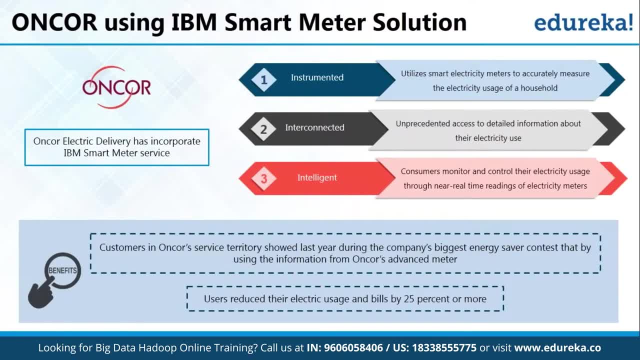 So what are the benefits they got is that it enabled Encore to identify and fix outages before the customers. That means they were able to identify the problem before it even occurred, and it also improved the emergency response on events of severe weather events and views of outages. 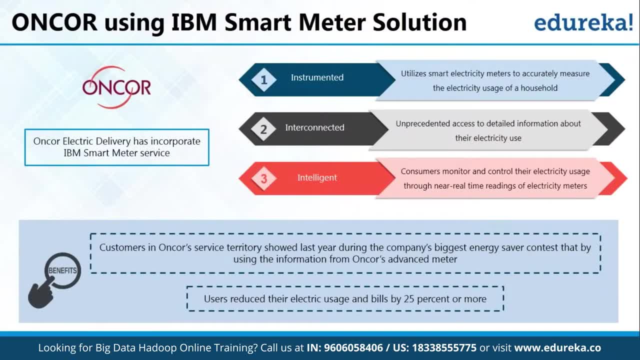 And it also provides the customers the data needed to become an active participant in the power consumption management, and it enabled every individual household to reduce their electrical consumption by almost five to ten percent. And this is how Encore used the IBM solution and made huge benefits out of it. 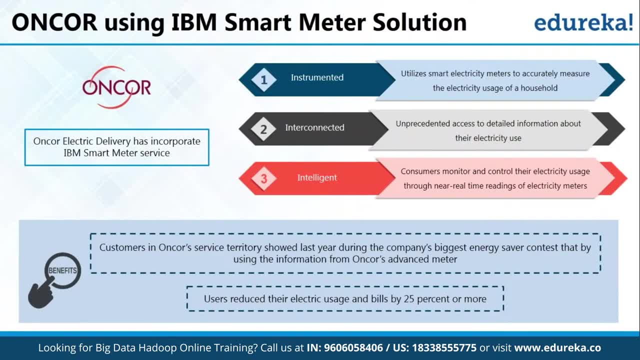 Just by using big data analytics that IBM performed. But let me just interrupt right now. So since Reshma told us, in the beginning as well, that there are no free lunches in life, right, So this is an opportunity, But there are many problems to encase this opportunity, right? 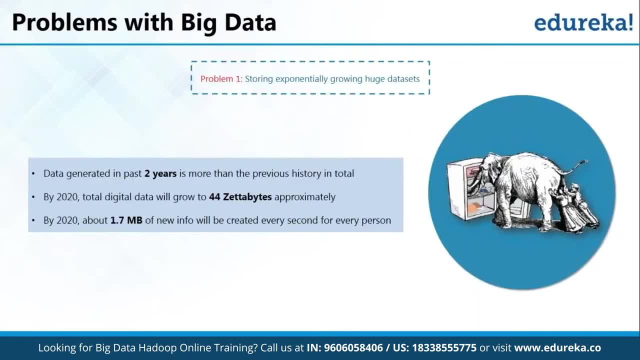 So let us focus on those problems one by one. So the first problem is storing colossal amount of data. So let's discuss few stats that are there in front of your screen. So data generated in the past two years is more than the previous history in 2020.. 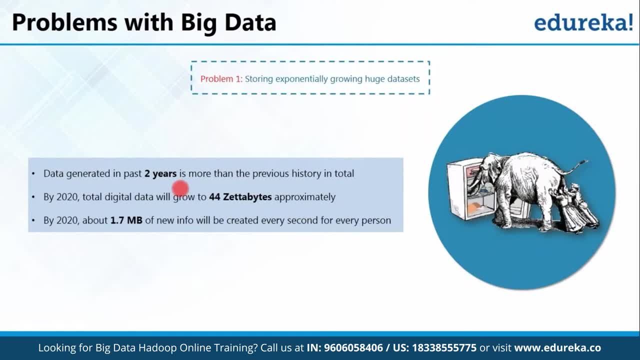 So, guys, what are we doing? Stop generating so much amount of data. It is said that by 2020, total digital data will grow to 44 zettabytes approximately, And there is one more stat that amazes me is about 1.7 MB of new information will be. 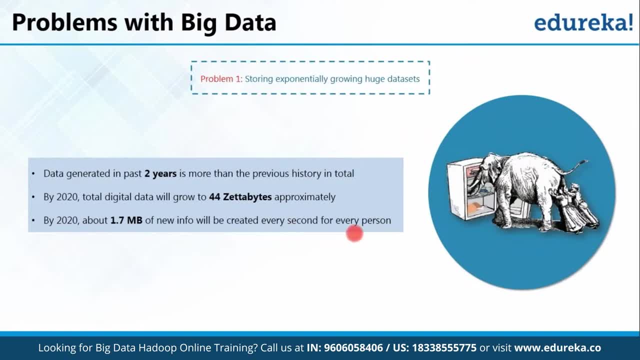 created every second for every person by 2020.. So storing this huge data in traditional system is not possible. The reason is obvious: The storage will be limited for one system. For example, you have a server with a storage limit of 10 terabytes. 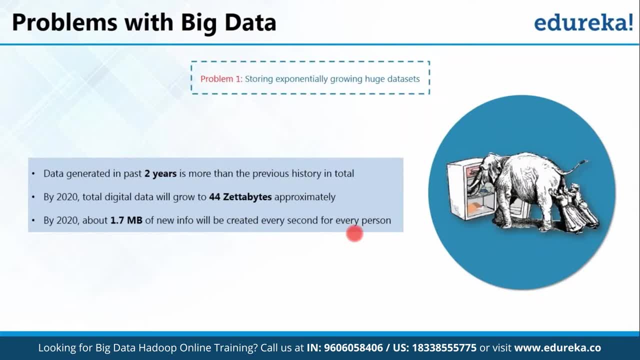 But your company is growing really fast and data is exponentially increasing. Now, what you will do Now, at one point you will exhaust all the storage. So investing in huge servers is definitely not a cost effective solution. So, Reshma, what do you think? what can be the solution to this problem? 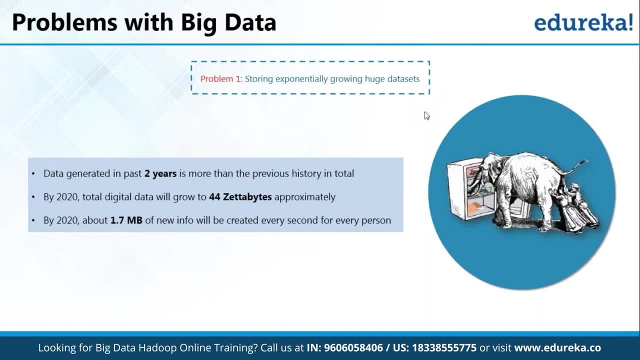 According to me, a distributed file system will be a better way to store this huge data, Because with this, we will be saving a lot of money. Let me tell you how. Because, due to this distributed system, you can actually store your data in commodity hardware instead of spending money on high end servers. 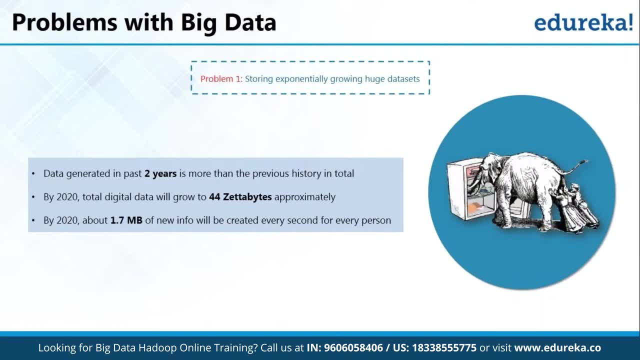 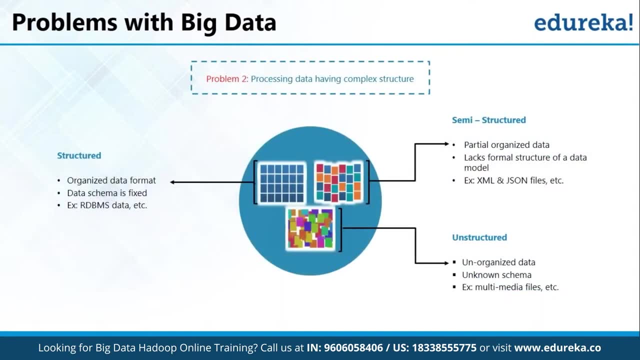 Don't you agree, Saurabh, Completely. Now, we know storing is a problem, but let me tell you guys, it is just one part of the problem. Let's see a few more. Ok, so since we saw that the data is not only huge, but it is present in various formats, 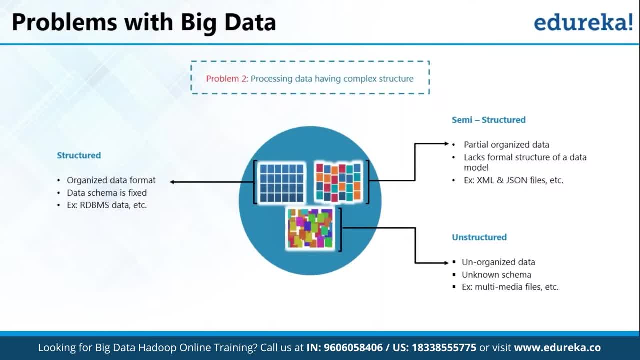 as well, Like unstructured, semi-structured and structured. Let me tell you how. So you not only need to store this huge data, but you also need to make sure that a system is present to store this varieties of data generated from various sources. 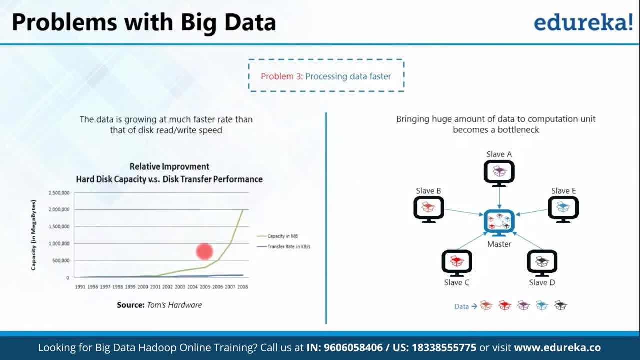 And now let's focus on the next problem. Now let's focus on the diagram. So over here you can notice that the hard disk capacity is increasing, But the disk transfer performance or speed is not increasing at that rate. Let me explain you this with an example. 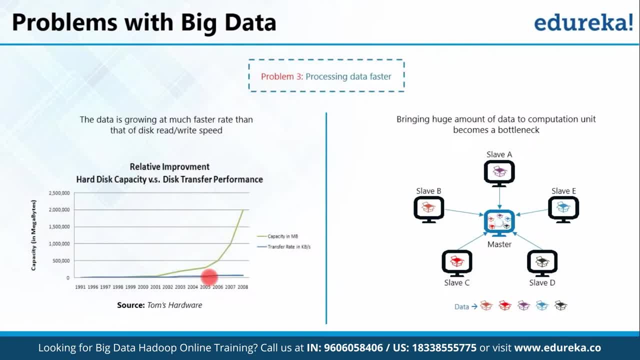 If you have only 100 Mbps input output, Ok, And you are processing, say, 1TB of data. Now how much time will it take? Let me calculate: It will be somewhere around 2.91 hours, right? So it will be somewhere around 2.91 hours. 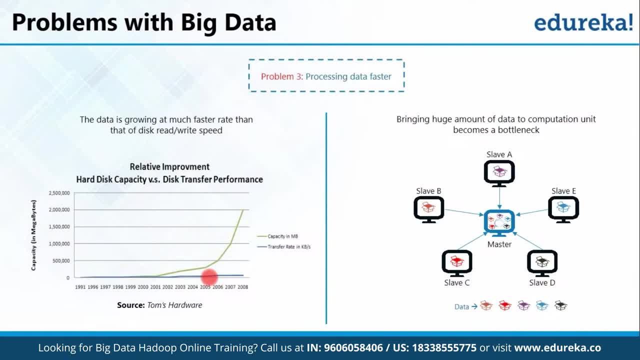 And I have taken an example of 1TB. What if you are processing some zettabytes of data? So you can imagine how much time will it take. Now what if you have 4 input output channels for the same amount of data? 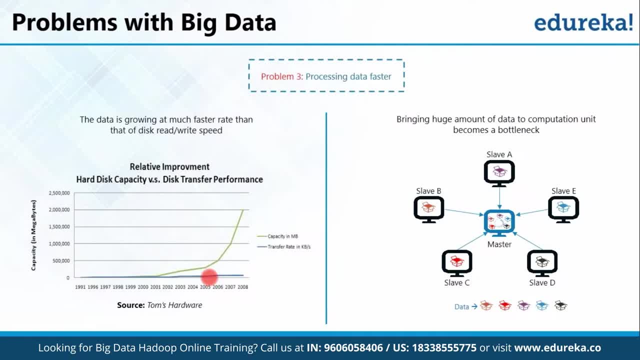 Then it will take approximately 0.72 hours, Or, converted to minutes, so it will be around 43 minutes approximately. right, And now imagine, instead of 1TB you have zettabytes of data. For me, more than storage, accessing and processing speed for huge data is a bigger problem. 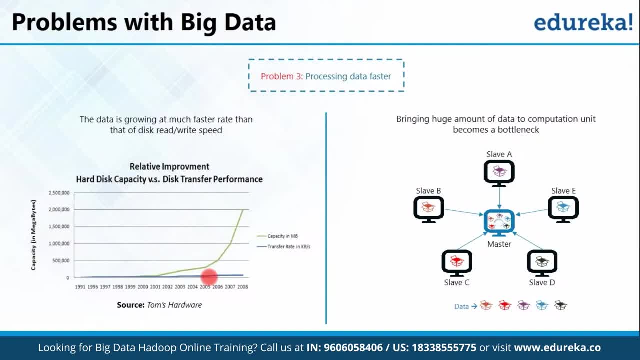 Ok, so Reshma has a very good example to discuss. Yeah, so since you were talking about accessing the data and you told us already about how Amazon, at different websites and YouTube, they make those recommendations, So If there was no solution for it, it would take so much time to access the data, the recommendation. 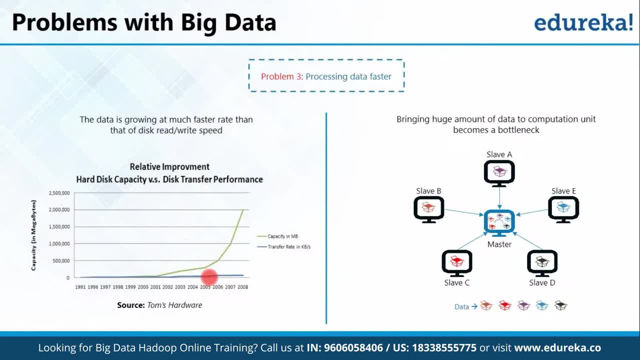 system wouldn't work at all And they make a lot of money just by recommendation system because a lot of people go there and click over there and buy that product right. So let's consider that it is taking like hours or maybe years of time in order to process. 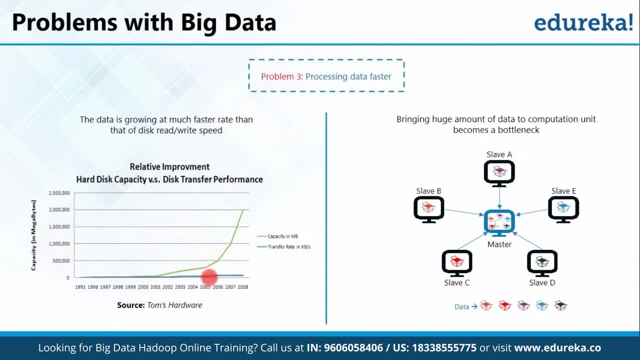 that big amount of data. So let's say that at one time I purchased an iPhone 5S from Amazon and after two years I'm again browsing onto Amazon And since it took so much time to access the data and I've already switched over to a new- 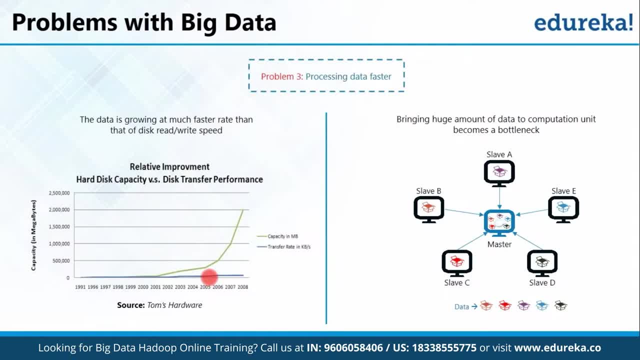 iPhone and they are recommending me the old iPhone case for 5S, So obviously that won't work. I won't go there and click it because I've already changed my phone right, So that will be a huge problem for Amazon. the recommendation system won't work anymore. 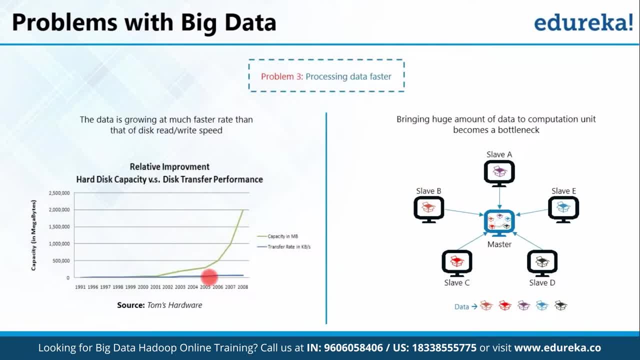 And I know that Reshma changes her phone every year. so if she has bought a phone and people are recommending, But if she has bought a phone now and someone's recommending the case for that phone after two years doesn't make sense to me at all. 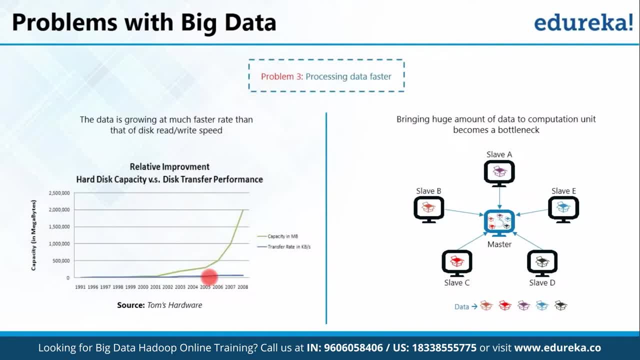 Yeah, only it will work if I have both the two phones at the same time. But yeah, I don't want to waste money on purchasing new iPhone case for my older phone. So basically it won't be fair if we don't discuss the solution to these problems. 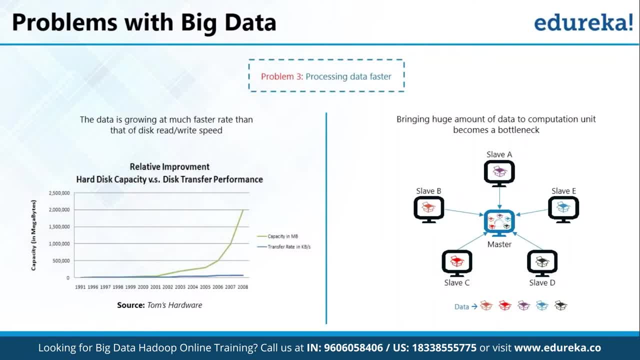 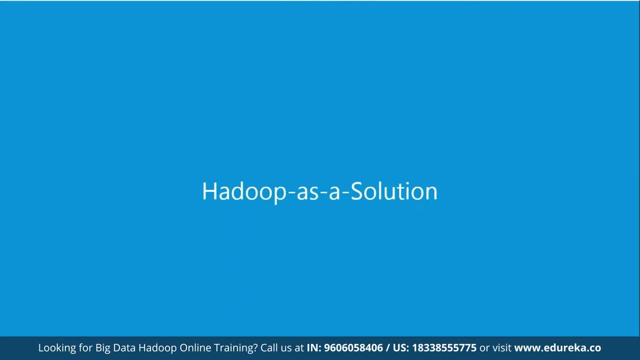 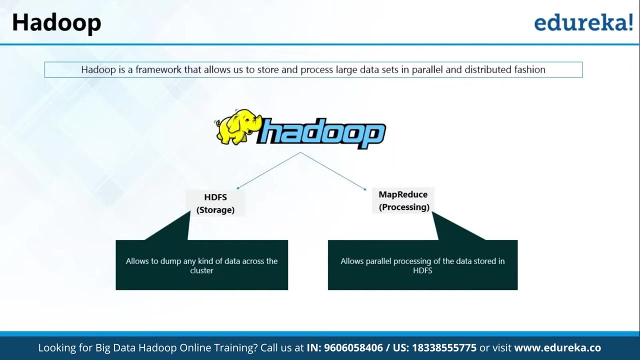 Reshma, we can't leave our viewers with just the problems. right, it won't be fair. What is the solution? Hadoop. Hadoop is a solution, So let's introduce Hadoop now. Okay, so now, what is Hadoop? So Hadoop is a framework that allows you to first store big data in a distributed environment. 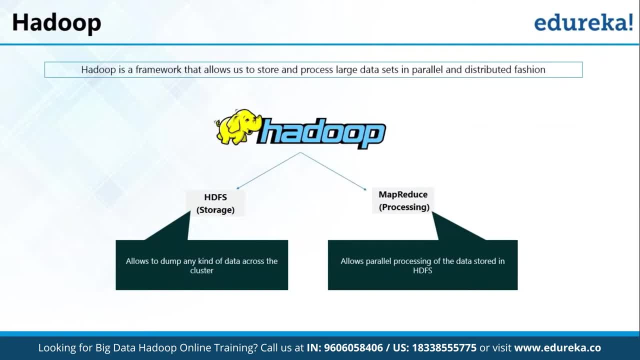 so that you can process it parallelly. There are basically two parts. One is HDFS, that is, Hadoop, distributed file system for storage. It allows you to store data of various formats across a cluster, And the second part is MapReduce. Now it is nothing but a processing machine. 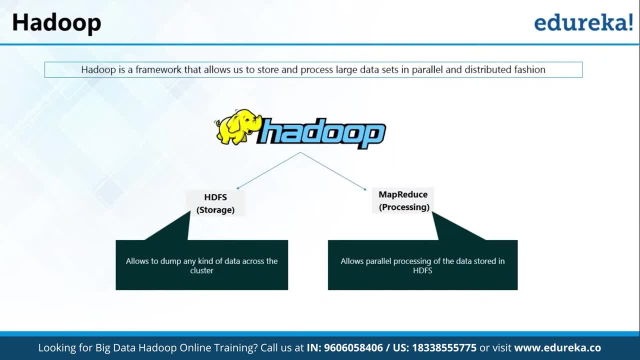 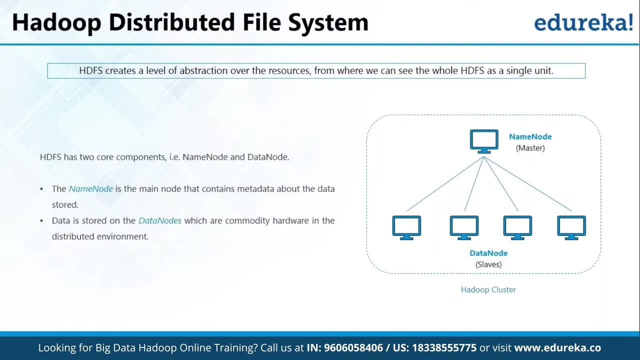 It is a processing unit of Hadoop. It allows parallel processing of data that is stored across the HDFS. Now let us dig deep in HDFS and understand it better. Yeah, so HDFS creates an abstraction of resources. Let me simplify it for you. 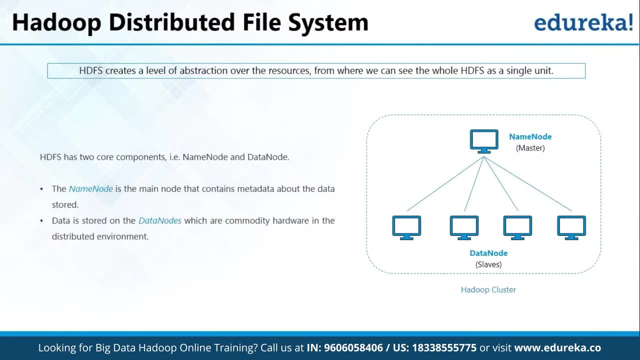 So similar to virtualization. you can see HDFS logically as a single unit for storing big data, But actually restoring your data across multiple systems, or you can say in a distributed fashion. So here you have a master slave architecture in which the name node is a master node and 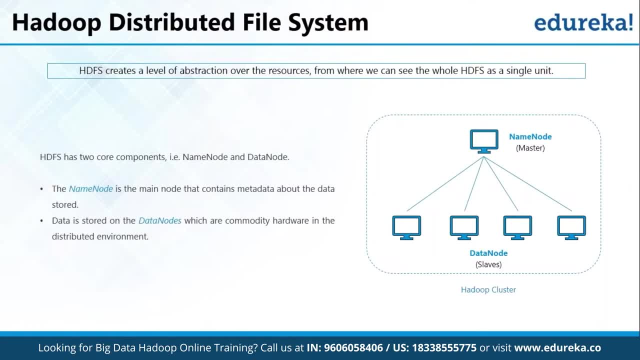 the data nodes are slaves And the name node contains the metadata about the data that is stored in the data nodes, Like which data block is stored in which data node, where are the replications of the data block kept and etc. etc. So the actual data is stored in the data nodes. 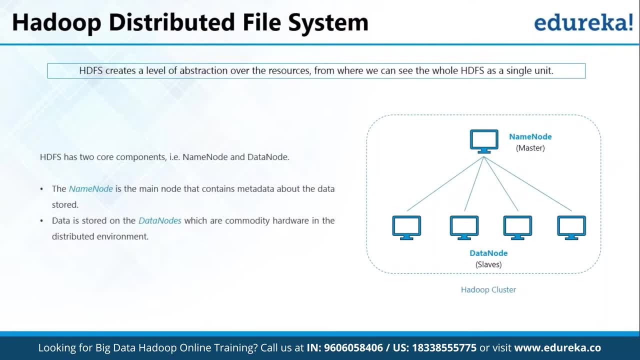 And I also want to add that we actually replicate the data blocks. that is present in the data nodes And by default, the replication factor is three, So it means that there are three copies of each file. So, Saurav, can you tell us why do we need that replication? 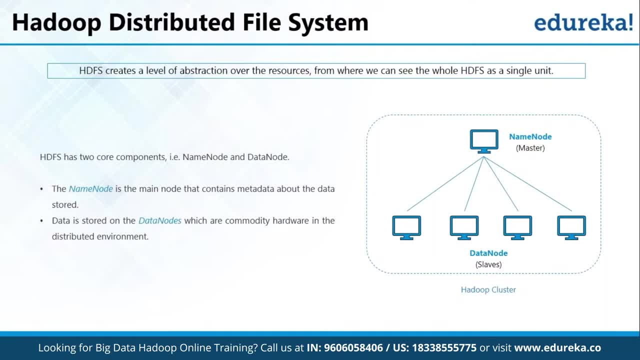 Sure, Reshma, Since we are using commodity hardware right, and we know failure rate of these hardwares are pretty high. So if one of the data nodes fail, I won't have that data block And that's the reason we need to replicate the data block. 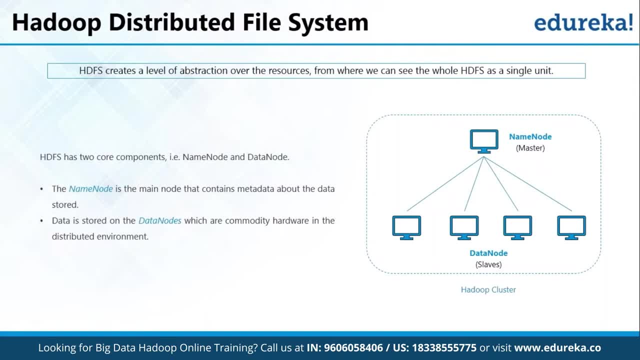 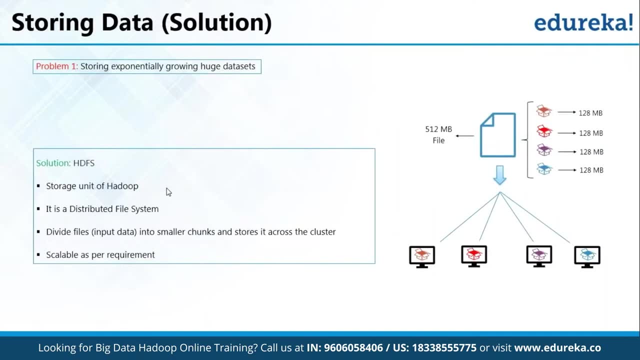 Now, this replication factor depends on your requirements. right Now, let us understand how actually Hadoop provided the solution To the big data problems that we have discussed. So, Reshma, can you remember what was the first problem? Yeah, it was storing the big data. 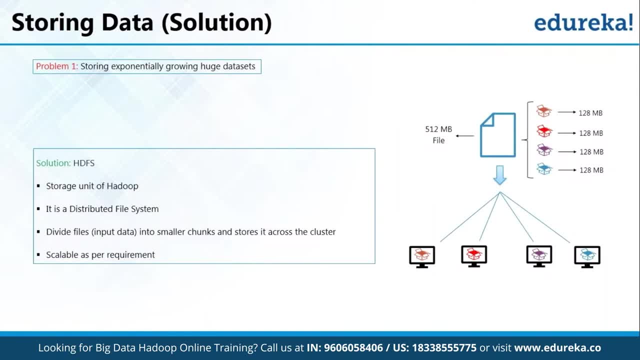 So how HDFS solved it, let's discuss it. So HDFS provides a distributed way to store big data. we've already told you that. So your data is stored in blocks, in data nodes, and you then specify the size of each block. So basically, if you have a five hundred twelve MB of data and you have configured HDFS such 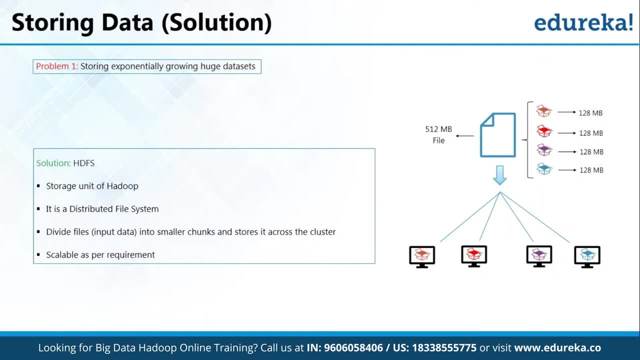 that it will create one twenty eight megabytes of data block. So HDFS will divide the data in four blocks because five hundred twelve divided by one twenty eight is four, and it will store it across different data nodes and it will also replicate the data blocks on the different data nodes. 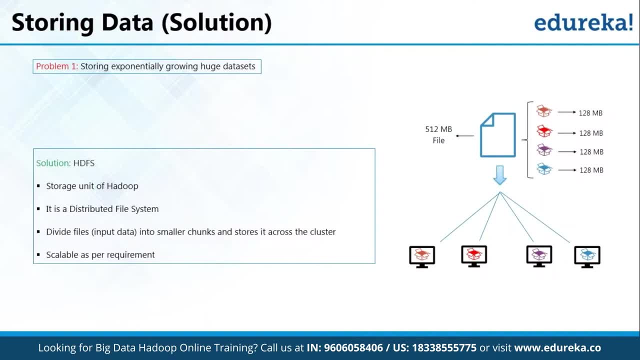 So now we are using commodity hardware and storing is not a challenge. So what are your thoughts on it, Saurav? I will also add one thing, Reshma. It also solves the scaling problem. It focuses on horizontal scaling Instead of vertical. now you can always add some extra data nodes to your HDFS cluster. 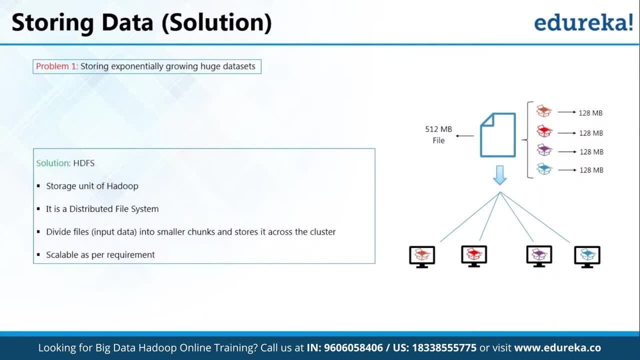 as and when required, instead of scaling the resources of your data nodes. So you're not actually increasing the resources of your data nodes, you're just adding few more data nodes when you require. Let me summarize it for you: So basically, for storing one TB of data, I don't need a one TB system. 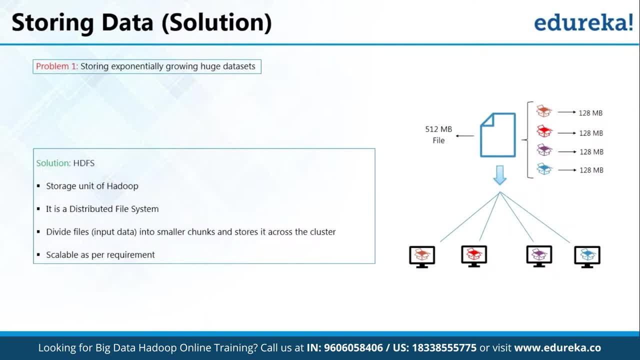 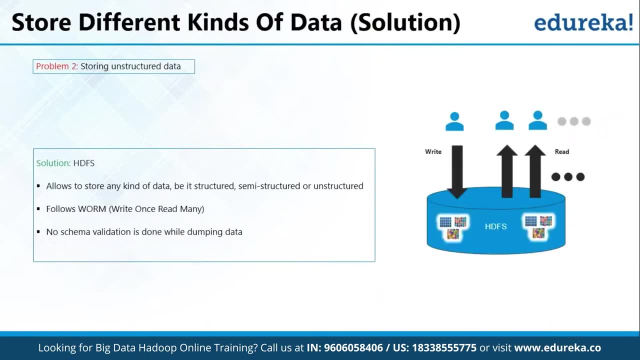 I can instead do it on multiple 128 GB systems, or even less. Now, Reshma, what was the second challenge with big data? So the next problem was storing variety of data, And that problem was also addressed by HDFS. So with HDFS you can store all kinds of data, whether it's structured, semi-structured or 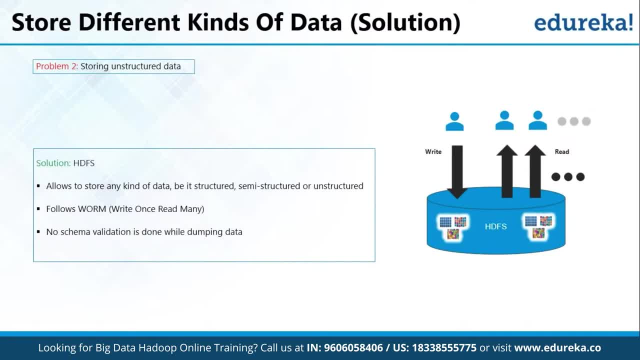 unstructured. It is because in HDFS there is no pre-dumping schema validation, So you can just dump all the kinds of data that you have in one place And it also follows a write once and read many model, And due to this, you can just write the data once and you can read it multiple times. for 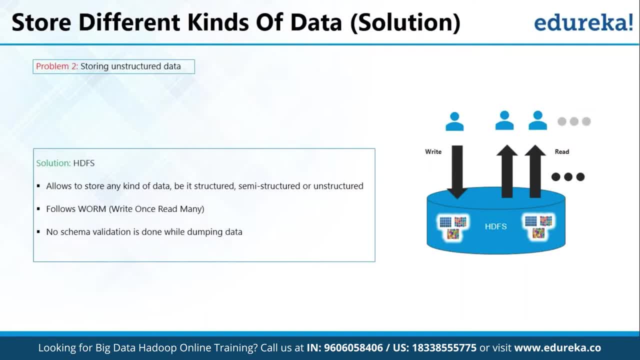 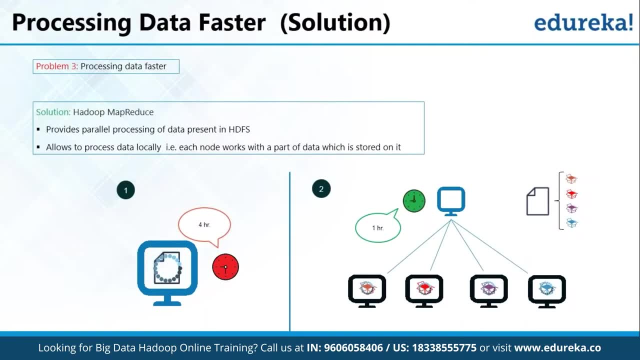 finding out insights. And, if you can recall, the third challenge was accessing the data faster. And this is one of the major challenge with big data And in order to solve it, we're moving processing to data and not data to processing. So what it means sort of just go ahead and explain it. 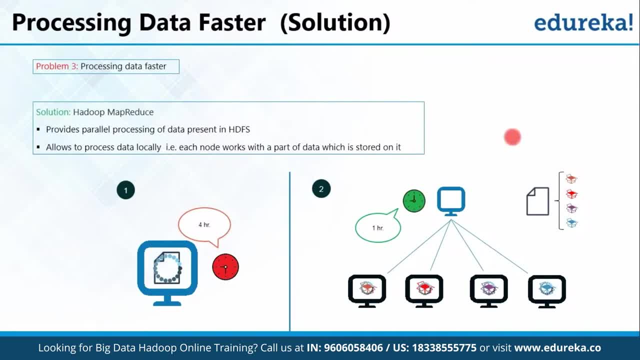 Yes, Reshma, I will. So over here, let me explain you what do you mean by actually moving process to data. So consider this as our master and these are our slaves. So the data is stored in these slaves. So what happens? one way of processing this data is what I can do, is I can send this data. 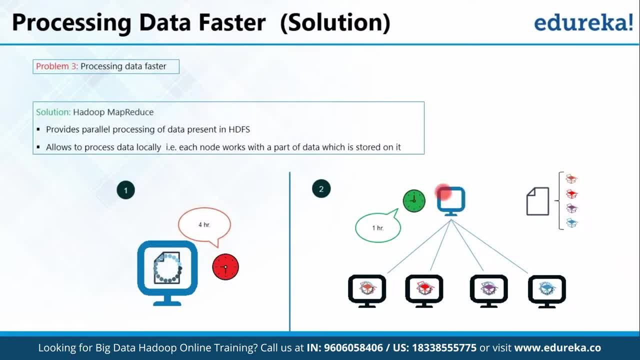 to my master node and I can process it over here. But what will happen if all of my slaves will send the data to my master node? It will cause network congestion plus input output channel congestion and at the same time my master node will take a lot of time in order to process this huge amount of data. 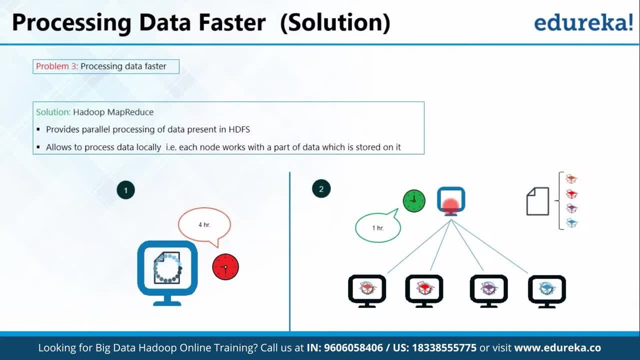 So what I can do? I can send this process to data. That means I can send the logic to all these slaves which actually contain the data and perform processing in the slaves itself. So after that, what will happen? the small chunks of the result that will come out will be sent. 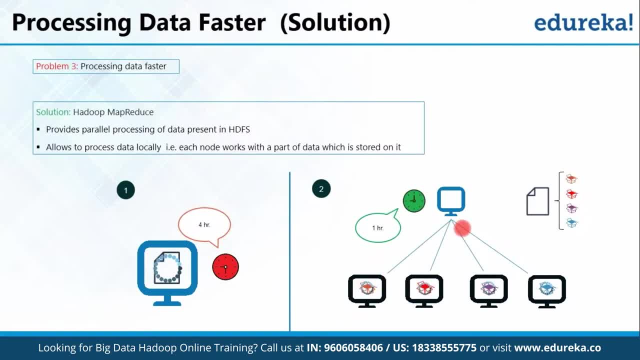 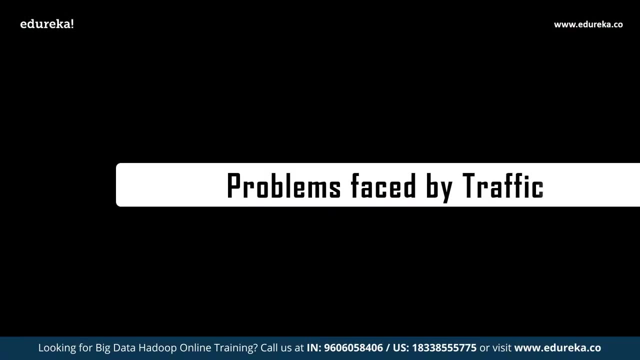 to our name node. So in that way there won't be any network congestion or input output congestion, and it will take comparatively very less time. So this is what actually means sending process to data. So now let's talk about some of the problems faced by traffic. 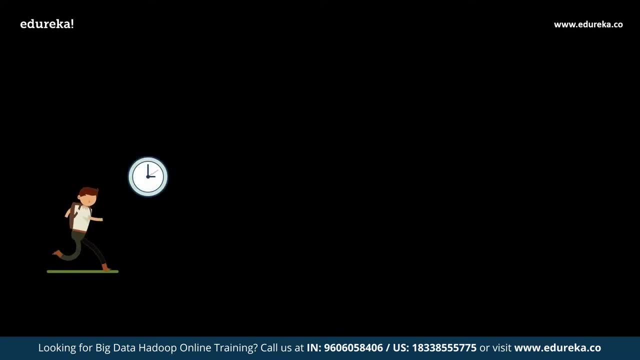 Now there are a hell lot of problems that are being faced by us in our day to daily lives. A few major problems are delays. The first thing many people think of when it comes to congested roadways are the delays. During the morning commute. there is an additional stress because of delays caused by traffic. 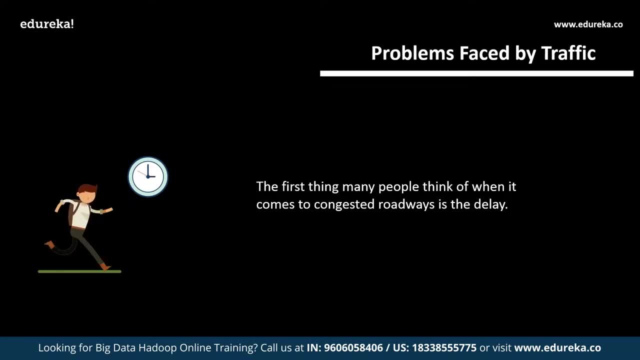 that can make people late for work And, at the end of the day, the afternoon rush is again frustrating time because of the workday is done And the people want to go home and relax, and the traffic is preventing it. These delays are common to most of the people because it is universal and everyone who has 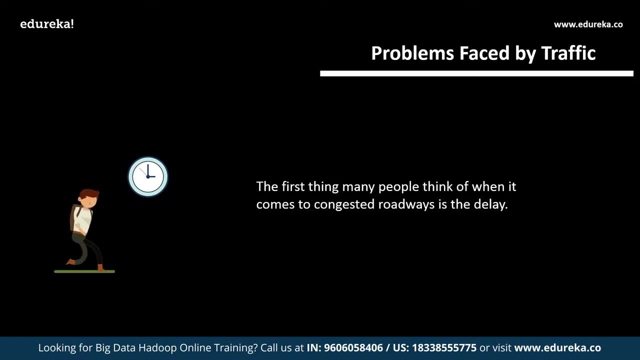 to maneuver through congested roads, Just in case time. a secondary effect of traffic congestion related to delays is the inability to estimate travel times. Those who regularly travel congested areas know approximately how long it usually takes to get to a particular area, Depending on the traffic. 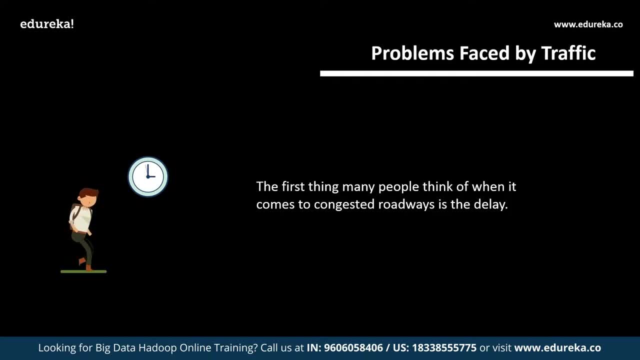 Depending upon the time of the day and the day of the week, These experienced city drivers have to build in time just in case the traffic is too bad. This takes away the time from their leisure and the time to do other tasks throughout the day. 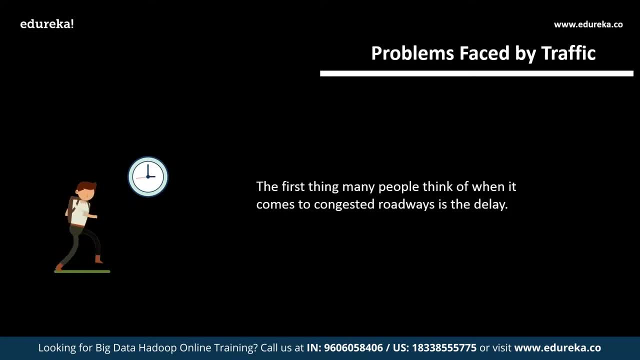 Also, on a few days when the traffic is usually light, the built in extra time may be of no use and the person arrives too early. Followed by the first problem, we move into the second problem, Which is the fuel consumption and pollution. 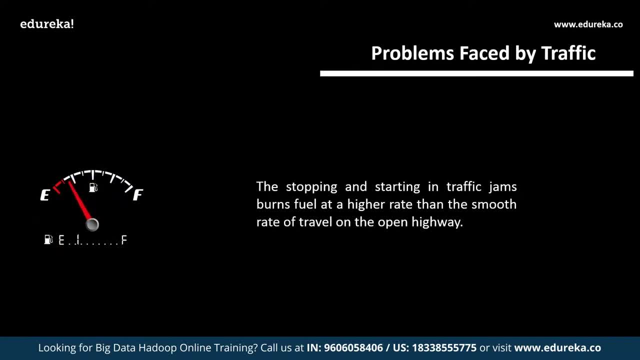 The stopping and starting in traffic jams burns fuel at a higher rate than the smooth rate of travel on the open highway. This increases the fuel consumption, costs commuters additionally for fuel and it also contributes to the amount of emissions released by the vehicles. These emissions create air pollution and are related to global warming. 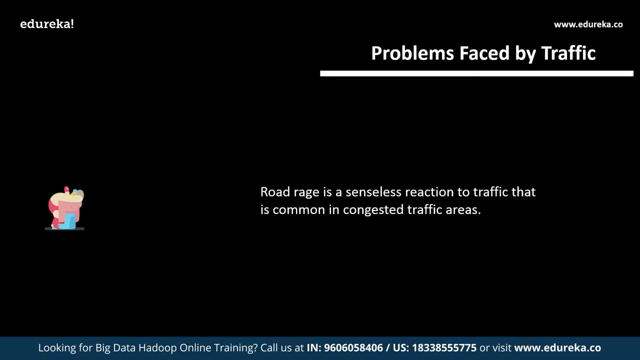 Followed by the second problem. the third major problem is the road rage. Road rage is a major problem in the city. Road rage is a senseless reaction to traffic that is common in congested traffic areas If someone is not driving as fast as the person behind him thinks he should, or someone cuts. 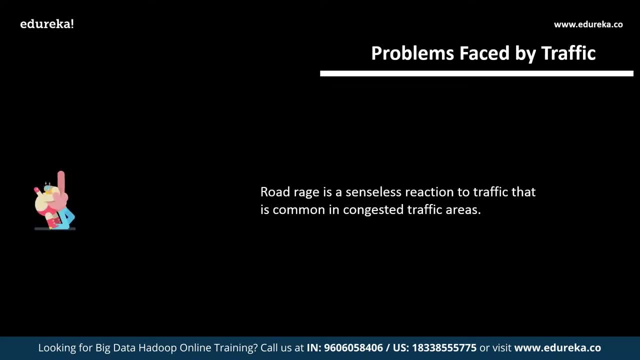 in front of someone else, it can lead into an incident that is dangerous to the offender and those around him on the road. Road rage often manifests itself as shouting matches on the road, intentional tailgating, retaliatory traffic maneuvers and, mostly, a lack of attention being paid to the vehicle. 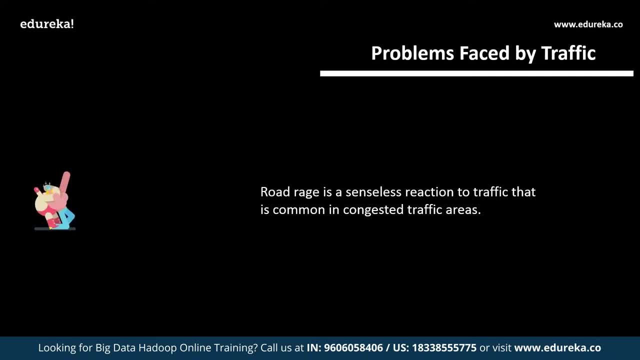 Road rage is a major problem in the city. Road rage is a senseless reaction to traffic that is common in congested traffic areas. If someone is not driving as fast as the person behind him thinks he should, or someone cuts in front of someone else, it can lead into an incident that is dangerous to the 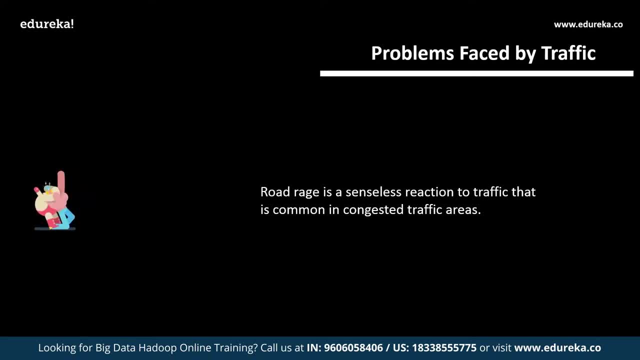 offender and those around him on the road. Road rage is a major problem in the city. Road rage is a major problem in the city. Road rage is a到 are available that help elevate this problem by allowing the emergency crews to automatically change the traffic lights to keep the line moving. So with this we move ahead into the next topic. 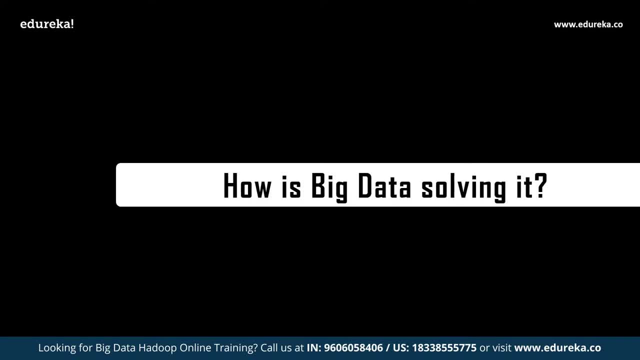 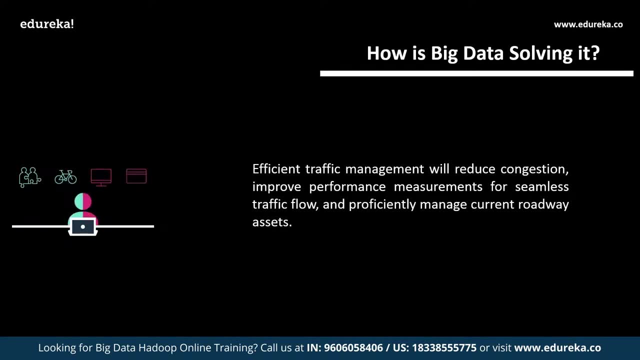 where we will learn exactly how big data is solving it. The higher risk of passenger safety, loss of productivity, increase in fuel consumption and fuel is all the effects of urban traffic congestion. Efficient traffic management will reduce congestion, improve performance measurements for seamless traffic flow and proficiently manage current roadway assets. Government organizations. 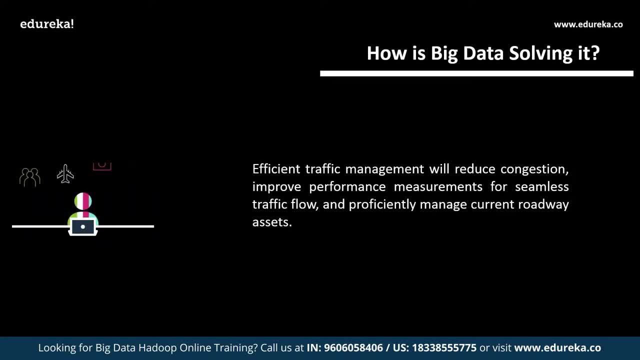 and administrative authorities are implementing coordinated traffic signals and variable messages to manage traffic congestion. By implementing big data solutions, administrators can leverage historical trends, a combination of real-time information and new age algorithms to improve and traffic networks in urban areas, The growing focus on the development of intelligent network systems and the use of big data analytics. 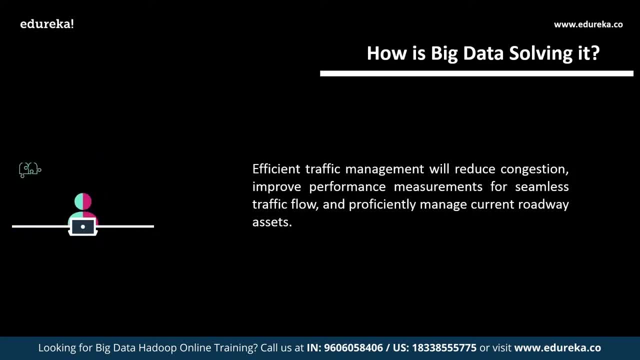 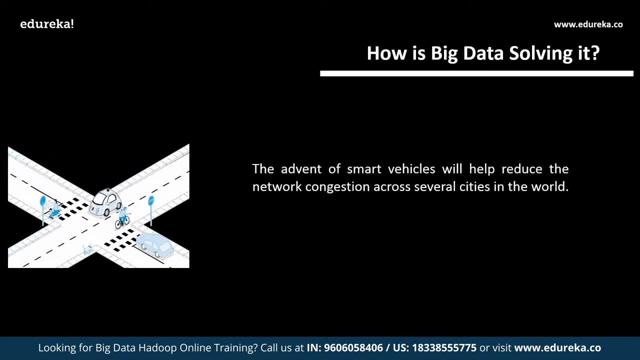 will assist traffic management and result in reduced congestion and roadblocks. The adoption of advanced sensors and GPS signal systems is revolutionizing the urban traffic network. These systems are designed to help reduce network congestion and act as alerts that notify traffic authorities of potential roadblocks and how to avoid them. The sensors are installed in trucks. 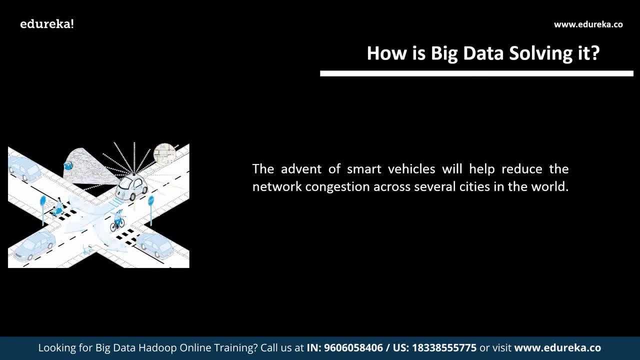 ships and airplanes that give real-time insights into drivers' capabilities and the traffic. GPS signals are utilized for bottlenecks and predict the condition of the transportation network. Followed by that, we have the emergence of smart vehicles, The advent of smart vehicles. 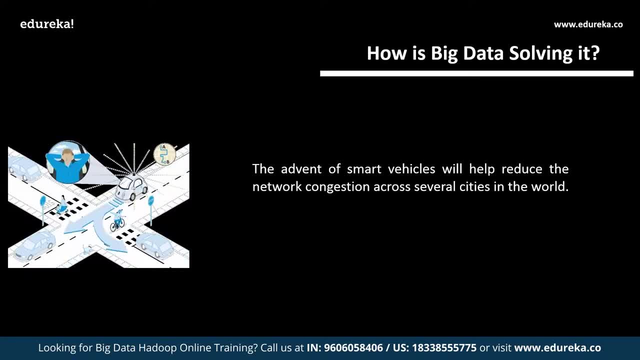 will help reduce the network congestion across several cities in the world. These are connected vehicles that provide real-time estimation of traffic patterns that help authorities with the deployment of management strategies. These systems are designed to improve the communication vehicle to infrastructure communications and monitor the traffic control to reduce collisions and accidents. Additionally, the 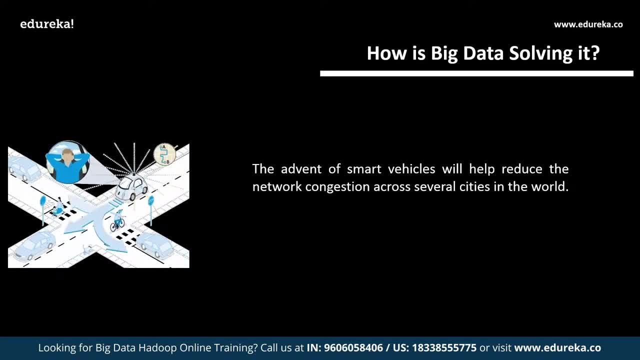 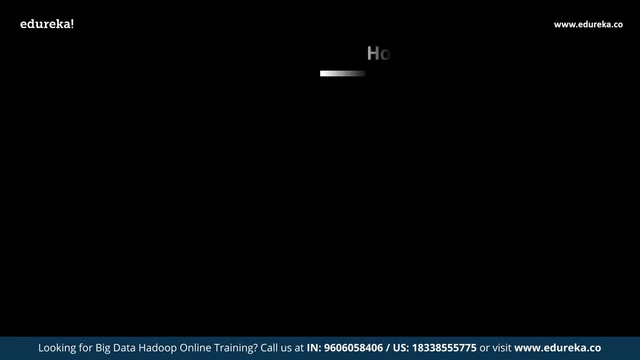 implementation of speed trackers, traffic sensors and display boats will result in smarter roads and help control speed and traffic issues effectively. Followed by that, we have telematics solutions. Telematics is extensively used in traffic management to provide statistics and information data. 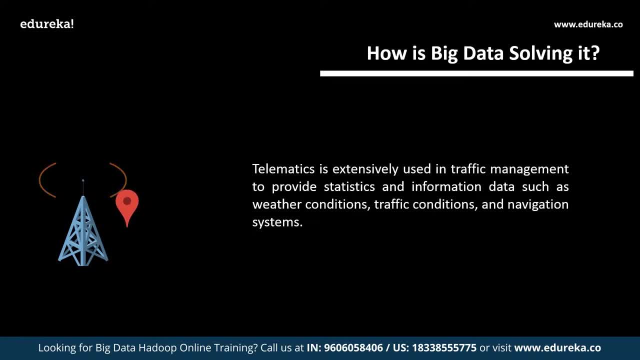 These systems provide real-time information and authorities leverage predictive analysis to determine the state of the transportation network. Moreover, telematics provide speech-based internet access to the consumers through wireless links that monitor the driver's state and stress levels and send alerts to the systems if there is any issue, to avoid or reduce chances. 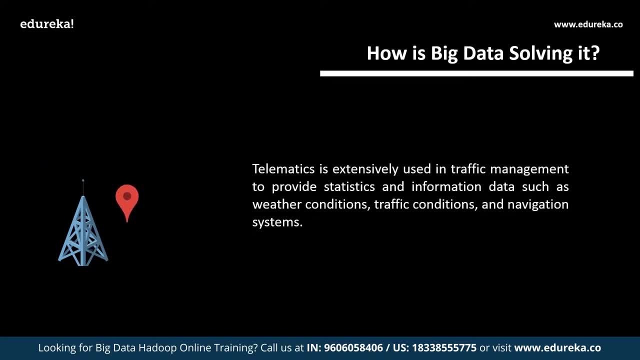 of collision. Now we shall discuss the outcomes and solutions. The outcomes and solutions offered: Big data analytics assessments on traffic network congestion identifies a set of transportation indicators that are measured using the mobile phone data available to travel agencies to optimize route planning. Some of the solutions offered are: 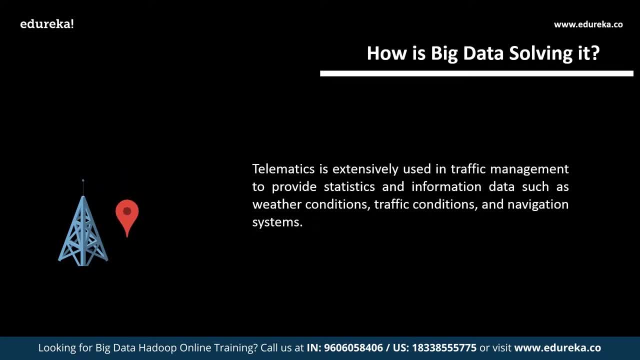 developed an integrated platform to perform data analysis in a scheduled, easy and controlled way, using a user-friendly interface. Offered an exhaustive understanding of how traffic demand is distributed in the transportation network, The outcomes and solutions offered are developed an integrated platform to perform data analysis in a scheduled, easy and controlled 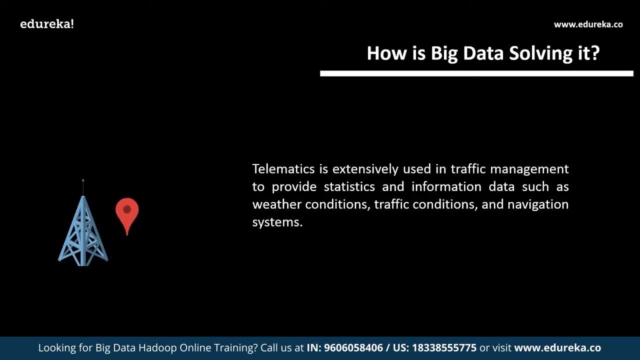 way using the mobile phone data. The outcomes and solutions offered are developed: an integrated platform to perform data analysis in a scheduled, easy and controlled way, using a user-friendly interface. These are entitled data analysis and analysis and analysis, The outcomes and solutions that have been provided include the following: 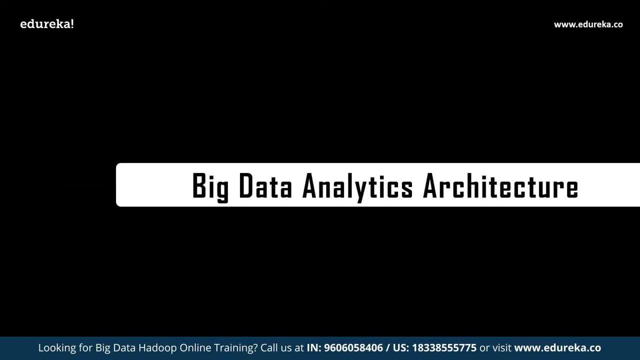 1. A comprehensive analysis of total number of trips made to and from each zone, based on date, time, month and holiday. 2. evidence-based data analysis for daily and traffic management systems. ITS generally has cameras set up on most populated areas of. 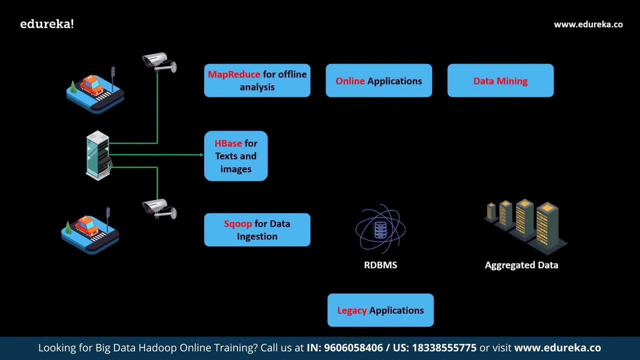 metropolitan cities. These cameras collect the visuals data in the form of photos and videos. This data is collected and stored in a storage unit. Generally, HBase is used for the job, as it is capable of storing all sorts of data, regardless of the type of data. Now there are 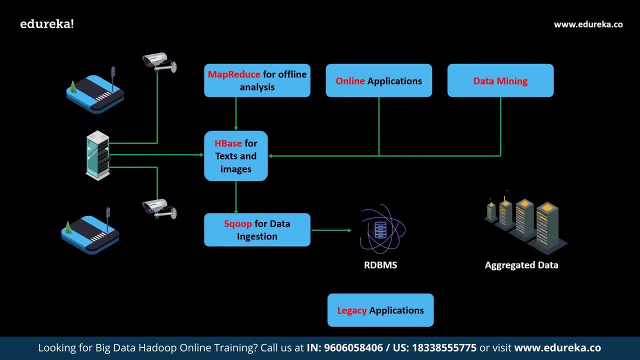 n number of calculations and processing that is applied onto the collected data. So for an offline data processing procedure, we use MapReduce, whereas on the other hand we use some high-end processing frameworks for online and interactive applications. The procedure involves active data mining for fetching most accurate data. The data is ingested. 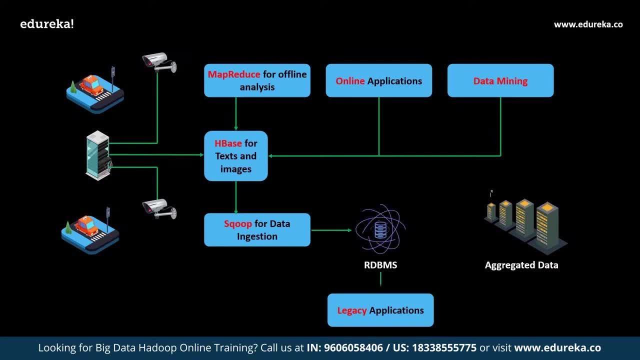 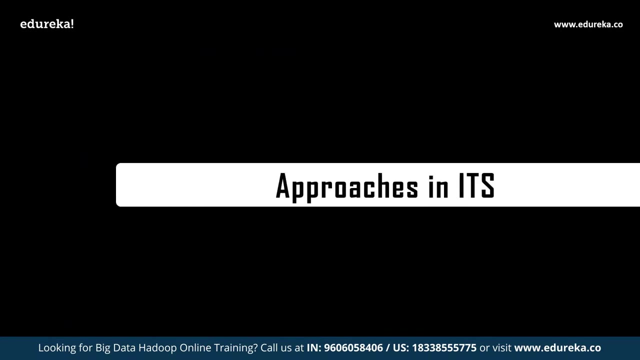 into RDPMS and other servers using Scoop, where the data is aggregated and the legacy applications are run over The data to analyze the data and provide the traffic department with latest updates in the live traffic. Now our next concern would be learning the approach to intelligent traffic. 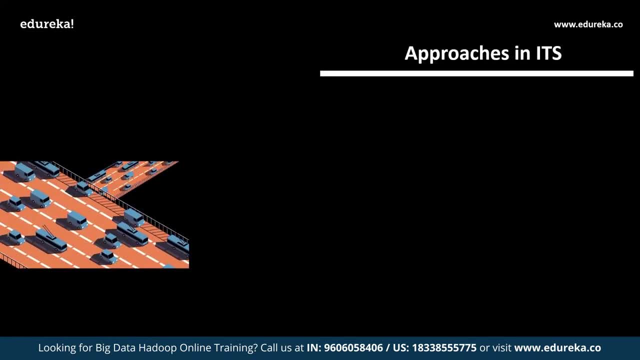 systems. There are five different stages in which the intelligent traffic control system works. They are traffic data collection, traffic data transmission, traffic safety measures, traffic data analysis and, lastly, providing the traveler with latest traffic updates as per his needs. Let's discuss each one of them. 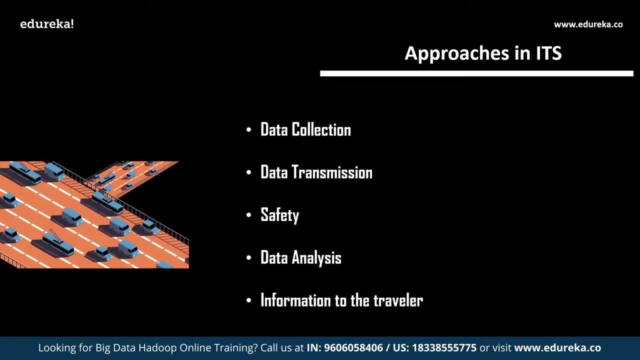 The first one, traffic management center. Traffic management center is the vital unit of ITS. It is mainly a technical system administered by the transportation authority. Here all data is collected and analyzed for further operations and control management of the traffic in real time or 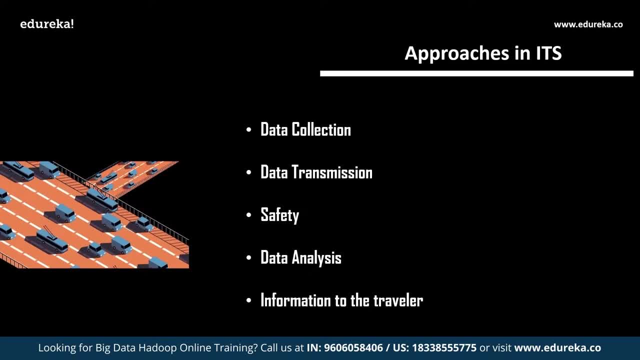 information about local transport vehicles. Well-organized and proficient operations of traffic management center depend on automated data collection with precise location and information, that analysis of data to generate accurate information and then transmitting it back to travelers. Let's understand the entire process in a more detailed way. 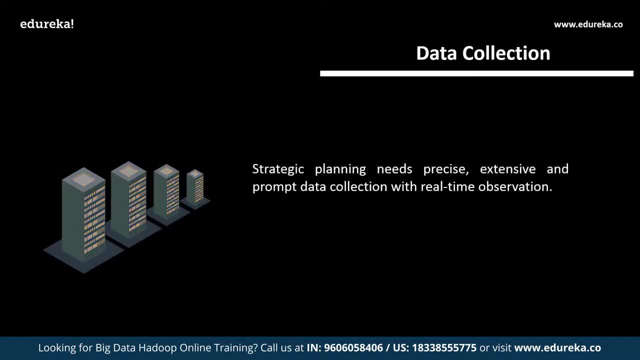 The first stage is data collection. Strategic planning needs precise, extensive and prompt data collection with real-time observation. So the data here is collected via varied hardware devices that lay the base of further ITS processes. This data is collected and stored into a storage unit. 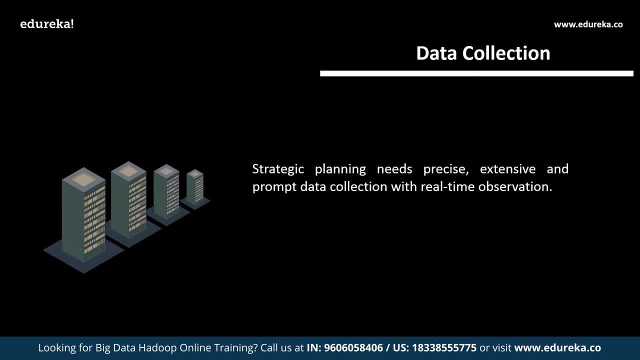 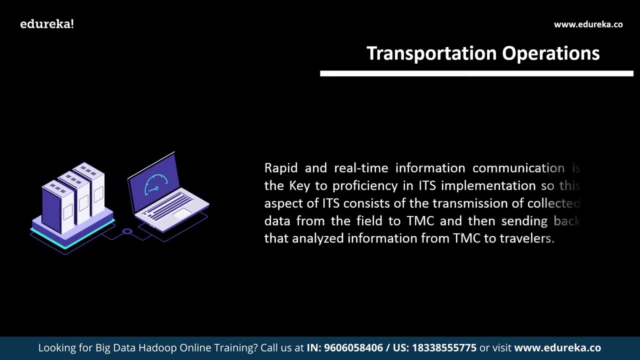 Generally, HBase is used for the job, as it is capable of storing all sorts of data, regardless of the type of data. Now there are n number of calculations and processes that need to be applied onto the collected data. The next stage is data transmission: Rapid and real-time information. 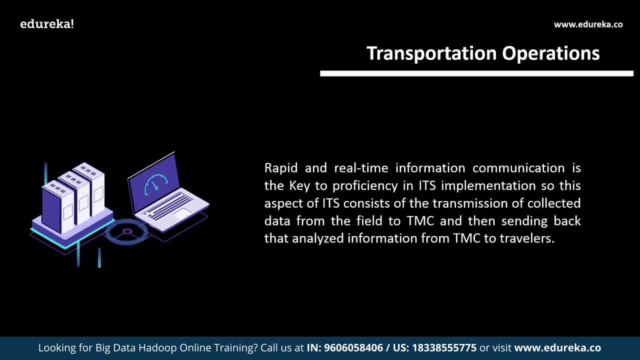 communication is the key to proficiency in ITS implementation. So the aspect of ITS consists of the transmission of collected data from the field to TMC and then sending data to the traffic department authorized by TMC. The data is then sent back to the DMC, in particular to 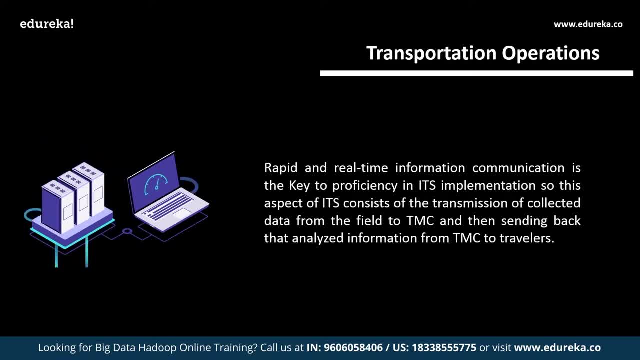 be processed. The list of traffic related announcements is divided into separate sections. TL and DMS are the three main sections. on the right to the DMS, The first step is the traffic related announcements, but you can follow up on the going. The last step is the. 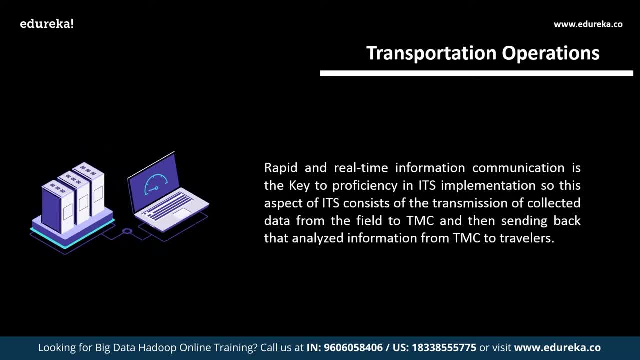 message communication. and the third step is the communication over the internet via SMS or on-board units of vehicles. The last step is the short-range communications through your 6G telecommunication. Other methods of communication are dedicated short-range communications, or DSRC, using radio and continuous air interface. long and medium range That. 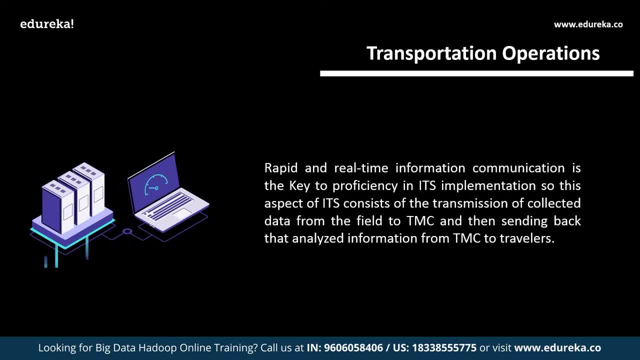 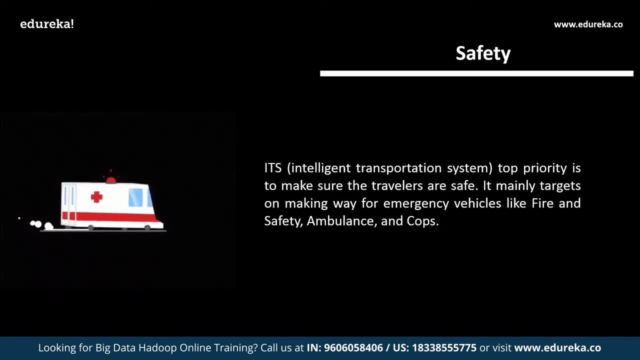 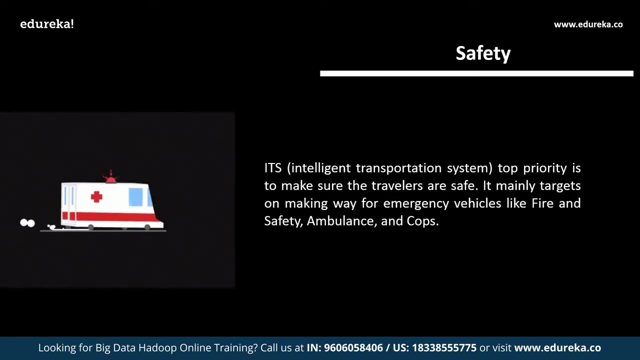 is CAILM, using cellular connectivity and infrared links. Followed by this, we have the safety. This is the safety. Intelligent transport systems' top priority is to make sure the travelers are safe. It mainly targets on the making way for emergency vehicles like fire and safety, ambulance and curbs. 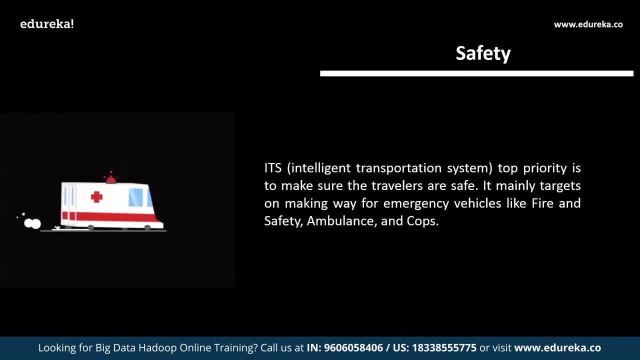 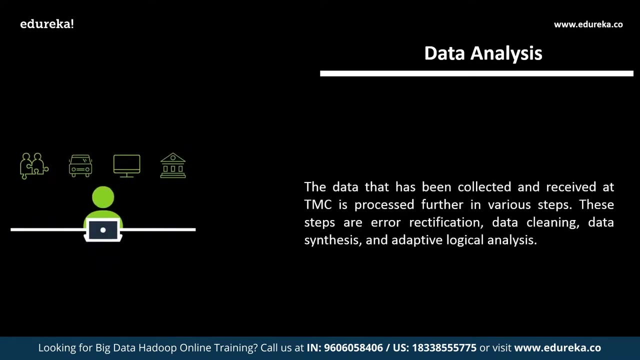 It looks after real-time traffic information, analyzes it and redirects the emergency vehicles to the most favorable routes to reach their destination faster and safer. The next stage is data analysis. The data that has been collected and received at TMC is processed for further in various steps. 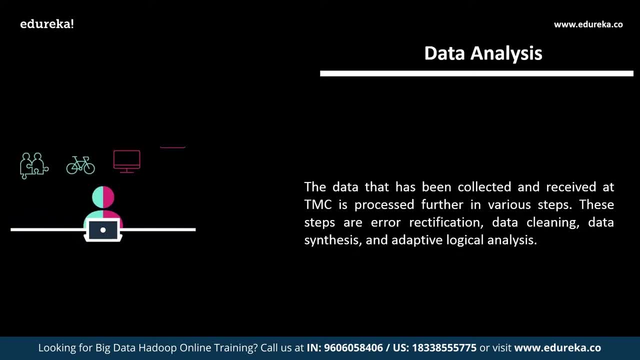 These steps are error rectification, data cleansing, data synthesis and adaptive logical analysis. The inconsistencies in data are identified with specialized software and rectified. After that the data is further alterated and pooled for analysis. This mandated collective data is analyzed further to predict traffic scenarios. 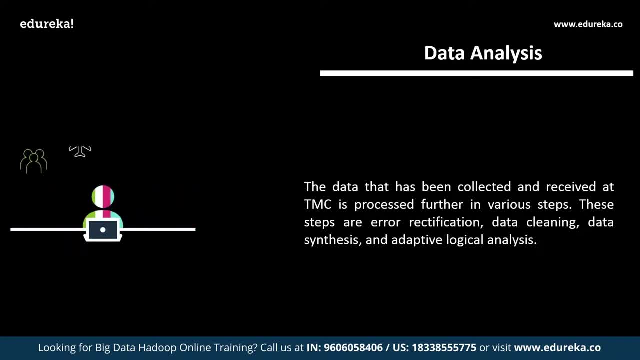 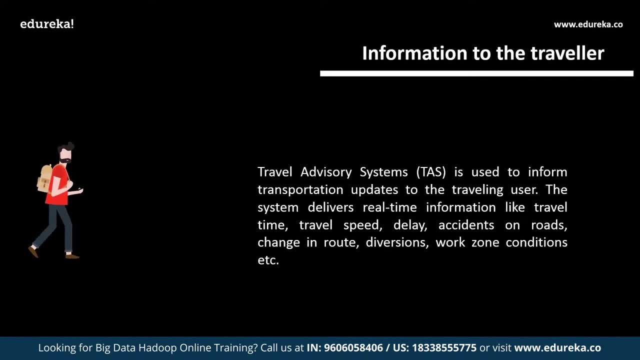 which are available. This is done to deliver appropriate information to users. Lastly, the traveler information. Travel Advisory Systems, or TAS, is used to inform transportation updates to the traveler. The system delivers real-time information like travel time, travel speed, delays, accidents. 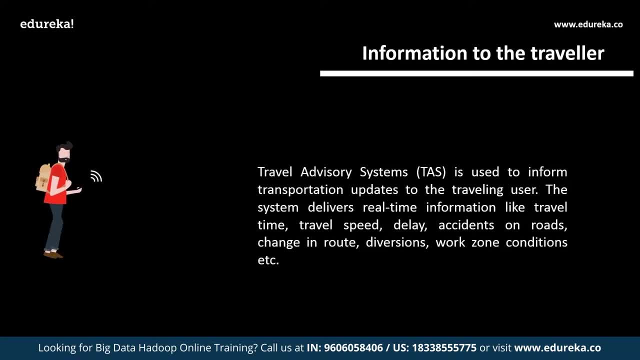 on roads, change in route diversions, work zone conditions, etc. This information is delivered by a wide range of electronic devices like variable message signs, highway advisory radios and other devices. You can access private information from a nearby flight information okay. 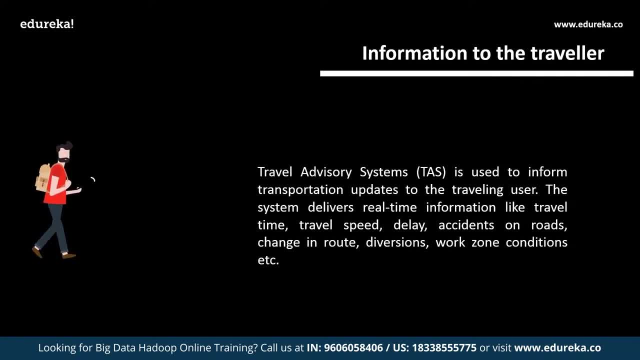 It will serve as a camera by watching video, internet SMS and automated cell call. In no time, traffic on this route will be regarded as text and glass: reaching high speeds, sharing the data if needed, getting know where it provides safety and comfort to citizens, and easy maintenance and surveillance. 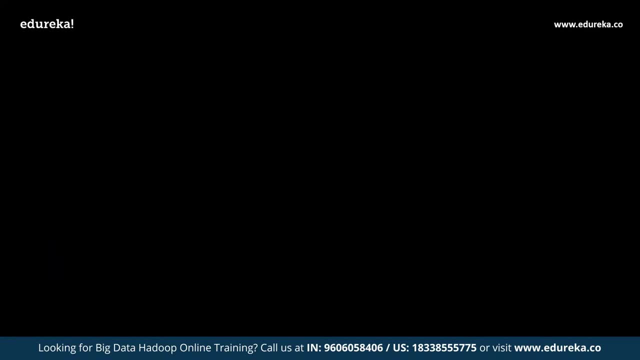 to city administrators. Now, moving ahead, we shall understand the hardware requirements of ITS. The hardware requirements for ITS are categorized into three major components. Those are the field equipment, communication systems and traffic management center. Now these three components have further requirements, which are mentioned below. They are field equipment that. 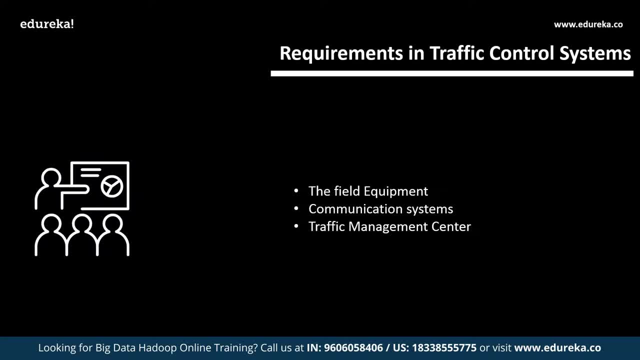 is the inductive loop detectors, magnetic detectors, infrared and microwave detectors, acoustic detectors and video imaging Moving ahead. the next one is the communication system, which requires wired and wireless communications. Followed by that, the last one is the traffic management center, which requires basic facility of staff signal control unit traffic surveillance. 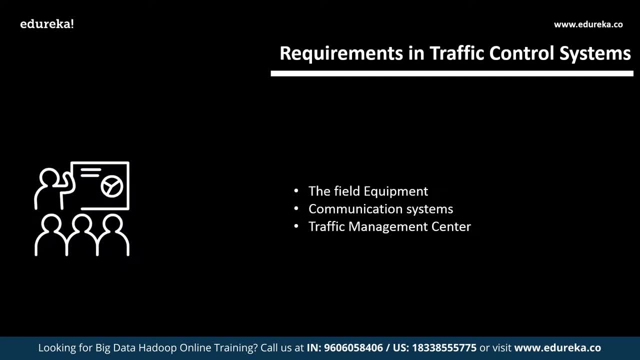 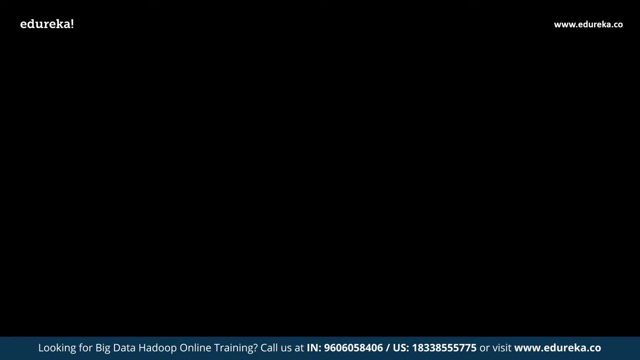 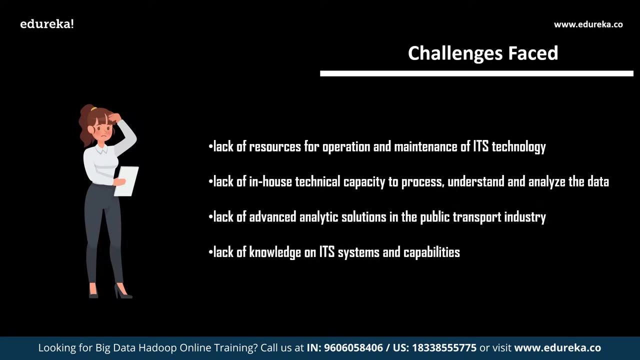 let's move ahead and understand the major challenges faced by ITS. So the major challenges faced by ITS are: lack of resources for operation and maintenance of ITS technology. lack of in-house technical capacity to process, understand and analyze the data. lack of advanced analytic solutions in the public transport industry. lack of knowledge. 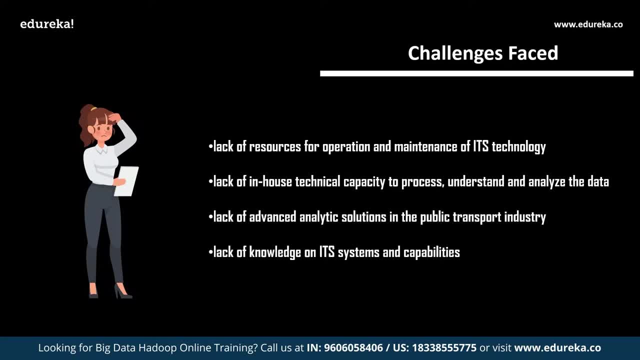 on ITS systems and capabilities to specify suitable terms when contracting ITS services to vendors. Followed by that, the lack of knowledge among vendors on specific needs of public transport operations, which significantly affects the utility of the end product. Now, with this, we shall now move ahead and wind up our session discussing the benefits of ITS. Data is stored. 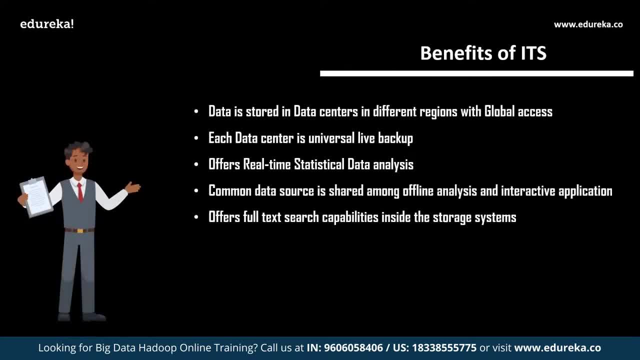 in data centers in different regions with global access. Each data center is universal live backup. It offers real-time statistical data analysis. It has common data source which is shared among offline analysis and interactive applications. It offers full text search capabilities inside the storage systems. It has an inbuilt indexing system to offer synchronization of traffic data. 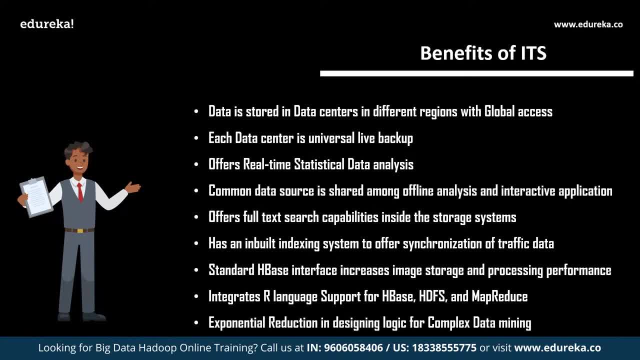 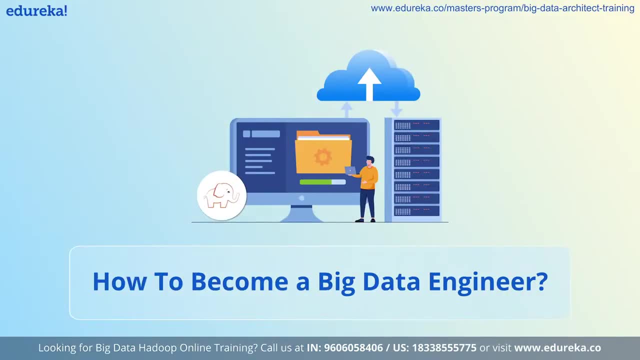 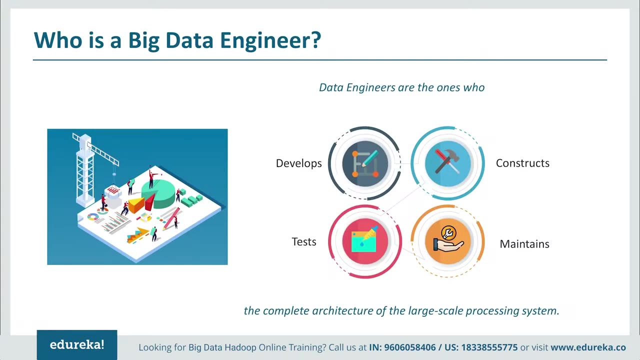 Standard edge-based interface increases image storing and processing performance. It integrates our language support for edge-based HDFS and MapReduce. Finally, exponential reduction in designing logic for complex data mining. So who's a big data engineer Now? every data driven business needs to. 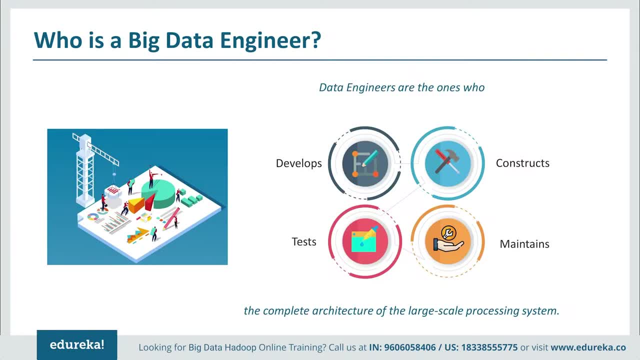 have a framework in place for the data science and data analytics pipeline, And a data engineer is the one who's responsible for building and maintaining this framework. Now, these engineers must ensure that there is an uninterrupted flow of data between servers and applications. So, in simple words, a data engineer builds tests, maintains data. 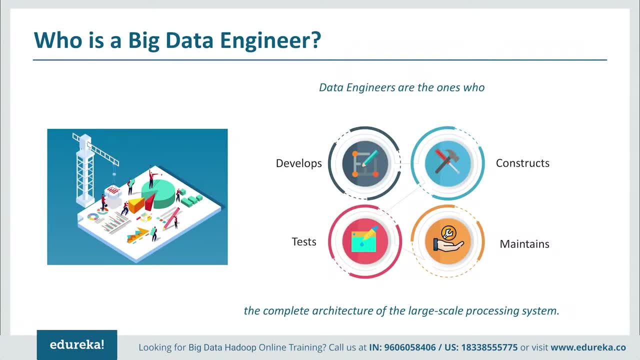 structures and architectures for data ingestion, processing and deployment of large-scale data intensive applications. Now, data engineers work in tandem with data architect, data analysts and data scientists, So they must all share these insights to other stakeholders in the company through data visualization and storytelling. But what does a big data engineer do exactly? 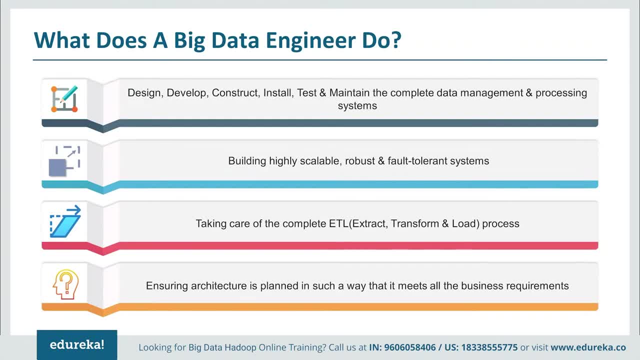 Now the most crucial part of a big data engineer is to design, develop, construct, install, test and maintain the complete data management and processing systems. They are basically the ones who handle the complete end-to-end infrastructure for data management and processing. They build a. 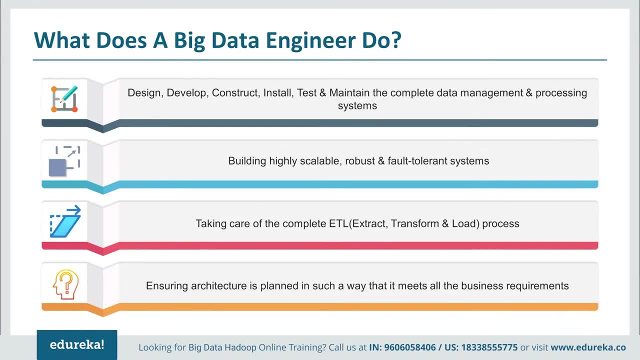 pipeline for data collection and storage and funnel the data to data analysts and scientists. So, basically, what they do is they create the framework to make data consumable for data scientists and analysts so they can use the data to derive insights from it. Note that the data engineers are the builders of data systems and not those who mine for insights. 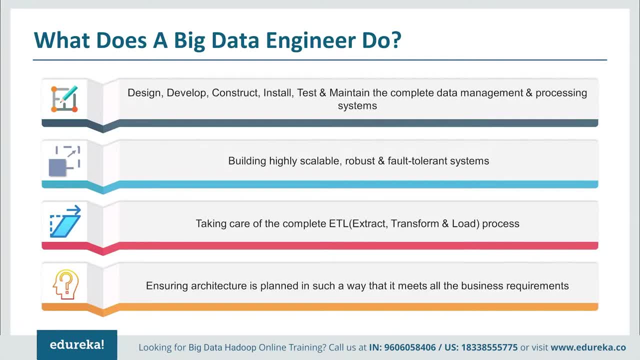 So the data engineer works more behind the scenes and must be comfortable with other members of the team producing business solutions from this data. Now, all their responsibilities revolve around this. They need to take care of a lot of things while performing these activities. Hence one of the most sought-after skills. 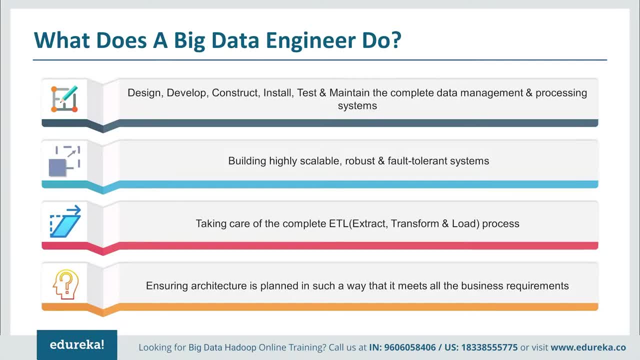 in data engineering is the ability to design and build data warehouses. This is where all the raw data is collected, stored and retrieved from. Without data warehouses, all the tasks that a data scientist does will become obsolete. It is either going to get too expensive or 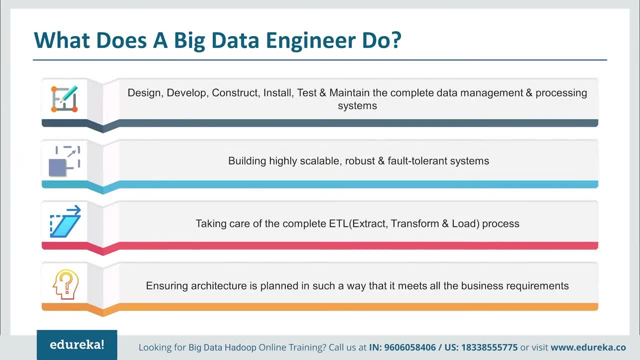 very, very large to scale. Now, data engineers should always keep in mind that the system which he or she builds needs to be scalable, robust and fault tolerant, so that the system can be scaled up while increasing the number of data sources and can handle a huge amount of heterogeneous data. 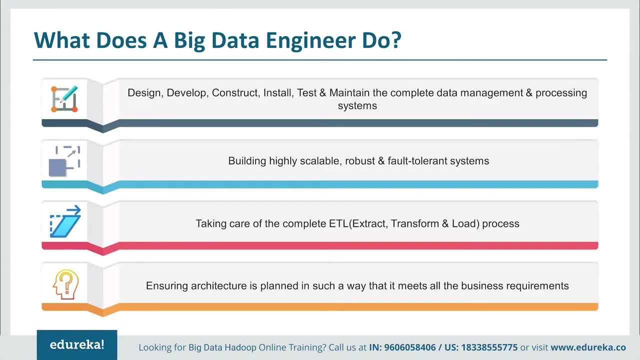 without any failure. Now imagine a situation wherein the source of data is doubled or tripled, but the system cannot scale up. Will it not cost a lot more time and resources to build the same system again which is suitable for this kind of intake? Exactly This is why the big data 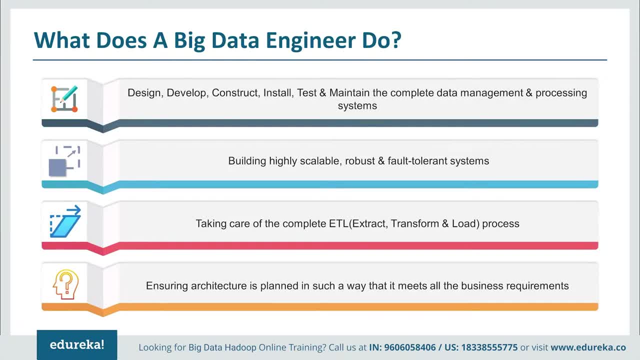 engineers have a role here. Next, he or she is the one that handles the extract, transform and some other tasks. This is where the data engineers can contribute to the development of data load process, which is basically the blueprint for how the collected raw data 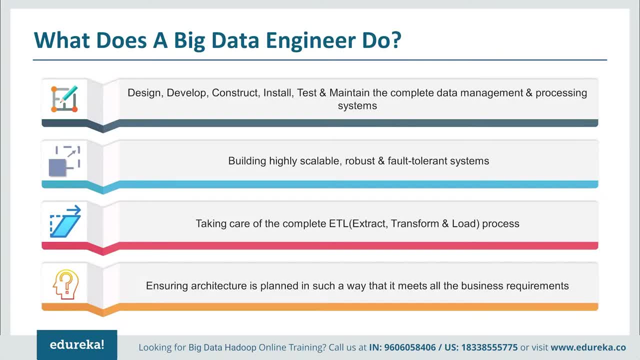 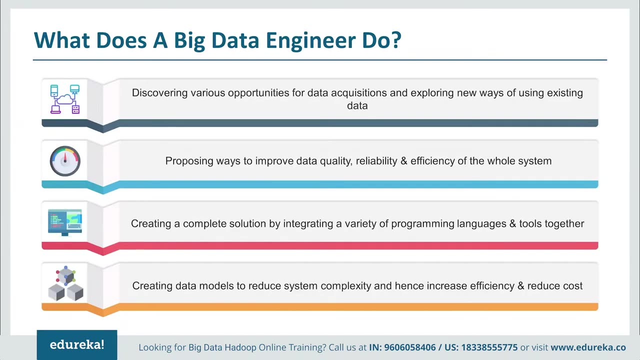 is processed and transformed into data ready for analysis. now you're going to acquire a lot of data from different sources. how do you bring them together to one platform? ETL is your answer. apart from all this, a data engineer should always aim at deriving insights by acquiring data from new sources. some of 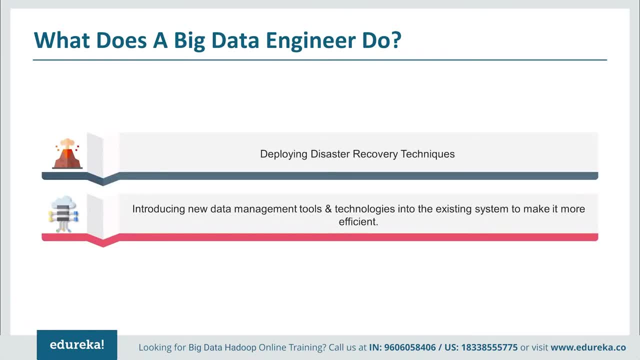 the responsibilities of a data engineer also include improving data foundational procedures, integrating new data management technologies and the software into existing systems and building data collection pipelines. and finally, one of the major rules of a data engineer is to include performance tuning and make the whole system way more efficient, which is pretty. 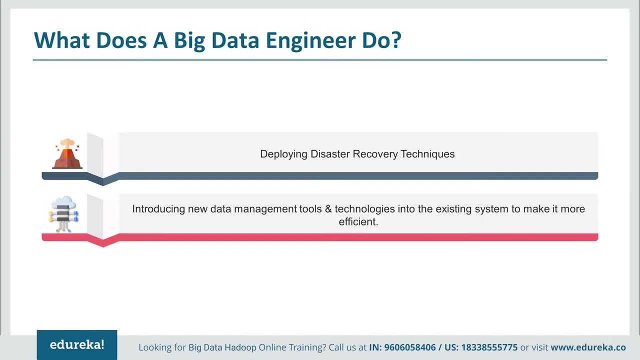 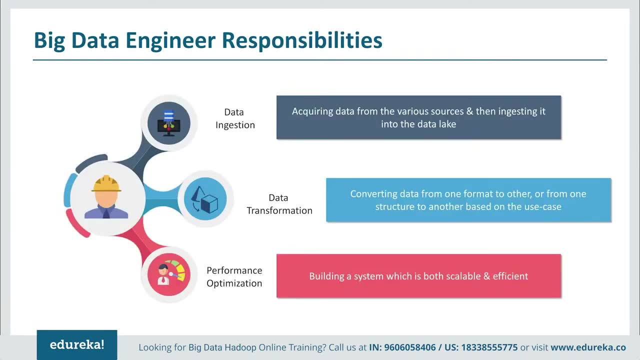 self-explanatory, if you ask me. now, most of us have some idea about who a big data engineer is, But there's still some confusion about their responsibilities. now this ambiguity further increases when we gain more information about the role. now let me help you debunk all your queries about it. so let's talk about some big 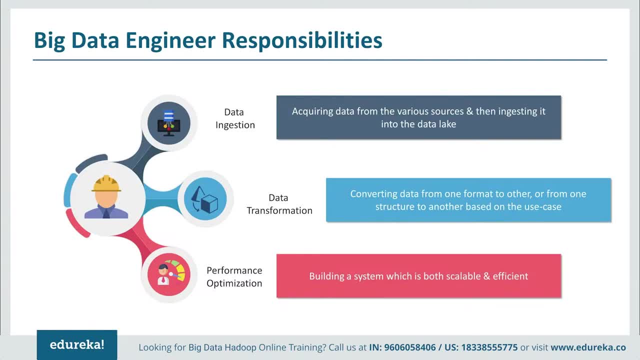 data engineer responsibilities. first up, we have data ingestion. now this is associated with the task of getting data out of the source systems and ingesting it into a data lake. now a data engineer would need to know how to efficiently extract the data from a source, including multiple approaches for 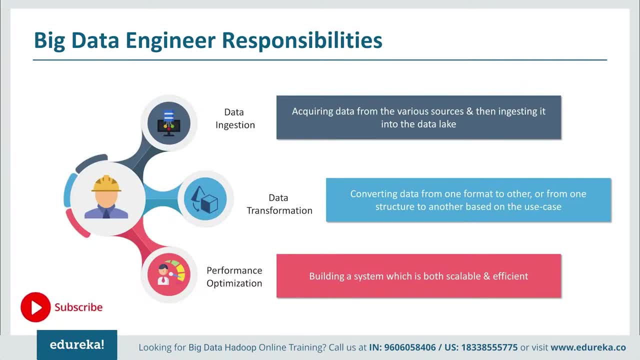 both batch and real-time extraction, as well as needing to know about the incremental data loading fitting within small source windows and parallelization of data loading as well. now, another small subtask of data ingestion is data synchronization, but because it's such a big issue in the big data world, we are 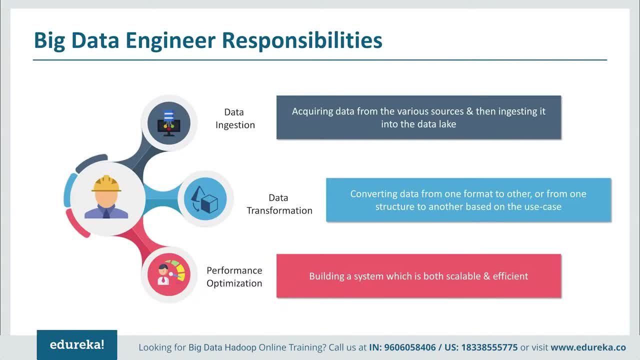 gonna talk about it now. since Hadoop and other big data platforms don't support incremental loading of data, A data engineer would need to know how to deal with detecting changes in the data source, merge and sync- change data from sources into the big data environment. next, 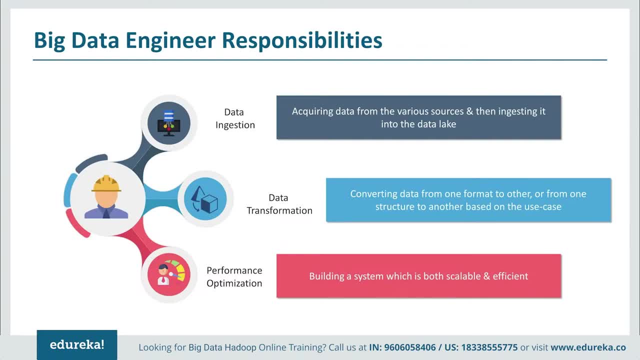 We have data transformation. This is basically the tea in the extract, transform and load that we had discussed earlier. It is basically focused on integration and transformation of data for a specific use case. Now, a major skill set here is the knowledge of SQL. as it turns out, not much has changed. 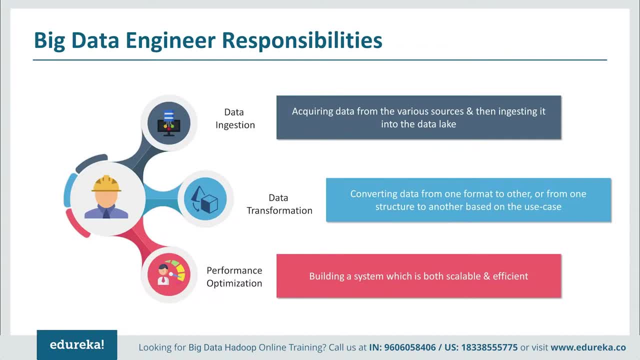 in terms of the type of data transformations that people are doing now compared to purely relational environments. Now imagine all this data that you've acquired from various sources. What would you have to do to make them all palatable in the same platform? You need to transform that data, and this is what a data engineer does here and finally, 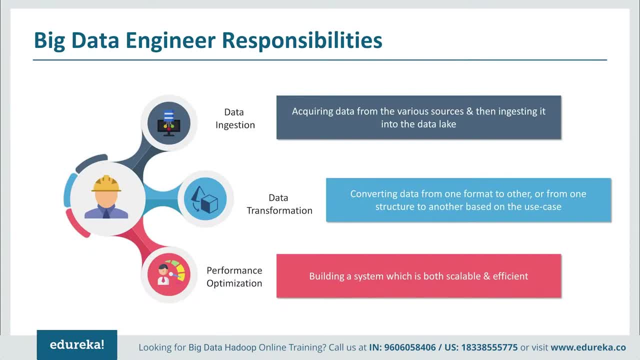 we have performance optimization, which is one of the tougher areas, because anyone can build a slow-performing system. The challenge is to build data pipelines That are both scalable and efficient. So the ability and understanding of how to optimize the performance of an individual data pipeline and the overall systems are a higher level of data engineering skill. 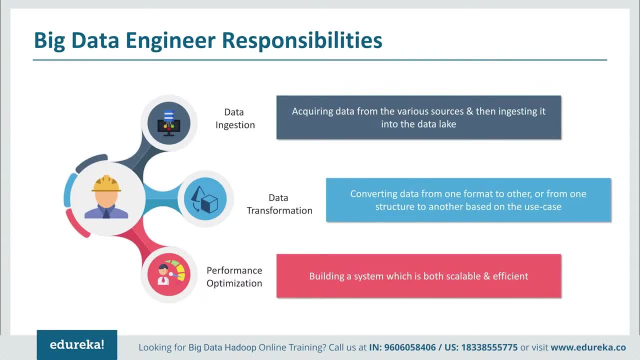 Now, for example, big data platforms continue to be challenging with regard to query performance and have added complexity to a data engineers job. in order to optimize performance of queries and creation of reports, the data engineer needs to know how to denormalize, partition and index data models. 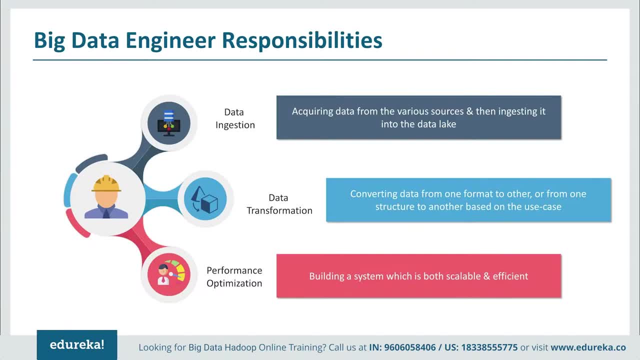 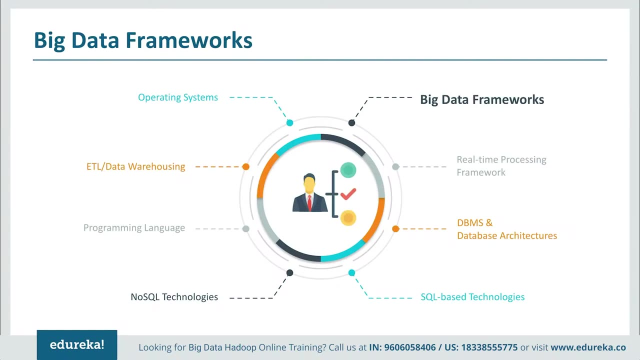 He also needs to understand tools and concepts regarding in-memory models and OLAP cubes. Now let's quickly move ahead and look at the required skills to fulfill these responsibilities. Now we'll be going through these skills in a clockwise order. So, starting with big data frameworks, now with the rise of big data in the early 21st century. 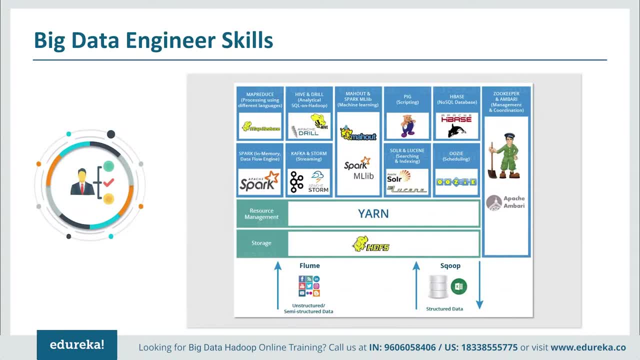 a new framework was born, and that is Hadoop. all thanks to Doug cutting for introducing this framework. It not only stores big data in a distributed Manner, but also processes the data parallelly. there are several tools in the Hadoop ecosystem which catered differently for different purposes and professionals. for a big data engineer: 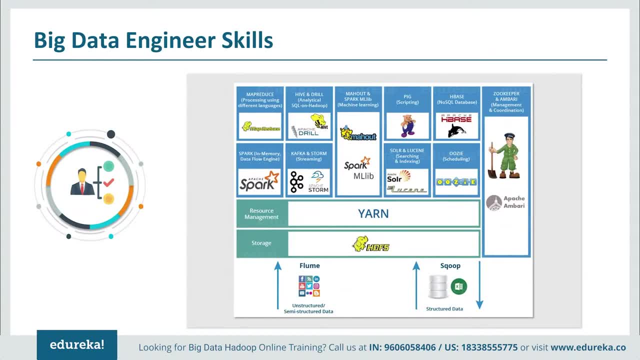 mastering big data tools is a must. some of the tools which you will need to master. First of all, you have HDFS, which is the storage part of Hadoop, being the foundation of Hadoop. knowledge of HDFS is a must to start working with Hadoop framework. 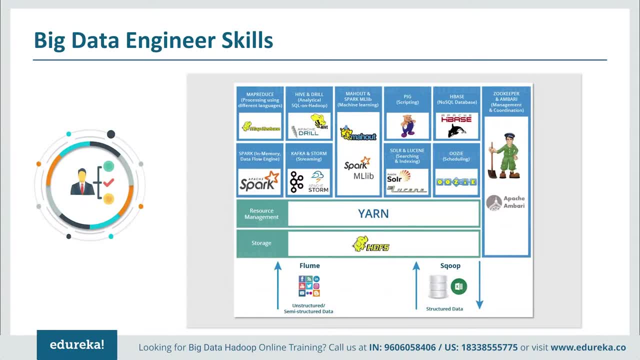 Next we have yarn, which performs resource management by allocating resources To different applications and scheduling jobs. now MapReduce is a parallel processing Paradigm which allows data to be processed parallelly on top of the HDFS. next we have big and hive. now, hive is a data warehousing tool on top of HDFS which caters to professional 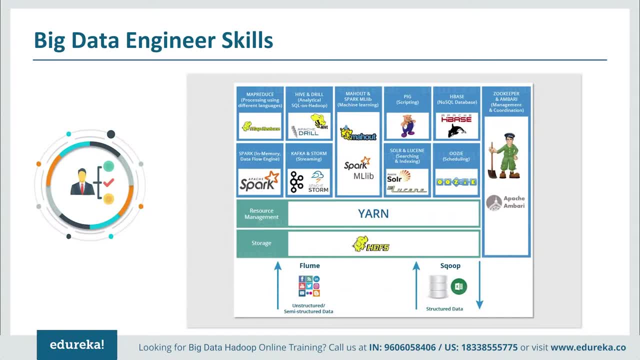 from an SQL background to perform analytics on top of HDFS, Whereas Apache, pig is a high-level platform which is used for data transformation on top of Hadoop. Now, hive is generally used by data analyst for creating reports, Whereas pig is used by researchers for programming. both are pretty easy to learn if you already. 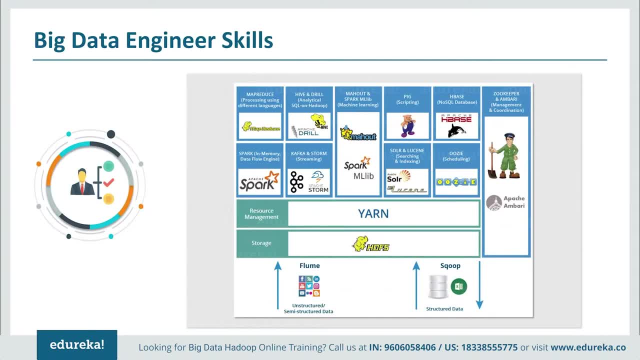 familiar with SQL. next we have flume and scoop. flume is a tool which is used to import unstructured data to HDFS, and scoop is used to import and export structured data from our DBMS. Now, next, we have zookeeper, which acts as a coordinator among the distributed services. 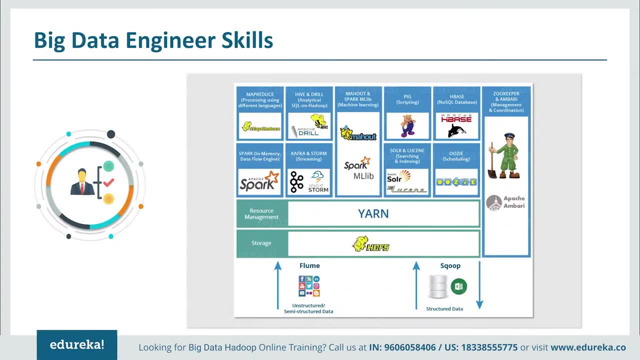 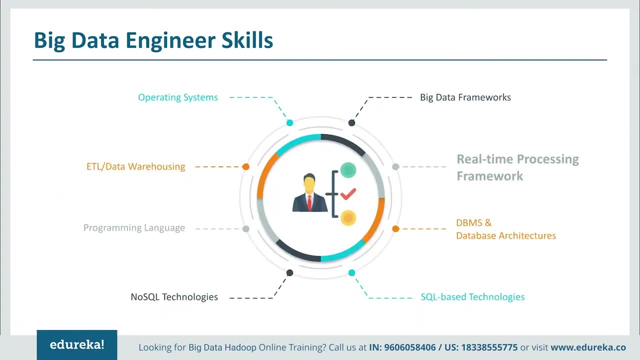 running in a Hadoop environment, Basically helps to configure, management and synchronize services. and finally, we have Uzi, which is basically a scheduler which binds multiple logical jobs together and helps in accomplishing a complete task. next up, We have real-time processing frameworks. now, real-time processing with quick actions is 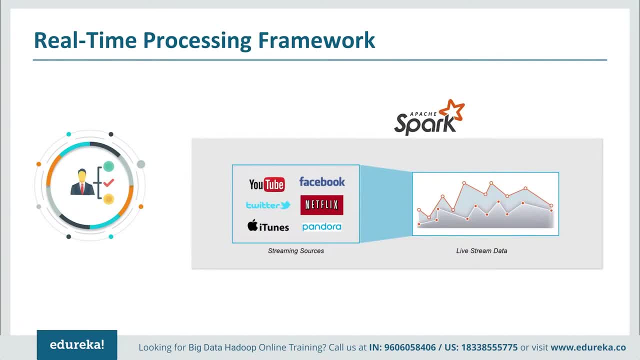 the need of our either it is a credit card fraud detection system or a recommendation system. Now imagine if you wanted a red dress today and Amazon To suggest it to you a month later now. wouldn't that be completely useless for you? in this case, you need real-time processing. it is very important for a data engineer to have knowledge. 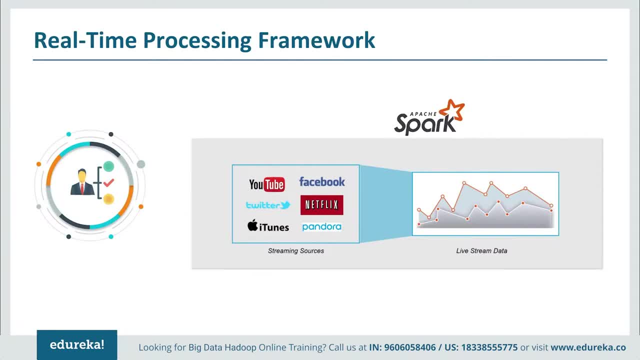 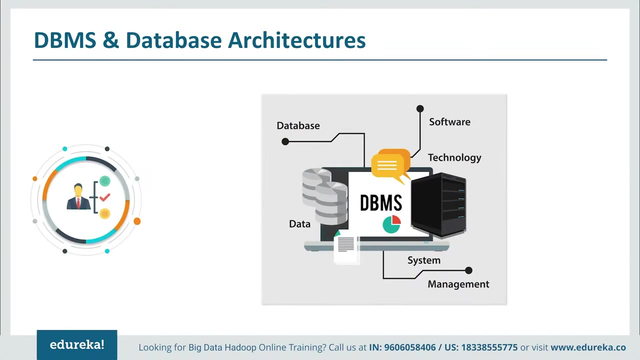 of real-time processing frameworks. Now Apache spark is one of the distributed real-time processing frameworks which is used in the industry rigorously. It can be easily integrated with Hadoop leveraging HDFS as well. Next, we have DBMS, now a database management system. 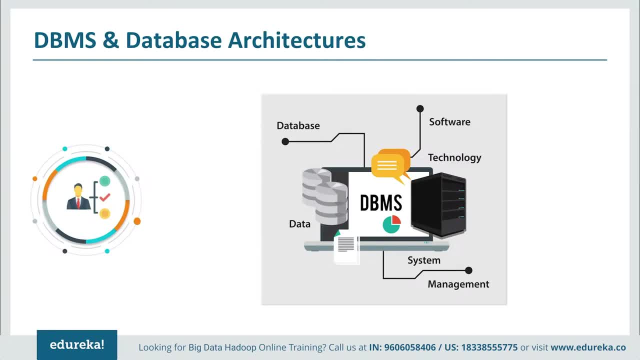 Stores, organizes and manages a large amount of information within a single software application. Now data engineers need to understand the database management system to manage data efficiently and allow users to perform multiple tasks with ease. This will help data engineers in improve data sharing, data security, data access. 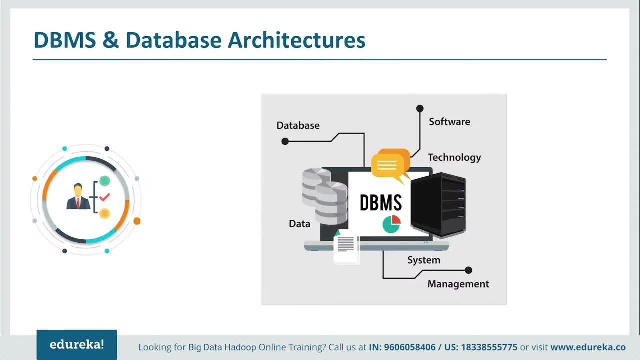 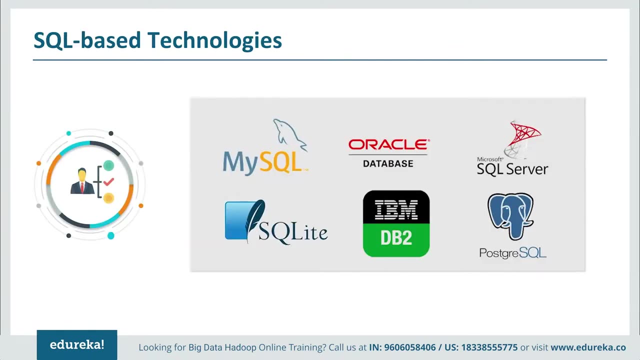 and better data integration, with minimize data inconsistencies. These are the fundamentals that data engineers should know prior to building a scalable, robust and fault-tolerant system. Next, we have SQL based Technologies. Now there are various relational databases that are used in the industry, such as Oracle. 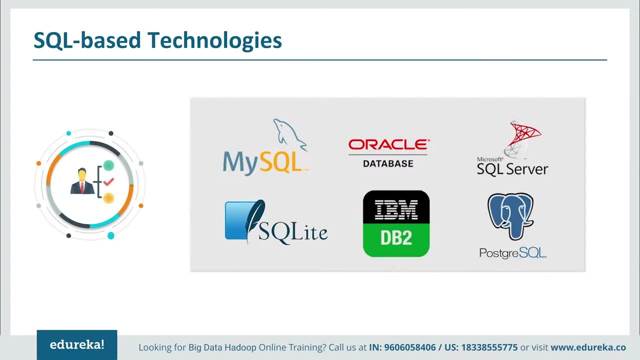 DB, Microsoft SQL Server, Etc. Now data engineers must have at least the knowledge of one such database. Now, knowing SQL is also a must. this structured query language, as SQL, is also known as, used to structure, manipulate and manage data stored in relational databases. As data engineers work closely with our DBMS, is they need to have a strong command on? 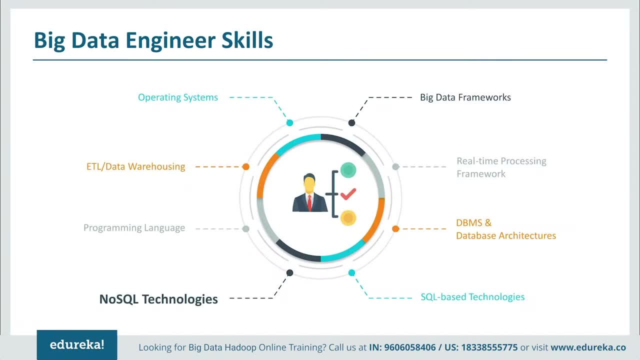 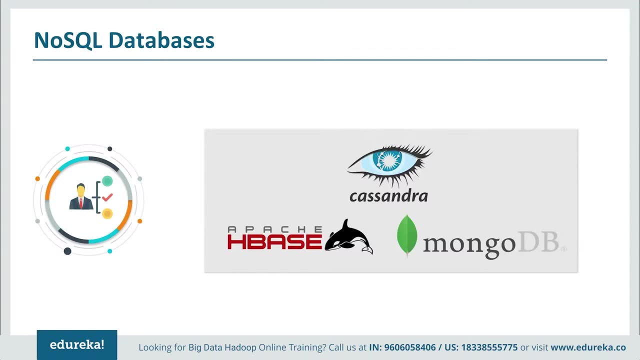 SQL Now. next, we have no sequel Technologies. as the requirements of organizations have grown beyond structured data, No sequel databases have been introduced into this environment. It can store large volumes of structured, semi-structured or unstructured data, with quick iteration and agile structure as per application requirements. some of the most prominently used data: 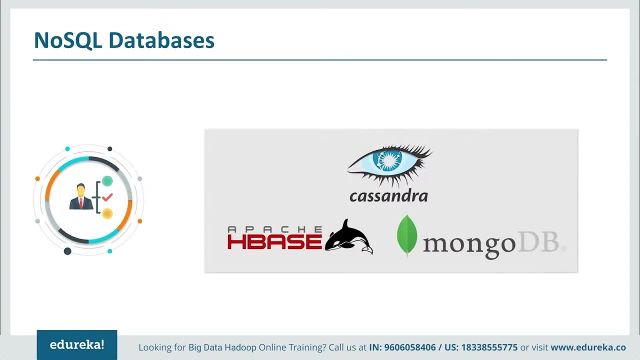 Bases are HBase, Cassandra and MongoDB. now, HBase is a column oriented, no sequel database on top of HDFS, which is great for scalable and distributed big data stores. It is also great for applications with optimized read and range based scan and it provides 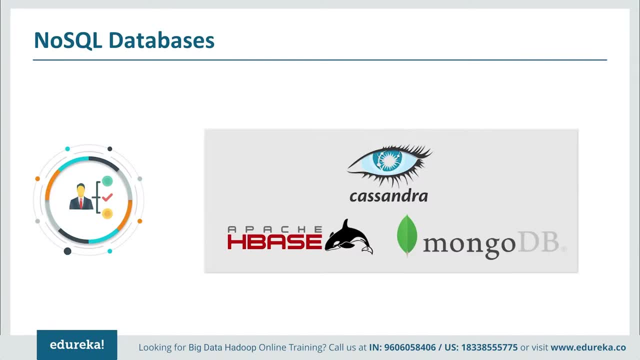 consistency and partitioning out of CAP. now Cassandra is a highly scalable database with incremental scalability, and the best part about Cassandra is the minimal administration and no single point of failure. It's good for applications with fast and random read and writes. it provides available and partitioning out of CAP. and finally, we have MongoDB, which is basically a document oriented. 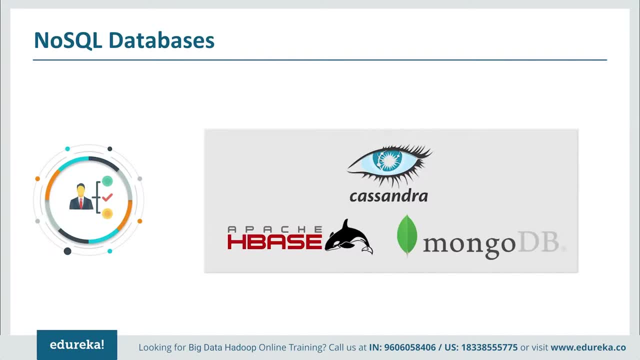 no sequel database, which is a schema free database. It gives full index support for high performance and replication for fault tolerance. It has a master slave sort of architecture and provides CP out of CAP. It Is rigorously used by web applications and semi-structured data handling. next, 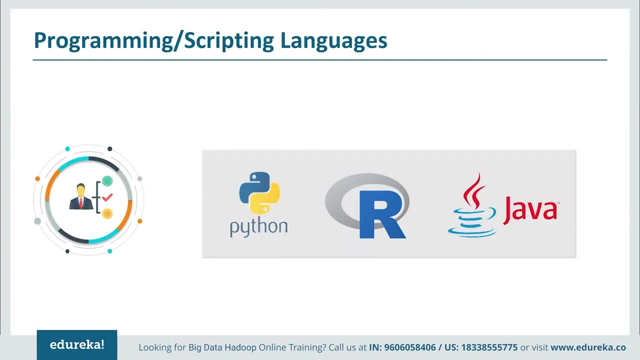 We are going to discuss programming and scripting languages, So various programming languages can serve for the same purpose. So knowledge of one programming language is enough. and seeing this, because the flavor of language may change, but the logic remains the same. If you're a beginner, you can go ahead with Python, as it is an easy language to learn. 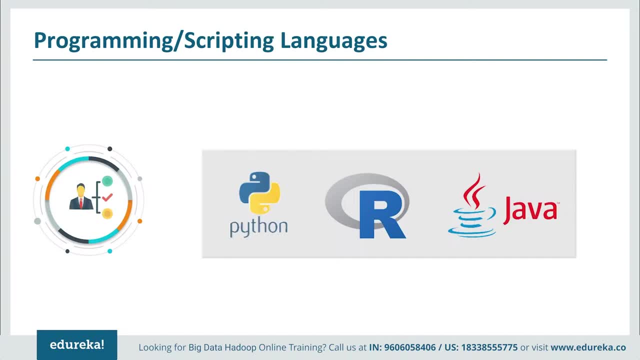 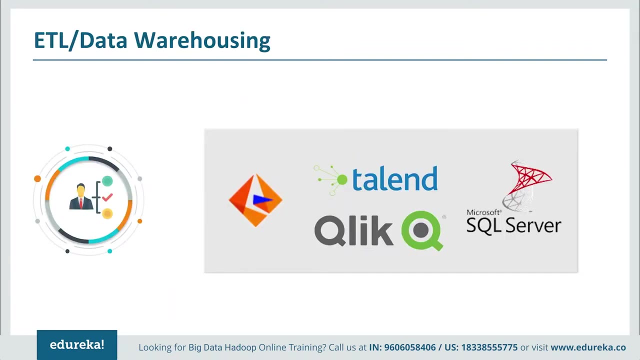 due to its syntax and good community support, Whereas R has a steep learning curve, which is developed by statisticians, and it is mostly used by analysts and data scientists. The next skill we're going to discuss is an important one. It is ETL, or data warehousing. now, data warehousing is very important. 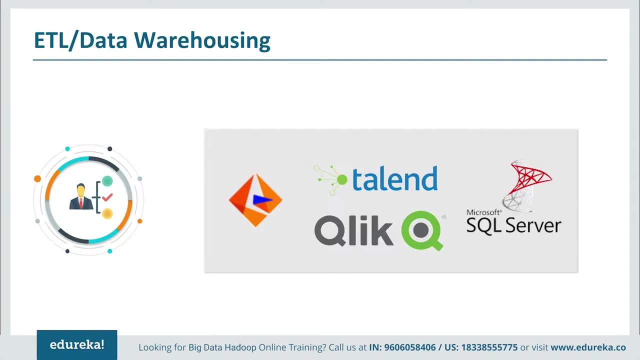 when it comes to managing a huge amount of data coming in from heterogeneous sources where you need to apply, extract, transform and load. now, data warehousing is used for analytics and reporting and is a very, very crucial part of every business intelligence Solution, because this is the part which is going to take you most time. 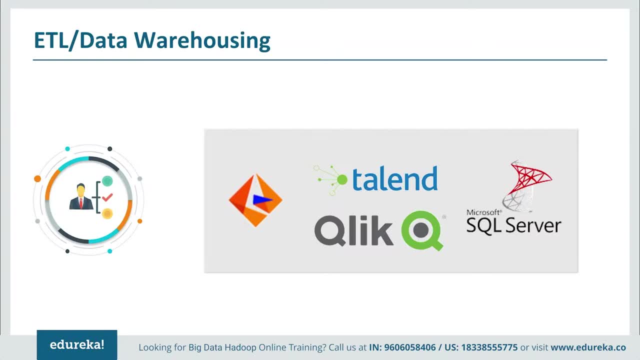 Now it is very important for a big data engineer to master one data warehousing or ETL tool. after mastering one, it becomes pretty easy to learn new tools and as the fundamentals remain the same now, informatica, click view and talent are very well-known tools used in the industry informatica. 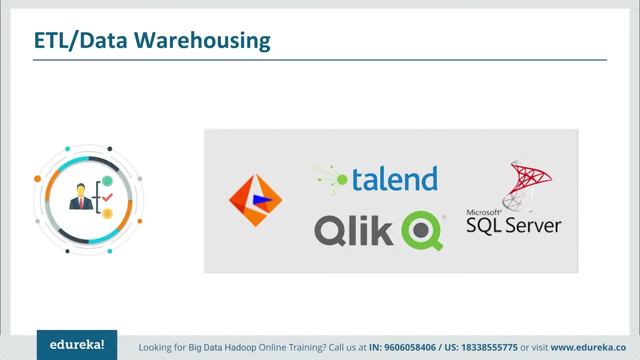 and talent open studio are data integration tools with ETL architecture. The major benefit of talent is its support from the big data frameworks. if you're new to data warehousing and ETL tools, I would definitely recommend you start with talent, because after learning this, any data warehousing tools will become a piece of cake. 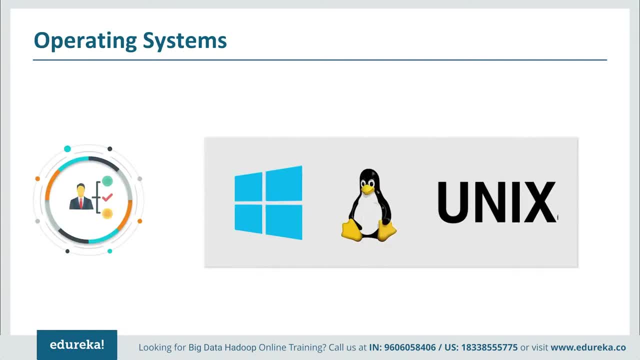 and finally, we have our operating systems. now, intimate knowledge of Unix, Linux and Solaris is very helpful, as many mathematical tools are going to be based off of these systems due to their unique demands for root access to hardware and operating system functionality Above and beyond that of Microsoft's Windows or Mac OS. now some level. 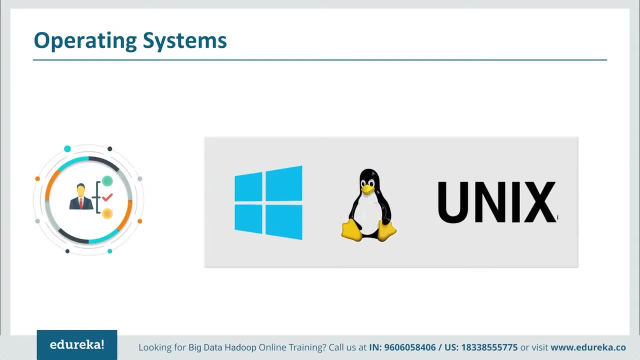 of understanding of how to act upon this data is also very valuable for data engineers. for this reason, some knowledge of statistical analysis and the basics of data modeling are also hugely valuable. knowledge of machine learning and cloud also will serve as a big plus. while machine learning is technically something relegated to a data scientist knowledge 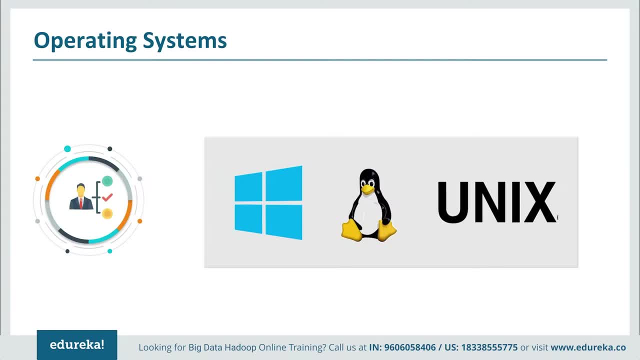 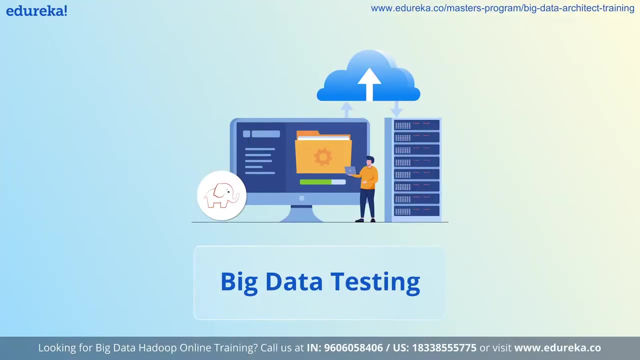 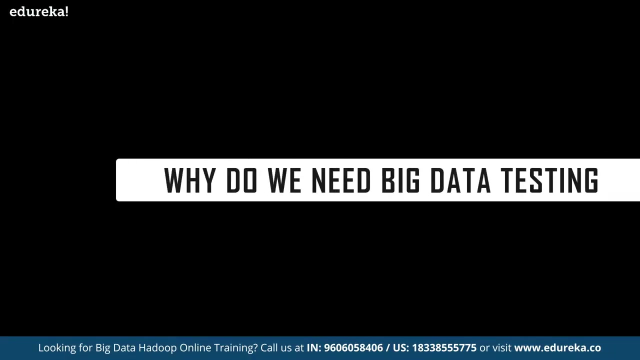 in this area is helpful to construct solutions usable by your cohorts. Now, this knowledge has the added benefit of making you extremely marketable in this space, as being able to put on both hats in which case makes you a really formidable tool. Now let us quickly start with our first chapter. 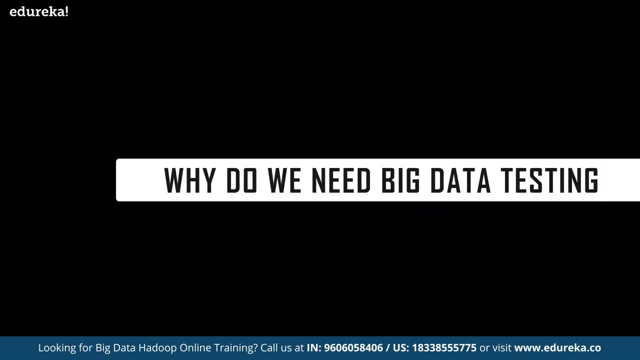 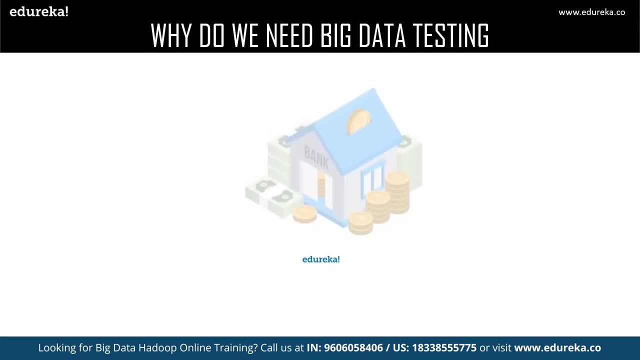 The first chapter is about learning why exactly we need to test the big data. Most of the users might end up with one question that asked why exactly we need to test the big data. You might have written the queries correct and your architecture might be just fine, yet 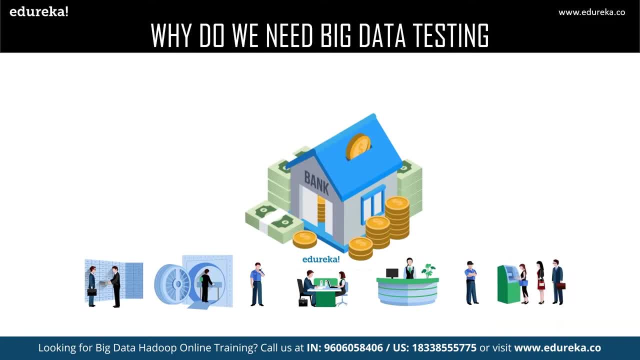 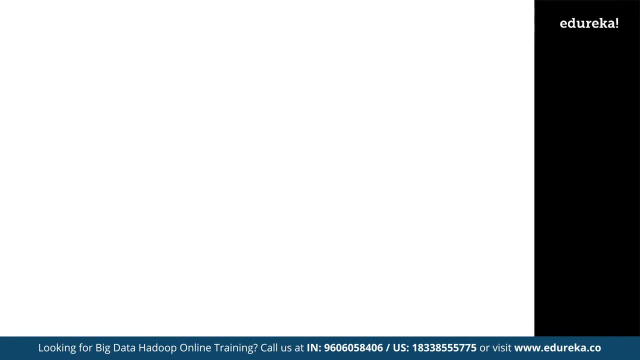 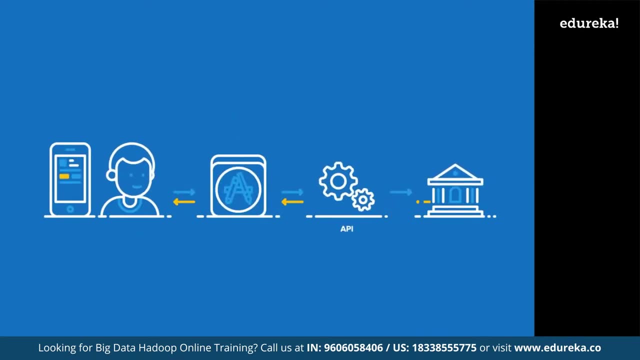 There might be many possibilities for a failure. Let us assume a classic case of a drastic failure that occurred in a bank. The designers of the bank database wanted to create a phone application which could enable phone banking to the customers. So the designers of the bank database name the customer name as CN. 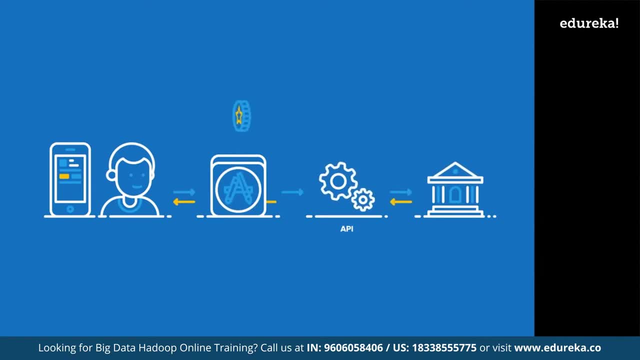 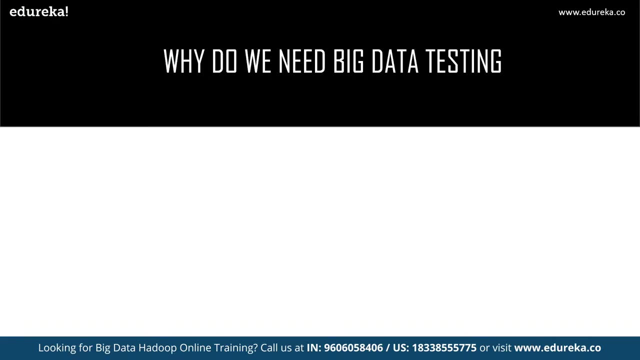 the customer bank location: pin code as CL, customer ID as C ID and customer phone number as CP. Now the bank wants to make key value pairs of customer ID, which is CI, and customer phone number, that is CP. in this scenario, The MapReduce algorithm gets messed up between the letters P and L. 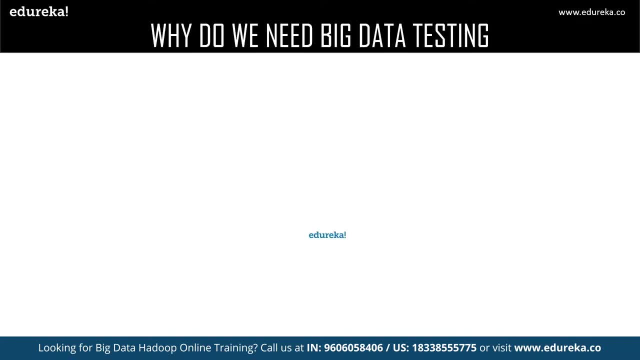 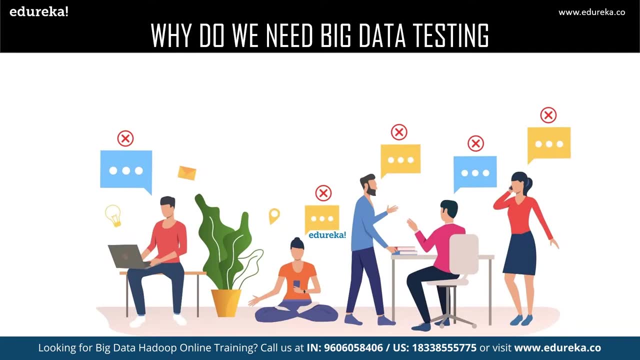 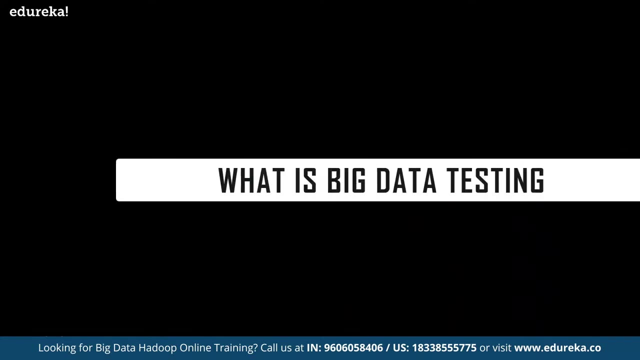 which is a keypad error or the typing error. Now the customers won't be getting the OTP and the phone banking facilities. just imagine This scenario in a real-time situation. horrible, right. So to avoid such mistakes in real time, we prefer the big data testing now. 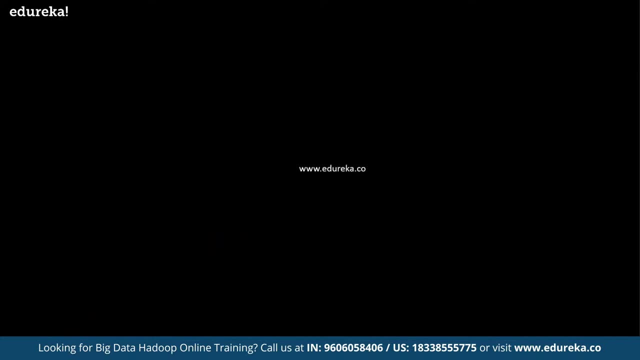 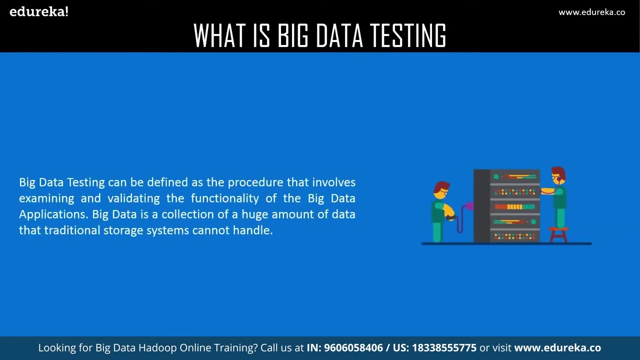 we shall understand what exactly is big data testing. So big data testing can be defined as a procedure that involves examining and validating the functionality of big data applications. The big data is a collection of a huge amount of data that traditional storage systems cannot handle. testing. 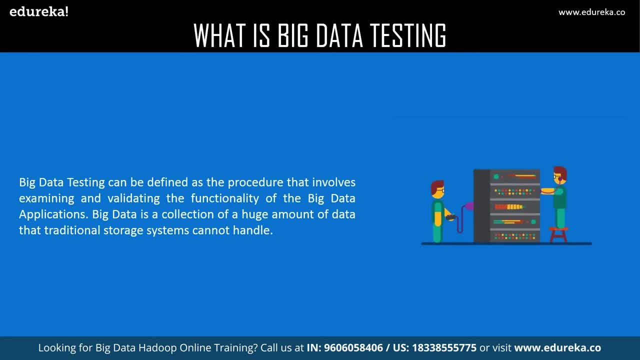 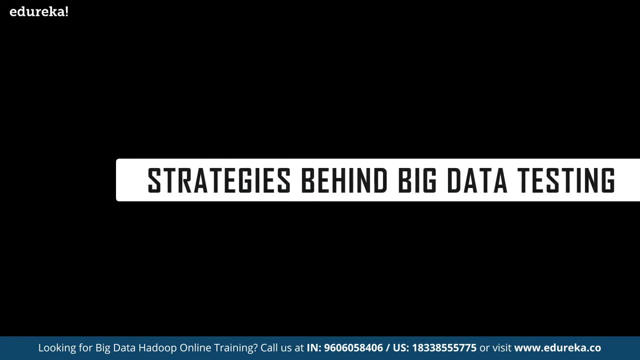 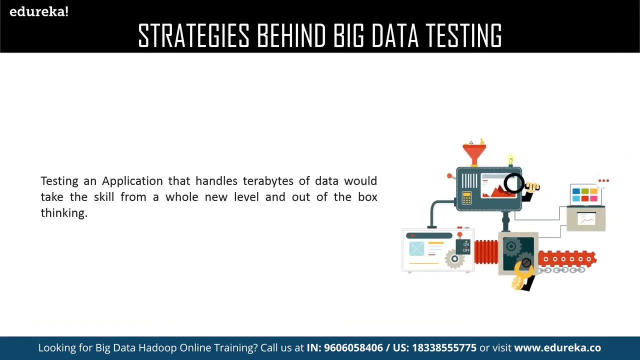 such a huge amount of data would take some special tools, techniques and terminologies, which will be discussed in the latest section of this tutorial. followed by this, We shall understand the strategies behind testing the big data. Testing an application that handles terabytes of data would take the skill from a whole new level. 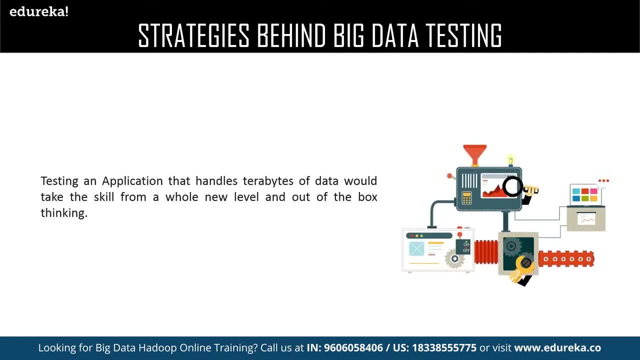 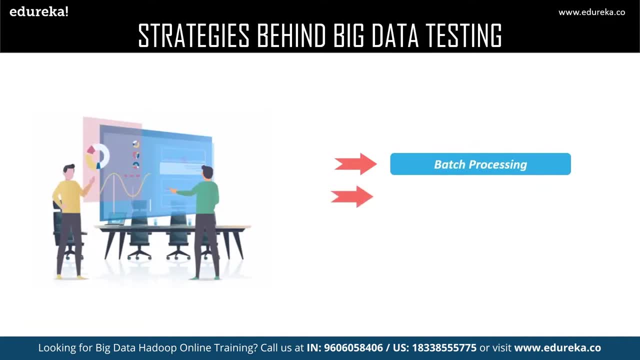 and out-of-the-box thinking. the core and the important test that a quality assurance team concentrates is based on three scenarios, namely batch data processing test, real-time data processing test And, lastly, the interactive data processing test. So what exactly is batch data processing test? 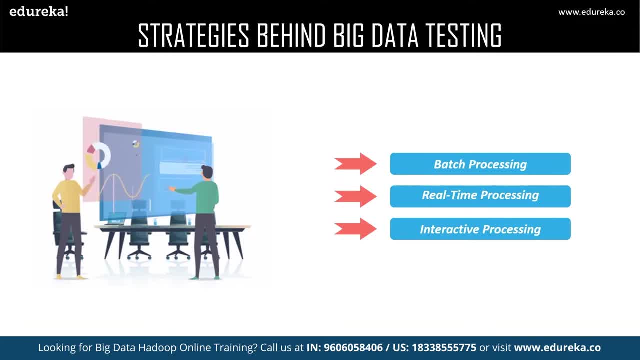 the batch data processing test involves test procedures that run the data when the applications are in batch processing mode. where the application is processed using batch processing storage units such as HDFS, The batch data processing test involves test procedures that run the data when the application is in batch processing mode. in this, 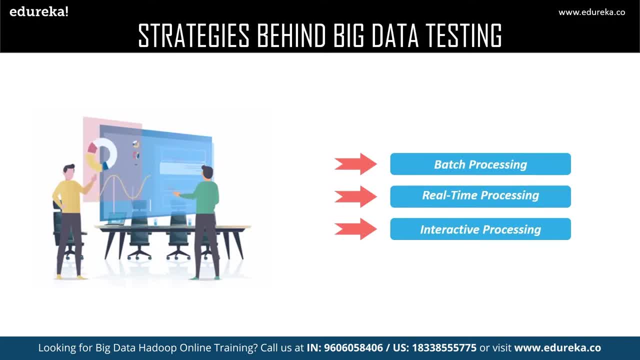 the application is processed using batch processing Storage units such as HDFS. the batch processing test mainly involves running the application against 40 inputs varying the volume of the data. now next comes as the real-time processing test. the real-time data processing test deals with the data. 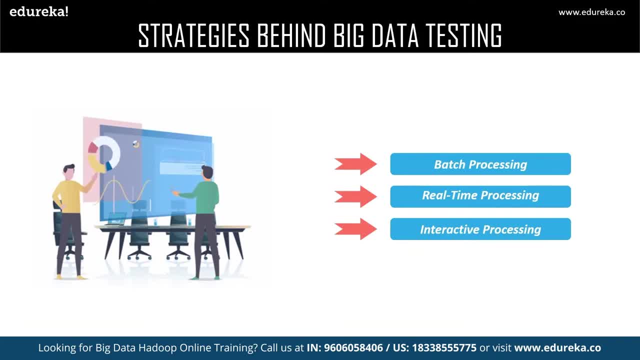 when the application is in real-time data processing mode. The application is run using the real-time processing tools, such as spark. real-time test involves application to be tested in the real-time environment and it is checked for stability. And the last one is interactive data processing test. 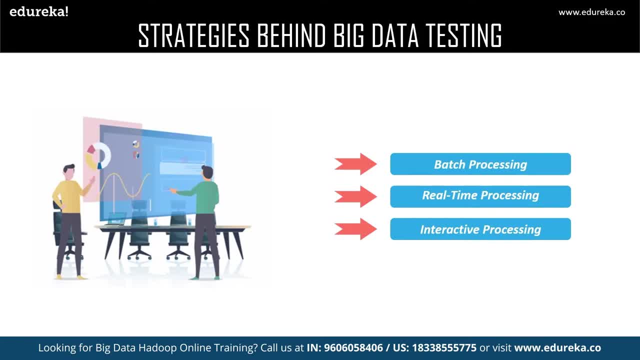 the interactive data processing test integrates the real-time test protocols that interact with application as in a view of the real-life user. the interactive data processing mode uses interactive processing tools such as hive sequel. now, moving ahead, We shall understand the different forms of big data. 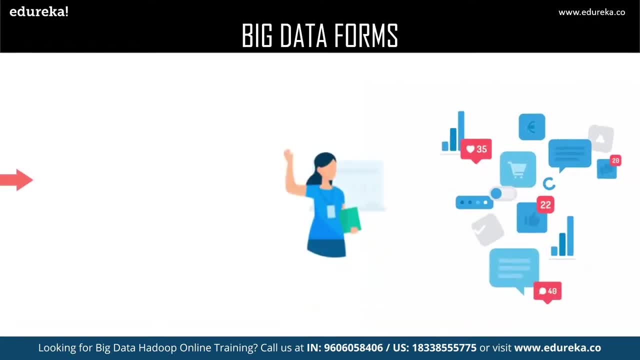 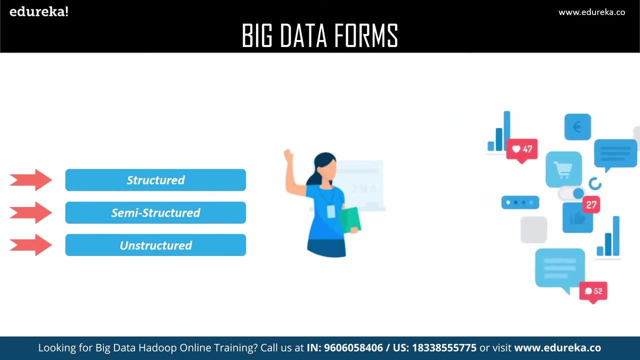 So there are three main forms of big data, which are structured format, semi structured format and unstructured format. Firstly, we shall understand What is the meaning of structured data. any tabular data which is meaningfully organized under rows and columns with easy accessibility is known as structured data. 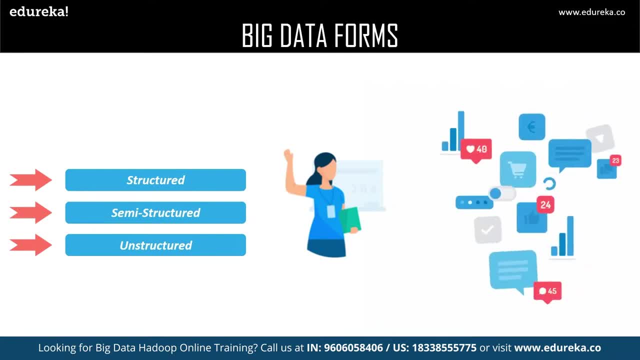 It can be organized under named columns using different storage units, such as an rdbms, for example, any tabular data stored in an rdbms. Now we shall understand what is semi structured data. semi structured data lies perfectly between structured and unstructured data. 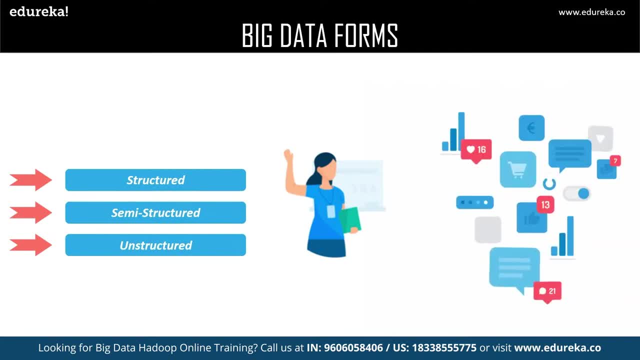 It cannot be directly ingested into an rdbms, as it includes metadata tags and sometimes duplicate values. data needs some operations to be applied on it before the data is ready to be ingested, For example, dot CSV format and dot Jason format. Now, lastly, we shall understand what exactly is unstructured data. 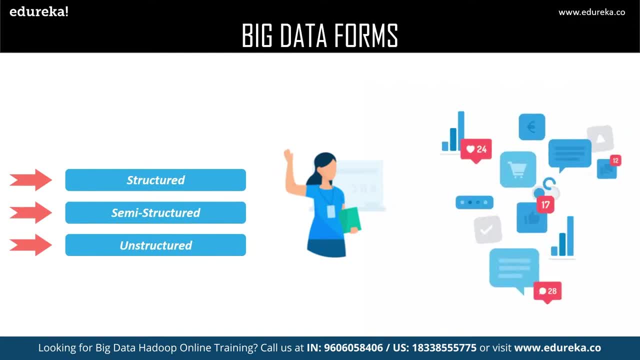 data that does not obey any kind of structure is known as unstructured data. unlike the structured data, The unstructured data is difficult to store and retrieve. most of the data generated by organizations is unstructured type of data, For example, image files, video files and audio files. 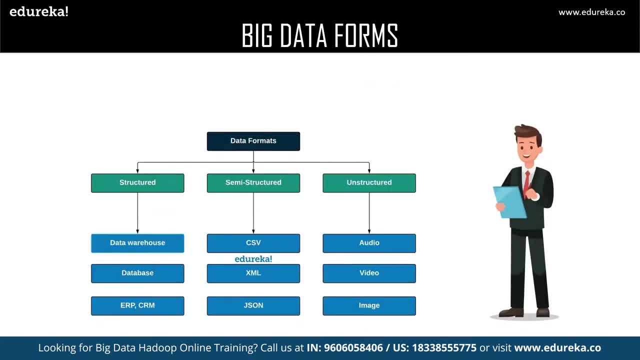 Now we shall understand the big data formats in a little detailed way, where we have the examples for structured, semi structured and unstructured. Firstly we shall deal with the structured data. So the structured data is available from the sources, like data warehouses, databases, ERP and CRM. 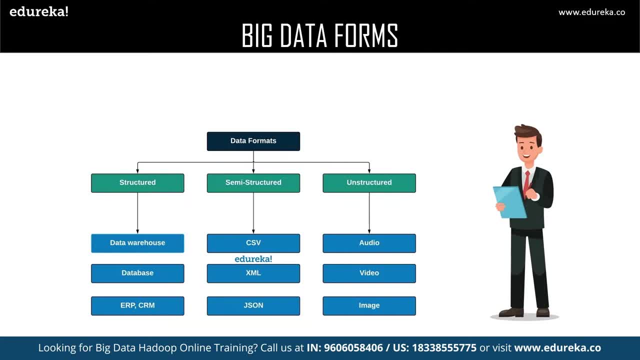 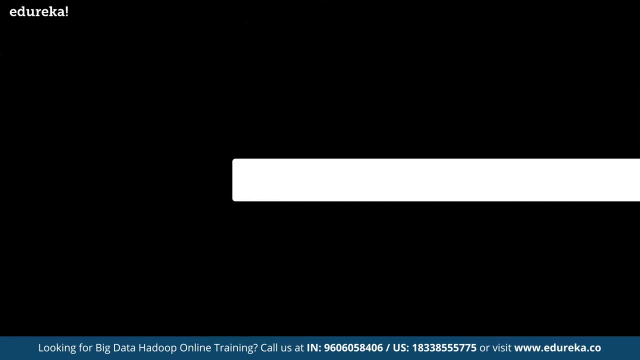 Now, when we enter into semi structured data, we find the sources from dot. CSV files, dot XML files, dot Jason files and finally we come into the unstructured data and the sources for the unstructured data, or audio files, video files and image files. Now we shall move ahead. 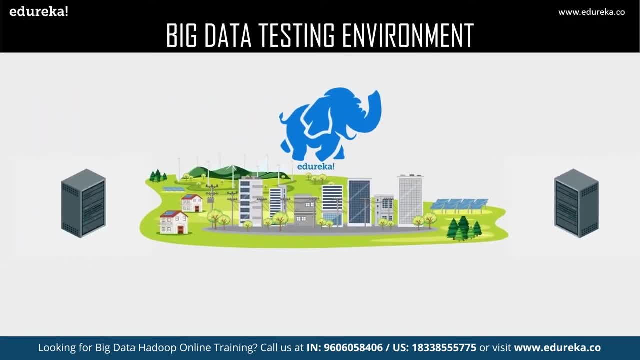 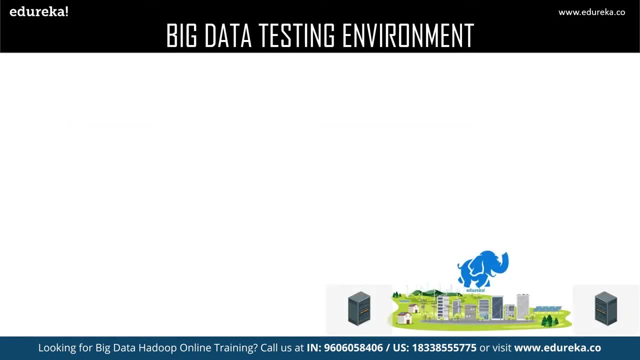 and understand the big data testing environment. owning a perfect environment for testing big data applications is very crucial. the basic requirements for big data testing are as follows. firstly, space for storing, processing and validating terabytes of data should be available. then the cluster and its respective nodes should be responsive. 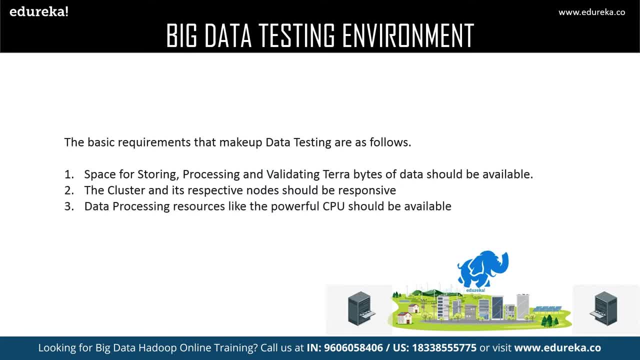 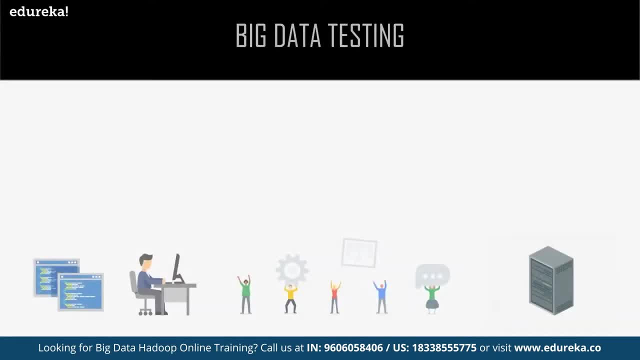 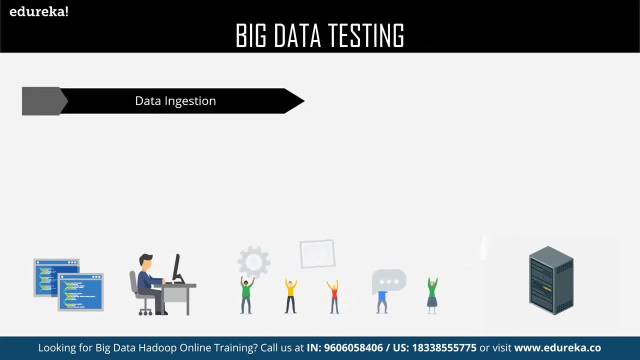 And lastly, the data processing resources, such as a powerful CPU, should be available. Now, with this, let us enter the big data testing. So the general approach in big data testing involves three stages. firstly, the data ingestion stage. in the data ingestion stage, The data is first loaded from the source to the big data. 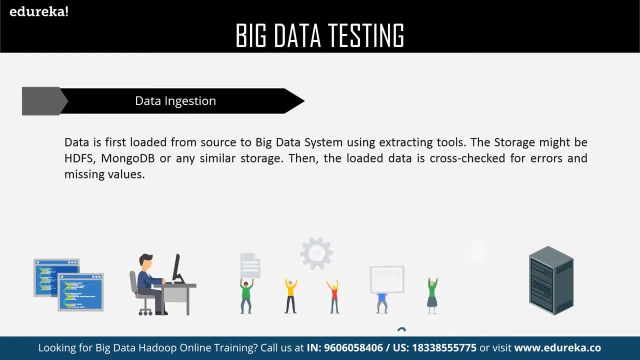 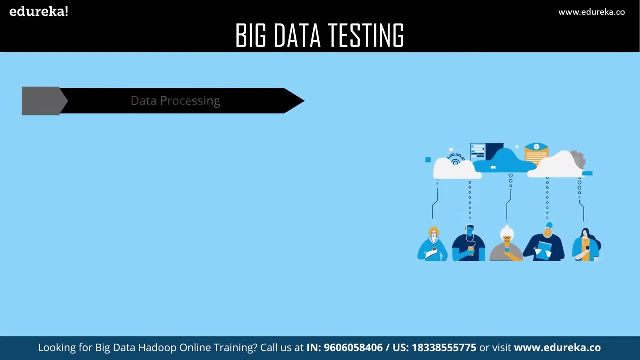 system using extracting tools. The storage might be HDFS, MongoDB or any other similar storage. then the loaded data is cross checked for errors and missing values. The basic example for data ingesting tools is talent, followed by the data ingestion phase. We have data processing phase. in this stage, the key value pairs 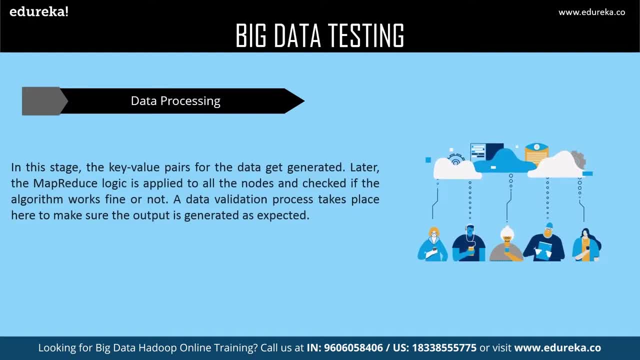 for the data get generated. later, The MapReduce logic is applied onto the nodes and checked if the algorithm works fine or not. a data validation process takes place, where we make sure that the output generated is as expected. And finally, the last stage is about the validation. 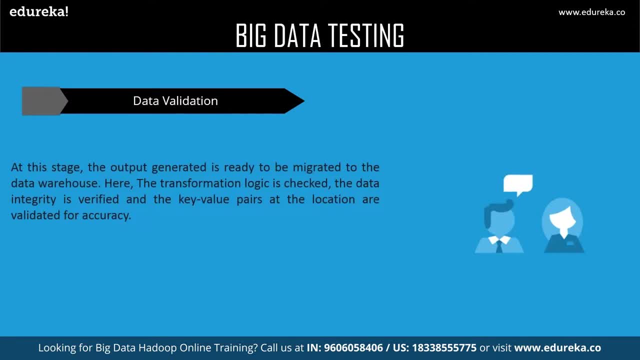 of the output. at this stage, The output generated is ready to be migrated from the data warehouse. here The transformation logic is checked, the data Integrity is verified and the key value pairs at the location where the data needs to be dumped is validated for accuracy. 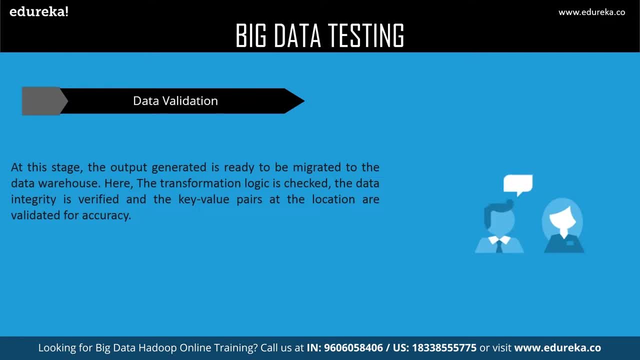 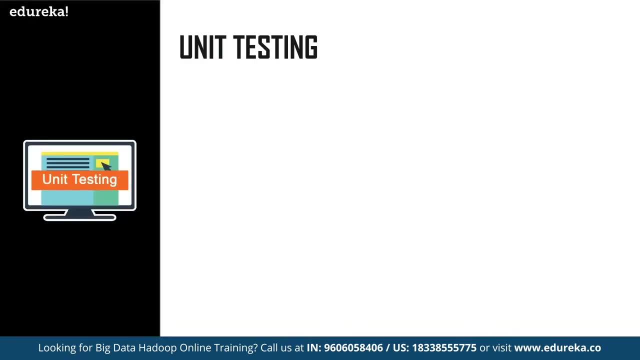 So these are the three phases in which the big data is tested. So with this letter into the next chapter, where we will deal with the different categories in which a big data application can be tested, Firstly, unit testing. unit testing in big data is completely similar. 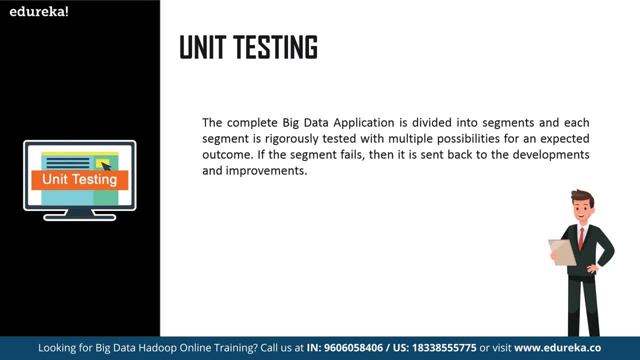 to any other unit testing in similar applications. The complete big data application is divided into segments and each segment is rigorously tested with multiple possibilities for an expected outcome. If any segment fails, then that particular segment is sent back to the development stage for improvements. now, after unit testing, we enter functional. 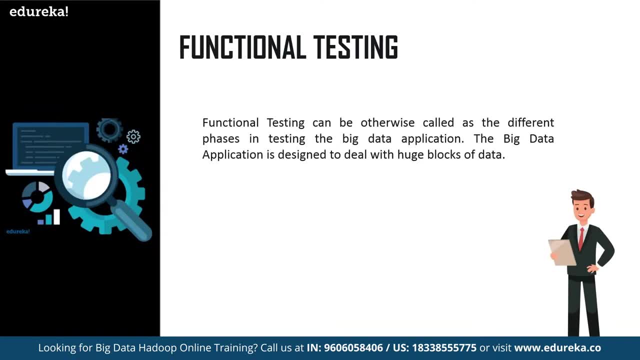 testing. functional testing can be otherwise called as different phases in testing. the big data application. The big data application is designated to deal with huge blocks of data. such a huge volume and variety of data is often prone to bring data issues such as bad data, duplicate values, metadata, missing values. 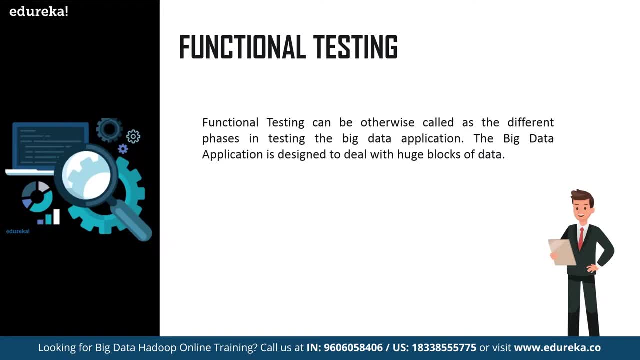 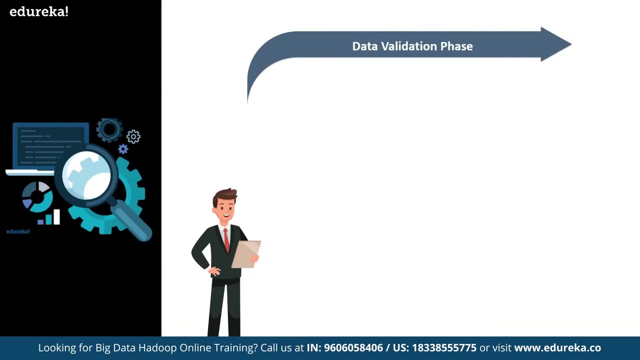 and what not. this is exactly why the pioneers in testing the big data design the procedure for functional testing of big data. the different phases in which the big data is tested are as follows: Firstly, the validation phase: data validation phase days with the business logic and the layers of big data application. 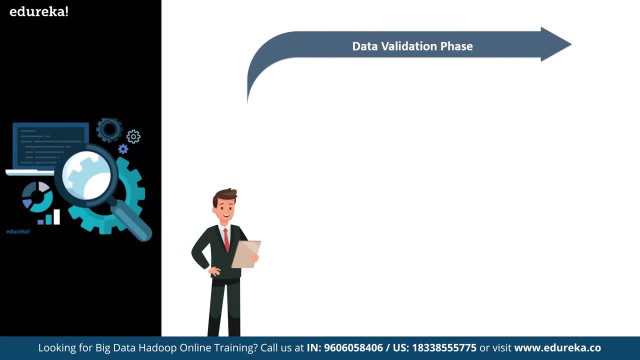 The data is collected from the source and it is run against the business use case. data collected is checked for accuracy and moment through the different layers of the application. at this stage, The big data is tested with aggregation and filtering mechanisms. the data undergoes End-to-end validation. 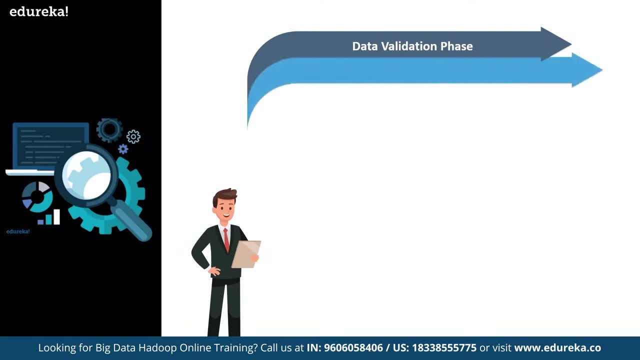 and transformation logic based on business rules. The next stage is data Integrity phase. data is checked for completeness with referential Integrity, validation, data constraints and duplication is verified against error conditions. boundary testing recognizes schema limits for each layer in Integrity phase. The next phase is data ingestion phase. 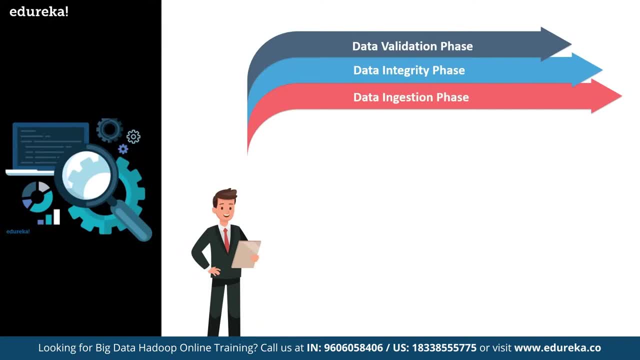 This is a very important phase where the data gets ingested into the Hadoop ecosystem. The ability of the application to connect with different data modules is checked here, The data is replayed with messaging systems and loss of data is monitored. the main motto of this phase is to achieve the following qualities: 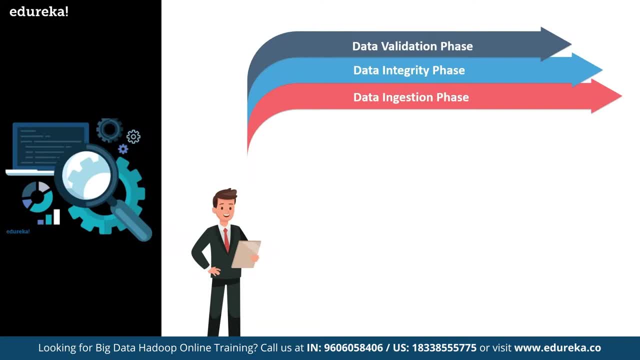 Firstly fault tolerance, then continuous data availability and lastly, stable connection with a variety of data streams, followed by data ingestion phase. We have data processing phase. the data processing phase carefully examines and executes the business logic. The business rules are cross validated, the MapReduce logic. 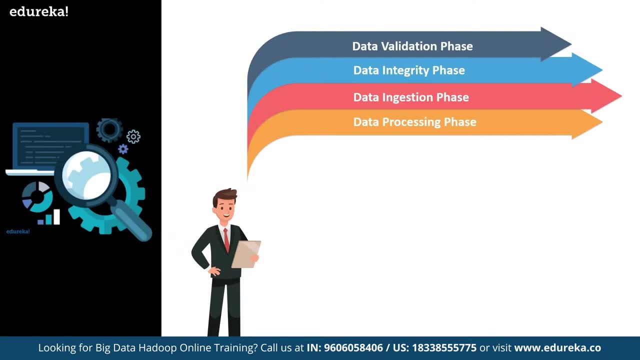 is validated at every stage, data is processed from end to end, The application is checked for exceptions and they get perfectly handled, followed by the data processing phase, We have the data storage phase. the data storage phase concentrates on the following parameters, which are the read and write timeouts, continuous data availability. 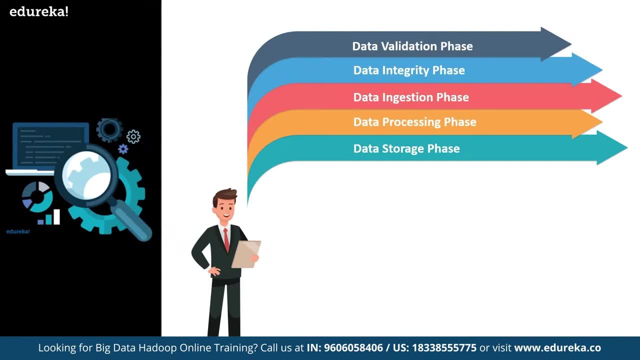 load balancing and, finally, the query performance analysis. after all these stages, We have one final stage, which is called the report generation phase. It is the final stage in functional testing and it deals with the following: data validation for measures and dimensions, real-time reporting, data drill. 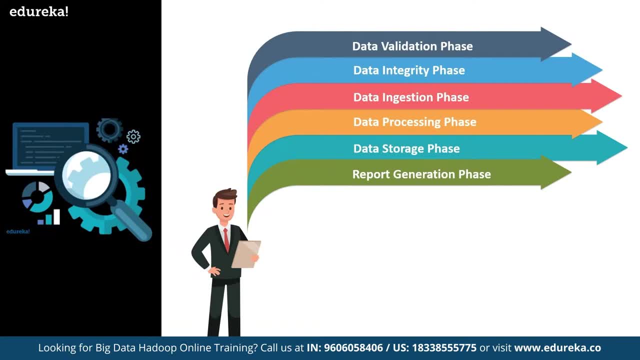 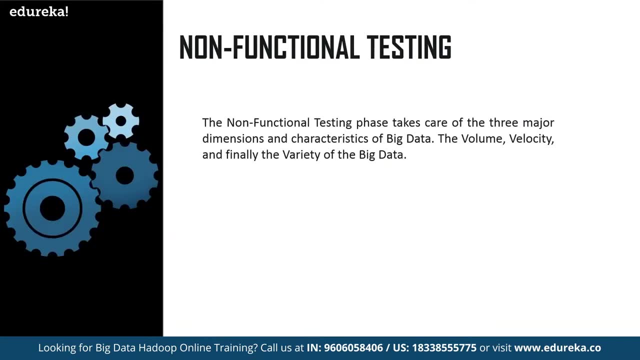 up and data drill down mechanisms And, lastly, the business reports and chats. So this was the functional testing. now let's move ahead and understand non-functional testing. the non-functional testing phase takes care about three major dimensions and characteristics of big data, Which are the volume, velocity and variety of big data. 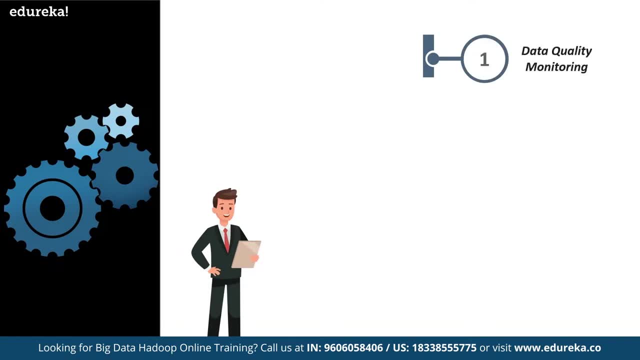 There are five stages involved in non-functional testing, which are data quality monitoring, infrastructure, data security, data performance and failover testing mechanism. Firstly, we shall understand data quality monitoring. data quality monitoring checks for erroneous data records and messages. data quality monitoring make sure that the following parameters about the data are available: 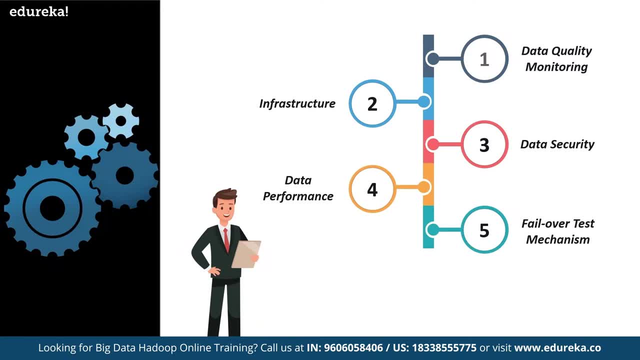 which are the data accuracy, data precision, data timeliness, data consistency, data profiling. now the next stage is the infrastructure. the infrastructure make sure that there is a continuous service availability in both external big data processing applications and internal big data processing applications. infrastructure also takes care about the data replication factor: data backup. 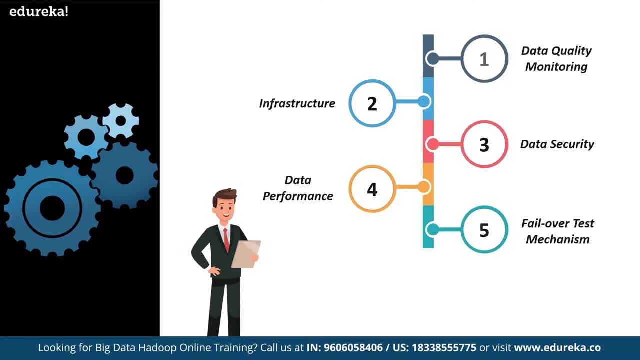 and data restore point, followed by the infrastructure. We have the data security. data security is called to be the most important aspect of the big data application data security stage protects the sensitive data. It manages user authentication and checks user role-based authorization. data security also takes care about the data. 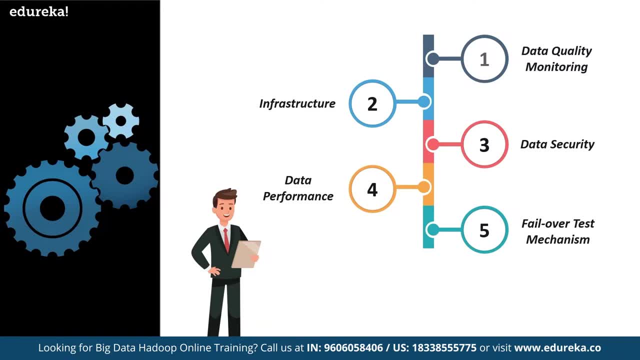 encryption and masking of personal information, followed by data security. We have data performance. data performance evaluates every single component. it evaluates maximum data processing speed. evaluates maximum data capacity size. checks the message transfer speed and response time. calculates the number of operations performed per unit time. engages pilot job monitoring. 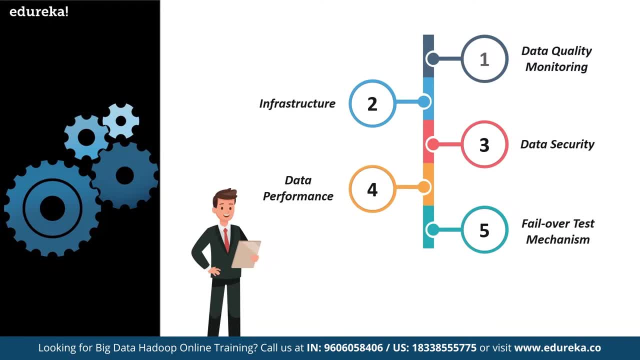 and finally, performs read, write and update operations on real-time databases. And lastly, we have failover test mechanism. failover test mechanism ensures seamless data processing while switching to neighboring data nodes. It creates data recovery points and parallely. it will be ready for any unexpected calamities. 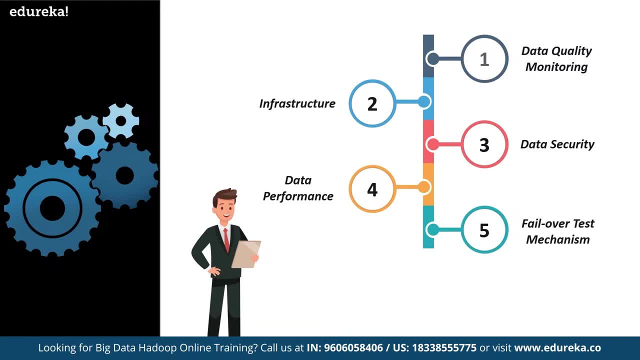 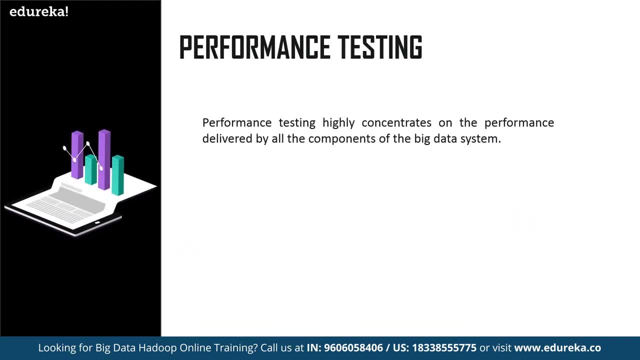 failover test mechanism will be ready to replay the data using multiple offsets. It enables dynamic clustering. with this, Let us move ahead into the next type of testing, which is based on the performance testing. performance testing highly concentrates on the performance delivered by all the components in the big data system. performance testing: 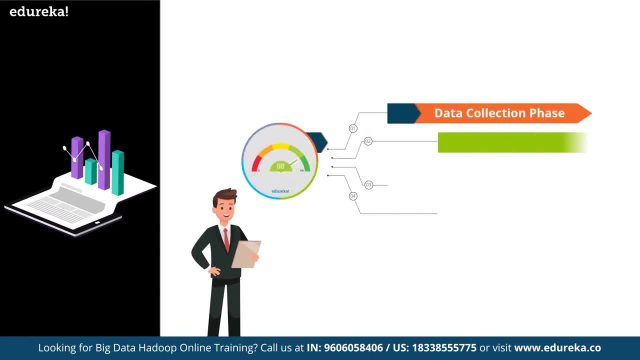 includes the following categories: Firstly, the data collection phase, data ingestion phase, data processing phase and, finally, component testing phase. Firstly, we shall understand what is data collecting phase. in this stage, The big data system is validated based on its speed and capacity to grasp the data within the given frame of time. 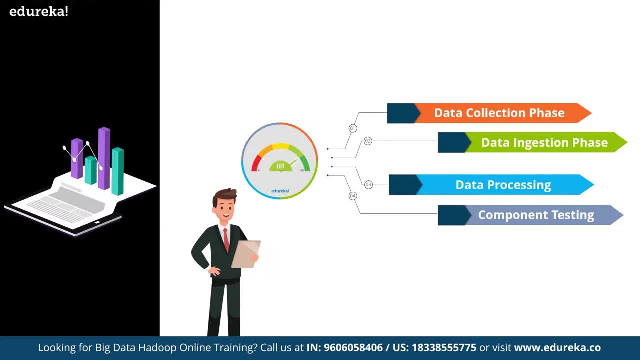 data can be collected from different sources, such as rdbms, databases, data warehouses and many more. the next stage deals with the data ingestion. here The application is tested and validated based on its space and capacity to load the collected data from the source to the destination, which might be HDFS, MongoDB, Cassandra. 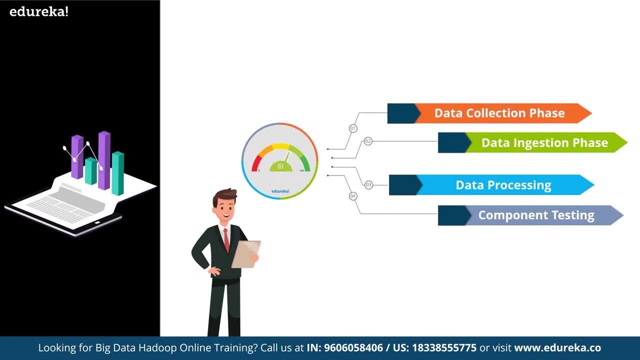 or many other similar storage units, Followed by the second stage. The third stage is data processing stage. here The application is tested based on the MapReduce logic written. the logic is run against every single node in the cluster and the processing speeds are validated. the queries: 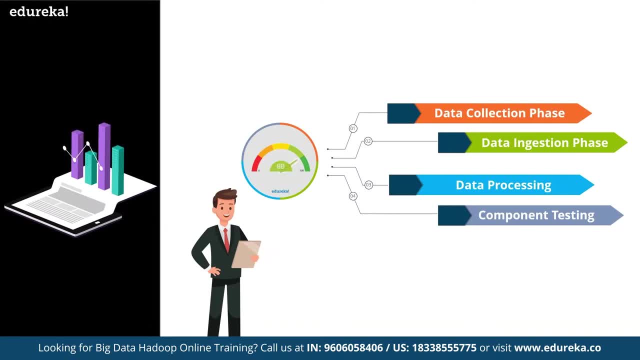 to be executed are expected to perform with high speeds and low data latency. And finally, we have the component testing. this stage is related to the component performance. each component in the system should be highly available and connected. the component backup should be online when any note fails. high-capacity data exchange should. 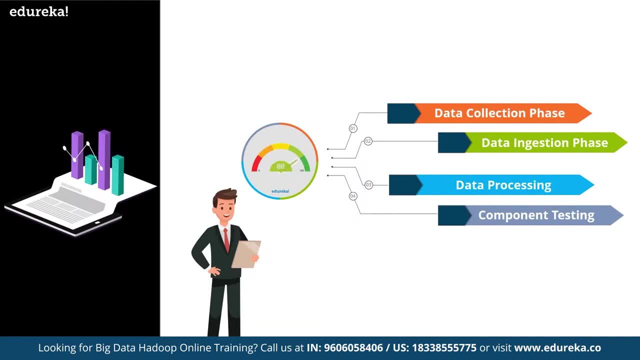 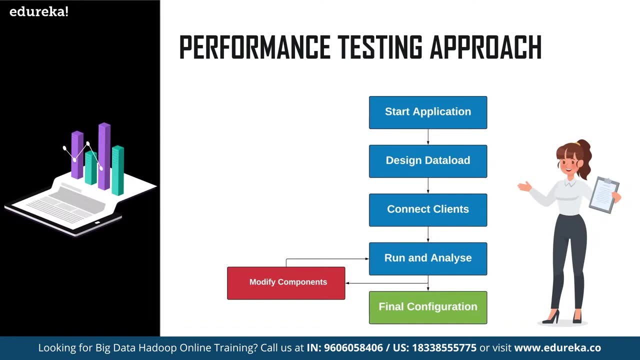 be smoothly supported. now, with this, let us move ahead and understand the performing testing approach. the performance testing approach can be understood through the following flow diagram. Firstly, the procedure begins by establishing a big data cluster and running the application. later, the big data developer designs the workload required to run the test. then 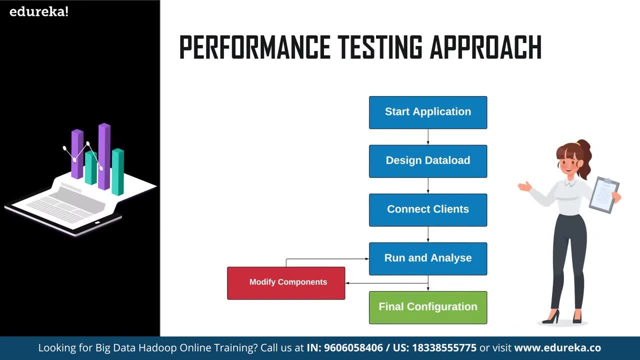 in the next stage, we involve the clients into the test and take their feedback. after that execute the application With data and analyze the results. and now, if we find the application to be performing with optimum stability, then the process is finished. else We applied the required modification. 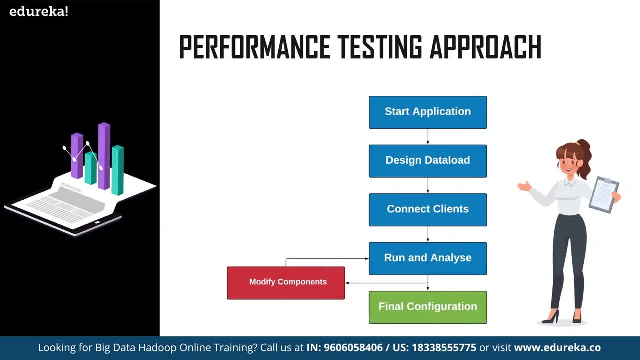 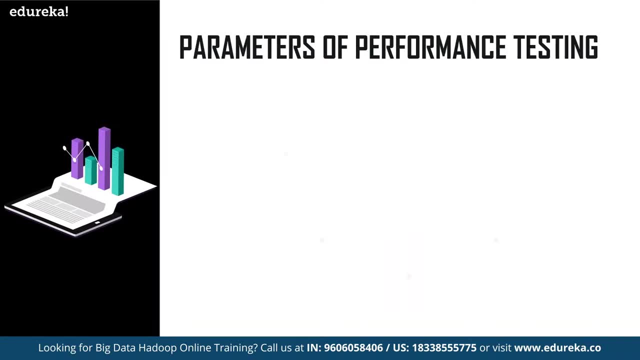 and retest the application. So this is the performance testing approach. now, followed by this, we shall understand the parameters involved in performance testing. So the parameters involved in performance testing are data storage. data storage takes note of the orientation in which the data gets stored in the system. 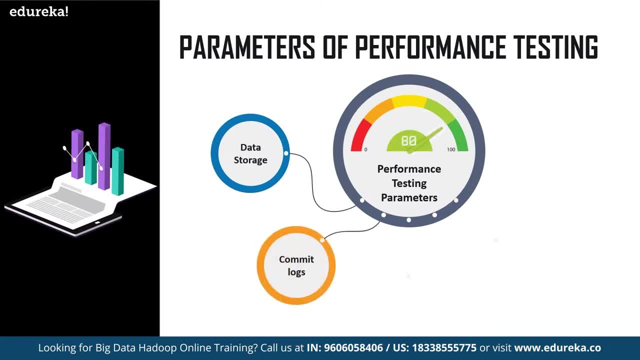 followed by that, We have commit logs, which marks the limits for committing logs. followed by that, We have the concurrency, which checks the number of threads allocated for the read and write process. and next to the concurrency, We have caching. caching includes dedicated row cache and key cache. and finally, we have timeouts- the timeout set. 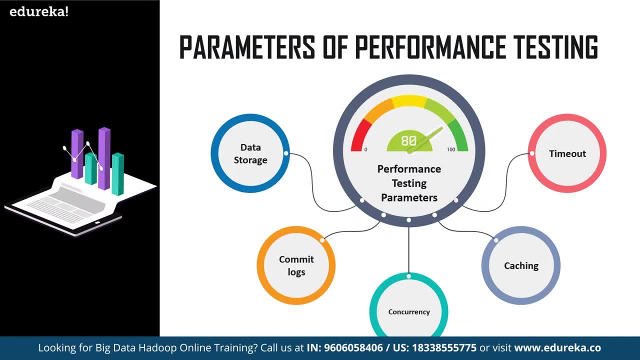 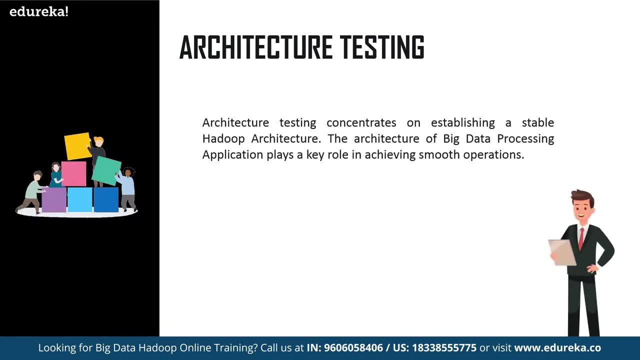 the timeout for the application, which are related to the connection and queries, Etc. followed by the performance testing. We have architecture testing. Architecture testing concentrates on establishing a stable Hadoop architecture. The Hadoop architecture of big data processing application plays a key role in achieving smooth operations. 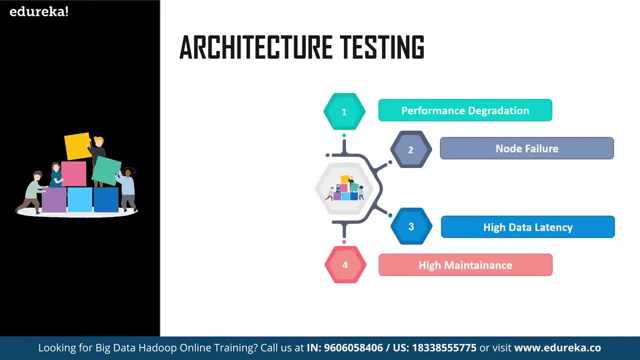 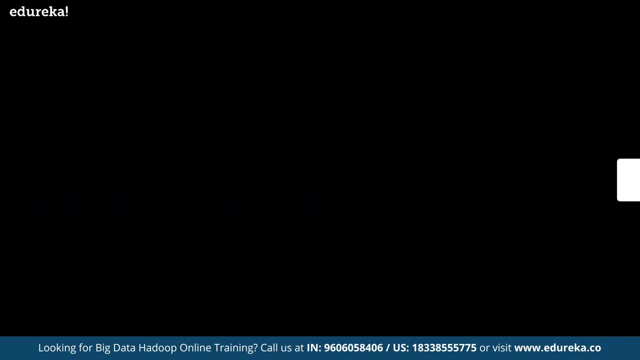 poorly designed architecture leads to chaos, which might be performance degradation- note failure, high data latency- and may require high maintenance. So these were the chaos which may show up if you have a poor architecture in your big data application. followed by this, we shall understand the big data testing. 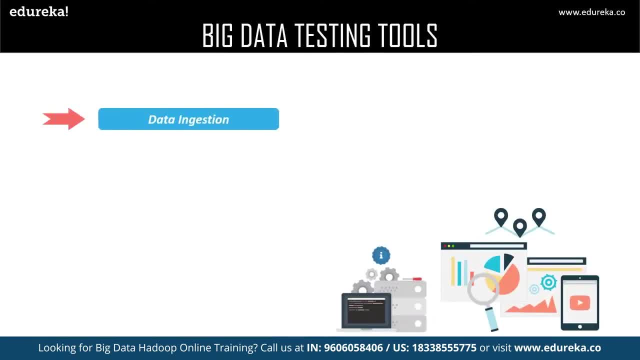 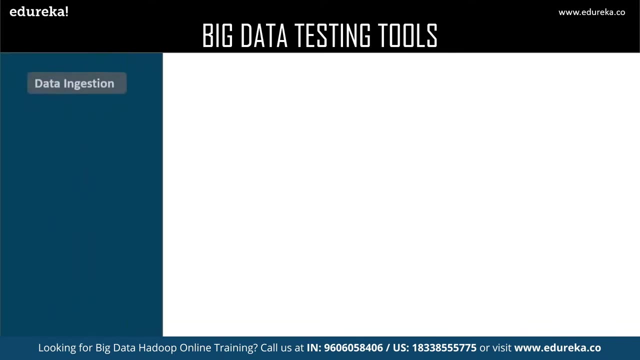 tools. So the big data testing tools are majorly classified into four categories: Firstly, big data ingestion tools, then big data processing tools, followed by that We have the big data storage tools and lastly, we have big data migration tools. Now we shall look at the examples based on each one. 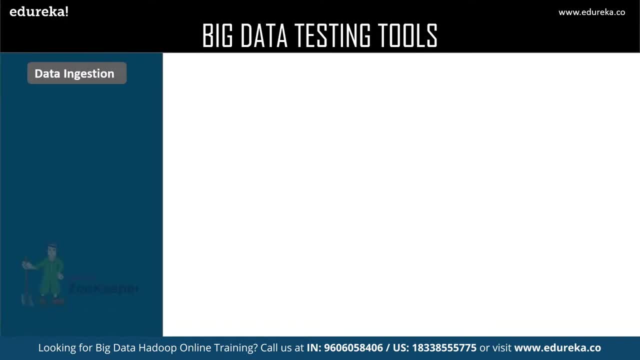 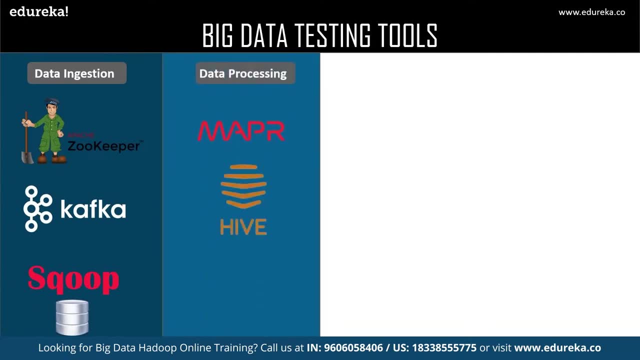 of them. firstly, the big data ingestion tools. zookeeper, Kafka and scoop are the best examples for data ingestion. next, We have data processing, and the popular tools used in big data processing Are map, are Hive and Apache pig. the next kind of tools are the data storage tools. the most famous examples 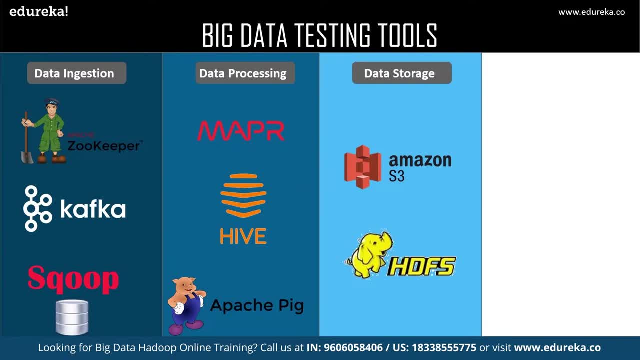 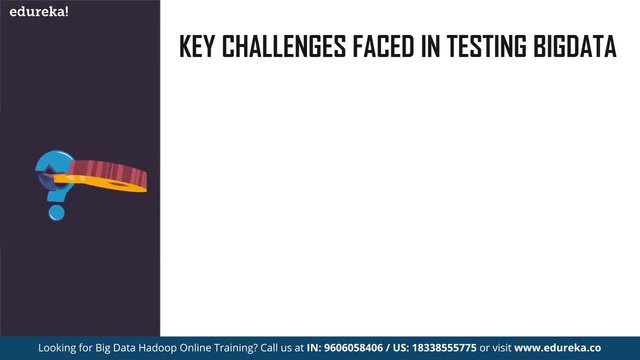 for data storage are Amazon s3 and HDFS. Finally, we have the data migration tools, and the popular examples for data migration are talent and clove DX. now, with this, we shall move ahead and understand the challenges faced in big data testing. So the key challenges faced in big data testing are: big data. 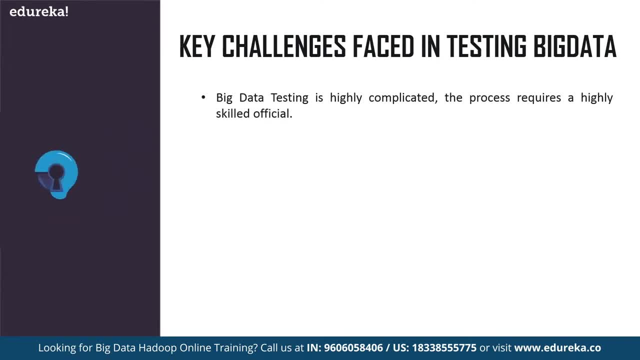 testing is highly complicated And the process requires highly skilled official automated big data testing procedures are predefined and they are not suited for unexpected errors. virtual machine latency creates latency in tests, and managing multimedia is a big hassle. followed by that, The volume of the data is one major challenge. 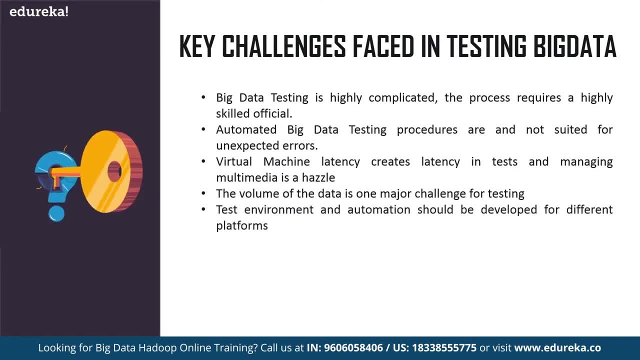 for big data testing. the testing environment and automation should be developed for different platforms. each component is from a different technology has it requires isolated testing. No single tool can perform end-to-end testing, followed by that high degree of scripting is required for designing test cases. 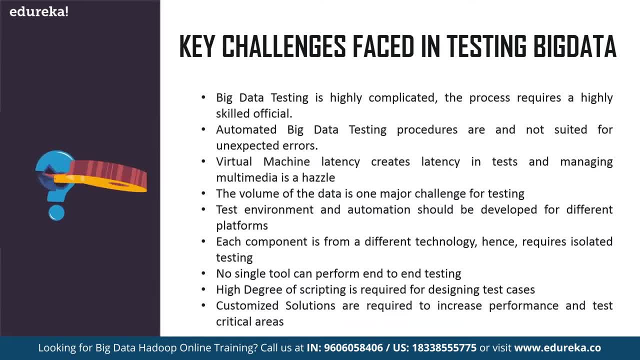 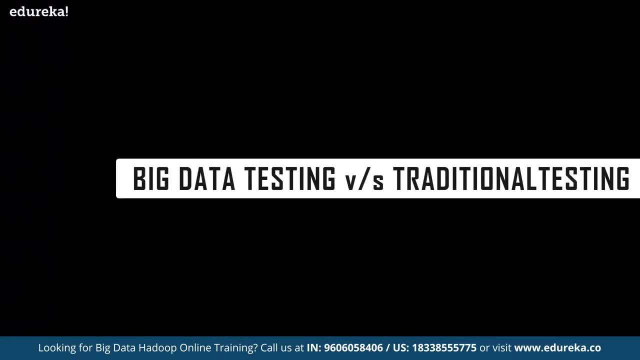 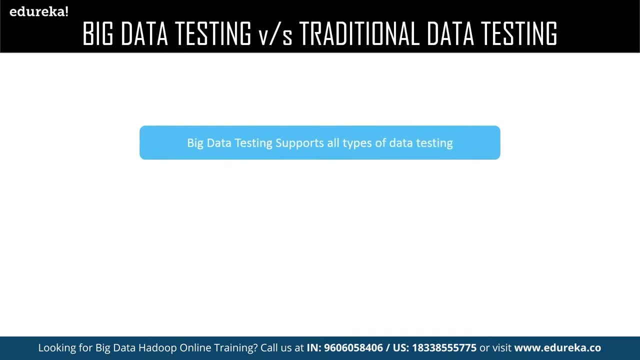 And finally, customized solutions are required to increase performance and test in critical areas. So with this we shall move ahead into the last topic, which deals with the difference between traditional testing and big data testing. So the first difference is the big data testing supports all type of data testing, whereas the traditional testing supports 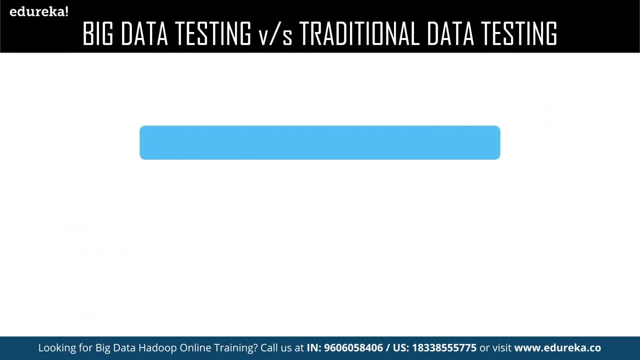 only structured testing. the next difference between the both is big data testing requires research and development, whereas in traditional data testing we don't require research and development. The third difference is the data size is unlimited in big data testing, whereas the data size is limited in traditional testing. followed by the third difference. 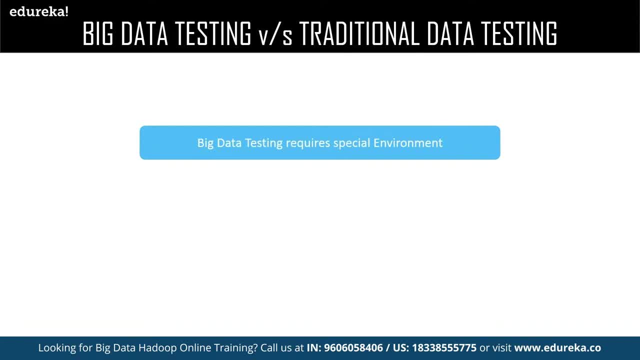 We shall enter the four difference, which says big data testing requires special environment, But whereas the traditional testing doesn't require any kind of special environment. So now we shall enter into the last difference, which says only highly skilled and qualified candidates can perform big data testing. 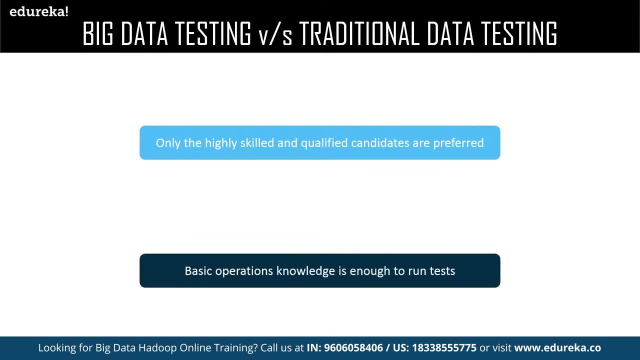 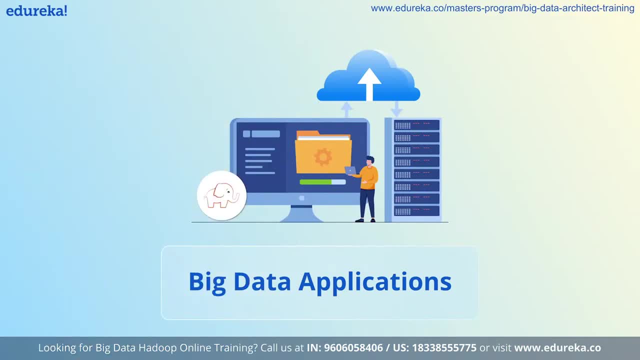 but when it comes to traditional testing, the basic operations, knowledge is enough to run the tests. Let's take a look at the various application domains that big data offers to the industries. as big data is growing at an exponential rate, various fields in day-to-day life are using big data. 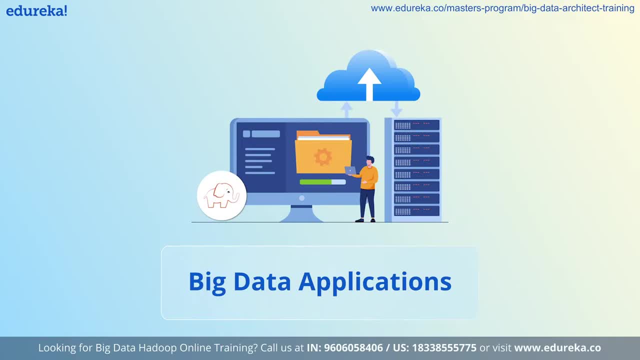 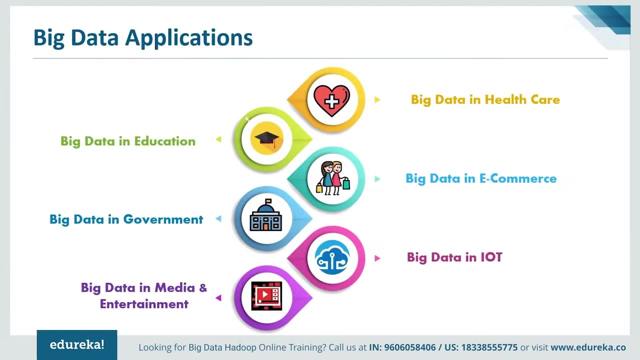 to ease the process of storing and processing the data. So here I have listed few of the sectors that have been implementing big data, like healthcare, education, e-commerce, government, IOT and even in media and entertainment. Now let's look at each of these domains in depth. first, 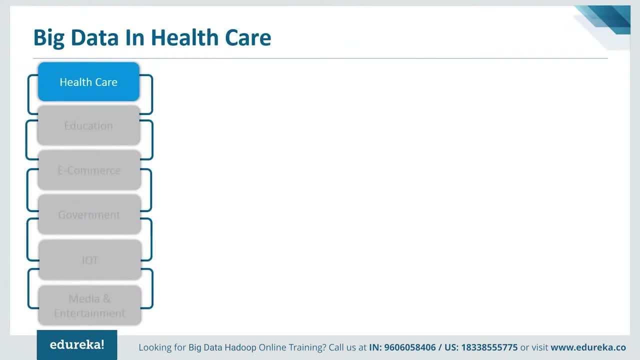 Let's see how big data is used in healthcare Industries. guys, You all know that there is a huge amount of data generated in healthcare Industries, and that data includes patient records, transactions, research data and many more. So, traditionally, what happened? they failed to use the big data. 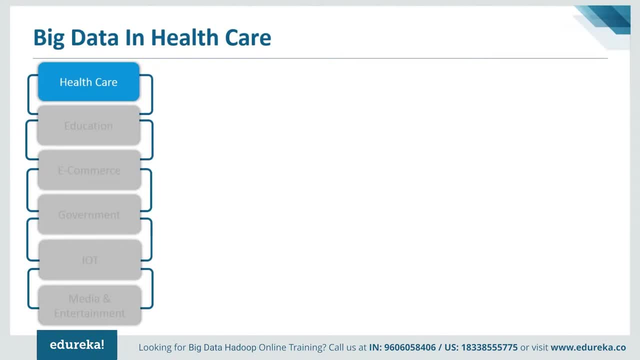 Why? because they had the limited ability to store and consolidate the data. Okay, I got a query from Piyush. He asks how big data analytics has improved healthcare Industries. Thank you, Piyush, for this question. I'll explain you how big data analytics have improved. 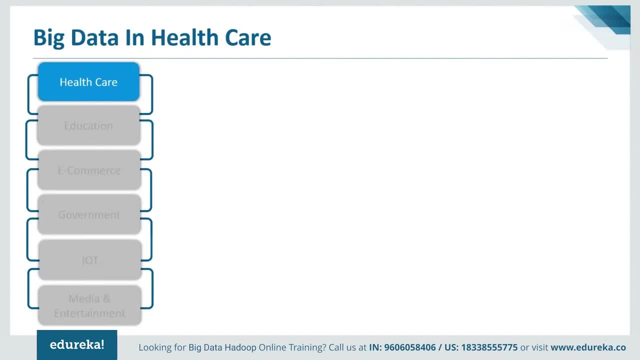 the health care by providing personalized medicine and prescriptive analytics. not only that, but also the researchers are mining the data to see what kind of treatments are more effective for particular conditions and, based on that, they identify the patterns that are related to drug side effects and then provide the solution. 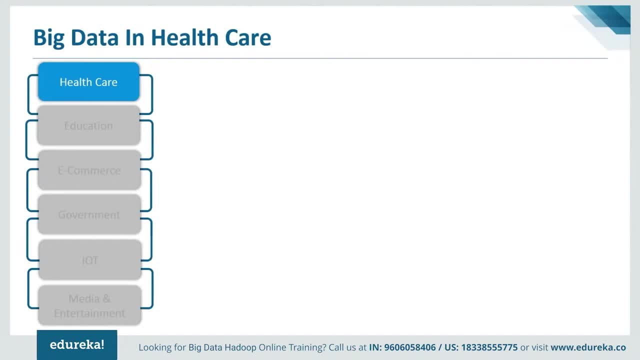 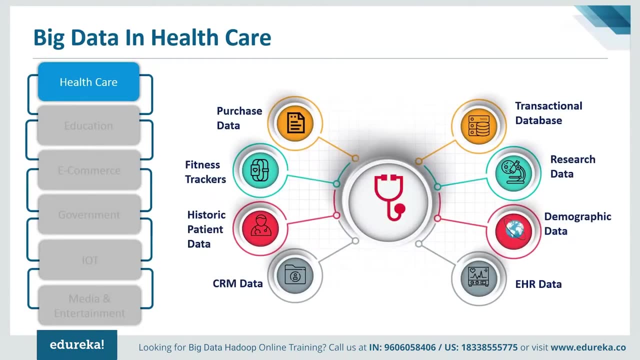 that can help the patients and reduce the cost, and also on adoption of m health, e health And variable Technologies. the volume of data is increasing and that includes electronic health records, data, CRM data, that is, customer relationship management data, fitness trackers, historic patient research data, purchase data and many more. 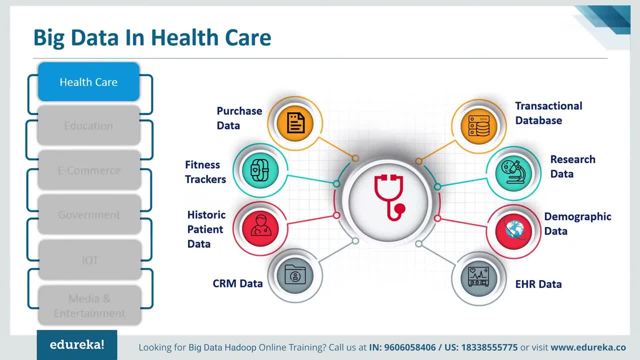 So now let me tell you why demographic data plays a vital role in healthcare Industries. here What we do is we map the health care data sets with the geographical data sets, and by doing that it's possible to predict The disease that will escalate in specific areas. 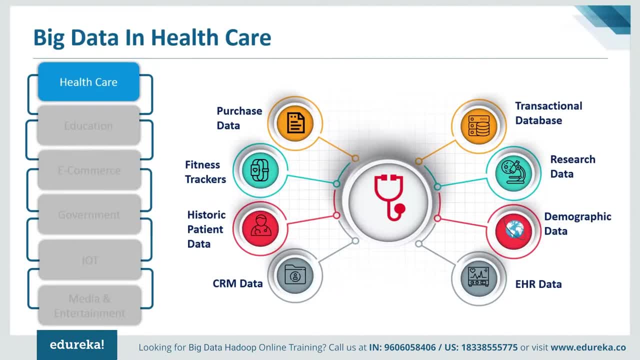 and based on these kind of predictions, It is very easy to strategize the Diagnostics and then plan for stocking serums and vaccines. So this is how big data analytics has enhanced the healthcare Industries. Now let's see how big data is used. 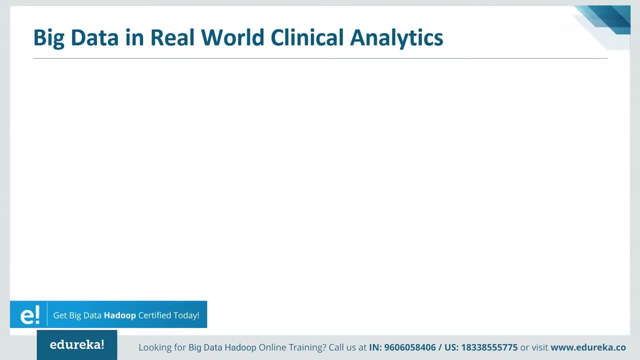 in real-world clinical analytics. healthcare Industries wanted to replace their legacy data warehousing solution with the data Lake that could manage high volumes of data. in order for this, healthcare Industries selected a company called CTS tech, which is a specialist provider for health care, to build the solution. 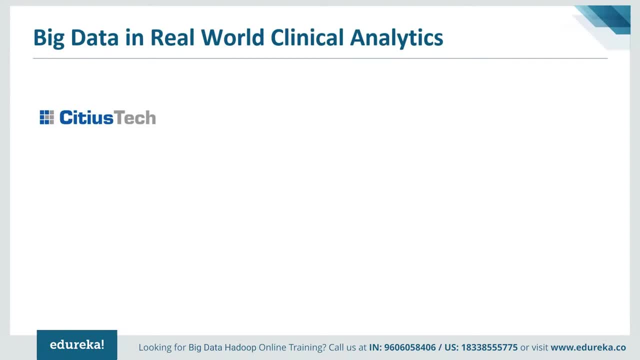 So CTS tech designed the solution based on cloud era Hadoop distribution map reduce, Spark, streaming and other Hadoop Technologies. So here is how it works. here We have diagnostic results and billing messages. This is nothing but the data source, from where we get the data. 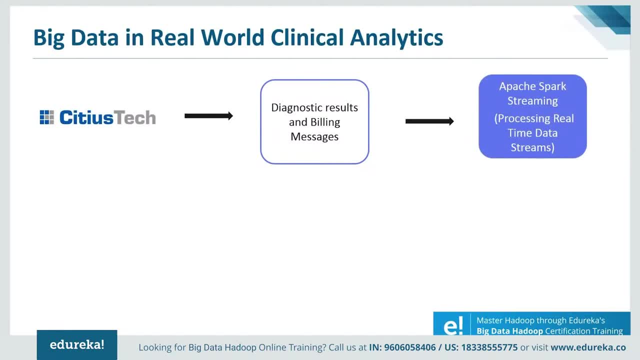 and this data is injected into the data ingestion stream Fair in it undergoes Spark streaming and produce real-time beta streams, and these real-time beta streams are capable of processing 20,000 records per second and they are then landed on to the cloud or a landing zone. 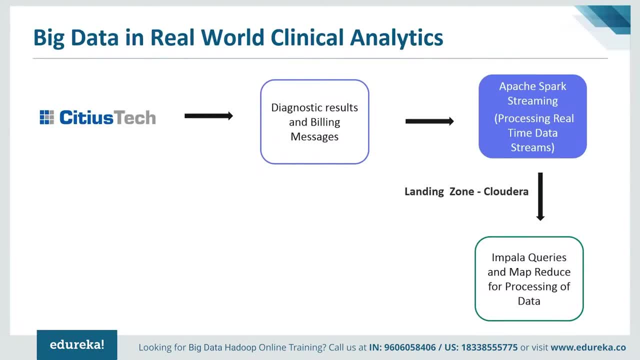 wherein it undergoes deduplicating, cleansing and standardization of the data, and once deduplicating, cleansing and standardization of the data is done, It is then processed using MapReduce job and data processing stream, and this process data is queried using Cloudera Impala. 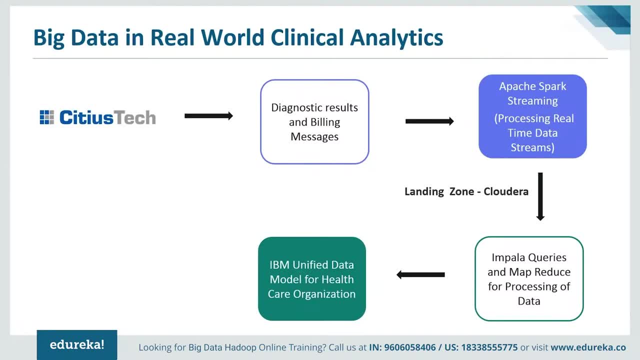 Now we populate and store the messages from Cloudera Impala into IBM Unified data model for healthcare organization and from there we visualize the results and dashboard and then we arrive at the solution. So this is how CTS tech has used big data analytics and provided the solution in real-world clinical analytics. 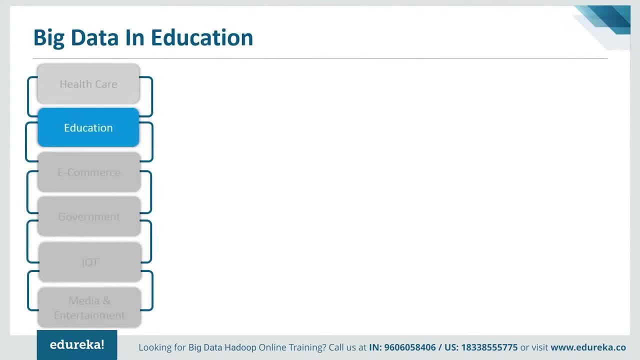 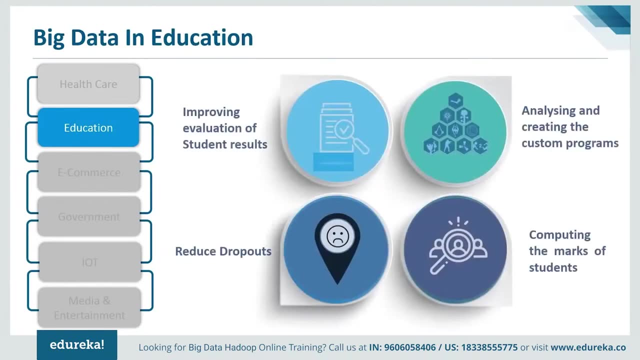 Now let's see how big data is used in education sector. Big data is revolutionizing the way we manage education sector. so how is it doing that? Here have jotted down few of them. First, let me tell you how it is used. 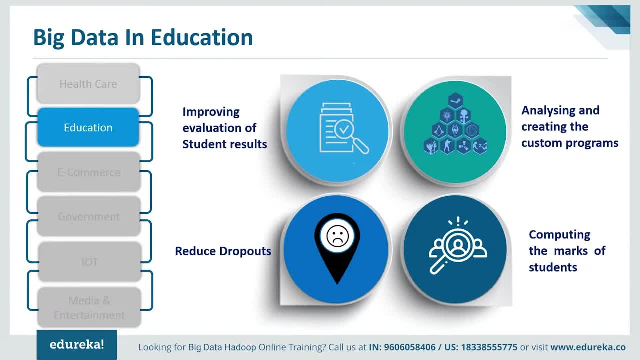 in improving evaluation of student results. Guys, can you guess what is the only way to assess the performance of a student? The only measurement of the performance of a student is the answers that they write to assignments and exams, correct? So, however, during his or her life, each student generates a unique data trail. 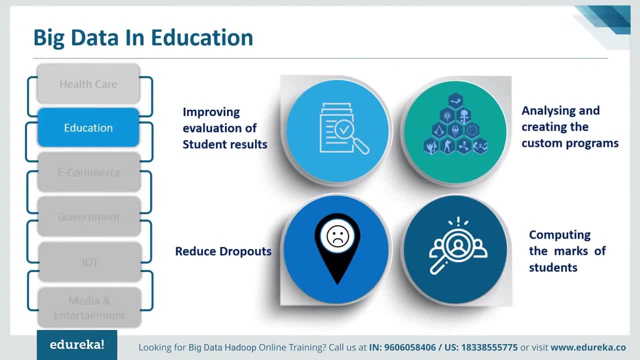 and analyzing this data trail in real time, one can understand the individual behavior of students and that helps to create an optimal learning environment for the students. And also it is possible to monitor student actions, such as how long they take to answer a question, which sources they use for exam preparation. 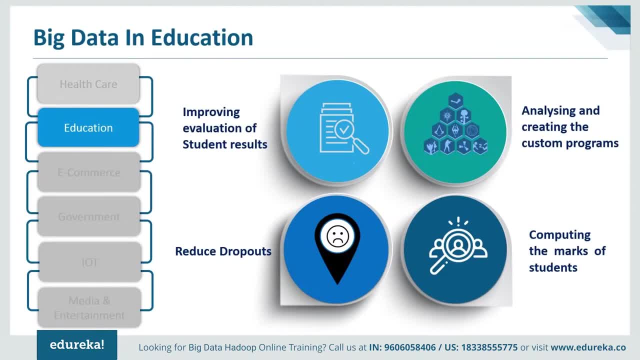 which questions do they skip? and many more. So by considering all these factors, one can improve the evaluation of student results. Next, learning and creating the custom programs. You all know that we have lakhs of students from each and every universities, but customized programs for each and every individual student can be created. 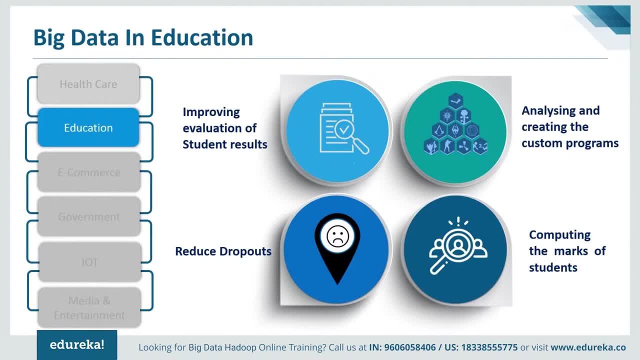 Everyone wondering how That is possible with the help of a technique that is called as blended learning, Confused. What is this blended learning? It is very simple. It is just a combination of online and offline learning, and that gives the students the opportunity. 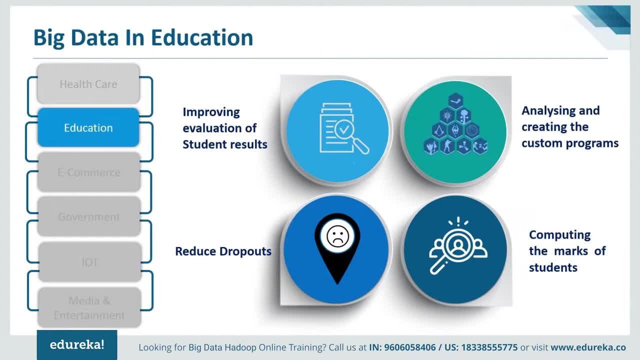 to follow the classes that they are interested in, and also they have the possibility for offline guidance by professors. Next, how big data helps us to reduce the dropout rates. as we have already discussed that, it would help to improve the evaluation of student results. It's a obvious fact that the dropout rates at schools and colleges would also reduce. 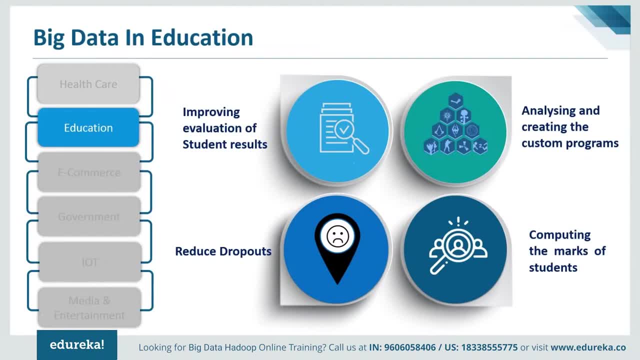 So what does educational institutions do? They use predictive analytics on all the data that is collected to give them Insights on future student outcomes, and such kind of predictions will also help to run a scenario analysis on a course or a program before it is introduced into the curriculum. 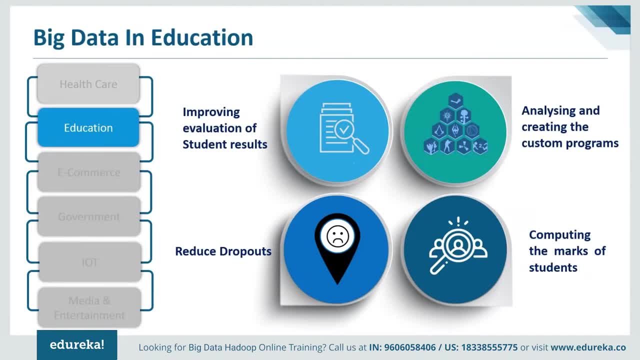 and this minimizes the need for trial and error. Next, now let's see how to compute the marks of students. Let me take an example here, Say, let me take attendees names itself. Consider Priyad scores 90 marks in mathematics and 60 in geography. 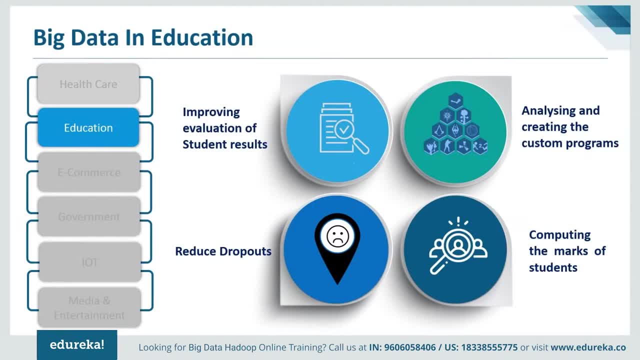 but Chaitra scores More in geography and less in mathematics. So what does big data analytics do? It helps to combine and analyze all the data of students and, based on that, importance can be given to each of the students who lag this course, and also to give an insight about how to improve the performance. 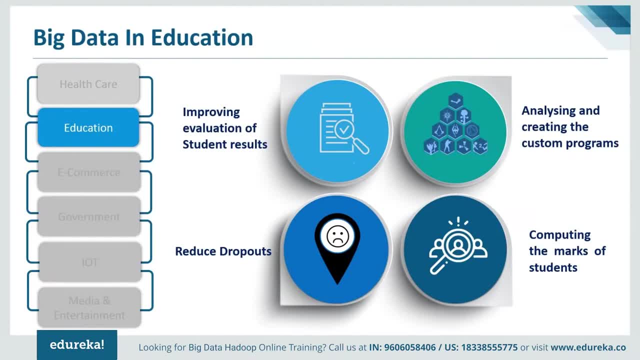 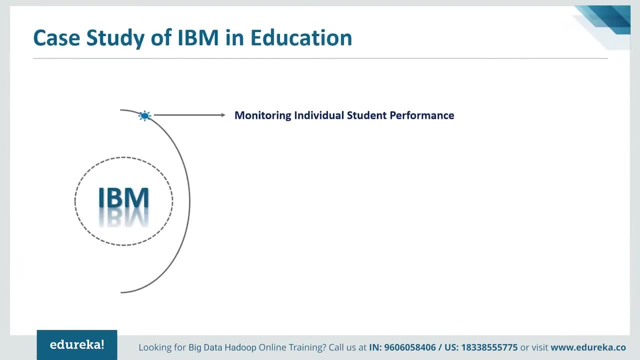 So these are the various ways where we use big data analytics in education sector. Now let's see a case study of IBM in education. It is used to monitor individual student performance. to prevent attrition from a course or a program. next, to identify outlines for early intervention. to identify: 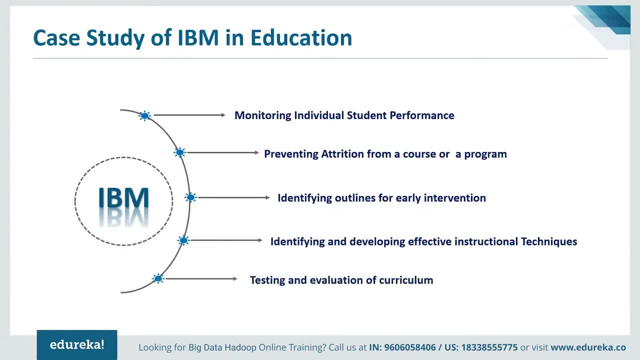 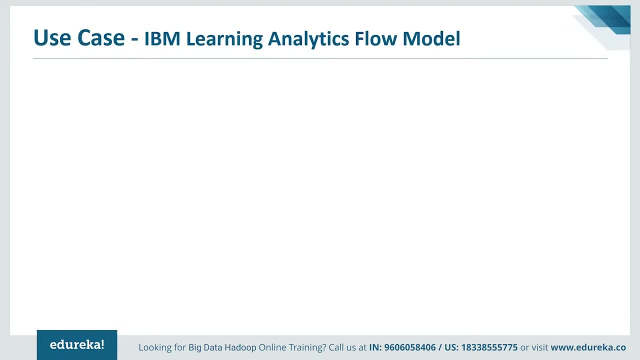 and develop effective instructional techniques for testing and evaluation of curriculum. Now let's see how IBM has used big data analytics in learning analytics floor model. here We capture instructional transactions as they occur, and these instructional transactions- Actions, occur, in a time-sensitive learning application. 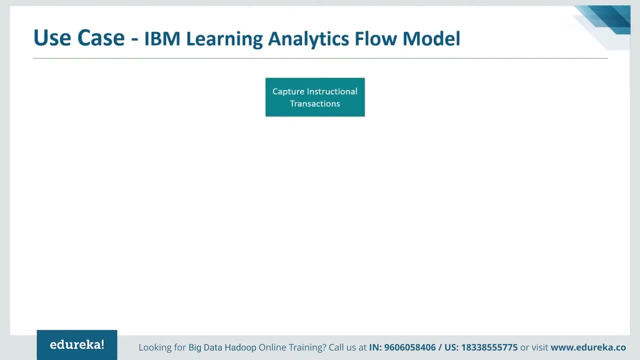 and this would be actually possible within a learning management or a course management system, and we use full capabilities of a learning management system and then generate a 15-week online course, and this 15-week online course would generate thousands of transactions per second, and then we perform real-time analysis on these transactions. 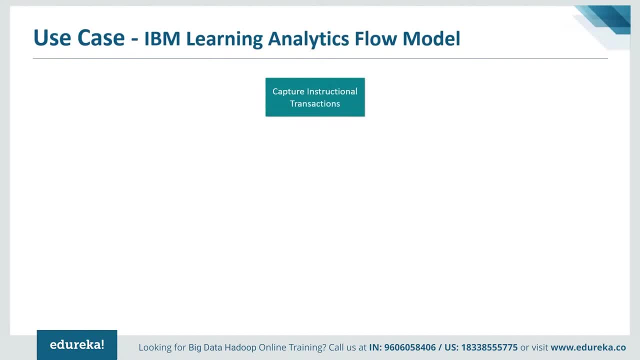 and that would be used to feed a learning analytics app. and to process all these data, We need a big database system. without the help of analytics software, It is not possible to process the data and big database system, So we use Apache spark for data processing. 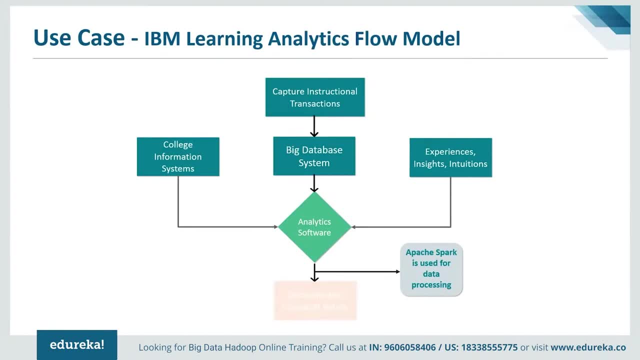 and then we analyze the transactions and establish a pattern, and then we arrive at decisions and course of action, and these decisions and course of action is then introduced into a curriculum or a course management system. So this is how IBM has made use of big data analytics. 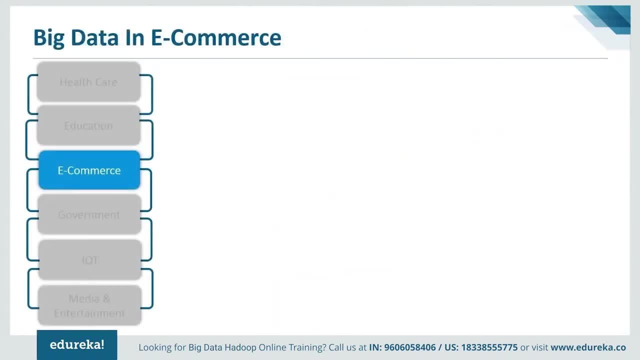 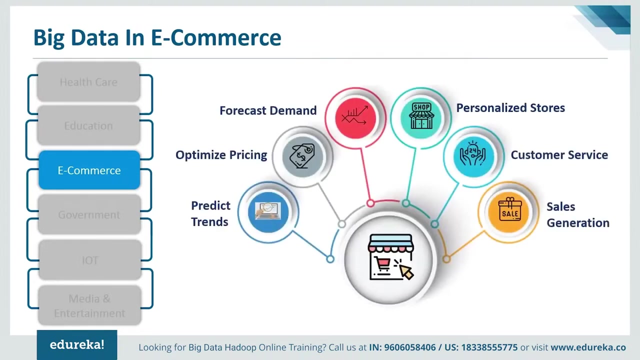 and learning analytics- Low model. Now let's see how big data is used in e-commerce Industries. Big data is a game changer when it comes to retail and e-commerce. retailers and e-commerce Brands are using more of analytics to drive strategic action and offer better customer experience. 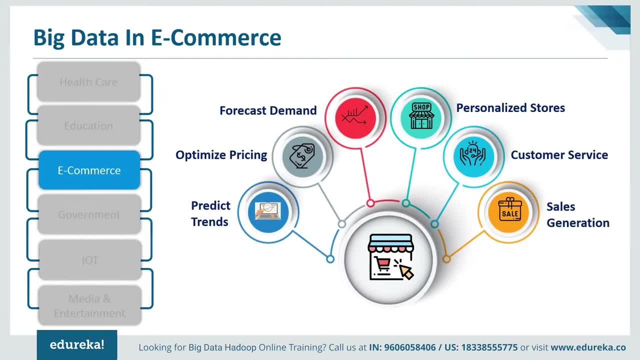 So these are few of the usages. first, it is used to predict the trends. in order to predict the trends, We use a trend forecasting algorithm, and this trend forecasting algorithm combines the data from social media, post and web browsing habits to identify what is causing a bus. 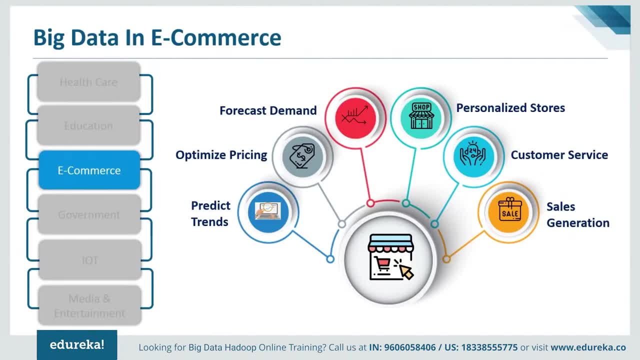 and also to know which product is discussed more of online. We perform sentiment analysis task and, based on sentiment analysis and trend forecasting algorithm, It is very easy to predict the trends in the market. next, optimized pricing: big data enables retailers to identify best price for goods. 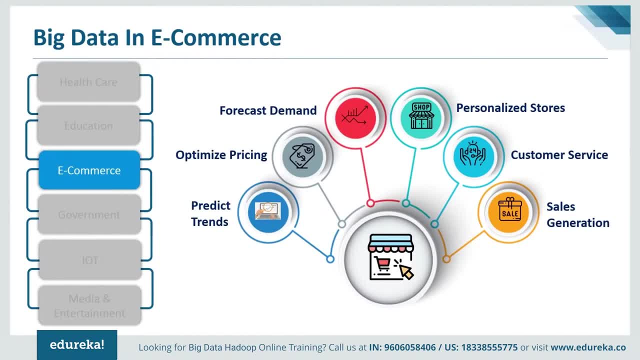 by tracking transactions, competitor and cost of goods. and not only that, but retailers can also map the rise and fall of demand and match the pricing accordingly. Now let's see how analytics has enhanced Amazon to forecast its demand. analytics enables Amazon to predict the traffic on the website. 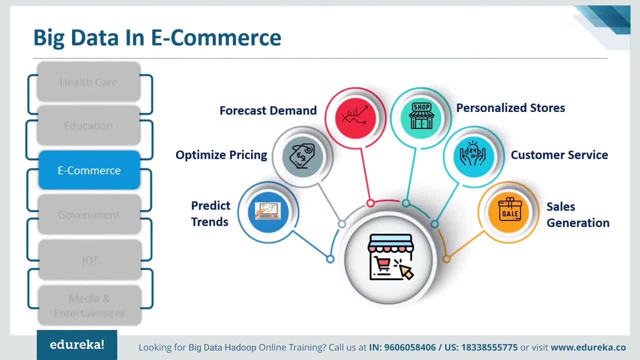 along with the possible conversion rate, and through the Amazon Web Services cloud, the business has the flexibility to scale up in a real time. So, as it can scale up in a real time, analytics enables Amazon to forecast It's demand. next, how one can create a personalized store. 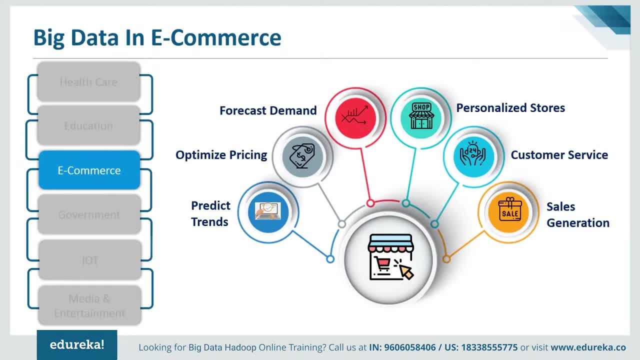 We have something called as fast web server Technologies, and this fast web server Technologies, in combination with big data, businesses can generate dynamic websites that are filled with relevant products based on the historic behavior of a consumer and their personal preferences. So by grouping the personal preferences and the historic behavior of a consumer, one can create a personalized stores. 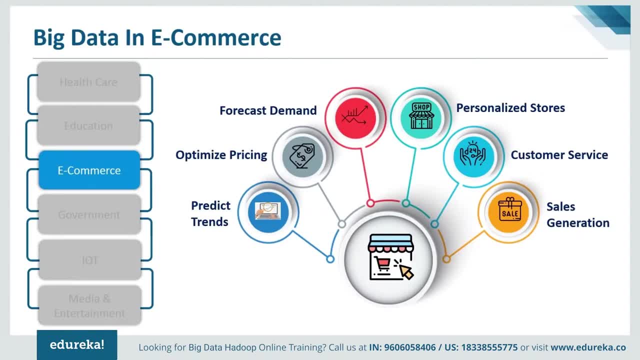 next customer service. customer service is available 24: 7 in all the e-commerce Industries. So big data analytics allows business to optimize this customer service. And how does it do? it compiles the data from previous online and offline transactions, social media information, purchase history. 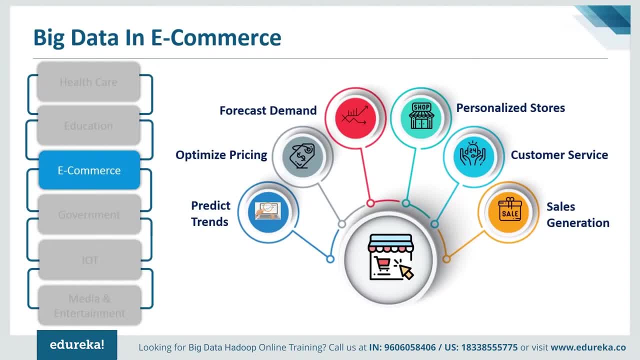 and many more, and by this, businesses can create a 360-degree view of the customer and, based on that, they provide enhanced customer experience. next sales generation. the main motto of all the e-commerce Industries Is to sell their goods and products, and retailers use big data to offer a personalized experience. 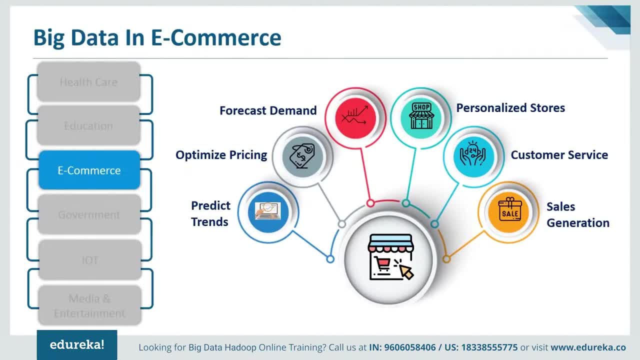 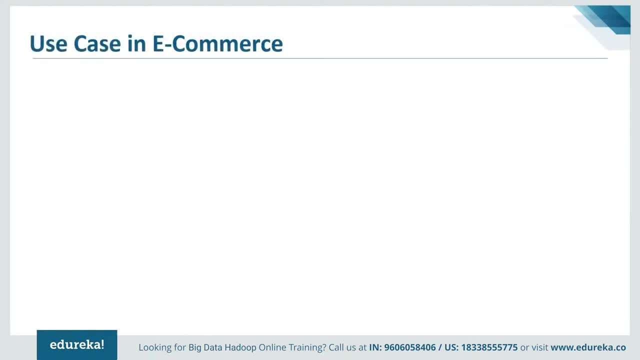 and prevent potential abandonment. So by this we can have more number of sales generated. So these are a few of the usages in e-commerce Industries. Let's see a real-time use case in e-commerce. here We have a user. user communicates with the e-commerce server portal in data stream. here 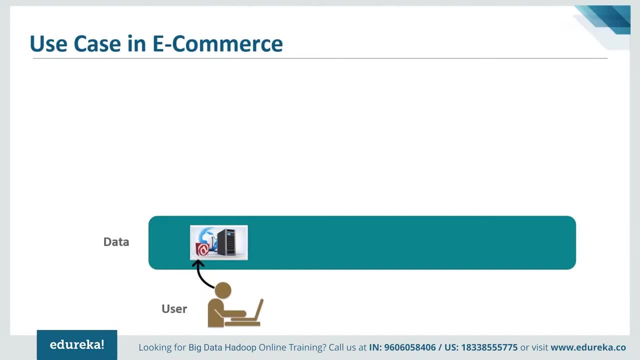 The data is collected from various sources, and that includes customer information, purchase history, reviews and many more, and we have something called as input selection module to remove the noise from the data. So this input selection module is based on two factors: one, singular value decomposition. second, dimensionality reduction. 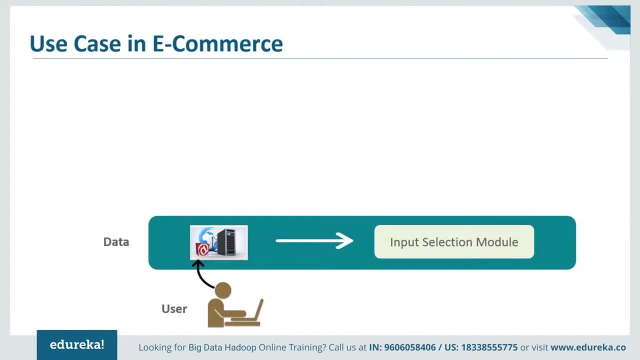 So what is the singular value decomposition? It is nothing but the technology that is used to speed up the recommendations with very fast online performance and that requires just few simple Arithmetic operations. So the data which is used to speed up the online performance is selected. next, 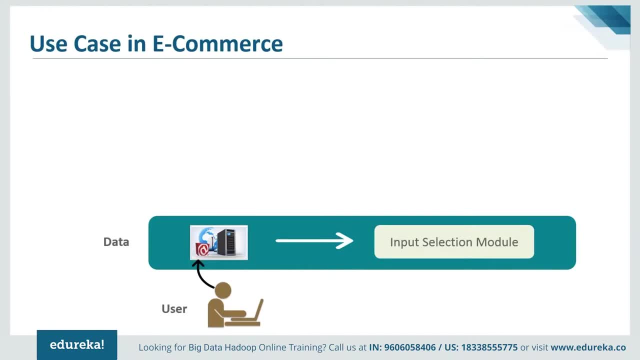 What is the initiality reduction? here We reduce the number of random variables and the consideration that are not required in the data. So, based on these two factors, the input selection module removes the noise from the data. So this noise-free data is fed as an input to HDFS input. 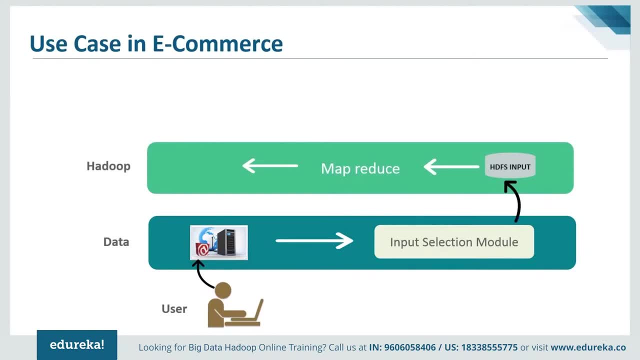 in Hadoop stream and that input undergoes MapReduce job and produces HDFS. This output, the data that we get after applying MapReduce job, is ready for analyzing. So in the data analytics stream we use our tool to analyze the data and from there we arrive at textual and graphical. 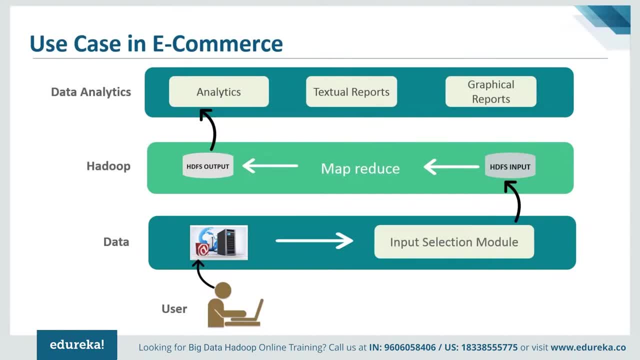 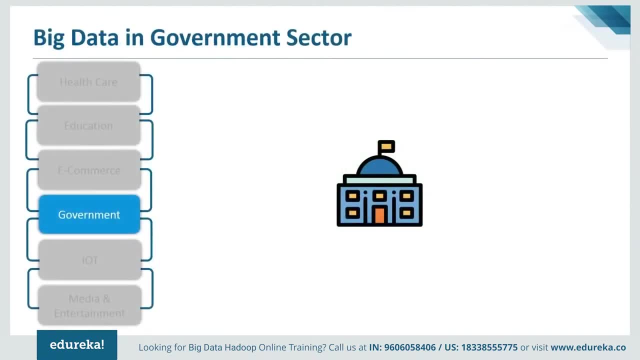 reports- and they are nothing but the reports- that are used in prediction of trends, forecasting demand and in sales generation. Now let's see how government sector has made use of big data analytics. in government use cases, The same data sets are often applied across multiple applications. 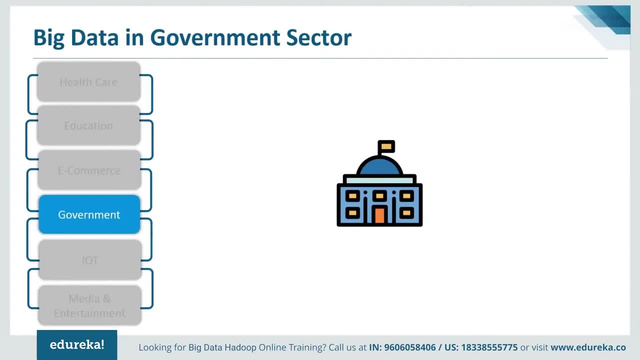 And that requires multiple departments to work in collaboration. Okay, I got a query from Kalgi. She asks why big data analytics is needed in cyber security and intelligence. Kalgi, I'll surely tell you, but for now let's see how it is used in. 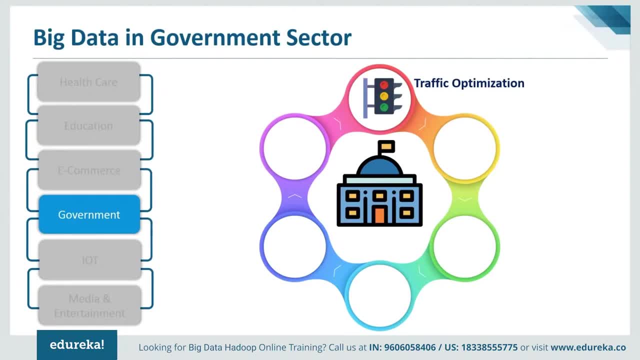 traffic optimization. big data helps to aggregate the real-time traffic data generated from road sensors, GPS device and video cameras. the potential traffic problems in dense areas Can be prevented by adjusting public transportation routes in real time. Kalgi. Now I will tell you why it is used in cyber security and. 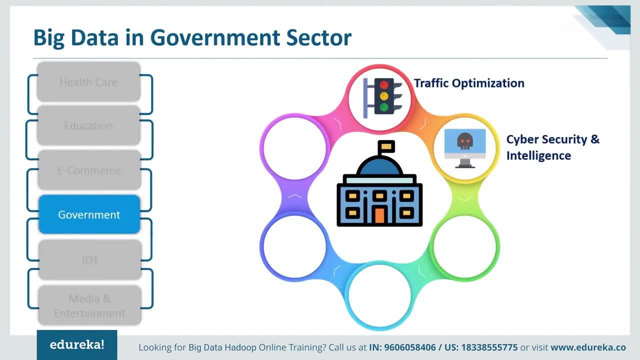 intelligence. You all know that the cyber attacks are increasing in volume and complexity, and that's becoming a tedious task for traditional analytics tools. but companies have to protect themselves against all kind of attacks and they also need to be able to detect and respond fast. 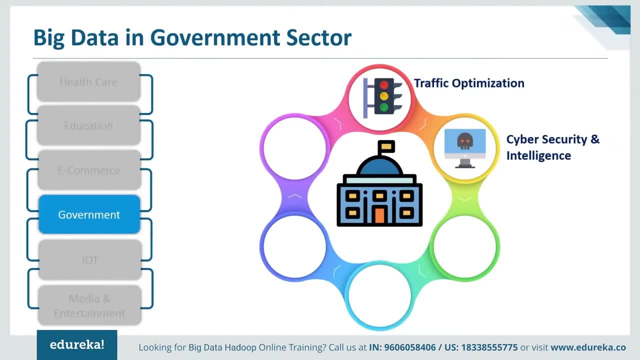 So it's nothing but a PDR paradigm, That is, Prevent, detect and respond. and in order to prevent, detect and respond at a faster rate and quickly, there comes the big data analytics approach, and these challenges can be prevented and overcome with the help of big data analytics. 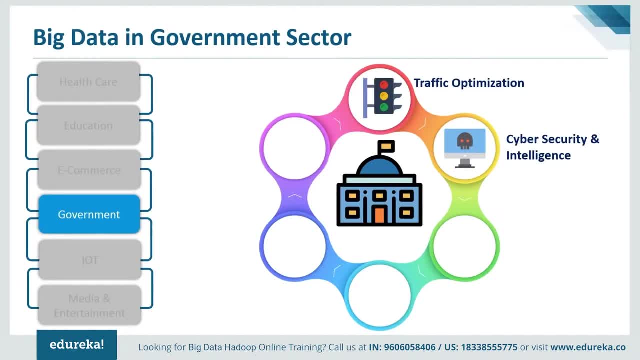 For example, you can say it is used in enterprises to fight against cyber threats. I hope you got an idea about it, Kalgi. Now let's see how it is used in crime prediction and prevention. police departments use advanced and real-time analytics to 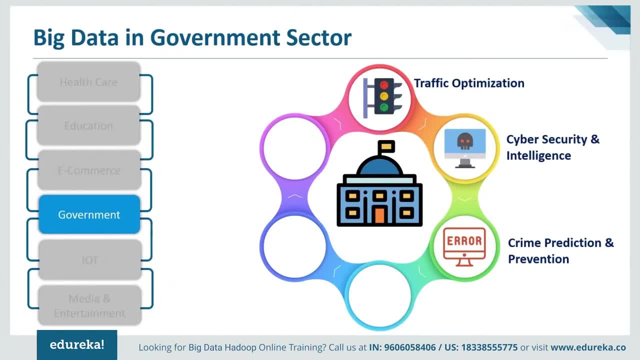 understand the criminal behavior, identify crime and uncover location-based threats. next weather forecasting. the National Oceanic and Atmospheric Administration gathers every minute of every, data from land, sea and space based sensors and on a daily basis, National Oceanic and Atmospheric Administration uses big data to analyze and extract value from over 20 terabytes. 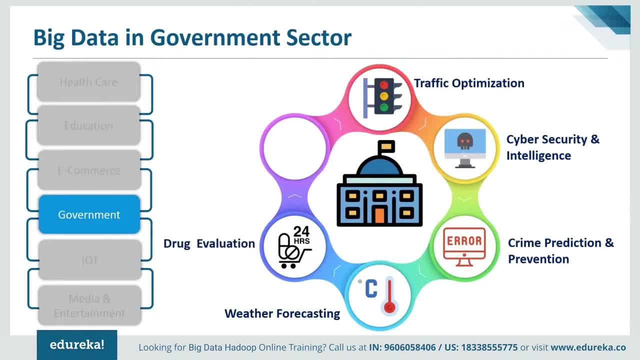 of data. next, Drug evaluation. the National Institution of Health uses big data technologies to access large amounts of data to evaluate drugs and treatment. next, tax compliance. big data applications can be used by tax organizations to analyze both unstructured and structured data from a variety of sources in order to 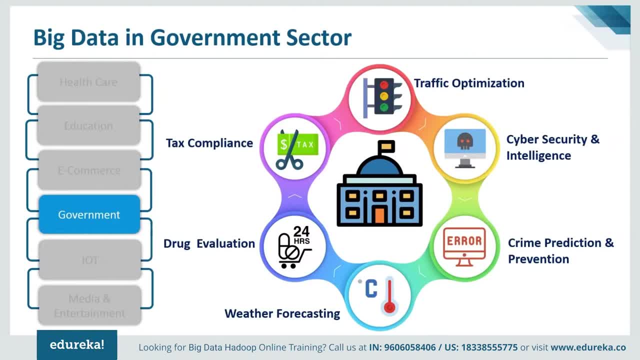 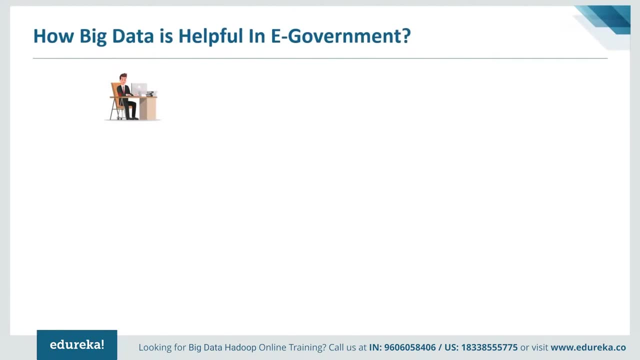 identify suspicious behavior and multiple identities. this actually help in tax fraud identification. So these Are the various sector where big data is used in government. Now let's see how it is useful in e-government portal. So what is the sea government portal? 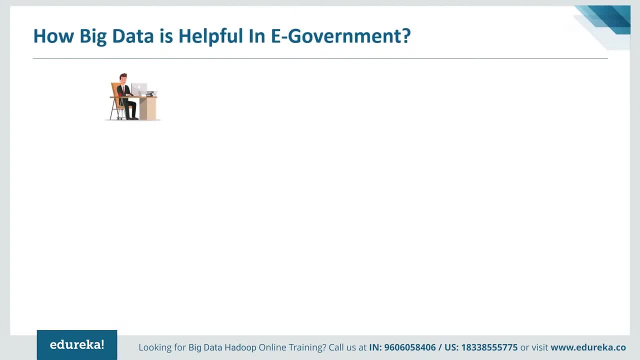 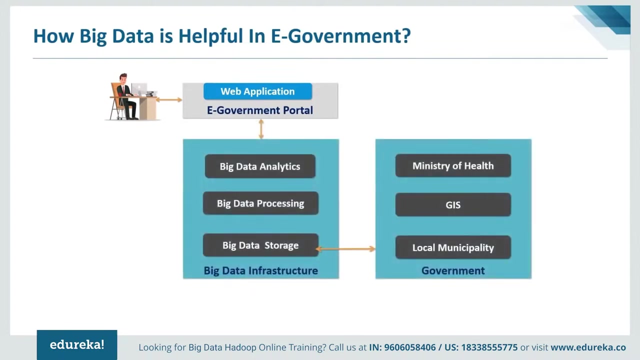 It is an application that uses electronic communication devices, computer and the internet to provide public services to citizens and other people. so citizen or Enterprise user use certain services via e-government portal. So these user requests are sent to big data infrastructure in order to be processed and this big data infrastructure. 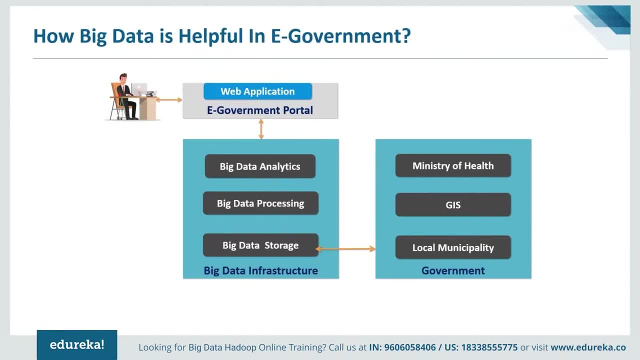 Structure has a database that is not centralized and hence it integrates with database of different ministries, government agencies and local authorities. So both the databases are then deployed to cloud infrastructure, and in this solution We use cloud infrastructure to reduce the cost for storage. and here we have how to framework to process the data. 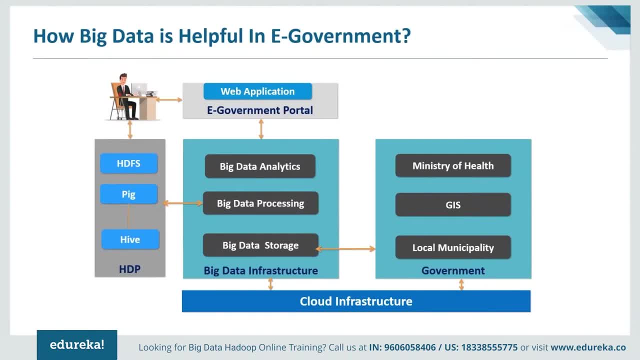 We run pig and hive queries on a Hadoop data platform and then store this data into HDFS and then the response is sent back. So now let me tell you the workflow. Use a sensor request to the network using an appropriate interface. in this case, the appropriate interface is nothing but the web. 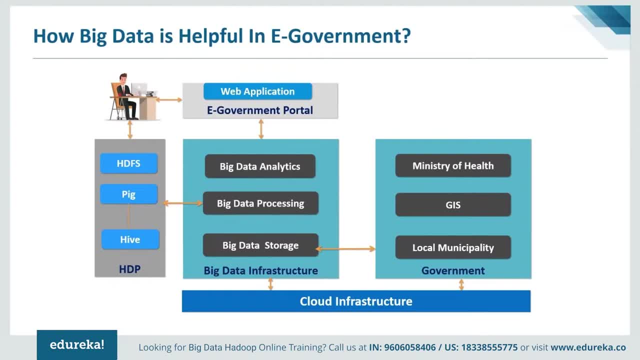 application that he interacts with and the request is then forwarded to big data and the processing happens using these technologies and hence the response is sent back. So this is the internal working that happens but for the use of any communicates or interacts with the web application. 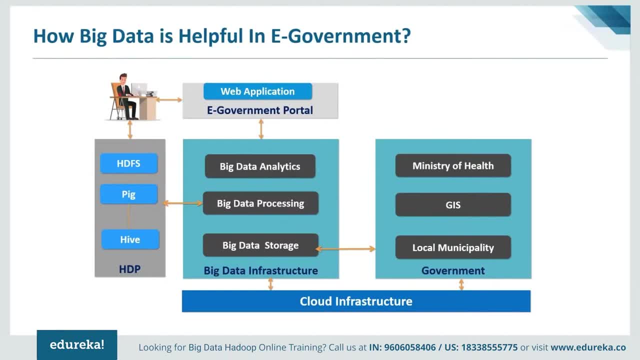 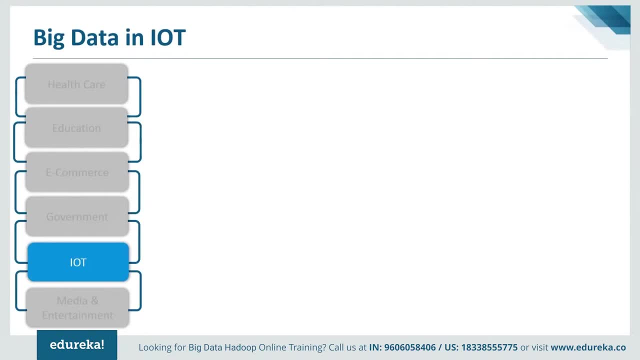 He gets a response immediately. So this is how big data analytics is used in e-government portal. Now let's see how big data is used In iot. data extracted from Internet of Things devices provides a mapping of device interconnectivity. such mappings have been. 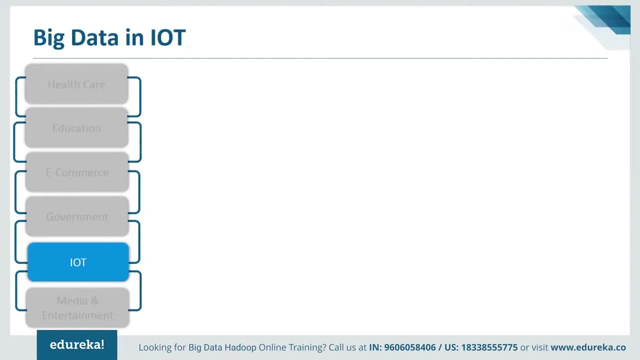 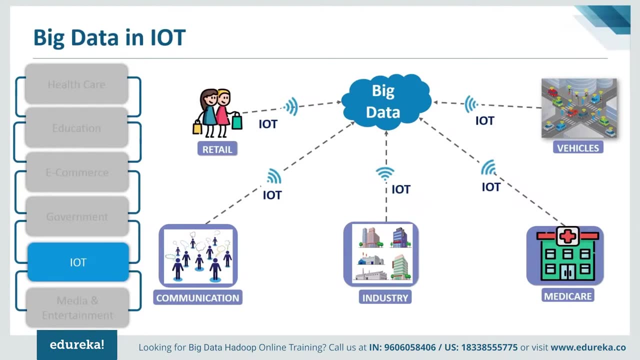 used by various companies and governments to increase efficiency, and iot is also increasingly adopted as a means for gathering sensory data, and this sensory data is used in Medicare, industry, retail vehicles, communication and many more. so iot represents the connected devices, but as there is enormous amount of data, 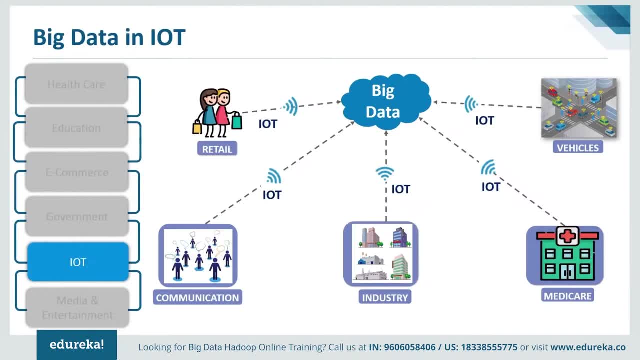 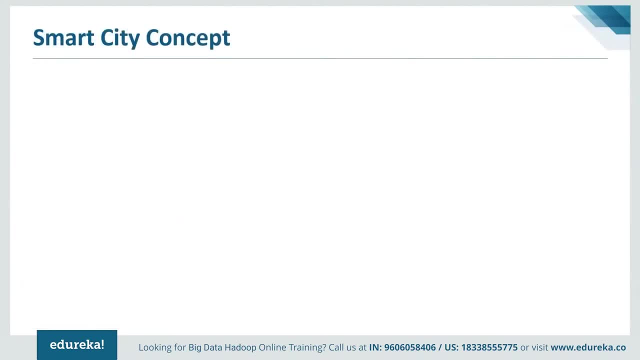 these devices Are connected through iot, and big data technologies is used to store and process this huge amount of data. Let's take a look at the smart city concept. the combination of iot and big data is an unexplored research area that has 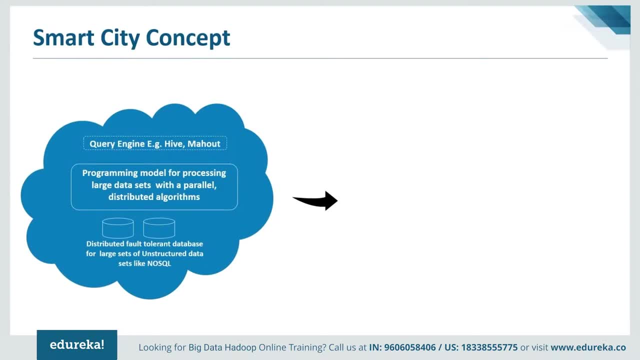 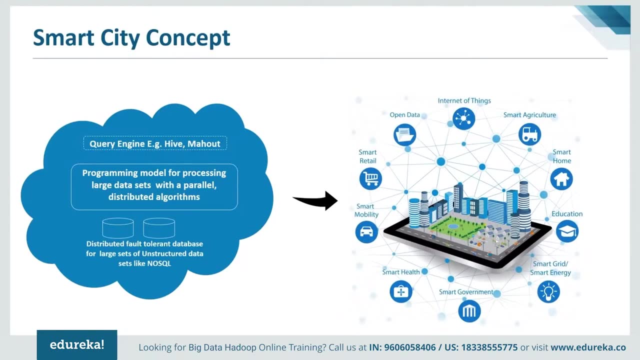 brought new and interesting challenges for achieving the goals of future smart cities. You might have heard of Amsterdam. right, It is the pioneer in the concept of smart city. Now you might be wondering how it does introduce the concept of smart city. Amsterdam has introduced the concept of smart city in smart. 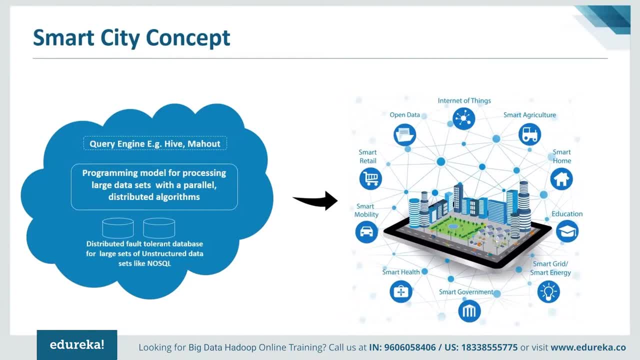 government, smart health, smart retail, smart agriculture and many more. I got one more query here, and this query is from Gino. He asks how Amsterdam has implemented the concept of smart city in smart home. Gino, I will explain you now in case of smart city. 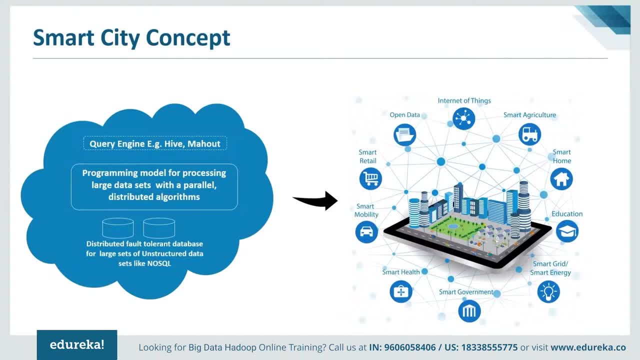 They use a variable technology, that is, any person in the home can wear the fitness band. that is a variable technology, and the techies have programmed and integrated this smart thing in such a way that, when the person wakes up, the lights will automatically turn on and the coffee machine starts to. 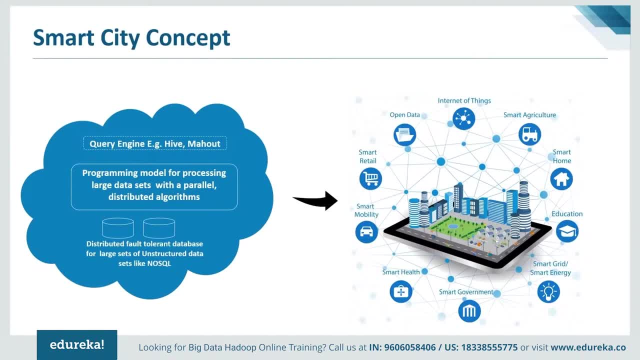 prefer the coffee, and it is vice-versa. when the person who is wearing the fitness band goes back to sleep, the light turns off. I hope you got an idea about it, Gino. Now let's move further. in this case, various smart applications exchange information using embedded sensor devices and other. 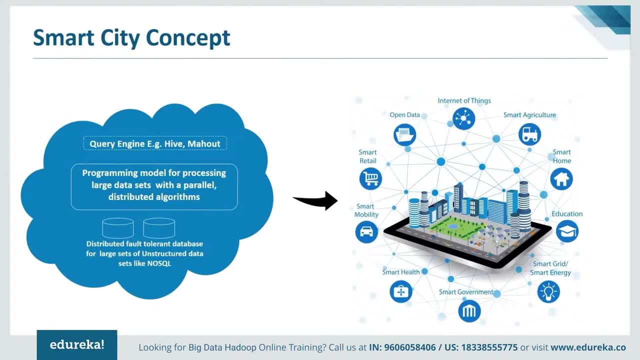 devices that are integrated, But cloud computing infrastructure to generate large amounts of unstructured data, and these large amounts of unstructured data are collected and stored in the cloud or a data center using a distributed fault-tolerant database that is no SQL and that is used to improve the single service or application. 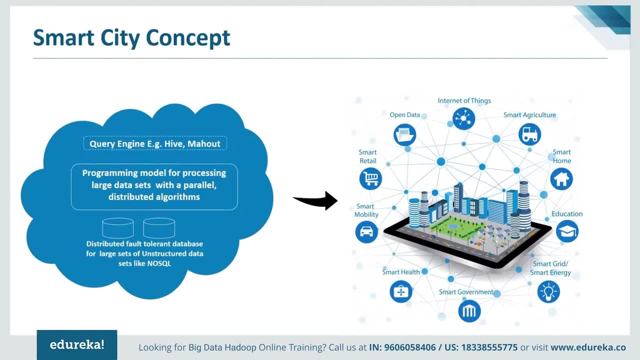 and is shared among various devices. and you also have a programming model for processing large data sets with the parallel distributed algorithm and that can be used for data analytics to obtain the value from the data. here We have query engine like hive and mahout to query and structure. 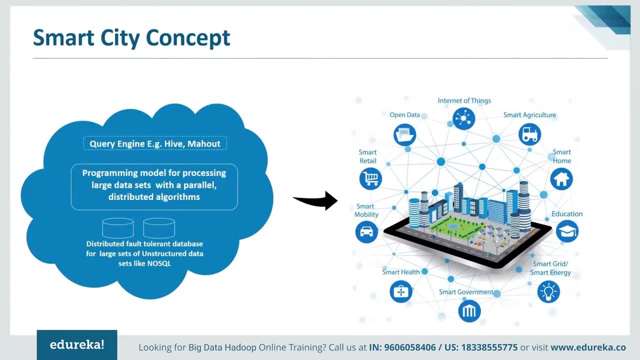 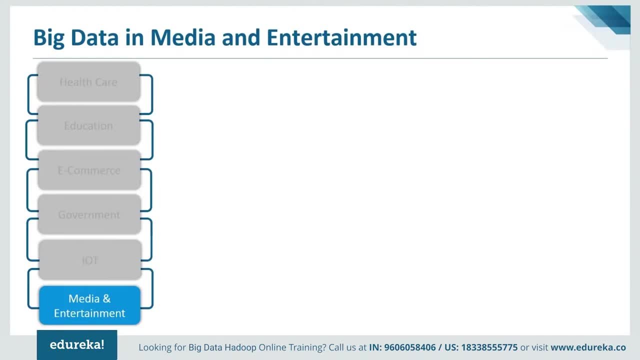 the data. So this is how cloud and big data both are used in the smart city concept. last but not the least, Let's see how big data is helpful in media and entertainment. various companies in the media and entertainment Industries, like publishers, broadcasters, cable companies, YouTubers, are 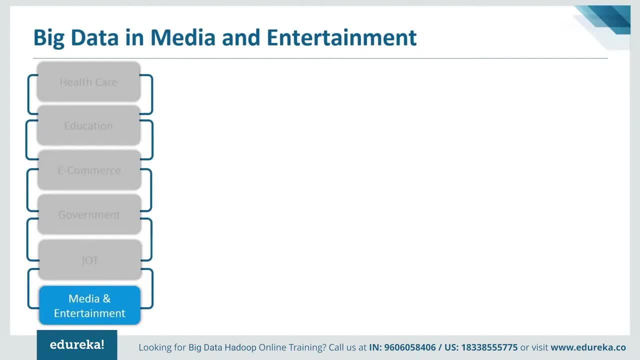 facing new business models for the way they create, market and distribute their content. And that is happening because of the current consumer search and the requirement of accessing this content anywhere, anytime and on any device, and big data provides actionable points of information about millions of individuals. and all these, 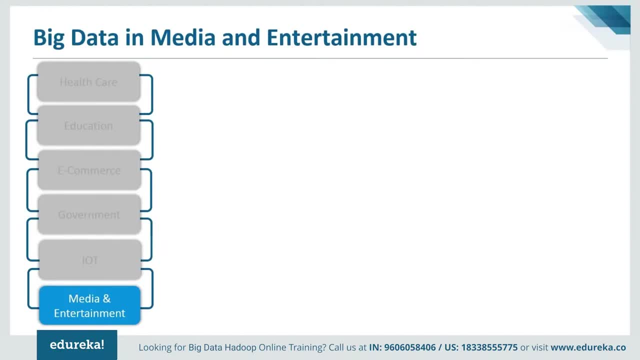 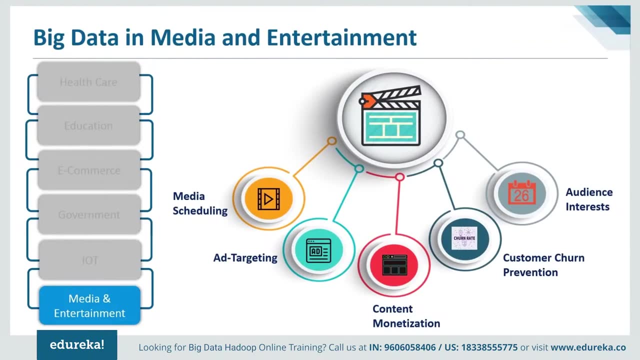 insights are gathered through various data mining activities and big data applications. benefits media and entertainment industry by media scheduling at targeting content, monetization, audience interest, customer churn prevention. So now let me tell you how to prevent a customer churn. customer churn is a serious menace that media companies find almost impossible. 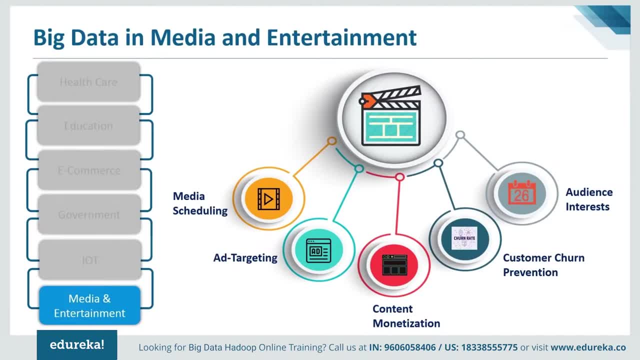 to tackle, and it has been found that at least 30% of the customers share their views to social media, and until big data arrived, combining and making sense of this user data was next to impossible, and with the advent of big data analytics, it is possible to know. 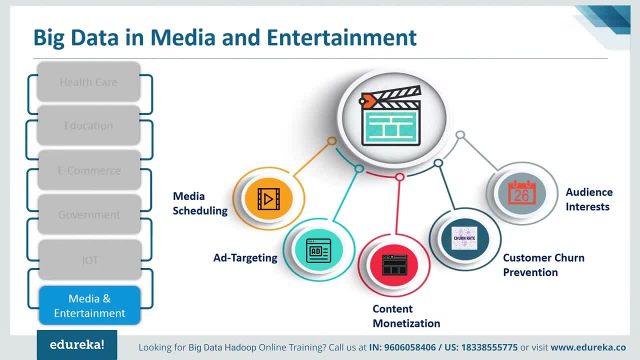 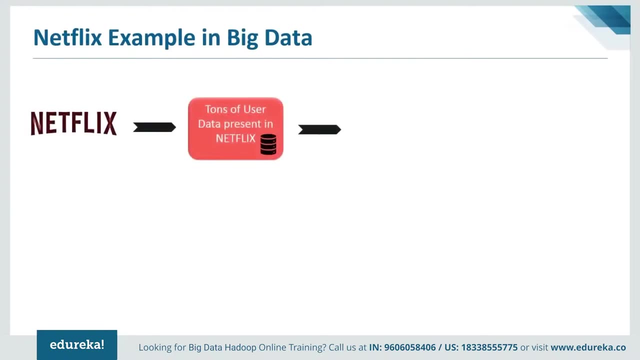 why customers subscribe and unsubscribe and what kind of programs they like. this like with Crystal Clear clarity. So banalizing all these factors, It is very easy to prevent the customer churn. Let's take a look at the Netflix example. in big data, Netflix has tons of user data present in its database system. 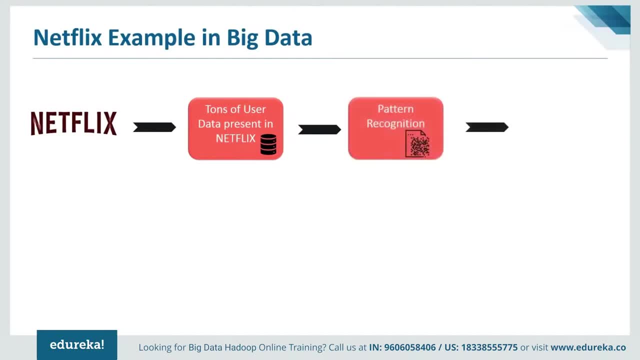 and this data is processed and analyzed and we recognize the patterns for that. and here we have a new user request and this user comes and search for a video in the Netflix search engine and, based on the video Preferences and the user choice, we rank the video. 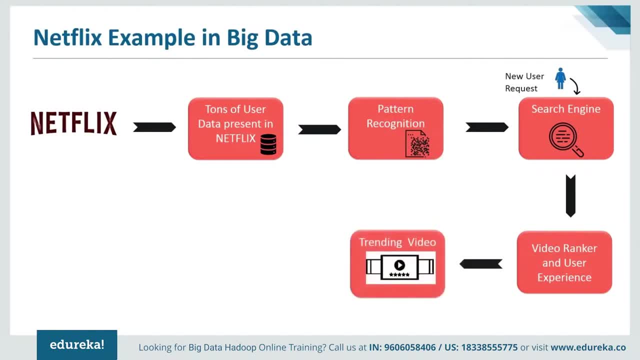 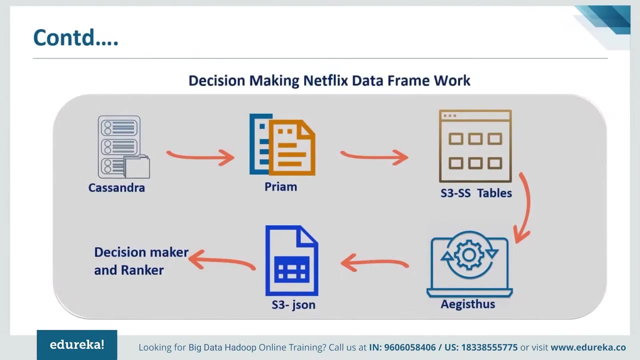 and also we give user experience and then we continue to watch the trending video and we arrive at video similarity algorithm. So now let's see how the decision is made and the video ranking is being given. This is decision-making. Netflix data framework. Netflix uses Cassandra. 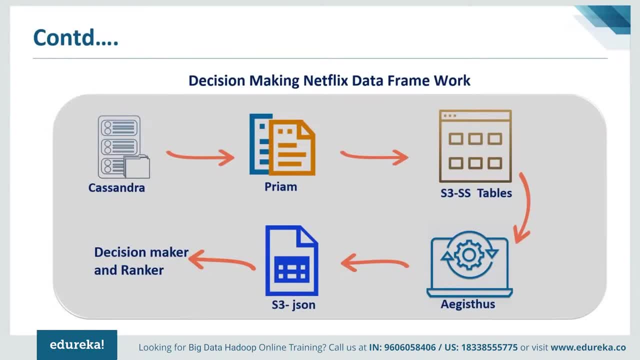 because it is highly scalable and strong and performance. here We have Cassandra that is a no SQL database and it is used by Netflix because it is very strong on performance. and we have Brian that is a Cassandra helper tool and also it is a Netflix cluster management tool. 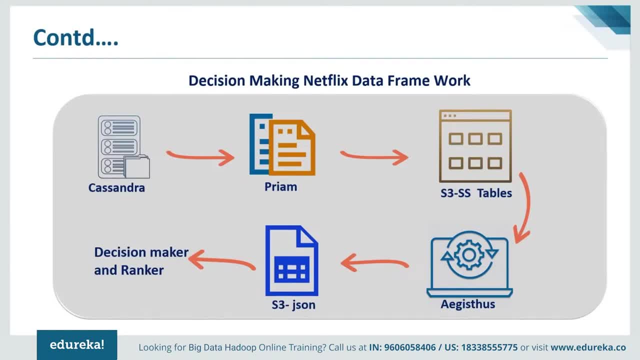 that simplifies the Netflix administration and it also uses API to query the Cassandra metrics. and next we have x3 assist tables. The query data is stored in s3 assist table in a table format, and we have a justice. that is a platform built by Netflix engineer. 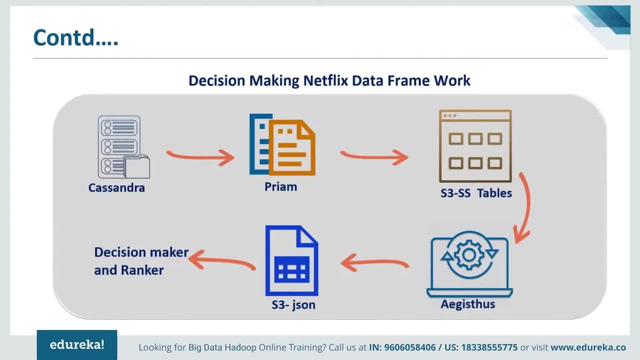 to work on Hadoop MapReduce, and this, a justice, converts the Cassandra s3 assist tables into query able format. And we have s3, Jason, that is a javascript object notation and that is used to structure the query data and hence, based on all these factors, the decision is made. 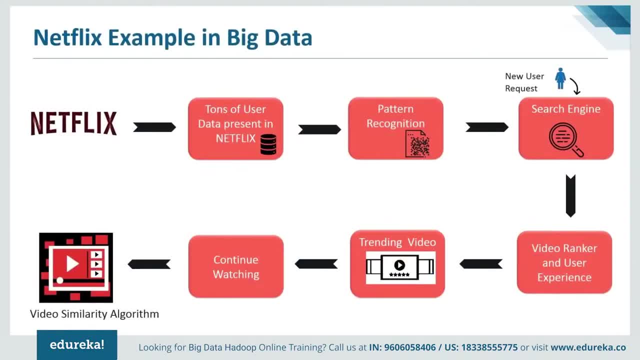 and the video ranking is being given. So if you go back, you continue to watch the trending video and you get the video similarity algorithm. So this is how Netflix has used big data analytics. Now let's move further and see the scope of big data. that will create a havoc. 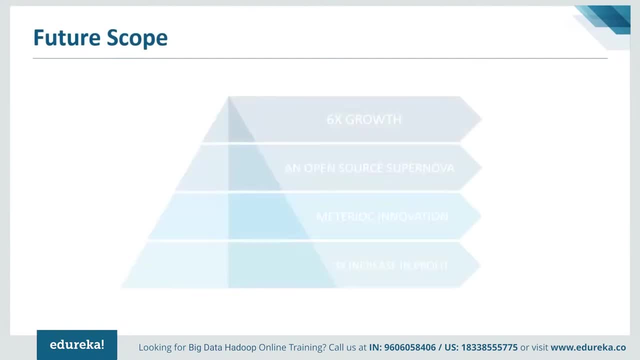 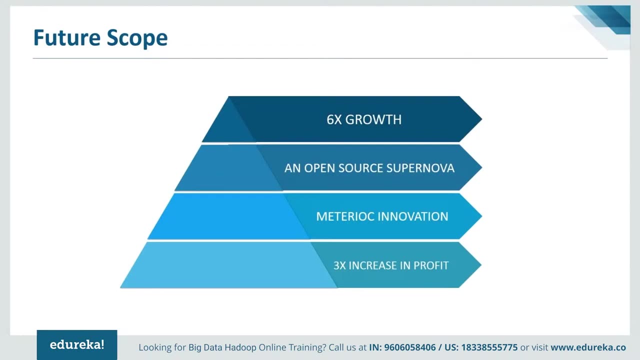 in the near future. first, 6x Growth. it's obvious fact. the amount of data that will be generated in the next five years will be 6x times more than that what was generated in the past five years. So imagine we'll be having huge, huge amount of data. 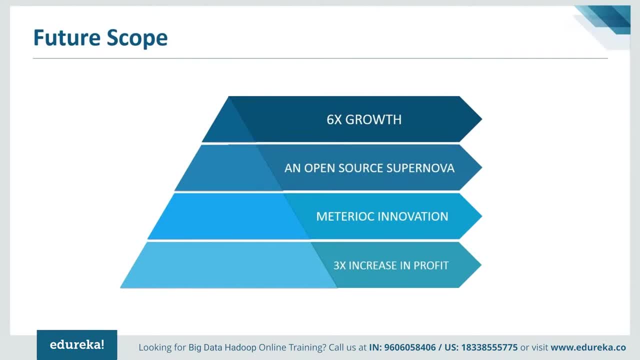 and not only that, but also the Hadoop adoption is growing at 29 times more than that of US GDP. next and open-source supernova. Let me bring out the comparison here. In 1998, only 10% of the companies used to use open-source. 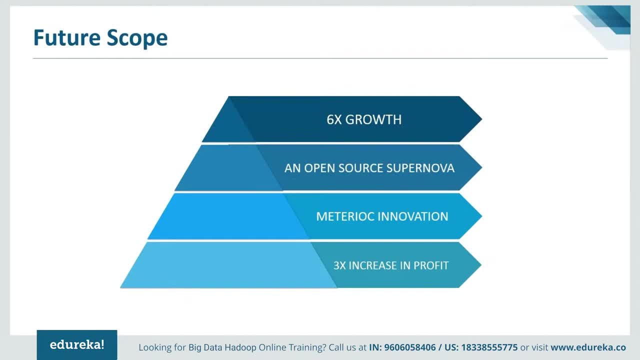 networks, and that gradually increased to 50% in 2011 and now 78% of the companies use open-source office and in the next year's, entire hundred percent of the companies use open-source office. and these Advancements is because of the growth of big data in the market. next, why it is termed: 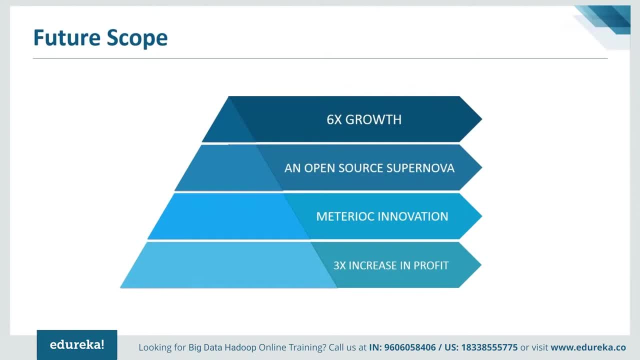 as meteoric innovation. You all know that in 2008.. There were more things connected to the internet than people and now iot devices represent over 6.48 billion devices connected and in 2020, the iot market will connect to over 21 billion devices and, by 2030, self-driving cars. 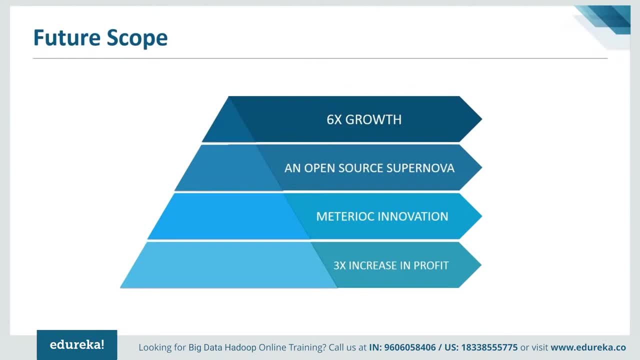 will rule the roads of the world and that is why it is termed as a meteoric innovation. the next 3x increase in profit based on the above three terms, That a 6x growth, open-source softwares: meteoric innovation. It is an obvious fact that as the technology is evolved, 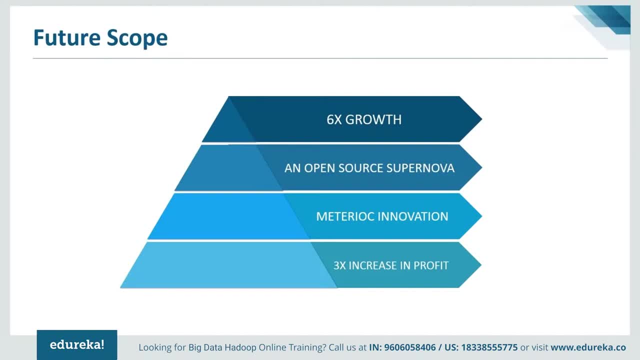 the growth will be evolved and that leads to 3x increase in profit rate as well. So in the next few years, the profit rate will tends to increase to 3x times more than that what it is there in today's world. So this is why we say that big data is going to create. 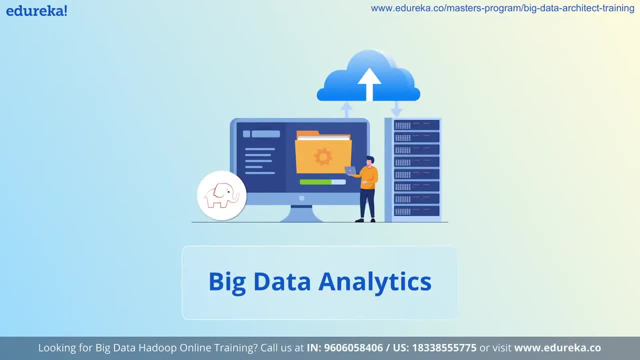 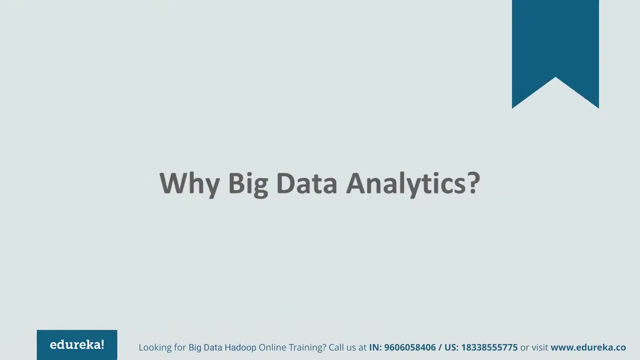 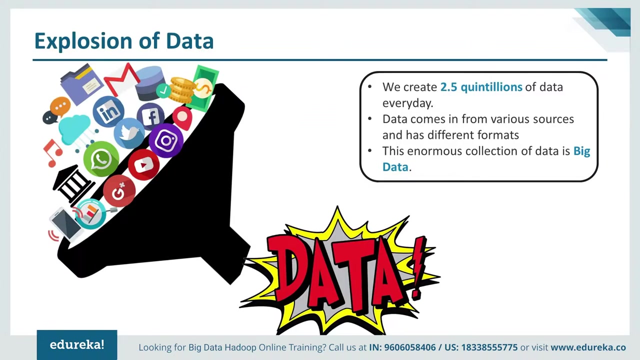 a Havoc in the near future. Why do you think big data analytics is so important And why do you feel that we need to study this topic, or we should know what exactly it is? So now let me tell you why. so, just like the entire universe. 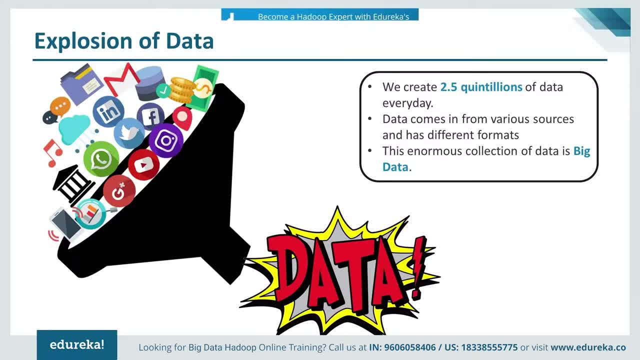 in our Galaxy said to have formed due to the Big Bang explosion. Similarly, data has also been growing exponentially, which is leading to the explosion of data, So this can simply be termed as big data, and you know that we are creating about 2.5 quintillion bytes of data. 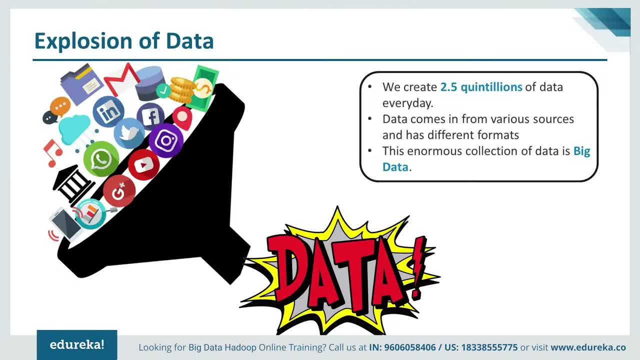 Every day, and one quintillion amounts to around 10 raised to the power of 18 bytes. So you can do the math and imagine the amount of data that we are creating every day. and this data, as you can see from the image that I have depicted here, is coming in from various 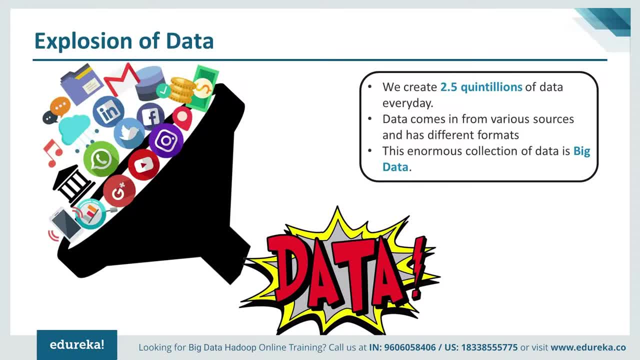 sources, whether it is from social media, from banking sectors, from governments, from various other institutions, All right. and this data is not in the same format, So it is coming from various sources, So it is in different formats. So now, guys, what do you think? that is big. 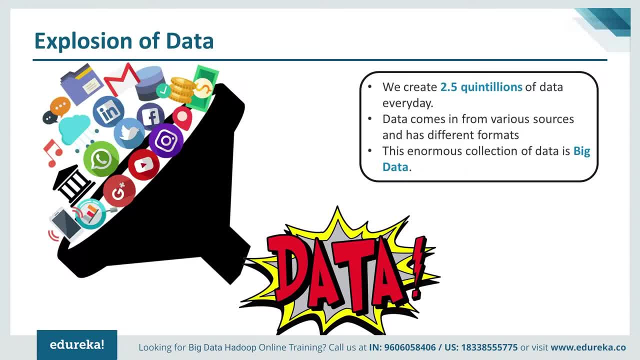 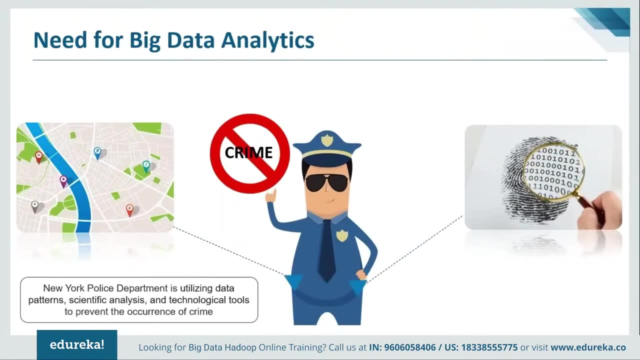 Data only limited to the volume or the enormous amount that is being generated or does it define, with various other characteristics that you know exactly define, what big data is. So I have put down four such reasons here to tell you that why it is so important and how it is helping many organizations. 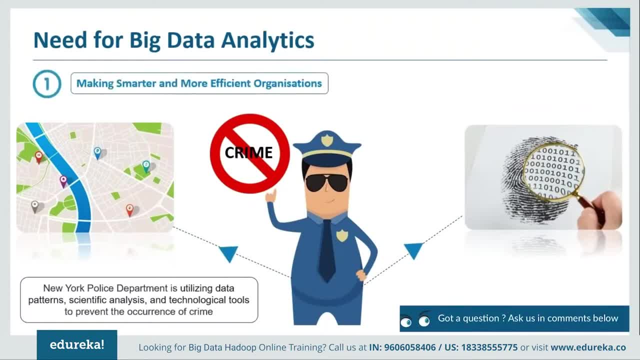 all around the globe. So the first reason here that I've stated is for making smarter and more efficient organizations. So big data analytics is basically highly contributing to this. factors and organizations are Opting this to basically lead them to faster decision-making. So one such example that I you know came across that I wanted. 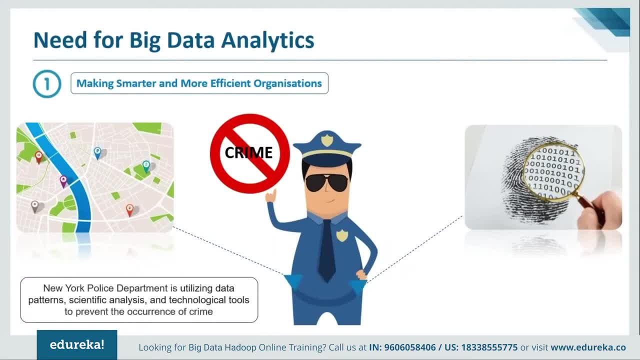 to share with you guys is about the New York Police Department, in short, which is the NYPD. So big data and analytics are helping the NYPD and the other large police departments to anticipate and identify the criminal activity before it occurs. So what they do is that they analyze the entire big data technology. 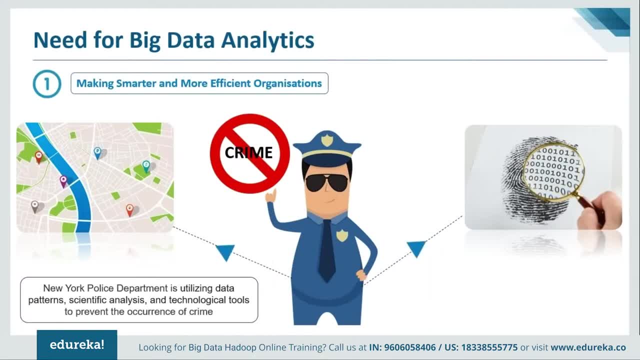 to geolocate and then analyze the historical patterns, and they map these historical patterns with sporting events, Rainfalls, traffic flows and federal holidays. So essentially what the NYPD is doing: that they're utilizing these data patterns, scientific analytics, technological tools to do their job and they're ensuring that by using these different tools. 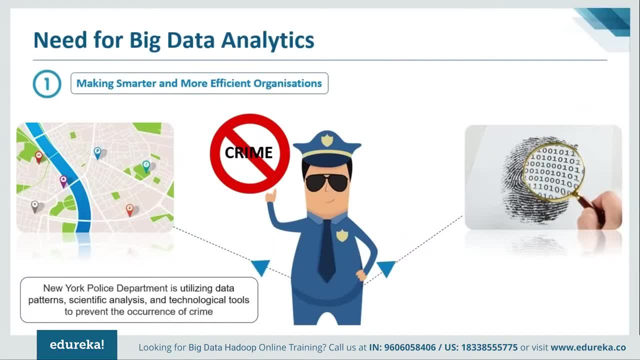 they're doing their job to the best of their ability. So, by using a big data and analytics strategy, the NYPD was able to identify something called crime hotspots. So basically, where crime occurrence was more so, they were able to identify these hotspots. And then 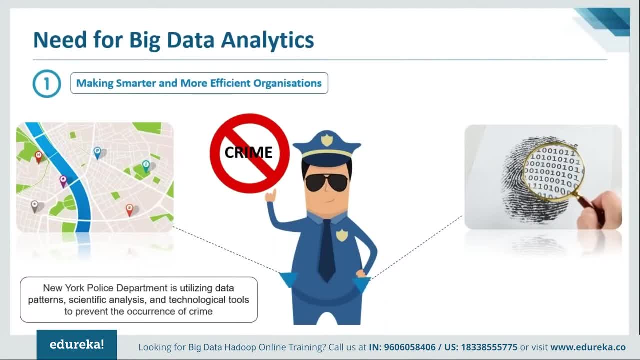 From there they deployed their local officers so that they could reach there on time, before it was actually committed. So this is how NYPD basically utilizes entire- you know this- field of big data analytics so that they can prevent crime and make New York a board safer place. 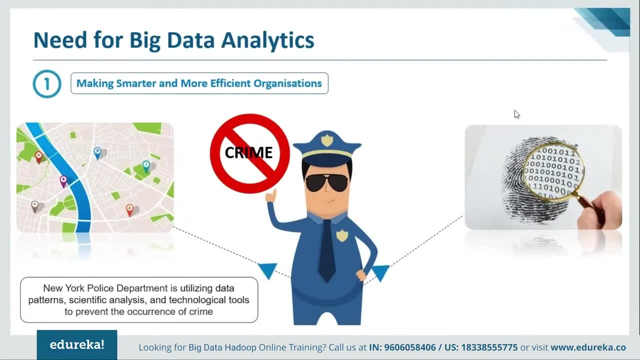 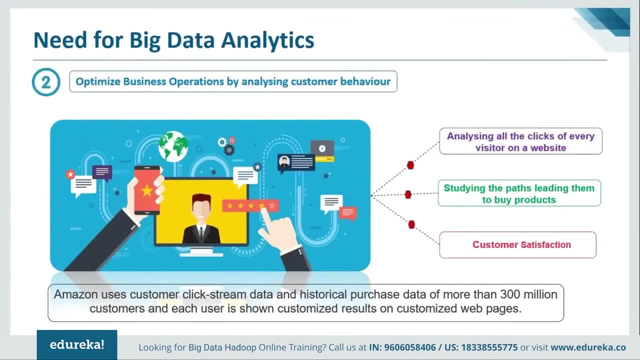 So now, after exploring the first reason, let's move on to the second reason and see what is it. The second reason here is to optimize business operations by analyzing customer behavior. So the best example For this is Amazon. We all know how much Amazon is popular and how much we use it on. 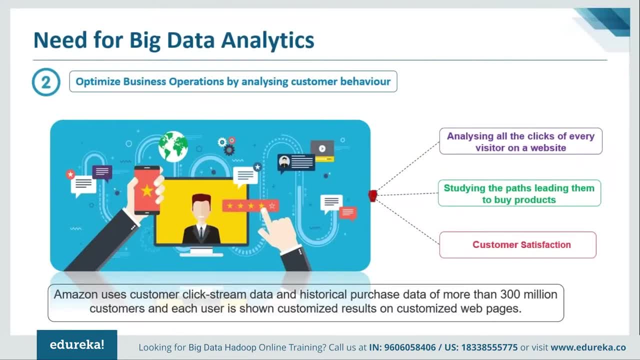 our daily basis. So Amazon basically uses our clickstream data, that is, the customers. So they use our clickstream data and the historical purchase data of more than 300 million customers which have, you know, signed up for Amazon, and then they analyze each user's data, how they are. 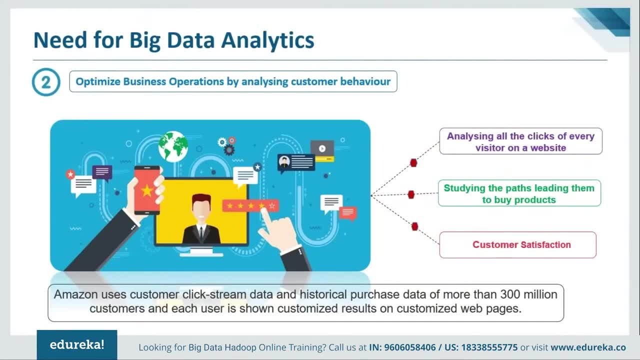 clicking on different products and how they navigating through their site. So basically, they show each user customized results on customized web pages. So after analyzing all these clicks of every visitor on their website, they're able to better understand their site navigation behavior, the parts that people are taking to buying their products. 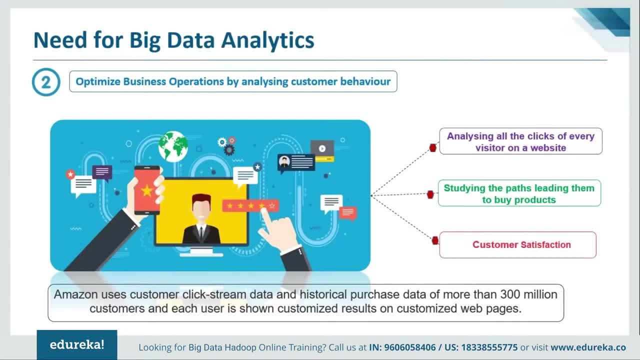 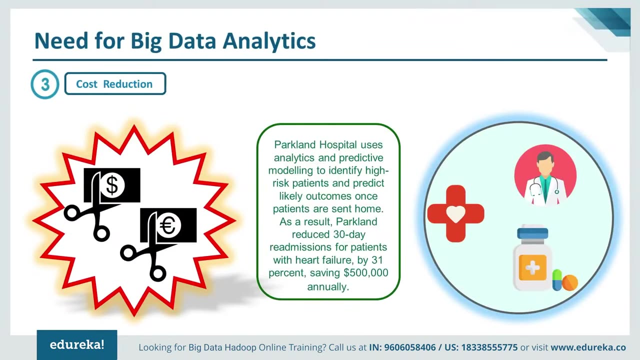 and services and what else a customer looked on while buying that product, and also the parts that led a customer to leave their page. So this information basically helps Amazon to improve their customer experience and hence expand their customer base. So, guys, let's see what the third reason is now. so big data technology. 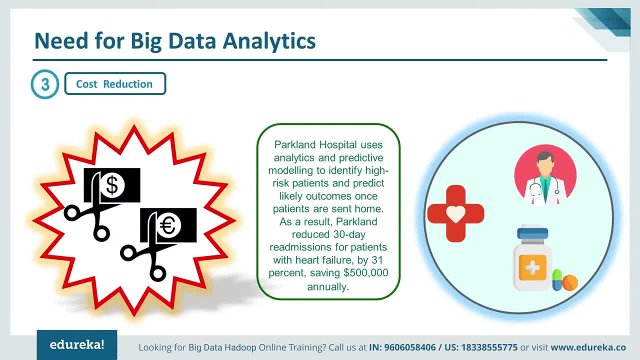 is like Hadoop and cloud-based analytics. They basically reduce your cost significantly for storage of big data, because for storing big data if you buy like huge servers and you know huge machinery, So that is going to cost you a lot. So by using Hadoop technology- so what Hadoop does, basically stores- 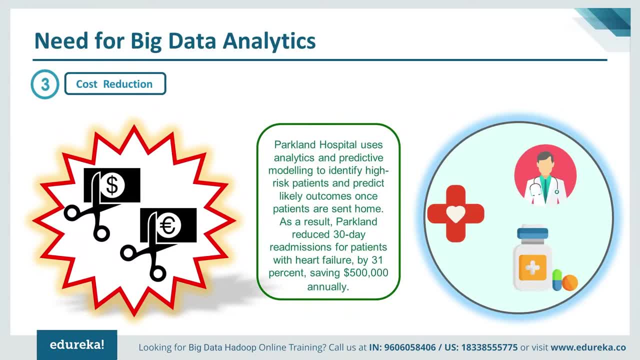 big data in a distributed fashion so that you can process it parallely. So it reduces your cost a lot. So by using commodity hardware, they are reducing their costs significantly. So which brings us to our third reason: you must have gauged what the 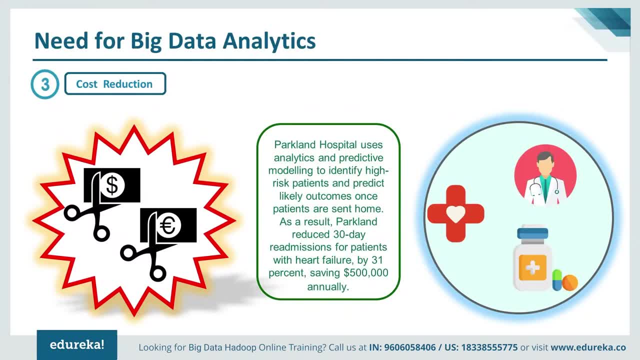 third reason Is it is cost reduction. So now let us see how healthcare is using big data analytics to curb their costs. So using new data tools that send automatic alerts when patients are due for immunizations or lab work. more and more physicians could reduce the hospitalizations by practicing better preventive care. 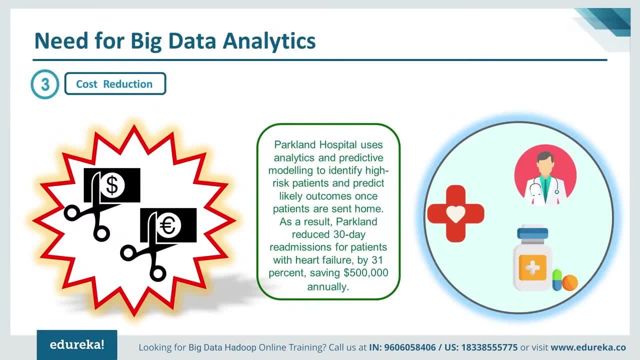 So you know what the patient started using these new sensor devices at home and on the go. So these new sensor devices- they basically, you know- deliver constant streams of data that can be monitored and analyzed in real time. So they help the patients avoid hospitalization by self-managing their 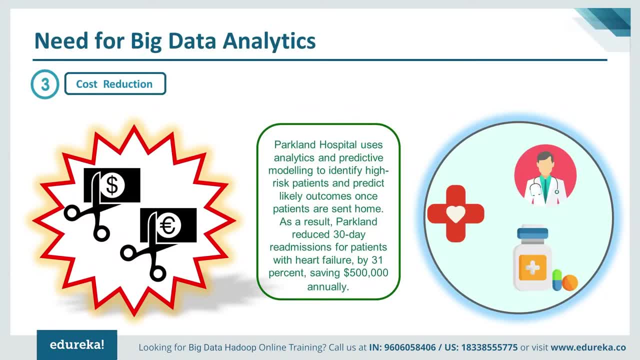 conditions. Now, for hospitalized patients, physicians can use predictive analytics to optimize outcomes and then reduce the readmissions. So Parkland Hospital in Dallas, Texas, is one such example, which has been using analytics and predictive modeling to identify these high-risk patients and then they predict likely outcomes once the patients are. 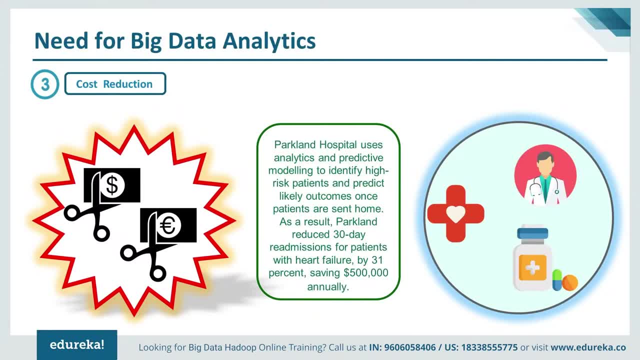 sent home. So as a result, Parkland has been able to reduce hits, 30-day readmissions back to Parkland And all area hospitals for Medicare patients with heart failure by around 31%. So for Parkland, that you know, estimates about a savings of $500,000. 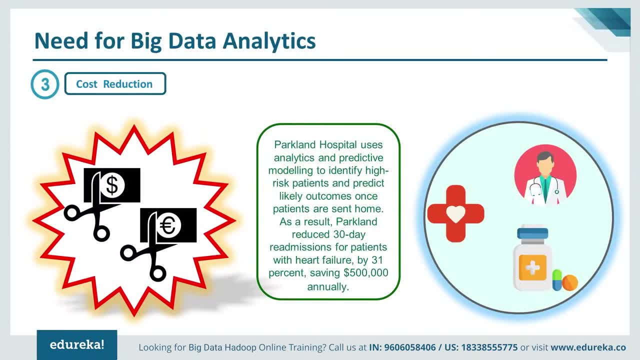 annually and, of course, not to mention that, the savings which patients are also realizing by avoiding these readmissions. So this is how healthcare is. you know widely using big data analytics to reduce their costs significantly. Now let's move forward to see the last reason for why big data. 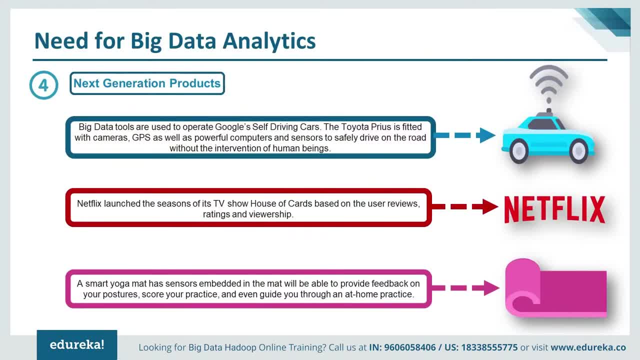 analytics is so essential. So our last reason is next-generation products And how big data analytics is really really contributing to generate more such. you know, high-tech products, So you know to see how customers needs can be satisfied and how they can use these new generation products for their own benefit. 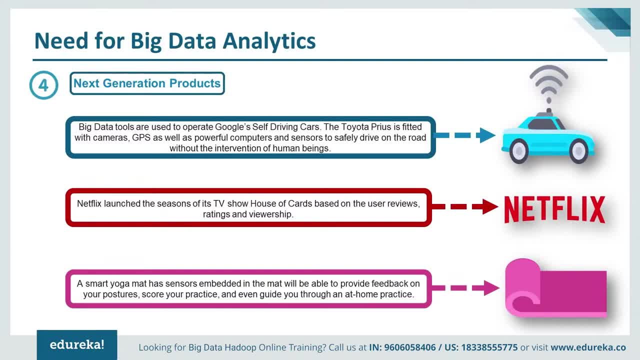 So I have cited three such examples here for you guys. So the first example here is Google self-driving car. I'm very sure that most of you guys must have heard about it. What Google self-driving car basically does? it makes millions of calculations on every trip that help the car decide when and where to 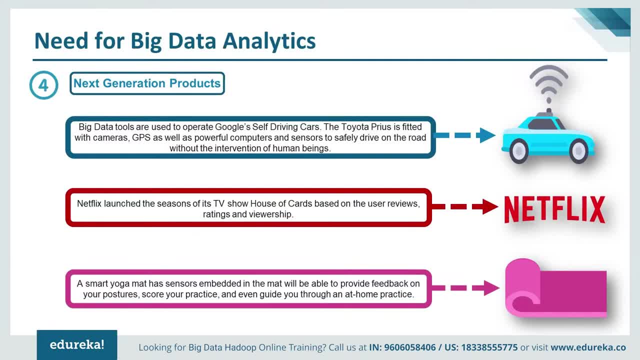 turn, Whether to slow down or speed up, and when to change their lanes. So the same decision a human driver is making behind the wheel. Google self-driving car is also doing that with the help of big data analytics. Another example of a self-driving car is the Toyota Prius, which is fitted 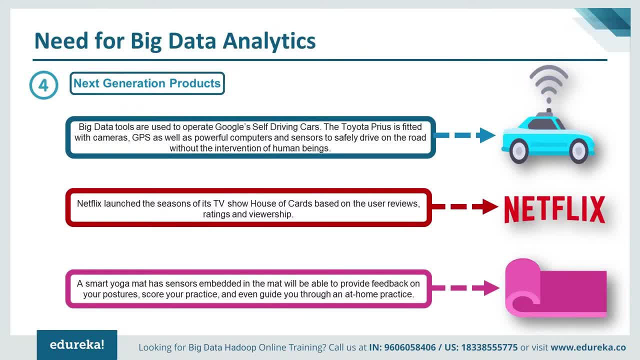 with cameras, GPS, as well as powerful computers and sensors to safely drive on the road without the intervention of human beings. So this is how it is, you know, really really contributing to making such high-tech products which, in the long run, we'd be using, probably, and 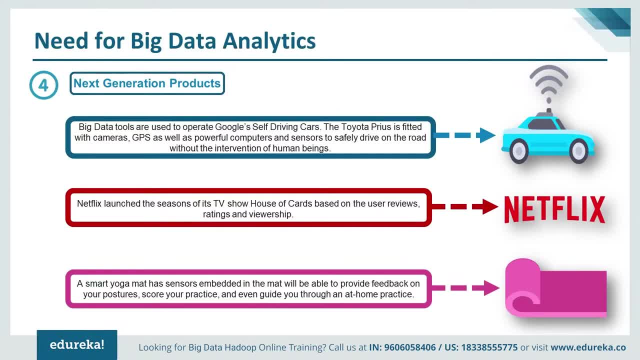 it will make our life more Easier. now, moving on to the second product that I'm going to cite here. So it's really fascinating product. Let me ask you a question: How many of you all love watching TV shows and how many of you all prefer 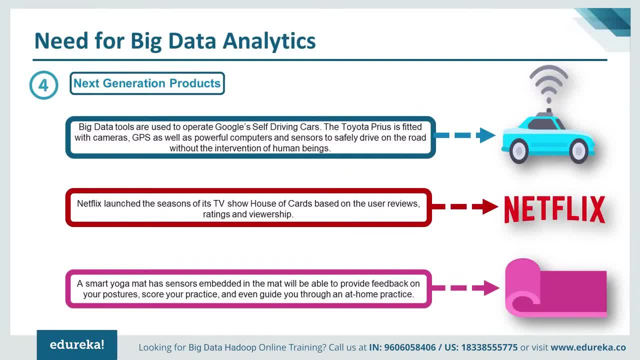 spending your weekends doing nothing but Netflix and chill? Let me guess almost all of us do. I mean, I love binge watching shows over the weekend, So I know by now you would have guessed what example I'm arriving to. So it is Netflix. 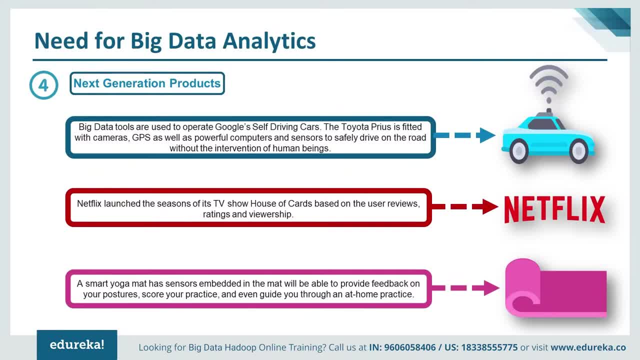 So Netflix committed for two seasons of its extremely popular show, House of Cards, Without even Seeing a single episode of the show, guys, and this project of you know, House of Cards, of two seasons, It costed Netflix about hundred million dollars. So, guys, how do you think that Netflix was able to, you know, take such a? 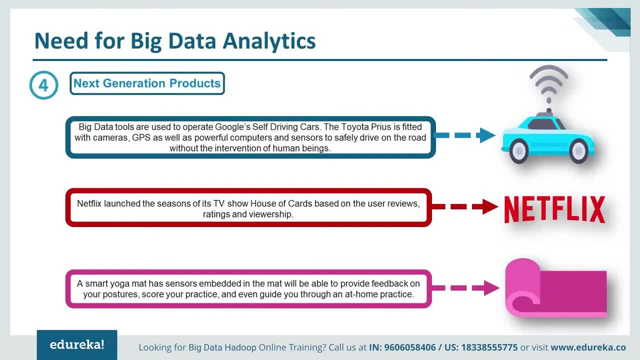 big risk monetarily. So the answer to this, my friends, is big data analytics. So, by analyzing the viewer data, the company was able to determine that the fans of the original House of Cards which aired in the UK. They were also watching movies that start Kevin Spacey who is playing. 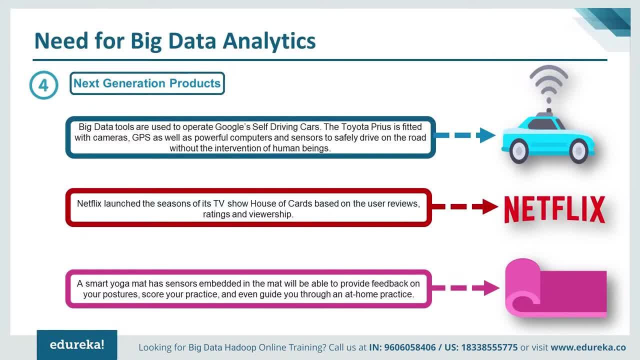 the lead in the show House of Cards, And they were directed by David Fincher, who's also one of the shows executive producers. So basically, Netflix is analyzing everything. So from what show you are watching, to when you pause it, or to when even you turn it off. 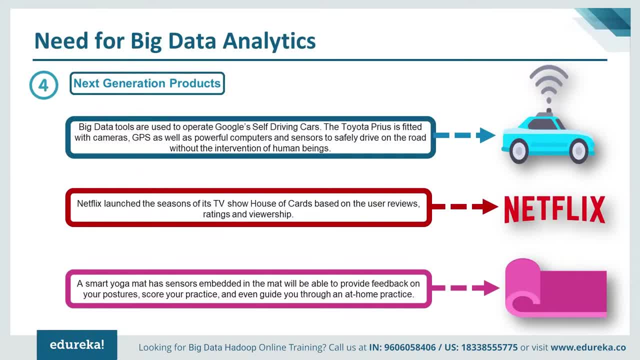 So last year Netflix grew its subscriber- US subscriber- base by around 10%, and then they added nearly 20 million subscribers from all around the globe. So how fascinating is that? I mean, this is brilliant. I am sure that the next time you guys are watching a show on Netflix, 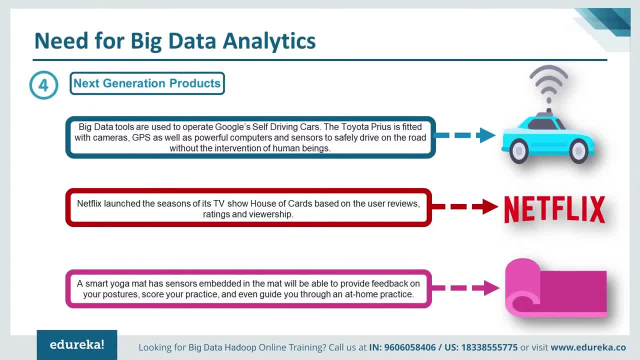 you'll be really happy Because you already know how the back end is working and how Netflix is recommending you new shows and new movies. So now, moving on to the third example that I've cited here. So it's one of the really cool things that I've come across. 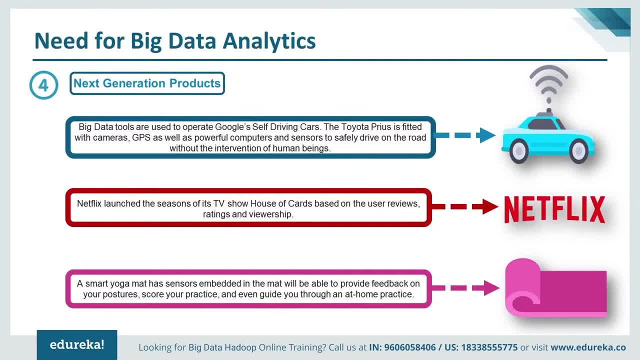 So this is a smart yoga mat. Now, This has sensors embedded in the mat which will be able to provide feedback on your postures, score your practice and even guide you through an at-home practice. So the first time you use your smart mat, it will take you through a 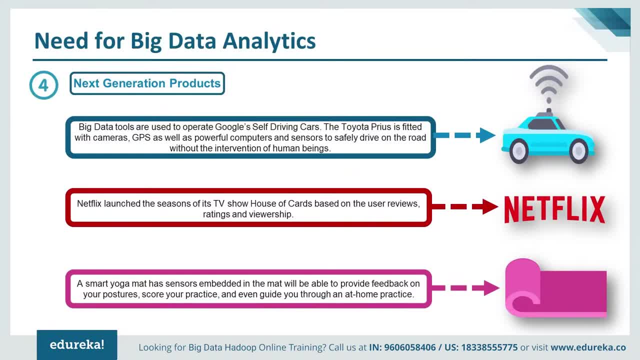 series of movements to calibrate your body shape, size and personal limitations. So this personal profile Information of yours is then stored into your smart mat app and this will help the smart mat detect when you're out of alignment or balance. So over time, it will automatically evolve with updated data as you. 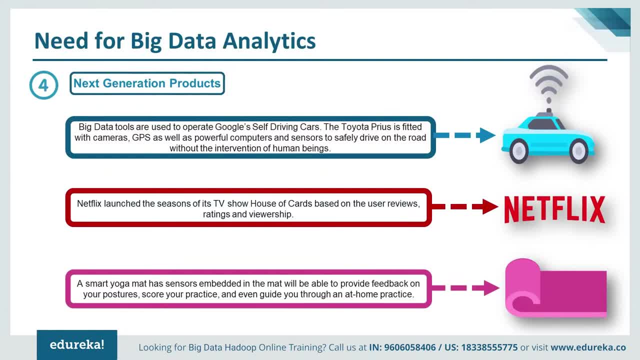 improve your yoga practice. So now, I'm sure that with these you know very interesting and exciting examples, you would have got an idea about what exactly big data analytics is doing and how it is improving various organizations in their sales and marketing sector. 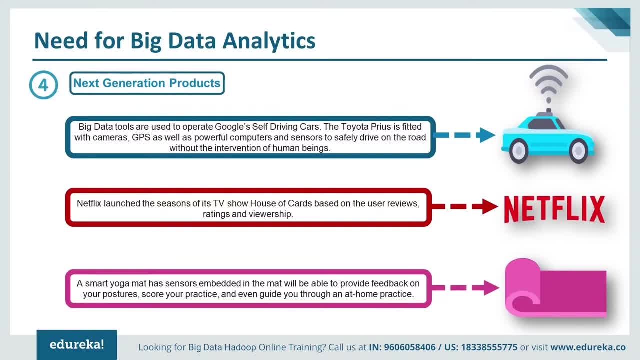 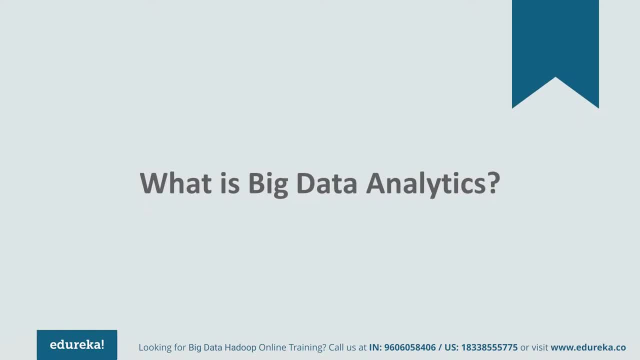 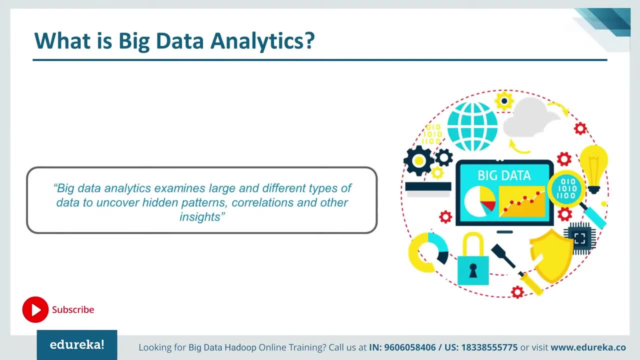 So now let's move forward and finally, you know, formally define what big data analytics is. So, guys, what is big data analytics? Big data analytics examines large and different types of data to uncover hidden patterns, correlations and other insights. So, basically, what big data analytics is doing? it is helping large. 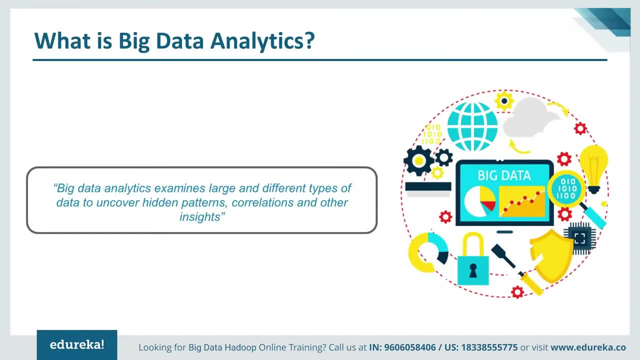 companies to facilitate their growth and development. So this majorly involves applying various data mining algorithms on a given set of data, which will then aid these organizations and making better decisions. So now that you know why We need big data analytics. What is exactly big data analytics? 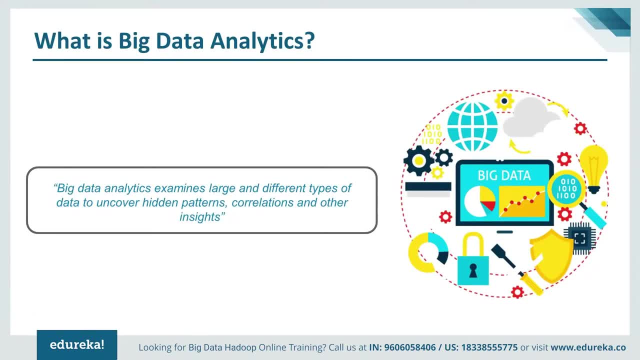 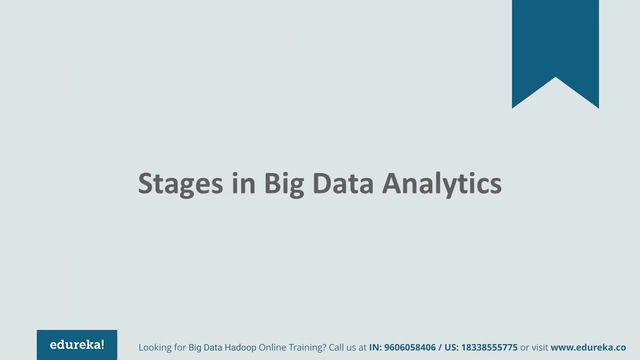 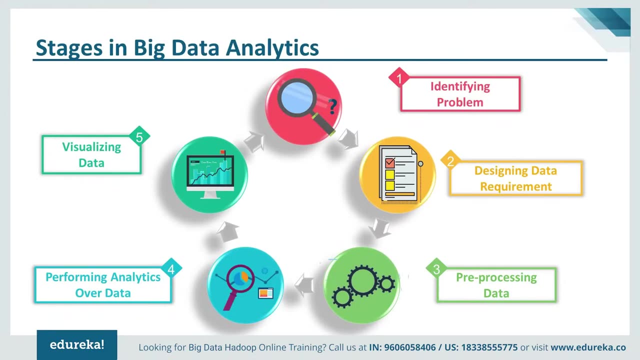 Now let us see and explore What are the different kind of stages which are involved in this procedure of a big data analytics. So these are the different stages involved in this entire procedure. So the first stage is identifying the problem. So what is our problem that we need to solve? 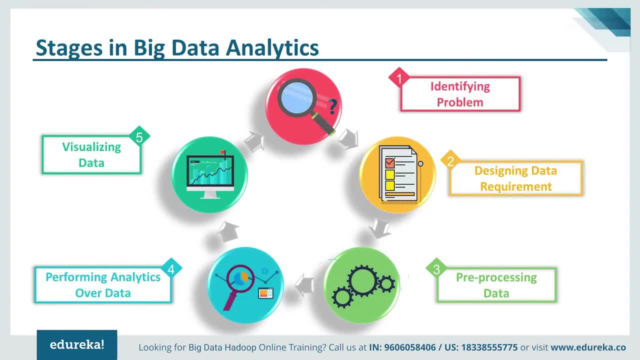 This is the most important step, of course, and this is the first step of the process. The second step is to design our data requirements. So, of course, after identifying the problem, we need to decide what kind of data is required for analyzing this particular problem. 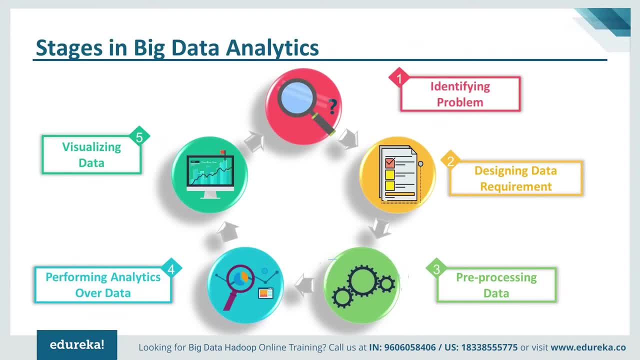 The third step is pre-processing. So in the pre-processing step, basically cleaning of data takes place and you perform some sort of processing. Now, after the processing stage, we come to the fourth stage, which is the analytics stage. So in this stage you would be basically analyzing the process. 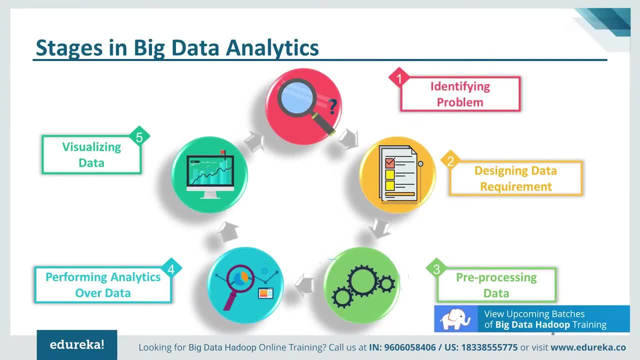 data using various methods. After the analytics stage, we'll move to the final stage, which is data visualization. So in visualization of data Data stage, you will basically visualize the data using tools like Tableau, AngularJS, but the visualization of data will only. 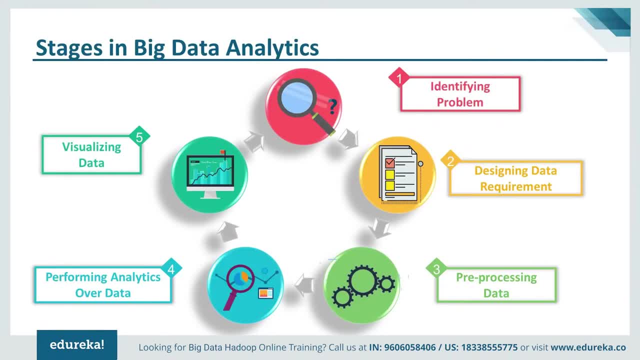 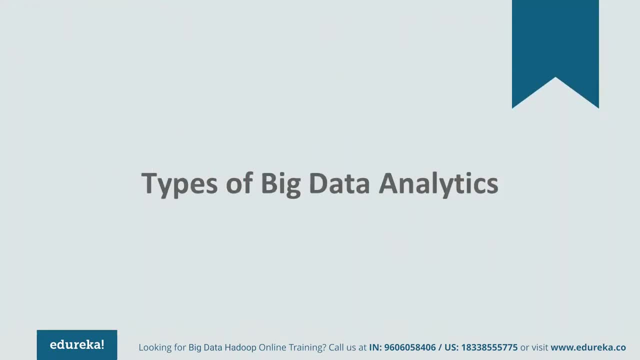 take place in the end. So these are the basic five stages in this entire procedure. Now that you've understood this, let's move forward and understand what are the different types of big data analytics. So there are four basic types. One is descriptive analytics. 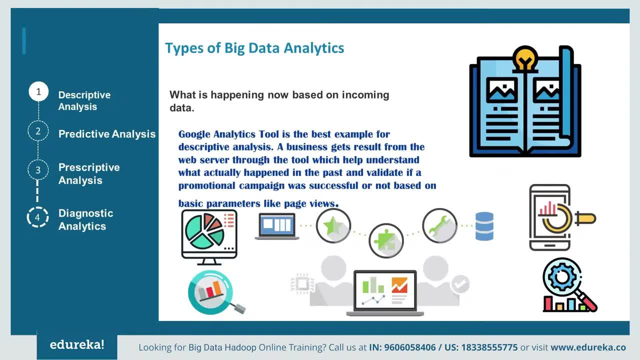 Second is predictive analytics, Third is prescriptive analytics and fourth is diagnostic analytics. So let us understand The first type, which is descriptive analytics. So descriptive analytics basically answers your question: What has happened and how does descriptive analytics answer this question? It uses data aggregation and data mining techniques to provide insight. 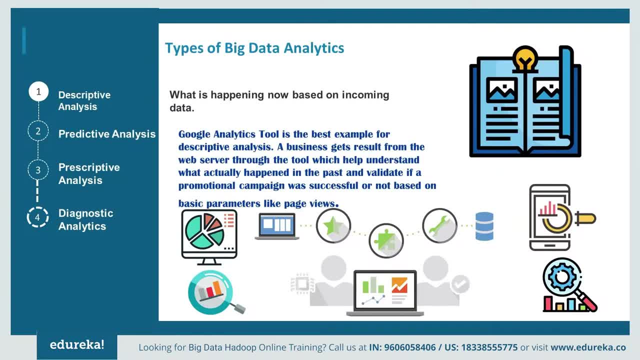 into the past and then it answers what is happening now based on the incoming data. So basically, descriptive analytics is exactly what the name implies: It describes or summarizes the raw data and it makes it something which is interpretable by humans and the past which I just referred in. 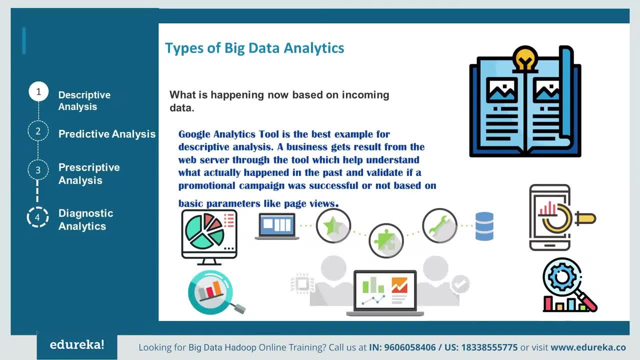 this context Basically can be one minute ago or even a few years back, So the best example that I could cite here for descriptive analytics is basically the Google Analytics tool. So Google Analytics basically is aiding organizations or different businesses by analyzing their results through Google Analytics tool. 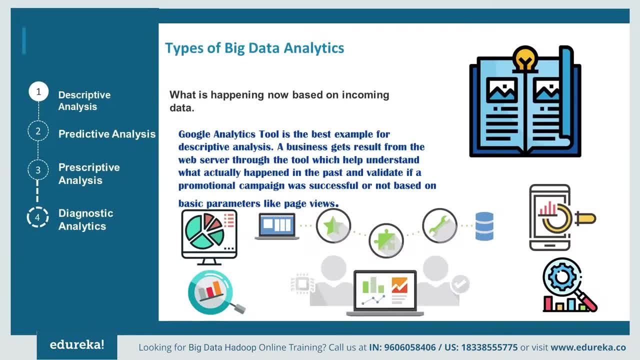 So the outcomes that help the businesses understand what actually has happened in the past, and then they validate if a promotional campaign was successful or not based on the basic parameters like page views. So, basically, descriptive analytics is therefore an important Source to determine what to do next. 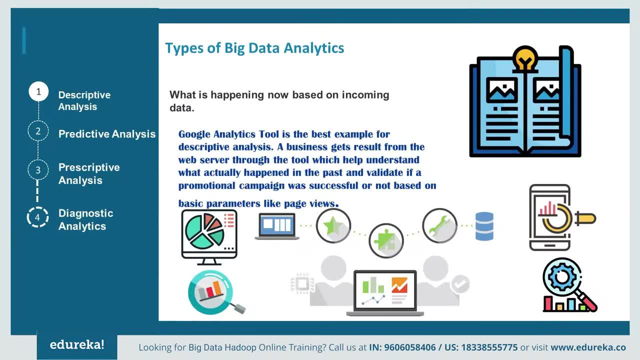 Another example is what we saw earlier in the new generation product, which is Netflix. So Netflix basically uses descriptive analytics, as I told you guys, to find the correlations among the different movies that a subscriber is watching and to improve the recommendation engine. They use historic sales and customer data. 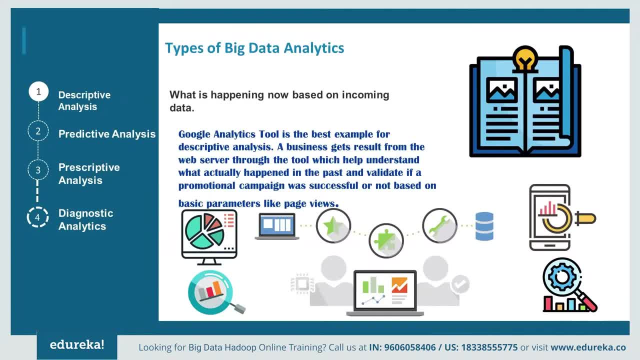 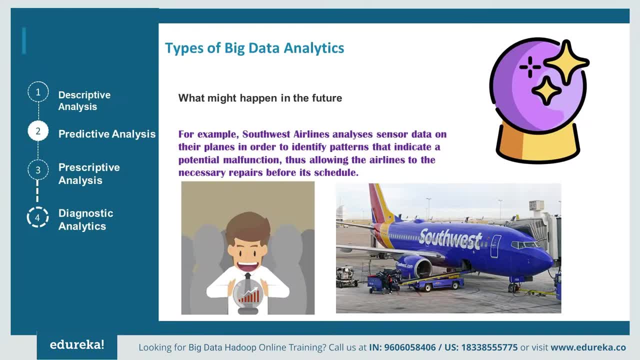 So this is what descriptive analytics is. Now let's move forward to the second type, which is predictive analytics. The second type, which is predictive analytics, basically uses statistical models and forecast techniques To understand the future and answer what could happen. So basically, as the word suggests, it predicts. we are able to understand. 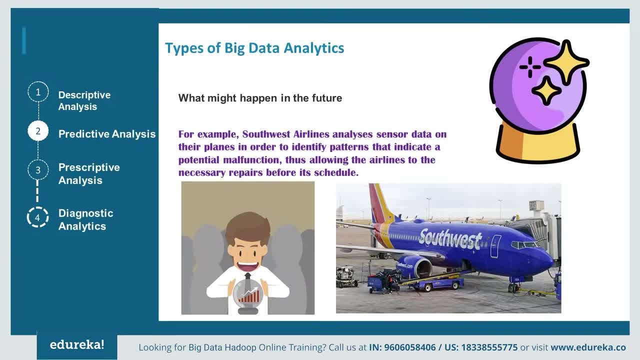 through predictive analytics that what are the different future outcomes? So basically, predictive analytics provides the companies with actionable insights based on the data. So through sensors and other machine-generated data, companies can identify when a malfunction is likely to occur. So then the company can preemptively order paths and make repairs. 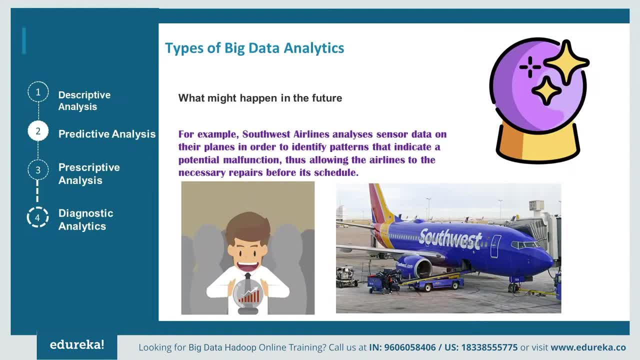 to avoid downtime and losses. So an example of this type Of analytics is the Southwest Airlines. So Southwest analyzes their sensor data on the planes to identify the potential malfunctions or safety issues. So basically, this allows the airline to address the possible problems and then make repairs without interrupting the flights or putting 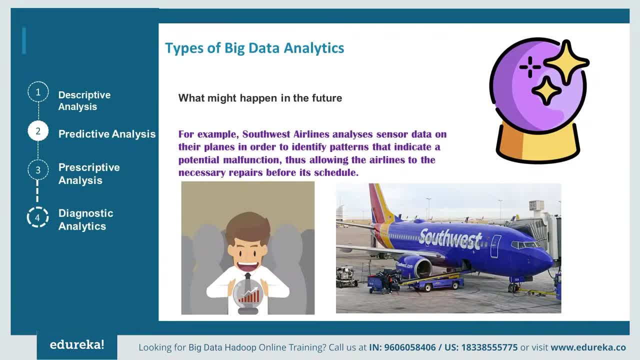 the passengers in danger. So this is a very great use of, you know, predictive analytics to how basically reduce their downtime and losses and as well, as you know, prevent delays and various other factors like accidents. So now let's move forward to the third reason, which is 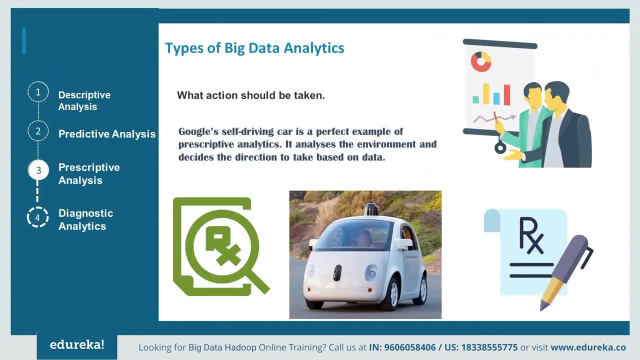 prescriptive analytics. Prescriptive analytics uses optimization and simulation algorithms to advise on the possible outcomes and answer the question: What should we do? So, basically, it allows the users to prescribe a number of different possible actions and then guide them towards a solution. So, in a nutshell, these analytics are all about providing advice. 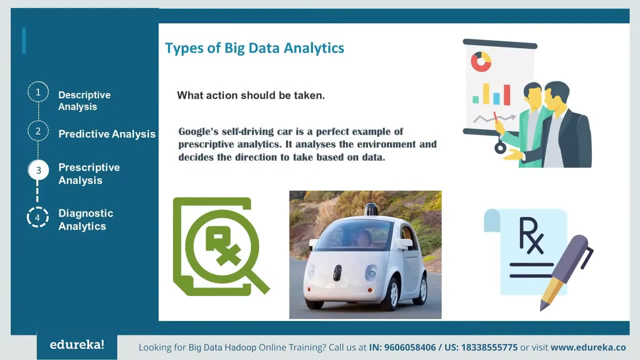 So, prescriptive analytics, they use, you know, a combination of techniques and tools such as business rules, algorithms, machine learning and computational modeling procedures. So then, these techniques are applied against input from many different data sets, including historical and transactional data, real-time data feeds and then big data. 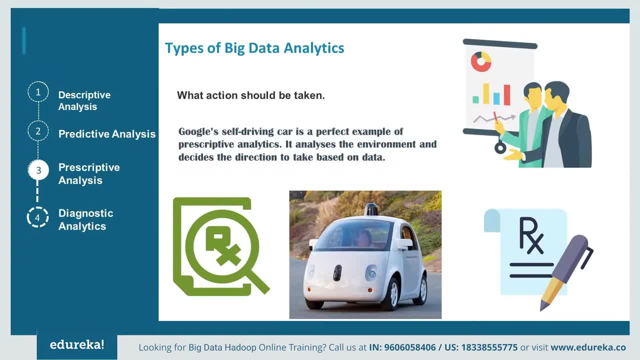 So these analytics go beyond descriptive and predictive analytics by recommending one or more possible courses of action, and the best example for this is the Google self-driving car. This example also we have already seen in the new generation product section. So basically, Google self-driving car analyzes the environment and 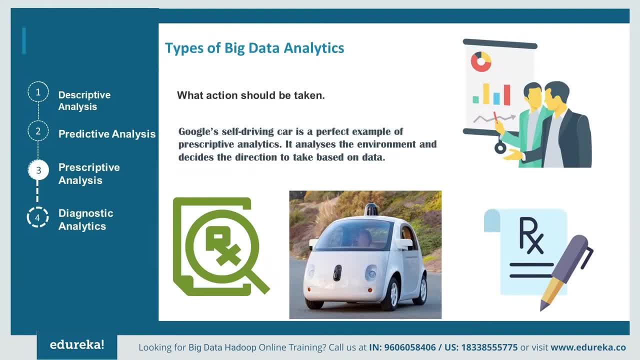 then decides the direction to take Based on the data. So it decides whether to slow down or speed up, to change the lanes or not, to take a long cut to avoid traffic or prefer short routes, etc. So in this way it functions just like a human driver, by using data. 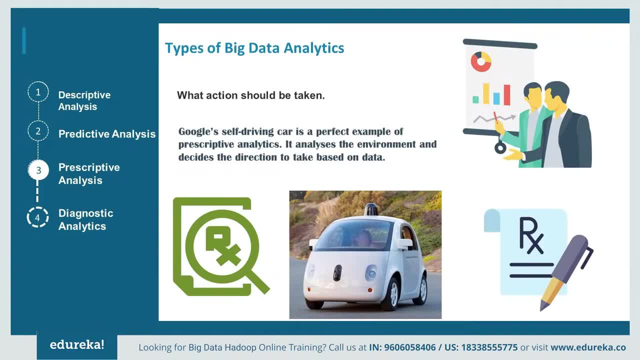 analytics at scale. Now, prescriptive analytics is a little complex type of analytics and it is not yet adopted by all the companies, but when implemented correctly, they can have a large impact on how the businesses make their decisions. So now let's move on to our last type, which is diagnostic analytics. 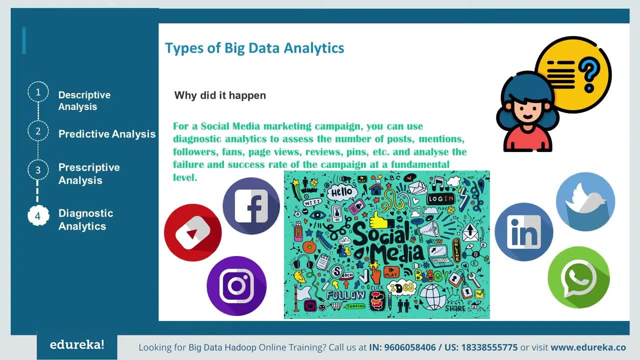 So diagnostic analytics Is used to determine why something happened in the past. So it is characterized by techniques like drill down, data discovery, data mining and correlations. So diagnostic analytics, It takes a deeper look at the data to understand the root cause of the events. 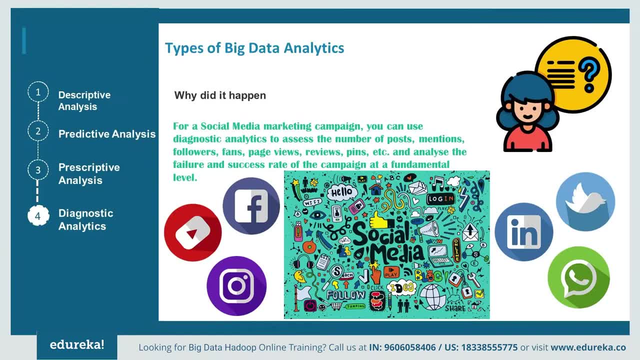 It is helpful in determining what kind of factors and events contributed to a particular outcome. So mostly it uses probabilities, likelihoods and the distribution of data for the analysis. So, for example, in a time series data of sales, diagnostic analytics would help you to understand why the sales of a company has decreased. 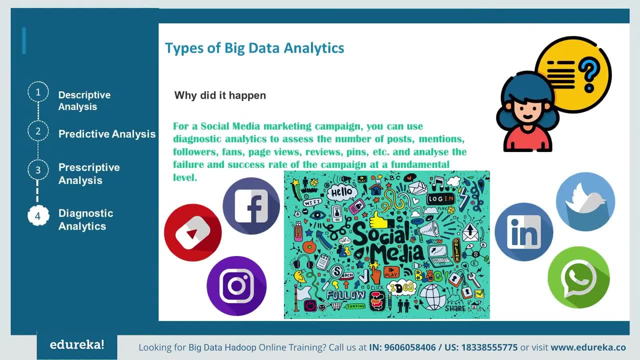 or increase for a particular year, and so on. So examples for diagnostic analytics could be a social media marketing campaign, So you can use diagnostic analytics to assess the number of posts, mentions, followers, fans page views, reviews, pins, etc. So, and then you can analyze the failure and the success rate of a 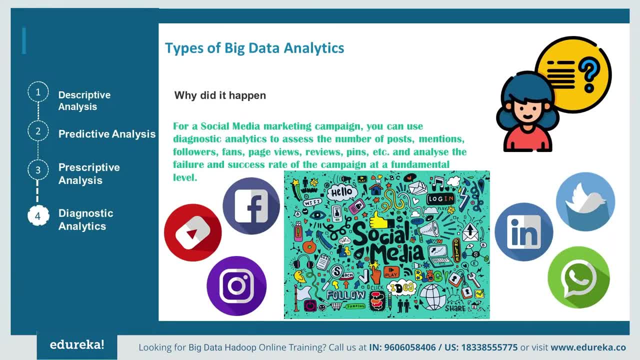 campaign at a fundamental level. So, therefore, they can be thousands of online mentions that can be distilled into a single view to see what worked in your past Campaigns and what did not. So, now that we have seen all the four types, I hope that you've understood the different examples of all the 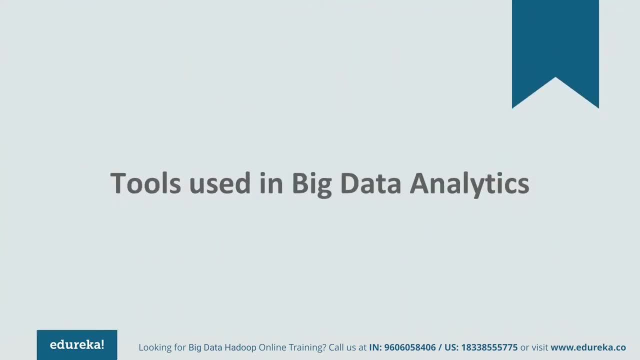 four types and the difference between them. Now let's move forward and have a look at the tools which are required for big data analytics. So these are some of the tools that I have listed down here. So there are more such tools which are used for big data analytics. 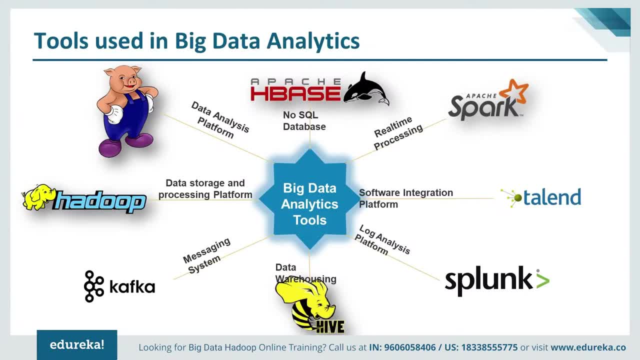 but let's explore the ones which I have mentioned over here. So let me name them: Hadoop, big Apache, edgebase, Apache, spa, Talent, Splunk, Apache, Hive, Kafka. So now let me start with the first one, which is Hadoop. So Hadoop is basically a framework that allows you to store big data. 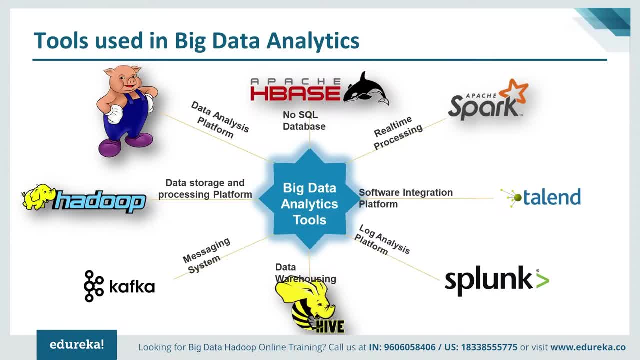 in a distributed fashion so that you can process it Apparently. Apache big is a platform that is majorly used for analyzing large data sets and then represent these data sets as data flows. So basically, pig is used for scripting and the language is pig- Latin. now coming to Kafka. 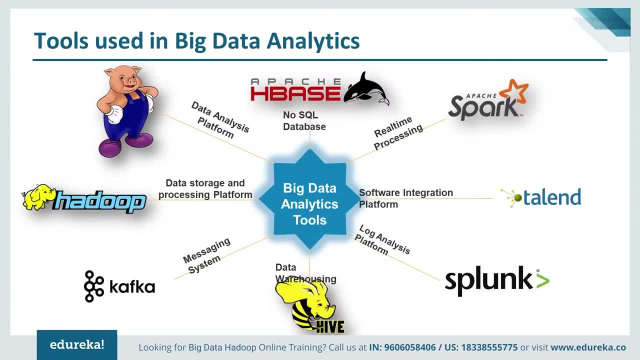 So Kafka is a messaging system. Now, guys, what is a messaging system? A messaging system is basically something which is responsible for transferring data from one application to another, so the applications can focus on the data and they do not need to worry about how to share. 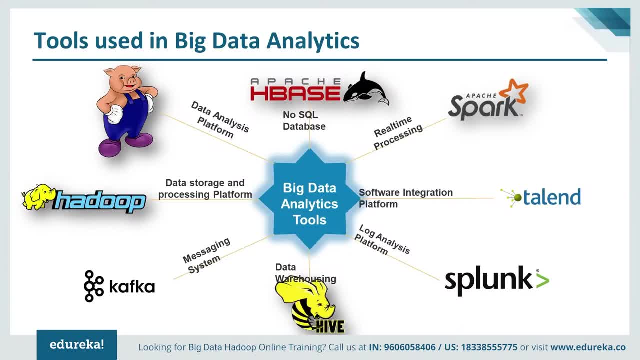 it. So this is what Kafka does. now coming to Apache Hive. now Apache Hive is a data warehousing tool, So it allows us to perform big data analytics using Hive query language, which is similar to sequel. coming to Splunk: So Splunk is a log analysis tool. 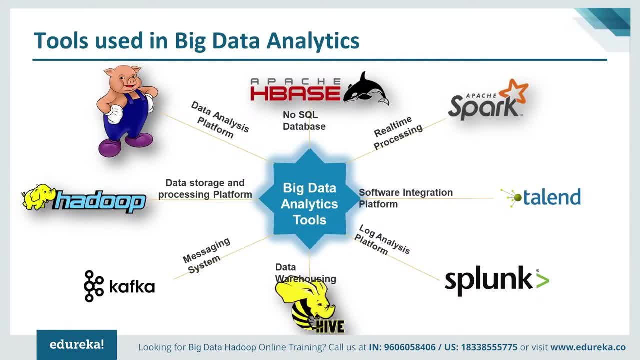 Now, what are logs? So logs are generated on computing as well as non-computing devices, and they are stored in a particular location or directory, So they contain details about every single transaction or operation that you guys have made. So next is talent. talent is an open-source software integration. 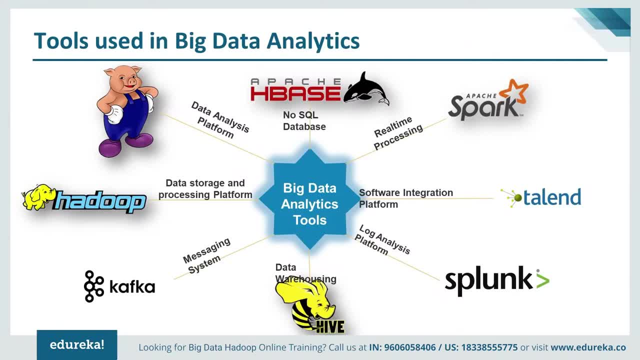 platform, which helps you to analyze effortlessly and then turn the data into business insights. So it helps the company in taking real-time decisions and become more data-driven. next is Apache spark. So Apache spark is an in-memory data processing engine that allows us to efficiently execute streaming. 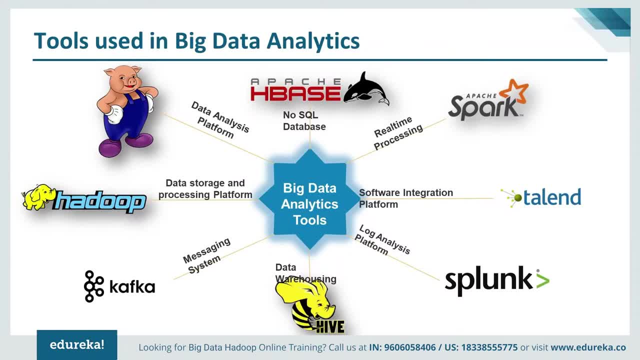 Machine learning and SQL workloads, and it requires fast iterative access to data sets. So, basically, it is used for real-time processing. now moving to the last one, which is Apache HBase. So Apache HBase is a no sequel database that allows you to store. 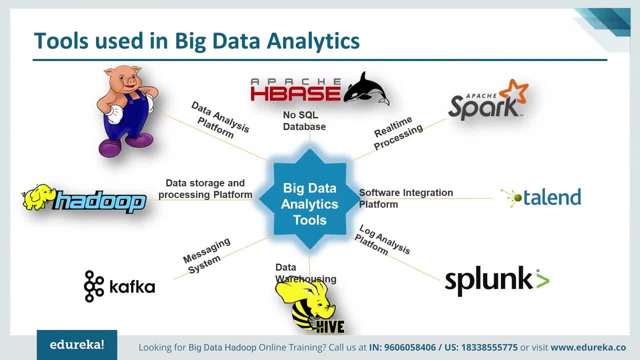 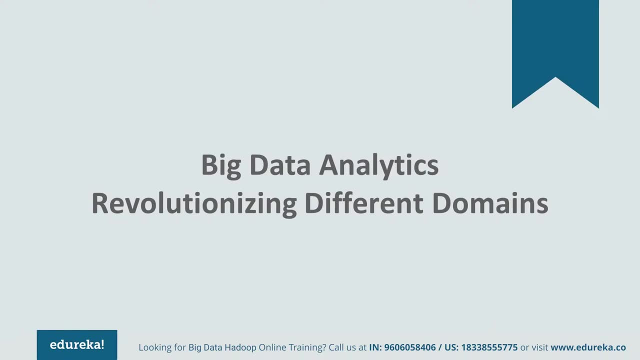 unstructured and semi-structured data with ease and provides real-time read or write access. So these were the tools that I could list down, and I have also told you about the different functions, in brief, that they perform. So now it is move forward and explore the different kind of domains. 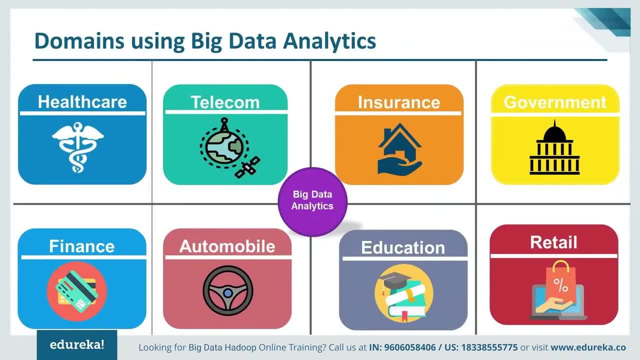 which are, you know, using big data analytics. So these are some of the domains that I've listed out for you guys to understand how they're using big data analytics and how widely it is being used in different kinds of domains. So healthcare- we've already discussed previously- has been using 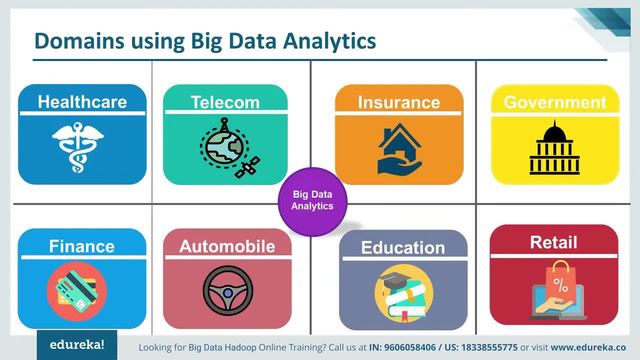 big data analytics, to you know, reduce cost, predict epidemics, avoid preventable diseases and then improve the quality of life in general. So one of the most widespread application of big data in healthcare is electronic health records, which is EHRs. I'm sure that most of you must have heard about it. 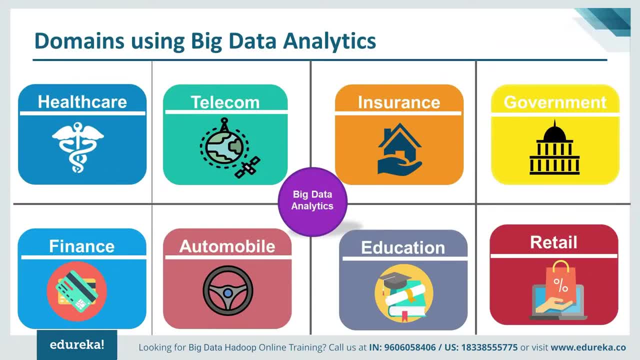 It basically stores the patient's entire data. now coming to telecom industry, So telecom industry is one of the most significant contributors to big data. So telecom industry basically analyzes all our call data records in real time and then they identify fraudulent behavior and acts on them immediately. 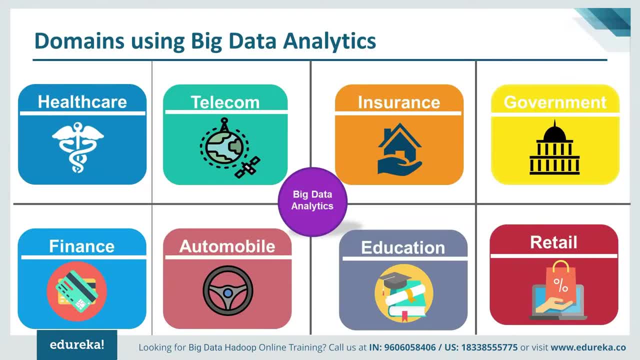 Now the marketing division of telecom industry. It basically modifies their campaign to better target its customers and then use these insights, Which are Are gained by them, to develop new products and services coming to insurance companies, for insurance companies. use big data analytics for risk assessment, fraud detection, marketing customer insights. 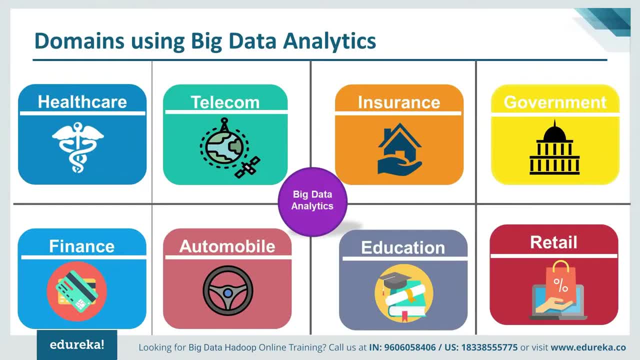 customer experience and much more. now governments across the world are also adopting big data analytics. the Indian government, for example, had used big data analytics to get an estimate of the trade in the country. So the economists used central sales tax invoices for trade between two states to estimate the extent to which the 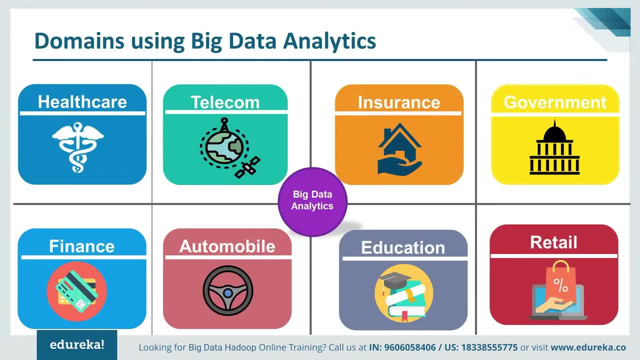 States were trading between each other. coming to banks and financial firms- now banks and financial services firms- They use analytics to differentiate fraudulent interactions from legitimate business transactions. So, by applying analytics and machine learning, they're able to define the normal activity of a user or a customer based on their history. 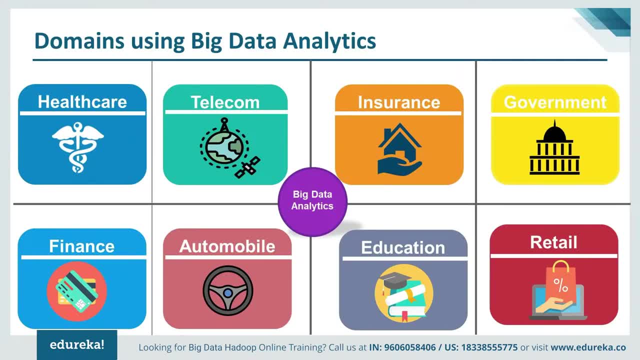 and then distinguish it from the unusual behavior indicating fraud. So then the analysis systems. they suggest immediate action, such as blocking the irregular transactions, which stop the fraud Before it occurs and improves the profitability. now moving on to the next domain, which is automobile. So many automobile companies are utilizing big data analytics, and one 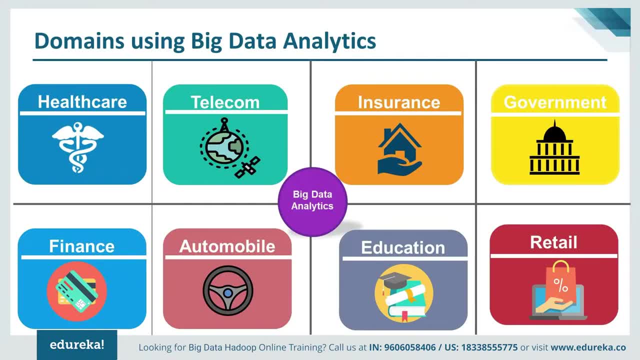 example is Rolls-Royce. So Rolls-Royce embraced big data by fitting hundreds of sensors into its engines and propulsion systems, and these sensors basically record every tiny detail about the operation of these engines and propulsion systems. So then the changes in the data in real time are reported to the 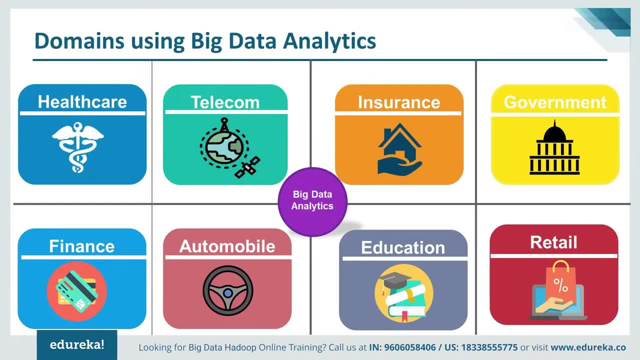 engineers, who will then decide the best course of action, such as scheduling or maintenance or dispatching The engineering teams if the problem arises Now. the next domain is education. So education is one field where big data analytics is very slowly and gradually being adopted, but it is very important that we utilize big 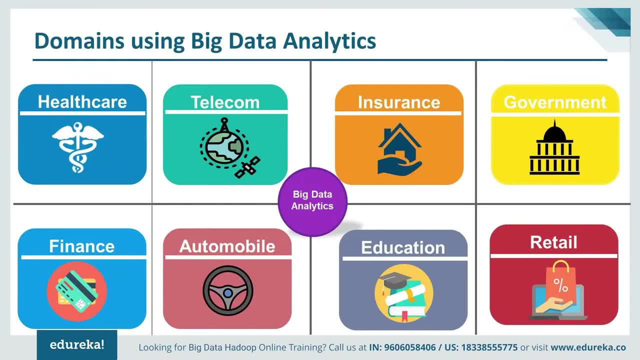 data analytics in this field, because so by opting for big data power technology, you know, as a learning tool instead of the traditional lecture methods, we can enhance the learning of a student as well as it can aid a teacher to basically track the performance in a better manner. 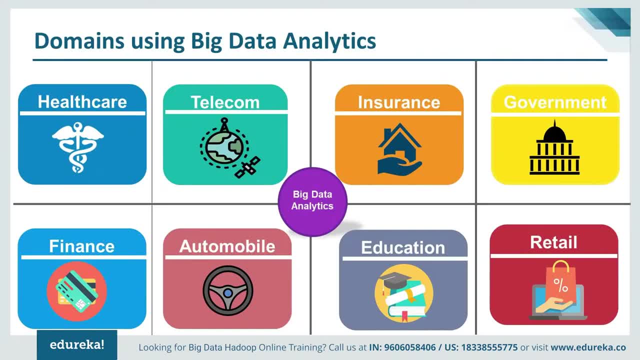 Now coming to the last domain, which is retail. So retail includes both E-commerce and in stores, and they are widely using big data analytics to optimize their business strategies. So we already saw that with the example of Amazon. So now that we've explored the various domains, let me show you the 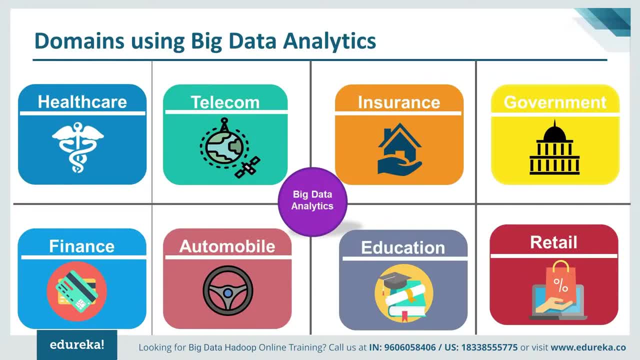 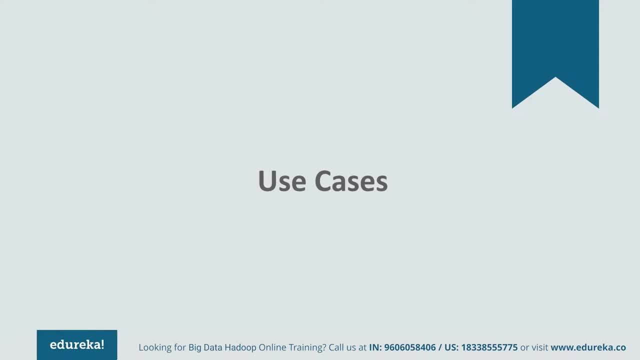 use cases that I have taken here to explain you about how big data analytics is widely being used. So I've taken two such use cases here. So the first use case is of Starbucks. So the leading coffeehouse chain makes use of behavioral analytics by 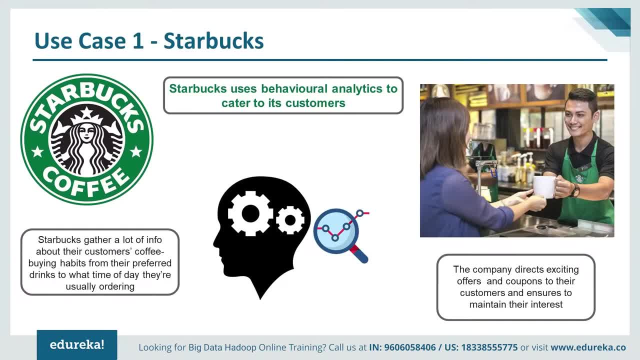 collecting the data On its customers purchasing habits in order to send personalized ads and coupon offers to the customers mobile phones. So the company also identifies trends indicating whether the customers are losing interest in their product, and then they direct offers specifically to those customers in order to regenerate their interest. 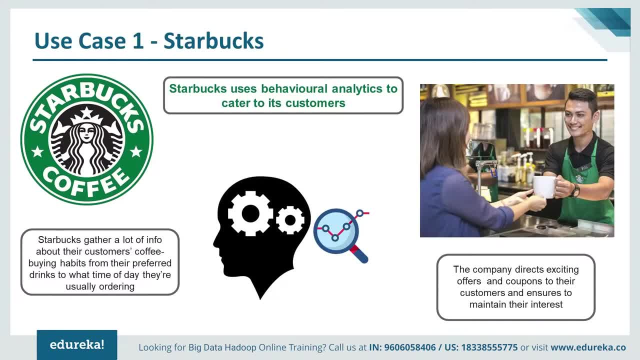 So I came across this article by Forbes, which reported how Starbucks made use of big data to analyze the preferences of their customers to enhance and personalize their experience. So they analyzed, you know every members coffee buying habits, along with their preferred drinks, To what time of the day they are usually ordering. 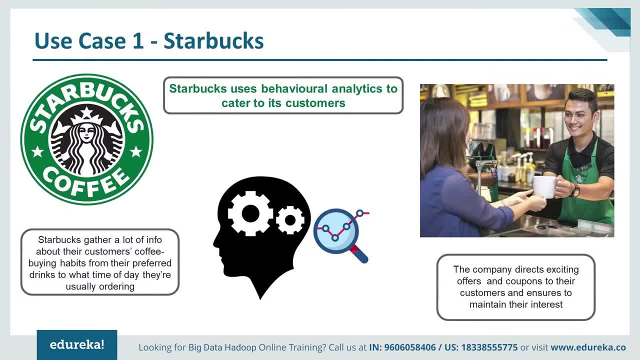 So, even when people visit a new Starbucks location, that stores point-of-sale system is able to identify the customer through their smartphone and then the barista gives them their preferred order. So, in addition, based on ordering preferences, their app, which is a Starbucks app, will suggest new products that the customers might be. 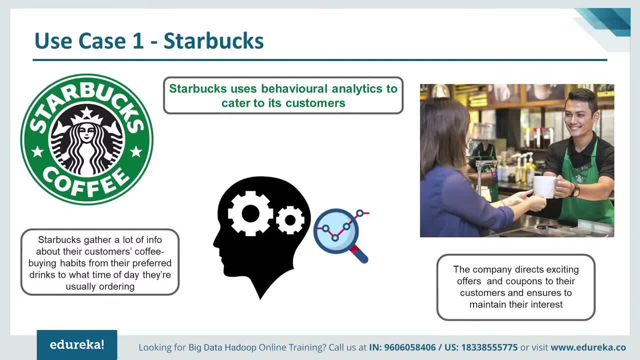 interested in trying. So this is how Starbucks is basically optimizing their business strategies and improving and basically increasing their customer base. Now let's move on and see what is the second Use case that I want to share with you guys. The second use case is of P&G, Procter & Gamble. 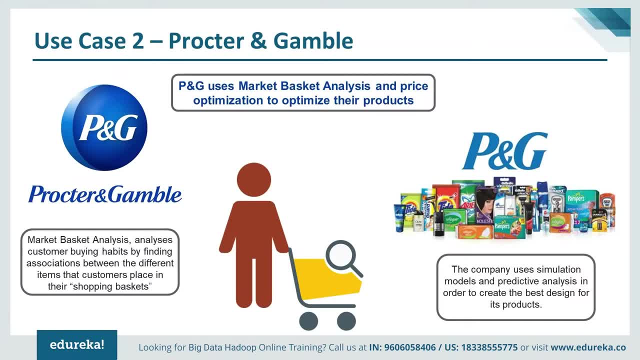 So Procter & Gamble uses market basket analysis and price optimization to optimize their products. So market basket analysis analyzes customer buying habits by finding associations between the different items that the customers place in their shopping baskets. So this is what exactly market basket analysis does. 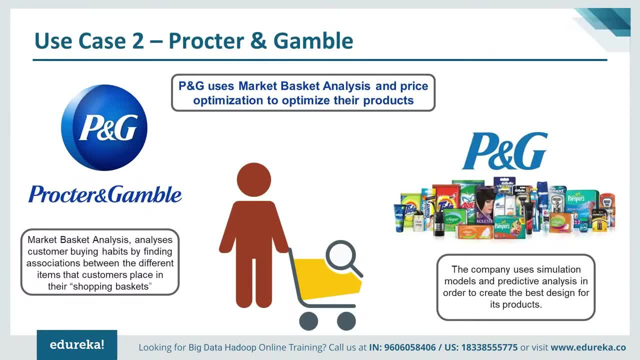 So, apart from this, market basket analysis may be performed on the retail data of customer transactions at your store. So stores- Target, Walmart, etc. That they use market basket analysis to basically increase their sales and marketing. So you can then use the results to plan marketing and advertise your. 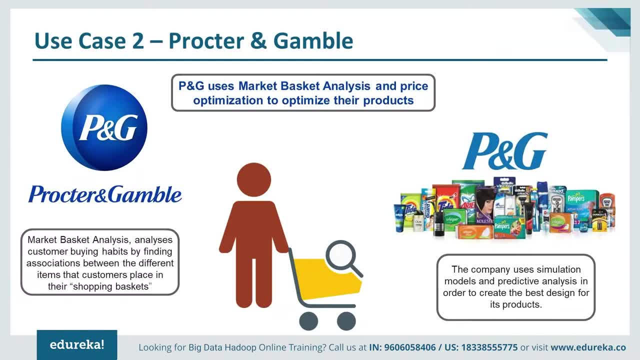 strategies or even design a new catalog. So, for instance, market basket analysis may help you design different store layouts. In one strategy, items that are frequently purchased together can be placed in close proximity to further encourage the combined sales of such items. So example: I'm going to a store. 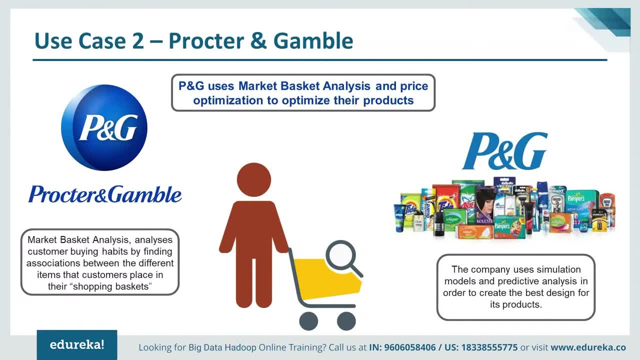 I want to buy bread, Then I also, you know, site butter, So I will want to buy butter as well. So that's how you know. stores optimize their sales. So they place all these products like butter, bread, milk, eggs- in close proximity, because they know when a customer comes to buy bread. they. 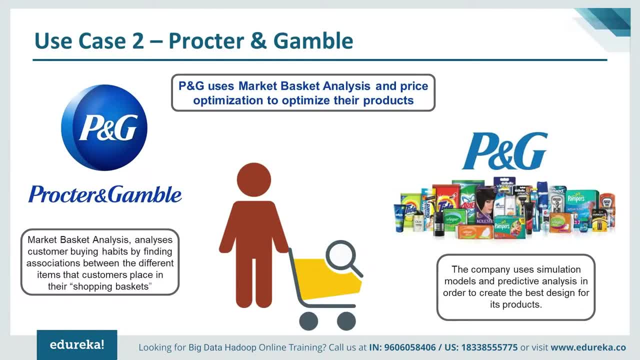 might also want to buy butter or milk or eggs. All right, So this is one such examples. So how P&G basically utilizes it is: the company uses simulation models and predictive analytics in order to create the best design for its products. So it creates and sorts through thousands of iterations in order to 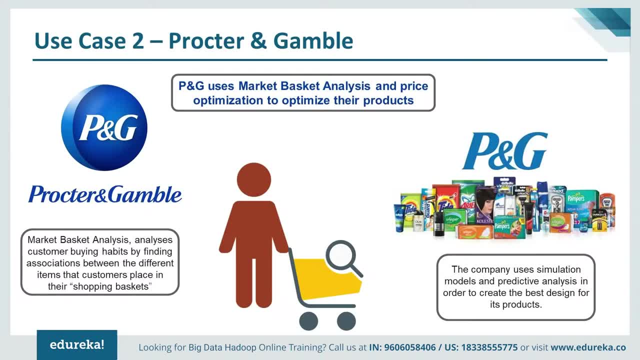 develop the best design, for example, for a disposable diaper, and then they use predictive analytics to determine how moisture affects fragrance molecules in a dish, So so that the right amount of fragrance comes out at the right time during the dishwashing process. I mean so we can't even imagine that a simple product like a dish soap 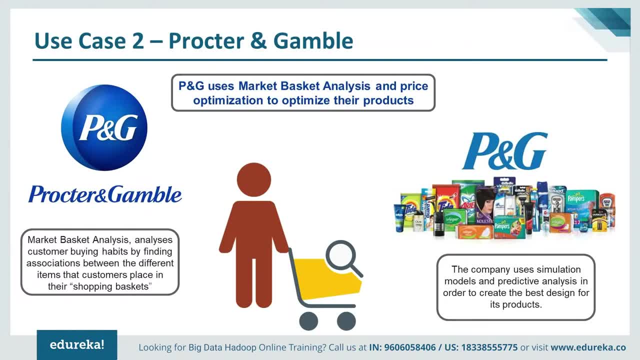 also has so much thought process behind it and also has so much strategies or, you know, analytics applied behind it. So I hope that you guys found both these you know use cases really interesting, and how more such companies, By utilizing big data analytics in a more proficient manner in order to 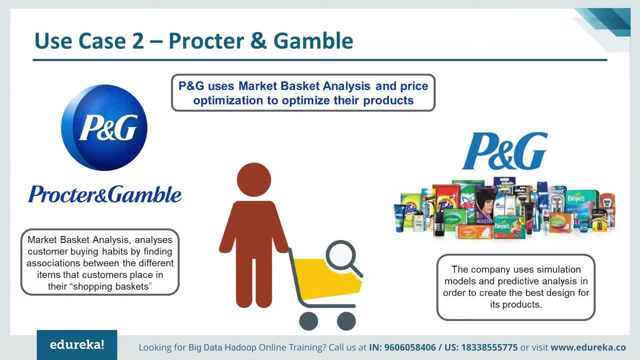 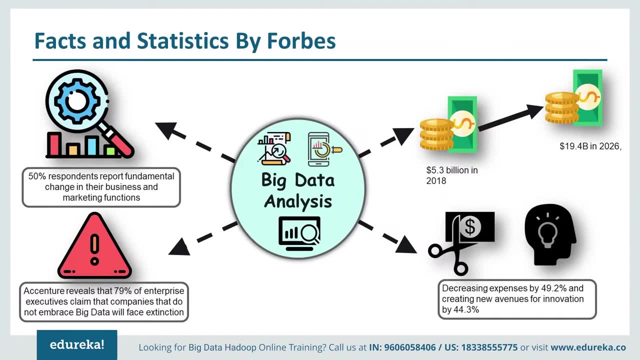 basically increase their sales and marketing. So now let's move forward and see the next one, which is facts and statistics by Forbes. So I've collected some of these, so for which I found really interesting and I wanted to share with you guys. So the first one here basically states that nearly 50% of respondents to 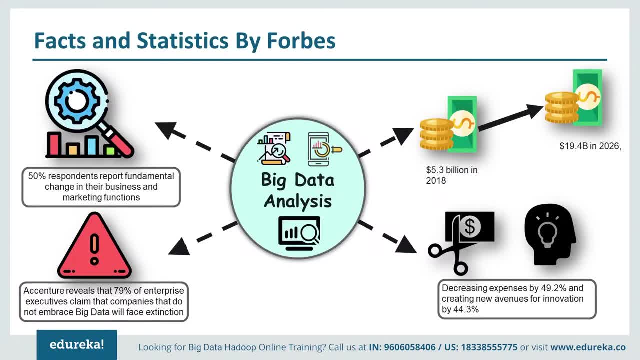 a recent McKinsey analytics survey, say that analytics and big data have fundamentally changed business practices in their sales and marketing functions. So we also have seen examples of this by, you know, like by Starbucks, of PNG, of Amazon. So these are such companies which are responding to such surveys. 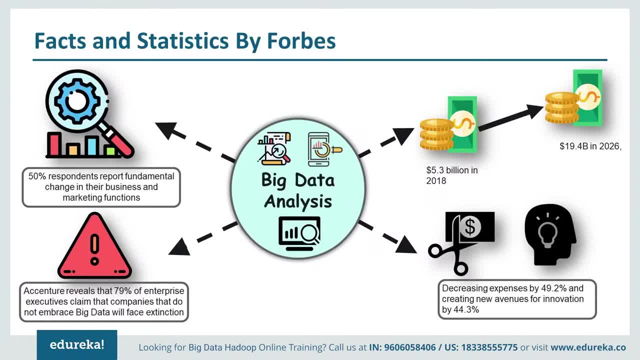 Now the next one is showing that how big data applications and analytics is projected to grow from about 5.3 billion dollars in 2018 to 19.4 billion dollars in 2026, which attains about a compound aggregate of 15.49%. 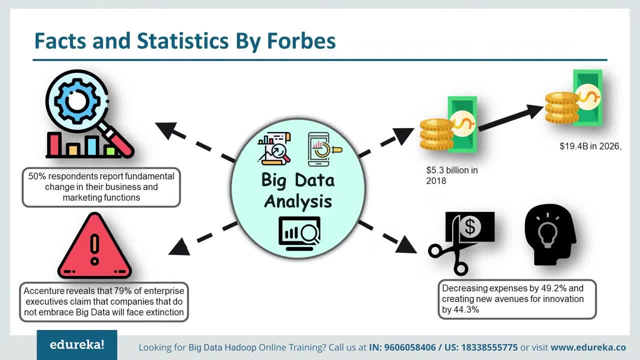 So the next one here is an extremely important fact Or a stat which I found out, and it is basically an eye-opener. So, according to an Accenture study, 79% of Enterprise executives agree that companies that do not embrace big data will lose their competitive. 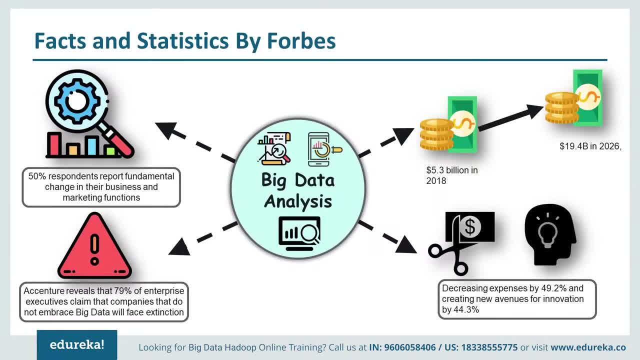 position and could face extinction even more. 83% have pursued big data projects to seize a competitive edge. So this very fact, guys, tells you that how important this field is, and if your particular organization or company is not adopting big data analytics in the future, it is going to lead to Obsolation. 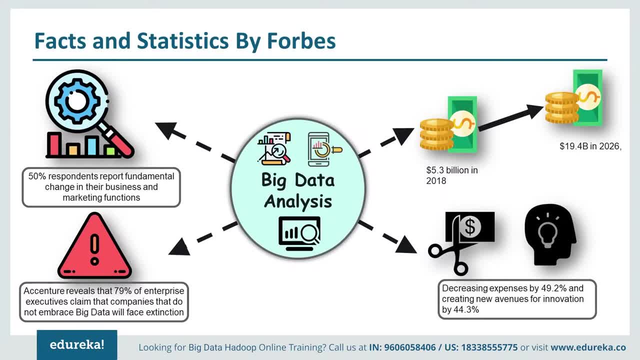 So now let's see which is the last fact that I have stated here. So, according to new Vantage Venture Partners, big data is delivering the most value to enterprises by decreasing their expenses by about 49.2% and creating new avenues for innovation by about 44.3%. an example of both of 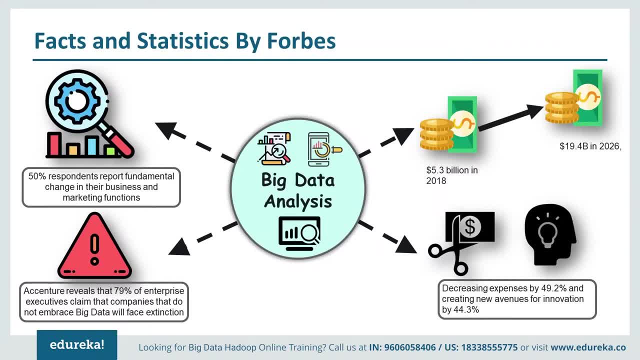 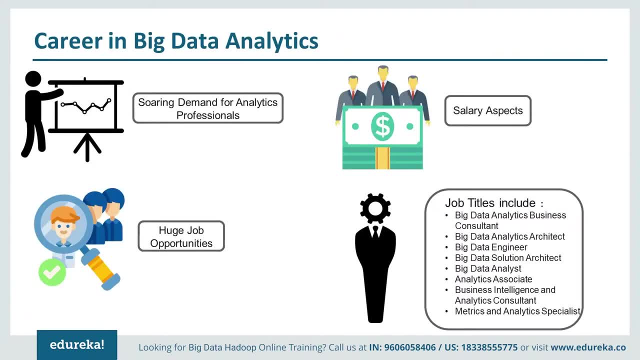 these facts We saw in new generation- why we need big data analytics section, where we spoke about cost reduction as well as new generation products. This is an example of that. So now let's move forward and look at the career prospects in big data analytics. 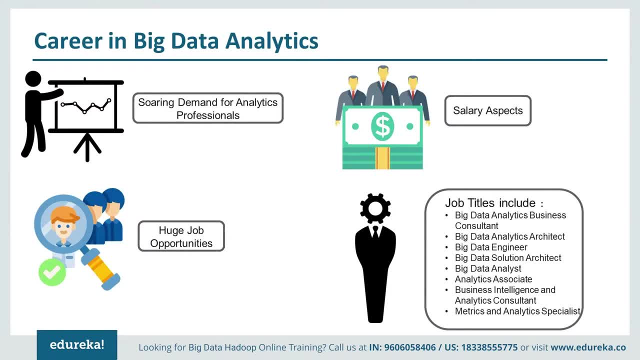 So the first one here that I've stated here is there is a soaring demand for analytics professional. So technology professionals who are experienced in big data analytics are in high demand as organizations are looking for ways to exploit the power of big data. So therefore, there is a soaring demand for analytics professional and 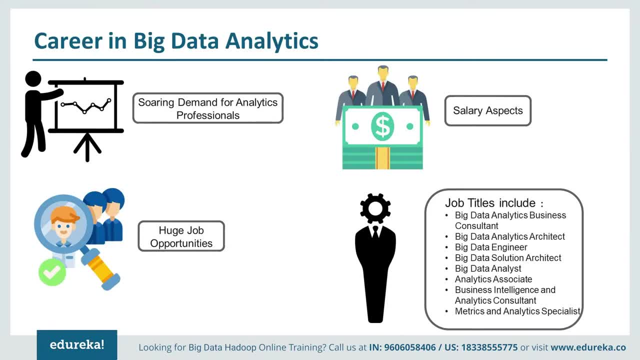 as and when the data is going to grow more, such people will be required to analyze that data. So that leads us to our second point, which is huge job Opportunities. There are more job opportunities in big data management and analytics than there were last year, and many IT professionals are prepared to. 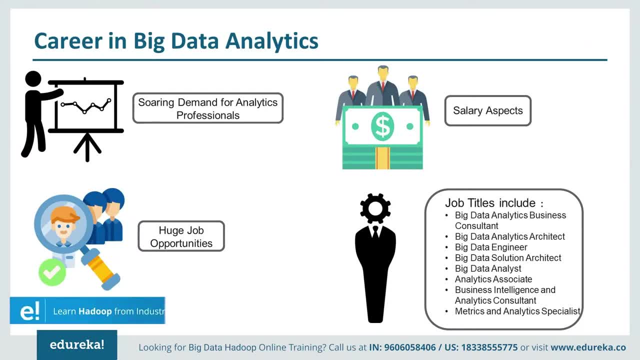 invest time and money for the training. So now that companies under various domains are adopting big data analytics, So there are definitely more huge job opportunities. So now let's see what are the salary aspects. So I think this is one of the most important ones again, because we need 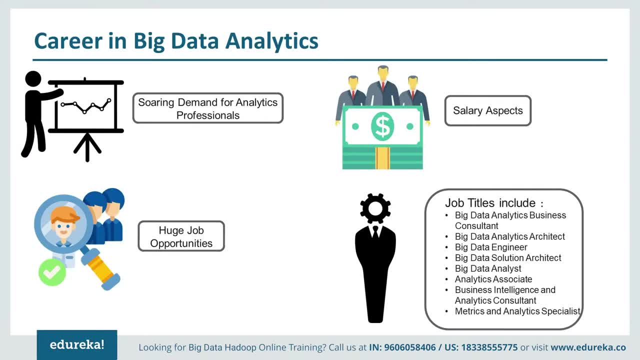 to know that. what kind of salary are we going to draw if you become a big data analytics professional? So six analytics and data Jobs are included in Glassdoor's 50 best jobs in America for the year 2018.. These include data scientist, analytics manager, database administrator. 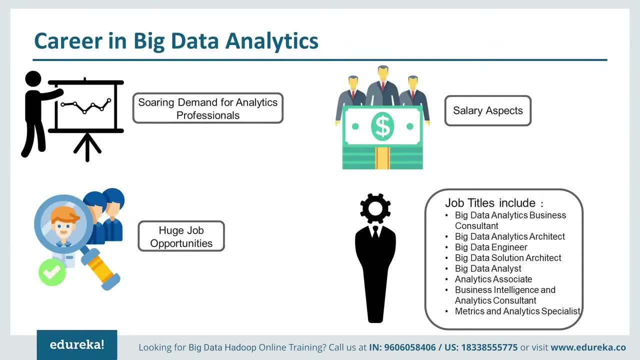 data engineer, data analyst and business intelligence developer, and the average salary of the six analytics jobs that I just stated, along with data science jobs, is about $95,000, which is absolutely amazing, and data scientist has been named the best job in America for about three years running. 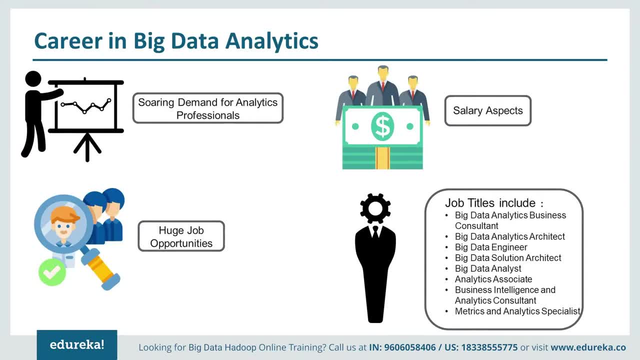 So you guys can see that how great the prospects are in this field and if you guys are interested, then you should definitely learn more about this field and you know who knows that you might be drawing such kind of a salary. So, but in India, the percentage of analytics professionals commanding 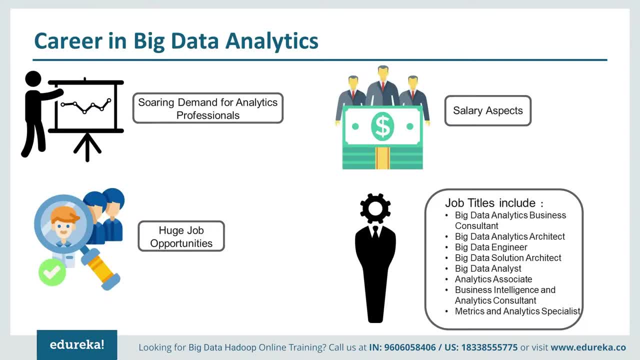 the salaries lesser than 10 lakhs. It has gone lower, which is great. So the percentage of analytics professionals Earning more than 15 lakhs has increased from about 17% in 2016 to 21% in the last year, 2017 and to the current 22.3% in this year 2018.. 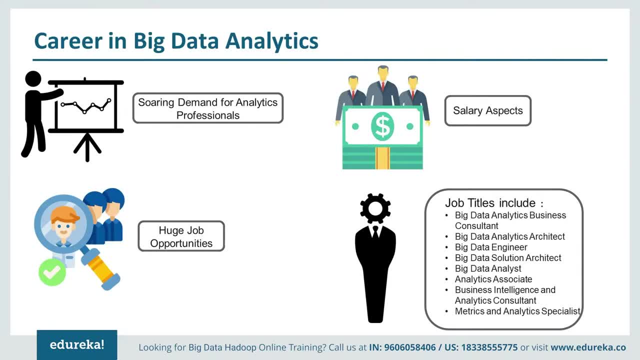 Now let me tell you what kind of job titles are there in this field. So the first one here is big data analytics business consultant. second is big data analytics architect. third is big data engineer. fourth is big data solution architect. fifth is big data analyst. sixth is analytics. 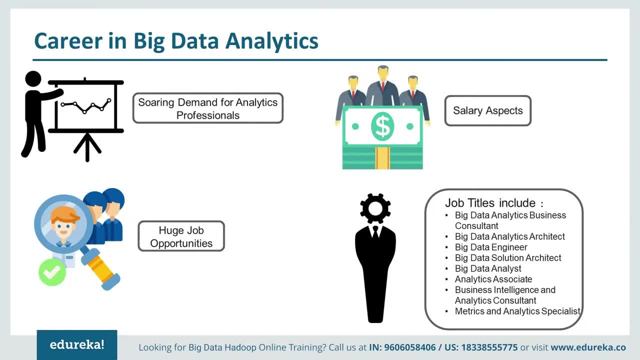 associate. Seventh is business intelligence and analytics consultant and the last one is metrics and analytics specialist. So I've just stated eight over your, so these might be addressed in different names and different. you know job titles and there are more such job titles, I'm sure, so you can explore that. 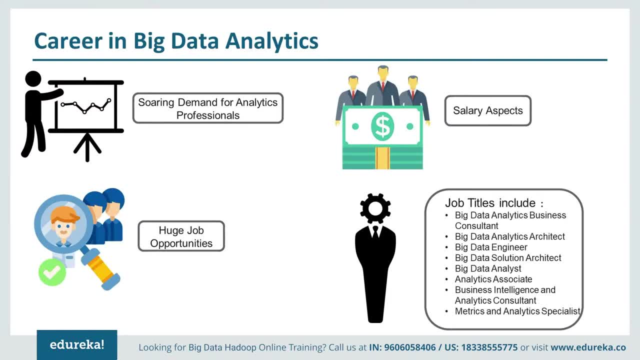 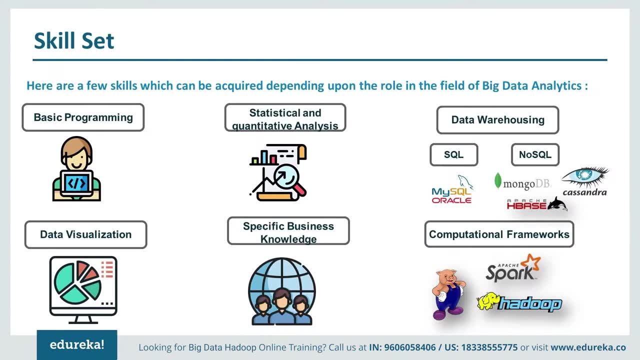 So now let's move on to see what are the skill sets that you require if you want to become an analytics professional. So these are the few skill sets that I've mentioned over here, and there can be more depending on the role that you're going to play, or maybe. 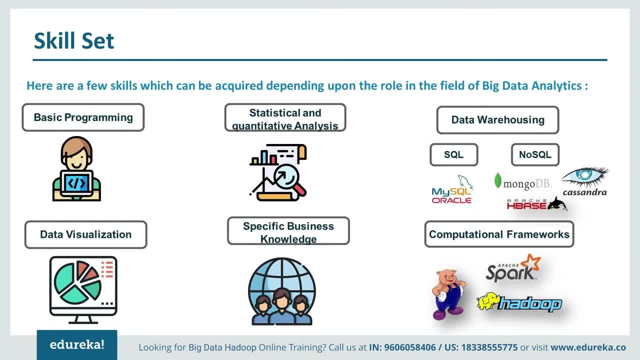 even, you know, restricted to one particular skill set. so depends upon what role are you going to play in this field of big data analytics. So the first one is that I've put down here is basic programming, So you would obviously be expected to know some kind of a general. 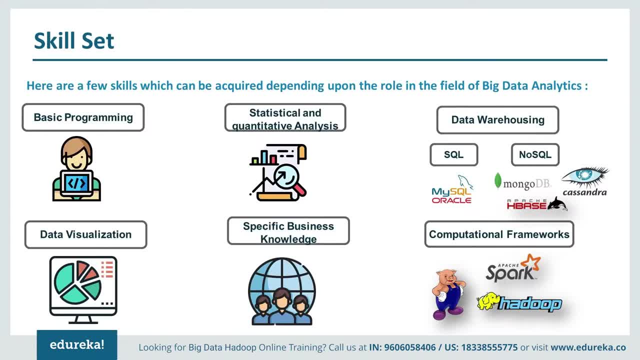 purpose programming language. The second one here is statistical and quantitative analysis. So it is preferable if you know about the statistics and quantitative analysis. now moving on to data warehousing, so knowledge of you know sequel and no sequel, database languages such as my, SQL and no sequel. 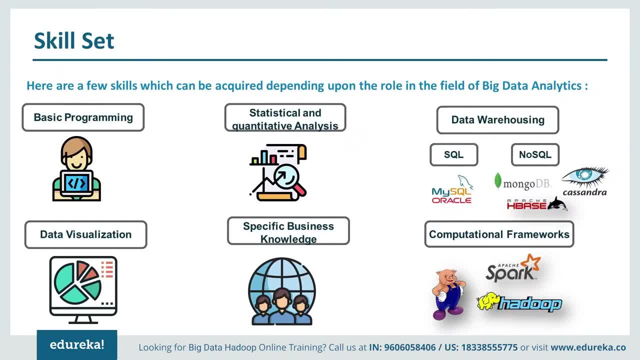 has MongoDB, HBase and Cassandra, So knowing these databases is also very important. The next one is data visualization, which is, I think, one of the most important skill sets which are required, So, as an analytics professional, you should know how to visualize the. 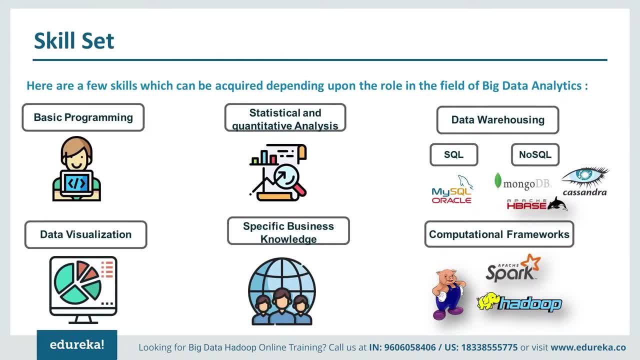 data in order to you know, basically improve your business. So you need to know what kind of trends are going to be there in the data and how it is increasing and what kind of insights this data is going to provide you. So you should be able to visualize the data. 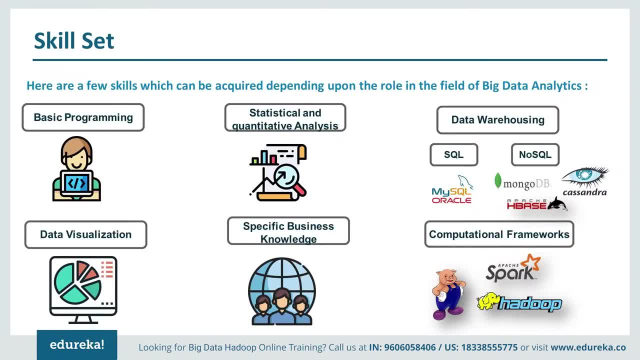 You should be able to understand what the data is indicating. The next one is specific business knowledge. So this is extremely necessary, according to me, because if you're an analytics professional and you don't know what business your company is basically working on and you're not aware about it, you won't be able to. 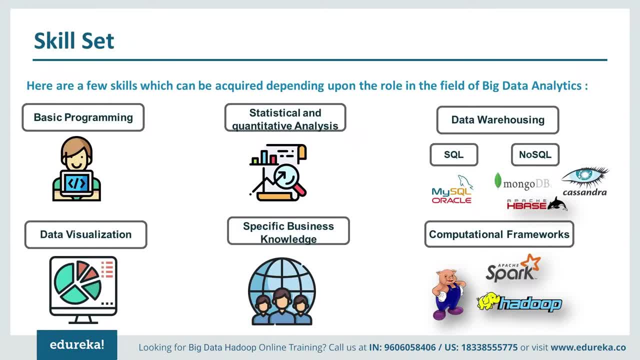 apply your knowledge of analytics to basically increase the sales and marketing of the company. All right, So the business knowledge of a particular company or the area which you're working on is extremely important. The last skill set that I've mentioned over here is computational. 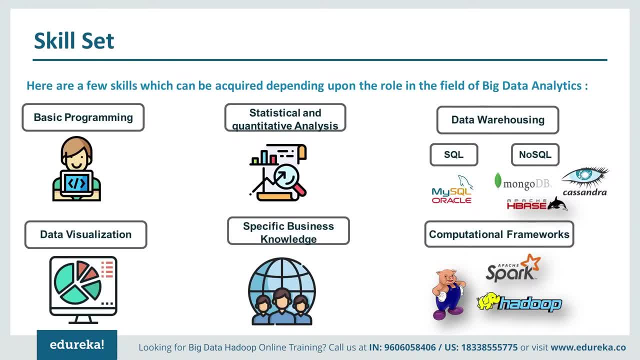 frameworks. So out of the tools that we discussed in the previous section, one is expected to know at least more Then one. So if you know Apache, Spark, Hadoop Pig also- again, that is depending upon the job role that they're going to play- 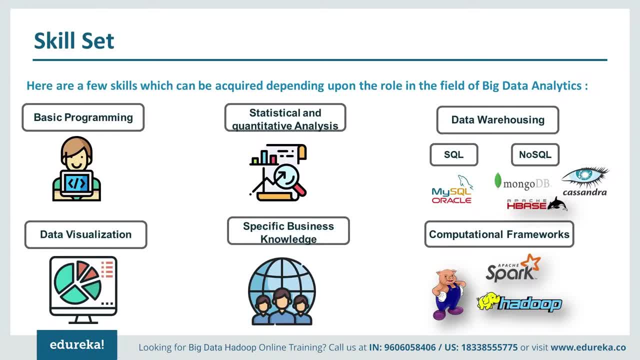 So it is important that you are aware about at least one or more tools which are, you know, required for big data analytics, and one or two such computational frameworks, because it is going to, of course, help you and you will have a basic knowledge about how these tools are used for. 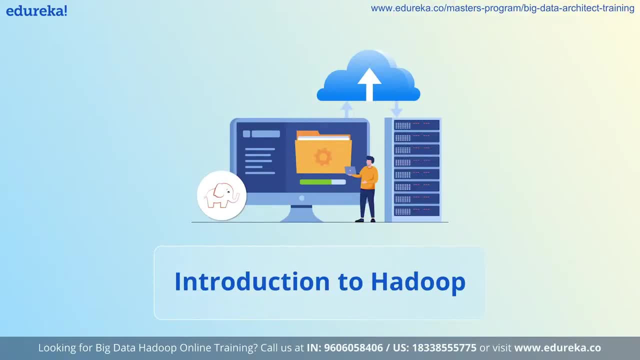 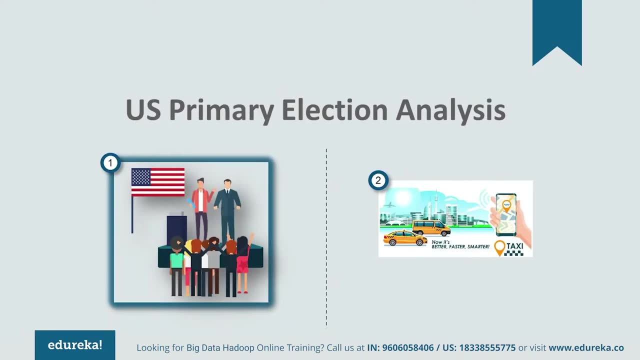 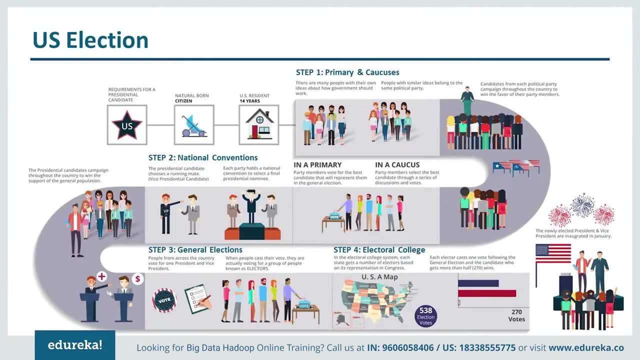 analyzing the data. Let us start with the US primary election use case first. In this use case, we will be discussing about the 2016 primary elections. In the primary elections, the contenders from each party compete against each other to represent his or her own political party in the final. 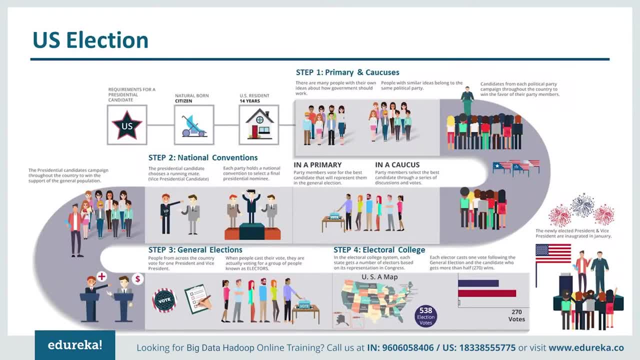 elections. There are two major political parties in the US: the Democrats and Republicans. From the Democrats, the contenders were Hillary Clinton and Bernie Sanders, and out of them, Hillary Clinton won the primary elections, And from the Republicans, the contenders were Donald Trump, Ted Cruz and. a few others. As you already know, Donald Trump was the winner from the Republicans. So now let us assume that you are an analyst already and you have been hired by Donald Trump and he tells you that I want to know what were the different reasons because of which Hillary Clinton won. 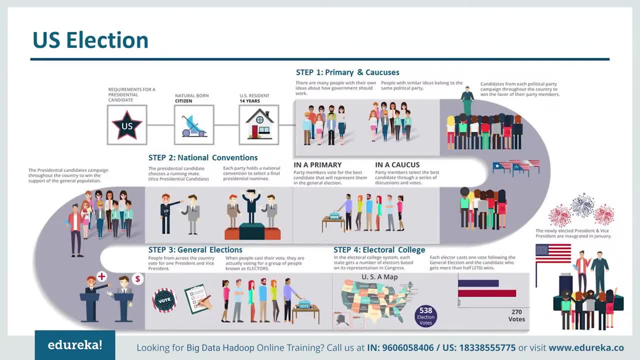 And I want to carry out my upcoming campaigns based on that, so I can win the favor of the people that voted for her. So that was the entire agenda. So this is the task that has been given to you as a data analyst. So what is the task? 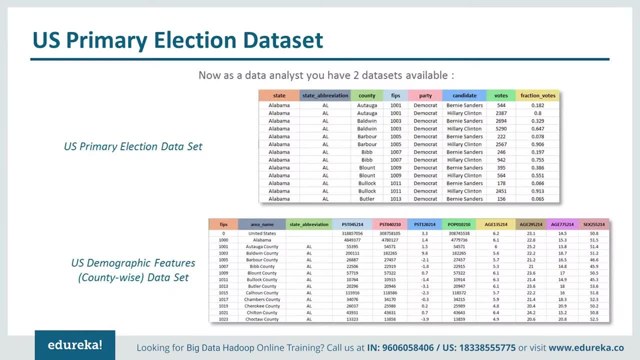 What is the first thing that you will need to do? The first thing you'll do is that you'll ask for data, and you have got two data sets with you, So let us take a look at what this data set contains. So this is our first data set, which is the US primary election data set. 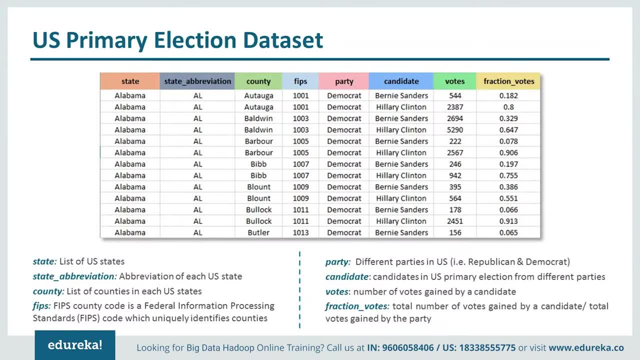 So these are the different fields present in our data set. So the first field is state. So we've got the list of the state of Alabama. The state abbreviation for Alabama is AL. We've got the different counties in Alabama, like Artuga, Baldwin, Barber. 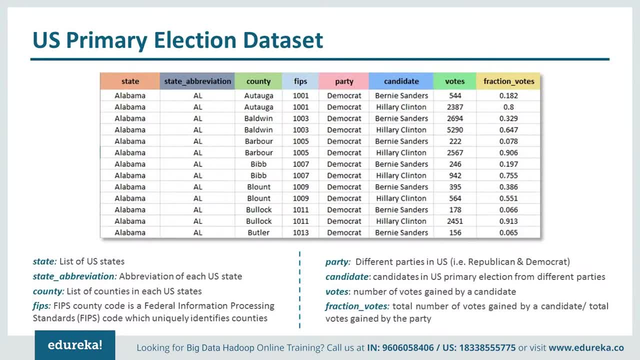 Bibb, Blount, Bullock, Butler, Etc. And then we've got FIPS. Now, FIPS are federal information processing standards code, So this is basically means zip code. Then we've got the party, So which we will be analyzing- the Democrats only because we want to know. 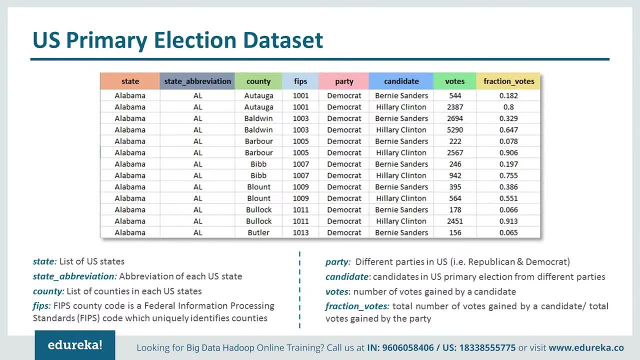 what was the reason for Hillary Clinton's win? So we will be analyzing the Democrats only, and then we've got the candidate And since I told you, there were two candidates, Bernie Sanders and Hillary Clinton, so we've got the name of the candidate here and the number of the 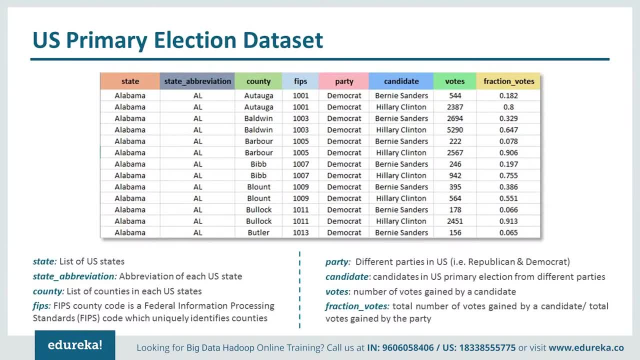 votes each candidate got. So Bernie Sanders got 544 in Artuga County and Hillary Clinton got to 2387 in this field over here represents the fraction of the votes. So if you add these two together you will get a one. So this basically represents the percentage of vote each of the candidates. 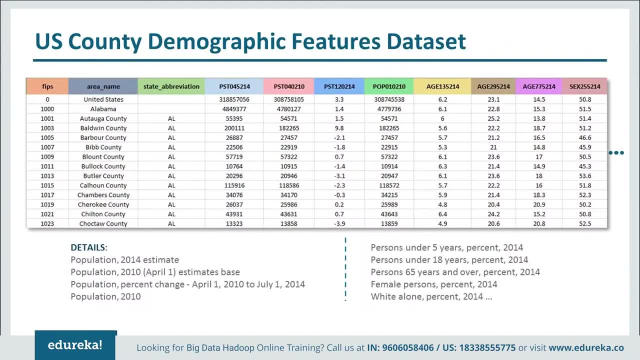 got. So let's take a look at our second data set now. So this data set is the US County demographic features data set. So the first: we will have again FIPS in the area name: Artuga, County, Baldwin and different other counties in Alabama and other. 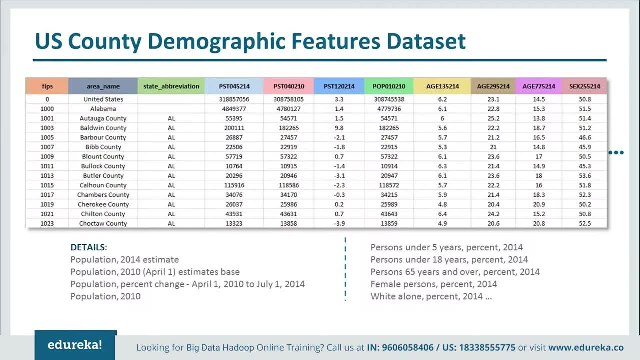 states also the state abbreviation, So here it is only showing Alabama, and the fields that you see here are actually the different features. You won't know what this exactly contains, because it is written in a coded form, But let me give you an example what this data set contains. 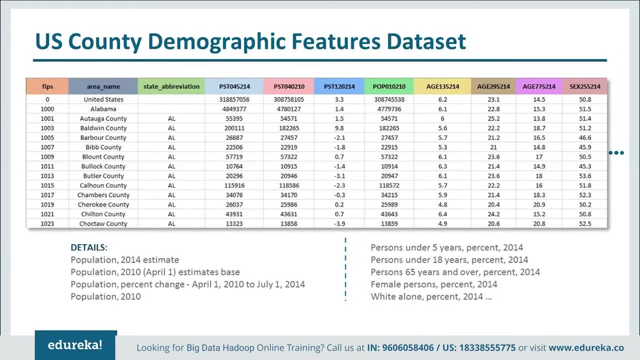 Let me tell you that I'm just showing you a few rows of the data set. This is not the entire data set, So this contains different fields like population In 2014 and 2010, the sex ratio- how many females, males- and then, based on: 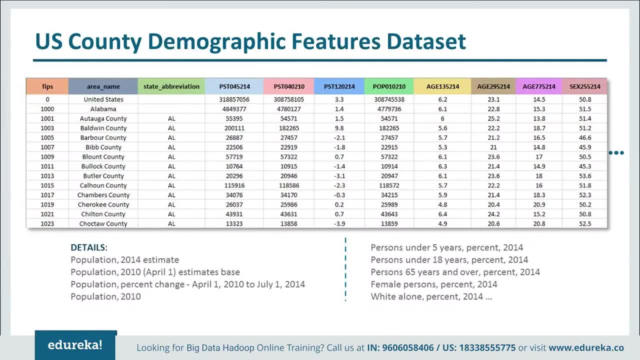 some ethnicity: how many Asians, how many Hispanic, how many black American people, how many black African people? and then there is also based on the age groups: how many infants, how many senior citizens, how many adults? so there are a lot of fields in our data set and this will help us to analyze. 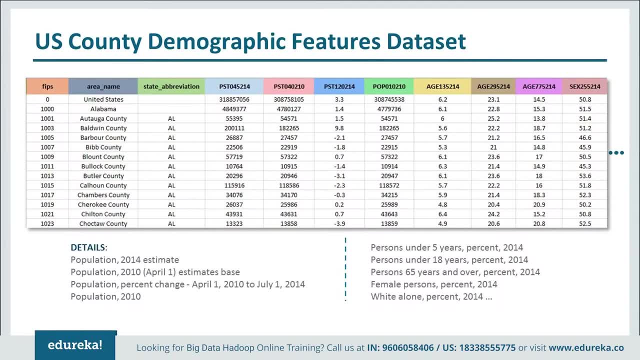 and actually find out what led to the winning of Hillary Clinton. So now you have seen our data That you have to understand your data set, You have to figure out what are the different features or what are the different columns that you are going to use, and you have to think of a. 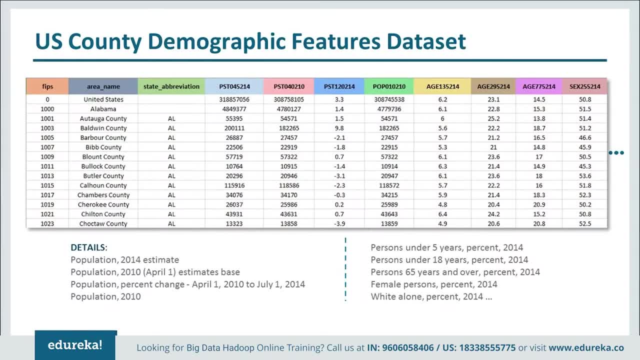 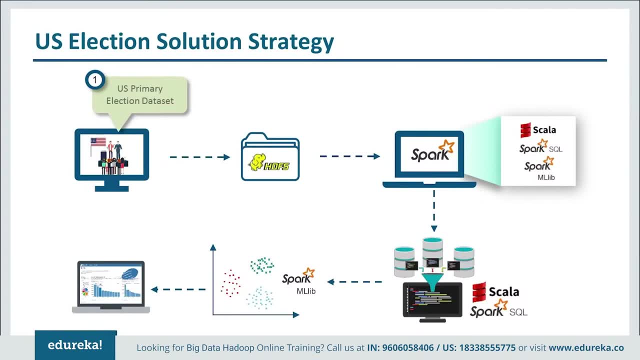 strategy, or think of how you're going to carry out this analysis. So this is the entire solution strategy. So the first thing you will do is that you need a data set, and you've got two data sets with you. The second thing that you'll need to do is to store that data into HDFS. 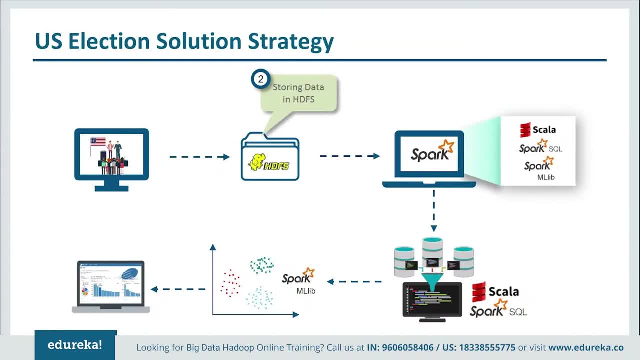 Now HDFS is how to have distributed file system, So you need to store the data. The next step is to process that data using spark components. We will be using spark SQL, spark MLib, Etc. So the next task is to transform that data using spark SQL. transforming here. 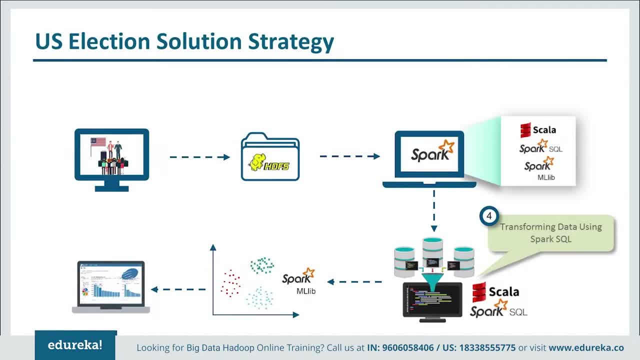 means filtering out the data and the rows and columns that you might need in order to implement or in order to process this. the next step is clustering this data using spark MLib, and for clustering our data, We will be using k-means, and the final step is to visualize. 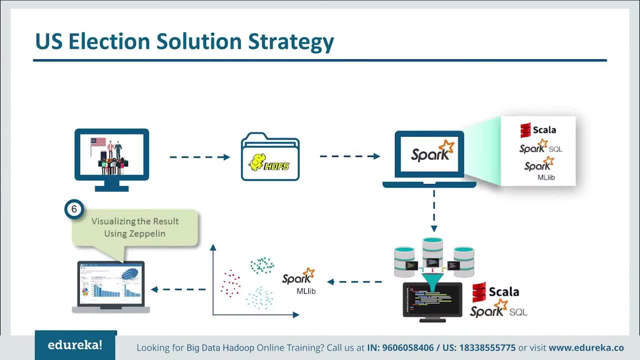 The result using Zeppelin. now visualizing this data is also very important because without the visualization, you won't be able to identify what were the major reasons and you won't be able to gain proper insights from your data. Now don't be scared if you're not familiar with terms like spark, SQL, spark. 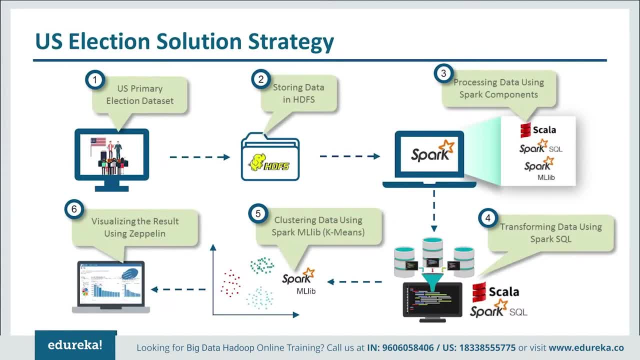 MLib k-means clustering. you will be learning all of these in today's session, So this is our entire strategy. This is what we're going to do today. This is how we're going to implement this use case and find out why Hillary. 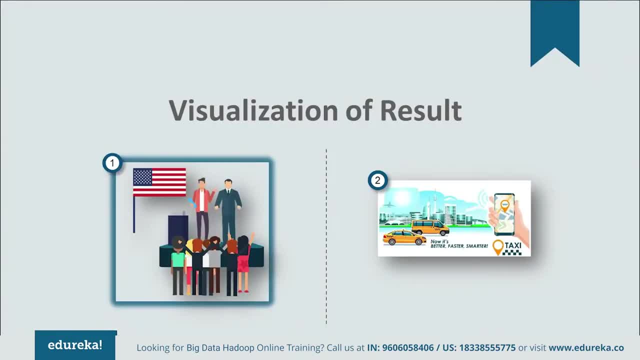 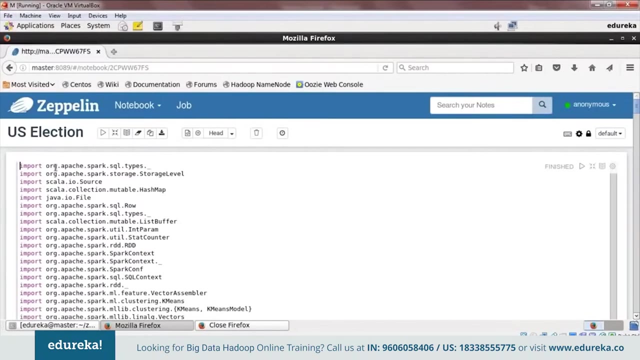 Clinton won. So now let me give you a visualization of the results. So I'll just show the analysis that I have performed and I'll show you how it looks. So this is Zeppelin, which is in my master node, in my Hadoop cluster, and this 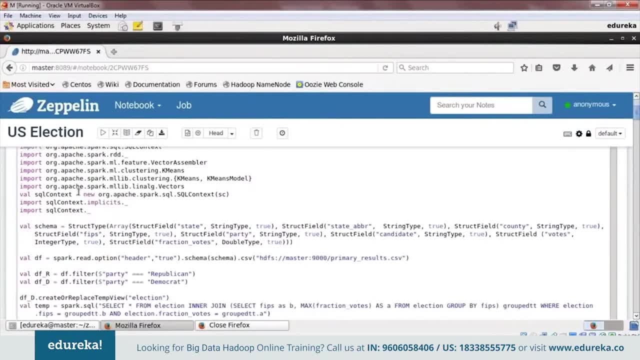 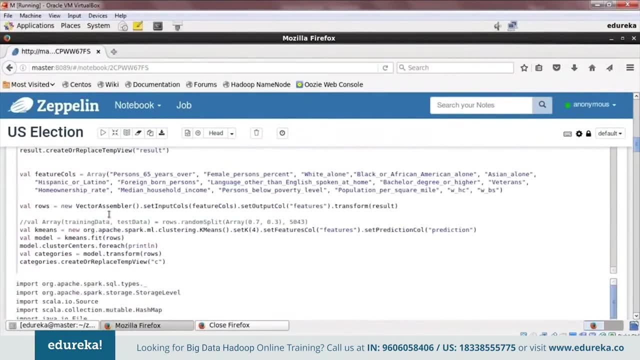 is where we're going to visualize our data. So there's a lot of code. Don't be scared, This is just scale of code with spark SQL and at the end you will be learning how to write this code. So I'm just jumping onto the visualization part. 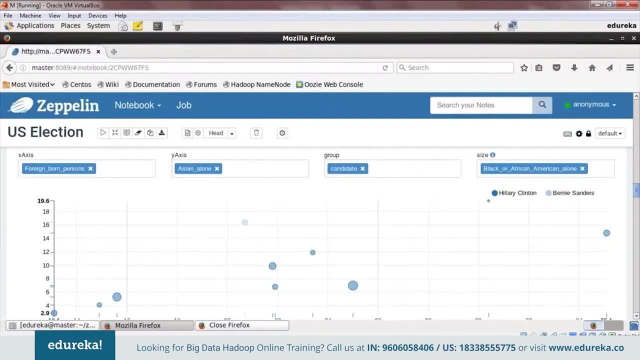 So this is the first visualization that we have got and we've analyzed it according to different ethnicities of people. For example, in our x-axis we have foreign-born persons and in y-axis We're seeing that among the foreign-born people. What is the popularity of Hillary Clinton among the Asians and the circles? 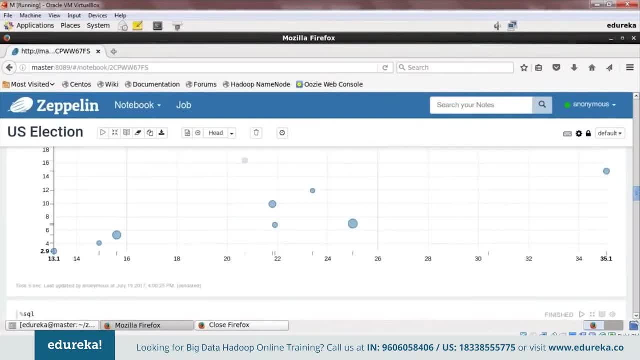 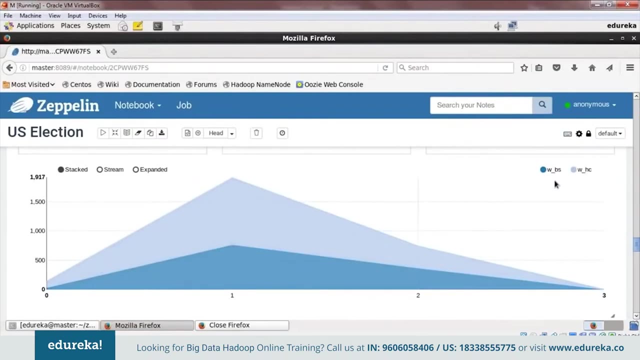 represent the highest values. The bigger circle is, the bigger counts. So we have made a few more visualizations. So now we've got a line graph that compares the votes of Hillary Clinton and Bernie Sanders together. again, We have got an area graph also that compares Bernie Sanders and Hillary. 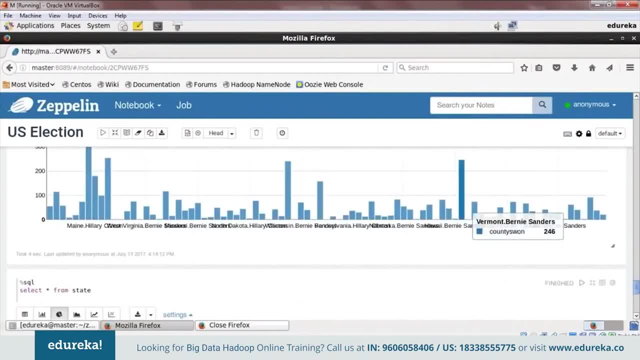 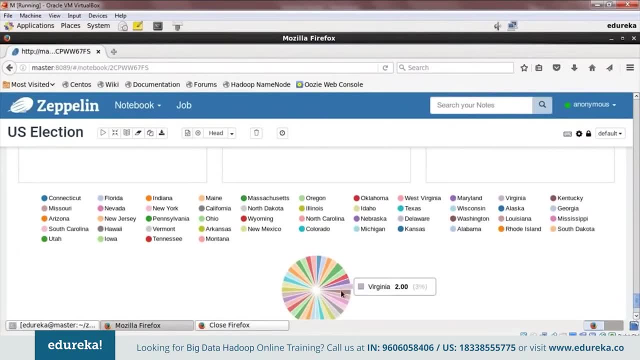 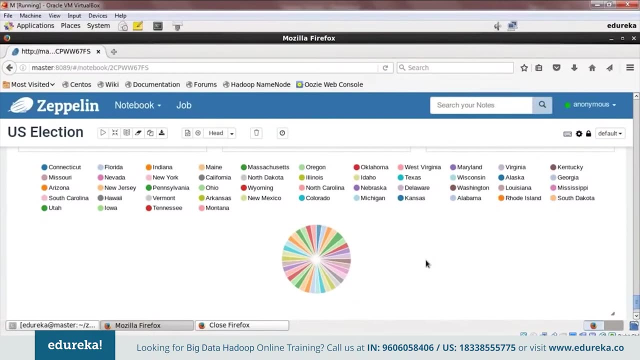 Clinton votes, and hence we have a lot more visualization. We have got our bar charts and everything. Finally, we also have state and county wise distribution of votes. So these are the visualizations that will help you derive a conclusion, To derive an answer, whatever answer that Donald Trump wants from you. 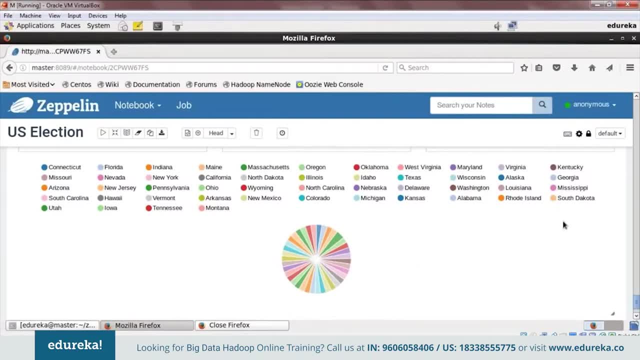 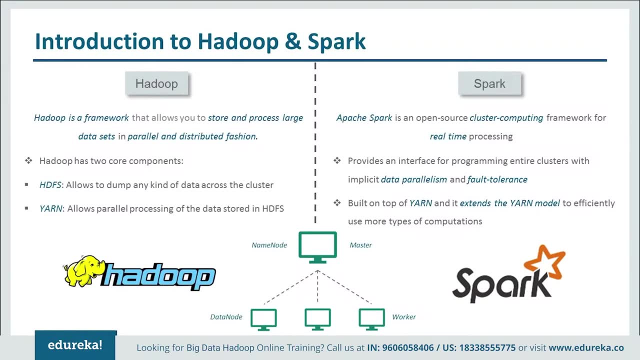 And, don't worry, you'll be learning how to do that. I'll explain each and every detail of how I've made these visualizations. So let's get started with Hadoop and Spark. We will start with an introduction to Hadoop and Spark. 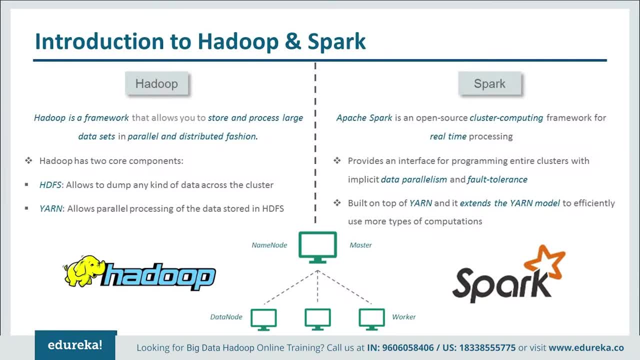 So now let's take a look at what is Hadoop and what is Spark. So Hadoop is a framework where you can store large clusters of data in a distributed manner And then process them parallelly. Then Hadoop has got two components for storage. 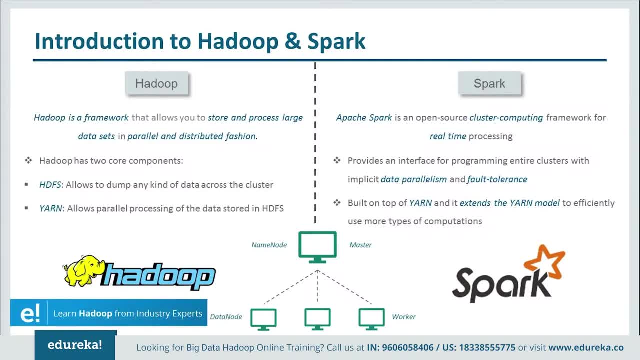 It has HDFS, which stands for Hadoop Distributed File System, And it allows to dump any kind of data across the Hadoop cluster And it will be stored in a distributed manner in commodity hardware before processing. You've got YARN, which stands for Yet Another Resource Negotiator. 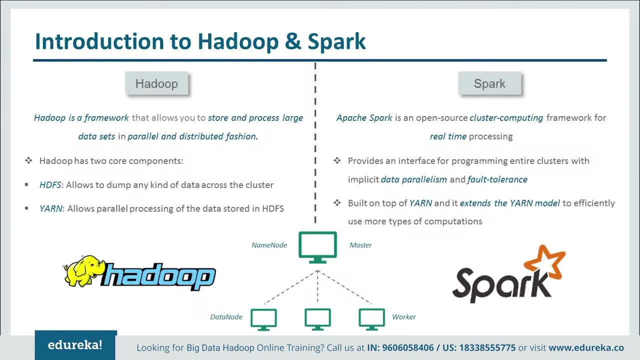 And this is the processing unit of Hadoop, which allows parallel processing of the distributed data across your Hadoop cluster in HDFS. Then we've got Spark, So Apache. Spark is one of the most popular projects by Apache And this is an open source cluster computing framework for real time processing. 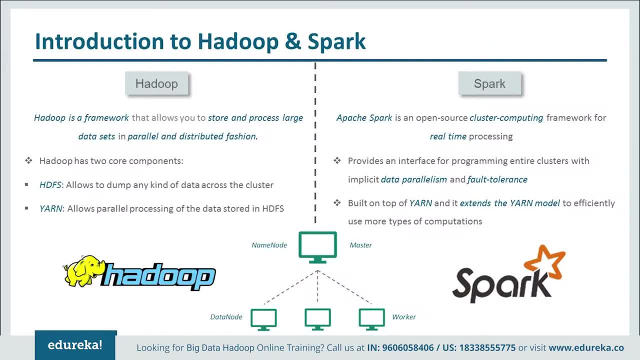 Where, on the other hand, Hadoop is used for batch processing, Spark is used for real time processing Because with Spark, the processing happens in memory And it provides you with an interface for programming entire clusters with implicit data parallelism and fault tolerance. So what is data parallelism? 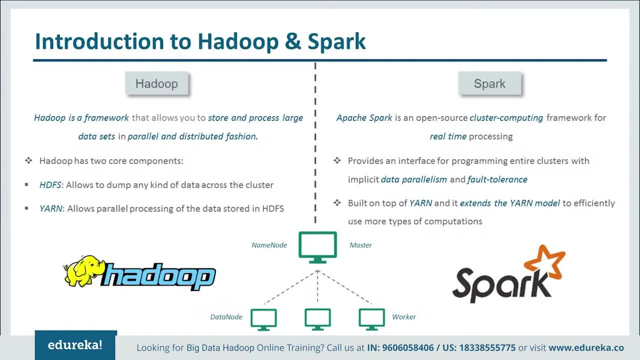 Data parallelism is a framework. It's a form of parallelization across multiple processes in parallel computing environments. A lot of parallel words in that sentence, So let me tell you simply that it basically means distributing your data across nodes which operate on the data parallel. 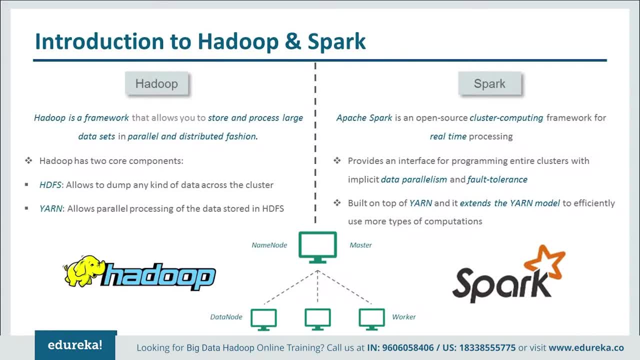 And it works on fault tolerant systems like HDFS and S3.. And it is built on top of YARN, Because with YARN you can combine different tools like Apache, Spark for better processing of your data And, if you see the topology of Hadoop, 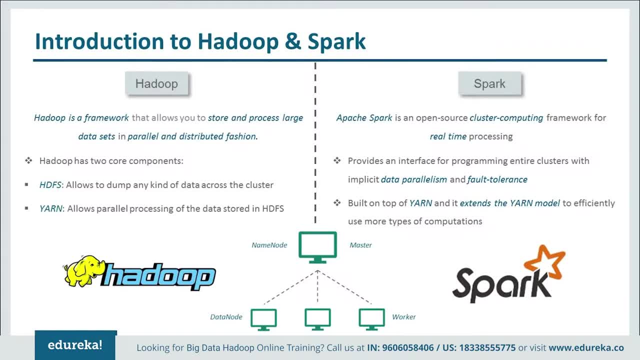 Hadoop and Spark. both of them have the same topology, Which is a master- slave topology. So in Hadoop, if you consider in terms of HDFS, The master node, as known as the name node, And the working node or the slave nodes, are known as data node. 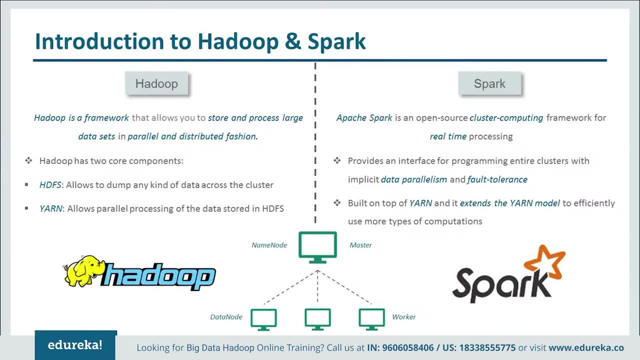 And in Spark, the master is known as master And slave are known as workers. So these are basically demons. So this is a brief introduction to Hadoop and Spark, And now let's take a look at Spark complementing Hadoop. There's always been a debate about what to choose. 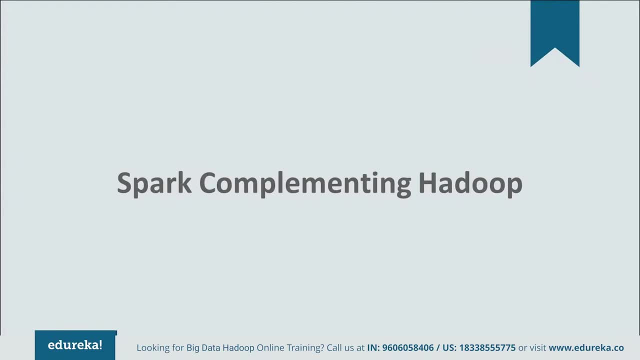 Hadoop or Spark. But let me tell you that there is a stubborn misconception that Apache Spark is an alternative to Hadoop And that is likely to bring an end to the era for Hadoop. It is very difficult to say Hadoop versus Spark. 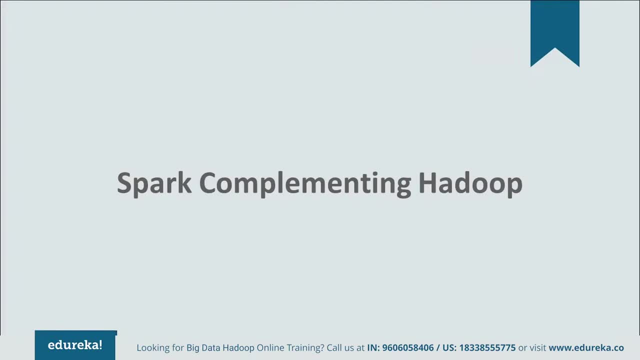 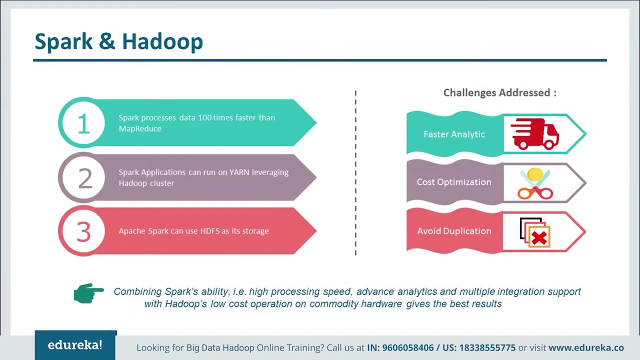 Because the two framers are not mutually exclusive, But they are better when they are paired with each other. So let's see the different challenges that we address when we are using Spark and Hadoop together. You can see the first point: Spark processes data 100 times faster than MapReduce. 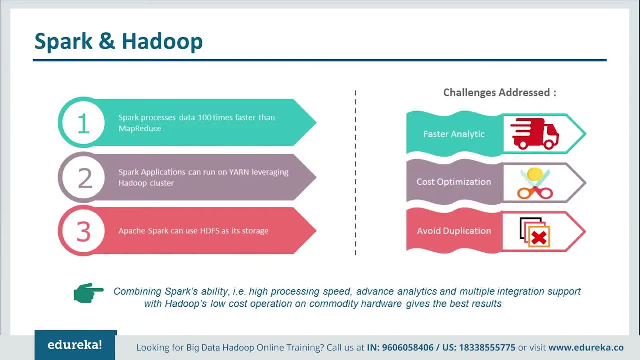 So it gives us the results faster and it performs faster analytics. The next point is Spark applications can run on Yarn leveraging Hadoop cluster, And you know that Hadoop cluster is usually set up on commodity hardware. So we are getting better processing. 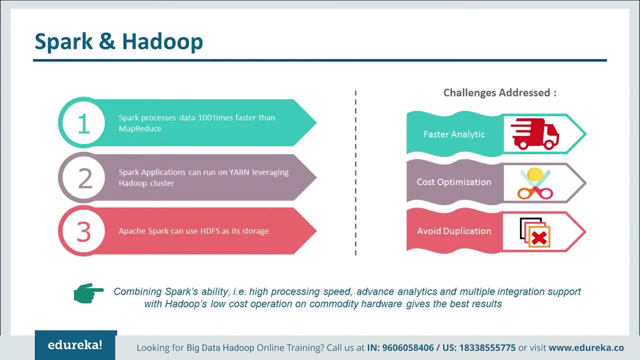 But we are using very low cost hardware And this will help us cut our costs a lot, So hence also the cheap cost optimization. The third point is that Apache Spark can use HTML And Apache Spark can use HDFS as storage, So you don't need a different storage space for Apache Spark. 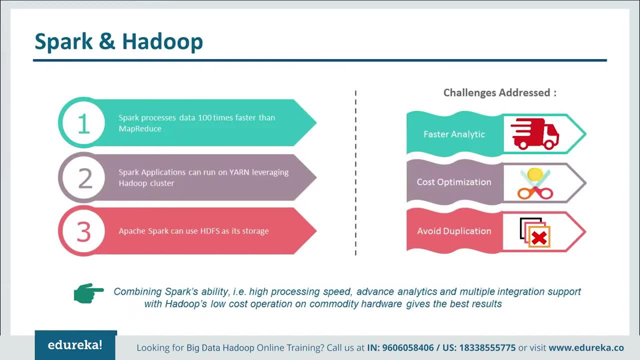 It can operate on HDFS itself, So you don't have to copy the same file again, And if you want, to process it with Spark, So hence you can avoid duplication of files. So Hadoop forms a very strong foundation for any of the future big data initiatives. 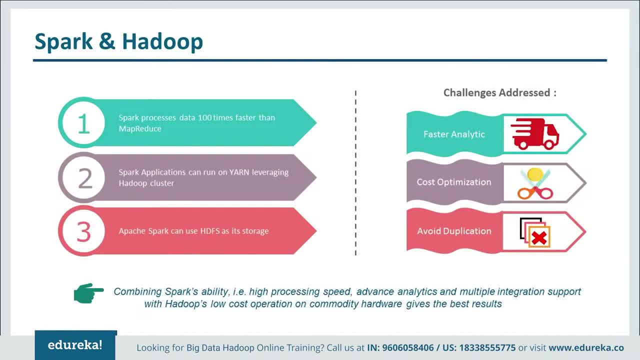 And Spark is one of those big data initiatives. It has got enhanced features like in memory, processing, learning capabilities, and you can use it with Hadoop, And Hadoop uses commodity hardware Which can give you better processing with minimum cost. These are the benefits that you get when you combine Spark and Hadoop together. 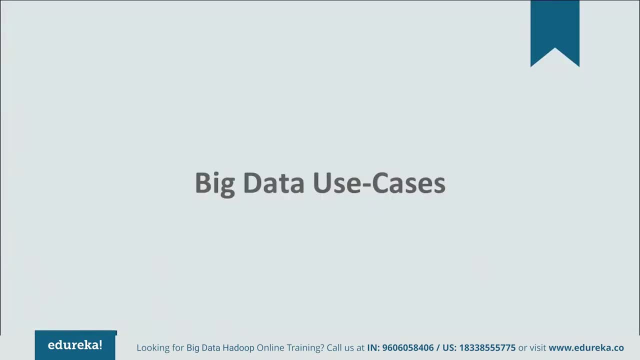 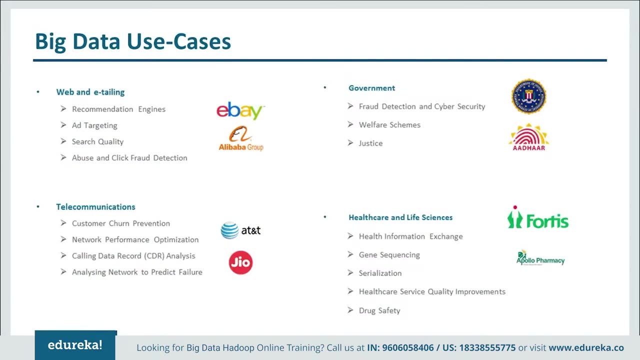 In order to analyze big data. Let's see some of the big data use cases. So the first big data use case is web e-tailing The recommendation engines whenever you go out on Amazon or any other online shopping site In order to buy something. 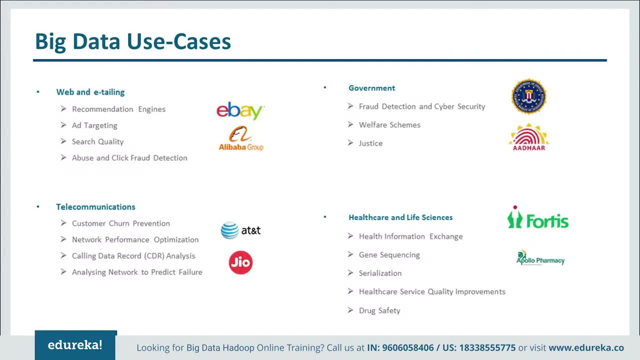 You will see some recommended items popping below your screen Or to the side of your screen, And that is all generated using big data analytics and ad targeting. If you go to Facebook, you see a lot of different items asking you to buy them, And then you got search quality abuse and click fraud detection. 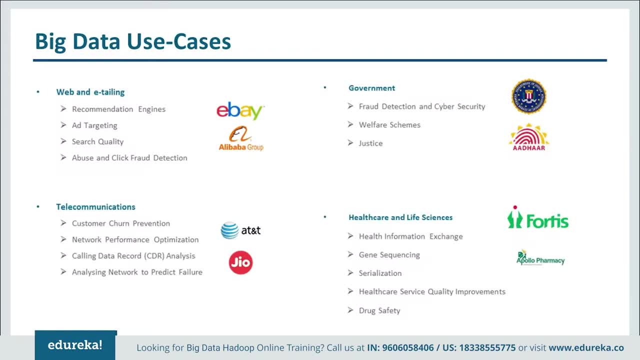 You can use big data analytics and telecommunications also In order to find out the customer churn prevention, The network performance optimization Analyzing network to predict failure, And you can prevent loss before the error or before the fault actually occurs. It's also widely used by governments for fraud detection and cyber security. 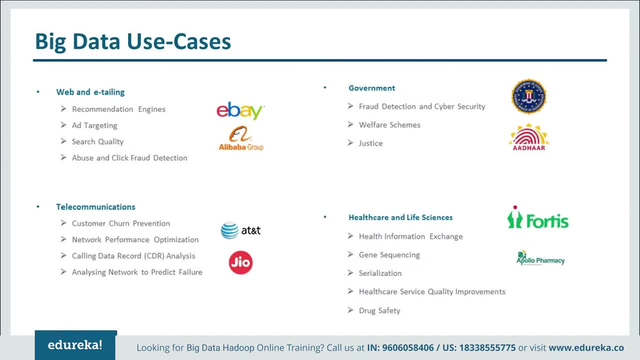 In order to introduce different welfare schemes. Justice: it has been widely used by healthcare and life sciences For health information exchange, Gene sequencing, serialization, Healthcare service quality improvements and drug safety. Now let me tell you that, with big data analytics, It has been very easy in order to diagnose a particular disease. 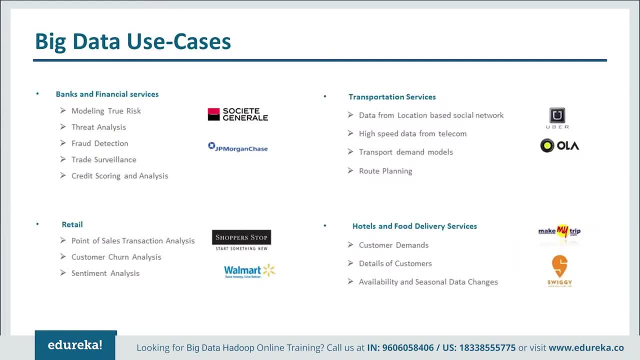 And find out the cure also. So these are some more big data use cases. It is also used in banks and financial services For modeling, true risk, fraud detection, credit card scoring analysis and many more. It can be used in retail transportation services, hotels and food delivery services. 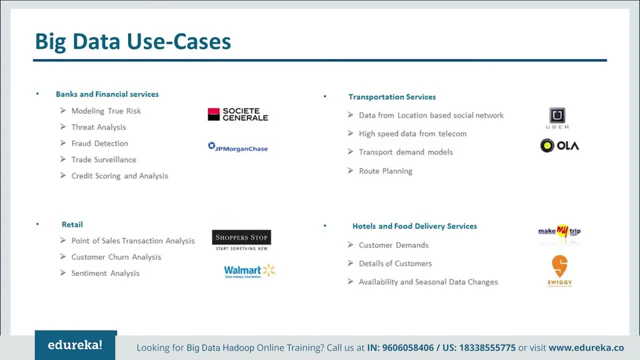 And actually every field you name. No matter whatever business you have, If you are able to use big data efficiently, Your company will grow and you will be gaining different insights By using big data analytics And hence improve your business even more. Nowadays, everyone is using big data. 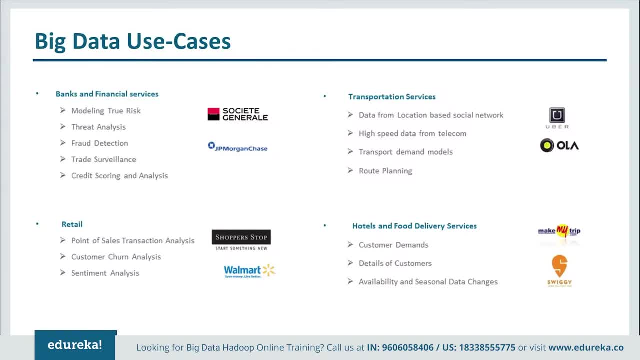 And you've seen different fields And everything is different from each other, But everyone is using big data analytics And big data analysis can be done with tools like Hadoop and Spark, etc. So this is why big data analytics is very much in demand today. 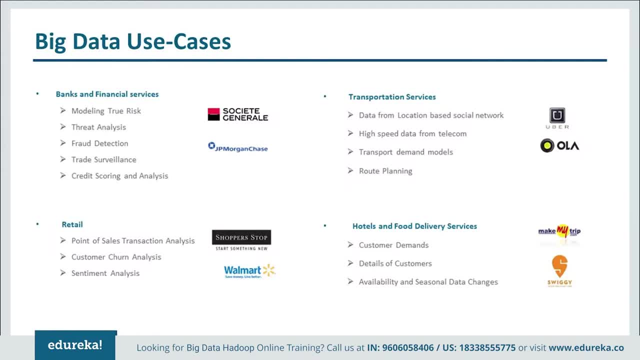 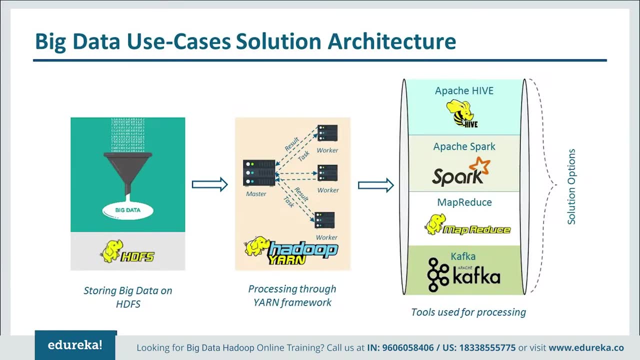 And why it is very important for you to learn how to perform big data analytics with tools like this. So now let's take a look at a big data use solution architecture As a whole. You're dealing with big data. now, The first thing that you need to do- 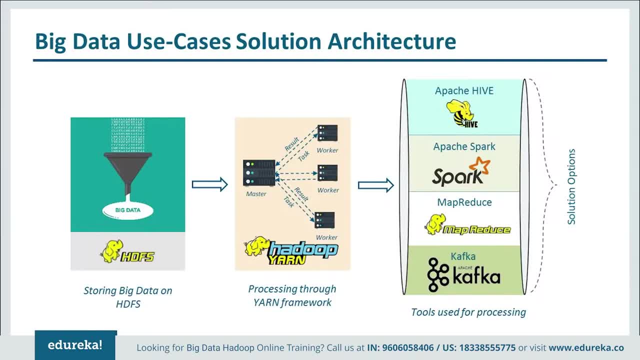 Is you need to dump all that data into HDFS And store it in a distributed way, And the next thing is to process that data So that you can gain insights. And we'll be using Yarn, Because Yarn can allow us to integrate different tools together. 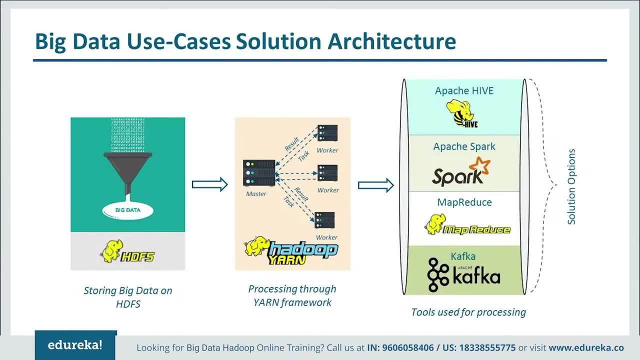 Which will help us to process the big data. These are the tools that you can integrate with Yarn. You can choose either Apache Hive, Apache Spark, MapReduce, Apache Kafka In order to analyze big data, And Apache Spark is one of the most popular. 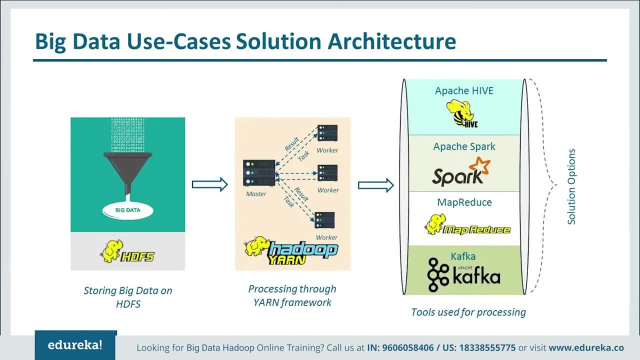 And most widely used tools, with Yarn, In order to process big data. So this is an entire solution As a whole. Now So let's take a look at Apache Spark. Apache Spark is an open source cluster computing framework For real time processing. 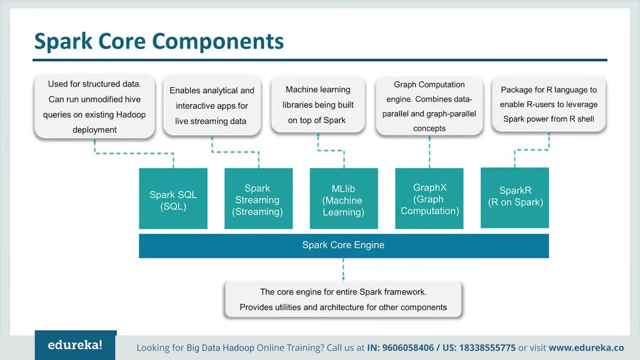 And it has been the thriving open source community And is the most active Apache project at this moment. And Spark components are what make Apache Spark fast And reliable, And a lot of Spark components were built To resolve the issues that cropped up. 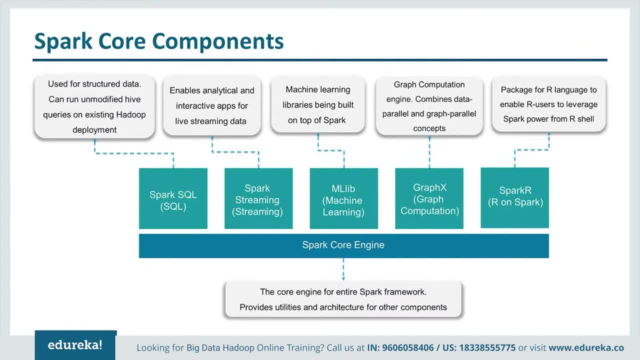 While using Hadoop MapReduce. So Apache Spark has got the following components: It's got the Spark core engine. Now the core engine is for the entire Spark frameworks. Every component is based on And it is placed in the core engine. So at first we've got Spark SQL. 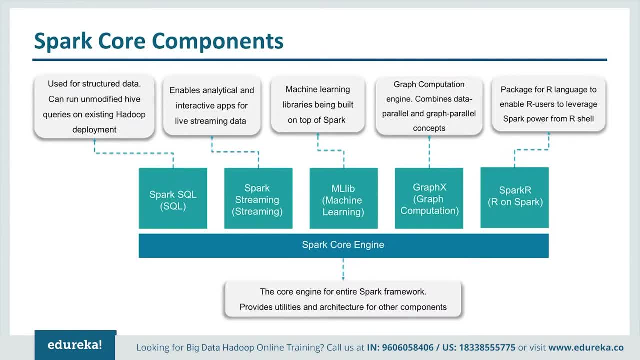 So Spark SQL is a Spark module for structured data processing And you can run a modified Hive queries On existing Hadoop deployments. And then we've got Spark streaming Now. Spark streaming is the component of Spark Which is used to process real time streaming data. 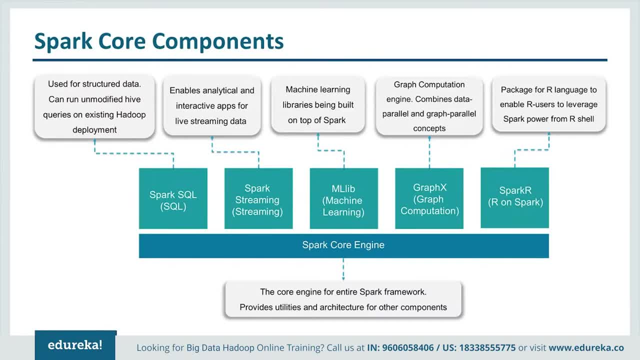 And is a useful addition to the core Spark API, Because it enables Hive throughput And fault tolerance Stream processing of live data streams. And then we've got Spark MLib. This is the machine learning library for Spark, And we'll be using Spark MLib. 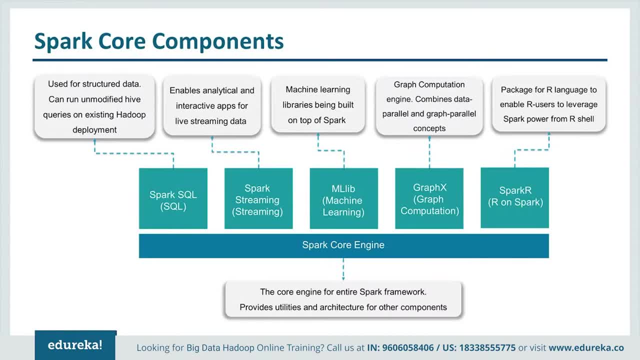 To implement machine learning in our use cases too. And then we've got GraphX, Which is the graph computation engine, And this is the spot API for graphs And graph parallel computation. It has got a set of fundamental operators Like subgraph, joint purchases etc. 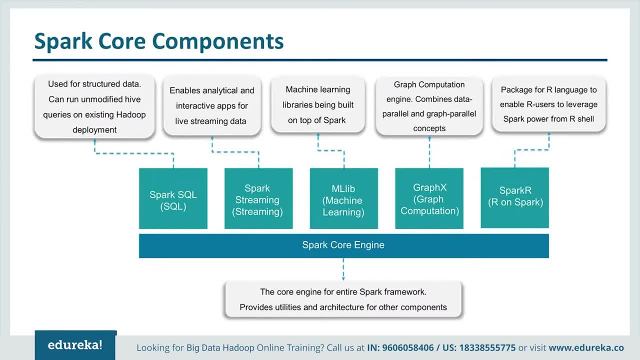 Then you've got Spark R. So this is the package for R language To enable our users to leverage Spark power from R shell. So the people who have already been working on R Are comfortable with it And they can use R shell directly at the same time. 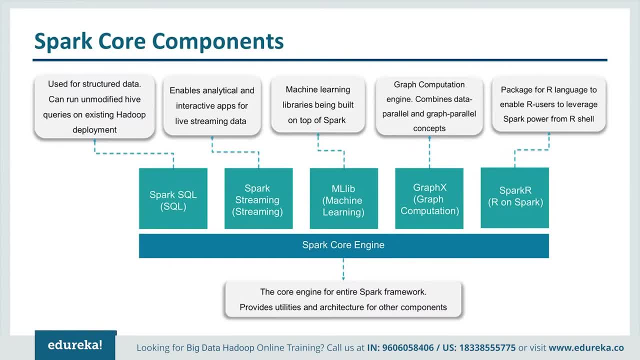 And they can use Spark. using this particular component, Which is Spark R, You can write all your code in the R shell And Spark will process it for you. Now let's take a deeper look at a realistic people And all these important components. 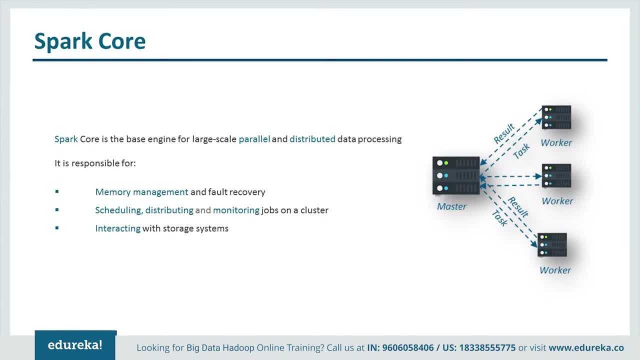 So we've got Spark core, And Spark core is the basic engine For large scale parallel and distributed data processing. The core is the distributed execution engine And Java, Scala and Python APIs offer a platform For distributed EDL development And further additional libraries. 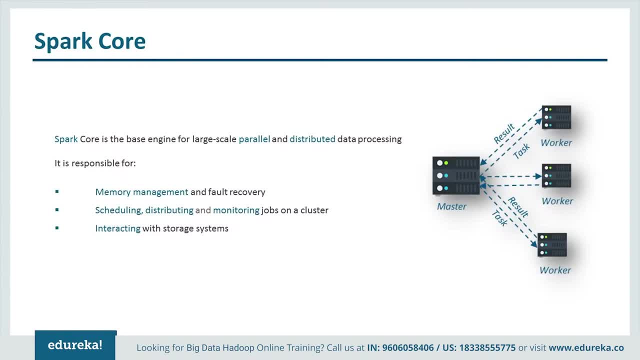 Which are built on top of the core Allow for diverse streaming, SQL and machine learning. It's also responsible for scheduling, Distributing and monitoring jobs In a cluster And also interacting with storage systems. Let's take a look at the Spark architecture. 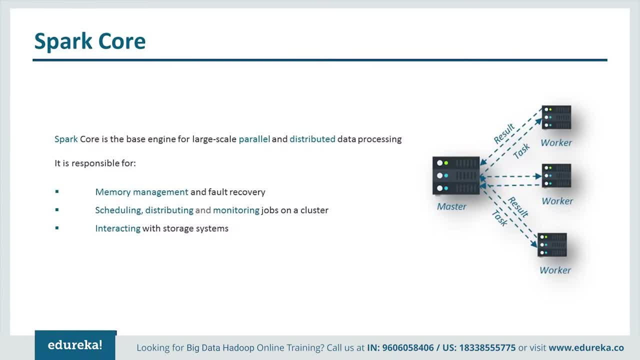 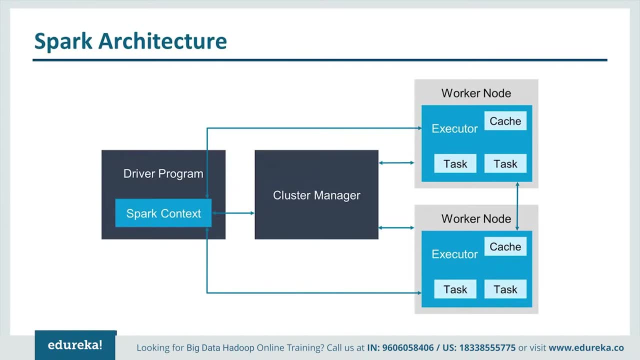 So this is Spark R And Spark R And Spark R. So Apache Spark has a well defined And layered architecture Where all the Spark components and layers Are loosely coupled and integrated With various extensions and libraries. First let's talk about the driver program. 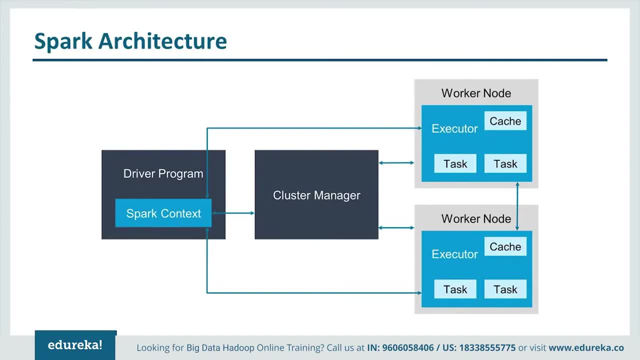 This is the Spark driver, Which contains the driver program And Spark context. This is the central point And entry point of the Spark shell And the driver program Runs the main function of the application And this is the place where Spark context. 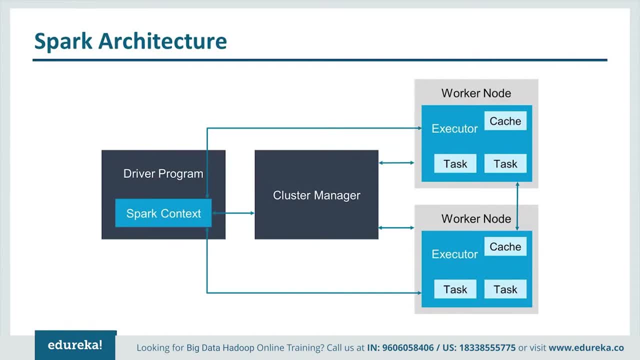 Is created. Well, what is Spark context? Spark context represents the connection To the entire Spark cluster And it can be used to create Resilient distributed data sets, Accumulators and broadcast variables On that cluster, And you should know that. 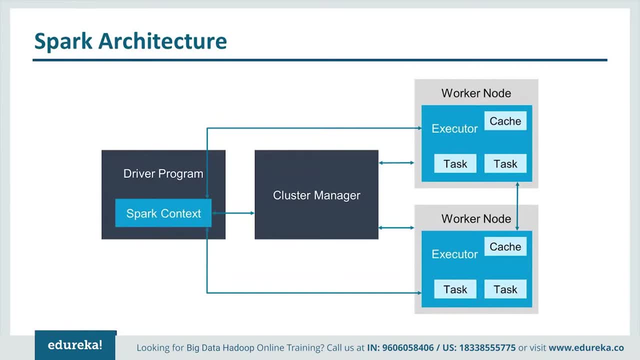 Only one Spark context May be active per Java virtual machine And you must stop Any active Spark context Before creating a new one. Let's talk about the driver program First. let's talk about the Spark cluster. The Spark cluster is the master. 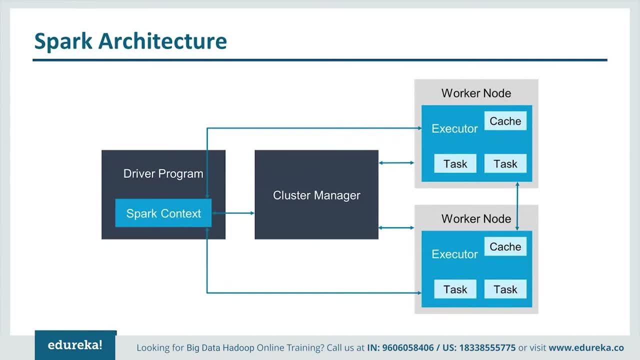 Knob of the Spark cluster. It schedules the job execution And negotiates with the cluster manager. This is the cluster manager over here And the cluster manager is an external service That is responsible for acquiring resources On that Spark cluster And allocating them to a Spark job. 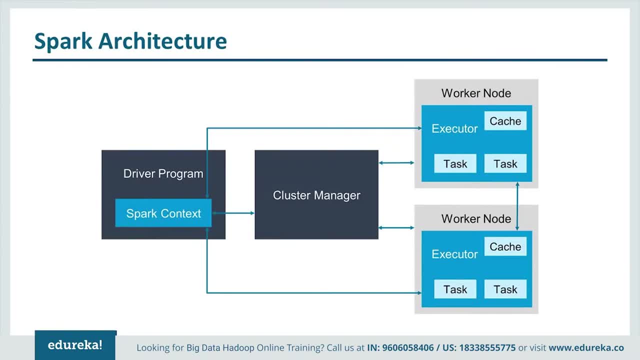 Then in the worker node, We have got the executors. The executor is a distributed agent That is responsible for the execution Of tasks, And the Spark application Has its own executor process. Executors usually run for their entire lifetime Of the Spark application. 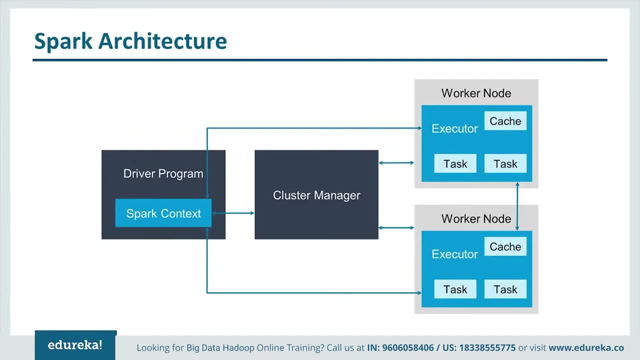 And this phenomenon is also known as Static allocation of executors. But you can also opt for Dynamic locations of executors, Where you can add or remove Spark executors dynamically To match with the overall workflow. Okay, Now let me tell you what actually happens. 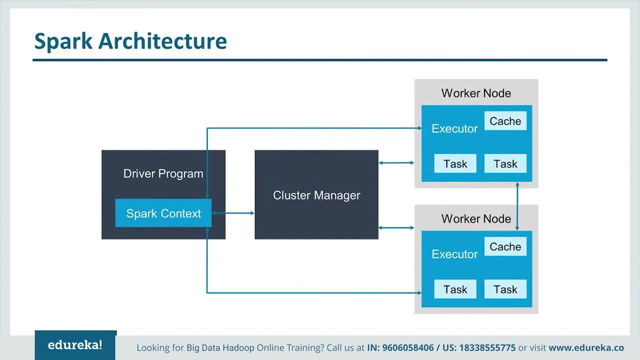 When the Spark job is submitted, When a client submits a Spark user application code, The driver implicitly converts the code Containing transformations and actions Into a logical directed Asylic graph, or DAG, And at this stage the driver program Also performs certain kinds of. 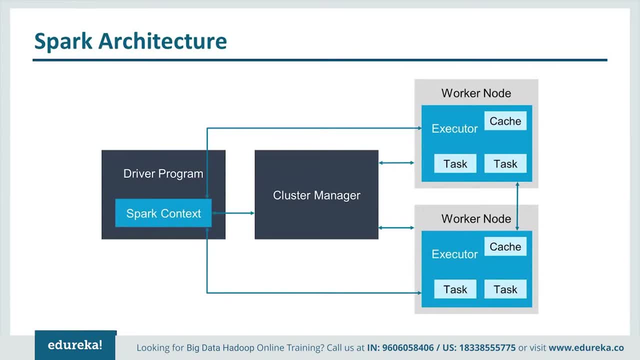 Optimizations like pipelining Transformations, And then converts the logical DAG Into a physical execution Of a plan With a set of stages, And after creating a physical execution plan, It creates more physical execution Units That are referred to as 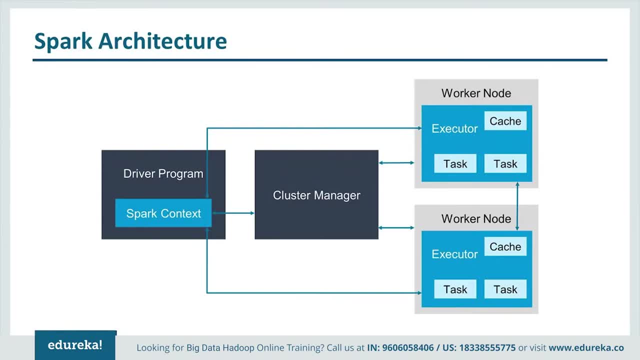 Tasks under each state And these tasks are bundled To be sent to the Spark cluster. So the driver program Then talks to the cluster manager And negotiates for resources And the cluster manager Then launches the executors On the worker nodes. 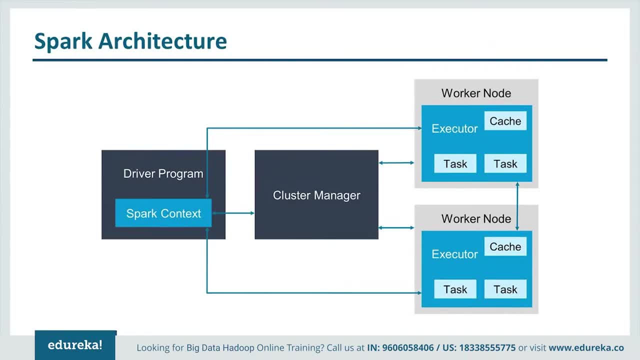 On behalf of the driver And at this point the driver Sends tasks to the cluster manager Based on the day replacement, So that the driver has got A holistic view of all the executors. Now the executors Will execute the various tasks. 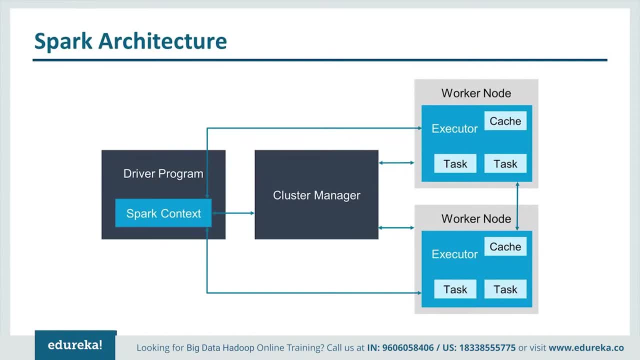 Assigned to them by the driver program. And at any point in time When the Spark application is running, The driver program will keep On monitoring the set of executors That are running the Spark application code. This driver program Here also schedules future tasks. 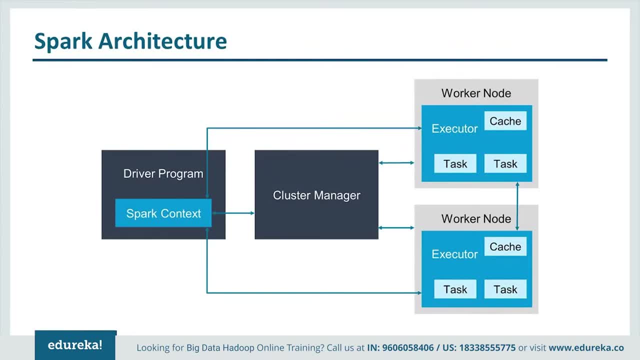 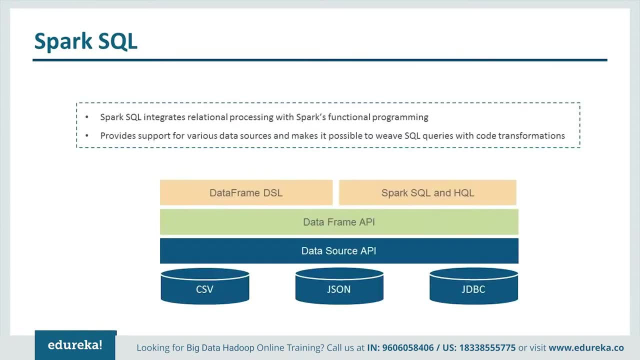 Based on data replacement By tracking the location of the cache data. So I hope you have understood What Spark does for Spark. Any doubts? Alright, no doubts. Now let's take a look at Spark SQL And its architecture. So Spark SQL is the new module in Spark. 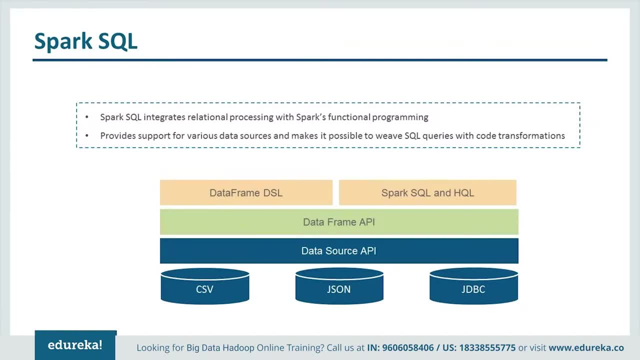 And it integrates relational processing With Spark's functional programming API. And it supports querying of data Either via SQL or via Hive query language. So for those of you Who have been familiar with RDBMS, So Spark SQL will be a very easy transition. 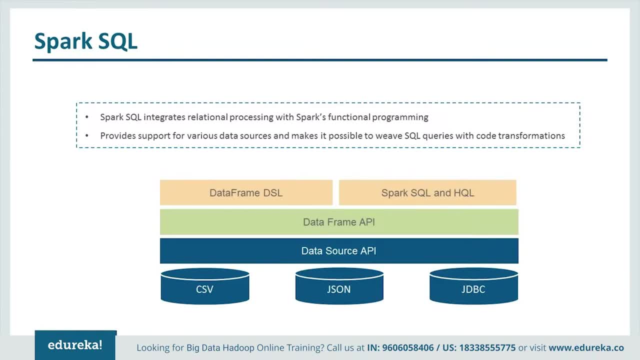 From your earlier tools Because you can extend the bounds Of traditional relational data processing With Spark SQL And it also provides support For various data sources And makes it possible To read SQL queries with code transformation, And that is why Spark SQL. 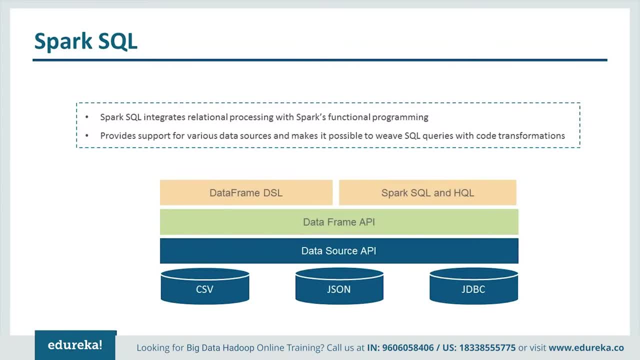 Has become a very powerful tool. This is the architecture of Spark SQL. Let's talk about each of these components One by one. First, we have got the data source API. So this is the universal API For loading and storing structured data. 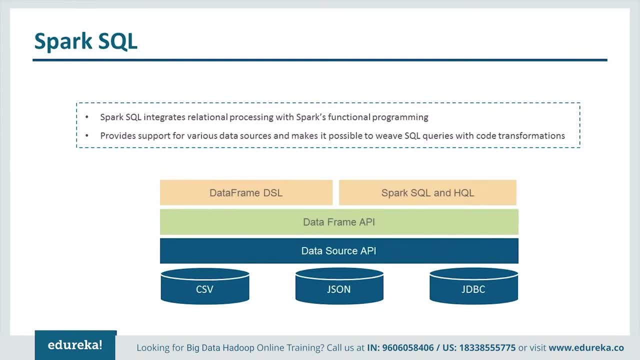 And it is built on Support for Hive, Avro, JSON, JDBC, CVS, Parquet, Etc. So it also supports the third party integration Through Spark packages. Then you have got the data frame API. Data frame API. 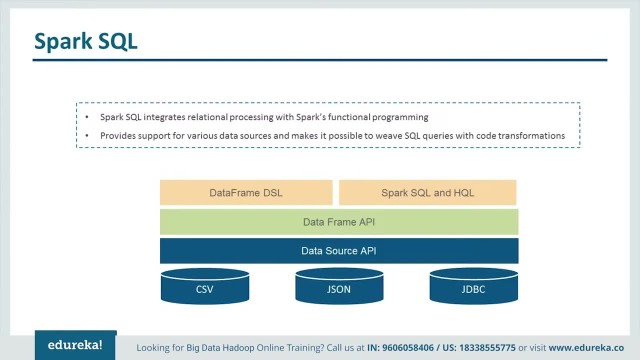 Is the distributive collection of data That is organized into named columns And is similar to relational table in SQL. That is used for storing data in tables And is applicable on structured And semi-structured data. So it processes data from kilobytes to petabytes. 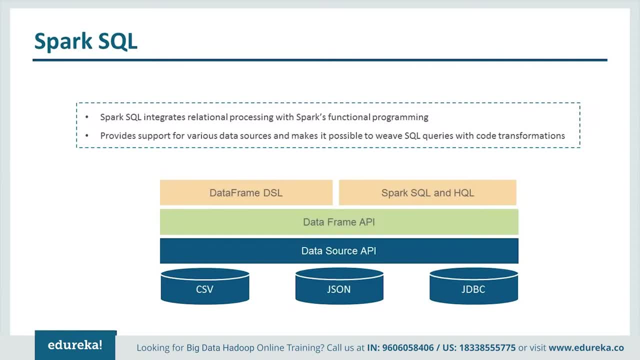 On a single node cluster To a multi-node cluster, And it provides different APIs For Python, Java, Scala and our programming. So I hope you have understood All the architecture of Spark SQL. We will be using Spark SQL In order to solve our use cases. 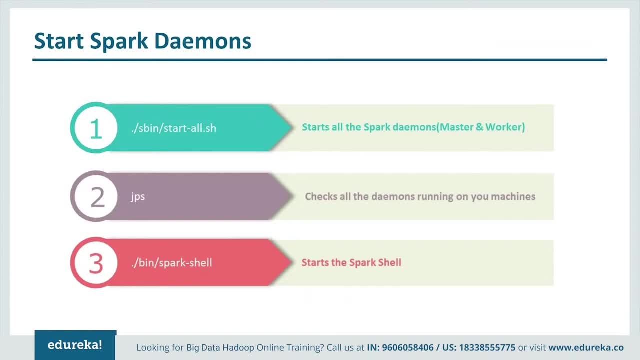 So these are the different commands To start the Spark daemons. These are very similar to Hadoop commands To start the HDFS daemons, To start all the Spark daemons. So the Spark daemons are master and worker And you can use this command. 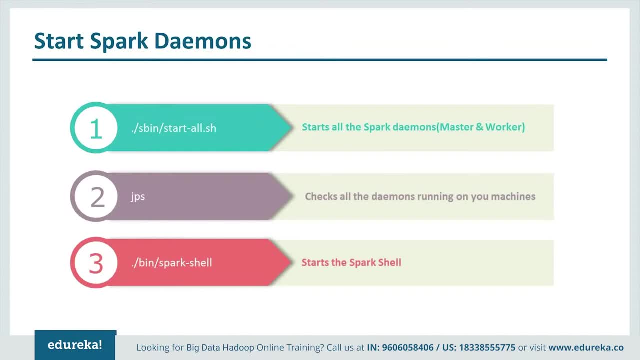 To check if all the daemons are running On your machine, You can use JPS, like Hadoop, And then, in order to start the Spark shell, You can use this, And you can go ahead and try this out. So this is very similar to the Hadoop part. 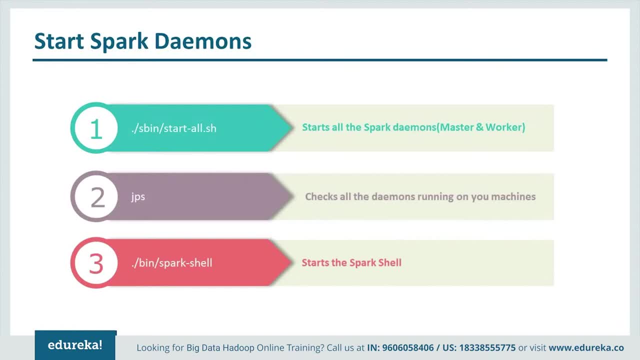 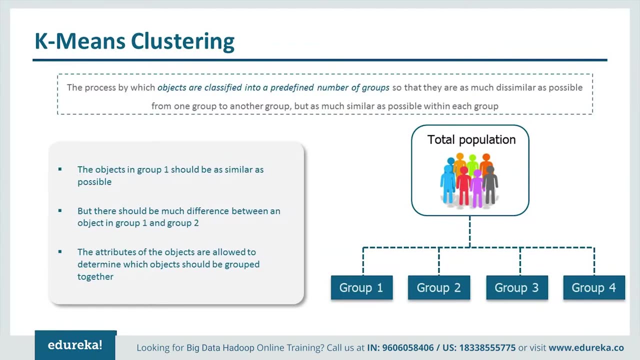 That I just showed you earlier, So I am not going to do it again. And we have seen Apache Spark also. So now let's take a look at K-Means and Zeppelin. K-Means is the clustering method And that is what we are going to use. 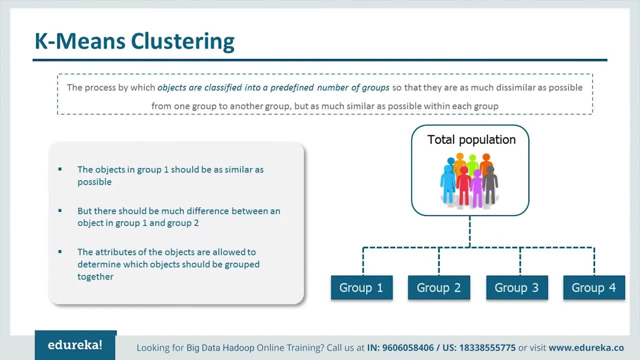 In order to visualize our data. So let's talk about the K-Mean clustering now. K-Means is one of the most simplest Unsupervised learning algorithms That solves the well known clustering problem. So the procedure of K-Means. 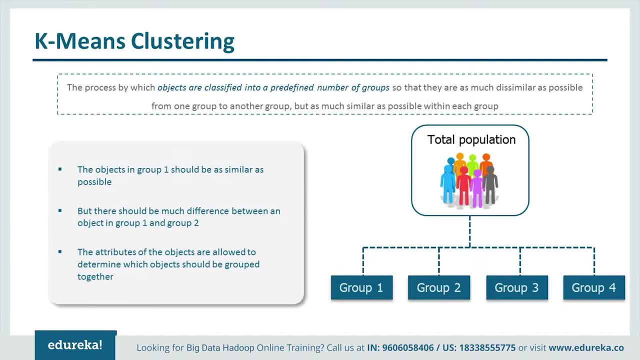 Follows a simple and easy way To classify a data set To a certain number of clusters, Which is fixed Prior to performing the clustering method. So the main idea is Define K centroids, One for each cluster And one for each cluster. 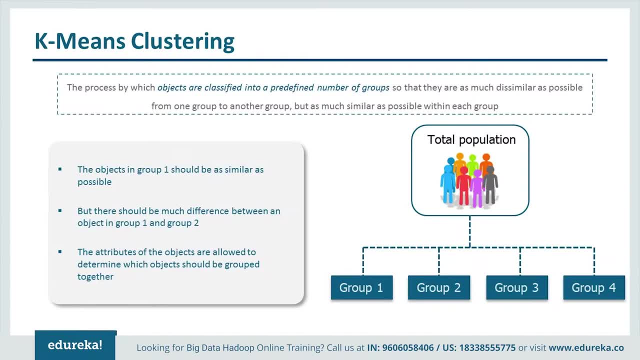 So the K centroids should be placed In a very cunning way, Because of different location Causes different results. So here let's take an example. So let's say that we want to cluster A total population of a certain location, And so we want to cluster them. 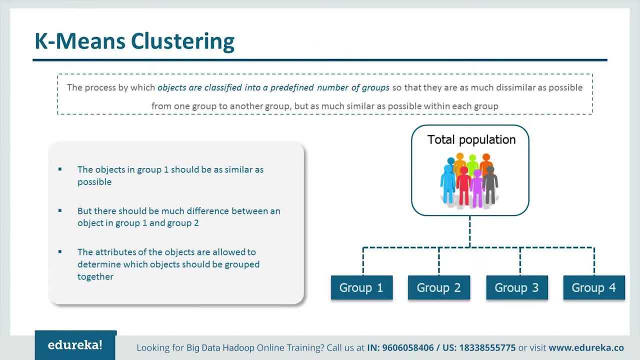 Into four different clusters, Namely group 1,, 2,, 3 and 4.. So the main thing that we should keep in mind Is that the objects in group 1. Should be as similar as possible, But there should be. 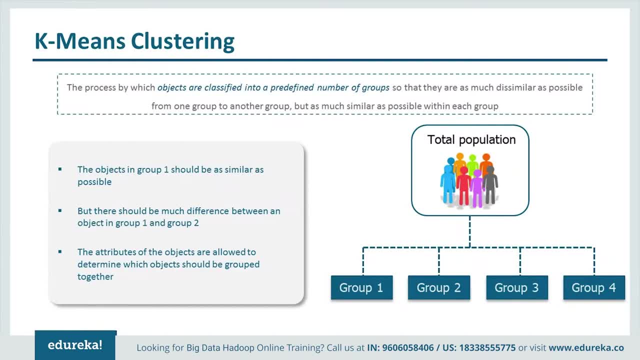 As much difference between an object In group 1 and group 2.. It means that the points That are lying in the same group Should have similar characteristics And it should be different from the points That are lying in a different cluster. 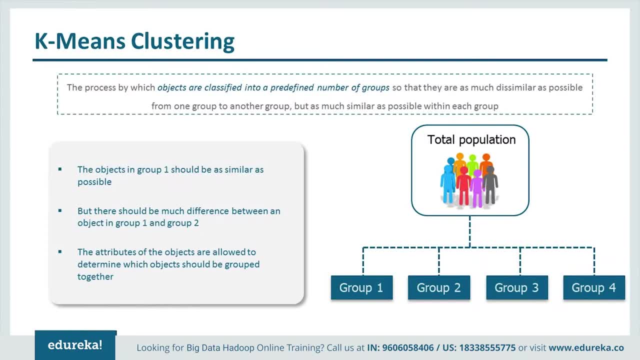 And the attributes of the objects Are allowed to determine Which object should be grouped together. For example, Let us take in the same sample That we are using in the US county. So let's consider the second data set We have used. 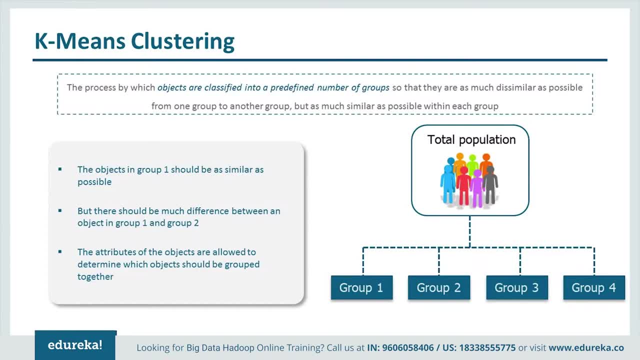 Data features that I already told you, Like there are age groups, And they are categorized by professions, And they are also categorized by the ethnicity, And so This is the thing that we are talking about. So these are the attributes That will allow us to cluster our data. 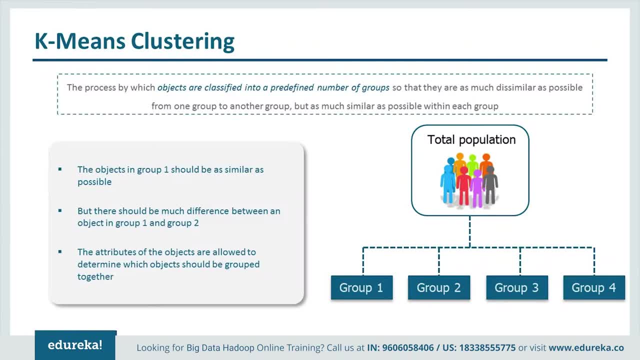 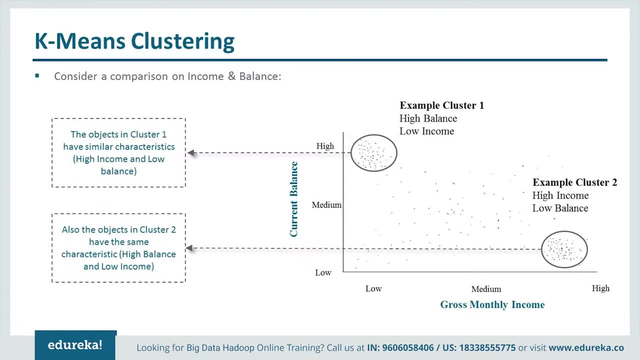 So this is. K means clustering. Here is one more example. Let us consider a comparison on income And balance. So in my x-axis I have the gross monthly income And in the y-axis I have the current balance. I want to cluster my data. 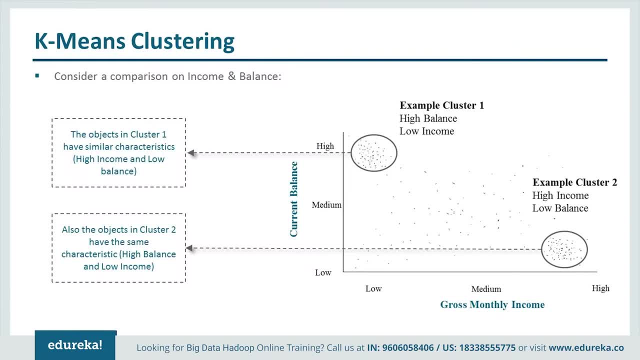 According to these two attributes Here. If you see, this is my first cluster And this is my second cluster, So this Is the cluster that indicates The people who have high income And low balance in the account And they spent a lot. 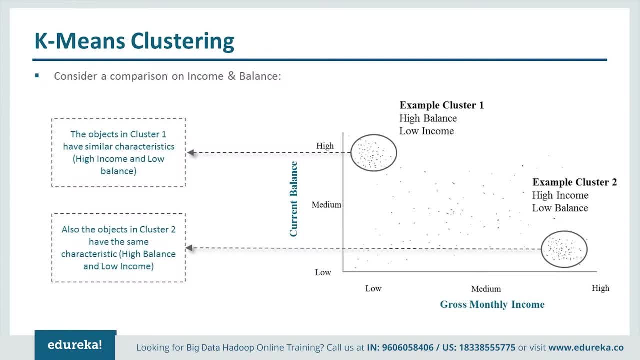 And this cluster comprises Of the people who have got a low income But a high balance, And they are safe. You can see that all the points that are lying here Have similar characteristics: That they have got low income And high balance. 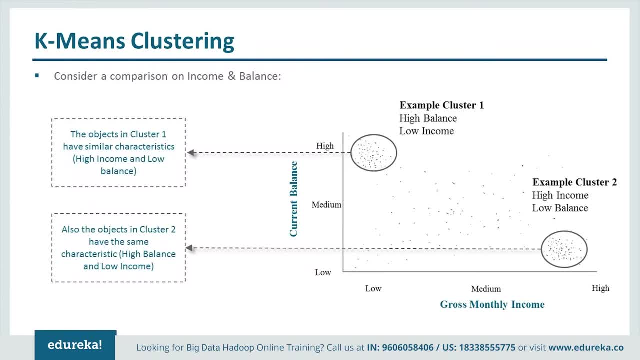 And here are the people who share the same characteristics, Where they have got low balance And high income, And there are a few outliers here And there, But they don't form a cluster. So this is an example of k means clustering. 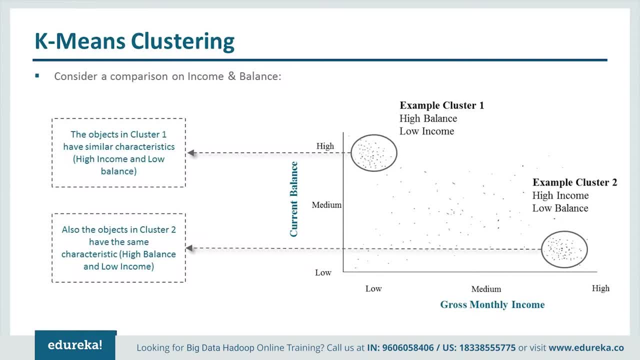 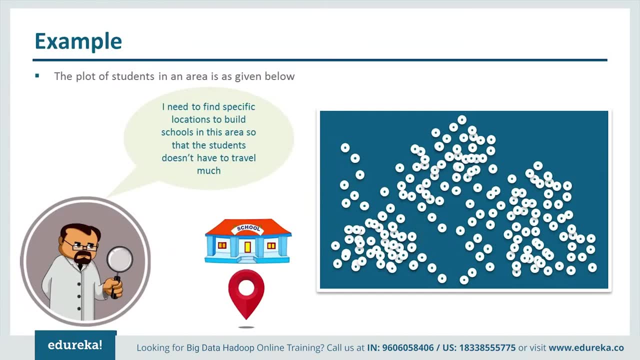 And we will be using that In order to solve our problems. So does anybody have any questions? So here is one more example And one more problem for you That you guys will tell me now. So the problem is that I want to set up schools. 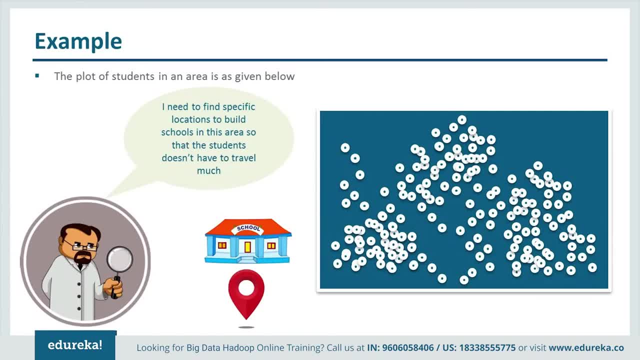 In my city, And these are the points which indicate Where each student lives. So my question to you is: Where should I be building my school If I have students living Around the city In these particular locations? And in order to find that out, 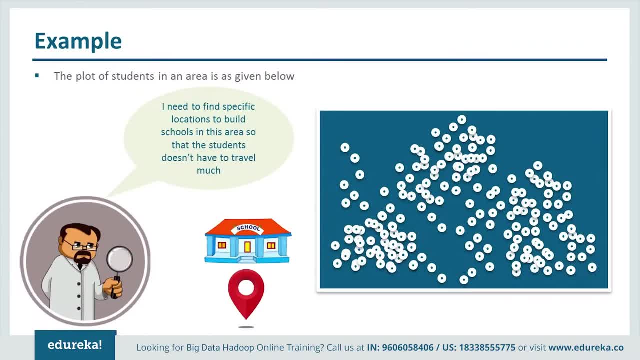 We will do. k means clustering And we will find out the center point. So if you can cluster and make groups Of all these locations In the center point of each cluster, That would be optimum, Isn't it? Because that is how the students have to travel less. 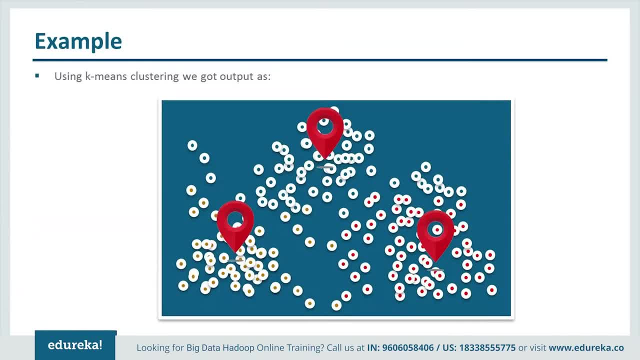 It will be close to everyone's house And there it is. So we have formed three clusters. So you can see the brown dots are one cluster And the blue dots are one cluster And the red dots are one cluster, And we have set up schools. 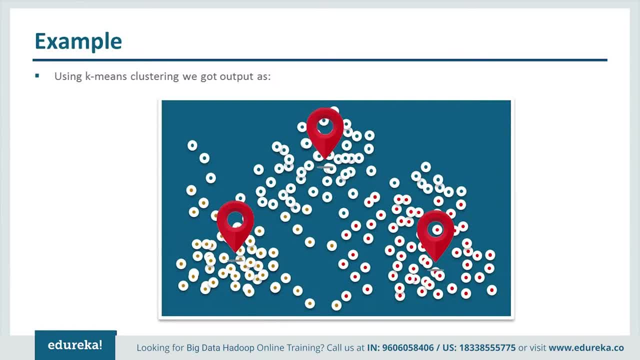 In the center points of each cluster. So here is one, Here is one, And here is yet another one, And I need to set my schools up So that my students do not have to travel that much. So that was all about k means. 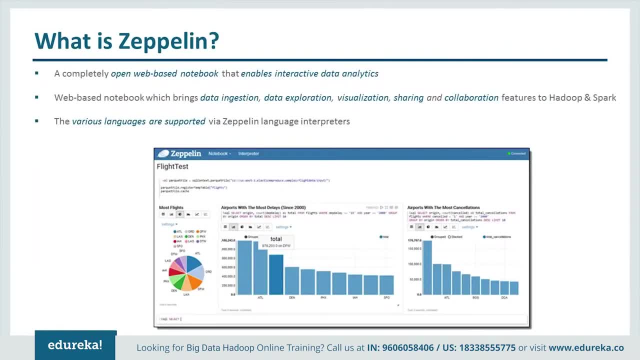 And now let's talk about Apache Zeppelin. This is a web page notebook Which brings in data ingestion, Data exploration, Visualization, Sharing and collaboration features To Hadoop and Spark. So remember when I showed you my Zeppelin notebook. You can see that we have written the code there. 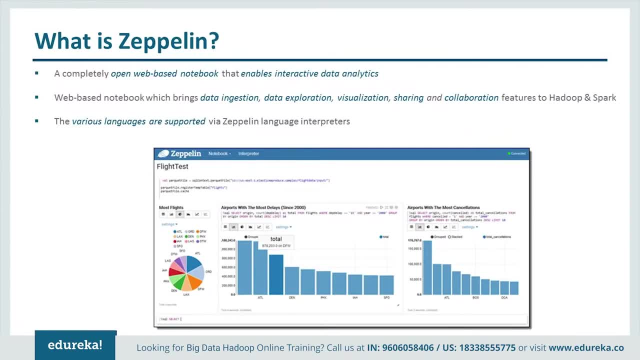 We have even run sequel codes there And we have more visualizations By executing codes. So this is how interactive Zeppelin is And it supports many, many interpreters And it is a very powerful visualization tool That can use. That goes very well with Linux systems. 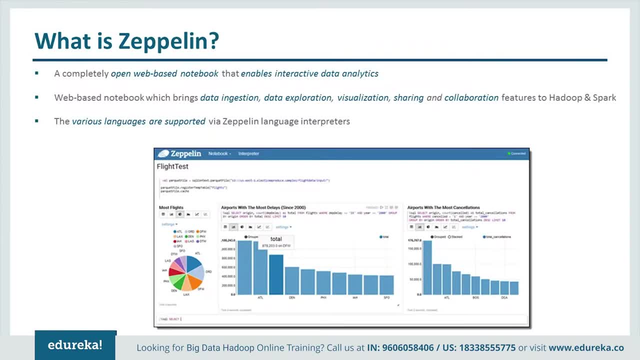 And it supports a lot of language interpreters. It supports R, Python And a lot of other interpreters. So now let's move on to the solution of the use case. So this is what you have been waiting for. First, we will solve our US county solution. 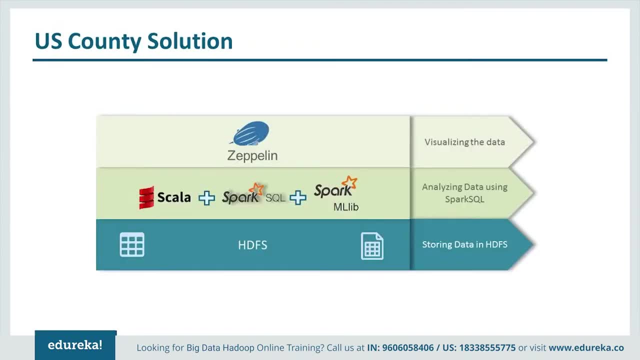 So the first thing we will do Is that we are going to use the code, We will store the data into HDFS And then we will analyze the data By using Scala, Spark SQL And Spark ML Live, And then, finally, 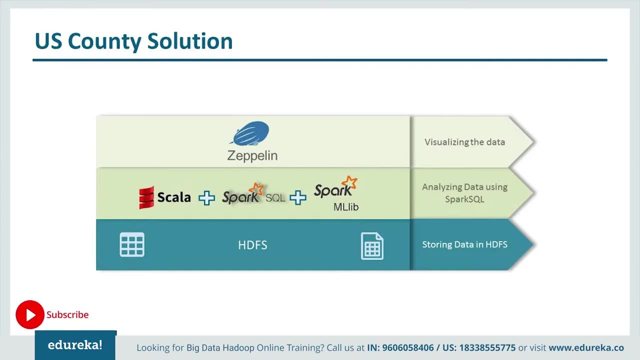 We will find out the results And visualize them using Zeppelin. So this was the entire US election solution strategy That I told you. Now I don't think I should repeat it again, But if you want me, I can, Should I repeat. 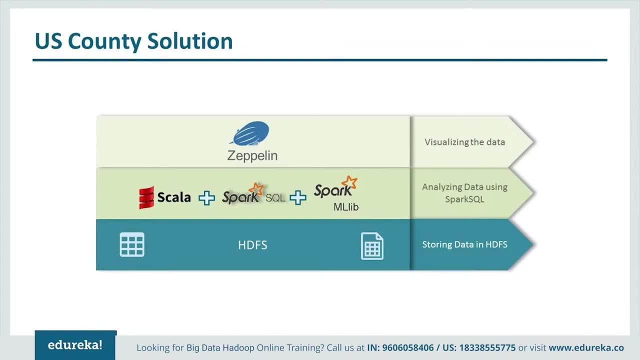 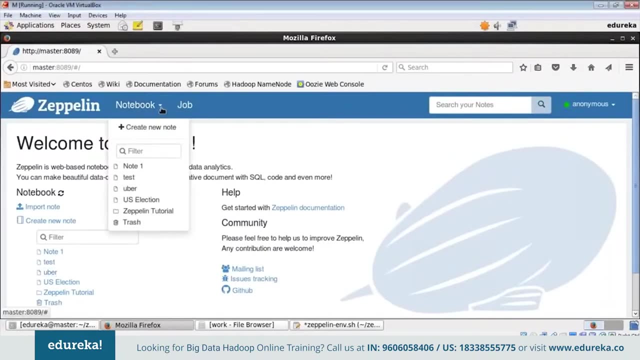 Alright, so most of the people are saying no, So I will go right through this one again. So let me just go to my VM And execute this for you. So this is my Zeppelin And I open my notebook here And let us go to my US election notebook. 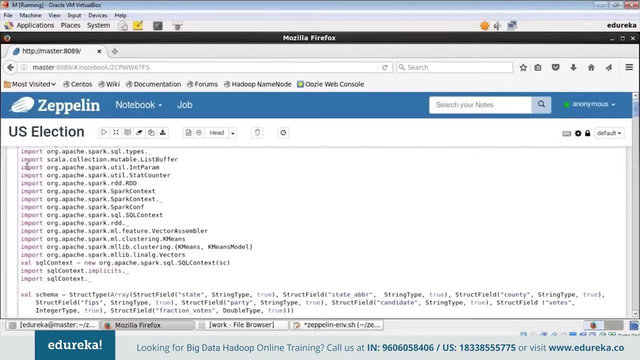 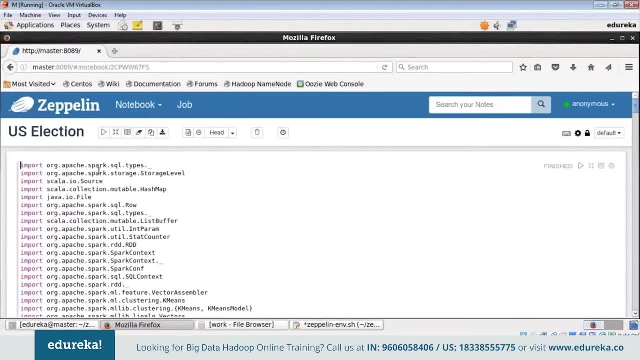 And this is the code. So, first of all, what I am going to do Is that I am importing certain packages, Because I will be using certain functions That are in those packages. So I have imported Spark SQL packages And I have also imported 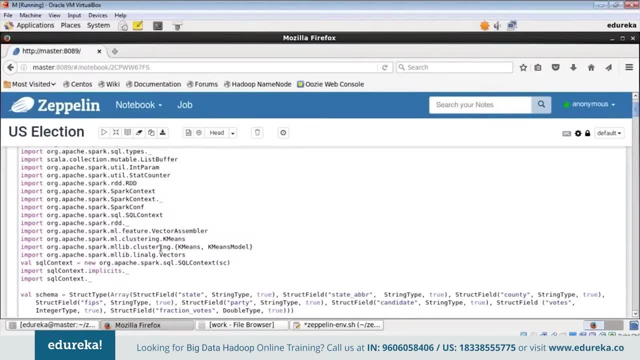 Spark ML Live packages, Because I will be using K-Means clustering. So Vector Assembler enables me Certain machine learning functions. Over here I have the Vector Assembler package That gives me certain machine learning functions That I am going to use. 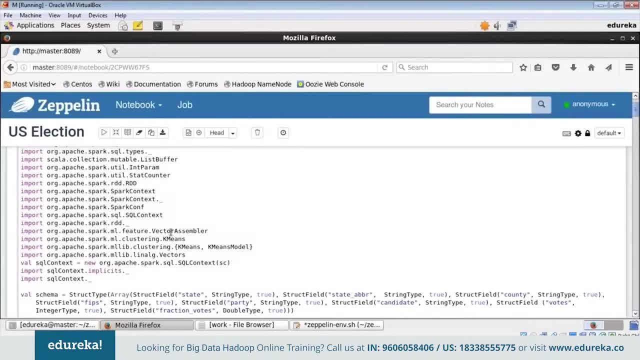 I have also imported the K-Means package Because I will be using K-Means clustering. Then the first thing that you need to do Is that you need to start the SQL context. So I have started my Spark SQL context here. 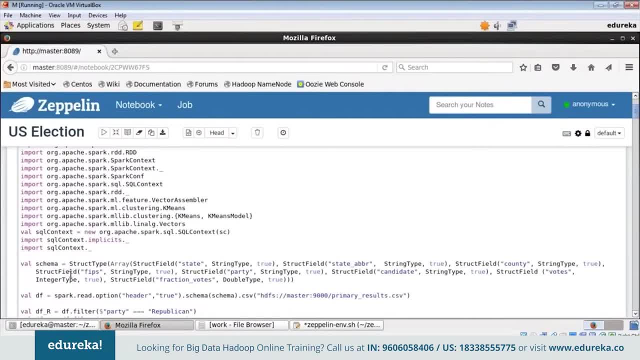 And the next thing that you need to do Is that you need to define a schema, Because when you want to dump our data set, Or we want to dump our data, It should be in a particular format And we have to tell Spark. 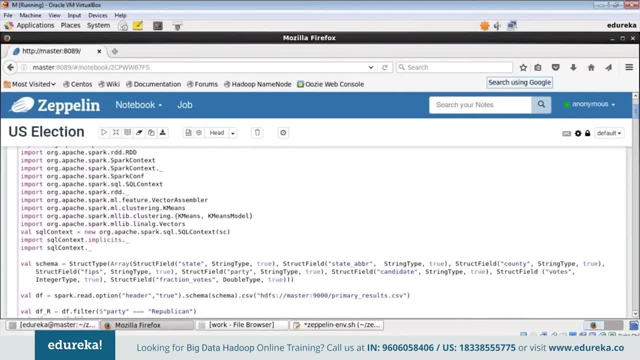 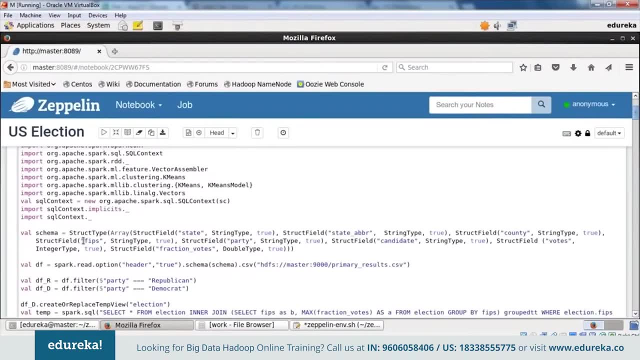 What it should be. So we are defining a schema here. So let me take you through the code. So I am storing schema In a variable called schema And we have to define the schema In a proper structure. So we are going to start with struct type. 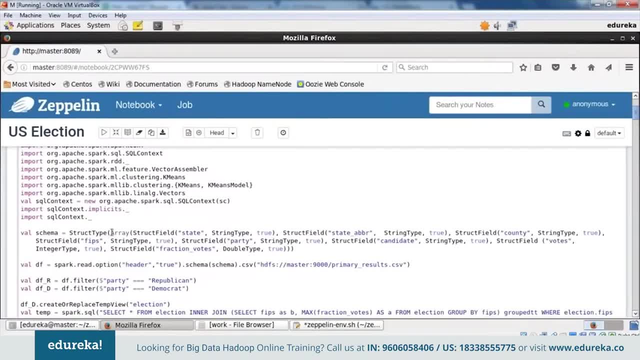 And since you know that our data set Has got different fields as columns, We are going to define this as an array of fields And this is an array and struct. So we are defining the different fields now. So we will start with the first field. 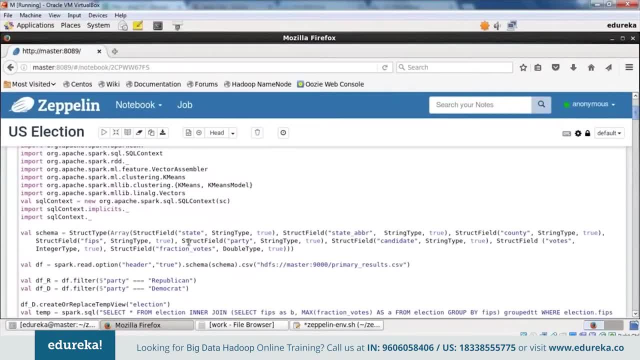 By defining it as struct field, And I have mentioned What should be the name of that particular field, So I have named it as state. It should be a string type And true, that means it is a string type. Next we have got FIPS. 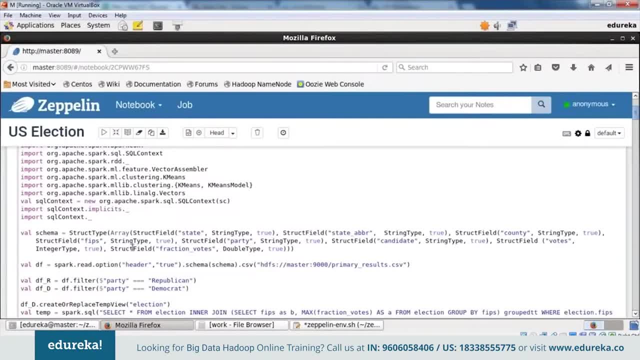 Which is of string type. Now, I know that FIPS is a number, But since we are not going to do any kind of numeric operation on FIPS, We are going to let it stay as a string. And we have got party as a string type. 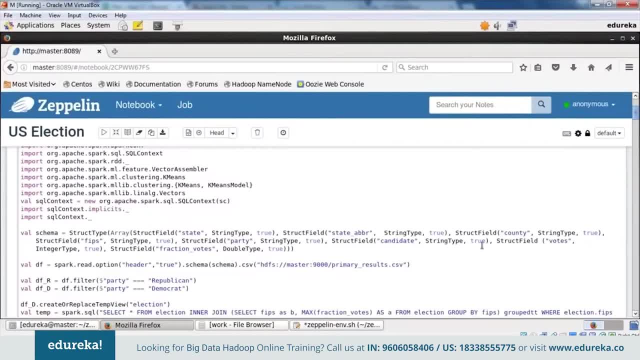 Candidate as a string type And then votes as integer type, Because we are going to count the number of votes And there is going to be certain numeric operations That we are going to perform That will help us to analyze our data. Then we have got fraction votes. 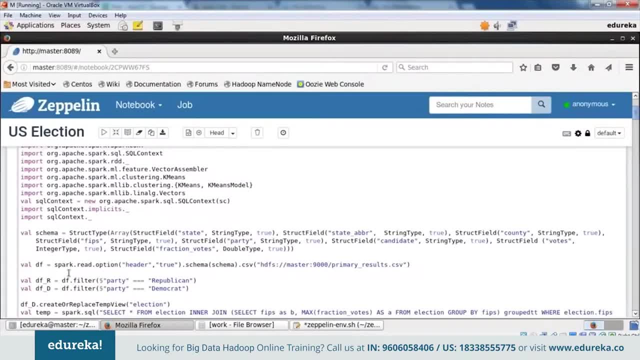 Which you know is a decimal type, So we have to keep it as double type. The next thing you need to do Is that Spark needs to read the data set From the HDFS, So for that you have to use the command. 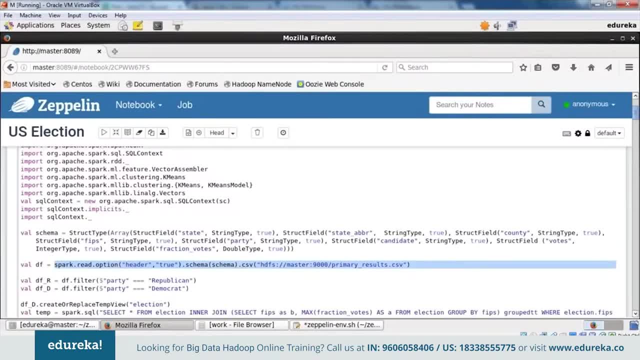 Spark read Option: header true. Header true means that you have mentioned And you have told Spark That my data set already contains column headers Because state as AVVR. But they are column headers, So you don't have to explicitly define. 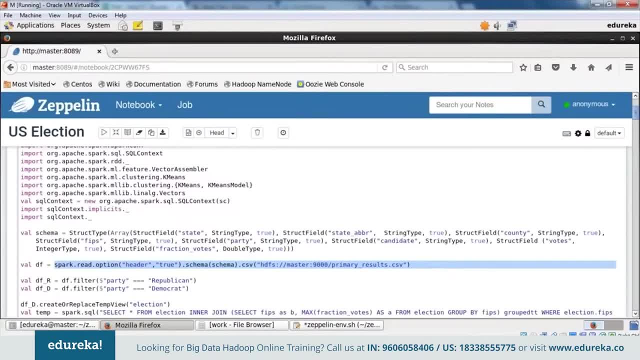 The column headers for it. Neither will Spark choose any random row As a column header, So it will choose only the column headers Your data set has. Then you have to mention the schema That you have defined. So I have defined it in my variable schema. 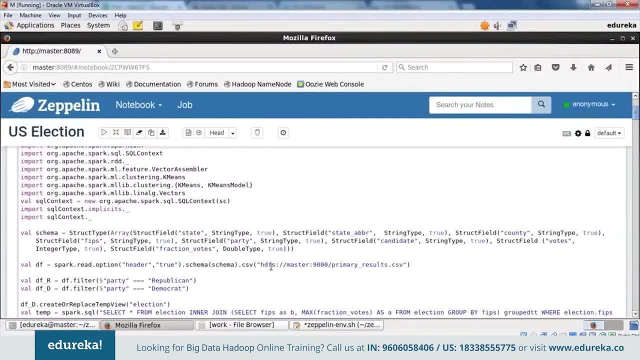 So that is why I have mentioned it in my file. It should be in CSV format. Then I have mentioned the path Of the file in my HDFS. This is the path Of my data set in my variable DF. Now what I am going to do. 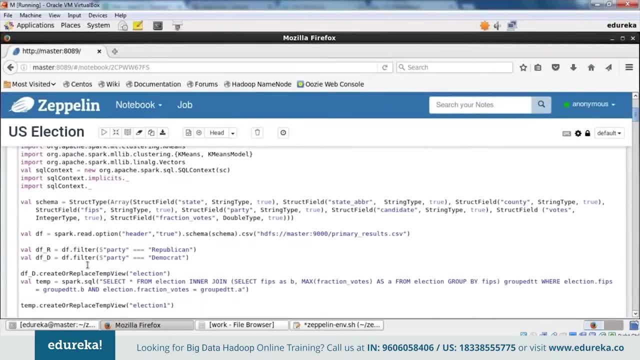 Is that I am going to divide up Certain rows from my data set, Because you know that my data set Contains both the Republican and Democrat data And I just want the Democrat data right Because we are going to analyze The Hillary Clinton and Bernie Sanders part. 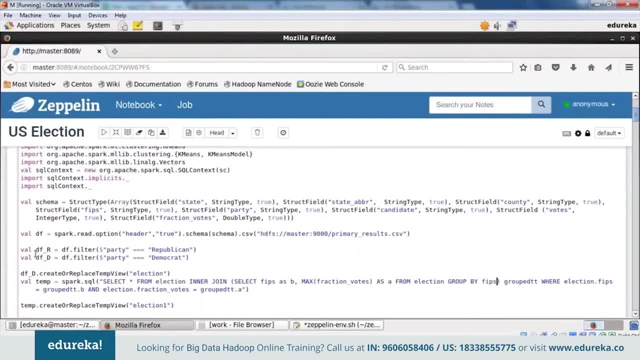 So this is how you divide your data set. So the first thing that we have done Is that we have created one more variable Called DFR And we have applied a filter To the Republican, And then we are storing the Democrat party data. 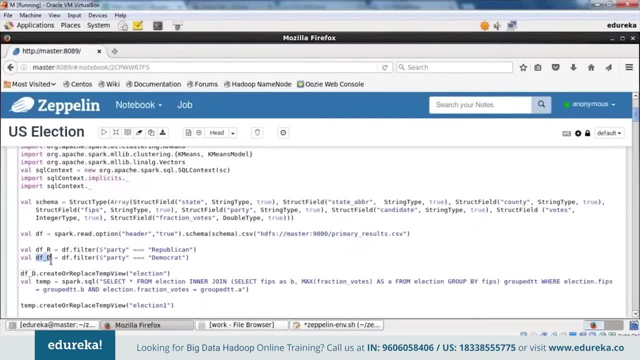 Into DFD, So we are going to use the DF underscore D From onwards, And DFR- the Republican data- Is going to be your assignment for the next class. Now I am going to analyze the Democrat data And then, after this class is over, 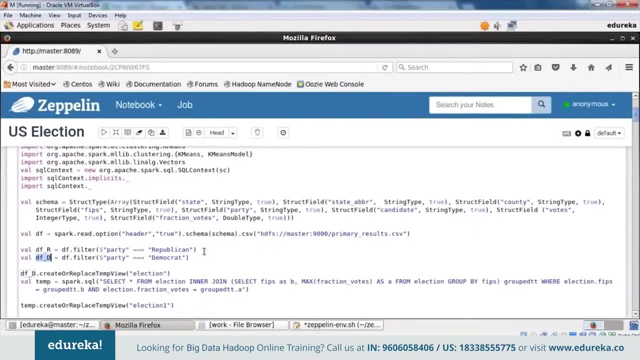 I want you guys to take the Republican data. This data set is already available In your elements And you have got the VMs Also with everything installed. So please, when you are at home, Just analyze the Republican data And tell me what were the reasons. 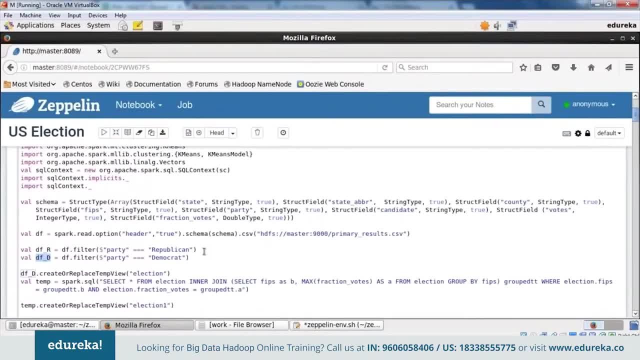 That Donald Trump want. I want you to do all that analysis And come up with that in the next class And we will discuss about it And whatever results and conclusions That you have made after analyzing The Republican data, And that way, you will also learn even more. 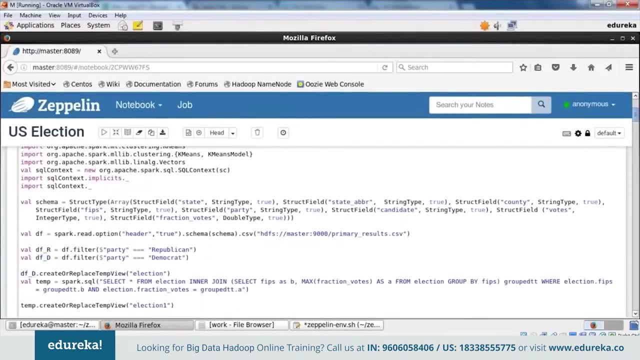 And it will also be practice for you After today's class. So we are going to take DF underscore D now, And the first thing that we will do Is that we will create a table view As election, And let me just show you what it looks like. 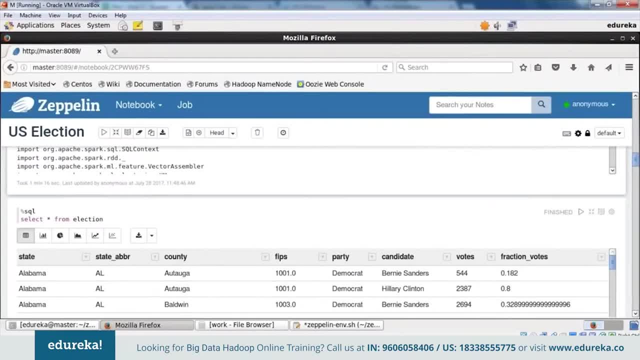 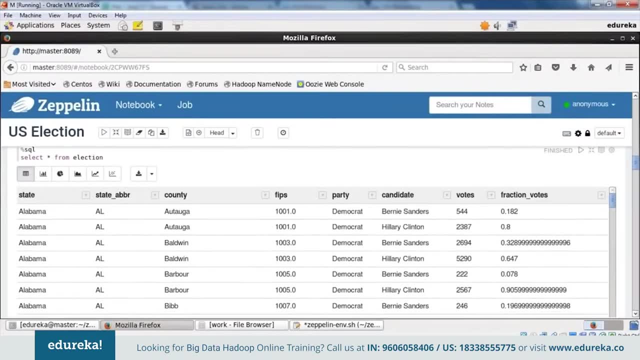 And what it has. So this is the command that I have run in Zeppelin. So this is SQL code That I have run in Zeppelin And you can see that I have got states, State underscore, ABVR And I have only got the Democrat data. 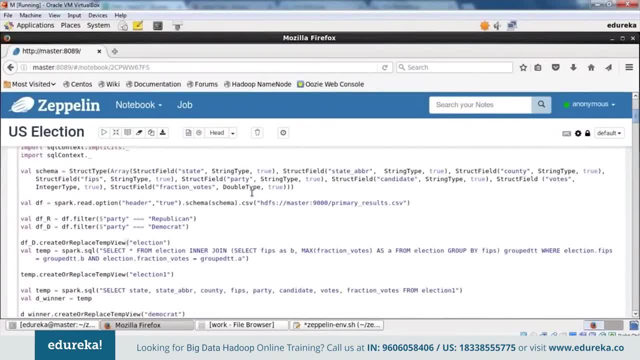 Alright, Let's go back. Alright. So, after creating the table view, Now all of the Democrat data is in my election table. So now what I am going to do Is I am creating a temporary variable And I am running Spark SQL code. 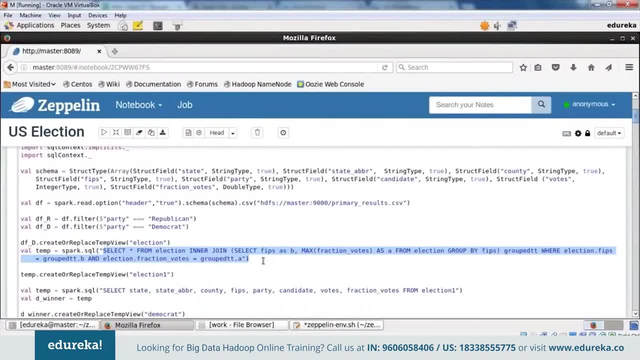 So what I am actually doing by writing this code, The motive of writing this SQL code Or the SQL query, Is that I want to refine my data even more. So what I am trying to analyze here Is how a particular candidate actually won. 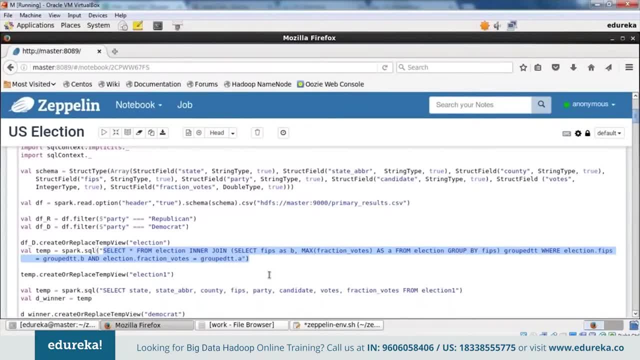 I don't have to do anything with the losing data, Because you know that each of FIPS contain One of the losing candidate members And one of the winning candidate members. It contains the data of the winning candidate And the losing candidate also. 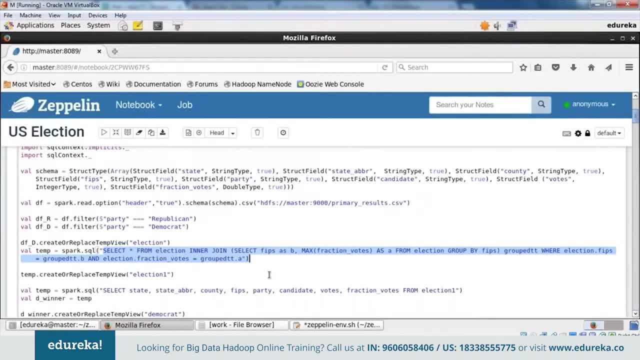 It contains the data of Bernie Sanders and Hillary Clinton. In some parts, Bernie Sanders won And in some counties Hillary Clinton won, So I just want to find out That who are the winners in a particular county? Okay, So I am going to refine that data. 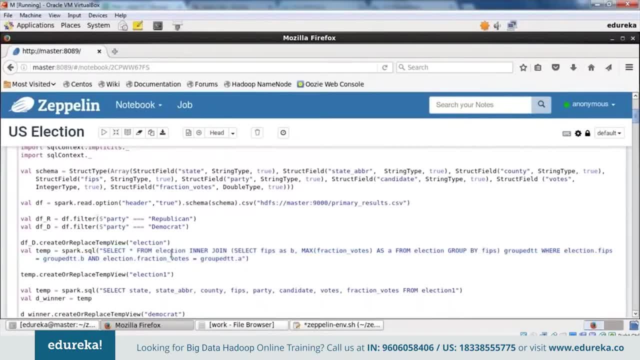 And for that I am using this query. So I am going to select all from election And then I am going to perform an inner join With their query. So this is one more query inside this query, And let me tell you what I am actually doing. 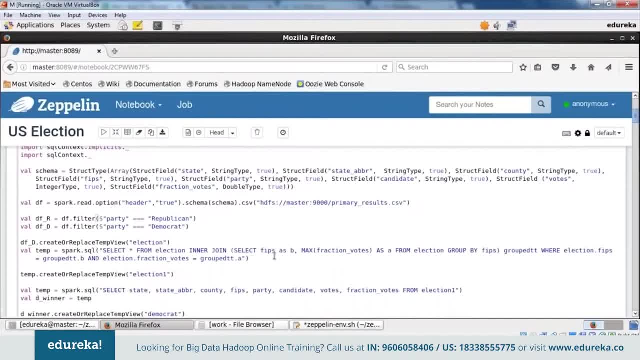 So first of all, What we have done is That we have selected FIPS as B. You know that now You have got two entries for each FIPS, So each FIPS actually appears Twice in the data set. So I have named it as B. 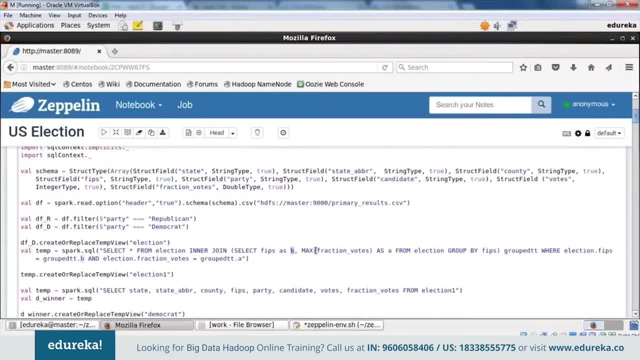 And now we are counting the maximum fraction votes. So you know that in each FIPS We have the maximum fraction vote And then we can find the winner By actually seeing who has got the maximum fraction votes, And then we have named it as A. 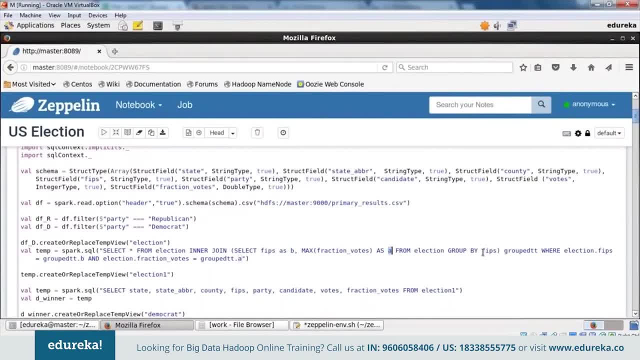 The maximum fraction votes. column Is named as A And we are grouping by FIPS. Each of my FIPS will be selected Which has a maximum fraction vote And I have two columns for that FIPS, which is 1001.. 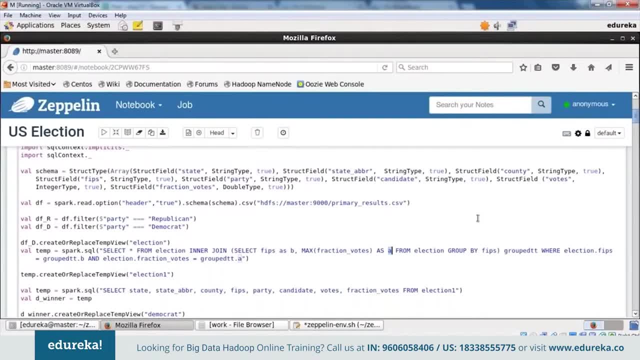 And 1001.. So the only row will be selected Which has the maximum fraction votes. Now I will have the winner data And I have named this entire table Inside this query As group TT, And then I am validating it. 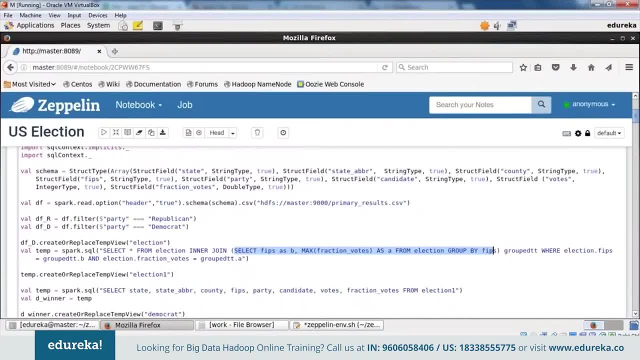 As where electionFIPS, The main table viewFIPS Should be equal to the B column And electionFractionVotes Should be equal to group TTA. So any doubts On this query And about how I have written this? 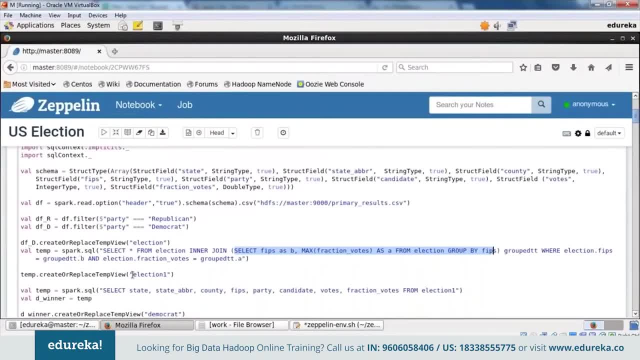 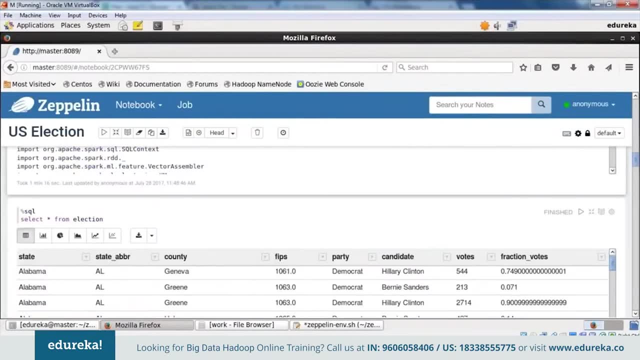 So now what we are going to do Is that whatever data that we have got here, I am storing that in election 1.. Let me just show you What is in election 1 now. So this is my election table only, And you can see that I have got two FIPS. 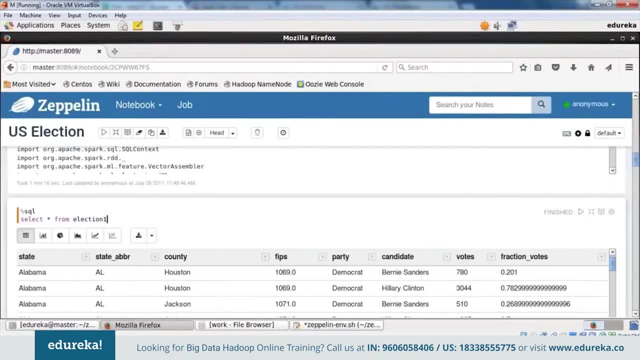 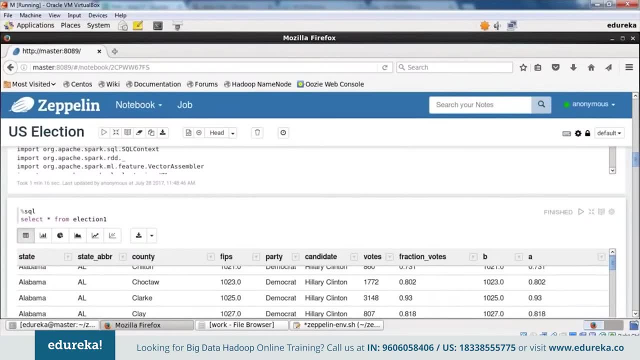 So 1067.. 1067.. Now let me show you election 1.. So there, now I can see that I don't have repetition of FIPS. I have only One entry for FIPS And that is the row which tells me. 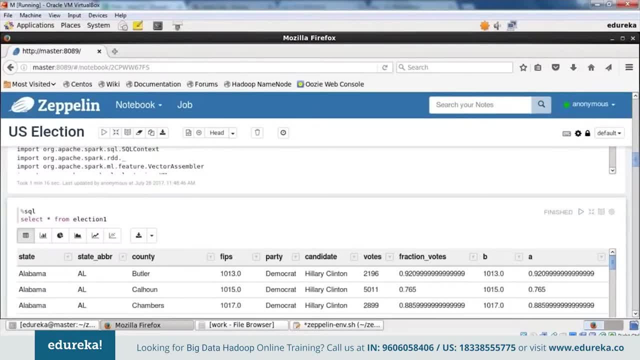 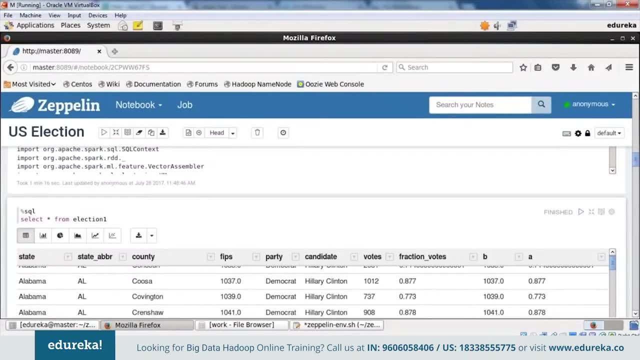 Who won in that county, Or in that particular FIP, Or in the FIP associated with the particular county. And you can see: for Bullock It was Hillary Clinton, For Cahoon it was Hillary Clinton, Cherokee also Hillary Clinton, And then State House District 19.. 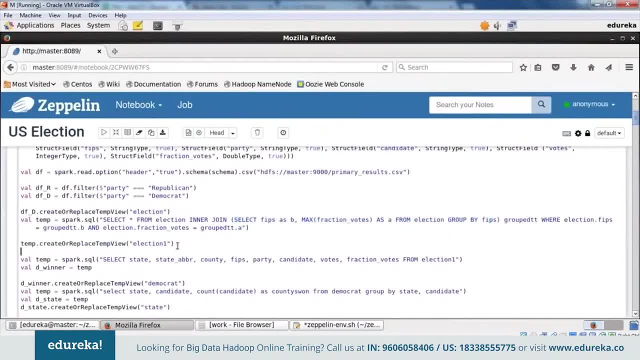 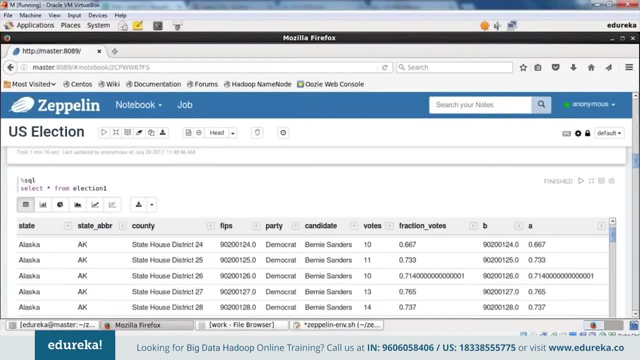 Is Bernie Sanders. So this is what we have done now, And then you can see That we have also got additional columns As B and A. So A tells you the maximum fraction votes And B tells you the FIPS. So the data in FIPS. 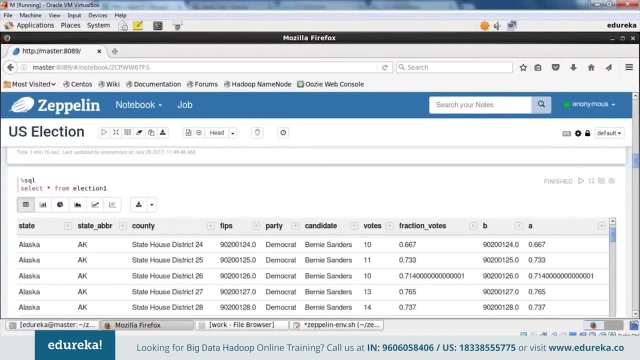 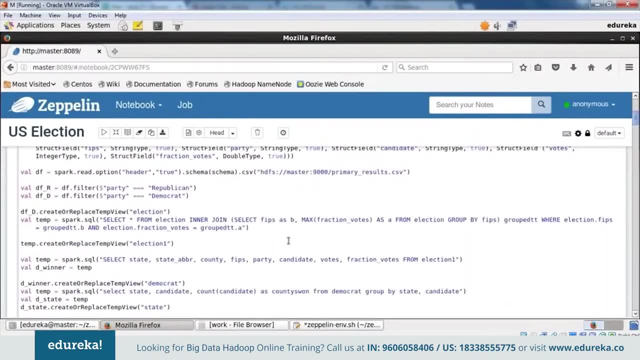 And the data in B are the same And the data in fraction votes And the data in A is the same, Right? What I am going to do now is, Since my columns are repeating And they have the same value, So what I am going to do is. 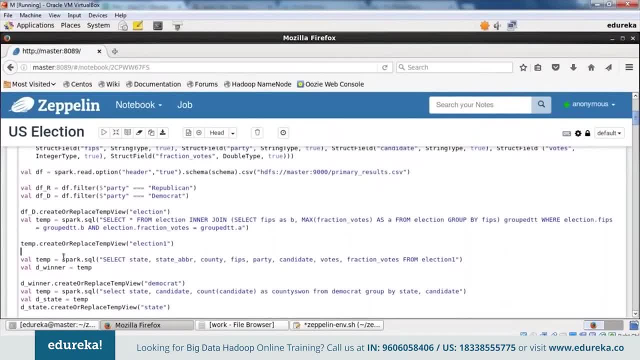 I am going to filter out the columns I don't need- And in this case I don't want B and A, And what I am going to do is I am going to make a temporary variable again. So I am using the temporary variable. 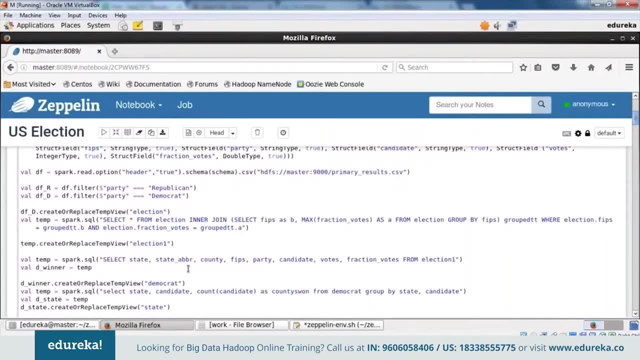 To store some data temporarily. So I am writing to the Spark SQL code To select only the columns that I want. I want the state, State abbreviation, county: FIPS Party candidate votes. Fashion votes from election one. I am storing everything in DWinner. 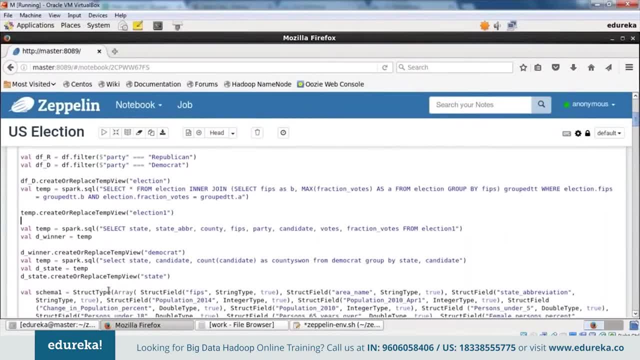 I have created this new variable In temp, I am assigning it to DWinner And now I have got only the winner data. So I have got all the counties And I have got who won in that particular county And by how much in the fraction of votes. 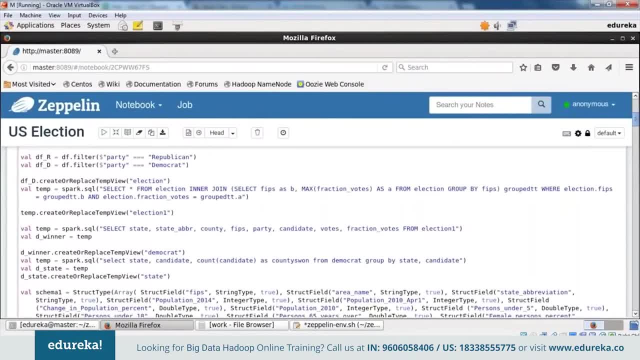 What I am just doing till now Is that I am just refining our data set So that it will be easy for us to make some conclusions Or gain some insights from that data Right. And also let me tell you that it is not always necessary. 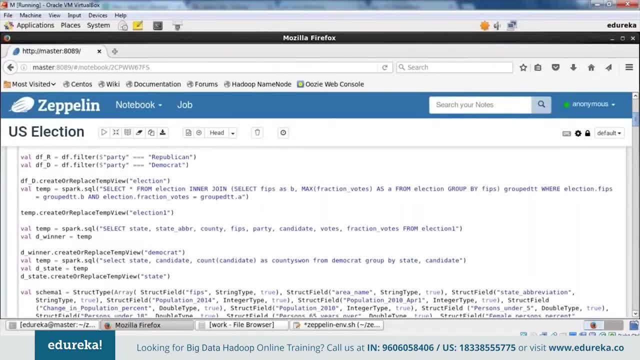 That you are filing your data set In the exact way that I am doing it. If you have something in mind And understand your data And you find out what actually you need to do, You can carry out different steps to do that also. 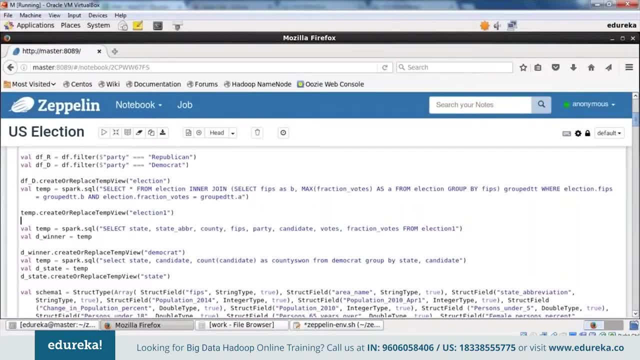 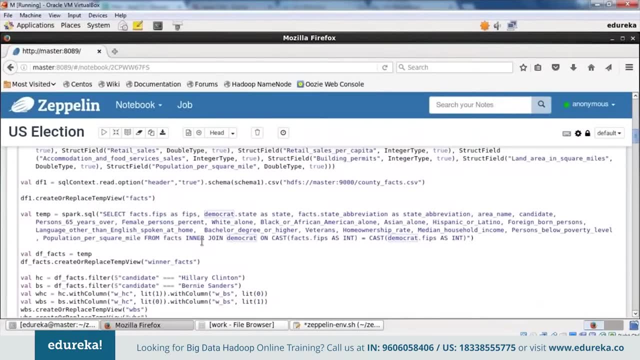 This is just one way of doing it And this is my way of doing it. So I am just telling you. And then we are creating a table for DWinner And we are going to name it as Democrat. So let me go again. 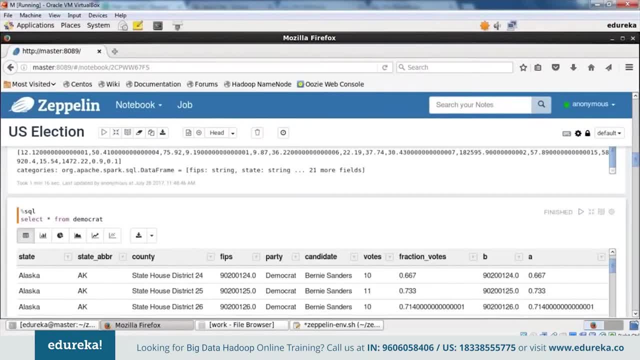 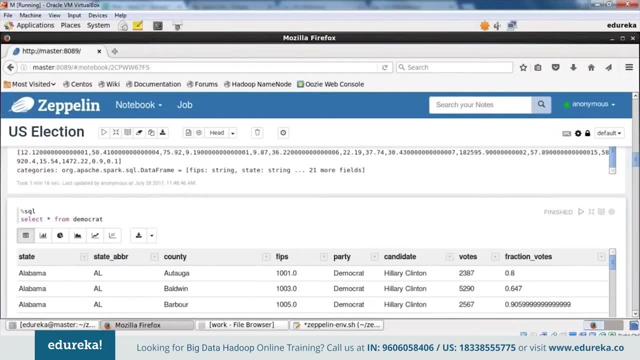 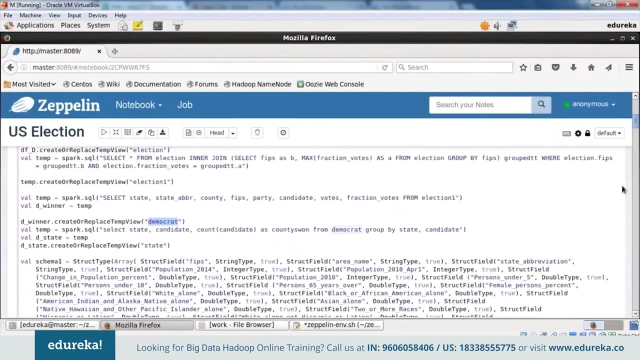 And let me show you what the Democrat table view looks like. You can press shift enter. So there you have. We have column A and B That we had in election one, And so I have just got The winner data. So now, 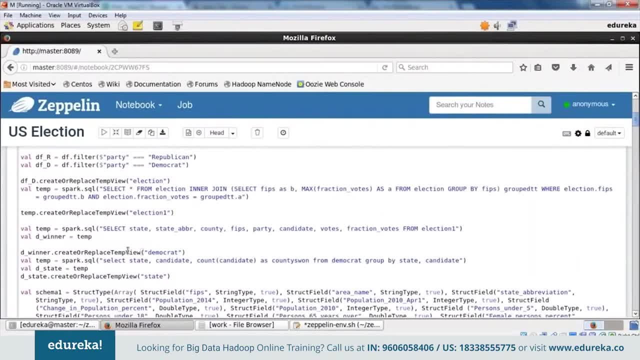 Let us go back and find out. What we are going to find Is that I want to find out That which of the candidates Won my state, And then, whatever date and whatever result Will be stored in the temporary variable When I am assigning everything. 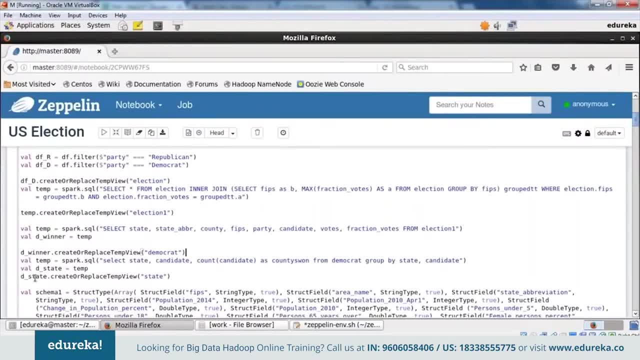 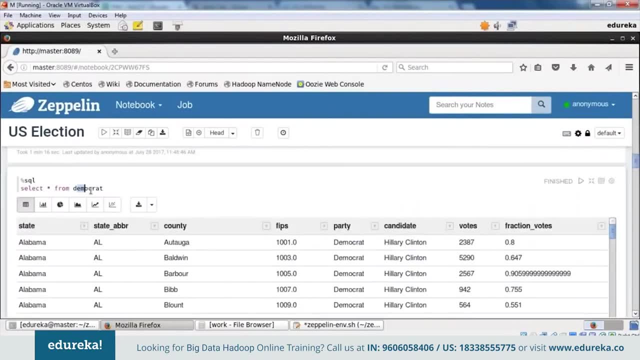 That will be stored In the temporary variable to a new variable Called DState. Similarly, I am going to create A table view for DState, Which is state. Let me show you what my state table view actually contains. So there it is. 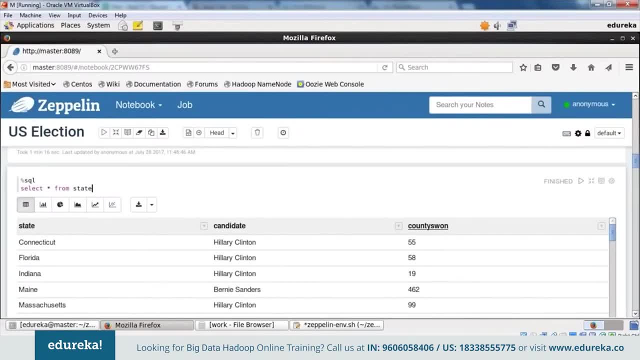 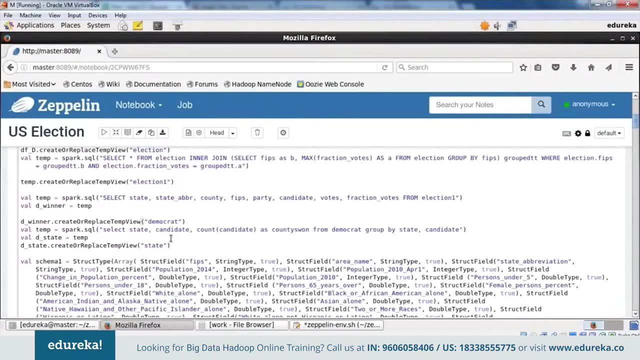 So I have got state Connecticut: Hillary Clinton won 55 counties. Florida: Hillary Clinton won 58 counties. So this is what we have come up to for our first data set. So now let us see what we can do with our second data set. 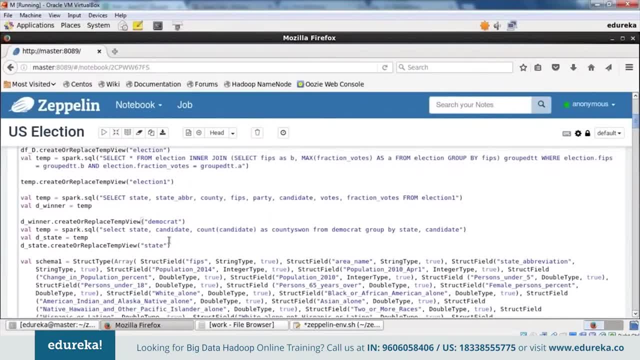 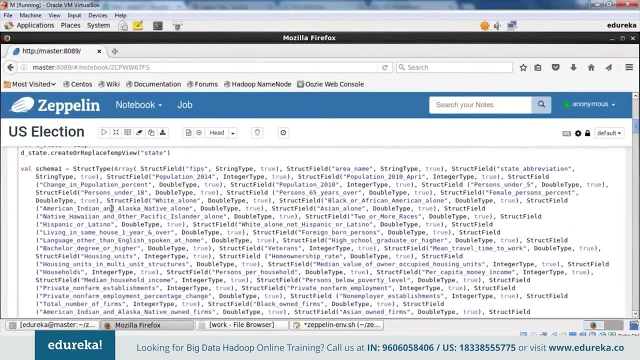 That contains all the different demographic features. First thing: Again, you have to define a schema. This time I am naming that schema Schema 1. Since you know that we have got Almost 54 columns, So I have to define all those 54 columns. 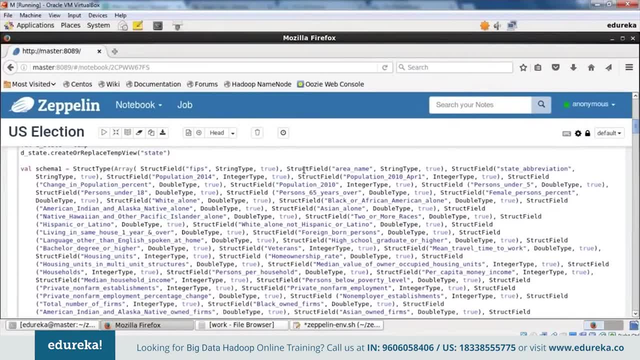 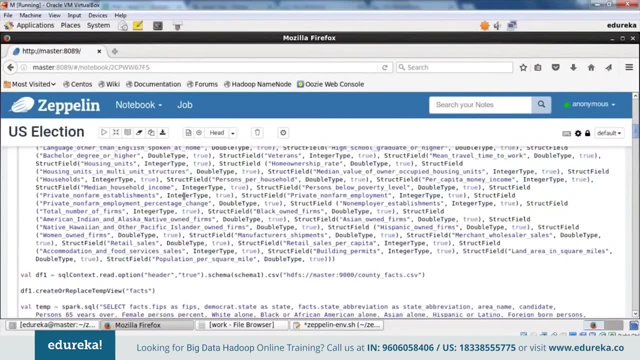 Also So you remember what Each of those columns contains. So this is exactly what I have done And I don't need to go through every line. But, like I already told you How to define a schema, You can have the code in your LMS. 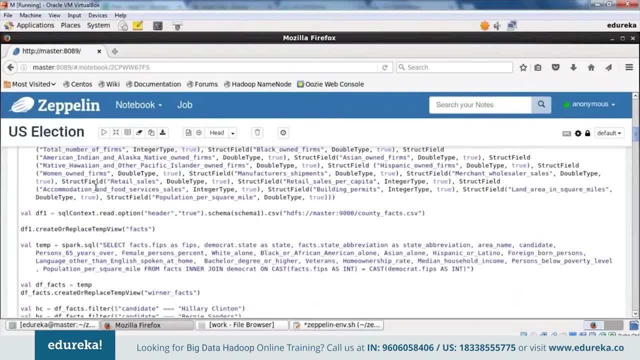 So you can take a look at it. So the next thing we are doing Is to create a data set, And I am storing my data set Into a new variable called df1.. And this is the path in my HDFS Where my data set was. 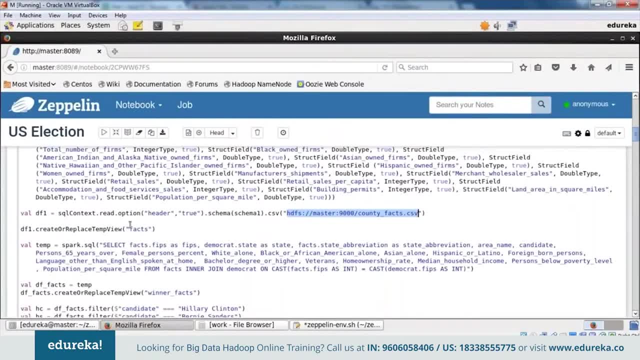 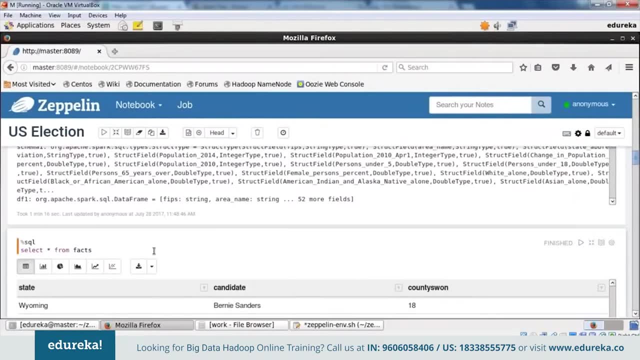 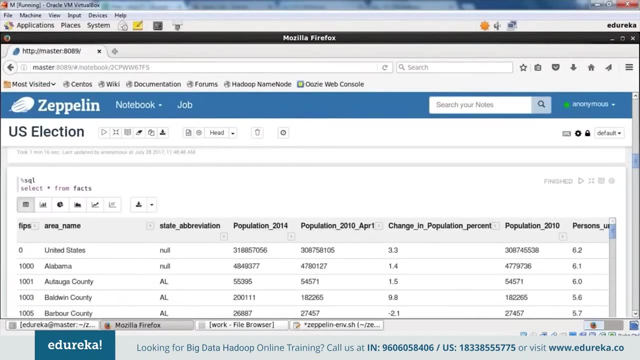 And then I have created a table view For my data set, Which is called facts. Now let me show you What facts contain. As you can see That it contains abbreviations: State abbreviation- Population- 2014.. So, instead of using the code now, 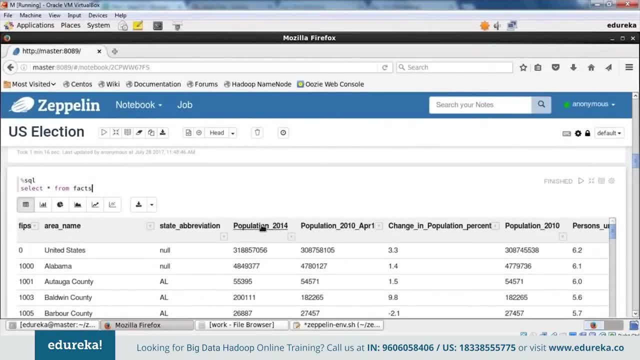 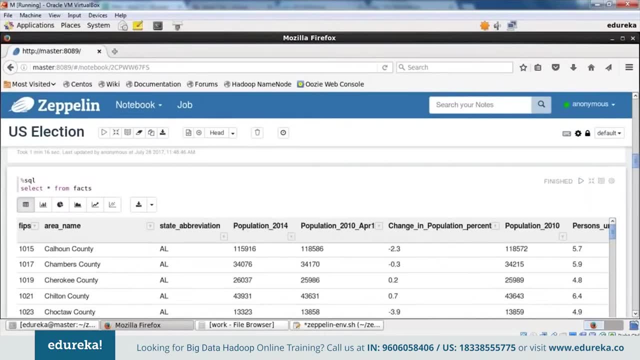 Or the encoded form That was actually there. in my data set, I have given a varied meta name That would describe what it contains, Right? So instead of PST 214.. I have got population 2014.. So does that make sense? 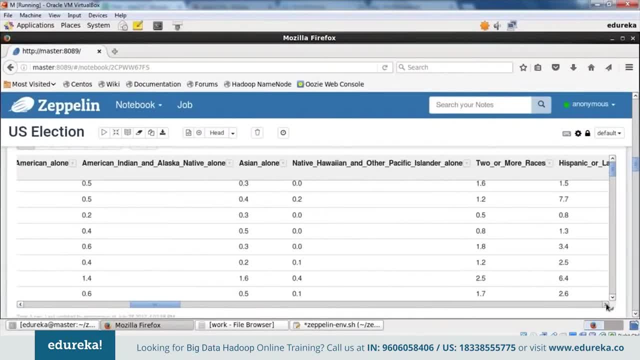 It contains all the 54 demographic features Or different features That was in my data set. White alone, Not Hispanic or Latino. Living in the same house Same year and over. Foreign born persons. Language or other than English Spoken at home. 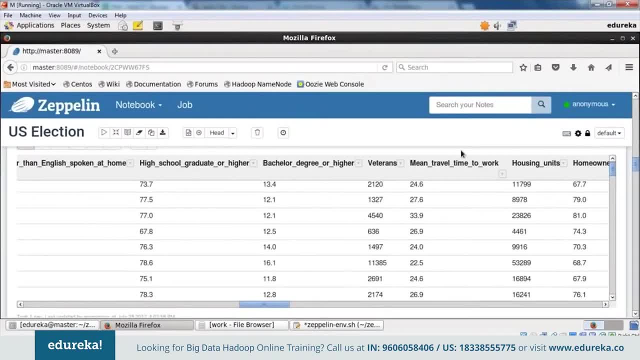 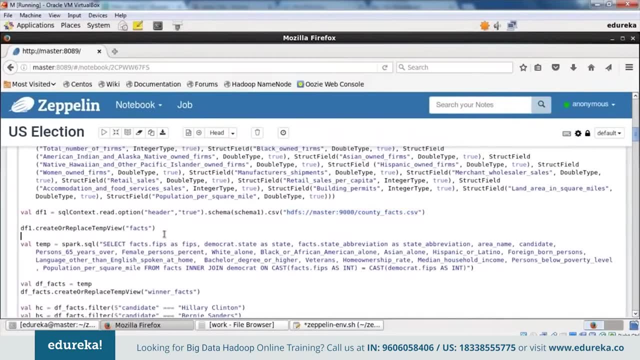 High school graduate or higher. So it contains basically all the different features Or all the different columns. That actually was in my data set That I have defined in my schema. So this is what facts I have. So now what I am going to do. 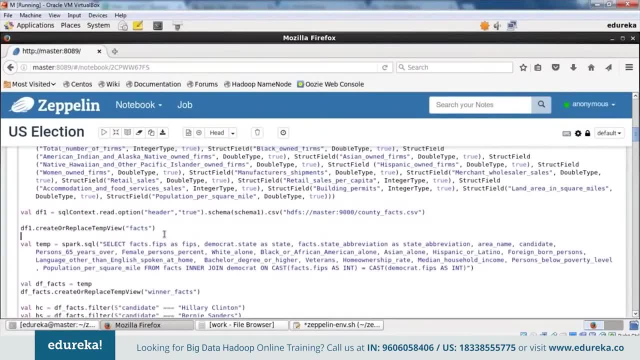 Is that I am not going to analyze my whole data Based on all these different features. I am going to choose some specific features In order to analyze it. Add one. So these are the different features That I am going to use. 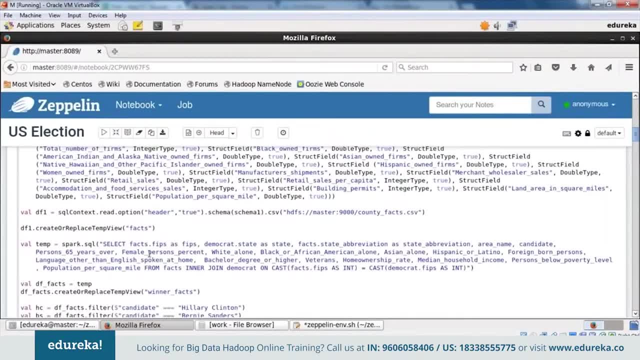 I am going to use FIPS. I am going to use state. I am going to use state abbreviation, Then area name. Candidate and people who are over 65 years. Senior citizens. Female people. White alone. Black African alone. I am choosing Asian alone. 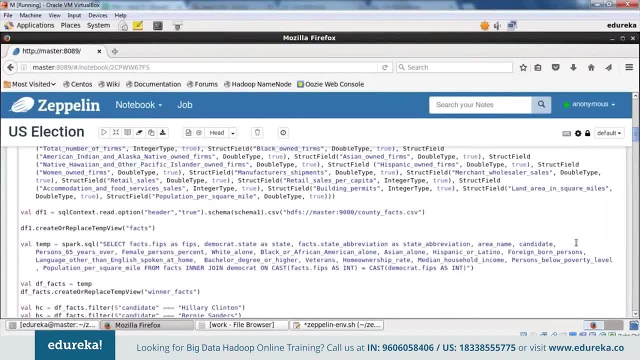 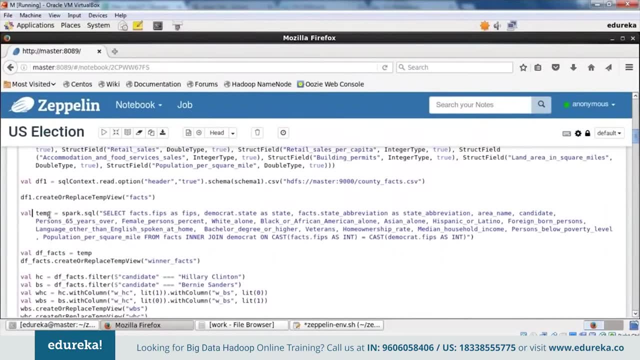 Hispanic or Latino. So I am choosing white people, Black people and Hispanic people. So I am just trying to analyze it And you know that I have stored this In a temporary variable again And then whatever result I will get By running this Spark SQL code. 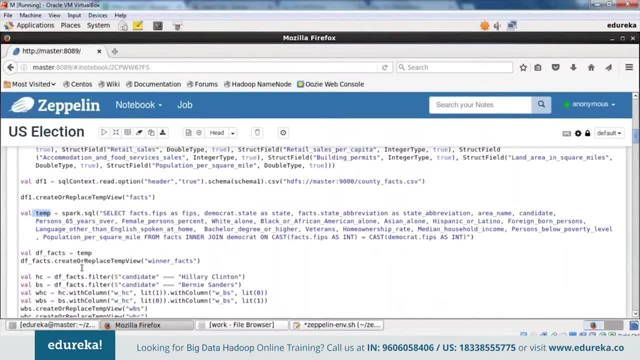 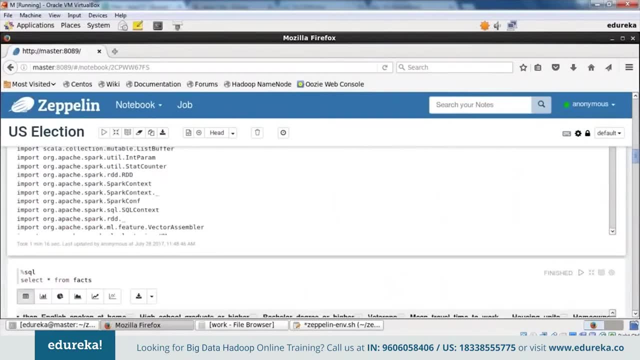 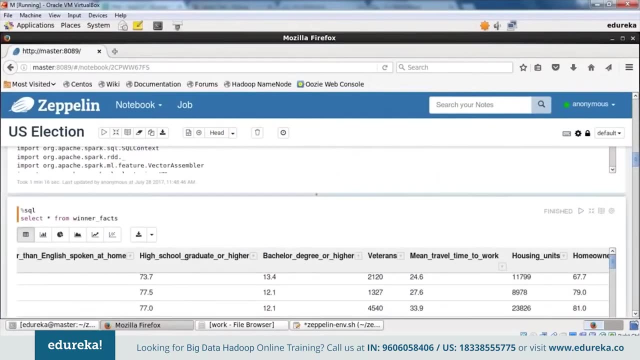 I will store it in a different variable Called DFX, And then I will make a table view For DF facts, such as winner facts. So let me show you What winner facts look like. So it is winner facts At FIPS. The state is Alabama State abbreviation is AL for Alabama. The area name Is Artuga County. The winner was Hillary Clinton And the people over 65 years In that particular county Is 13.8%. Female percentage is 51.4%. 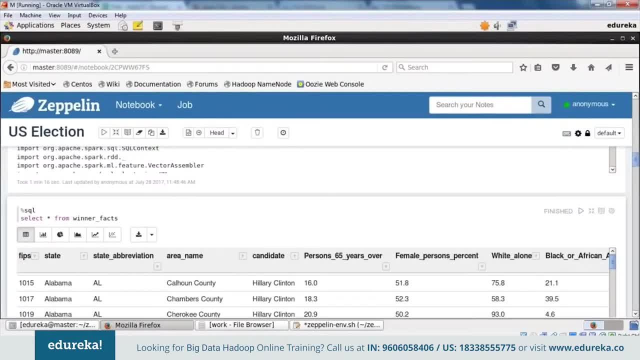 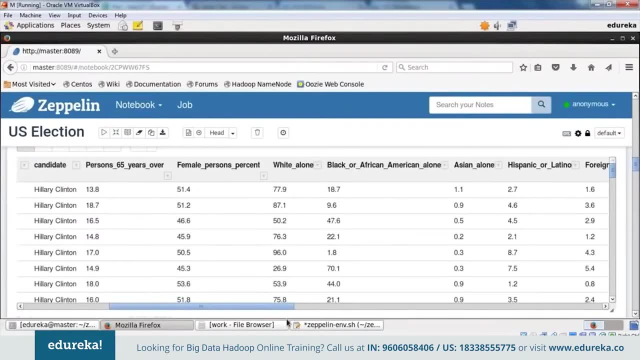 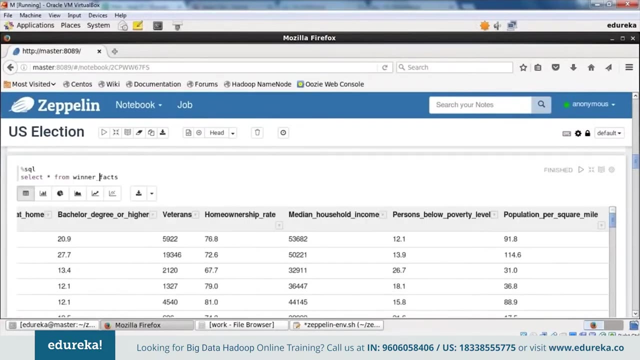 White alone: 77.9%. And so these show you the data. So Black, white or African Is Asian, 18%. And then I have got the different fields That I have selected: Asian alone, Hispanic or Latino, Foreign born. 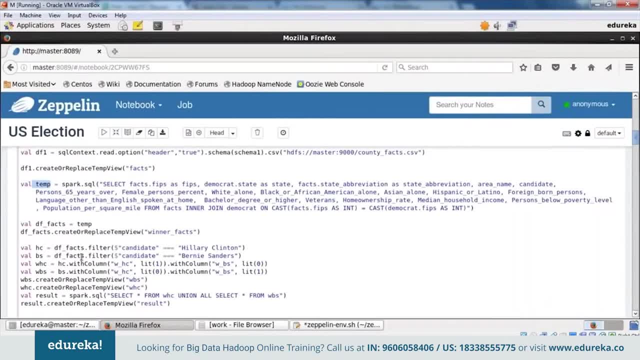 So I have chosen 14 features to analyze it from. Alright, So now what I am doing again Is that I am going to divide the Hillary Clinton data And the Bernie Sanders data So that we can analyze only why Hillary Clinton won. 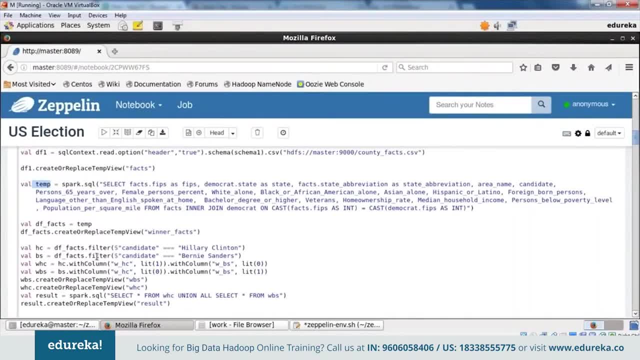 Or why Bernie Sanders won In some particular counties. So I am going to divide the Hillary Clinton data From our initial primary result data set. So this is what you have done. So you know that is stored in DFX, So we are putting a filter in DFX. 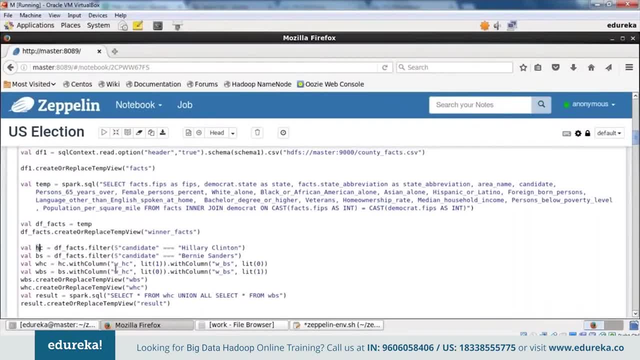 Where a candidate is equal to Hillary Clinton, So that will be stored in HC And the data of Bernie Sanders will be stored in BS. So after that, What we are doing Is that we are doing a one hot encoding, So we will add two more columns in our data set. 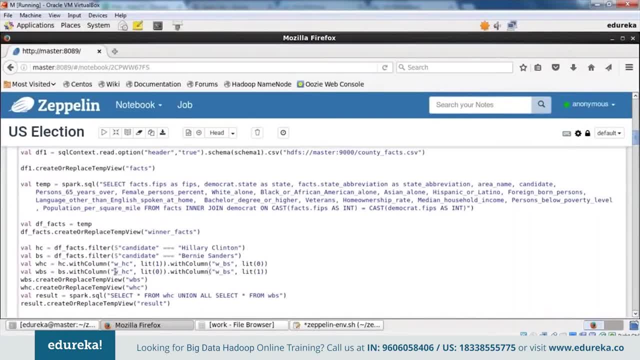 A WBS and WHC. In this case, We are going to do one hot encoding And what we are going to do Is that we are going to include Or we are going to attach two more columns In winner facts As WHC. 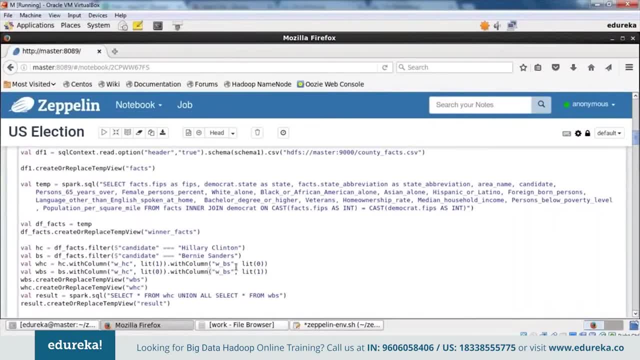 And WBS. So it will just contain Either one or zero. So you can edit it in that way, Whichever county. So if you are considering a county, Let's say Artuga County. Say if Hillary Clinton is the winner. 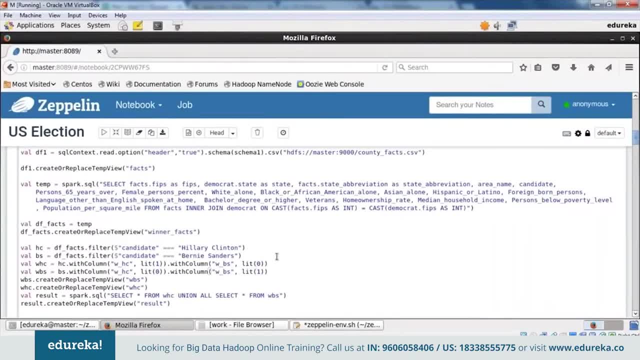 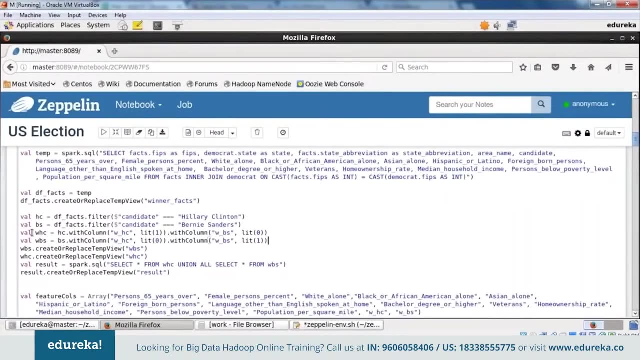 It will have a one In WHC And in WBS It will have zero. Similarly, in which counties Bernie Sanders won, So Bernie Sanders will have one, So WBS will have one And WHC will have zero. And then we are creating different views. 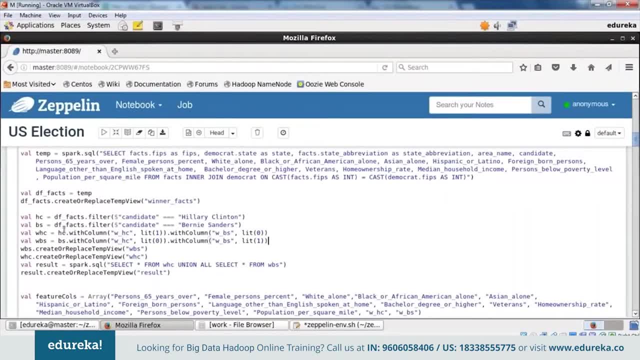 For both of these two together. So this will only tell me Wherever WHC is one. That means this will only show me The counties where Hillary Clinton won. This will only show me the counties where Bernie Sanders won, And we are creating a view. 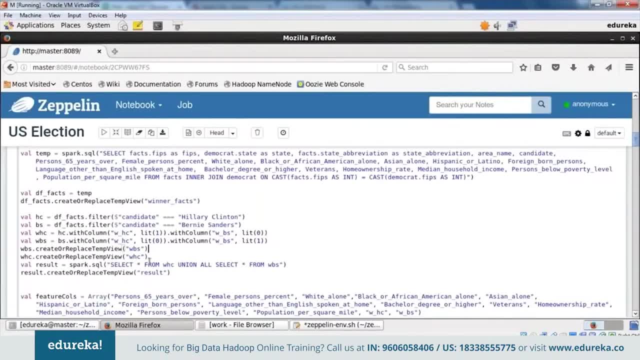 For both of these. So for Bernie Sanders the view is WBS And for Hillary Clinton it is WHC. Then, finally, we are merging both of them together using union. So select all from WHC Union, all select from WBS, And finally you have stored it. in result, 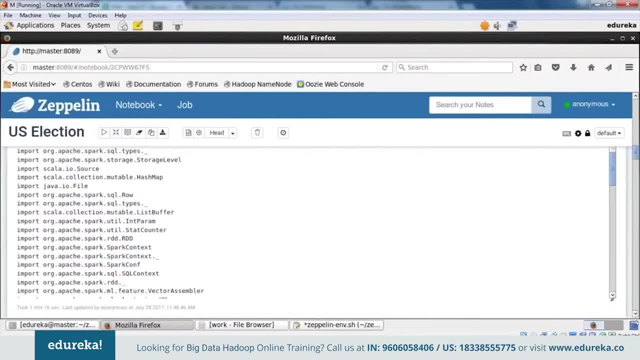 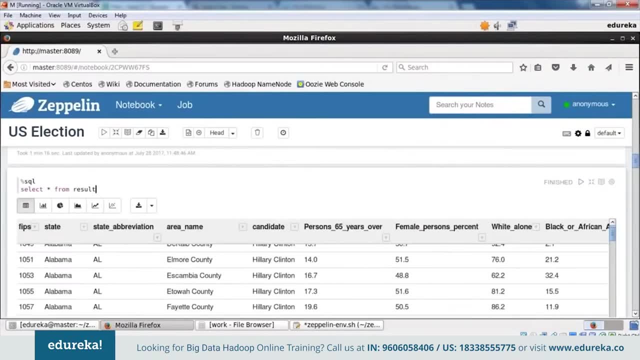 And we have created a table view, Known as result. So let me show you what this result contains. So there it is. For Artuga it was Hillary Clinton, So we have got the Bernie Sanders data Over here At the bottom. 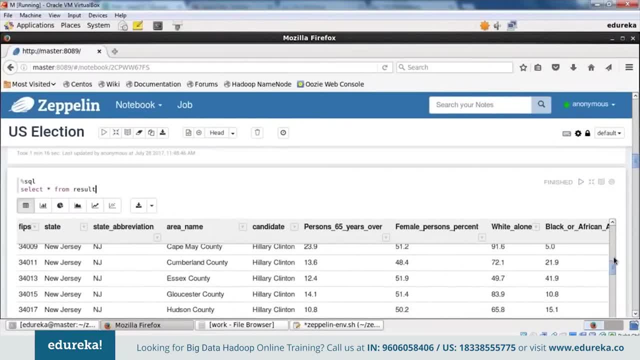 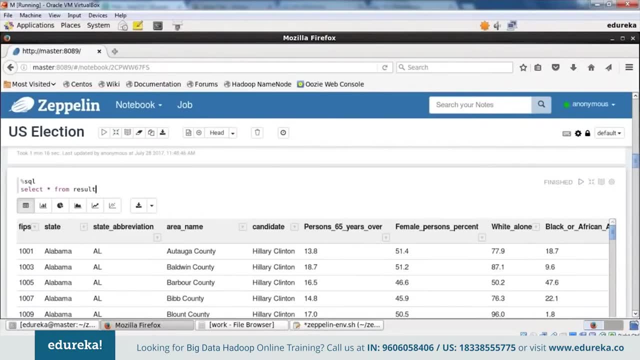 I have got all the different fields, Also from my Second data set, The different features That I chose from my second data set To analyze it. So now comes the actual analyzing part. This is where we are going to perform k-means. 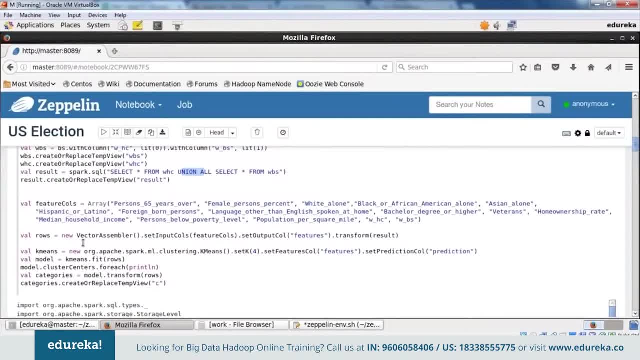 But first we have to define The feature columns. Actually, you have to define what is the input That you are going to feed So that you get an output. So this is actually the input That you are going to feed To the machine. 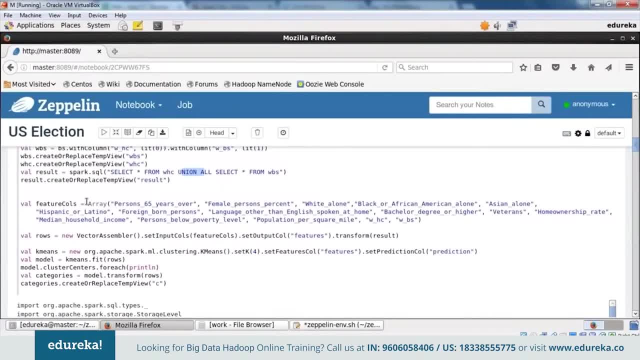 So that the machine learning goes on And finally it gives you some kind of result, Right? So this is where I am defining. Again, I am using an array to define all the different fields From my data set. So I am using person: 65 years and older. 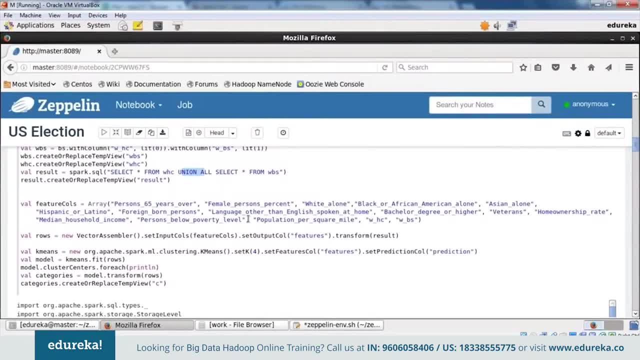 Female person percentage. White alone or black or African American alone. Asian alone. Hispanic or Latino. Foreign born persons. Language other than English. Income Persons below poverty level. Population per square mile, WHC and WBS. Then I am going to use the vector assembler. 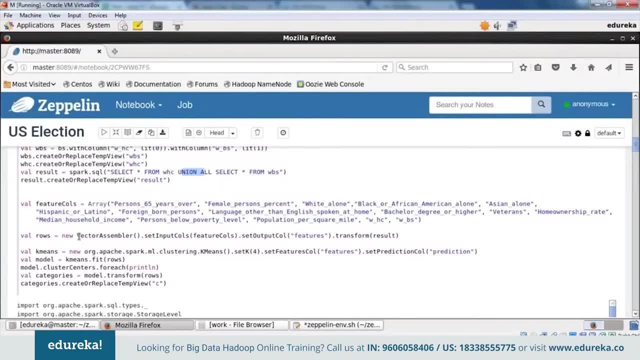 So this is what enables different machine learning algorithms Where we are using k-means. So my input column Is features calls. So this is going to be the input And my output column Will be called features. So whatever result that I am going to get, 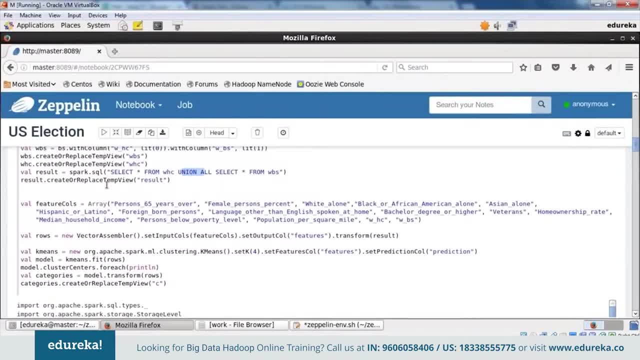 Is features And we have to transform The results. So this is the final table view that we have created, And you know what transforming means, Or transforming again means. So in our strategy We already saw that we have to transform the data first. 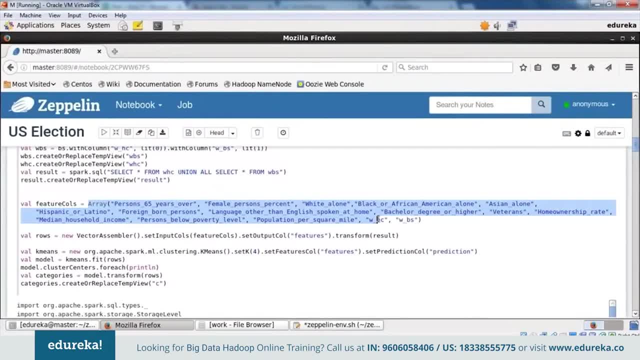 So my updated data set was results. So I am going to transform result And put columns as going to be these, Which is feature columns, And output table view Will be called features, And then we are going to perform the k-means clustering. 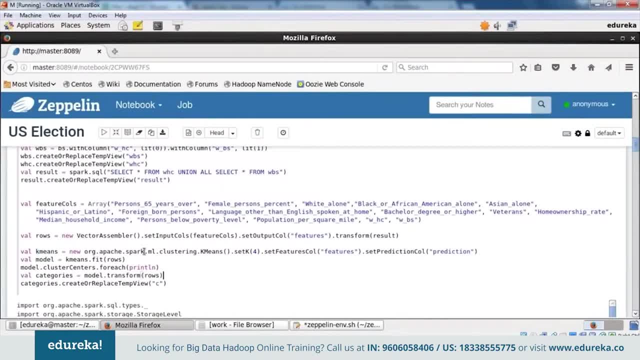 And we are going to store it in a variable called k-means. So we are using different functions From spark library And we have chosen spark With clustering k-means. And you know that in k-means We already defined. 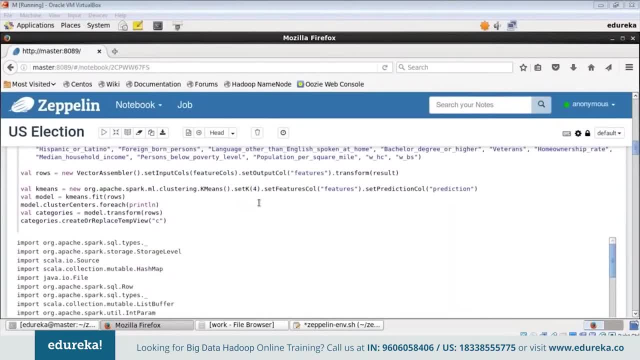 That. how many clusters do we need? And we need four. So we have selected four clusters And then we are going to set feature columns as features And then set prediction column As predictions. So after that we are going to make a model. 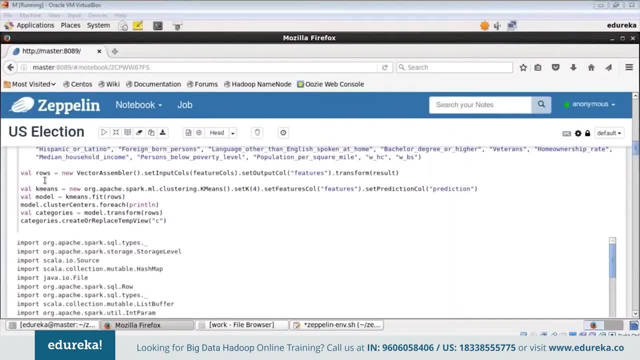 And we have defined our input And output columns in rows. We are going to use keynesfitrow And whatever predictions we will get, We are going to store it in a model And then we Are going to do this And that we are going to print the cluster centers. 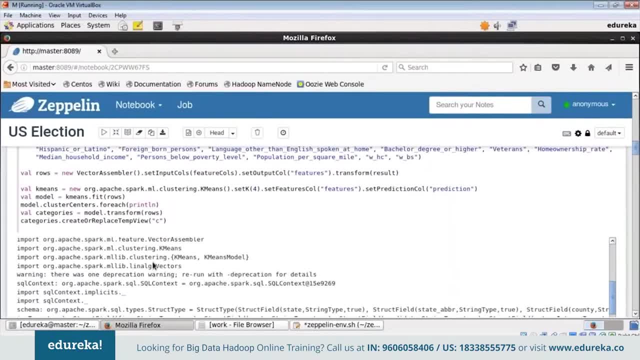 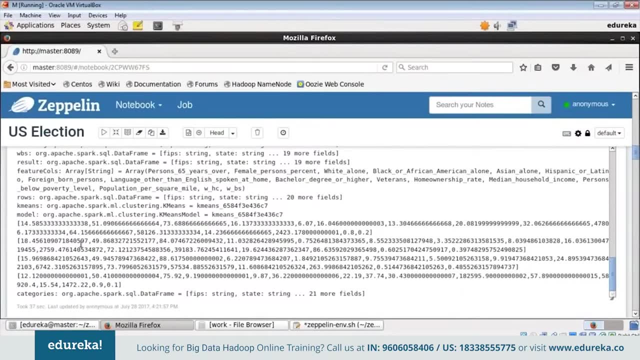 For each cluster. So let me show you what my cluster centers are. So after we run this code, You can see that these are the different cluster centers. So just what I can make you understand About what we are going to do After k-means clustering. 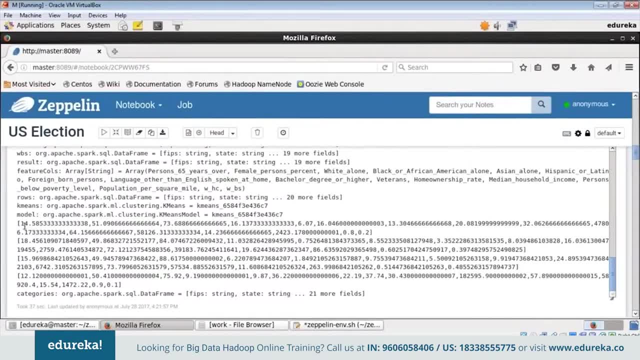 And how to analyze it. So the numbers are present. They are placed very haphazardly. So what I have done Is that I have picked out each of the cluster center points And then I have made a new table. Yes, 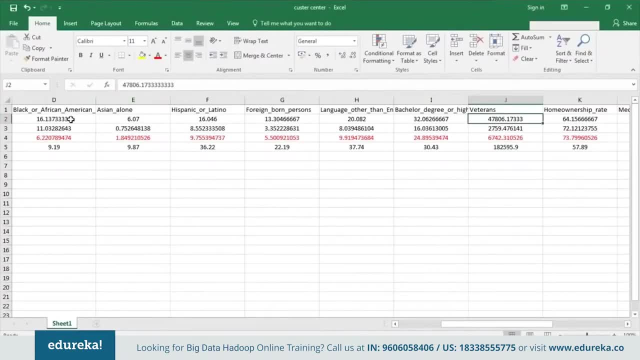 So this is it. So you know that we have four clusters. We have got the zeroth cluster, First cluster, Second cluster And third, So zero. one, two, three, So four clusters, And we have found out this cluster centers. 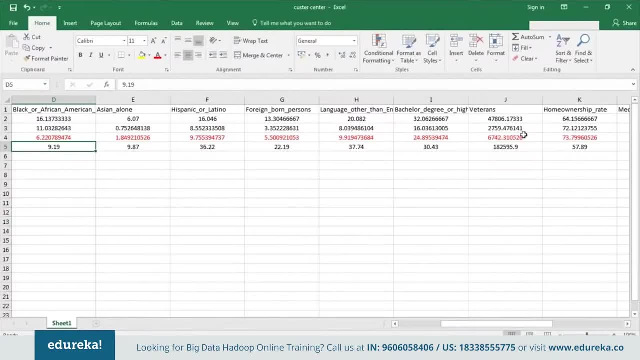 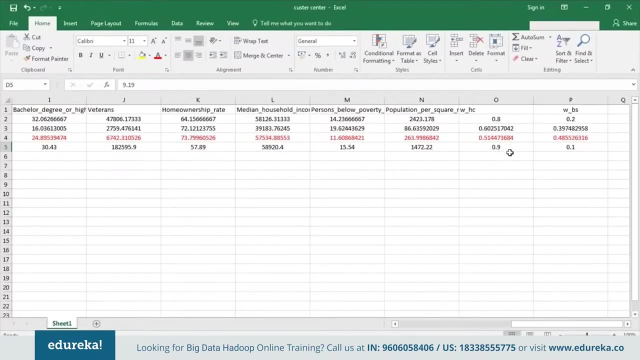 That we fed into my k-means algorithm. So what we observed here In WHC and WVS Is that the winning percentage Or the winning chances of Hillary Clinton Was 0.9.. Whereas winning chances for Bernie Sanders Was 0.1.. 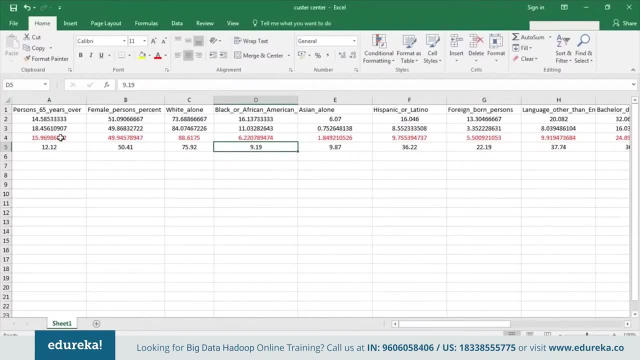 And then If you observe The differences in the cluster centers For each feature Here, you can see that there is not much difference, Not even here: 50, 49,, 49,, 51. And then It is well. 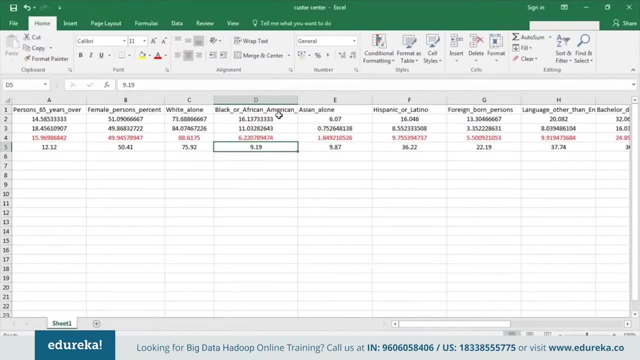 Again, it is not much of a difference. But if you see here that it is 9. And it is going to 16. So you can do a more detailed analysis On black or African American. So if you want to know the real support, 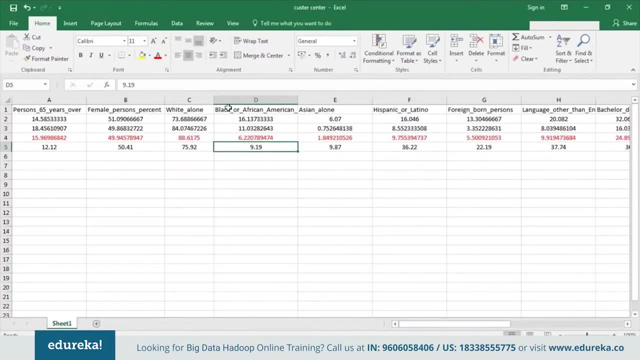 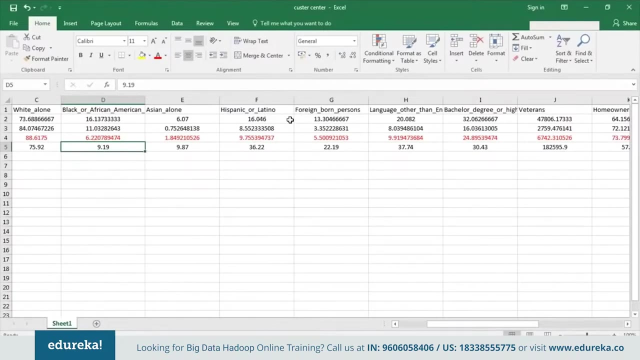 Of black or African American And you want to see What was Their voting pattern Or how popular was Hillary Clinton among them. Maybe this could be a good field to analyze, Because you see the variations In the number. Similarly, you can check out other features. 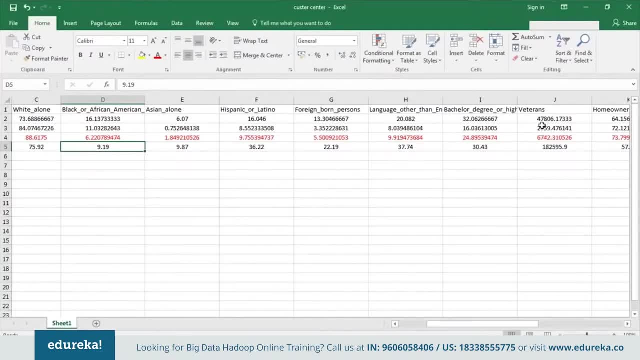 And you can check out here at 16,, 8,, 9, and 36.. So maybe again Hispanic or Latino field And you should do some more analysis on it. And even here you can see in veterans There is 47,806.. 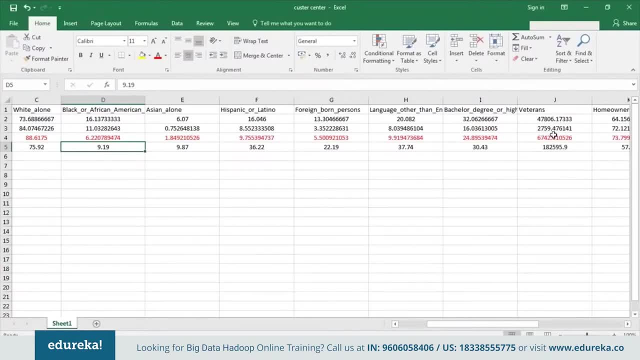 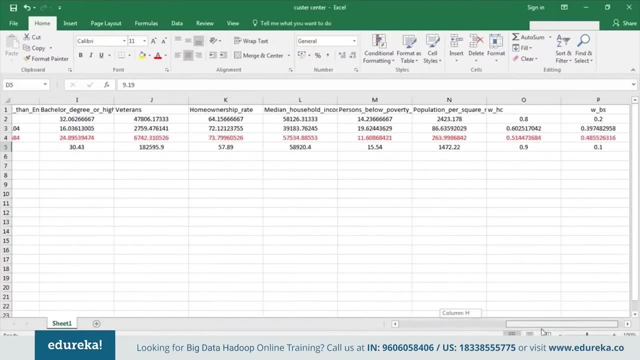 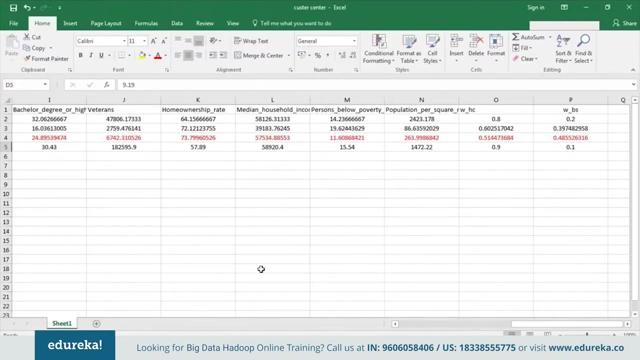 Whereas we have got 182,000 all. So there is Also a lot of difference. And here Is only 2759.. And we have got in the 10,000s. We have got numbers And even 100,000s here. 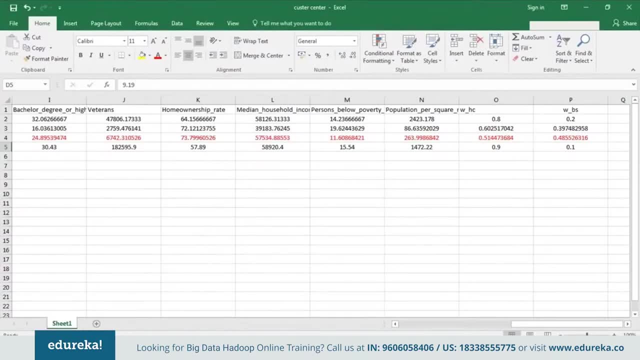 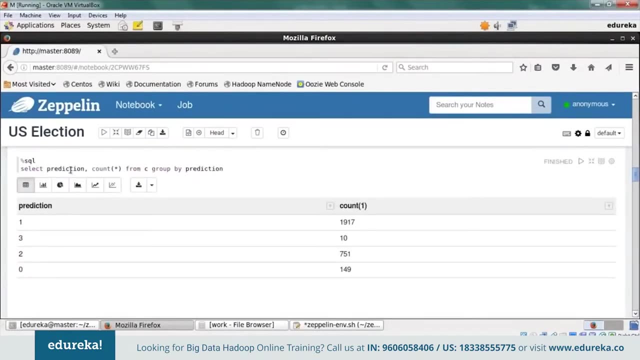 So this is how we can identify that, Which are the fields Or which we can find the main reasons Of the main points Where you should make your analysis. So let's go back to our Zeppelin notebook, And here it is. 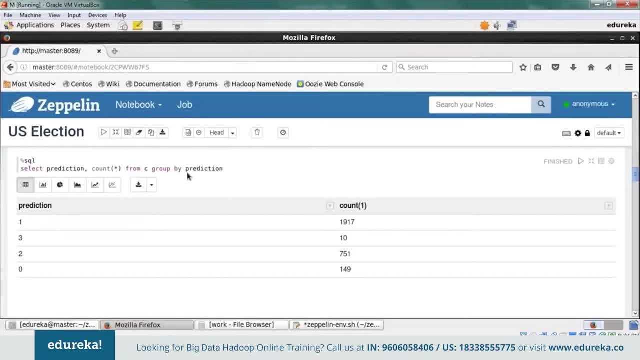 So now, what we are going to do Is that we are going to visualize the result first, So we are counting from predictions. Prediction means Prediction contains my cluster, Since you know that I have stored my clusters, My cluster information and prediction. 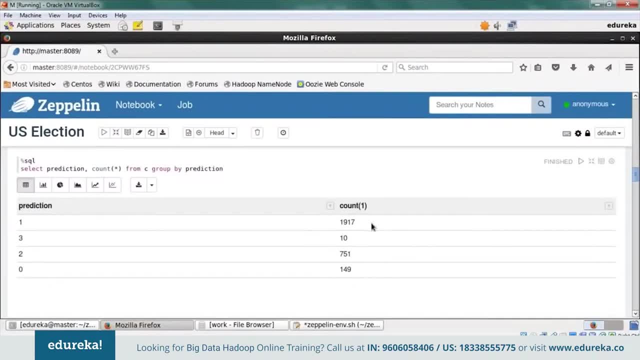 This is my output after k means. So I have got This many clusters. So this is the count of my counties, Or a count of different various That lie in my particular cluster. You can see that in cluster 1.. I have got 1,917.. 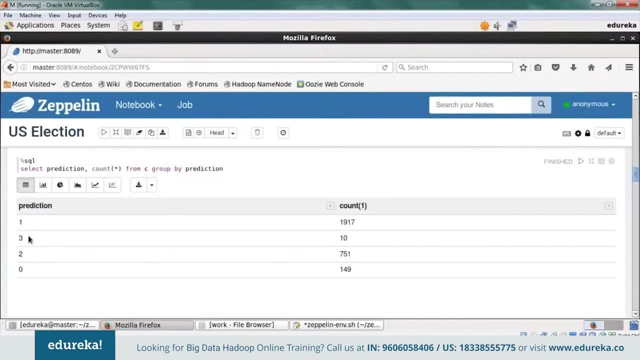 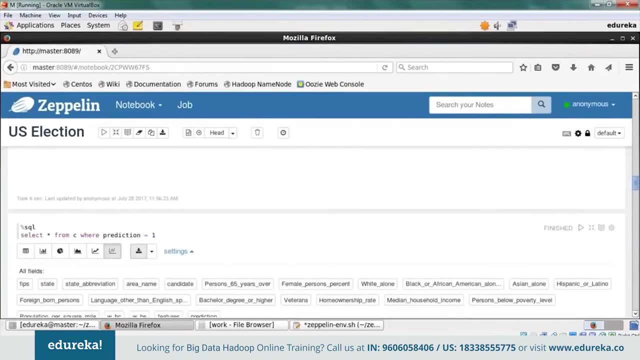 In cluster 2 I have got 751.. So maybe I should pay more attention To analyzing cluster 1.. Right, So that is why I have selected cluster 1 here And we are making different predictions. So you can see that in the x axis. 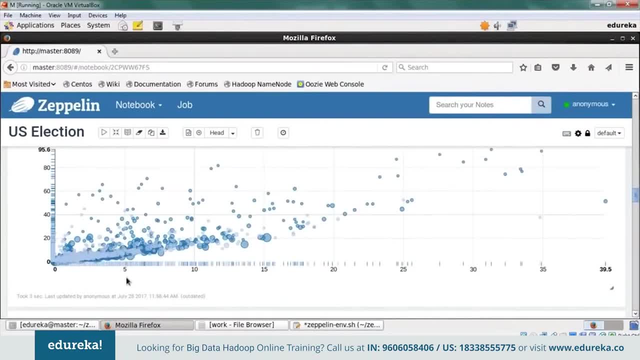 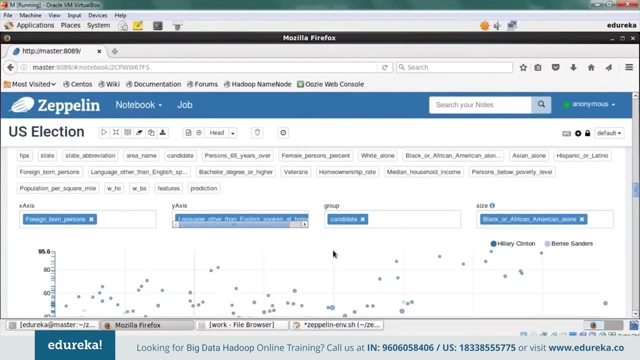 I have got foreign born people And in the y axis I have chosen Language other than English Spoken at home And then we are grouping it by candidate So you can see the lighter blue Is for Bernie Sanders And the more dark blue is for Hillary Clinton. 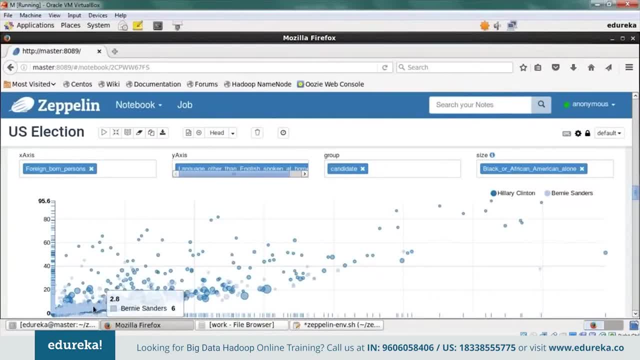 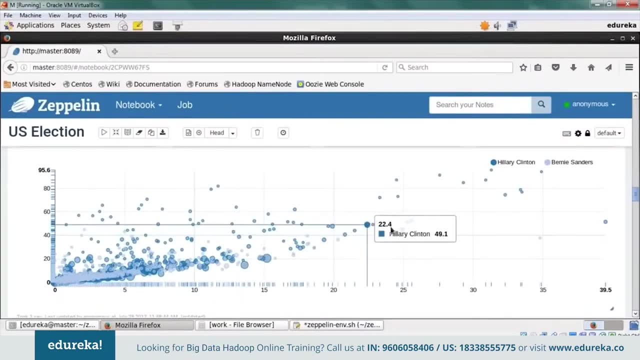 So all this light blue is for Bernie Sanders, And you can see That as the number of foreign people Increases, You can only see Hillary Clinton In the scatter plot here. So there might be a few outliers Like back here in the sizes defined. 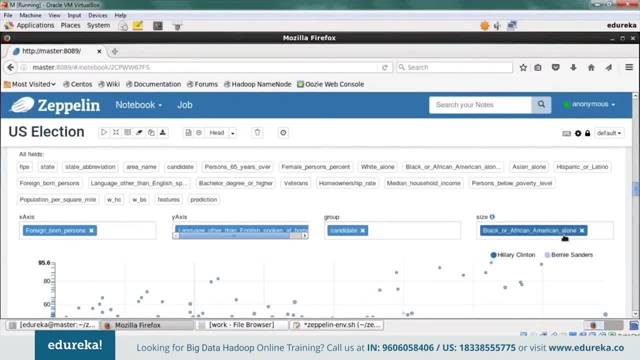 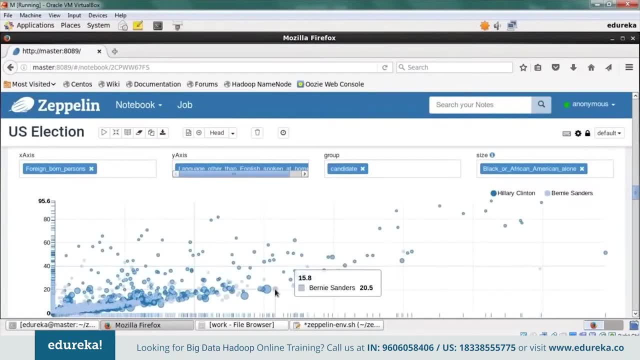 According to black or African American alone. So you remember that this was the feature Where we find a lot of variations In the numbers. So that is why we grouped it according to that And you can see: the bigger The circle represents, the more black. 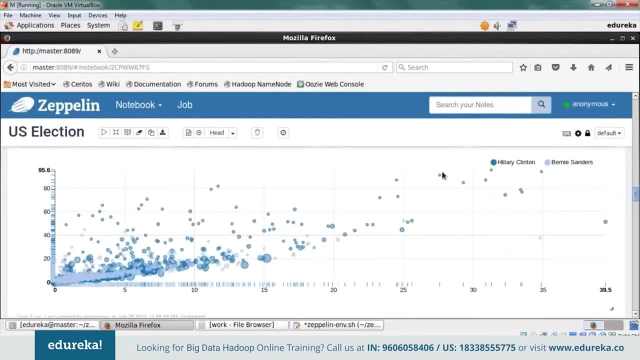 Or African American alone, And that is what the conclusion Is in the scatter plot, And we can see that as the number of foreign people increases, The popularity of Hillary Clinton Is more In larger groups of foreign people. You can also choose different parameters. 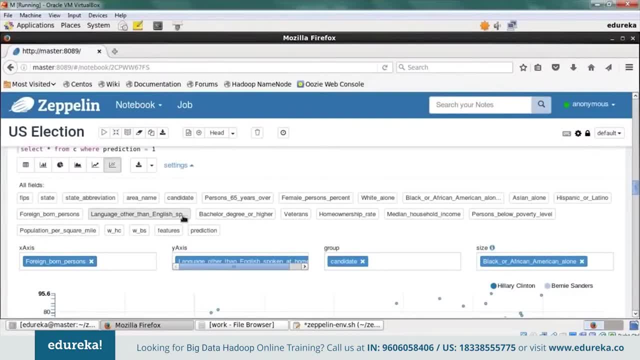 Out of all the different features That you have chosen. So remember that we have also seen The variation in veterans. So let's choose veterans in y axis. So let's also change x axis And let me just use y alone here. 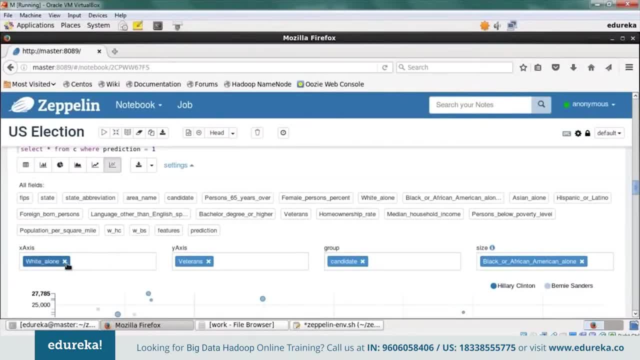 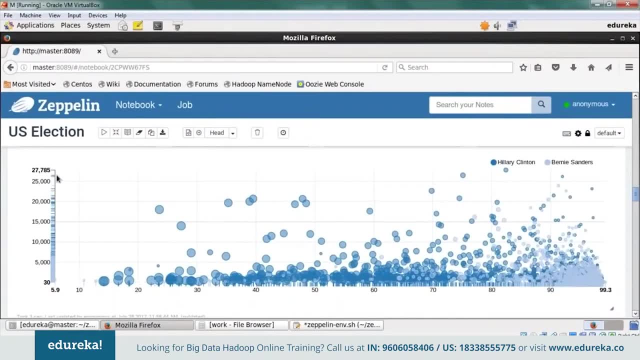 So you can see here that There is the X axis That has white alone And this is the veterans. So you can see that Hillary Clinton Is popular among veterans, Also in a smaller group of veterans, Since we have decided the size. 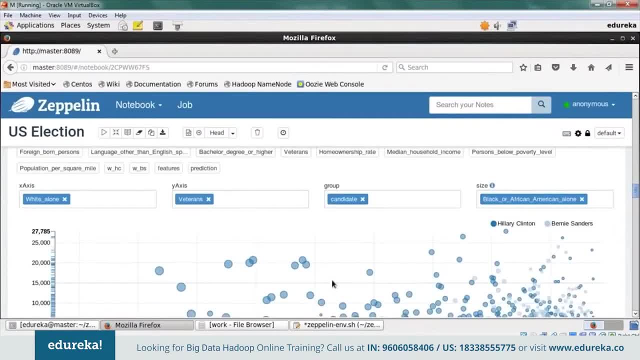 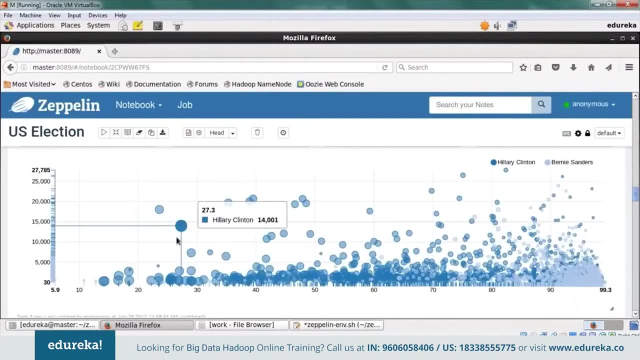 In black or African American alone. So the size Also represents some values. She is popular among the African American veterans And then, As you go ahead And as the count increases, You can see actually, And it almost represents that This is a point. 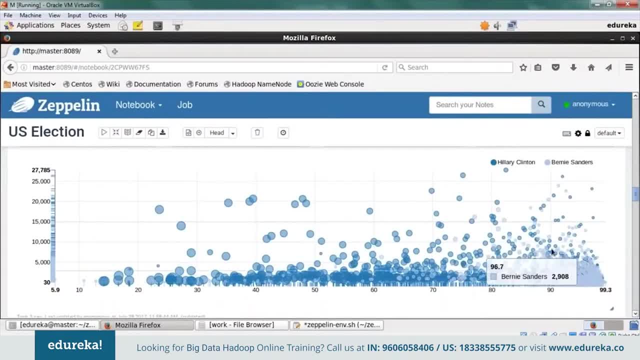 As the number of people increases, Or as the number of white people increases. The votes are equally kind of Distributed between Bernie Sanders and Hillary Clinton, Because there are a lot of points in this scatter plot Over here And you can go ahead and drag and drop different features. 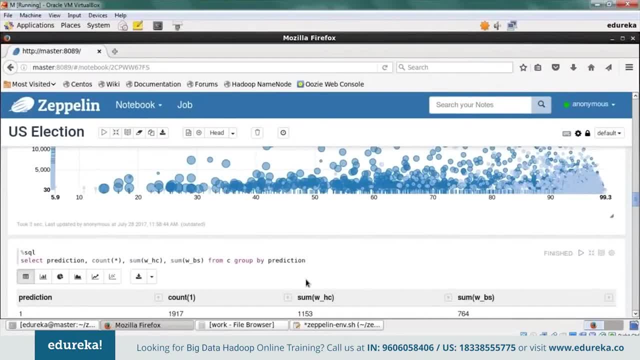 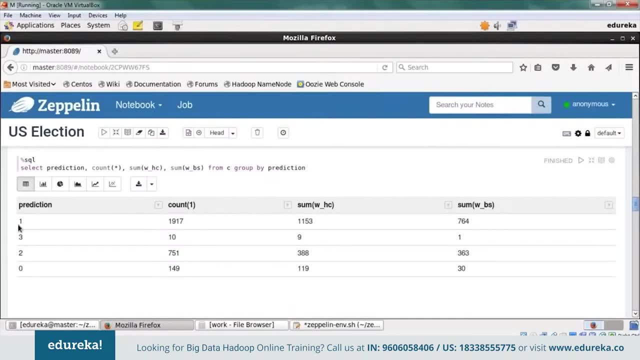 And you can make different visualizations on that. Now, what we have done Is that we know that there are 1917 counties in my cluster. One Is that I am going to see that Among these 1917.. How many were in favor for Hillary Clinton? 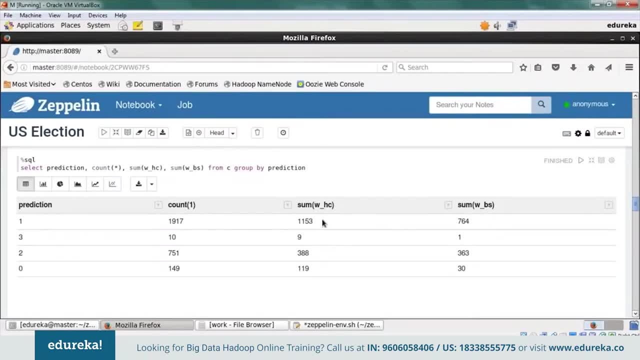 And how many were in favor for Bernie Sanders. So in cluster number one, You can see clearly Hillary Clinton is the winner And Bernie Sanders only has got 764, whereas she got 1153.. Similarly, in cluster three, again Hillary Clinton is the winner with nine. 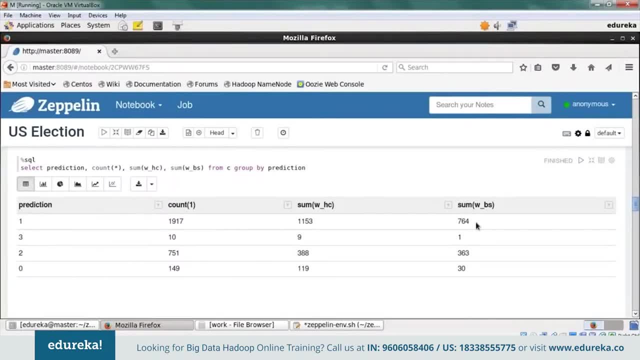 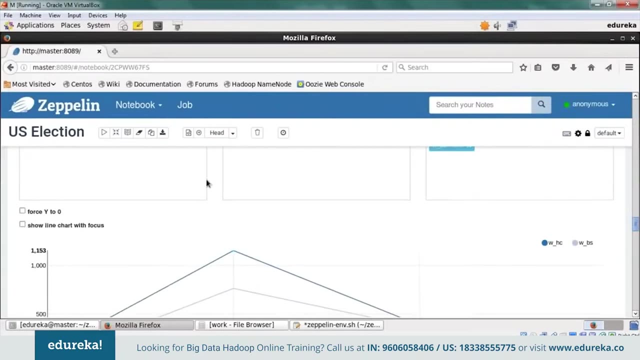 And Bernie Sanders With one, Then it Two, She has also got 388.. And Bernie Sanders was 363.. So this was very close call And again in zero you have got 119. And 30. And then we went ahead and created a line chart. 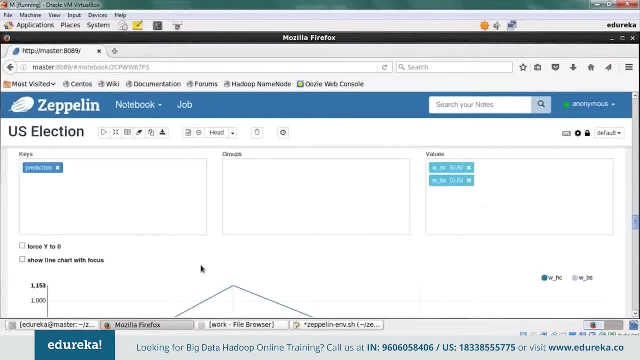 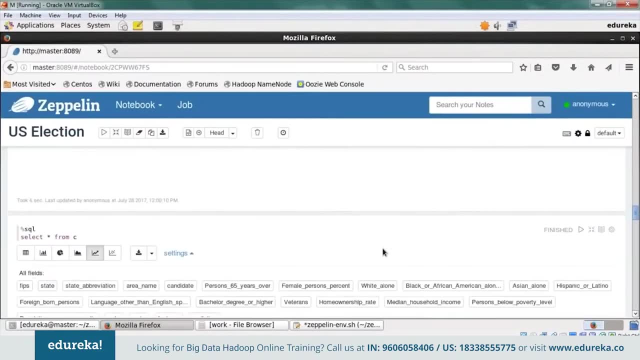 Also of the word distribution For Hillary Clinton and Bernie Sanders. So in keys we have selected prediction. The values here are WHC and WBS, The sum that we have got over here. So definitely Bernie Sanders is lagging behind, Even though you don't have that table for you. 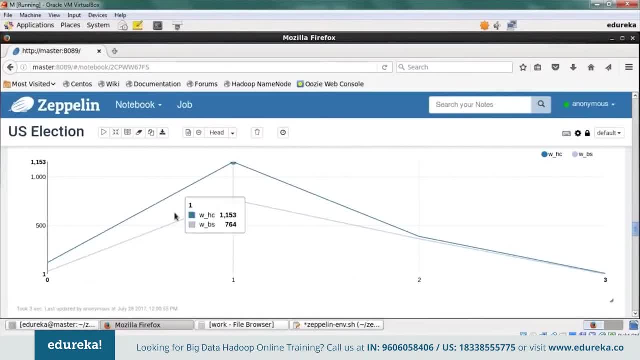 You can also find it out According to this line chart. So you can see that in cluster zero, Even again, Hillary Clinton was ahead of Bernie Sanders. In cluster two, There was a very neck to neck competition And you can see it. 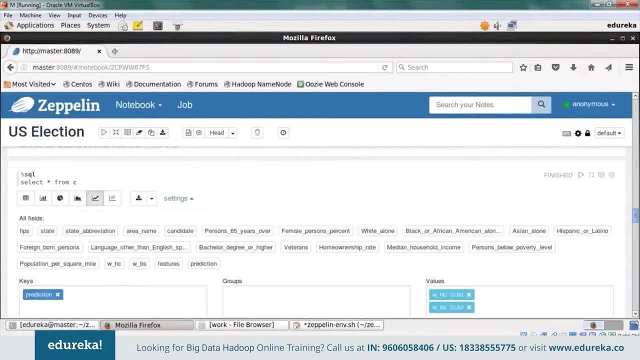 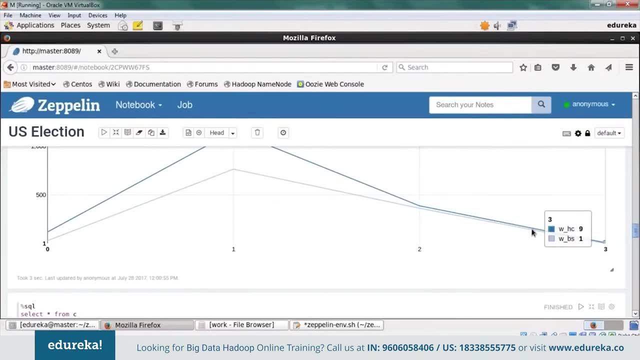 In the graph here. So this represents cluster two, And so you can see You have a neck to neck competition. And again in cluster three They have got neck to neck competition. So This describes the distribution of votes For Hillary Clinton and Bernie Sanders. 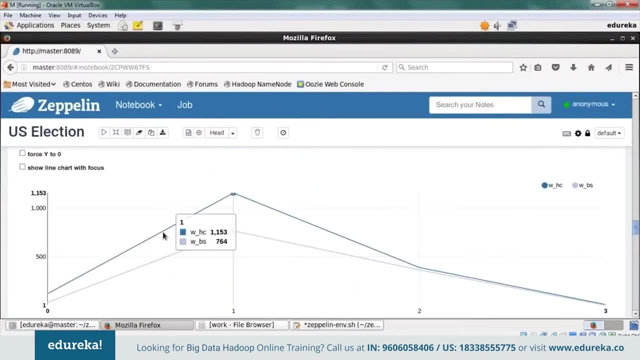 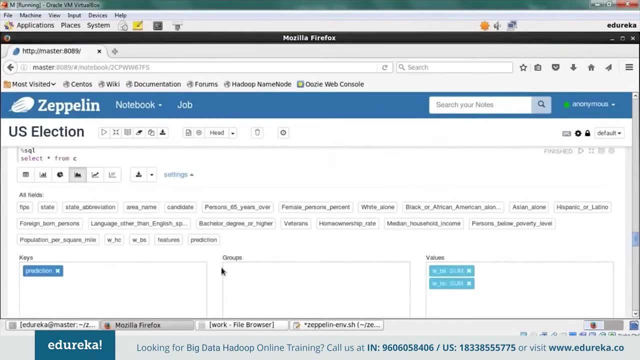 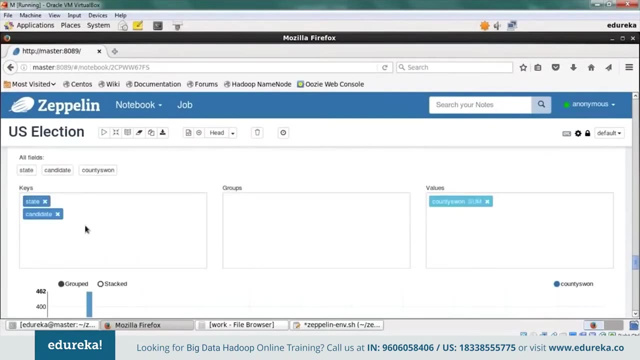 And definitely Hillary Clinton Knows ahead And that is why, of course, She won the primary elections. So again, you can go ahead And we have created the same graph. It is only just area graph Instead of a line graph. The key here are state and candidates. 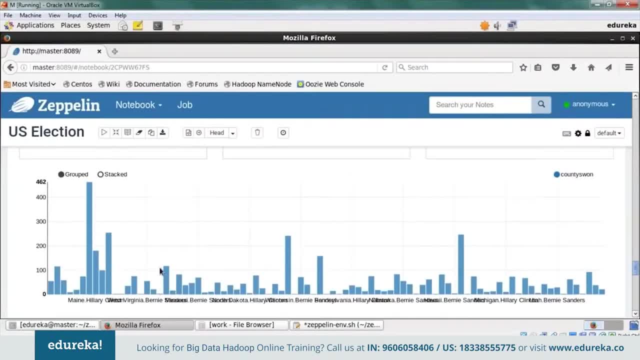 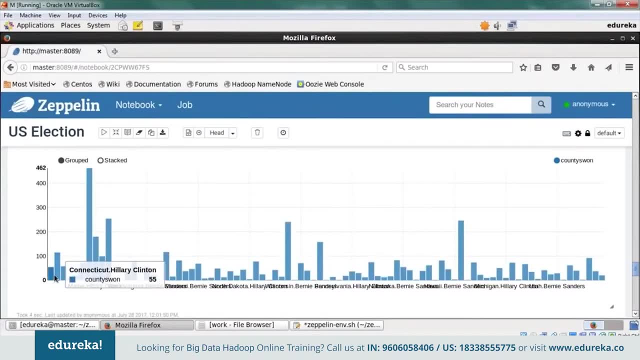 So I have got states and candidates Over here And the values is counties. Once You look at this bar chart, You can see that in Connecticut Bernie Sanders won 115 counties. In Connecticut, Hillary Clinton won 55 only. So in Florida, 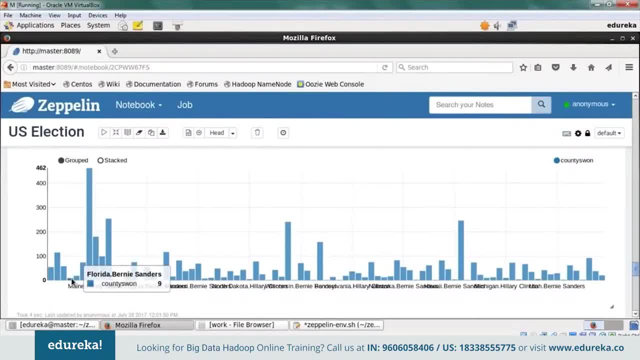 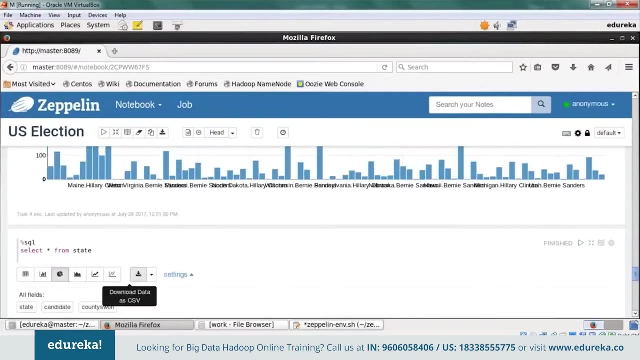 Hillary Clinton is 58.. And in Florida Bernie Sanders is 9.. Here you can see: in Maine Bernie Sanders won 462.. So Bernie Sanders got a majority of votes For Maine. So you can also classify it State wise And as Donald Trump. 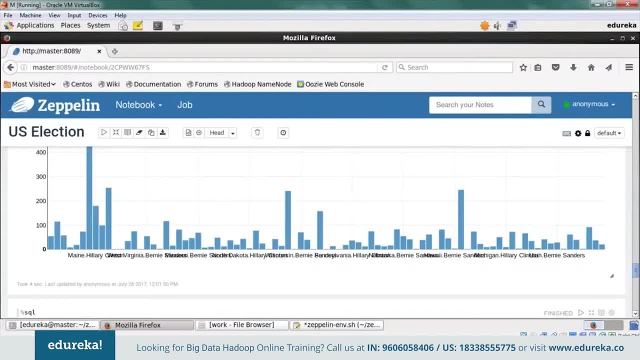 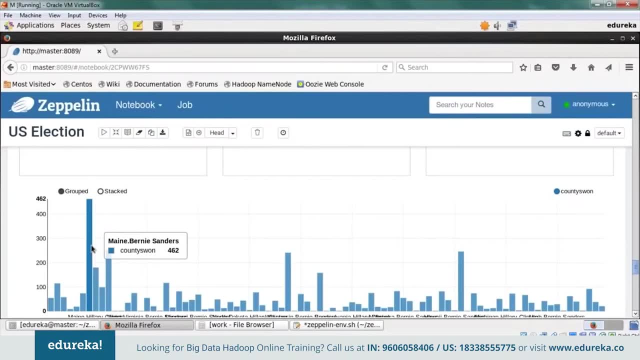 Now you will know Which are the states that you can target. So you know that in Maine A lot of people voted for Bernie Sanders, And maybe Hillary Clinton Is not popular, So you can go ahead and lead out So as Donald Trump's party member. 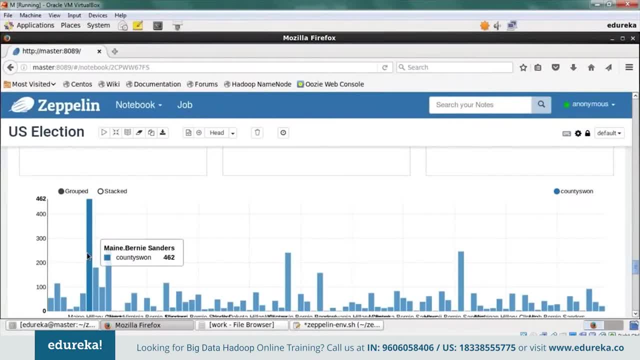 You can just advise him to go in Maine And carry out different campaigns, Because Hillary Clinton Is not so popular there, So maybe it would be a little easier To get votes For the people in Maine. So this is what you can make a conclusion from. 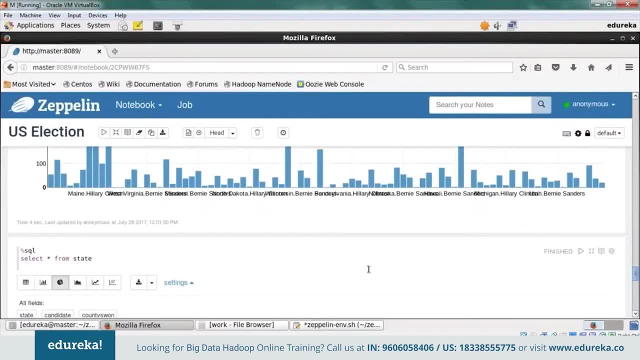 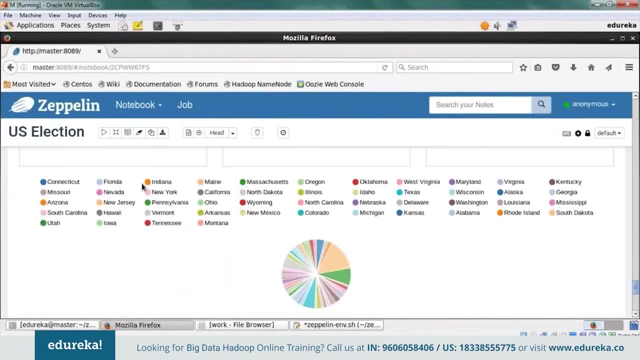 And it might not be very accurate, But this would be very close. The thing is that you can make different charts. You can make bar charts, You can make pie charts. So whatever counties won Have made in the bar chart, So they're here as a pie chart. 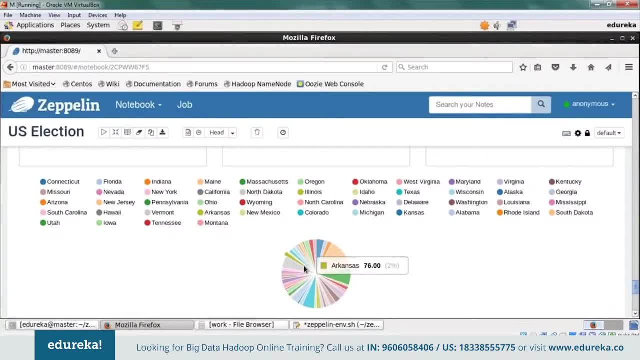 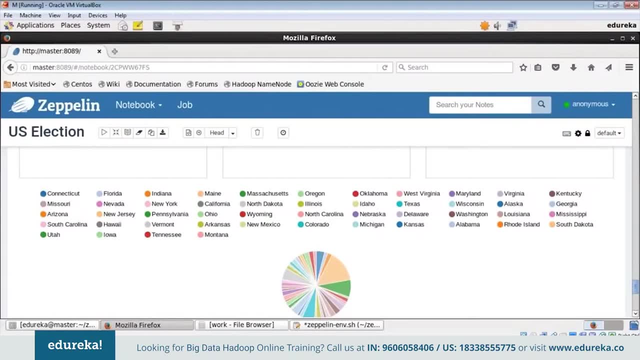 It looks better, But it's not maybe as insightful. I just placed it so that I can show you You can make pie charts also. So these are the insights And suggestions that you can actually go And tell Donald Trump That she is popular among the foreign people. 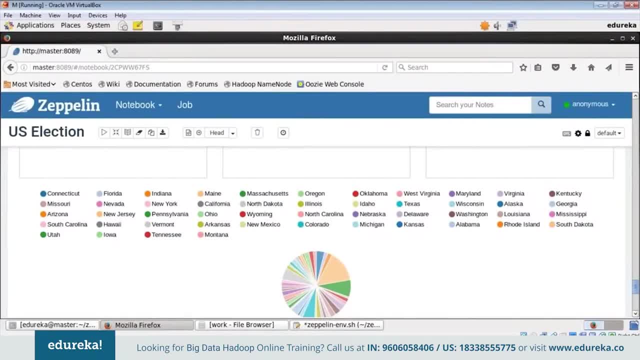 And the people who speak different languages. She is popular among the Hispanic people. And then in Maine She lost a lot of counties. She almost lost all of the counties in Maine. So these are different insights That you have got And then you can tell your superior. 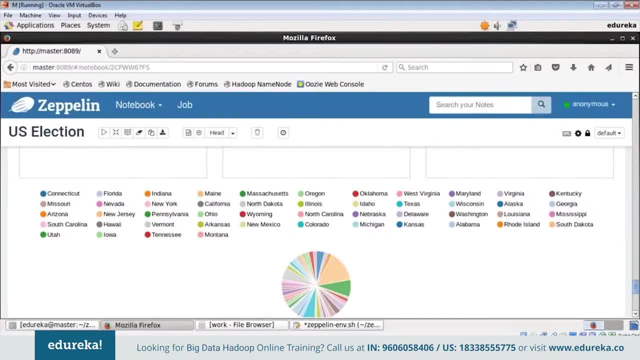 Or your employer Who has hired you to do that. So this is what you can present Right? So this is a beginner's level, And there are some more analytics That you need to do. I just showed you a few options. 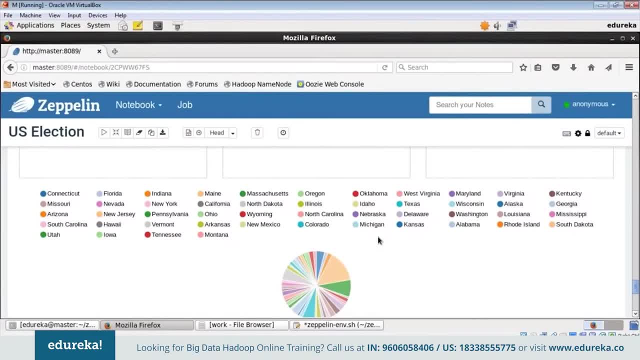 You can go ahead and try more In the Democrats section also, And you remember that you have to do it For the Republican party also. Now let me see what you have learned today. So if you have any questions right now, You can just go ahead and ask me. 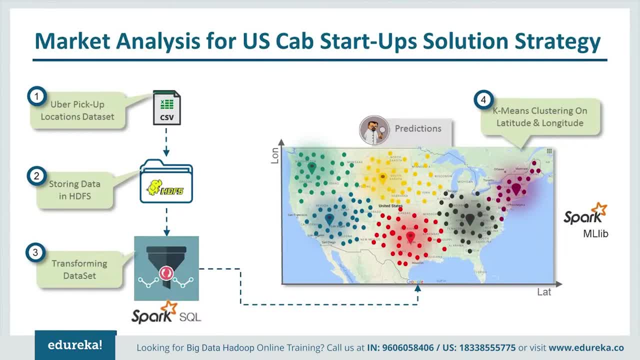 Does anyone have any questions? So now we will move on And find out the solution for the instant cab use case. You remember that we have got the Uber data set Which contains the pick up time And the location by two columns: Latitude and longitude. 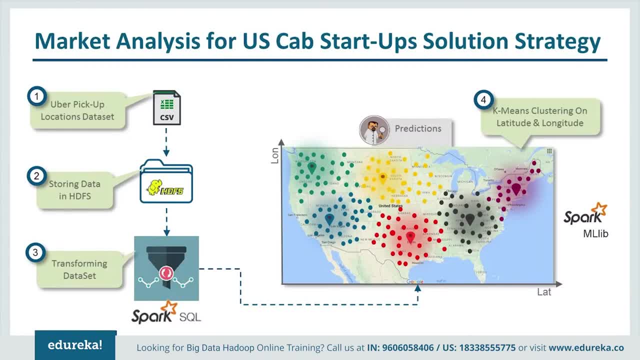 And we have also got the license number For a particular Uber driver, And what we have to do Is that we have to find the beehive locations. That is the point where we will find the maximum pick ups, And then we will also have to find out. 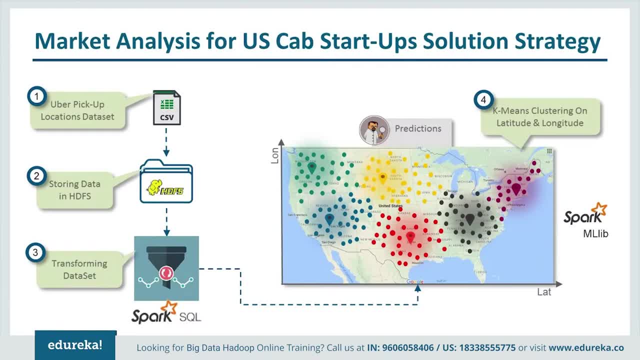 What is the peak hour of the day. So this was the entire strategy. So we have got the Uber pick up data set And then we store the data into HDFS. We will transform the data set And make predictions By using k-means clustering. 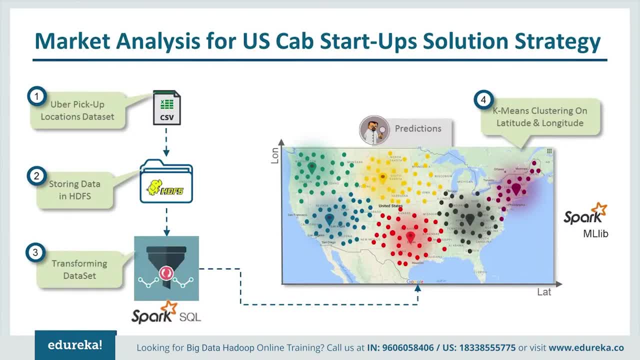 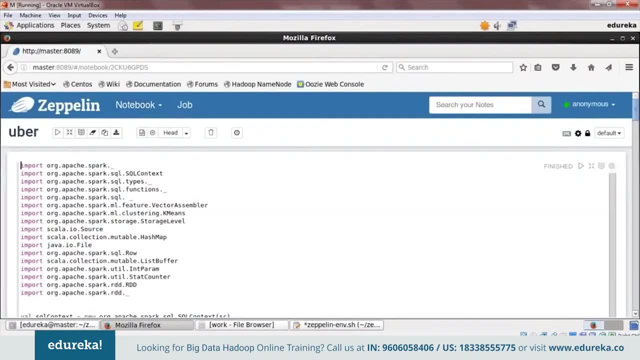 On the latitude and longitude And find out the beehive point. So now let me open my other notebook, The Uber notebook. So again, the first thing that you have to do Is copy the Uber data set into your HDFS. Now, we have done that before. 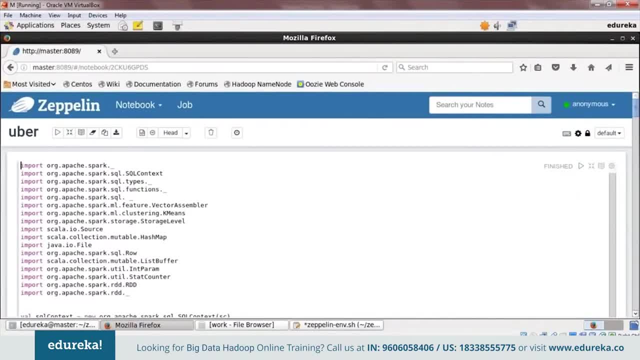 Explaining to you the US county analysis. So again the code is kind of the same. The first thing is that again We are importing some spark SQL packages And some spark ML lib packages Because we are going to use k-means clustering. 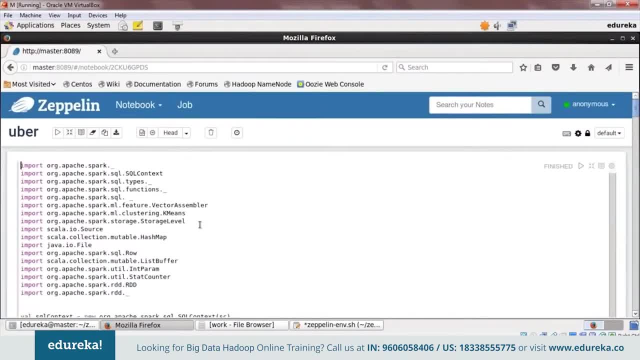 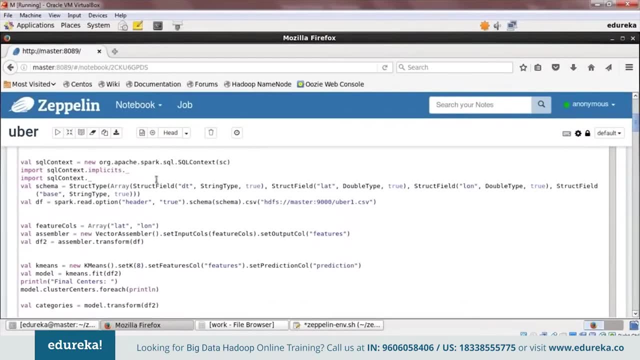 And you can see vector assembler: here again Spark ML, clustering, k-means And other spark SQL packages. So then we have to start our SQL context, And we are doing it the same way. Then the first thing again, We have to define a schema. 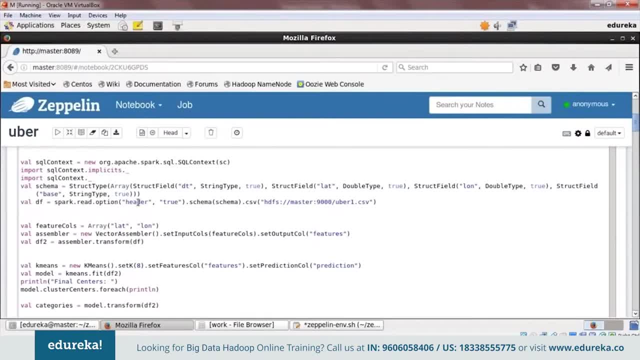 Now I don't have many fields. I have got only four fields, if I remember. So the first field was the date And timestamp that defines the time We are defining it as DT. The next field is the latitude, The longitude and base. 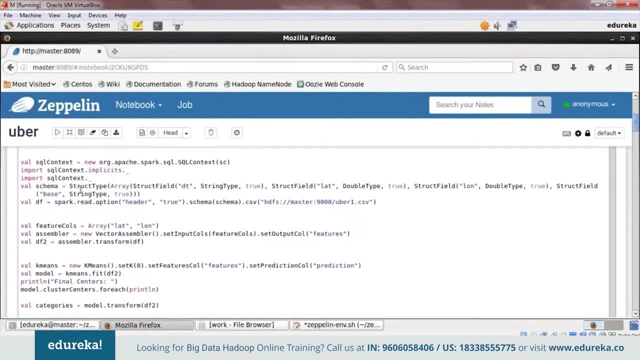 Then I am going to read my data set. This is the path in my HDFS Where my Uber data set is There. So I define schema as schema. here The header is true because, again, My data set contains column headers And I am going to store in DF. 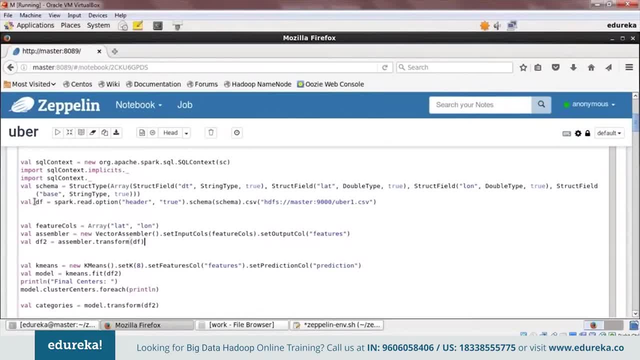 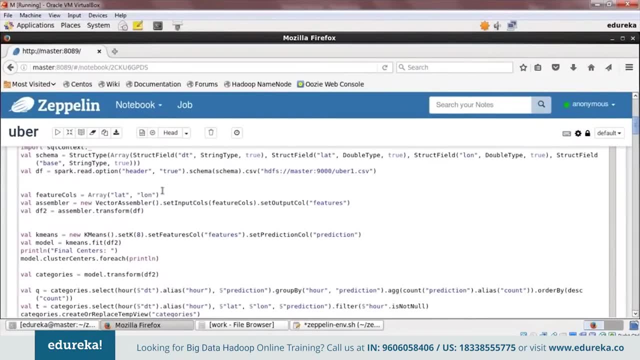 So feature calls here Is going to be latitude and longitude, Because I am going to find out The beehive point, The point where I will get my maximum Kick up from. So again, I have set the input Calls as feature calls. 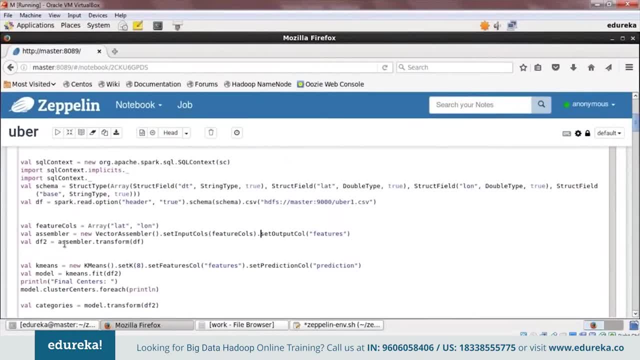 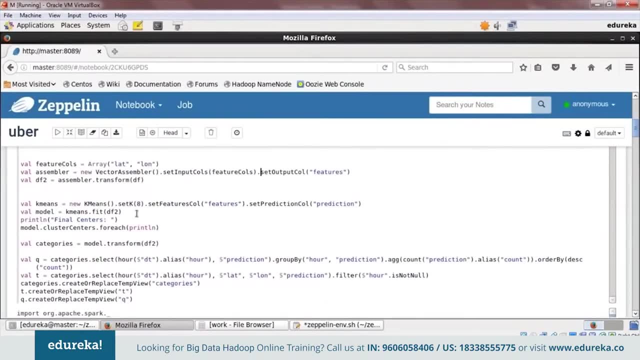 And output calls as features. So I am using the assembler To transform my data set And then again I am using k-means And we use the same elbow method. We found out that we should make eight clusters For this data set. 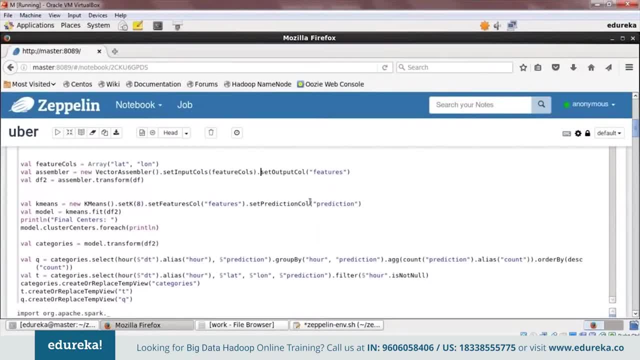 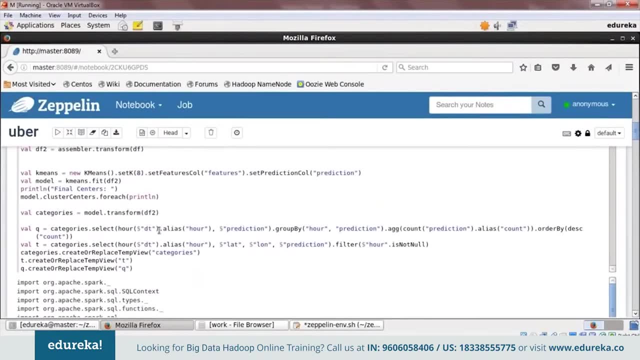 And then we are selecting the prediction column And the output column As predictions, And then we have printed the cluster centers For each cluster And finally, whatever result we are going to find, The cluster centers will tell me The exact location. 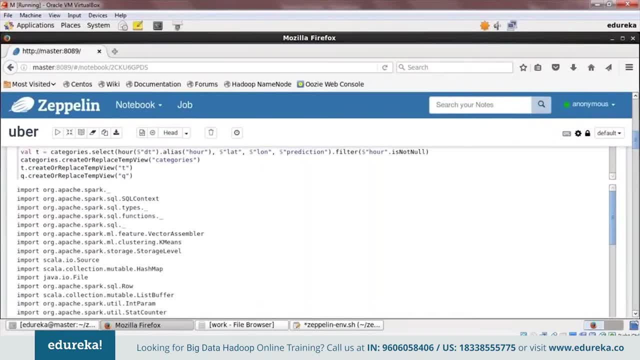 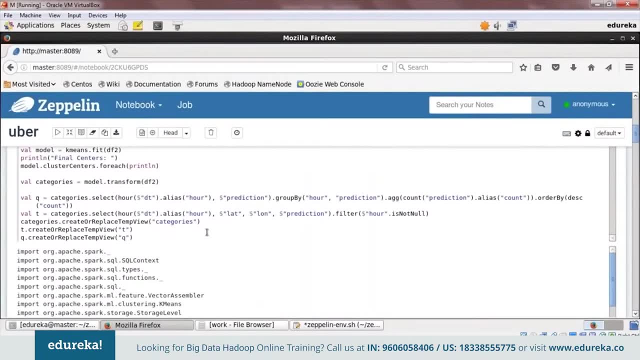 So this cluster centers That we will find after k-means Is actually the beehive point. This will be the point where I will find Maximum pickups. So here I have printed my cluster centers And this defines the latitude and longitude. 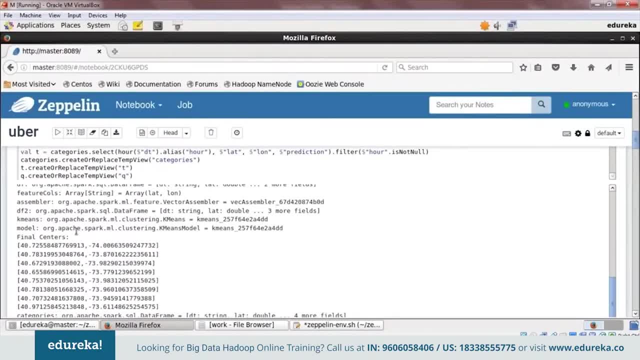 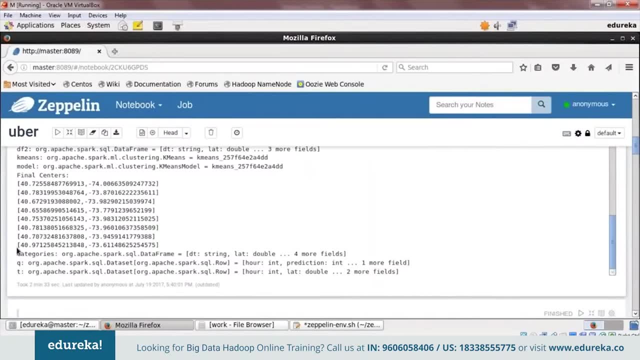 This is going to be my location, Where I am going to find the maximum pickups, And I got eight results Like that And defined the eight centers For different clusters. So this is exactly like the k-school problem That I explained to you in k-means. 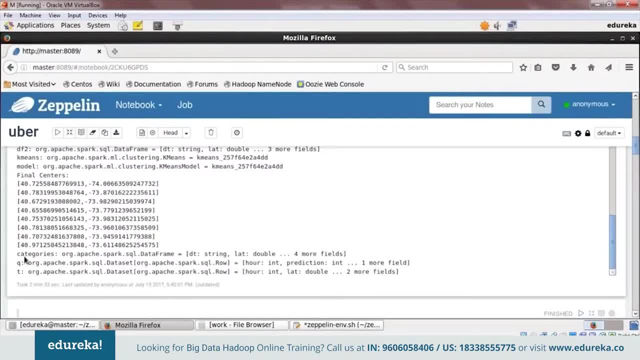 This is exactly what happens, Just as we found out the center of each cluster, And that is where we are replacing the school Or building the new school. So, similarly, this is going to be my beehive point And this is where I will place. 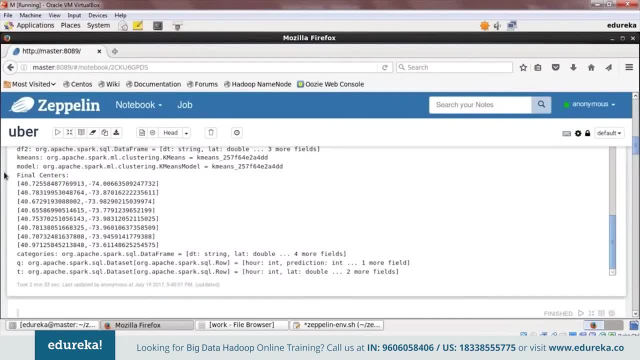 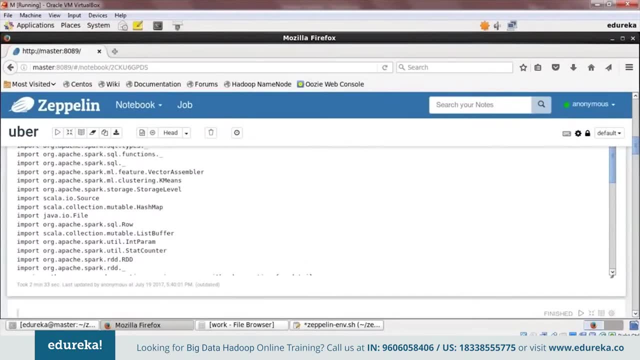 My maximum number of cabs. So we found out the beehive points. The next thing we will need to do Is we need to find the peak hours, But I also need to know At what time should I place my cabs. 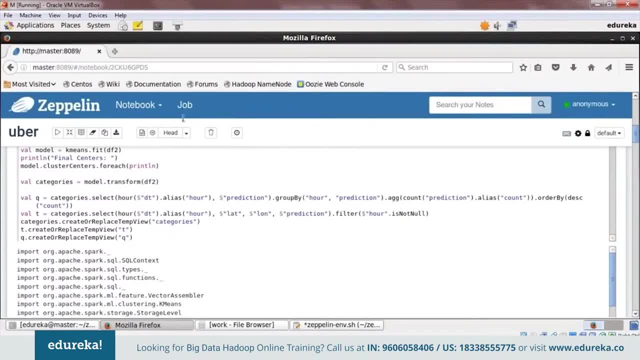 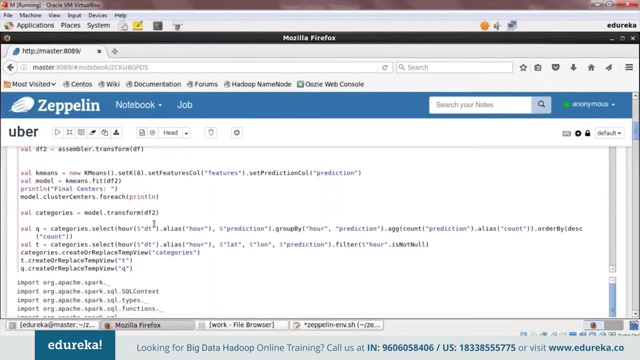 In the location. So what we are doing now, We are taking a new variable called q And we are selecting hour from the time stamp column And then the alias name should be hour And we are getting it from our prediction Or from the result that we got. 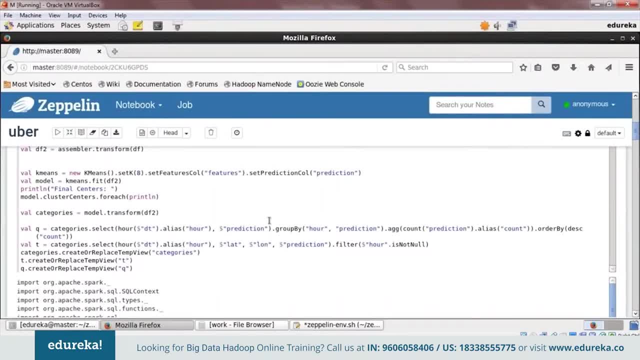 After my k-means clustering. So now we are grouping it And it will have the different hours of the day And then it will just show me the pickups At the different hours of the day In the location that we found out. 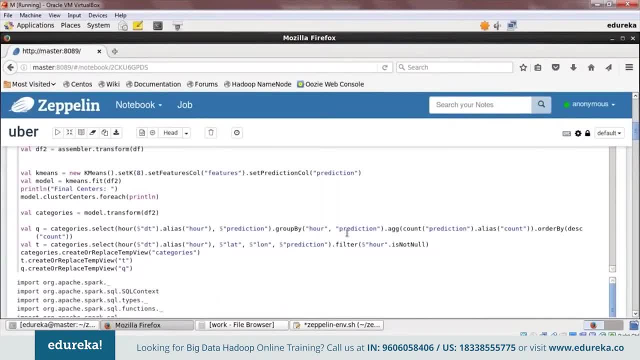 Or the beehive points, And then we are going to count How many pickups We are going to get from that place. So we are ordering it by descending, So the smaller pickup count Will be the first And then the larger will be at the bottom. 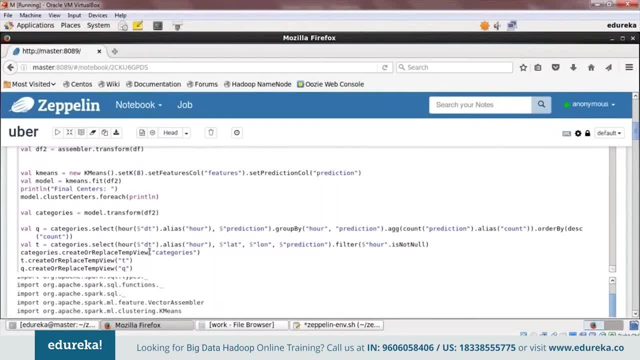 Similarly, again, We are creating a new variable called t, And we are going to do the same thing. So here, what we are doing Is we are selecting the time, The hour of the day, The latitude And the final values from here. 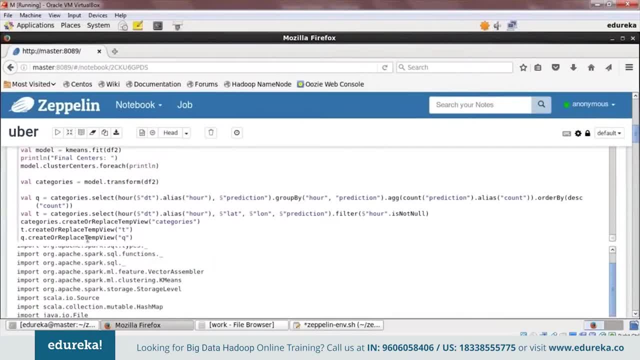 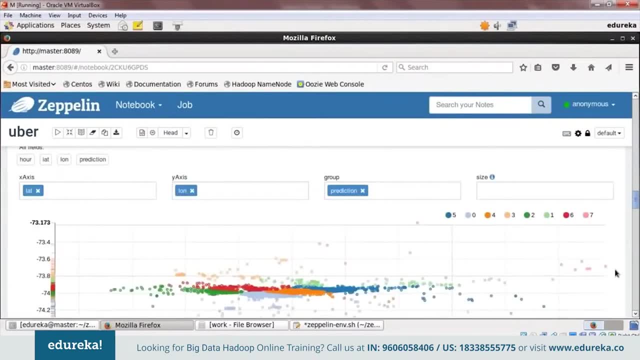 So now we have created a table view for categories. Let me show you what the categories contain. Ok, Let me just go down. So I have done some few operations here, So let's scroll back up And I will show. and again, we have created table views. 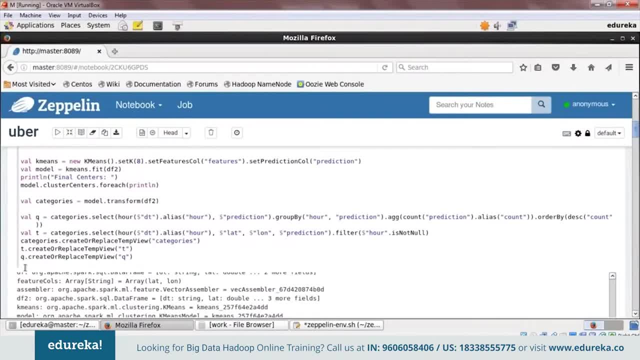 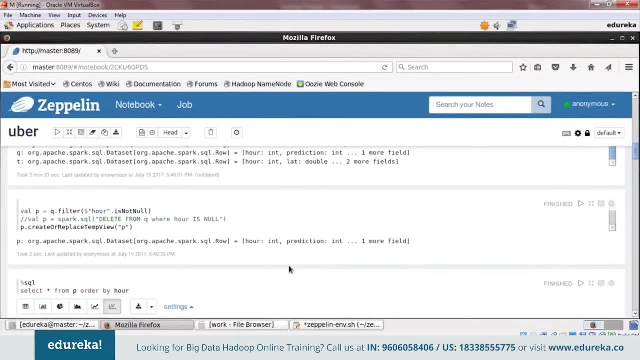 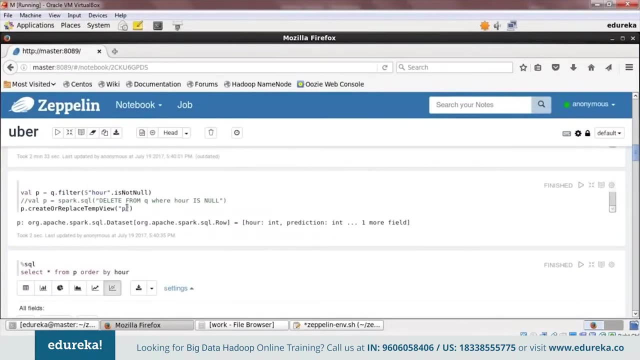 For t and q also, Which is again t and q, And then I have made some visualizations For each And we have created a value P, Where our is not null, null hours, and we have created a new view called p. So here is my hours, This is my. 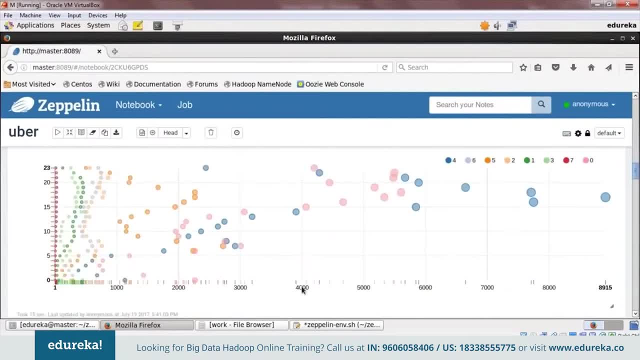 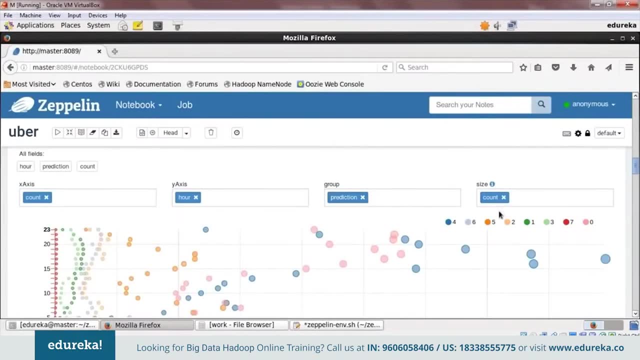 count and the x axis that show how many pickups were there, and this contains different hours of the day, and then I have grouped it by prediction, So the size is according to the count. So you can see that the bigger the circle means more pickups, So you can find out the biggest. 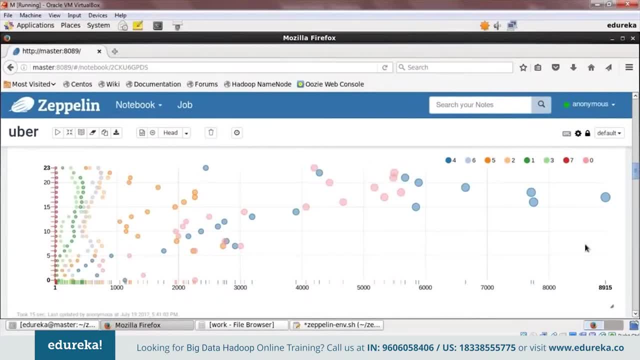 circle and you know that you can find the biggest circle as you go along the x axis, because this is where the count increases. So you can find out. the biggest circle would be here, and it lies in my fourth cluster and you can see that there are 8,915 pickups at. 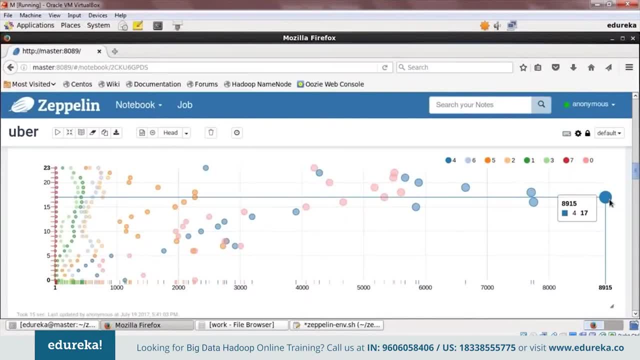 the 17th hour of the day, which is around 5 pm, And so you know that the maximum pickups are around 4 o'clock or 5 o'clock, and this lies all in my fourth cluster, And so it means my peak hours are around 4 or 5 o'clock in the evening, right? So this is what insight. 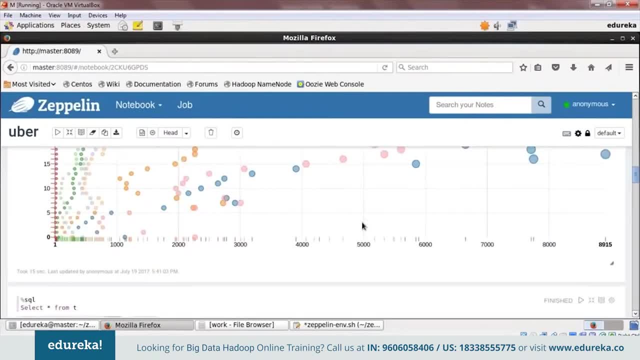 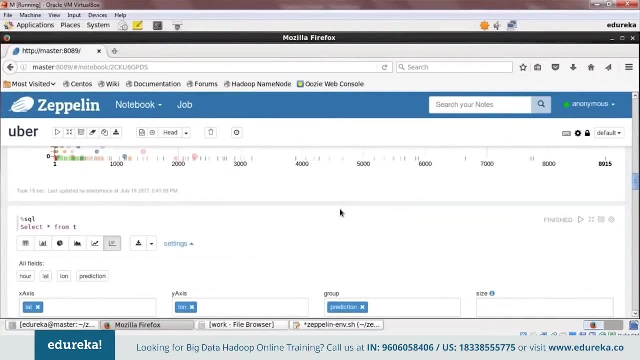 we have gained, And you can tell Instant Cab CEO that I have found out that your cabs should be ready around 4 or 5, because that's the time when people go home from offices or they're going out for dinner or something. And this is what another table view looks like, which is T. 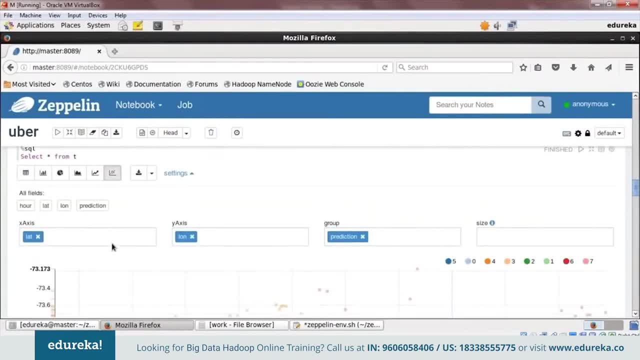 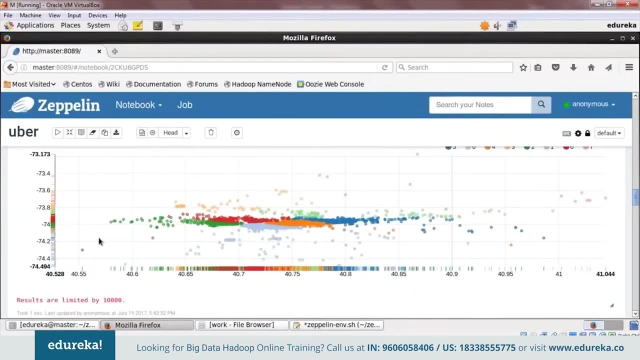 So here we have latitude and longitude and this is where we are finding the beehive locations. So I have got the distribution in a scatter plot again and you can see that we have got really dense points over here. It means that these represent the beehive points, So what? 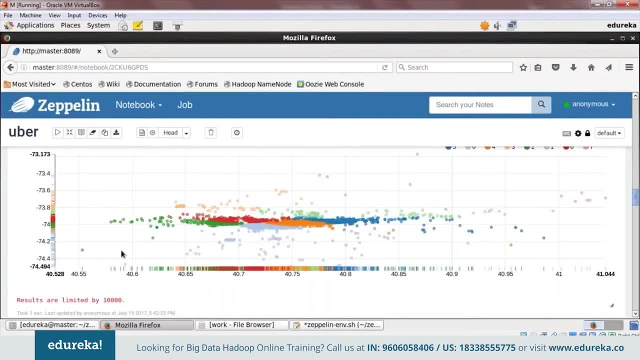 you can do is that you can just put the US map and scale it according to this scale over here, and then you can exactly find out what is the exact location where you need to put your cabs around the 17th hour or the 16th hour of the day. Alright, 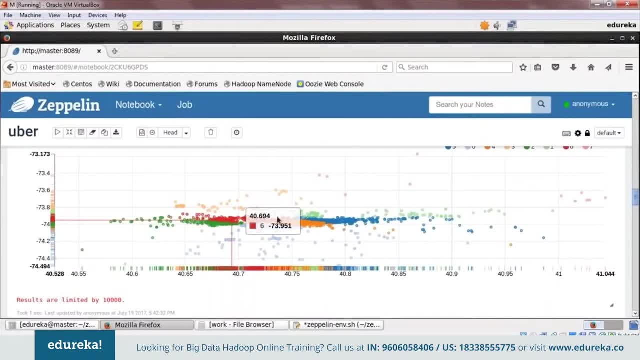 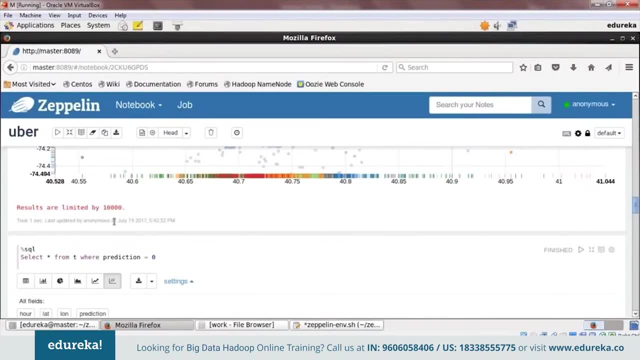 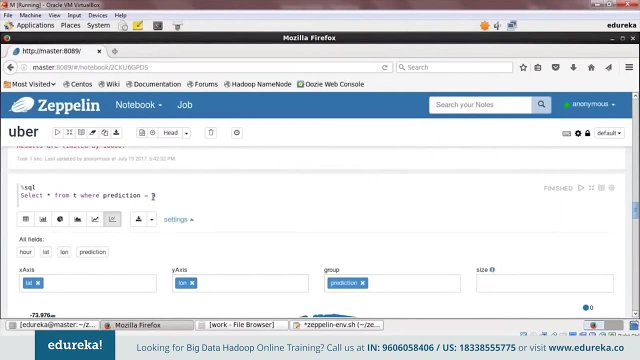 And you know that we had a lot of rows, but the results are only limited by 10,000, if it's around 10,000 rows. But we obviously had a lot more and you can check in different clusters. So now we are analyzing cluster 0.. So here, if you see, 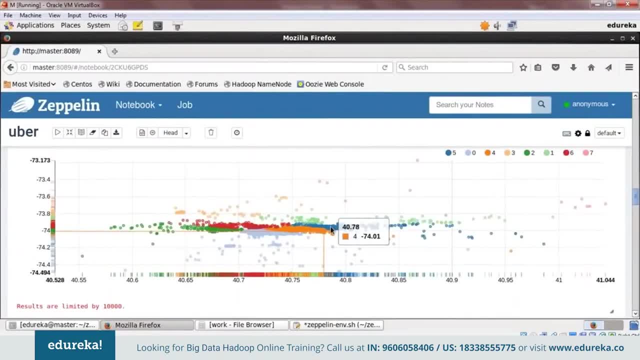 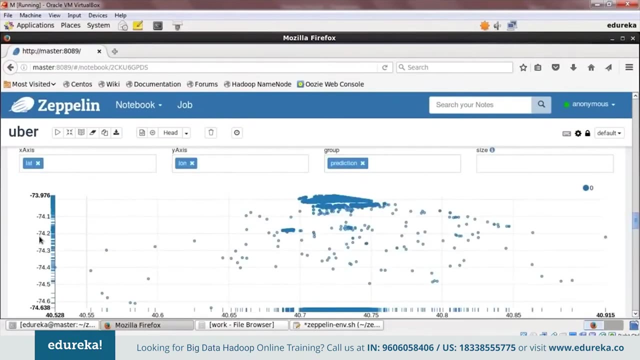 this point over here. this lies in cluster 4 and this lies in cluster 5 and this lies in cluster 0. So you can analyze each cluster also. So here I have just laid out the latitude and longitude for my zeroth cluster, So you can see here where prediction is equal to 0 and I've selected this. 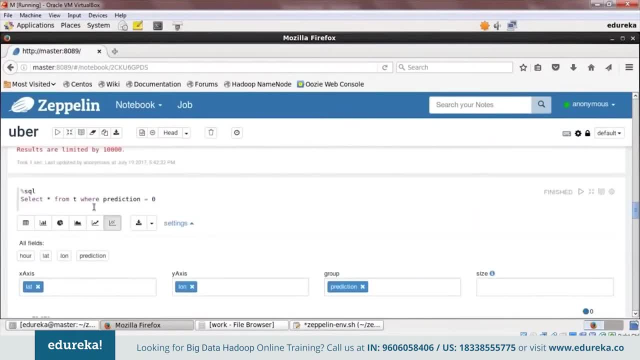 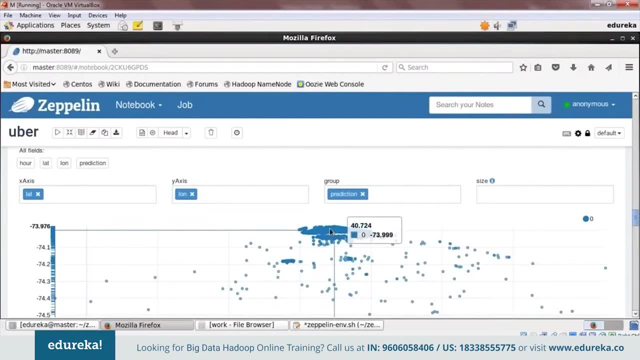 from the table view of t. So here you can find out the exact latitude and longitude, And here the latitude is 40.722 and the longitude is negative 73.995.. So this is how you can pinpoint location where your cab should be during the peak hours. Again, if you see this distribution, 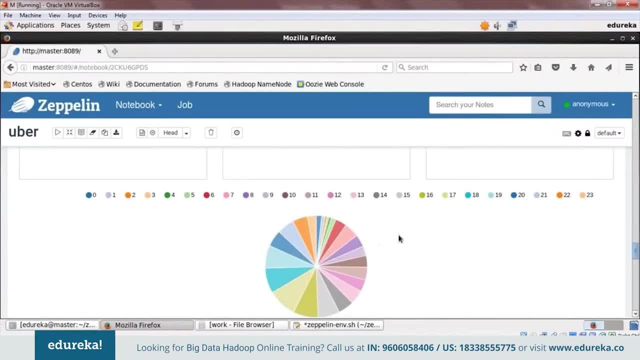 this is just a pie chart that I've created with that tells you what is the count of pickups at each hour of the days, starting from 0 to 23.. There are 24 slices in this circle, So you can see that these few slices are the bigger chunks, and this is the 19th hour of the day, which is 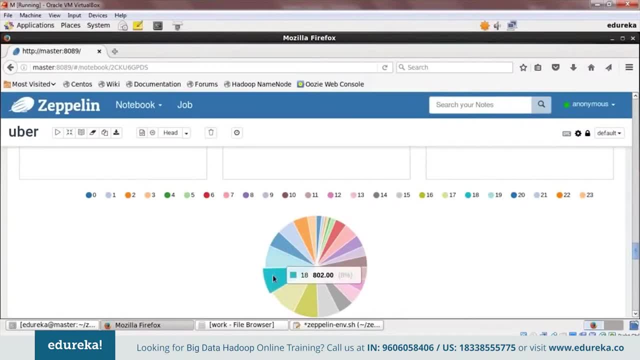 around 7 o'clock, 6 o'clock, 5 o'clock, 4 o'clock, 3 o'clock and so on, So you can see the midnight maybe nobody travels, So maybe your cabs could rest, or you don't have to travel, So you can see. 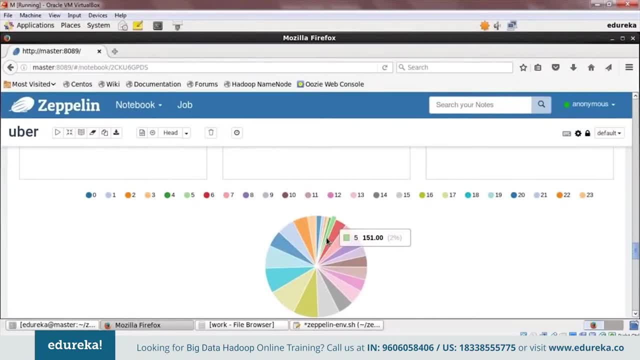 that you don't have to place any more cabs during this part of the day. These are the insights that you gain, So any questions on that? I think after doing the US county election, this was pretty easy to do, and this is also pretty easy to understand, and the results, which were also much. 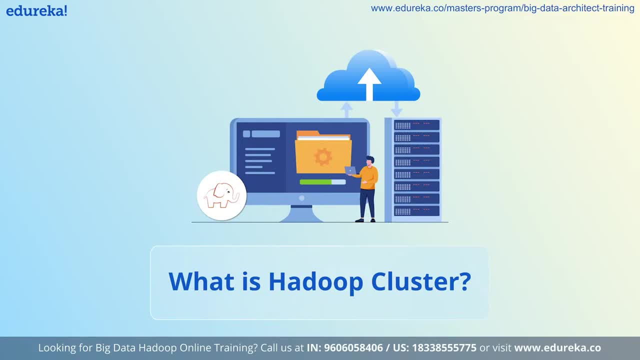 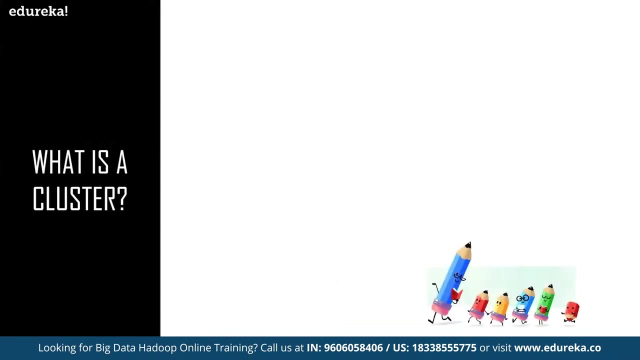 more clear correct: What is a Hadoop cluster? Before getting started into the Hadoop cluster, let us understand what actually a basic computer cluster is. a cluster basically means that it is a collection. a computer cluster is also a collection of interconnected computers which are 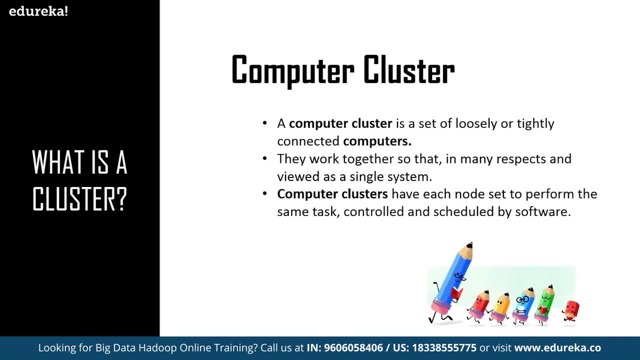 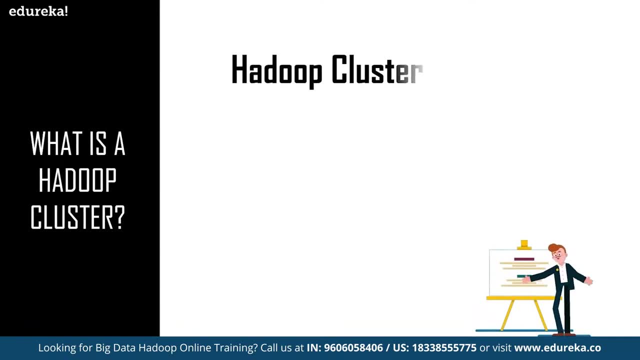 capable enough to communicate with each other and work on a given task as a single unit. Similarly, Hadoop cluster is also a collection of commodity hardware which can be computers and service, interconnected with each other and work together as a single unit. Hadoop cluster has a master. 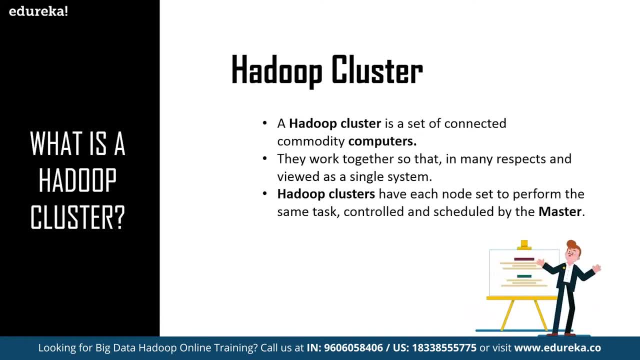 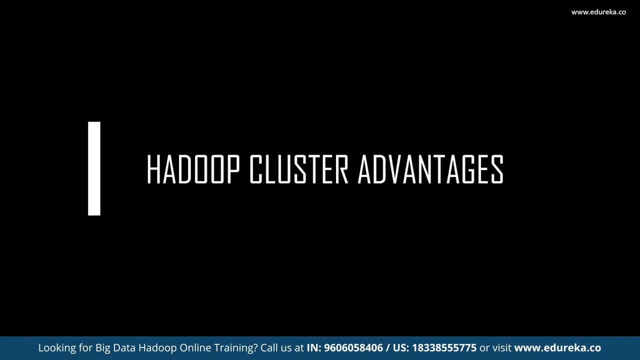 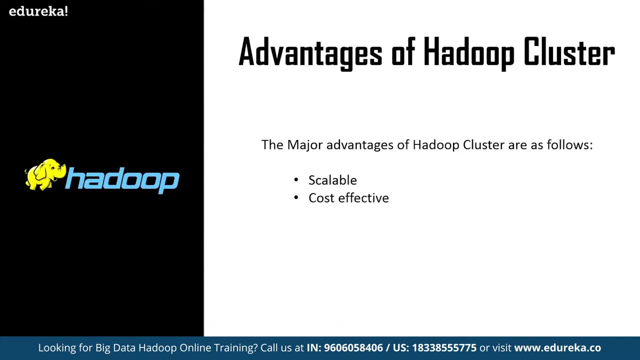 and numerous number of slaves. master assigned The task and guides the sleeves. now that we know what a Hadoop cluster is, Let us now understand its advantages over the other similar data processing units. Some of the major advantages of Hadoop cluster are: Hadoop cluster is scalable, cost-effective, flexible, fast and resilient to. 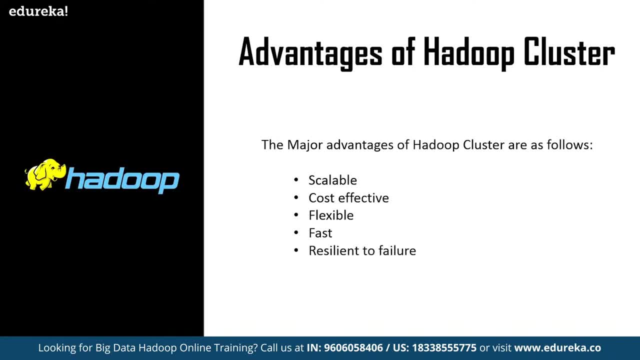 failure. Let us now discuss each one of them in detail. First, Hadoop cluster is scalable. Hadoop is a beautiful storage platform with unlimited scalability compared to rdb-ms. Hadoop storage net Work can be expanded by just adding additional commodity hardware, while rdb-ms can't scale. 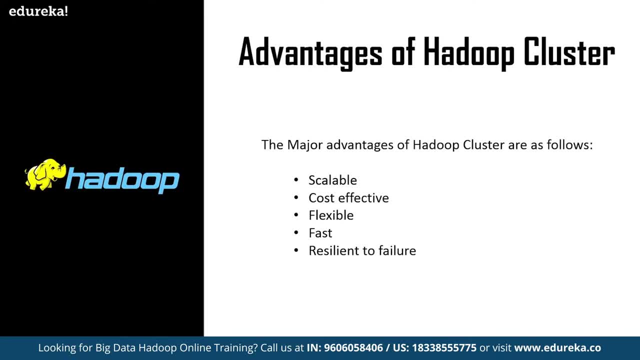 and process huge amounts of data. Hadoop, on the other hand, can run business applications over thousands of computers all together processing petabytes of data. second one: The Hadoop cluster is cost-effective. traditional data storage units had many limitations, and the major limitation was related to the storage. Hadoop clusters overcome it drastically by its distributed 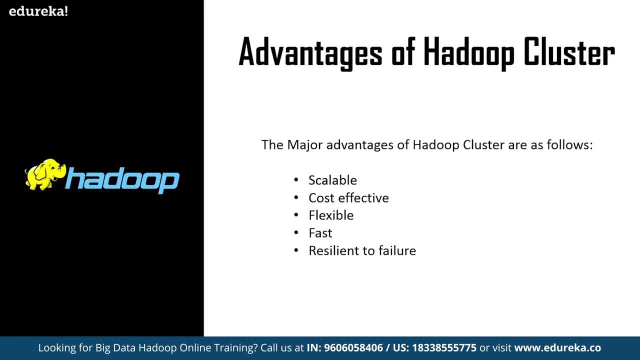 storage topology. Hadoop clusters use commodity hardware and the lack of storage Can we handle by just adding additional storage units to the system and the clusters functions as good as new. the third one is how to clusters are flexible. flexibility is the major advantage of Hadoop cluster. the Hadoop clusters can process any type of data, irrelevant whether it is structured. 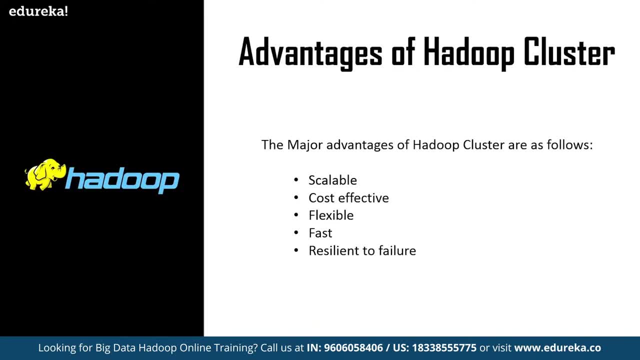 semi-structured or completely unstructured. this enables Hadoop to process multiple types of data directly from social media. The fourth advantages: Hadoop clusters are fast. Hadoop clusters can process petabytes of data Within a fraction of second. This is possible because of the efficient data mapping capabilities. 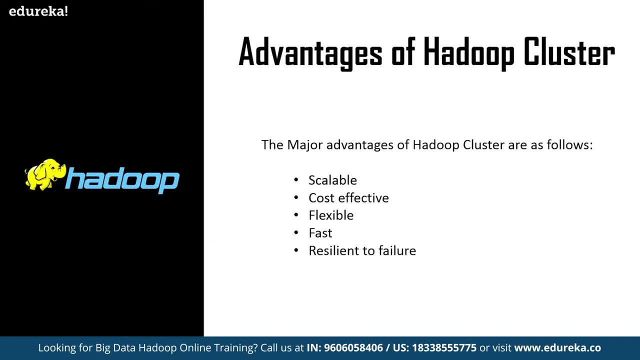 of Hadoop. The fourth feature is how to clusters are fast. Hadoop clusters can process petabytes of data within a fraction of second. This is possible because of the efficient data mapping capabilities of Hadoop. the secret behind high-speed performance is that the data processing tools are always kept available on the service That is the data processing. 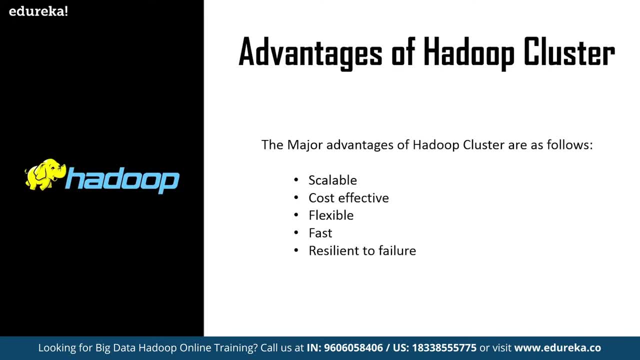 tool is available on the same unit where the data needed is stored. the fifth advantage is the data clusters are resilient to failure. The data loss in a Hadoop cluster is a myth. It is practically impossible to lose any data in a Hadoop cluster. as it follows the data replication. 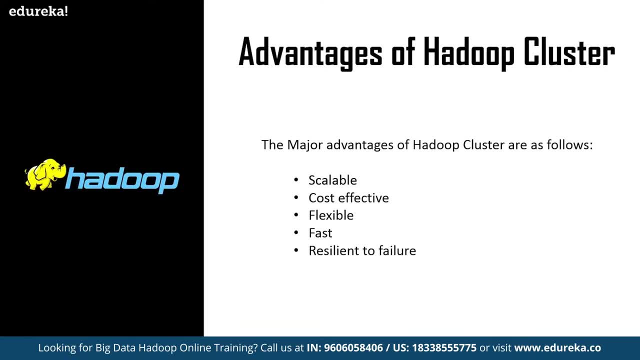 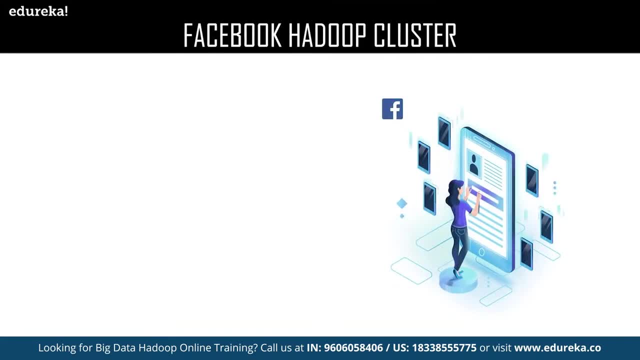 which acts as a backup storage unit in a case of a note failure. So with this, let us move on to our next topic, which is related to Facebook's Hadoop cluster. since 2004, from its launch, Facebook is one of the biggest users of Hadoop cluster. It is called as the beefiest Hadoop cluster. It approximately 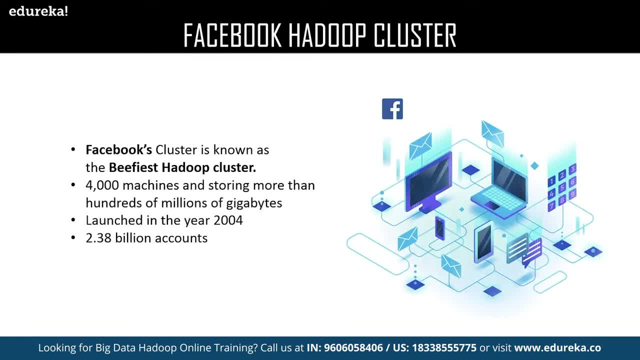 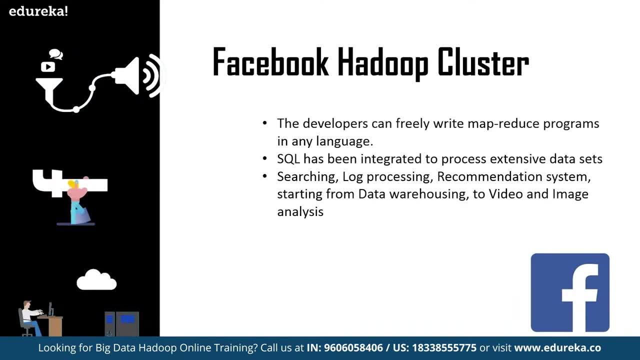 uses 4,000 machines And is capable to process millions of gigabytes. together, Facebook has 2.38 billion number of active users. to manage such a huge Network, Facebook uses multiple storage frameworks and millions of developers writing MapReduce programs in multiple programming languages. 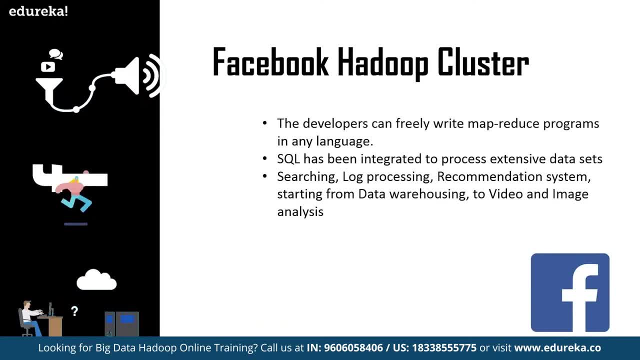 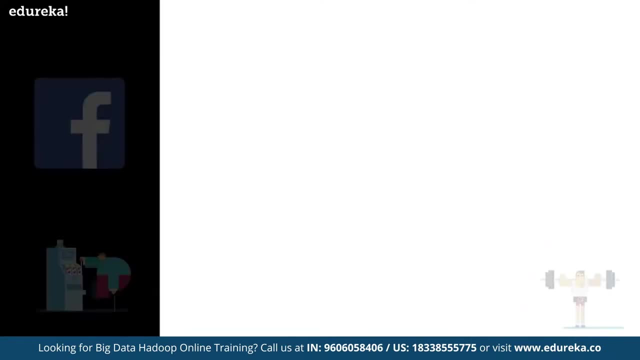 It also uses sequel, which drastically improve the process of search log processing, recommendation system, starting from data warehousing to the video and image analysis. Facebook is growing day-to-day by encouraging all possible updates to its cloud Luster scuba. with a huge amount of unstructured data coming across each and every day, Facebook 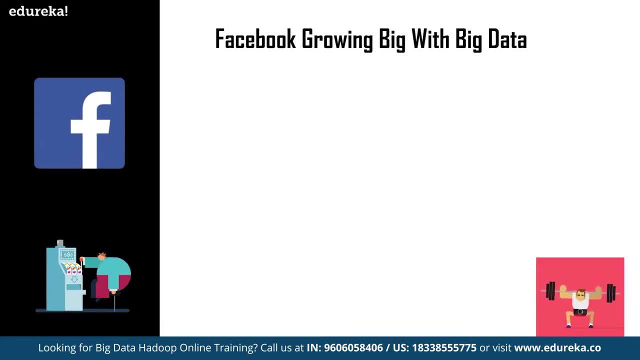 slowly realized that it needs a platform to speed up the entire analysis part. This is when the scuba was developed. Hadoop developers can dive into massive data sets and carry on ad hoc analysis in real time. The second update was Cassandra. the traditional data storage units started lagging behind. 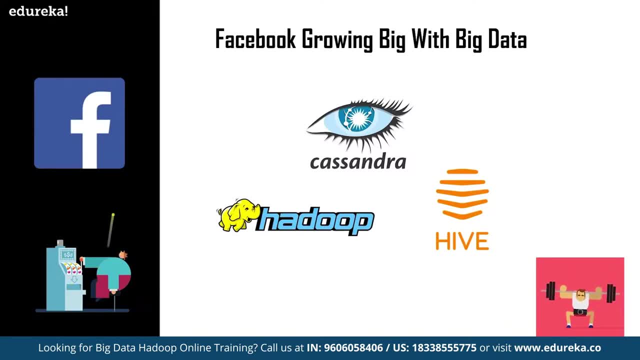 when Facebook search team discovered an inbox search problem, the developers were facing issues in storing The reverse indices of messages sent and received by the users. The challenge was to develop a new storage solution that could solve the inbox search problem and similar problems in the future. 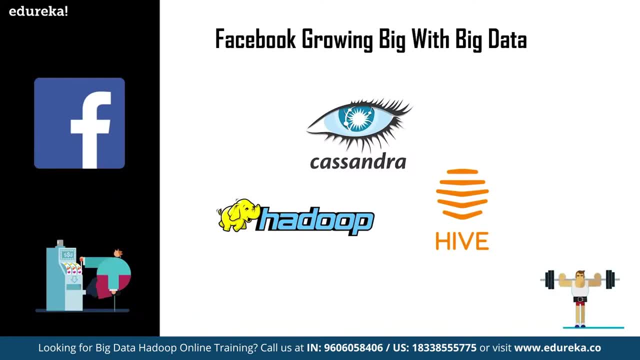 The objective was to develop a distributed storage system dedicated to manage a large amount of structured data across multiple commodity service without even failing for once. This is when the Cassandra was developed. The next update is hive, after Yahoo implemented Hadoop for its search engine, Facebook thought. 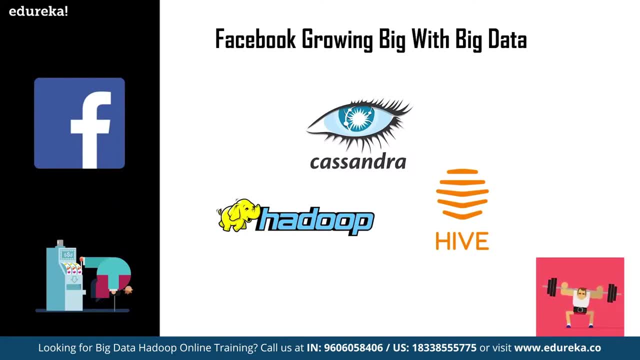 about Hiding the data scientists so that they could store larger amount of data in the Oracle data warehouse. Hence hive came into existence. this tool improve the query capability of Hadoop by using a subset of sequel and soon gained popularity in the world of unstructured data today, almost 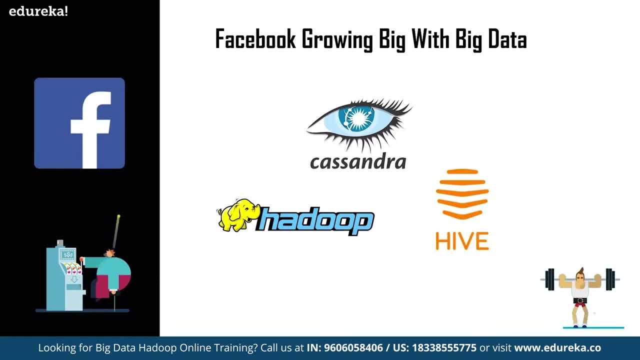 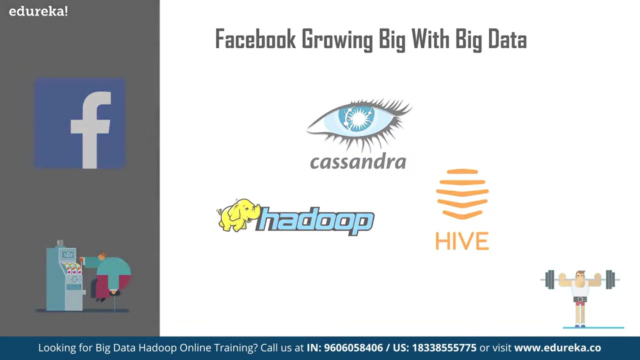 thousands of jobs are ran using this system to process a range of applications quickly. today, Facebook is one of the biggest corporations on Earth, Thanks to its active two and a half billion users. Let us have an overview on the Facebook's Hadoop cluster. then let us move on to the architecture of Hadoop cluster. 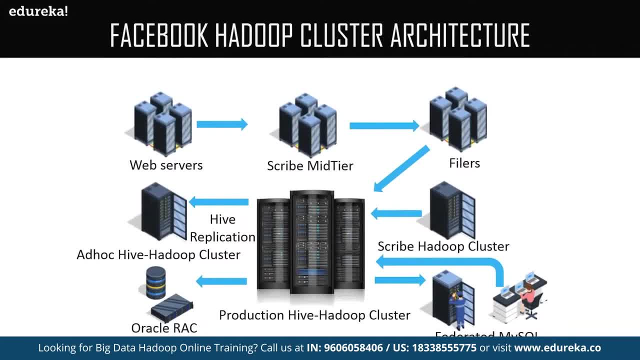 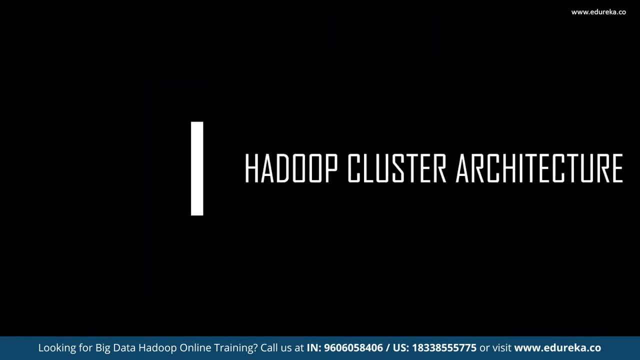 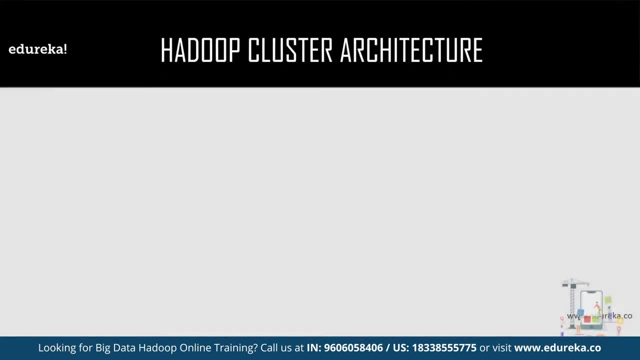 So this is the overview of Facebook's Hadoop cluster, which consists of web service, ad hoc Hive Hadoop cluster, production Hive Hadoop cluster and many more. now that we have gone through a few facts on Facebook's Hadoop cluster, Let us move on to the Hadoop architecture, which has the following components: the architecture: 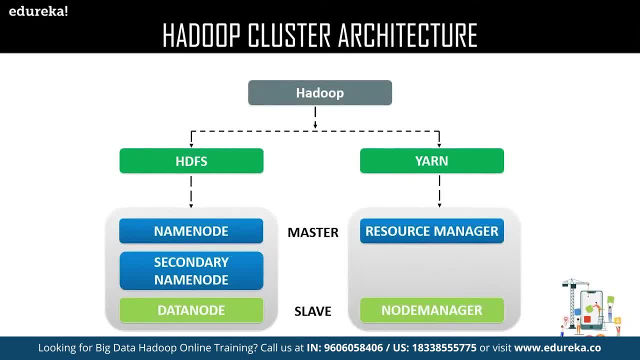 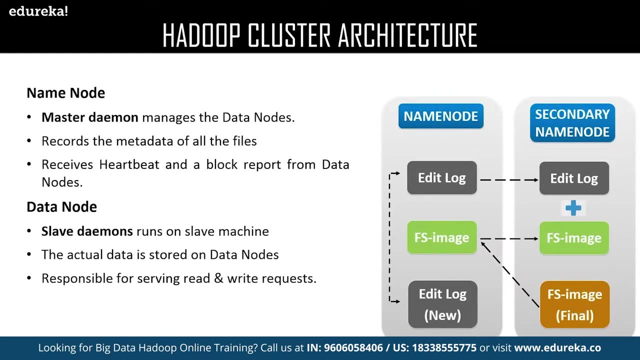 of Hadoop consists the following components: HDFS and yarn. let us now begin with HDFS. HDFS consists of the following components: the name node, secondary name node and data node. Let us discuss about each one of them in detail. name node: name node is responsible for running. 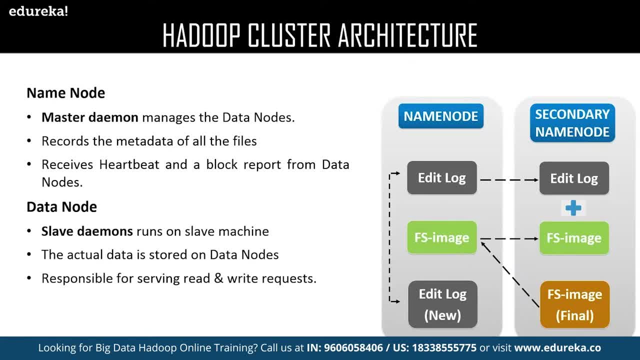 master demons name node is designed to store the metadata, which means the information about the actual data or, in short, the schema of the data name node is the first one to encounter the clients request for data. it then transfers the request to the data nodes which store the actual data. 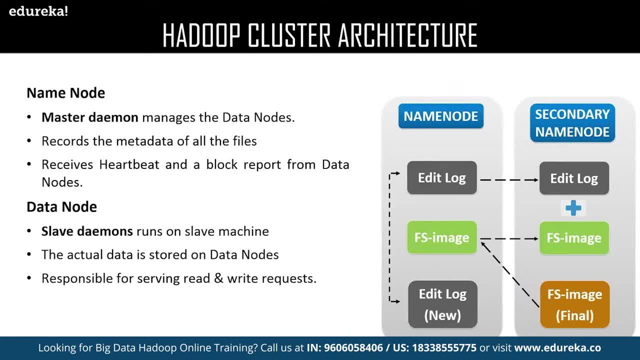 The name Node is responsible for managing the health of all the data nodes. it receives a heartbeat from all the data nodes at a particular interval of time and it also receives a status update of the task assigned. if any of the data node fails to respond with a heartbeat, then the 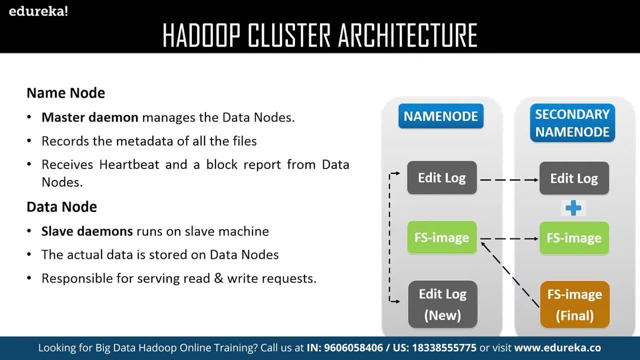 name node considers the data node to be dead and it reassigns attached to the next data node. The next one is data node. data nodes are called as a slaves of name node and they're responsible to store the actual data and also to update the task status and health status. 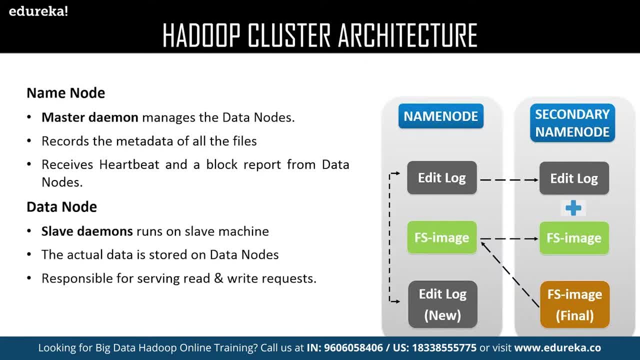 To the name node in the form of a heartbeat. Now the last one is the secondary name node. the secondary name node, as it speaks, is not actually a backup of name node, but it actually acts as a buffer which saves the latest updates to the FS image which are obtained in the intermediate process and finally updates them. 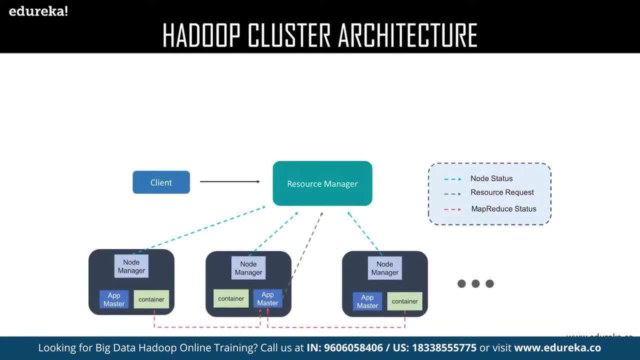 to the final FS image. Now let us discuss about Yann Yann, yet another resource negotiator. Yann consists the following elements: Node manager, app master and container. Let us discuss each one of them in detail. node manager: node manager is a Java utility. 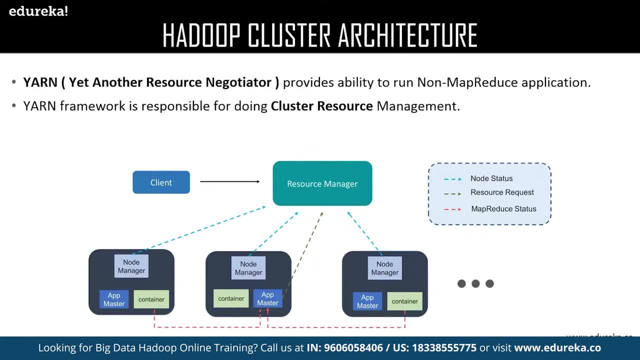 that runs as a separate process from web logic server. It allows you to perform common operations for a managed server, regardless of its location with respect to the administration server. The second one is app master. app master is responsible for negotiating the resources between resource manager and node manager. and the last one is the container. 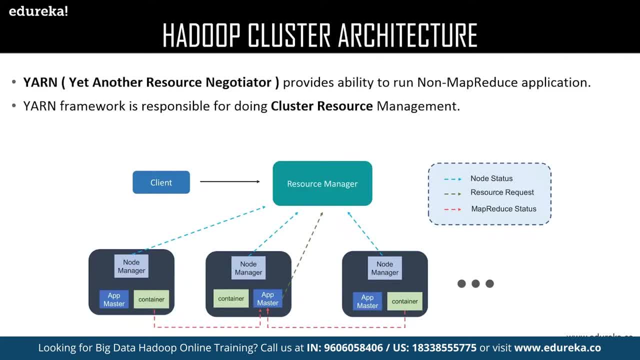 The container is actually a collection of reserved amount of resources allocated from the resource manager to work with the task assigned by the node manager. Now, with this, we shall have a look on the overview of the Hadoop cluster architecture and followed by that we shall look into the rack awareness algorithm. 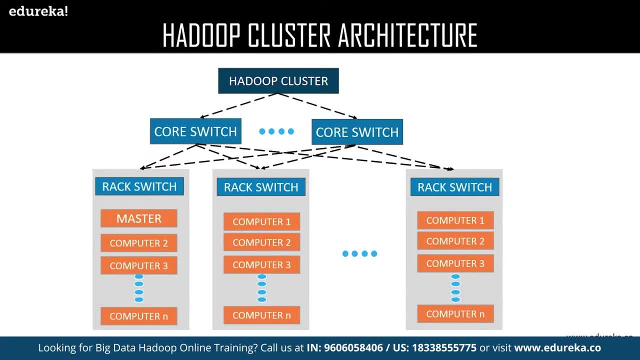 So this is the architecture of Hadoop cluster, which consists of racks. each and every rack consists of a set of computers and one of the rack consists master, and these racks use core switches to communicate between each other. Now let us move on to the rack awareness algorithm. 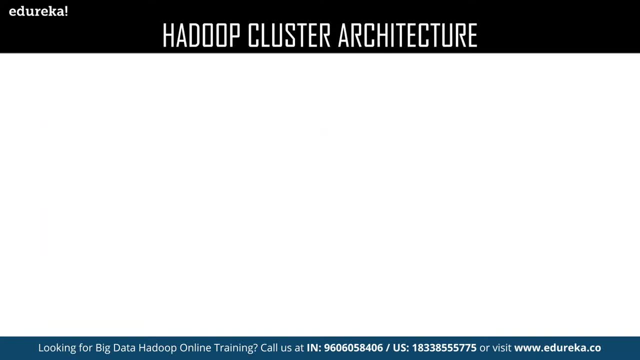 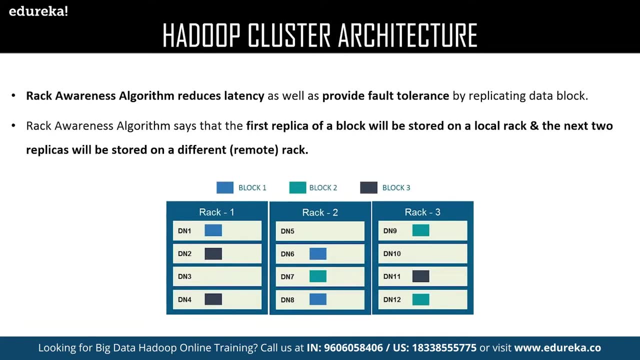 The rack awareness algorithm is all about data storage. It says that the first replica of the actual data must be located in the local rack and the rest of the replicas can be stored on a different, remote track. Let us look onto an example to understand this in a better way here. 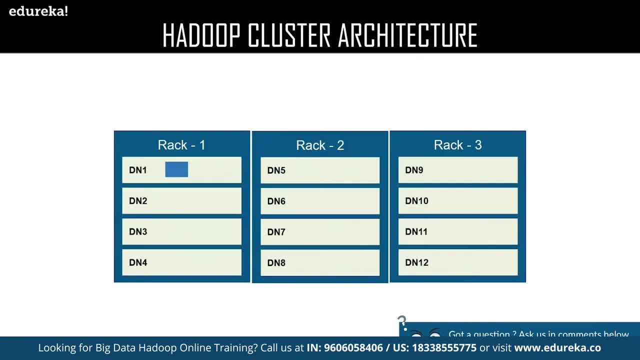 I'm having a data block on the data node one and the data node one is available on the rack one, which happens to be a local track. now, according to the rack awareness algorithm, the replica of the data block in data node one can be stored in the remote tracks which 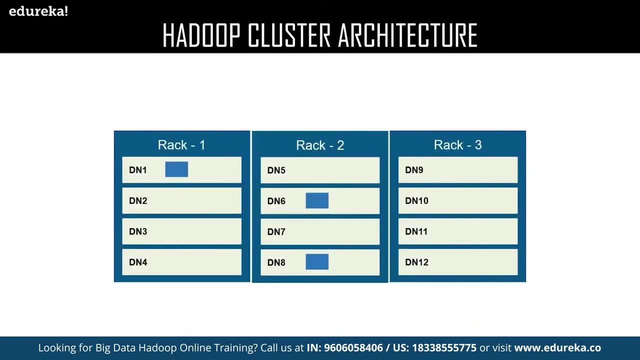 might be rack 2 or rack 3. as you can see, the replicas have been stored in a remote track, which is the rack number 2. now let us deal with a different block. as you can see, we have a new block in rack number 2, data node 7.. 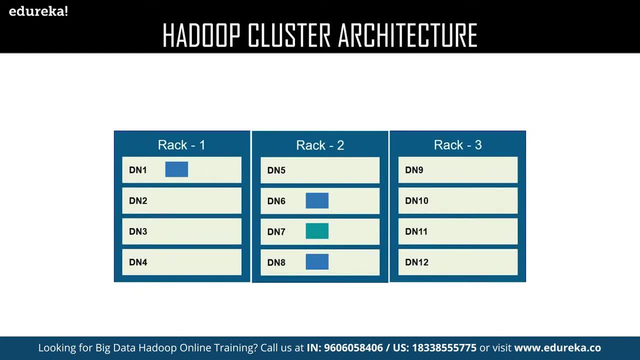 This is the local rack for the data block stored in data node 7.. Now let us see where the replicas of data node 7 are stored. the replicas of data node 7 are stored into them. As you can see, now we have a new data block stored in the data node 11, and rack 3 is a. 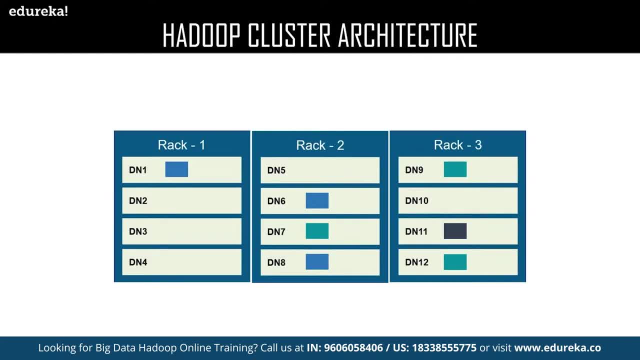 local rack for the data block stored in data node 11.. Now let us see where the replicas of data node 11 are stored. as you can see, the replica blocks of data node 11 are stored in the remote track, which is rack number 1 and the data blocks. 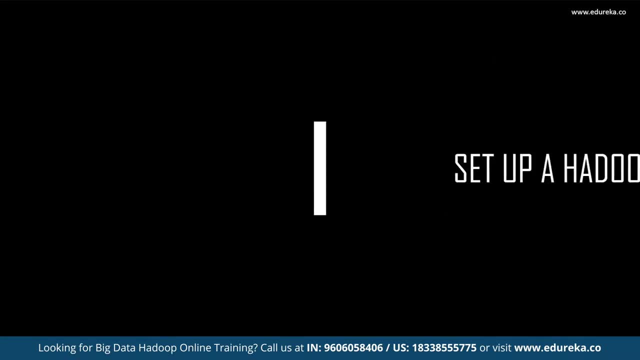 are stored in data node 2 and data node 4. with this we have finished our theory part. now let us get into the practical part, where we'll learn to set up a Hadoop cluster with one master and two sleeves. So let us begin with a practical session here. 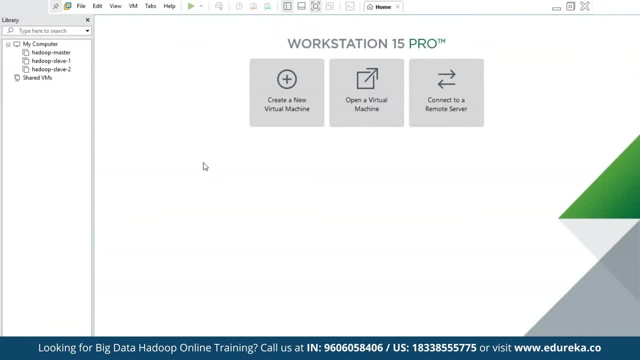 We must create three host systems, out of which one is the master and the other two are the sleeves. So I'll be choosing the Linux operating system for this, and I'll be using CentOS 7.. I'll be starting with creating a new virtual machine. 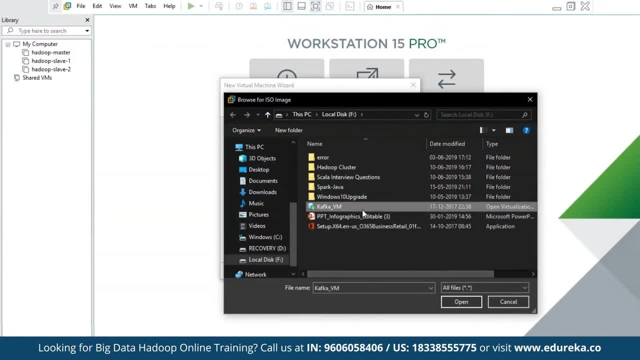 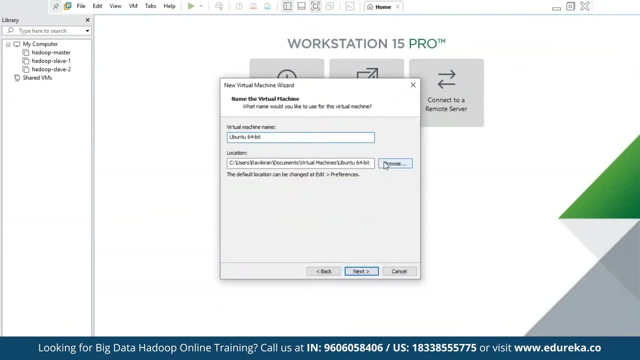 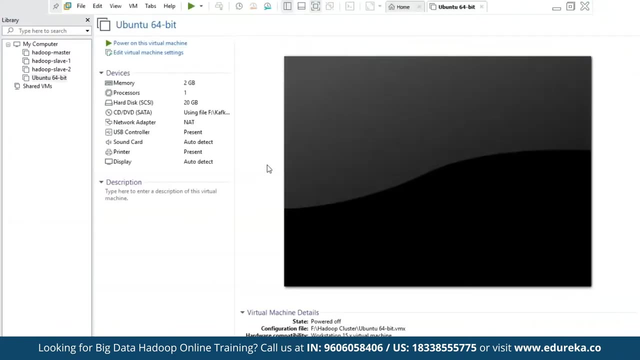 Here I'll be selecting my ISO image. This happens to be my ISO image, which has the Hadoop pre-installed. select the process, finish and, using the similar process, you must create two new host systems and you must name them as Hadoop, slave 1 and slave 2, as I have done here. as you can see, I have my Hadoop. 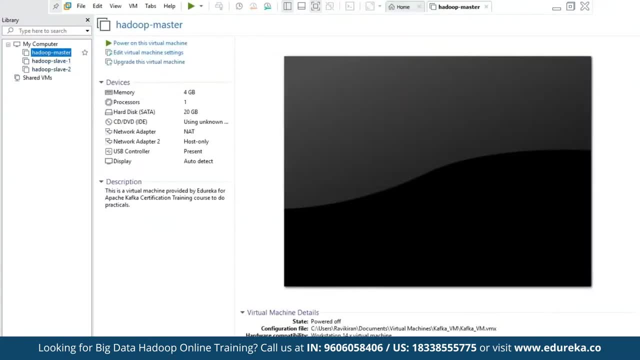 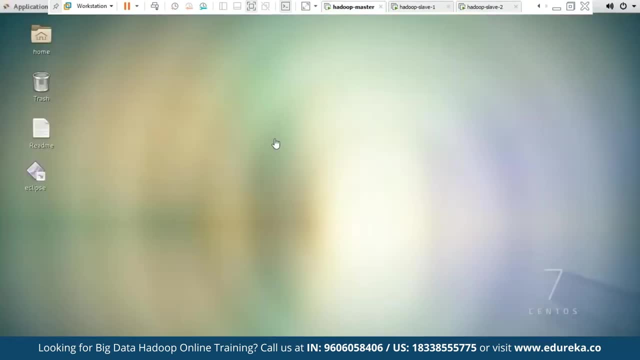 master here and Hadoop slave 1 and Hadoop slave 2.. Let me start each one of them Now. I have started my Hadoop master, Hadoop slave 1 and Hadoop slave 2. now all the components of Hadoop cluster, which are the Hadoop master, Hadoop slave 1 and Hadoop slave 2, all are 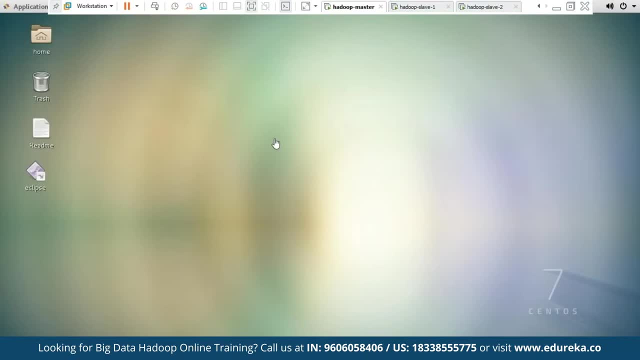 started assuming that you know how to install Hadoop. I have chosen a CentOS operating system which has the Hadoop pre-installed. now let us start our local host. Our local host is started. now let us see the HDFS web user interface. 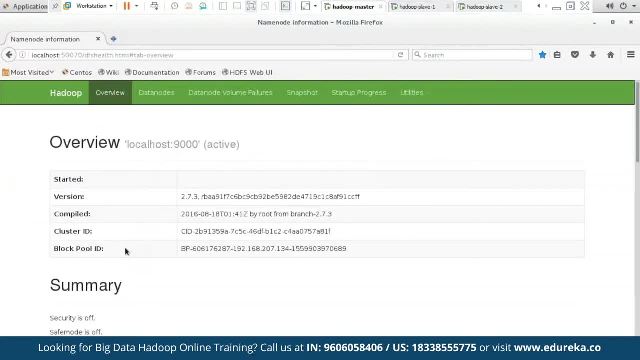 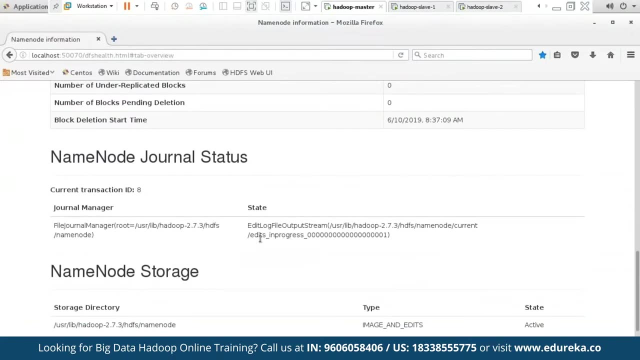 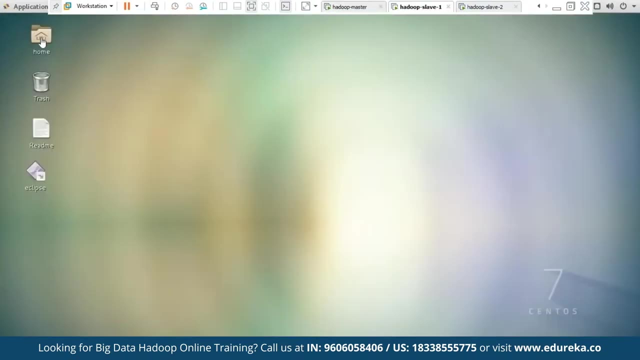 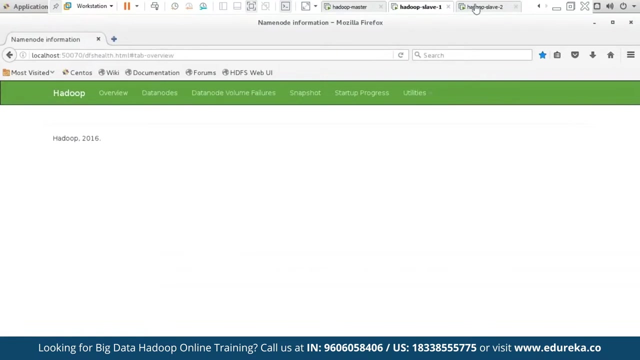 This is how our HDFS web user interface looks like and you can see our name. note is in progress and similarly, let us try to start the HDFS web user interface in our Hadoop slave 1 and slave 2.. As you can see, the HDFS web user is been successfully started on Hadoop master, Hadoop slave 1 and 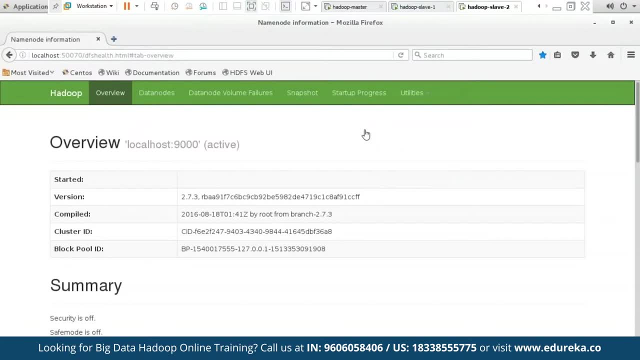 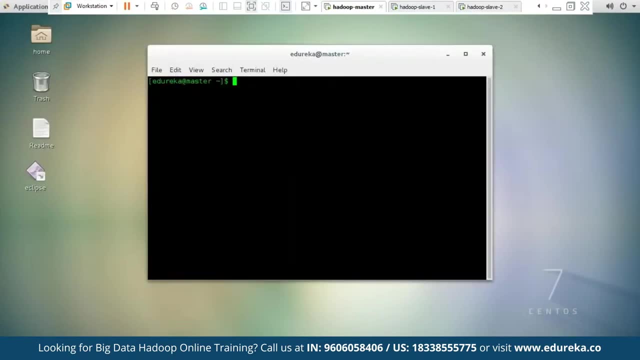 Hadoop slave 2. now let us begin with setting up our Hadoop cluster with Hadoop master and Hadoop slave 1 and slave 2.. Before getting started, our first job will be getting to know the IP address of our Hadoop master. to know the IP address of the Hadoop master. 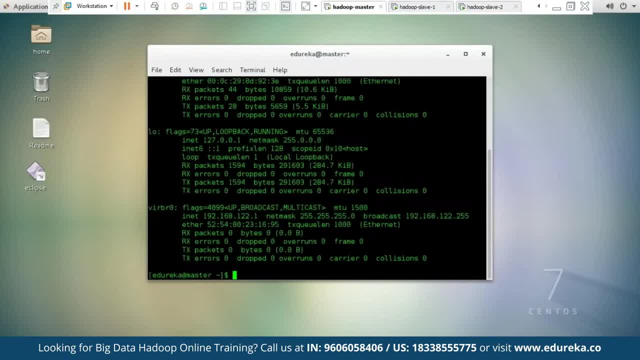 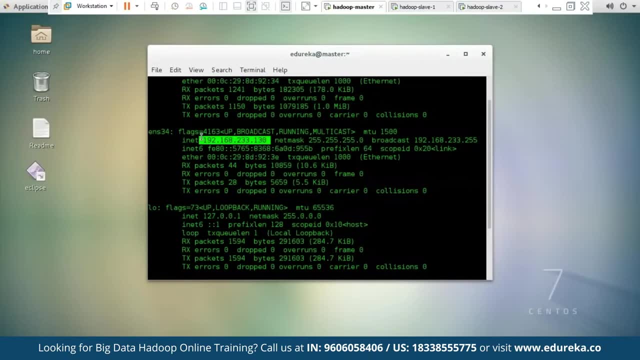 We can type in the command if config. this command will give us the IP address of our Hadoop master here. My IP address is 192 dot 168 dot 233 dot 130. similarly. similarly, let us find out the IP address of our Hadoop slave 1 and slave 2. now I'm in the slave 1 here. 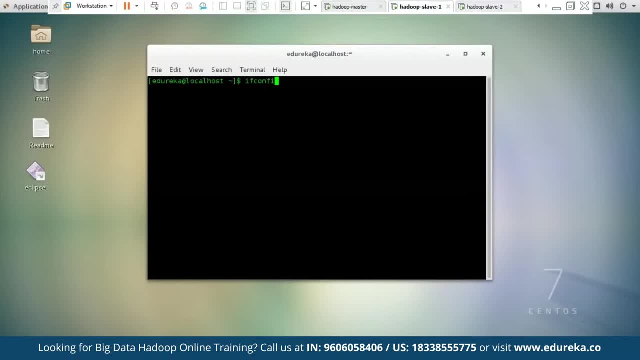 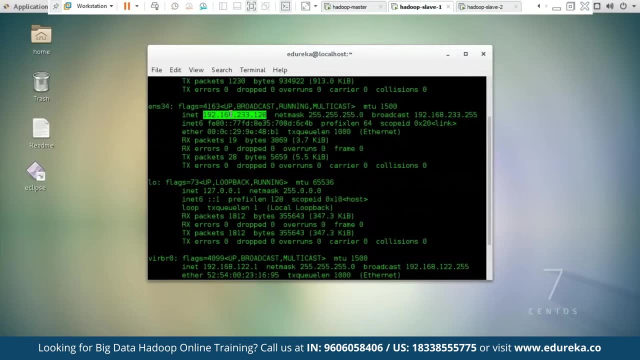 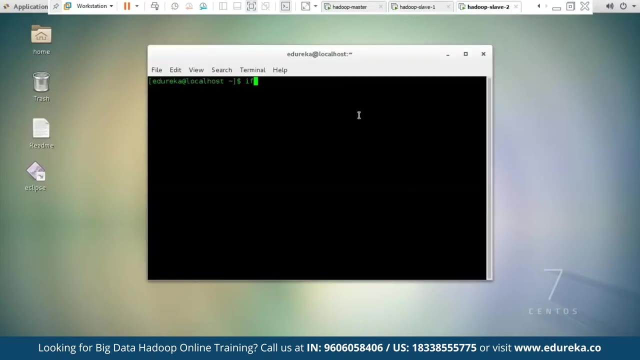 I'll type in my command if config, which must show me my IP address of slave 1.. So here, the IP address of the slave 1 is 192 dot 168, dot 233, dot 138.. Similarly, let us find out the IP address of slave 2. as you can see, the IP address of 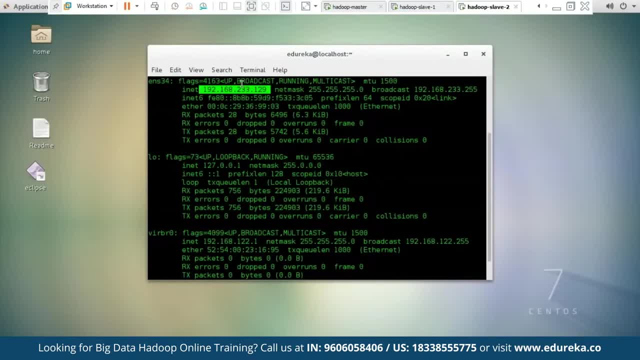 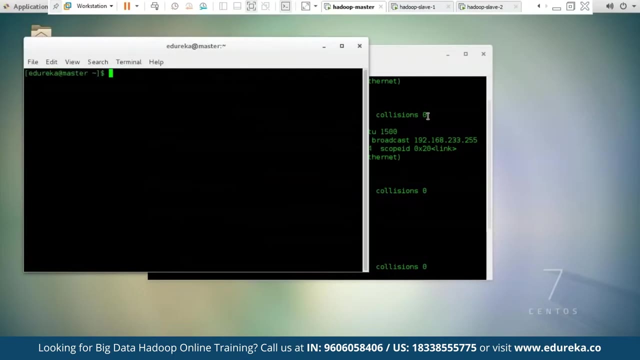 slave 2 is 192, dot 168, dot 233, dot 129.. Now our next job is to edit the host and set the IP addresses of the master and slaves. Now let us open a new terminal. You can edit the host by the command vi, etc. slash master. 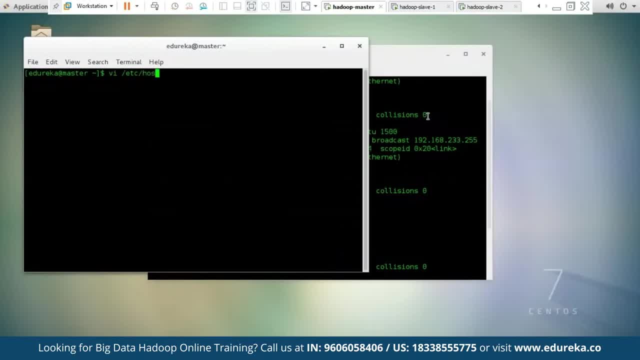 Now let us open a new terminal. You can edit the host by the command vi, etc. slash hosts. here I have already edited the host. as you can see, I have given 192 dot, 168 dot, 207 dot, 134 as my Hadoop master and 192 dot, 168 dot, 233 dot, 128 as my slave 1 and finally 192 dot. 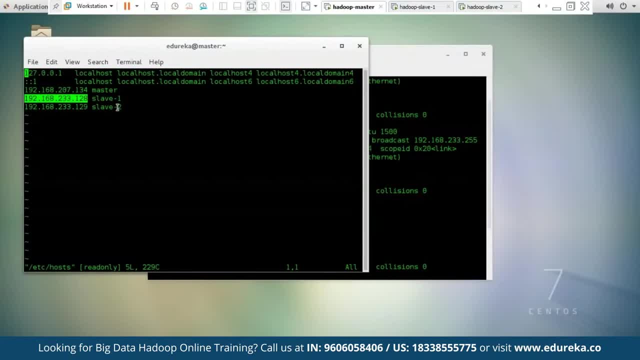 168, dot 233, dot 129 as my slave 2. this step must be followed on all the three machines, which is the Hadoop master, Hadoop slave 1 and Hadoop slave 2. once you define the IP addresses, you can simply press escape and colon wq to exit the terminal and save the changes you. 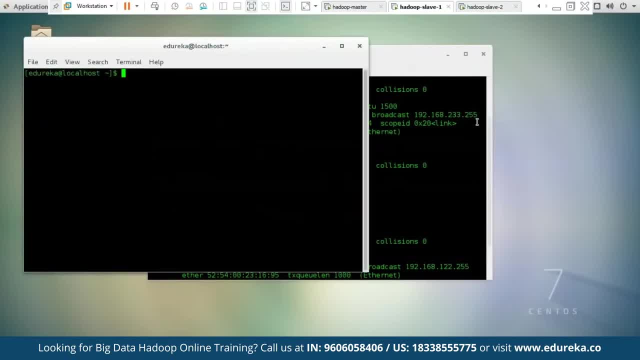 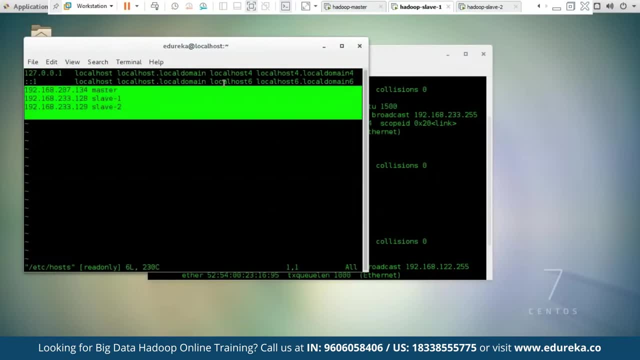 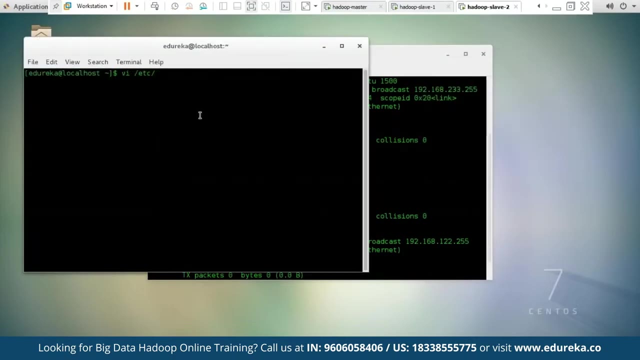 made in the terminal. As you can see, I have made the same changes in Hadoop slave 1 and you can also see the same changes in Hadoop slave 2.. Remember, Yes, Remember. you have to follow all these changes in all the three machines, which includes Hadoop. 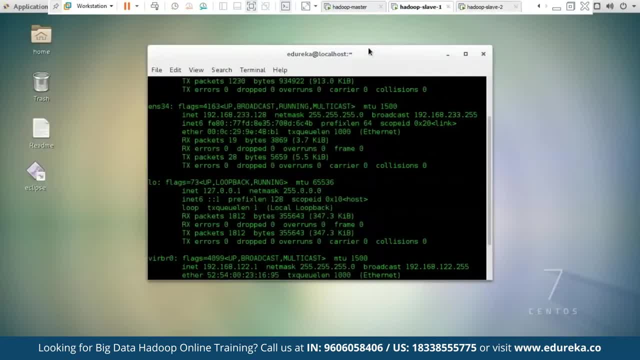 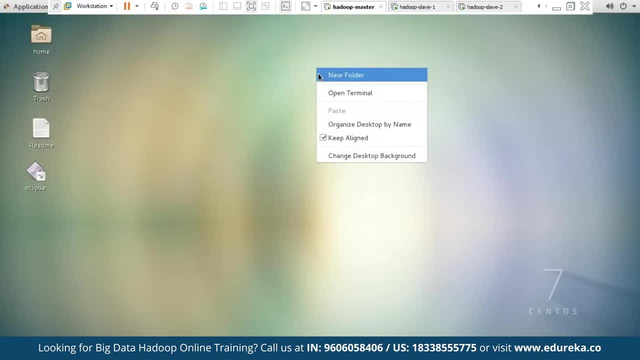 master and Hadoop slaves. Now we know that we have defined the IP addresses of all the three machines. to all the three machines. Now let us see if they work or not. Let me open a new terminal and try to ping the Hadoop slave 1.. 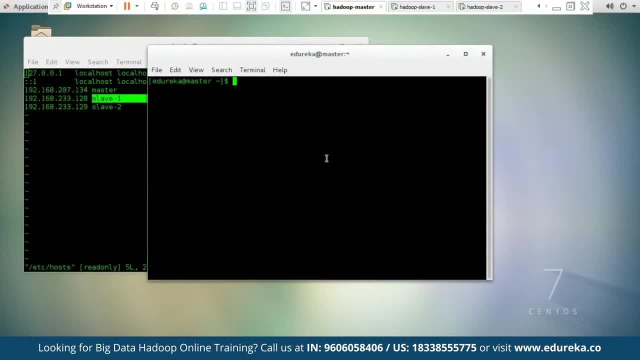 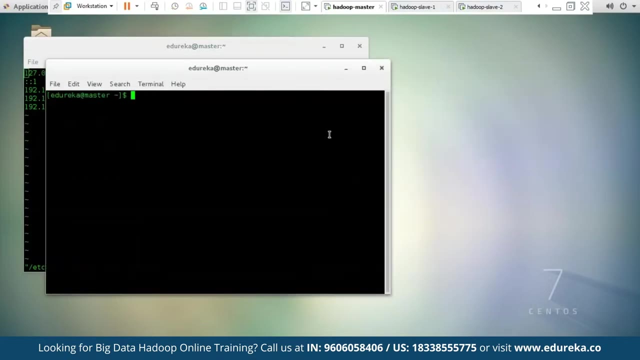 The name of my Hadoop slave 1 is slave 1.. So let me write ping to slave 1.. As you can see, the ping is successful and the data has been sent to the slave 1.. Now let me open a new terminal and try to ping to my next slave using the command ping. 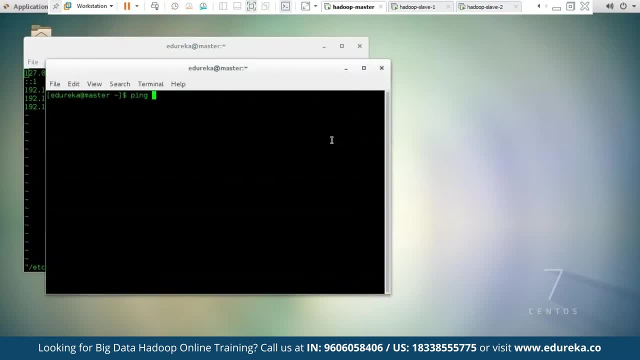 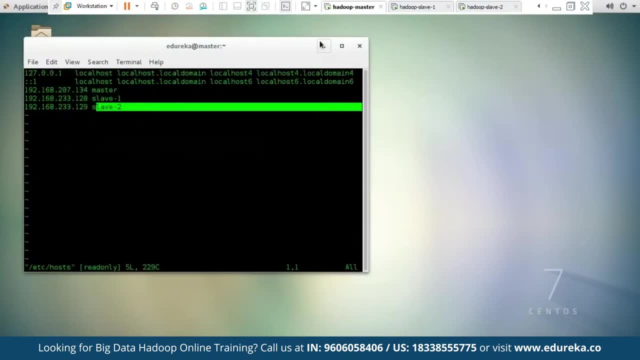 As you can see, my second slave name is slave 2.. So I'll be writing slave 2 and I'll start the ping. as you can see, the ping is successful Now. similarly, let us try this on our slaves. to let me open a new terminal on slave 1 and 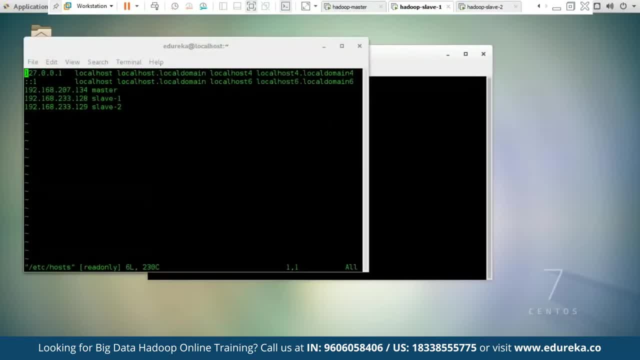 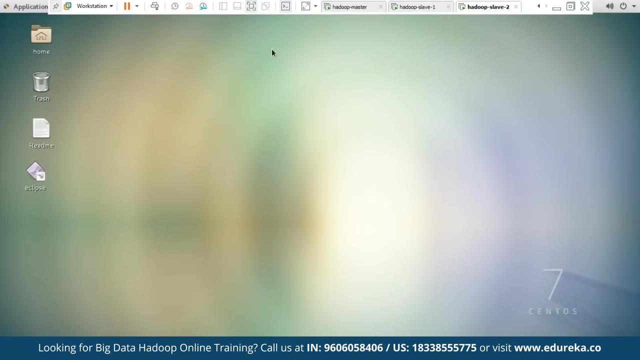 let me type in The command to ping the master. As you can see, the name of my master is master, So let us try to ping to the master. The ping is successful and the data has been sent. similarly, Let us try on a slave to if slave 2 can successfully send ping to the master or not. 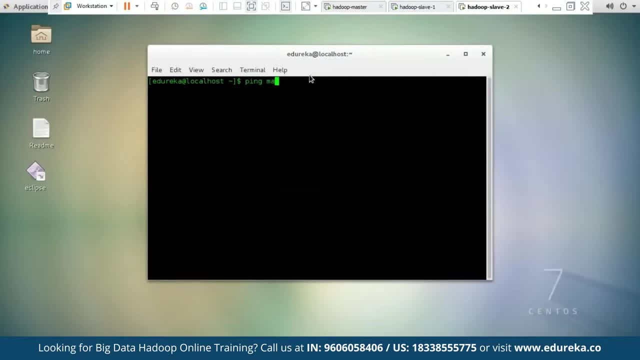 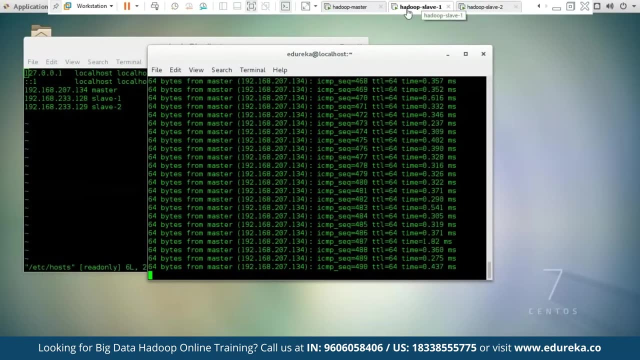 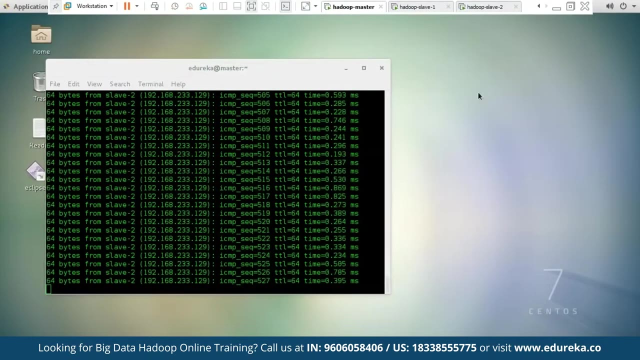 Let us open a new terminal and write in ping to the master. As you can see, the data has been successfully sent to the master here, So with this We have successfully established a Hadoop cluster consisting of Hadoop master and Hadoop slaves. 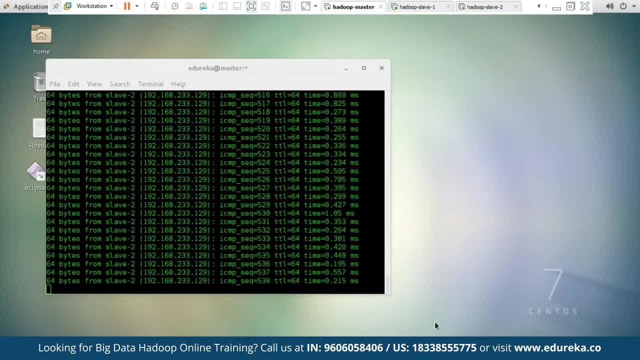 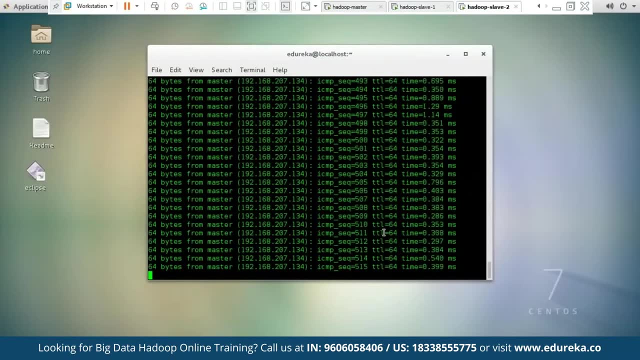 As you can see, the pings are successful. The master is communicating with both slave 1 and slave 2 and, similarly, the slave 1 is communicating with master and slave 2 is also communicating with master. Now, with this, we have finished our demo session. 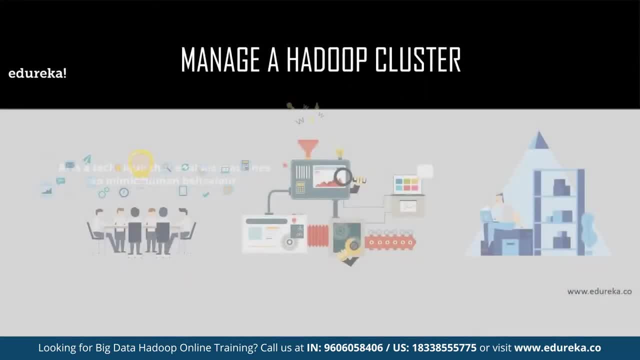 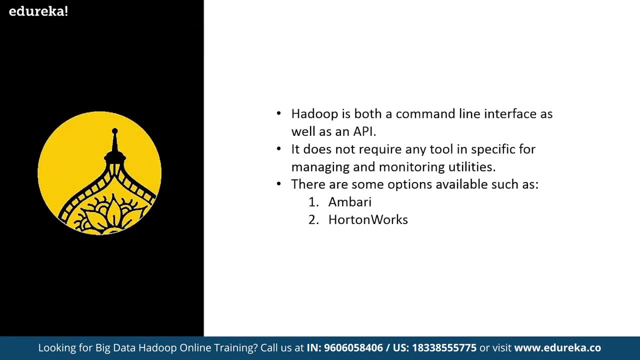 Now let us learn about managing a Hadoop cluster. Hadoop is both a command line interface as well as an API. It does not require any tool in specific for managing and monitoring utilities. yet There are some options available, such as Ambari and Orton works. 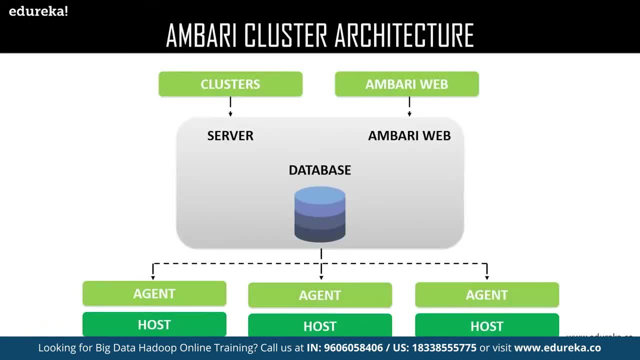 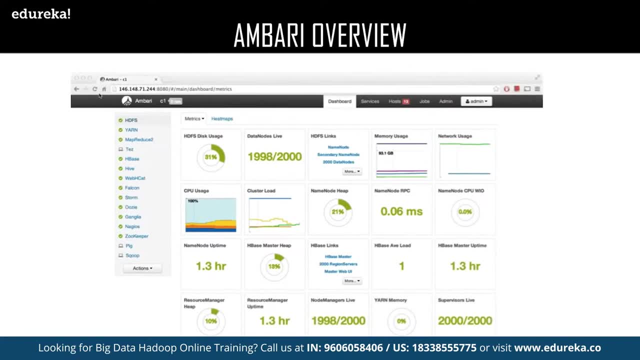 The most popular one is the Ambari. Let us see How does a typical Ambari user interface looks like. so this is how a typical Ambari user interface looks like. we can see the HDFS disk usage percentage data notes: alive memory usage. 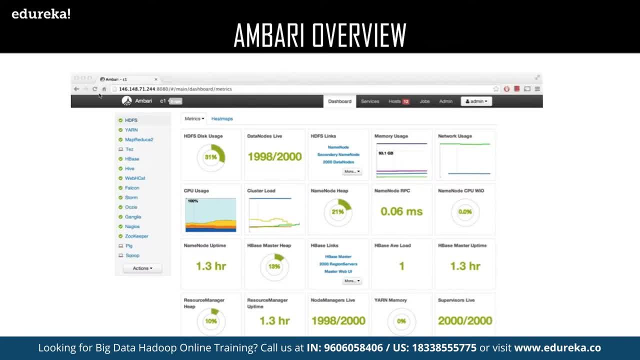 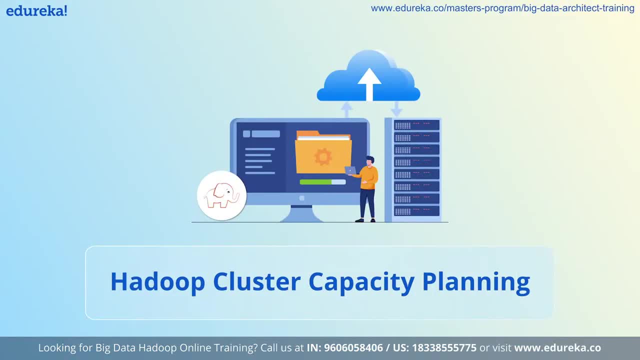 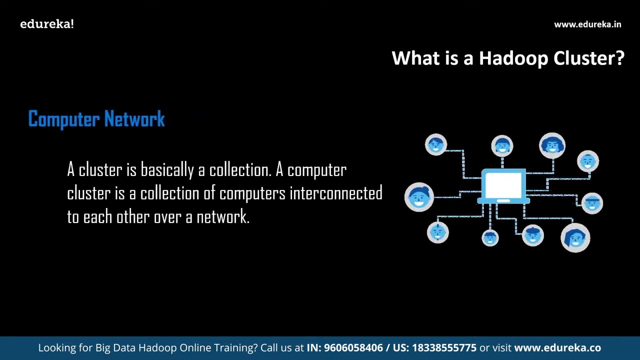 graph, network usage graph and CPU loads, cluster load, Name, node heap and many more. What is a Hadoop cluster? a cluster is basically a collection. a computer cluster is a collection of computers interconnected to each other over a network. Similarly, a Hadoop cluster is a collection of extraordinary computational systems designed. 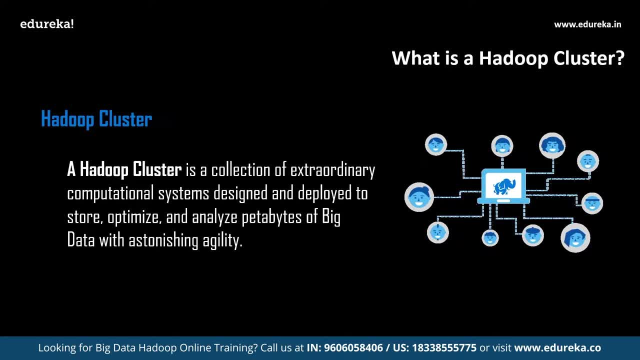 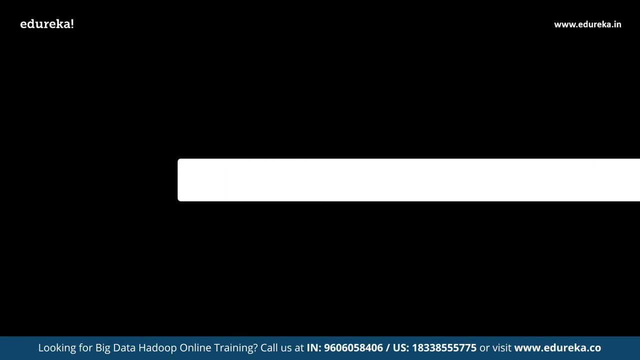 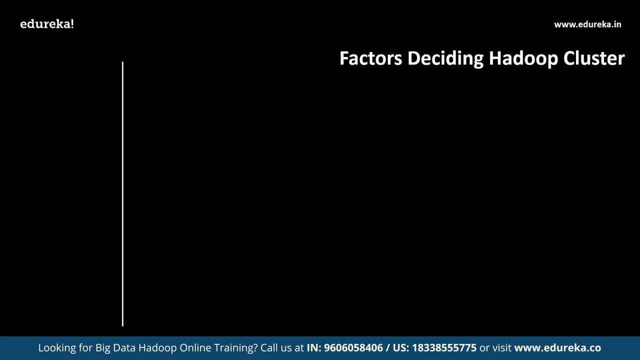 and deployed to store, optimize and analyze petabytes of big data with astonishing agility. Now that we are clear with the definition of Hadoop cluster, we shall move ahead and understand the factors that decide the Hadoop cluster capacity, The various factors that we need to look into in order to design and deploy an efficient 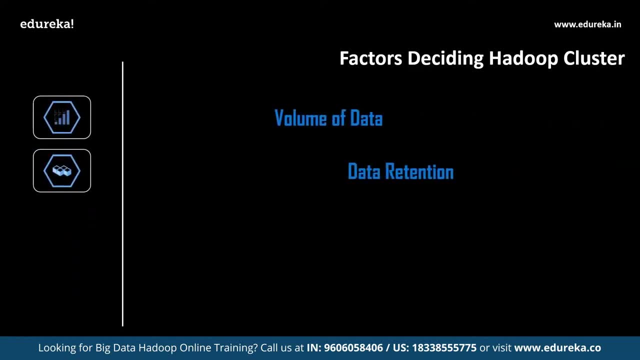 Hadoop cluster are volume of data, data retention, data storage and the type of workload. We shall discuss each one of them in detail. We shall discuss the first factor, which is the volume of data, and what is its role when it comes to deciding the capacity of a Hadoop cluster. 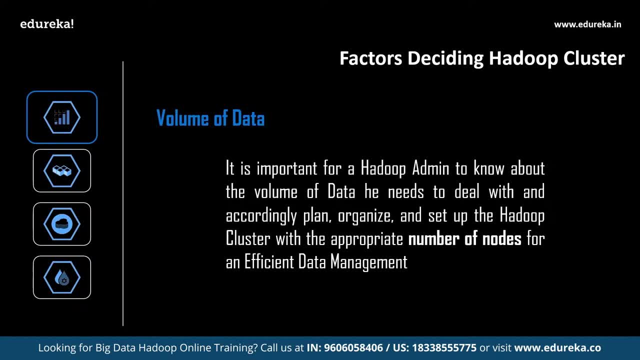 So if you ever wonder how Hadoop came into existence, then it is because of huge volume of big data that the traditional processing systems couldn't handle. since the introduction of Hadoop, the volume of data is increased exponentially, So it is important for a Hadoop admin to know the volume of data he needs to deal with and 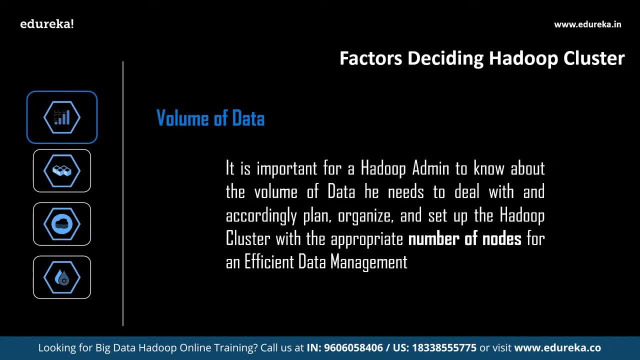 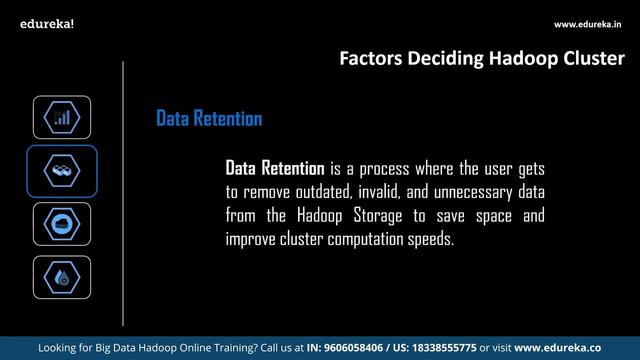 accordingly: plan, organize and set up the Hadoop cluster with appropriate number of nodes for efficient data management. followed by the volume of data, The next factor is data retention. Data retention is all about storing important and valid data. There are many situations where data arrived will be incomplete or invalid. that may affect 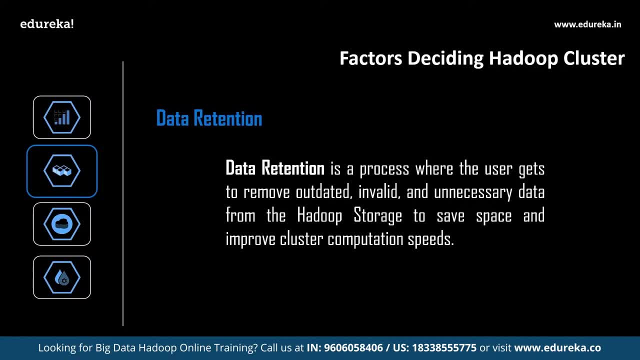 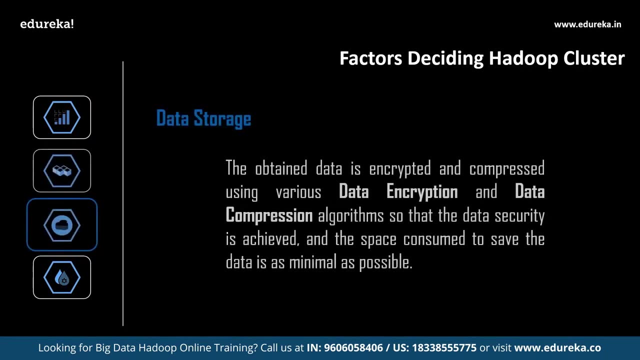 the process of data analysis, So there is no point in storing such data. Data retention is a process where the user gets to remove outdated, invalid and unnecessary data from the Hadoop storage in order to save and improve the cluster computation speeds, followed by data retention. 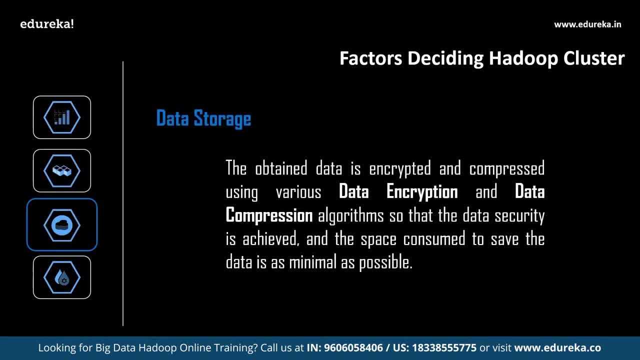 The next important feature is The data storage. data storage is one of the most crucial factors that come into picture when you are into planning a Hadoop cluster. data is never stored directly. as it is obtained, it undergoes through a process called data compression. here The obtained data is encrypted and compressed using various data encryption and data compression. 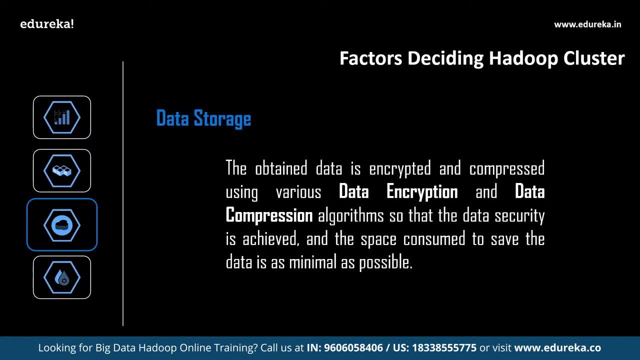 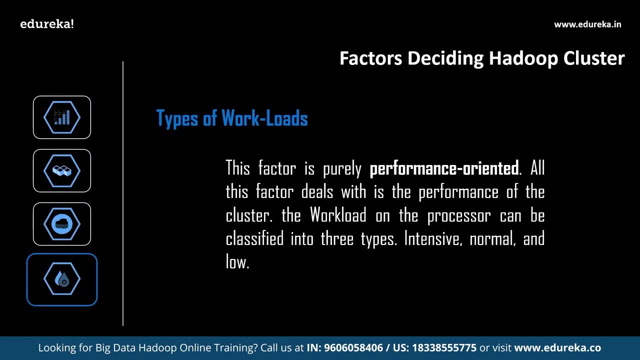 algorithms so that the data security is achieved and the space consumed to save the data is as minimal as possible, followed by the data storage. The last and the most important factor is the type of workloads. this factor is purely performance oriented. all this factor deals with the performance of the cluster, the workload. 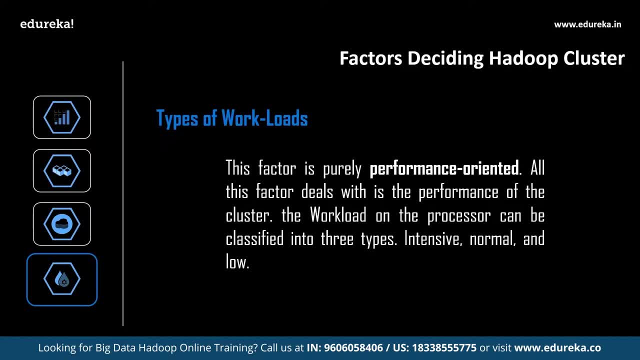 on the processor can be classified into three types: intensive, normal and low. some jobs, like data storage, will cause low workload on the processor. jobs like data querying will have an intense workload on both the processor and the storage unit on the cluster. So the type of workloads. 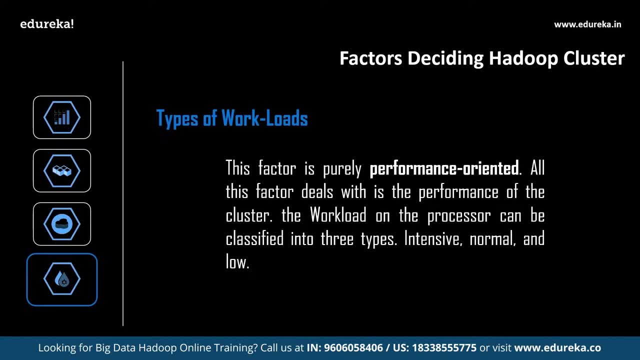 Also, It doesn't matter a lot. So if you want to have a smooth and efficient cluster, then the processes you use and the RAM you use should be high-end. So these were the factors that decide the planning of her to cluster, followed by this: 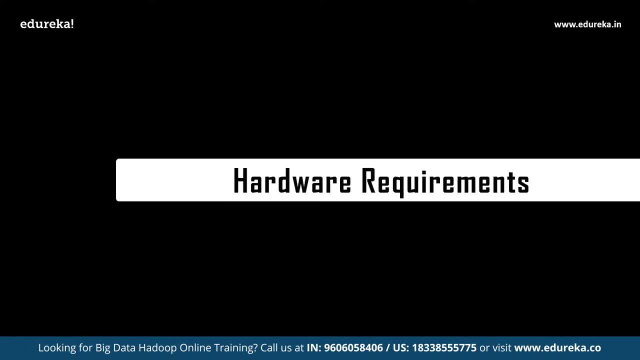 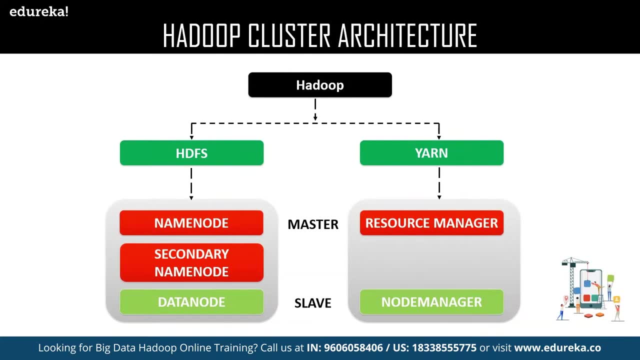 We shall move into the next topic, which deals with the hardware requirements of Hadoop cluster. But before that let us understand the Hadoop architecture. in the Hadoop architecture We have the following components: the HDFS and yarn. inside HDFS We have name node and secondary name node. 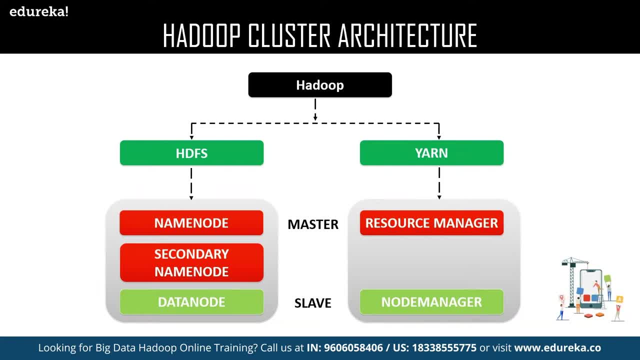 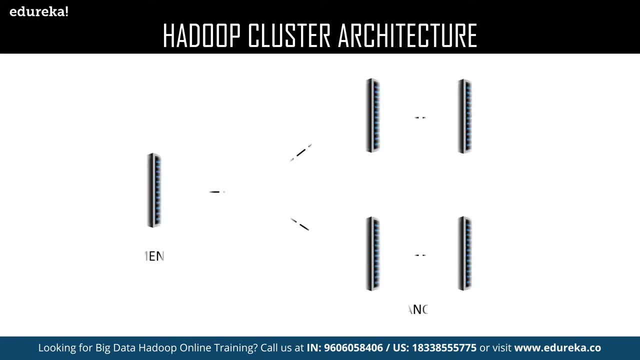 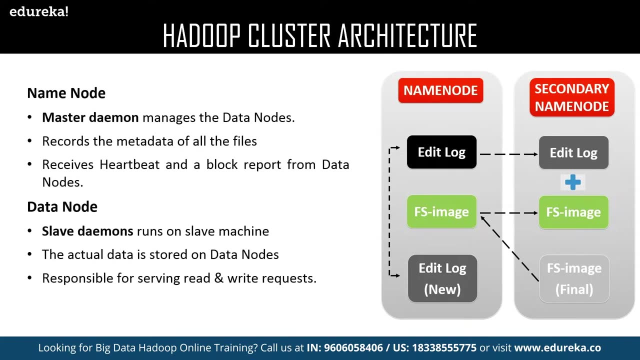 which are considered as Masters. similarly, Indian resource manager would be your master and when it comes to slaves, data nodes and node managers are the slaves. So basically, name node controls all the data nodes which are existing in a Hadoop cluster. name node is considered as the master demon that manages the data nodes. 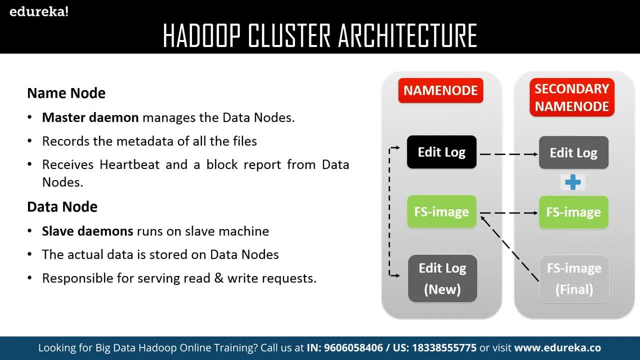 The name node records all the metadata or the schema of all the files which it receives, followed by that name node receives a heartbeat and a block report from all the data nodes. on the other hand, data nodes are considered as a slave demons that run on slave machines. 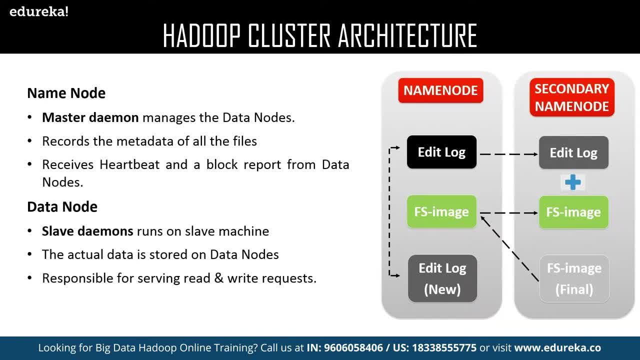 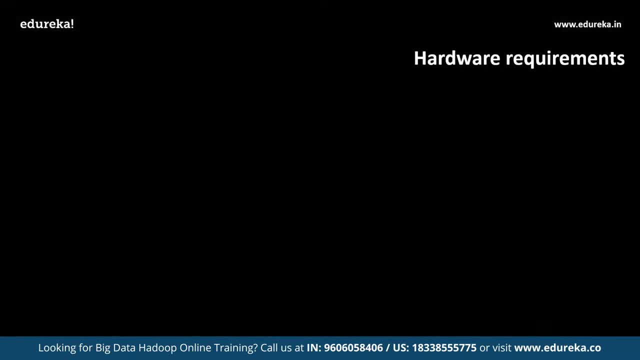 The actual data is stored on data nodes and the data nodes are responsible for serving read and write requests. So this was the architecture of Hadoop. Now let us discuss about the hardware requirements. The name node, secondary name node and job tracker are the Masters. the name node: 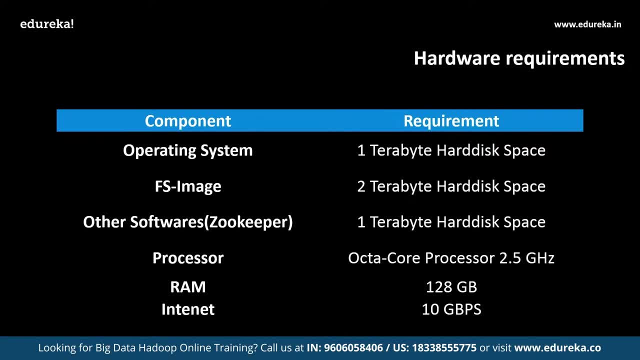 and secondary name nodes are the most crucial parts of any Hadoop cluster. They are expected to be highly available. the name node and secondary name node servers are dedicated To store all the namespace storage and edit log journaling. So the hardware requirements for these nodes are at least four to six essays storage tests. 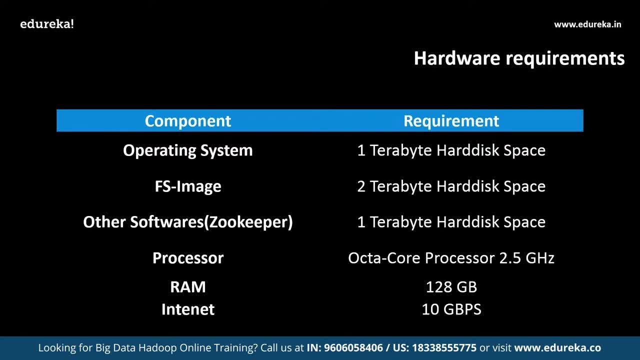 So these tests will be divided as follows: one terabyte hard disk space will be dedicated for operating system, followed by that, two terabyte hard disk space will be dedicated for FS image storage, followed by that, one terabyte hard disk memory will be given for other softwares like Apache, Zookeeper. 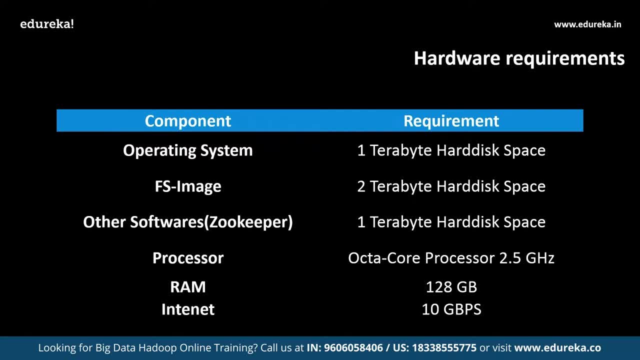 and other required softwares. Now, when we come into the processor, we require a hexa core or at least a octa-core processor with 2 to 2.5 gigahertz processing speed. And now, if we discuss about Ram, we have to include 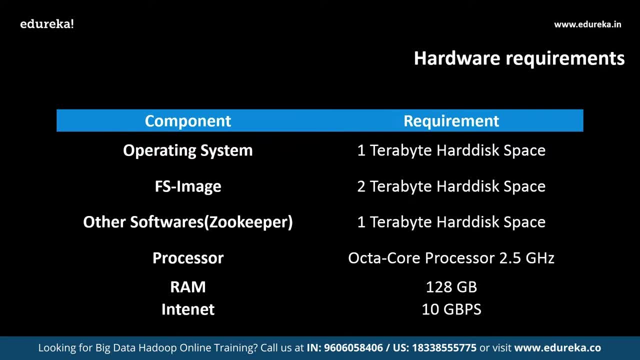 at least 128 GB capacity of RAM for an efficient and flawless performance. And finally, the major part, the internet. one should have at least 10 gbps speed internet to have an efficient workflow. So these were the requirements for name node, secondary name node and job tracker followed. 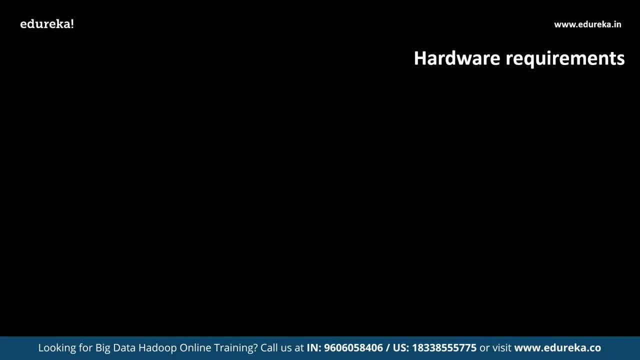 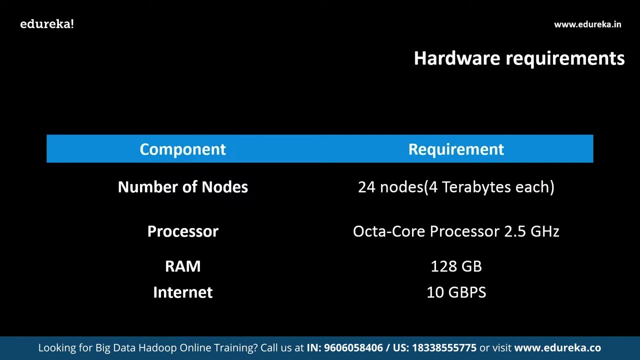 by the name node and job tracker. the next crucial components in a Hadoop cluster, where the actual data is stored and Hadoop jobs get executed, are the data nodes and task trackers respectively. Let us now discuss the hardware requirements for data node and task trackers. the number of nodes: 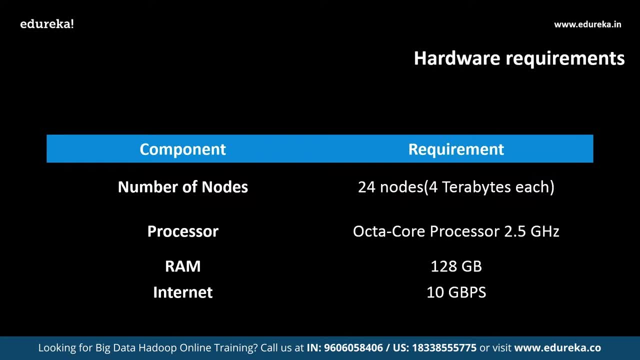 in a standard Hadoop cluster are 24 nodes, and each node should be having a capacity of 4 terabytes storage, followed by that, The next important requirement is the processor, similar to the name node. We also need a hexa-core or at least an octa-core processor of speeds 2. 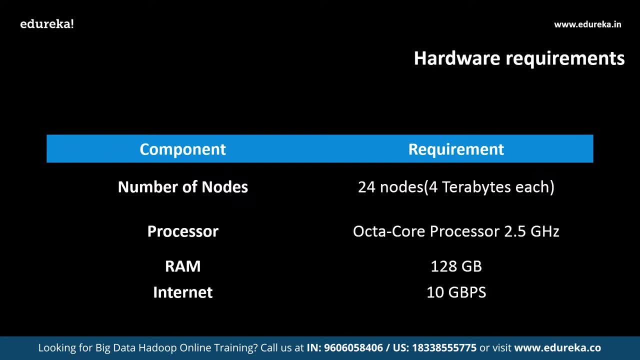 to 2.5 gigahertz, followed by that the Ram. we should have at least 128 GB of RAM and finally, the internet should be similar to the name node. that is 10 gbps. So these were the hardware requirements for the Hadoop cluster. 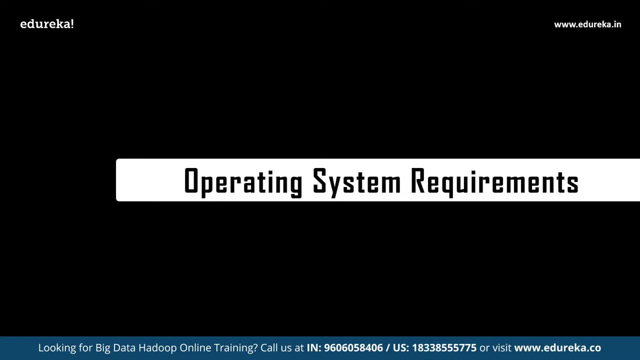 Now let us move ahead and understand the software requirements of the Hadoop cluster. when it comes to software, the operating system becomes the most important one. You can set up your Hadoop cluster Using the following operating systems of your choice: few of the most important. 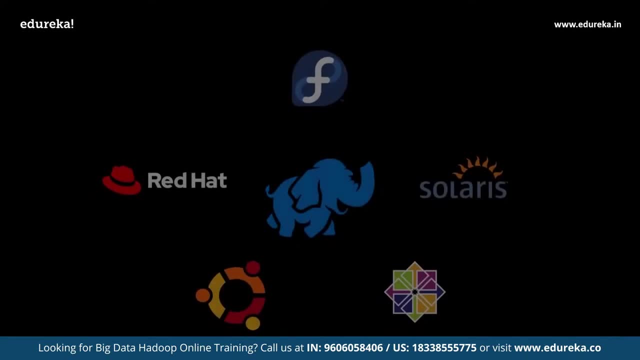 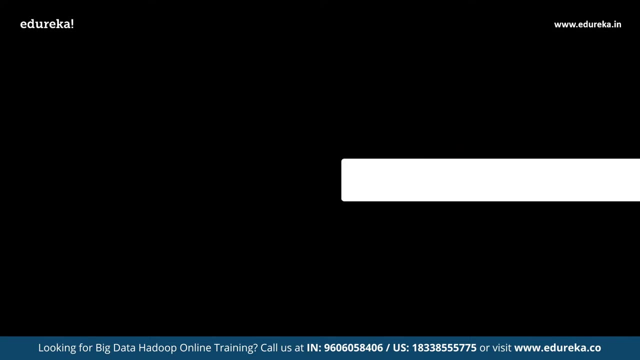 and recommended operating systems to set up a Hadoop cluster of Solaris, Ubuntu, Fedora, Red Hat and CentOS. now that we have understood the hardware and software requirements of our do classic capacity planning, We will now plan a sample Hadoop cluster for better understanding. the following problem is based: 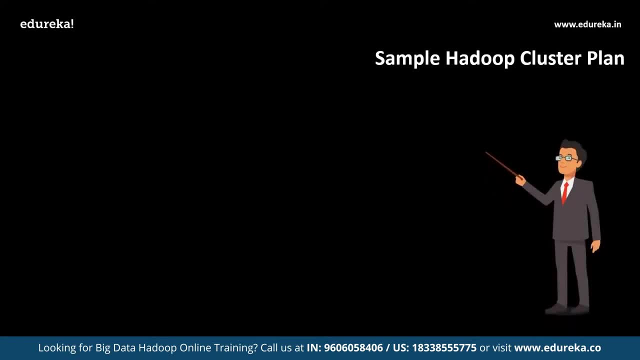 on the same. let us assume that we have to deal with minimum of 10 terabytes and assume that there is a gradual growth of data, say 25% every three months or every quarter of an year in future, assuming that the data grows per every year. 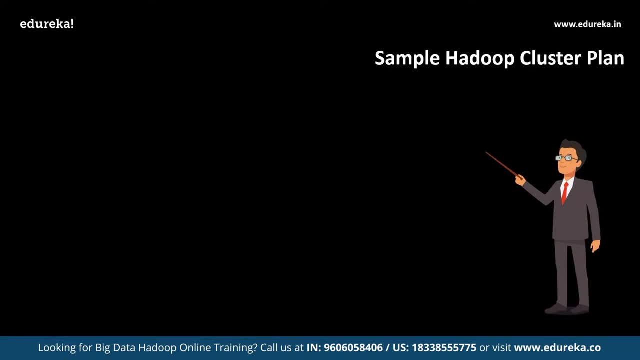 and the data in year one is 10,000 terabytes, by the end of five years, Let us assume that it may grow to 25,000 terabytes. If we assume 25% of year-by-year growth and 10,000 terabytes data per year, then in five years, 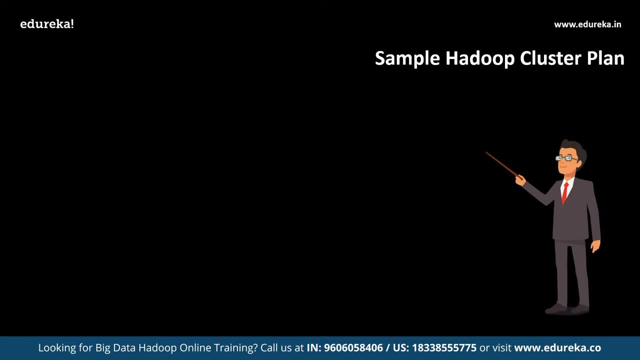 the resultant data may be nearly equals to one lakh terabytes. How exactly can we estimate the number of data notes that we might require to tackle this data? The answer is simple. using the formula which is mentioned here, Hadoop storage HS is equals to CRS divided by 1 minus I, where C is the compression ratio. 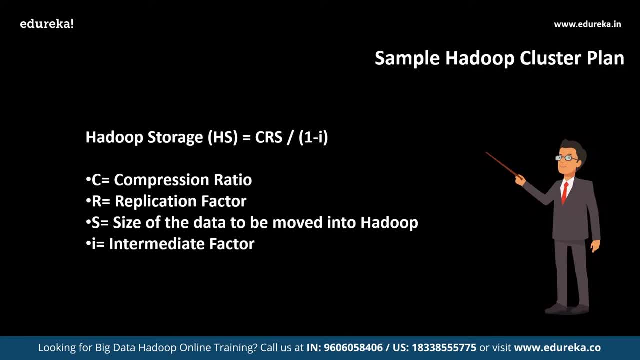 R is the replication factor, S is being the size of the data which is being moved into Hadoop, and I is the intermediate factor. Now let us calculate the number of notes required, assuming that we will not be using any sort of data compression here. 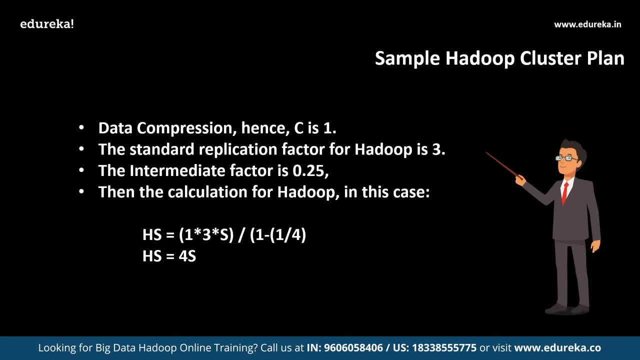 We shall keep C as a standard one, and we all know that the standard replication factor in Hadoop is 3, so R is equals to 3 and next the intermediate factor I is equals to 0.25.. Then the calculation for Hadoop in this case will result: 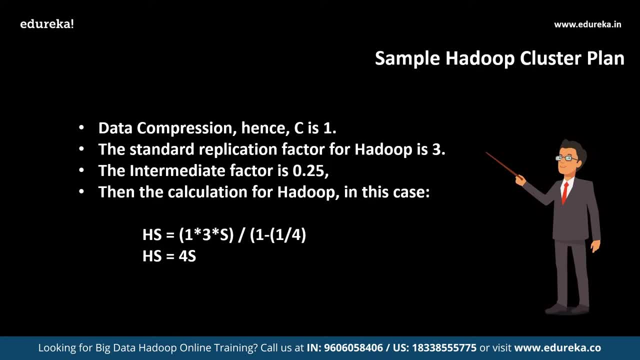 as follows: H s is equals to 1 into 3, into S whole, divided by 1. Minus 0.25, which will result in H is is equals to 4s. The expected Hadoop storage instance in this case is 4 times. 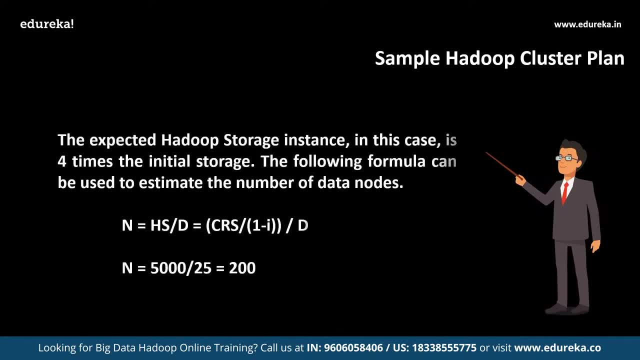 the initial storage. the following formula can be used to estimate the number of data notes, which is: n is equals to Hadoop storage divided by D, which in turn results as CRS divided by 1 minus I whole divided by D, where D is none other than the disk space available. 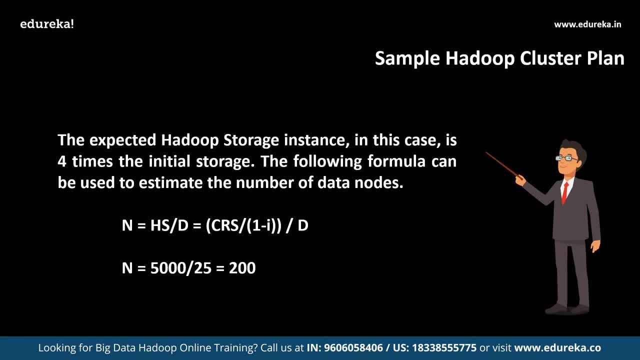 for each node. Let us assume that 25 terabytes is the available disk space for single note, each note comprising of 27 disks of 1 terabytes, each. here, 2 terabytes is dedicated to operating system. also, assuming the initial data to be 5000 terabytes and is equals to 5000 divided by 25. 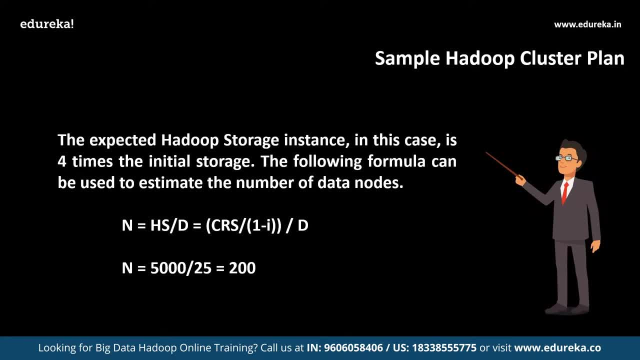 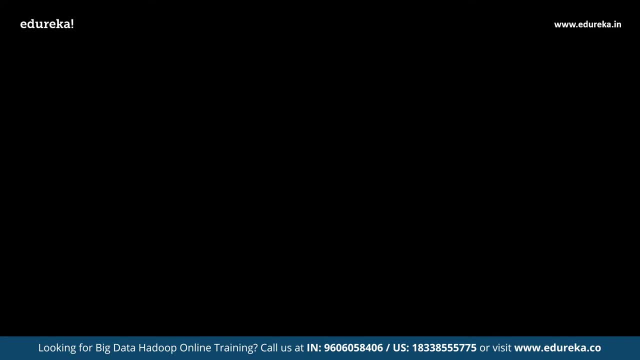 which results in 200. hence, we need 200 notes in this scenario. So that's how we plan a sample Hadoop cluster. Now that we have understood how to plan a sample Hadoop cluster, We shall move into the final topic for today's discussion. 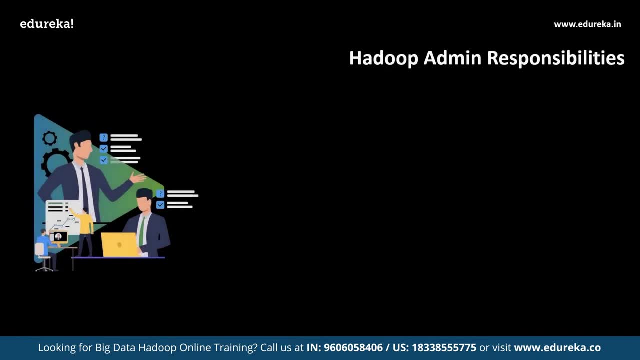 which is the Hadoop admin responsibilities. the Hadoop admin should be responsible for implementation and administration of Hadoop administration, followed by that he or she should be responsible for testing MapReduce, hive big, and should be having access for all the Hadoop applications. The third responsibility is the Hadoop admin should be taking. 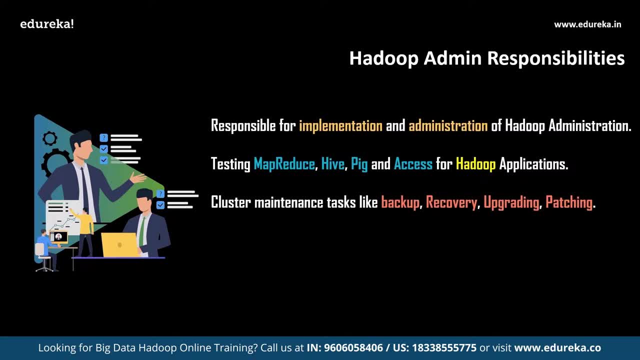 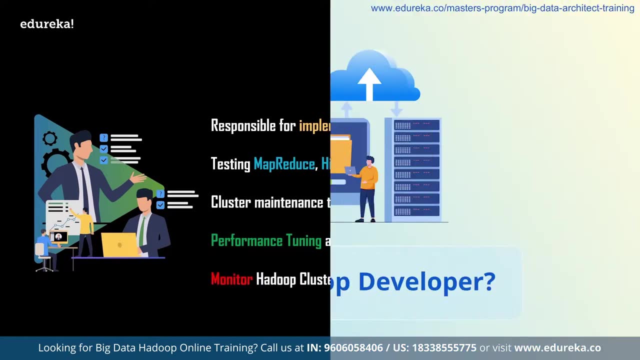 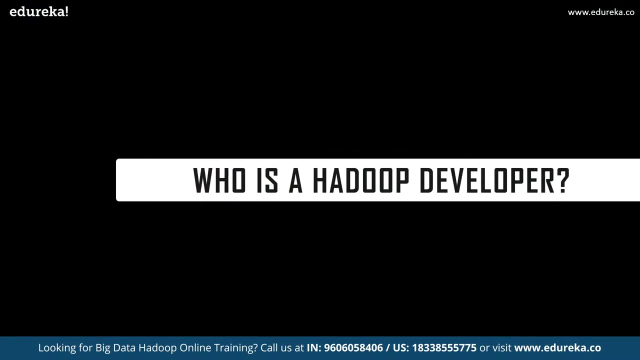 responsibility of cluster maintenance tasks like backup, recovery, upgrading and patching. the fourth responsibility is performance tuning and capacity planning for clusters. the last but the most important responsibility of a Hadoop admin is to monitor Hadoop cluster and deploy security. Who is a Hadoop developer? Hadoop developer is a professional. 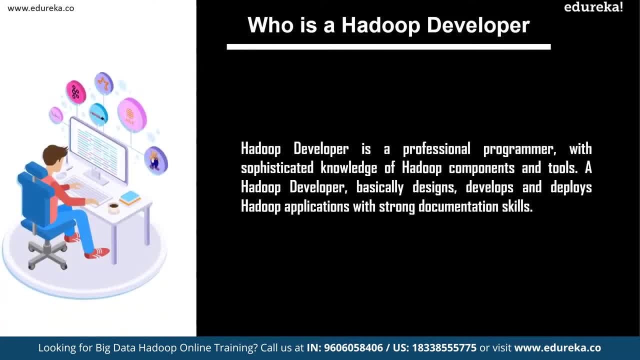 programmer with sophisticated knowledge of Hadoop components and tools. a Hadoop developer basically designs, develops and deploys Hadoop applications with strong documentation skills. So the basic definition of a Hadoop developer is as follows: a Hadoop developer is a professional programmer who has some sophisticated knowledge about Hadoop components. 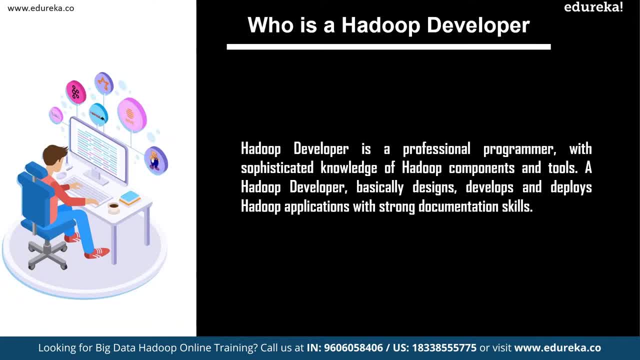 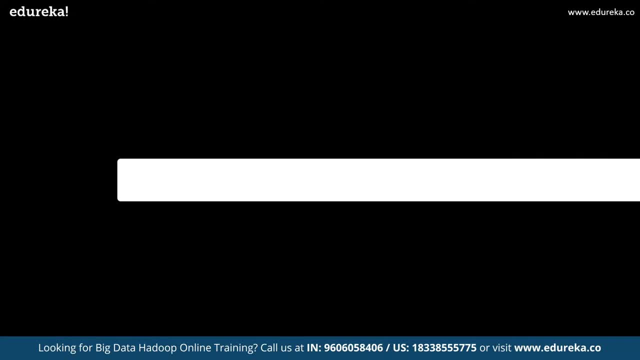 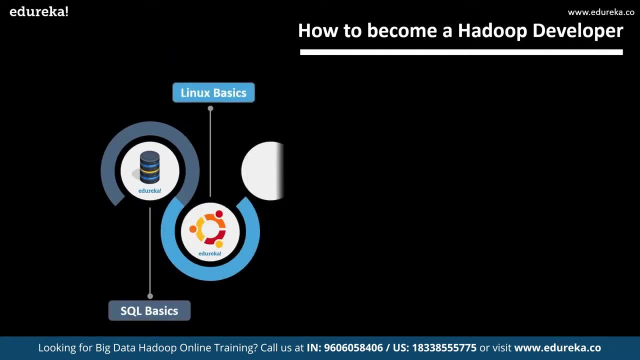 along with its tools. a Hadoop developer basically designs, develops and deploys Hadoop applications with strong documentation skills. Now let us move ahead and understand the roadmap to become a Hadoop developer. To become a Hadoop developer, This is the roadmap which you need to follow. firstly, 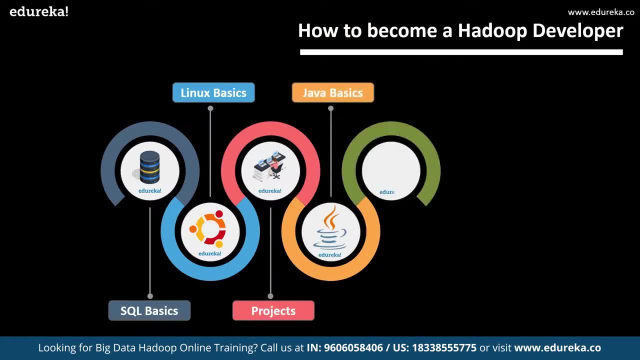 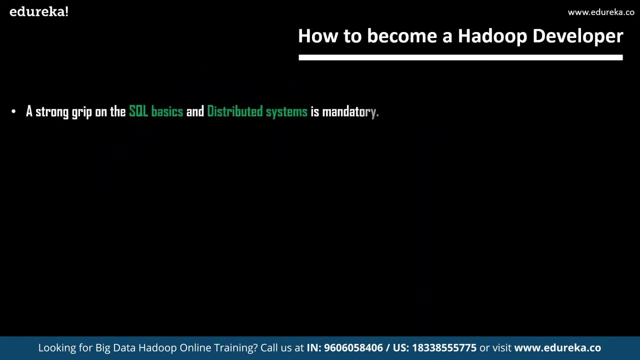 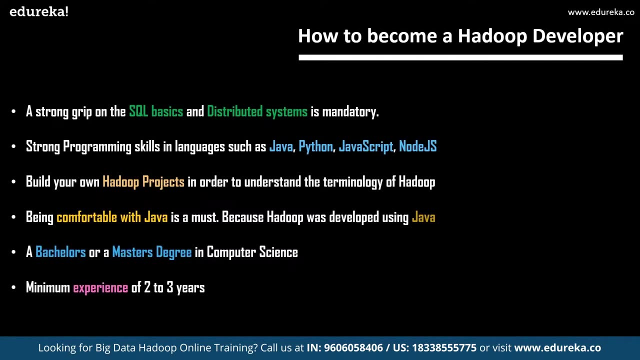 you need a strong grip on sequel basics and understand the terminology of distributed systems, which is mandatory. followed by that, the next important skill is that you need to be comfortable with Linux basics. You need to know the important commands and terminologies in Linux. then comes the next stage. 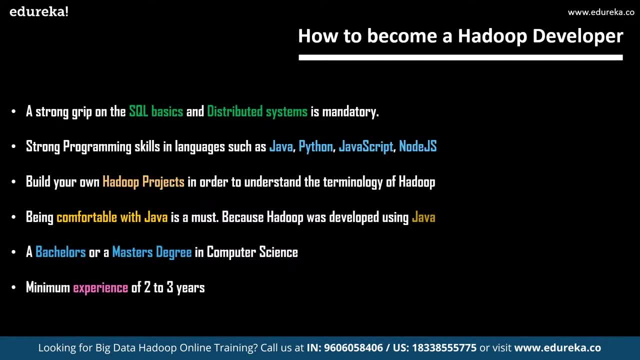 where you need to have strong programming sales in popular languages such as Java, Python, JavaScript, nodejs and many more. followed by that, you need to have your own Hadoop projects. in order to understand the terminology of Hadoop, then you need to be comfortable with Java. 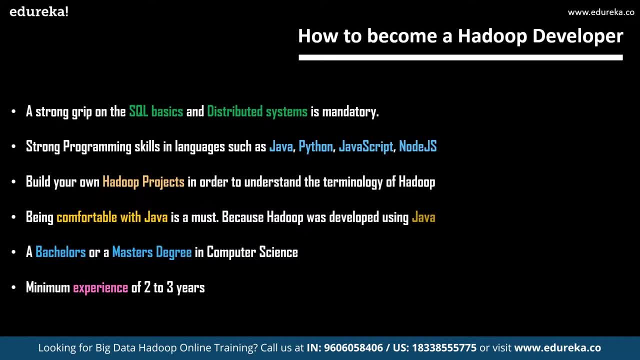 because Hadoop was developed using Java. and the most important thing is, you need to have a bachelor's or a master's degree in computer science and engineering technology And, finally, you need to have an experience of about two to three years. you might want to join some startup companies. 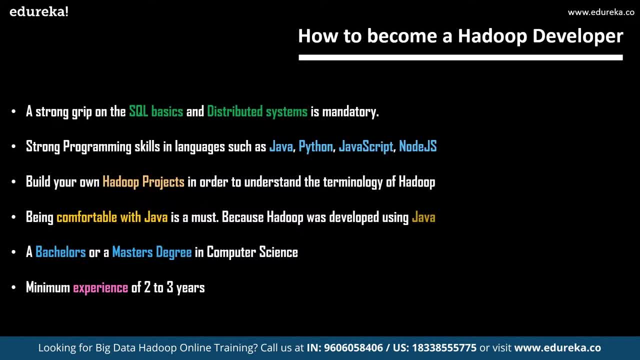 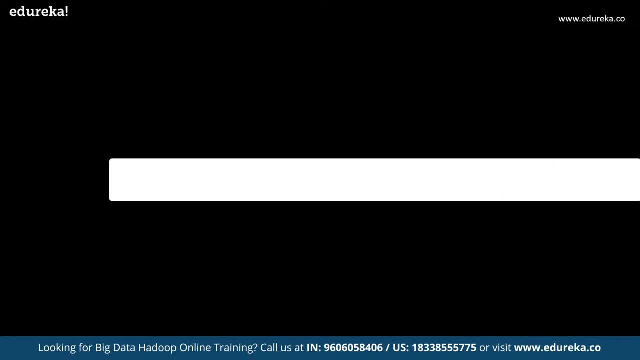 for experience, or you might also want to join some internships based on Hadoop. So this is the roadmap to become a successful Hadoop developer. Followed by this, we should discuss the skills that are required by a Hadoop developer. Hadoop development involves multiple Technologies and programming languages. 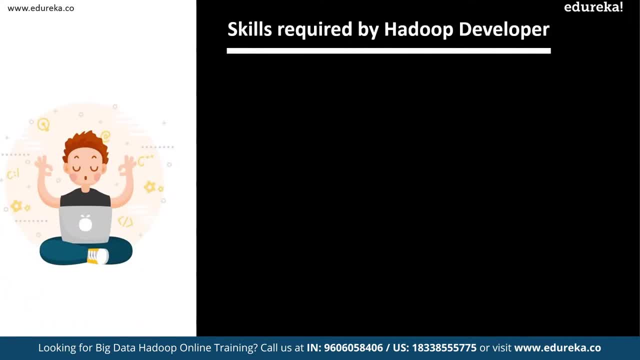 So the core and important skills to become a successful Hadoop developer are enlisted as follows. firstly, you need to have a basic knowledge of Hadoop and its ecosystem. later You should be able to work with Linux and execute some of the basic commands in Linux. followed, 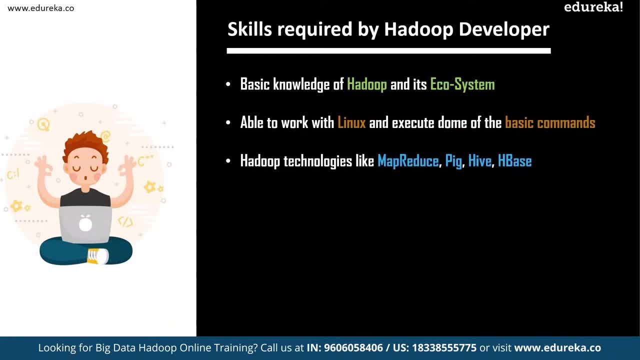 by that you are expected to have some hands-on experience with Hadoop core components. then Hadoop Technologies like MapReduce, big hive and HBase are mandatory. followed by that, you should be able to handle multi-threading and concurrency in ecosystem. Once you are familiar with that, your next stage is to work. 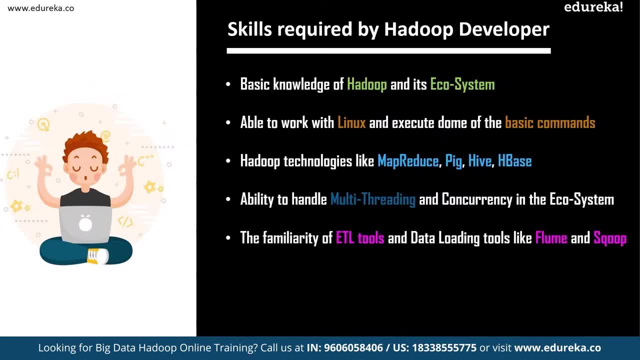 with the ETL tools. the familiarity with ETL tools, such as loading data and processing it using flu and scoop, is compulsory. followed by that, you should be able to work with them back in programming as well. Once you are done with that, you should be experienced. 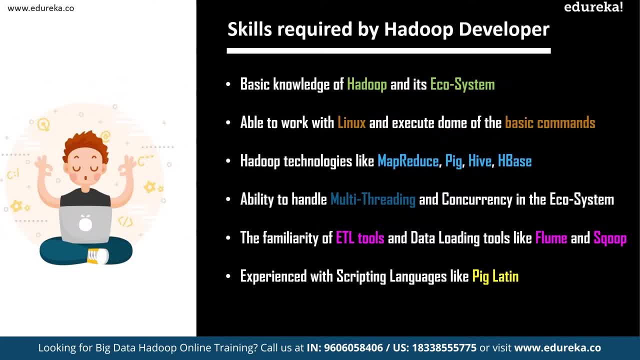 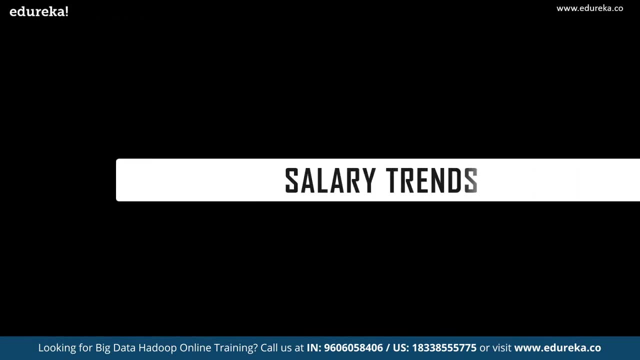 with some scripting languages such as big Latin, and after that you should be having a good knowledge of query languages like hiveQL. So these were the few important skills which you require to become a successful Hadoop developer. now let us move ahead and understand the salaries trends of Hadoop developer. Hadoop. 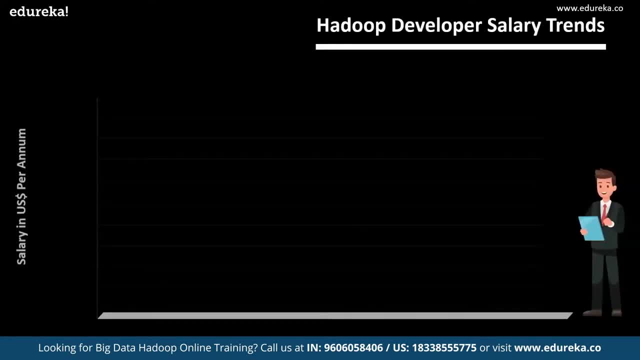 developer is one of the most highly rewarded profiles in the world of IT industry. salary estimations based on the most recent updates provided on media say the average salary of a Hadoop developer is more than any other professional. Let us discuss the salary trends of a Hadoop developer compared. 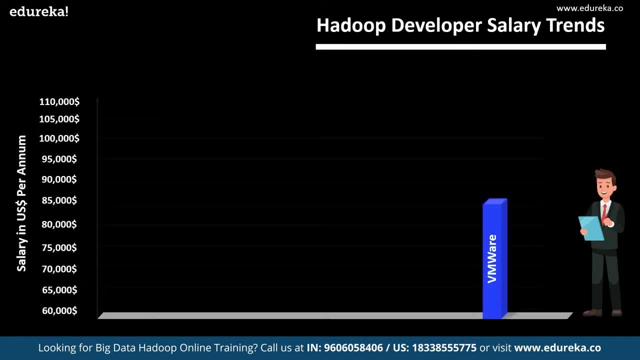 to other Technologies. firstly, VMware. you can see that the salary trends for a VMware professional lies between the $90,000 to $85,000, followed by that we have my sequel, So the mysql professionals also lie under the same segment. followed by that we have dotnet VB. 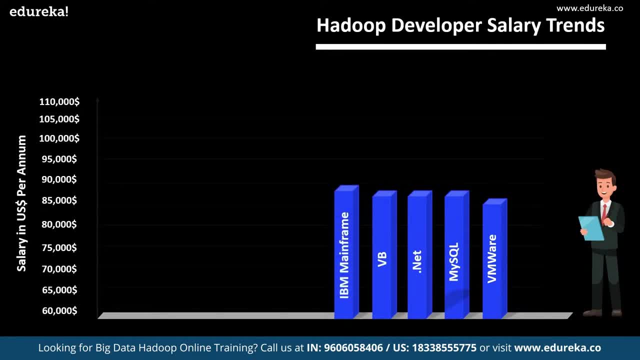 which is a visual Basics. then we have IBM mainframe developers. then, followed by that, we have C++ developers with an annual income of $90,000, followed by that We have JavaScript in the same segment, then SAP developers with a little hike, around $95,000 per annum. 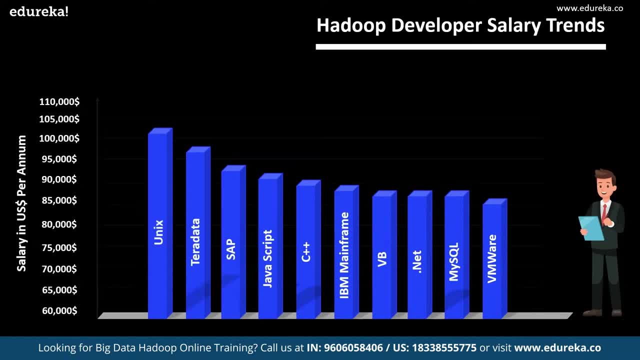 Then we have Teradata developers, Then we have the second highly paid Unix developers, which lie under the segment of hundred and five thousand dollars per annum, and finally you can see the Hadoop developers with the most highly paid profile, which lie under the segment of hundred and ten thousand dollars paid. 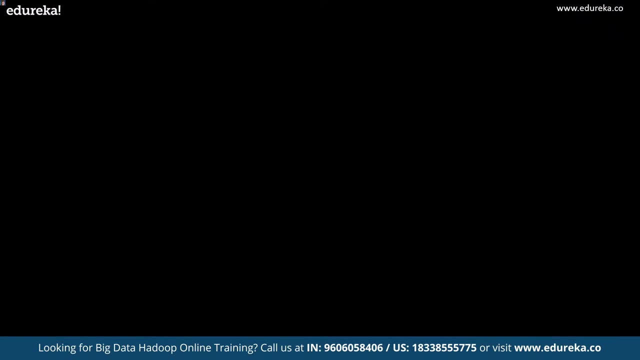 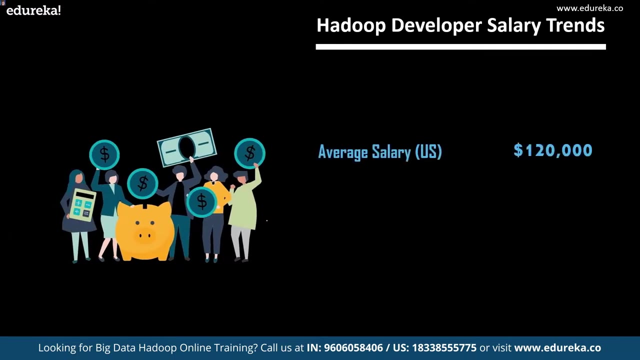 per annum. now, with this, let us move ahead and discuss the salary trends of Hadoop developer in different countries, based on their experience. Firstly, let us consider the United States of America. based on experience, You can see that the average salary of a Hadoop developer 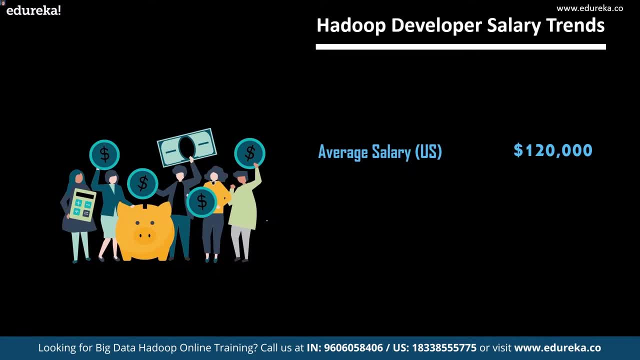 in United States of America with experience around 1 to 2 years, is around $120,000 per annum, followed by America. We have the average salary of a Hadoop developer in United Kingdom, which comes around 85,000 pounds per annum. 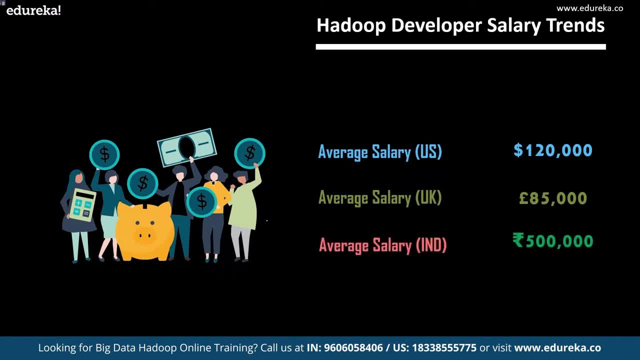 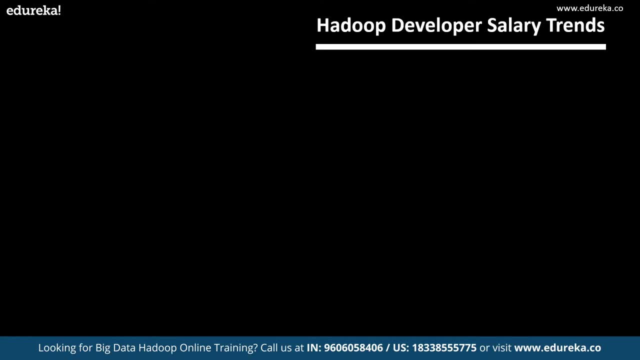 And finally, we have the average salary of a Hadoop developer in India, which is around 5 lakh rupees per annum. We should discuss the salary trends of Hadoop developers in a much detailed way. You can see that in America for an entry-level Hadoop developers. 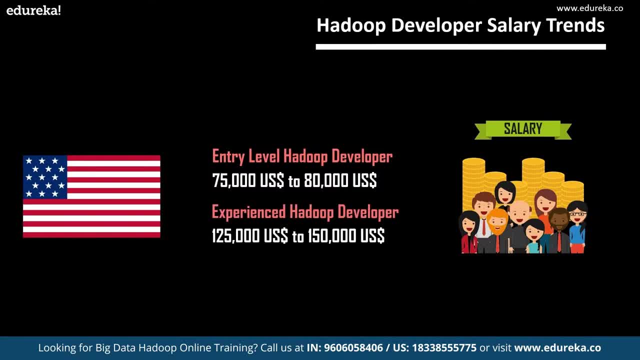 the salary begins from $75,000 to 80,000.. And you can see that for an experienced Hadoop developer, the salary Trends from 125,000 us Dollars to 150,000 us Dollars, now followed by the United States of America. 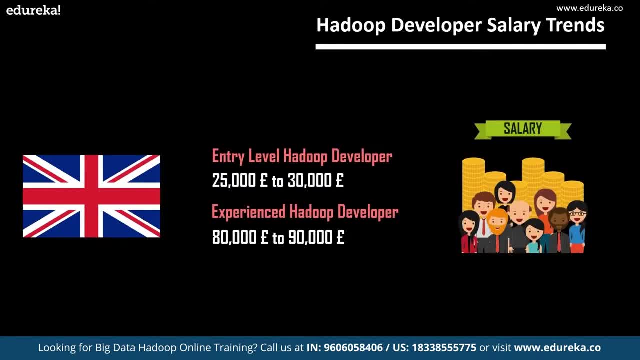 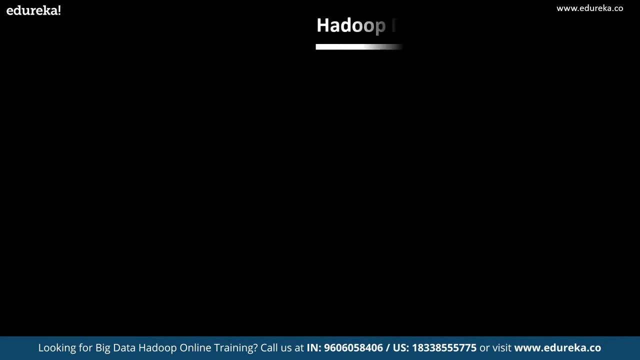 We have United Kingdom here. You can see that for an entry-level Hadoop developer, the salary starts from 25,000 pounds to 30,000 pounds, and whereas, on the other hand, for an experienced Hadoop developer, the salary Trends from 80,000 pounds to 90,000 pounds per annum. now in India. 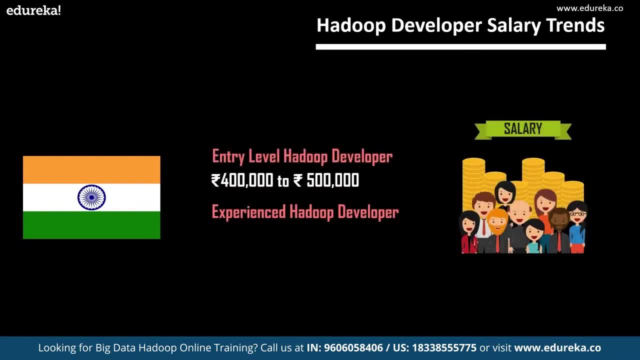 We have 4 lakh package to 5 lakh package for an entry-level Hadoop developer. on the other hand, for an experienced level Hadoop developer, the salary Trends from 45 lakhs to 50 lakhs per annum. Now we shall move ahead and discuss the job Trends for a Hadoop developer. You can see that, compared to other developers, Hadoop developers has seen a gradual growth in the rate of requirement. The number of Hadoop jobs has increased at a sharp rate from 2014 to 2019.. It has risen almost double in between April 2016 to April 2019: 50,000 vacancies related. 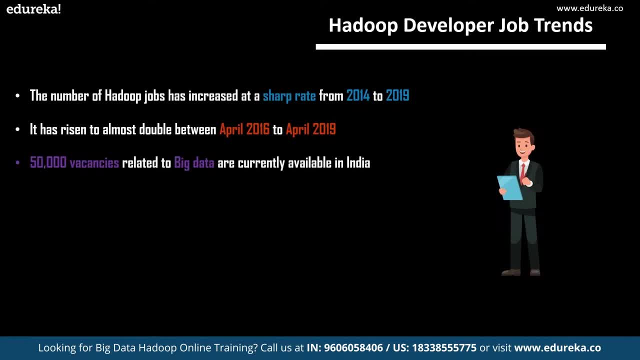 to big data are currently available in business sectors of India. India contributes to 12% of Hadoop developer jobs in the worldwide market. The number of offshore jobs in India is likely to increase at a rapid pace due to outsourcing almost all big MNC companies. 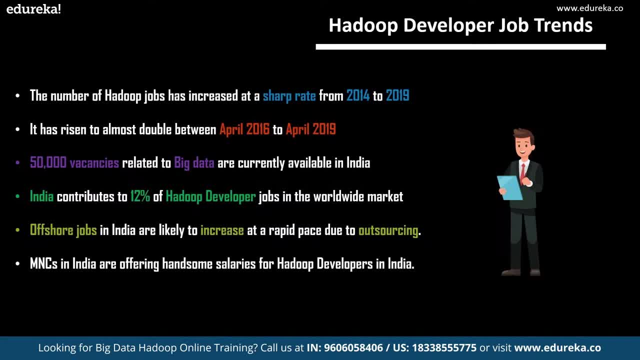 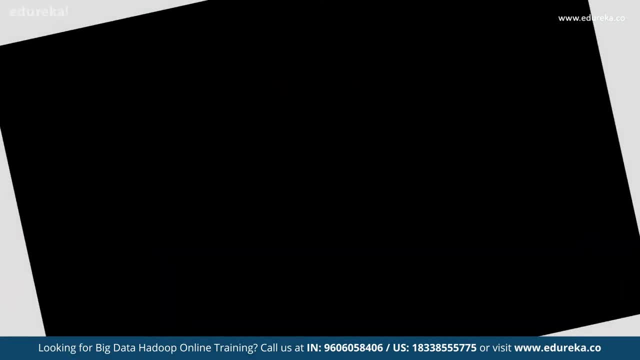 in India are offering handsome salaries for Hadoop developers. in India, 80% of Market employers are looking for big data experts from engineering and management domains. now, with this, let us move ahead and discuss about the top companies that are hiring Hadoop developers. The top companies which are hiring Hadoop developers are Oracle. 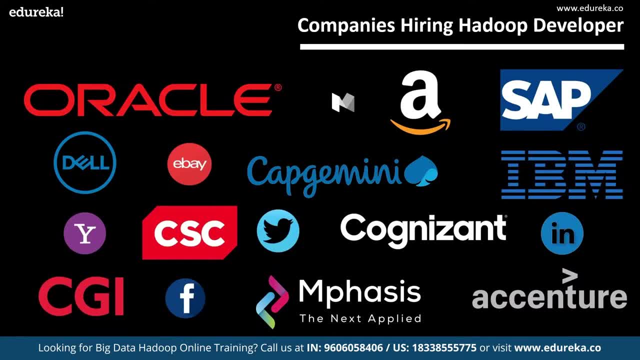 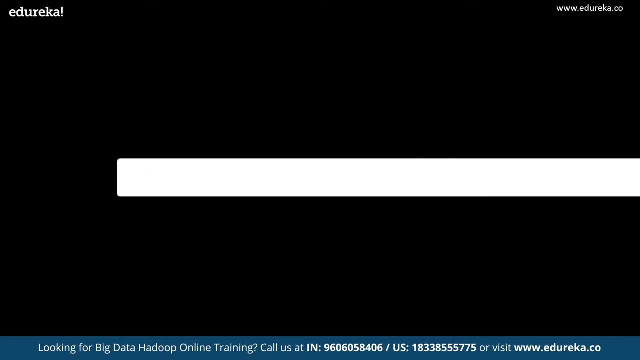 Dell, Capgemini, IBM, emphasis, CGI, Facebook, Twitter, LinkedIn, Yahoo, medium, Adobe, Infosys, cognizant, Accenture, Oracle, Dell, Amazon and many more. now Let us move ahead and understand the roles and responsibilities of a Hadoop developer. Different companies have different issues with their data. 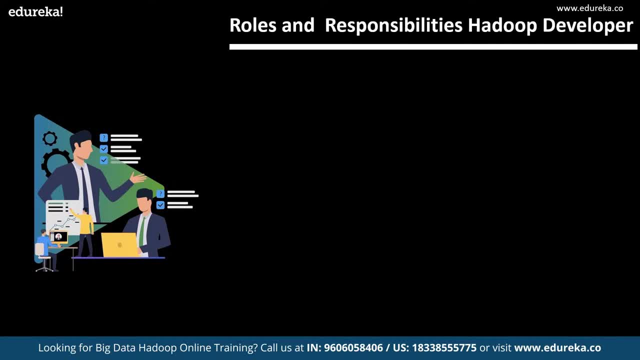 So the roles and responsibilities of the developers need to be a varied skill set to be capable enough to handle multiple situations with instantaneous solutions. Some of the major and general roles of a Hadoop developer are as follows. firstly, you should be capable enough to develop Hadoop. 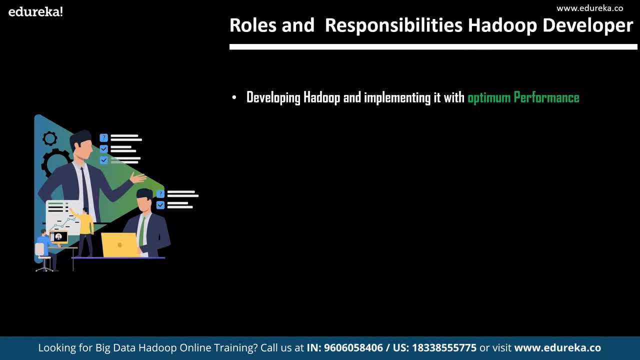 and implement it with optimum performance. followed by that, You should be able to load data from different data sources, which might be our DBMS, DBMS data warehouse and many more. followed by that, you should be capable enough to design, build, install, configure and support Hadoop system. followed by that. 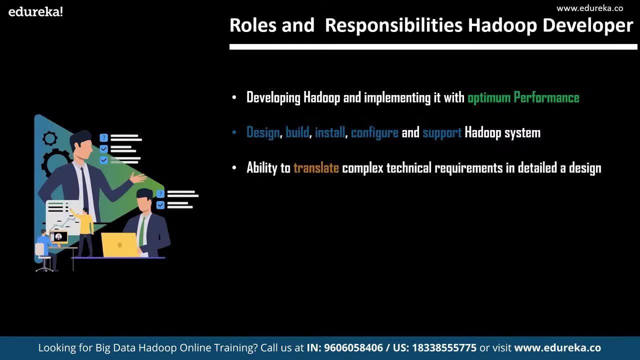 You should be able to translate complex technical requirements in a detailed design. You should be able to analyze vast data storages and uncover insights. You should be also able to maintain security and data privacy. you should be capable to design scalable and high-performance web services using data tracking high-speed. 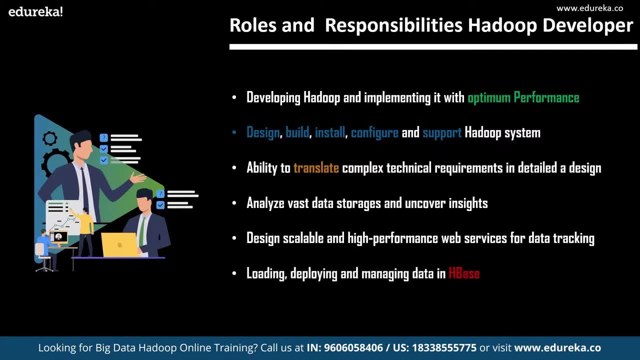 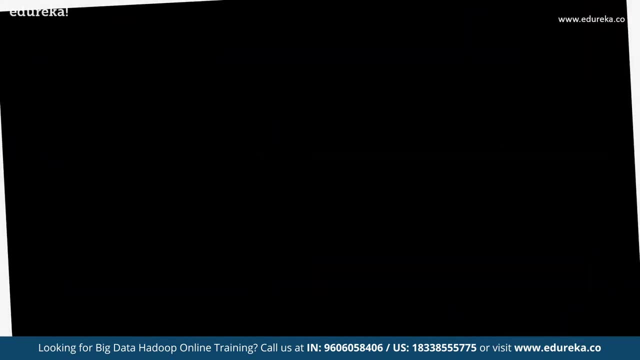 data querying is a must. you should also be able to load, deploy and manage data in edgebase. defining job flows using schedulers like zookeeper is mandatory and finally, cluster coordination services through zookeeper is also important. now with this, let us also discuss about the future. 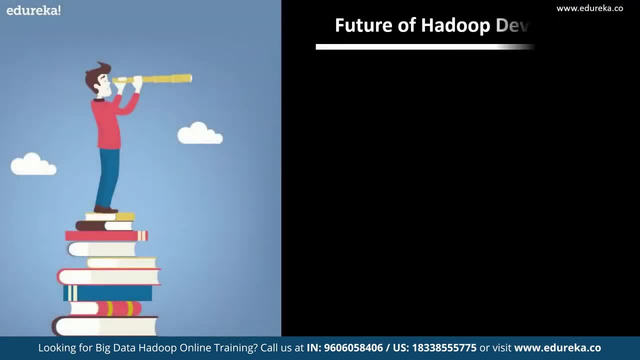 of Hadoop developers. major Large-scale enterprises need Hadoop for storing, processing and analyzing their big data. The amount of data is increasing exponentially, and so is the need for the software in the year 2018.. The global big data and business analytics market was standing 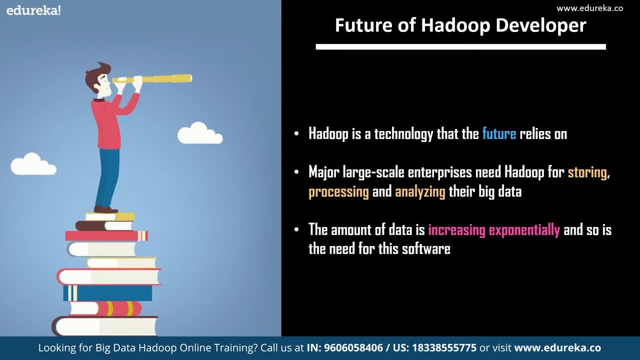 at 169 billion us Dollars and by 2022 it is predicted to grow to 274 billion us Dollars. However, a PwC report predicts that by 2020, there will be around 2.7. Million job postings in data science. 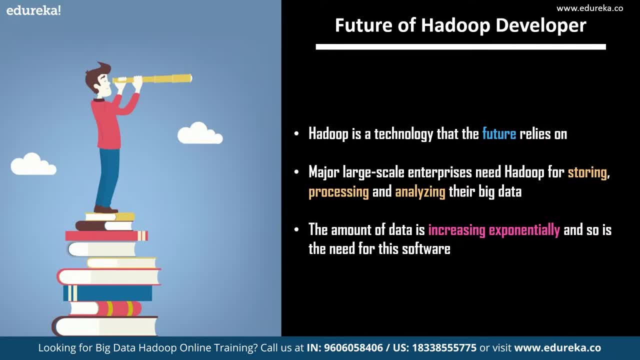 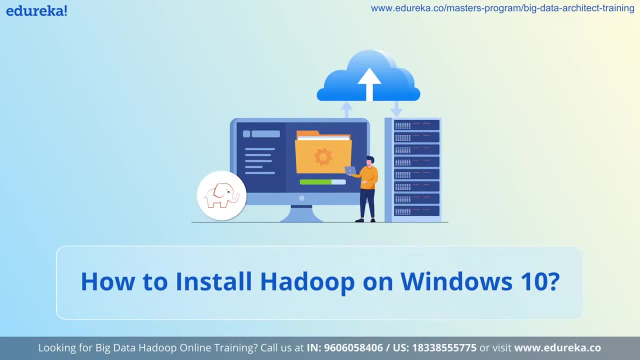 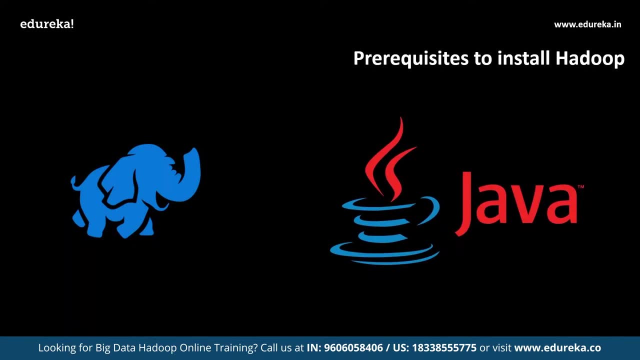 and analytics in the us Alone. if you're thinking to learn Hadoop, then it's the perfect time. The prerequisites to install Hadoop in Windows operating system are Java, So we all know that Hadoop supports only Java version 8.. 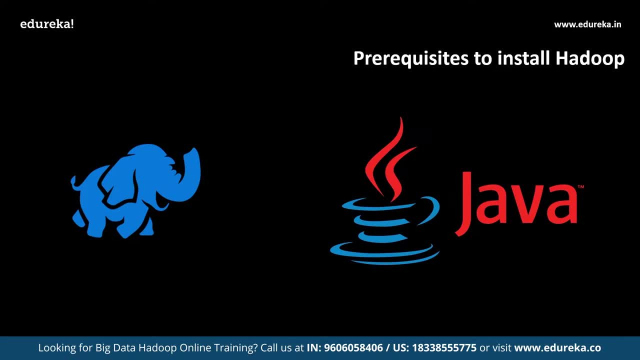 So firstly, we need to download Java 8 version, followed by that a latest Hadoop version, which we need for our operating system than the configuration files. So these were the prerequisites. now let's quickly go ahead and download Java 8 version into our local system, and also Hadoop. 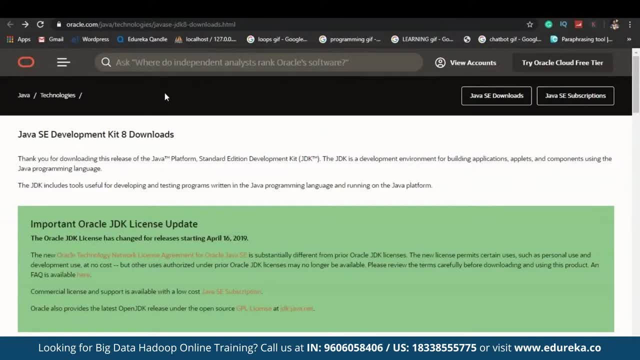 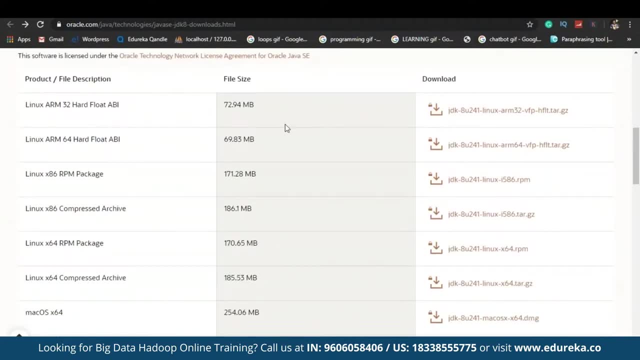 So you can see that this particular web page belongs to Oracle, and here you'll be getting your Java development kit number 8.. So these are the various versions available for Java 8, for Linux as well as Windows. So we need a JDK which is compatible with Windows. So here you can see that Windows x64 JDK version which will support Windows. So this particular link will redirect you and download JDK 8 for you into your local system. Once you click on it it will ask you to accept the license terms from Oracle. 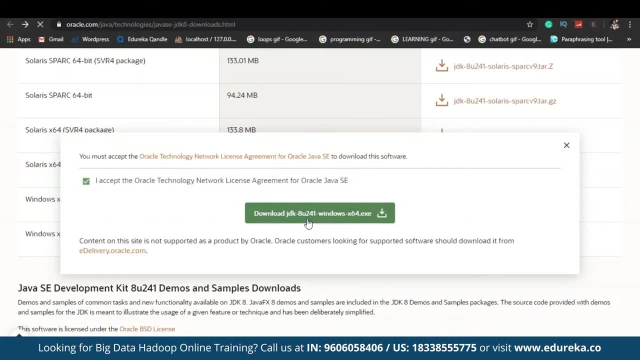 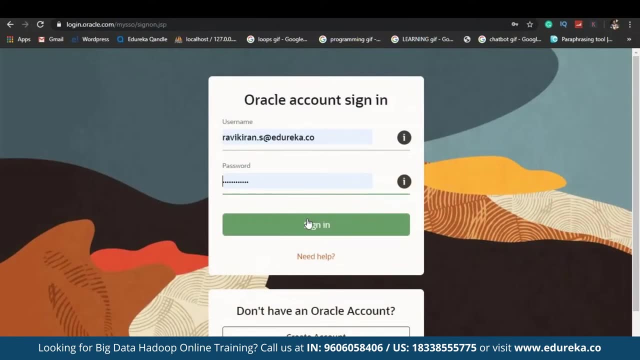 Now you can just click on download, followed by this. You will be redirected into a login page where you need to create your own account with Oracle so that you can download this JDK. Don't worry, This account is free of cost. So you can see the JDK is getting downloaded here. 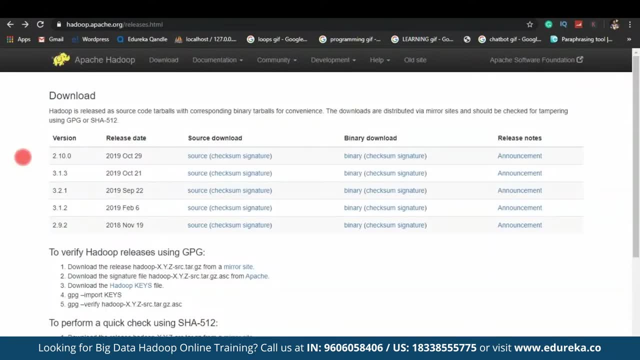 So as the JDK is getting downloaded, we shall now move ahead and download Hadoop for our local system. So this particular web page belongs to Apache organization, where we can download Hadoop for free. So these are the various versions available for Hadoop. 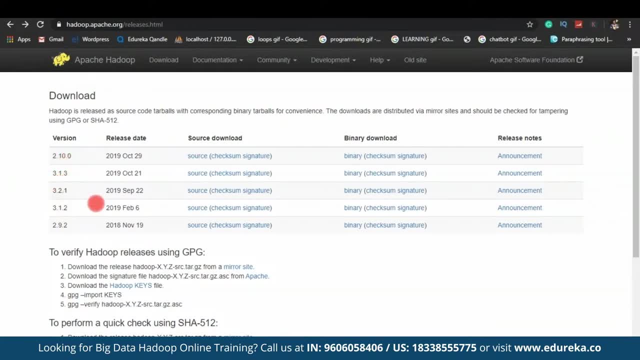 which are 2.10, 3.1.3, 3.2.1 and many more. So we shall select the latest version of Hadoop, But while you're selecting the latest version of Hadoop, please make sure that you're not actually downloading. 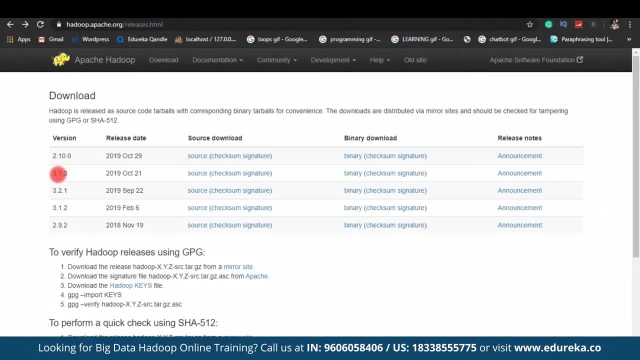 the exact latest version of Hadoop. here You can see we have three different versions: 3.1.3, 3.2.1, 3.1.2. as you can see, 3.2.1 is the latest version. We have to select the version which is earlier to it. 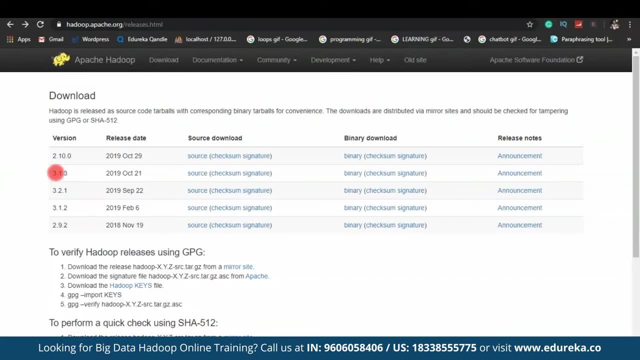 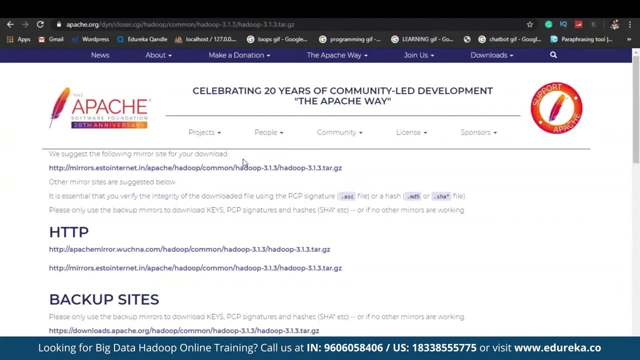 which is 3.1.3, because this particular version will be the stable version. now we shall move ahead and select binary. Once you select binary, you will be redirected into a new web page where you will have a mirror link. select that mirror link. and your Hadoop will be downloaded for your local system. As you can see, Hadoop 3.1.3 targz is getting downloaded Now. here you can see I have successfully downloaded Hadoop version 3.1.3 tar file, as well as JTK 8. 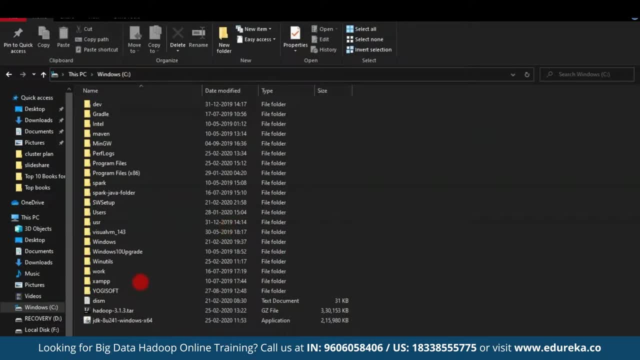 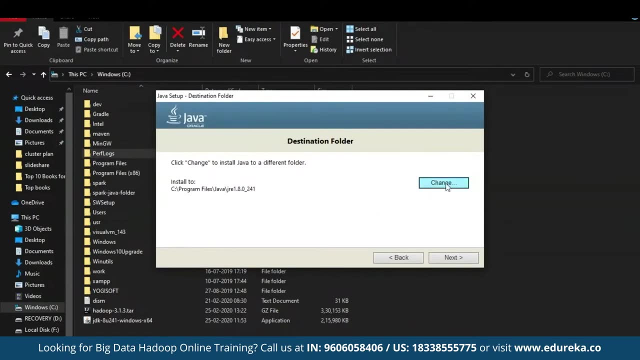 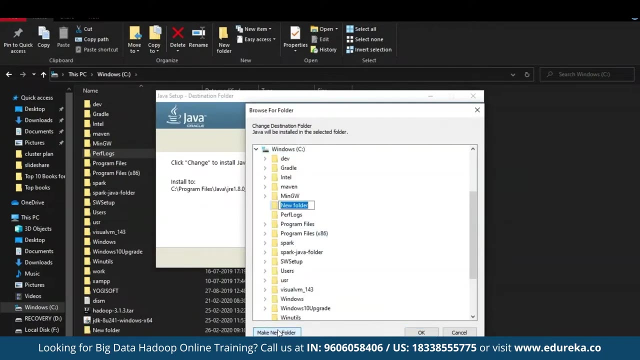 and those two files are successfully moved into my C drive. Now let's install Java first. now make sure you that you create a new folder for Java. So select change and here select Windows C drive, then select make new folder. now rename this new folder as Java click. 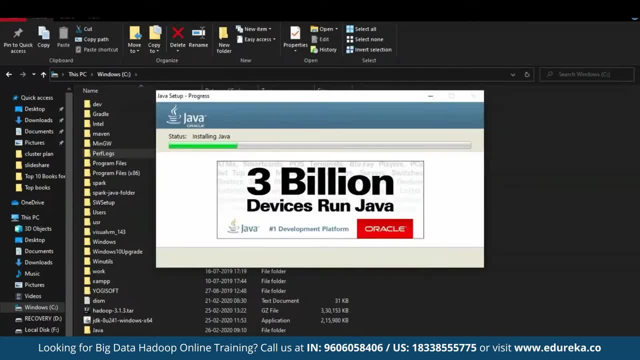 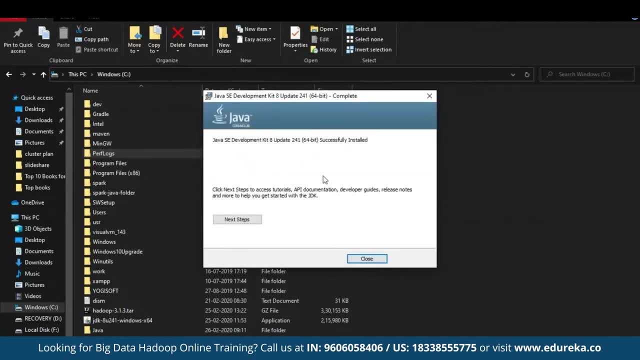 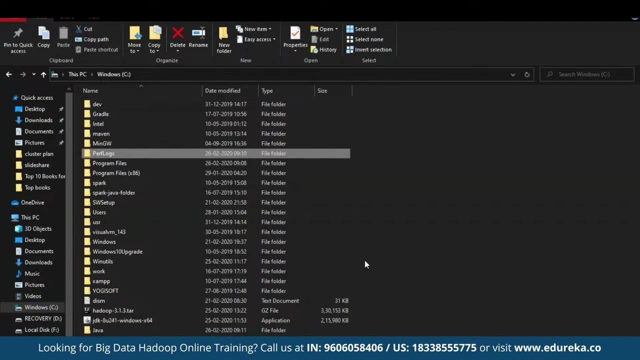 Okay, and now select next. you can see the installation procedure has now been started. You can see Java development kit. It has been successfully installed. now we shall enter into program files and move our JDK Into Java file, because sometimes there will be an error. 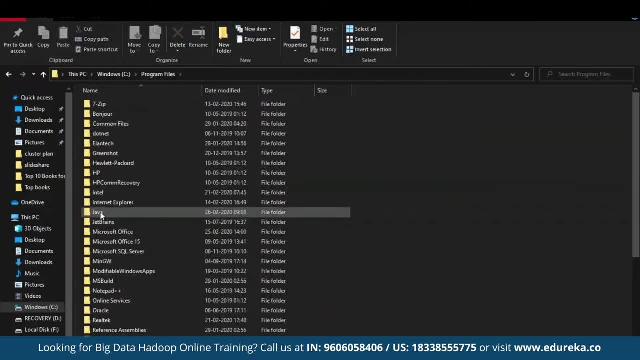 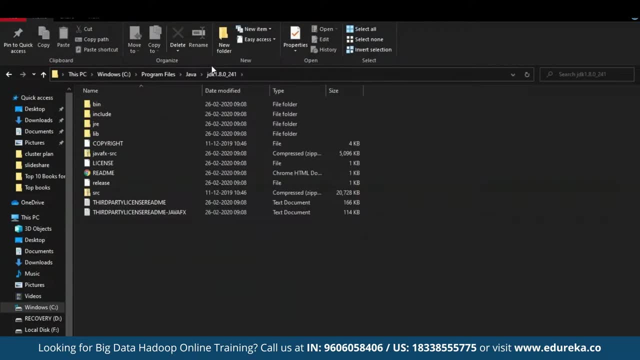 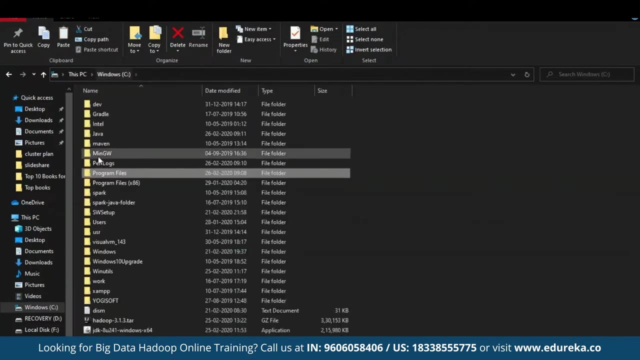 while we set environment variables for Java. So you can see, inside program files We have another folder called Java. So inside Java, there you have our JDK. So now what I'll be doing is just moving this JDK into Java file which we have created in C drive- this one. 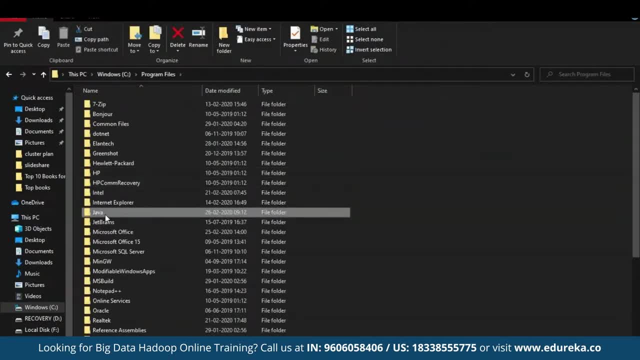 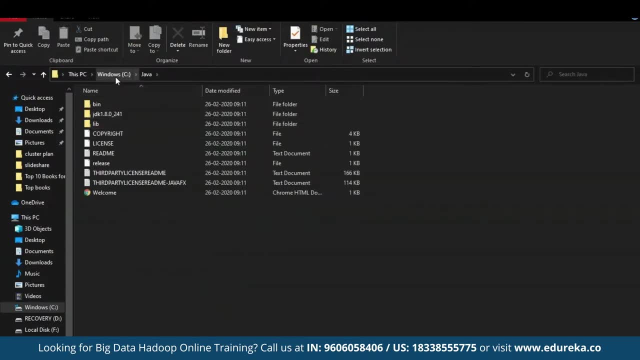 Now you can just delete this Java file from your program files, So that you don't have to mess with duplication of Java file. Now you have your Java and JDK in one single file, which is Java, that is, you have created in Windows C drive. 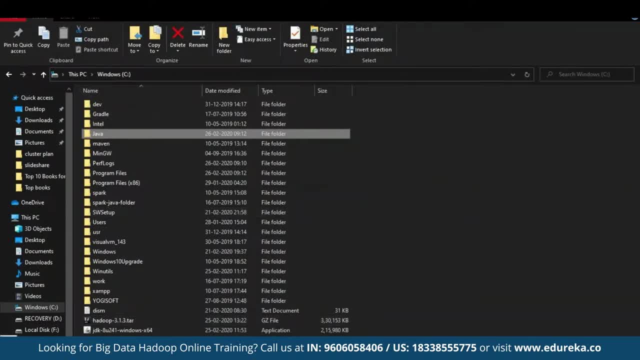 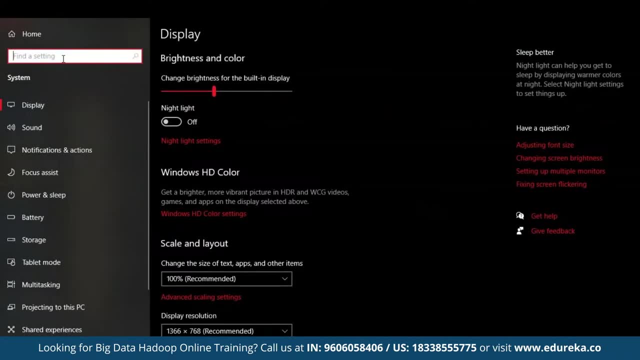 Now we shall move ahead and set the environment variables for Java. So click Windows and then enter into settings and inside the settings select system and inside system, just type in environment variables and there you go, select the, edit the system environment variables option And you have this dialog box here: select environment variables. 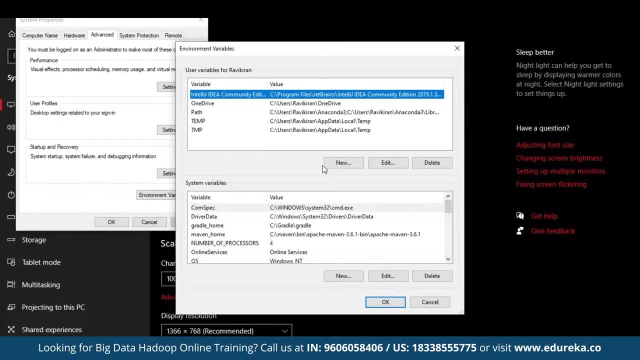 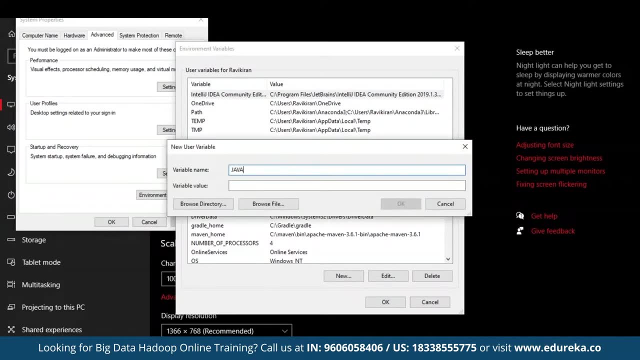 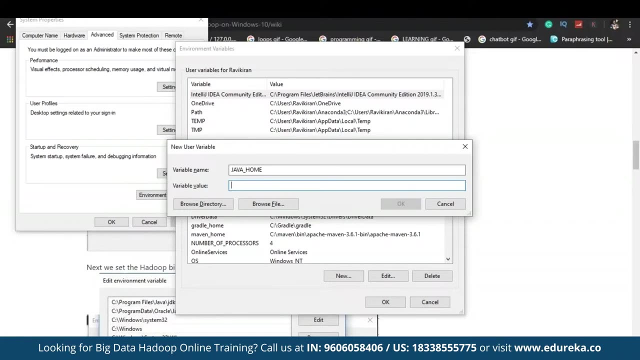 and inside the environment variables, You need to set the Java home as well as path for Java. now select new and here just type in Java home and here let us add the location of JDK bin. So here we will add in the variable value That is the JDK bin location. 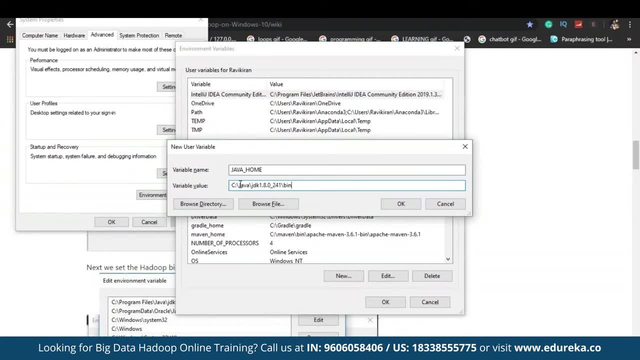 So our JDK bin location is in the C drive, and inside the C drive We have the Java folder, And inside Java folder We have a JDK 1.8.0 and inside JDK file We have the bin location. So this will be the home location for Java select. 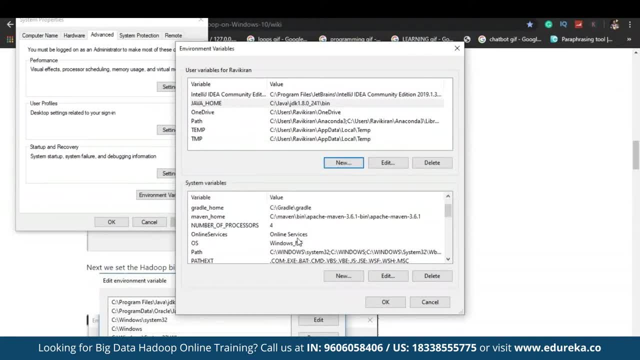 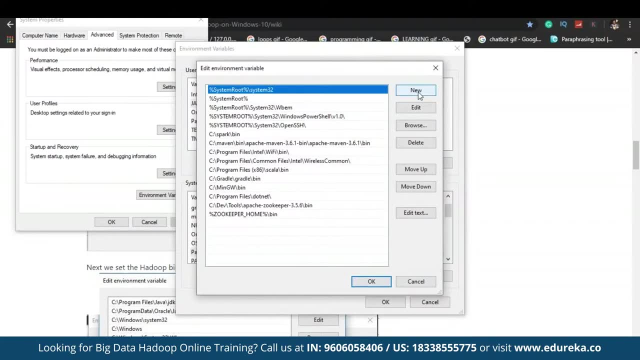 Okay, and then now move into the next dialog box, which is the system variables, and inside that select path and select edit. here create a new path variable which will be the JDK path, the same location, that is the bin of JDK select. Okay. 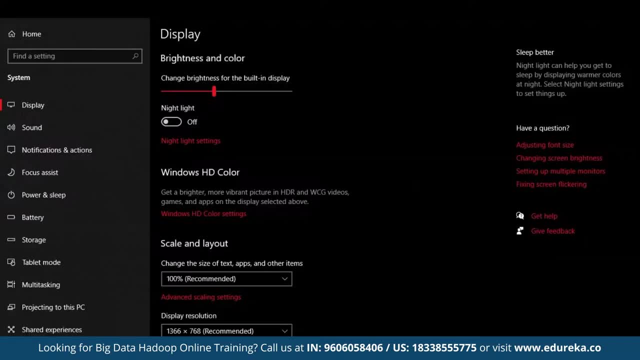 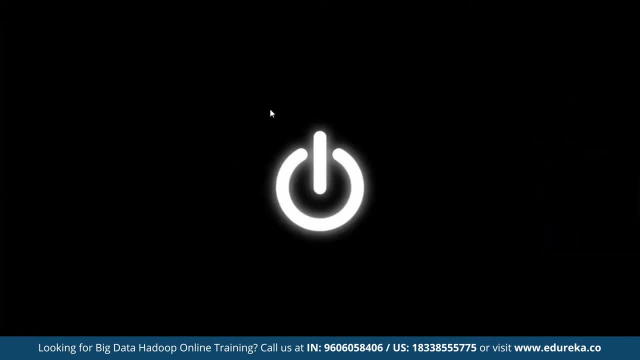 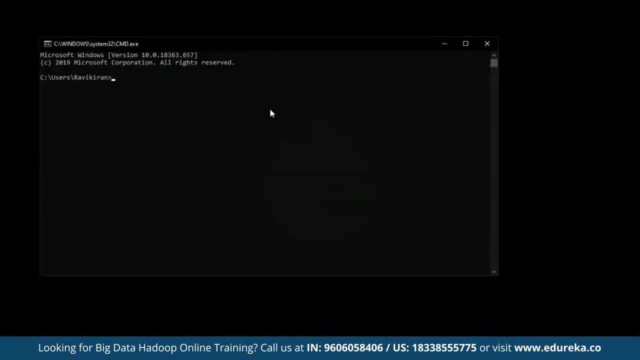 And now select okay again and now okay and close it. Now Java has been successfully installed into our local system. Now let's check Java is functional or not. We can do that by selecting Windows R and inside Windows R just type in cmd so that you can open your command prompt here. 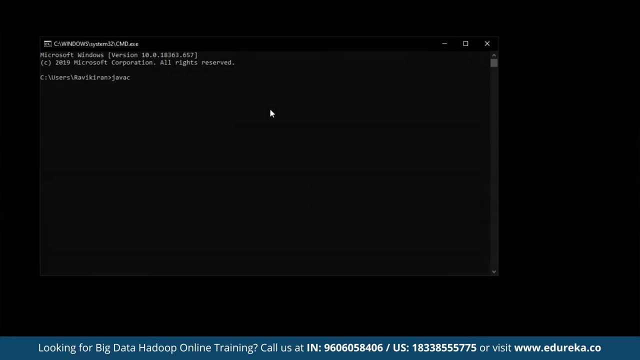 Just type in Java, see. if you see the set of files popping up into your terminal, then it means that Java is working properly. So you can see Java Is working just fine. Now let us check the version of our Java installed into our local system. 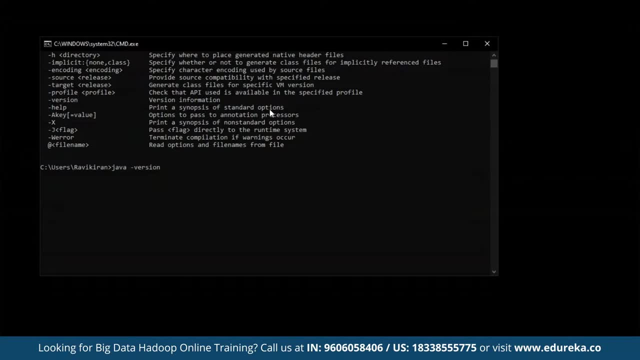 So this can be checked by typing in Java space hyphen version. So you can see we have 1.8 version which is running in our local system. Now that we have successfully installed Java into our local system, Let us now move ahead and install Hadoop into a local system. 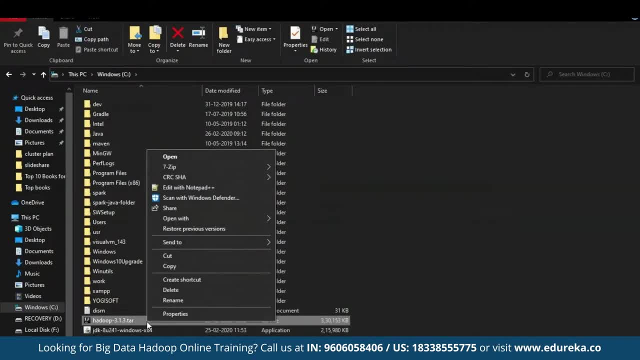 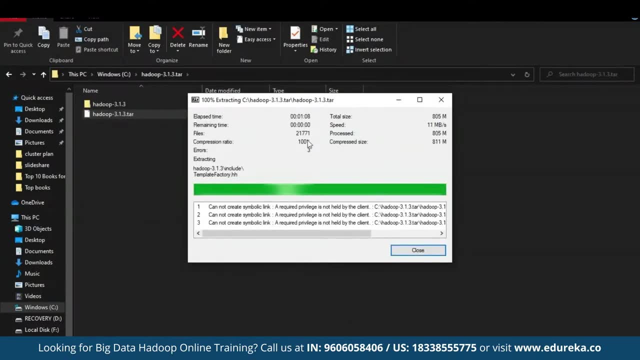 You can see that we have downloaded the tar version of Hadoop, So for that we need to extract it first. Now you can see that the process of extraction has been completely finished. that is hundred person, but you have three errors. You can ignore these errors. 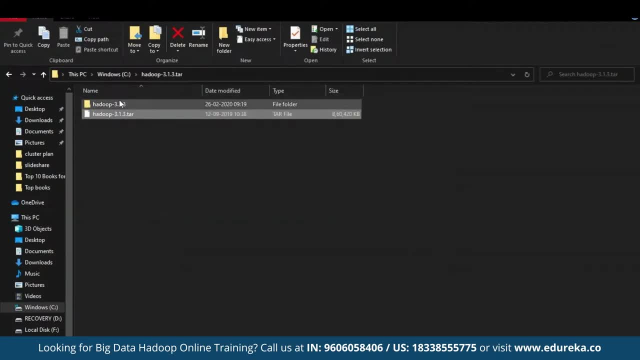 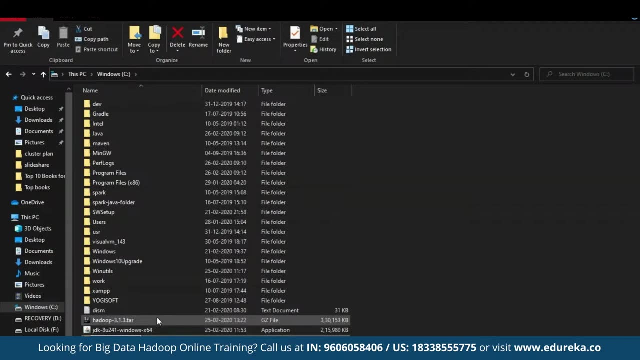 Now just close the extracting process. Then you have your Hadoop file. Now let us rename our Hadoop 3.1.3 as just Hadoop, to reduce the confusion. Now that we have successfully extracted Hadoop, Let's set environment variables for Hadoop. 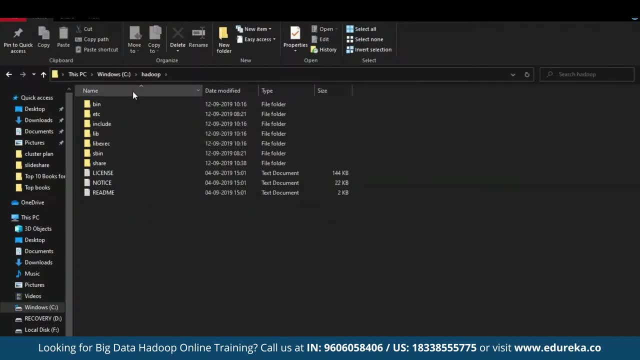 But before that let's set the configuration of Hadoop. You can select Hadoop and inside that you have a file called ATC. and inside ATC You have another folder with the name Hadoop and inside that you have a set of folders. 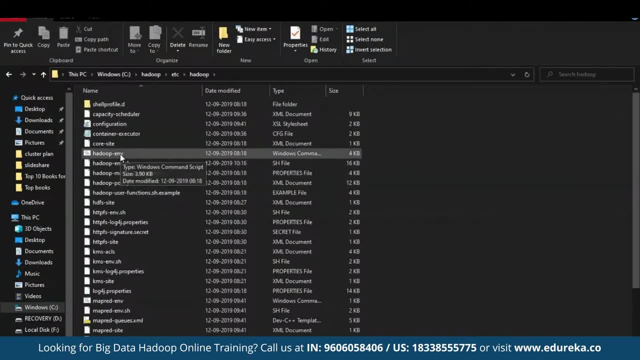 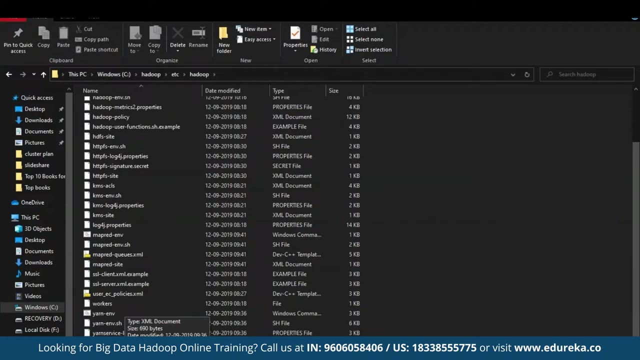 So, out of these all folders, we have four important folders. They are core site dot XML, then HDFS site dot XML, followed by HDFS. We have another one which is mapped site dot XML and last one, We have, quickly, the yarn site dot XML file. 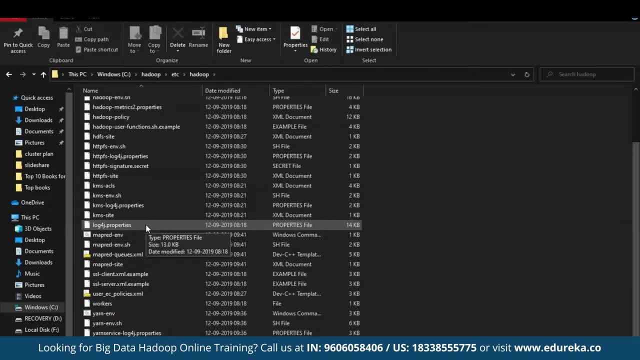 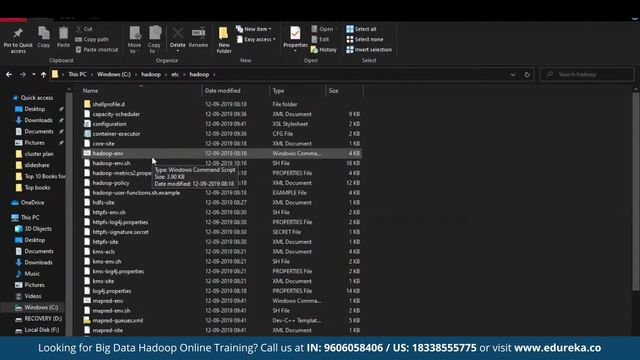 So we need to edit all these four different files, and once after we edit these four files, we need to edit one last file, which is the Hadoop ENV Windows command prompt file. So here you're just going to add in the Java home location. 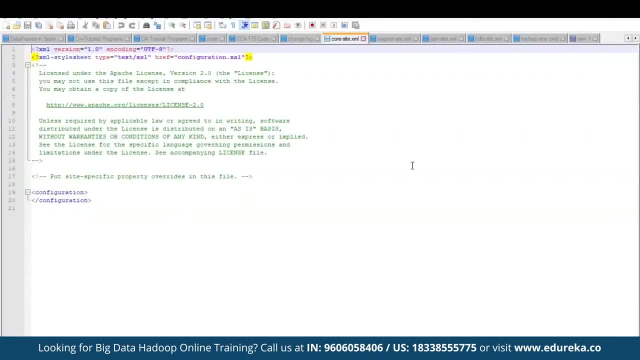 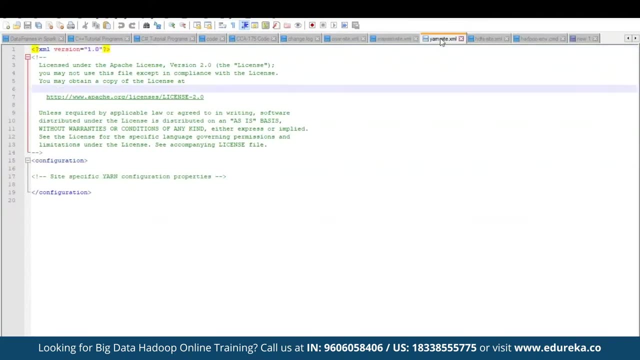 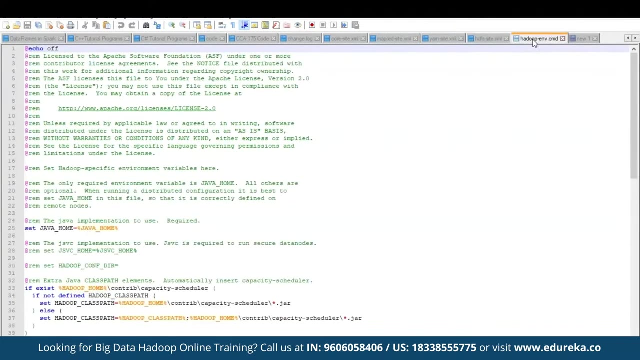 Now let's quickly edit all those four files. So we have successfully opened our four important files, which are: core site dot XML, map, reduce site dot XML, yarn site dot XML, HDFS site dot XML, followed by the four important files, the last file, which is the Hadoop environment dot cmd file here 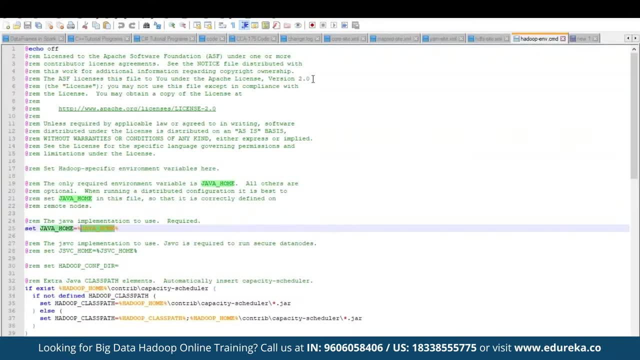 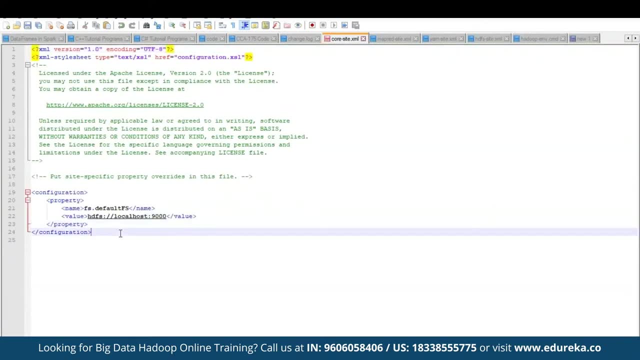 We are going to set this Java home location. Now let's first set the values for core site dot XML. So the values that are changed in cosine dot XML are the properties. So inside the configuration I have added one property, which is the file location, that is FS dot default file system. 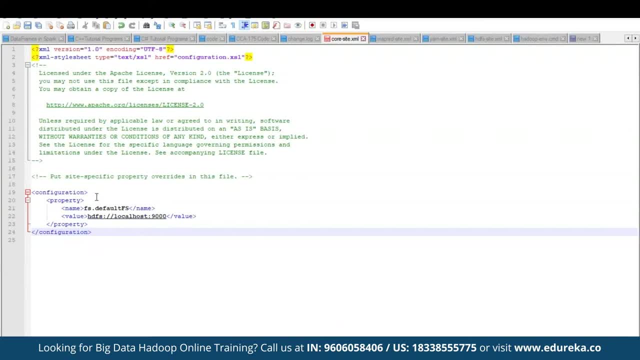 and the local host location, that is 9000. now let us save this core site dot XML. Similarly, We need to also edit MapReduce site dot XML files. here inside this, we need to add some properties. as you can see, We have also edited the configuration files. 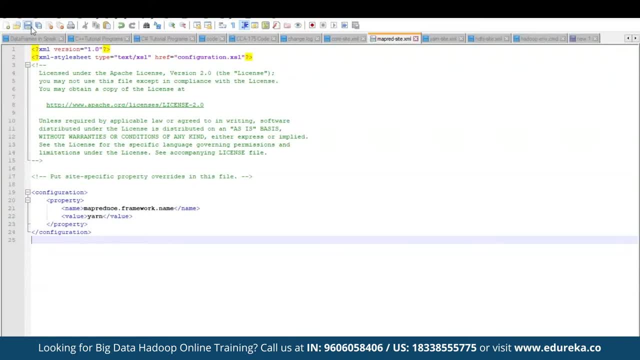 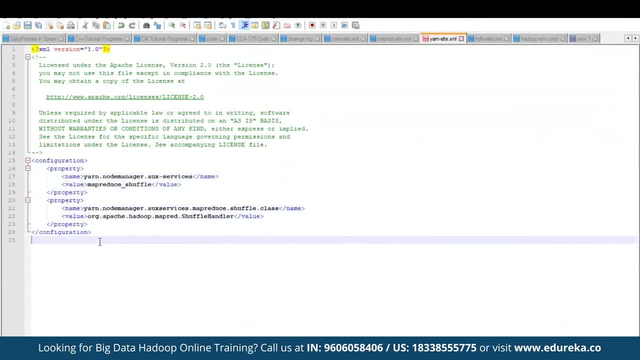 of MapReduce site dot XML. Let's save it now, followed by the MapReduce site dot XML. We have yarn site dot XML. Let's edit this also. As you can see, the yarn site dot XML is also being updated. No worry about it. 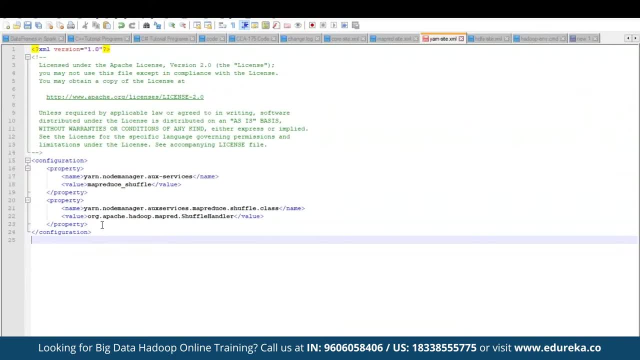 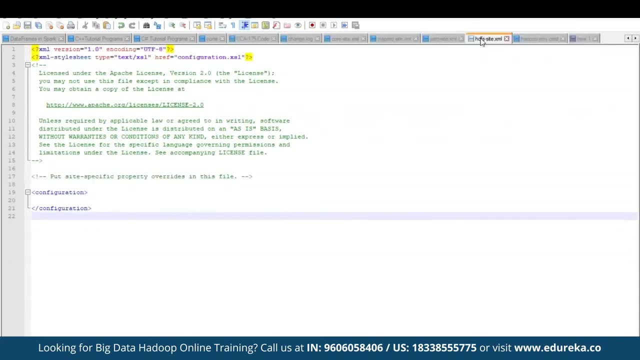 This property file. I will link this in the description box below. you can have the access to it and you can use the same configuration file and install Hadoop, followed by yarn- site dot XML. We have the last one, which is HDFS- site dot XML. 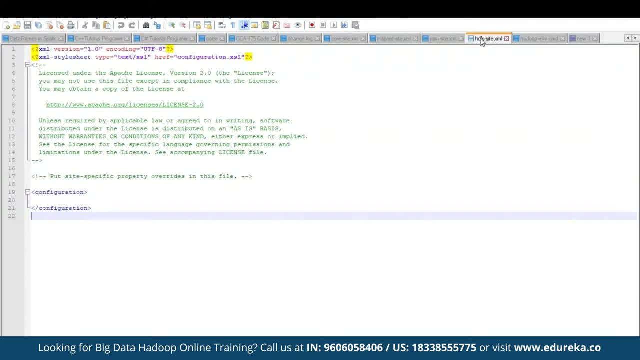 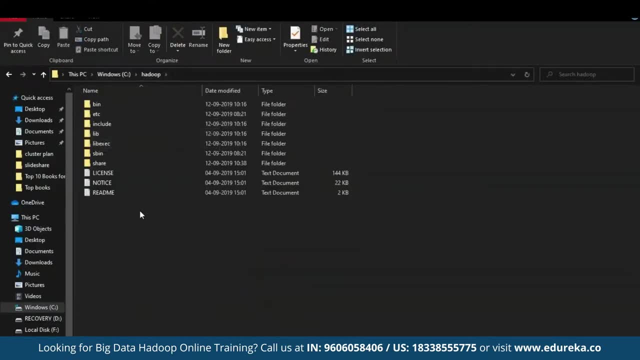 But before editing this particular file, I want you to create a new folder in Hadoop location, which is data. Let's see how to create it. So this particular folder is inside C drive, This is Hadoop, and inside this Hadoop file. 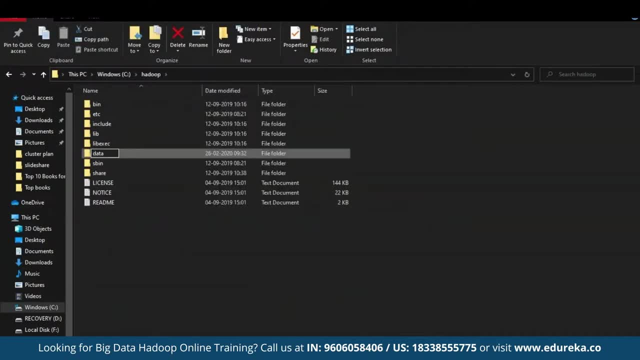 You need to create a new folder with the name data. inside data You need to create two more new files which are data node and name node. So the first folder will be name node and now another folder which will be our data node. So now let's copy the location of data node and name node. 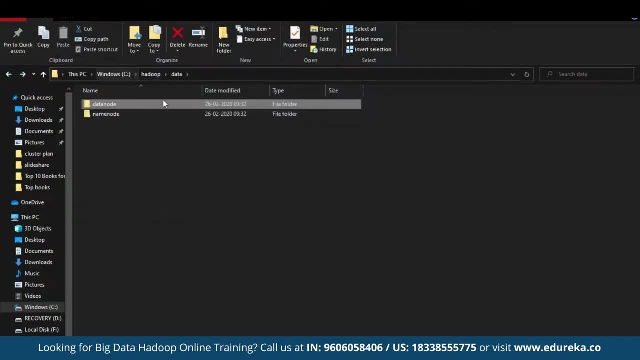 So this location is the data node location and, followed by that, the name node location. So this particular location will be the name node location. We have the two locations copied onto our clipboard. Now let's go back to the HDFS site. dot XML file. 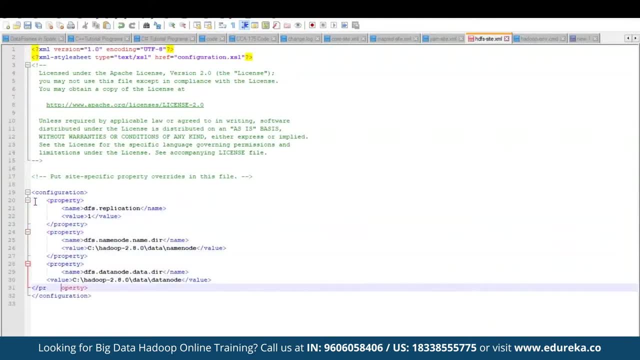 and edit the configurations here. So you can see that we have edited the configuration file of HDFS site dot XML and inside the configuration We have provided the replication factor, which is the first property, and we have set the value as one, since we are using our local system. We might want to save memory. So the replication is only one, but the default value for the Hadoop replication factor is 3- and followed by the first property, the second property, which is our name node- So we have provided our name node location. 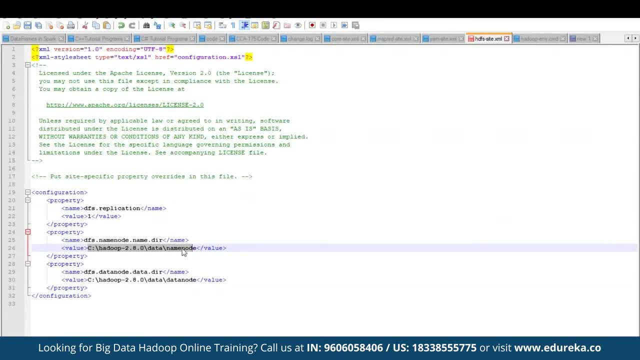 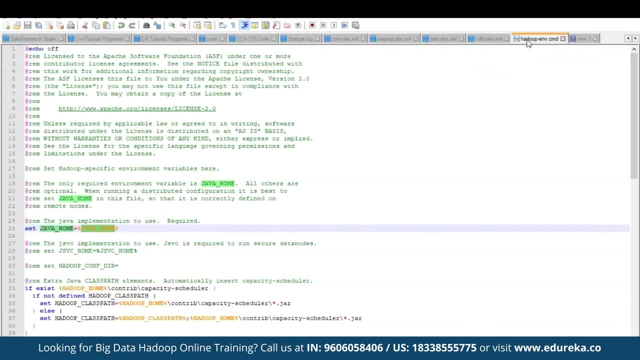 which is Hadoop file, and followed by that the data file, and inside that we have the name node and similarly the last property, which is the data node property. So here the value is Hadoop data data node. Now let's save it, Now that we have successfully edited all our four important files. 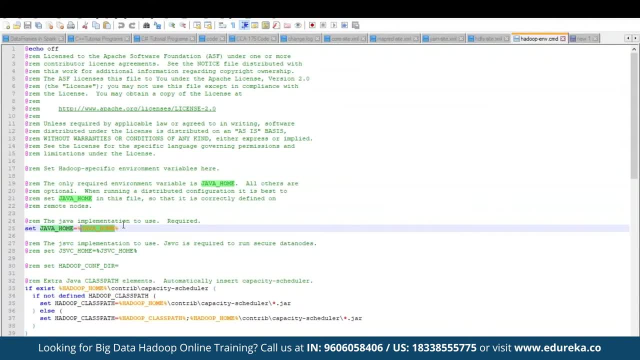 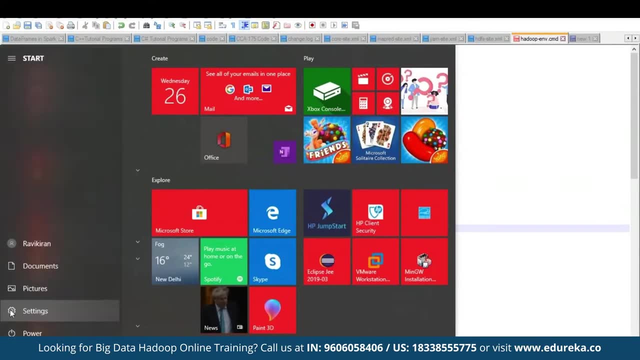 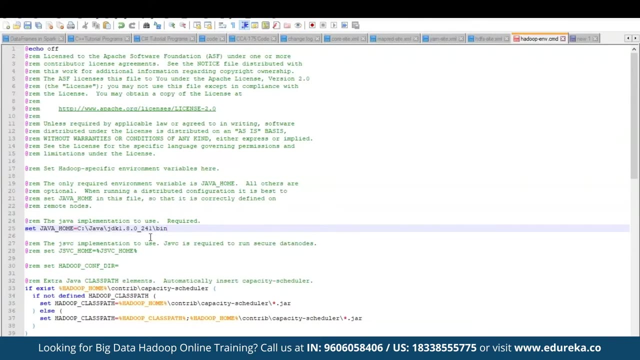 Let's get back to Hadoop ENV dot CMD file And edit the Java home location. So, for safer side, let's get back to environment variables and get our JDK location. So this particular location is the location for Java home. We might want to remove the bin over here. 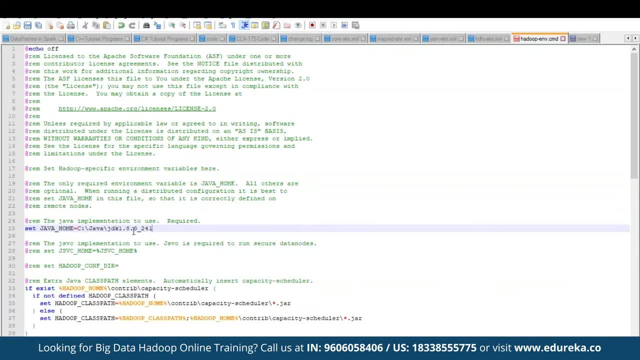 So only see, Java JDK is enough to set the Java home into our Hadoop ENV dot CMD file. Now let's save this particular file and close it. So all the important files have been now successfully edited. Now let's go back to environment variables. 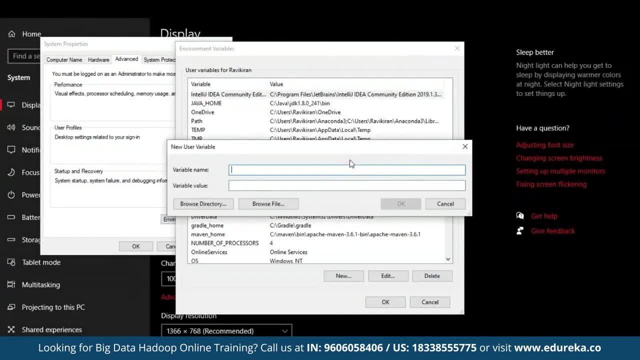 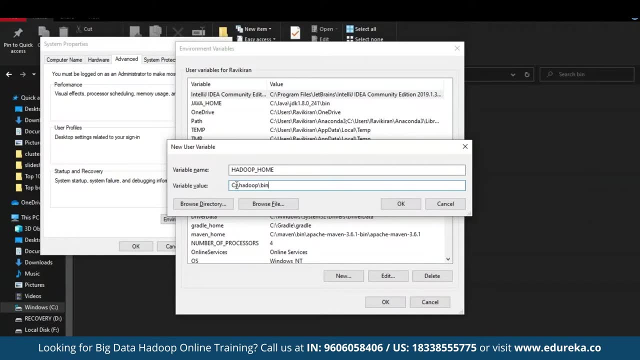 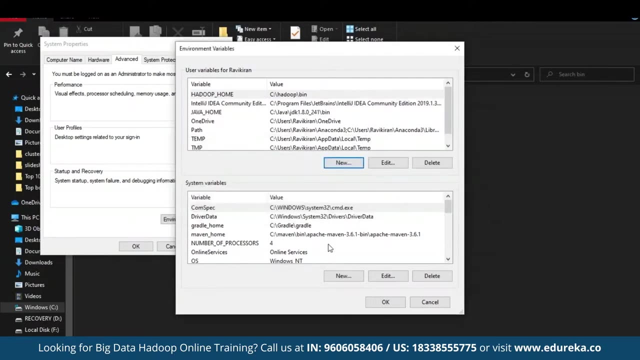 and set home and path for Hadoop. Now select new and write in Hadoop home. So this particular location, that is, see Hadoop bin, is the location for Hadoop home. now select. Okay. Now let's get back to path and set path for Hadoop files in here. 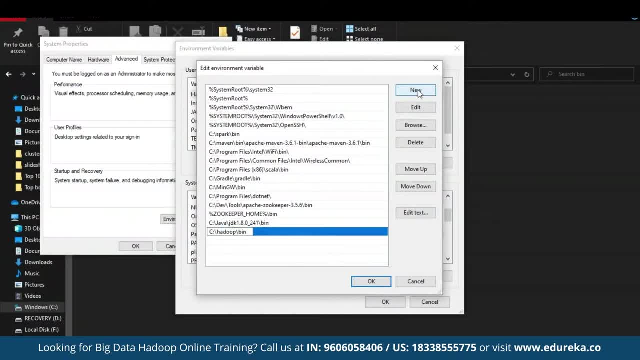 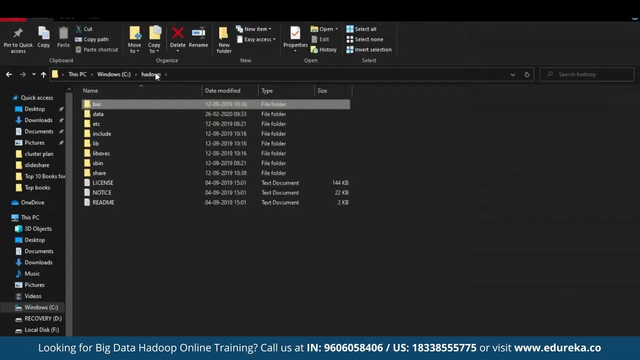 Let's set up a new path variable, that is Hadoop bin, and now remember to create another path variable, that is your S bin. So to locate S bin, get back into Hadoop and select S bin and this will be the location or path value for your S bin. 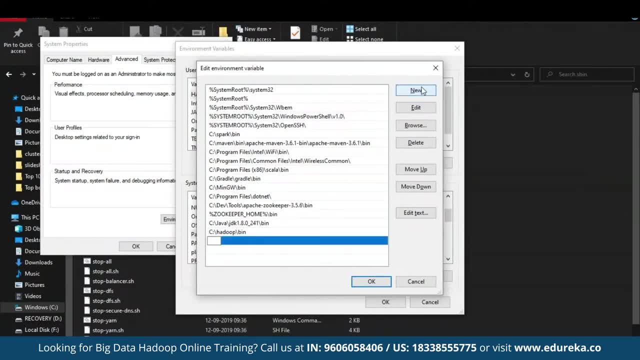 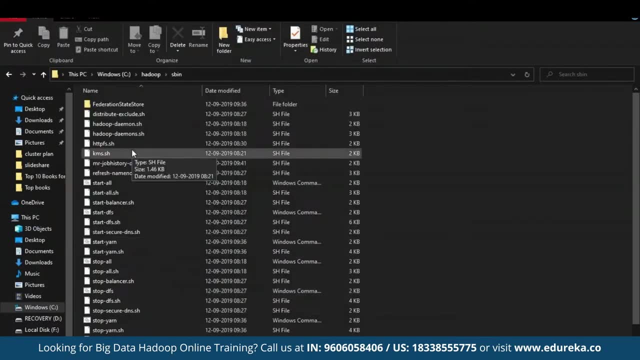 Select that and edit a new variable in path and paste it. So that's how you set S bin and select Okay, Okay And finally another okay and close the system properties. Now that we have successfully set home and path for Hadoop. 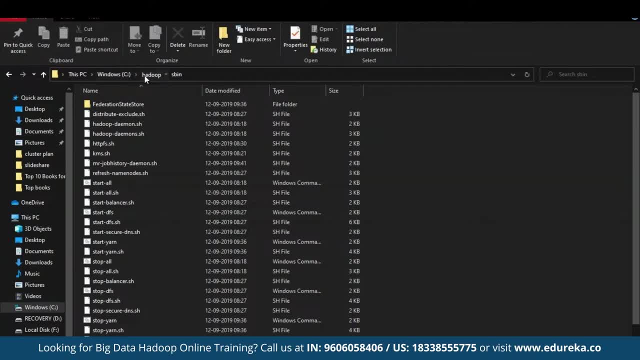 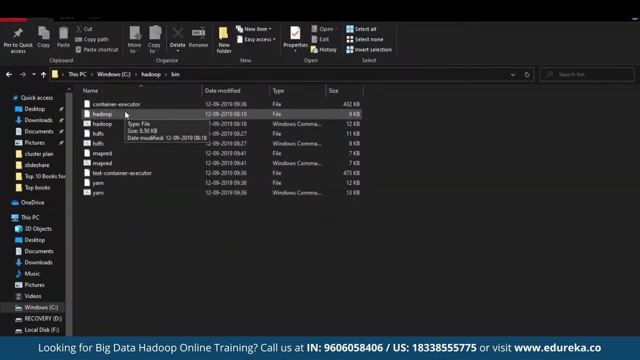 Let's go ahead and fix the configuration files. You can see that inside the bin folder of Hadoop We are missing some important configuration files. to fix this, We need a new configuration file, which will be available in the description box below. You can click on that particular link. 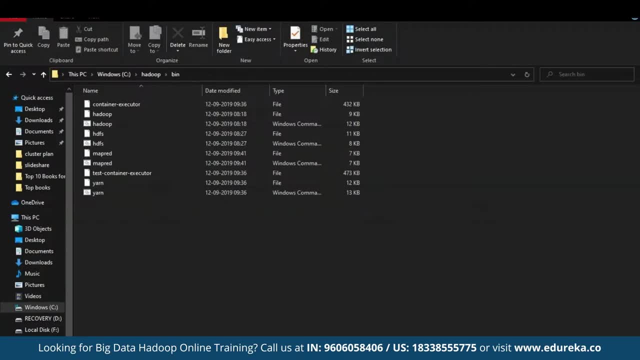 and the required configuration file will be downloaded into your local system and all you need to do is just replace that particular file with your bin folder in your Hadoop. You can see that there is a new file in my Hadoop, which is Hadoop configuration FIX, bin 1, dot Rar. 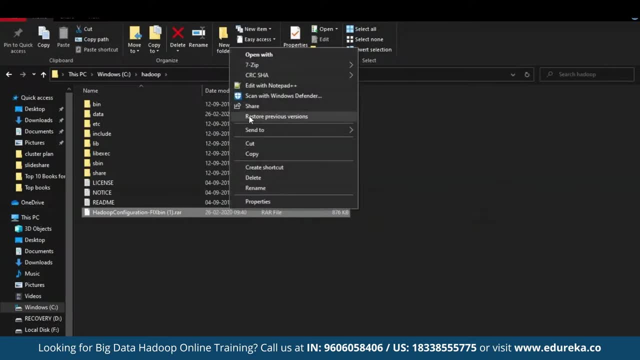 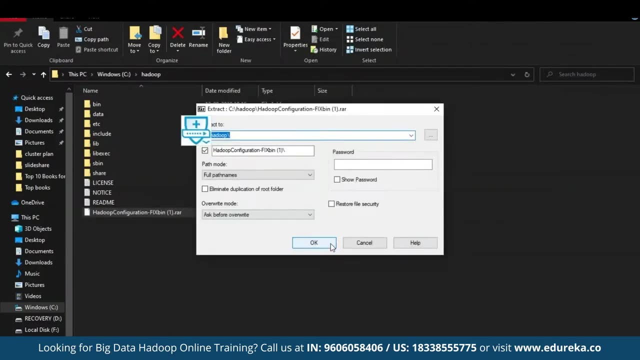 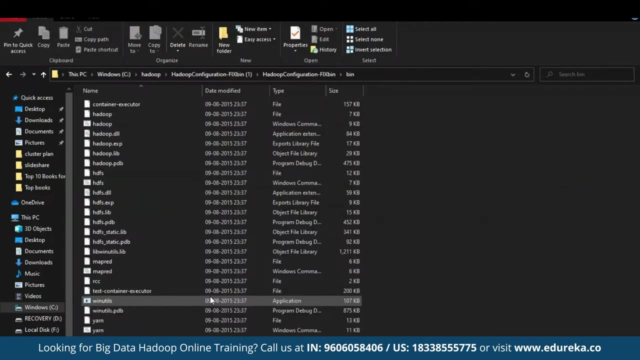 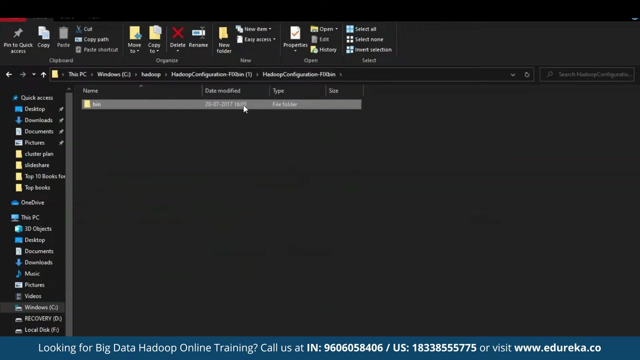 Now all you need to do is just extract this particular folder. You can see that the folder is been successfully extracted and all the executable files that you require in your Hadoop have been downloaded successfully. Now what you need to do is just move this bin into your Hadoop bin. 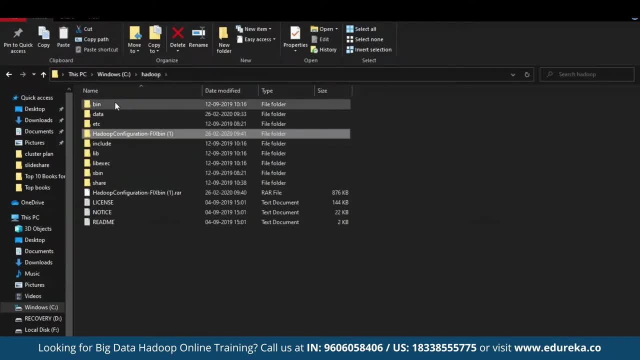 So cut this bin and get back to Hadoop and enter bin. So just delete this particular bin and replace it with a new one. So there you go, You have successfully done it. Now let's delete the unnecessary files. There you go, as good as new. 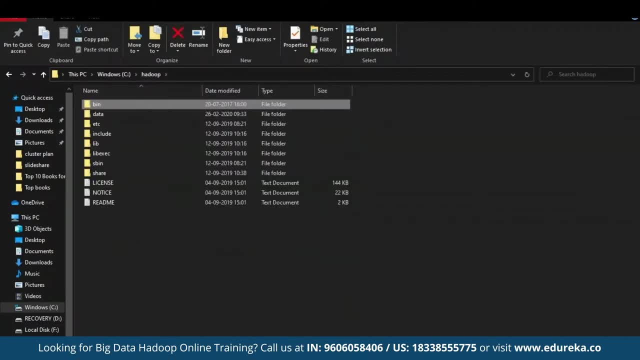 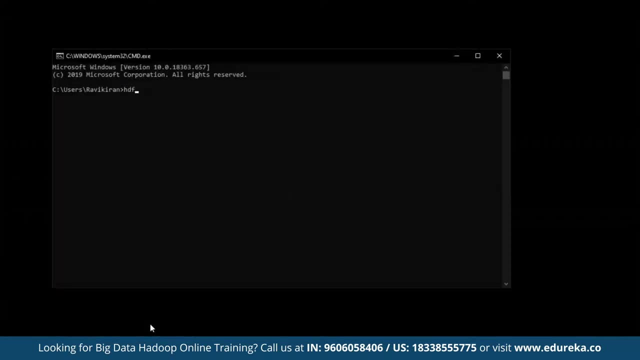 So you have all the executable files and your Hadoop has been set. to check if Hadoop is functioning properly or not, Let's open cmd and type in HDFS space name, node, space hyphen, format. If you see a set of files popping up on your terminal. 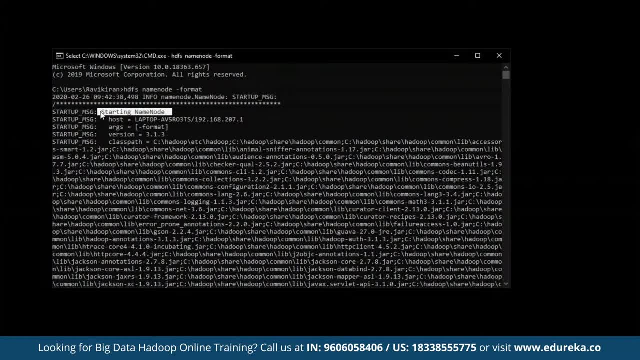 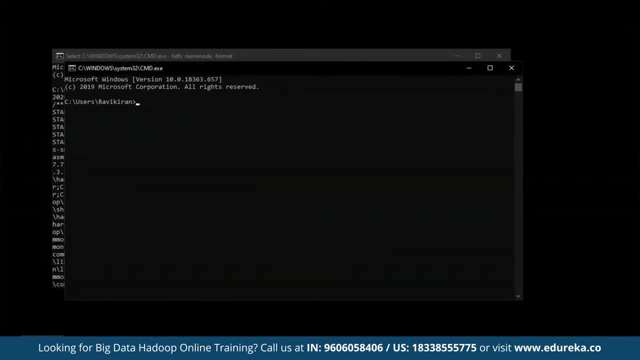 that means you have successfully installed Hadoop. You can see that the name node has been successfully getting started. Now let's open a new terminal and start all the Hadoop demons here. You just need to enter your Hadoop location file, That is CD space Hadoop. 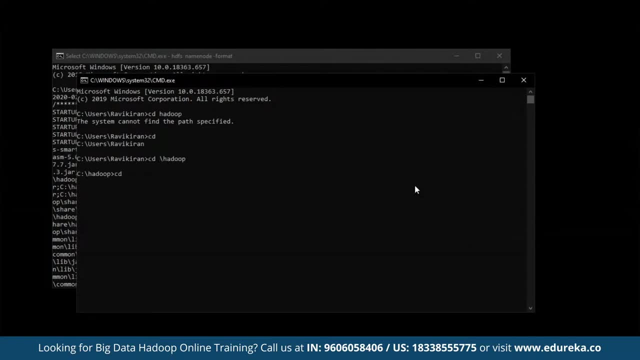 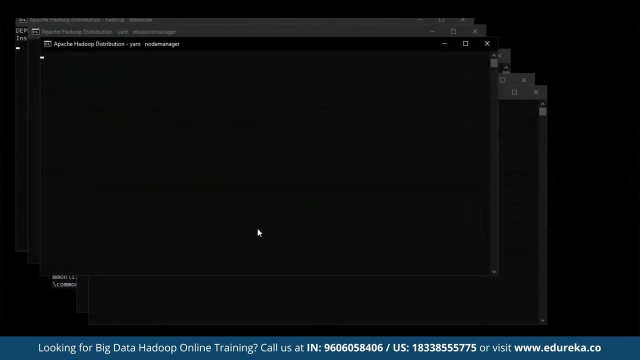 Now you are inside Hadoop and inside Hadoop, enter a spin. Now you're inside, has been. now you need to type in: start all dot, shr, start all dot, cmd. And there you go, All your demons are getting started. So that's how you install Hadoop. 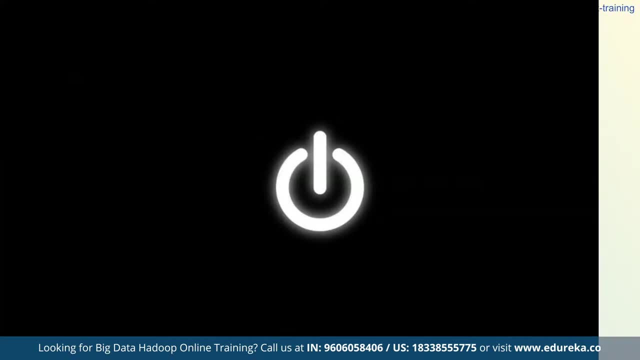 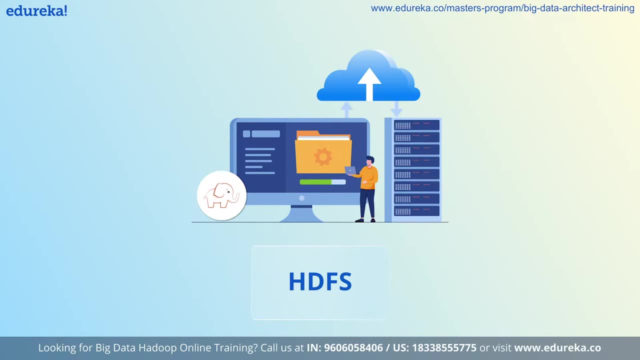 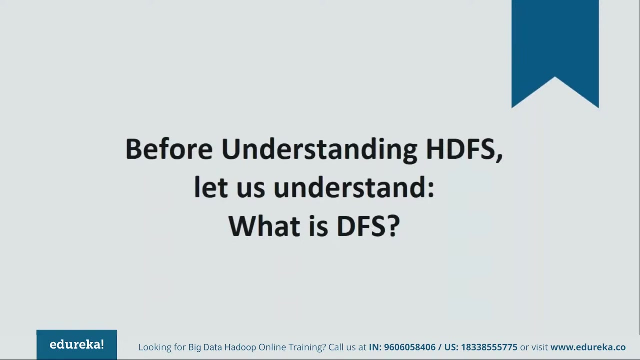 into your local Windows operating system with the version Windows 10.. Now you would be thinking: how does HDFS work? First of all, as you know, HDFS stands for Hadoop- distributed file system. So let us take a step back and understand what actually is a distributed file system. 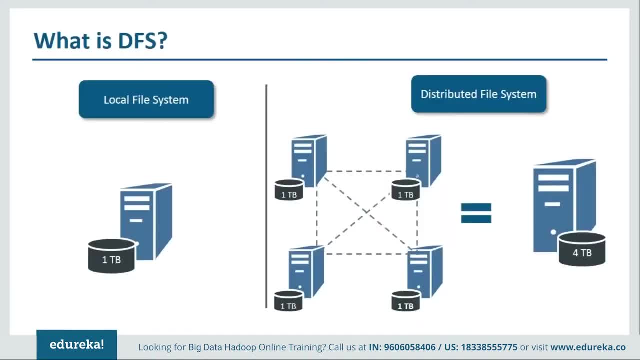 in the first place. a distributed file system talks about managing data, that is, files or folders, across multiple nodes or computers. It serves the same purpose as the file system provided by the OS in your PC. For example, for Windows, you have something called as NTFS. 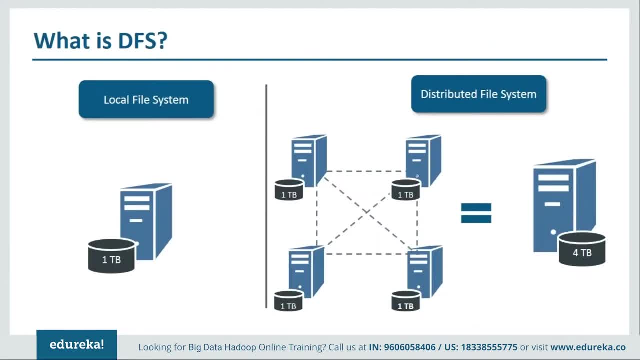 or for Mac, you have something called as HFS. The only difference between the file system that is there in your PC, that is, your local file system, and a distributed file system is that, instead of storing data in a single machine, in case of distributed file system, your data is stored in a cluster. 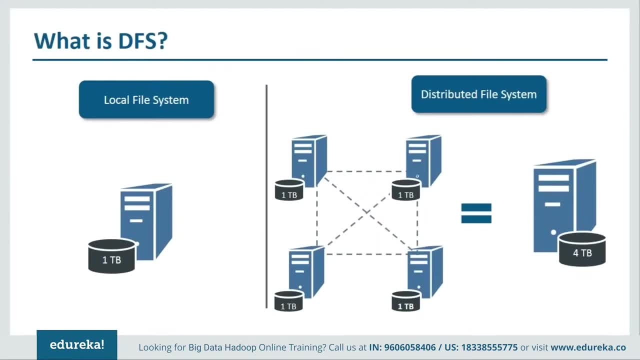 which is again nothing but a bunch of computers connected to each other, forming a network, Even though the files are stored across a cluster. the DFS will organize and display your data in a such a manner that if you try to access the data from any one of the machine in the cluster, you will feel. 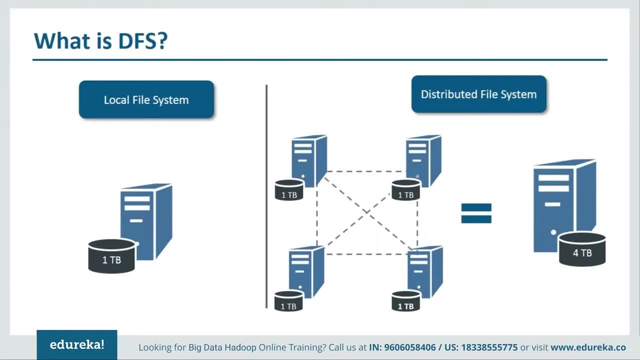 as if the data is stored in the machine that you were using. In other words, DFS provides you an abstraction of a single big machine that has a combined disk capacity equal to sum total of disk capacity of each nodes in the DFS cluster. Now let me give you an example just to clarify things further. 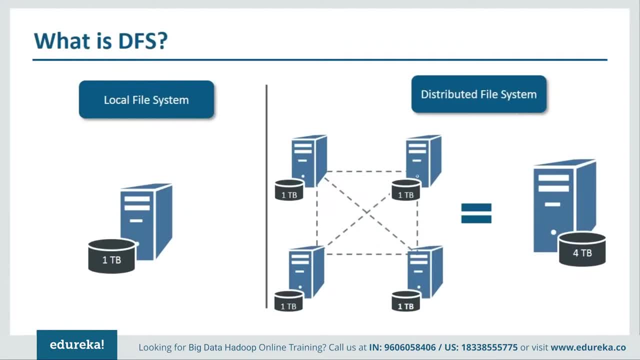 Suppose you have a DFS comprising of four computers where each computer has a disk capacity of one TV. in this case the DFS will provide an abstraction of a very big machine that has combined storage of 4 TV. Now you can go ahead and store a single file of, let's say, 3 TV. 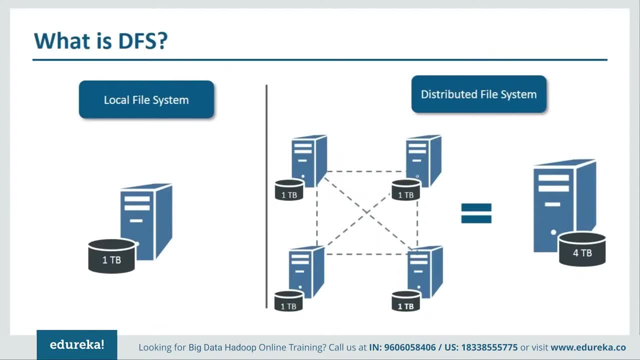 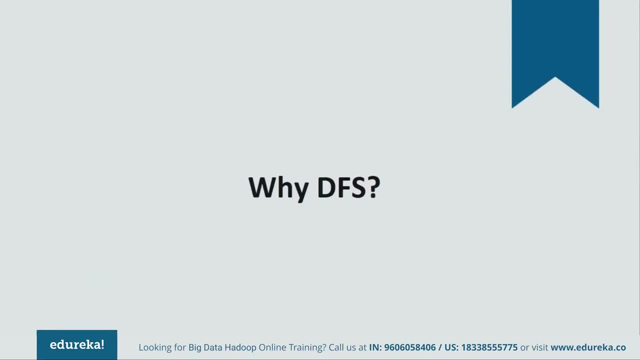 which will eventually get stored and distributed across the four computers. So this is all about DFS, guys. next you may ask why we need DFS in the first place. I mean, we could have just increased the disk capacity of single machine to whatever that is required. 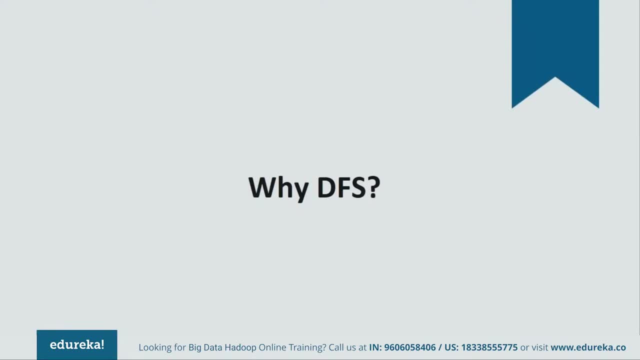 Well, first thing is there is a limit up to which you can increase the disk capacity of a single machine. Even if you somehow manage to store all of the data on a single machine, it would lead to another big problem, That is, it would take a lot of time to process. 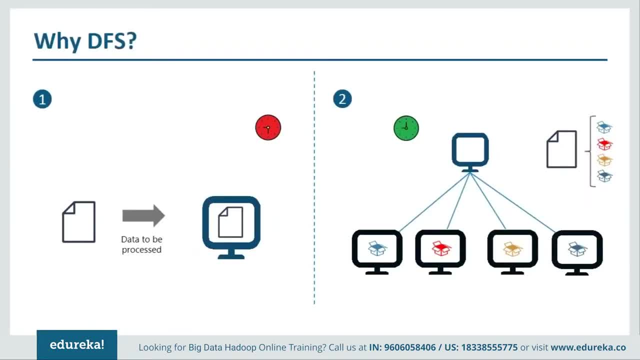 the data using a single machine. Let us take an example to understand this. for example, let us say I am having a 4 GB file that takes 4 hours to completely process it using a single PC. Now what I did? I used DFS and stored the same 4 GB file in a four node. 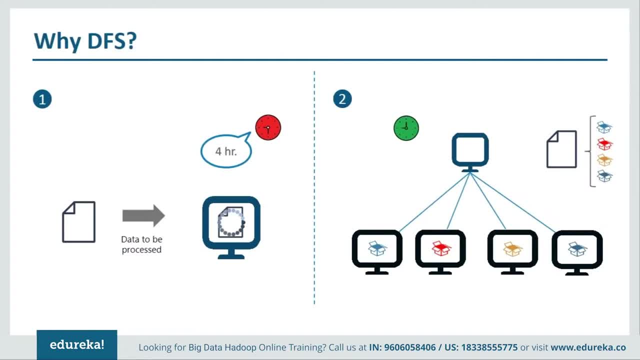 cluster where each node was storing a chunk of file. that file that will be equal to 1 GB. So therefore, in total, the 4 GB file was distributed across the cluster. Now what I can do: I can process each chunk of file finally using the four computers, thus reducing 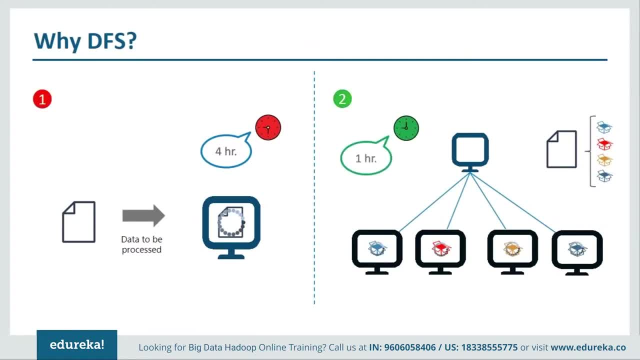 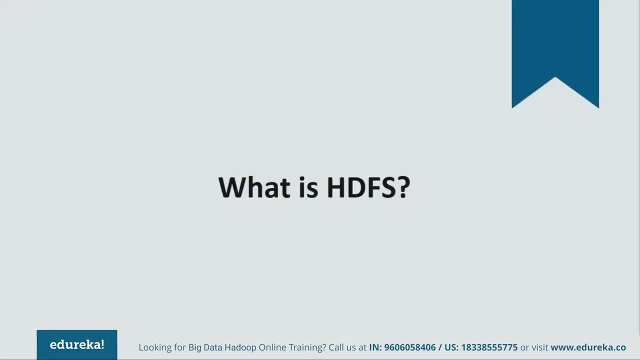 the entire processing time, which will be reduced to 1 4th of the former. that is equal to 1 hour. So that is the advantage that you get with DFS. So I guess by now you would have understood what is DFS or why do we need it. 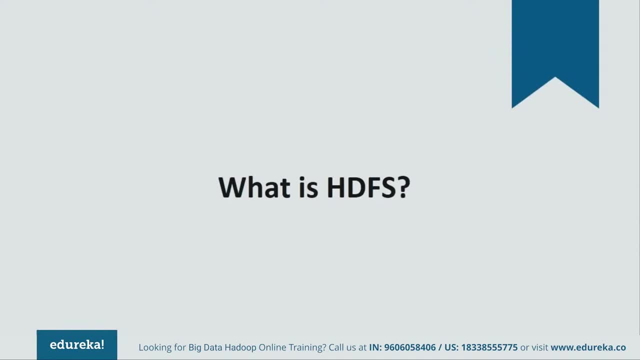 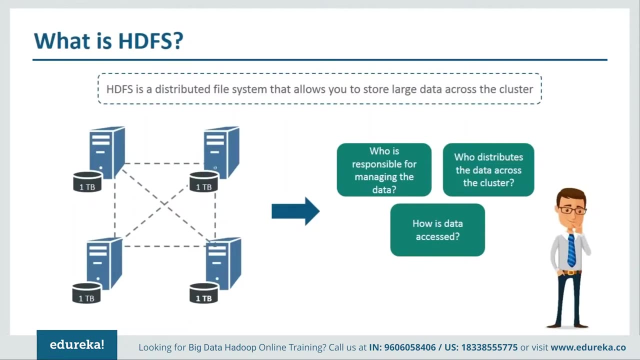 Let us come back to SDFS again. So again, SDFS is also a distributed file system, but for Hadoop. that allows you to store huge data sets, that is, terabytes and petabytes of data across the cluster or multiple machines, so that you can go ahead. 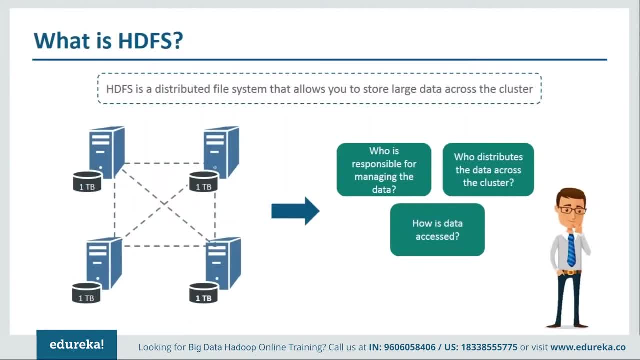 and process the data stored in each machine in parallel. Simple, yet quite powerful idea, isn't it? So that is the main reason why Hadoop, or SDFS, became so famous. Now, the next question that would be pondering in your mind is: how does SDFS manages the data? 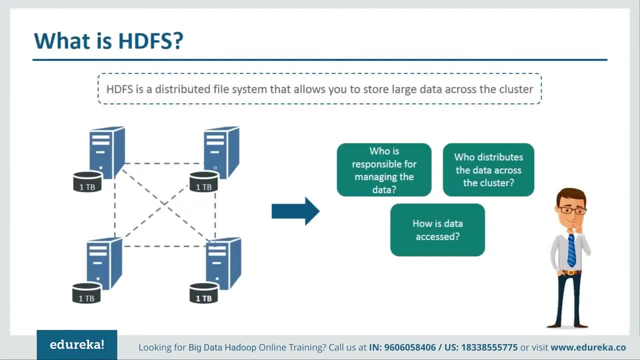 or who distributes the data across the cluster? How can one access the data present inside SDFS? To answer this questions, you need to understand the architecture of SDFS. Now, SDFS, or Hadoop cluster, follows master-slave topology. It means that you have one master node. 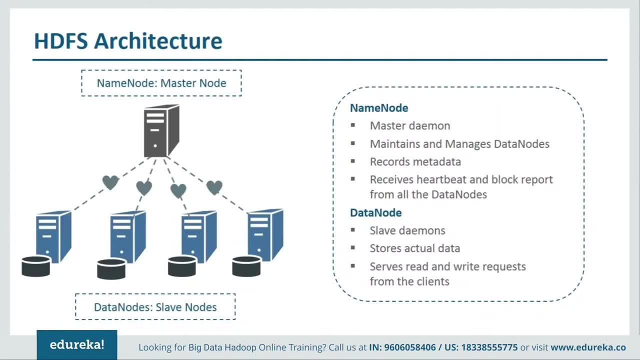 and remaining all other nodes are slave nodes. In SDFS, the master node is called as name node, whereas the slave nodes are called as data nodes. Now, data nodes are actually responsible for storing the actual data, Whereas name node, being the master node, is responsible for managing all the slave nodes or data nodes. 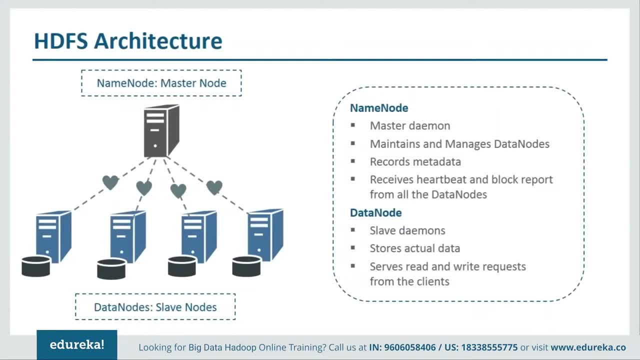 Other responsibility of name node includes maintaining and managing metadata. Metadata is information about data that is there or present inside the data nodes, So name node will be keeping all those information regarding which data are stored in which other data nodes Along with that data node are supposed to send some hard bit. 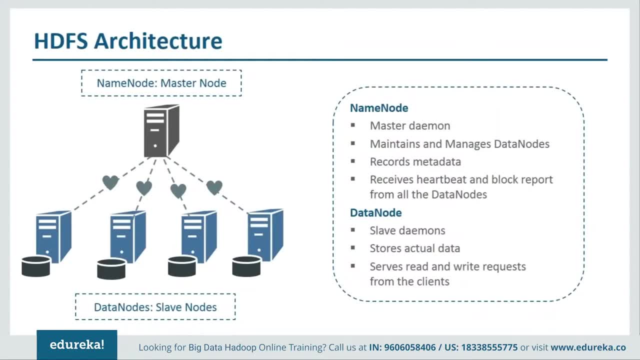 or a signal so as to ensure that all the data nodes are working to name node. So if, let's say, one of the data nodes stop sending that signal, the name node will, as a result, assume that that particular data node has been failed and that same will be notified to the admin. 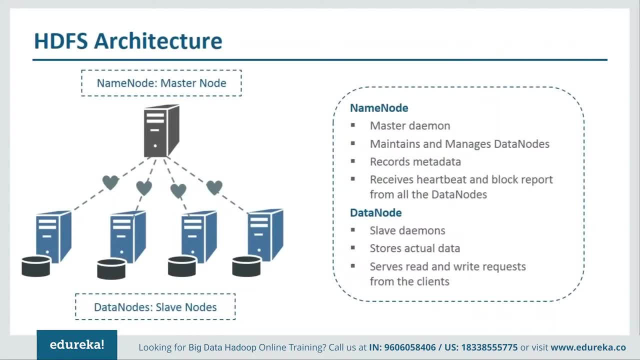 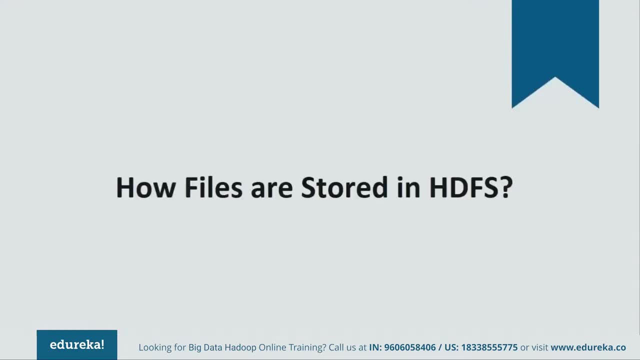 so that a new data node can be commissioned. So other information in the metadata are like file permission, directory permission, the data locations and all that. So all those stuffs are there in the name node metadata. So now that you have understood the architecture, that is followed by HDFS, where we have one master node. 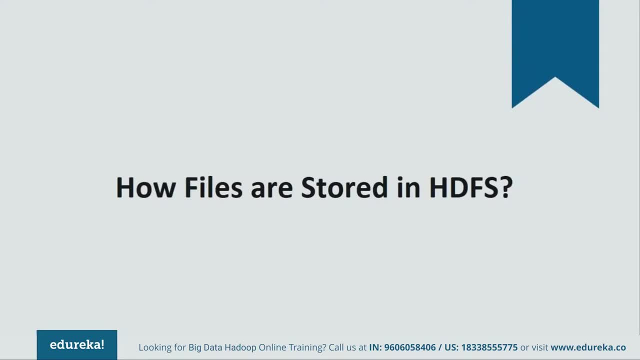 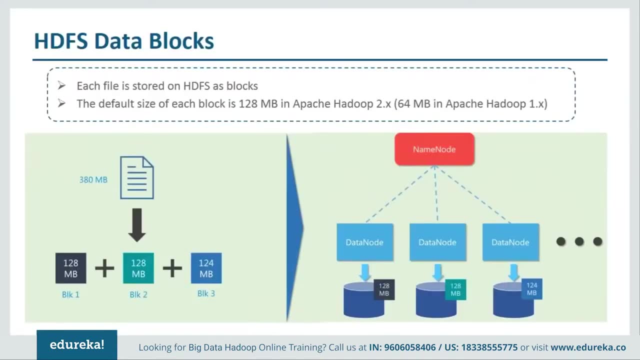 and when we have slave nodes as data nodes. Now the question is how files are actually stored inside HDFS. Just like any file system, in case of HDFS also, the files are stored as blocks. The only difference between the file system block size- in that is there in your system- to that of our HDFS. 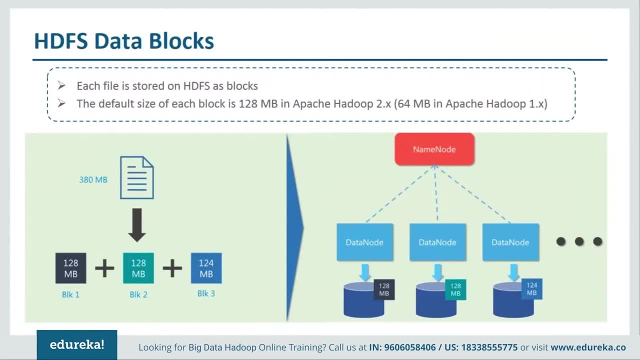 is. the default size of each block in HDFS is 128 MB. since we are dealing with a large or huge amount of data set, It is configurable and you can go ahead and change the default block size as per your use case. Now let us understand. how does this work? 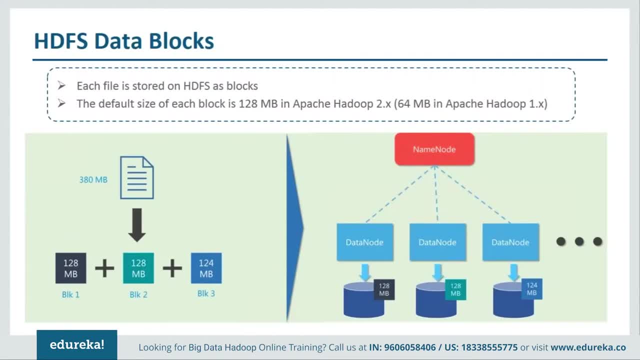 For example, let's say I want to put a file of 380 MB into HDFS. So this 380 MB file will be broken down into three data blocks, where the first two data blocks will be of 0.28 MB, just making 256 MB. 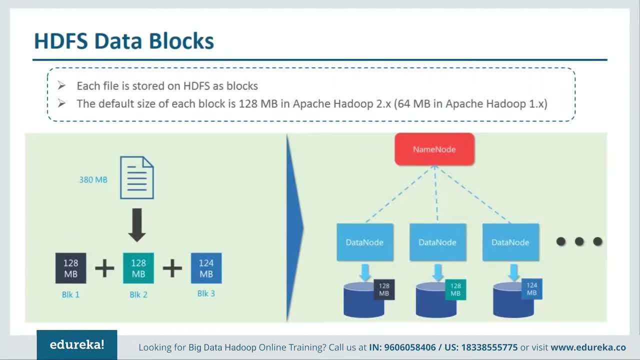 and the last block will be occupying 380-256 MB, that is equal to 124 MB. Then, finally, these data blocks will be distributed across the cluster, that is, in different different data nodes. Now, when you will look at this implementation, you will find one more problem. 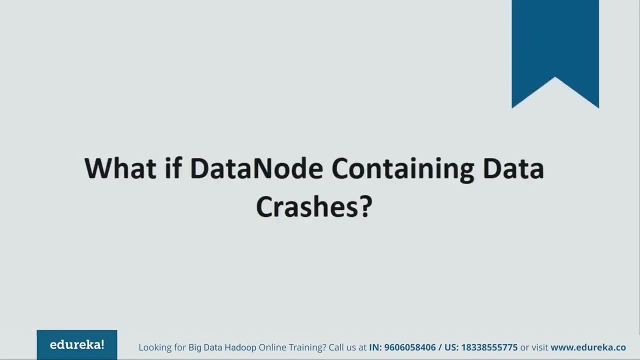 What will happen if one of the data nodes containing the data blocks crashes? So how will name node ensure, or how will HDFS ensure, fault tolerance with respect to the current implementation that we are doing? Let's understand this problem with an example, So we'll take the same example. 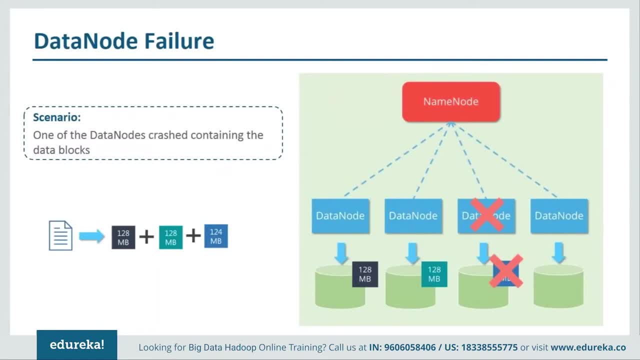 that we were having in the previous case, where we are having one file of 380 MB that has been distributed across the HDFS with three blocks. Now, let's say, the third data node, having the 124 MB block, has been crashed. So in this case, 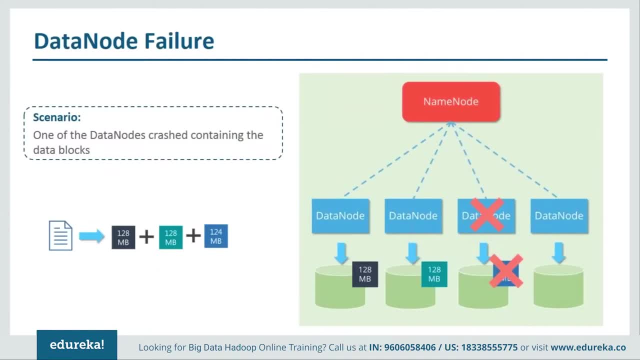 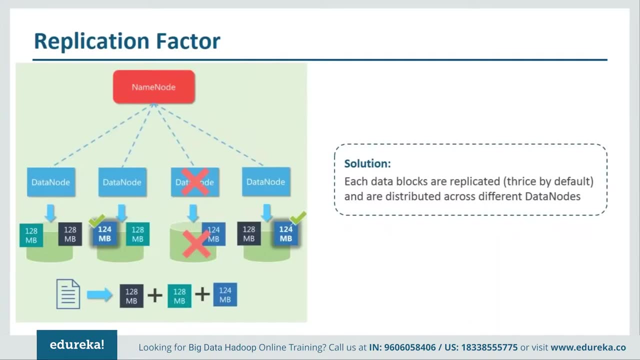 we will not be able to retrieve the data or we will be facing data loss issue. So HDFS has a solution for it, called as replication factor. So what happens is, whenever you are storing any data or copying any file into HDFS, it is broken down into blocks. 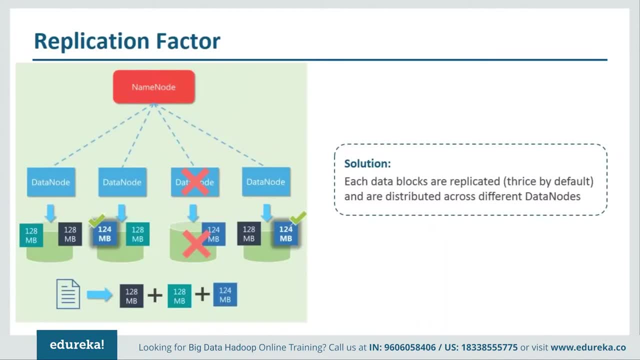 and each blocks are replicated thrice by default and are distributed across the data nodes In case if any of the data nodes fails. in that case we can again retrieve the data by having a replica that will be stored in some other data nodes. 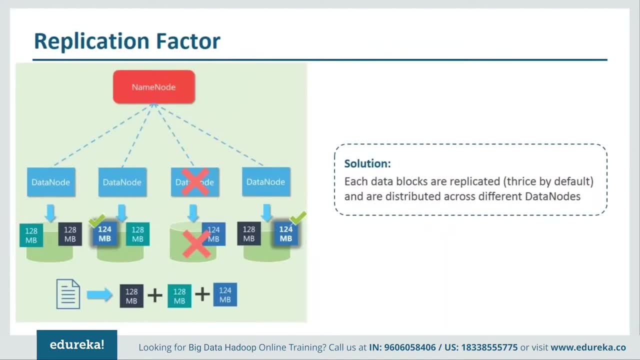 So that is how your HDFS ensures fault tolerance capability. Also, there is one more advantage of having master-slave topology is that we can go ahead and add more nodes on the fly. So, for example, let's say I want more disk space in my cluster. 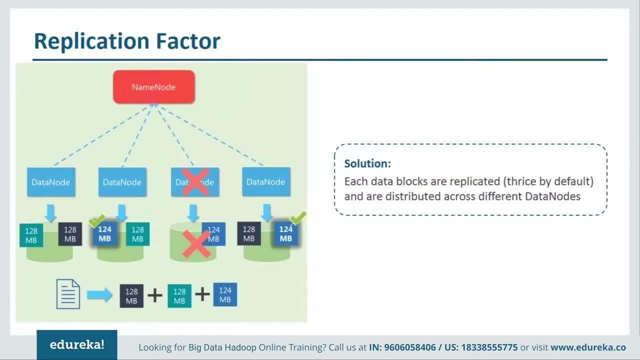 In that case, what I can do. I can commission new data nodes on the fly without affecting the current infrastructure. So enough of the theory, guys. So let's go ahead and have a look at the real cluster. How does it look like and what are the different ways? 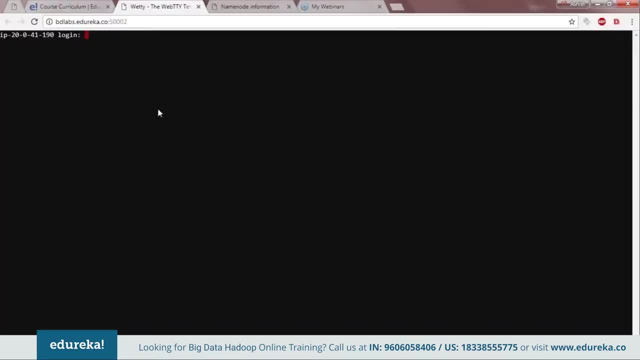 via which we can go ahead and access HDFS. So these are edge node guys. Let me log in. All right. So basically we'll be having two type of file system over here. One will be the local file system with respect to your edge nodes. 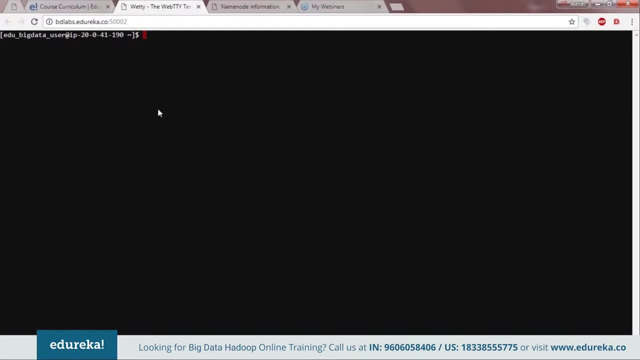 where all the files will be there, and then there will be distributed file system with respect to HDFS. So let me list all the files and directory. in both the cases, For example, for local file system, I will be using local shell command, which is LS. 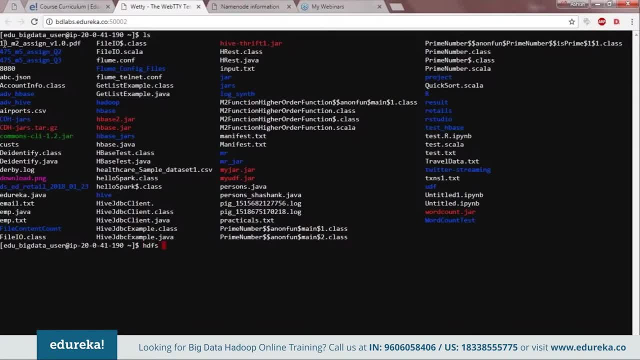 and using that you can see. these are the files that is there inside my edge node. Now for listing out the directories and files that is there inside my SDFS, I'll be using SDFS shell command. So for that you have to go ahead with HDFS DFS. 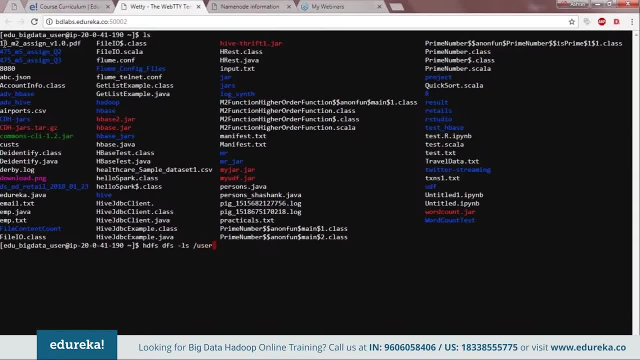 then hyphen LS and then you provide the name of the directory on which you want to list the files or sub directories. For example, in my case, I'll be looking at my profile directory. that is slash user- slash edu- underscore: big data user. So, as you can see, these are the files. 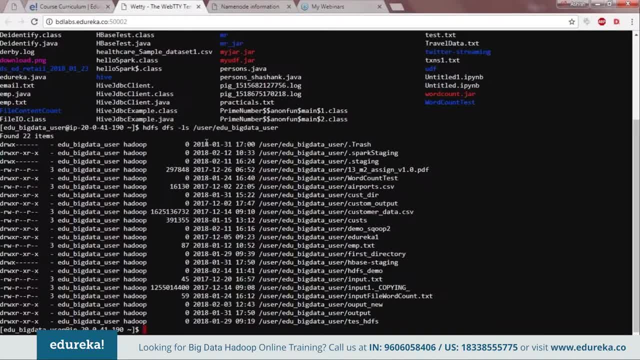 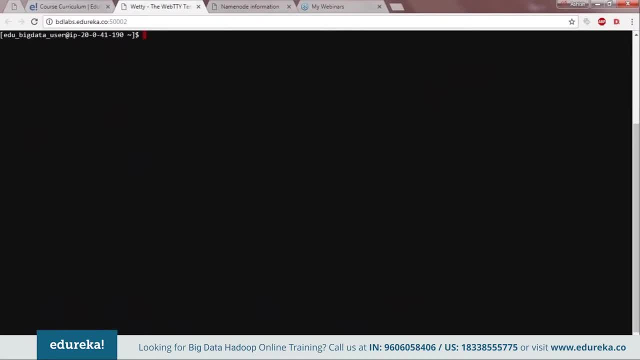 and directories inside my profile directory. So now you would be understanding how SDFS provides you that abstraction that you are using a single big machine. So let's go ahead and do some demos as well. For example, let's say I want to create a directory inside my DFS. 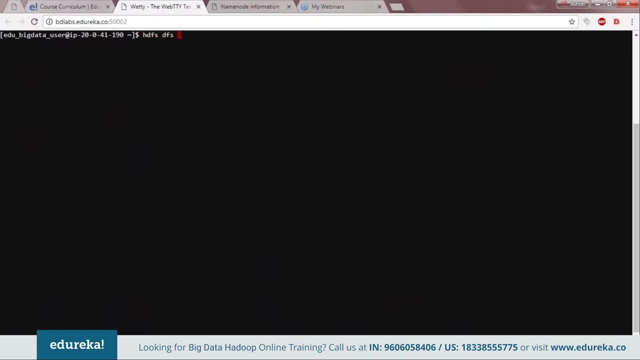 So for that I'm going to go ahead and say HDFS, DFS, hyphen, make the IR, and we'll go ahead with the name of the directory, which will be user slash, edu, big data, user, and let's name the directory as SDFS DIR. All right, so directory has been created. 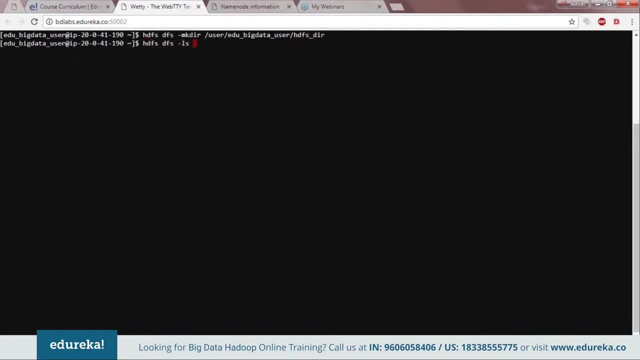 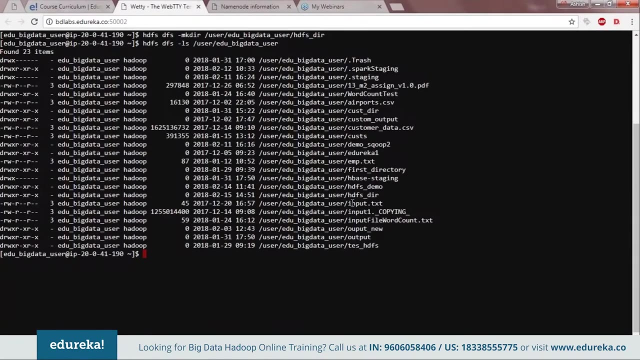 Let's go ahead and list all the files that is there inside SDFS again. For that again I'm going to go ahead and say: slash user, slash edu, big data- slash user. Oops, I made a mistake, Sorry. So here you can see I'm having a subdirectory call as SDFS DIR. 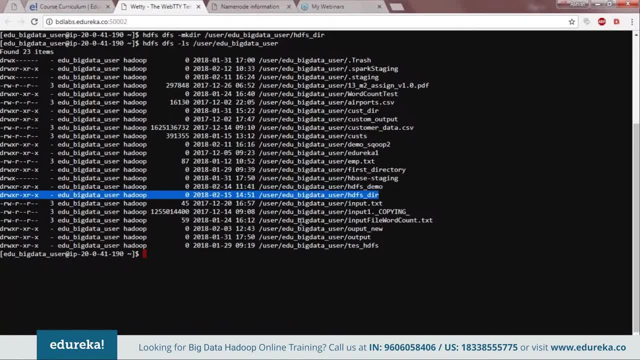 which has been created recently. All right, Now let's go ahead and copy some of the data from edge node to HDFS. So, if I do LS, these are the files that is there inside my edge node. Let me choose one file. 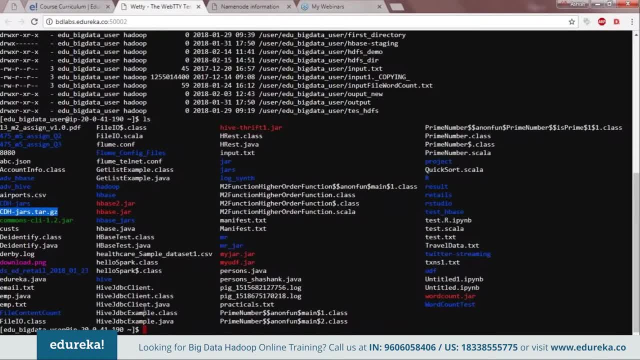 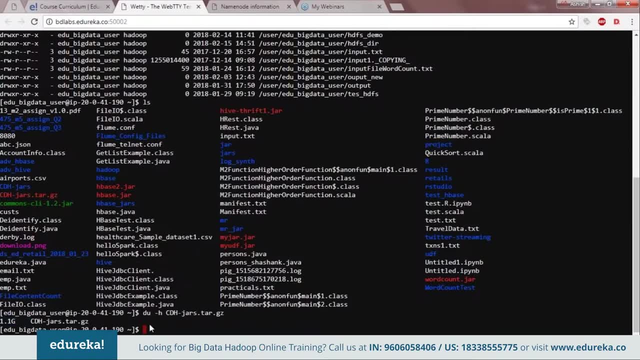 So basically, I'll be copying this particular tar file. So let me check the size of this tar file. All right, the file size is of 1.1 GB. Let's go ahead and copy it into the cluster. So I'll say SDFS, DFS. hyphen put. 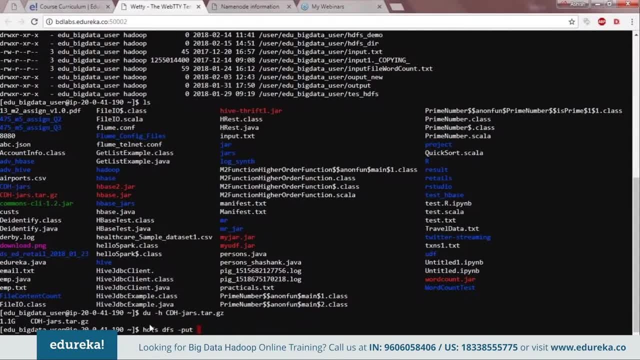 Put is for moving data from your local system to SDFS, and then I'll mention the name of the file, which is CDH. hyphen put Char dot tar dot cheesy. and then I'll mention the directory where I want to copy it inside HDFS. 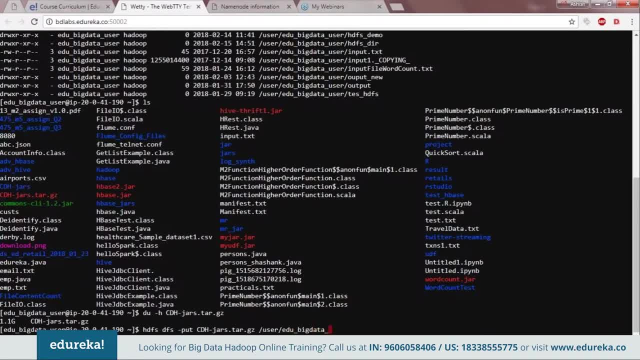 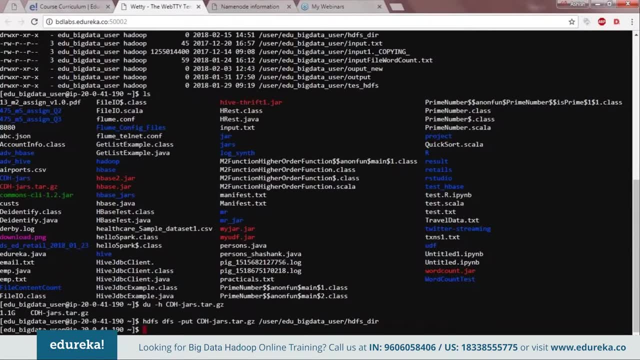 So, which will be: slash user. slash edu big data user. slash SDFS underscore DIR, the directory that we have created recently. Now let's go ahead and list the files that is there inside the newly created directory So as to ensure whether the copy has been done successfully. 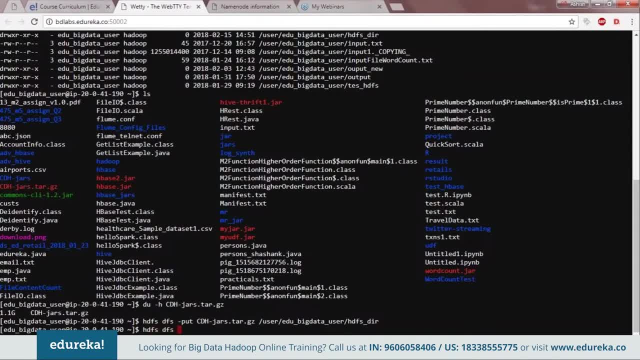 or not. for that I'm going to again do SDFS, DFS, hyphen LS. then will mention the directory path, So let me copy it and paste it over here. So, as you can see, found one item. that is the file that we have copied recently. 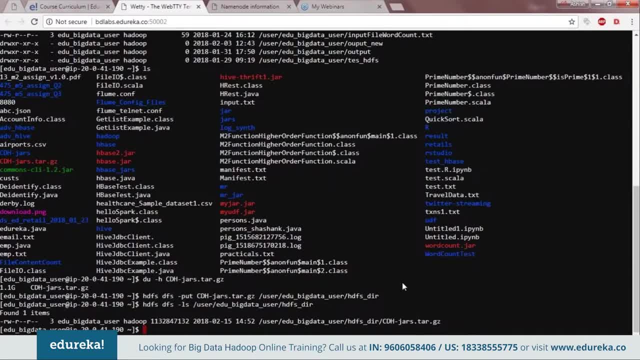 Now let us go ahead and check the number of blocks that has been made with respect to this particular file that we have copied inside SDFS. So I'm going to say Hadoop, I'm sorry, Hadoop, ffck, and then again: 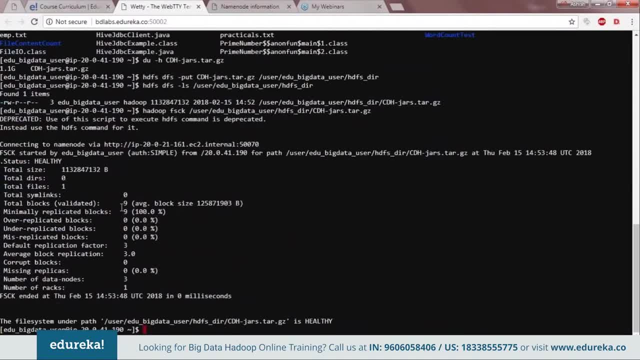 I'm going to mention the directory path. So, as you can see, we have total of nine blocks that has been created with respect to 1.1 GB file and each block has been replicated thrice by default. So in total of there will be 27 blocks there residing in SDFS. 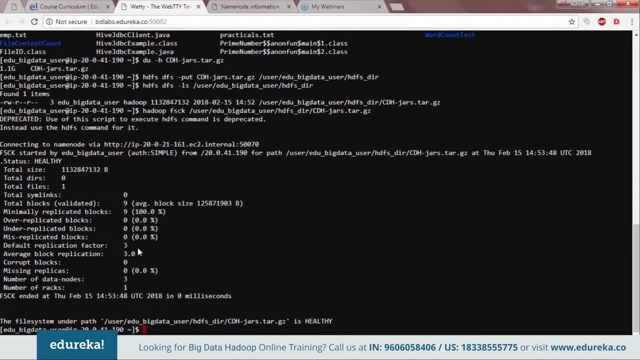 in different different data nodes. So this is how your SDFS works, guys. Now for a programmer again. I don't have to worry about how data blocks are being created or how it is being distributed among different nodes. All I have to worry about is the logic that I'll be working. 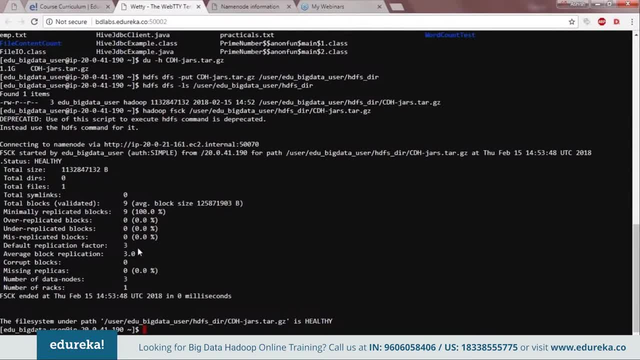 on these data. So that's why your SDFS provides you all those abstraction and provides you tools and all those API, So so that it is very easier for you to go ahead and access it and manage the data that is there inside as DFS. 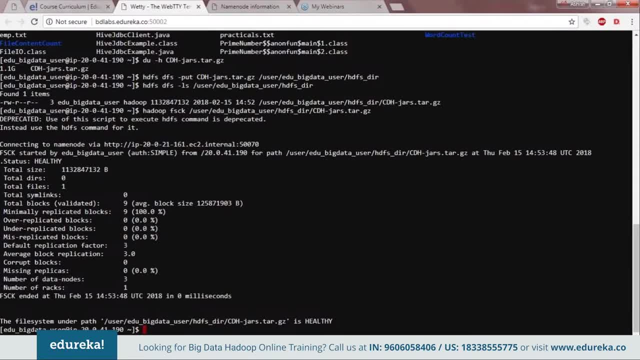 with the given fact that, even if I run a job or even if I process the data, that again the data will be processed locally in the each node in a distributed and parallel fashion, Thus will be getting a reduced processing time. So whenever you're talking about huge amount of data sets, 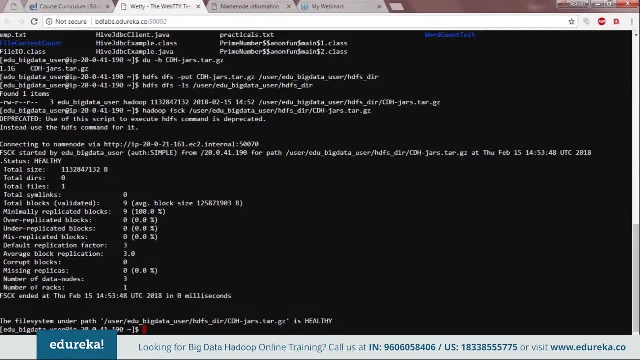 or huge data sets, SDFS is the best option. The last fact that I'm going to mention is that all these SDFS Hardware's are commodity Hardware. So basically, Hadoop is a very cost-effective solution to big data problem. in case if you have a specific use case, 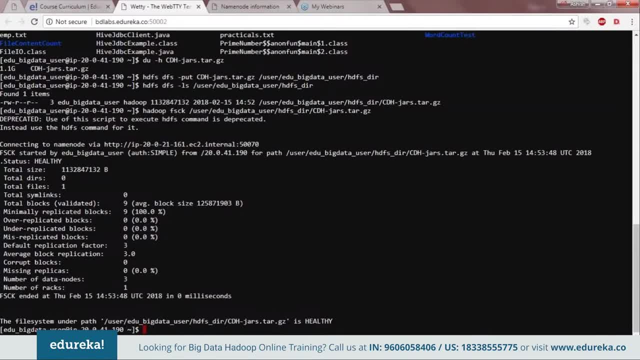 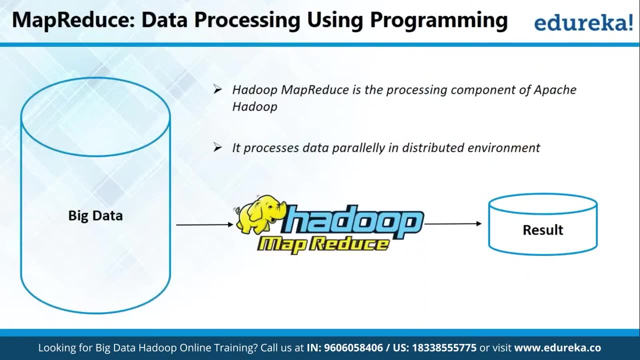 that requires more cluster configuration. then you can go ahead and upgrade your cluster or Hardware on the fly. You can add more nodes to it so that more parallelism can happen and you can again process a large data sets. What is Hadoop MapReduce and why is it required? 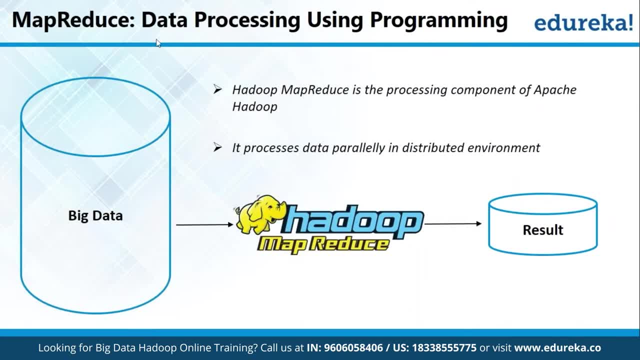 So Hadoop MapReduce is actually the processing unit of Hadoop, using which you can process the big data that is present on Hadoop HDFS or that is stored on Hadoop HDFS. But what is the requirement? Why do we need Hadoop MapReduce in the first place? 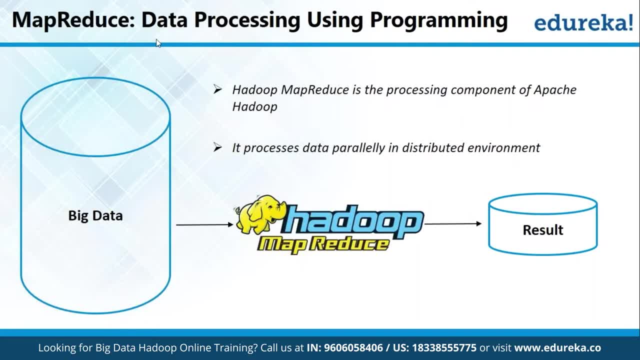 It is because the big data that is stored on Hadoop HDFS is not stored in a traditional fashion. The data gets divided into chunks of data, which is stored in respective data nodes, So there is no complete data that is present in one single location. 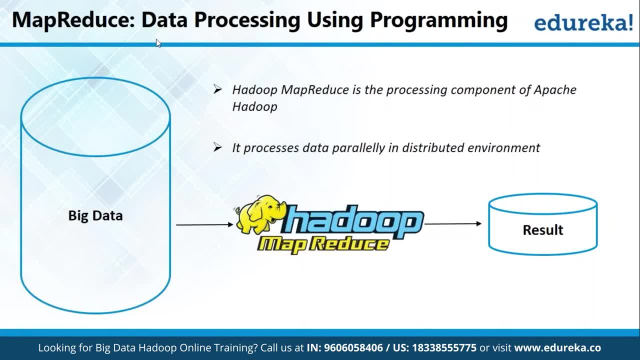 or one centralized location. Hence a native client application, which used to be there like a Java application or any other application, cannot process that data right away, And hence we needed a special framework that has the capability of processing the data that stays as blocks of data. 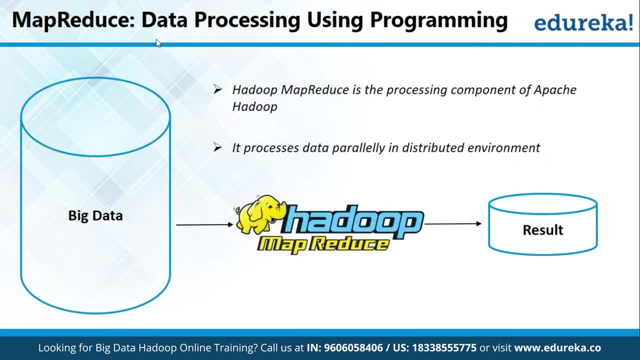 into respective data nodes and the processing can go there and process that data and then only bring back the result. So that kind of framework is Hadoop, MapReduce, And we will move on to the next slide and we will see MapReduce in a nutshell. 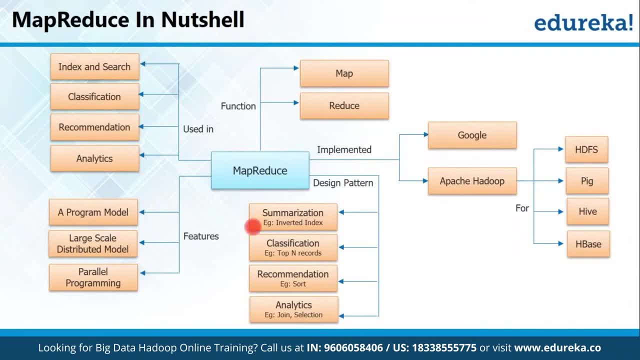 So this particular slide basically gives you the overview of MapReduce and what are the things that are related to MapReduce. To start with, what are the applications of MapReduce or where it is used? For example, it is used for indexing and searching. It is used to create classifiers. 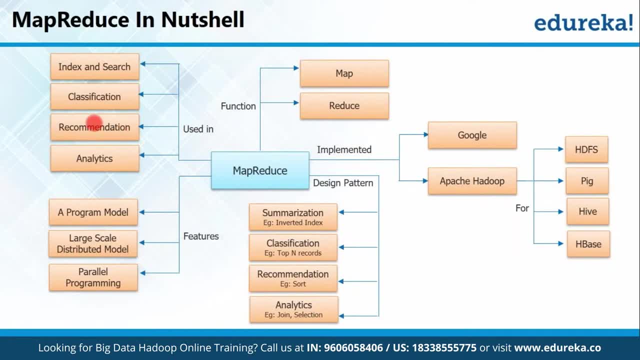 It can be used to create recommendation engines, like it has been created by big e-commerce companies like Amazon, Flipkart. It can be used for analytics by several companies. When we talk about the features of MapReduce, it is a programming model. It can be used for large scale distributed model. 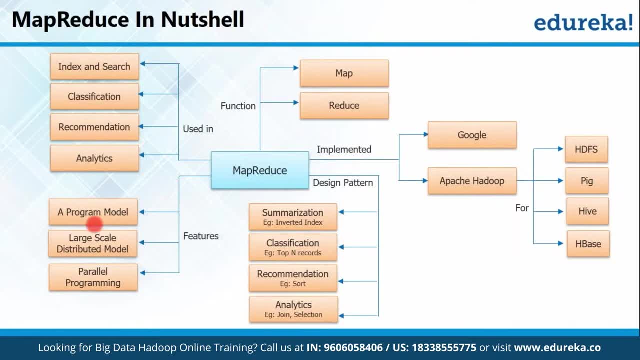 like Hadoop HDFS, It has the capability of parallel programming, which makes it very useful. When I talk about functions that are present in MapReduce, there are basically two functions that get executed. One is the map function and the second is the reduce function. 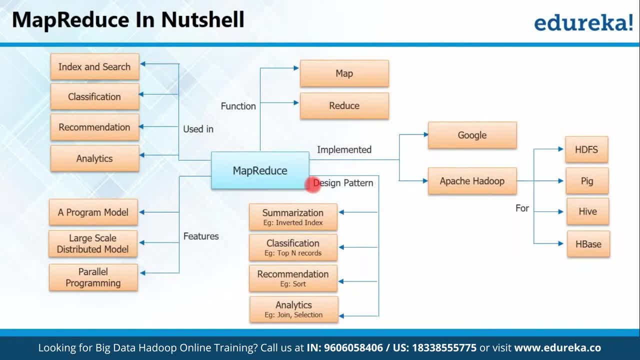 If you talk about design patterns, that has already been there in the industry for a long time. Yes, you can also implement all those design patterns using MapReduce, like summarization, classification, recommendation, or analytics like join and selection. MapReduce has been implemented by major giants like Google. 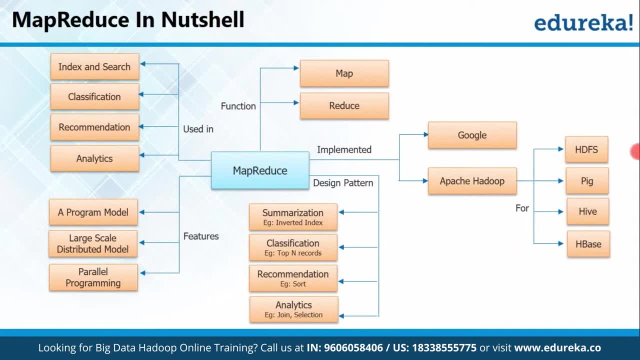 and it has also been adopted by Apache Hadoop for HDFS, for processing data in HDFS, for processing data using PIG, for processing data using Hive or for storing data or executing queries over the big data using HBase, which is a NoSQL database. 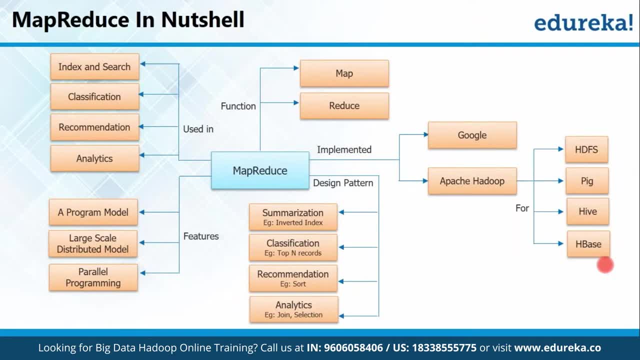 This is something which actually gives you the overview of MapReduce, and what are the various features, what are the applications where it is implemented, what are the functions that are used. That kind of information is given in this slide. Guys, are you able to grab that information? 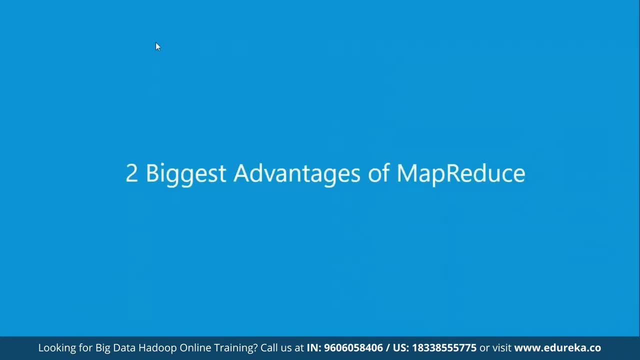 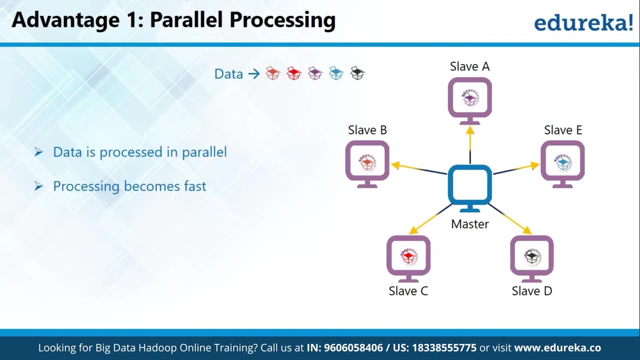 And now we will explore the two biggest advantages of MapReduce. The very first advantage is parallel processing. You must be aware of parallel processing from before as well, because it is not a very new term. Using MapReduce, you can always process your data in parallel. 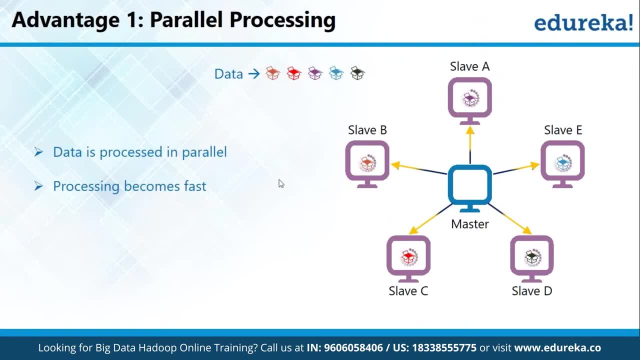 As you can see in the diagram, there are five slave machines And there is some data that is residing on these machines. These boxes are nothing but representing a chunk of data, a block of data or a HDFS block, which is getting processed in the respective slave machines. 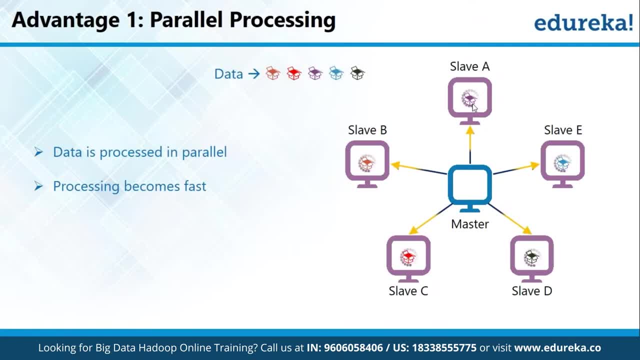 You can see a circle going on. So this simply represents the processing. So in here data gets processed parallelly using Hadoop, MapReduce, and hence the processing becomes fast. So it is as simple as the work time problem that you would have solved in your school days. 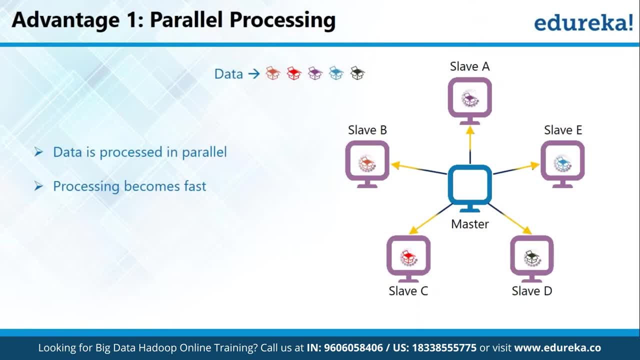 For example, you would have solved a problem like: if a particular task is done by one person, he is going to take one day. So same task, if it is done by three persons, how many days it is going to take to finish the job? So what are we doing there? 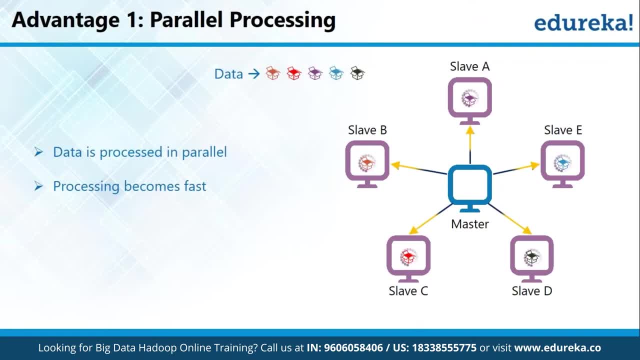 We are actually distributing the task among three people, and hence the time that is taken to execute that job becomes less. Similarly, same happens in Hadoop MapReduce. What happens is entire chunk of data gets divided by Hadoop HDFS into HDFS block. 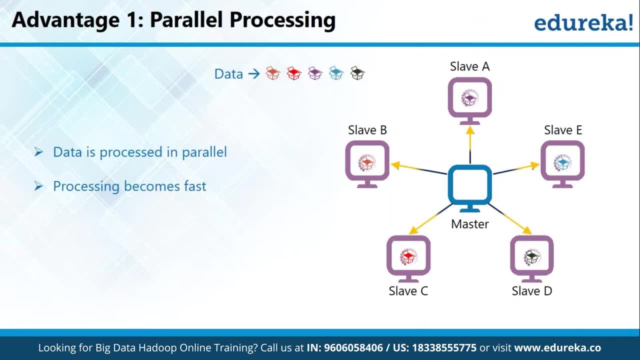 And the processing now processes this data in parallel and hence the processing becomes fast. So I will move on to the next slide and we will explore the second advantage of Hadoop MapReduce, that is, data locality. This is one versatile thing that is given by Hadoop MapReduce. 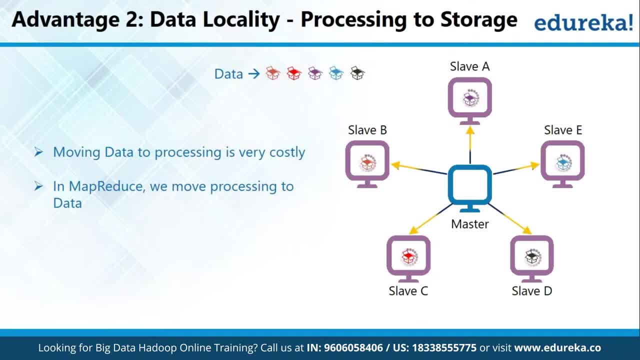 that is, you are able to process the data where it is. What does it mean? Let me tell you: The data that you move into Hadoop cluster gets divided into HDFS blocks and these blocks are stored in the slave machines or the data nodes. 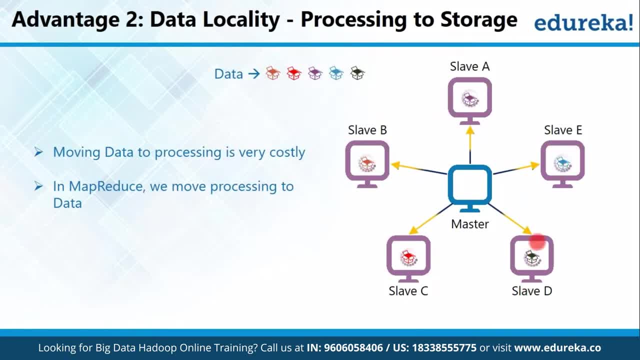 As you can see, the data is stored in all these slave machines that are there in this picture. What MapReduce does is it sends the processing, it sends the logic to the respective slave nodes or the respective data nodes where the data is actually residing as HDFS blocks. 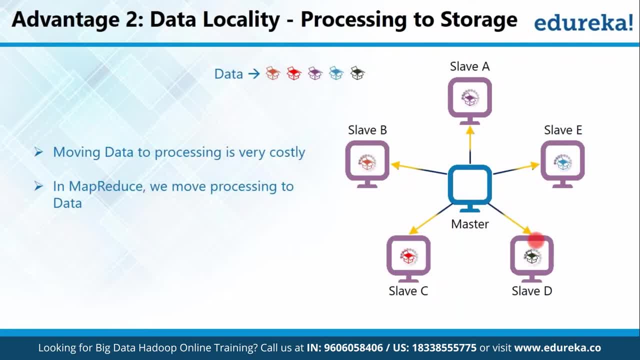 So what happens is the processing is executed over a smaller chunk of data in multiple locations in parallel. This saves a lot of time, as well as it saves the network bandwidth that is required to move big data from one location to other. Just remember that this was big data, which was broken down into chunks. 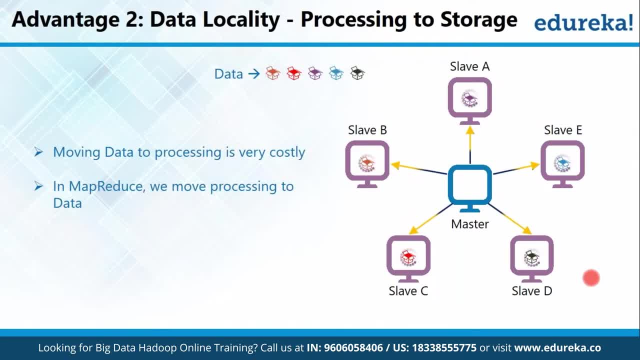 If you start moving that big data through your network channels into a centralized machine and then process it, it will give you no advantage because you are going to consume the entire bandwidth just in moving the data to a centralized server. So using MapReduce, you are not just doing this. 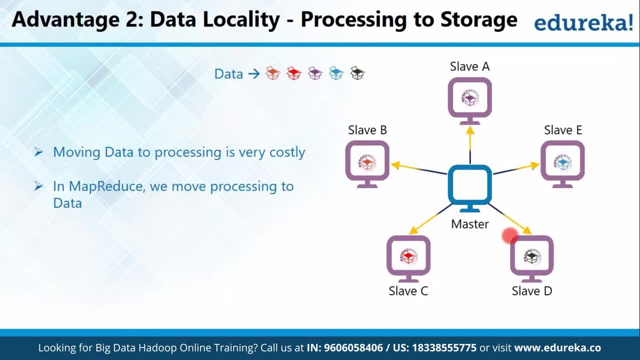 you are doing parallel processing. however, you are also moving the processing, the logic that you would like to execute over big data, into the respective slave nodes where the chunks of data are present, and hence you are also saving a lot of network bandwidth, Which is very beneficial. 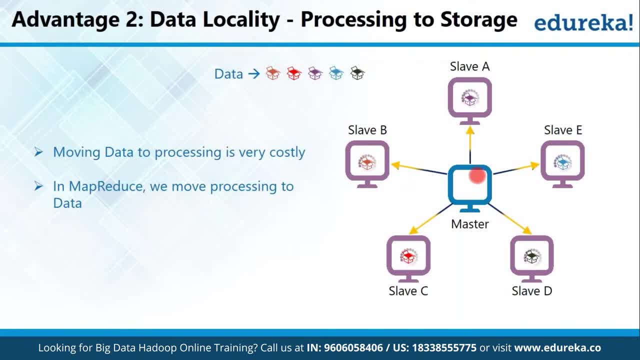 Finally, when the slave machines are done with the processing of the data that is stored at the slave machines, they send back the results to the master machine, because the results are not as big as the blocks that were stored on the slave machine. hence it will not be utilizing a lot of bandwidth. 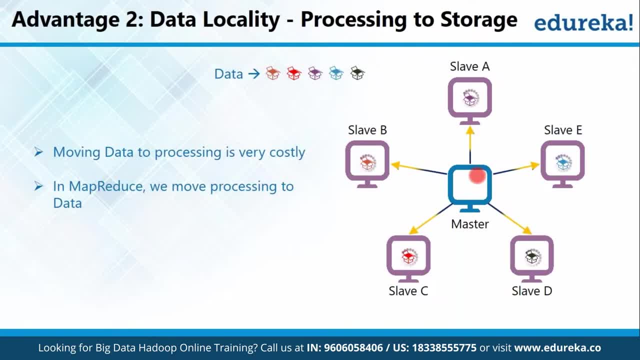 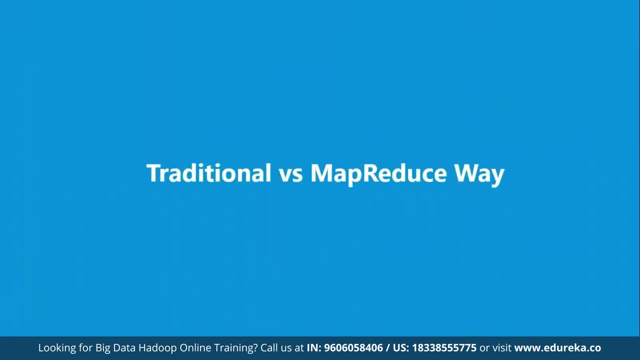 So what they do is they send the results back to the master machine, these results are aggregated together and the final result is sent back to the client machine which actually submitted the job. So we will move on to the next slide and we will explore the traditional versus the MapReduce way. 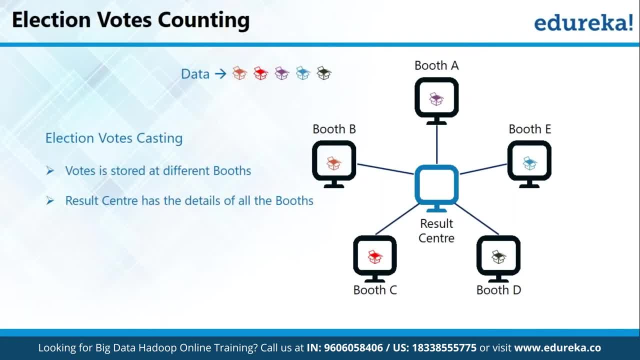 For this we will take a real life analogy of election votes counting. Everyone would be aware of elections, right? It happens everywhere, So you would be aware of votes as well. So votes are the location where people come and cast their votes, right. So there are n number of votes spread across the country, right? 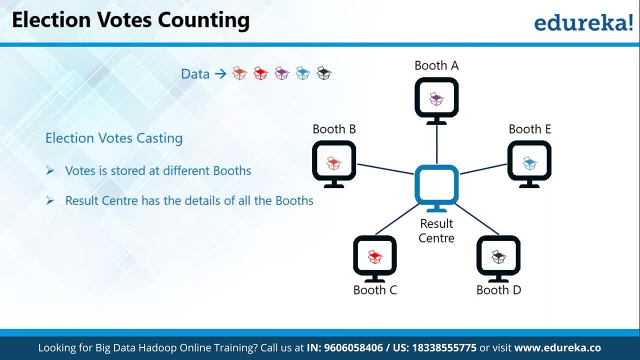 Let's take a scenario where we have 5 votes where people will go and cast their votes. Now we also have a result center which has all the information of the votes that are there and where they are located. However, when people come and cast their votes in these respective votes, 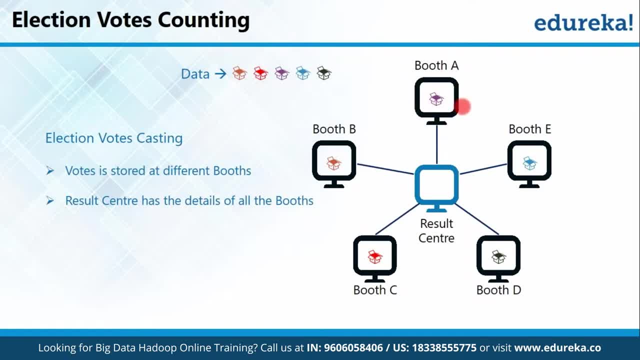 the votes are kept there itself. So in this case, both A will have its own n number of votes. both B will have n number of votes. both C will have n number of votes. similarly, both D and E will also have n number of votes that were casted there itself. 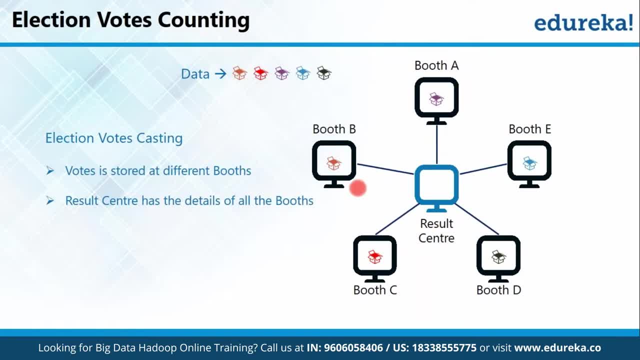 That information is not shared with the result center, right? So let's move on and let's see how does the vote counting will happen in the traditional fashion, So if you solve this problem using the traditional way, all these votes will be moved to a centralized result center. 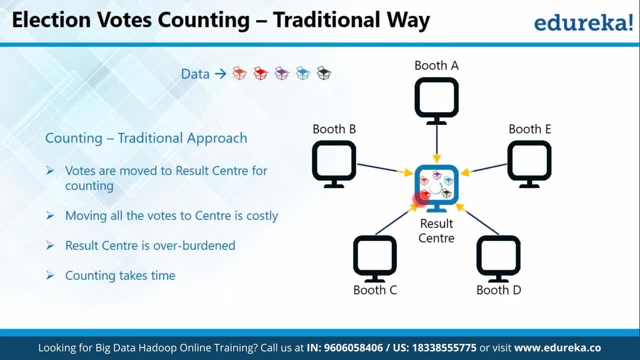 right here, and then the counting would start Now. in this case, if we do this, what happens is we need to move all the votes to a result center, which is a costly affair, right, That is, you will have to gather all the votes and move to a center location. 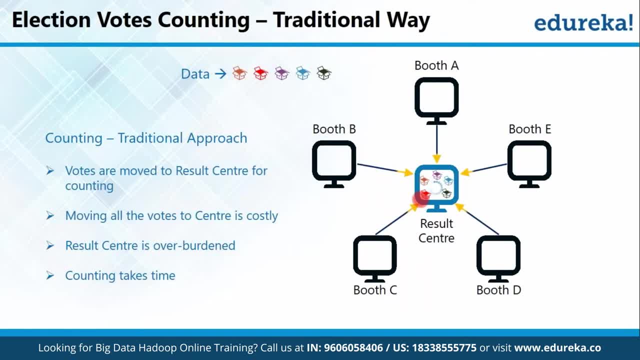 So there is a cost involved along with that, along with the effort right. Second point is: result center also gets overburdened because it has to count all the votes that were casted in these respective votes right, As well as, since they are counting votes that were casted in all the votes. 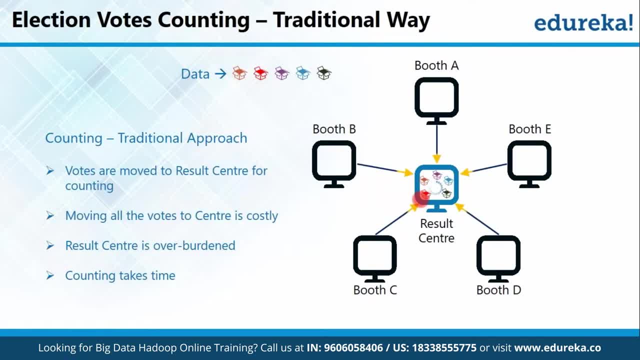 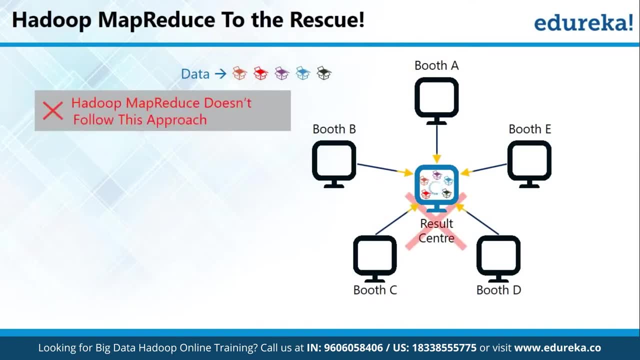 it is going to take a long time, So this process doesn't work very well. Let's see how does MapReduce solves this problem. So the very first thing is: MapReduce doesn't follow this approach. Now, when you see the MapReduce way, what happens is: 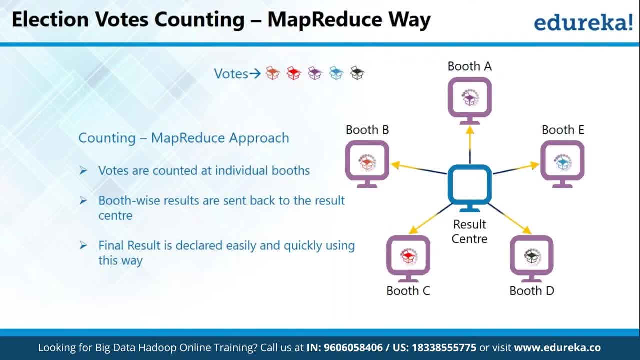 as you already learned in our previous slide, that is, MapReduce follows data locality, right? So that means it is not going to bring all the votes into a centralized result center. instead, it will do the counting in the respective votes itself in parallel, right? So what is happening is: 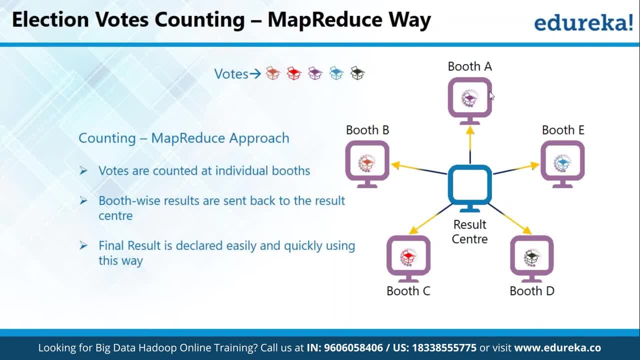 so once the votes that are casted on every vote are counted, they are sent back to the result center and the result center now only has to aggregate the results that was sent from respective votes and announce the winner. So this way, declaring the result becomes easy and very quick. 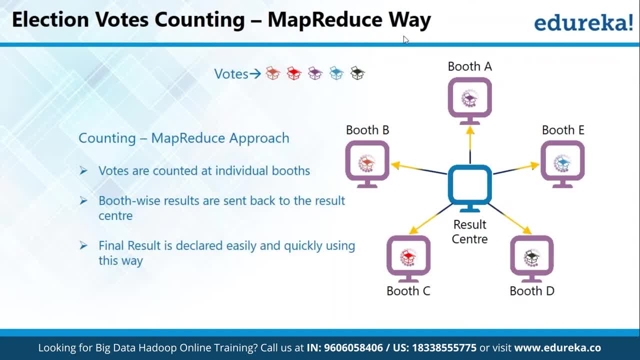 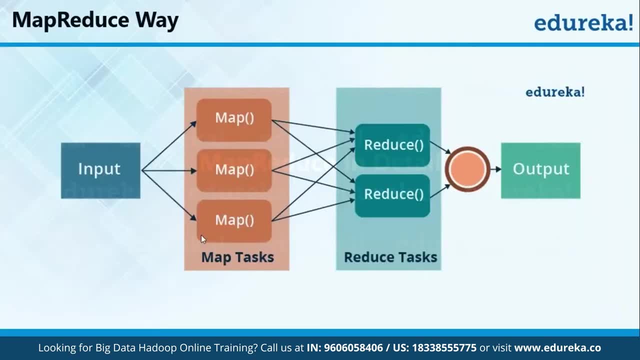 Otherwise I will move on to the next slide. Okay, let's move on Now. let's understand MapReduce in detail. Now, what did we do in the previous example? So we had an input and that input was distributed among various votes. Now, every input was processed by a respective map function. 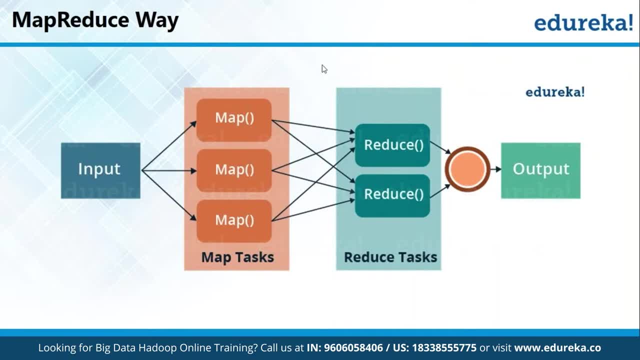 In the starting I told you that MapReduce has got two functions: one is map and the other is reduce. So the counting part that I talked about, which was done on the respective votes, was done by the map function. So every input at every vote was counted using the map function right here. 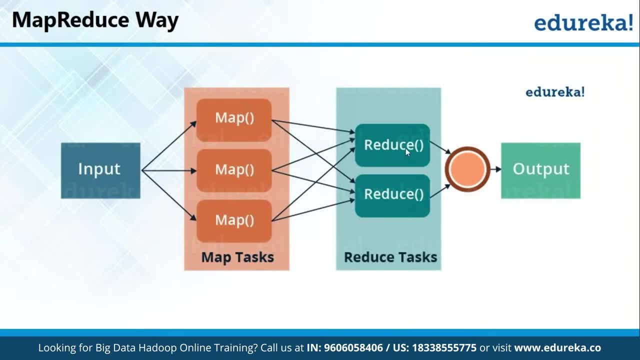 After that, the results were sent to the reduce function. so the aggregation part is done by the reduce function and the final result is given as the output. So this is what has happened in our previous example. Okay, so the entire thing can be divided into map task and reduce task. 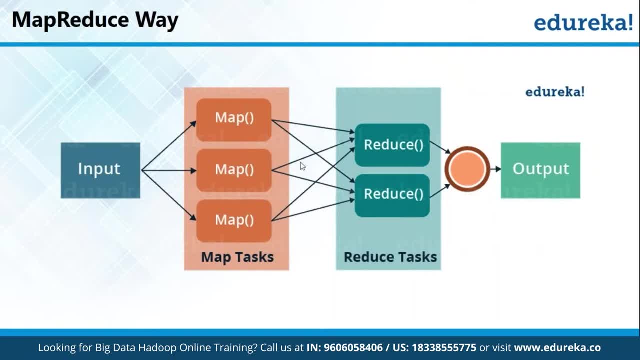 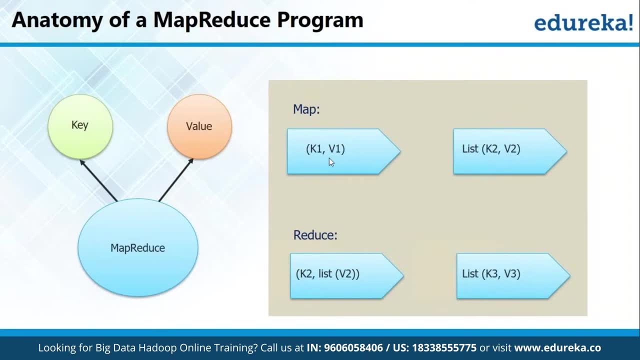 Map task gets an input. the output of the map task is given to the reduce task and this reduce task gives the output function Finally to the client. In this slide you will understand the anatomy of MapReduce. So what happens is a MapReduce task works on a key value pair. 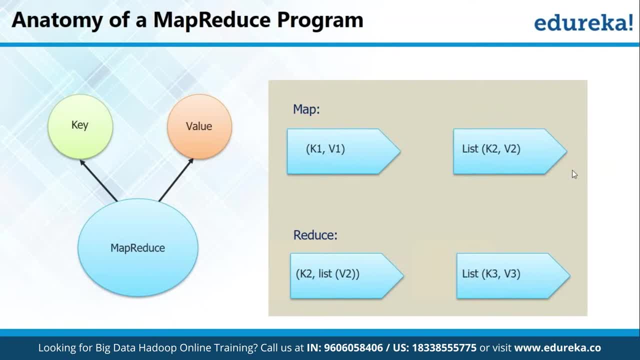 as you can see on the left. So when I talk about a map, a map takes the input as key value and gives an output as a list of key value. Now this list of key value goes through a shuffle phase and an input of key and a list of values is given to the reducer. 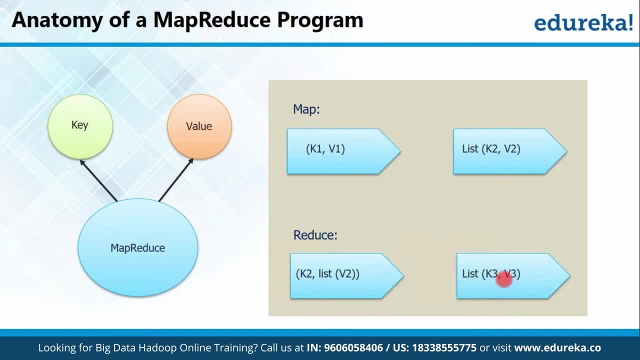 Finally, the reducer gives you a list of key value pairs. Okay, in this slide, what you need to understand is MapReduce works with key values itself and the remaining thing. we will be understanding this in the coming slides. We will move on to the next slide. 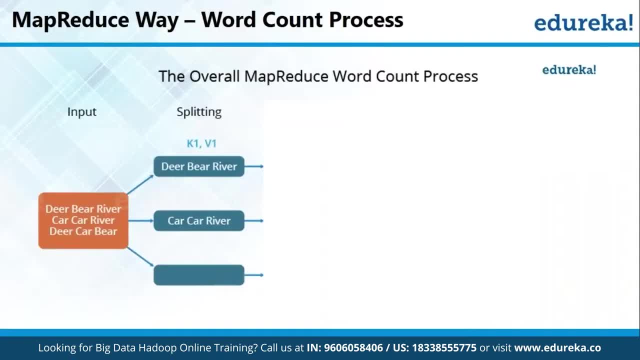 Now let us take an example to understand the MapReduce way. Okay, so we had an input. right, The input that you have gets divided or it gets splitted into various inputs. Okay, so that process is called input splitting, So the entire input gets divided into split. 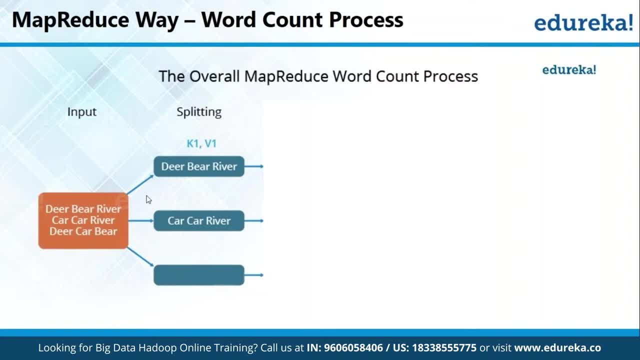 and splits of data on the basis of the new line character. The very first line is the first input, that is, deer, bear and river. The second line is the second input: car, car and river. Okay, it would be deer, car and bear. 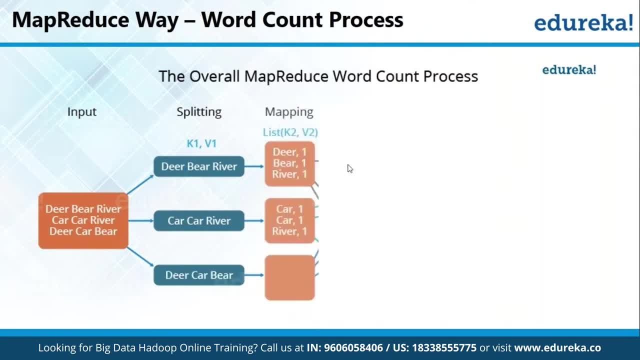 Now let us move on to the next phase, that is, the mapping phase. Now in the mapping phase, if you can see, what we do is we create a list of key value pairs. Okay, so the input is key and value, The key is nothing but the offset of the line number. 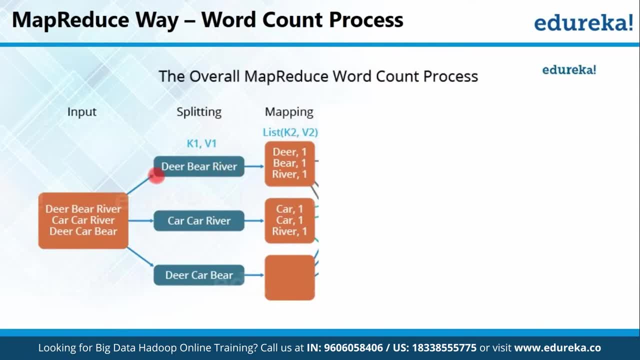 The line number is the key and the entire line is the value. Okay, so line 1, the offset, would be the key and the value would be deer, bear and river. In real life, the line number or the offset is actually a hexadecimal number. 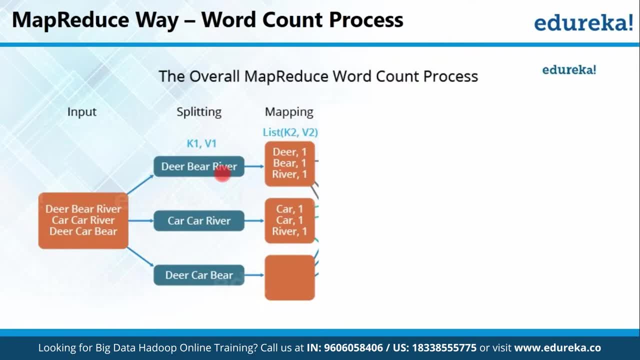 However, to make it easy, we will only consider it as 1 or 2, right? So line number 1 would be the key and this, the entire line, would be value. Okay, Now let us pass to the mapping function. What mapping function will do is it will create the list of key value pairs. 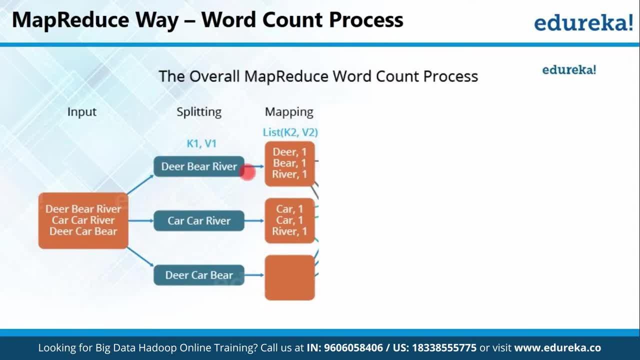 For example, deer. So what it will do is it will read every word from the line and it will mark 1 after the comma. Okay, it will mark 1 as a value. So deer comma 1, bear comma 1 and river comma 1.. 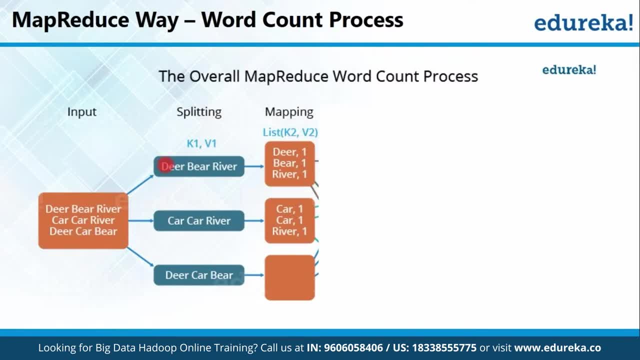 Why are we putting 1 after every word? It is because deer is 1 count, so deer comma 1.. Bear in itself is 1 count, so bear comma 1.. River in itself is again a 1 count, so river comma 1.. 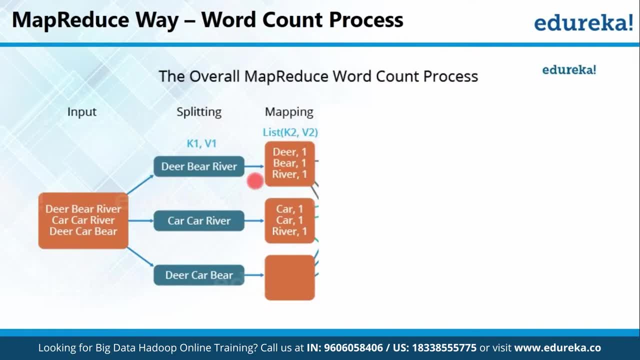 So we have key value pairs, that is, deer comma 1, bear comma 1 and river comma 1.. Similarly, when we come to the second line, we will read each word from the line that is car and we will mark 1 against it, because it is 1 count in itself. 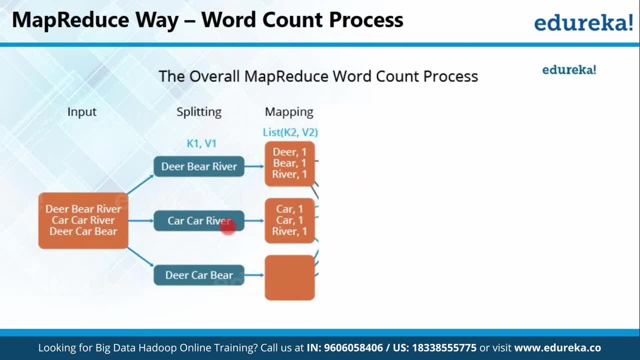 So car comma 1.. Again car, comma 1 and again river comma 1.. What will happen with the third line? What will be the result of the mapping function When this is the input? It is exactly the same, that is deer 1.. 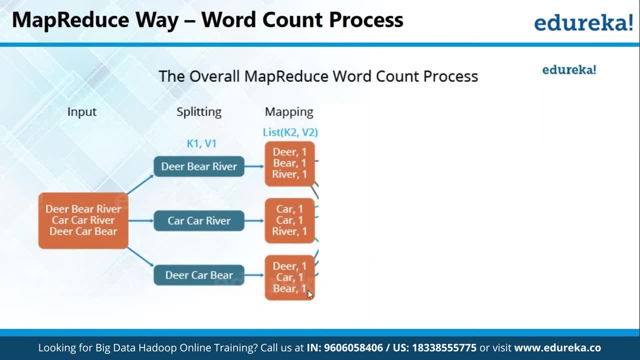 Deer is in itself 1.. Car in itself is 1 and bear in itself is 1.. Let's move on, and let's go on to the shuffling phase. So let's see what happens in shuffling phase. In shuffling phase, for every key there is a list prepared. 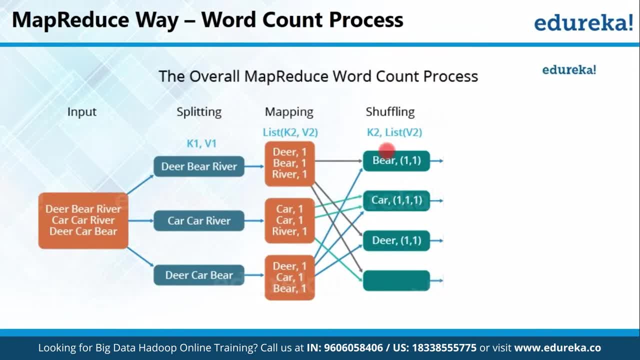 So k2 comma list v2.. For every key there is a list of values that will be prepared in shuffling phase. So what shuffling phase will do is so it will find the appearance of key bear and it will add the values into the list. 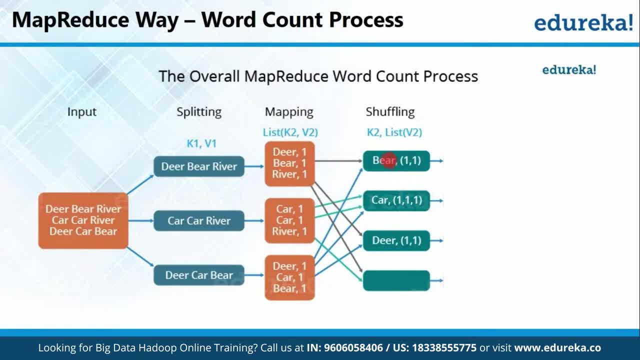 So let's see what is happening. You can see that there are two incoming arrows. The first arrow is coming from list 1. So bear, and then in the list it has added 1.. The other arrow was coming from this list, So bear, comma 1.. 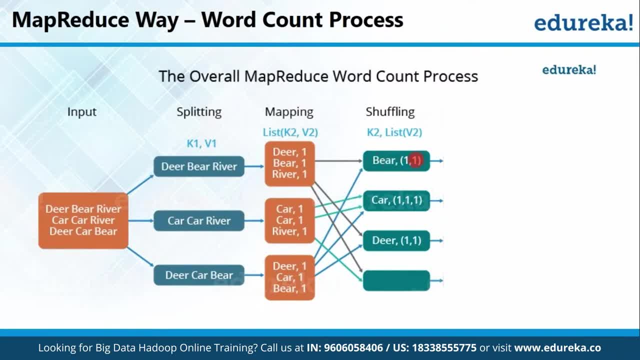 Again. so what it did? instead of adding another key, it just added the value 1 in the list of values part. So the result would be k2 comma list 1 comma 1, because there were two occurrences of bear in two different lists. Similarly, when I talk about car, 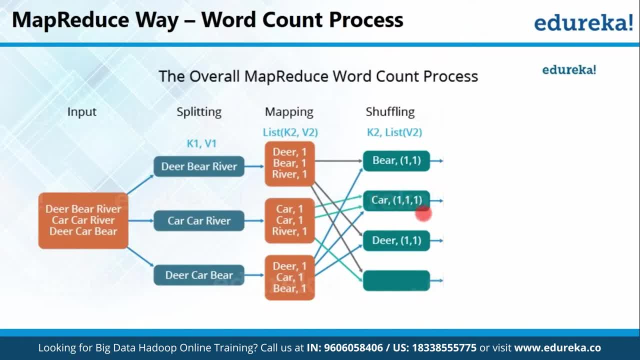 so, again for car, another list will be prepared for values. So, as you can see that there are three incoming arrows, Two arrows are coming from the same list, So car 1, comma 1, and the third arrow is coming from the last list, again comma 1.. 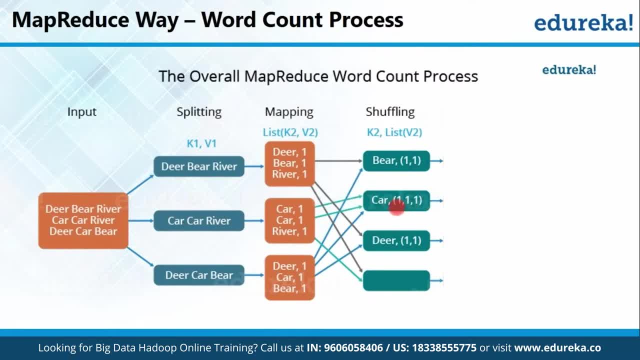 So since there were three occurrences of car, hence the list of values will have three ones: 1 comma, 1 comma 1.. Similarly goes with deer. Now, deer was there in the first list and the third list, Hence there were two occurrences, So deer, comma 1 and 1.. 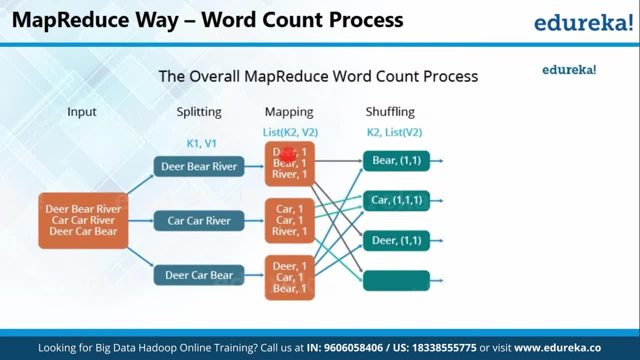 1 and 1 is nothing but the values that are against the respective keys in the map face. Can you tell me what will be the fourth answer? The answer would be river 1, comma 1.. It is because river was found in two different lists. 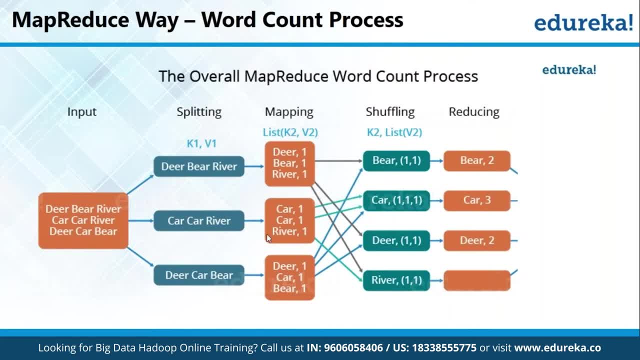 The first list: river 1.. So first occurrence, And then river. 2. So river and then the list of values. that is 1 comma 1.. Now comes the reducing phase. In reducing phase, what we are doing is we start aggregation of the values. 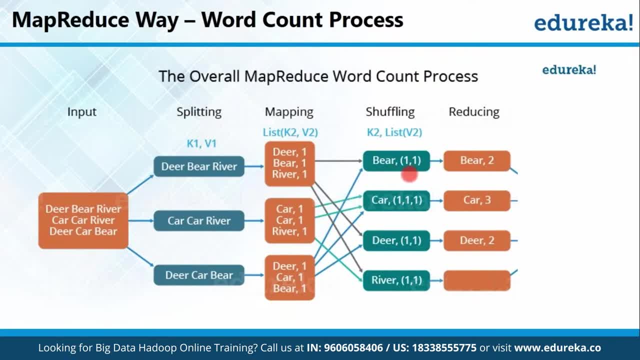 that were present in the list against every key. So for bear, there were two values present in the list: 1 comma 1. So the summation of these values will be done. So bear, comma 2.. Similarly, for car, the values will be summed. 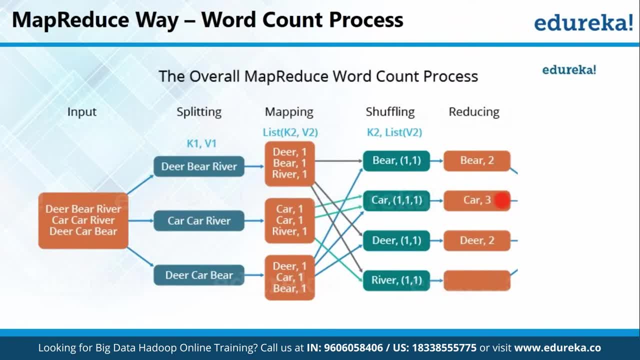 So 1 plus 1 plus 1 becomes 3.. Result from reducing function would be car 3.. For deer it becomes 1 plus 1, deer 2.. What will be the last answer? The answer would be river, comma 2.. 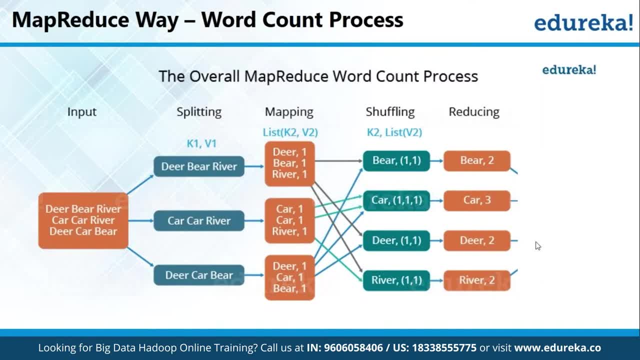 It is because the values are 1 and 1, and 1 plus 1 becomes 2.. So this will be the result for river And at last the final result will be sent back to the client with bear comma 2, car comma 3, deer comma 2 and river comma 2.. 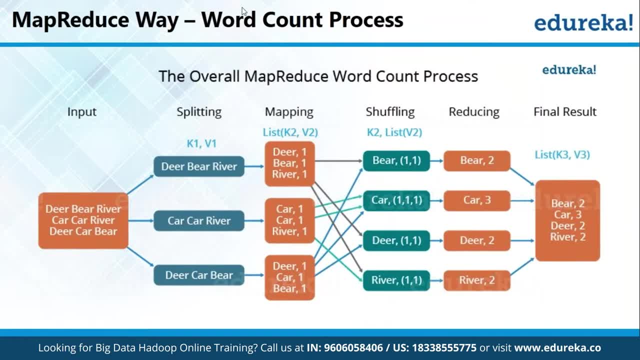 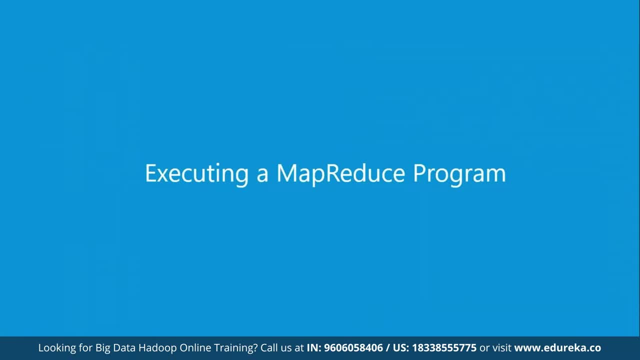 This is how the entire word count process works when you are using MapReduce way. Now let's execute this program practically. I showed you the entire process. Now let's execute this program. Execute a word count program over the same input file that we saw. 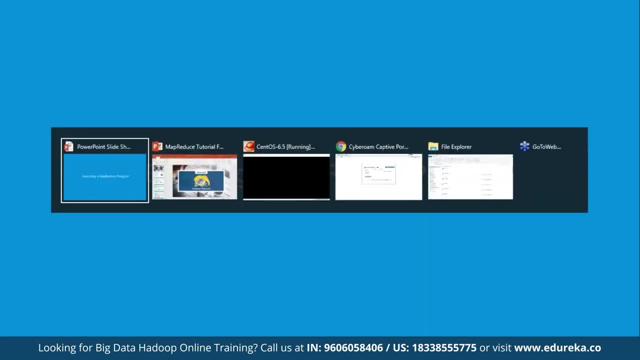 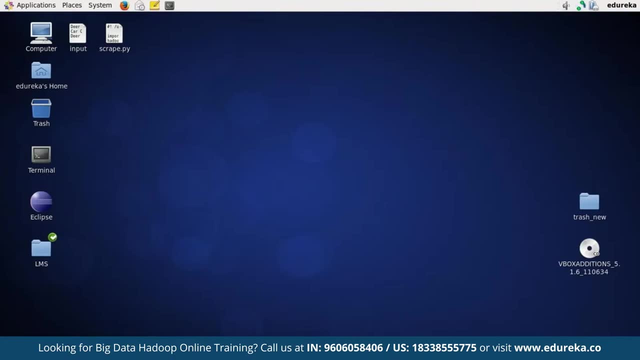 and see what is the result. So I'll enter the password. This is the Edureka virtual machine that you can download from your LMS. I am sure that the setup is already ready on your end, In case you are not ready with the program. 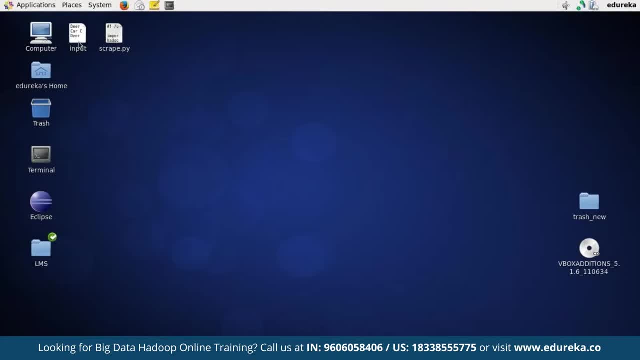 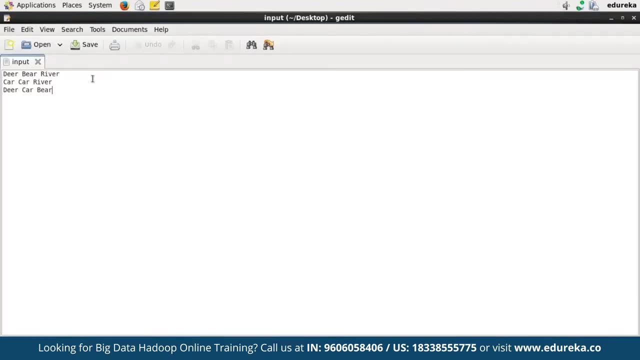 with the setup guys, please do that. So this is the input file that I have already created to save time. So this was the input in the example right: Deer bear river- car car river- deer car bear. 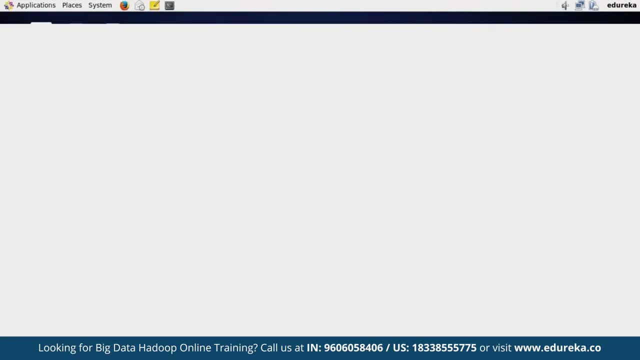 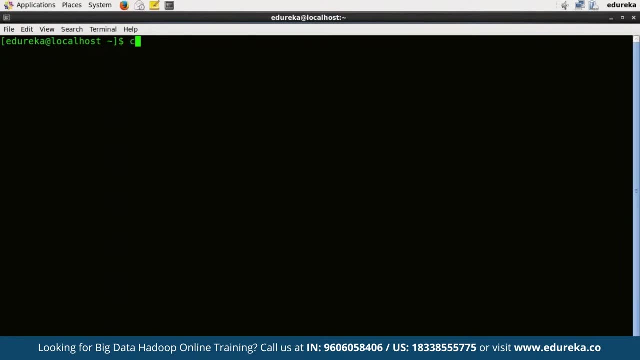 So what we are trying to do is execute a word count program over this. For your information, let me tell you that. so there are set of MapReduce example that already comes with the Hadoop package that you download, So let me just show you. 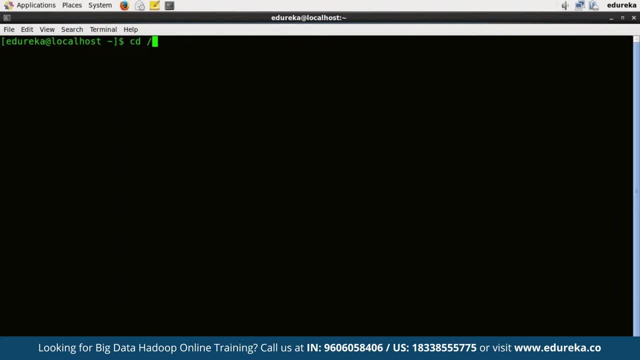 Even word count example is also a part of it, So I'll just take you there. My Hadoop is installed in userlabhadoop. Let us see the contents of this folder. The MapReduce example jar is present in the share folder. I'll just change the directory sharehadoop. 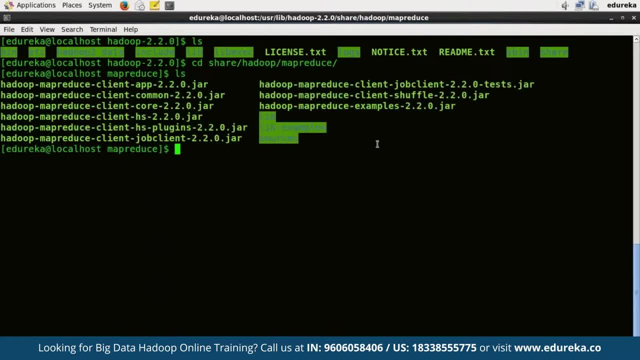 and we need to go to the MapReduce part. We'll find the jar in this. This is the jar that I am talking about, that is, Hadoop MapReduce examples jar. Let me show you the examples that are present in this jar. first, 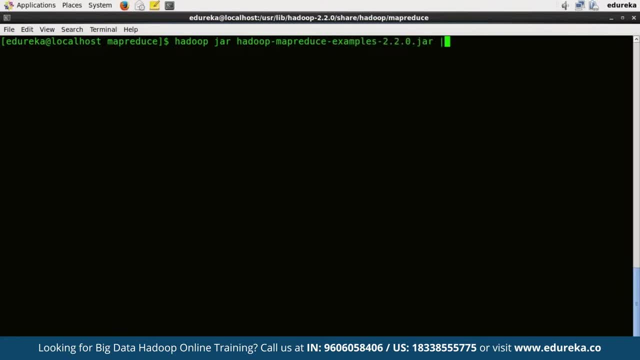 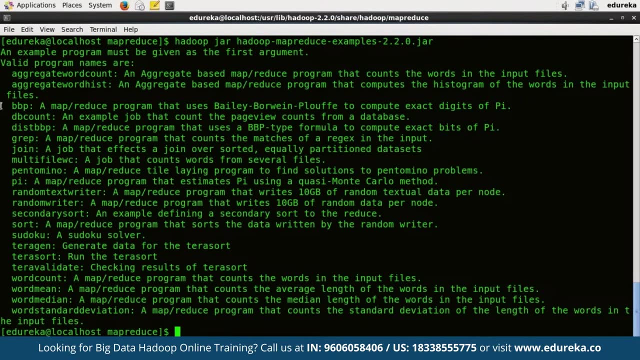 So Hadoop jar, Hadoop MapReduce examples 2.2.0.jar. So I'll execute this command. It will give me the list of all the classes, all the examples that are there within this jar. As you can see, one is aggregate word count, aggregate word list, bbp, along with the description. 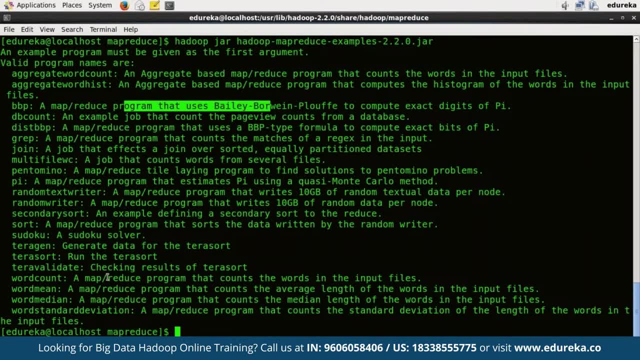 So you guys can go through this, Go through it and try all the examples. What we are going to try is the word count example: a MapReduce program that counts the words in the input files. So this is what we are going to execute now. 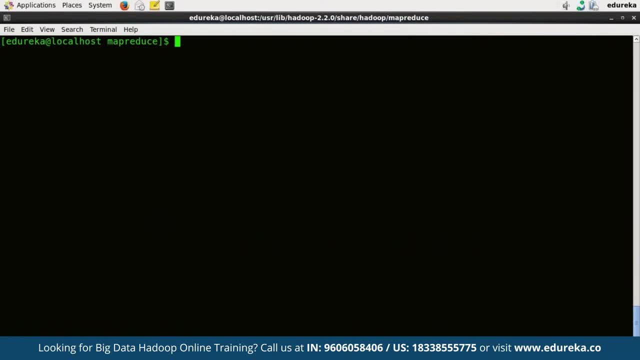 You can try other examples as well, As you have already seen the list of examples that is present in the Hadoop examples jar. Now it's time we execute the word count example, But before that we need to move the input file to HDFS first. 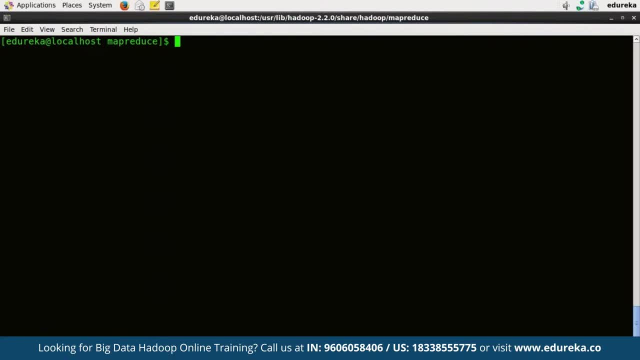 And then only we can execute the MapReduce example. It is because MapReduce takes the input from the HDFS and dumps the output to the HDFS. So very first thing is I'll move the file. So Hadoop DFS, that is, Hadoop, Distributed File System, hyphen put. 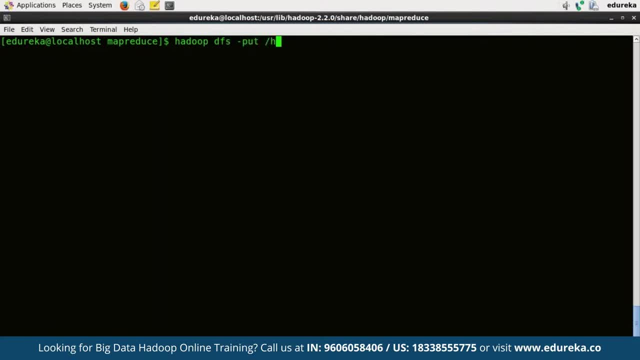 That is, I'm trying to put a file into HDFS. I'll give the path of my file that is present on my local file system, That is, home, edureka desktop, and then the name of the file input, And then I'll give the HDFS directory. 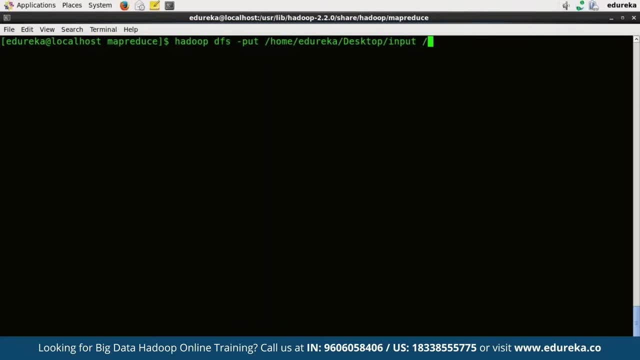 That is I would like to store on the root directory of HDFS. I'll press enter. I'm sure by now you would be very clear with the HDFS commands. In case you are not, I request you to please execute the HDFS commands that are present in the HDFS tutorial blog. 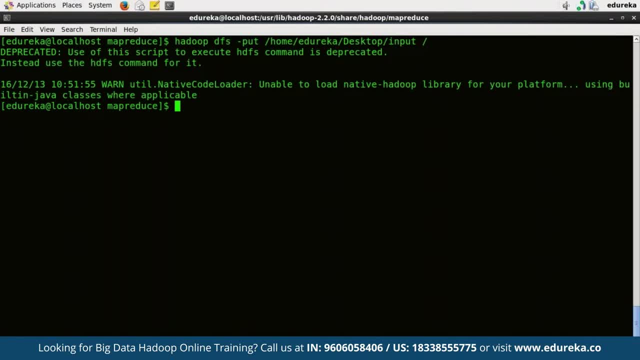 Or you also have a document in the LMS. So looks like a file has been copied to HDFS folder. Let me just check if it has been done. So, Hadoop DFS, I'll directly cat, That is, I'll read the file directly. 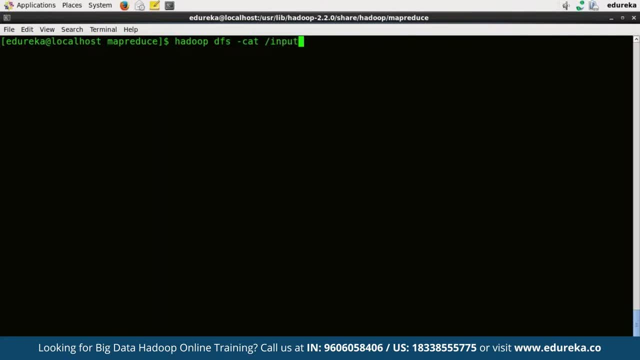 And I'll put the name of the file that is input. So I'm telling that go look for the file input that is present in the root directory of HDFS and read it. Okay, So this was the file that we copied, right, Good? 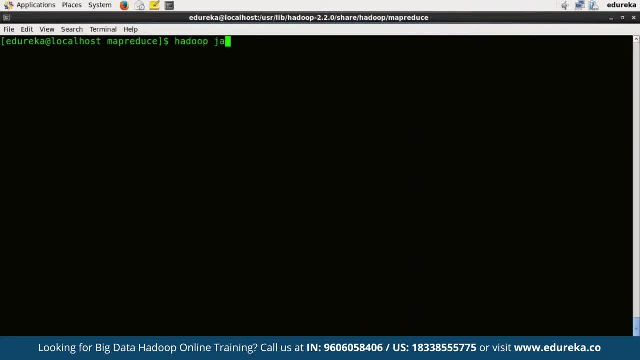 So let's execute the word count. example: I'll write Hadoop jar And I'll mention the name of the jar. That is Hadoop MapReduce examples jar. I'll mention the class That I want to execute. That is word count. 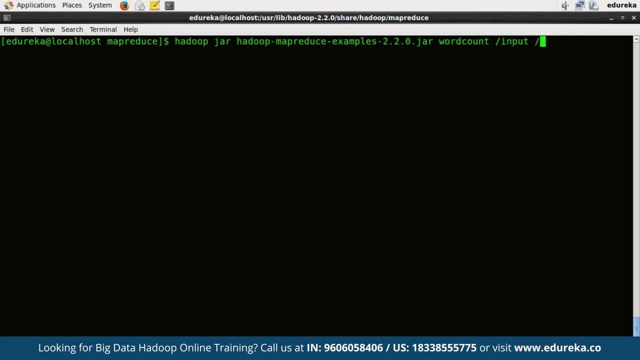 I'll give the input part of HDFS, That is backslash input, And then I'll mention the output directory. That is first example out And I'll press enter. So looks like it has started the execution. It is again connecting to resource manager. 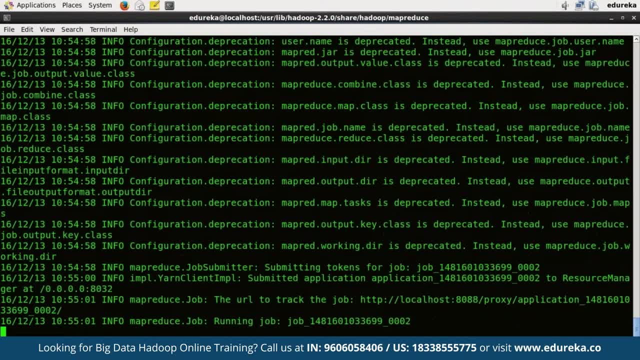 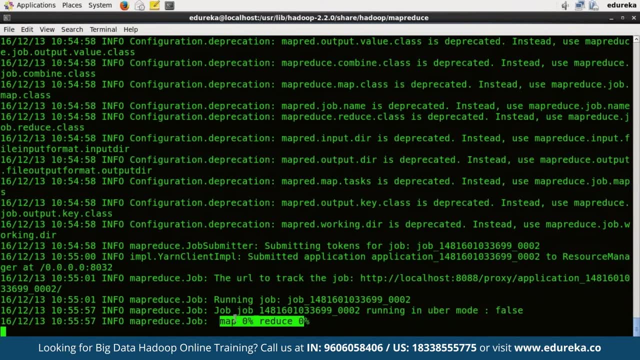 It is because the client submits the job to the resource manager. Right, Good, As you can see, the map and reduce task has started now. First, the map task would be executed. You can also track the status of your job at this particular location. 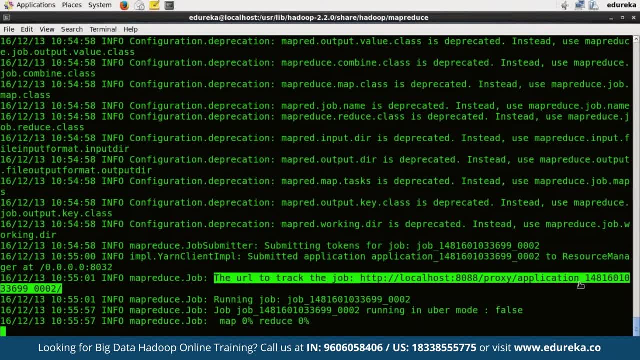 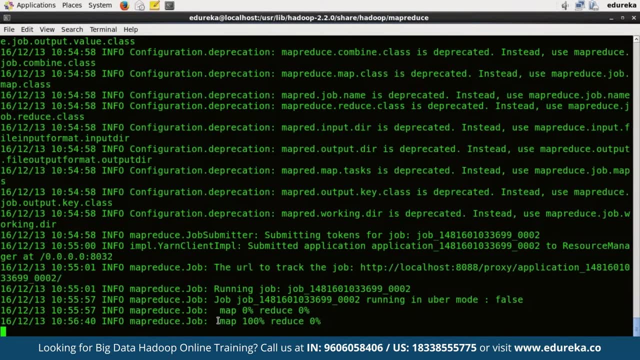 Okay, So for every job there is an ID- application ID- that is generated, So you can always go to port 8088, which is nothing but resource manager's port. Now, as you can see, the map has finished 100% And finally, the reduce phase would be executed. 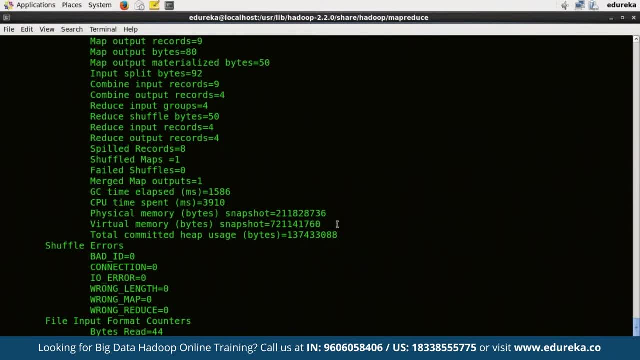 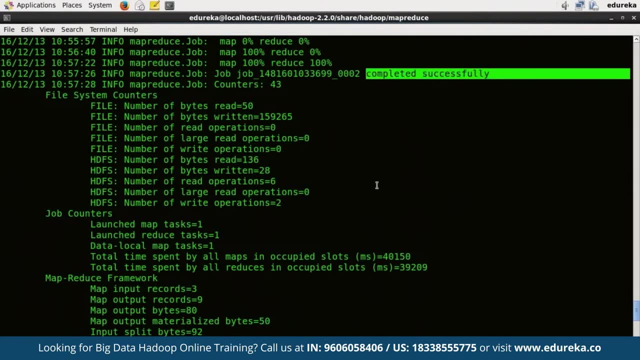 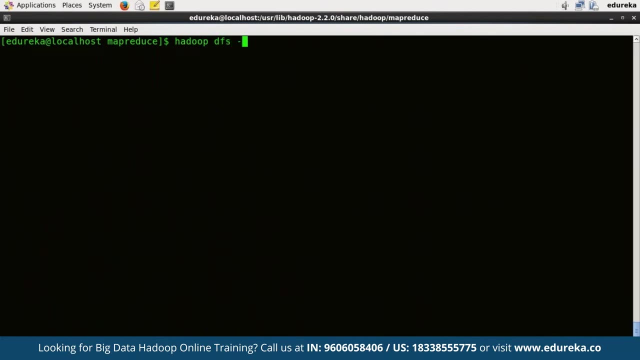 So reduce phase is also complete now. Now, finally, the job has executed successfully. Okay, As you can see, completed successfully. Let's go and check the output. Okay, I'll clear the screen. So Hadoop, DFS, hyphen LS and the name of the directory was first example out. 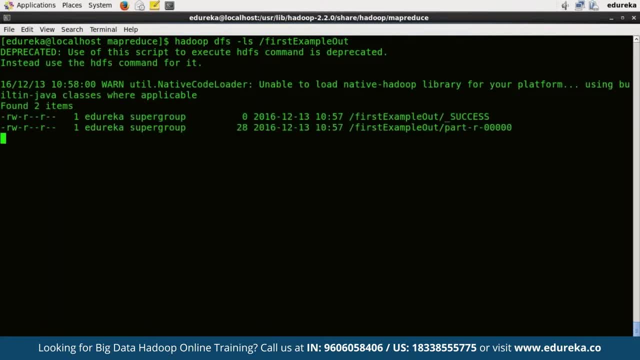 And enter. As you can see, there is a success file that has been created and a part file. The output is always present in the part files. Okay, So we'll just read the part file now Instead of LS. now I'll use the command cat. 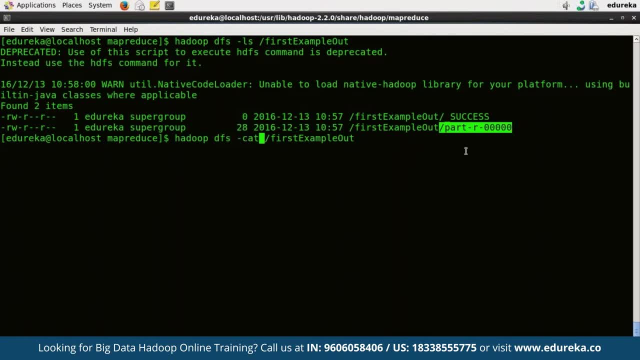 And I'll copy this part And I'll paste at the end of first example: output. Okay, And let's press enter. This is the command that I'm using to read the final part file, The output. So this is the output. 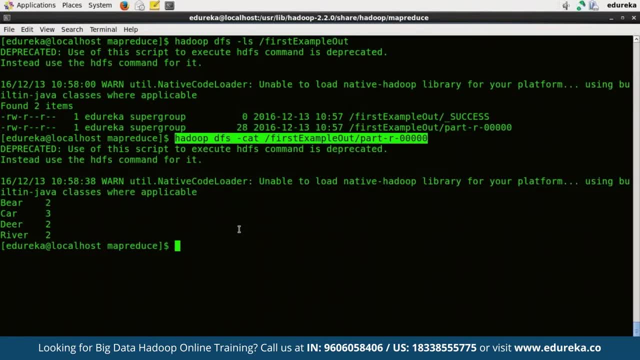 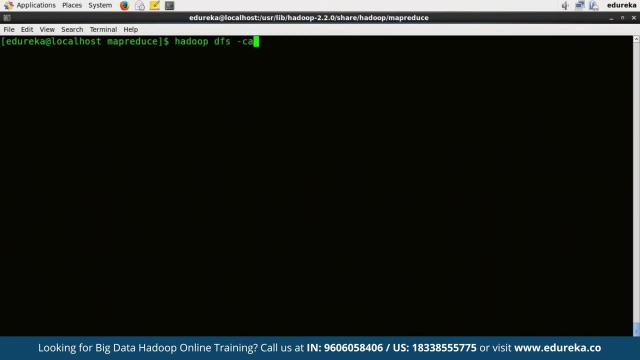 Beer 2, car 3, deer 2 and river 2.. Let's try and compare this with the input file itself. So first we'll read the input file: Hadoop DFS hyphen- cat backslash input Right. So this is the input file. 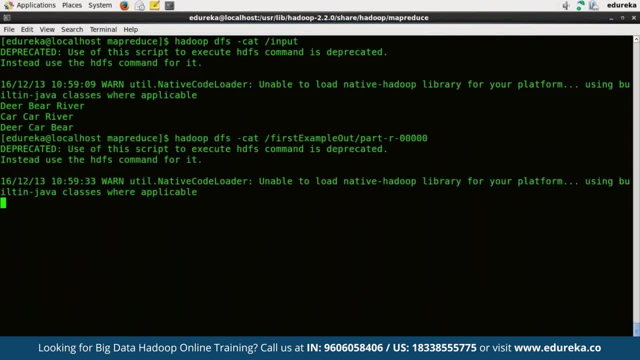 And now we'll read the output file again, The part file. Now, guys, can you compare? Is the result correct? Let's check Beer. It says it has come twice, So beer 1 and then beer 2.. Right Car has come thrice. 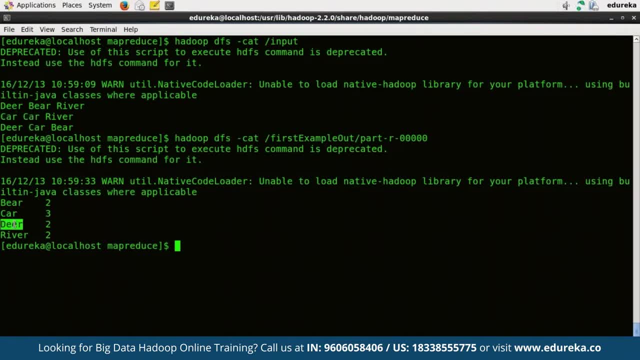 So car 1, 2 and 3.. Deer has come twice, So deer 1 and then second. Finally, river came twice So river 1 and river 2.. So we can see that the output that has been given by the word count example is absolutely correct. 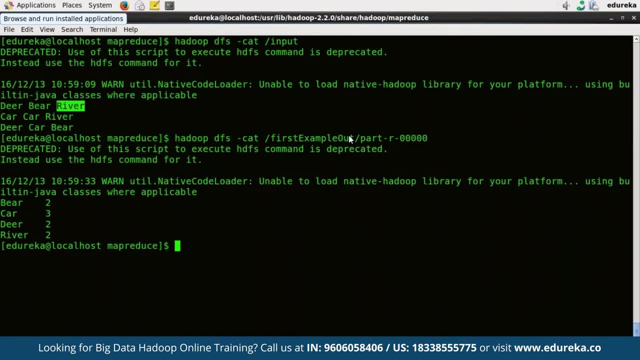 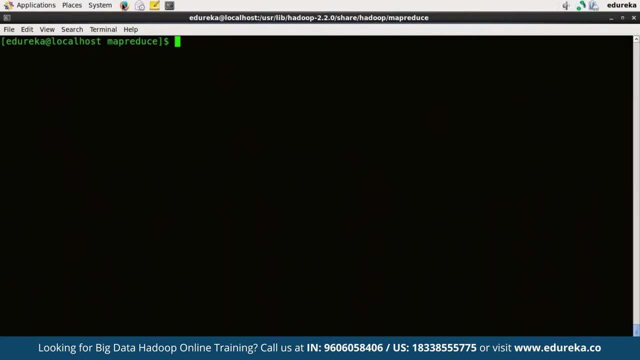 Now do you want me to execute the same word count example on a bigger file? Will that be interesting? Let me just show you So. for that, what I'll do is: let's open the browser first. Let's select the website. like Apache, Hadoop itself. 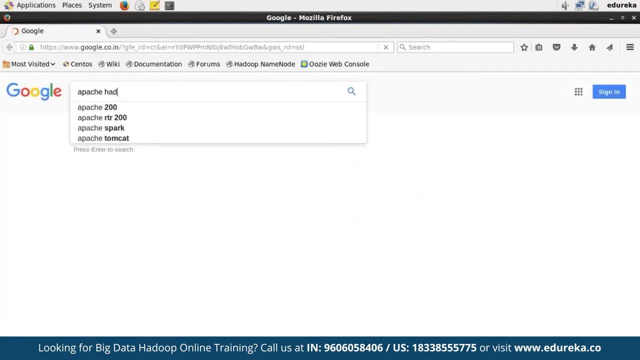 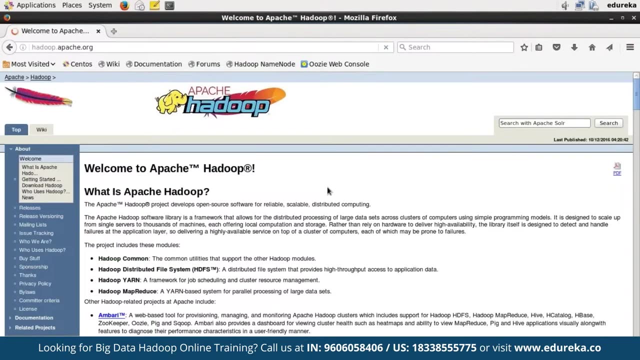 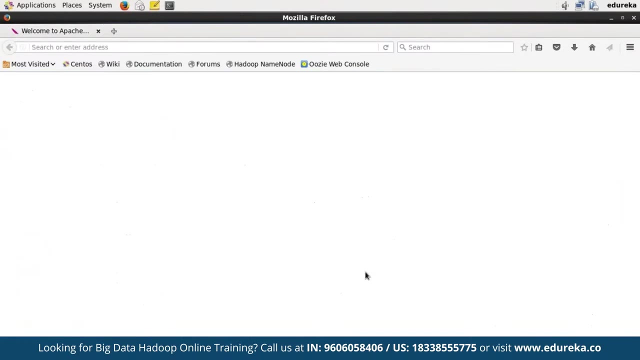 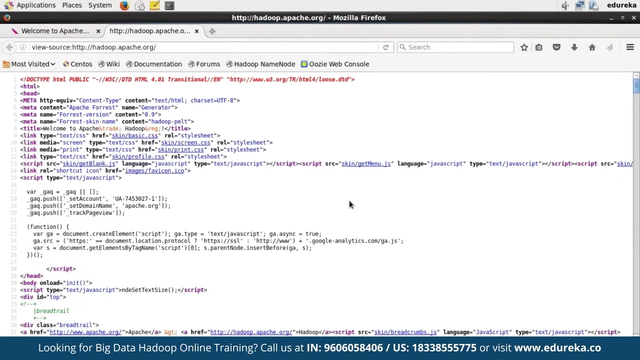 Okay, So let's open Apache Hadoop. Apache Hadoop, So we'll open this website. So, as you can see, there's multiple words there. Let me open the source file of this page. I'll go to view page source. So how about running the MapReduce program on this page source and find out the frequency? 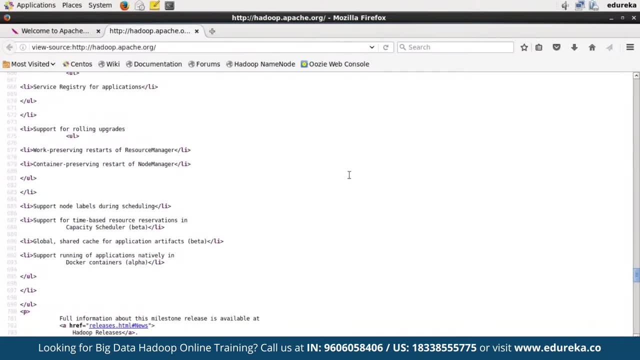 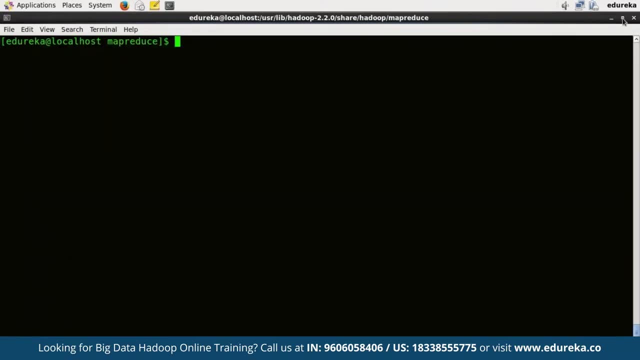 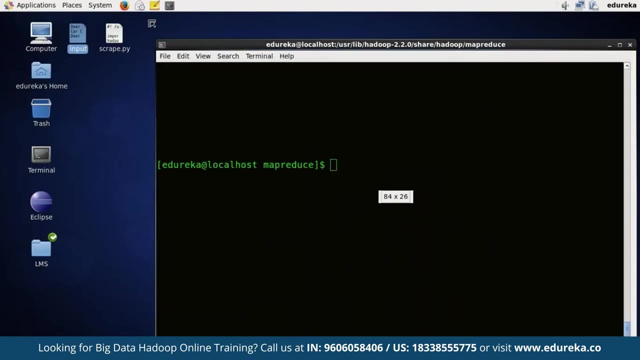 of every word that is coming in this page. Will that be something you would like to see? Good? So what I've done is I've written a small Python script. Okay, I'll just show you Using that Python script. I'm trying to scrape the page that we have just opened, that is Apache Hadoop org. 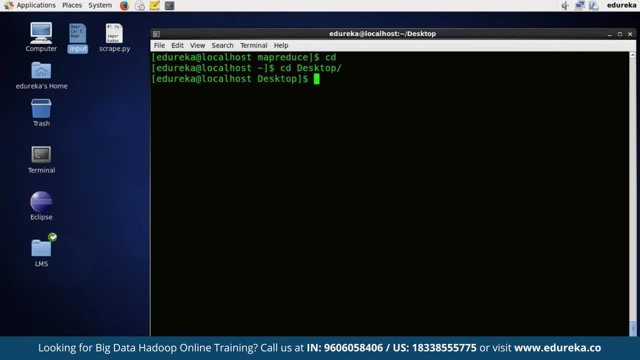 Okay, So I'll just change my directory to desktop. first I'll clear the screen. So the name of the script is scrapepy. Since it is a Python script, its extension is scrapepy. I'll open the file scrapepy. So in this just I'm telling that this is where my Python is located. 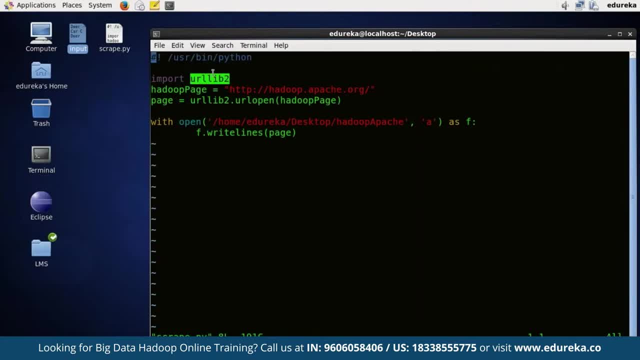 I'm importing a library and that is called urllib2.. The page that I would like to scrape is http- Hadoop dot Apache dot org. That I've already shown you. now, Using this command that is urllib2 dot url, open Hadoop page. 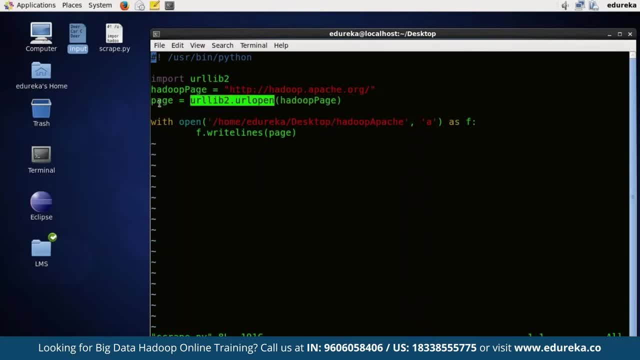 I'm able to fetch the entire source code of this page in one variable that is called page. And then, finally, I'm writing this page variable- the content of this page variable- in a file that is called Hadoop Apache. Okay, That will be created on the desktop. 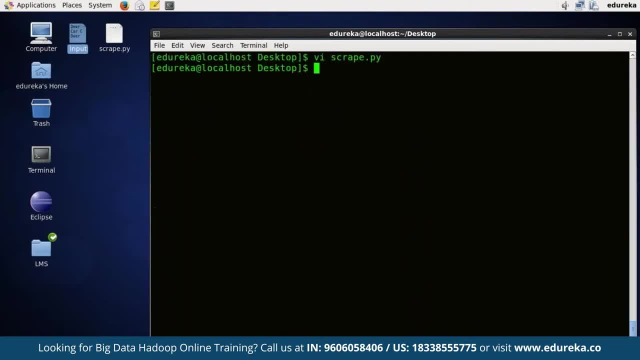 Okay, Very simple script. I'll just save the file And I'll execute the script by a dot backslash scrapepy. So you'll see that there will be a file that will get created once this script is finished. So right here. 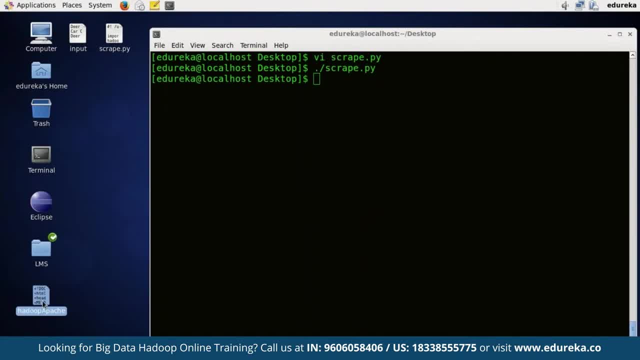 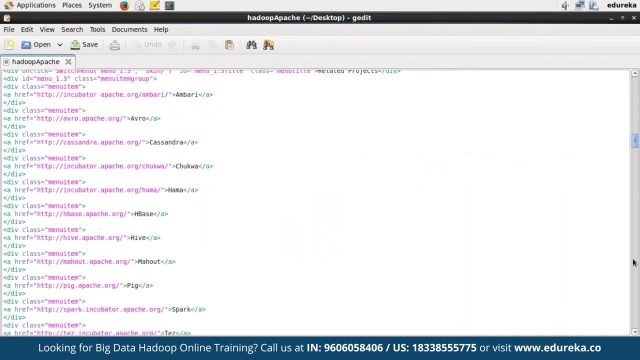 As you can see, Hadoop Apache is the file that has been created. I can open it for you, So it has the entire source code that was there in the Apache's website, Right Interesting. Now what I'll do is I'll execute the same word count, example. 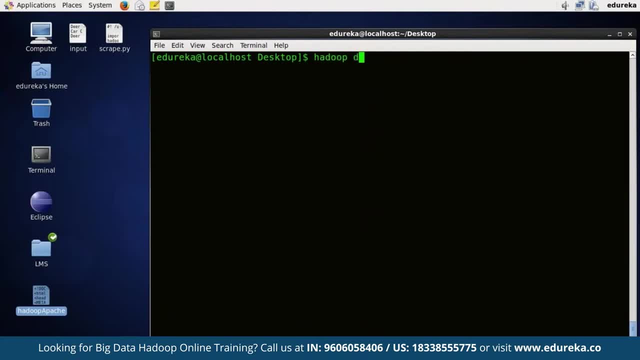 But before that I need to move the file into Hadoop HDFS, Right, I hope you remember. So I'll do: Hadoop DFS, hyphen put: I'll give the path of this file, that is Hadoop Apache, the local path, And then I'll mention backslash, that is, I would like to move this file to the root directory of Hadoop. 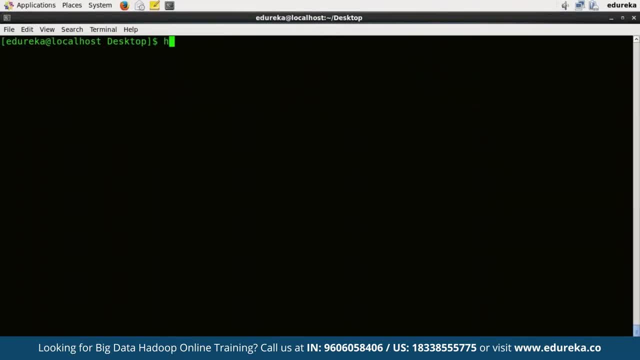 Okay, I'll make the terminal full screen now. Now the file has been copied. Now I'll execute the word count example on this. So I'll do jar. I need to give the entire path where my jar is located. That is user. 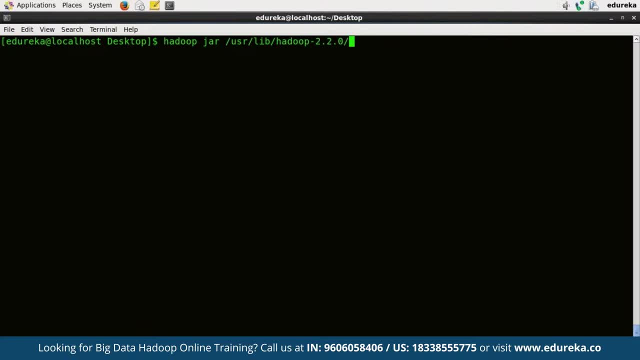 Lib Hadoop Within that share folder, Hadoop, MapReduce, And then there will be the Hadoop MapReduce example jar. Next I need to mention the class I would like to execute. that is word count. Now I'll mention the name of the input file that is present on HDFS. 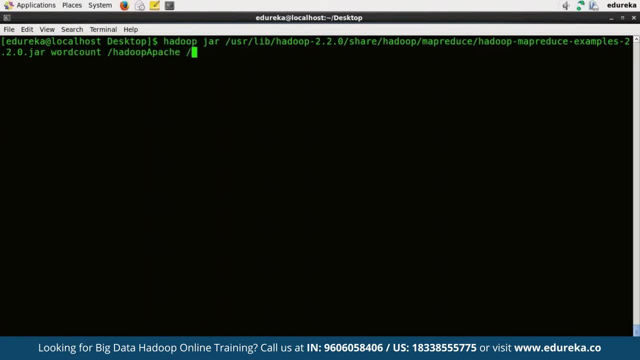 That is Hadoop Apache, And I'll give the name of the output directory where I would like to store the final result of this MapReduce program And I'll name it as second example out. Okay, And let's press enter. As you can see, it's connecting to resource manager again. 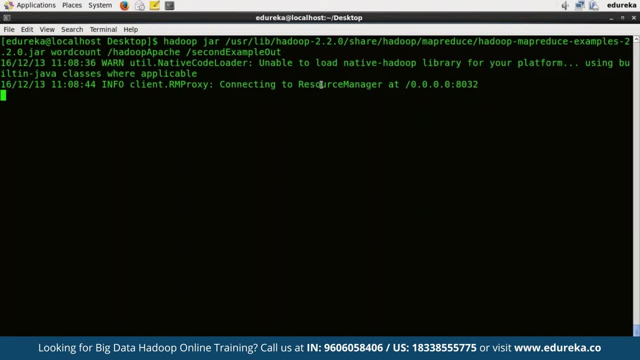 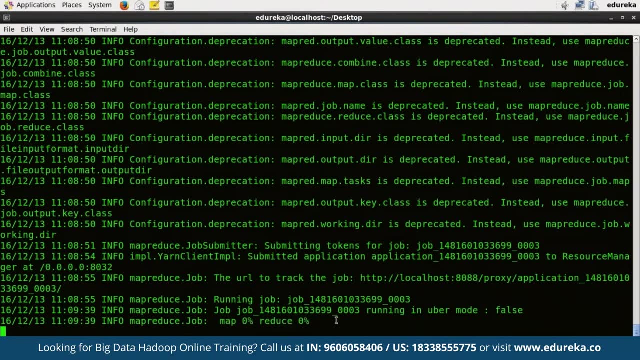 It is because it is somebody who executes all your jobs that are submitted from the client. So the MapReduce task has started now, As you can see, Which will be the first phase that will get executed, guys, Is it Map or Reduce. It will be Map itself. 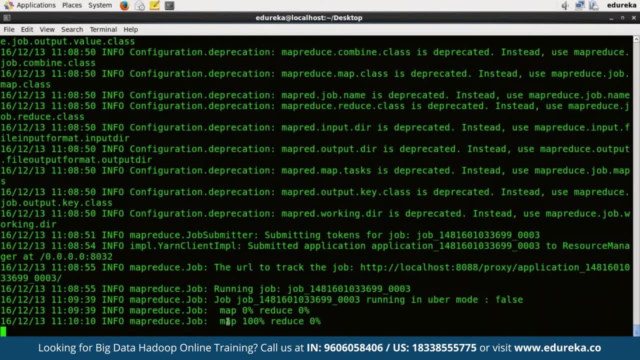 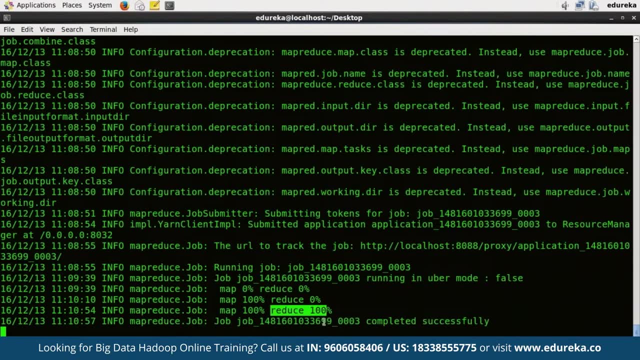 Okay, I hope everyone is very clear that Map will get executed first. So, as you can see, Map has executed now. Even the Reduce phase is also over, As you can see, And we have the results written on HDFS. I'll clear the screen. 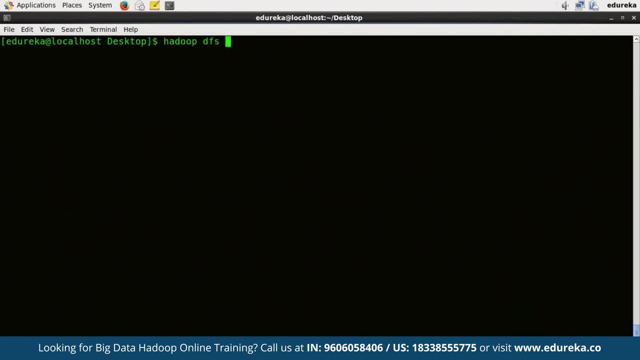 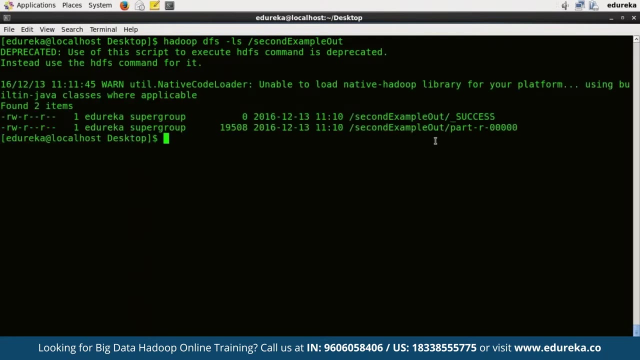 So let's check the results quickly. So Hadoop DFS hyphen LS. The output directory was second example out And we'll find the part files within it Which will have the final output. So, as you can see, this is the part file. 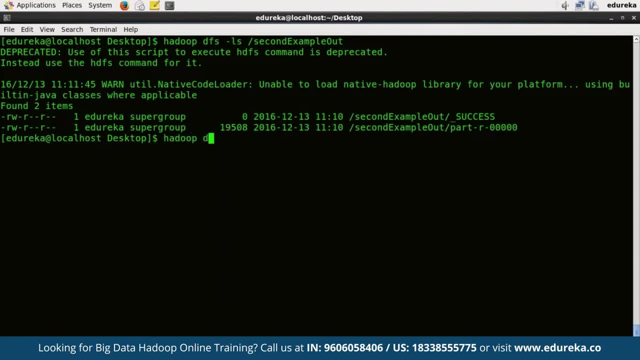 Let's try and cat it. Okay, So Hadoop DFS hyphen cat. I need to mention the entire part. I'll copy this And paste And enter. It will be a huge file. It is because the number of words that were present in the file was more than the previous input that we gave. 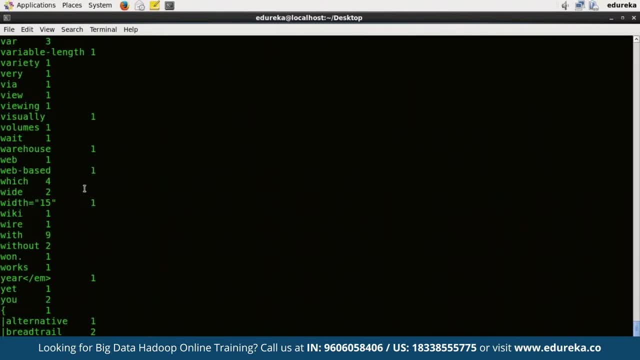 Right. As you can see, for every character, every word that was there in the file, You have the word count, Right. So let me just clear this. So let's try and find out the count for Hadoop. Okay, So I'll simply execute a Linux command, that is grep Hadoop. 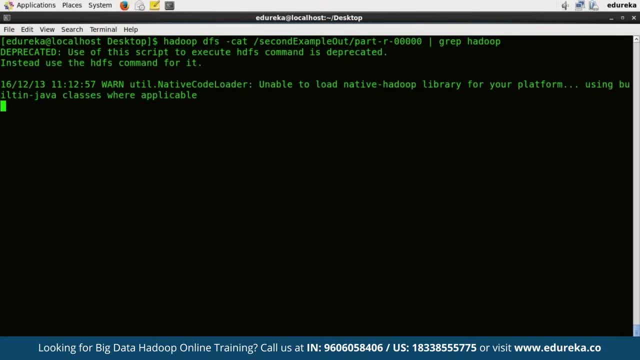 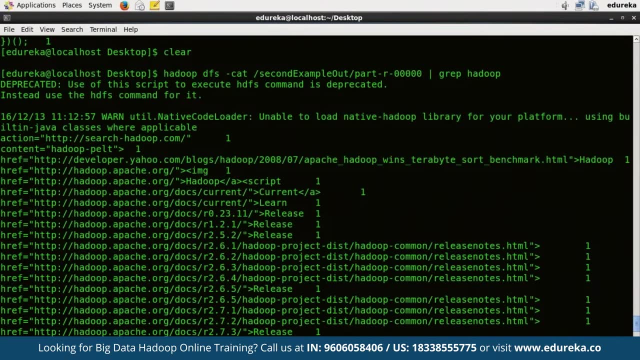 On the output that will be received from after reading the file. I'll simply look for the word Hadoop. So Hadoop came into so many words, as you can see Right here. So this is the command that I executed, And here is the result. 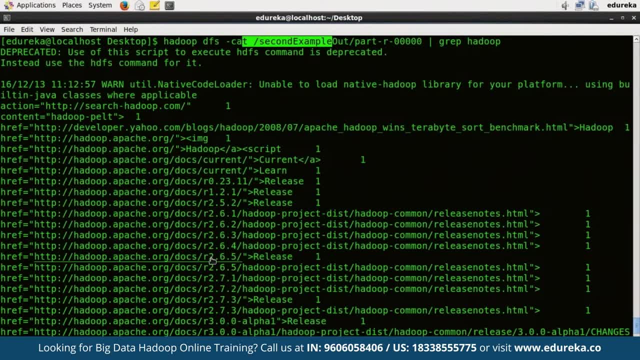 Okay, So since this was the source code, it is a little messy. However, when you're working with real data set, you'll be cleaning that data set first and then only you'll be executing your final processing. Okay, Even for cleaning, you'll be writing a MapReduce program. 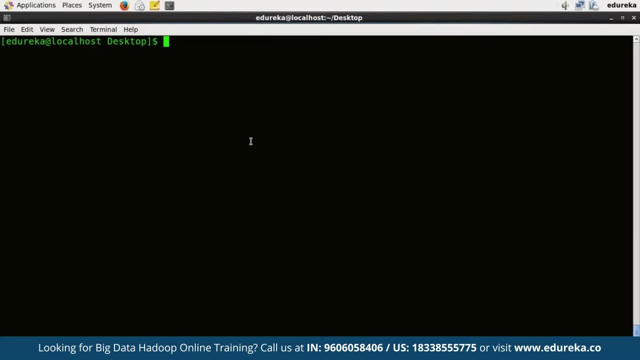 Okay, So how did you like the example? Matthew already says that, wow, that's a great example to observe. It gives the taste of real data set. Okay, So let's try and see how it works. Okay, So let's try and see how it works. 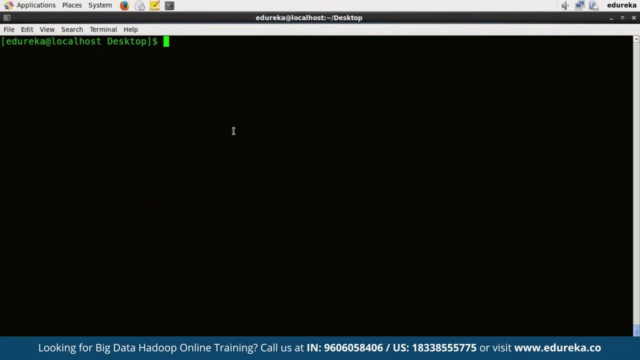 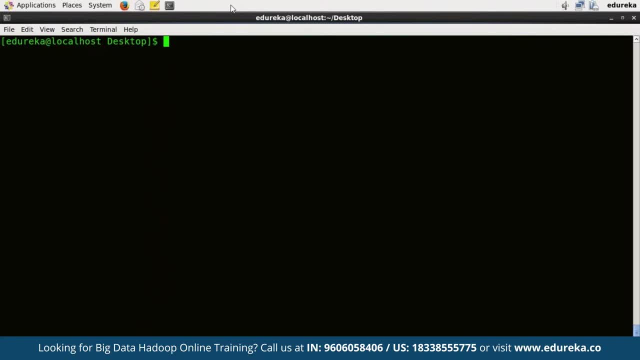 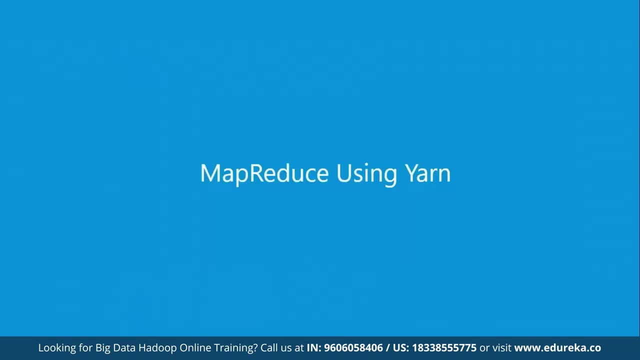 Okay, There are a lot of other things that can be done using MapReduce, because the limit of MapReduce is endless. Okay, Let's go back to our lives now. Now let's understand how MapReduce is using Yarn to execute the jobs over the cluster. 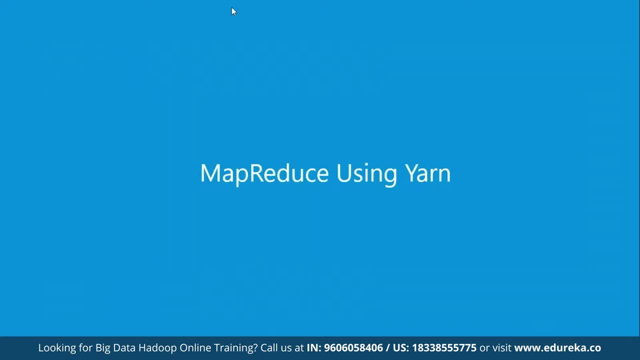 But before we go ahead, Okay, what does YARN stand for? Yet another resource negotiator. It is the one which allocates the resources for various jobs that needs to be executed over the Hadoop cluster. It was introduced in Hadoop 2.0 itself Till Hadoop 1.0 MapReduce was. 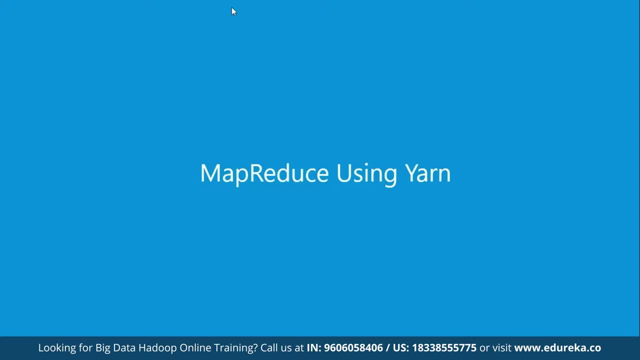 the only framework or only processing unit that can execute over the Hadoop cluster. However, in Hadoop 2.0, YARN was introduced, using which we were able to go beyond MapReduce as well, as you can see in this slide. So we have HDFS. 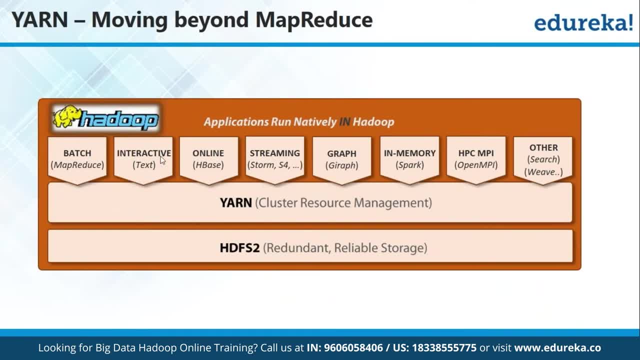 in the bottom. in between we have got YARN and using YARN lot of frameworks are able to connect and utilize HDFS. So now even MapReduce has to connect using YARN, request for resources and then only it can execute the job over HDFS. that is Hadoop cluster. Similarly, Spark can connect other 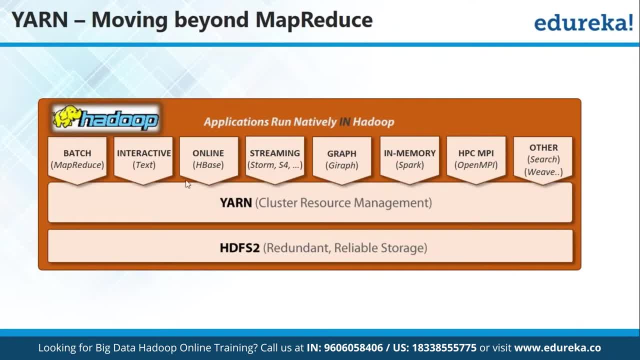 search engines can connect to HDFS, Storm can connect to it, HBase, which is a NoSQL database, which can connect to it. So the applications of HDFS became huge just because YARN was able to open the gates for other frameworks, other big data analytics tools as well. Let's move on. Let's talk. 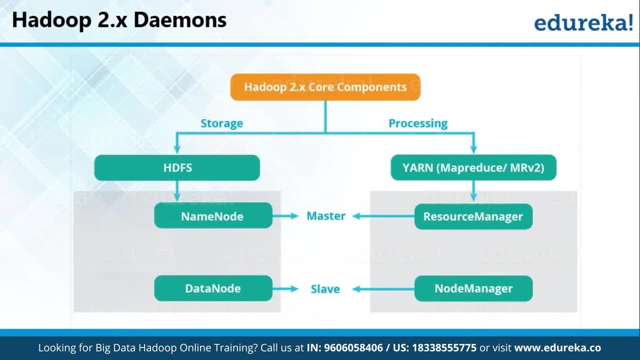 about the demons present in Hadoop 2.x cluster, which runs the components, that is, storage and processing. Let's understand: how does resource manager and node manager works in Hadoop 2.x cluster and manages the processing and the job that needs to be done? 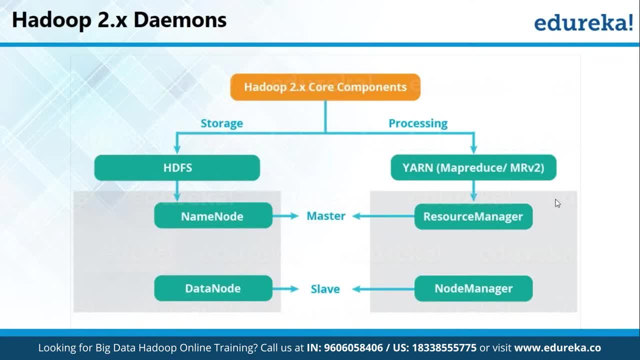 Executed over the Hadoop cluster. So what is resource manager? Resource manager is the master demon that runs on the master machine, which is a high-end machine. Node manager, on the other hand, is the demon that runs on the slave machines or the data nodes, along with the data node process. 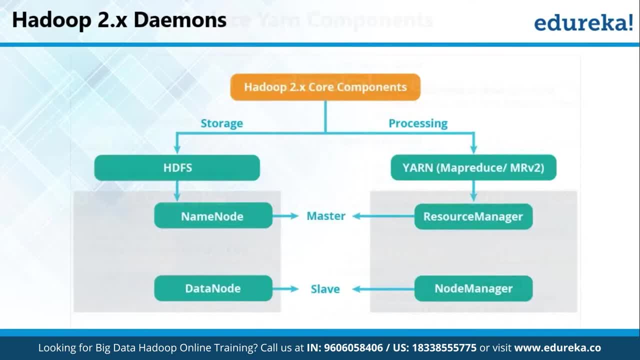 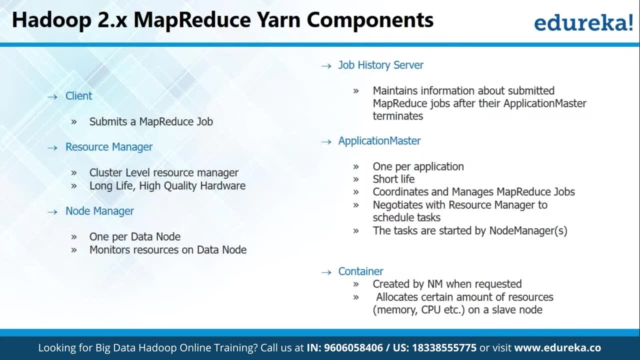 Let's understand this in a little more detail and explore other components as well. So what is a client? A client is nothing, but with some it's a MapReduce job, like we did from the CLI. okay, that is command line interface, So it is also a client using which we 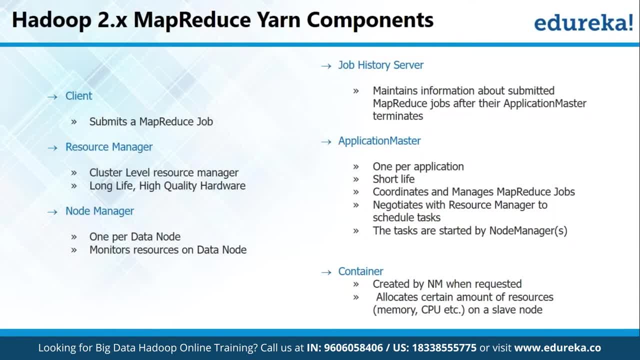 were able to submit the MapReduce job. Okay, so it is a client. Similarly, a client could be a Java application or anything. Now, what is a resource manager? Resource manager, as I said, is the master demon to which all the jobs are submitted from the client. It is the one which allocates all the cluster level. 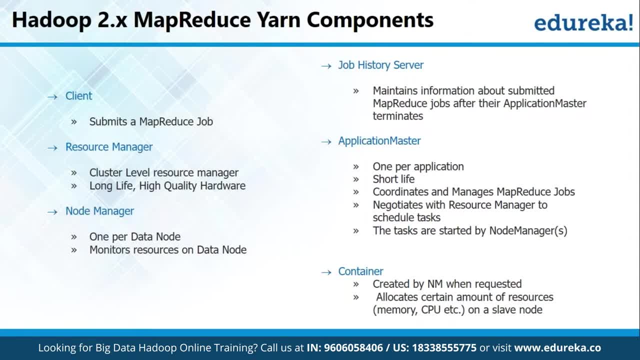 resources for executing a particular job. The source manager runs on a machine which is actually a high-end machine with good configuration, because it is the master machine which has to manage everything over the cluster. What is node manager? Node manager is a slave demon that runs on the slave machines or the data nodes. Every slave machine will. 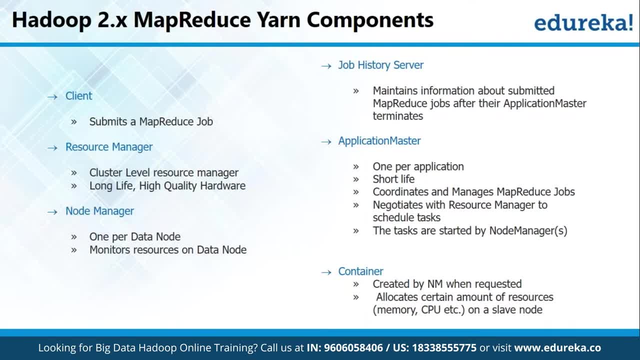 have a node manager running. It monitors the resources of a particular data node Resource. manager manages the cluster resources and Node Manager manages the data node resources. So what is job history server? It is someone who keeps a track of all the jobs that has been executed. 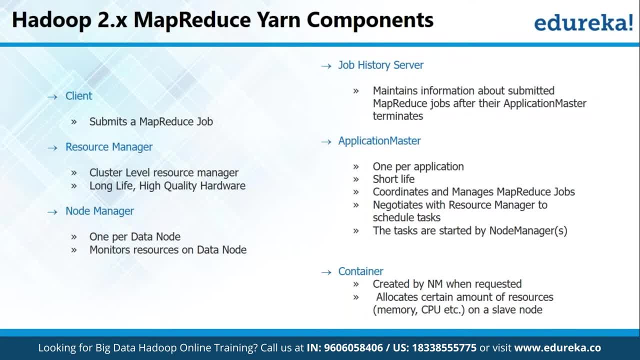 over the cluster or has been submitted on the cluster. it keeps the track of their status as well. okay, it also keeps the log files of every execution happened over the Hadoop cluster. okay, so what is application master? application master is again a process that is executed on a node machine, on a slave. 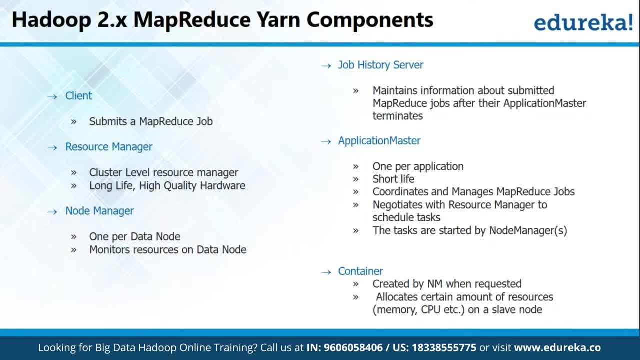 machine and created by a resource manager to execute and manage a job. it is the one which negotiates the resources from the resource manager and finally coordinates with the node manager to execute the task. okay, similarly, what is a container? a container is created by the node manager. 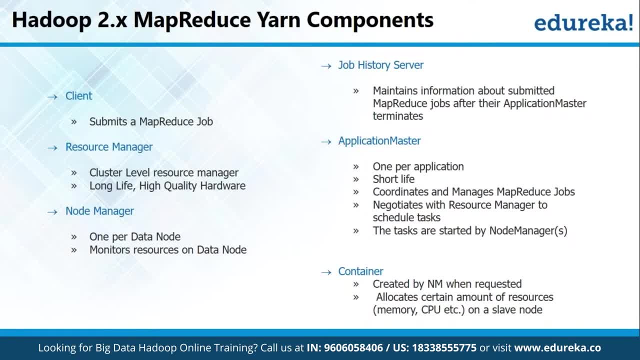 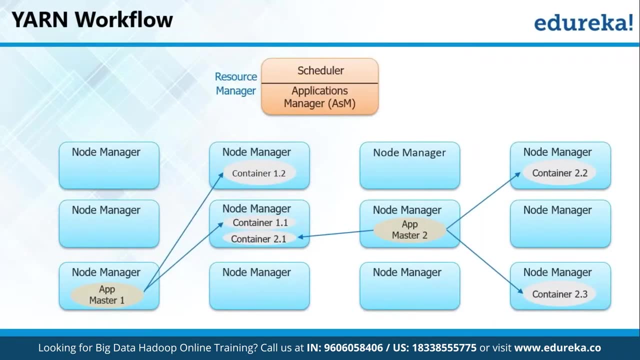 itself, which has been allocated by the source manager, and within the container, all the jobs are finally executed. okay, let me give you a pictorial representation of this process. so yarn, application workflow in MapReduce. so, as I said, the source manager, so there is a resource manager to which all 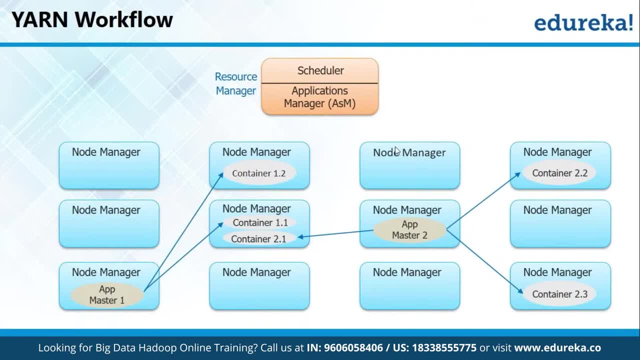 the jobs are submitted. there is a cluster in which there are slave machines. on every slave machine there is a node manager running. okay, the source manager has got two components: one is scheduler, another one is application manager. okay, so Matthew says: what is the difference between application master and application manager? application manager: 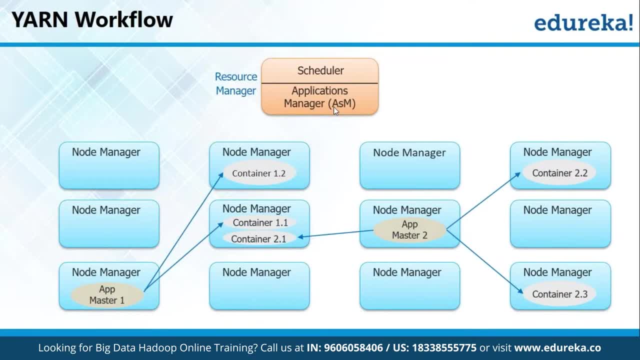 is a component of the source manager which ensures that every task is executed and an application master is created for it. application master, on the other hand, is somebody who executes the task and requests for all the resources that are required to execute it. okay, now, let's say a job is submitted to the 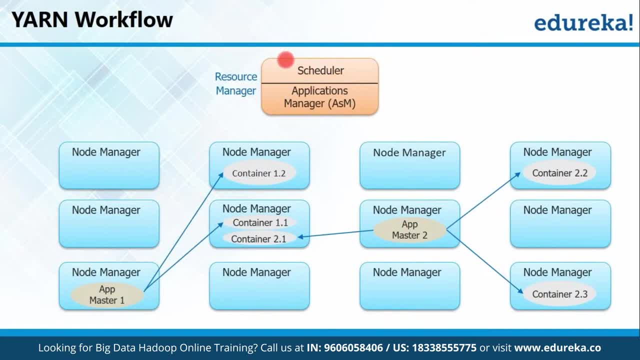 resource manager. as soon as the job is submitted, scheduler schedules the job. once the scheduler schedules the job to be executed, application manager will create a container in one of the data nodes. within this container, application master will be started. this application master will then register with the resource manager and request for a container to execute the task. okay now. 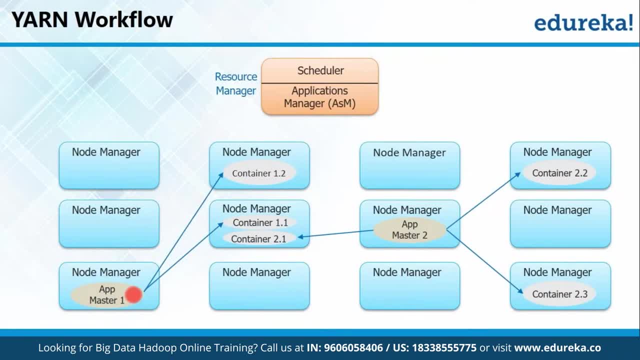 as soon as the container is allocated, application master will now connect with the node manager and request to launch the container. so, as you can see, application master got allocated these two data nodes. now this application master requested the node manager to launch these containers. okay, as soon as. 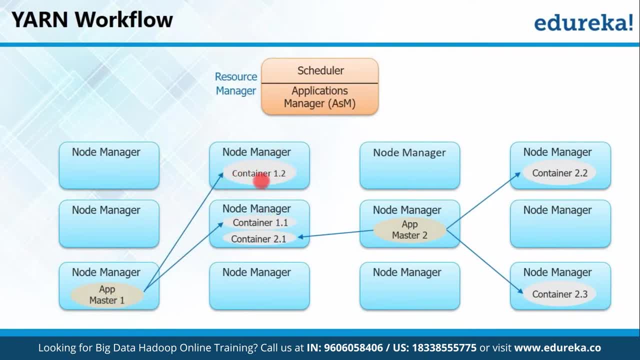 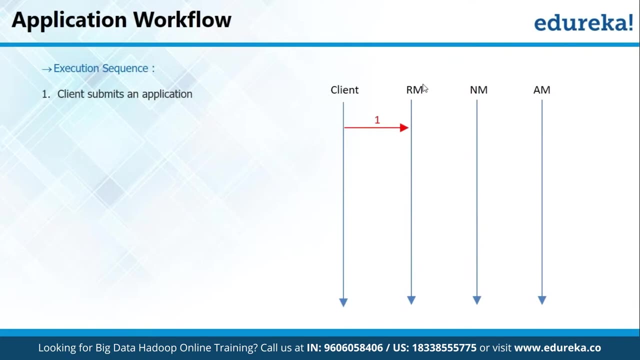 the containers were launched, application master executed the task within the container and the results are done was sent back to the client. let's understand this in a little sequential manner. okay, so on the right, as you can see, these are the lines. the first one is the client, the second one is the resource. 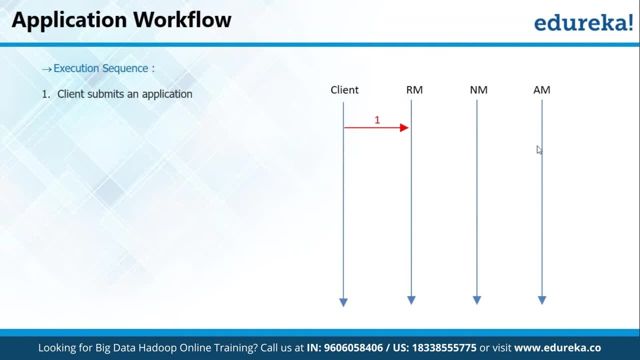 manager, third one is the node manager and the fourth one is the application master. so let's see how are the steps executed between them? okay, so very first step is: client submits the job to the resource manager, as you can see right here now. the second step is: resource manager allocates a. 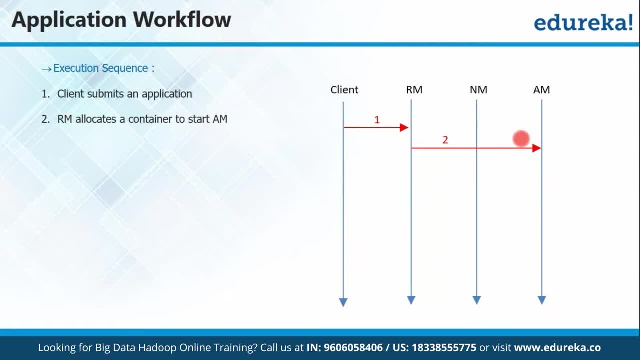 container to start the application master on the slave machines right. the third step is: application master registers with the resource manager. as you can see right here, as soon as it registers it requests for the containers to execute the task. that is the fourth step. after that, application master notifies the node manager on which the container needs to be launched. 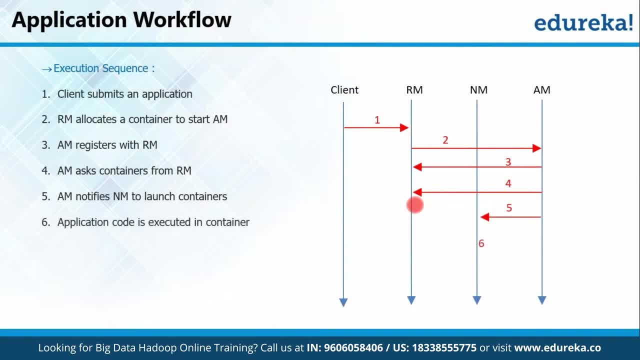 you, once the node manager has launched the containers, application master will execute the code within these containers. finally, the client contacts the resource manager or the application master to monitor application status. okay, and at the end, finally, the application master unregisters itself from the resource manager and the result is given back to the client, right? so this is one. 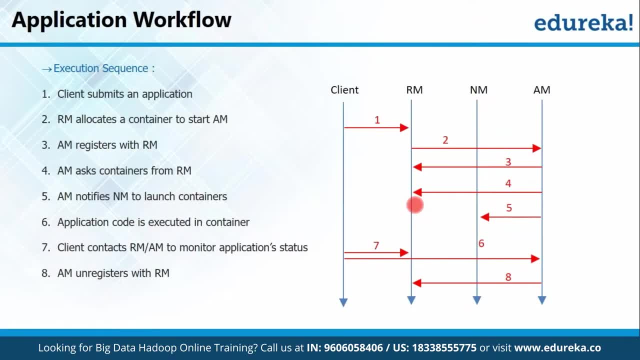 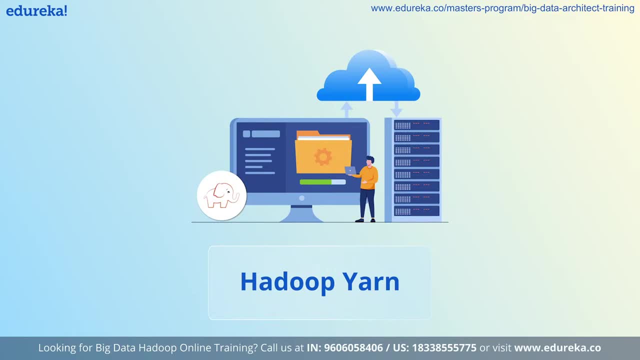 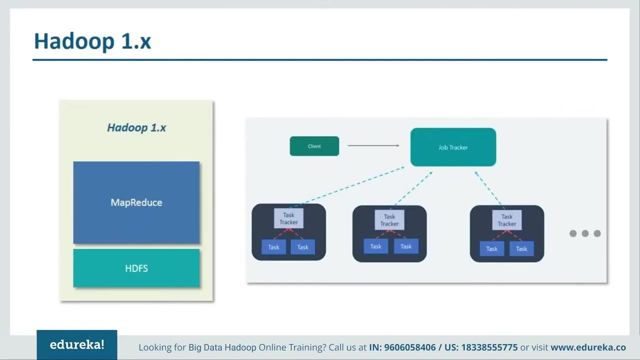 simple sequential flow of how a MapReduce program is executed within the resource manager and the Task Manager and the service manager using YARN framework. let me take this opportunity to explain you what is YARN and how it works. we'll first start with hadoop version one, where we had MapReduce version one. 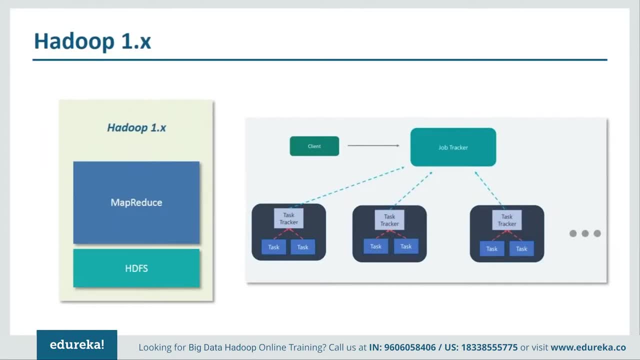 so in MRV1 the two core services were hdfs, that is, hadoop distributed file system, and MapReduce, which forms the basis of almost all hadoop functionality. all other components are built around these services and must use map reduce to run the service and Hadoop distributed system as one of the main components in YARNек implementation. 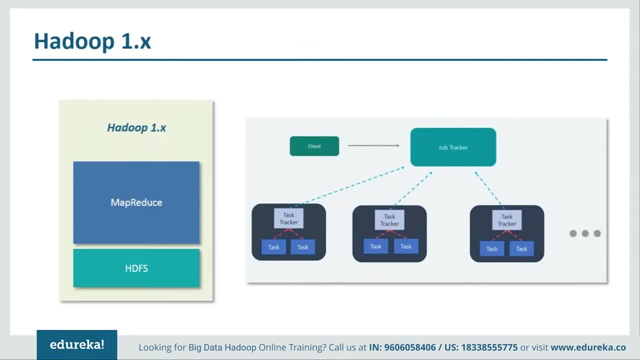 So let's start with the first one. We'll open the YARN framework and let's first do this one first. So let's start with YARN environment to run Hadoop jobs, while MapReduce method enables user to focus on the problem at hand rather than. 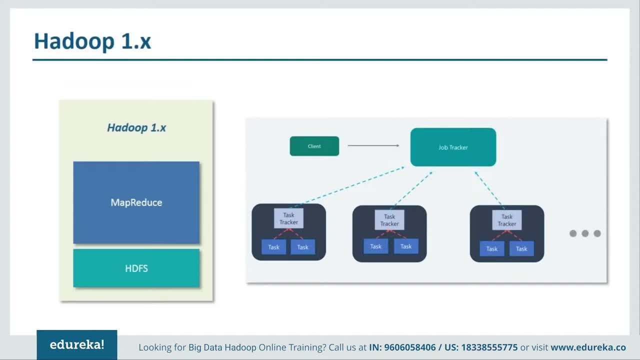 the underlying processing mechanism. They do limit some of the problem domains that can run in Hadoop framework. So now let us know how MapReduce version 1 works in order to understand its limitations. The MapReduce processing model consists of two separate steps. The first step. 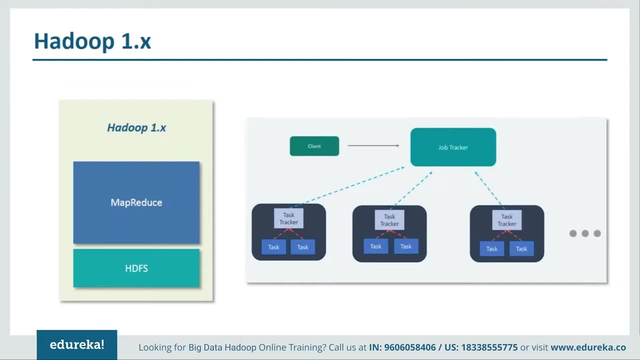 is parallel map phase, in which input data is split into discrete chunks that can be processed independently. The second phase is the reduce phase, in which the output of map phase is aggregated to produce the desired result. This is simple and fairly restricted nature of programming model, which lends itself to a very efficient and extremely large scale implementation across. 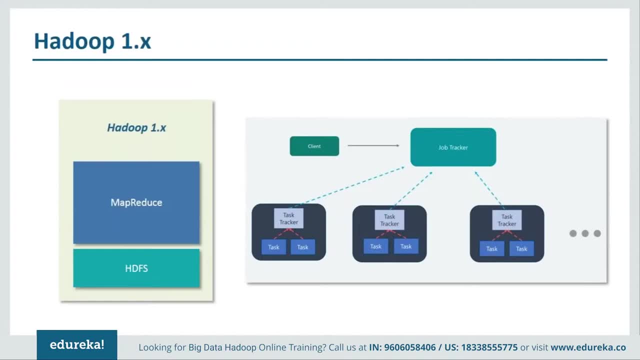 thousands of low cost community servers. When MapReduce is paired with a distributed file system such as HDFS, which can provide high aggregate IO bandwidth, the economic of the system becomes extremely compelling. This is a key factor in the popularity of MapReduce. One of the key to Hadoop performance is the lack of data motion, such as compute task are moved to. 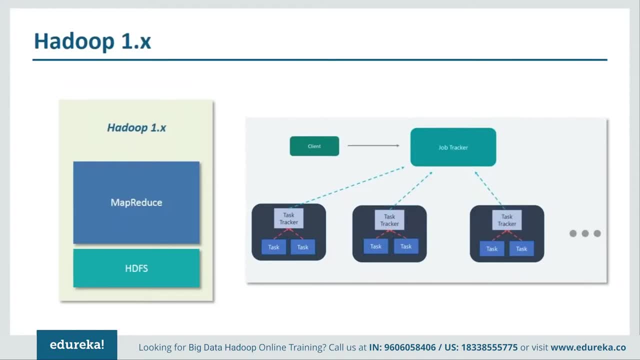 server on which the data resides, and not the other way around. Specifically, the map task can be scheduled on the same physical nodes on which data resides, in HDFS, which exposes the underlying storage layout across the cluster. This design significantly reduces the network input output. 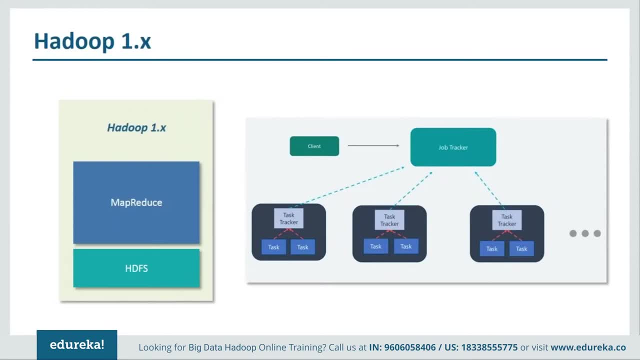 patterns and keeps most of the IO on local disk or on a neighboring server within the same server rack. To understand how MapReduce works, let us know in the comment section. To understand the new YARN process flow, it is helpful to review the original Apache Hadoop MapReduce. 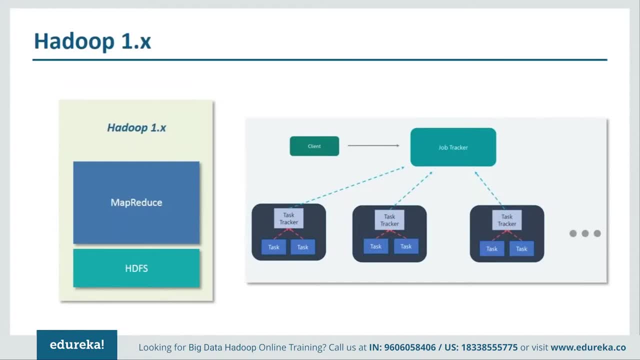 design As a part of Apache Software Foundation. MapReduce has evolved and improved as an open source project. MapReduce project itself can be broken down into the end-user MapReduce APIs for programming the desired MapReduce applications, the MapReduce runtime, which is the implementation. 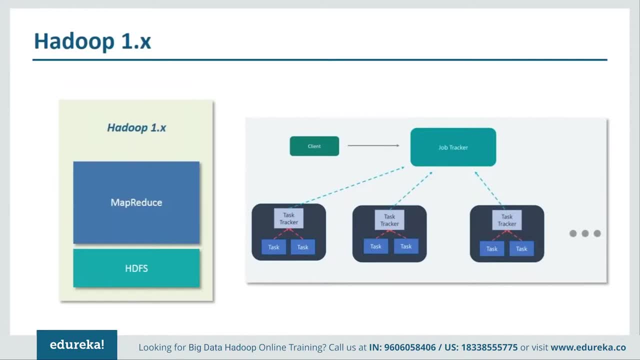 of various phases, such as map phase, shot, shuffle or merge aggregations and the reduce phase, and the MapReduce framework, which is the backend infrastructure required to run users' MapReduce applications, manage cluster resources and schedule thousands of concurrent jobs, among other things. This separation of concerns has high, significant benefits, particularly for end-users. 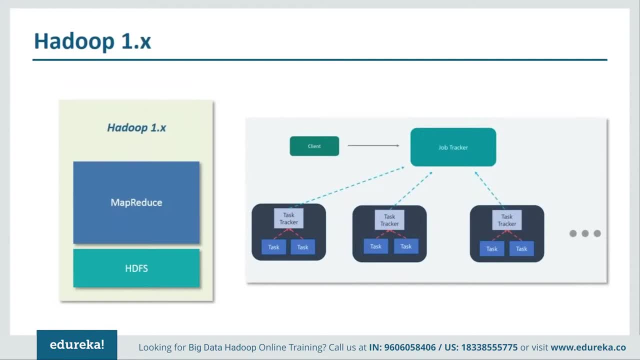 where they can completely focus on their applications via the API and let the combination of MapReduce, runtime and the framework deal with the complex details such as resource management, fault tolerance and scheduling. As you can see in the right hand side image, the master process is. 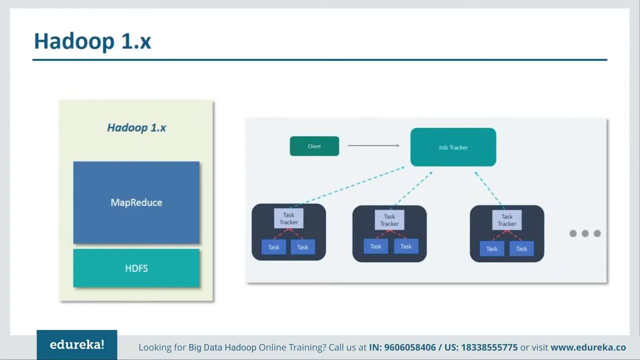 the job tracker, which serves as the clearinghouse for all MapReduce jobs in the cluster. Each node is a job tracker process that manages tasks on the individual node. The task tracker are controlled by the job trackers. The job tracker is responsible for resource management, tracking resource. 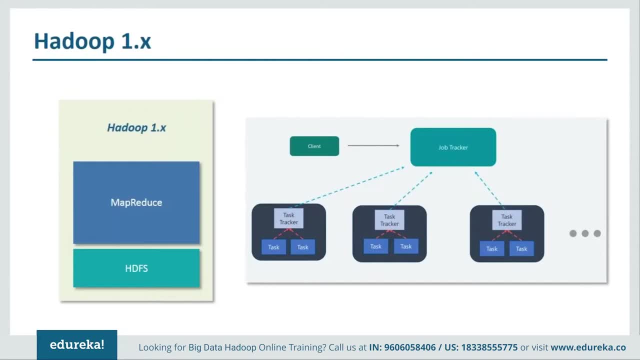 consumption, availability and job lifecycle management, like scheduling individual tasks of the job tracking, progress, providing fault orders for tasks, etc. The task tracker has simple responsibilities like launch or tear down tasks on order from job tracker and provide task status information to the job tracker periodically. 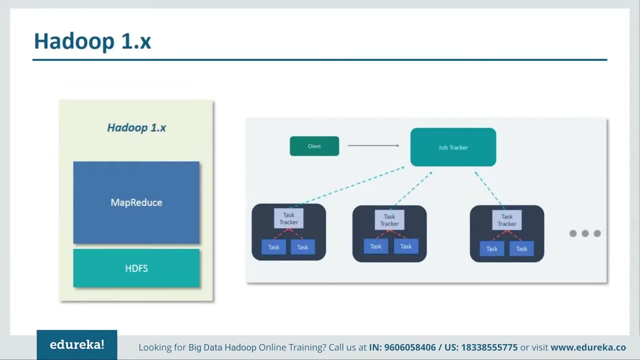 The task tracker has exhibited some growing pains. in particular, with regard to the job tracker, several aspects, including scalability, cluster utilization, ability to control you upgrade to the stack and support for workloads other than MapReduce itself- MapReduce is great for many applications, but not everything Other programming model better serves. 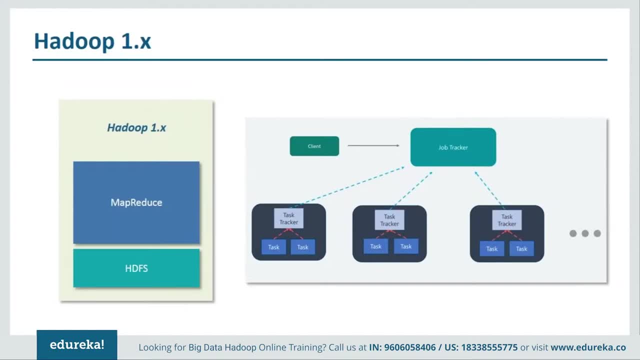 requirements such as graph processing and iterative modeling using message passing interface. As is often the case, much of the enterprise data is already available in Hadoop HDFS and having multiple paths for processing the data in Hadoop HDFS. For example, if you want to use Hadoop HDFS, 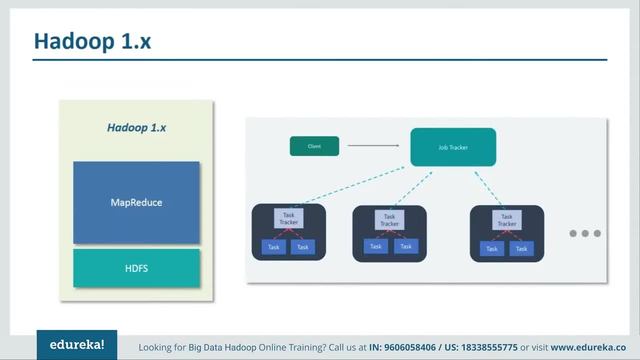 for processing is critical and clearly necessary. Furthermore, given the MapReduce is essentially for batch processing, support for real-time and near real-time processing has become an important issue for the user base. A more robust computing environment within Hadoop will enable organizations to see an increased return on their Hadoop investment by lowering their operational cost. 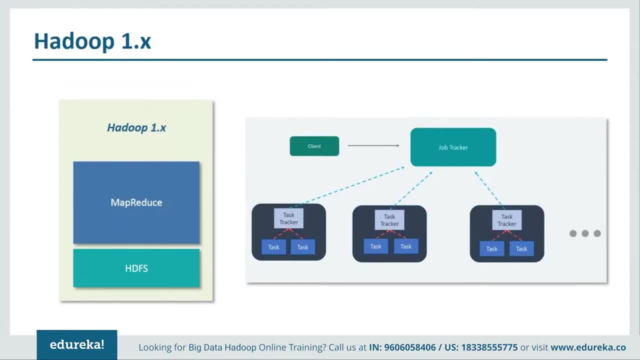 The first challenge was scalability. The processing power available in data center continues to increase rapidly. Consider the additional hardware capability offered by a commodity server over a three-year period. In 2009,, we had 8 cores, 16 GB of RAM and 4 x 1 TB of disk. 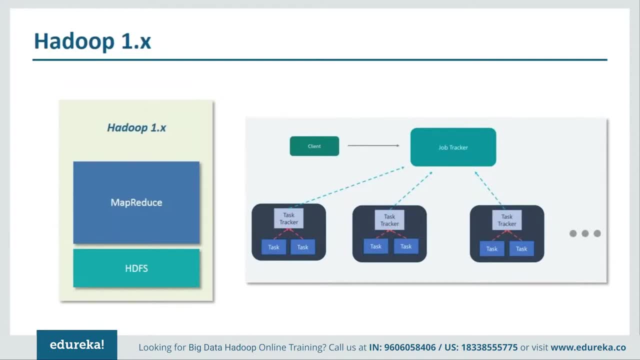 Coming down to 2012,, we had 16 plus cores, 72 GB of RAM and 12 x 3 TB of hard disk. These new servers are often available at the same price. In general, servers are twice as capable today as they were two or three years ago. MapReduce is known to scale to production. 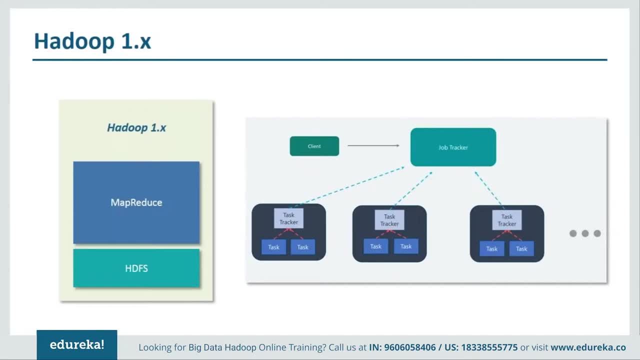 deployment of approximately 5000 server nodes in 2009 vintage For the same price. the number of CPU cores, amount of RAM and local storage available to the user will put continued pressure on the scalability of new Apache Hadoop installations. So the next point is utilization. So in the current system the job tracker views the cluster. 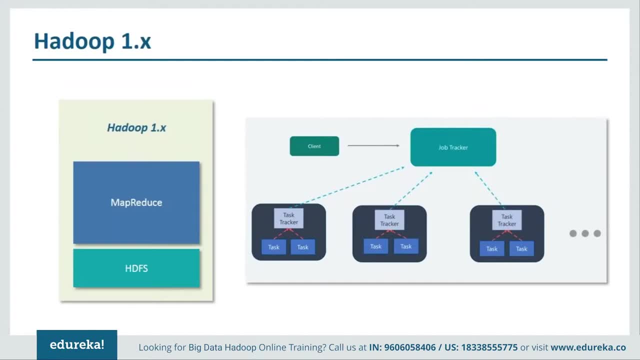 as composed of nodes with distinct map slots and reduce slots, which are not fungible. Utilization issues occur because, if map slots might be full while reduce slots are empty, or a vice versa scenario, Improving this situation is necessary to ensure the entire system could be used to its maximum capacity for high utilization and applying 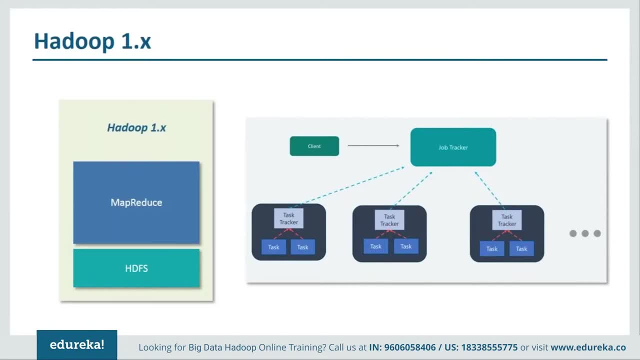 resources when needed. Next is user agility In a real-time deployment. Hadoop is very commonly offered as shared multi-tenant system. As a result, changes to Hadoop software stack affects a large cross-section of enterprise. Against the backdrop, users are very keen to 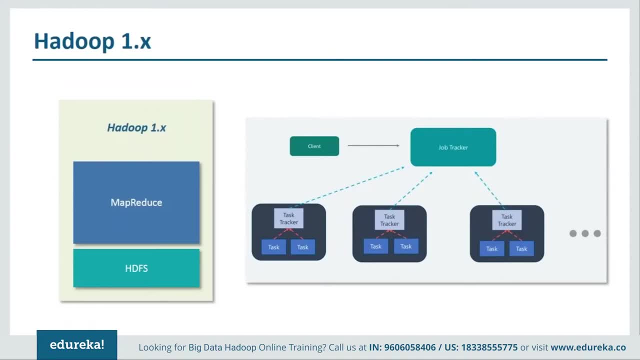 control upgrades to the software stack, as such upgrades have a direct impact on their applications. Now let us discuss a problem that Yahoo faced. Yahoo was the first company to embrace Hadoop in a big way and it was a trendsetter within the Hadoop ecosystem. In late 2012,, it struggled to handle iterative and stream processing system. 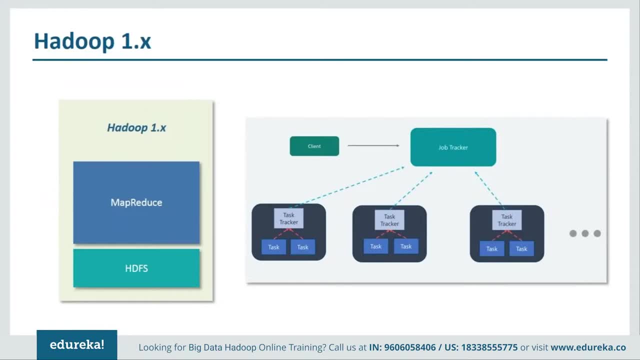 of data on Hadoop infrastructure due to map-reduced limitations. Scalability bottleneck was caused by having a single job tracker. According to Yahoo, the practical limits of such design are reached up to a cluster of 5000 nodes and 40000 tasks running concurrently. 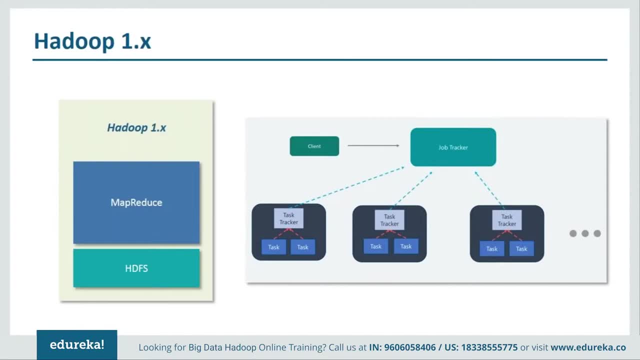 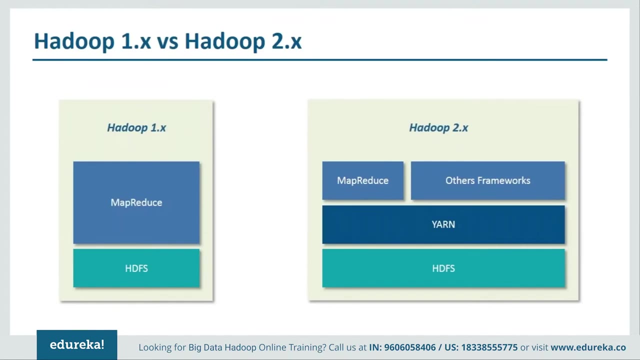 After implementing YARN in the first quarter of 2013,, Yahoo installed more than production nodes on spark for iterative streaming, storm for stream processing, hadoop for batch processing, etc. such a solution was possible only after yarn was introduced and multiple processing frameworks were implemented. so, to address these needs, the yarn project was started by apache. 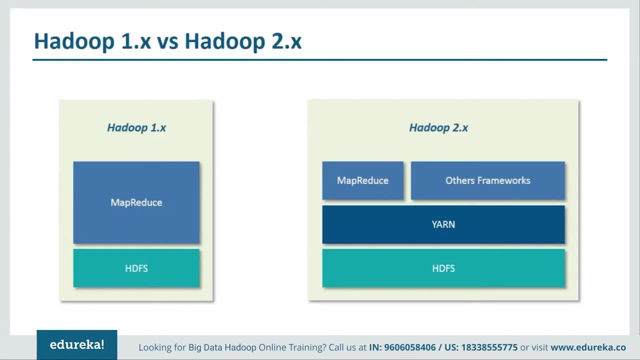 hadoop community to give hadoop the ability to run non-map reduce jobs within the hadoop framework. yarn provides a generic resource management framework for implementing hadoop applications. in hadoop version 2.x, map reduce has undergone a complete renovation. yarn is also known as mrv2. 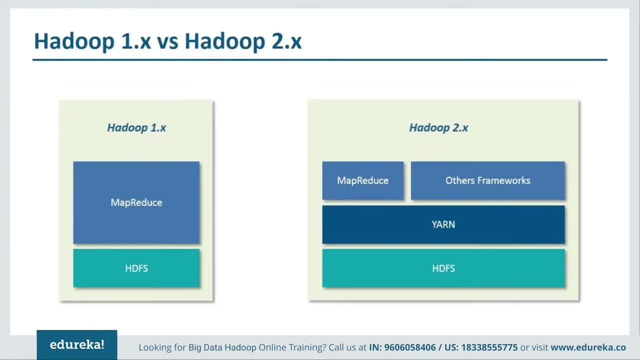 that is, map reduce version 2.. yarn provides both full compatibility with existing map reduce application and a new support for virtually any distributed application. the introduction of yarn does not change the ability of hadoop to run map reduce jobs. it does, however, position map reduce as a merely one of the application frameworks within hadoop, which works the same way as it. 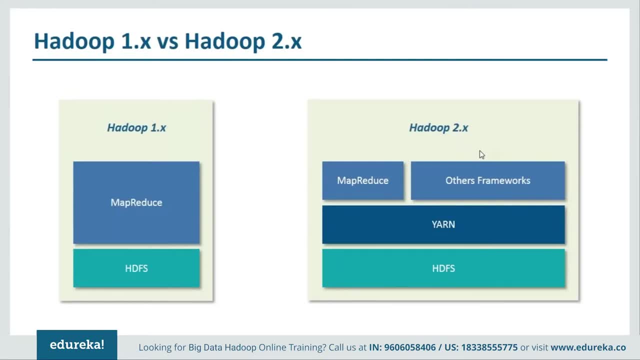 did in mrv1. the new capability of hadoop is that it is able to run map reduce jobs within the hadoop ecosystem. so the first step that hadoop offers by yarn is to use the new non-mapped reduce frameworks. that adds many new features to the hadoop ecosystem. so, as you can see here in hadoop, 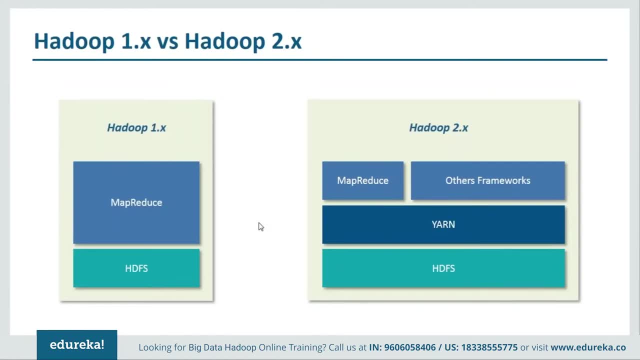 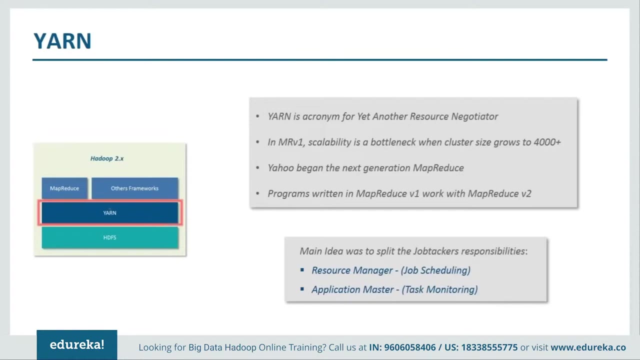 1.x. map reduce serves two purpose, that is, processing paradigm as well as resource management. now in hadoop 2.x, yarn takes all the responsibilities of resource management. or map reduce or other frameworks can be used as processing paradigms. the fundamental idea of yarn is to split the two. 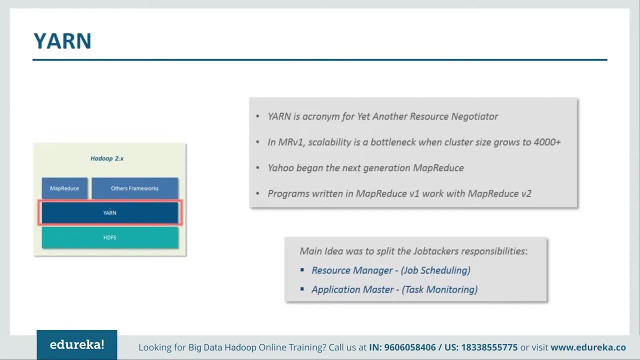 major responsibilities of job tracker- that is, the processing paradigm and the non-mapped resource management and job scheduling or monitoring- into separate demons: a global resource manager and a per application application master. the resource manager and per node slave. the node manager forms the new and generic operating system for managing applications. 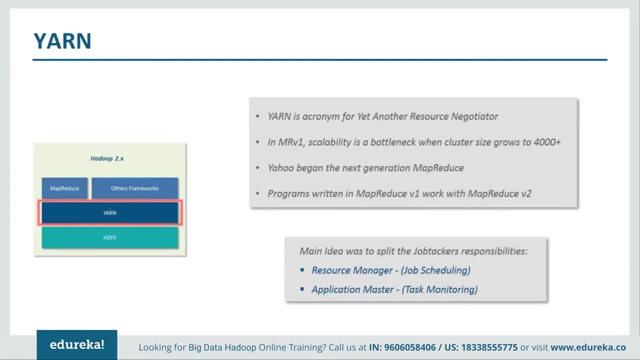 in a distributed manner. yarn relies on these three main components for all its functionalities. The first component is the resource manager, which is the arbitrator of the cluster resources. It has two parts: a pluggable scheduler and an application manager that manages user jobs on the cluster. 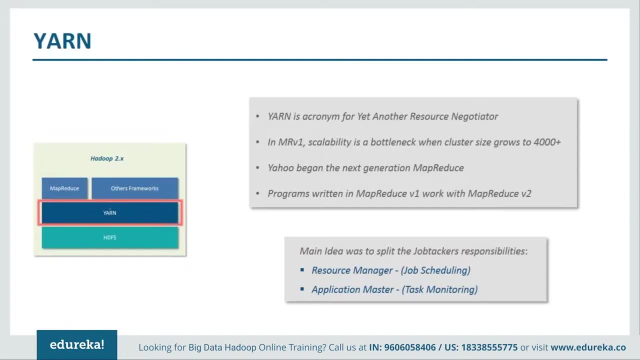 The second component is the per node node manager, which manages user jobs and workflow on the given node. The central resource manager and the collection of node manager creates a unified computational infrastructure of the cluster. The third component is the application master: a user job lifecycle manager. 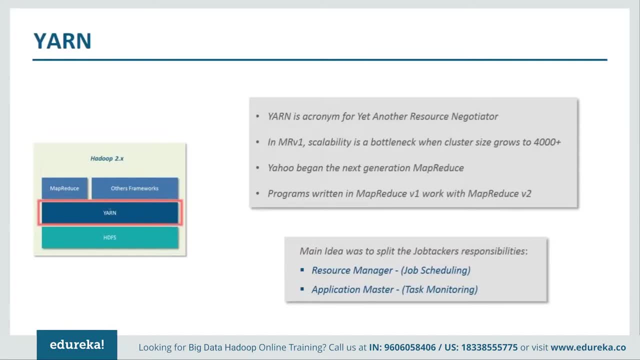 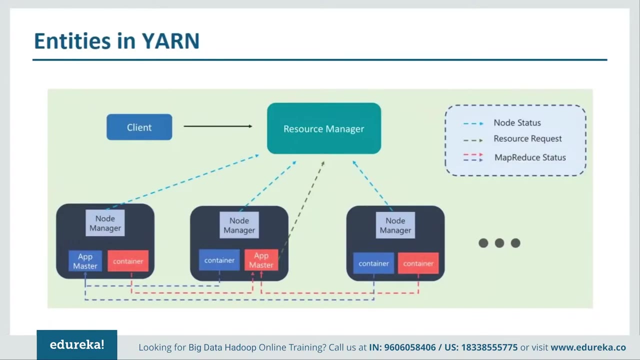 The application master is where the user application resides. together These three components provide a very scalable, flexible and efficient environment To run virtually any type of large-scale data processing jobs. So the resource manager is the ultimate Authority. that are by traits, division of resources among all the applications. 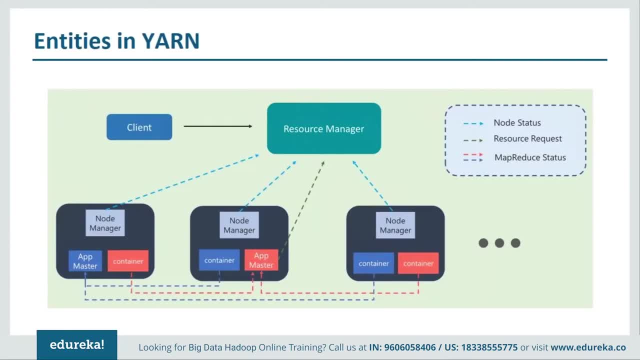 in the system per application. application master is a framework specific entity and is tasked with negotiating for resources from the resource manager and is working with the node manager to execute and monitor the component tasks. The resource manager has a pluggable scheduler component which is responsible for allocating resources to various running. 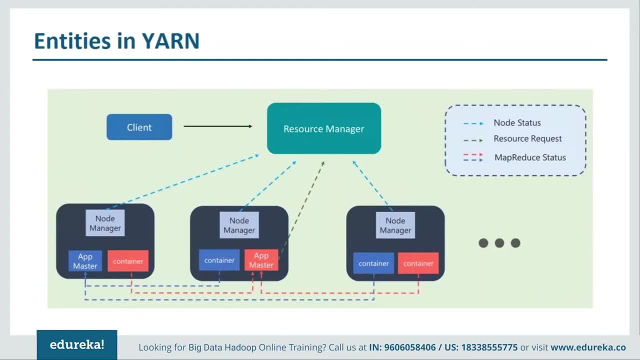 applications Like capacity Q and other factors. The scheduler is a pure scheduler in the sense that it performs no monitoring or tracking of status for the application, offering no guarantees on restarting tasks that are not carried due to either hardware failure or could be application failure. 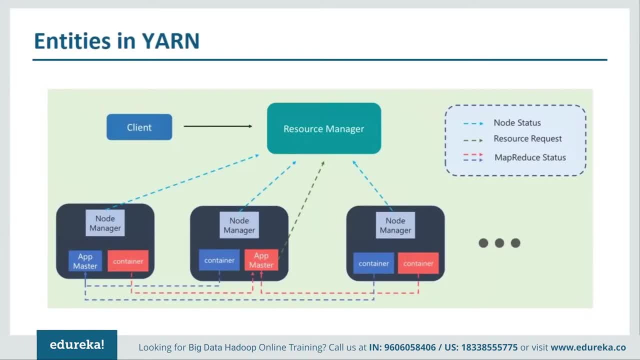 This scheduler performs its scheduling function based on the resource requirement of an application by using the abstract notion of resource container, which incorporates resource dimensions like memory, CPU And network. the node manager is the per machine slave, which is responsible for launching the application containers, monitoring their resources, like CPU, memory, disk, Network and reporting the 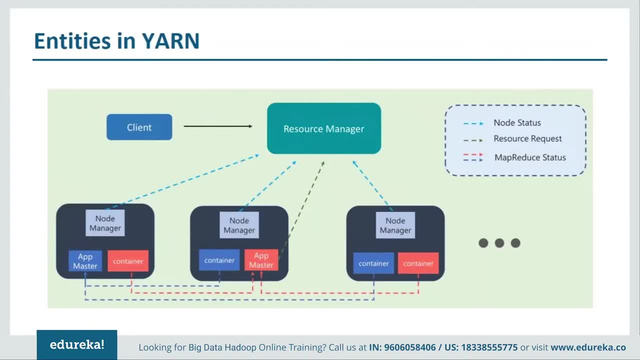 same to the resource manager. the per application application master is responsible for negotiating appropriate resource containers from the schedulers, tracking their status and monitoring the progress from the system perspective. The application master runs a normal container, one of the crucial implementation details of MapReduce within the new yarn system. 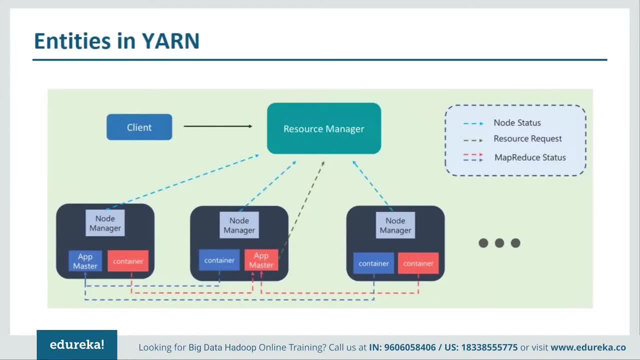 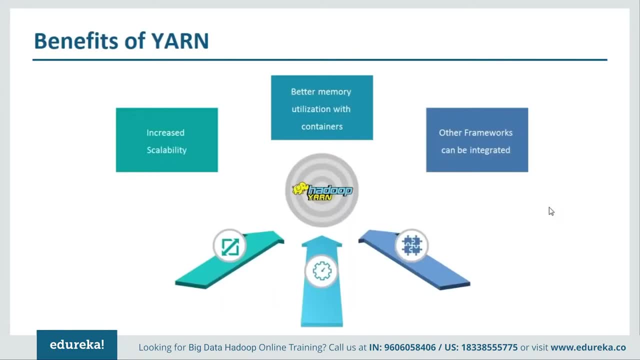 is the reuse of existing MapReduce framework without any major surgery. This step was very important to ensure compatibility of existing MapReduce applications and users. Now the major benefits of yarn is increased scalability, better memory utilization with containers, and the third one is other frameworks can be integrated, like spark, storm, hive, etc. 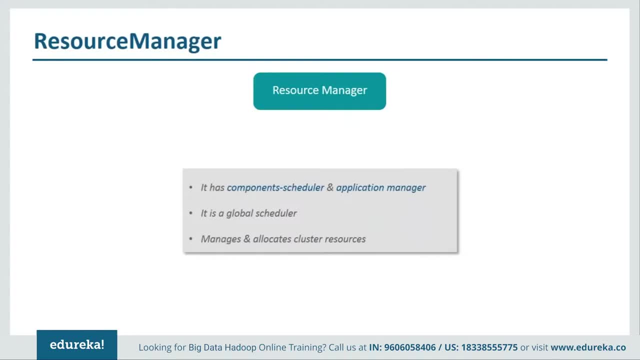 Now, by adding new functionalities, yarn brings new components into Apache Hadoop workflow. These component provides finer grain control for the end user and simultaneously offer more advanced capabilities to Hadoop ecosystem. Let's look at them one by one. So first is resource manager, as mentioned earlier, the yarn resource. 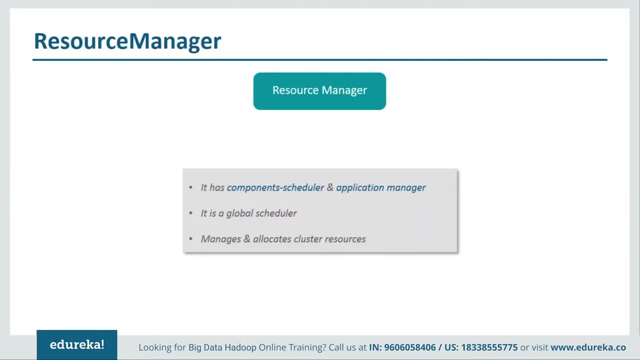 manager is primarily a pure scheduler. It is strictly limited to arbitrating request for available resources in the system made by competing applications. It optimizes the cluster utilization like keep all resource in use all the time. Again, It has various Constraint, such as capacity guarantees, fairness. 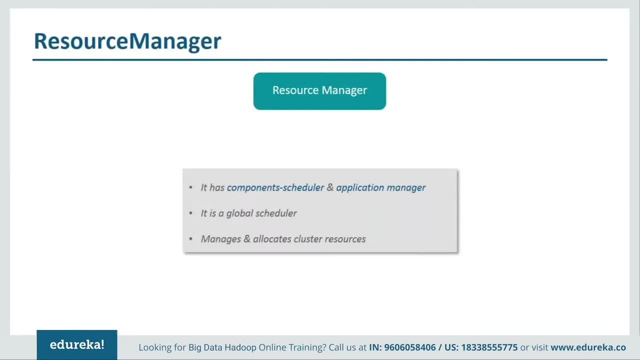 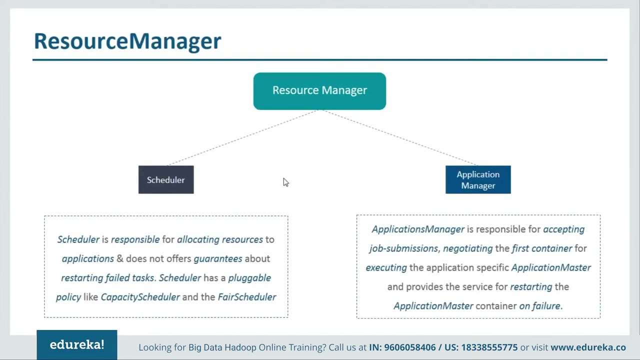 and SLS to allow for different policy constraints. the resource manager has a pluggable scheduler that enables different algorithms, such as those focusing on capacity and fair scheduling, to be used as necessary. So, as we discussed, resource manager has two components, that is, scheduler and application manager. 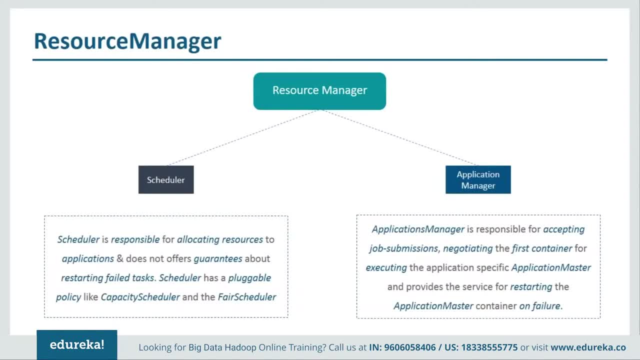 So the scheduler is responsible for allocating resources to applications and does not offer guarantees about restarting failed tasks. Scheduler also have pluggable policies, that is, capacity scheduler or a fair scheduler, Etc. Moving down to application manager, application manager is responsible for accepting job submission, negotiating with the first container. 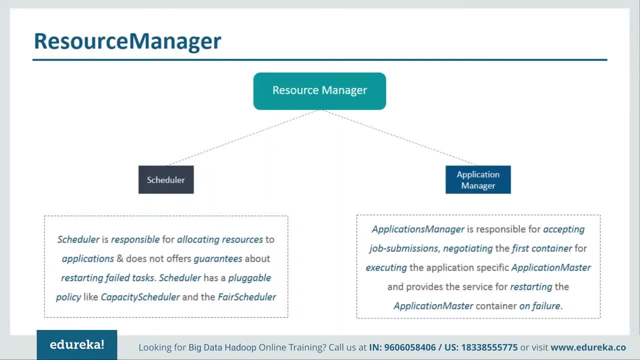 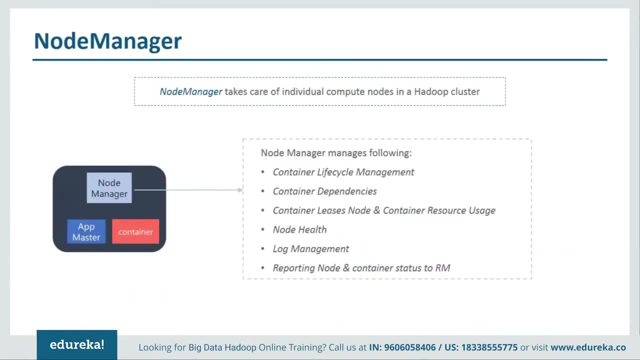 for executing the application specific application master and it also provides the service for restarting the application master on failure. Next is node manager. The node manager is yarns per node worker agent taking care of individual compute nodes in Hadoop cluster. Its duties include keeping up-to-date with resource manager, overseeing 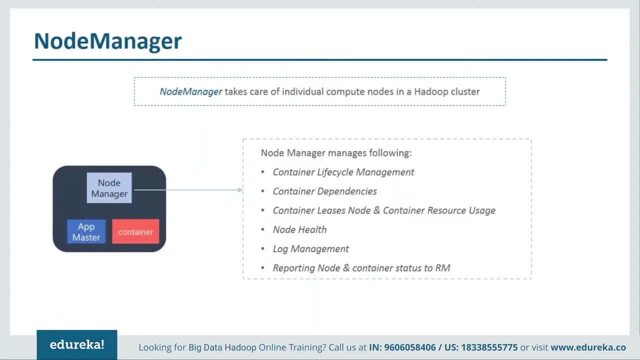 application containers, lifecycle management, monitoring resource uses like memory, CPU, Network, Etc. of individual containers, tracking node health, log management and auxiliary services that may be exploited by different yarn applications. on startup, the node manager registers with the resource manager. It then sends heartbeat with status and waits for the instruction. 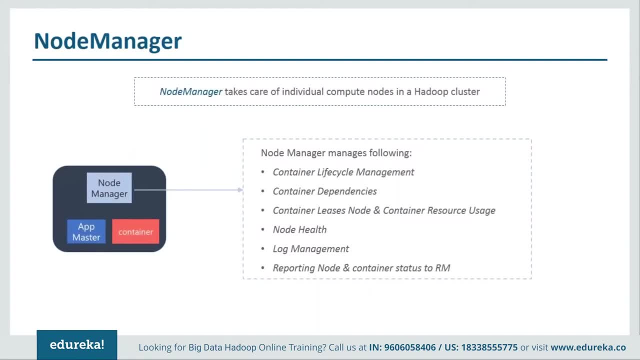 Its primary goal is to manage Containers assigned to it by the resource manager. yarn containers are described by a container launch context, that is CLC. this record includes a map of involvement variables, dependencies stored in remote, accessible storage, security tokens, payload for node manager services and the command necessary to create the process after violating the. 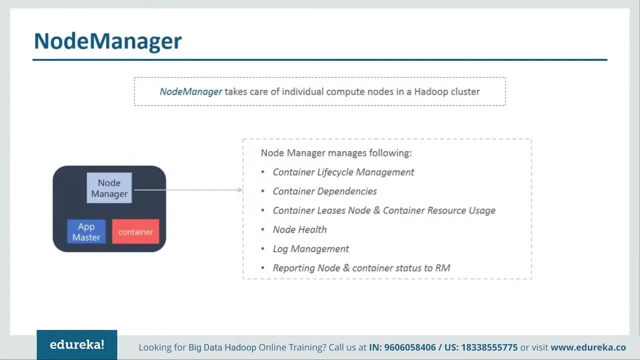 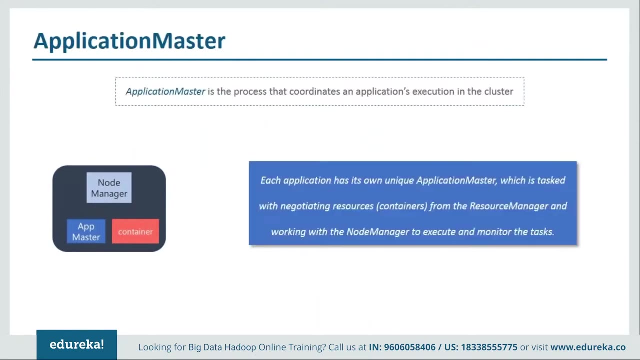 authenticity of the container lease. the node manager configures the involvement for the container, including initializing its monitoring subsystem. With a resource constraint specified application, the node manager also kills container as directed by the resource manager. Now next is application master. So application master is an important concept in yarn. the application: 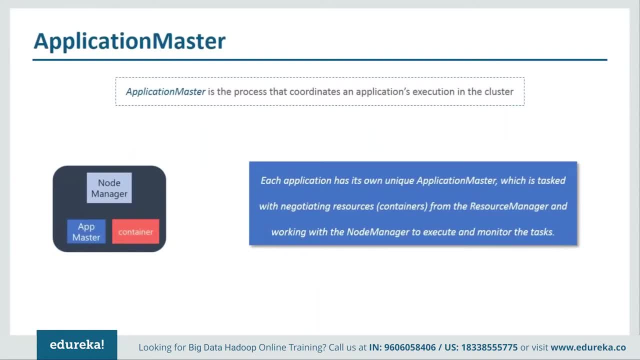 master is ineffective and instance of the framework specific library and is responsible for negotiating resources from the resource manager. It is also working with the node manager to execute and monitor the containers and their resource consumption. It has the responsibility Of negotiating for appropriate resource containers from the resource. 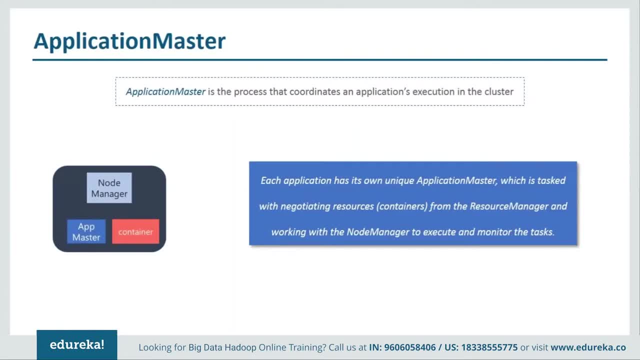 manager, tracking their status and monitoring progress. The application master is the process that coordinates and applications execution in the cluster. Each application has its own application master, which is tasked with negotiating resources from resource manager and with the node manager to execute and monitor the task. in yarn design, MapReduce is just one. 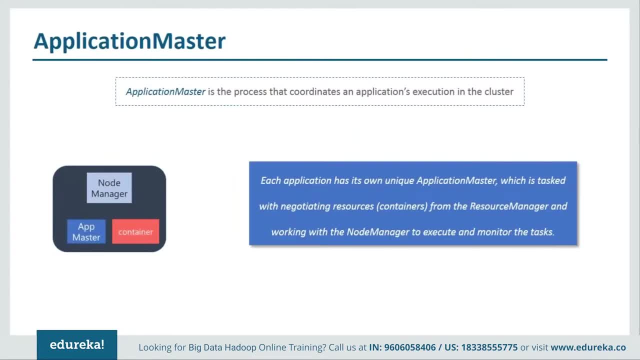 application framework. this design permits building and deploying distributed applications using other frameworks. Once the application master is started, it will periodically send heartbeats to resource manager to affirm its health and to update the record of its resource demands after building a model of its requirement. 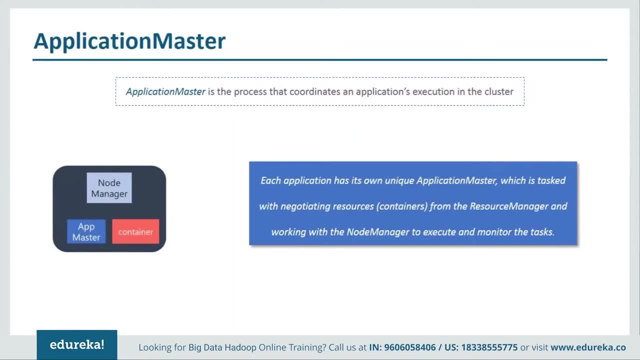 The application master encodes it preferences and constraints in a heartbeat message to the resource manager. in response to subsequent heartbeats, the application master will receive a lease on container bounds to a location of resources at the particular node In the cluster, depending on the containers it received from the 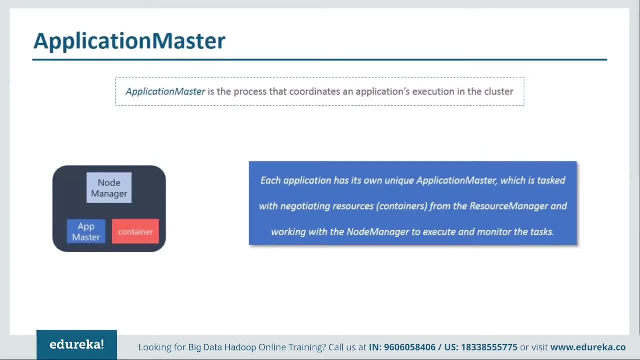 resource manager. The application master may update its execution plan to accommodate the excess or lack of resource. container allocation or deallocation can take place in dynamic fashions as an application progresses. the application master design enables yarn to offer some important features like scalability. the application master provide much of the job oriented. 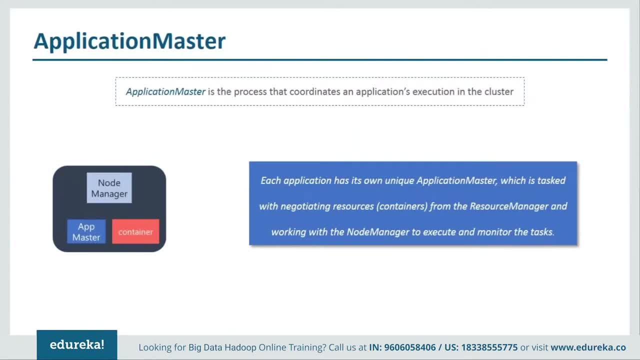 functionality to the job tracker so that the entire system can scale more dramatically. simulations have shown That jobs may scale to 10,000 node clusters composed of modern hardware without any significant issue. as a pure scheduler, the resource manager does not have to provide fault tolerance of resources across the cluster. 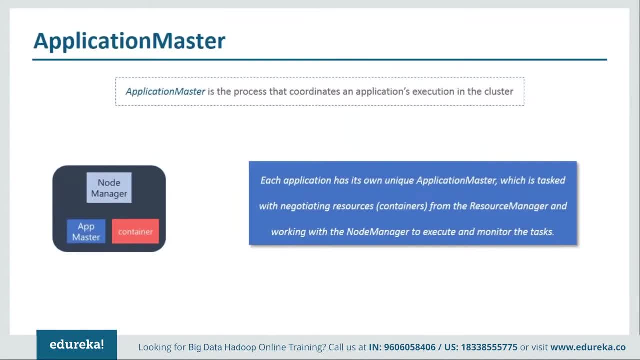 by shifting fault tolerance to application master, instance control becomes local rather than global. second is moving all the application framework specific code into the application master generalizes the system so that it can now support multiple frameworks such as, That is, message passing interfaces and graph processing. in reality, every 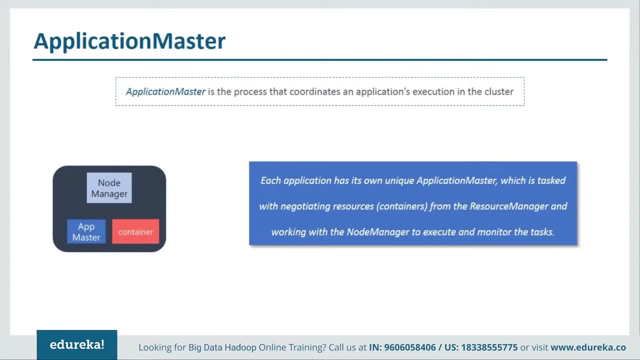 application has its own instance of an application master. However, it is completely feasible to implement an application master to manage a set of applications. Furthermore, this concept has been stressed to manage long-running services which manage their own applications. example: launching HBase in yarn via a special HBase app master. 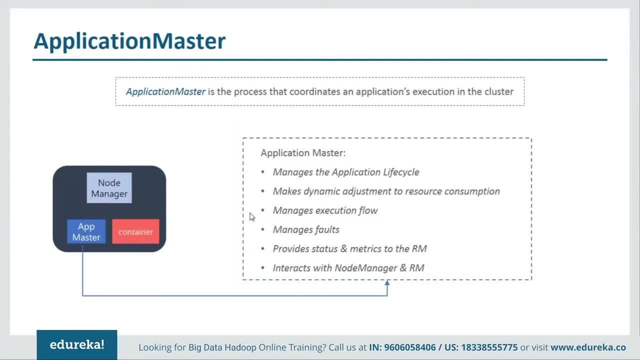 So you can go ahead and see the responsibilities of application master, that is, managing the application Lifecycle, making dynamic adjustment to resource consumptions, managing execution flow, managing faults, providing status and metrics to the resource manager, interacting with node manager as well as resource manager, and so on. 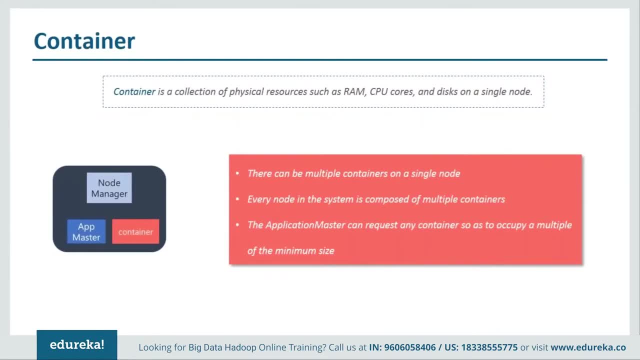 So next component is containers. yarn has a pluggable scheduling component. depending on the use case and user needs, administrator may select either a simple that is first in, first out capacity or a fair share scheduler. The scheduler class is set in yarn default XML file. at the fundamental level, a container is a collection of physical 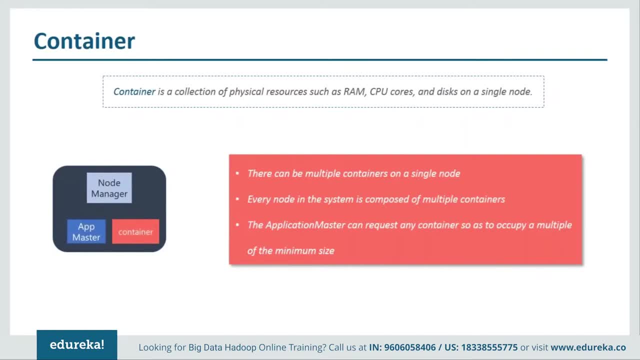 resources such as RAM, CPU cores and disk on a single node. There can be multiple containers on a single node. Every node in the system is considered to be composed of multiple containers of minimum size of memory and CPU. the application master can request any container so as to occupy a multiple of minimum size. a container is supervised. 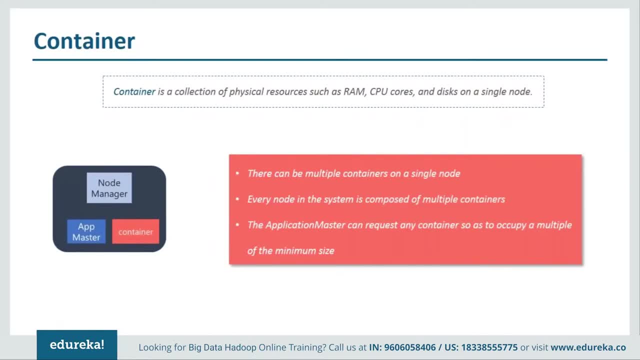 by the node manager and scheduled by the resource manager. Each application starts out as an application master, which is itself a container, often referred as container 0. once started, the application master must negotiate with the resource manager for more containers. container requests can take place in a dynamic fashion at runtime. 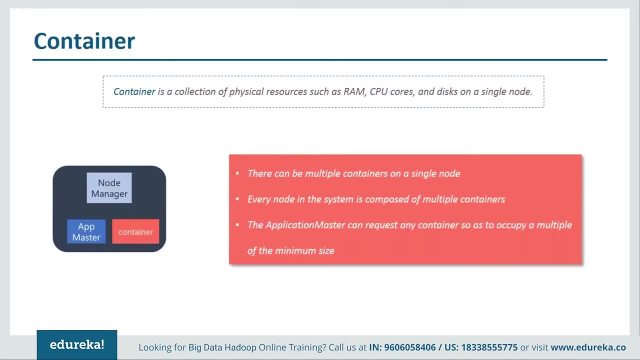 For instance, a MapReduce job may request a certain amount of mapper containers as they finish their task. it may release them and request more reducer containers to be started now. as we have already discussed, yarn containers are described by a container launch context, that is CLC. 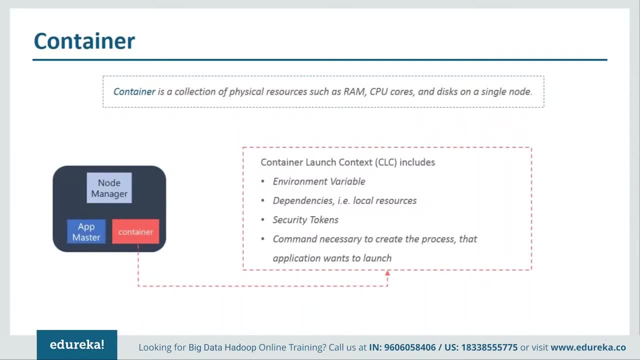 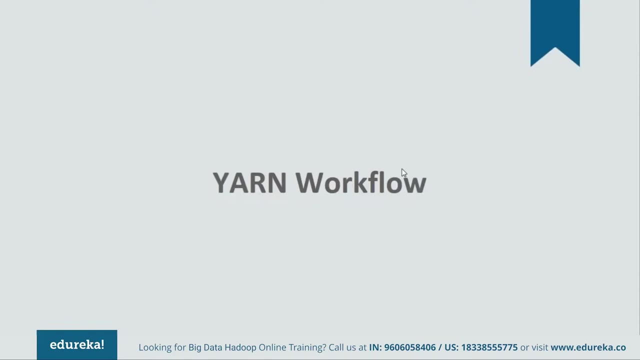 So this record includes a map of environment variables, dependencies stored in remotely accessible storage, security tokens, payload for node manager services and the command necessary to create the process. So a CLC include everything's that you need to launch a container moving ahead. Let us understand the yarn workflow. 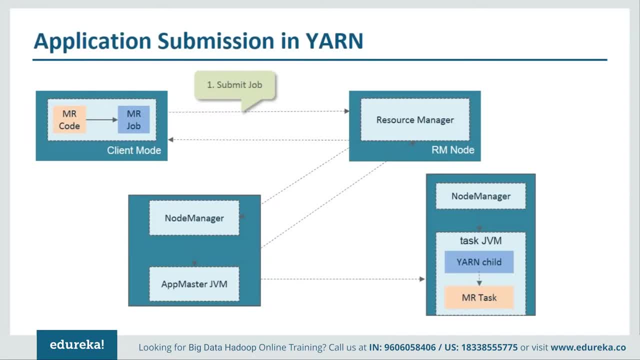 So in earlier Hadoop versions, each node is the cluster was statically assigned the cap Ability of running a predefined number of map slots and a predefined number of reduced slots. the slots could not be shared between maps and reduces. the static allocation of the slot wasn't optimal because slot requirements vary. 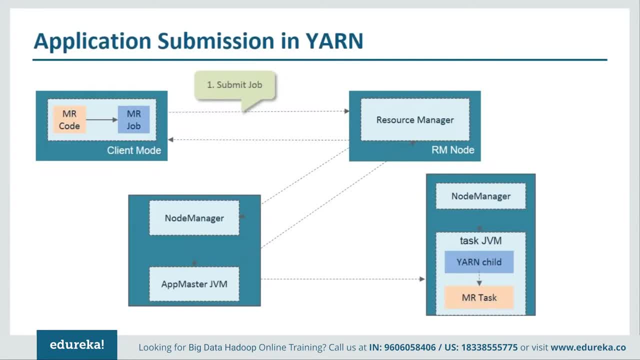 during the MapReduce application lifecycle. Typically, there is a demand of map slots when the job starts, as opposed to the need of reduced slots towards the end of the job. the resource allocation model in yarn addresses the inefficiencies of static allocation by providing a greater flexibility. as discussed previously, resources are requested in: 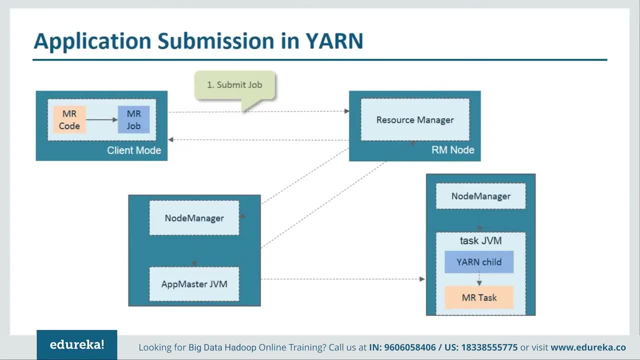 form of containers where each container has a number of non-static attributes. yarn currently has attribute support for memory and CPU. the generalized attribute model can also support things like bandwidth or GPUs. So first let's look at the client resource request. So, as you can see, a yarn application starts with a client resource request. 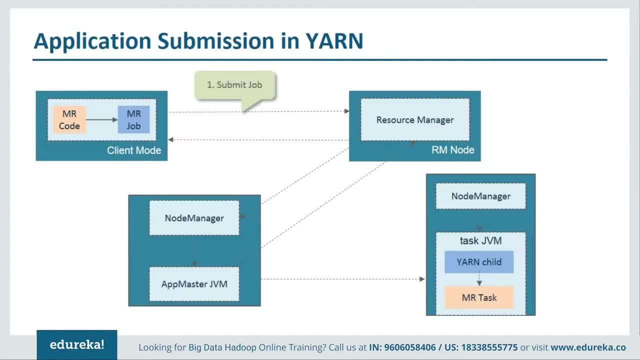 a client communicates with the application manager- component of the resource manager. to initiate this process, the client must first notify the resource manager that it wants to submit an application. the resource manager responds with an application ID and information about the capabilities of the cluster. that will aid the client in requesting resources. next, the 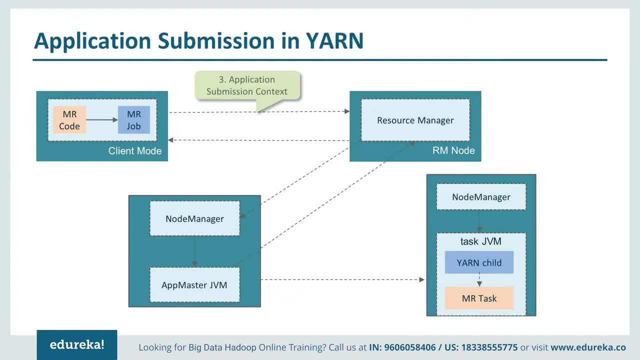 client responds with an application submission context. the application submission context contains the application ID, user queue and other information needed to start the application master. In addition, a CLC, that is, container launch context, is sent to the resource manager. as we already have discussed about CLC, that it contains job file. 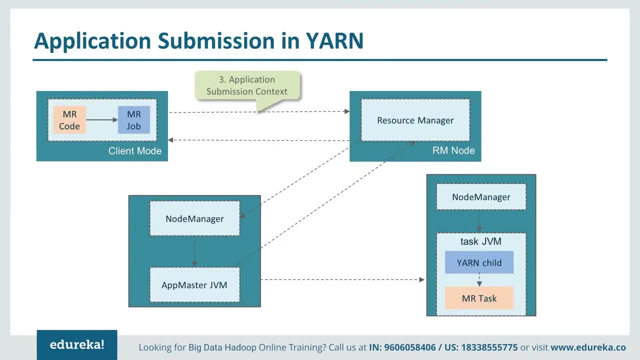 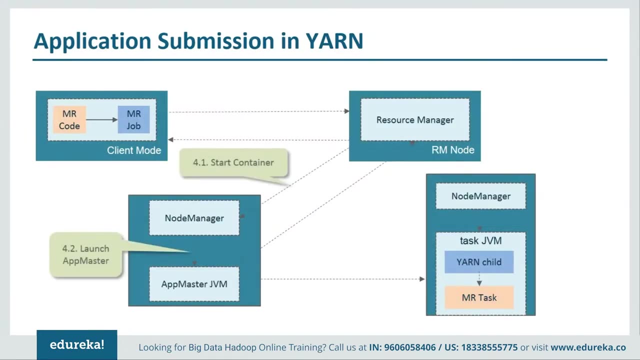 security tokens, resource requirements and other information needed to launch an application master on the node. Once the application has been submitted, the client can also request the resource manager kill the application or provide status report about the application when the resource manager receives the application submission context from a client. 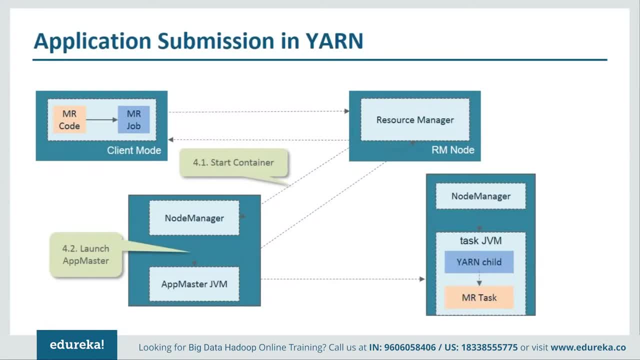 It schedules an available container for the application master. if there are no applicable containers, the request must wait. if a suitable container can be found, then the resource manager contacts the appropriate node manager and start the application master. as part of the step, the application master RPC port and tracking URL for monitoring the application status will be 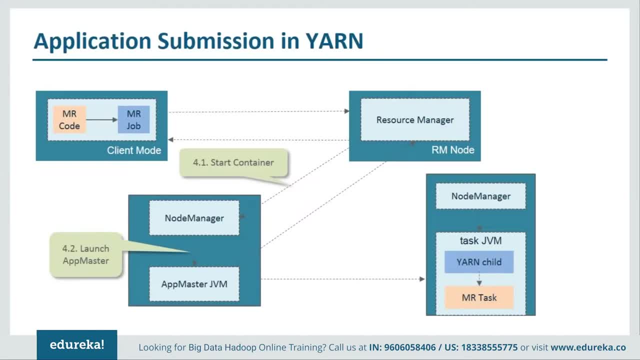 established, using which your client can see the application status. in response to the registration request, the application master will send information about the minimum and maximum capabilities of the cluster. at this point, the application master must decide how to use the capabilities that are currently available, based on the available capabilities reported from the. 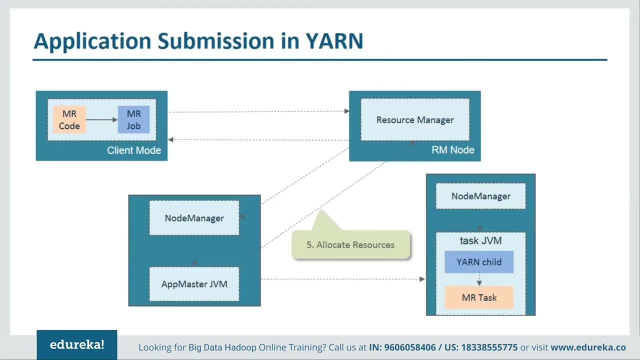 resource manager. The application master will request the number of containers. the request can be very specific, including containers with multiple of resource minimum values. the resource manager will respond as best as possible to the request with container resources that are assigned to the application master. As a job progresses, heartbeat and process, information is sent from the 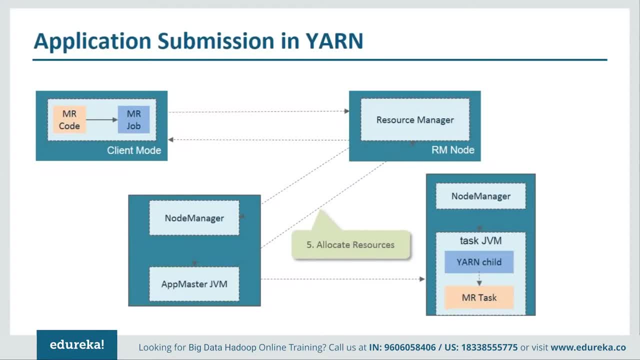 application master to the resource manager. within these heartbeats, It is possible for the application master to request and release containers. when the job finishes, the application master sends the finished message to the resource manager and exits. next is application master and container communication. at this point, 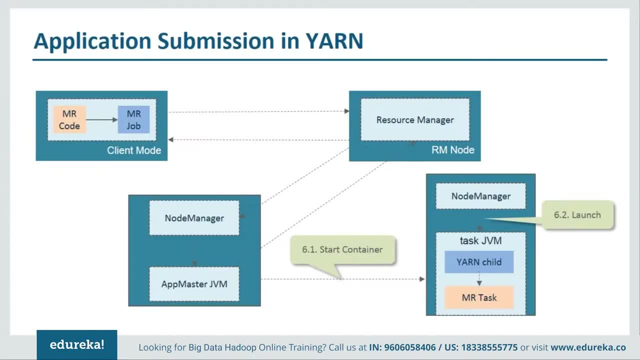 The resource manager has handed off control of assigned node managers to the application master. The application Master will independently contact its assigned node managers and provide them the container launch context that includes involvement, variables, dependencies located in its remote storage, security tokens and commands needed to start the actual process. next, the node manager launches the. 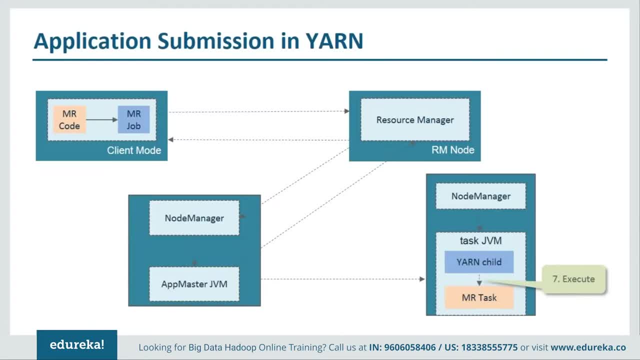 container. when the container starts, all data files, executables and necessary dependencies are copied to local storage on the node. dependencies can potentially be shared between containers running the application. once all container have started, Their status can be checked by the application master. the resource manager is absent from the application progress and is free to schedule and. 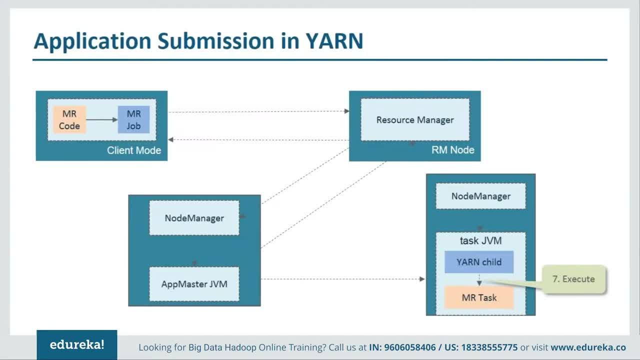 monitor other resources. The resource manager can direct the node manager to kill containers. expected kill events can happen when the application master informs the resource manager of its completion or the resource manager needs nodes for other applications. When a container is killed, the node manager cleans up the local working. 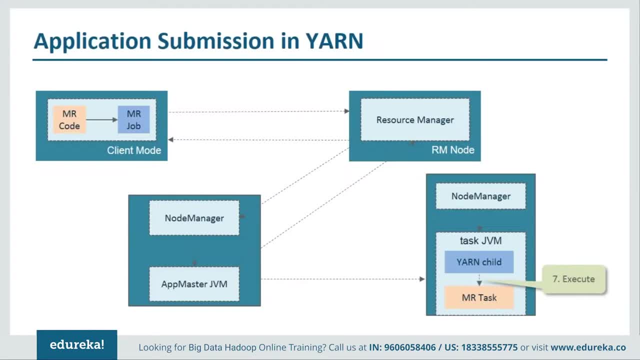 directory. when a job is finished, The application master informs the resource manager that the job is completed successfully. the resource manager then informs node manager to aggregate logs and clean up container specific files. The node manager are also instructed to kill any remaining containers, including the application master, if they have not already exited. now let us quickly move. 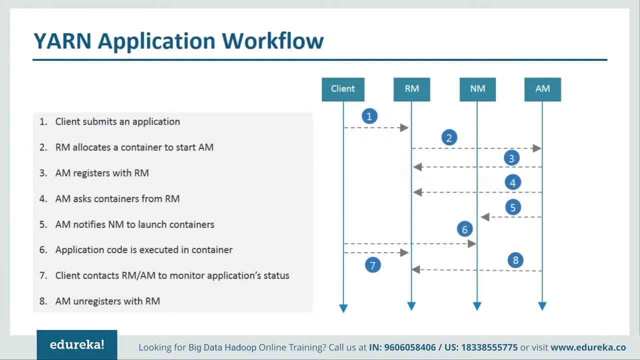 ahead and look at the summary of the yarn application workflow. So first, client submits an application to the resource manager. then resource manager allocates the container And starts the application master. then application master registers the container with resource manager. second, the application master asked for the. 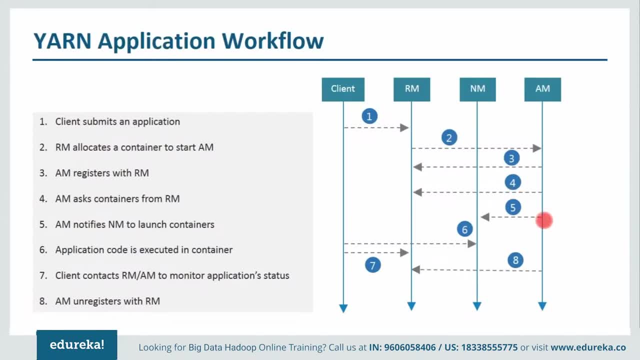 containers from resource manager. moving ahead, application master notifies node manager to launch containers. application code is executed in containers. then client contacts resource manager and application master to monitor the application health. at last, application master and registers with the resource manager and leaves all the resources acquired by it. 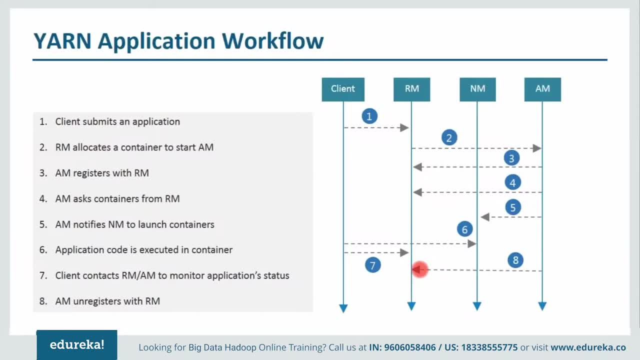 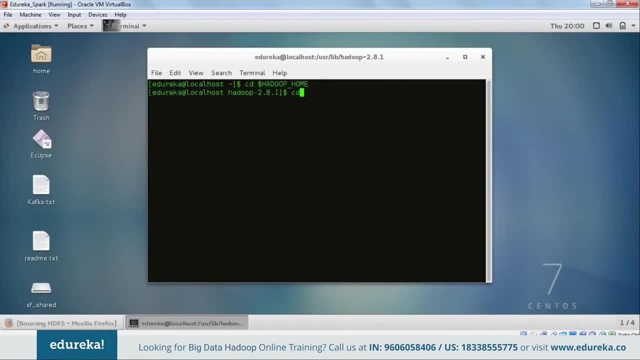 So let us now quickly understand how yarn works. Let's go to VM. So this is our VM. I'll be executing a simple word count example. So let us go to our Hadoop home in share Hadoop MapReduce. So we have a sample Hadoop MapReduce examples. 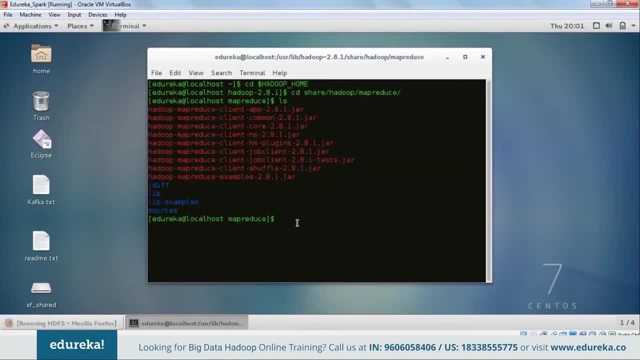 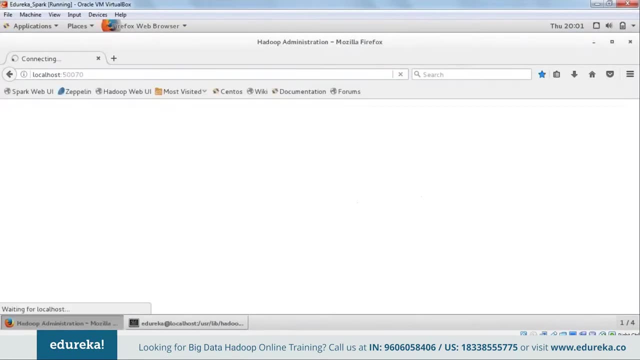 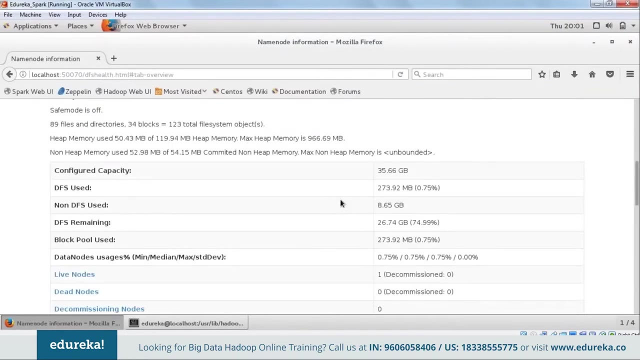 So in this chart we have a word count file which we can execute and check the status of yarn. But before that I'll show you The HDFS. So this is the HDFS. You can see we have one data node. Let us browse the file system. 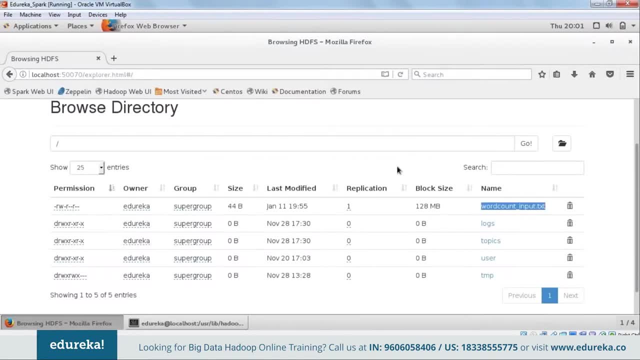 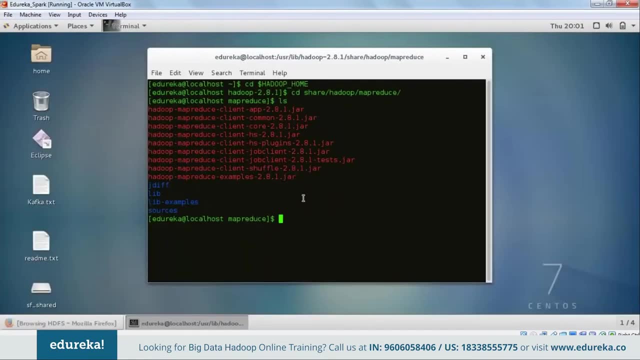 So this is the word count. underscore: input dot txt file which I'll be giving as input for the word count. If you are not having any file on your HDFS, you can go ahead and execute put command. So let us quickly go ahead and execute this command. 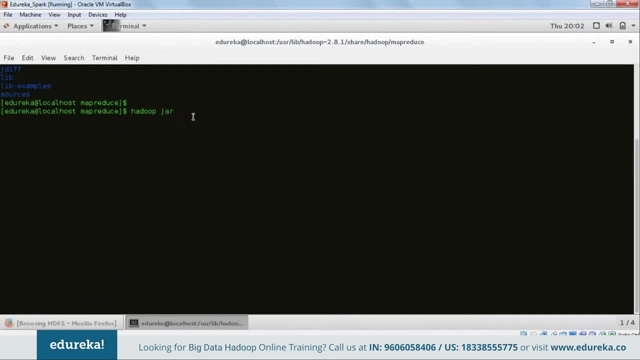 The command is Hadoop jar, Then the name of the jar file that is Hadoop MapReduce examples. The name of the class is word count And then we'll give the input file, that is- let me tally it- word count, underscore: input dot txt, and the output files will be stored in output directory, which is in the root. 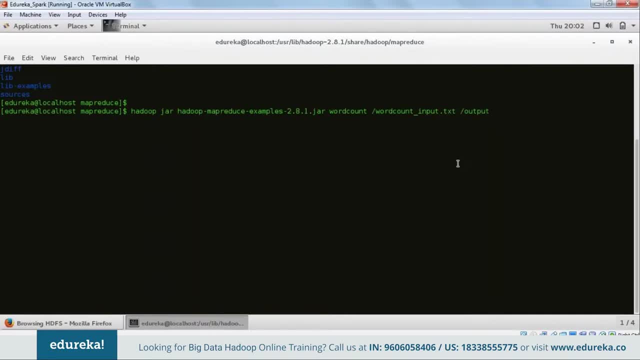 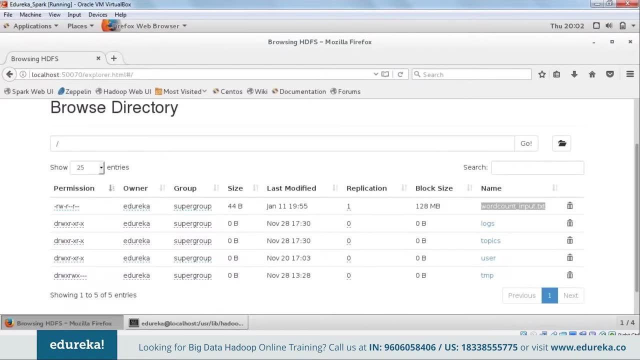 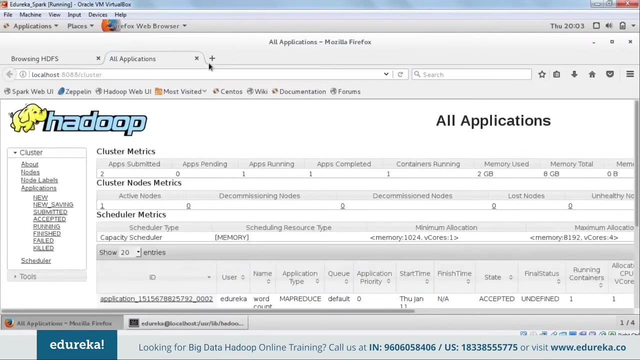 of HDFS. So let us quickly go ahead and execute this command. Meanwhile, we'll go to our yarn web UI. That is eight zero 88.. So this is the yarn web UI. As you can see, this is the application that we're executing. 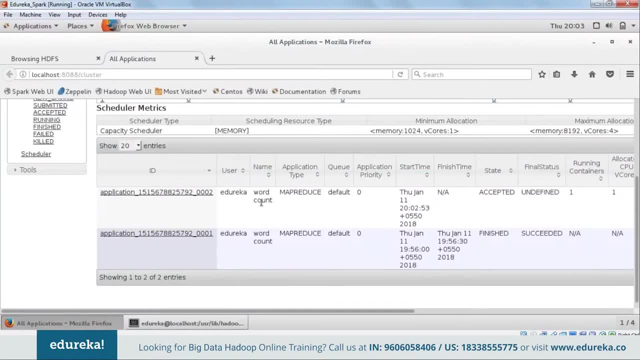 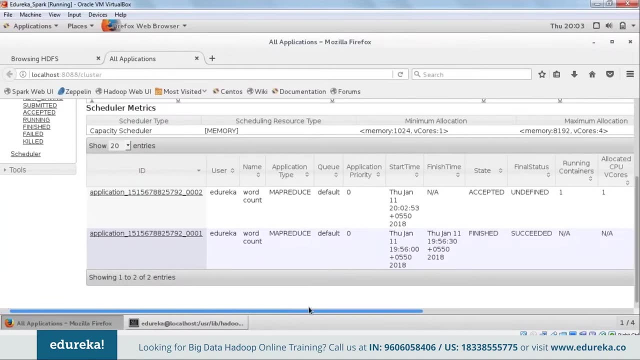 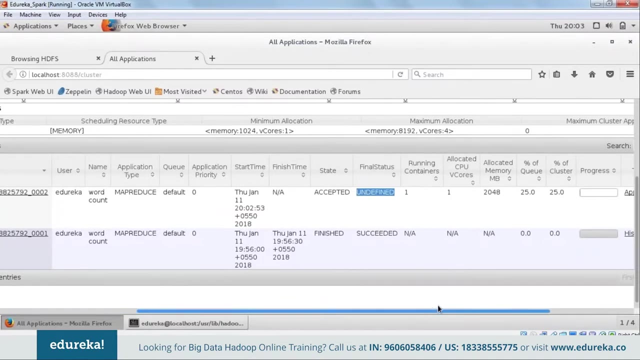 This is the application ID. the user to the name of the application. That is word count. type of application: Again, the status is accepted. final state is undefined. There is one container running a located CPU. V course is one, And here you can track the progress. 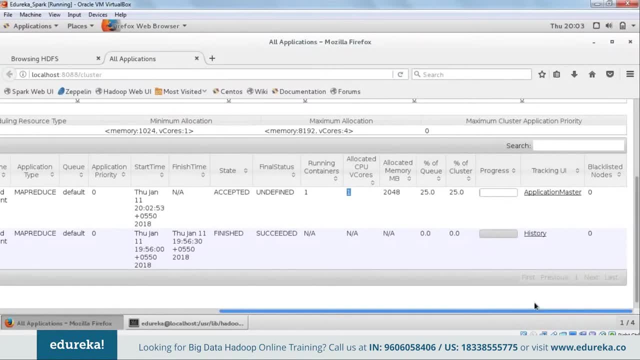 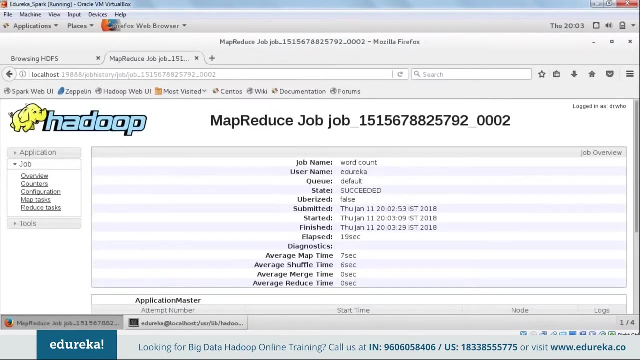 Of the application. This is the tracking UI. Let us go to the tracking UI. So, state is succeeded. Let us go back to our terminal. as you can see, the program has been successfully executed. You can also see the parameters over there, like number of bytes to be read. number of bytes. 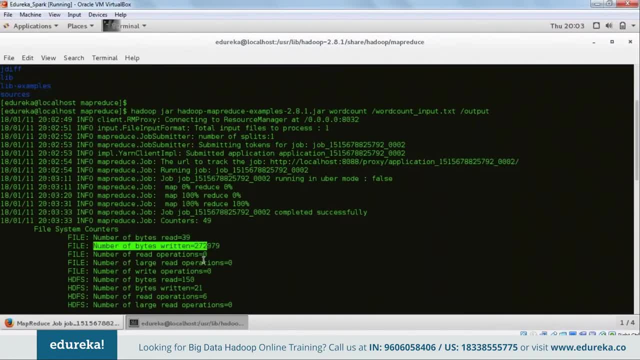 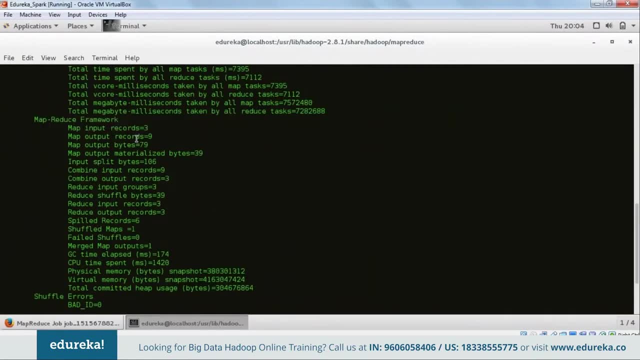 to be written. number of read operations. the number of write operations. again, you can figure out the MapReduce framework: How many number of map input record, some of my output records, And then we have all the MapReduce details over here, So let's not worry about them. 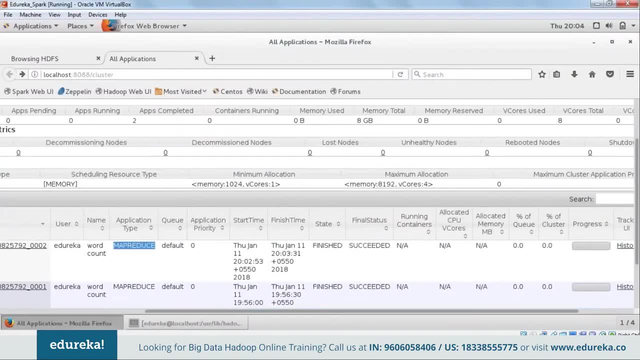 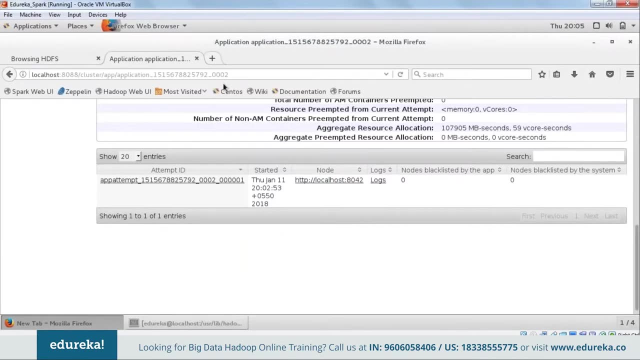 So it gives you all the details related to that job which you have executed. You can see the log files that has been created while executing this job. You can also track it on your web history server That is localhost for 9888. 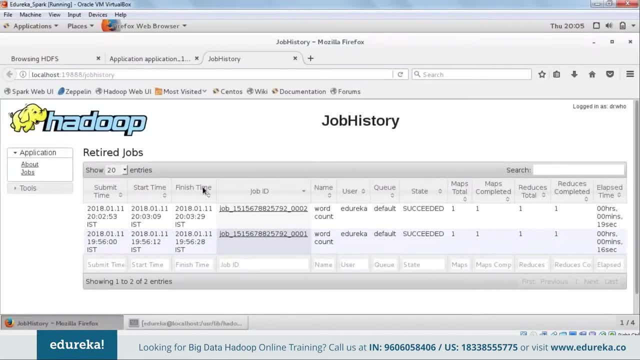 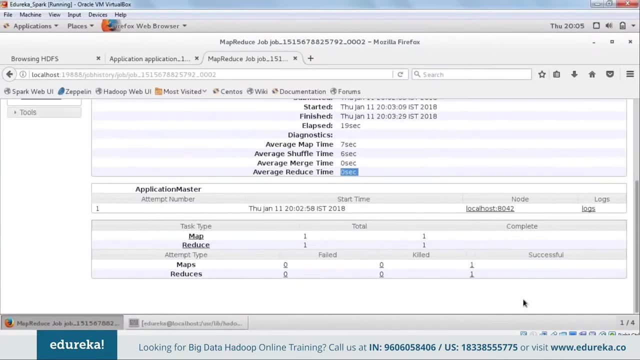 So again you can see this word count job and you can again track the details that average map time, shuffle time, average reduce time. So these are the details, guys. Let us go to that STFS browser and look at the output file that has been created. 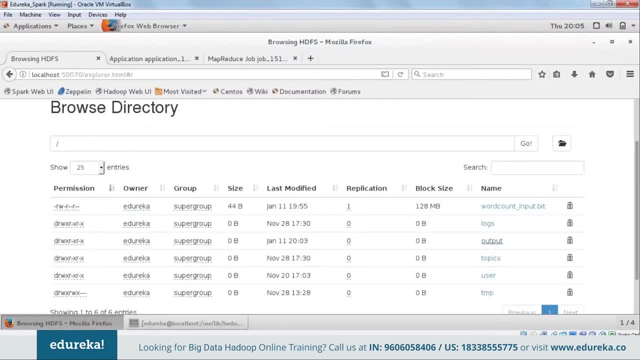 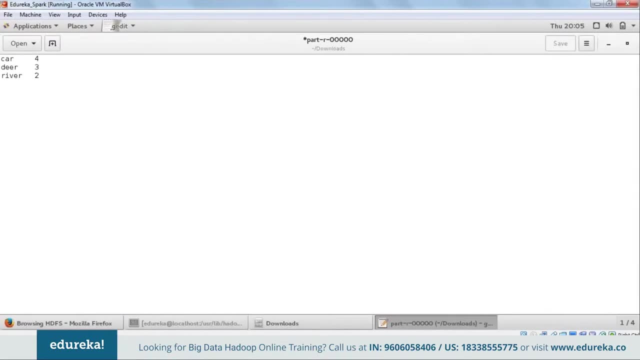 So this is the output file. Let's go ahead and download it. So, as you can see, the number of count for car is 4, deer is 3 and the river is 2.. So this is the output that we received. I've given a simple input file. 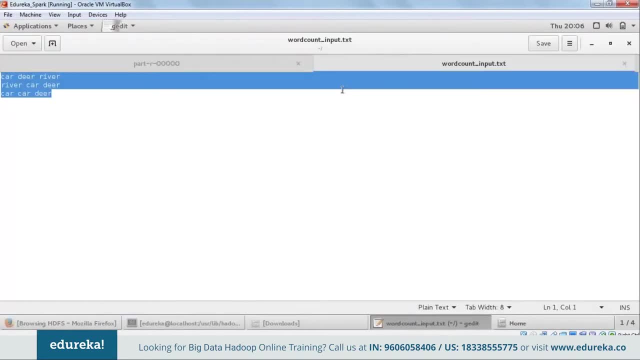 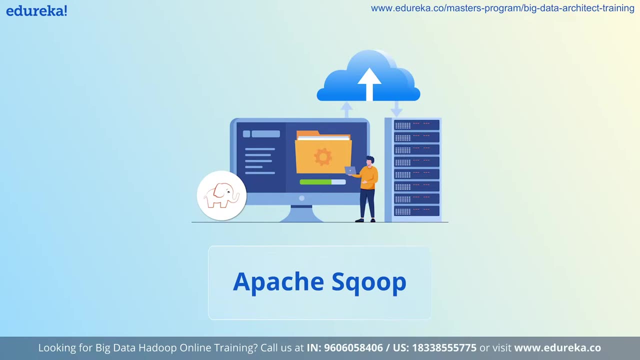 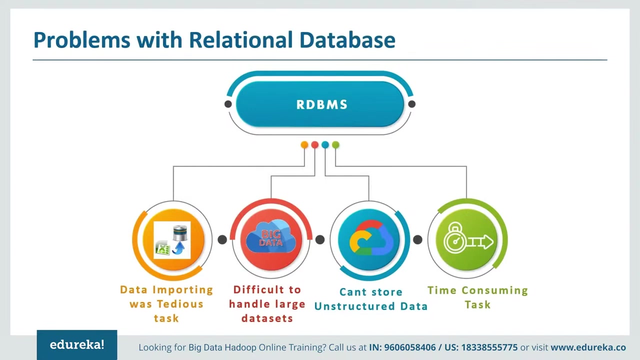 Let me show you the file as well. This is the input which we have given and this is the output which we have received. So what were the problems associated with the relational database system? as I have already mentioned that, for a Hadoop developer, actual game starts after the data is being loaded in HDFS. 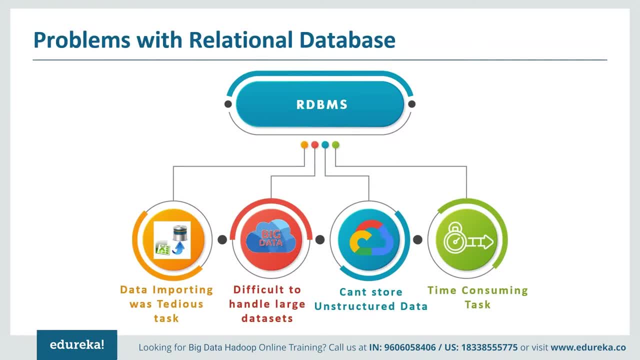 and the developers play around this data in order to gain various insights that are hidden in the data stored in HDFS. So for this analysis, the data residing in the RTB MS needs to be transferred to HDFS, and you all know that the task of writing MapReduce code. 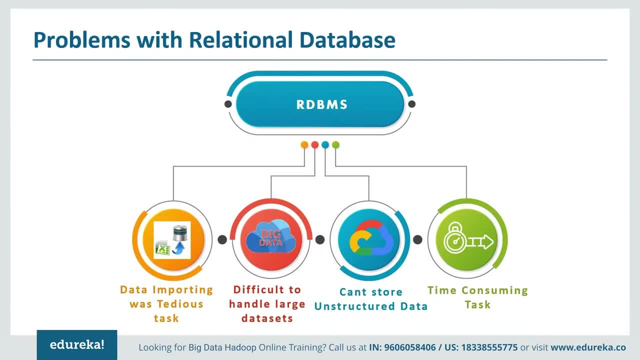 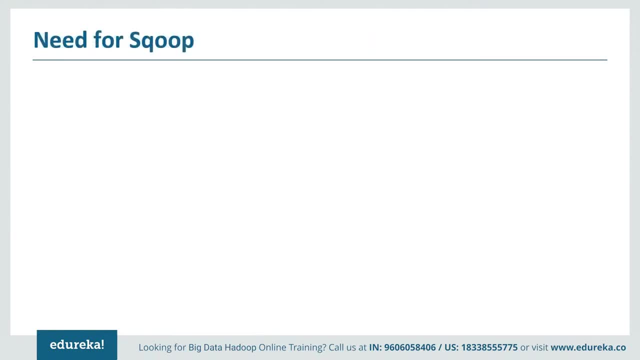 for importing and exporting the data from relational database to HDFS is tedious. So this is where Apache scoop comes to rescue and remove the pain of data ingestion. So why do we need scoop? It's a known fact that before big data came into existence, 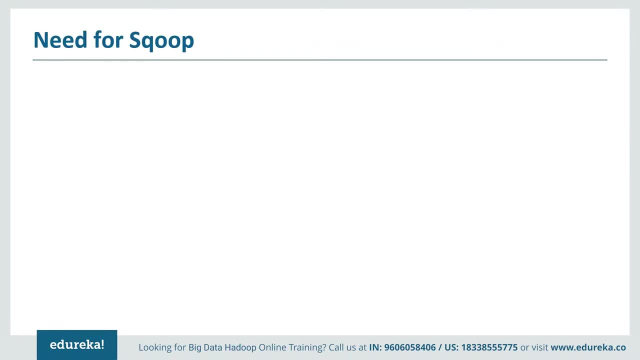 The entire data was stored in relational database servers and the relational database structure, but with the advancement of school it makes the life of developers easier By providing CLI for importing and exporting the data and scoop internally converts a command into MapReduce task, which are then executed over HDFS. 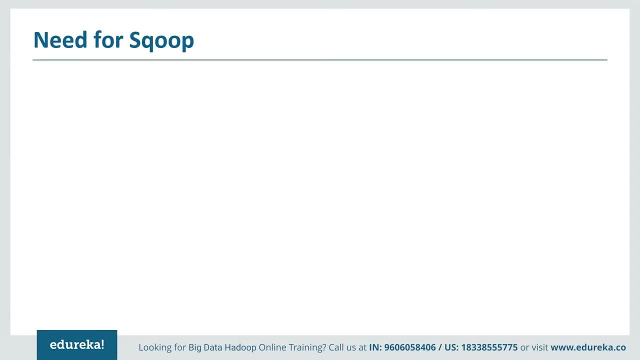 It uses yarn framework to import and export the data which provides fault tolerance on top of parallelism. It also uses yarn framework to import and export the data which provides fault tolerance on top of parallelism. Not only that, it is also very useful for data analysis high. 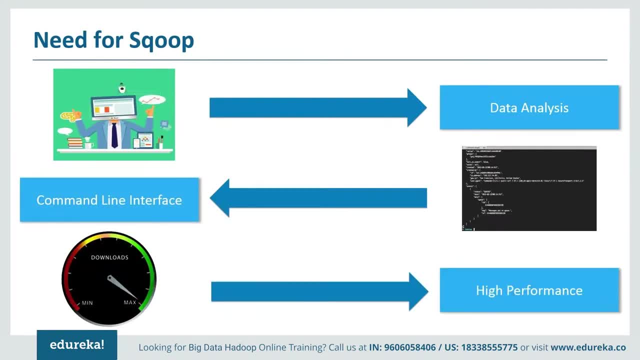 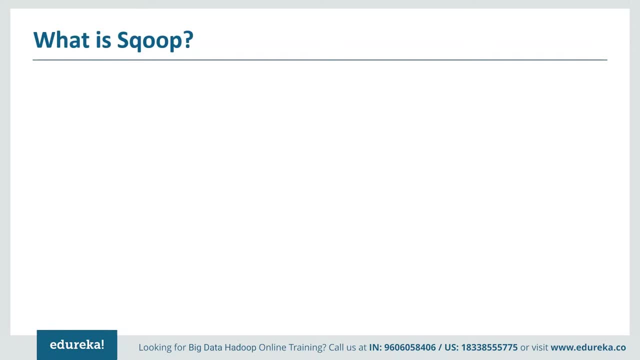 in performance and provides command-line interface. Now let's understand what a scoop. So before I tell you what a scoop, let me tell you how to name. scoop came into existence by now. I hope that you have got an idea that it is used. 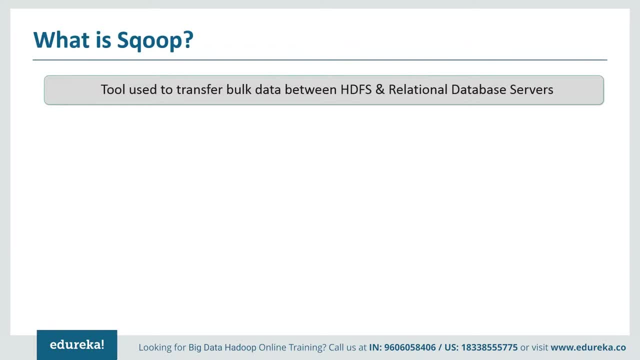 for data transfer between relational database and HDFS. So before I tell you what a scoop, let me first tell you how the name came into existence. The first two letters in school stands for the first two letters in SQL, and the last three letters in scoop refers to the last three letters in Hadoop. 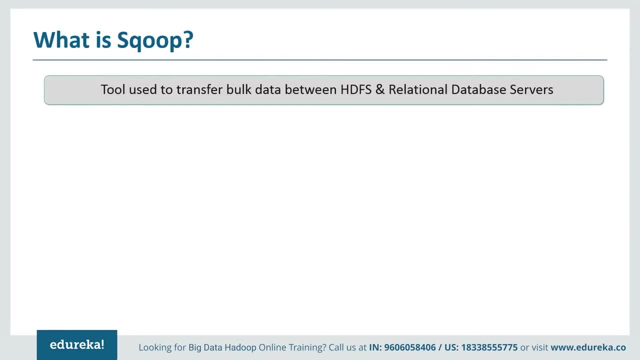 That is OOP, So it clearly depicts that it is SQL to Hadoop and Hadoop to SQL. that is how the name of scoop came into existence. So what is cool? It is a tool used for data transfer between our DBMS, like my sequel, Oracle, SQL, Etc, and Hadoop, like Hive, HDFS, HBase. 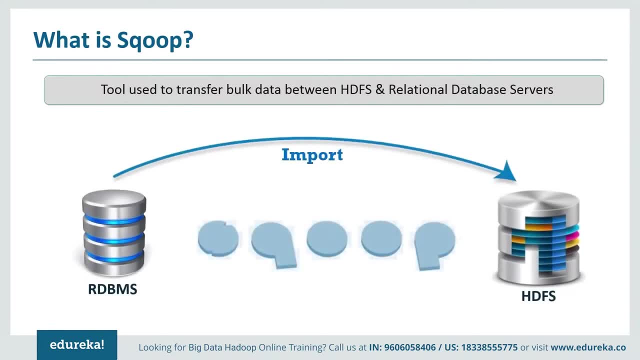 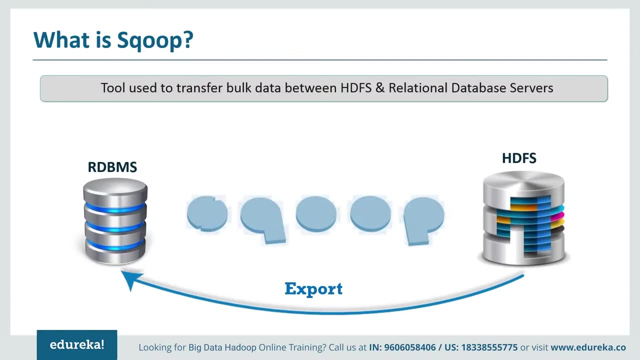 Etc. It is used to import the data from our DBMS to Hadoop and export the data from Hadoop to our DBMS. simple again. scoop is one of the top projects by Apache Software Foundation and works brilliantly With relational databases such as Terra. data net is the Oracle, my sequel, Etc. 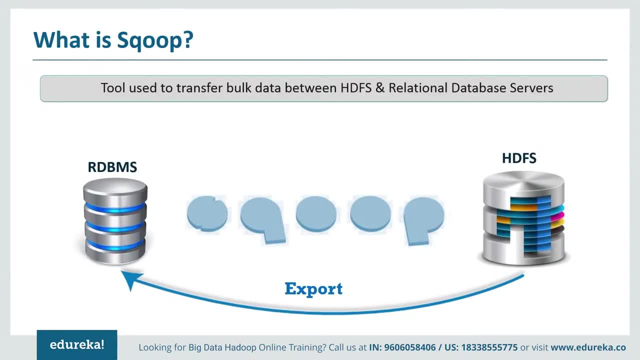 It also uses MapReduce mechanism for its operations, like important export work and work on a parallel mechanism, as well as fault tolerance. as I have already mentioned that, it provides command-line interface for importing and exporting the data. the developers just have to provide the basic information, like database authentication. 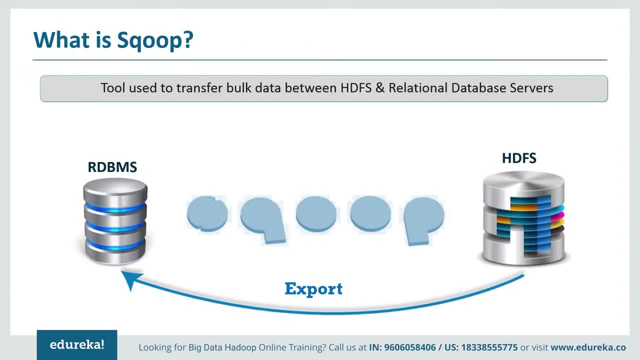 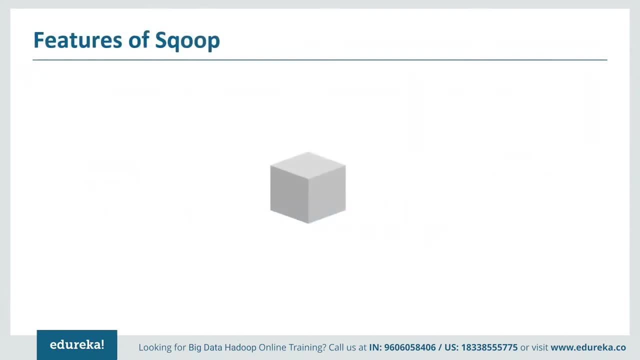 source, destination operations, Etc. and the rest of the work will be done by scoop tool itself. sounds much reliable, correct? Now let's move further and talk about some of the amazing features of school for big data developers. first, full load: Apache scope can load whole table by a single command. 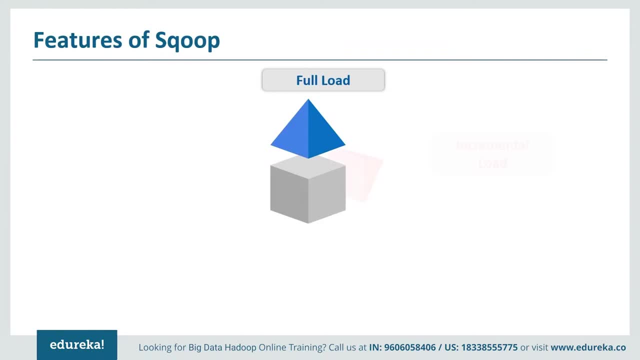 You can also load all the tables from a database using a single command. next, incremental load: school provides the facility of incremental load, where you can load the parts of a table wherever it is updated. next, paddle: import and export. again, as already mentioned, scoop uses yarn framework to import and export the data, which provides fault tolerance. 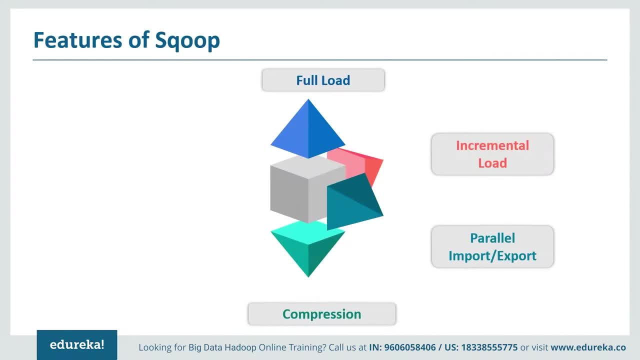 on top of parallelism. next, compression. You can compress your data by using gzip algorithm with compressed argument or by specifying compression codec argument. next, Kerberos: security integration. So what is Kerberos? It's a computer network authentication protocol which works on the basis of tickets to allow the nodes 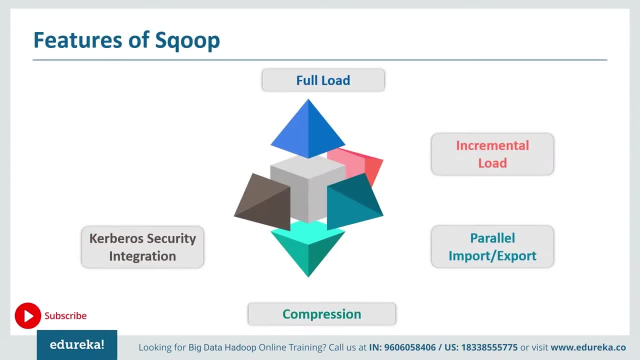 that are communicating over a non-secure network to prove their identity to one another in a secure manner. Next, load data directly into hive and HBase. here It is very simple: You can load the data directly to Apache Hive for analysis and you can also dump your data in HBase. 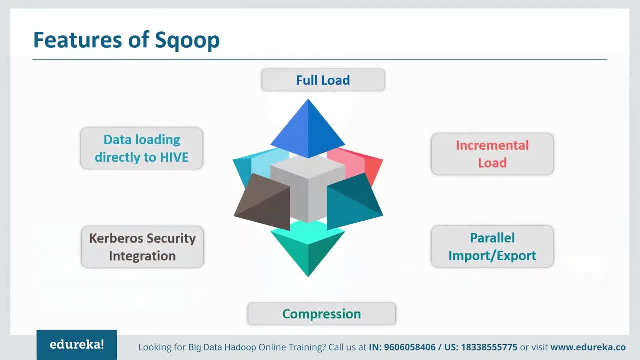 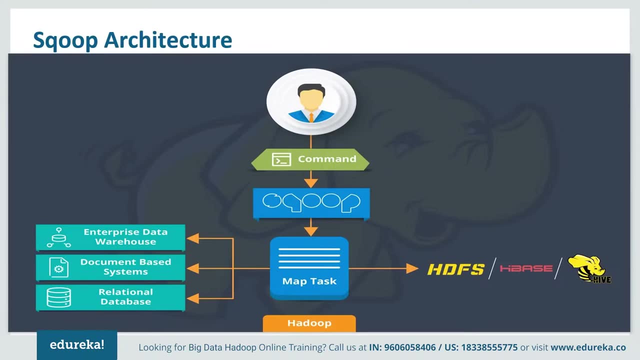 which is a no sequel database. Now let's see what's next. the architecture is one of the empowering Apache scope with its benefits. Now, as we know the features of Apache scope, let's move ahead and try to understand Apache scoops architecture and it's working. 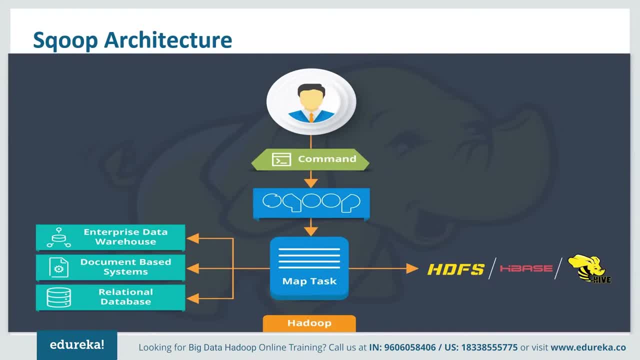 So when we submit our job or a command through scope, it is mapped into map task, which brings the chunks of data from HDFS and these chunks are exported to a structured data destination and, combining all these exported chunks of data, We receive the whole data at the destination. 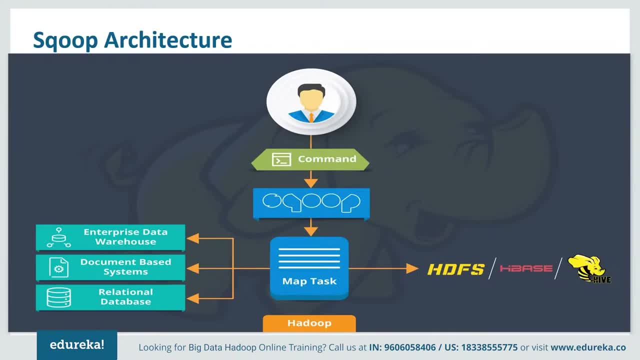 which in most of the cases is our DBMS server. next, reduce phase is required in case of aggregations, but Apache scope just imports and export the data. It does not perform any aggregations. map job launch multiple mappers depending on the number defined by the user. 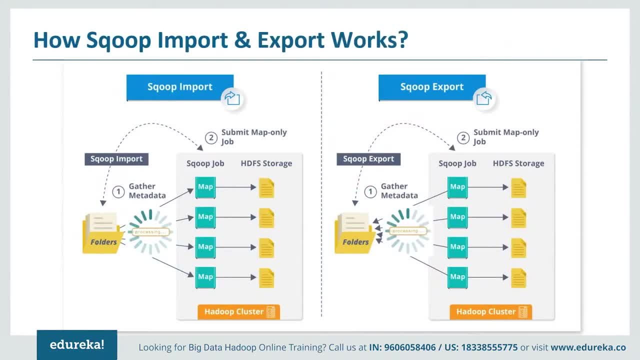 For scoop import. each mapper task will be assigned with the part of data that is to be imported, and scope distributes the input data among all the mappers equally in order to achieve high performance. Then each mapper creates a connection with the database using gdbc and fetches the part of the data assigned by the scoop. 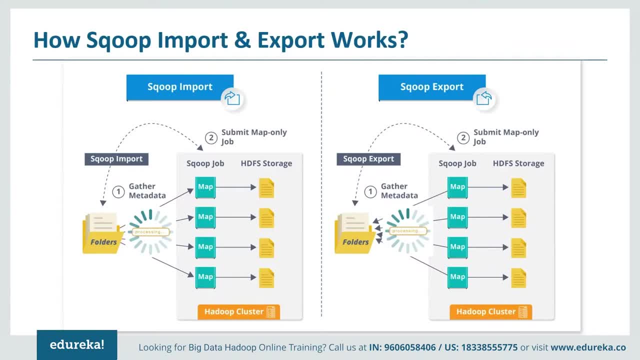 and then writes that data to HDFS, Hive or HBase based on the arguments provided in the command line interface. So this is how scope import and export works, like they gather the metadata Again, it submits only map job. The reduced phase will never occur here. 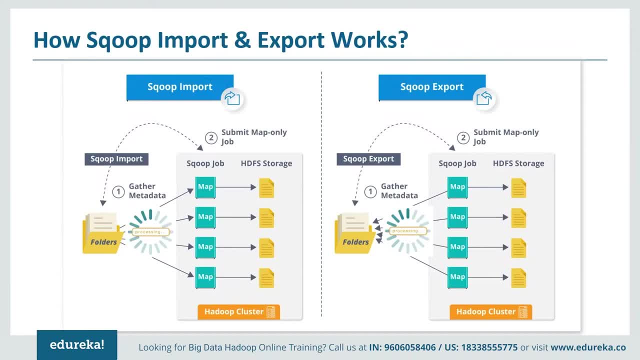 and then it stores the data in HDFS storage. coming to scoop export, It's the same thing: The data will be reversed back to our DBMS. So here the scoop import tool will import each table of the RDBMS in Hadoop and each row of the table will be considered. 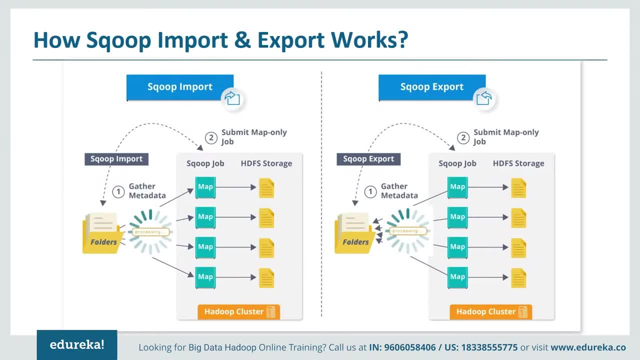 as a record in the HDFS and all the records are stored as text data in the text files or binary data and sequence files. On the other hand, the scoop export tool will export the Hadoop files back to the RDBMS tables. Again, the records in the HDFS files will be the rows of a table. 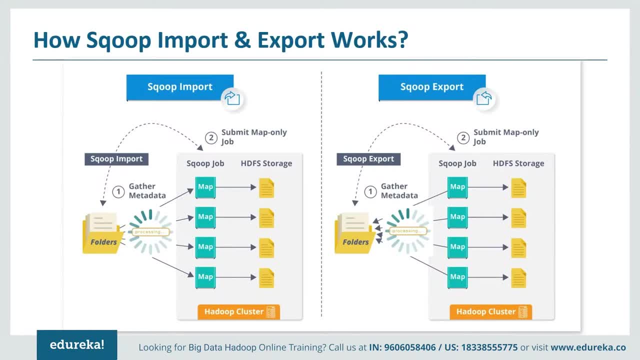 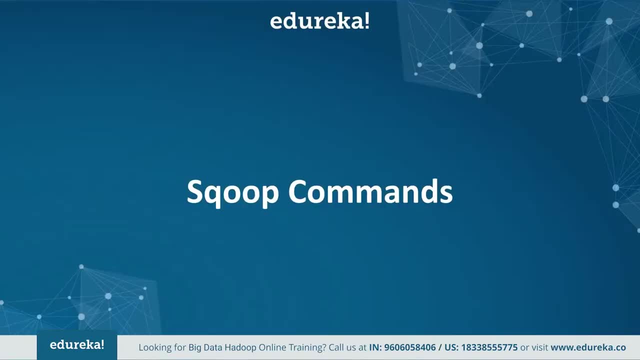 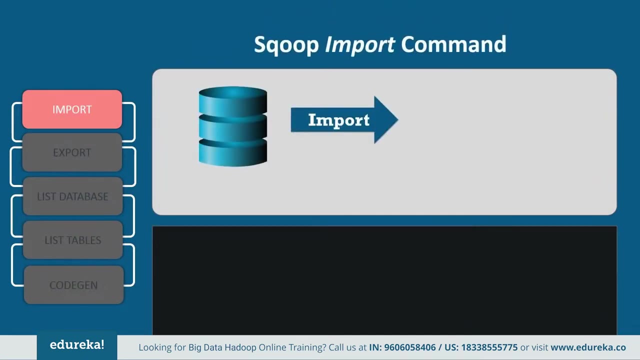 and those are read and passed into a set of records and delimited with the user specified delimiter. So this is all about the scoop architecture and its import and export. now let's execute some scoop commands and understand how it works. So at the first we have scoop import, that is, it imports the data. 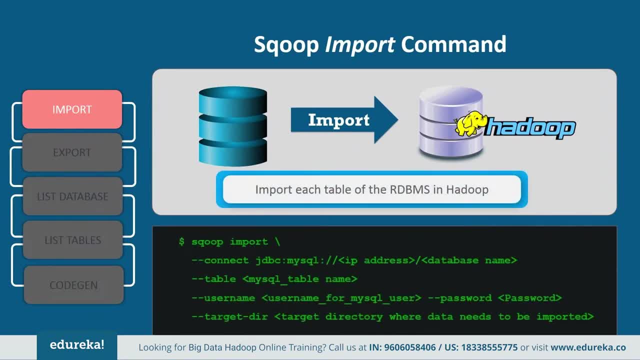 from our DBMS in Hadoop. the command goes very simple here. You have to just provide the connection for my sequel, your IP address, your database name, your table name, the username for my sequel user. If you have set privileges for password, you can specify the password or it is not required. 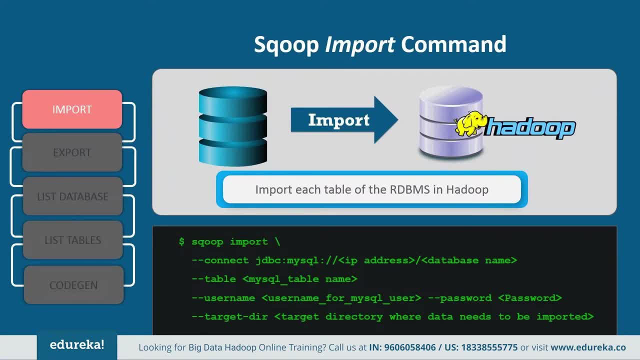 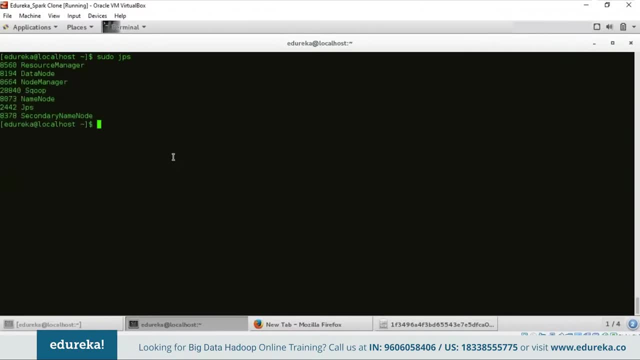 and the target directory. now let's see how to execute. So I'll open my terminal and check whether all my Hadoop demons are up and running or not. So I can see that all my Hadoop demons are up and running. So now let's execute: scoop help and see whether the scoop 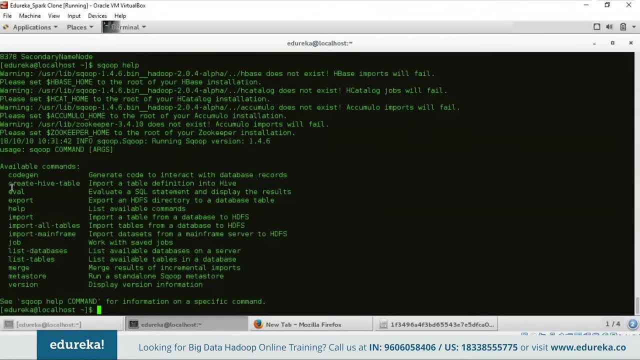 has been properly installed or not. So these are the available commands in school. here I will show you the execution and explain you few of these commands. now This is also properly being set. now I will open another terminal and connect to my sequel database. 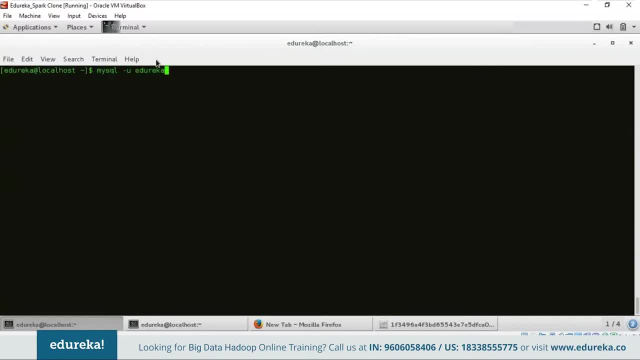 The command goes like this: My user is a Durica, So I'm giving it as a Durica. You can give it as root if your user is root, simple. So now I'm into my sequel database, If you want to create a database. 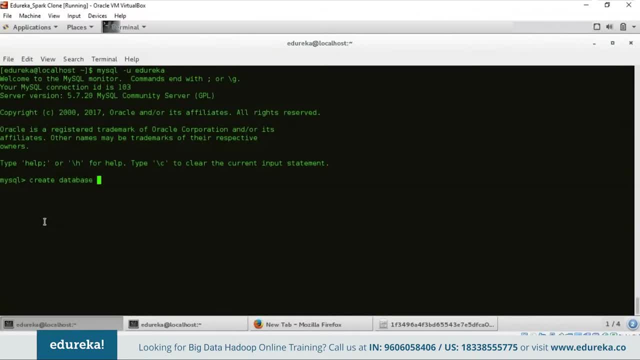 you can create a database by giving this command: create database, database name: Etc. as I have already created a database, So I'll just specify show databases command to list the database present in the my sequel database. So now these are the list of database present here. 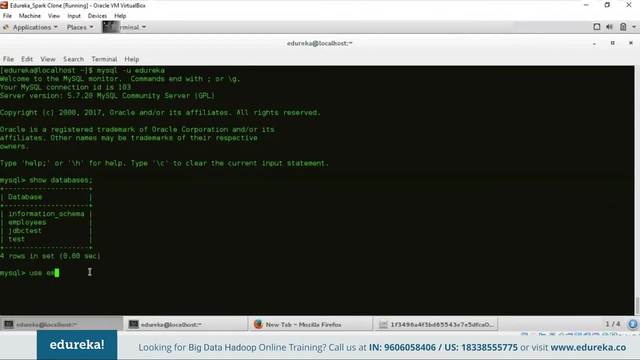 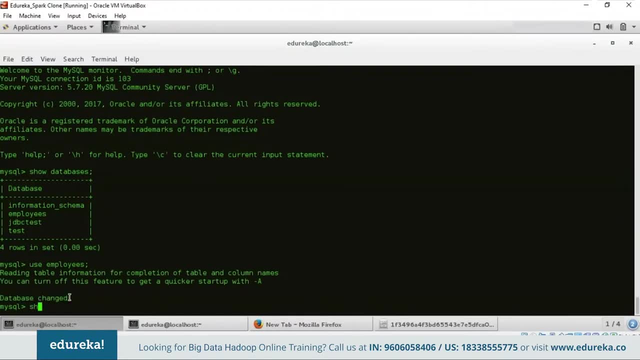 So now I want to use the employees database, So I'll give use. employees database got changed. Now I want to list the tables present in the employees database So I'll give show tables. So these are the 11 tables present in the database: employees. 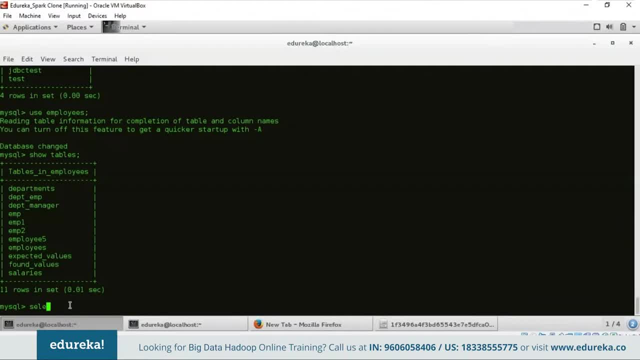 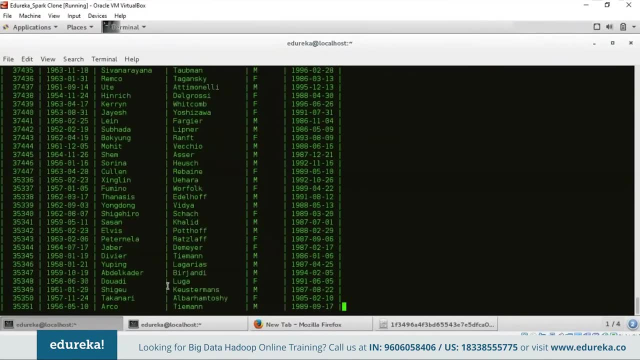 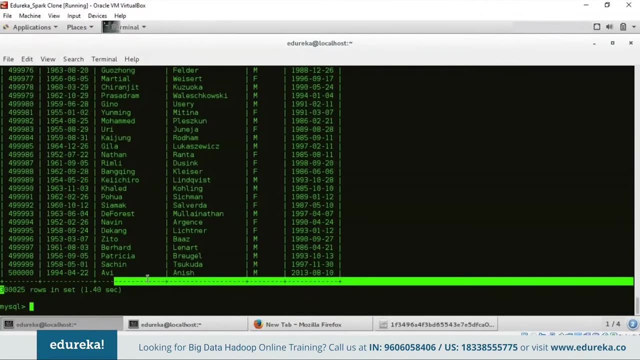 Now let's say I want to use employees table. So what will I do? I'll just give select star from employees. that is table name. So it's just a huge amount of data that is present in this database. So there are these many rows present in this table. now open. 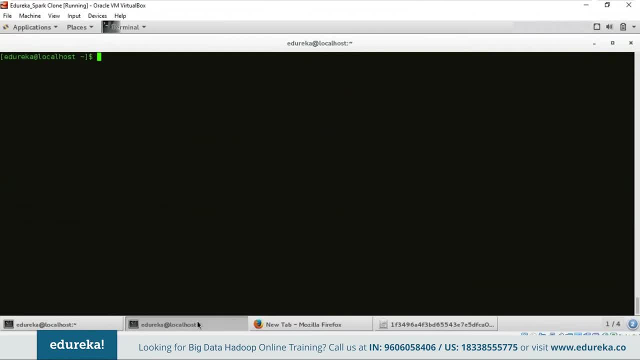 the other terminal where you have executed this command, and here I will show you how to import the data present in that table to HDFS. So how we are going to do that? by using scope import command. the command goes like this: The IP here is local host. 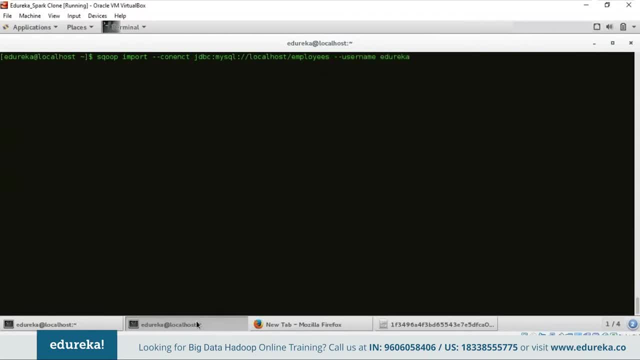 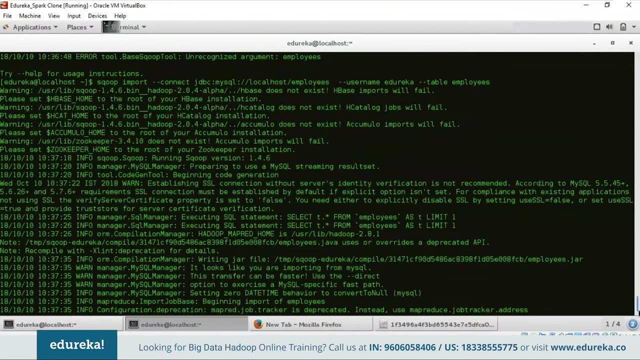 and you know that employees is my database name and the username will be a durica And the table that I have chosen is employees. So I have not set any privileges for password, So I'm not specifying the password over here. So it got executed. 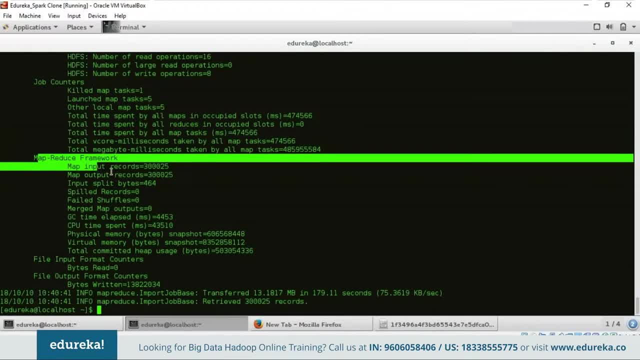 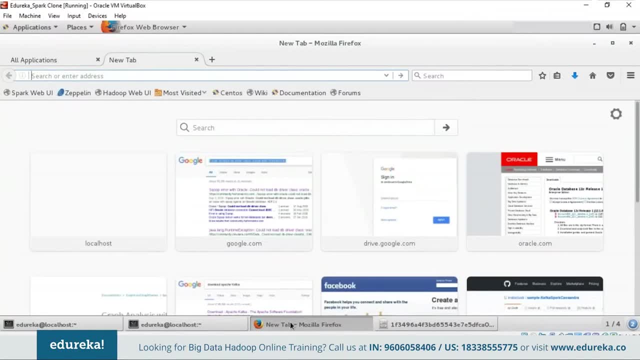 and you can see the number of job counters, the MapReduce framework, the input records, output records, etc. So what happens after executing this command? the map task will be executed at the back end. Now let's check the web UI of HDFS. 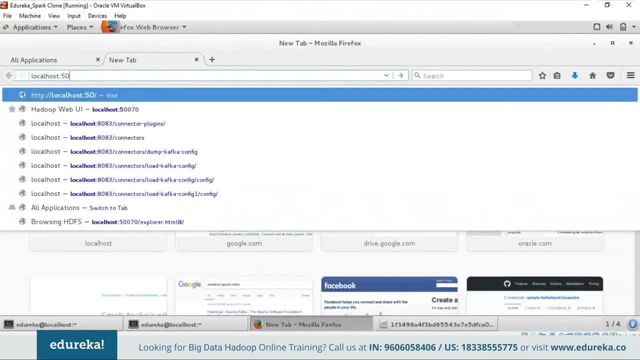 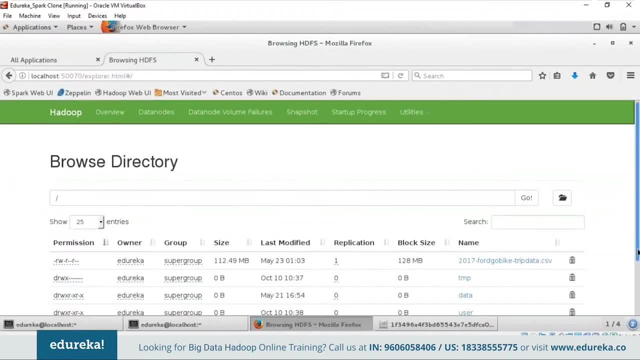 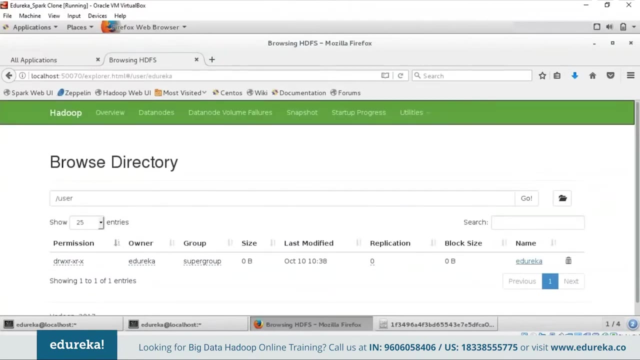 That is the web UI. code for HDFS is localhost 50070 and let's see where the data got imported. One important thing to note: I have not specified target directly, So by default the data will be imported to this folder. user: a durica and employees. 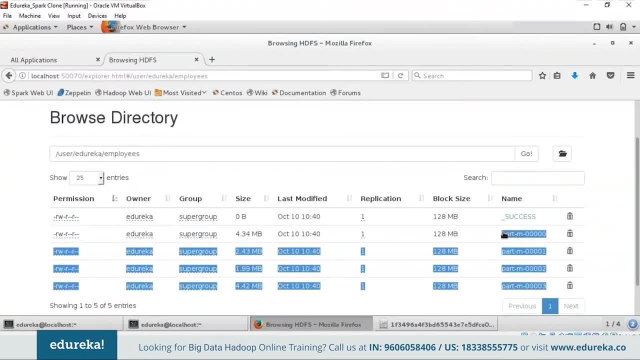 So here you can see the four different part files where our data got imported. So you might be thinking why, for correct here I have not specified the number of mappers, So by default it takes the number of mappers to three and then gives the output in four different part files. 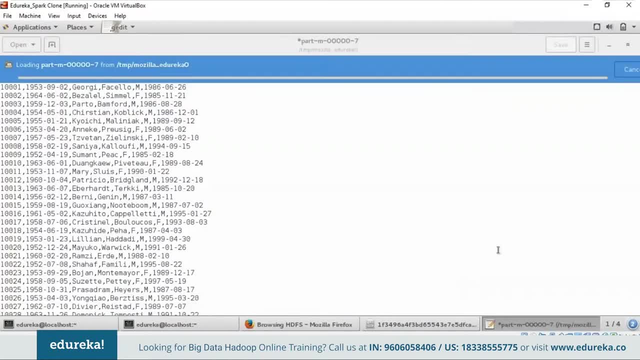 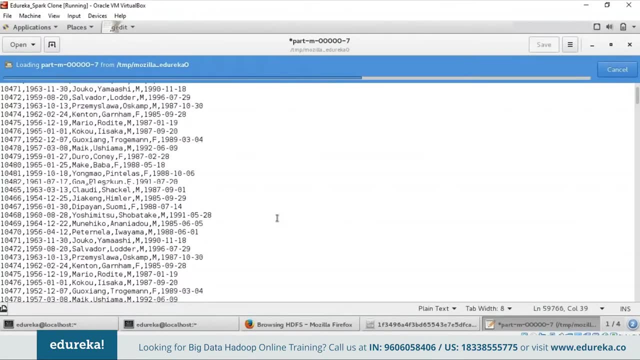 So let's open the part file and see how the output will be. So here you can see the data is imported from our DBMS to HDFS. There's lots of data being present over here. I'm just scrolling down and it's not coming to an end. 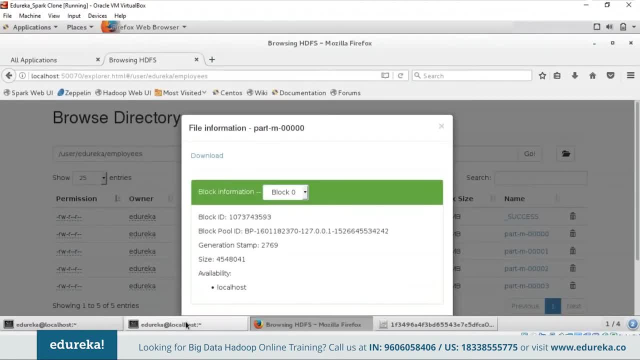 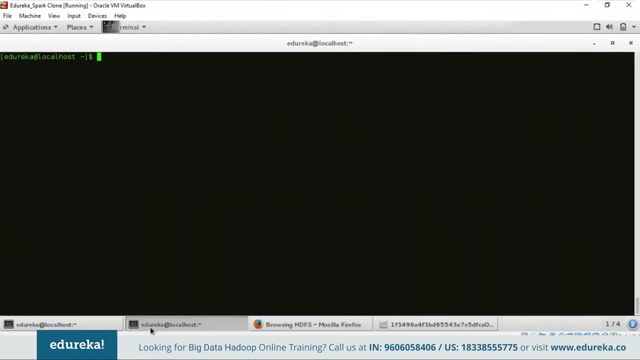 Similarly, the output will be same in the other part files as well. So this is all about the simple scope import command without specifying the target directory and the number of mappers. Now let's see how to import the data from our DBMS to HDFS by specifying the target directory. 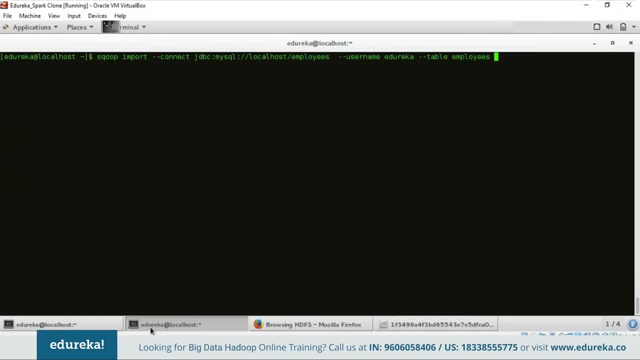 This part remains out to be the same. now I will do one thing: I specify the number of mappers as one, so that your output will be in just one single part file, and then I will specify the target directory as well, And I will name the target directory as employee 10 enter. 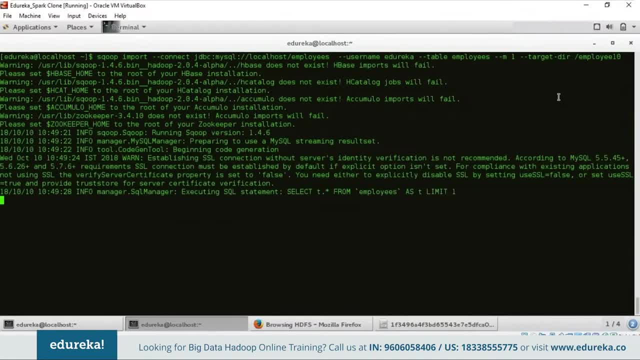 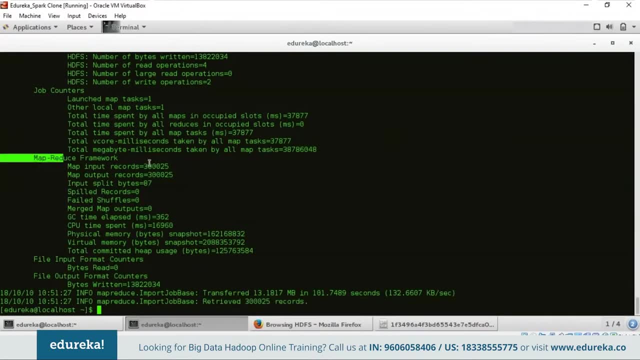 again, It takes a lot of time to execute because there is a lot of data present in the database. So it got executed and retrieve these many records again. You can see the MapReduce framework, the number of bytes. written Number of read operations. write operations. 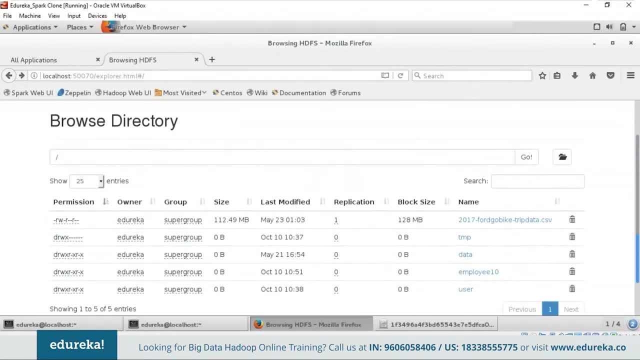 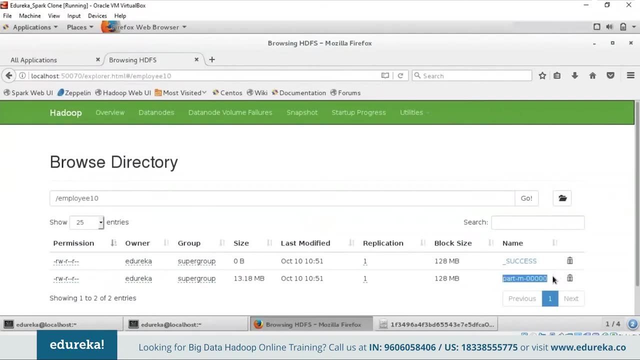 etc. Now again, let's go to the HDFS browser and see the output. So I had specified the target directory name as employee 10, so you can see it here and the output is just in one single part file because I have specified the number of mappers as one. 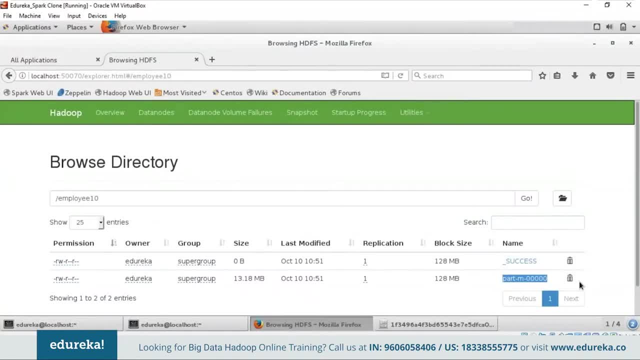 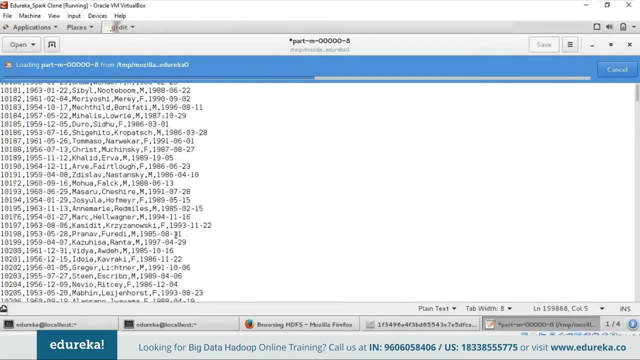 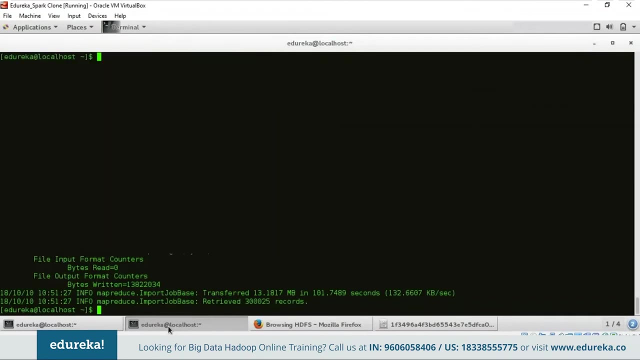 in this case you can control the number of mappers independently from the number of files present in the directory. So the entire records will be present in one single part file. So this is output. now let me tell you how to import the command using where clause. 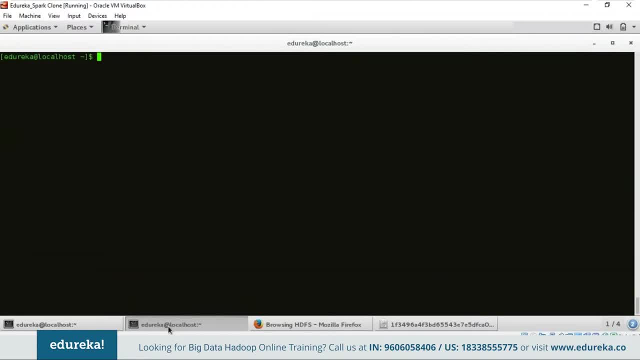 here you can import a subset of the table using the where clause and scoop import tool. It executes a corresponding SQL query in the respective database server and stores the result in a target directory in HDFS. So this is how the command goes, the same command as before. 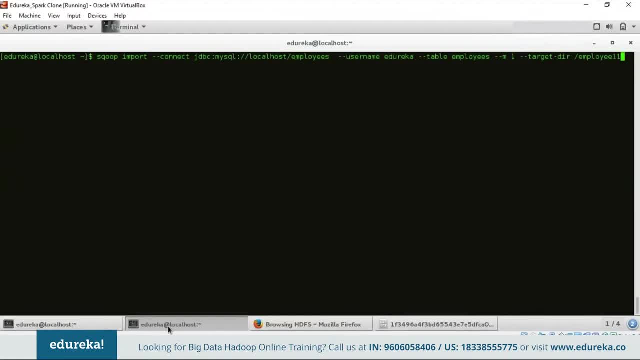 I'll just change the name of the target directory, I'll specify employee 11 and I will increase the number of mappers to 3, and here I will specify the where clause. So let's give a condition like where the employee number will be greater than 49,000. 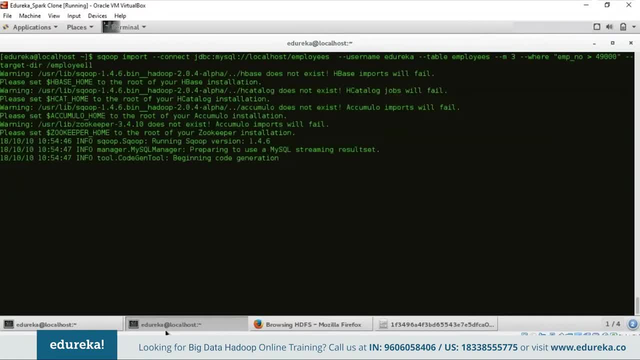 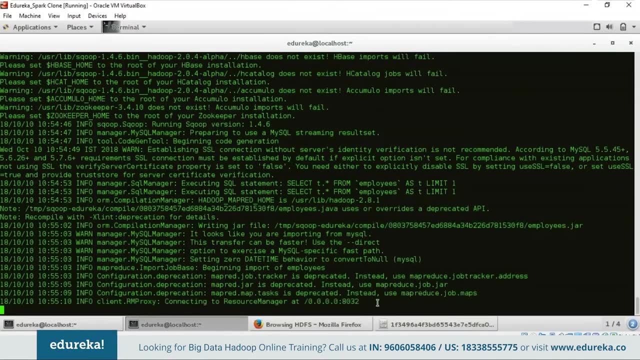 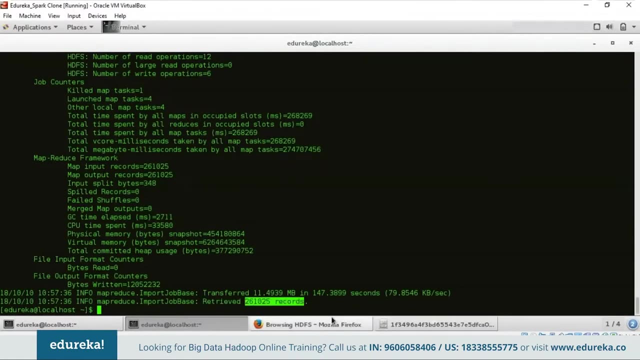 It should display the output enter. So what you expect, your output will be so here at this place, the output records of the employees whose employee number is greater than 49,000.. So here it retrieved these many records which are about the employee number 49,000.. 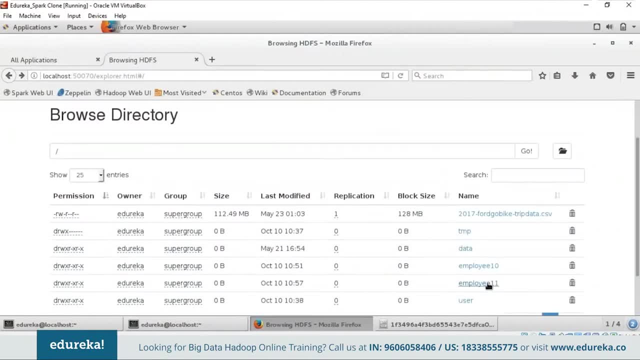 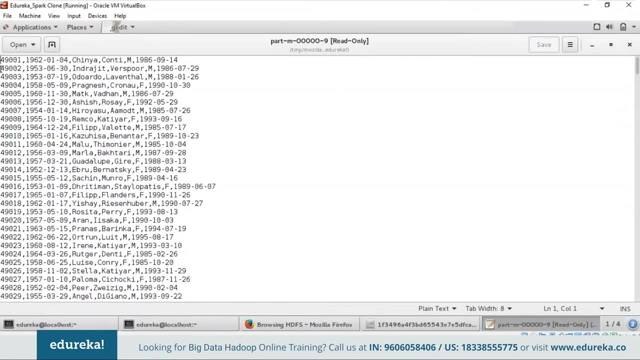 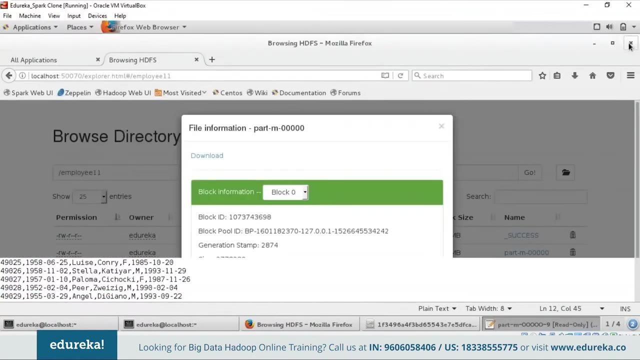 Now let's check the output. So I have specified the target, The directory name, as employee 11.. So here you can see the output that it has retrieved the records of employee number, which is more than 49,000.. So I hope you understand how to do this next. 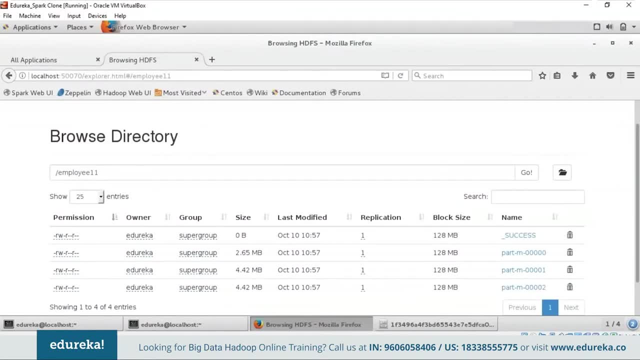 Let's see how to import all the tables from the rdbms database server to the HDFS. here Each table data is stored in a separate directory and the directory name is same as a table name. It is mandatory that every table in that database must be. 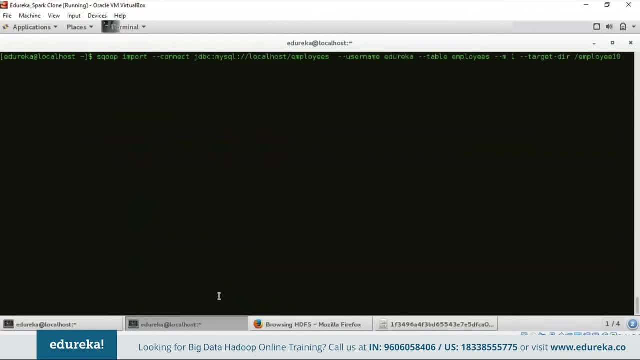 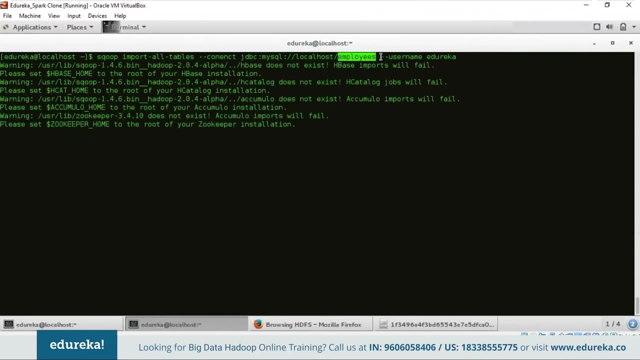 have a primary key field. The command will be simple, like simple import, but just said you have to remove the table name and you have to replace the import with import all tables, That's all. So it will retrieve all the tables present in the employees. 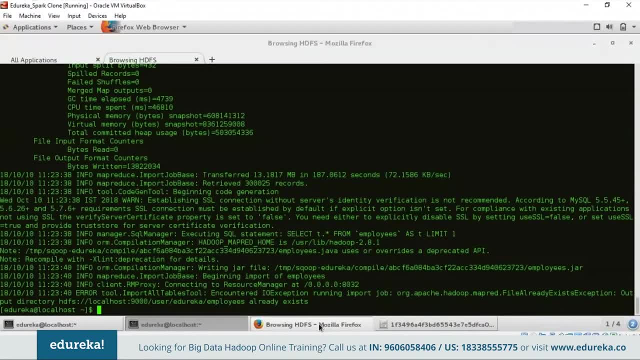 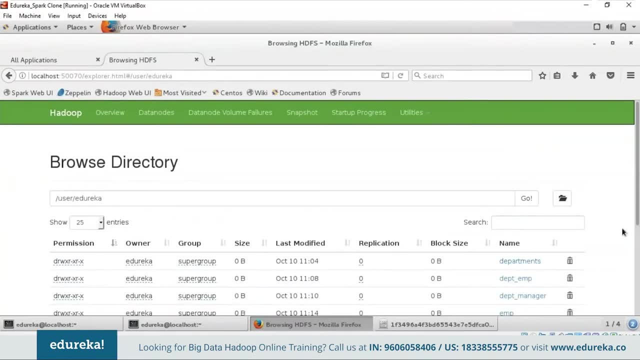 Okay, so it imported all the tables from rdbms to HDFS. Now let's check the output Again. I have not specified the target directory file, So by default it will be in user at Eureka and you can see here. it imported all the tables present. 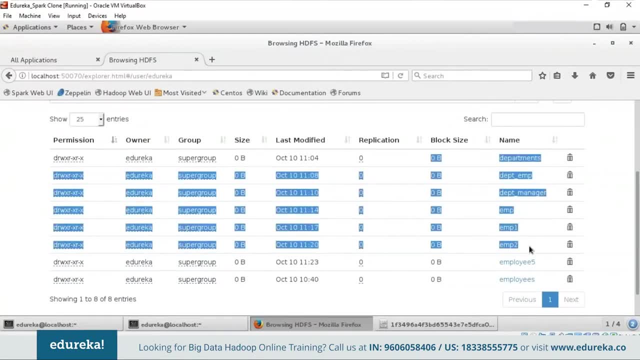 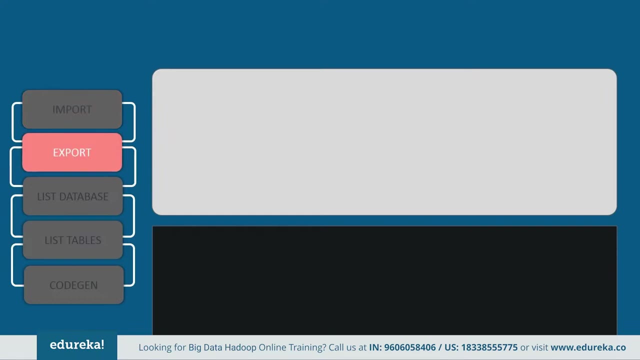 in the database to HDFS. So these are the various tables present in rdbms and now it is present in HDFS. So this is how import all tables command works. So this was all about executing import command in various ways. Now let's move further. 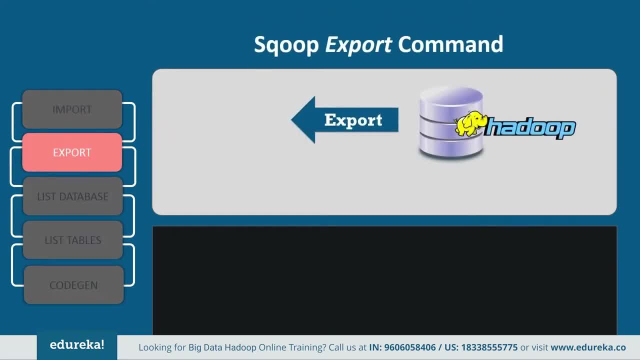 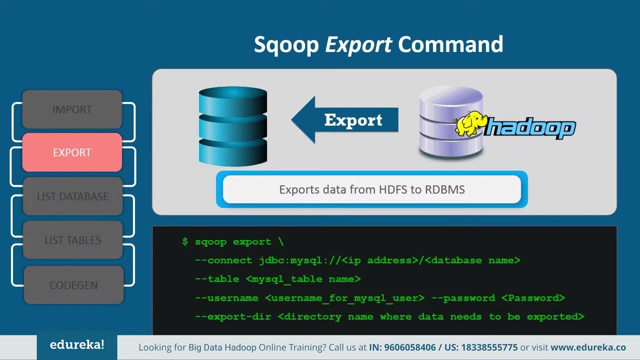 and see how does coop export work. It exports the data from HDFS to rdbms. correct Again. The command goes very simple. You have to specify the connection, your table name, username and instead of the target directory you have to specify the export directory path. 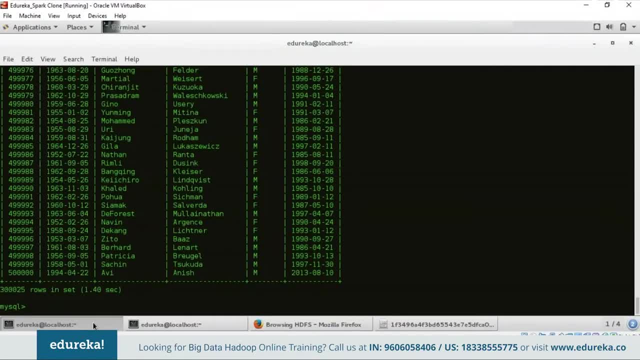 So let's see how it works. one important thing to notify: the target table must exist in the target database, That is, the data is stored as records, HDFS, and these records are read and pass and delimited with the user specified delimiter. The default operation is to insert all the records from the input files. 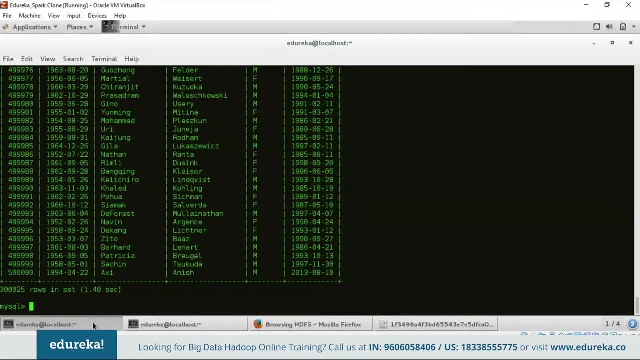 to the database using the insert statement in update mode. scoop generates the update statement that replaces the existing record in the database. So first we are creating an empty table where we will export our data. I'm going to create a table called employee 0.. 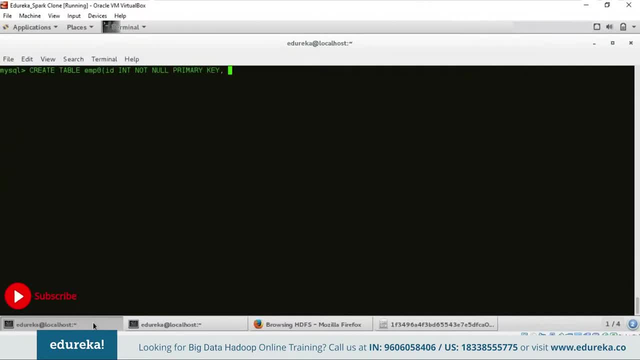 The primary key value should never be null, So I'm specifying it as not null. So here I created an empty table called employee 0, and now I'll show you how to scope export works Here. instead of import, I'll make it as export. 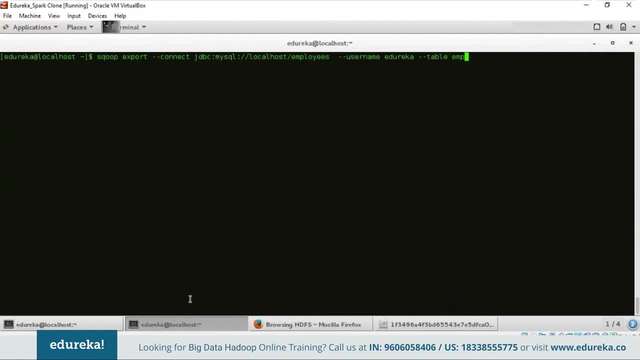 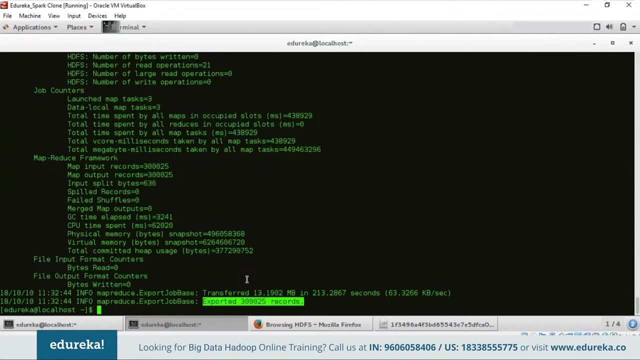 This is the database name and I have created a table called employee 0 and I'm going to specify the path for export directory. Simple, that's all. So you can see here. it exported all these records into the rdbms, So now let's cross check. 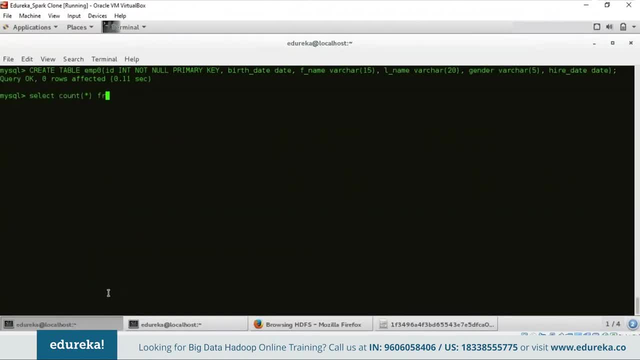 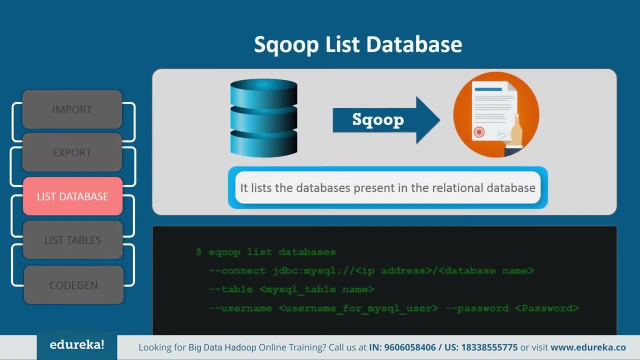 I'm going to give select count star from the table name that I have specified to export the tables, So you can see the entire records got exported to this table. So this is how the scoop export works. Now let's see how to list the database present. 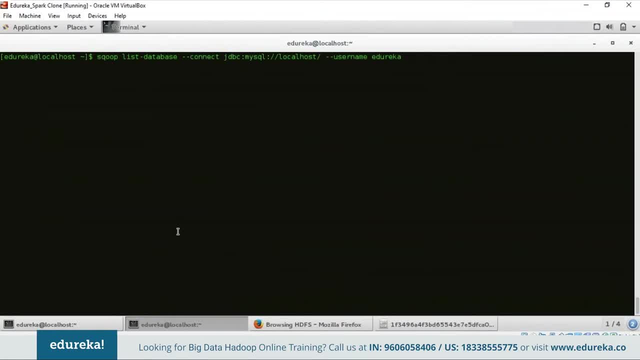 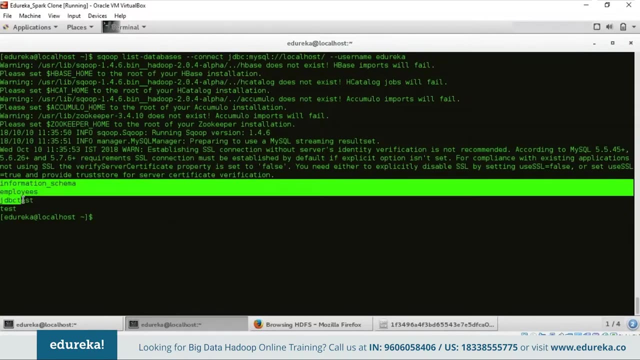 in the relational database. here You need not even specify the database name, because you're going to list the database that is present in the relational database system. So you're going to specify, list databases And execute the command. So the database is present in the relational database system. is test JDBC, test employees. 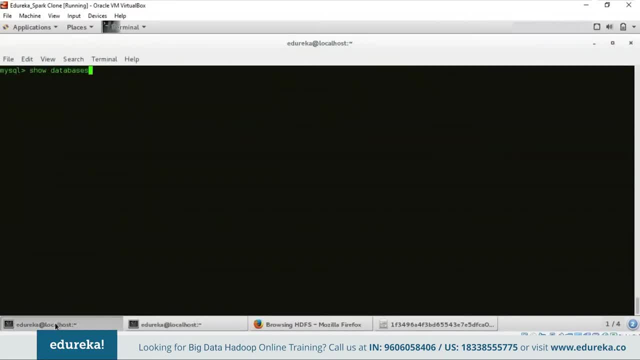 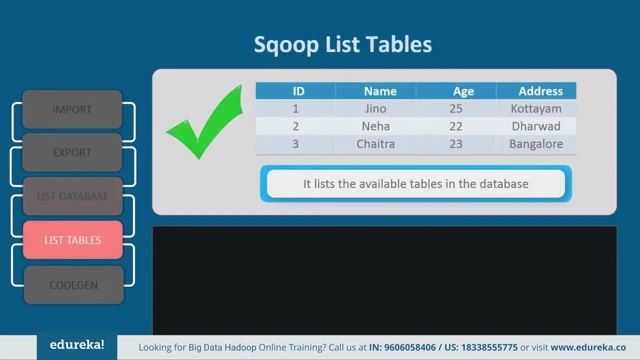 and information schema. again, Let's cross check. I'm going to give show databases. it retrieve the same database, So the result tallies, so we can also list the tables present in the database. Let's see how to list all the tables present in the database. 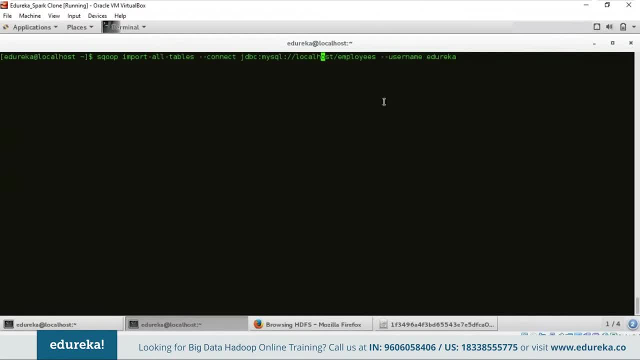 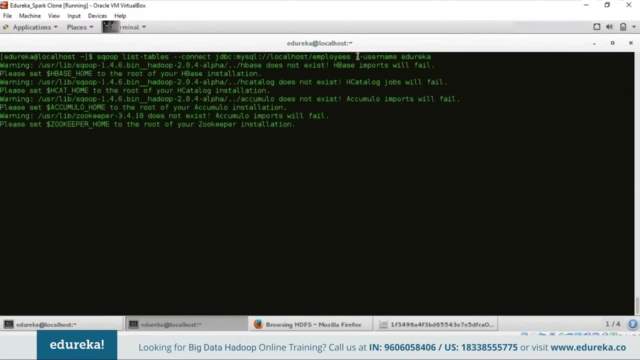 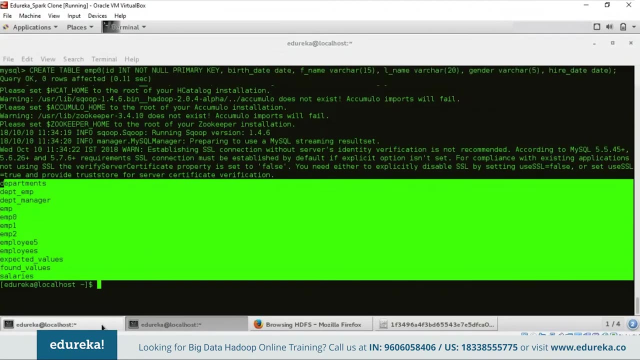 Again, it's very simple. You have to just specify the database name, like here, And give list tables instead of import, So you can see that it listed all the tables present in the database employees. So again, let's cross check: show tables. 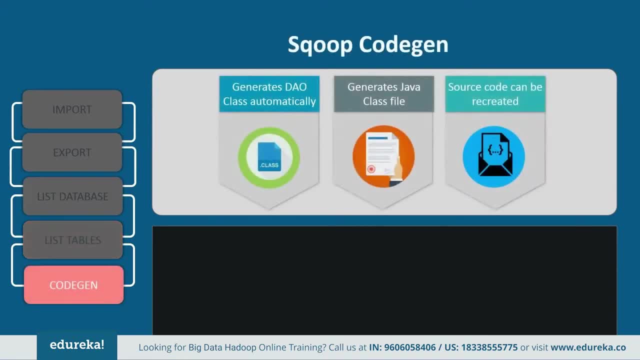 Same thing. and now let's see what is courting in object-oriented application. Every database table has one data access object class that contains getter and setter methods to initialize objects and coach and generates the AO class automatically, and it also generates the DAO class and Java based on the table schema structure. 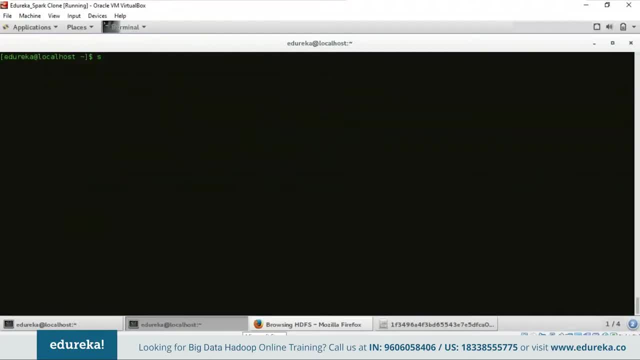 So this is a simple command. Let's see how to execute it here. I will give scope, code gen And give the connection and the database name as employees, And I'm going to specify the table name as well. So it is going to create a employee jar file. 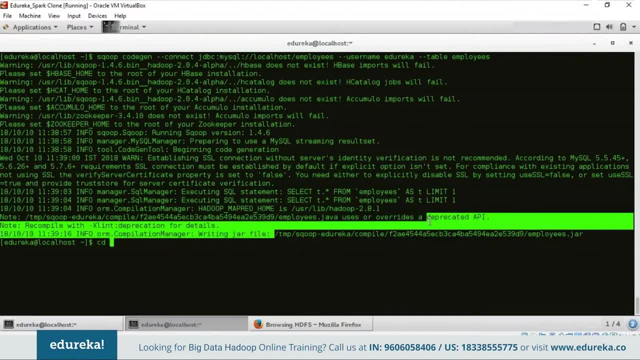 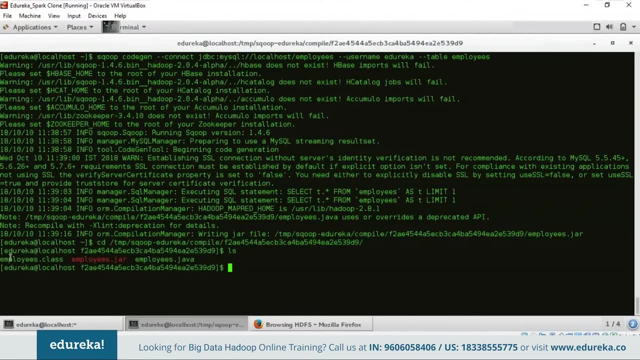 in which the backend code will be generated. So I'll copy this path and jump into this directory. So you can see here that it created employees class jar file and the Java object file as well. So now let's open the file system and check for the file. 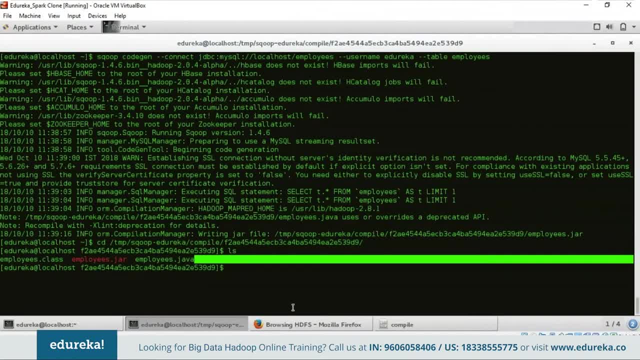 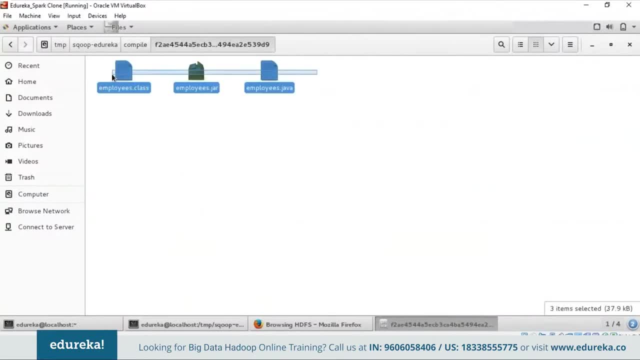 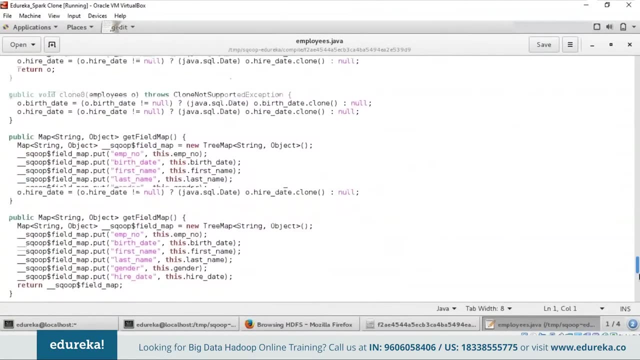 So what was the name of the file? It ends with 5, 3, 9, D, 9.. So here is the folder. So in this you can see the object file that is being generated. So this is a back-end code that has been generated. 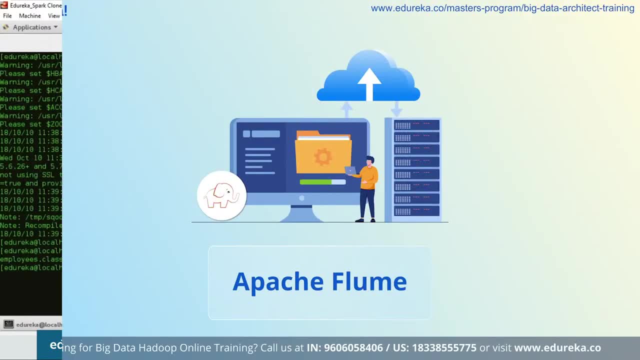 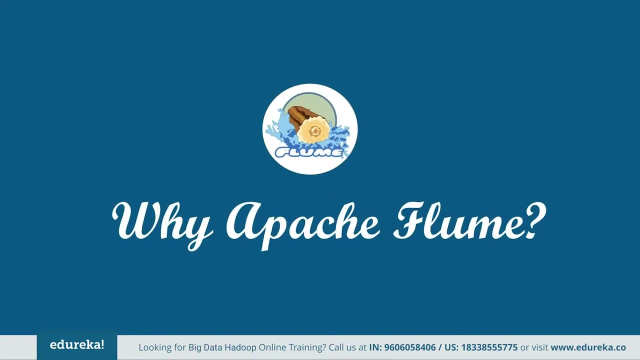 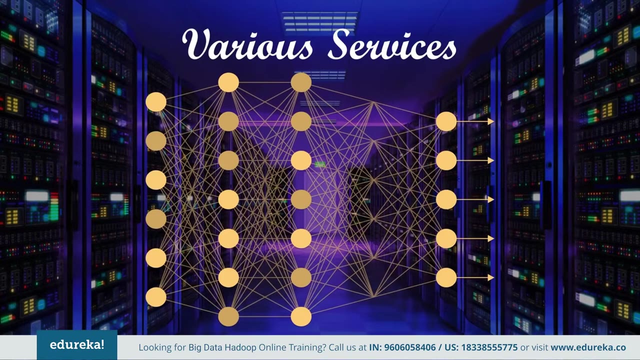 So this is all about how the scope code gen works. Why do we need flume for data ingestion? Let's take a scenario here. Say we have hundreds of services running in different servers and that produce lots of large logs which should be analyzed together. 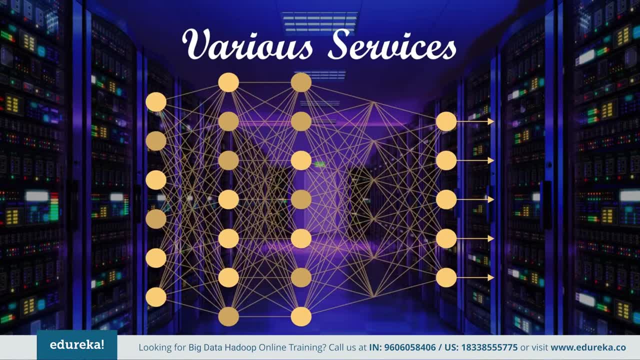 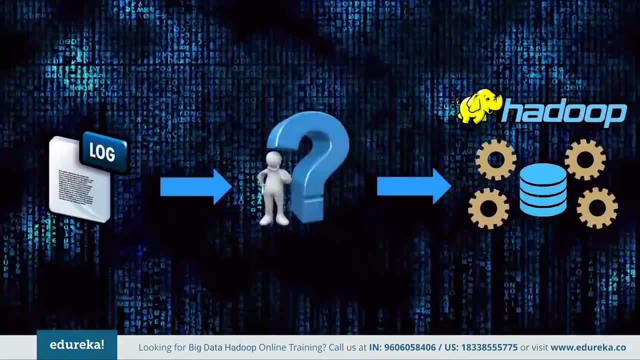 and we already have Hadoop to process these logs. So how do we send all the logs to a place that has Hadoop? It's obvious fact that we need a reliable, scalable, extensible and a manageable way to do it. So to resolve this problem, Apache flume came into picture. 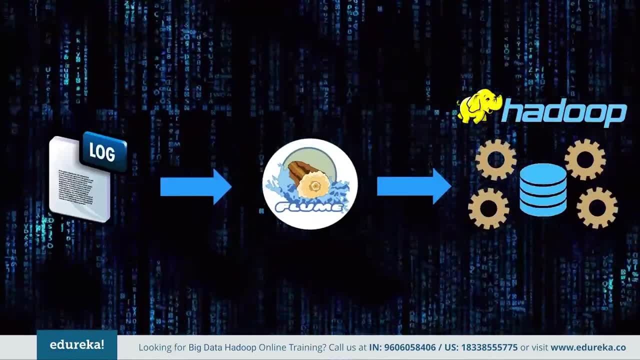 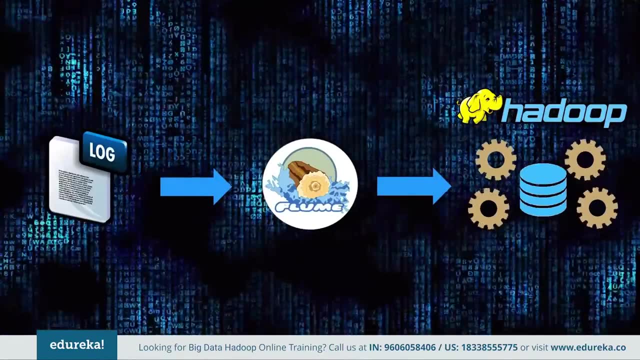 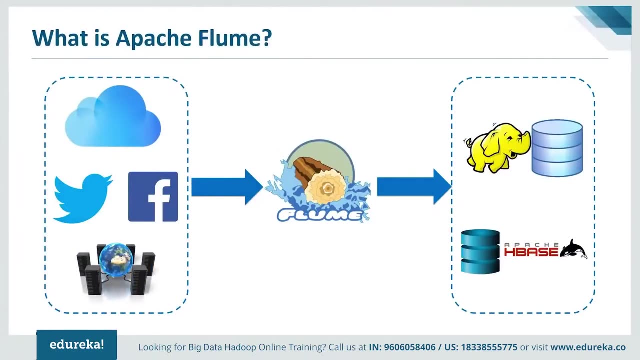 which is the most reliable, distributed and available service for systematically collecting, aggregating and moving large amounts of streaming data into the HDFS, and that's why and where we need flume. So what is Apache flume? by now, you all might have thought that flume is a tool for data ingestion in HDFS. 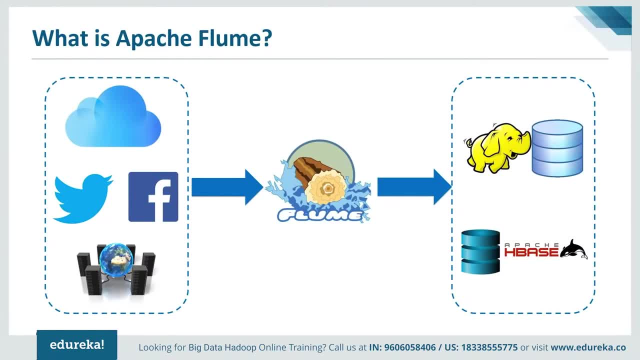 It collects, aggregates and transports large amount of streaming data, such as log files, events from various sources like network traffic, social media, email messages, etc. The main idea behind the flumes design is to capture streaming data from various web servers to HDFS. It has very simple and flexible architecture based. 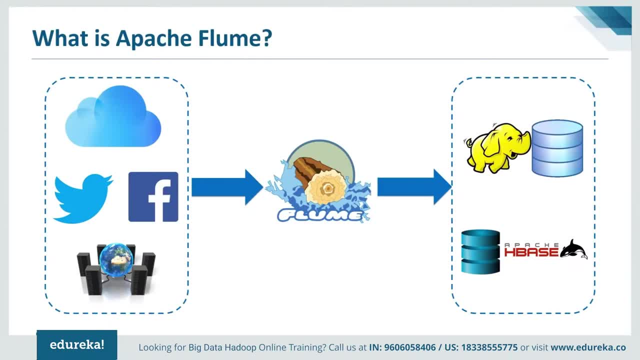 on streaming data flows. It is fault-tolerant and also provides a reliability mechanism for failure recovery. again, flume can easily integrate with Hadoop and dump all the unstructured as well as a semi-structured data on HDFS, and that complements the power of Hadoop. 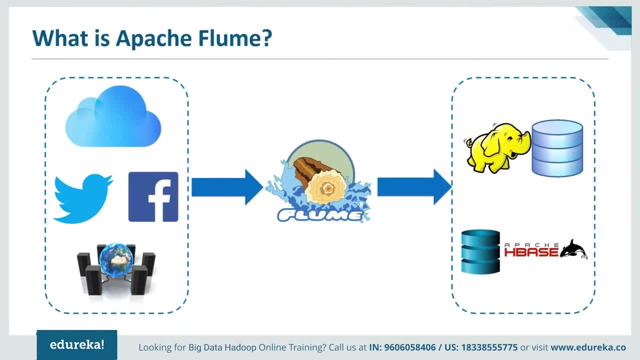 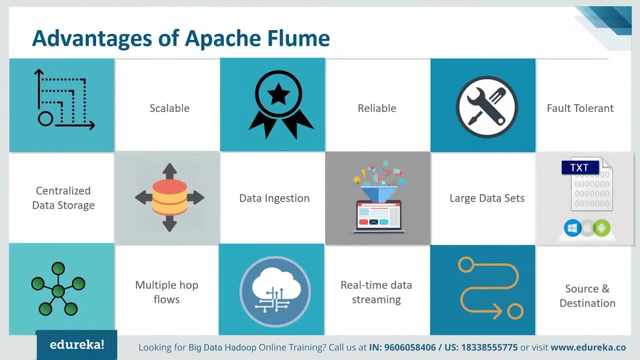 This is why Apache flume is said to be the most important part of Hadoop ecosystem. Now let's move further and see the benefits of flume. There are several advantages of Apache flume, which makes it a better choice over others. I have listed some. 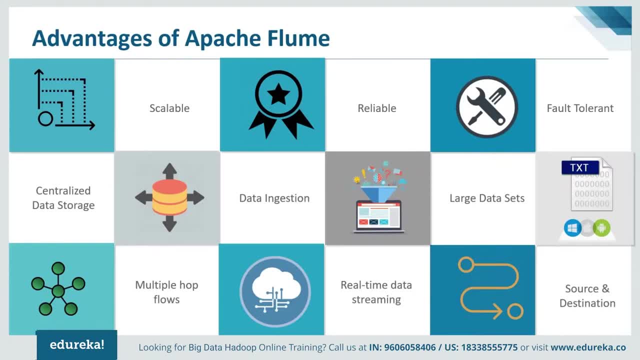 of the benefits: flume is scalable, reliable, fault-tolerant and customizable for different sources and sinks. It can also store the data and centralized storage like HBase, HDFS, etc. If the read rate exceeds the write rate, flume provides a steady flow of data between read and write operations. flume. 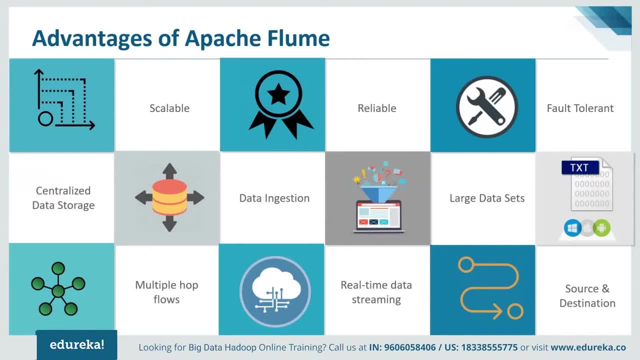 also provides a reliable message delivery. the transactions in the flume are channel based, where two transactions are maintained for each message, that is, one sender and one receiver for each message. using flume, We can ingest the data from multiple servers into Hadoop and it also helps us to ingest online streaming data. 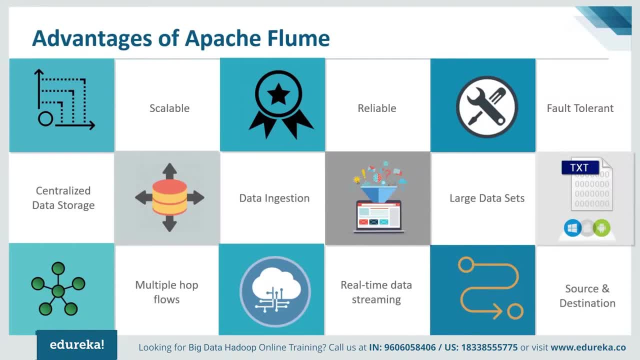 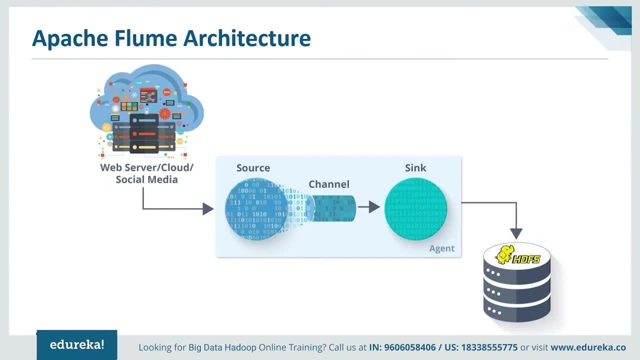 from various sources and supports a large set of sources and destination types. So let's see what's next. the architecture is the one which is empowering Apache flume with its benefits. Now, as we know the advantages of Apache flume, let's move ahead and understand Apache flumes architecture. 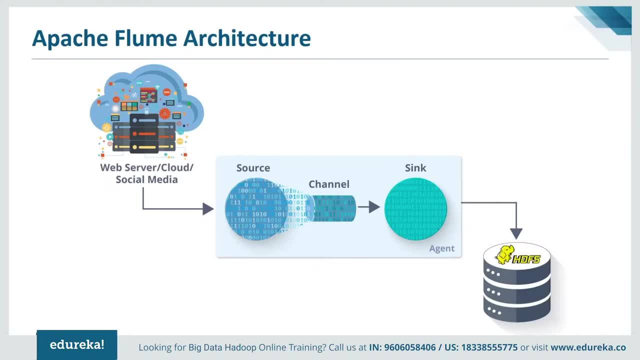 one important thing to note here: There's a flume agent which ingest a streaming data from various data sources to HDFS. from this figure You can easily understand that web server, Facebook, cloud, social media- all these indicate the data source from where we are getting the data. 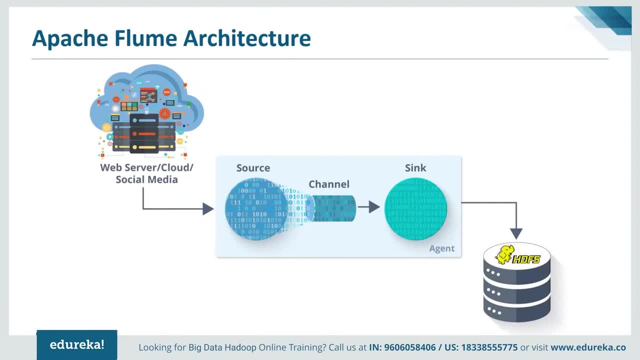 and Twitter is among one of the famous sources for data streaming. and now coming to flume agent. It comprise of three components: source, sync and channel. first source: it accepts the data from the incoming stream line and stores the data in the channel. now coming to channel. 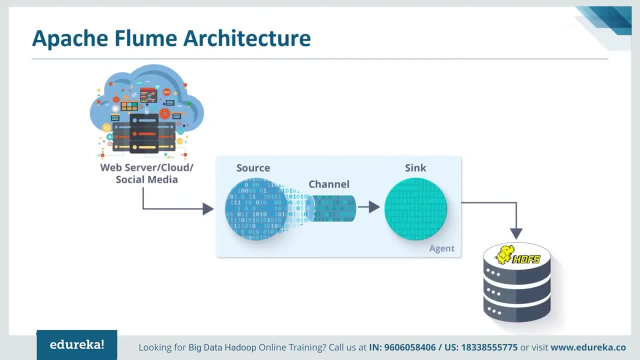 in general, The reading speed is faster than the writing speed. Thus we need some buffer to match the read and write speed difference. basically, what happens? the buffer acts as a intermediary storage that stores the data which is being transferred temporarily and therefore prevents data loss. 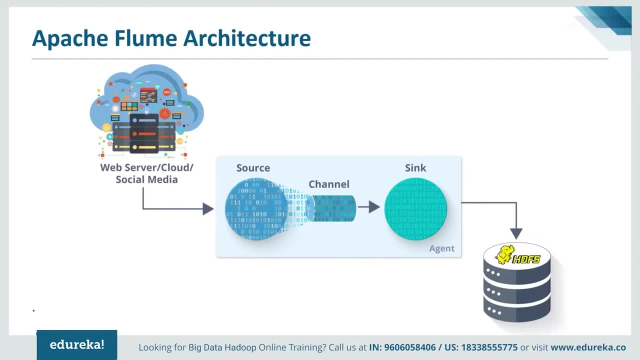 Similarly, channel acts as a local storage or a temporary storage between the source of data and the persistent data in HDFS. now coming to our last component, sync. it collects the data from the channel and commits or writes the data in the HDFS Permanently. 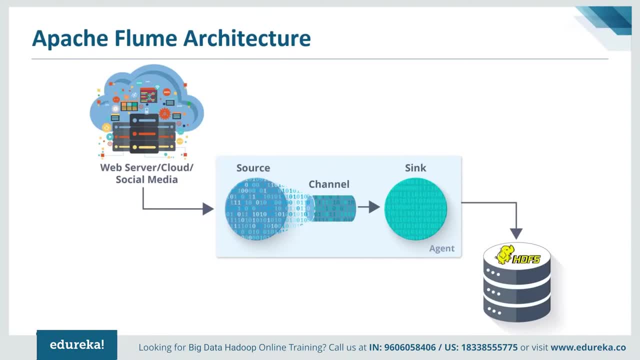 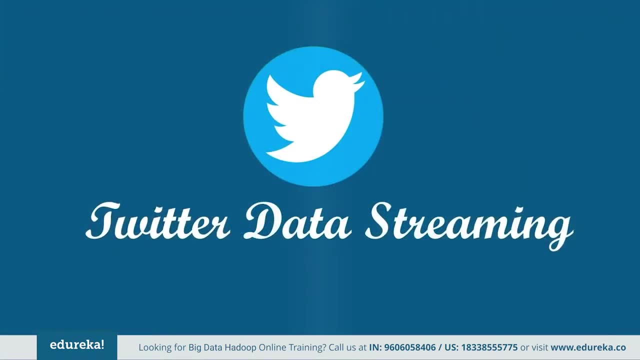 So this is all about the working of flume architecture. as we know how Apache flume works, Let's take a look at the practical, where we will sing the Twitter data and store it in the HDFS. in this figure You can see there is lots of data generated from Twitter. 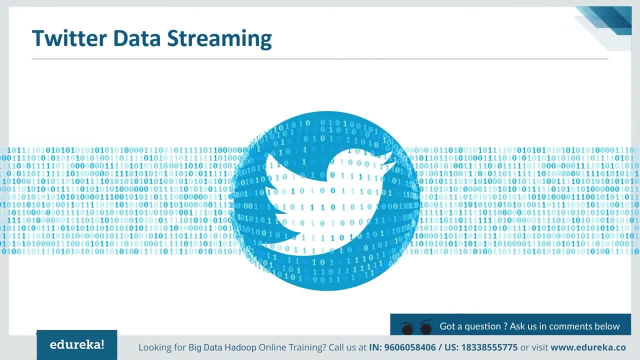 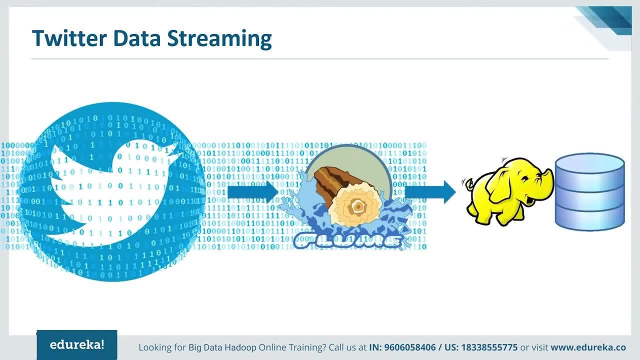 Now you want to go ahead and stream this data, So how will you do it? for this, We have Apache flume, which will help us to do the real-time data streaming of Twitter data and store it in the HDFS. So let's see how to do it. 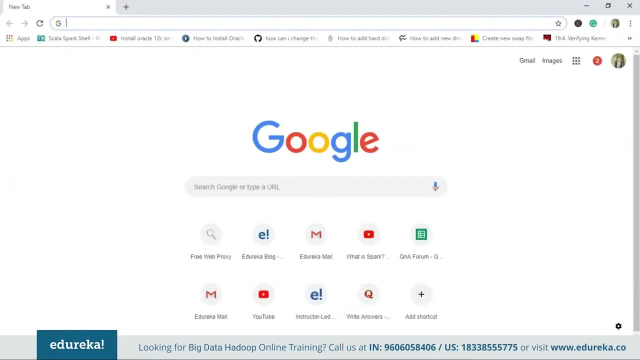 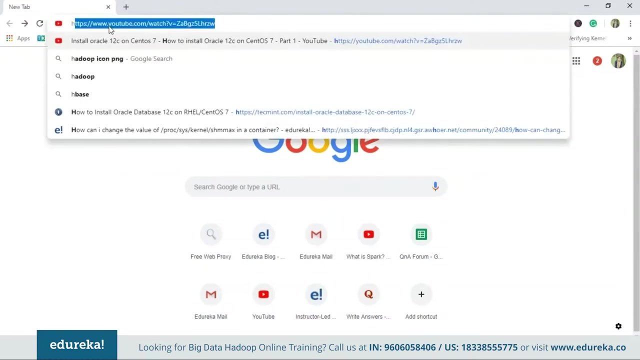 So first we will create an application and get the tweets from it. here We use experimental Twitter source provided by Apache flume. So here we will use memory channel to buffer these tweets and HDFS sync to push these tweets into the HDFS. The first step is to create a Twitter application for this. 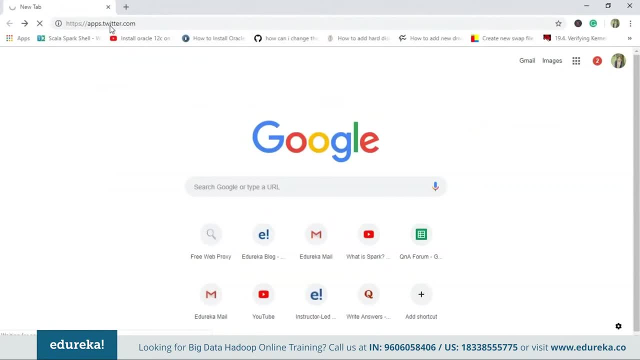 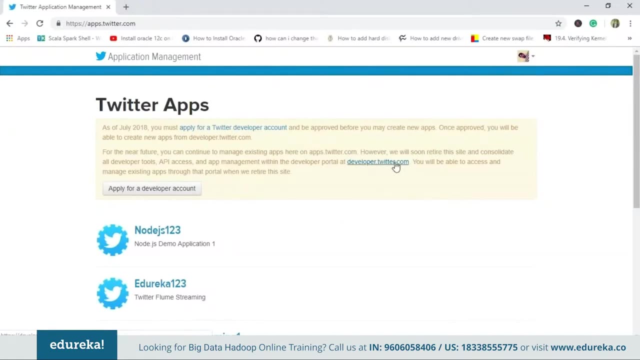 You have to go to this URL that is appstwittercom, and you have to sign into your account. If you do not have developer account, you have to apply for the one by completing the firm. as I already have a developer account, I'll just click on developertwittercom. 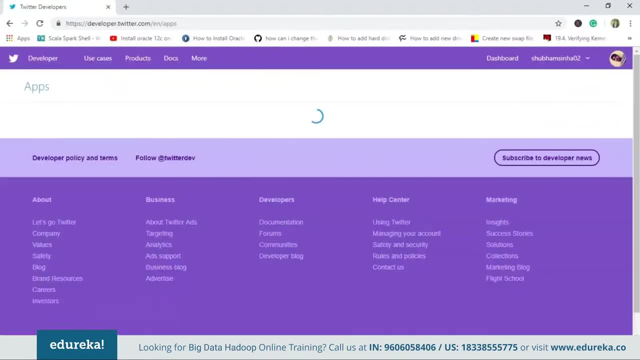 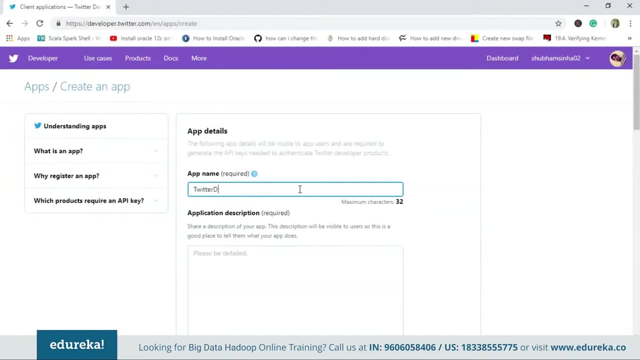 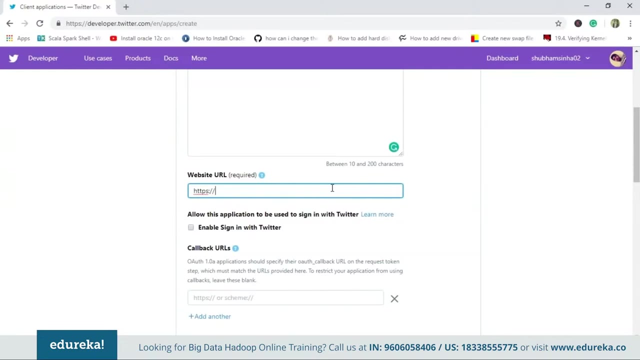 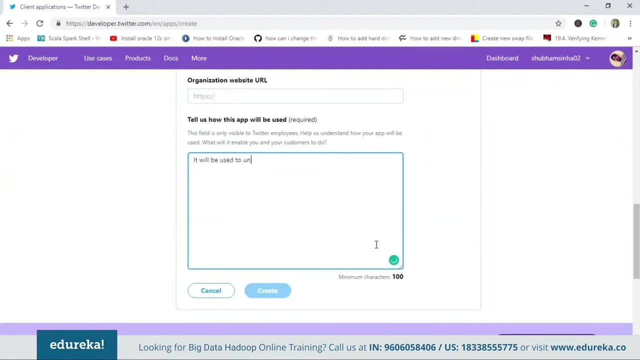 and click on my profile and choose apps. So here you have application called create an app. here You have to fill these required fields: first, app name. Now, while filling the website address, you have to give the complete URL pattern like this: And then you have to specify how this app will be used. 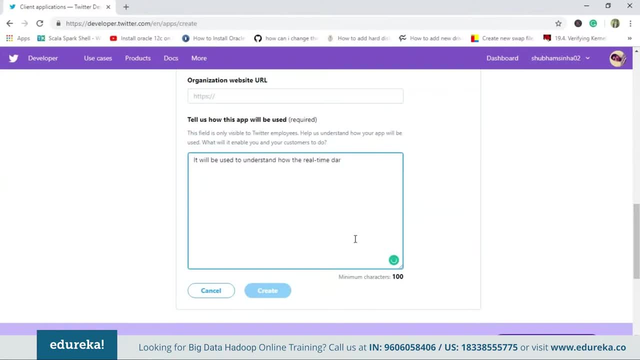 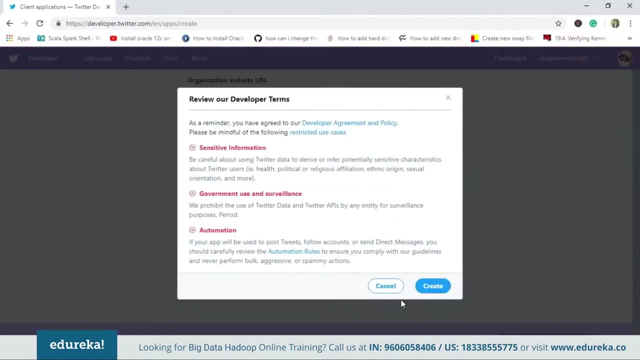 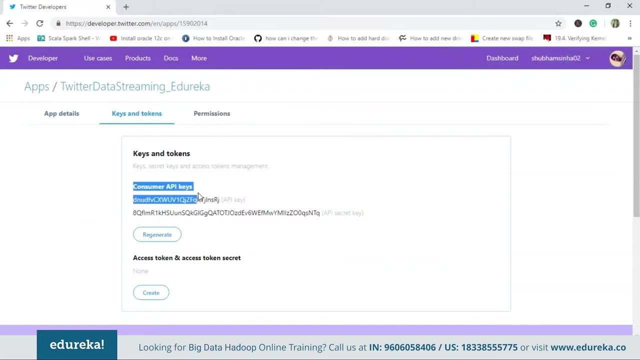 I'll say something like this: So after everything is done, you have to just click on create. your application got created. now click on keys and tokens and here you will find something called as consumer API keys and access token and access token secret. You have to reach and read this. 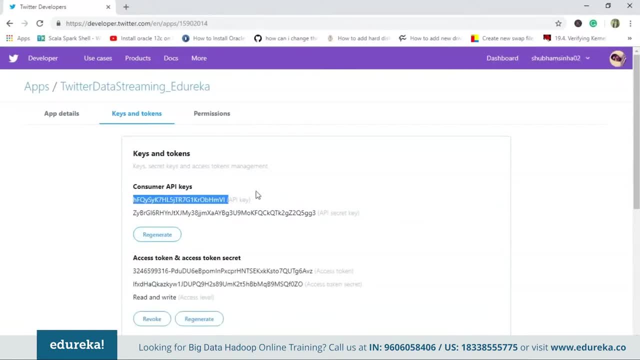 and you have to create an access token keys. Now we've got the API key, the API secret key, the access token and the access token secret as well, So copy the key and access token. So you might be thinking why you need to copy these things. 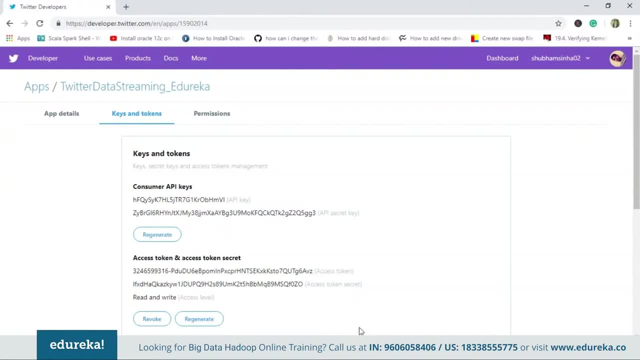 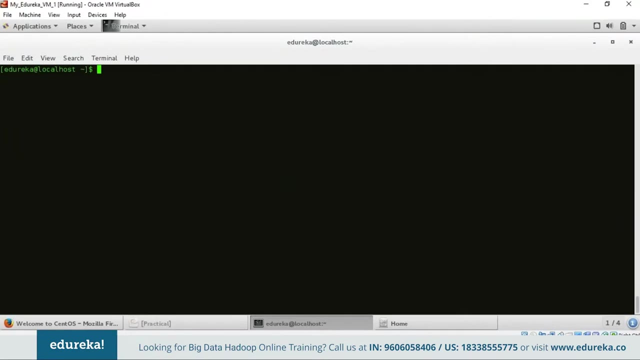 We need to pass these tokens in our flume configuration file to connect to this Twitter application. So I'm going to copy this. make sure you copy it properly. Now let's create a flume configuration file in the flumes root directory. I have already created a flumecom file. 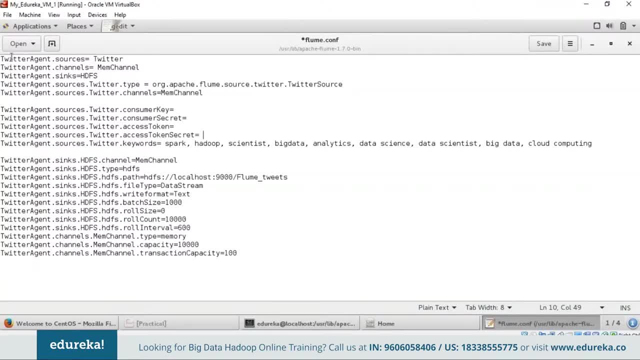 I'll show you how to specify the parameters. as we have discussed in the flumes architecture. I have configured source, sync and channel here. Our sources Twitter channel is memory channel and the sink is HDFS. in source configuration We are Passing the Twitter source type as this: 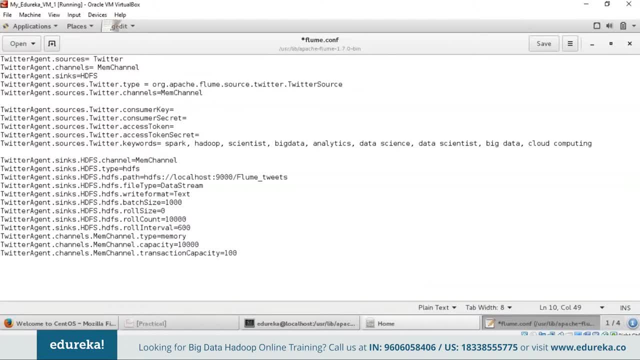 then we are passing all the four tokens which we have received from Twitter, that is, the keys and the secret keys that I have copied. Make sure you pay some properly at last. in the source configuration, We are passing the keywords on which we are going to fetch. 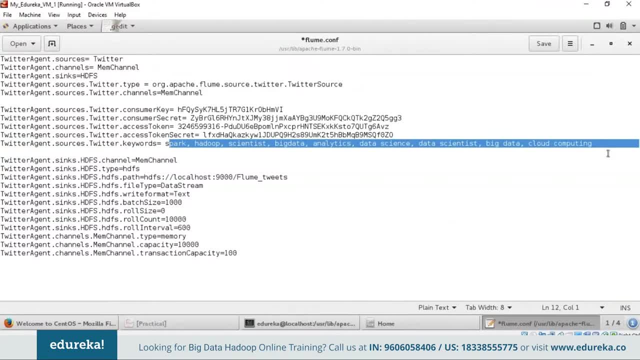 These are tweets, So I have specified some keywords like spark or do, big data, analytics, cloud computing, Etc. Now in the sync configuration, I have configured the HDFS properties, that is, HDFS channel, as memory channel. The type will be HDFS, the path of HDFS: 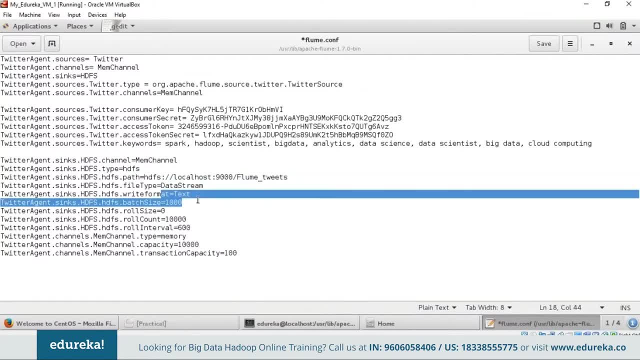 where the flume tweets will be stored. the file type, the right format, will be always text. Remember that the batch size, roll size, roll count, Etc. And at last, we are going to set the memory channel properties, like the type capacity and the transaction capacity. 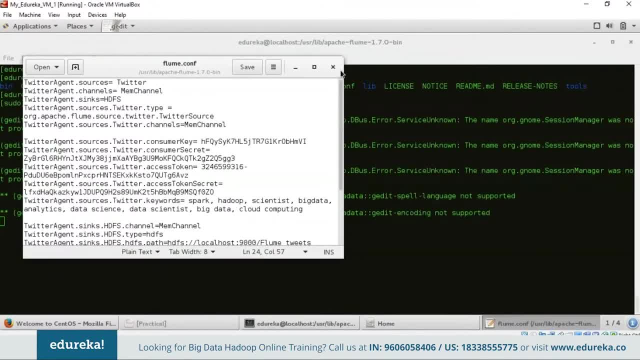 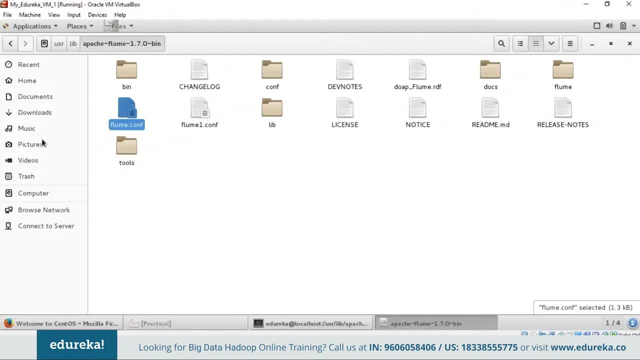 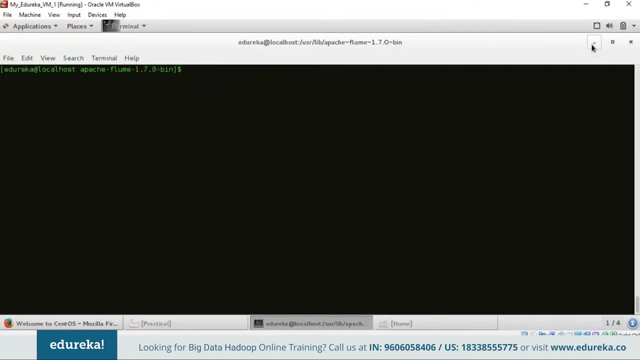 now save this file and close it. For my convenience, I'll copy this file from flume directory and paste it in the home directory. Okay, Now we are all set for execution. Let's go ahead and see how to execute this command. 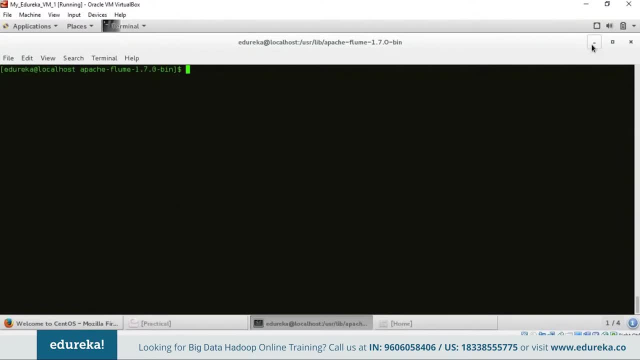 Now I have placed a flumecom file from the flumes root directory to home directory, So I'll go back to the home directory and then run the command. The command goes like this: That is flume- ng-agent, con file path. that is home Edureka and the con file name. 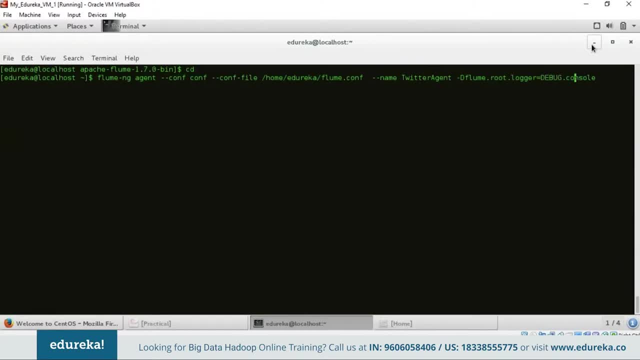 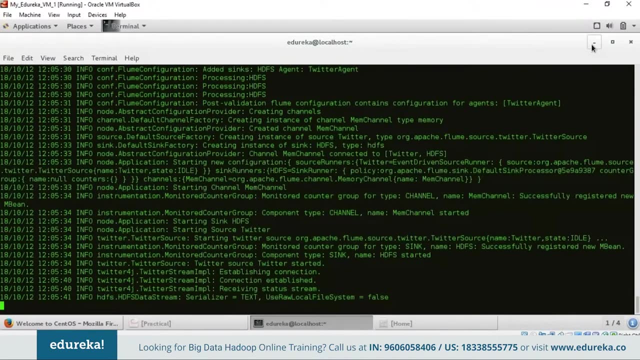 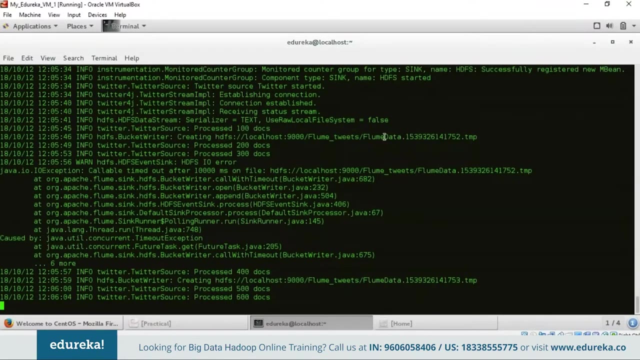 The name will be Twitter agent and the flumerootlogger will be debugconsole- enter. now It started executing, So you can see here. it started processing the records and created this flume tweets folder in that you have this file. So after executing this command, 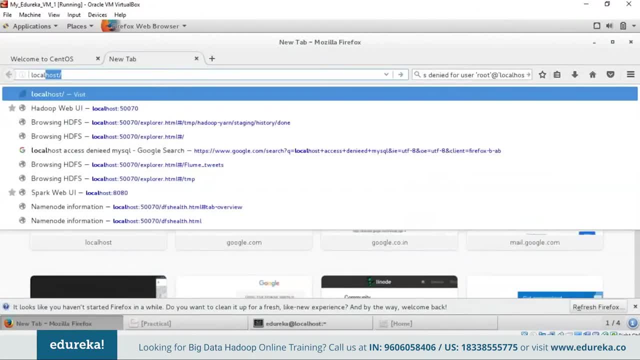 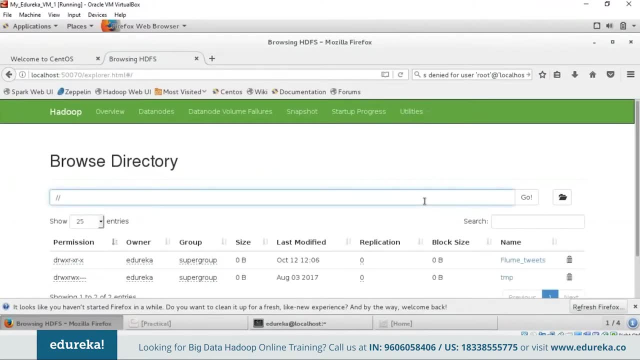 for a while. you can exit the terminal using control C. now let's open the web browser and go to HDFS web UI. So here in the mention path, you can check the file that is present. So here you have flume tweets. click on that. 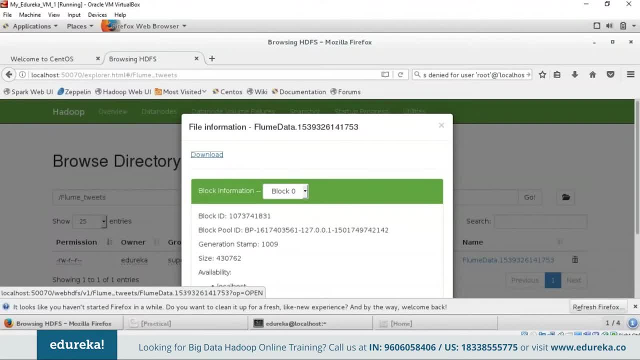 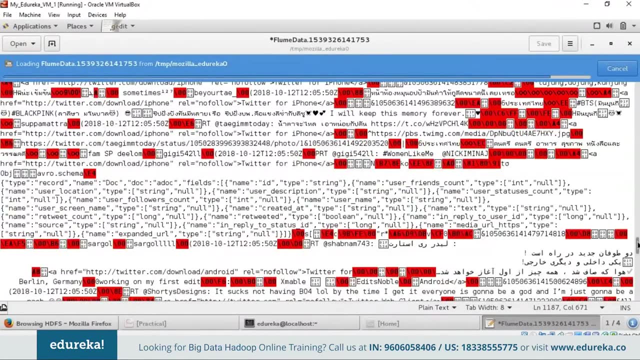 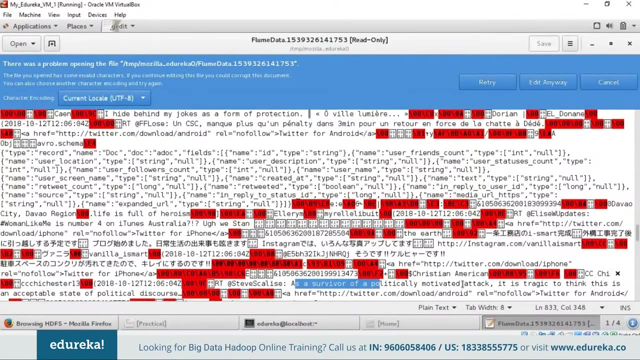 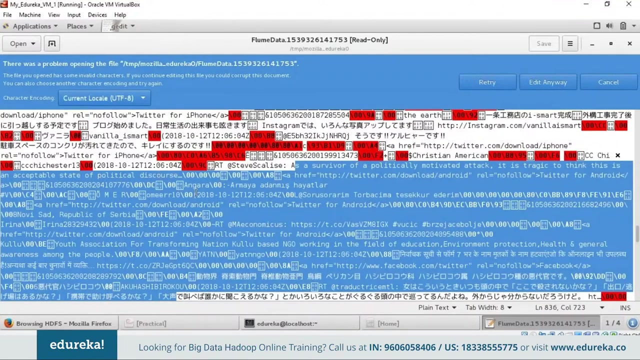 So this is output file where the data will be streamed. So this is output where you can see the tweets from the followers. Someone is saying: as a survivor of a politically motivated attack, It's tragic to think this is an acceptable state of political discourse. 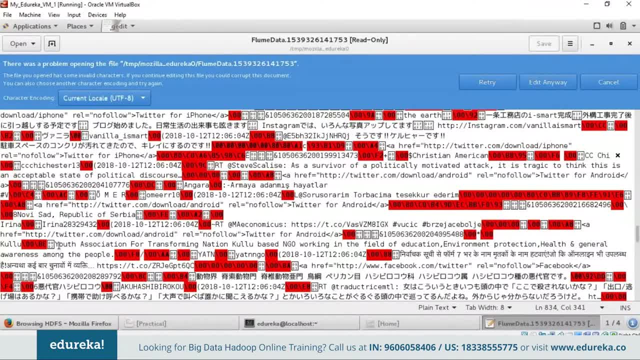 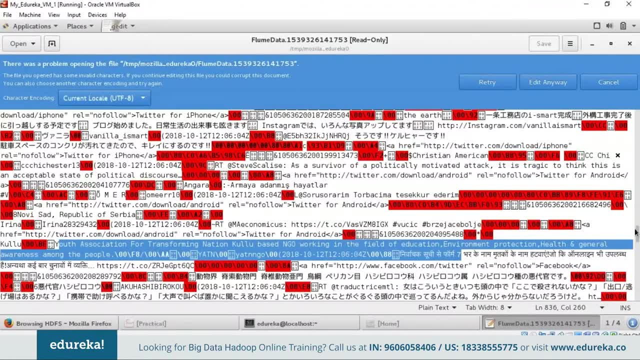 It depends, like, whatever you follow and you will get all those things. and here someone is saying youth Association for transforming National Kulu, based on NGO working in the field education, environment protection, health and general awareness among the people. So this output is nothing but the live data streaming of Twitter. 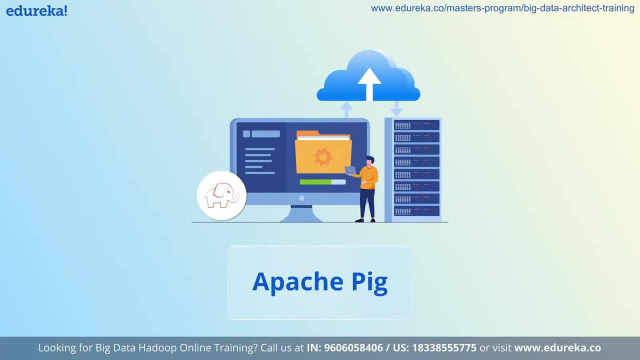 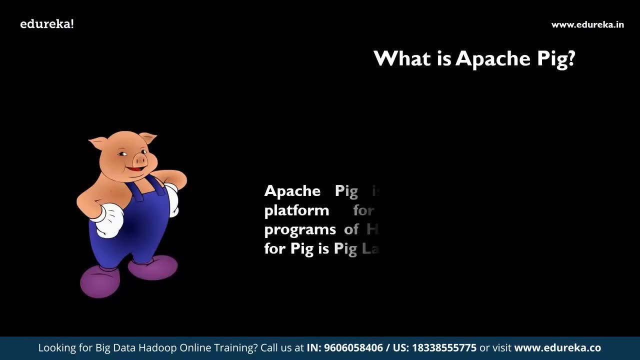 Data. What is Apache Pig? So Apache Pig is an abstraction over MapReduce. It is a tool or platform which is used to analyze larger sets of data, representing them as data flows. Pink is generally used. with Hadoop. We can perform all the data manipulation operations. 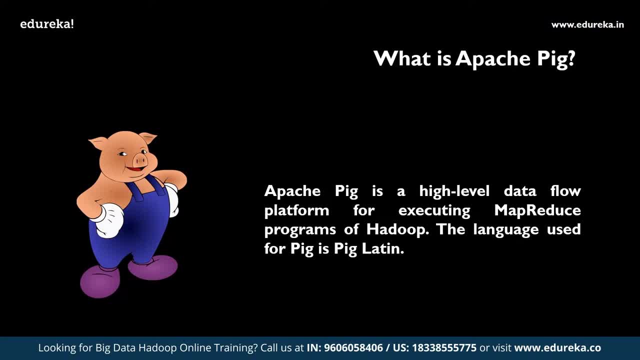 in Hadoop using Apache Pig to write data analysis programs. Pig provides a high-level language known as Pig Latin. This language provides various operators using which programmers can develop their own functions for reading, writing and processing data. to analyze data using Apache Pig, programmers need to write scripts using Pig Latin language. 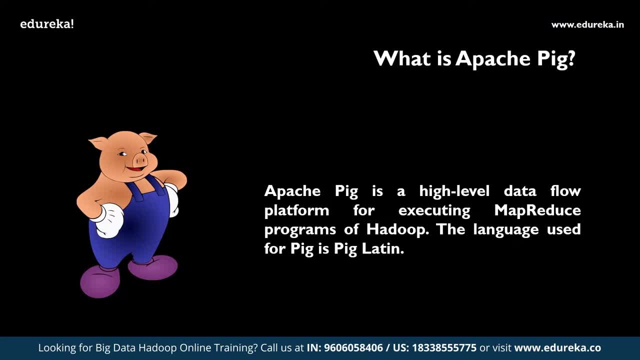 All these scripts are internally converted into map and reduce test respectively. Apache Pig has a component called Apache Pig engine that accepts the Pig Latin scripts as input and converts those particular scripts into MapReduce jobs. So this was the basic introduction to Apache Pig. Now moving ahead. 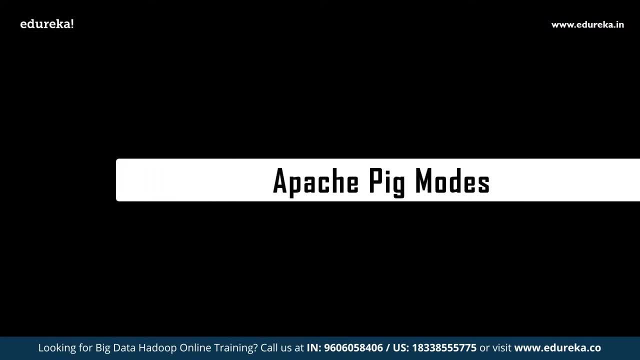 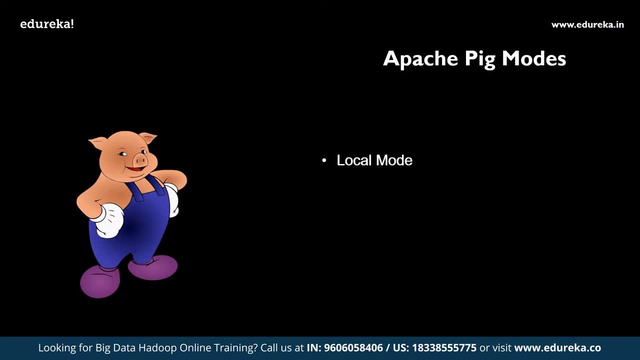 We shall understand the different modes in which Apache Pig functions. There are two particular modes in which Apache Pig functions. Those are the local mode and MapReduce mode. first We will understand what exactly is local mode. in local mode, Apache Pig is designed to execute in a single JVM. 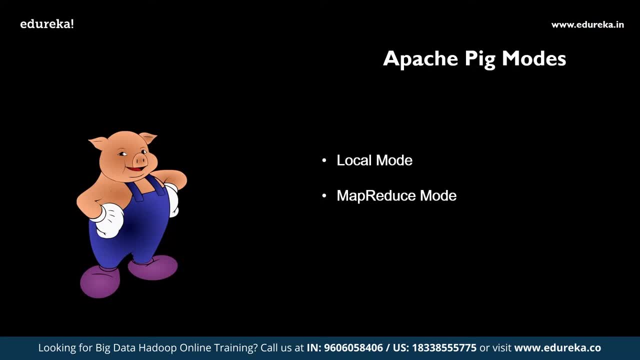 and is used for development, experimenting and prototyping. here files are installed and run using localhost. The local mode works on local file system and the input and the output data is stored in the local file system. to access the command or the crunch shell in local mode: 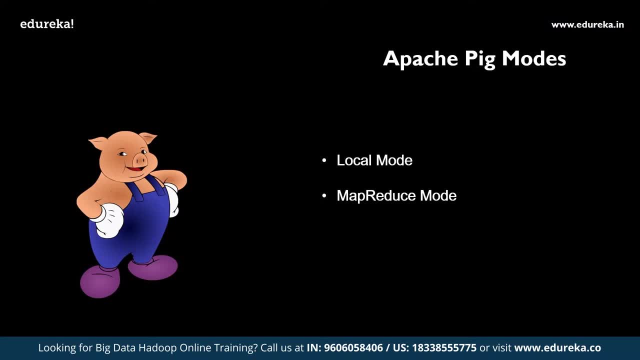 You need to execute a command called Pig, hyphen X local. We shall practically execute this in the demo section. Now, moving ahead, We shall discuss about the second type of mode in which Apache Pig can be run, that is, the MapReduce mode. The MapReduce mode is also known as Hadoop mode. 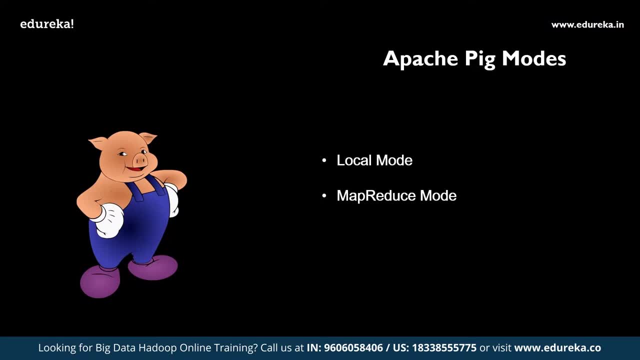 Apache Pig chooses Hadoop mode as its default mode and this Pig renders Pig Latin into MapReduce jobs and executes them on a Hadoop cluster. It can be executed against semi-distributed or fully distributed Hadoop installation. Here the input and the output are present on HDFS. 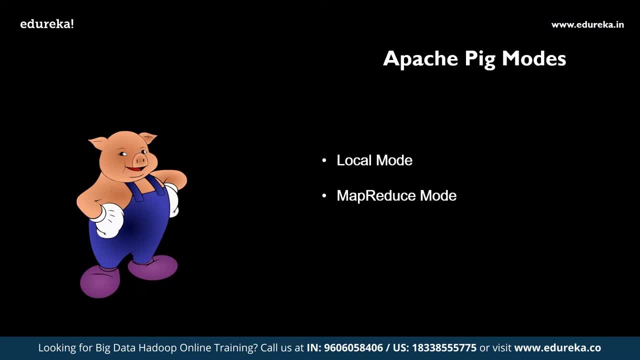 The command for executing Pig in MapReduce mode is Pig or Pig, hyphen X- MapReduce. Again, we shall discuss about this particular command in our demo section, where I'll show you both the modes and execute the Pig scripts there Now, followed by the Pig modes. 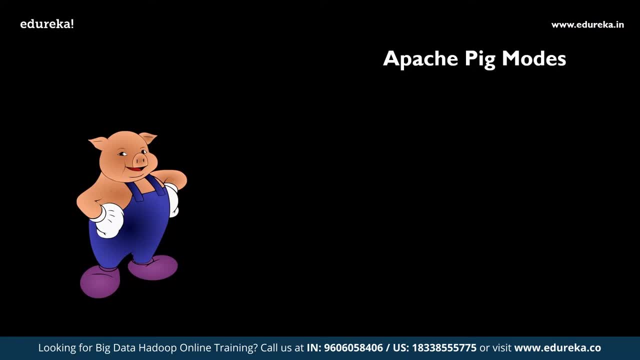 We shall understand the ways to execute Pig program. So basically, the Pig scripts are executed in three particular modes. Those are interactive mode, batch mode and lastly, the embedded mode. Don't worry, I'll explain to you each of these modes. Firstly, we shall discuss about the interactive mode. 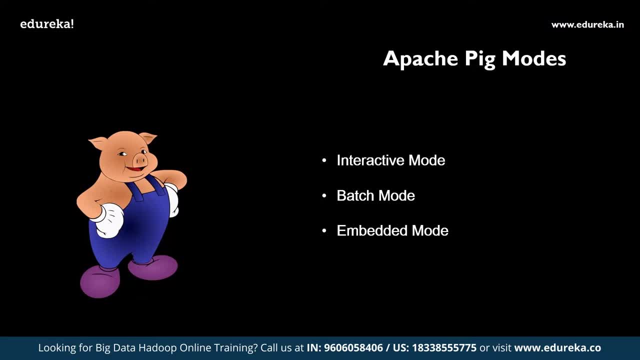 in this particular mode The Pig is executed in a grunt shell. to invoke grunt shell, run the Pig command. once the grunt mode executes, we can provide Pig Latin statements and command interactively at the command line itself. So the next mode is the batch mode in this particular mode. 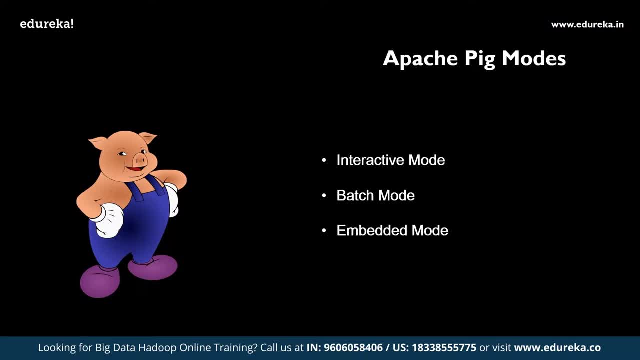 We can run a script file having a dot Pig extension. These files contain the Pig Latin commands. So basically what we do is we write the Pig command or the Pig script and store it in a location and using the terminal, we will access that particular location. 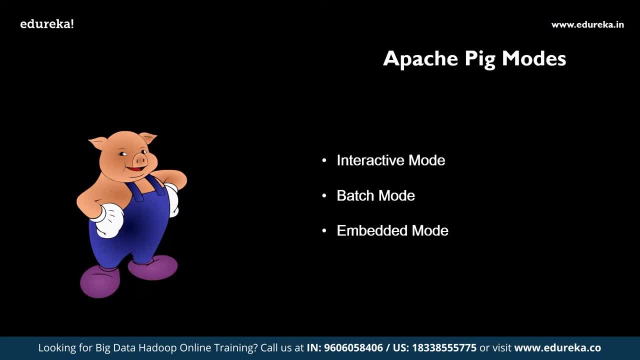 and that particular file and run the code present in that file. So this is what happens in batch mode. So, followed by that, the last mode is the embedded mode. in this particular mode We can Define our own functions. These functions can be called as user-defined functions here. 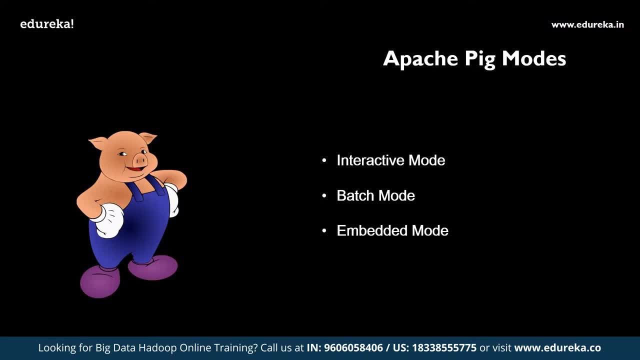 We use programming languages like Java and python to Define our own user-defined functions. So these were the three different modes in which we can execute a big scripts. now, moving ahead, We shall enter into our next topic, that is, the features of Pig. So there are five different and important features of Pig. 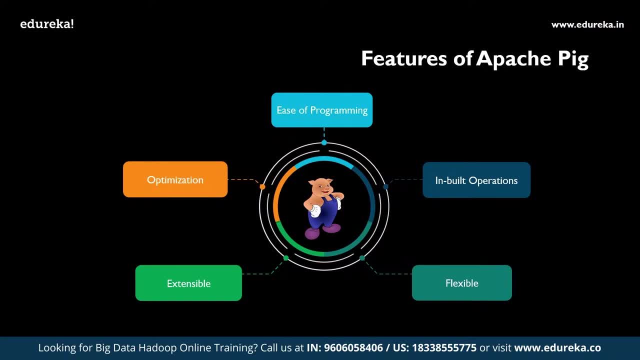 So first up we shall understand the ease of programming. writing complex Java programs for MapReduce is quite tough for non-programmers. Pig makes this process very easy. in the pig The queries are converted into MapReduce processes internally. So obviously it has grown the ease of programming followed. 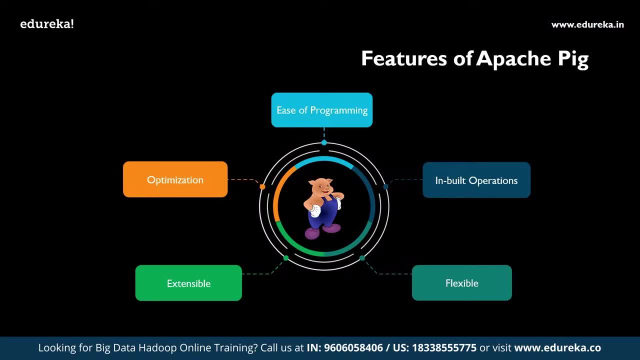 by that the next important feature, as the optimization opportunities. So what exactly is optimization? It is how the tasks are encoded, permits the system to optimize the execution automatically, allowing the user to focus on semantics rather than efficiency. So, followed by the optimization, we have the extensibility. 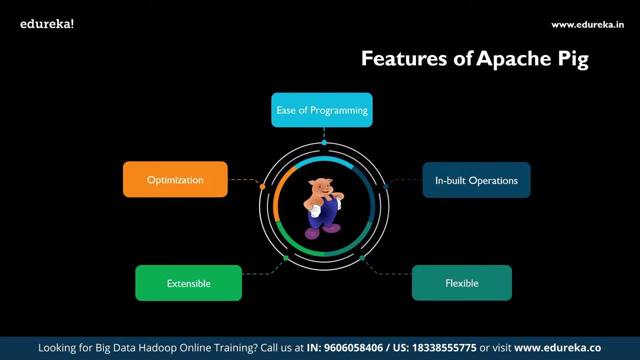 a user-defined function is written in which the user can write their logic to execute over the data sets. So this increases the extensibility of the programmer. followed by that, the next important feature is it is highly flexible. Apache Pig can easily handle structured as well as unstructured data. 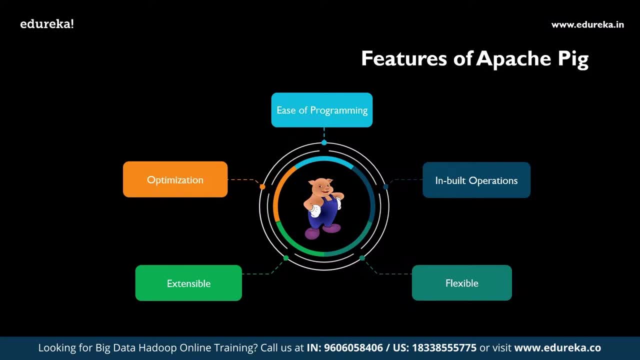 So Apache Pig tool is considered to be highly flexible, irrelevant of the data type. followed by that, the last and important feature is inbuilt operators. Apache Pig contains various types of operators, such as sort, filter, joints and many more, which are inbuilt. So here the programmer doesn't have. 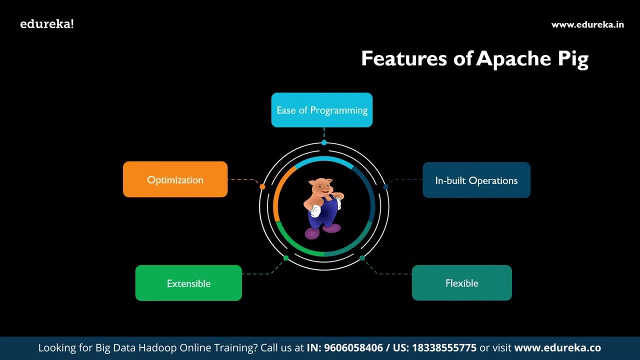 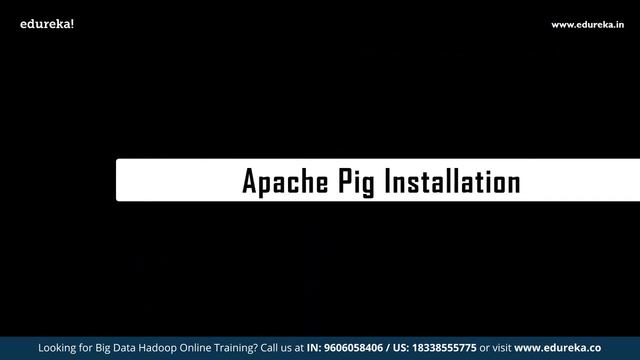 to program these functions externally. instead He can just directly get an access to those and build functions and execute them. So these were the five important features of Apache Pig. So the next topic in our today's discussion is Apache Pig installation into our local system. 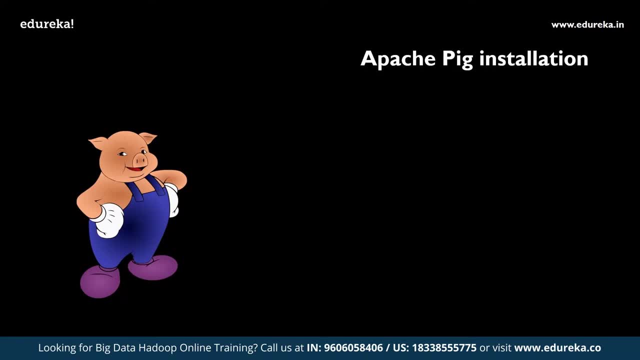 Now we shall discuss about one of the easiest ways to install Apache Pig into our local system. So today I'll explain you how to install Apache Pig into Windows operating system. So to do this, the easiest way is to download one of the virtual machines. 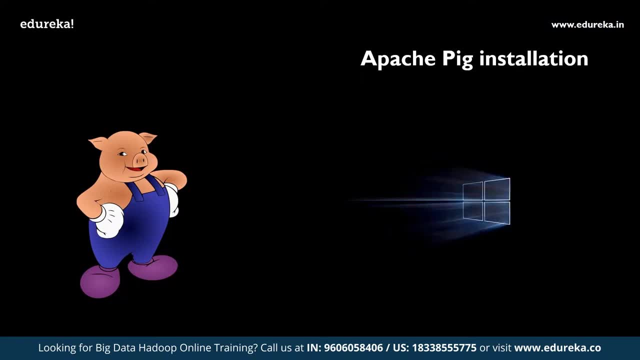 So I would prefer you to download Oracle virtual box for this particular task. followed by that, We shall also download a quick start VM of cloud around. Don't worry about the software's and drop down the link for those softwares in the description box below. 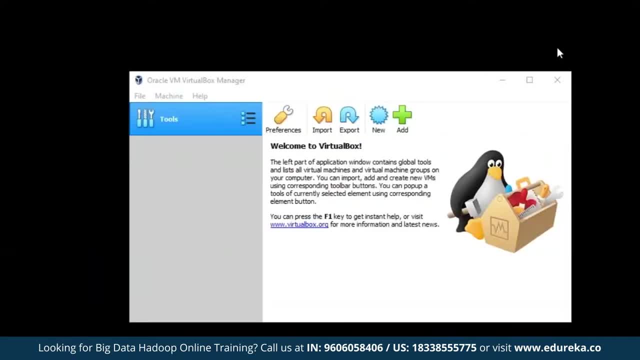 You can use that and download them. So, once after the Oracle virtual box is installed into a local system and it is running, This is how it looks like. now What we want to do is to add a new virtual machine into a virtual box. 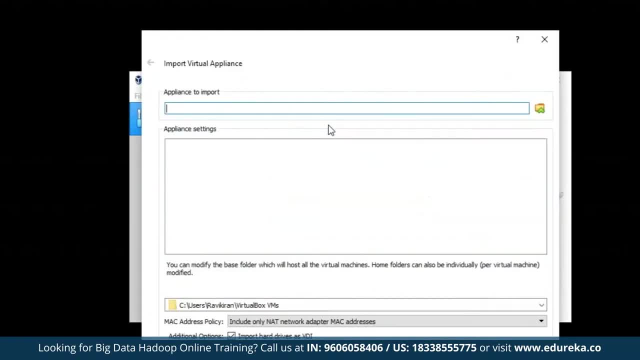 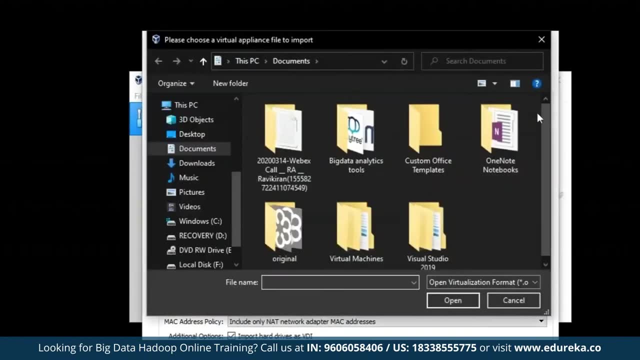 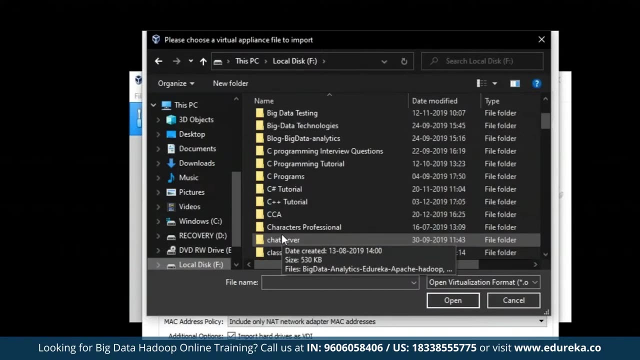 So for that you just need to select import option and it will give you a new dialog box and from here you must redirect to the location where your virtual box is located. So in my system it's located in F drive and inside F drive CCA cloud error virtual box. 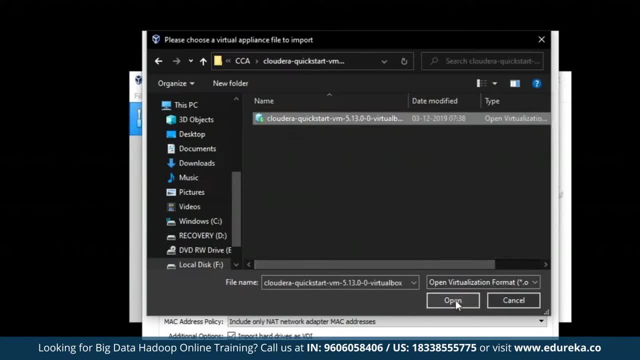 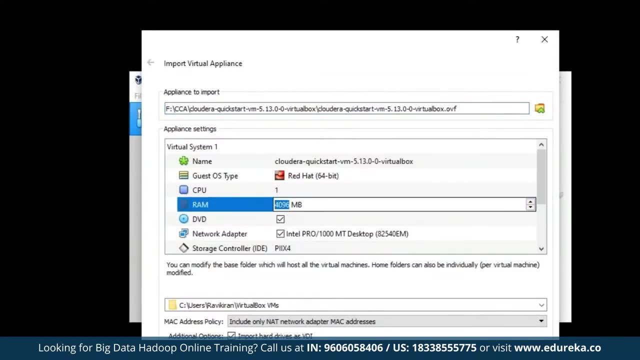 Cloudera quick start VM. So there you go. Now you just have to select open, and before we actually select the button import, you might want to select the RAM and increase its size to at least 8 GB. So just write in 9000 MB. 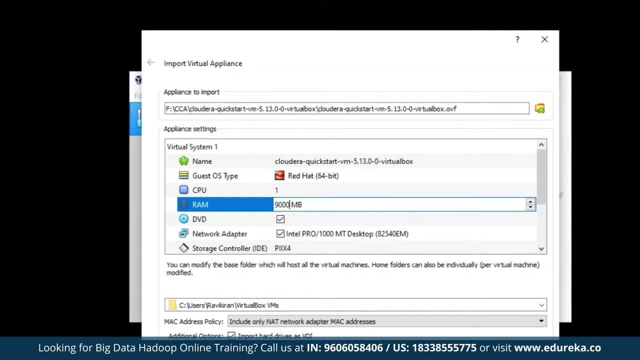 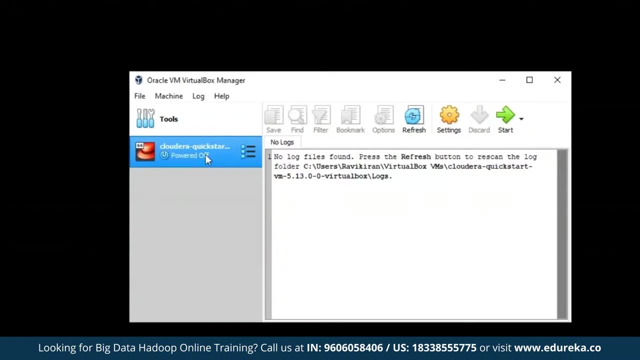 which is just a little about 8 GB. Now we are good to go. just select the option import and your virtual box will be imported. You can see that the quick start VM is getting imported Now. you can see that the virtual machine got successfully imported. now to start it. 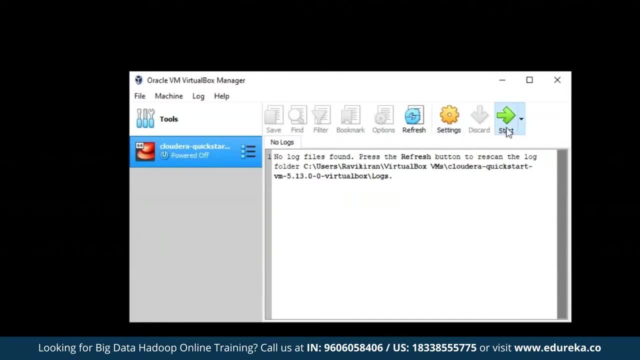 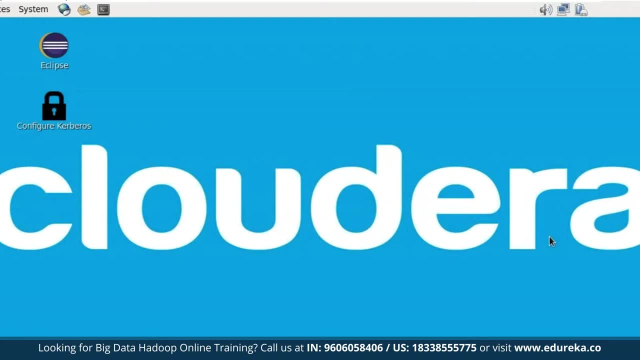 All you need to do is just click on it and then select the start button, So you can see that the cloud error quick start VM version 5.1. 3.0 has been successfully imported and booted up. Here we are. 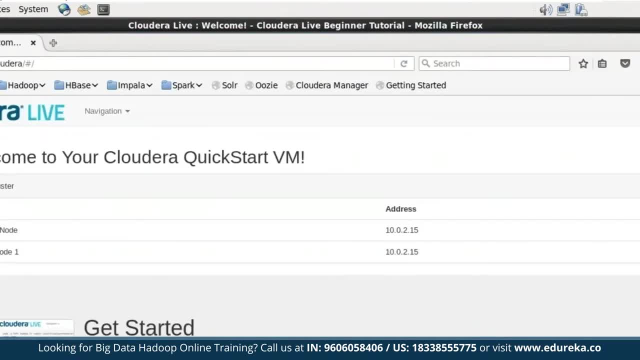 We have the quick start: Cloudera VM. welcome note. And now, if you want to start up with big editor, you might want to log into hue first or your HDFS. Remember, in cloud error the default username is cloud error and the password also is cloud error. 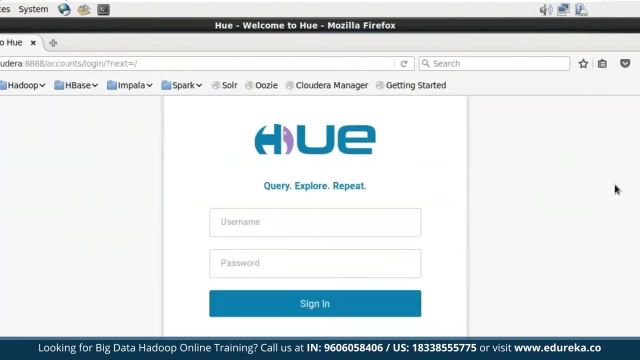 Now let me tell you in cloud error, the default username and password for everything is cloud error. For example, let's log into our hue using the username cloud error and password: cloud error. Now you might want to just select: remember to remember your password. 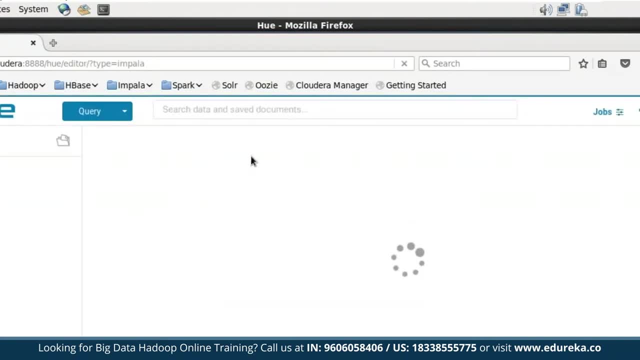 And there you go. You have successfully logged into hue And now, if you want your query editor for pic, you can just select the bottom arrow mark and then you can select editor and inside editor. You have the editor designed for pic. Now you are in the window where you can write big scripts. 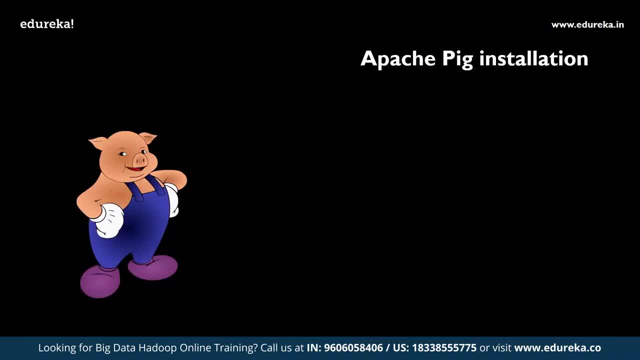 and execute them. Now we will move ahead into our next topic And after finishing the theory part, we shall come back into our cloud error and execute some of the basic operations on big terminal. So our next concept is understanding the pic architecture. 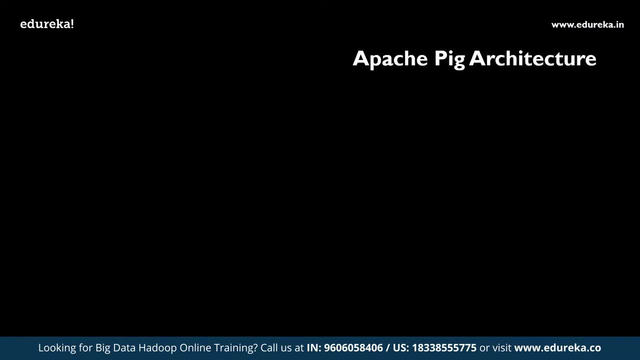 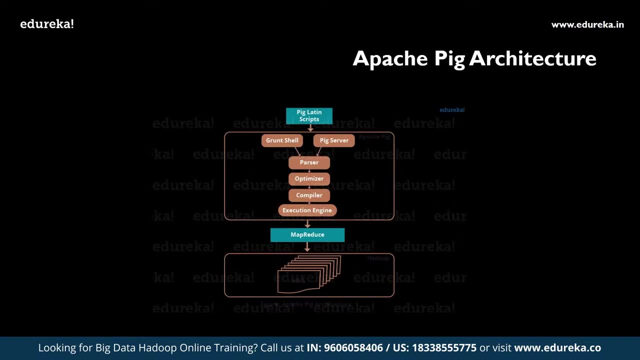 So first of all let us go through the diagram of big architecture. The following diagram represents the architecture of Apache pic. as shown in the figure, There are various components in Apache pic framework. Let us look at the major components. Firstly, the parser. 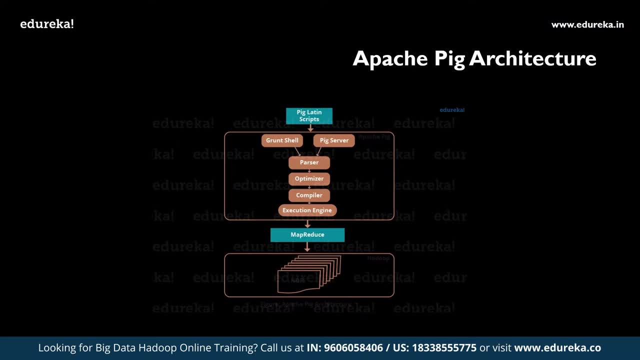 Initially, the pic scripts are handled by the parser. It checks the syntax of the script, does type checking and other miscellaneous checks. The output of the parser will be a DAG, which is directed acyclic graph, which represents the big Latin statements and logical operators. 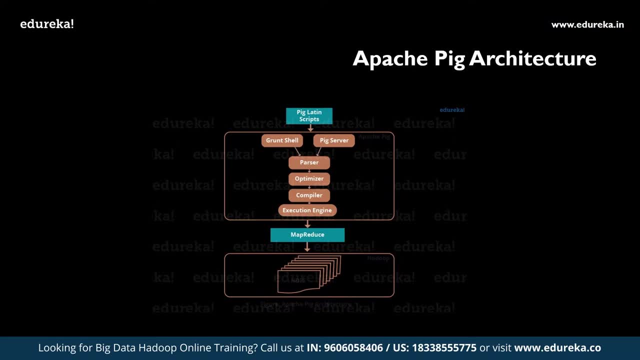 In directed acyclic graphs, the logical operators of the scripts are represented as the nodes, and data flows are represented as edges. And next the optimizer. The logical plan for directed acyclic graphs is passed to the logical optimizer. This carries out the logical optimizations. 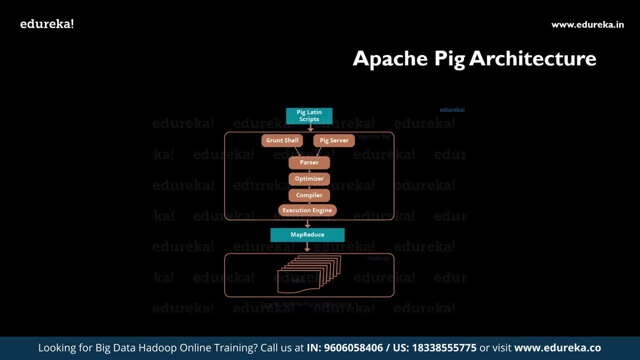 such as projections and push-downs. Next comes the compiler. The compiler is used to compile the optimized logical plan into the series of MapReduce jobs. Followed by that we have the execution engine. Finally, the MapReduce jobs are submitted to the Hadoop. 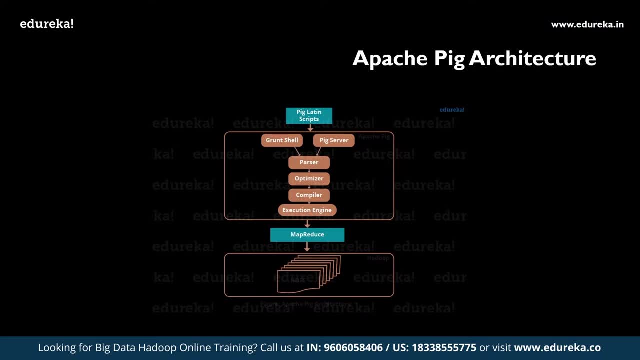 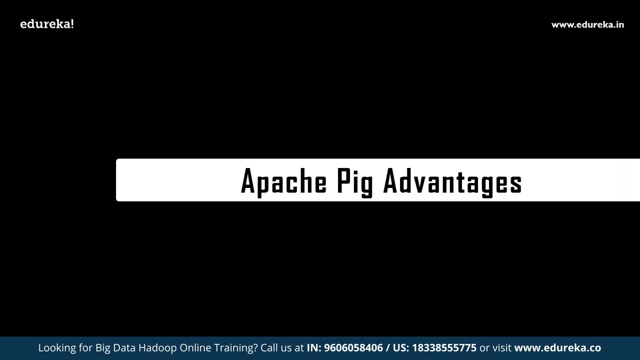 in a sorted order. Finally, these MapReduce jobs are executed On Hadoop, producing the desired results. So this was a basic explanation based on Apache Pig architecture. Now, moving ahead, we shall understand the major advantages of Apache Pig. So some of the major advantages of Apache Pig are: less code. 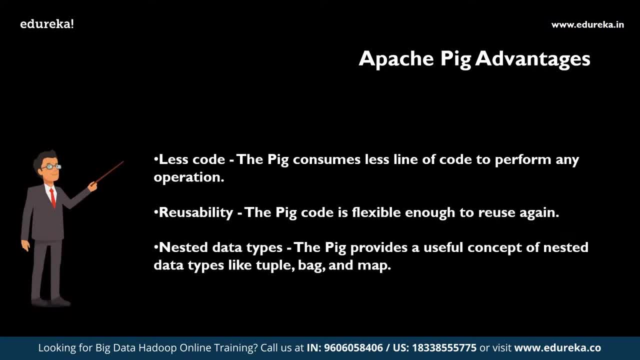 The pig consumes less than a line of code to perform any operation, So this reduces the number of lines included in the code, Followed by that code. reusability: The pig code is so flexible enough to reuse it again. You can basically write the pig script into a file. 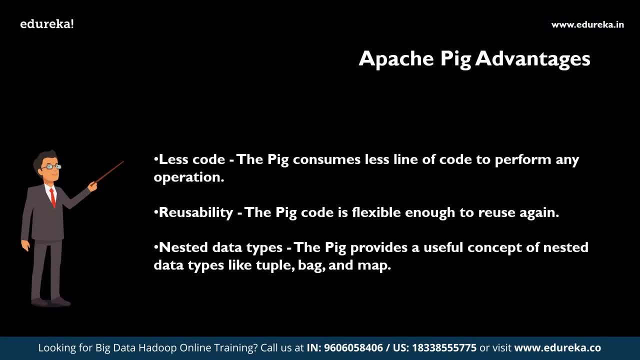 and access the file whenever you need it. So, followed by that, the next important advantage of Apache Pig is the nested data types. The pig provides a useful concept of nesting data types like tuple bag and map. So these were the few important advantages of Apache Pig. 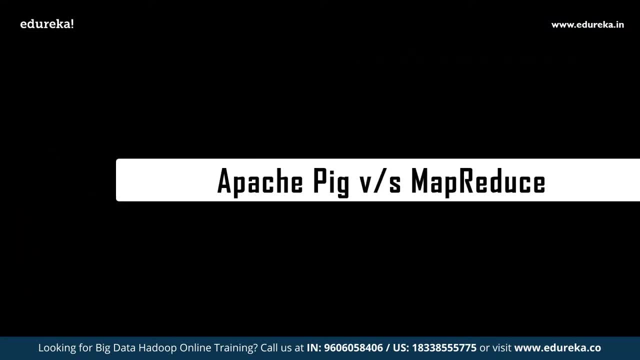 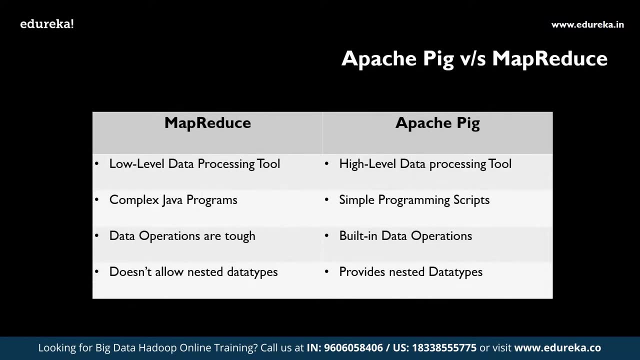 Now we shall move ahead into the next topic, which is about the differences between Apache Pig and Apache MapReduce. So there are basically four differences between Apache Pig and Apache MapReduce. So first up, we will begin with MapReduce. In MapReduce we have low-level data processing. 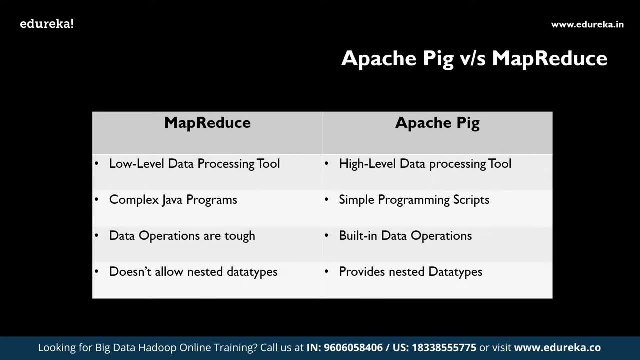 When it comes to Apache Pig, it is considered as a high-level data processing tool. Followed by that, the next important difference between MapReduce and Apache Pig is that we find complex Java programs when we are using MapReduce, But when we come into Apache Pig, 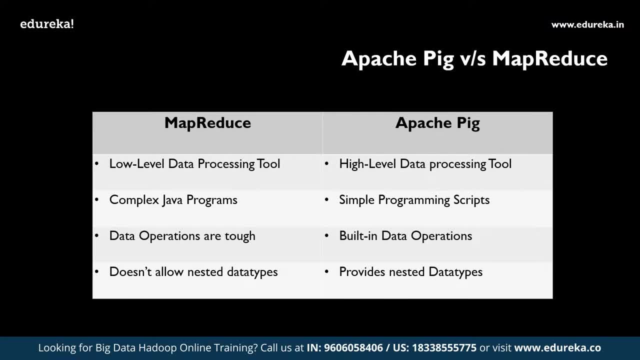 we have simple programming scripts which are shorter in code length and easily understandable. Followed by that, the third difference is the data operations are completely tough and complicated in MapReduce, But in Apache Pig you don't have to worry about those operations. 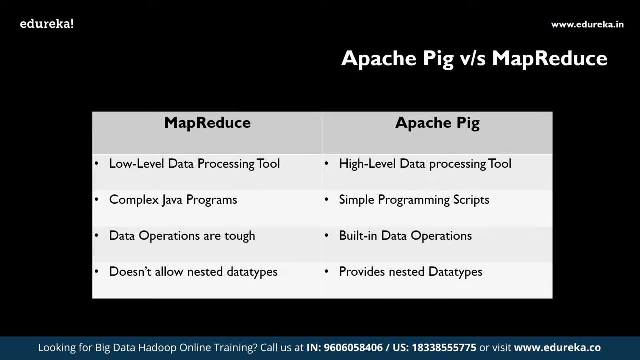 because they're already there, They're already built-in. Next and the last difference between MapReduce and Apache Pig is: Apache MapReduce does not allow nested data types, Whereas Apache Pig allows nested data types. So these were the basic differences between Apache MapReduce and Apache Pig. 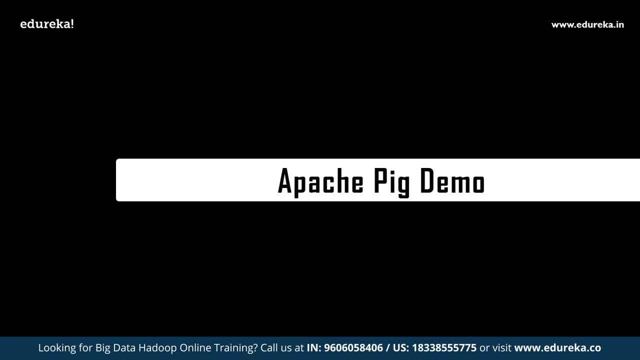 So the next topic is the Pig Demo. Here we will understand all the basic commands in Apache Pig and the basic functionalities which are available in Pig. Now, without further due, let's quickly begin with our demo for today's session. Now we have come back to our cloud era. 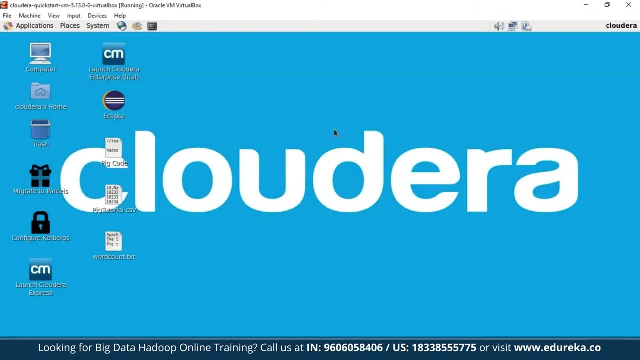 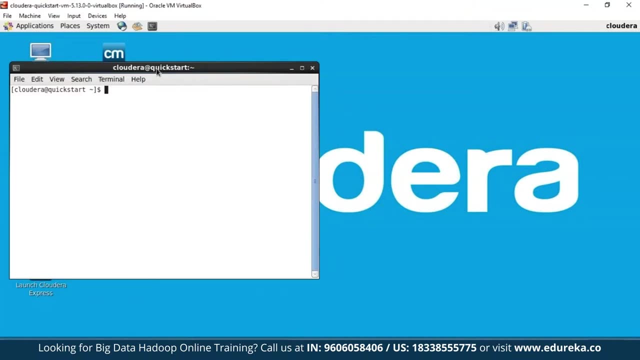 that we have installed into our local system. Now let's start Pig. As we have discussed before Apache Pig can be executed in two modes. They are the local mode and the MapReduce mode. Firstly, we shall execute an example based on local mode. 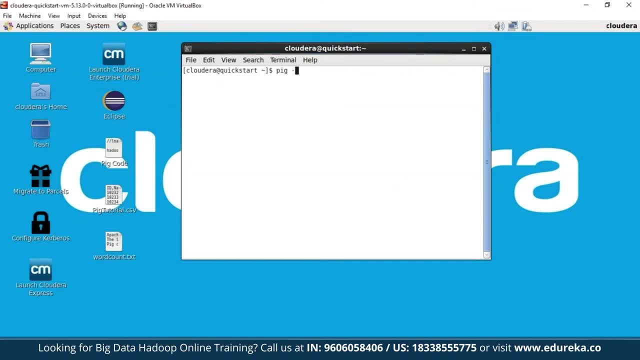 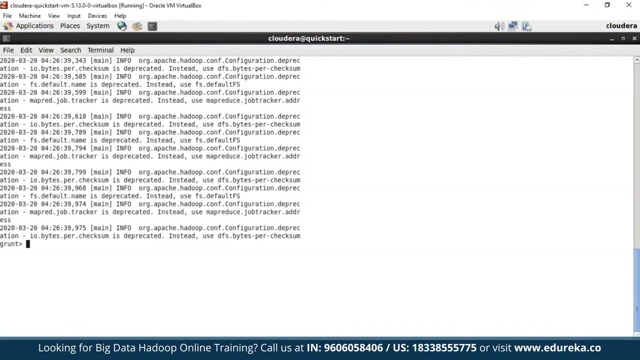 To start Pig in local mode, you need to type in the command Pig space hyphen X, space, local Firing. this command will enable Pig in local mode. As you can see, the command is getting decrypted. Now you can see that it has successfully started. 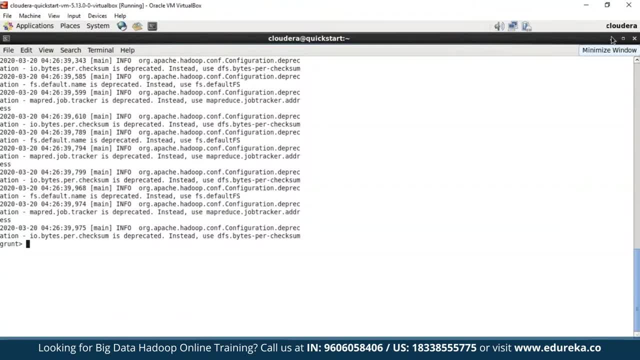 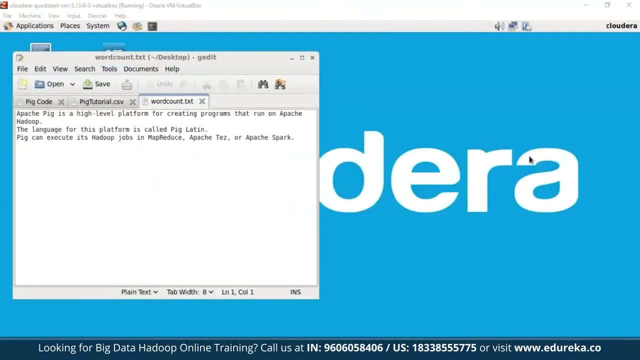 the grand shell in local mode. Now, what are we going to execute? We are going to execute a very simple word count program. For this particular word count example, I have considered a basic text, that is the definition of Apache Pig, Which happens to be: Apache Pig is a high-level platform. 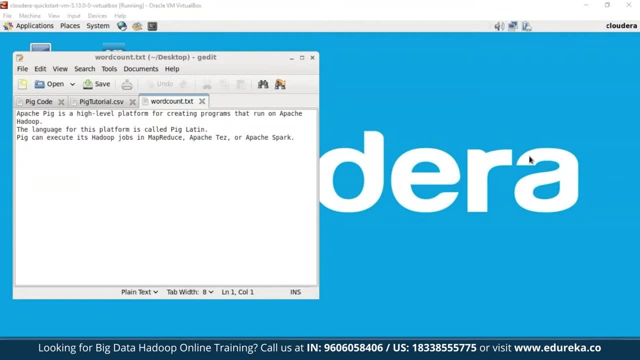 for creating programs that run on Apache Hadoop. The language for this particular platform is called Pig. Latin Pig can execute its Hadoop jobs in MapReduce, Apache Test and Apache Spark. So we will consider this particular paragraph and we will also count the number of words. 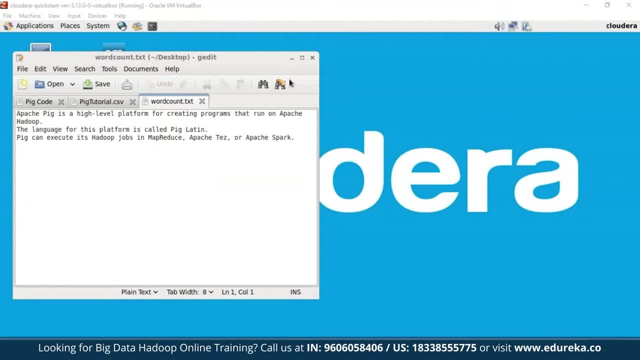 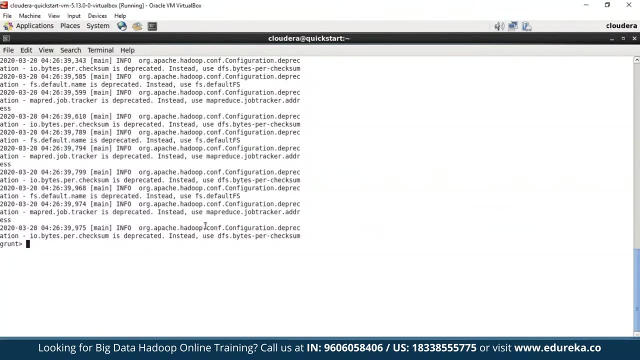 which are included in this particular paragraph. Now let's quickly go back to our terminal and execute our program. So now we have come back to our terminal, Let's clear it using the command control plus L. Now let's quickly start up typing our commands. 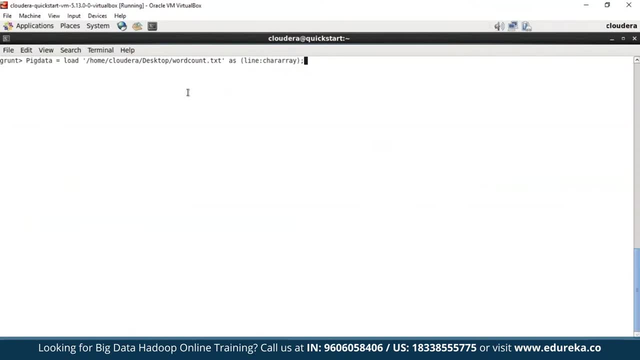 So, as discussed before, we are going to execute this particular program and local mode. So here we are not loading the data into HDFS. Instead, We are considering the local location, Which is the local location, that is, home cloud at our desktop word count. 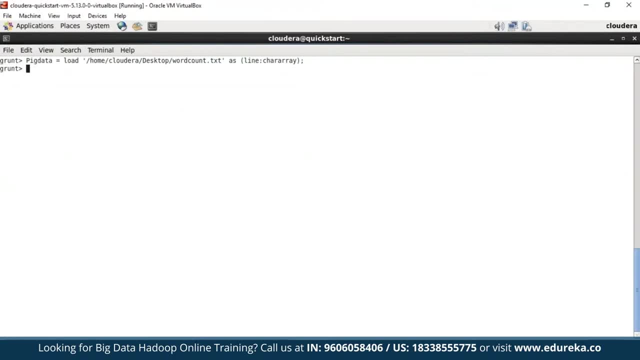 Now we are going to run this command and see the output. So the data has successfully loaded. Now we'll execute the next command. So now we are going to tokenize each and every single word in this particular paragraph and we will be considering each. 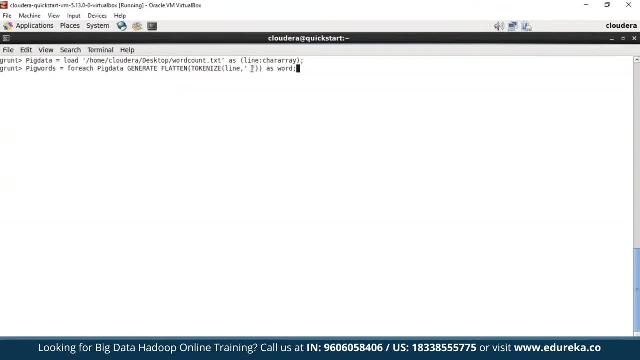 and every word as a single word, and we are going to separate each and every word by using a space. Now let's fire up this command and see the output. Yeah, the command just got executed, or the script just got executed. Now in the next script, 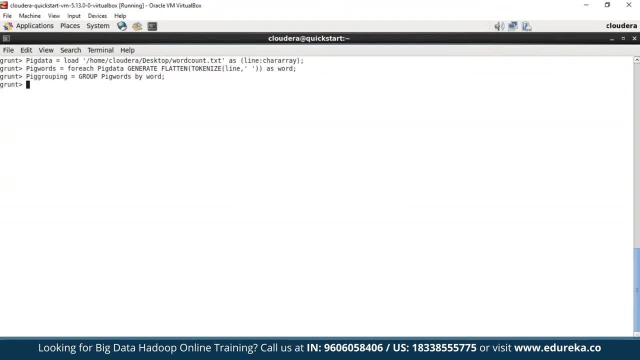 we are going to group the words according to their occurrence. Yeah, even that is done Now. the next script would help us to count the number of words which have been repeated. So even that is done Now. the last script would be dumping the output. 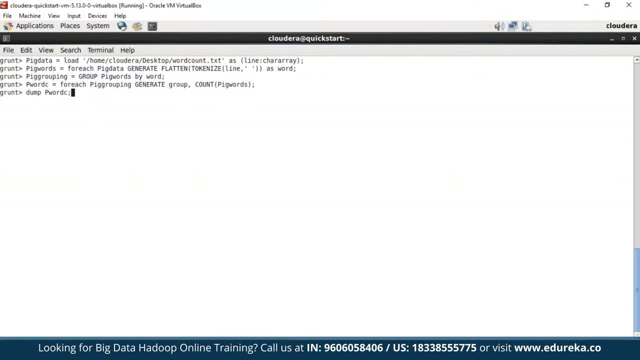 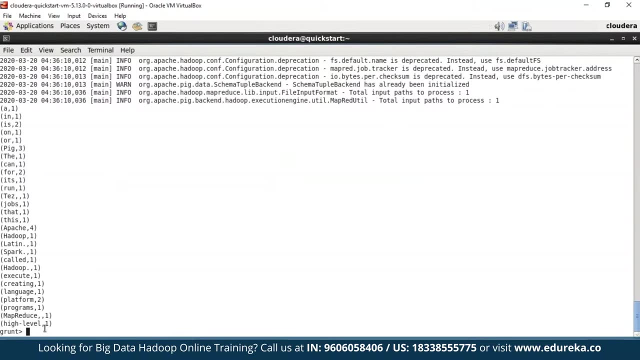 which is stored in P word C, which is big word count. Now let's enter the command and see the output. You can see some MapReduce jobs that are getting executed. And there you go, We have our output. So the words are a and on, for it stays: Hadoop Apache. 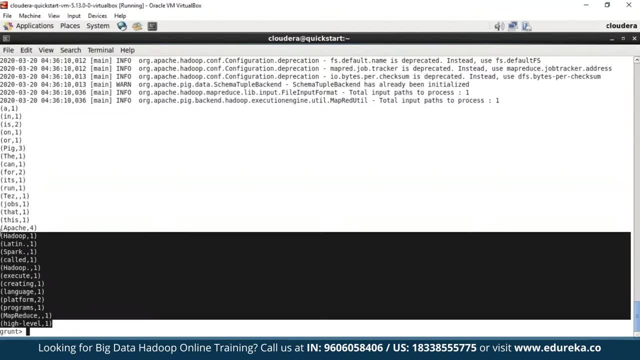 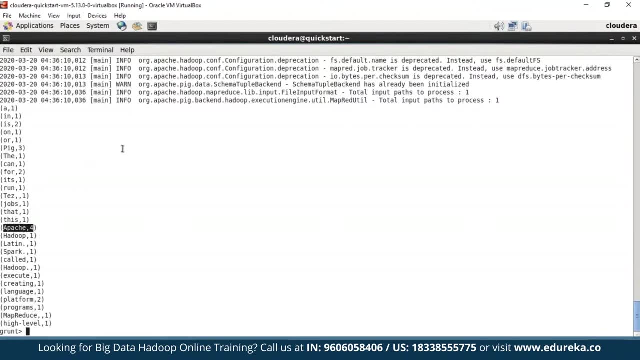 and all those words, and along with them, We also have the number of repetitions of each and every word. for example, we have Hadoop, which is repeated one time, and the word Apache is repeated for four times, and so on. So with this, now let us move ahead. 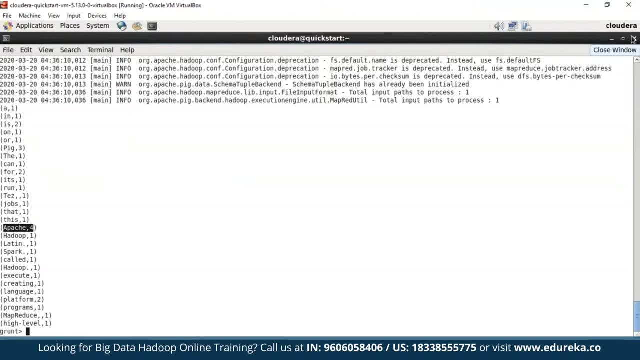 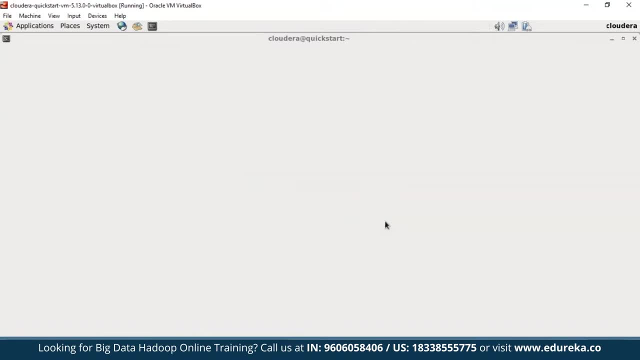 and execute some examples based on Apache's Hadoop mode or MapReduce mode. Now let's close this terminal and open a new one, and let's begin executing Hadoop in MapReduce mode. As discussed before, Apache pick can be executed in both local mode and MapReduce mode. 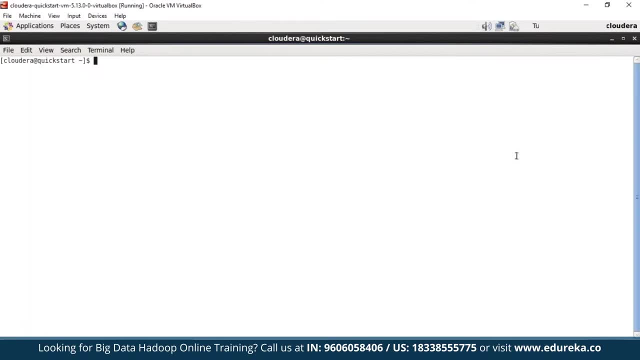 We have already executed some examples based on local mode. Now we should execute Some examples based on MapReduce mode. to do So, we will first load some local data into HDFS. So, using this command, I'll be loading my local data. that has picked tutorialcsv. 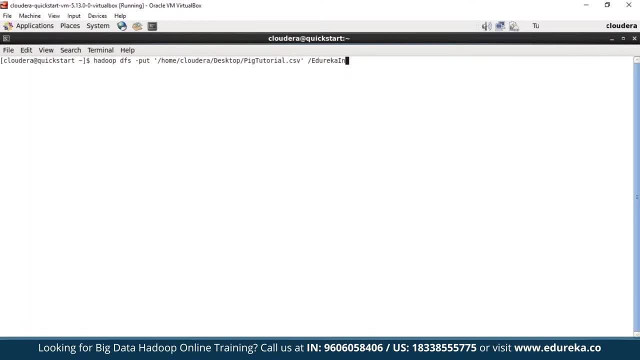 into my HDFS and I'll name it as Edureka in. as you can see, the command is getting deprecated And the data has been successfully loaded. Now let us use cat command and see what exactly is present in that particular data. As you can see, the command got deprecated. 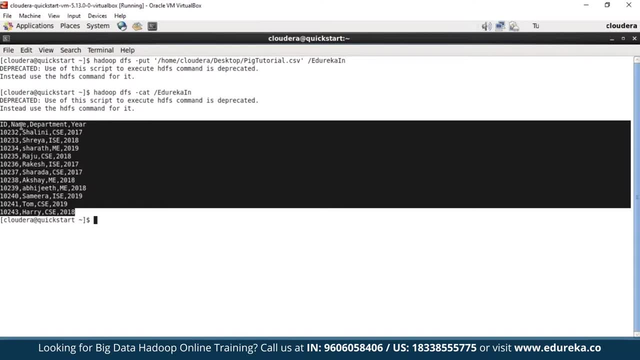 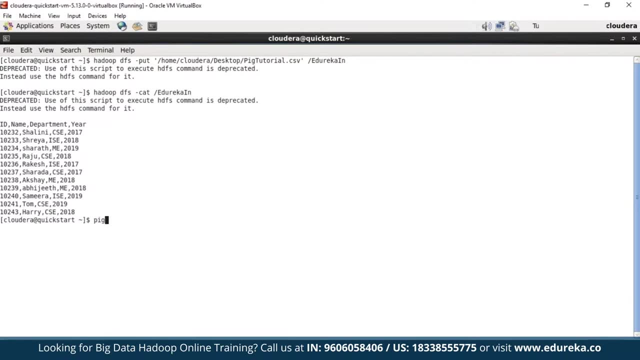 and the data is a simple CSV file related to students that has ID name, Department and year. Now let's start pick in MapReduce mode. to do So, we just need to type in pig and strike enter. There you go. We have successfully started pick in MapReduce mode. 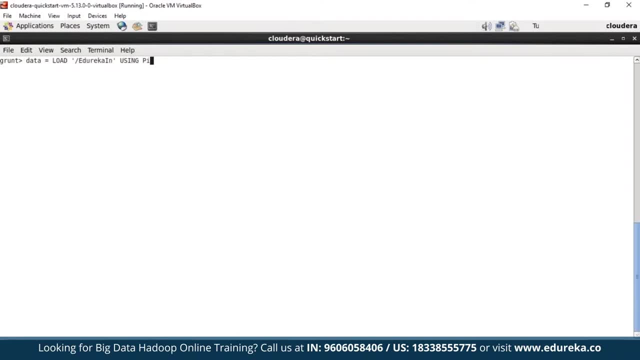 Now let's execute some commands. So, using this command, we will be loading at Eureka- And that is the data, the CSV file which we have discussed before, using pig storage as comma separated file, and schema for the data will be ID as character array, name as character array Department. 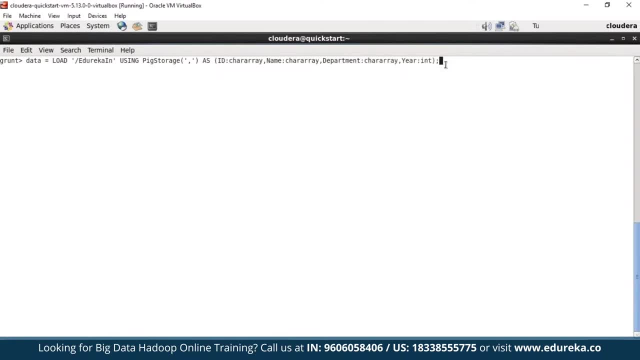 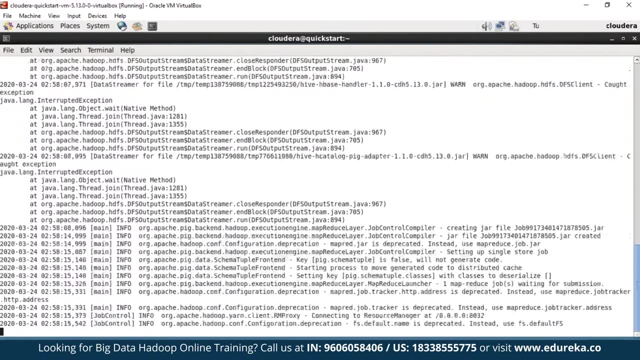 as character array and year as integer array. Now let's strike an enter and see the output. There you go. The data has been successfully loaded Now. Now let's use dump command to see the data, or have loaded. So there you go. 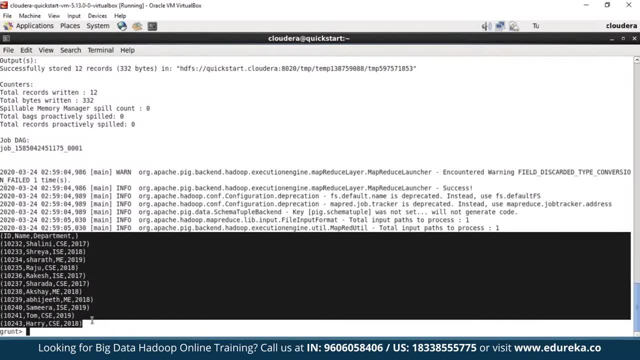 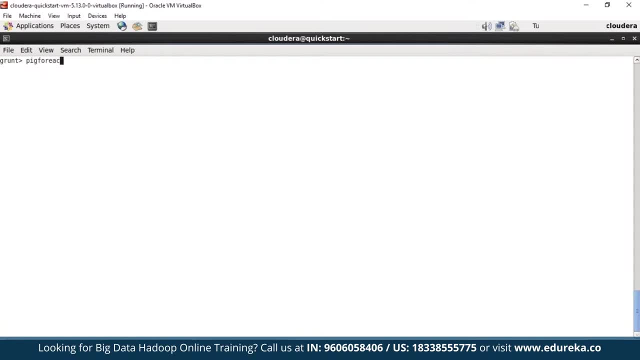 The data has been successfully dumped, So this was the data which we have loaded. Now let's move further and execute few more commands. Now we shall use: for each command and for each data present in our data file, we will generate ID, name and Department. 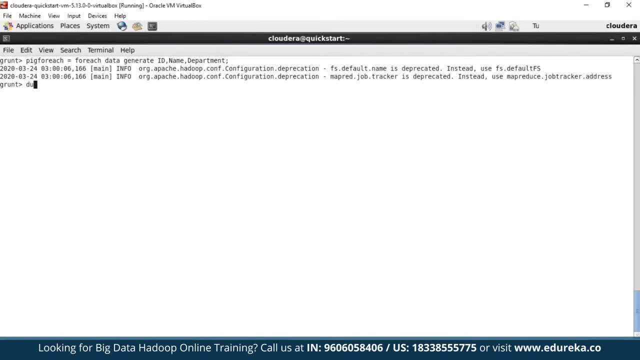 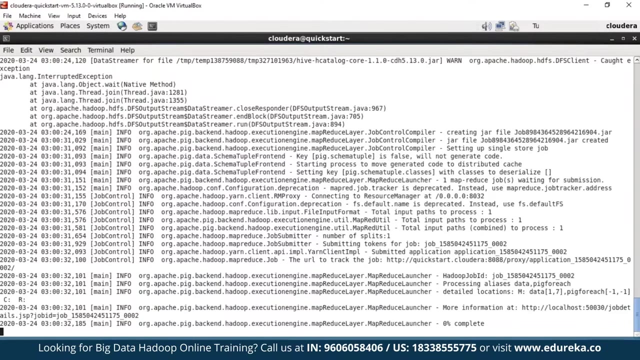 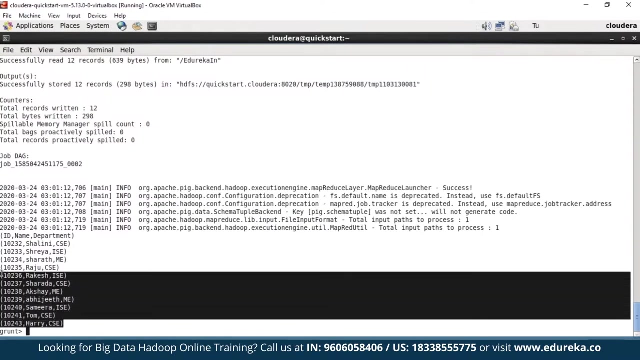 There you go. The command got successfully executed. Now let's dump the data using dump command. So pick for each is our variable that stores the data. Now let's type in semicolon and enter. So there you go. The for each command has been successfully executed. 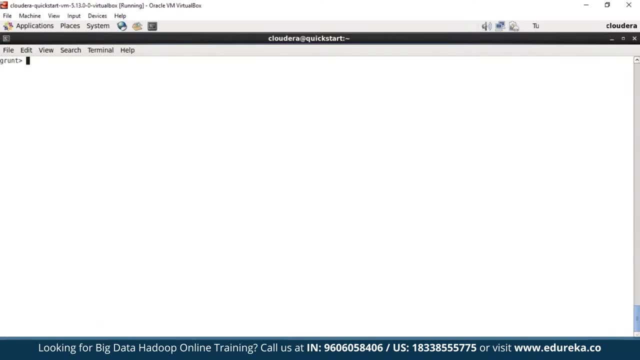 and we have generated ID, name and Department. Now we shall execute few more examples. Now we shall use descending operator to arrange the data in the form of descending order of ID. So it's been executed. Now let's dump the data and see the output. 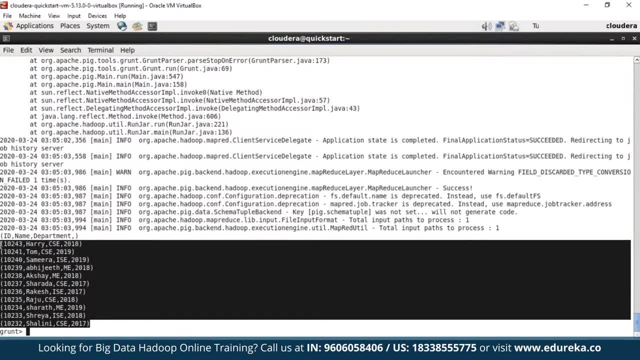 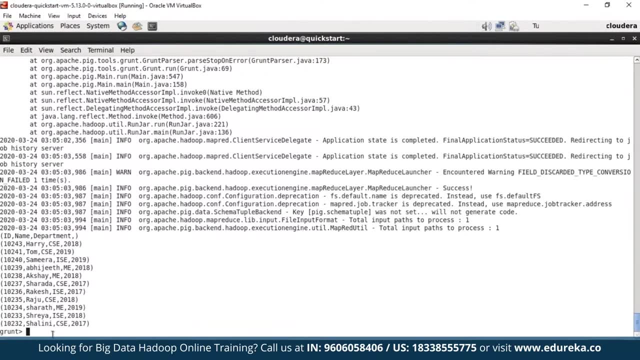 There you go. We have successfully executed the dumb command, and the IDs are arranged in the descending. Not enough, as you can see it Now. this is how the order by descending function works. Now let's move ahead and execute one last command. 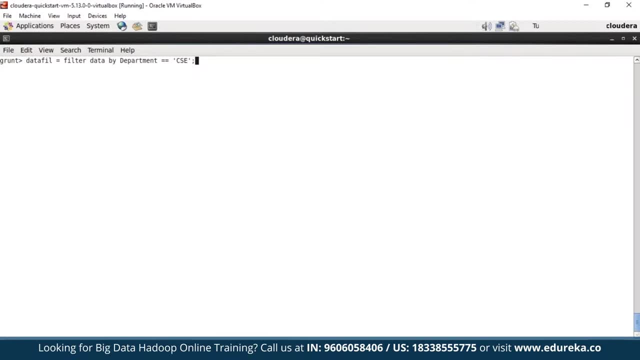 As you can see, here we are using filter operation. We are going to filter the students based on the department where Department is equals to CSE. So executing this command will give us the students which are inside the department CSE. Now the command got executed. 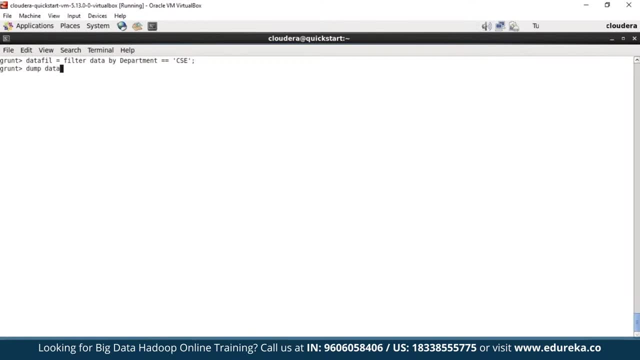 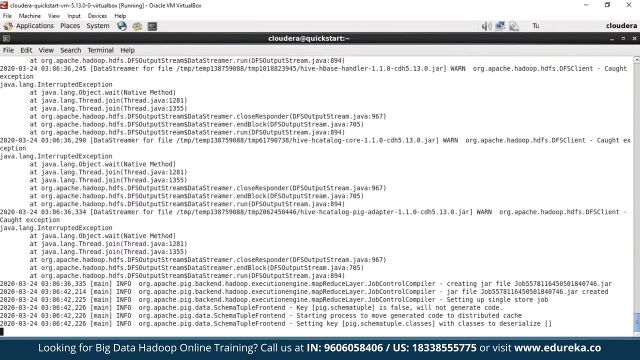 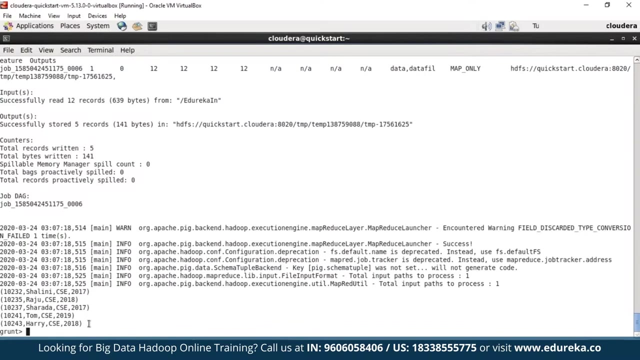 Now let's dump the data using dumb command. So there you go. You can see some commands getting deprecated Here. You can see the MapReduce shops getting executed. So there you go. You can finally see the output, which has the students. 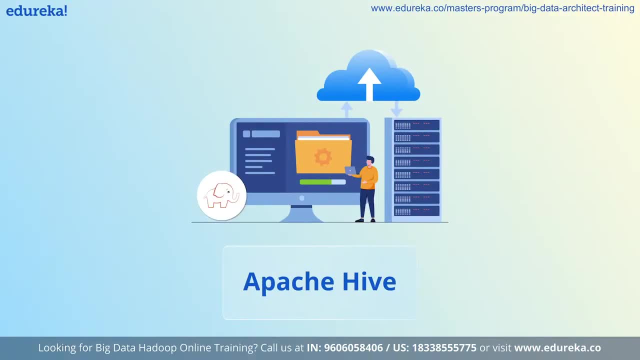 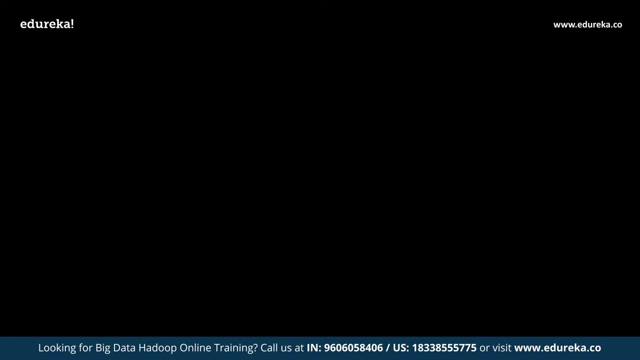 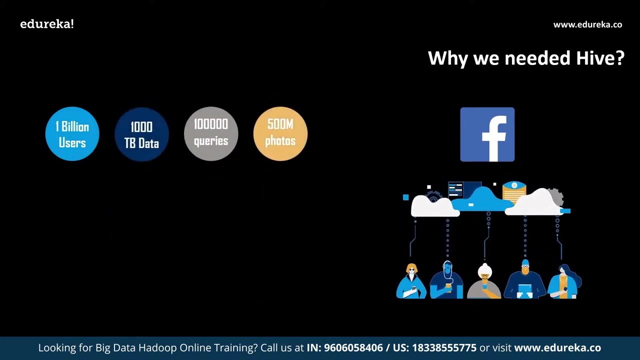 that belong to the CSE Department. Why exactly we needed Apache Hive? it all began in the early 90s when Facebook started. slowly, the number of users at Facebook increase- that is, nearly 1 billion users- and along with the users increase the data, which is nearly equals to thousands of terabytes of data. 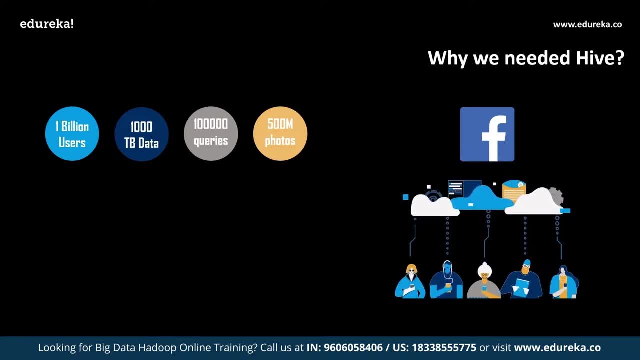 and nearly 1 lakh queries, then also 500 million photographs uploaded daily, and this was a huge amount of data that Facebook had to process, and the first thing that everybody had in their mind was to use RDBMS, and we all know that RDBMS couldn't handle such a huge amount of data. 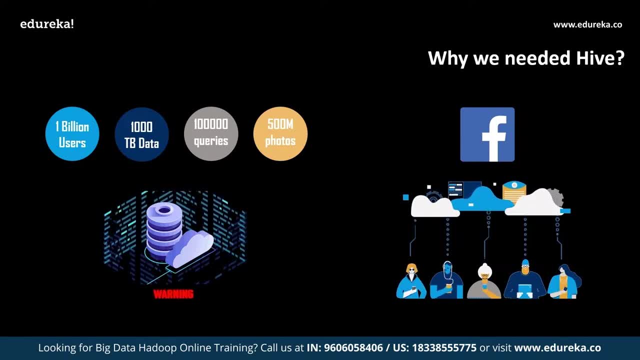 and neither it was capable enough to process it. and the very next big guy who was capable enough to handle all this big data was Hadoop. Even when Hadoop came into picture, it was not too easy to manage all the queries. it used to take a lot of time to execute all the queries perform. 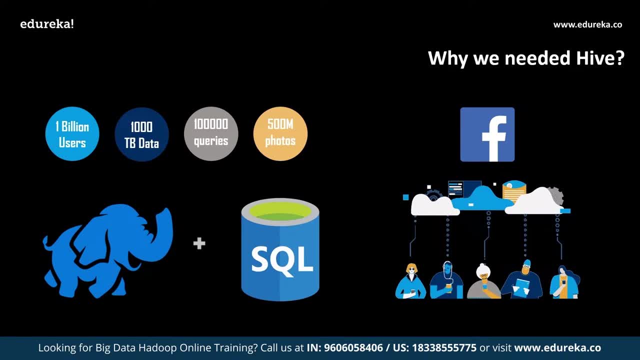 So one common thing that all the Hadoop developers had was the sequel. so they thought to come up with a new system, A solution that has Hadoop's capacity and interface like sequel. that is when Hive came into picture. So now we understand the exact definition of Apache: Hive, Apache. 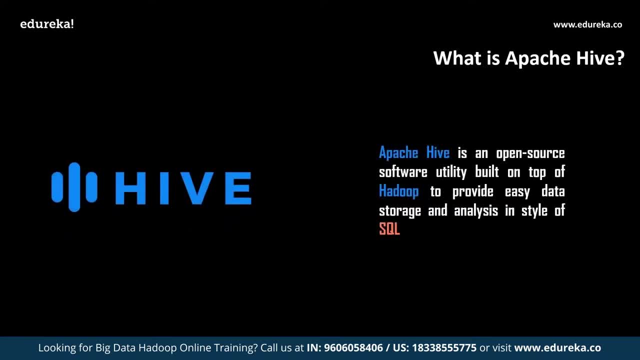 Hive is a data warehouse software project built on top of Apache Hadoop for providing data query and data analysis. Hive gives a sequel like interface to query data stored in various databases and file systems that integrate with Hadoop. also Apache Hive has data warehousing software. 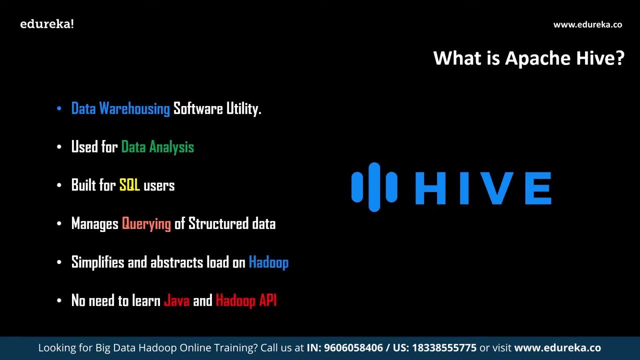 utility. It can be used for data analytics, It is built for sequel users, manages querying of structured data and it simplifies and abstracts the load that is on Hadoop. and, lastly, no need to learn Java and Hadoop API to handle data using Hive. 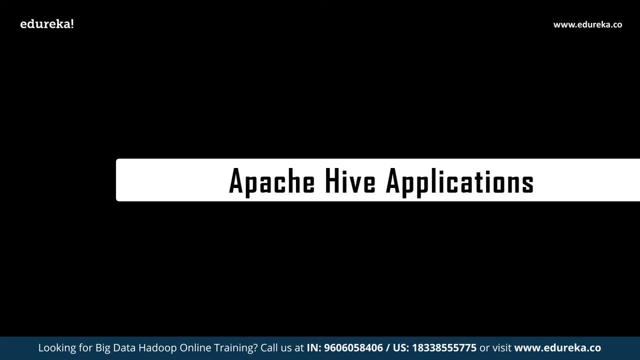 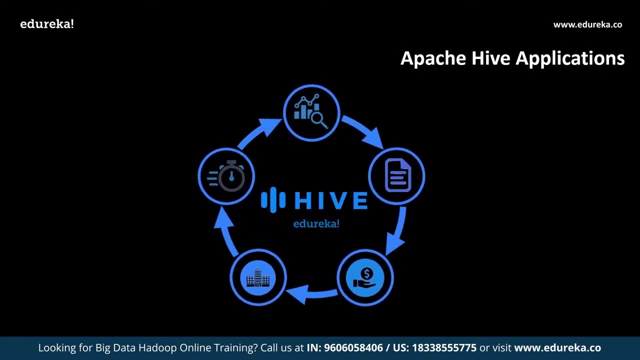 So, followed by this, we shall understand Apache Hive applications. Apache Hive is used in many major applications. few of the major applications are as follows: Hive is a data warehouse warehousing infrastructure for Hadoop. The primary responsibility of Hive is to provide data summarization, query and data analysis. 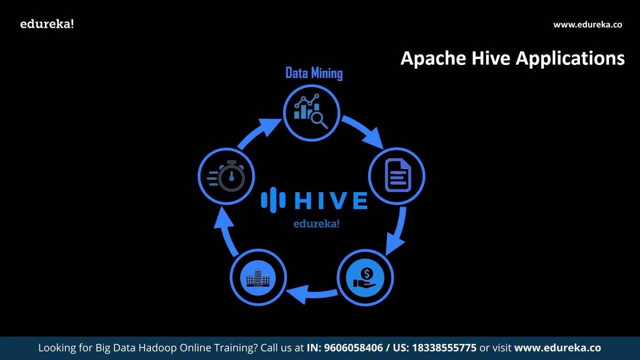 It supports analysis of large data sets in Hadoop, HDFS as well as on Amazon s3 file system. followed by that, we have document indexing with Hive. the goal of Hive indexing is to improve the speed of query look up on certain columns of a table. without an index, queries could 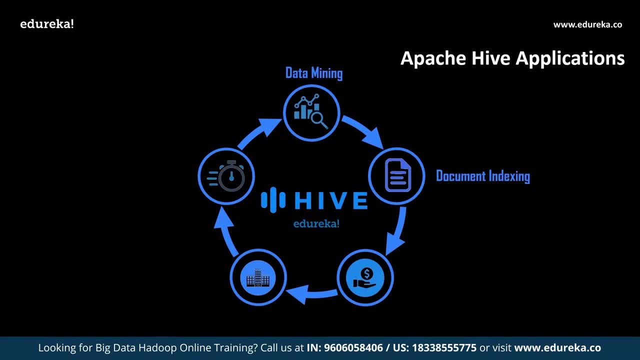 load an entire table or partition a whole process as rows. this would be troublesome, So with Hive we have solved this problem, followed by that predictive modeling. the data manager allows you to prepare your data So it can be processed in automated analytics. It offers a variety of preparation functionalities. 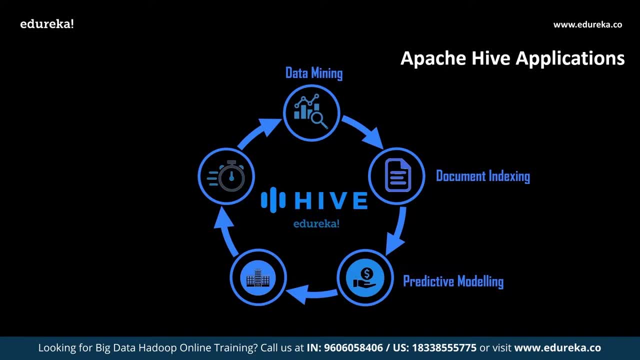 including the creation of analytical records and timestamp populations, followed by that. the next important application of Hive is business intelligence. Hive is a data warehousing component of Hadoop, and it functions well with structured data, enabling ad-hoc queries against large transactional data sets. Hence it happens to be a best-in-class tool available. 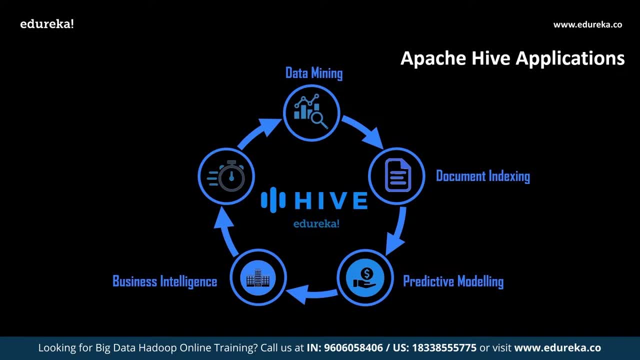 for business intelligence and helps many companies to predict their business requirements with high accuracy. last but not the least, log processing. Apache Hive is a data warehouse infrastructure built on top of Hadoop. It allows processing of data with sequel, like queries, and is very pluggable. 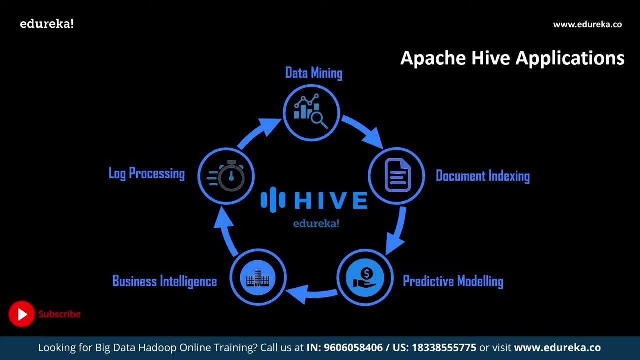 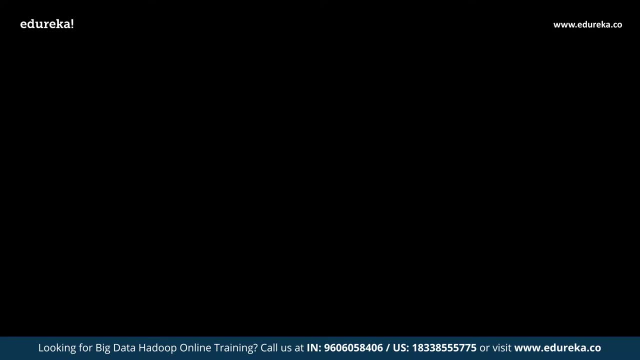 So that we can configure it to provide our logs quite easily. So these are the few important Hive applications. now let us move ahead and understand Apache Hive features. the first and the foremost important feature of Apache Hive is sequel type queries. the sequel type queries present. 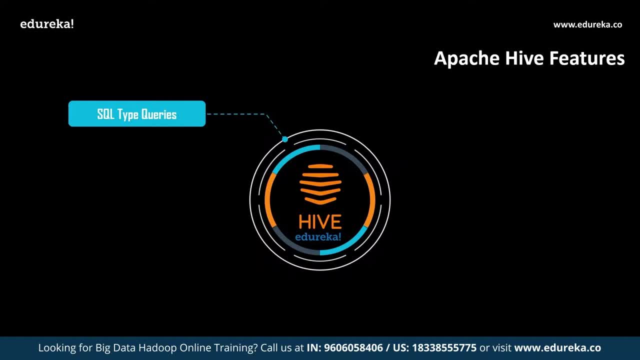 on Hive will help many of the Hadoop developers to write queries with ease. followed by that, the next important feature of Apache Hive is OLAP based design. OLAP is nothing but online analytical processing. this allows users to analyze database information from multiple database systems at one time. 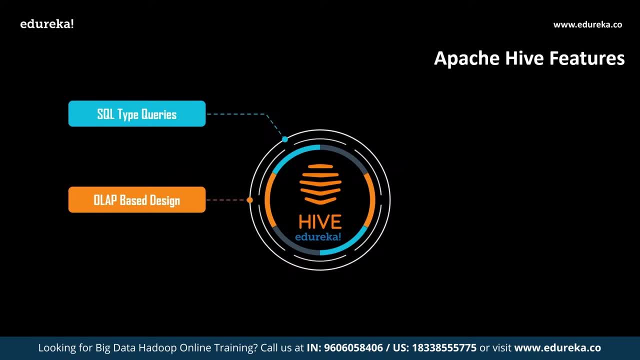 So using Apache Hive we can achieve OLAP with higher accuracy. followed by the second feature, We have the third feature which says Apache Hive is really fast, since we have sequel like interface in Apache Hive. using this feature on HDFS will help us writing queries faster. 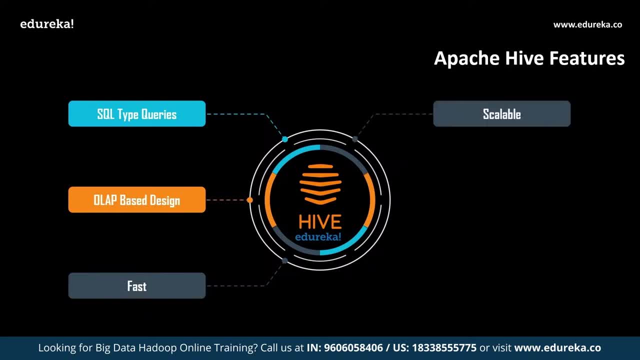 and executing them. followed by that, we believe Apache Hive is highly scalable. Hive tables are different directly in Hadoop file system. Hence Hive is fast and scalable and easy to learn, followed by that it is known to be highly extensible. Apache Hive uses Hadoop file system and Hadoop file systems. 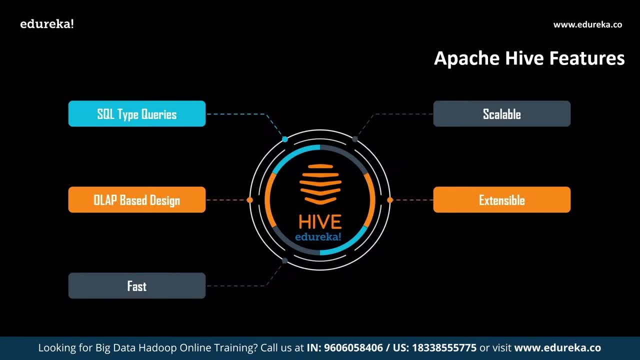 or HDFS, provides horizontal extensibility. and finally, the ad-hoc querying. using Hive, we can execute ad-hoc querying to analyze and predict data. So these were the few important features of Apache Hive. Let us move on to our next topic where we deal. 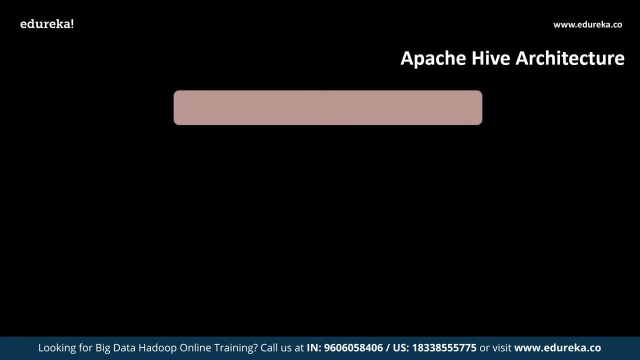 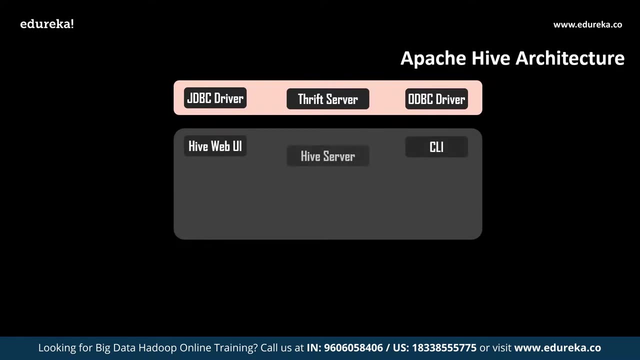 with Apache Hive architecture. the following architecture explains the flow of submission of query into Hive. The first stage is the Hive client. Hive allows writing applications in various languages, including Java, Python and C++. It supports different types of clients, such as thrift server, JDBC driver and ODBC driver. 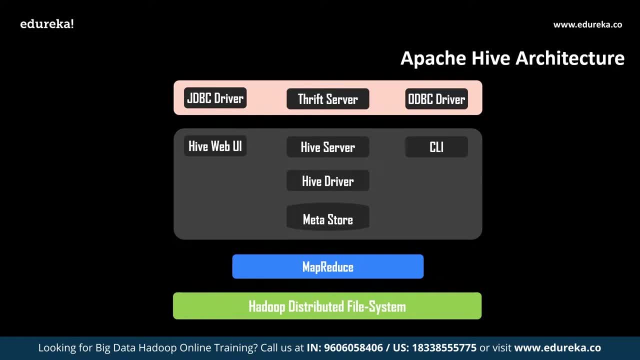 So what exactly is thrift server? It is a cross-language service provider platform that serves the request from all these programming languages that supports thrift, followed by that JDBC driver. It is used to establish connection between Hive and Java applications. The JDBC driver is present in the class or dot. Apache, dot Hadoop. 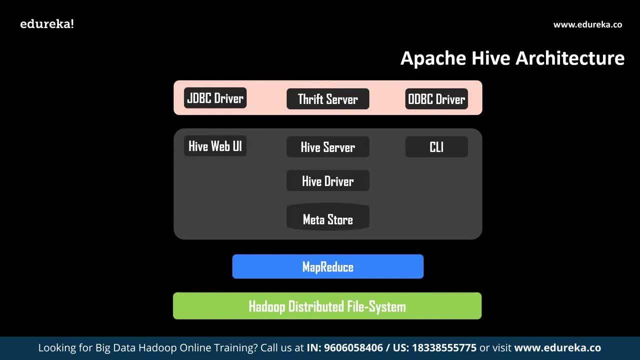 dot. Hive dot. JDBC dot. Hive driver. Finally, we come to ODBC driver. So what exactly is ODBC driver? ODBC driver allows the applications that support ODBC protocol to connect to Hive. followed by that we have the Hive services. the following other services provided by Hive: 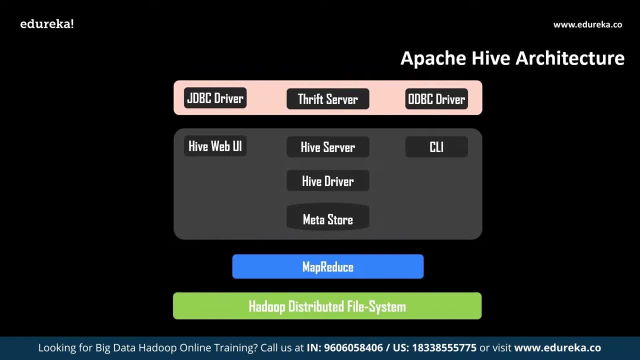 They are: Hive CLI, Hive web user interface, Hive Metastore, Hive server, Hive driver, Hive compiler and, lastly, the Hive execution engine, the Hive CLI, or command line interface. It is a shell where we can execute the Hive queries and commands. followed by that, the Hive web UI is just. 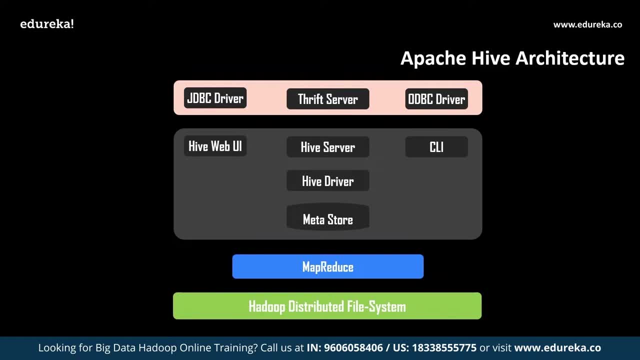 an alternative for Hive CLI. It provides a web-based graphical user interface for executing Hive queries and commands, followed by that the Hive Metastore. it is a central repository that stores all the structured information of various tables and partitions in the warehouse. It also includes metadata of column. 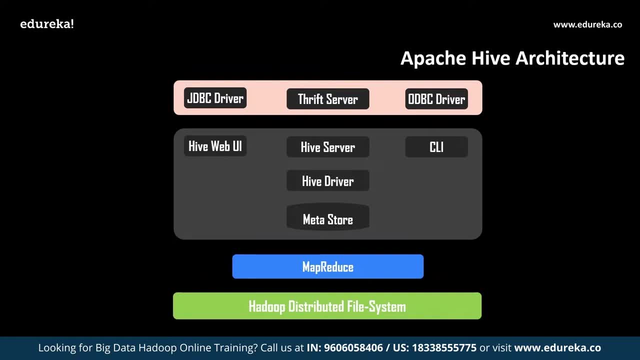 and its type. The serializers and deserializers, which is used to read and write data, and the corresponding HDFS files where the data is stored, followed by that the Hive server. It is referred to as Apache Thrift server. It accepts the request from different clients. 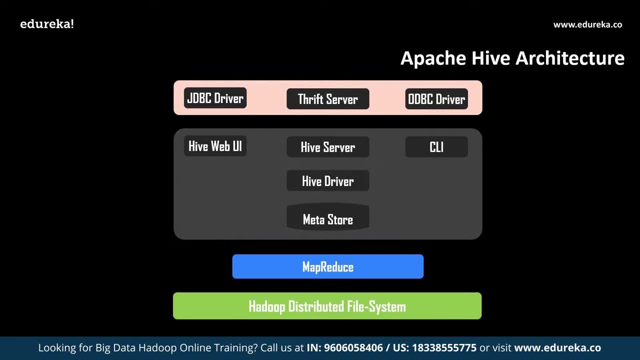 and provides to the Hive driver. moving on, We should deal with Hive driver. the Hive driver receives queries from different sources, such as web UI, CLI, Thrift and JDBC or ODBC drivers. It transfers the queries to the compiler, followed by that we have the Hive compiler. the purpose: 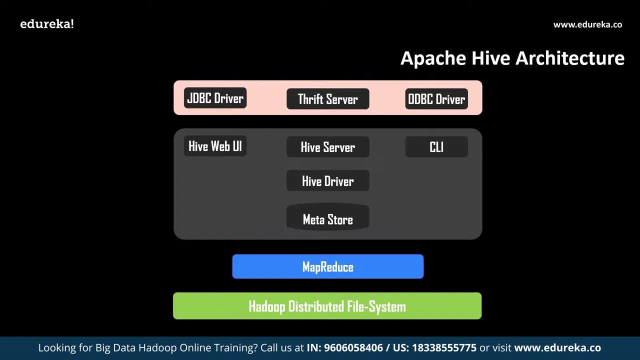 of Hive compiler is to pass the query and perform semantic analysis on the different query blocks and expressions. It converts Hive QL statements into MapReduce jobs. Finally, we have Hive execution engine. Hive execution engine is the optimizer that generates the logical plan in the form. 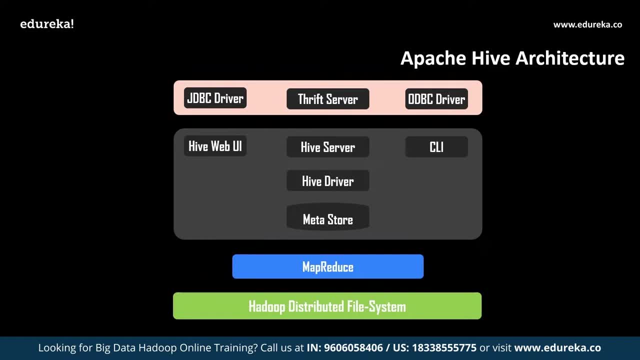 of DAG or directed acyclic graph of MapReduce Tasks and HDFS tasks. in the end, the execution engine executes the incoming task in the order of their dependencies. followed by that we have the MapReduce and HDFS. MapReduce is the processing layer which executes the mapping. 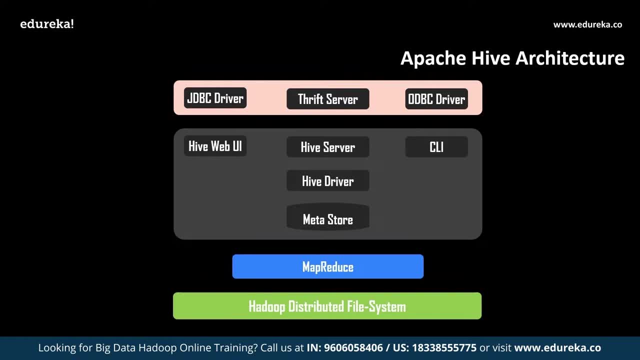 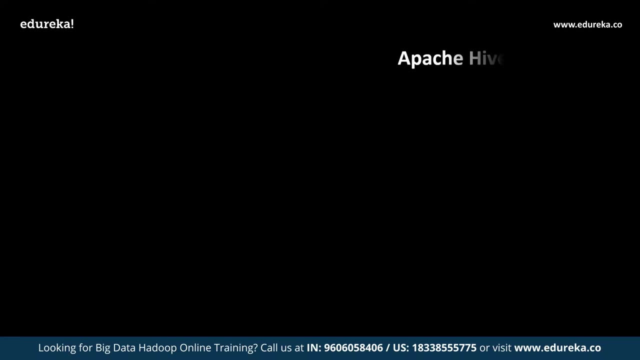 and reducing jobs on the data provided. lastly, the HDFS, or Hadoop, distributed file system is the location where the data which we provide is stored. So this is the architecture of Apache Hive. then, moving next, we have Apache Hive components. So what are the different components which are present? 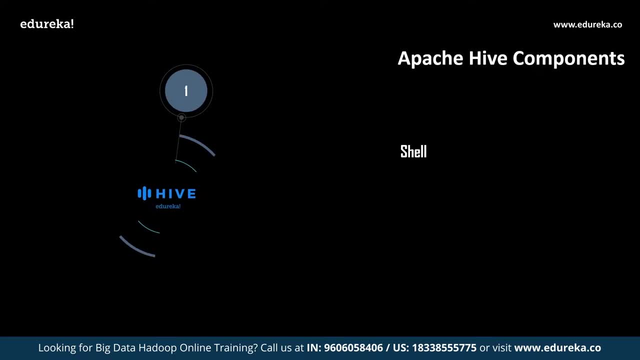 in Hive. they are first one, the shell. shell is the place where we write our queries and execute them. followed by that we have metastore, as discussed in the architecture. The metastore is a place where all the details related to our tables is stored, like schema, Etc. followed by that we have the execution engine. 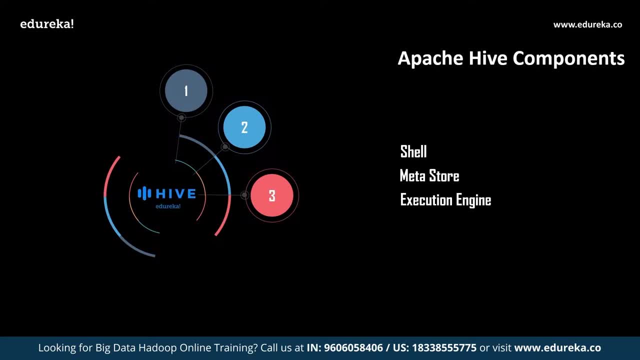 So execution engine is the component of Apache Hive which converts the query or the code which we have written into the language which the Hive can understand, followed by that driver is the component which executes the code or query in the form of acyclic graphs and lastly, the compiler. compiler compiles. 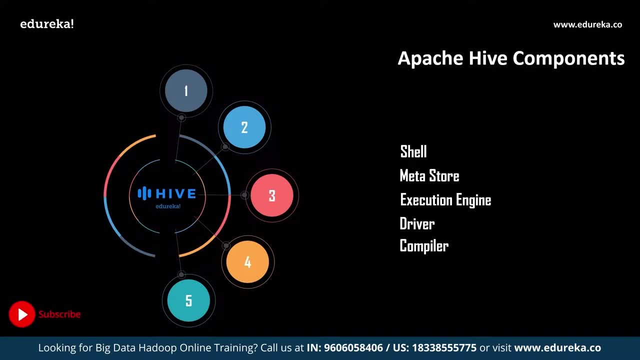 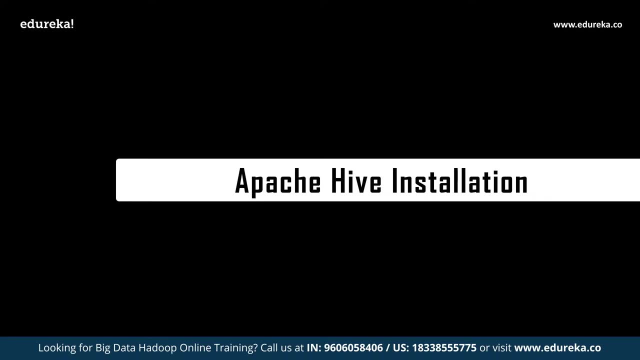 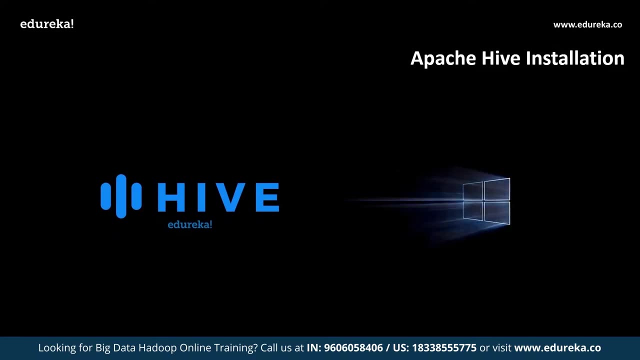 whatever the code we write and executes and provides as the output. So these are the major Hive components. moving ahead, We shall understand Apache Hive installation on Windows operating system. So it, Eureka, is all about providing the technical knowledge in the simplest way as possible and later play around. 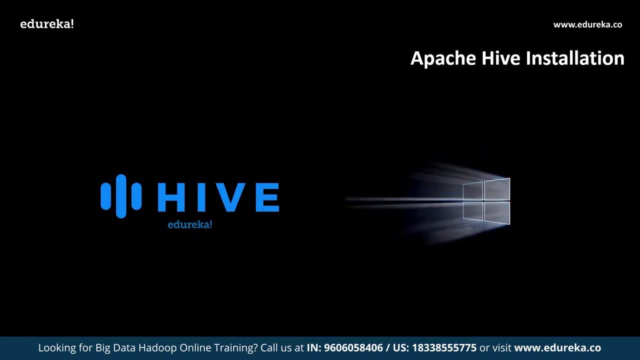 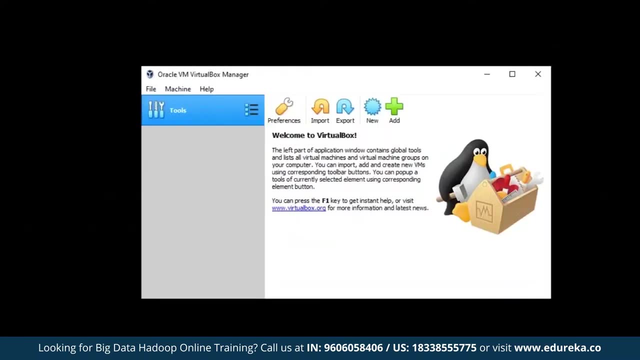 with the technologies to understand the complicated parts of it. So now let's try to install Hive into our local system in the most simplest way as possible. to do So we might need the Oracle Virtual Box, from which looks like this: So once after you download Oracle Virtual Box, 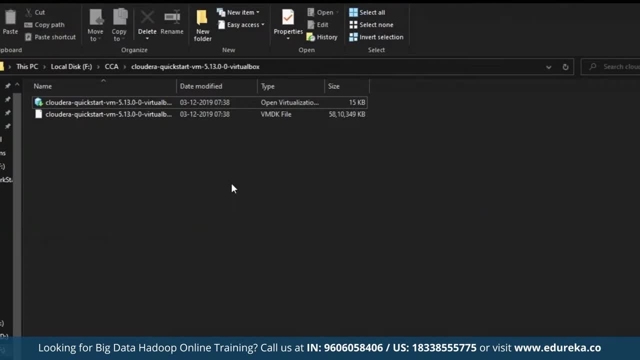 and install it into your local system. the next step would be to download the cloud Iraq Quick Start VM for your local system. The link to this will be provided in the description box below. Now let's quickly start our cloud Iraq Quick Start VM. 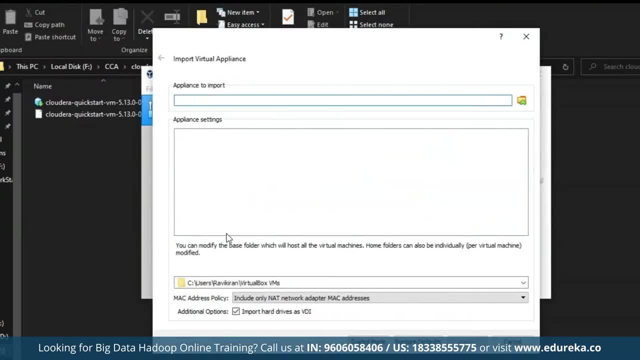 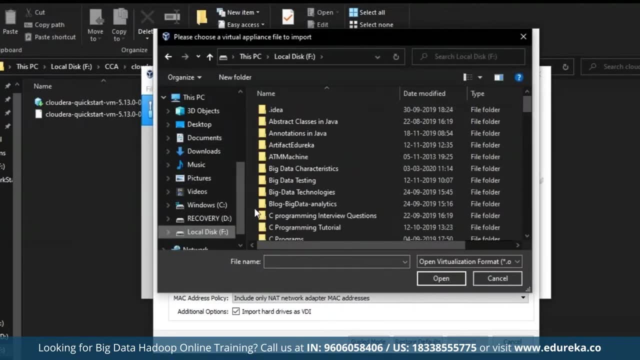 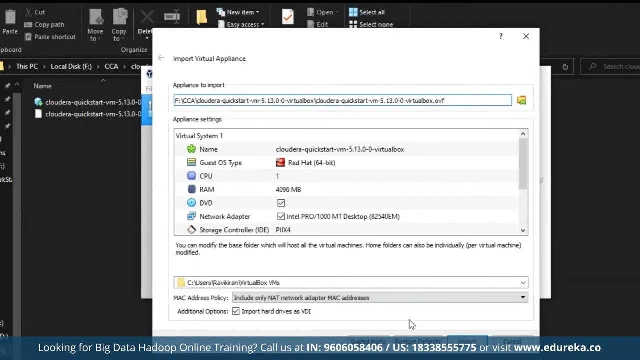 with our Oracle Virtual Box. select import option and now provide the location where your cloud Iraq Quick Start VM is existing. in my local system It is in the local disk drive F. There you go, Select open and now just make sure your RAM size is more. 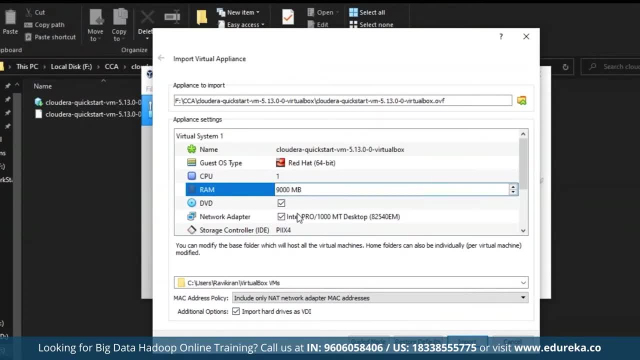 than 8 GB Just randomly. I'm providing 9000 MB, which is just about 8 GB, so that you have a smooth functionality of cloud around. now select import And there you go. You can see that cloud Iraq Quick Start VM is getting imported. 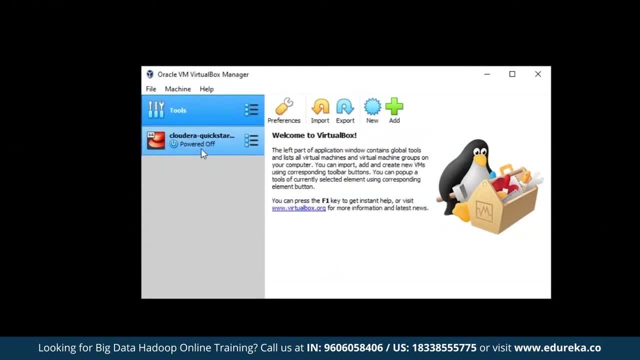 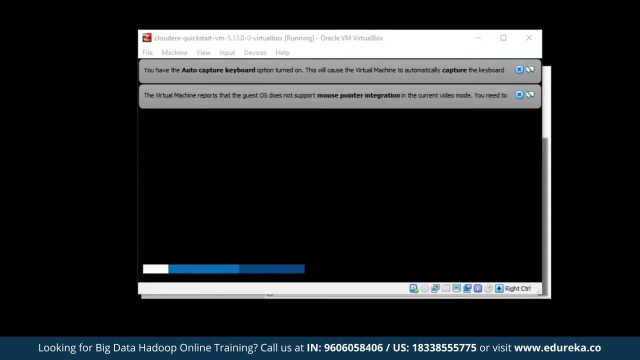 Now you can see that cloud Iraq Quick Start VM has been successfully important and it's ready for deployment. You can just double click on it and it'll get started. You can see that cloud Iraq VM has been successfully imported and it started, and also you can see: 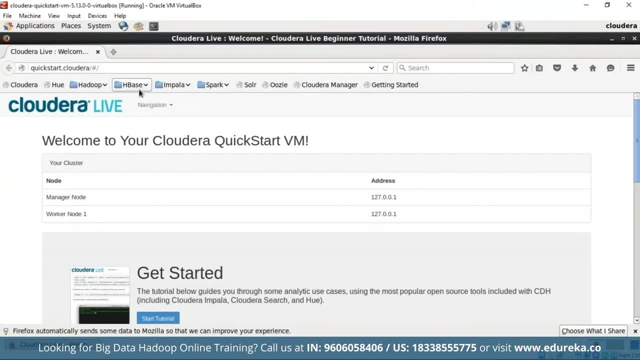 that we have gone live on cloud Iraq. You can see all the hue, Hadoop, edge, space, Impala, spark, which are pre-installed in cloud Iraq. Now our concern would be to start up hive. So to start hive, you need to start up hue first. 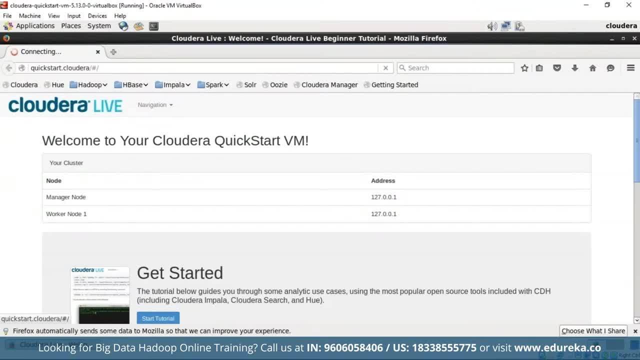 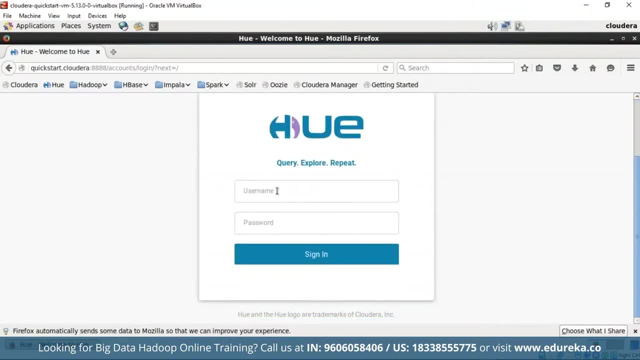 So let me remind you one thing: in cloud era, every single password and username is cloud era by default. So, for example, we have got hue username and password here, So the username that is the default username for cloud at us, hue- would be cloud era. 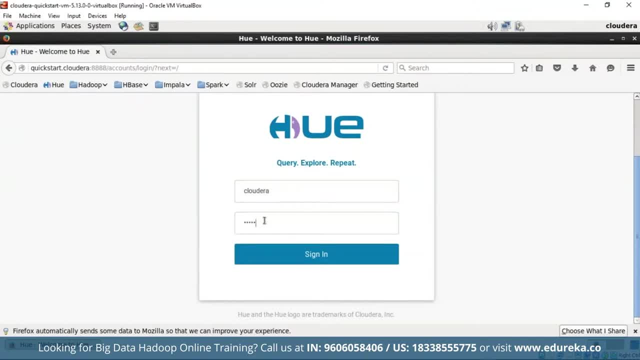 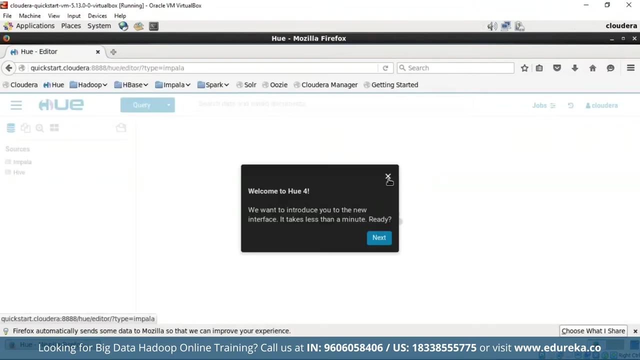 and along with that, even the password will be cloud era. that is by default. So we have got cloud era and cloud era as username and password respectively. Let's just sign in. you may select remember option in case if you forget your passwords. So now we are getting connected to you. 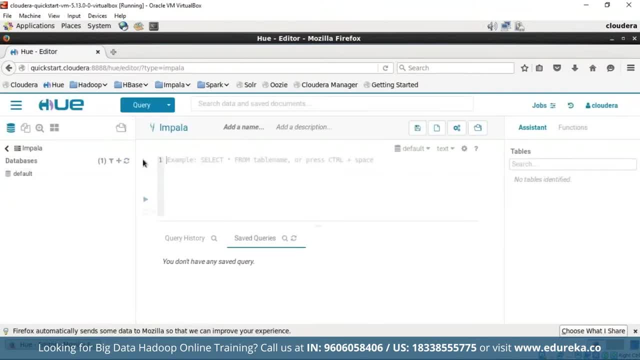 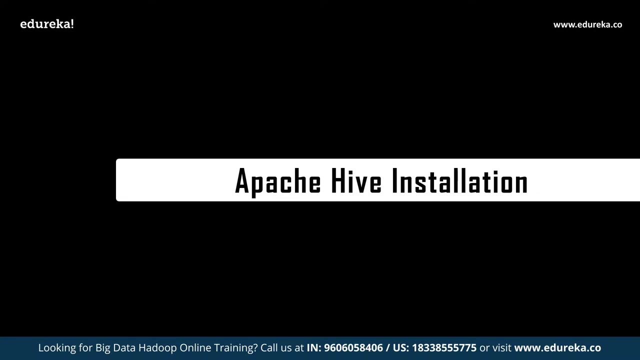 and we are live on here now. There you go. We've got started our hue, So now we'll enter into HDFS. There we go. We have a hype here. Now that we have successfully installed hype into our local system, Let us move further and understand few more concepts. 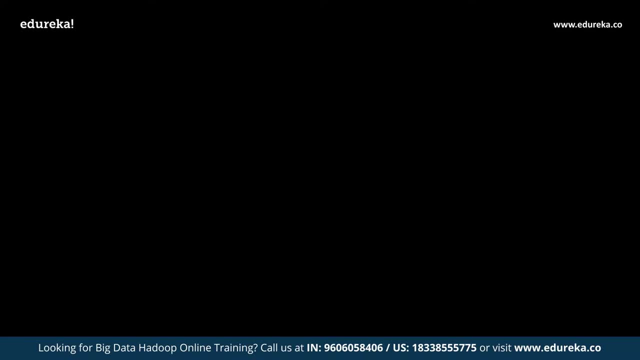 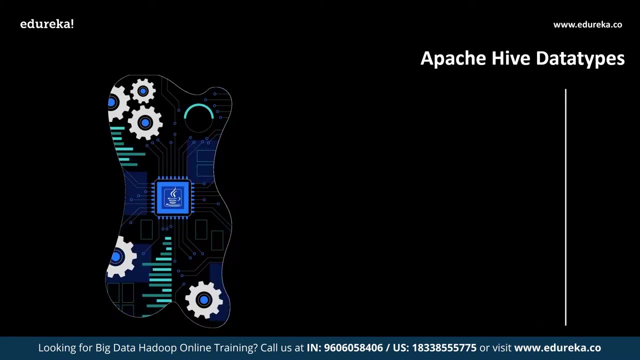 in Hadoop. Firstly, we should deal with the data types. The data types are completely similar to any other programming language, which we have their tiny and small and integer big, and similarly, followed by that, we have float, and inside high float is used for signal precision. 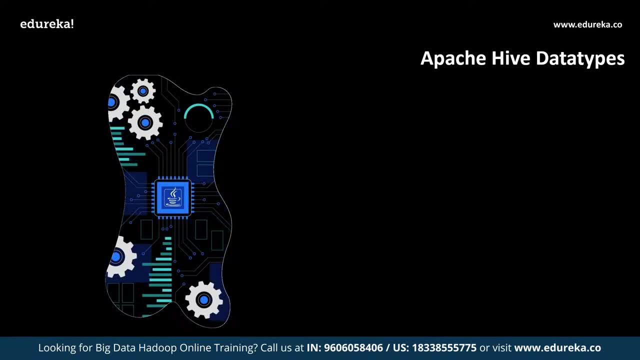 And if you want double precision, you can go ahead with double and followed by that, We have a string and Boolean which are completely similar to any other programming languages which we use in this daily life. followed by that, We have hive data models. So these are the basic data models. 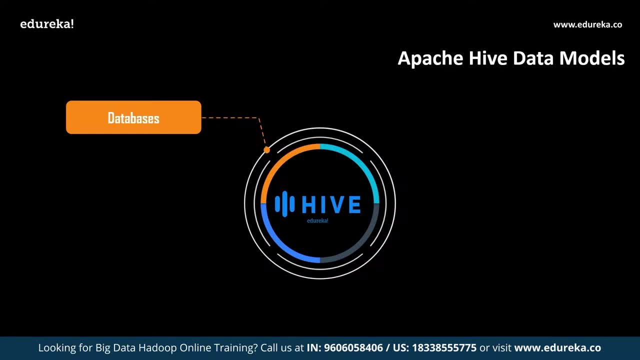 which we use in hype, that we basically create databases and store our data in the form of tables, and sometimes we also need partitions. We will discuss each one of these data models in our demo ahead. So we'll first create databases and inside databases We will be creating tables inside. 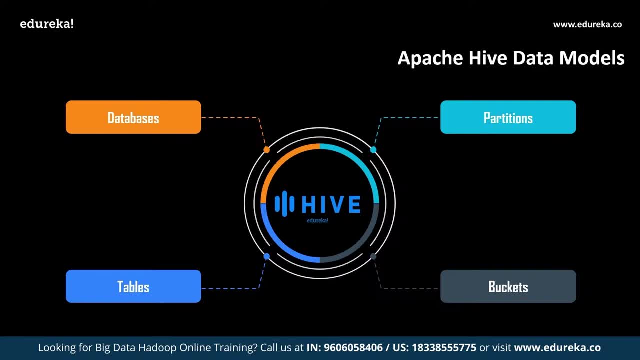 which we will be storing data in the form of rows and columns and along with that partitions, partitions, They are like advanced way of storing data, Like if you have just imagine you are in a school, say standard one, and inside standard one you have sections ABCD. 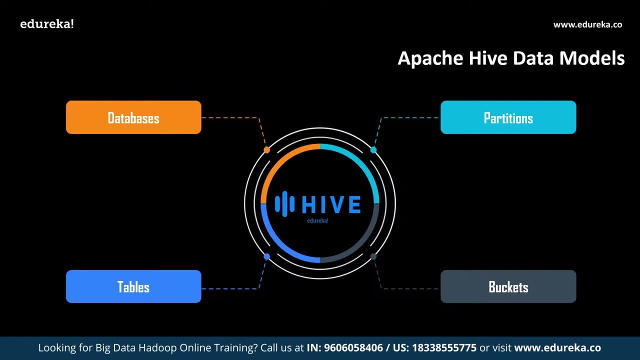 So partition is like you're getting partitions for section a, section B, section C and section D. You're storing different different students in different different sections so that when you're querying for a particular data, for example, say, you're searching for a kid called Sam- 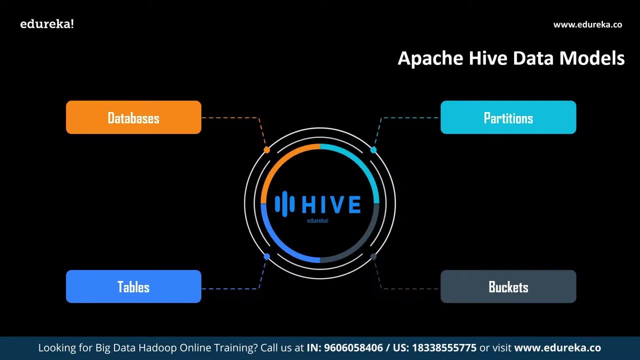 and you have the section of his class SB. So you just don't have to just search for some in all the four sections. You can just directly go into section B and call in Sam and you'll get access to him. That's how partitions work, followed by partitions. 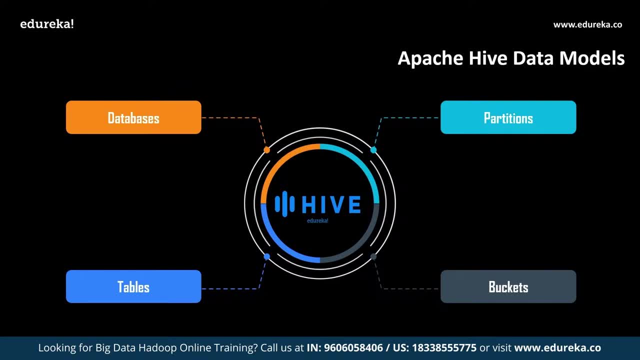 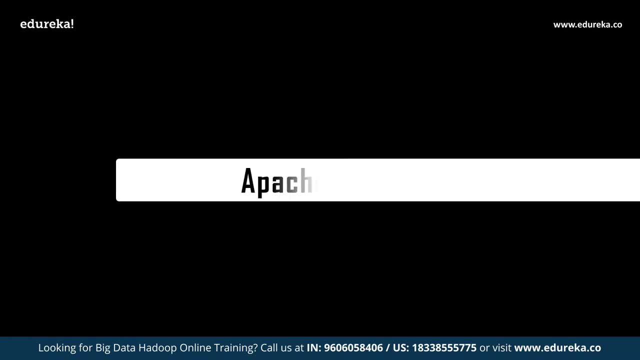 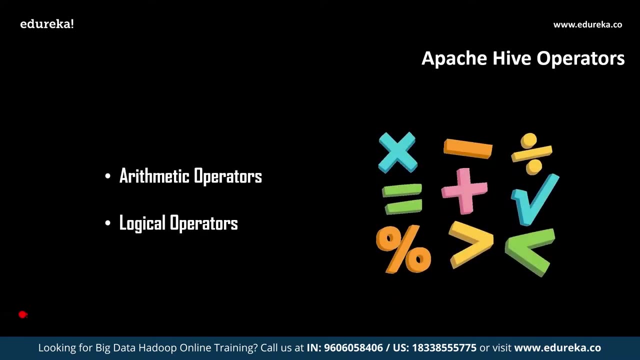 We have buckets, so similar to partitions. even buckets work in the same way. Let's understand each one of these in much better way through a practical demo. after data models, we shall understand about high operators. So what are operators? operators are any other operators that we use in normal programming languages. 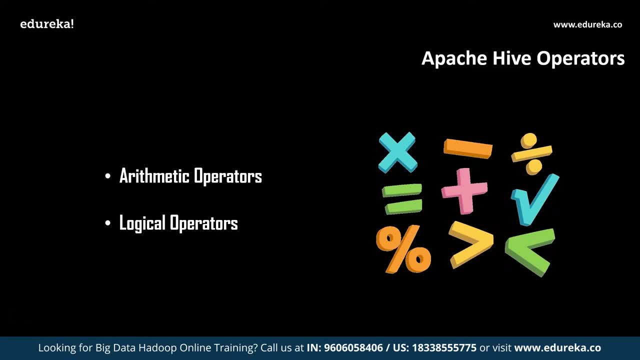 such as arithmetic operators, logical operators, which will also go through some examples based on a thematic and logical operators in Hive. in the Hive demo We will use some automatic operations as well as logical operations on the data which we have stored in the form of tables in Hive. 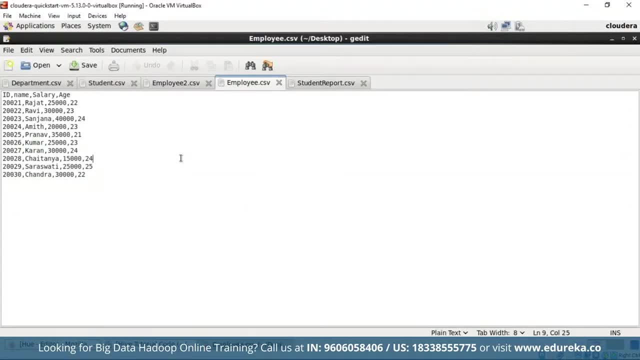 We shall go through a brief look on that as well. So before we get started, let's have a brief look on the CSV files that I have created for today's demo. These are the small CSV files that I've personally created using MS Excel. 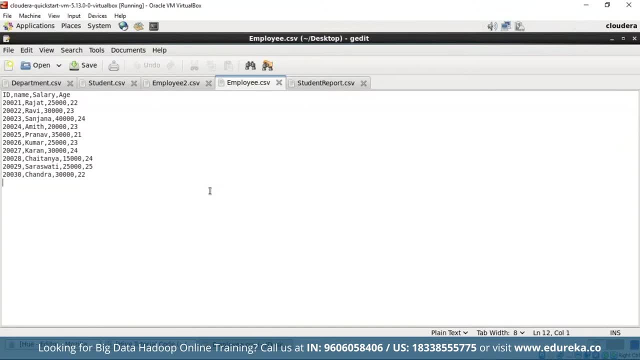 and I've saved them as dot CSV files. I've made the CSV files to be smaller because just to make sure the execution time consumed is as less as possible. since we're using cloud error, The execution time might be a little more, so it's better views: smaller CSV files. 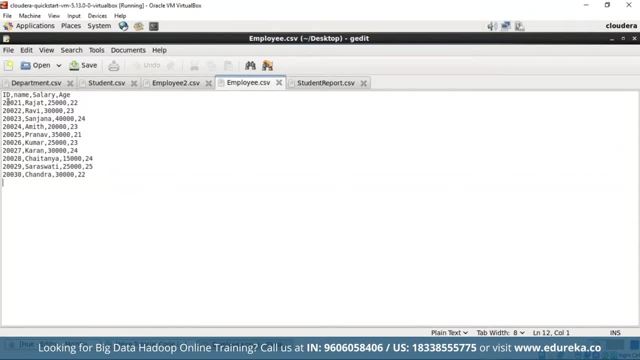 So this is my first CSV file, which is employee dot CSV, which has employee IDs, employee name, salary and age. Similarly, We have another employee to dot CSV file which has the same details, along with one more column, that is, the country column. 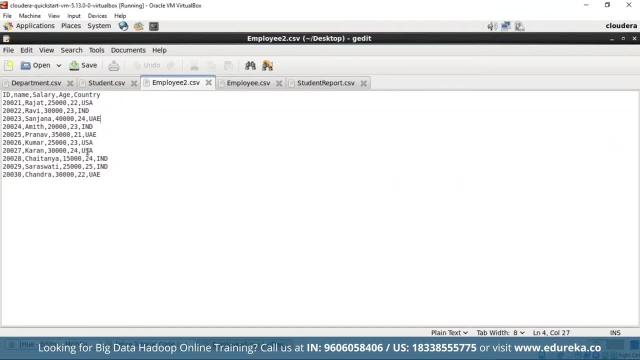 I've included country because we will be using this country column and joints that we will be performing in future. Followed by that, We have the department, So here we have department ID and department name. So we have development department, testing, product relationship, admin and ID support. 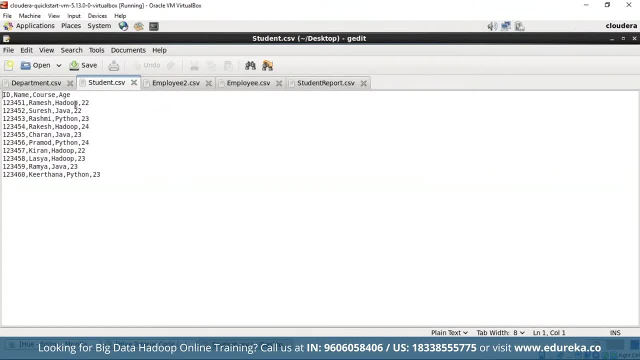 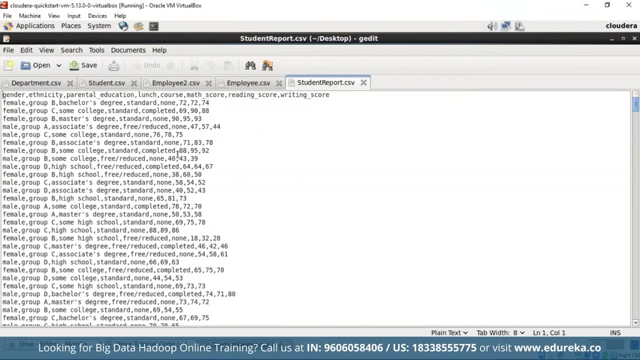 Similarly, We also have student CSV. This is another CSV file that I have created. This has ID, name, course and age of the student. followed by that We have another CSV- This is student report dot CSV, which has the reports of a particular student: gender authenticity. 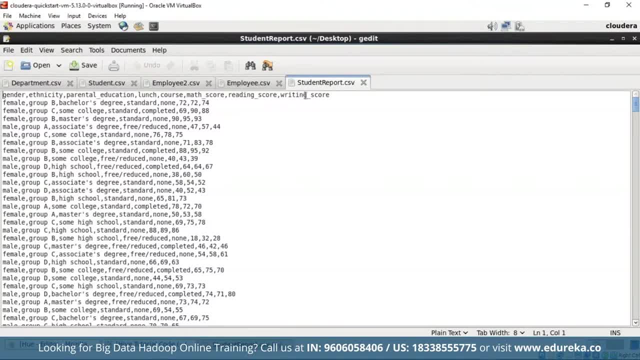 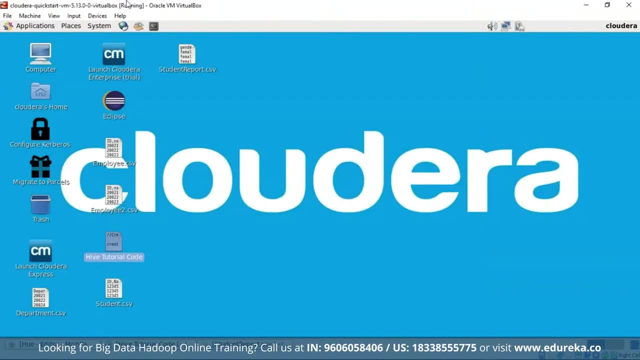 parental education, lunch course math Score, reading score, writing score and other. So these are the CSV files that we will be using in our demo today. So now let's quickly begin with our demo. So to start high, we shall open a terminal. So starting or firing up hive in cloud arise really simple. 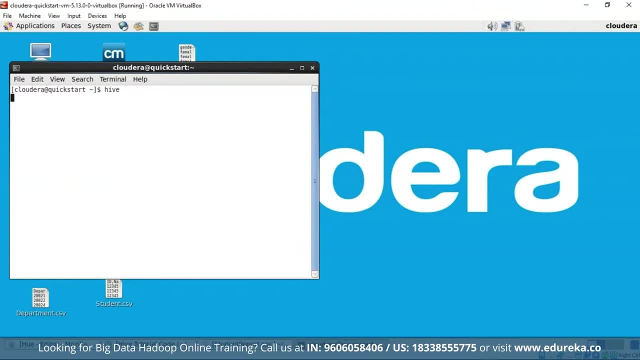 You just have to type in hive and enter. There you go, Logging initialized using configuration files and Etc. The hive CLI is deprecated and migration to be line is recommended. and there you go, your hive terminal. Our CLI has been started. So first let's try to create a database to save time. 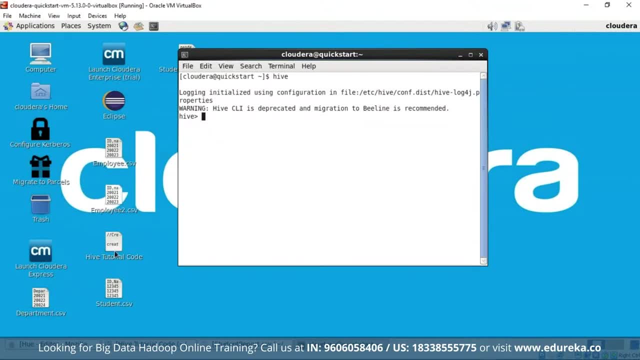 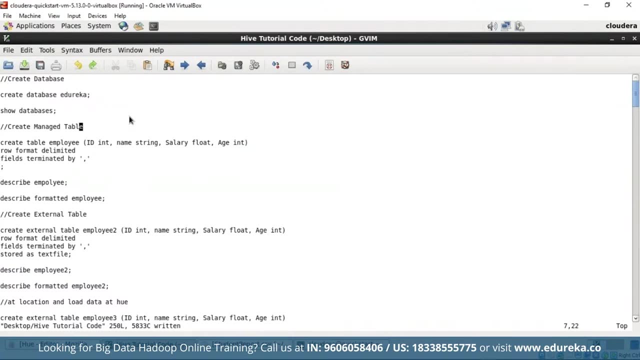 I've already created the document which has all the course that we will be executing today. So this is the particular file which I will be using today. So, don't worry, This file will be linked in the description box below. You can use the same file. 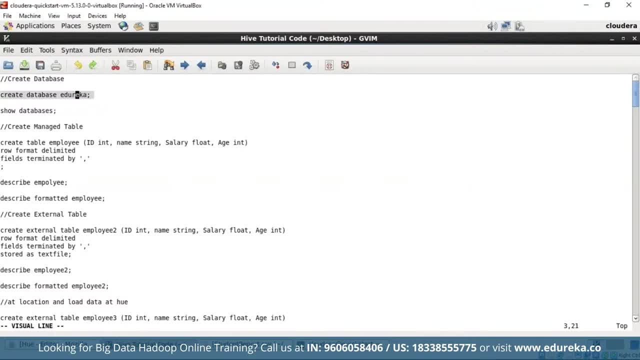 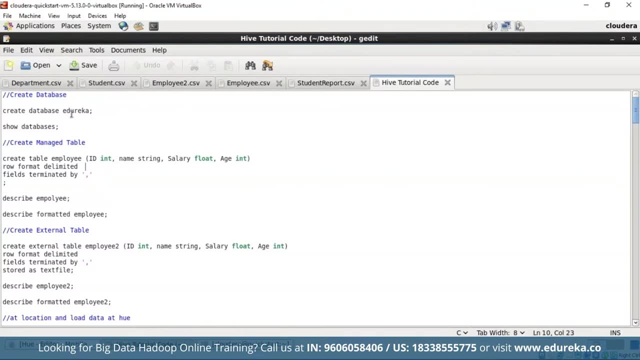 and try executing the same course in your personal systems, just for practice, if you feel so. so just to save time, I've already created the document which has the code set We are going to execute today. So this code, or this file, will be attached. 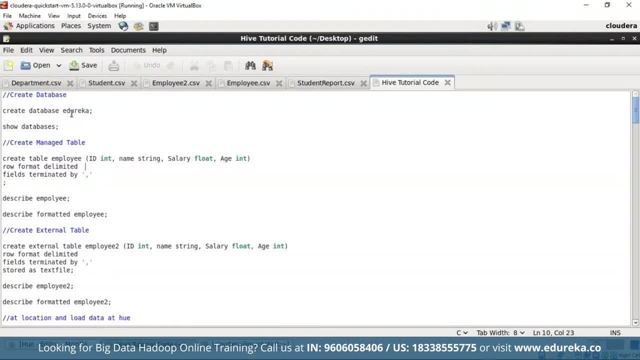 in the description box below. you can get access to it, and you can also execute the same course in your own personal system to have a practical experience about this particular hybrid or you. so the first thing that we will be doing today is to create a database. 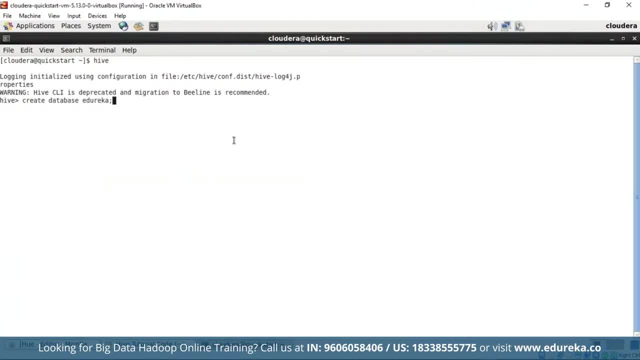 So I'm going to create the database using SQL type commands, which are: create database. name of the database, which is edureka. There you go, The database has been successfully created. So now you can also use the following command to check if your database has been created or not. 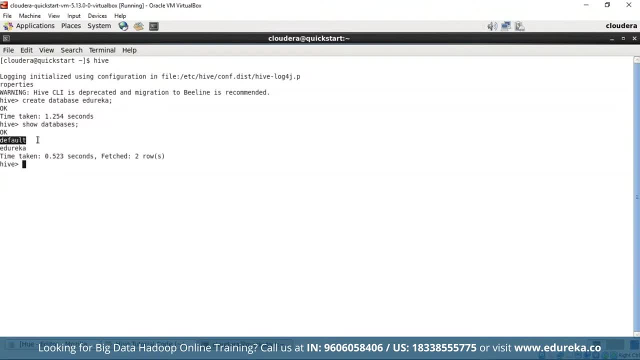 So show databases will help you to find it. So there you go. You can see the first database, which is a default database, which will be pre-existing, and followed by that You have our own database, which we have created now, that is edureka. 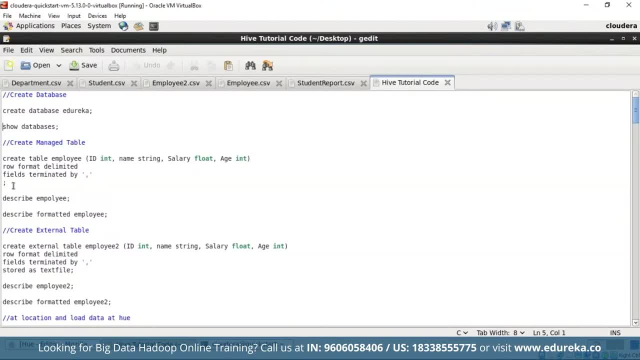 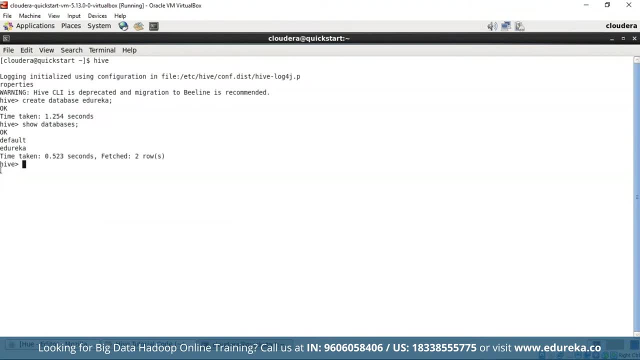 So, followed by this, next, we will move ahead and try to create a new table. So when you come into tables, you need to understand there are two types of tables in hive. They are managed tables or internal tables, followed by that external tables. So what is the difference between these two tables? 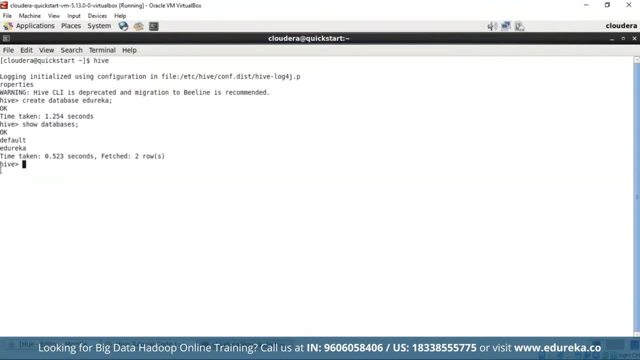 So internal table or managed table is the default table that will be created whenever you try to create a table in high. So, for example, if you're trying to create a new table, say edureka, then hive considers that particular table as an internal table by default. 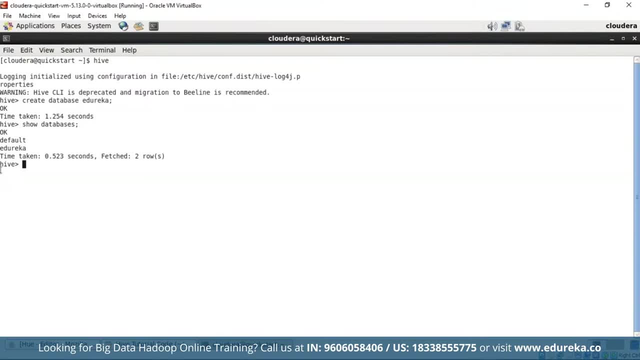 So when you create an internal table, your data is not secure. Understand this. so when you create an internal table, your data is not secure. in case, just imagine, you are working with a team and all your team members have access to your hive or hue. 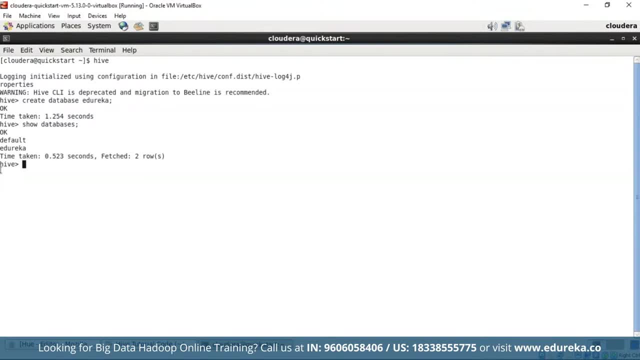 So the table has been existing in your hive and some random newbie or some random inexperienced guy tries to change few things in your table and accidentally he ends up deleting the table. So when you delete the table, then if the table was created using an internal table, 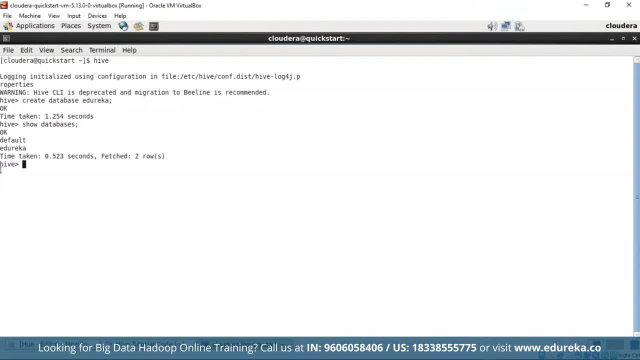 code, then your data will be erased. So that's the disadvantage of using internal tables. But in case, if you create an external table, even if somebody tries to delete your table, the table or the data, whatever is there, will be deleted from their own local system. 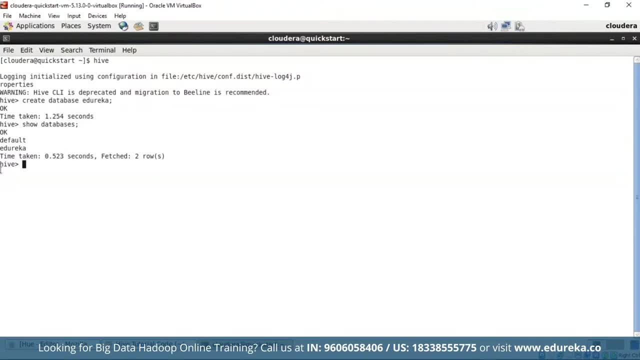 but not from high. So that's the best part of using external tables. Don't worry, We will discuss about internal tables and external tables as well. So first we'll try to create an internal table. So this particular code is based on internal tables. 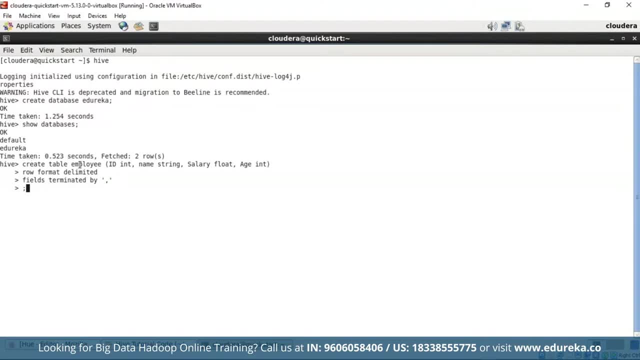 So we are using sequel type command here, which is create table and the table name is employee and the columns inside our table are ID of the employee, name of the employee, salary and age. So row format has been delimited, followed by that, since this is a CSV file. 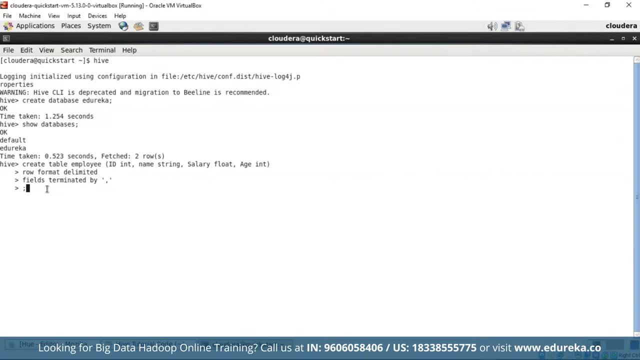 So the fields will be terminated by comma. and don't forget: you have to use semicolon. unless you use semicolon, your code is not complete. So let's fire and enter and see if the table gets created or not. Yeah, the table is created successfully now. 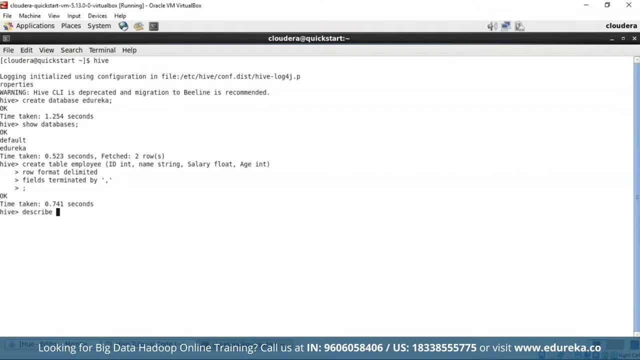 we shall see the table, or let's describe the table. So, describing the table means you can see what are the columns which are present in your table. So to describe a table you can use the keyword describe and name of the table, which is employee, and don't forget semicolon. 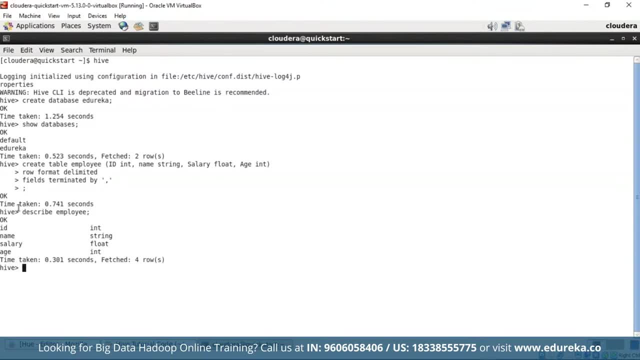 There you go. So your table has the columns ID name, salary age. So those are the four columns which you have included in your particular table: employee. Now let's move ahead and see if this particular table is an internal table or managed table or the other type of table. 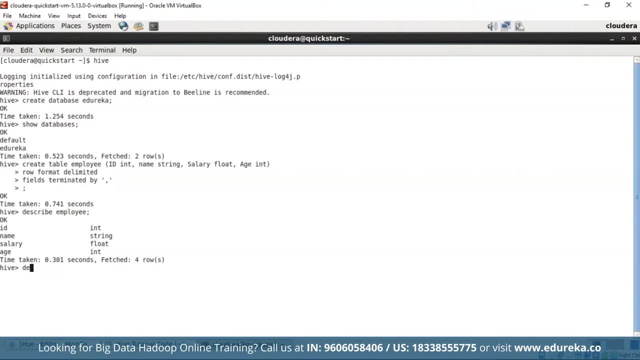 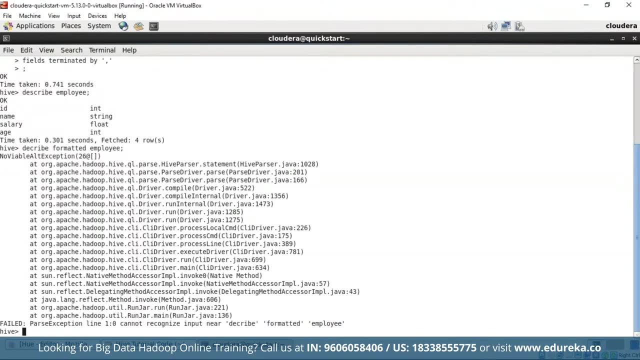 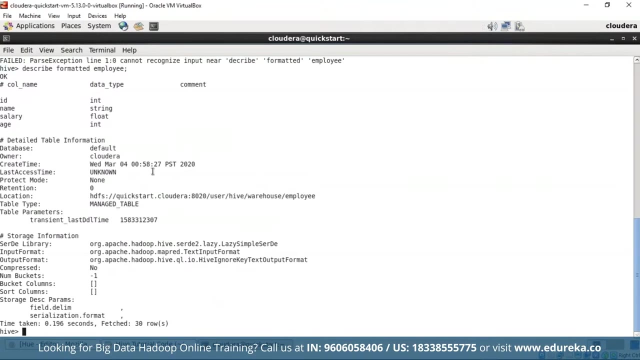 which is the external table. So to do that we can just write in describe formatted table name and semicolon. They might be a small issue here. Yeah, there is a typing mistake that is described missed s. So there you go, We got it. 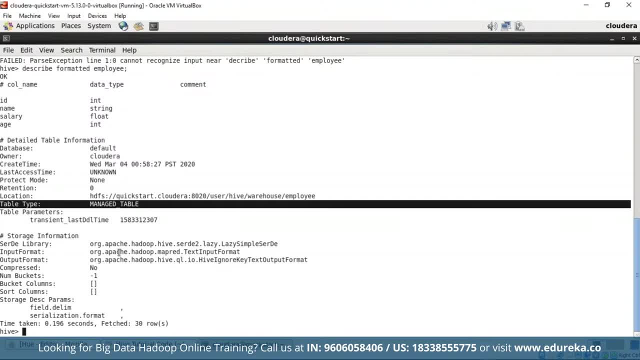 So this particular table is managed table, as you can see here. Now let's move ahead and try out external tables. Let's clear a screen first. You can use control plus L to clear your screen. There you go. We have a clear screen now. 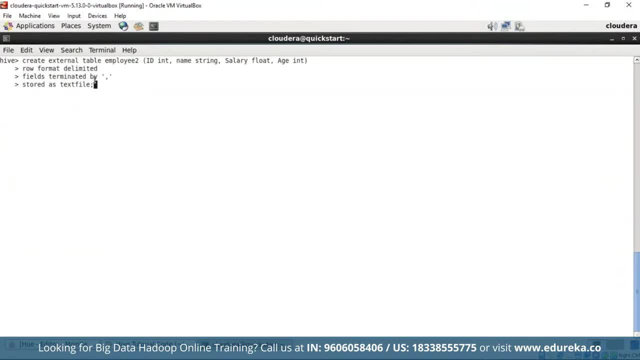 Now let's try to create an external table. creating an external table is completely similar to that of internal table, But the only difference is that you need to add in a keyword which is external. So this particular keyword is used to create an external table. 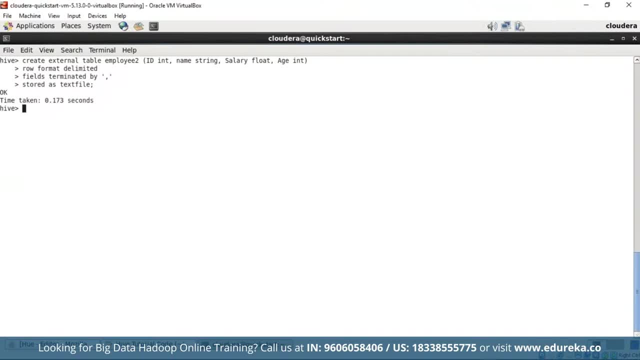 Now let's fire and enter and see if the table gets created. I'm not. you can see the table got created. Now let's try to describe the table employee. to don't forget the semicolon. I'm saying this again and again. 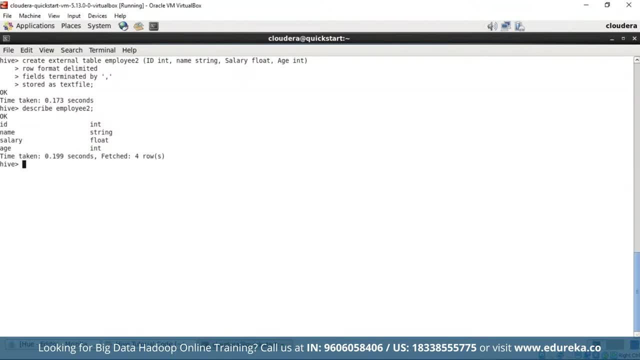 because most of the times we miss semicolon and we will get an arrow. so you can see the table got described and we have the following columns inside our table. Now let's move ahead and see if this particular table is an external table or a managed table to do. 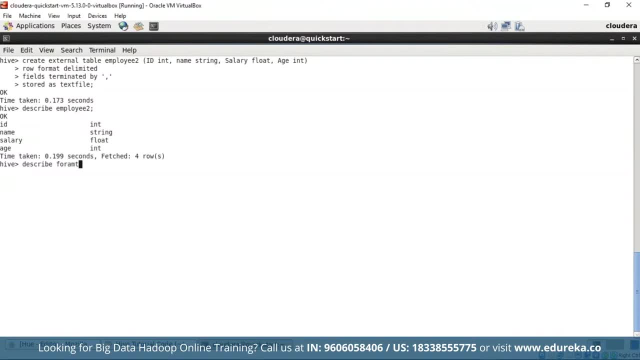 So you can type in describe: formatted the same code, What we have used earlier. that is described formatted name of the table that is employed to semicolon. Don't forget, there is some issue again. I think I've missed something or maybe a typing error. 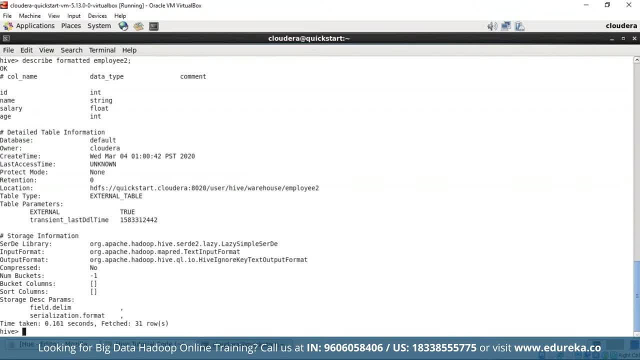 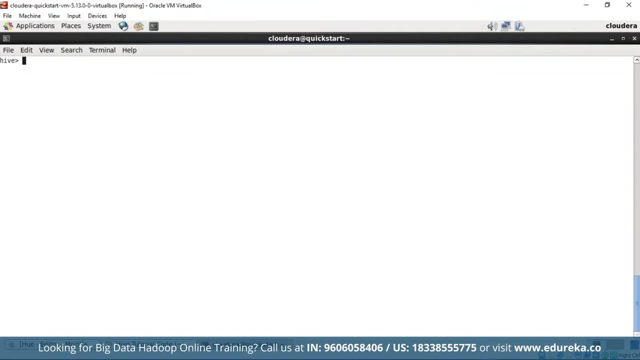 Yeah, this is a typing error. Yeah, there you go. The table type is external table. So that's how we create an internal table, or managed table and external table. So now that we have understood how to create a database, This and table and the two types of tables. 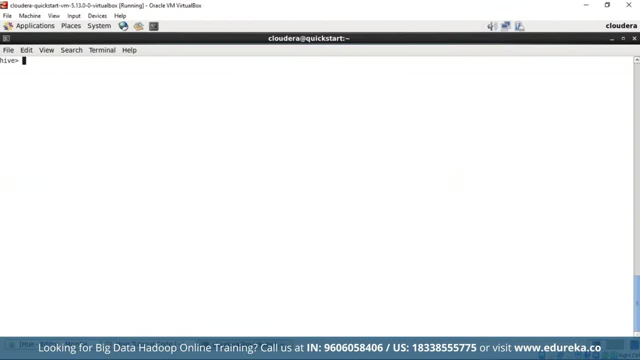 that are internal table or managed table, followed by that The second type of table, that is, the external table. Now let's try to create an external table in a particular location. So for that you can use the following code, but the only difference is you are specifying the location. 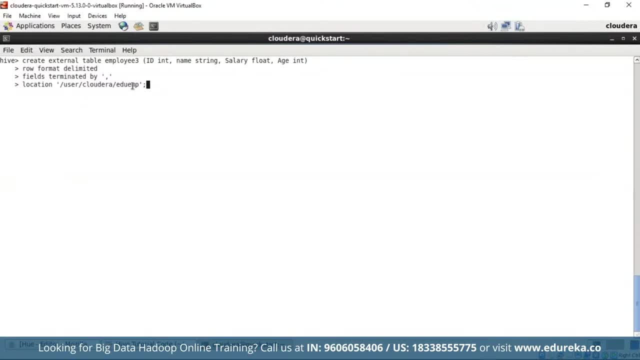 that is user Cloudera at Eureka, employee edu EMP is a file that we will be creating in our hive, So let's fire and enter and see it. that's created or not? Yeah, It's successfully created. Let's go back to Hugh. 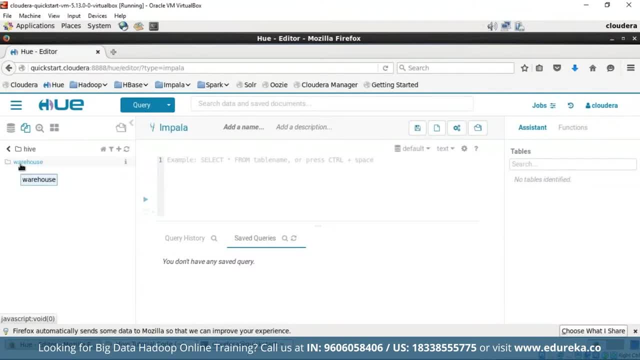 and see if the following table is created or not. So one thing you have to remember is when you fire in a commander, if you try to create a table, the first folder that will be created is a warehouse. So inside hive you have your warehouse and inside warehouse you have all the databases. 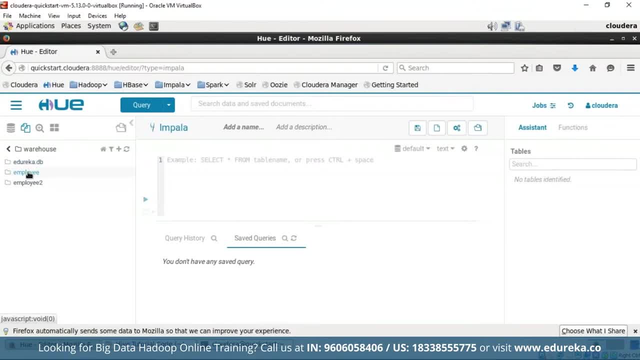 that we have created. our first database was the Eureka database, and after that we have created table which is employee, and the second table is employee too. So this is in the particular location which is user Cloudera, and the file is employed to. let's see: 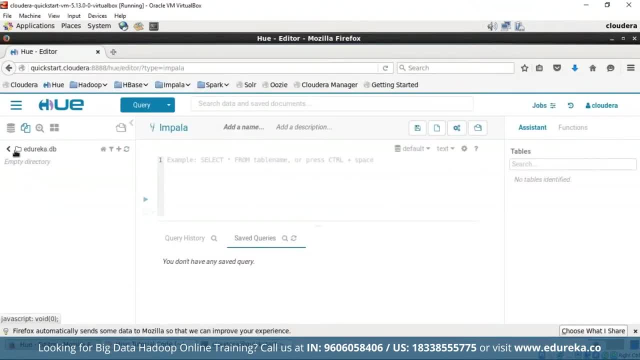 that this was the file. Yes, sometimes you will not show it because of network issues. You don't have to worry about it. You will get back that data now, followed by this: Let us enter into Hugh again. So when you come back into Hugh, if you have to upload a file, 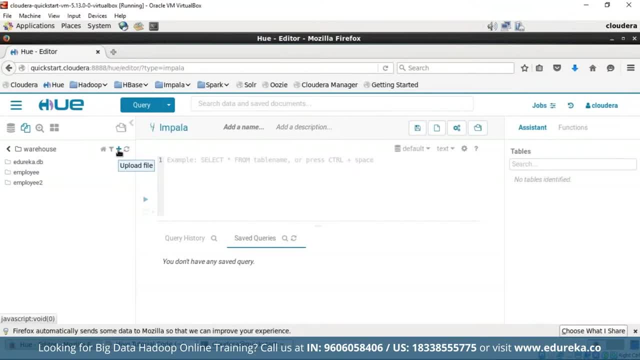 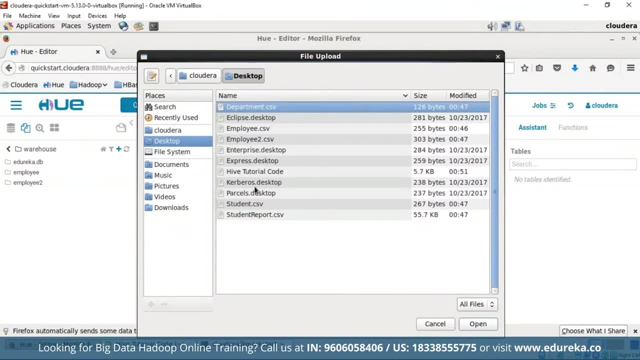 into Hugh. you can just select this particular option, which is plus so selecting This will give you a dialog box which will be something like this, and here you can just select any of the files which you want to upload into Hugh. now let me select a student report, dot. CSV, and select open. 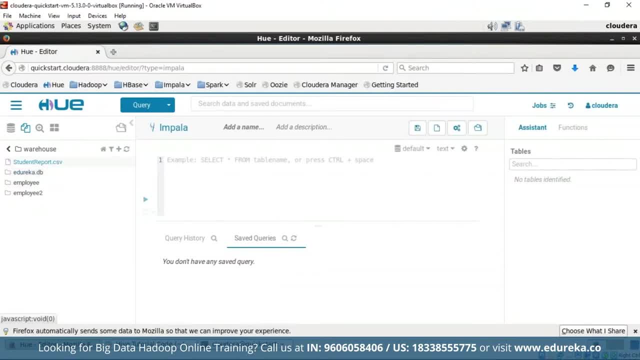 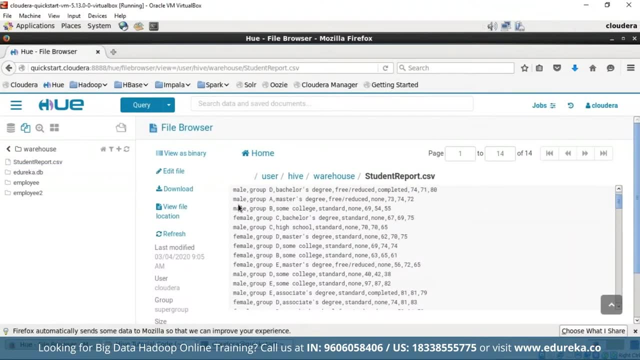 So there you go. upload is in progress. So the data file has been successfully uploaded. now, if you want to access your data file, you can just click on that. So there you go. You have all your data successfully loaded onto Hugh. You can also perform queries on this particular data. 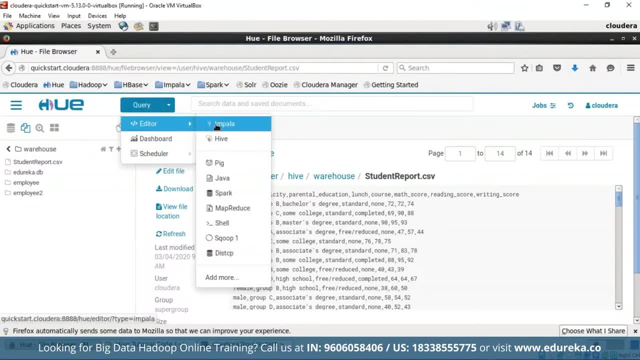 You can just select query and inside that you just need to select editor and you have various editors over here, which is big, Impala, Java, spark, MapReduce, shell, scoop, And we also have a hive in here. So if you just select hive and there you go. 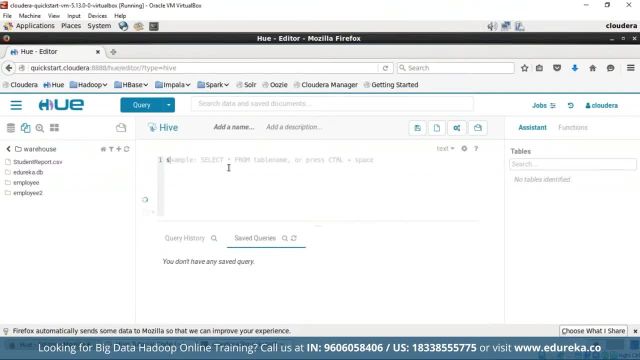 you have the editor here. You can just type in your commands or queries, whatever you have. So you have many dictionaries as well. You can just select any one of those select, and that's how you write queries on the hive terminal. Now, let's not waste much time here. 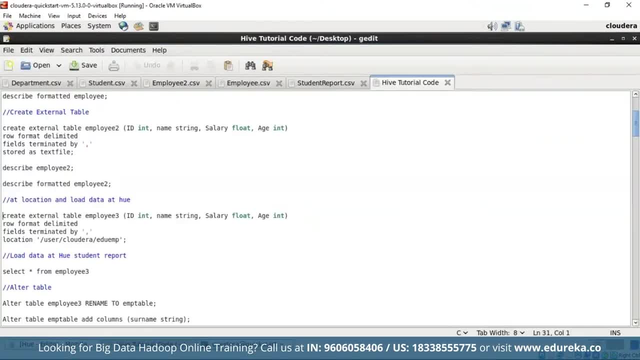 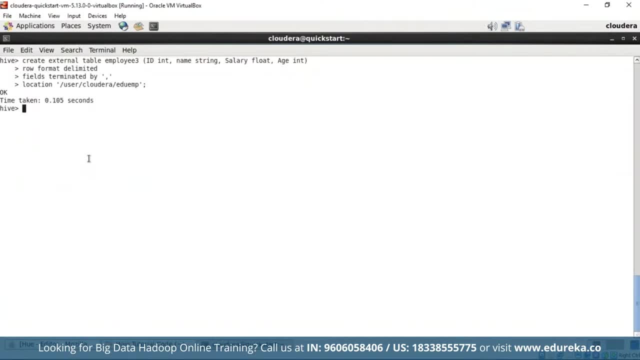 and we have a lot to learn. So let's continue with the next topics in our today's session. Now we shall try to edit the tables Now. we have created the new table, that is employee 3, and we have named the columns as ID name, string, salary age. 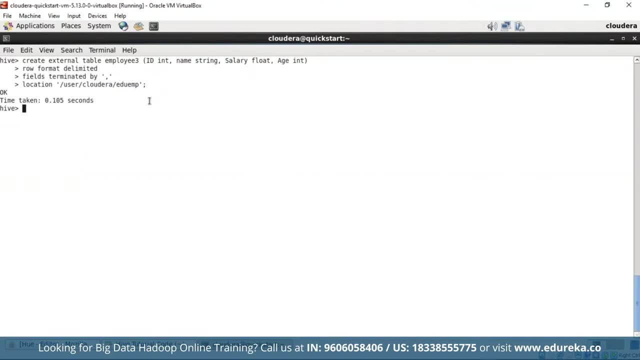 and flow. now we shall try to make some alterations to our table. So the first alteration that we will try to make to our table is to rename Our table as EMP table. you know that our employee table was named as employee 3 now. 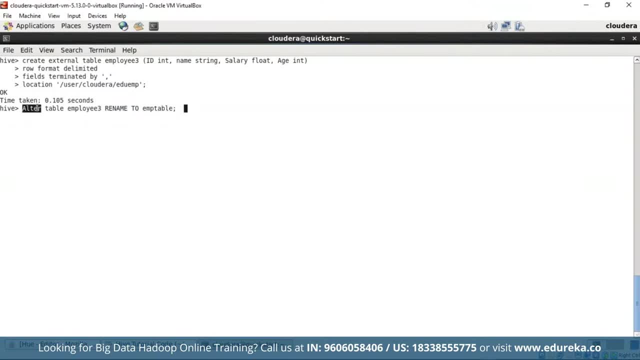 we are trying to rename it to EMP table, So we are using the keyword alter here. So just fire an enter and see if this is possible. Not not? Yeah, it is possible. The name has been changed to EMP table. Now let's try if it's completely changed. 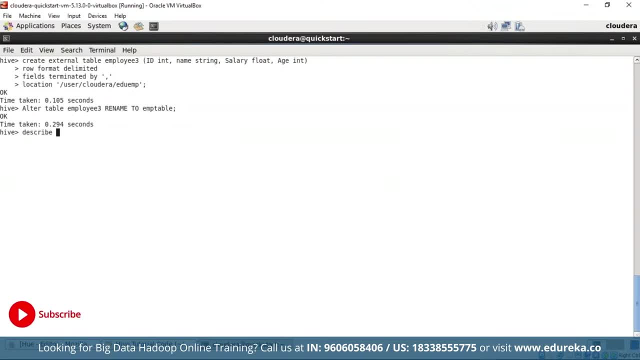 or clearly changed or not. You can just type in describe: EMP table semicolon. If we get the same table, same column names in our description, then it should be changed. So there you go. We can see the same columns here. So we have successfully changed the name to EMP table. 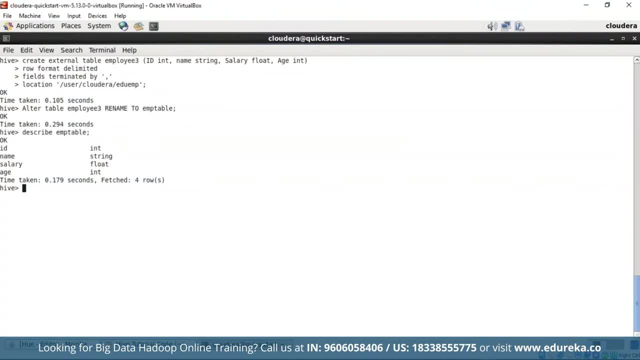 Now we shall also try to add in some more columns to our table, which is EMP table. So here we'll try to add in a new column that is the surname of string data type. So I'm doing that by using the keyword alter followed. 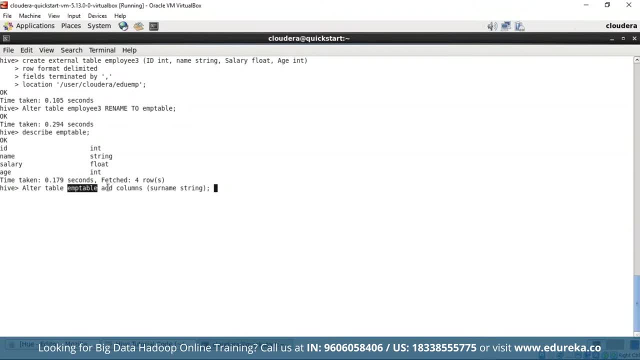 by that table. The table name is EMP And I'm using the keyword add columns and the column name is surname and the data type of that column is string. So now let's fire an enter, and there you go. We have successfully added a new row to our table. 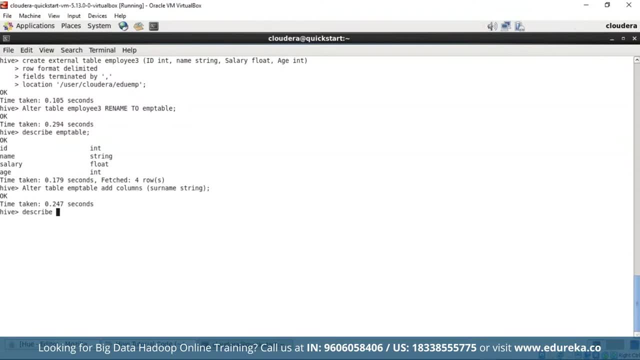 Now let's try to describe our table again and see if the column has been successfully added or not. There you go. You can see the last row, which is the surname that we have added most recently. So this is how you can alter the table. 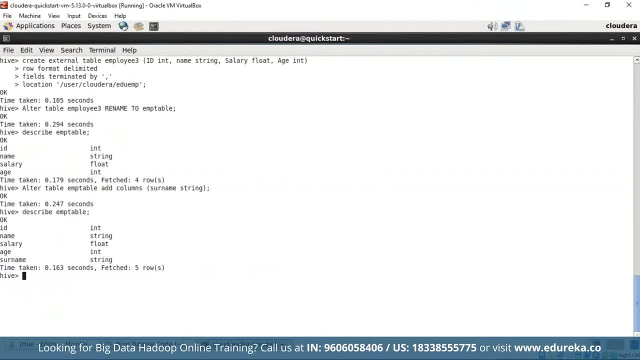 and you can also change the names of the existing columns. Let's try to do that one as well. Now, what I'm doing is I'm changing the column name to first name. So one of the column name in my table- EMP table- is the name. 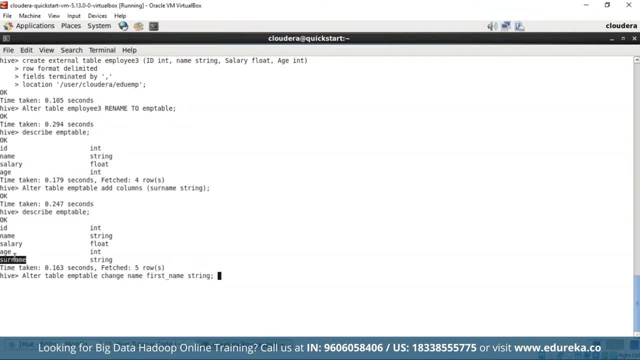 which gives me the names of the employees. So since I added surname, I'll change this column name from name to first name. So this is the command that I'm using for that operation right now. Let's fire an enter and see the result. 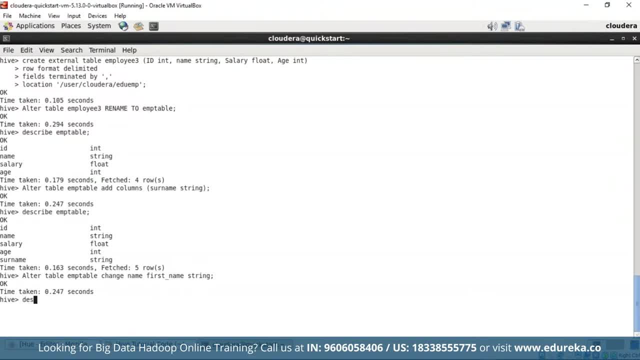 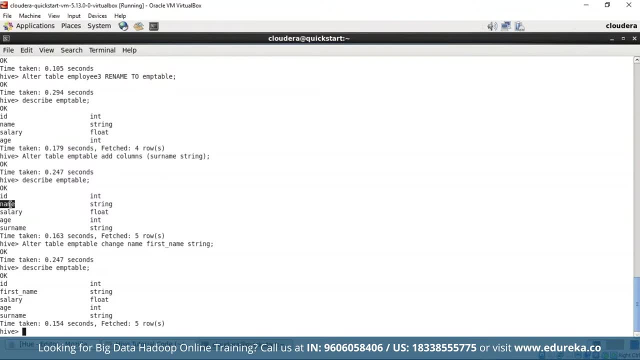 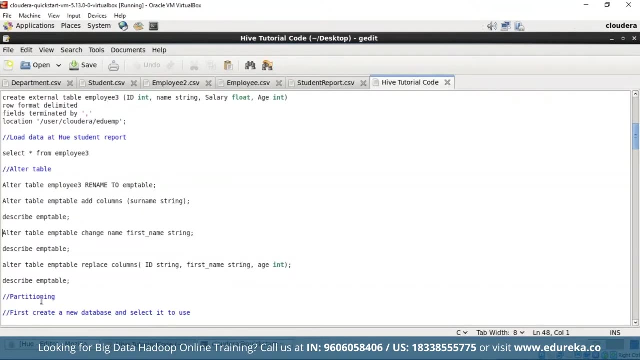 Yeah, the chain has been made. Let's describe our table. Don't forget the semicolon. There you go. You can see that earlier we had name. now It's been changed to first name and we also have a surname. Let's clear our screen. 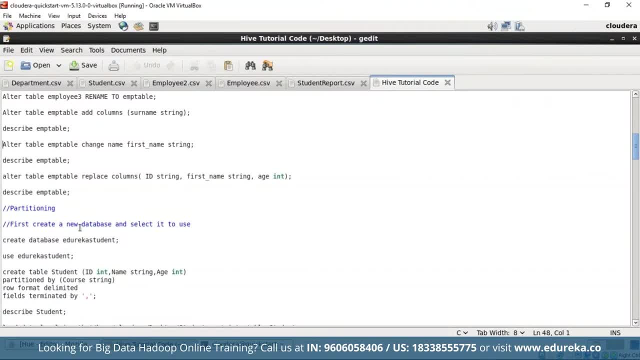 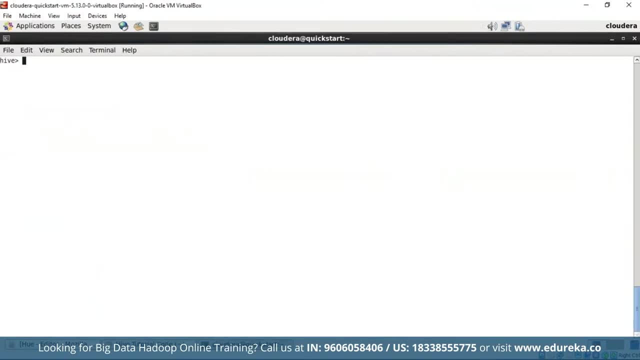 So that's all for alterations. Now we shall move ahead into our next major topic, or the data model, which is partitioning. So we have dealt with the first two data models, that are, databases and tables. So we have learned how to create a database. 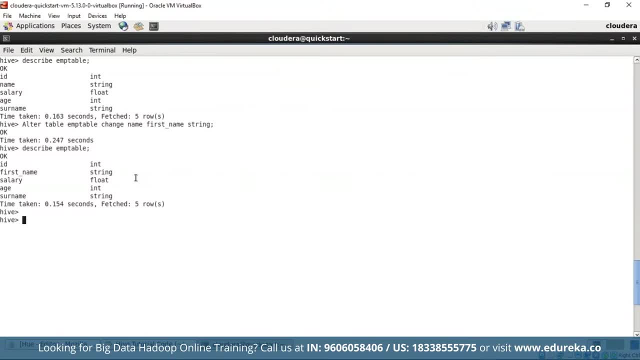 and we have learned how to create a table. We have learned how to create internal or manage table and also we have created external table. and also we have learned how to create an external table in a particular location in your hive and load data to your table. 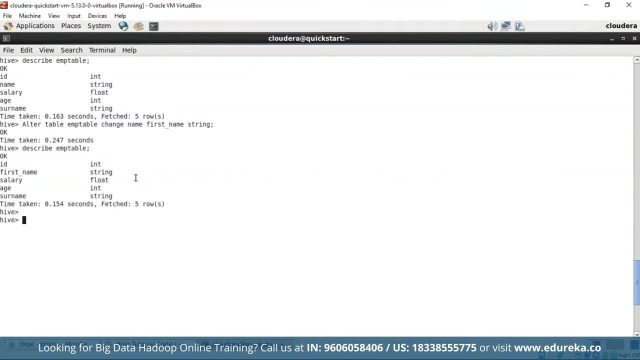 and also how to alterate your tables, the column names, the name of your table and how to add or delete new columns to your table. so far, so good, And now we shall continue with the next type of data model, that is, the partitioning. as we have discussed earlier about partitioning, 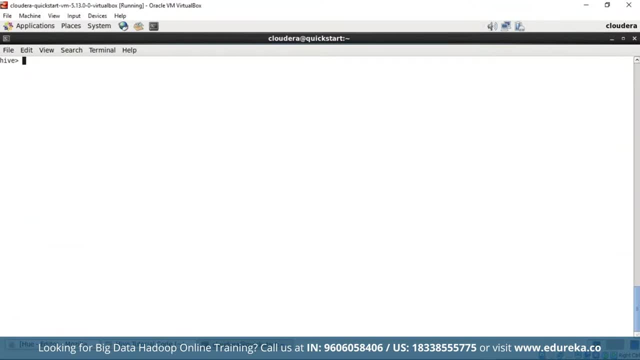 It's completely similar to a school or a college. Just imagine that you are in a college and you are in computer science section. So our college has many branches, So maybe computer science, mechanical and electronic And communications. So imagine your name is Harry. 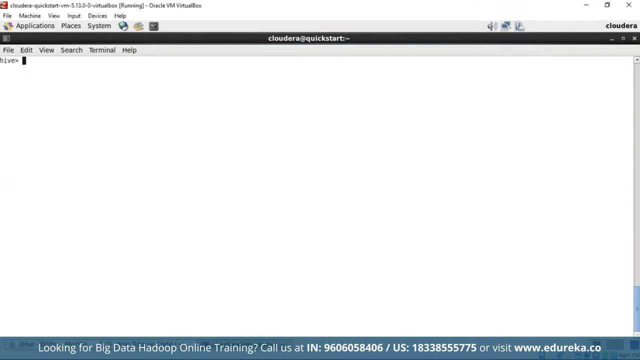 So if someone comes to your college and if he is looking for Harry- so there are many Harris in your school- So if the person is asking specifically about you, that is Harry from computer science, then can you imagine how simple is this query. So you don't have to search for electronics and mechanical. 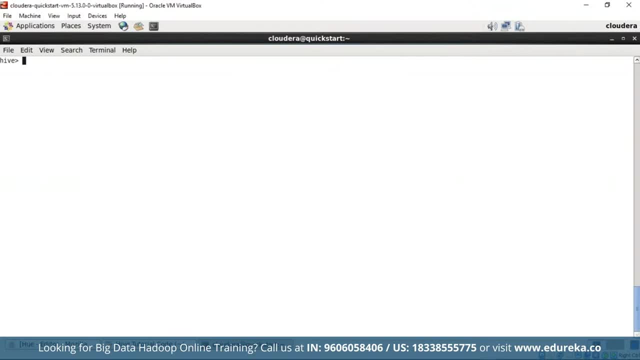 You just have to come into the class computer science and search for Harry, and there you go, your present. So that's how partitions work: To execute commands or to execute queries on partition. we will create a whole new database here. Let's start everything from fresh. 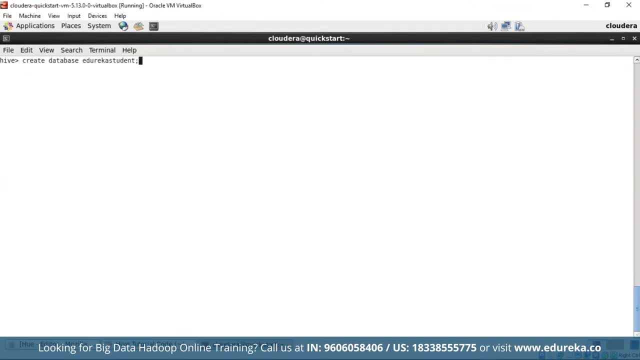 So we'll create a separate database for executing our new data model. that is partitioning, So I'm creating a new database that is at Eureka student. So there you go. The database has been successfully created, followed by that, Let's use this database. now to use the database. 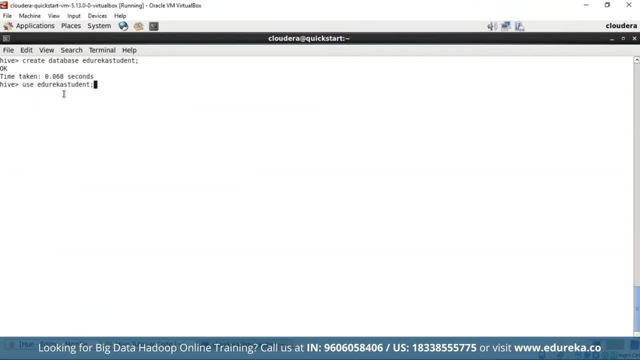 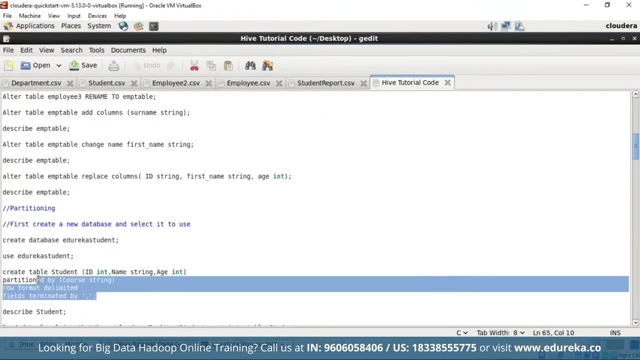 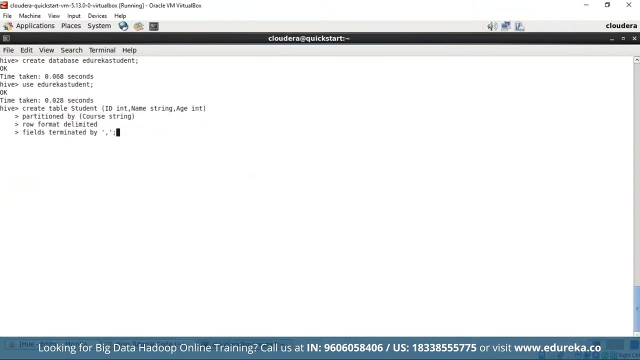 You just need to add in the keyword use and name of the database. So let's fire and enter. and now we are currently using a direct, a student database. Now let's create a table in a direct- a student database. So here I'm creating a normal table that has the managed table. 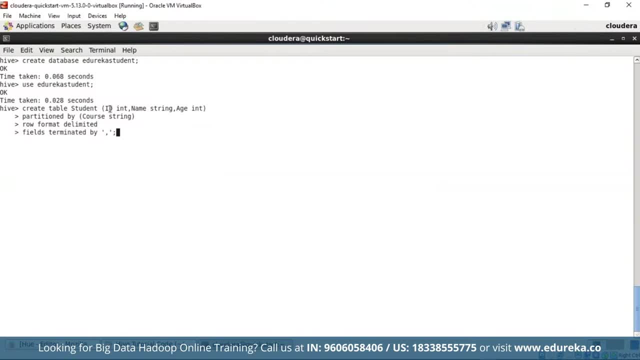 So inside my student table I'll be having some basic columns such as ID number of the student, name of the student, What is his age and course. So you're not finding course here because I'm going to partition the table Based on course. 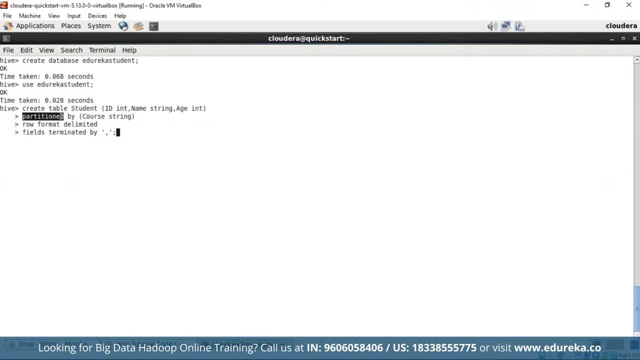 So here you can find the course. I'm using the keyword partition, and on what terms? so, on the terms of course, I'm going to partition students. So we have discussed about our students. CSV file right? So here we have a CSV file. 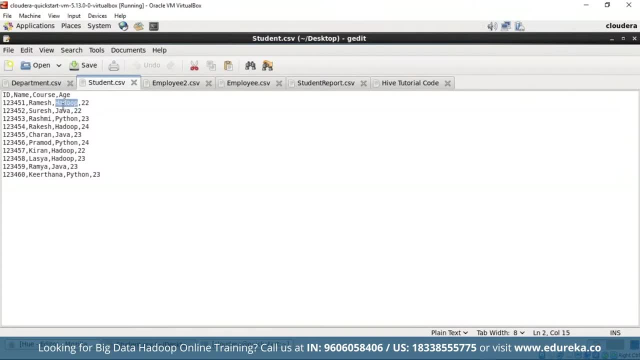 and the courses that this particular Institute is offering: our Hadoop, Java, python And yeah. so these are the courses that this particular Institute is offering. So I'm going to category Is, or I'm going to partition these students based on their courses. 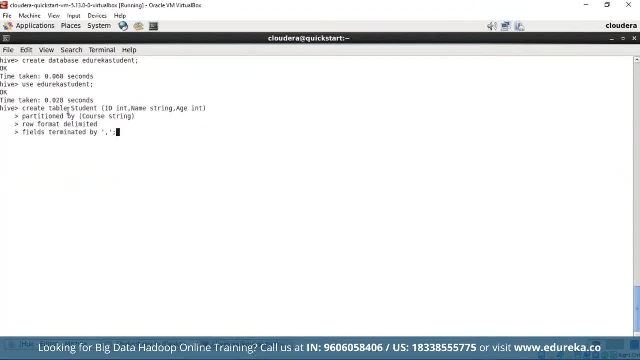 So this is how I'll be partitioning them, using this following code. So, basically, the table has all the columns and I'm going to partition the table using course. So let's find an enter and see the execution of this particular code. The partition has been done. 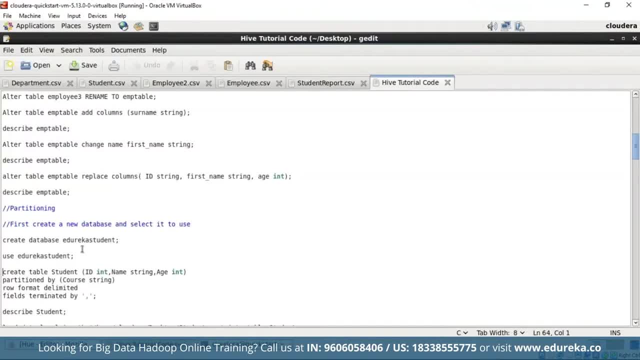 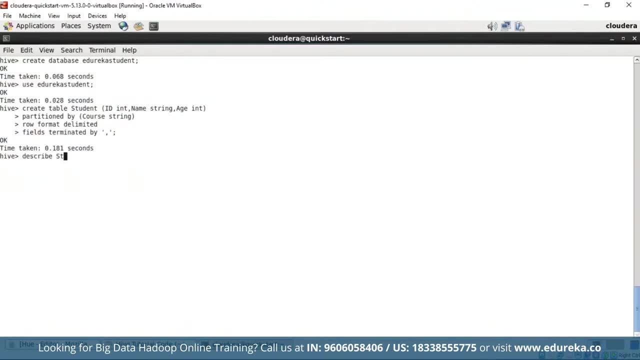 Now all we have to do is try to load in our data. Before that, let's try to describe it. Let's try to see what are the columns present in our particular table: student. So, as you can see, the course column is present. 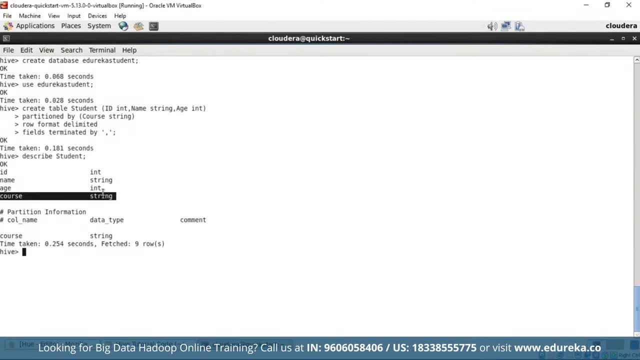 Don't worry, the code looks that we have missed out course, but we did not miss the course column. It is present in the table. The only thing is that we have just partitioned it based on the course that we are going to offer now. 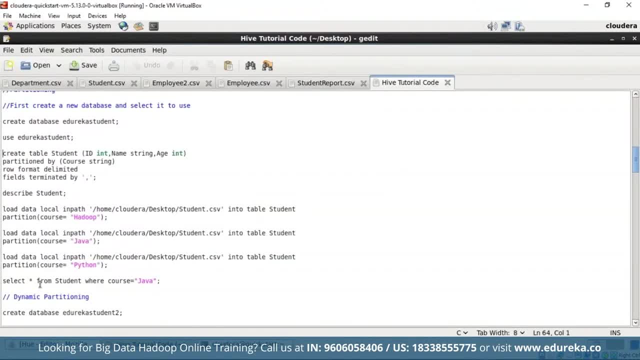 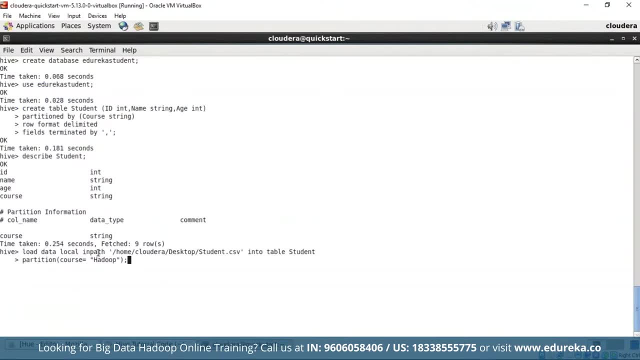 let's try to categorize the students based on their course. So you can do that by using the following code: We are going to load the data using the command load data local in path. So this particular folder, that is, the student dot CSV, is in my local location. 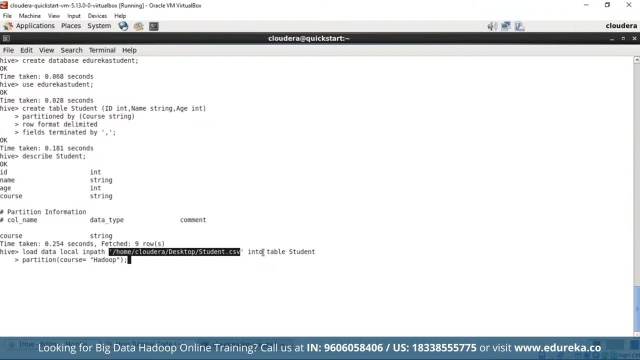 So that is a home cloud or a desktop student dot CSV and I'm loading the data present in this particular location into the student which is present in Hive right now. So I'm going to partition the student based on their course. I do now. 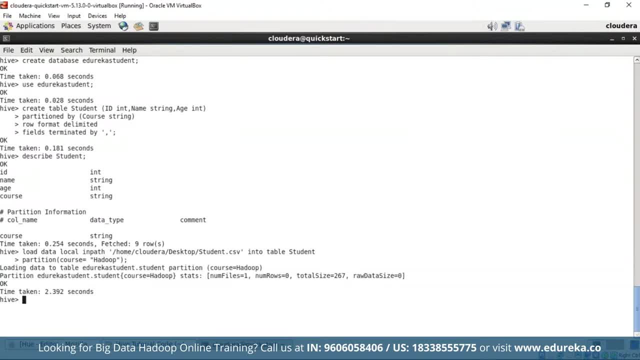 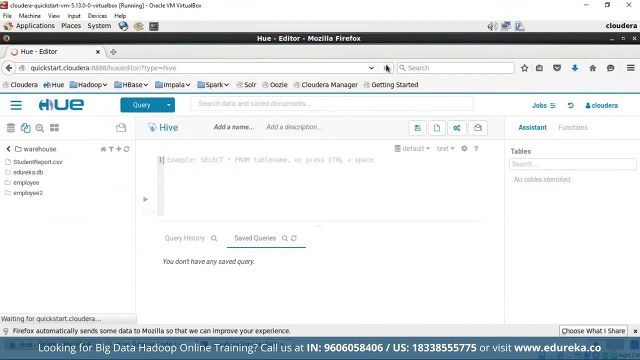 Let's fire in this command and see the output. Yeah, Now you can see some MapReduce jobs taking place. Yeah, the data has been successfully loaded. Let's now refresh our I've. you can refresh your Hive or hue based on two methods. 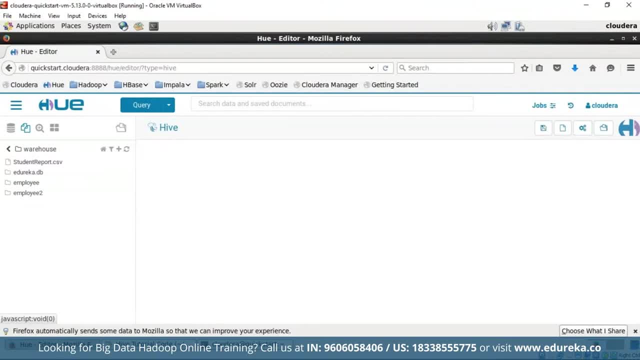 The first one is just clicking refresh button on the URL, or you can also select a manual refresh. This is the manual refresh and there you go. It's done. You can see the new database, that is, the at Eureka student database that we have right now created and inside. 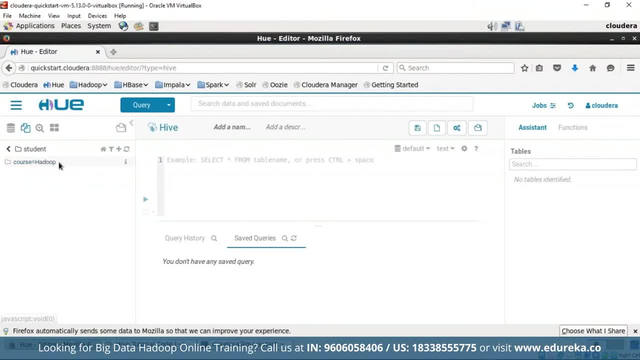 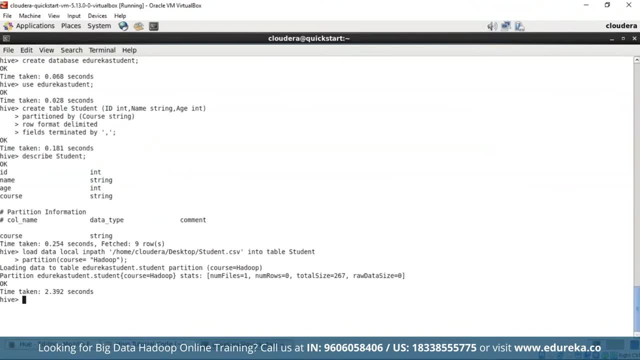 that you can see the student table that we have created. And there you go. We have the file of students Based on course Hadoop. now we will try to add in few more students based on the course Java. for that, All you need to do is just replace the course name. 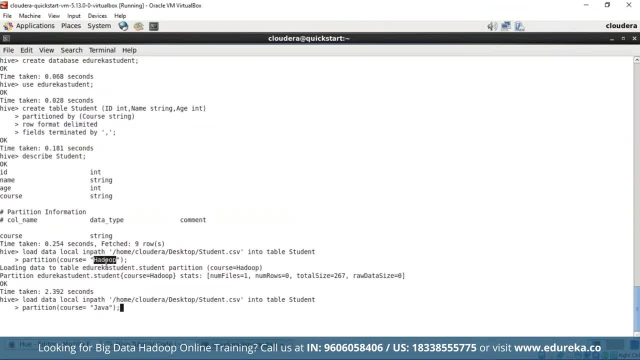 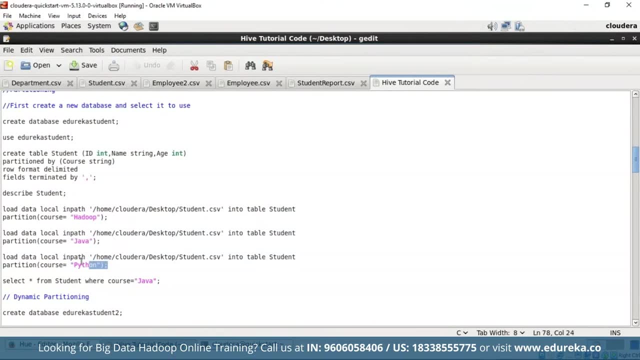 with Java. There you go. here We had Hadoop course, and now here we have Java course. just fire and enter and you can see the output, followed by that. We also had another course, that is python, So let's also execute a code for that. 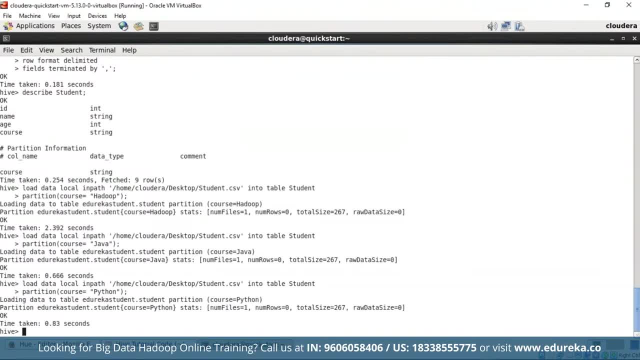 There you go, python. So now we have uploaded student Details into our hive and we have also partitioned the using one of our data model status partition into three categories that are based on Hadoop, Java and python. Now let's go back to our hue. 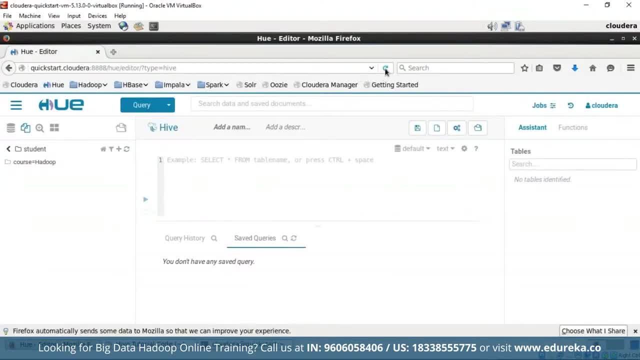 and see if the three categories are done or not. Yeah, we need to refresh that. There you go. You have successfully refreshed. still There is no sign of Java and python. Maybe a manual refresh could help? Yeah, the manual refresh has resulted in. 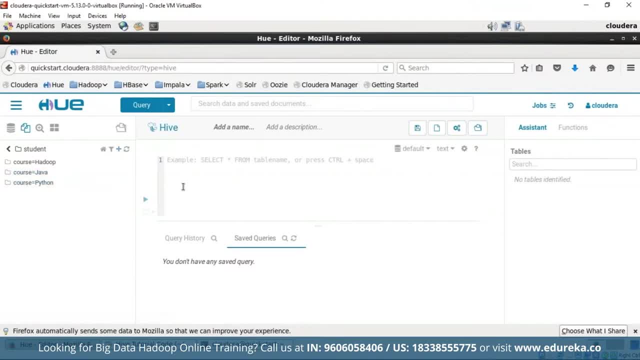 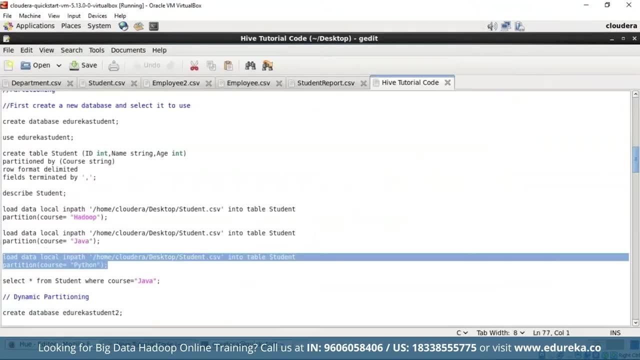 the two new files, which are Java and python. So you have all the three partitions here: Hadoop, Java and python. just enter them and you can see the student details. And now that we have understood partitioning- sorry that I forgot to mention we have two types. 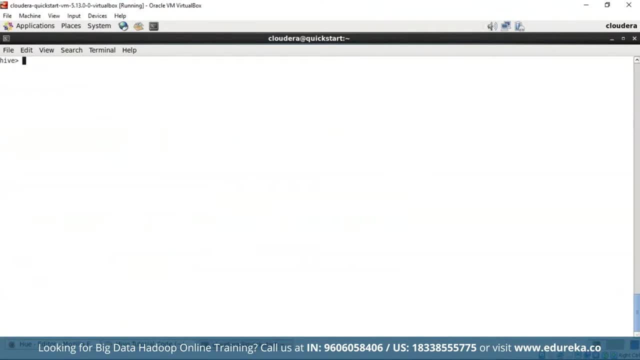 of partitioning, which are dynamic partitioning and static partitioning. So the static partitioning is in static or manual partitioning. It is required to pass the values of partition columns manually by loading the data into the table. Hence the data file does not contain partition columns. 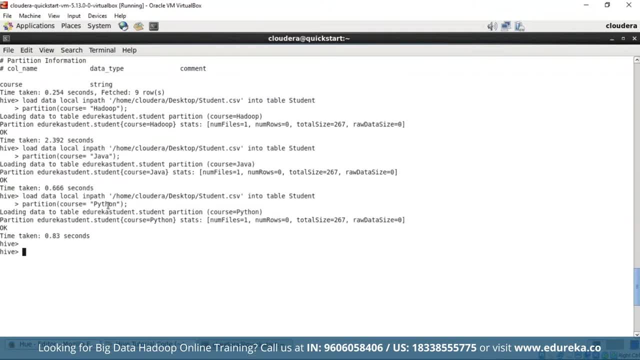 You can see that we have sent the partition columns manually for python, Java and Hadoop, But when it comes to dynamic partitioning, you just need to do it once and all the three files will be automatically configured and the files will be created. snow. 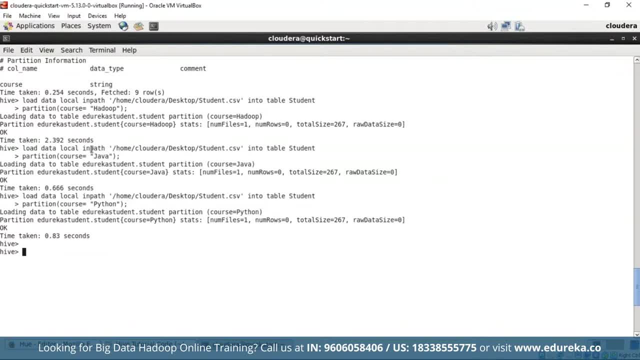 What is dynamic partitioning? So, dynamic partitioning: the values of partition columns exist within the table, So it is not required to pass the values of partition columns manually. Now, what is this? No worry, We shall execute the code based on dynamic partitioning. 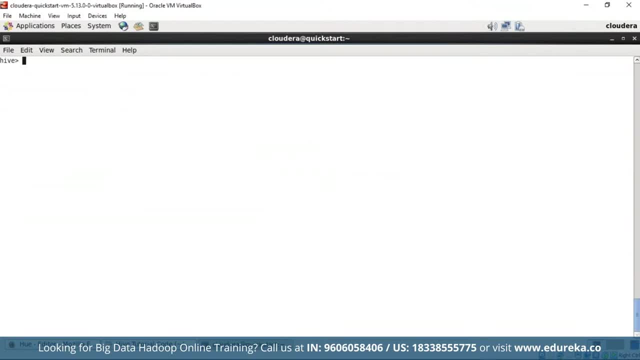 and we shall understand this in a much better way. Now let's clear our screen. Now let's start fresh again. Let's try to create a new database for dynamic partitioning and let's start again fresh. So here we'll be, creating a new database. 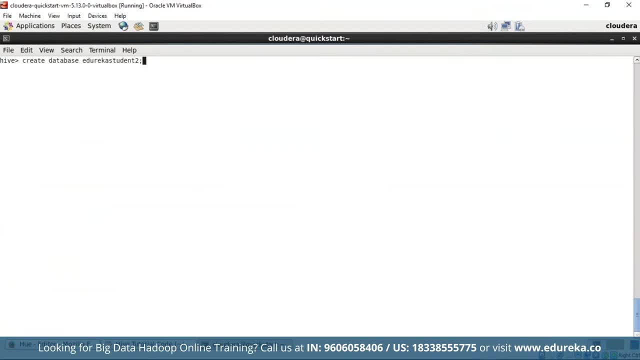 that has a duracast, who didn't do so earlier. We created a duracast student and now we'll be testing our dynamic partitioning on a new database that is edureka, student 2.. So there you go: The database has been successfully created. 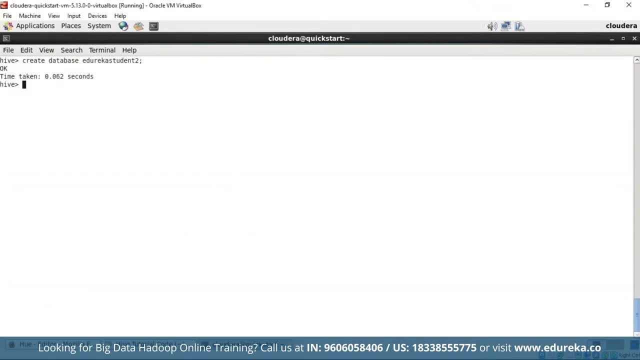 Now we shall use this particular database. currently- I'll be fair- in edureka: student to one database. Now we'll enter into student to database, So we'll use it now. Now we are in edureka: student to now. before we start. 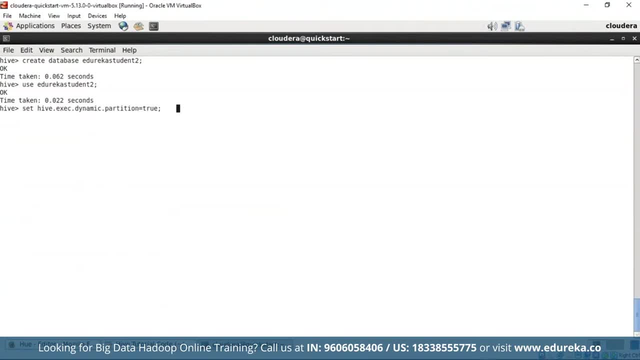 up with dynamic partitioning, We have to set high execution to dynamic partition is equals to true because by default the partitions that will be taking place in Hype will be static, So we need to convert that into dynamic partition by specifying this particular code. 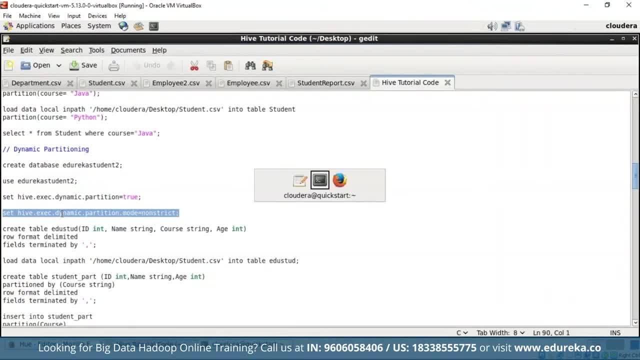 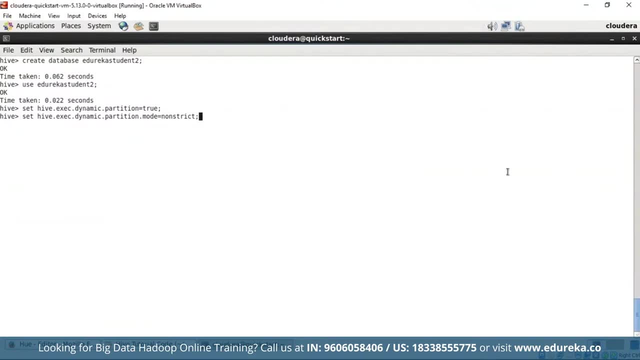 Now we are good to go with dynamic partitioning. along with that, We need to execute another command which says partition mode would be non-strict. So by default, when you are partitioning using the static partition, the partition mode will be strict. So now you're specifying it to be non-strict. 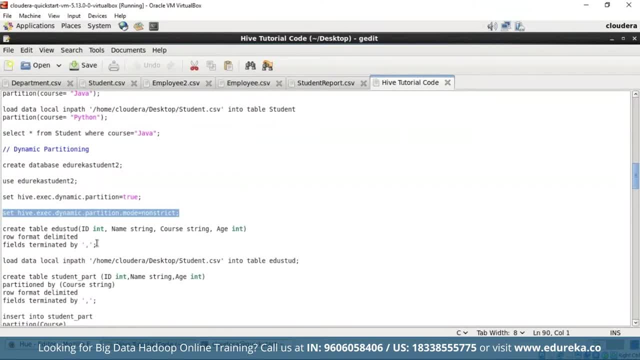 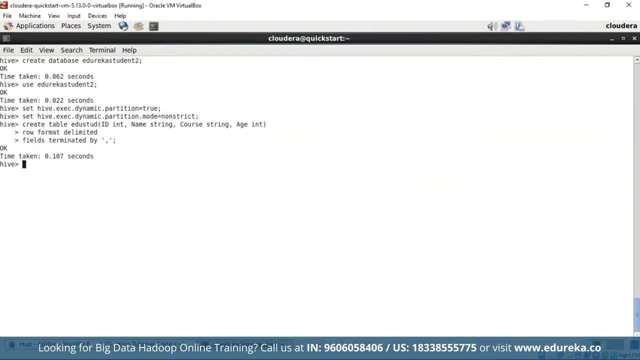 now let's execute this. So there you go. We have executed the two required codes for that. Now let's create a new table. So the name of the table will be edureka student, that is, edustud, and this will have the same columns. 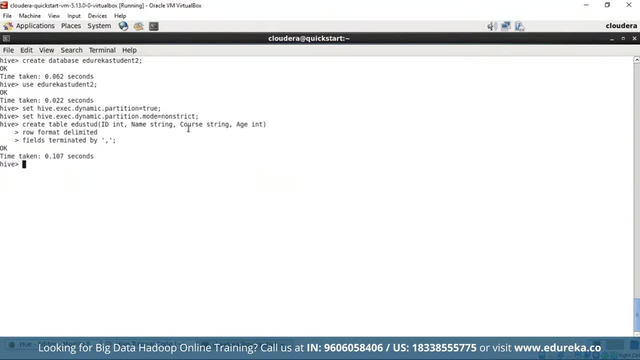 which are the ID of the student, name of the student course, age, Etc. Now we will try to load in the data from our local part- that is, home cloud or desktop- student dot CSV into the table edu. So the data has been successfully loaded. 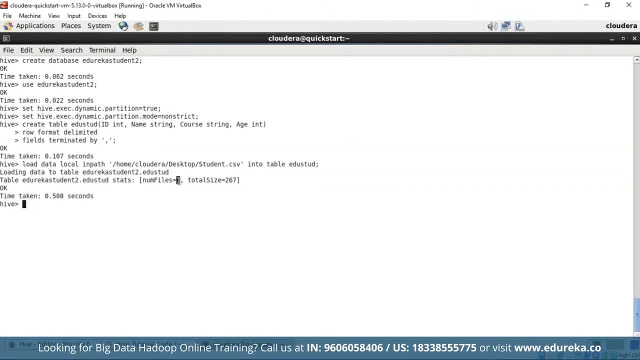 and the size is 267 KB. number of files as one. Now comes the tough part. So here we are going to partition. So we will be partitioning the table based on the same thing, which is the course, and we will be separating the data using the comma. 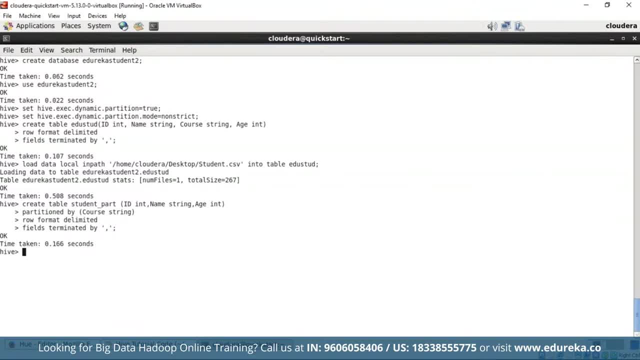 Now let's fire an enter. Now the table has been separated based on course, and now we will be Loading the data to this particular table, which is the student part. So this particular table that we have created based on dynamic partitioning. 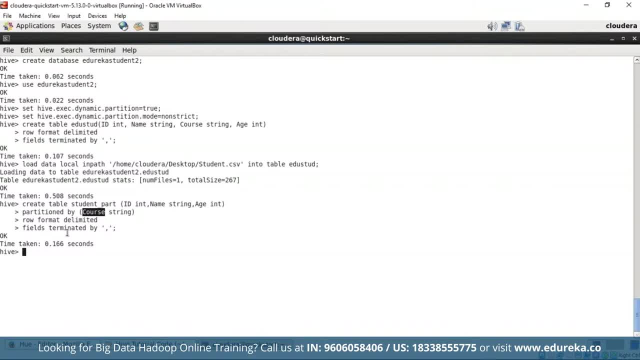 and we are going to partition the data based on course. now it's been created, So the student part table has been successfully created. Now the only part remaining is to load the data to this particular table. Now we will be writing a code. 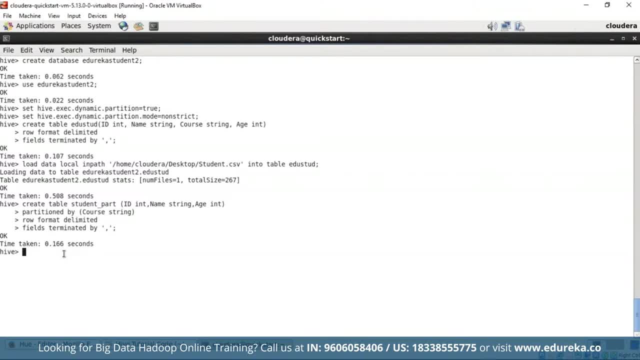 So, using that code, the MapReduce will automatically segregate the data members Or the students based on their courses. So the guys which are in Hadoop will be separated, guys in Java will be separated and loaded into different file, and similarly with Python. Now let's see how to do it using the code. 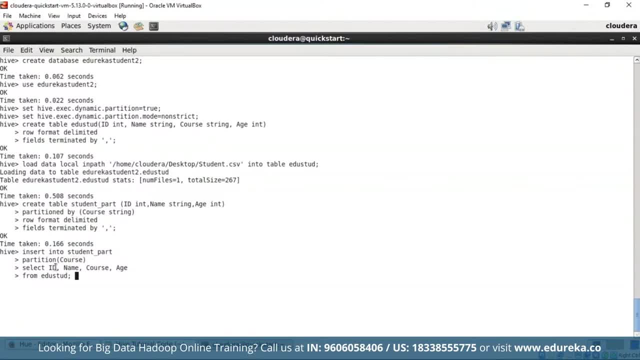 So there you go. We are going to insert into student part partition based on course select ID, name, course, age from the table at you. So the data will be imported from the table. What we have created here, that is a Dureka student, So this particular location has the student dot CSV file. 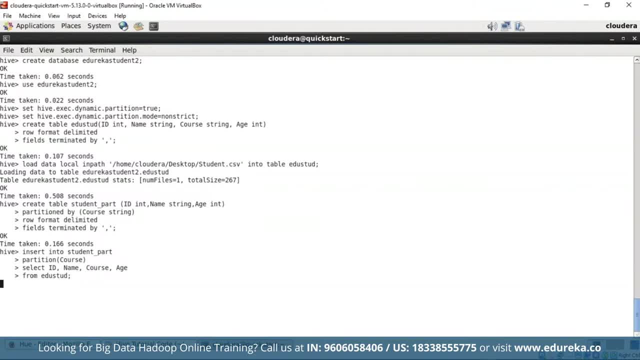 Now let's fire and enter and see if it's created or not. Fine, You can see some of the MapReduce jobs are getting executed. You can see we have three jobs. So first one is getting executed. We have three because one is for Hadoop, one is for Java. 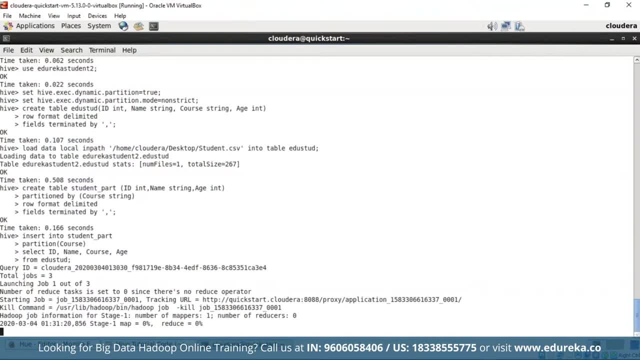 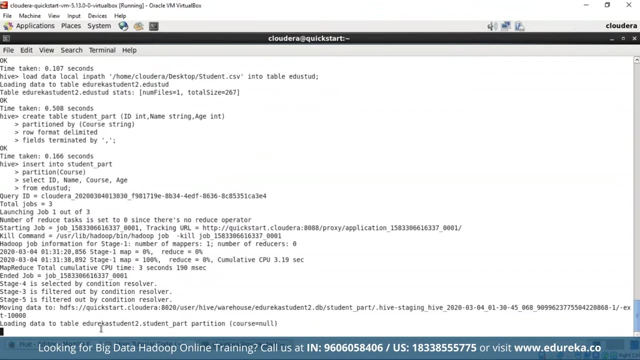 and one for python. So this will take a little time. So this is the reason why I have chosen smaller CSV file, So this save time when you take up the course from a Dureka. then you can work on real-time data so that you get hands-on. 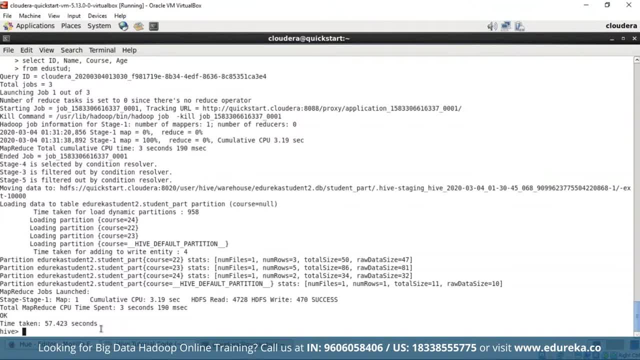 experience from real time and you can get yourself placed in some good companies with the experience what you gain from this particular course. So the stages are been successfully finished and the data has been loaded. Now let's see What are the data is present in the particular table: student. 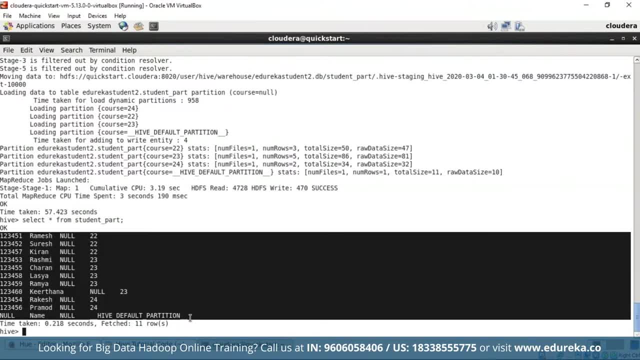 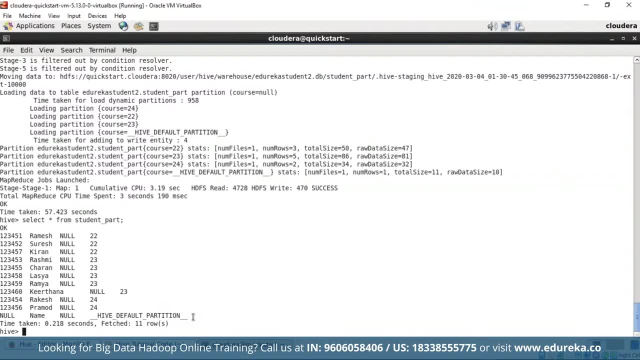 part. There you go, You have the output Executed in here. So these are the data members present in the partition student part. So these are the data members which are separated based on their courses. that is the partition based on their courses. that is how to Java and python. 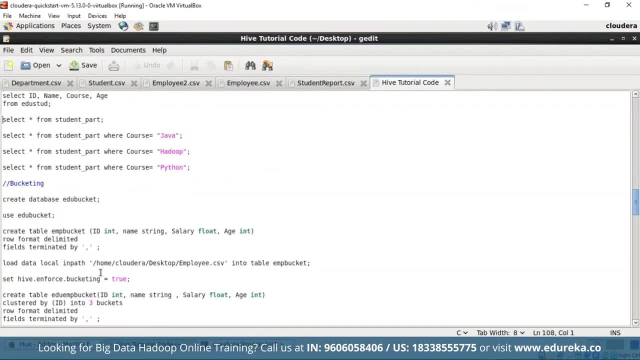 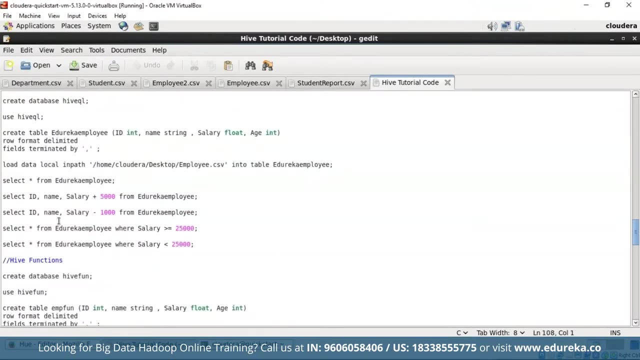 So now that we have understood dynamic partitioning and static partitioning, we shall move ahead into the last type of data model, which is bucketing. once after we finish the bucketing, We shall enter into some query functionalities of hive, Our query operations. 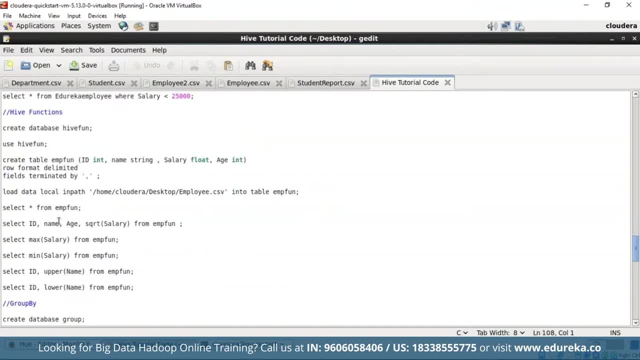 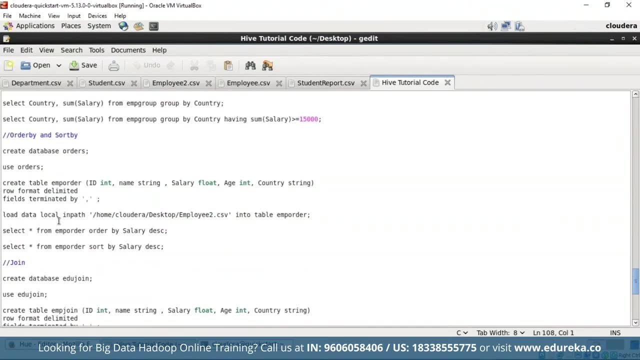 which can be performed in hive and followed by that We will also learn some functions which are present in hive and some of the other things like group by order, by sort by, and finally we shall wind up the session with joints which are available in hive for now. 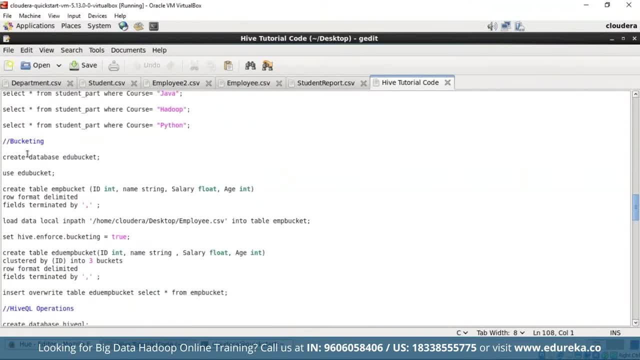 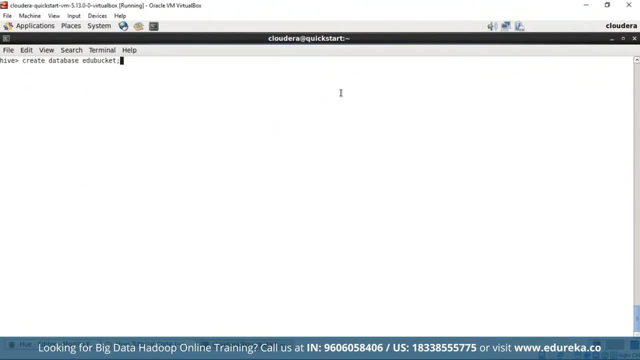 Let's get continued with bucketing, the last type of data model present in hive. So for that let's again start fresh. We shall create a new database for that. before that, Let's go back to You and check if our partition has been made or not. 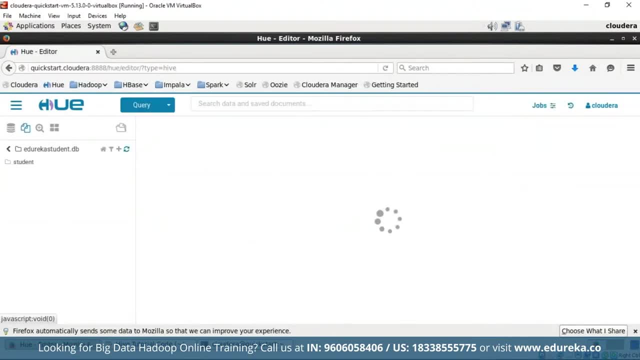 Let's refresh. Also, let us make a manual refresh. So our database was Nidhi Rekha, student to database and inside that we have the table, that a student part, and there you go You can see the files which are based on the partition. 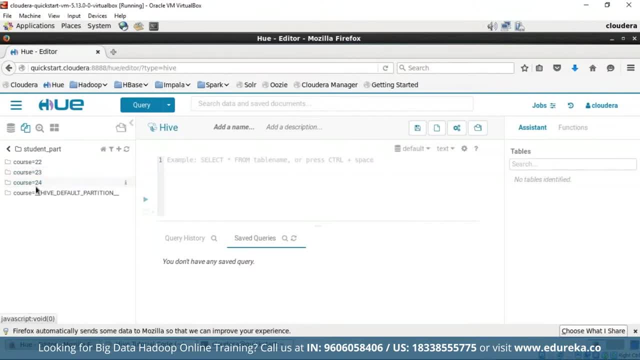 So 22 is for a different course, 23 is for a different course and 24 is for a different course, And this is the default partition, which has all the data members, as we discussed earlier. Now let's start with the last data model in hive. 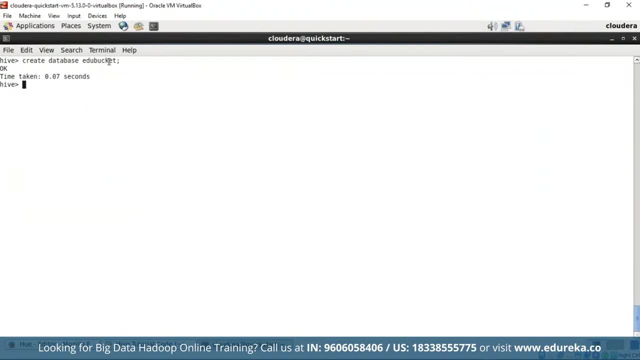 That is bucket. Now we have created a new database that is at Eureka bucket. Now we shall also create a new table for that. before that, We need to start with this particular database so we can use the command use at Eureka bucket. 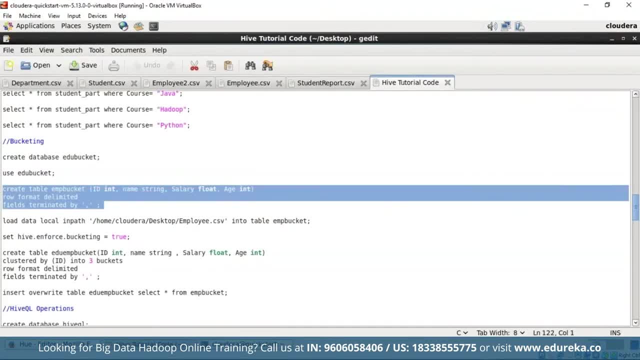 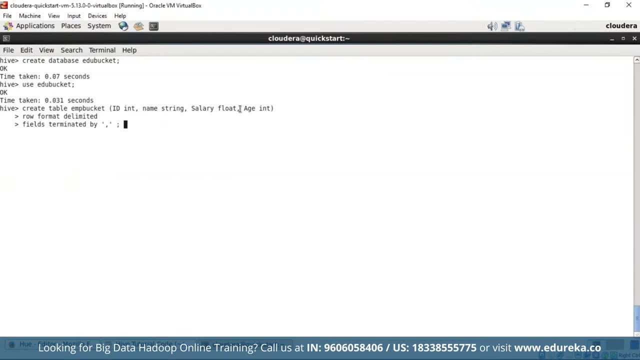 Now we are in Eureka bucket. Now let's create a new table. So the table name will be at Eureka bucket and it will be containing the ID name- salary age of the employees. The table is created. Now let's try to load the data. 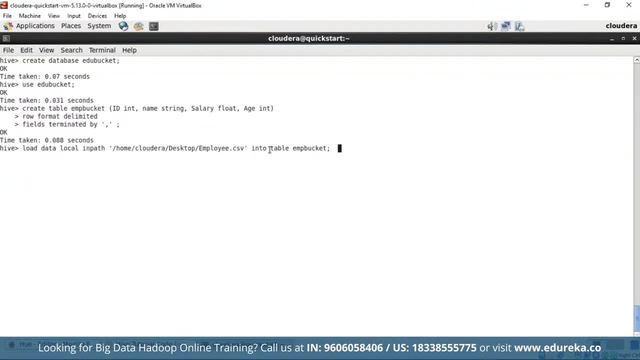 So the data file that we will be using is the same one, That is, the employee dot CSV. So the data has been successfully loaded into the location. Now comes to the major part, that is the bucketing part. So to start a bucketing in high: 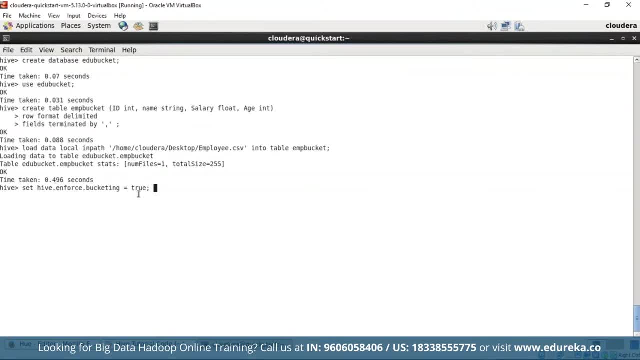 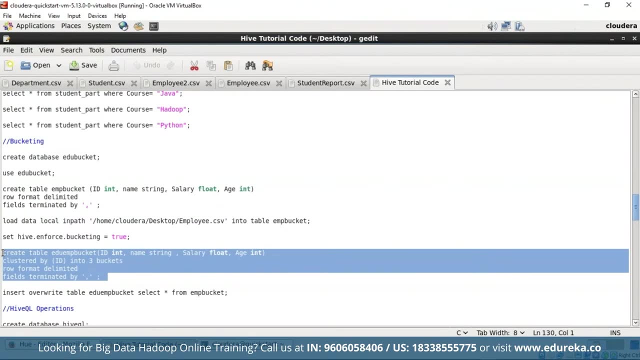 we need to use the command set hive dot info. Start bucketing is equals to true, So that's done. Now we will cluster or classify the data present in this particular file using this particular code. So we will be clustering based on the ID. 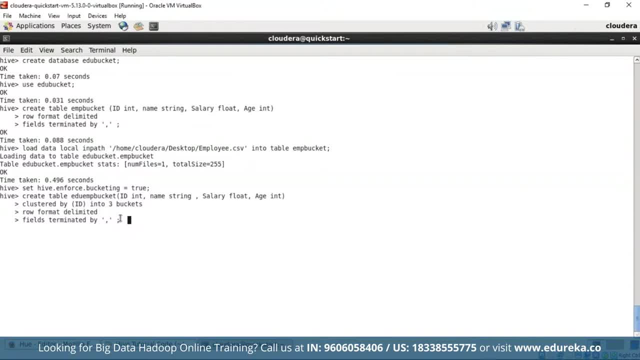 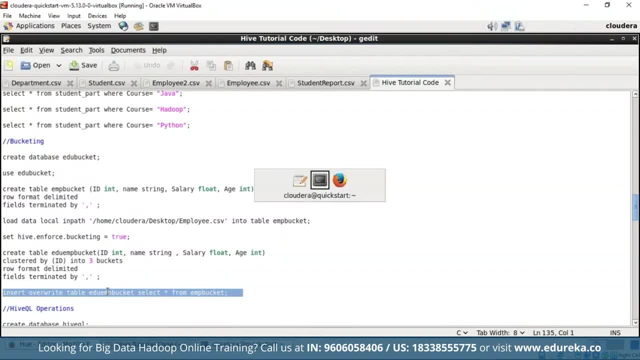 and we will be categorizing them into three different buckets. So let's fire in this command and see if it happens. Yeah, that's successfully done. Now we will override the data using the following command: Now we'll be inserting data into this buckets. 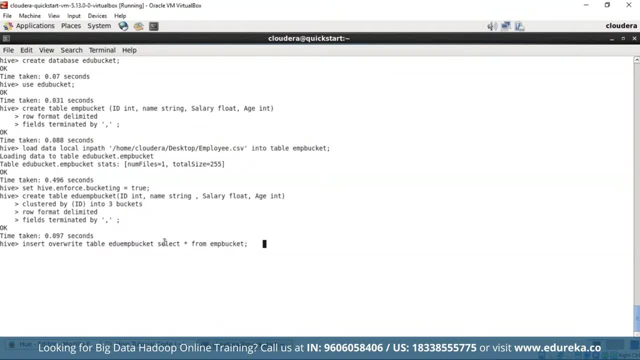 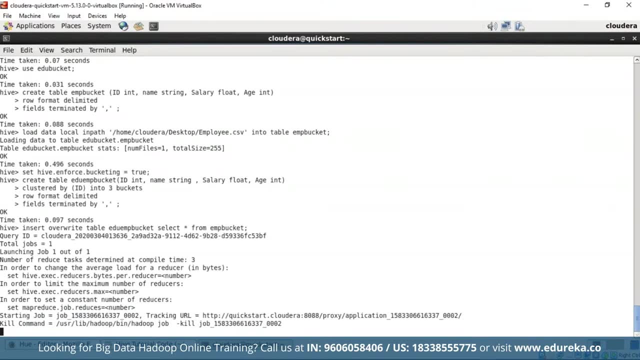 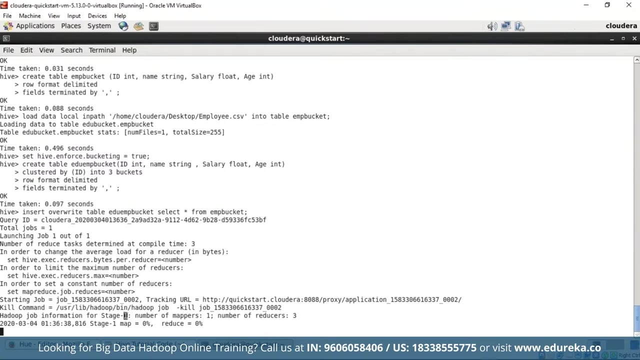 that we have made, that is three buckets, and we will override the table using this particular code. There you go. You can see some MapReduce jobs to be taken care of now. So one mapper and Red users are three for now. So stage one is getting done. 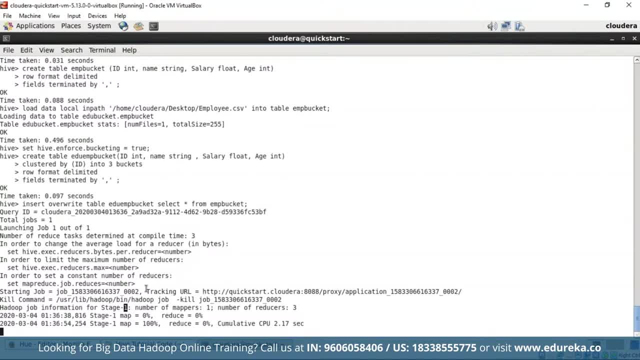 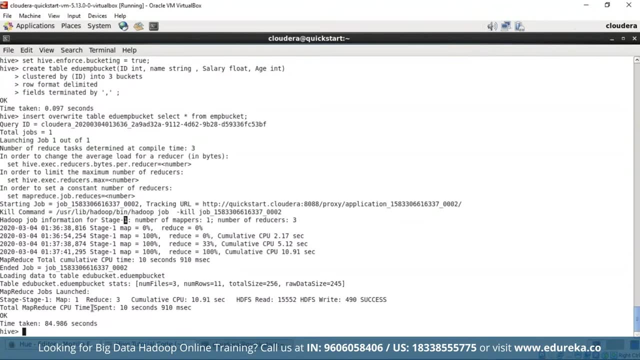 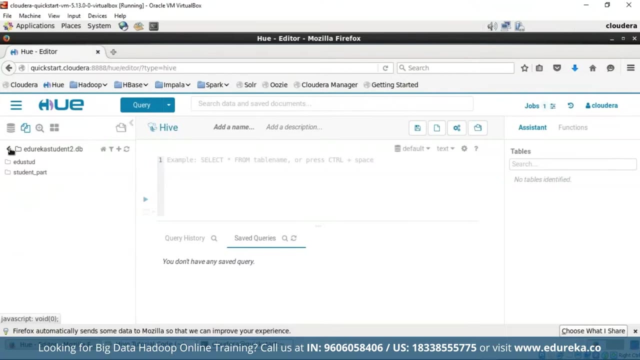 So we should be having three tasks, basically. So let's see Watch the output. stage one is finished, The process is finished and data has been successfully inserted. Now let's go back to hive and check if it's done or not. So before that, let's do a refresh. 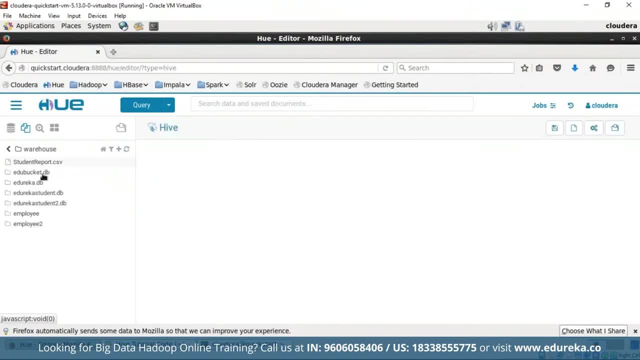 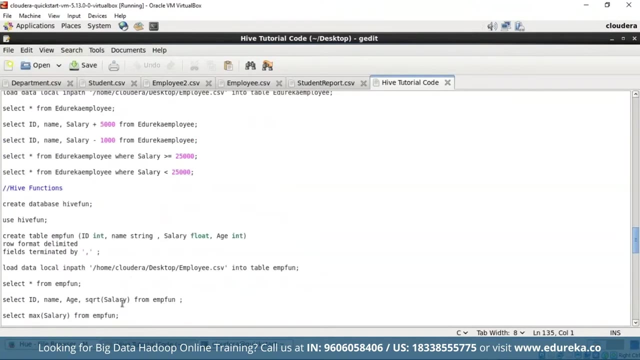 Now a manual refresh would be much better. There you go. We have our database here, which is at Eureka bucket, and inside at Eureka bucket We have EMP bucket and that's our data: employee dot CSV. There you go. Now let's move ahead. 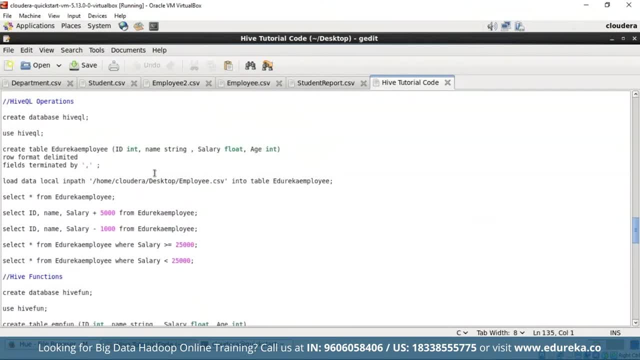 and understand the basic operations we can perform in hive. So for that, let's start fresh again. Let's create a new database. I'm creating a new database for each and every option or every operation that I'm performing in this particular tutorial. just to make things. 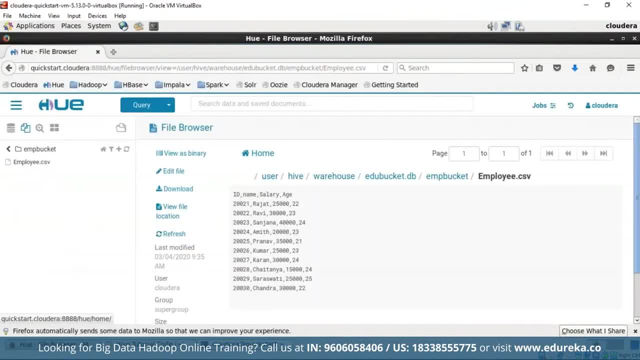 or keep things in a sorted manner. So as you can see here in our particular file system I have separated each and everything, like I have sorted everything. so for bucketing I've got a separate database and for partitioning I've got a separate database. 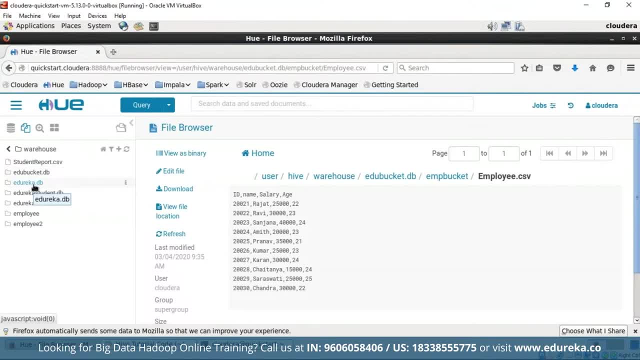 and for understanding how to create database and tables, have got a separate database for that, just to keep things arranged and sorted. This looks in a much better way. So now let's discuss about the operations that we could perform in high. So I'm creating a new database again for this. 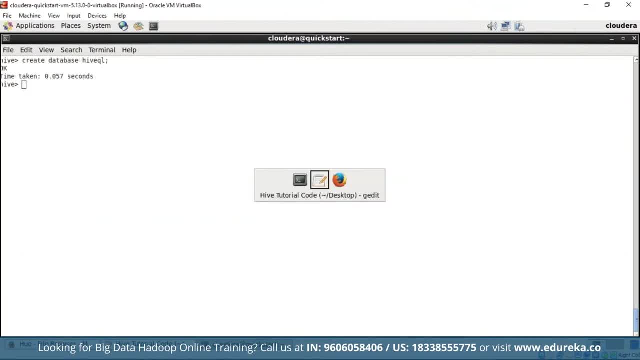 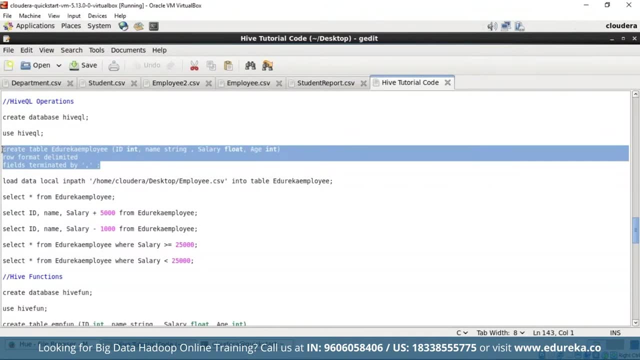 So the database would be hive query language. Now let's use this particular The database. this creates a habit of learning things in a better way, or it's like a revision for the things, what you have performed or learned. so far as you can see, the table has been successfully created. 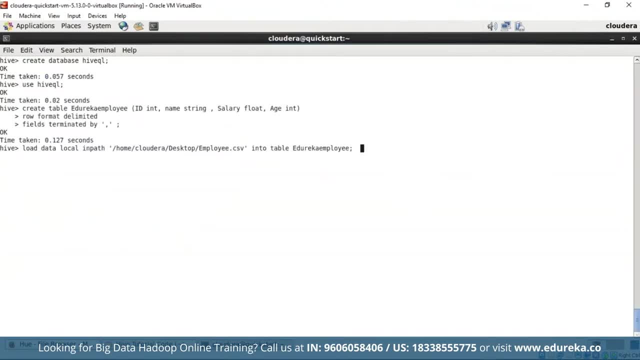 Now let's try to add in some data into this particular location, that is, employee data. It's been successfully loaded. Now let's try to see what are the details present in this particular file. We can use in the command select star from the table at Eureka employee. 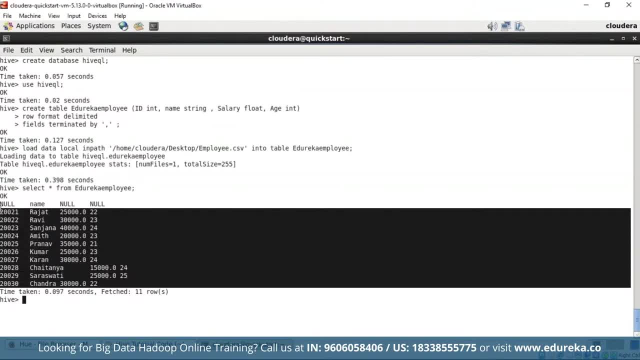 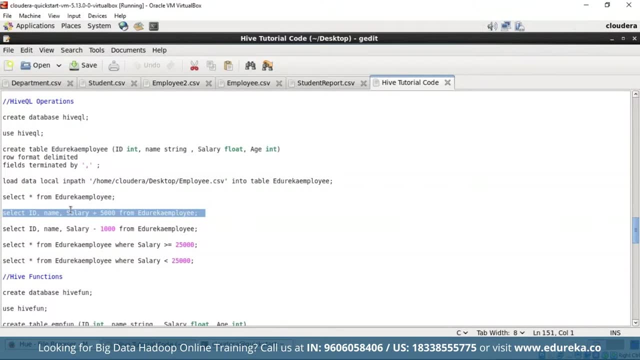 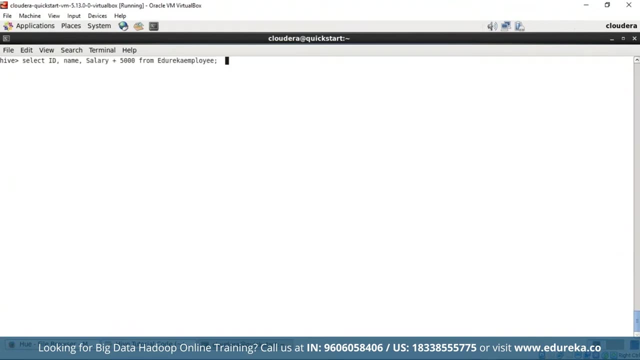 So there you go. These are the details or information present in the table at Eureka. employee. Now we shall see what are the functions that we can perform on this particular file. So, since we discussed that the mathematical operations and logical operations can be performed on high, 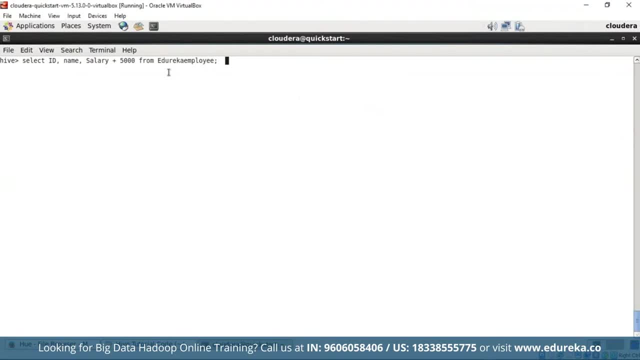 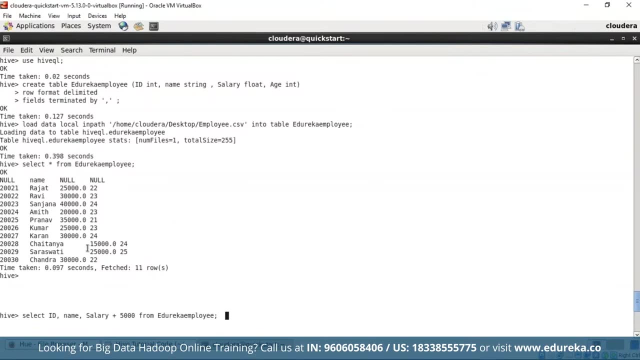 So let's try to perform an addition operation. So I'm selecting the column salary and, as we have seen here, the salaries are 25, 30, 40, 20 thousand rupees for every employee. now let me add in 5,000 more to each and every employee. 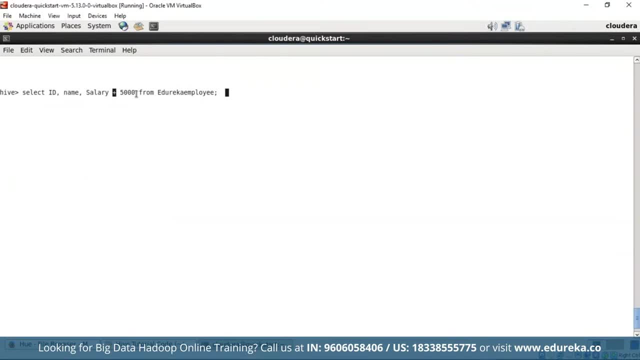 So I'm adding the value 5,000 by using the addition operation. So let's enter. you can see we have added 5,000.. So the first element was 25, now it's 13.. So, similarly, all the other employees got 5,000 rupees hike. 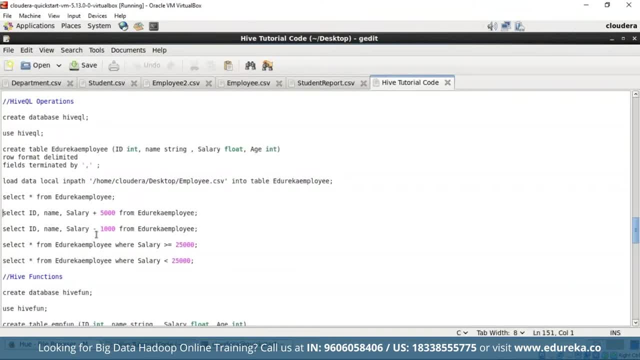 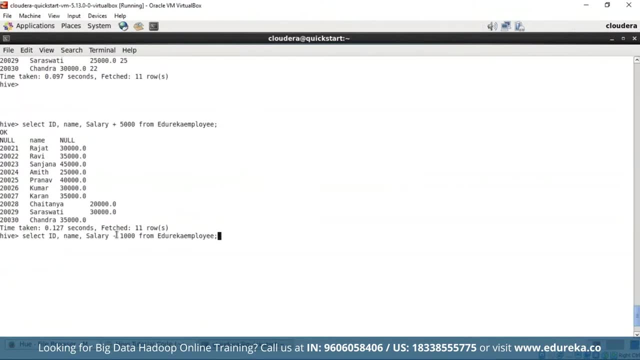 all of a sudden. now let's try to remove 1,000.. So to do so, all you need to do is replace the addition operation with a subtraction operation, that is, minus by an enter, and they go. each and every employee lost 1,000. 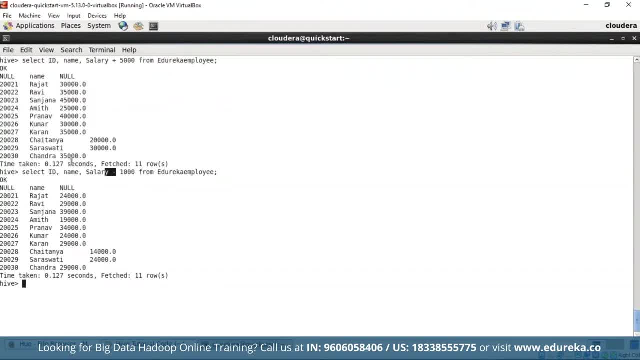 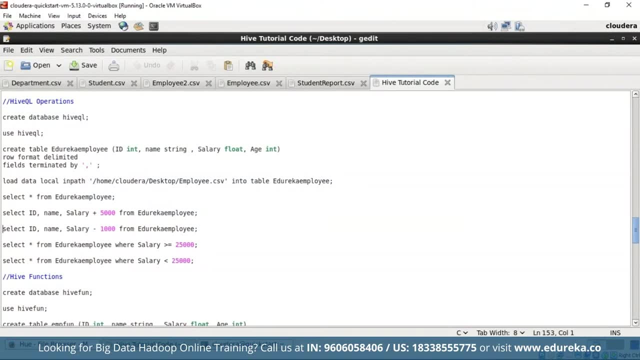 So the initial amount was 25,000.. So removing 1,000 from that will result in 24.. This is considering the first initial values. This is how it's working. followed by that, Let's also perform some logical operations. Let's clear the screen. 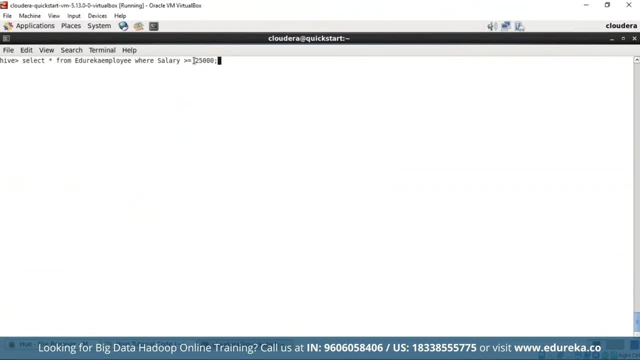 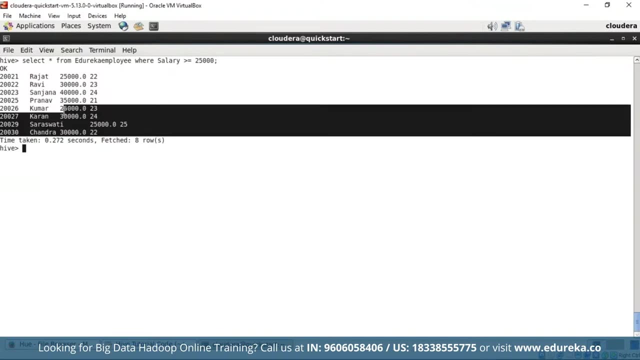 And yeah, here I'm fetching for the employees who are having a salary equal to or greater than 25,000.. So these are the employees which are having the salaries above or equal to 25,000. similarly, let's execute another one which detects the employees. 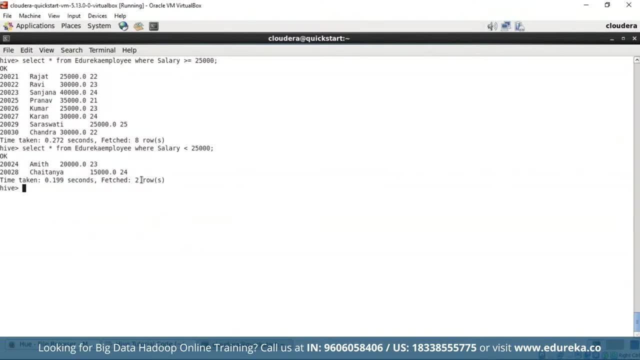 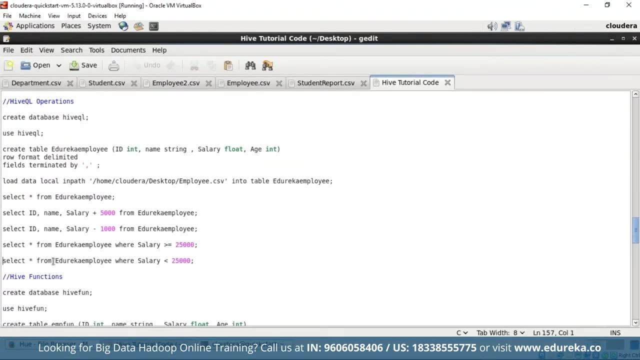 with salaries less than 25,000.. So do? we have got two employees which are having lower salaries, which are Amit and Chaitanya. fine, So this is how you perform some operations in high. So now let's move ahead and understand the functions. 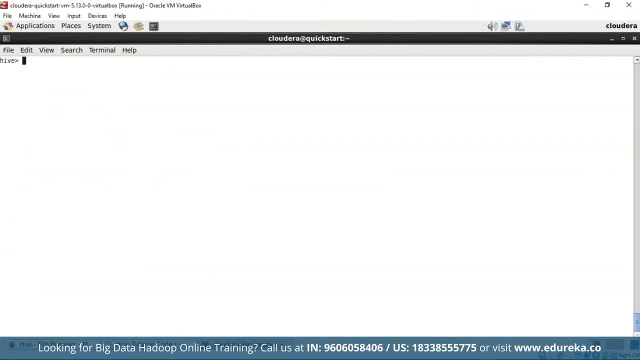 which you can perform on high. So, in the same way, let's create a new database again and let's use this particular database that has high functions. Now let's create a table in this particular database. So the table is employee function and it's created. 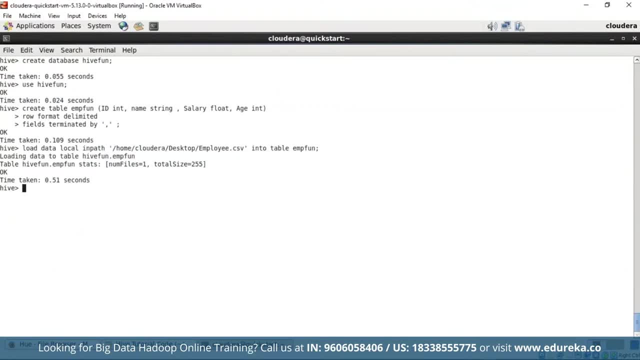 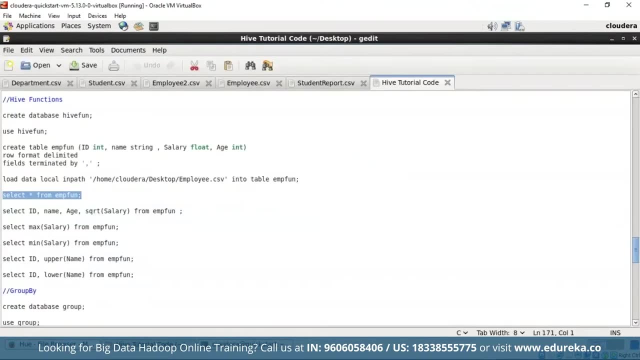 Now let's try to load in the data. Yeah, the data has been successfully loaded. and now let's see if the data is correctly loaded or not. Yeah, the data is loaded correctly. Now let's try to apply some functions. 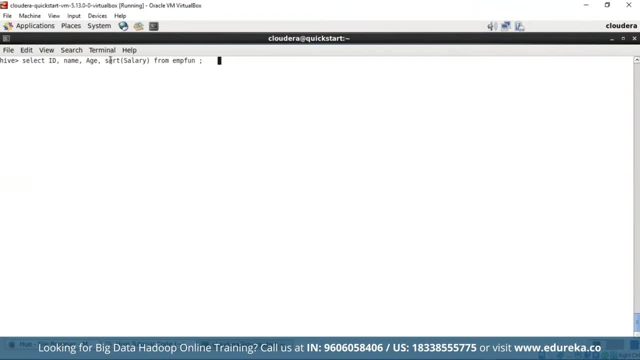 In this particular data. So the first thing or the first function I'm going to apply would be a square root function where I'll be finding out square root of the salaries of the employees. So there you go. The square root of 25,000 was 158 dot decimal numbers. 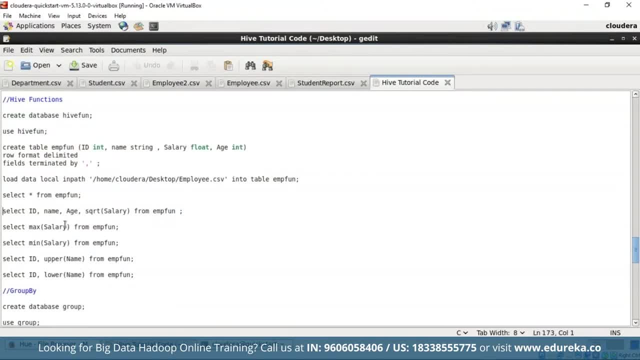 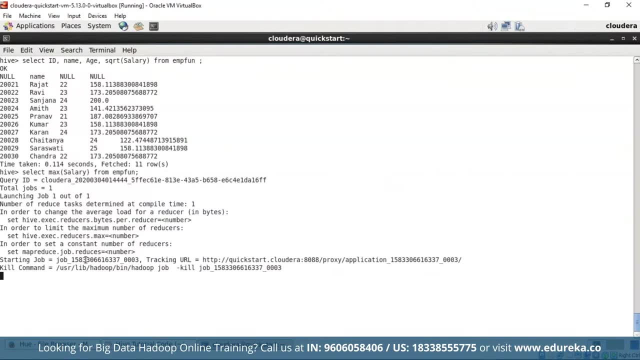 So this is how you perform some basic functions on your data. Now let's try to find out the maximum salary. So yeah, the job is getting executed. You can see some MapReduce chops here. I think the biggest salary would be from Sanjana. 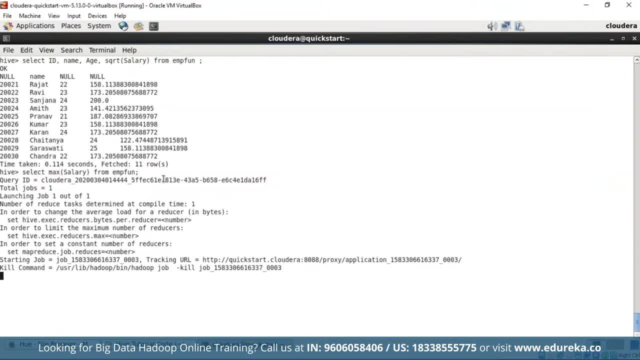 So the maximum salary is 40,000.. So this is how it works. Since we are working on cloud error and the system configuration is limited, The execution speed is a bit low, but if you're working in real time, then this process would take like few seconds and it's done. 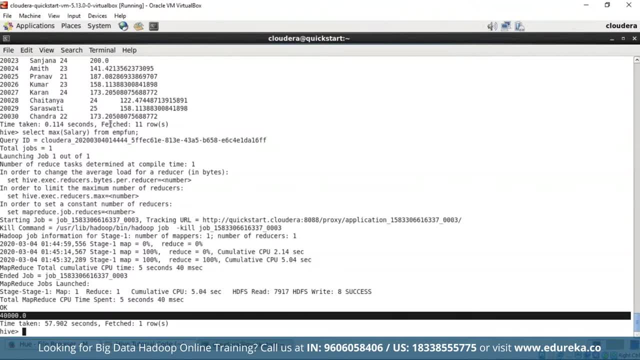 There you go. You have the value 40,000, as shown here. So 40,000- the employee name is Sanjana- is the maximum salary. So that's what we got here. Now let's try to find out the minimum salary. 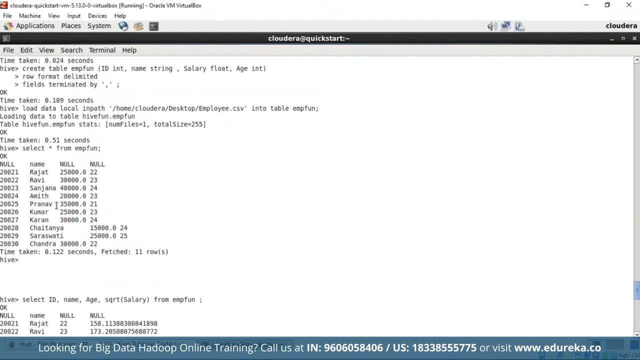 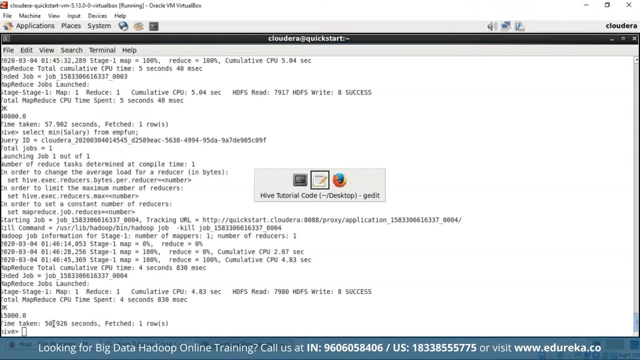 So the minimum salary is 15,000.. And who would that be? Yeah, it's Chaitanya, with minimum salary 15,000.. So that's how you do some operations And I let's execute some more operations, such as converting. 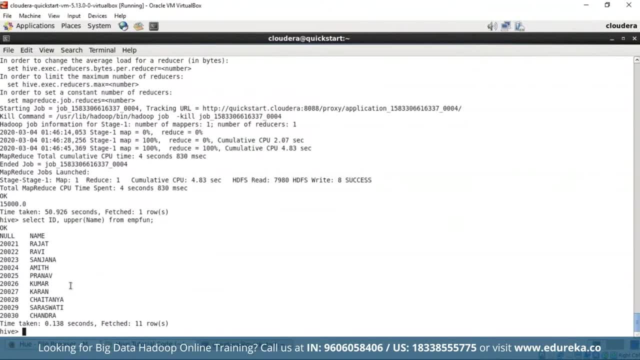 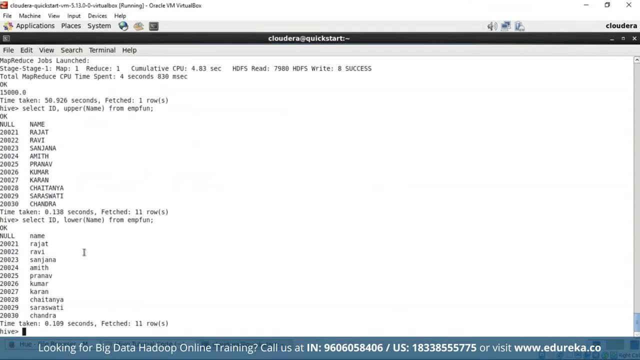 the names of the employees to uppercase. So you can see the employee names are converted to uppercase here. And similarly, let's try to convert to lowercase. So here you can see we have converted them to lowercase. So this is how you learn technology. 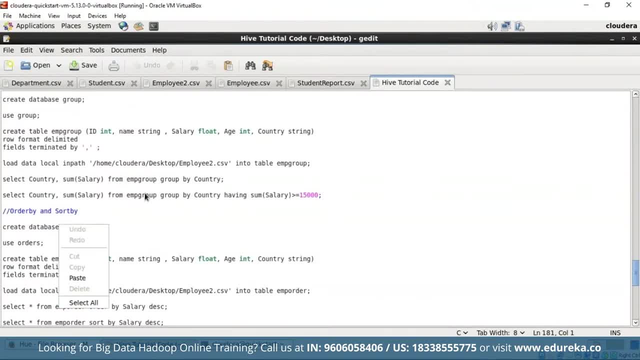 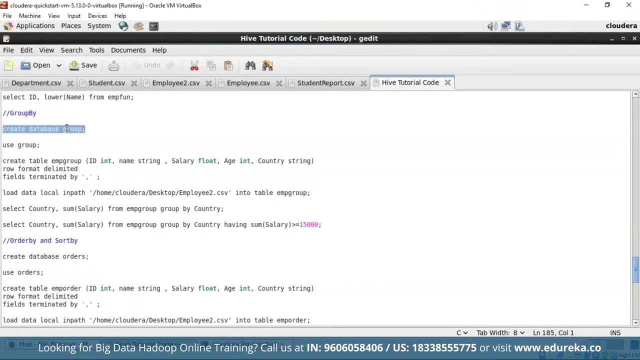 You need to play with the technology. Then you will come to know the advantages and disadvantages So you can learn the possible ways where you can make things work out. This is how you do it. Now let's move ahead and understand group by function. 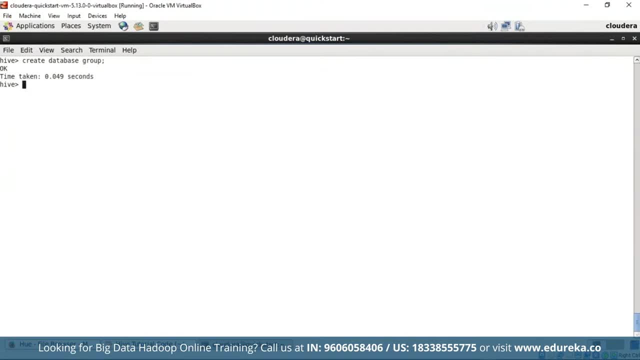 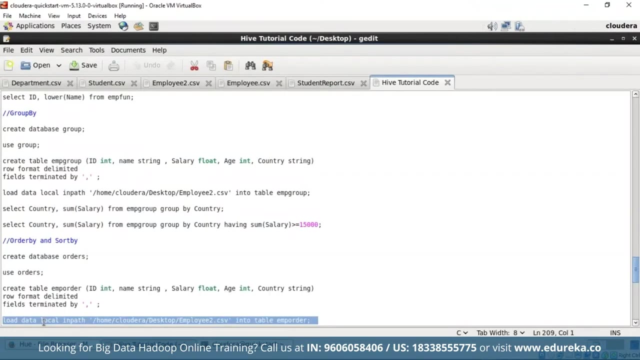 in five. So for that we'll be creating a separate database. that is group. Now we will use this particular database. that is group. So we'll type in command: use group semicolon. Now we'll create a table. So the table has been successfully created. 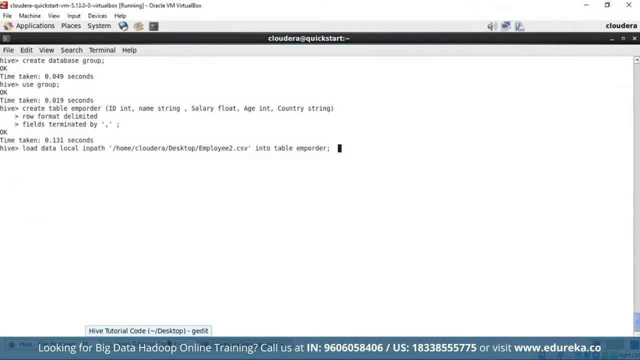 Now we will load data into this particular table. Now we will use the new CSV file which will be employed to dot CSV. Now we are using this particular table because we have an additional column in this particular table, which is the. 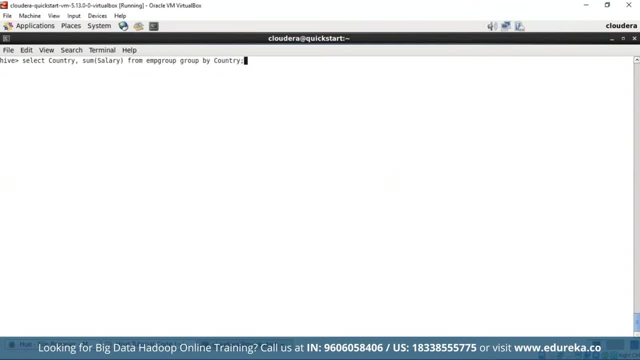 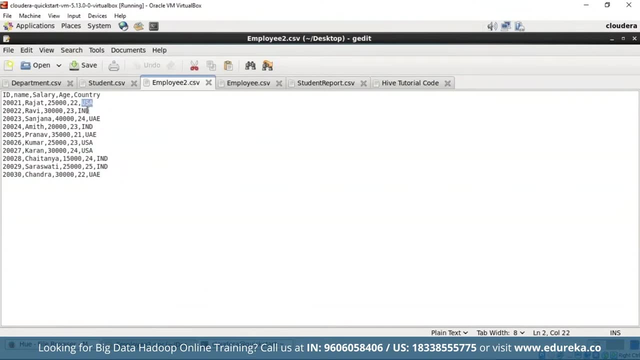 country column. Now, as discussed before, we will be grouping the employees based on country. Let's see our data first. So we have countries such as USA, India, UAE, So these are the three countries that we are having in our CSV file. 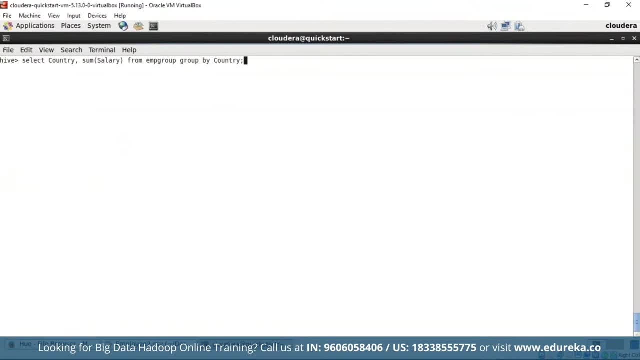 So we will be categorizing the employees based on their countries. So this is the particular command that we will be using. So let's see what we have here. So let's see what we have here. So maybe I made an error while creating the table. 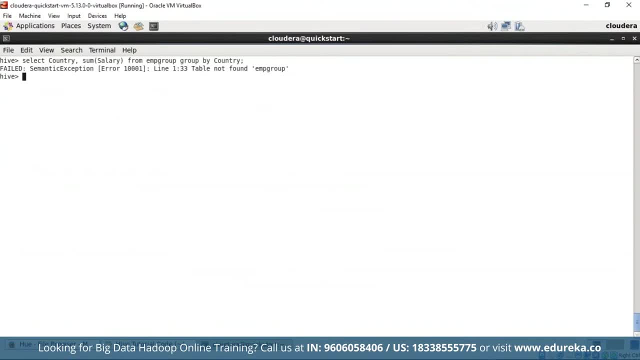 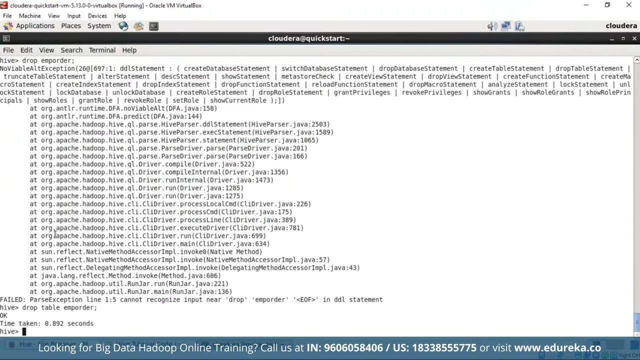 I think I gave a wrong table name here, So let's drop our table. So by mistake I gave different table. that is employee order. So to drop a table you just need to use the keyboard drop and it's done. Yeah, the keyword table was missing. 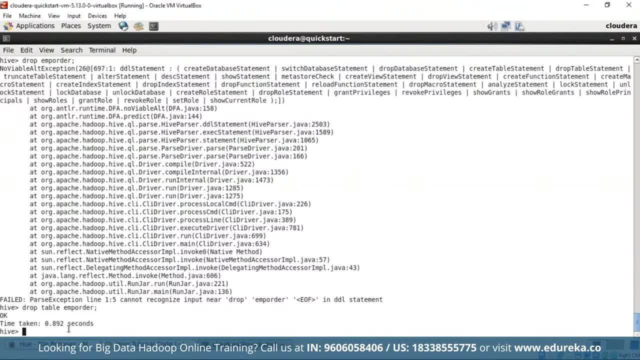 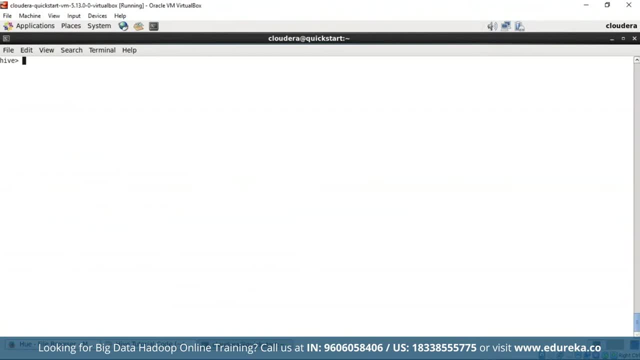 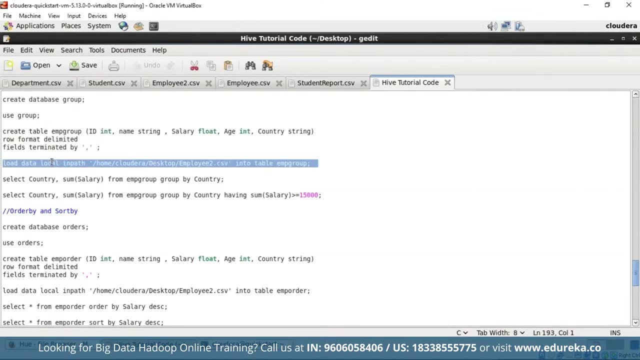 So you need to type in drop table and the table name and the table gets dropped. So we were supposed to create a different table, that as employee group. So now let's create a new table that is employee group. employee group has been created. Now let's try to add in data into the employee group. 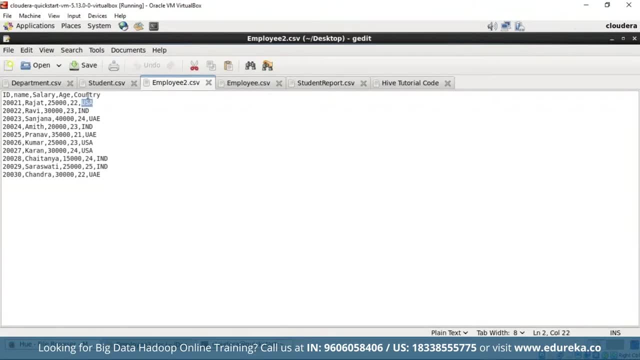 So we have used employee to here, because the employee to has another column which is based on country. So the countries that we are having here are India, USA and UAE. So we will be using the group by function here And we will categorize the employees based on their countries. 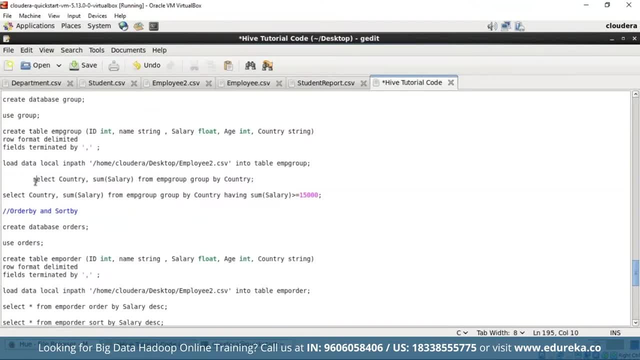 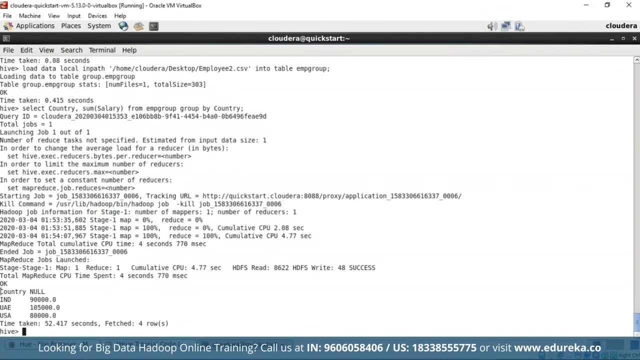 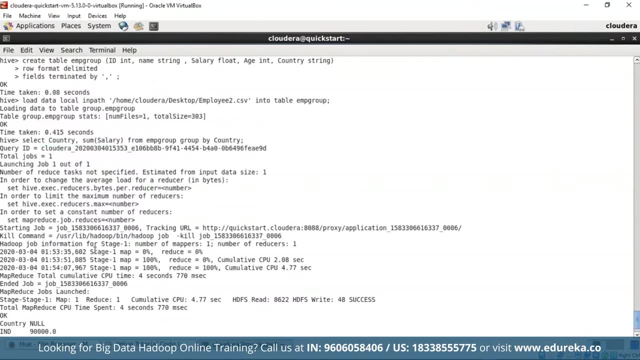 So there you go, You can see some MapReduce jobs getting executed. Yeah, there you go. We have categorized the employees based on their countries, that has India, UAE and USA- And the sum of the salary. So the guys working in India and their summation of the salary. 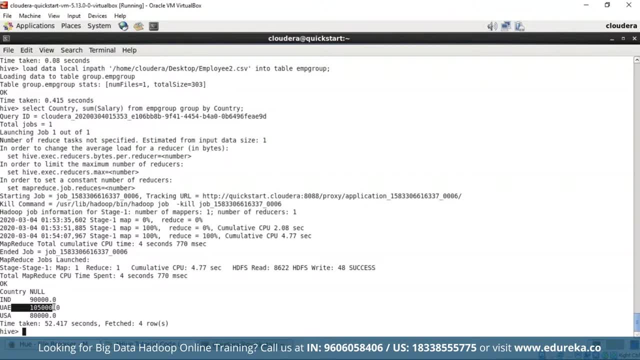 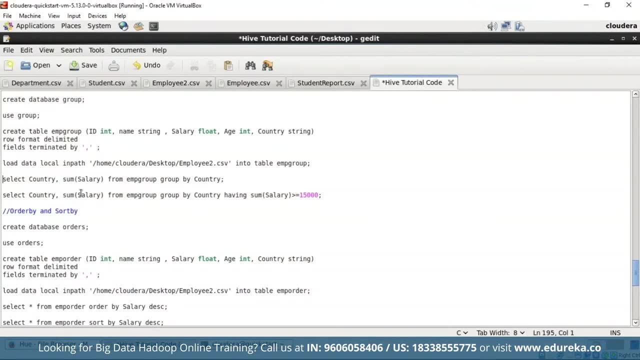 is 90,000.. And similarly, you is nearly 1 lakh 5000 and USA is 80,000.. Now let's also execute a different command based on group by. so here we'll be using group by function and we will categorize. 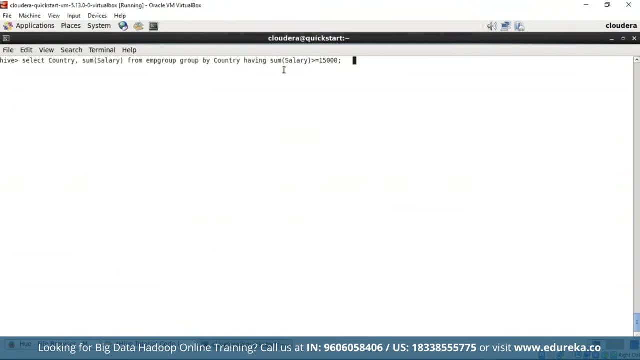 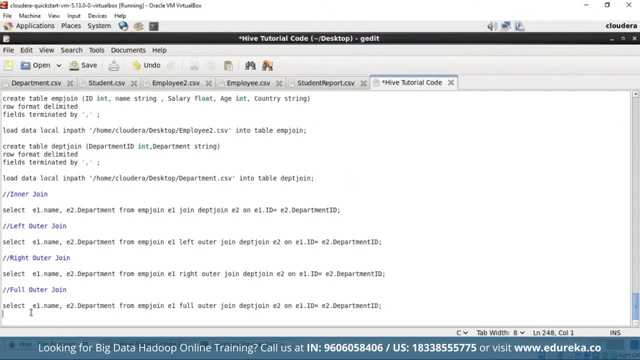 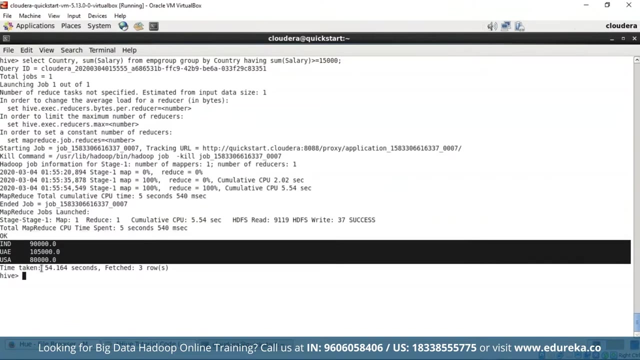 based on the country, as well as the summation of the salary, which is greater than or equals to 15,000.. So it's similar to the previous command. So you can see the data got executed and we got the same output. Now let's move ahead and understand order by and sort. 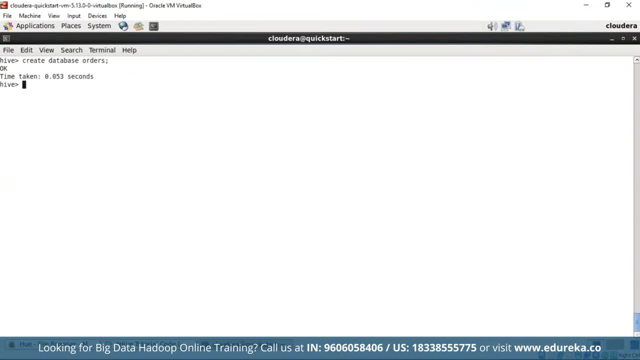 by methods. So for that we'll create a new database: orders Now. we'll use orders Now. let's create a new table again. So the new table is employee order and the table got created. Now let's load the data into this particular table by now. 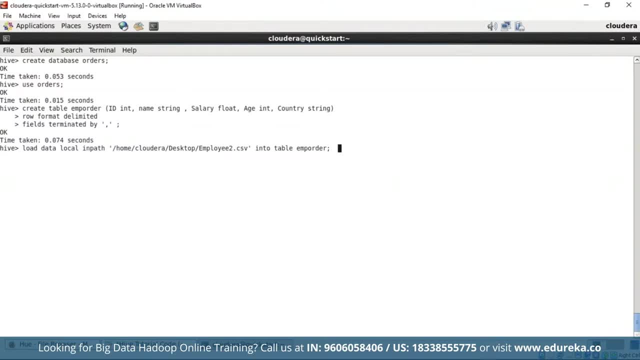 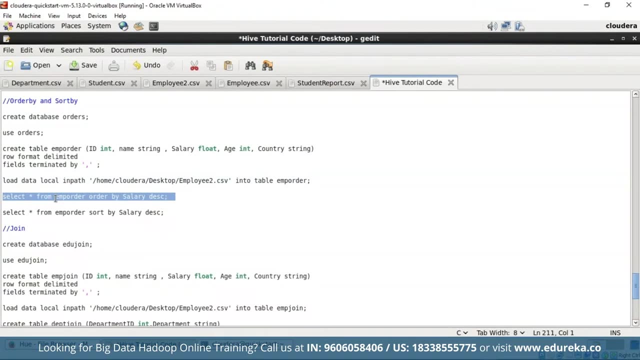 I think you have some good practice of how to create a database, How to create a table and how to load data into that particular table. So the data got loaded and now we are going to order the data present in this particular table based on the descending order. 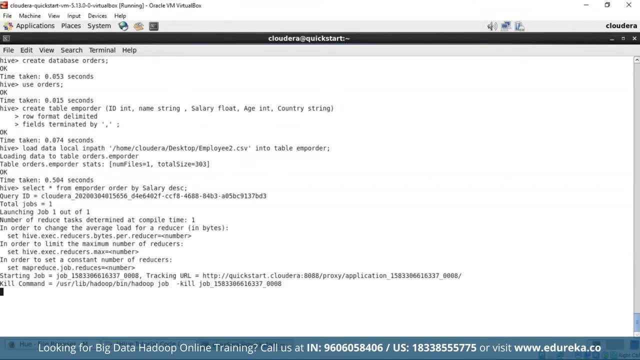 of their salary. So you're seeing some MapReduce jobs going ahead. So here we'll see the employees ordered based on their salaries in descending order. So the highest salary will be at the first place and the lowest salary will be at the last place. 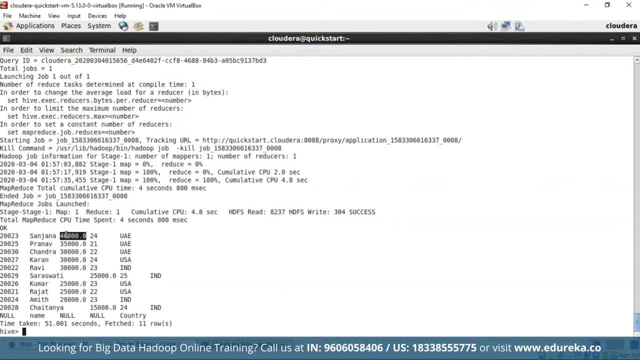 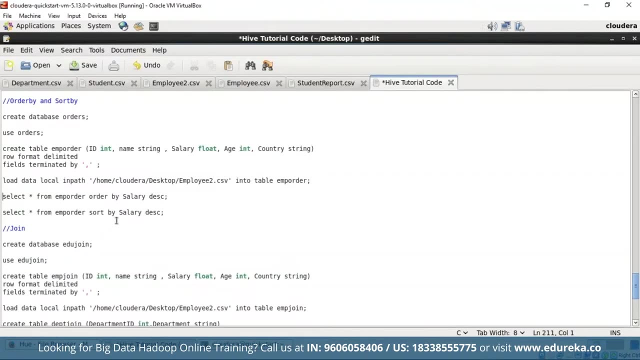 Yeah. So we have engine at the first position with the 40,000 as the highest salary, and she's working for you, ae, and we have Chaitanya with lowest salary- 15,000- working for India. Now let us also execute another command based on sort by. 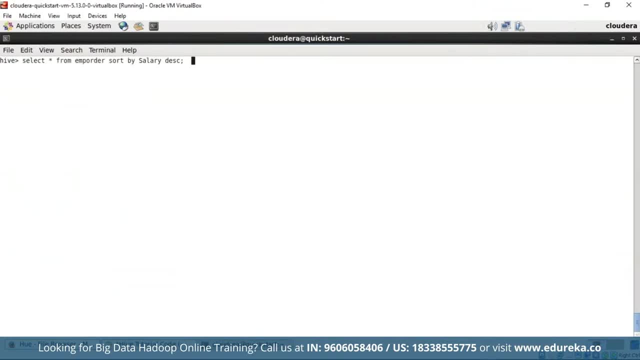 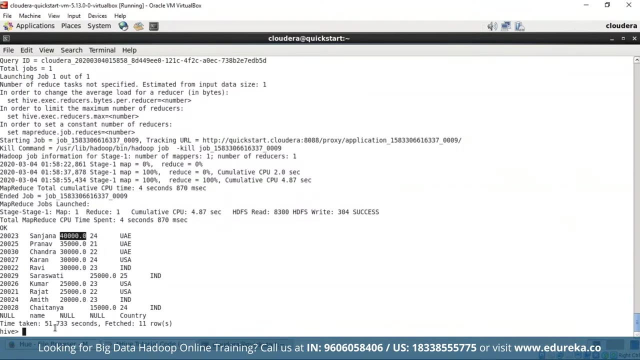 so first we try to execute a command based on order by. now let's see the same output using sort by. so basically both work in the same way. So there you go: We have sorted the records based on descending order of salary. now that we have learned. 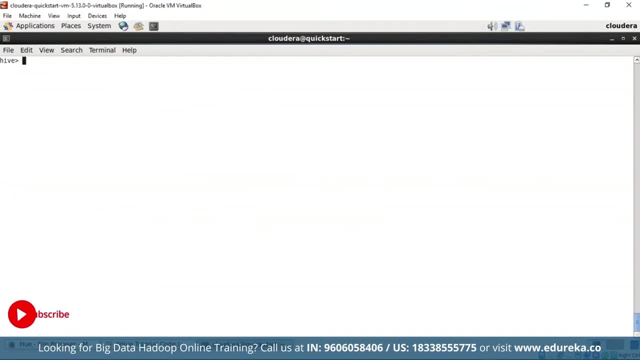 What are the various operations that can be performed in high? that are the automatic operations, logical operations and also some of the functions such as maximum, minimum. group by order, by sort, by. so these are the various operations and functions that you can perform in high. Now let's move ahead into the last type of operations that 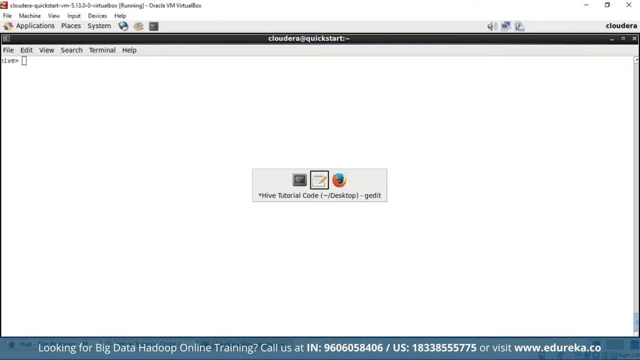 can be performed in high. Those are the joints. So for that, let's again create a new database. So here I'll be creating a new database that is at Eureka join, and followed by that, Let's use this particular database now for that. 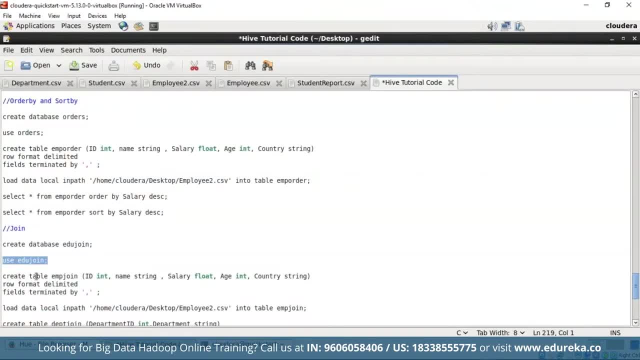 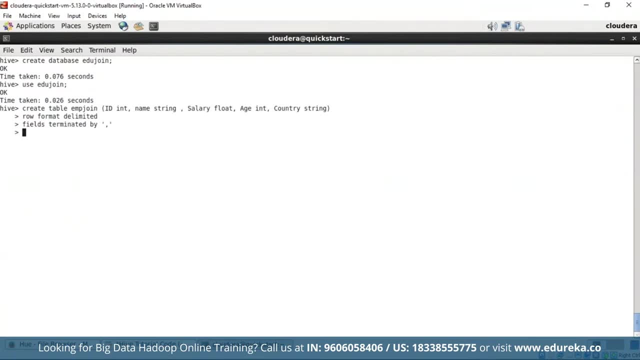 We need to use the keyword use and there you go, We are in at Eureka. join Now let's create a new table for that. So the table will be EMP: join here. You can see that I forgot to mention semicolon. 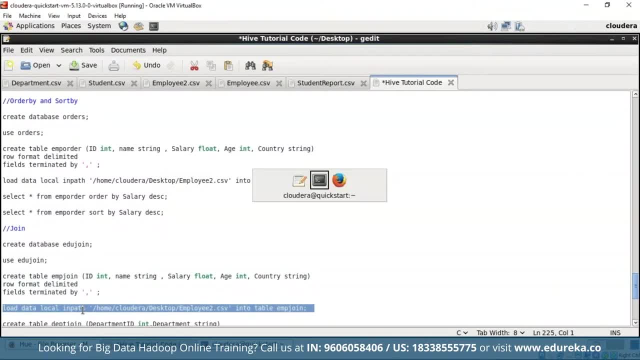 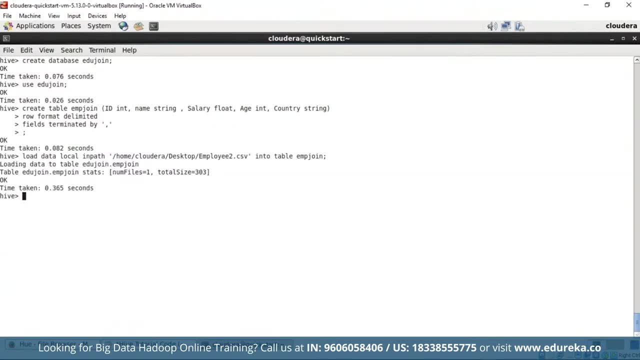 So now the table got created, now We should load the data into this particular table. So now I've created the first table, that is, employee table, and I'm loading the employee data into this particular table. now to perform join operations We always need two tables. 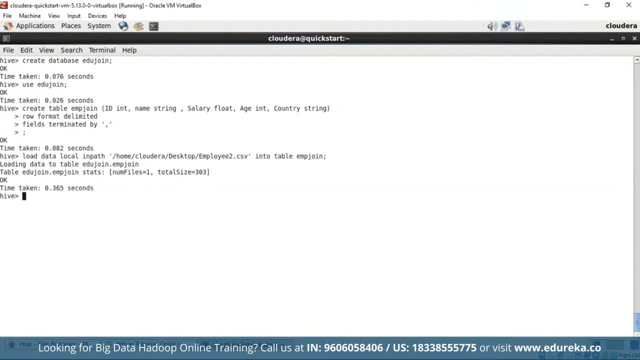 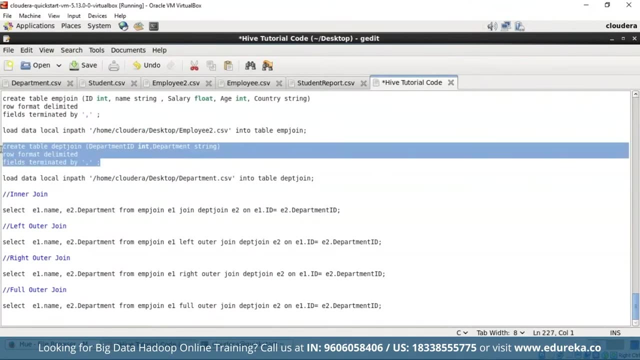 So in this particular database at Eureka join, I've already created the first table, that is employee join. Now let's create second table, that is the department table, which will be present in the same database. So this particular table is a department table. 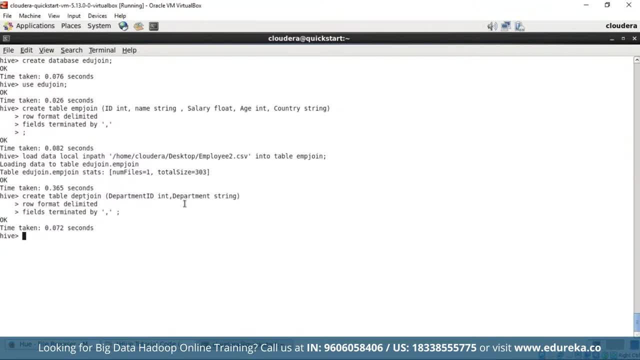 which will be having the entities that are, department ID and department name. Now let's load the data of department into this particular table. So the data has been loaded, So you can see the employee. two dots. Yes, we had the columns ID, name, salary agent country. 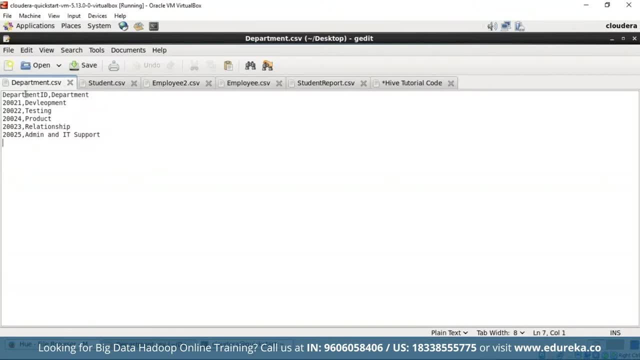 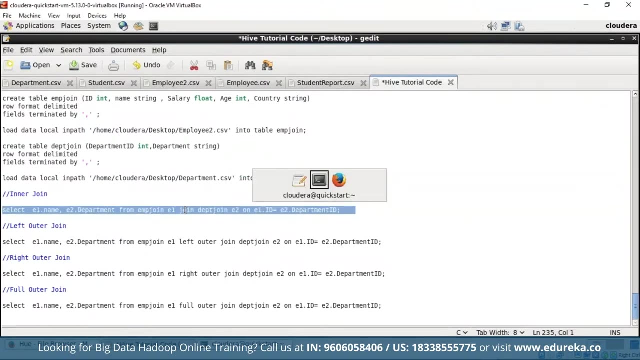 and similarly the department dot CSV has the entities, which are department ID and the department name. So the department IDs are in here and the names are development, testing, product relationship and admin and ID support. Now we have created both the tables and we have created 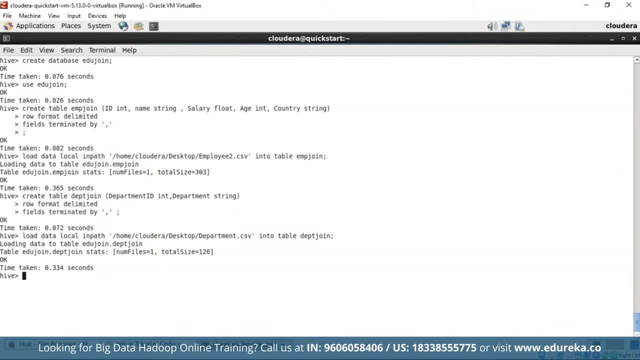 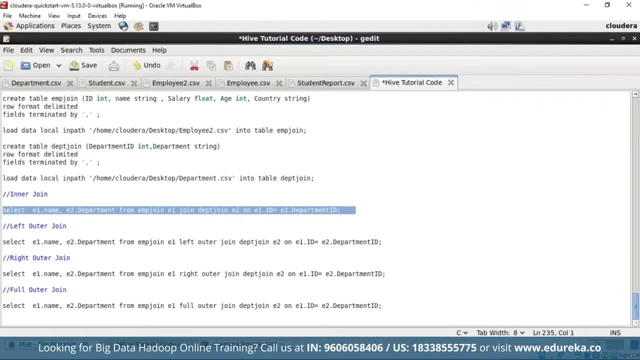 or we have loaded the data Also. Now we have four different joints available in Hype. They are in a joint, left outer joint, right outer joint and full outer joint. Now let's perform the first type of join, which is the inner. 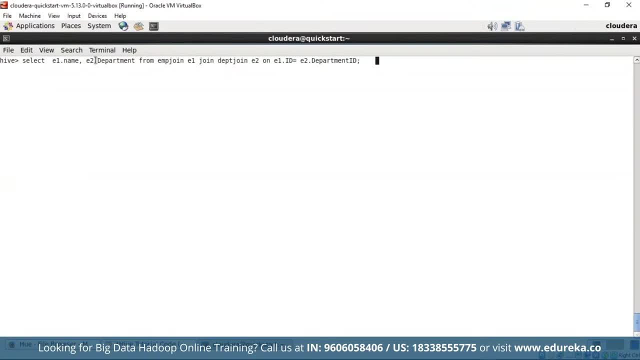 joint. So in inner joint we are going to select the employee name and employee department and, based on the employee ID and department ID, We are going to perform the joint operation that has the first joint in the joint. So you can see some jobs getting executed. 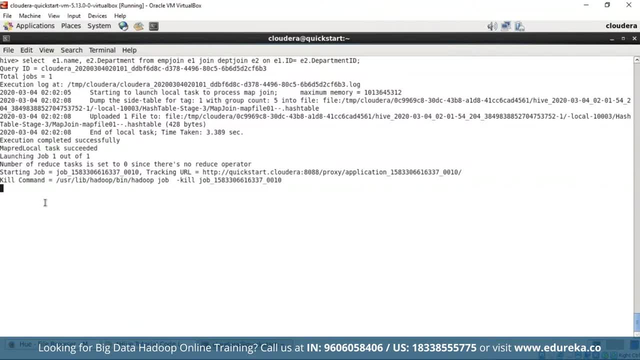 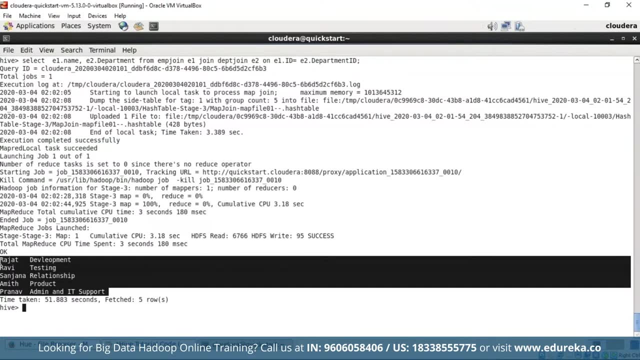 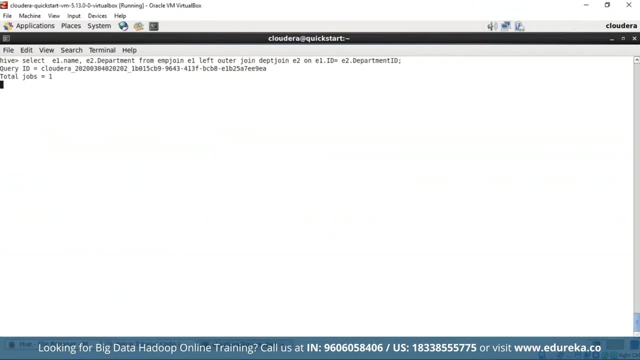 So the map reduced task successfully completed. So the first set of John has been successfully finished and the output has been generated. Now let's try out the second type of join that has the left outer join. So the only difference is that we are using the keyword left. 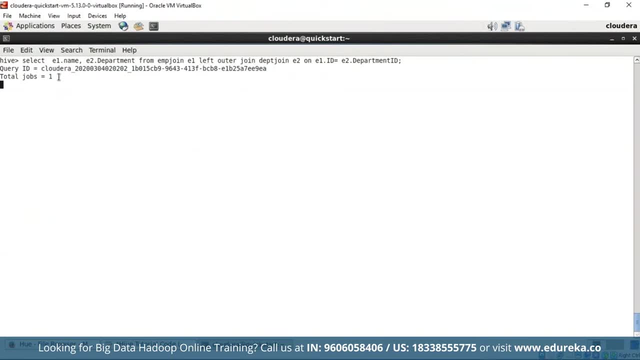 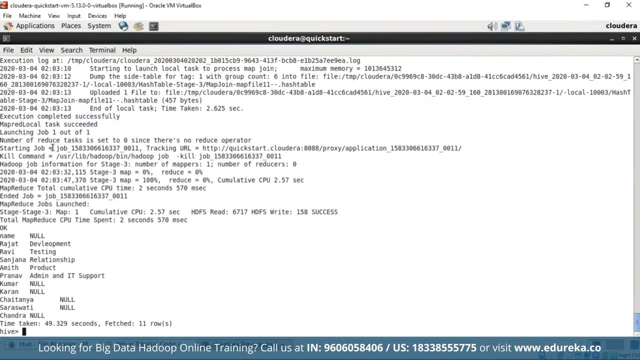 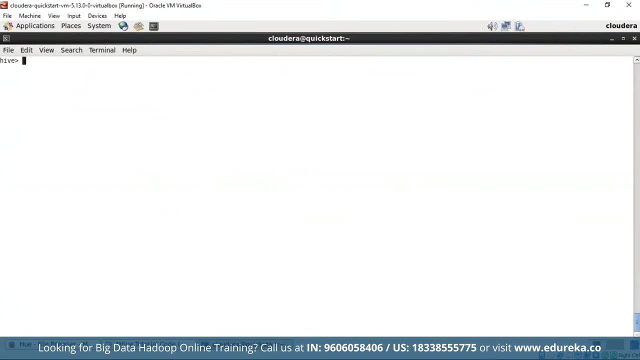 outer join. Now you can see one of the job got started, So you can see the output has been generated as well of the left outer joint. Now let's move ahead and understand right outer joint. So for right outer joint you need to use the keyword right. 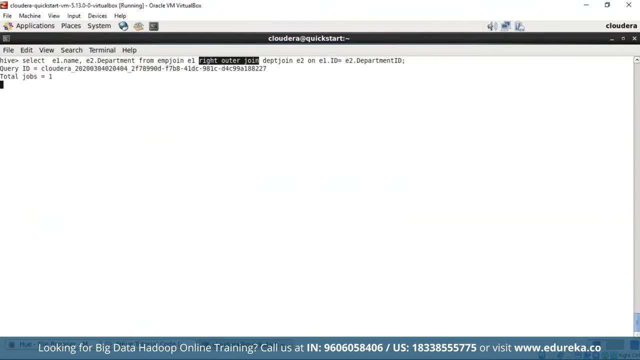 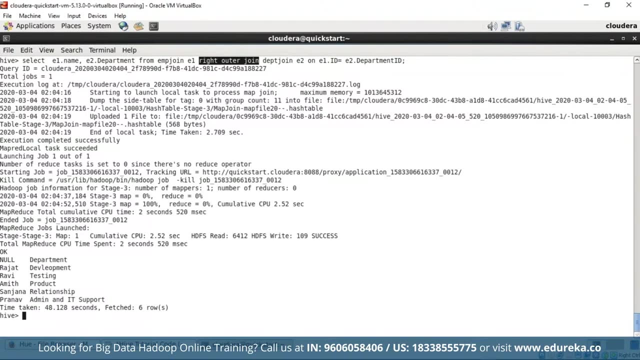 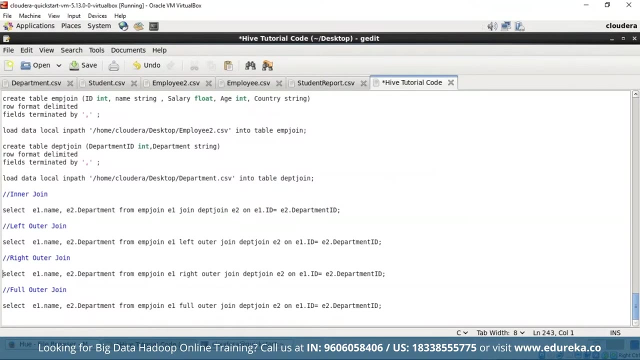 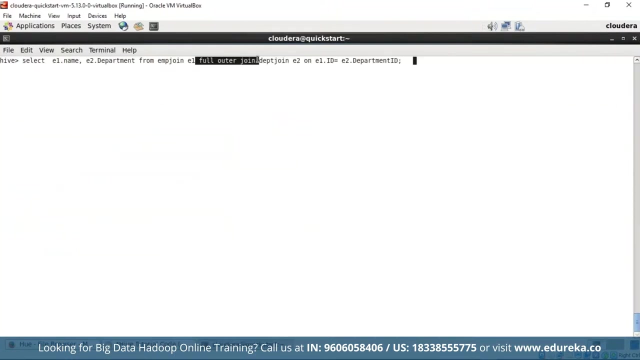 outer joint Fire in the command and you can see the jobs getting executed. So you can see the output of right outer joint has been successfully executed or displayed. Now let's type in the last join operation, that is full outer join. So here I'm using the keyword full outer join fire in the 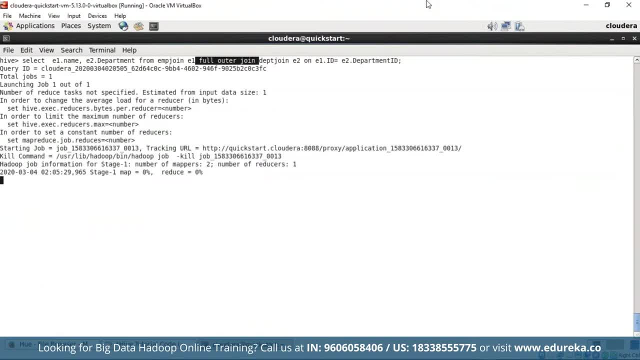 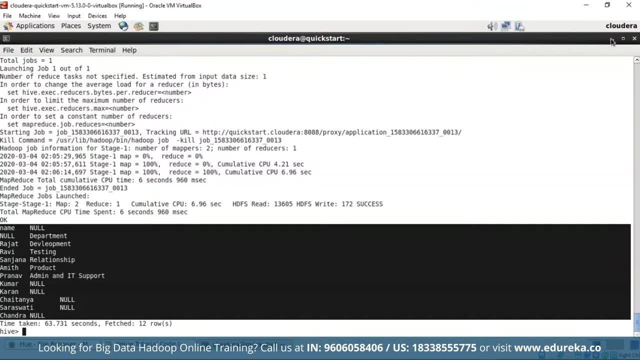 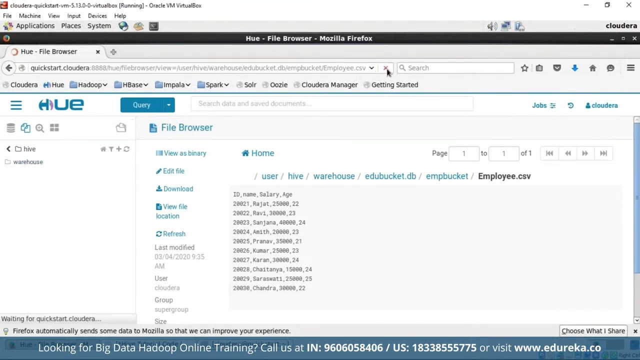 command and you can see it's getting executed. So the output for full outer joint has been displayed here. So this is how the joint operations are executed in hive. So we have learned how to create database, how to create table, how to load data and the various data models present in hive. 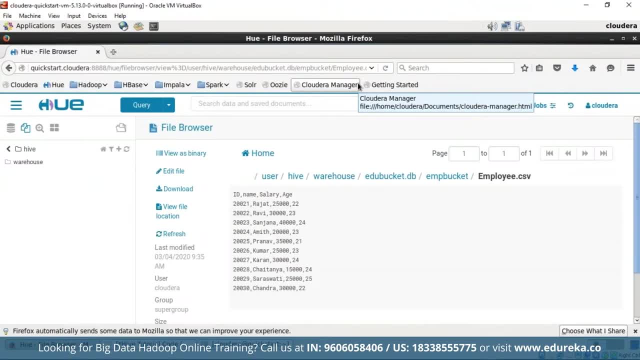 that are the tables, databases, partitions, bucketing, and after that we have also understood various operations that are the automatic operations, logical operations and functions that can be performed in hive, such as square root and summation, minimum, maximum, and after that other operations such as group by sort, by order by, and also the joints that are possible in 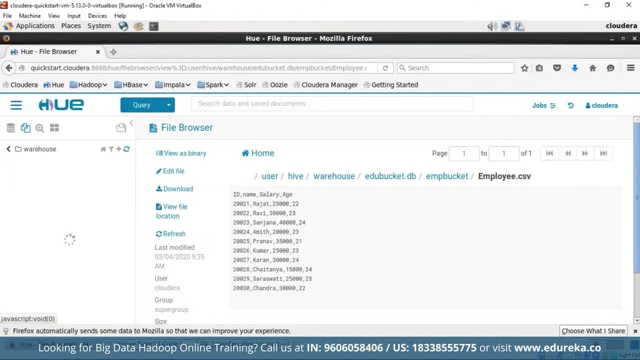 hive, which are in a joint left outer, right outer and full outer. So each and every operation that could be possibly executed in hive I've been displayed in this particular tutorial and everything is sorted here in the base of databases And you can get all the details about this and you'll also. 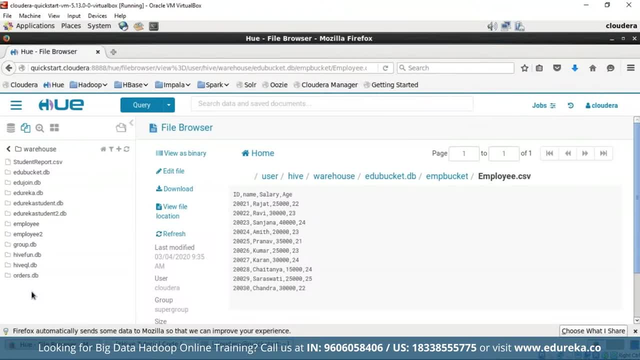 get the code that I have used in the description box below and you can try it out. And also, if you're looking for an online certification and training based on big data Hadoop, then you can check out the link in the description box below and during the 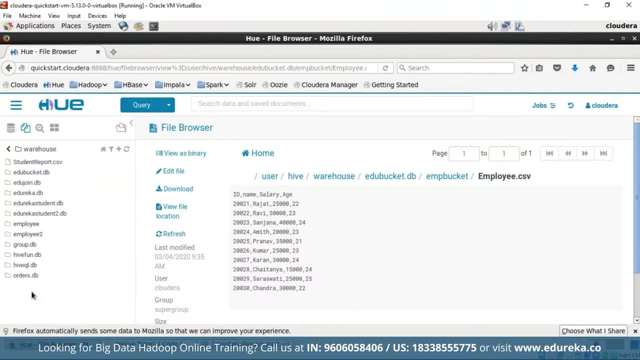 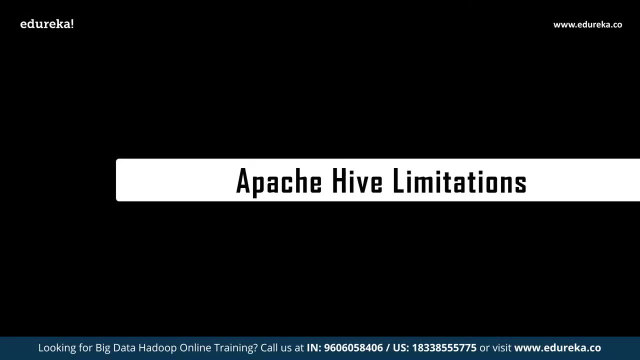 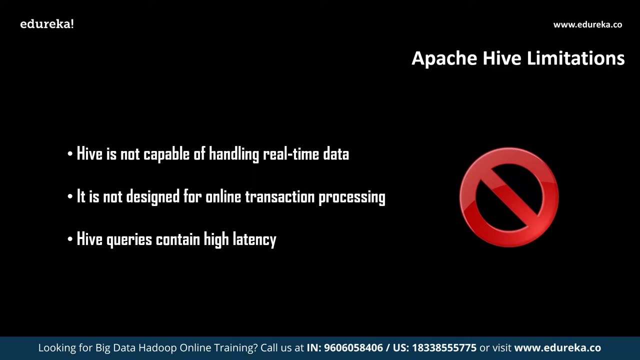 training you'll get to have real-time hands-on experience with real-time data. You learn a lot of things in the training and so far so good. Now we shall also discuss some of the limitations of hive. so Apache Hive limitations. So Hive is not capable of handling real-time data. 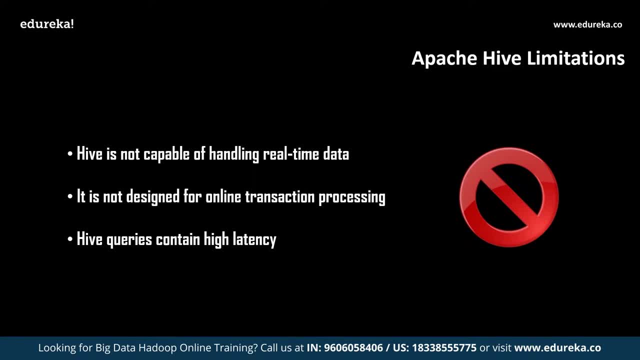 Hive is capable of batch processing. If you have to work with real-time data, then you have to go with real-time tools such as spark and Kafka, So it's like Hive will actually take in the data. For example, imagine you're working on Twitter and you have 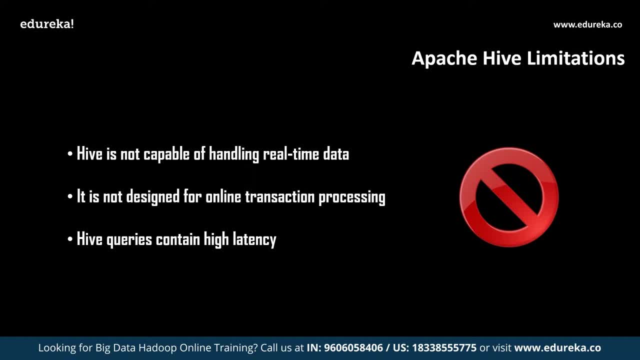 1 lakh comments on a particular post. So if you had to process those 1 lakh comments, you'll have to first load All those comments into Hive. then you need to process it. So while you're loading the data from Twitter to Hive, you may. 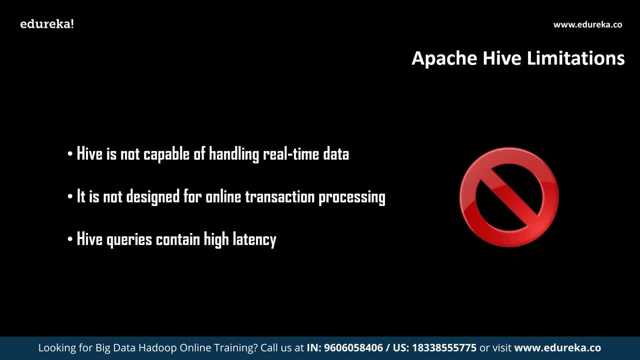 also get a few more comments that you will be missed out. So it's not preferable for real-time Hive is preferable for only batch more processing. so, followed by that, It is not designed for online transaction processing. So online transaction processing is something which only 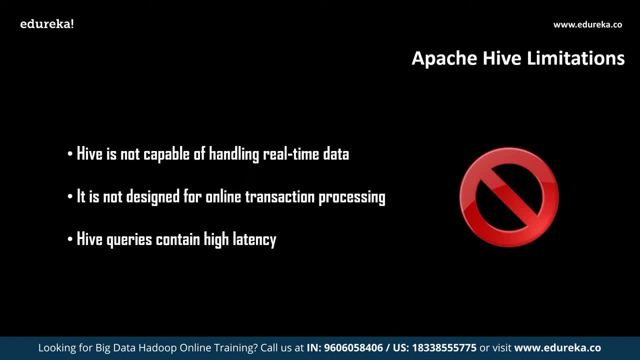 works in real time, So Hive cannot support real-time processing. So, last but not the least, high queries contain high latency. Yeah, Hive queries take a longer time to process. as you have seen, I have taken a smaller CSV file and the time consumed to process such a small CSV file was taking so long. 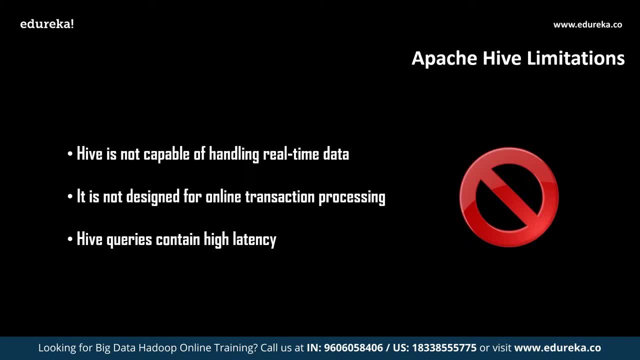 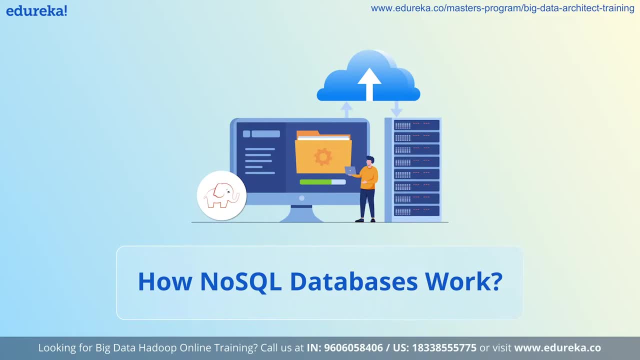 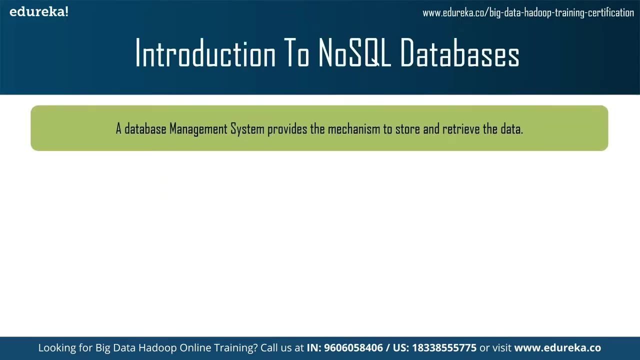 So, yeah, Hive queries contain high latency. So these are the few important noticeable limitations of Hive. Now let's just start with the data Basis. a database is a systematic collection of data, and the database management system supports storage and manipulation of data, which makes data management easy. 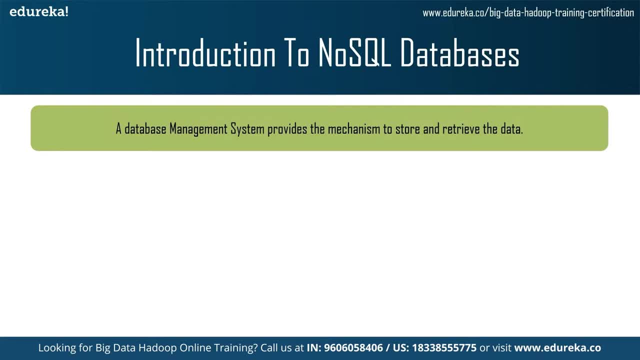 For example, an online telephone directory uses a database to store data of people, like phone numbers and other contact details that can be used by service provider to manage billing, client related issues and handle fall data, etc. So in simple words, We can say: a database management system provides the mechanism. 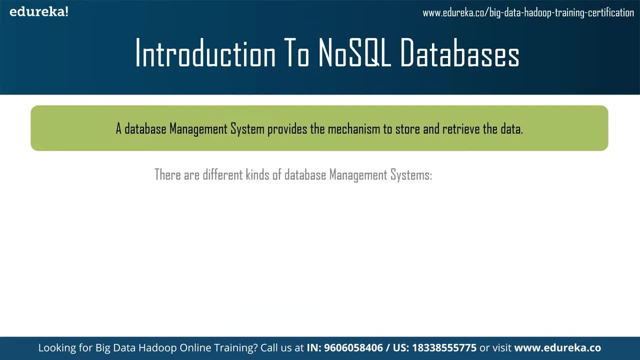 to store and retrieve the data. There are different kinds of database management systems present today, which are relational database management system, known as RDBMS, online analytical processing, known as OLAP, and no sequel, which is popularly known as not only sequel, no sequel refers. 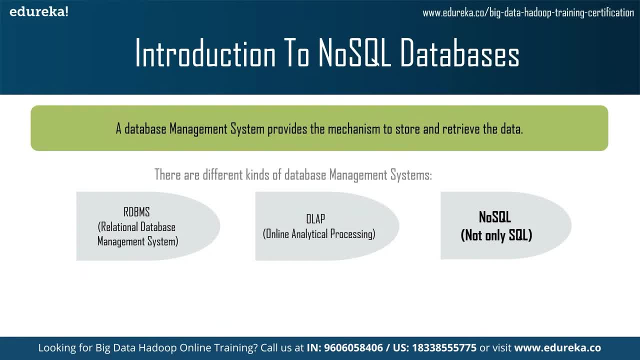 to all databases and data stores that are not based on the relational database management system System or RDBMS principles. No sequel is a new set of database that has emerged in the recent past as an alternative solution to relational databases. in 1998, called Strauss II introduced the term no sequel to name his file. 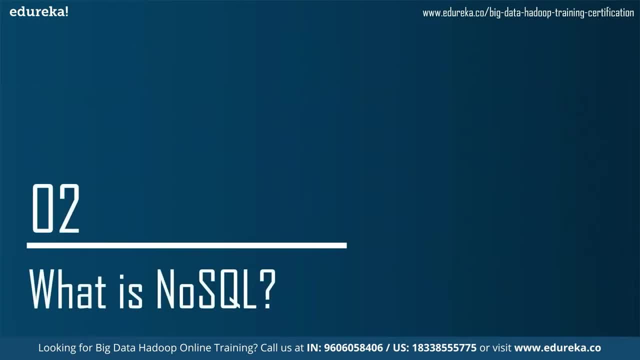 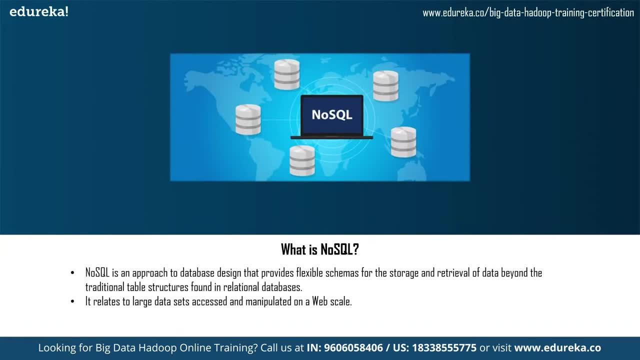 based database. So now we'll see what no sequel actually is. No sequel does not represent single product or technology, but it represents A group of products and various related data concepts for storage and management. No sequel is an approach to database management that can accommodate. 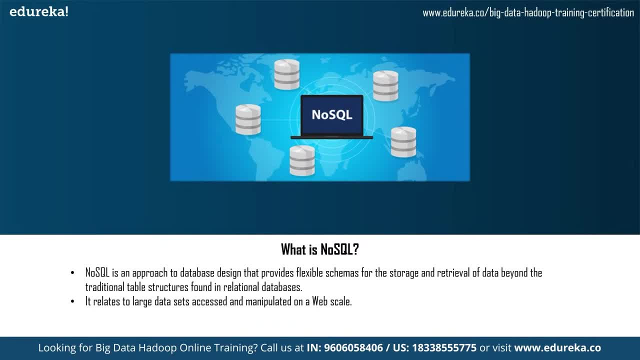 a wide variety of data models, including key value, document, column and graph formats. a no sequel database generally means that it is non-relational. it is distributed, flexible and scalable, so we can bind it up as an approach to database design that provides flexible schemas for the storage. 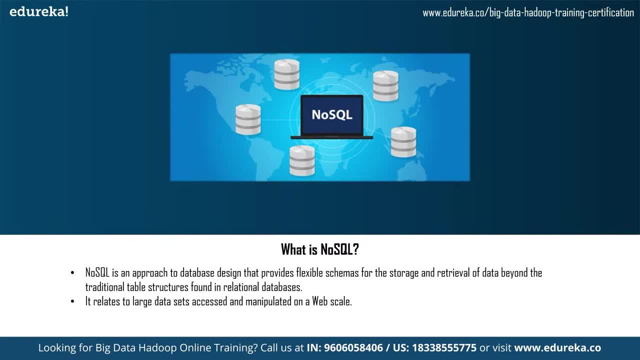 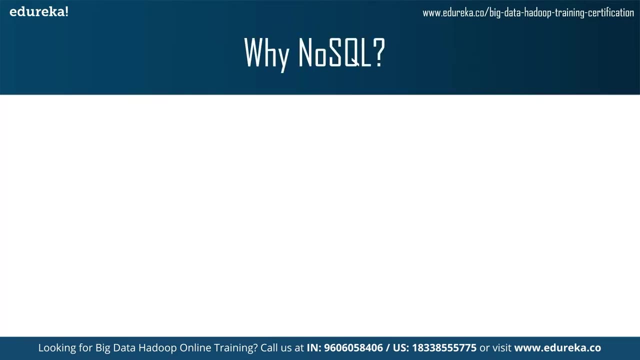 And retrieval of data beyond the traditional table structures found in relational databases. It relates to large data sets accessed and manipulated on a web scale. Now, when we have understood what is no sequel, the question arises is why to use no sequel? the concept of no sequel databases became popular. 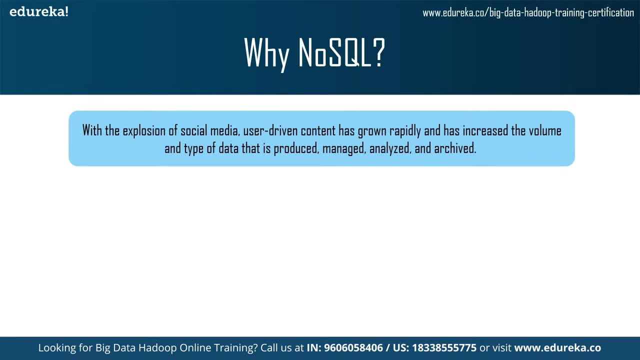 with internet Giants like Google, Facebook, Amazon, Etc. who deal with huge volumes of data, The system Response time becomes slow when you use our DMS for massive volumes of data. to resolve this problem, We could scale up our systems by upgrading our existing hardware. 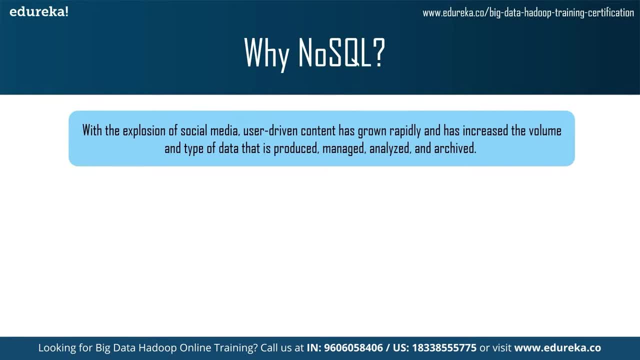 but this process is expensive, So the alternative for this issue is to distribute database load on multiple hosts whenever the load increases. This method is known as scaling out. no sequel databases are non-relational, So they scale out Better than relational databases, as they are designed with the web. 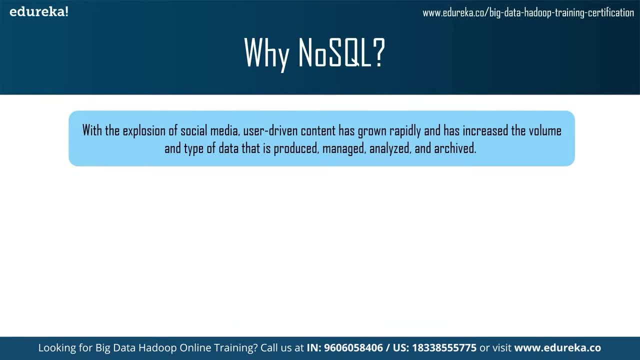 applications in mind. Now, the no sequel database is exactly the type of database that can handle all sorts of semi-structured data, unstructured data, rapidly changing data or big data. So we can say, to resolve the problems related to large volume and semi structured data. 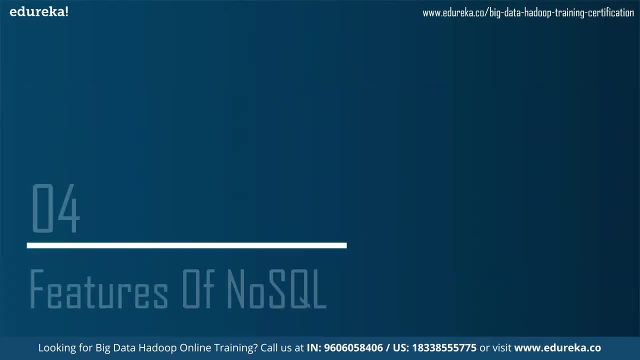 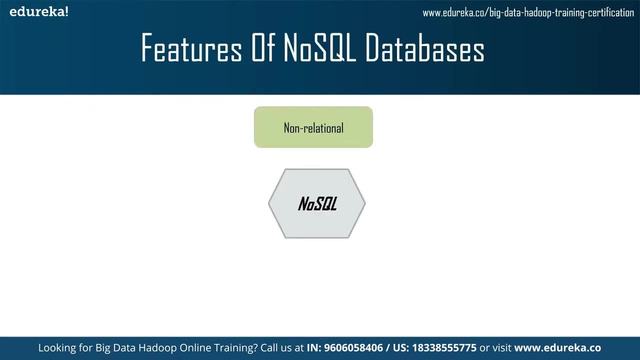 No sequel databases have emerged. now let's talk about the features of no sequel databases. No sequel databases never follow the relational model and don't provide tables with flat, fixed column records, So that doesn't require object oriented mapping and data normalization. Most of the no sequel databases are open source. multiple more sequel databases. 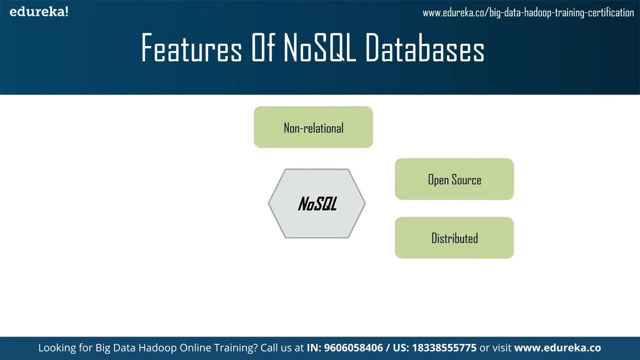 can be executed in a distributed fashion and they offer auto scaling and failover capabilities. They follow shared nothing architecture, which enables less coordination and higher distribution. No sequel databases are non-relational and offer heterogeneous structures of data in the same domain, which supports new generation web applications. 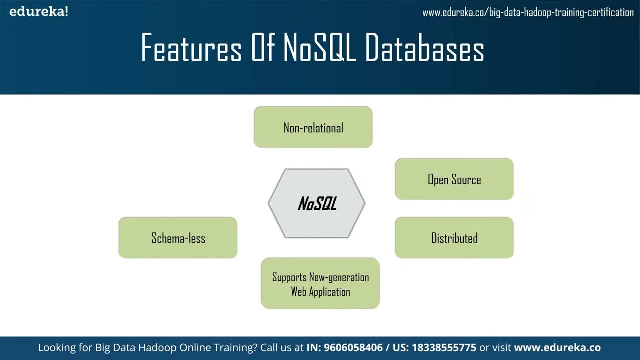 No sequel databases are either schema free or have relaxed schemas and do not require any sort of definition of the schema of the data. and no sequel databases offer easy-to-use interfaces for storage and query Data provided and APIs allow low-level data manipulation and selection methods. 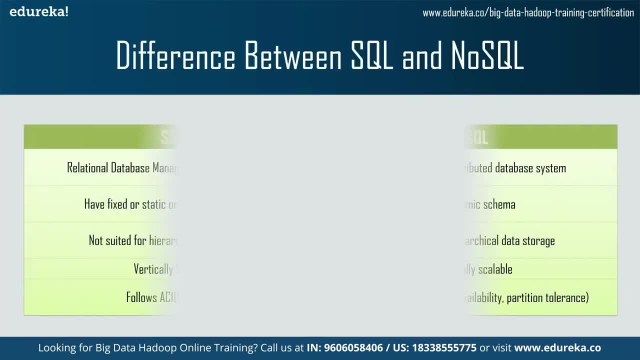 Now we can compare sequel and no sequel. on comparing sequel and no sequel, We can find the differences, like: sequel databases have fixed or static or predefined schema, while no sequel databases have dynamic schema. sequel databases are not suited for hierarchical data storage, while no sequel databases are best suited for hierarchical data storage, sequel databases are vertically. 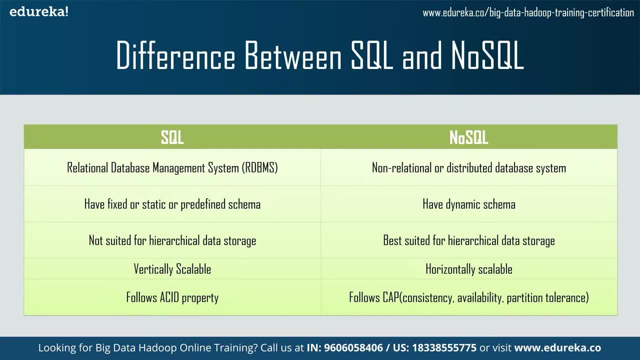 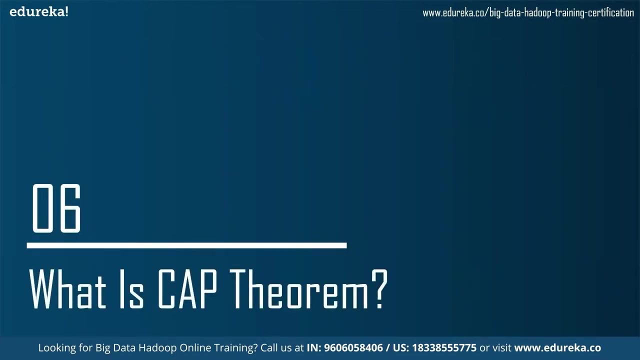 scalable, while no sequel databases are horizontally scalable as they are distributed. sequel databases follow acid property, That is atomicity, consistency, isolation and durability, while no sequel databases follow cap theorem, that is consistency, availability and partition tolerance. Now you must be wondering What is cap? 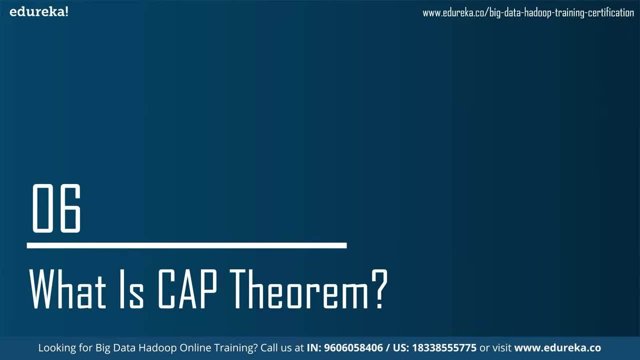 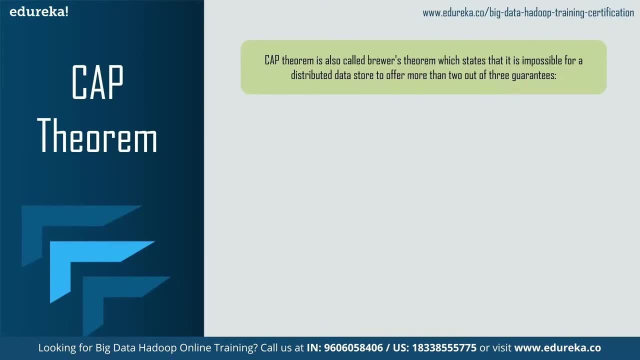 Theorem which plays an important role in no sequel databases- cap theorem- is also called Brewer's theorem and it states that it is impossible for a distributed data store to offer more than two out of three guarantees, which are consistency, availability and partition tolerance. So, basically, some no sequel databases offer consistency and partition. 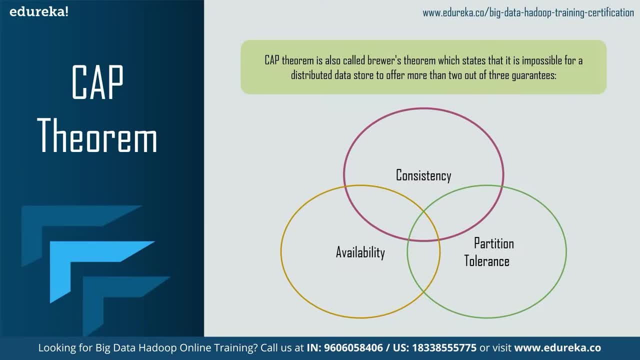 tolerance, while some offer availability and partition tolerance, But partition tolerance is common as no sequel databases are distributed in nature. based on the requirement, We can choose which no sequel database has to be used. different types of no sequel databases are available based on the data models. 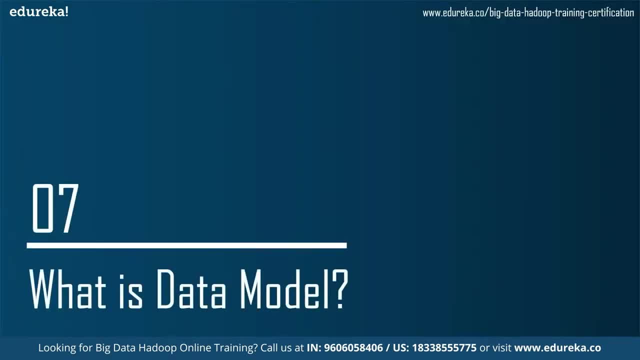 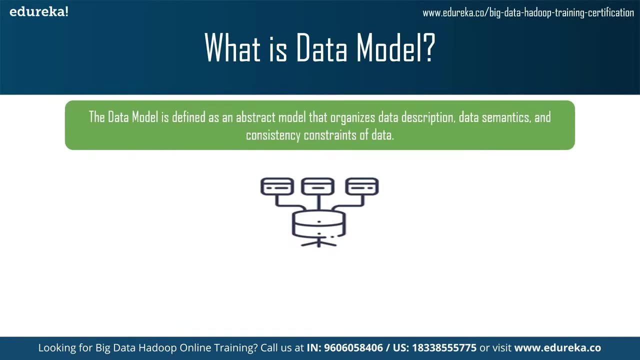 So, before talking about those, let's just understand what is data model. the data model is defined as an abstract model that organizes data, description, data semantics and consistency constraints of data. the data model emphasizes on what data is needed and how it should be organized, instead of what operations will be performed on data. 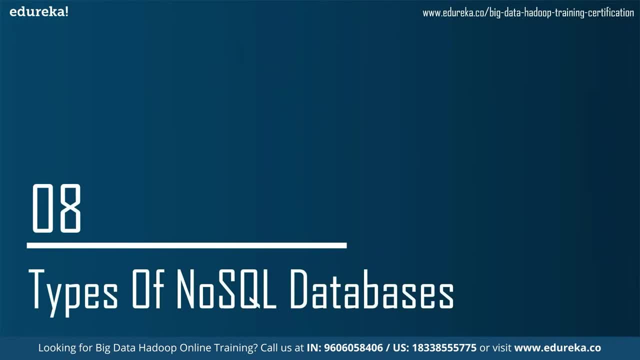 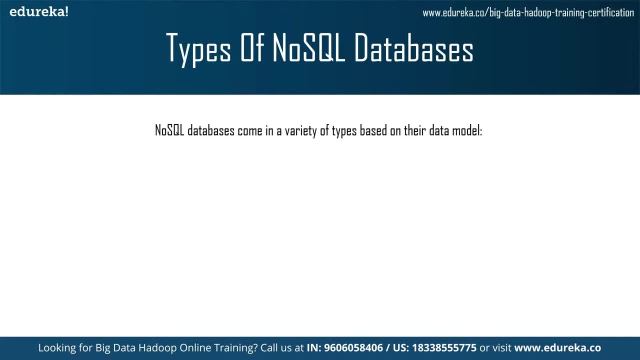 Now we can see the types of no sequel databases available, based on their data models. So no sequel databases come in a variety of types, which are key, value, pair based, graph based, column based and document based. Now we will see Each of these no sequel databases one by one. 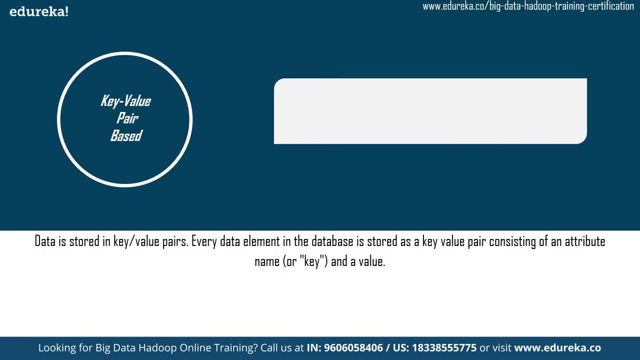 So let's start with key value pair based. no sequel databases in this. data is stored in key value pairs. each data element in the database is stored as a key value pair consisting of an attribute, name or key and a value. These databases are used to handle lots of data and heavy load. 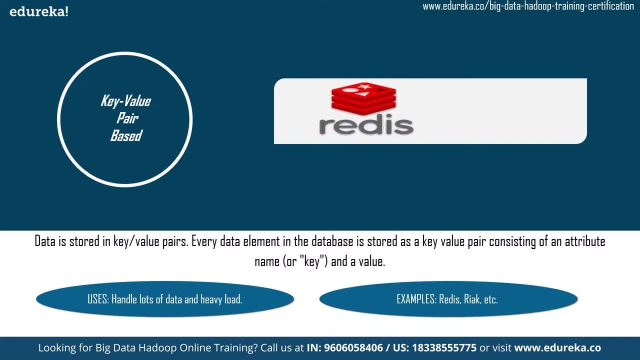 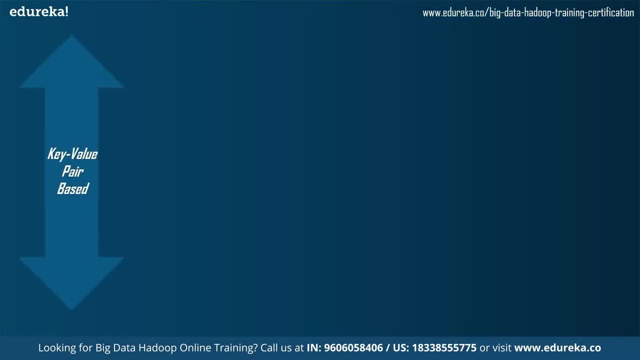 Some of key value pair based no sequel databases include Redis, react, Voldemort, etc. Now we will see a demo for key value pair based no sequel databases. data has to be stored as key value pairs, So here our key is name and value, for this key is Richard. 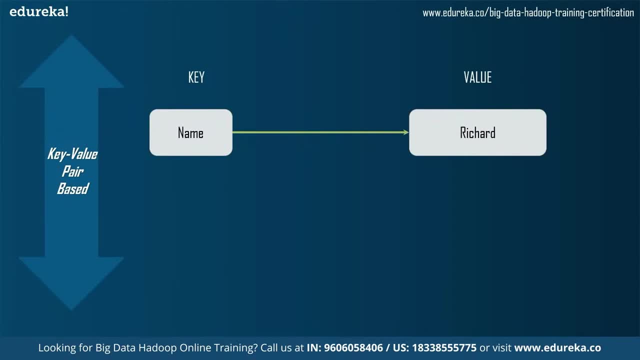 So it makes a pair of key and value. that is actually the data. Similarly, for dob key 2nd August 1988 is the value and for address key 32 W, NYC is the value. now, moving on, Let's understand column oriented. 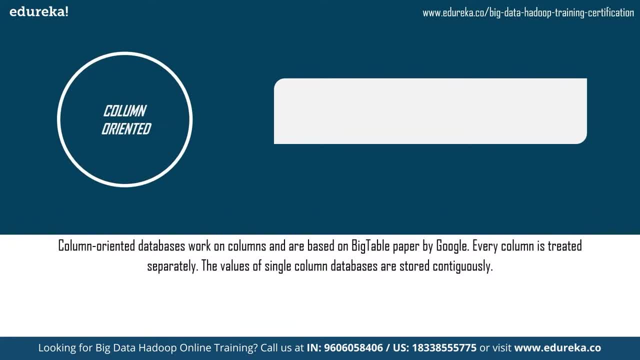 No sequel databases. column oriented databases work on columns where each column is treated separately and the values of single column databases are stored continuously. These databases are used to manage data warehouses, business intelligence, CRM, library card catalogs, etc. Some of column oriented no sequel databases include HBase Cassandra. 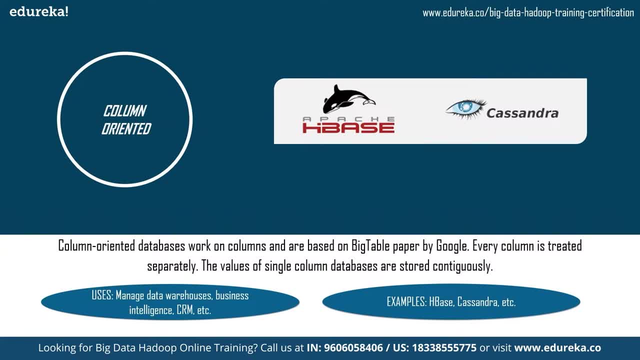 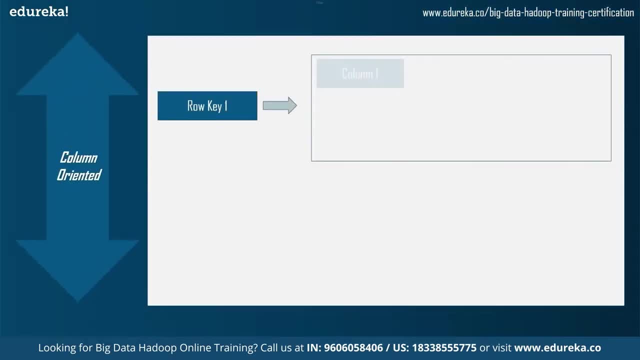 etc. And these databases are based on Big table paper by Google. Now let's understand this with a demo. We have row keys associated with the columns. So here we have a row key 1 associated to column 1, which has value 1, and the column 2, which has value. 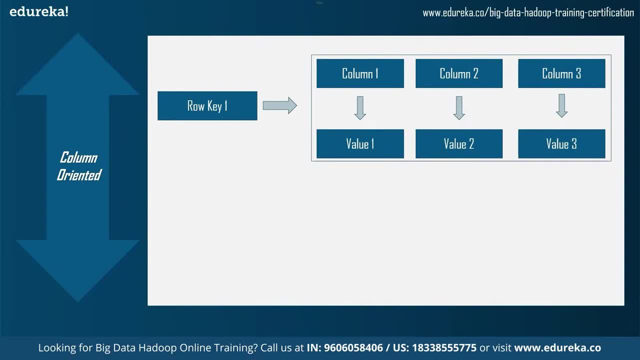 2 and column 3, which has value 3. we can see key 1 is associated to 3 columns, where each column has some value. Similarly, row key 2 is associated to column 1 and column 2, which have values Value 1 and value 2 respectively. here, row keys are for grouping the columns. 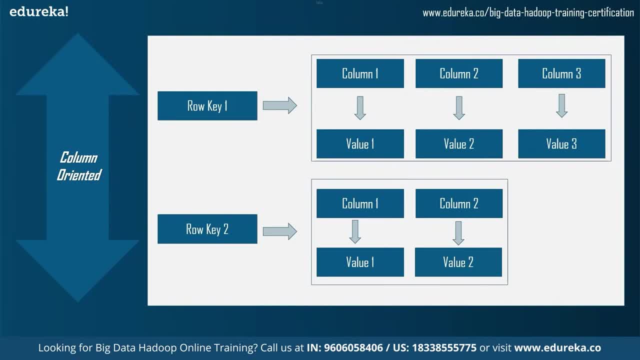 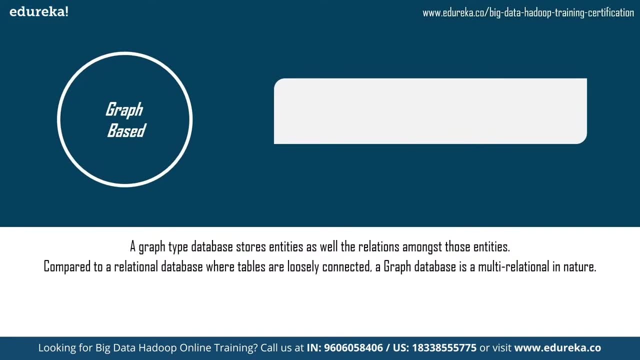 but actual data is stored in the columns. now, moving on, Let's understand the graph based databases, and graph type database stores entities as well as the relations amongst those entities, the entities stored as a node with the relationship as edges, and edge gives a relationship between nodes and every node and edge have a unique identifier. 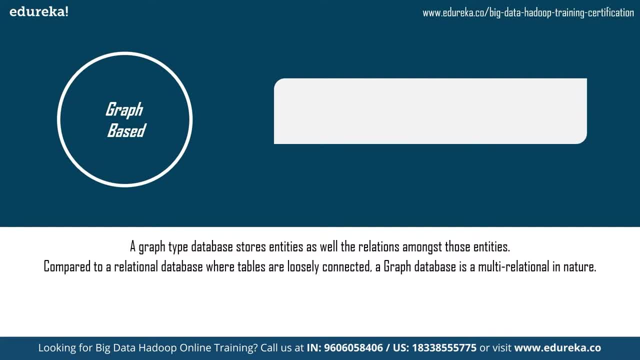 A graph database is a schema, less yet multi-relational in nature. These databases are used to manage social networks, logistics and spatial data. Some of graph based no sequel databases include Neo4j, Orient DB, etc. Now let's understand graph based databases with the demo. 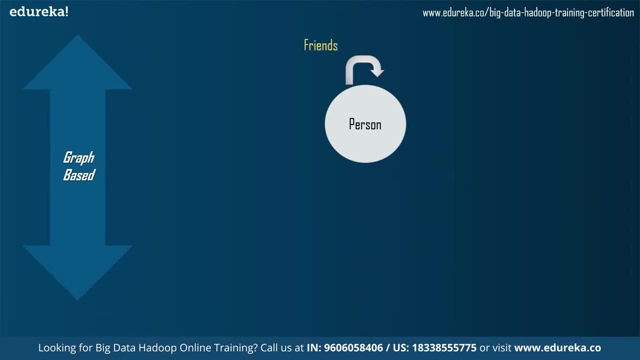 We have a person as node who has a relationship with another person as friend and he has other relationships with city that he lives in. a city Whose properties could be address as a node can have multiple relationships and properties. here The person has one more relationship with the city that he likes. the city and properties include the ratings. 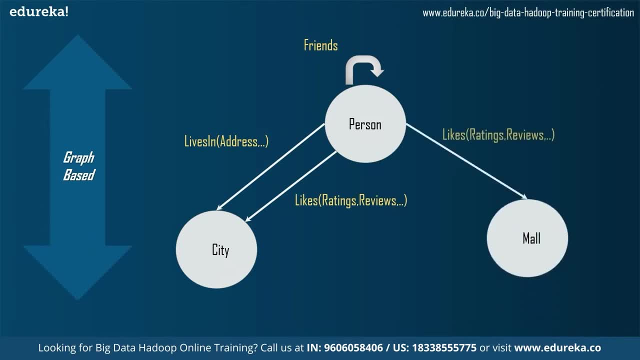 and reviews. Similarly, the person likes a mall based on the properties, like ratings and reviews, and the node mall has a relationship with the city that it is located in, a city and properties include address. so we can infer that in graph based databases The data is stored as nodes, relationships and properties, where properties can be of nodes as well as of relationships. 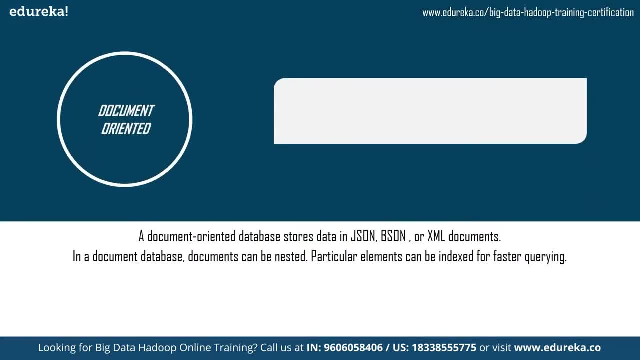 now moving further. Let's understand document oriented, no sequel databases. document database stores data in Jason Beeson and XML documents in a document database. documents can be nested and particular elements can be indexed for faster querying. document databases Make it easier for developers to store and query data in a database by using the same document model format. 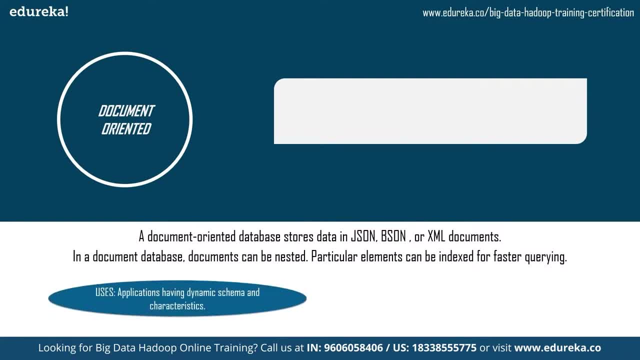 they use in their application code. These databases are used for the applications having dynamic schema and characteristics. some of document oriented no sequel databases include MongoDB, couch base, Etc, and MongoDB is the most popular database in no sequel databases. Now let's understand this with the demo. 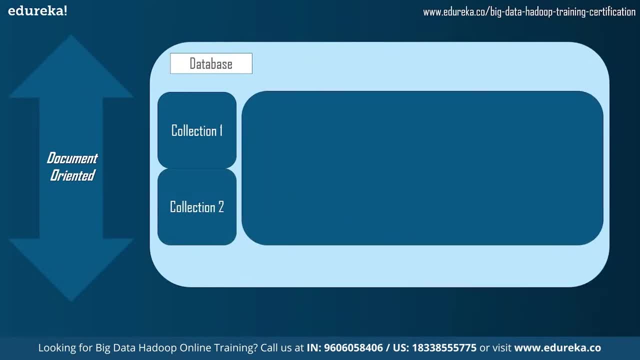 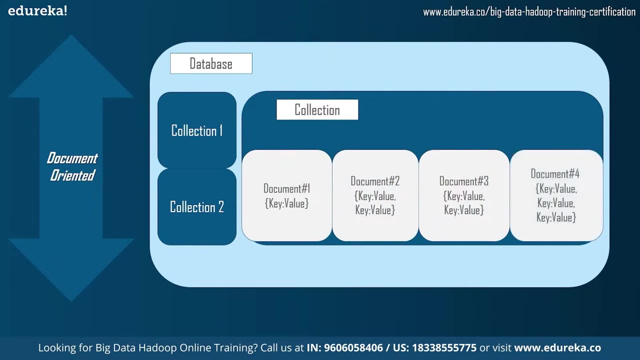 So we have a particular database which can have multiple collections. here We have collection 1 and collection 2.. Let's see how collection is made. each collection can have multiple documents with different schemas, as it has dynamic schema. So here we have document 1 with V 1 key value pair, then document 2 with 2 key value pairs, document 3 again with 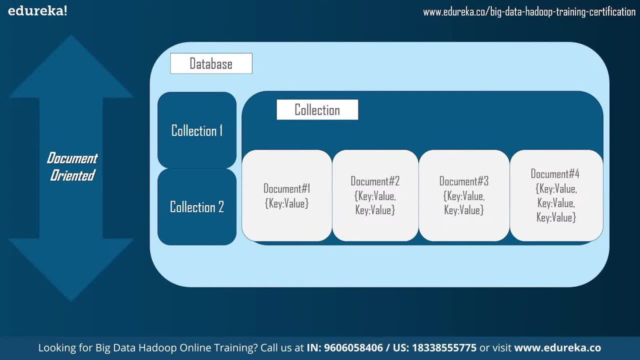 2 key value pairs And finally document 4 with 3 key value pairs. These key value pairs can be of any type, like string numbers, even another document as well. Basically, document oriented databases are hierarchical version of key value based databases. So with this we have covered all the four kinds of no sequel databases based on their data models. 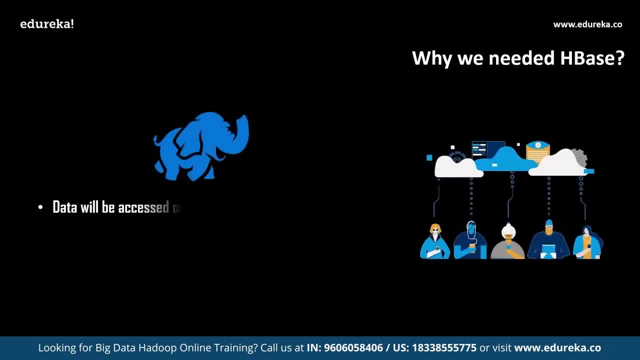 Why we needed edge base. We all know that the traditional data storage system, What we had was our DBMS, that is, relational database management system for storing data and maintaining the related problems. but slowly we face the rise of big data. So, since the rise of big data, 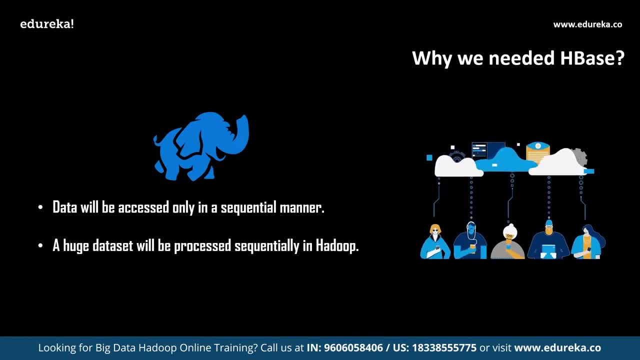 we have come across new solutions and Hadoop was one amongst them and we started using Hadoop. But when we start huge amount of big data inside Hadoop and try to fetch few records from Hadoop, It was a major issue because you had to scan the entire Hadoop distributed file system to fetch for a smallest record. 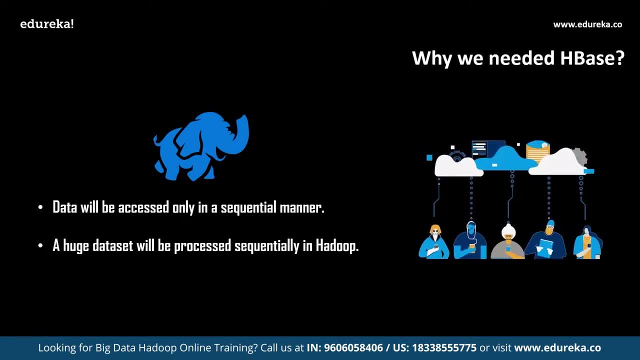 So this was the limitation of Hadoop: It did not provide random access to databases, So this problem was solved using H base. So H base is similar to database management systems, but it provides us the capability to access data in a random way. 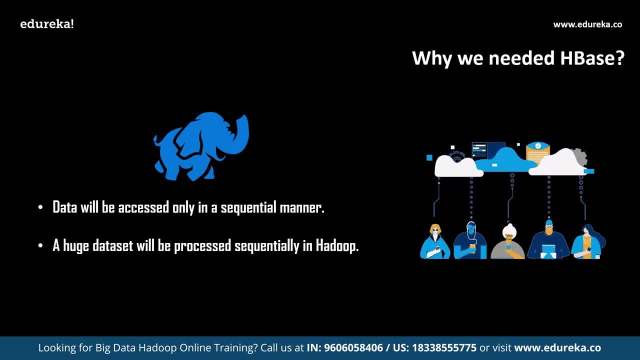 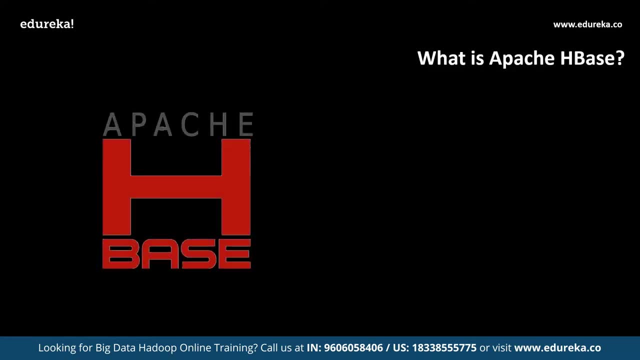 So this was the limitation of Hadoop and this is how H base solved it. Now, moving ahead, We shall understand the basic definition of H base. H base is a distributed column-oriented database built on top of Hadoop file system. It is an open-source project and horizontally scalable. H base is a data model. 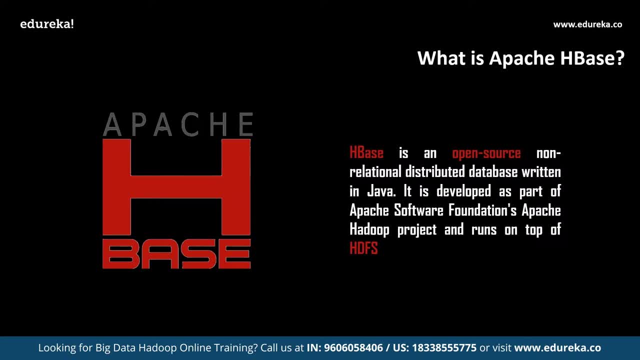 that is similar to Google's big data table, designed to provide quick, random access to huge amounts of structured data. It leverages the fault tolerance provided by Hadoop file system and it is a part of Hadoop ecosystem that provides random, real-time read and write access to the data in Hadoop file system. 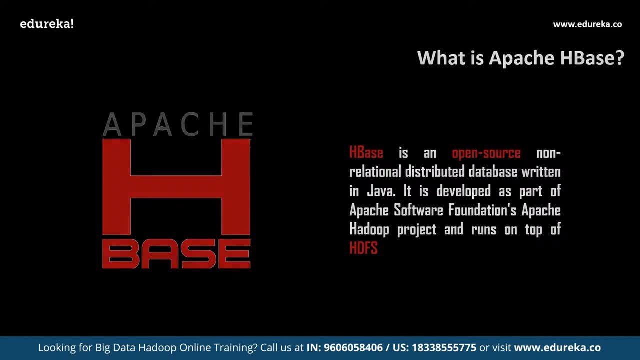 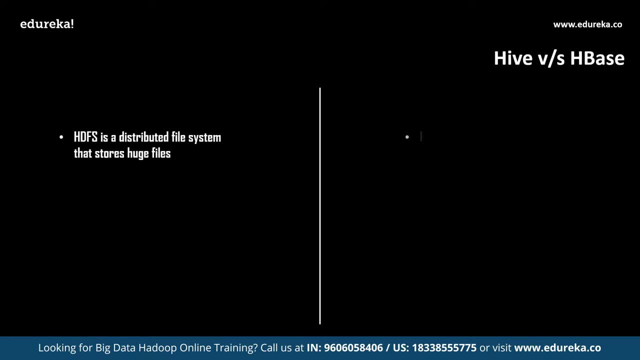 So now, this was the basic definition of H. Now we will move ahead and understand the basic differences between H base and HDFS. H base is built on top of Hadoop HDFS, Whereas HDFS is one of the major component of Hadoop. 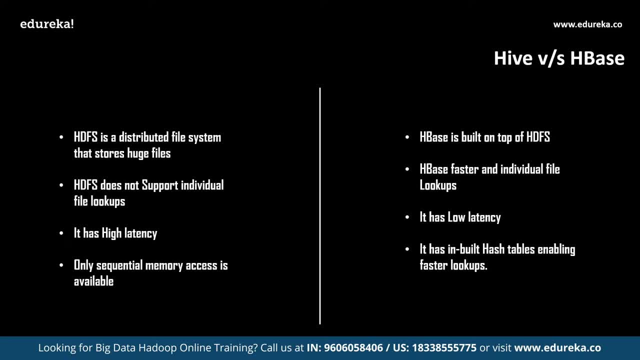 and it is built in a way to store the files in a distributed manner, followed by the first difference. H base provides fast lookups for larger tables And when we come into HDFS we all discuss this limitation. HDFS does not provide random access to the data. 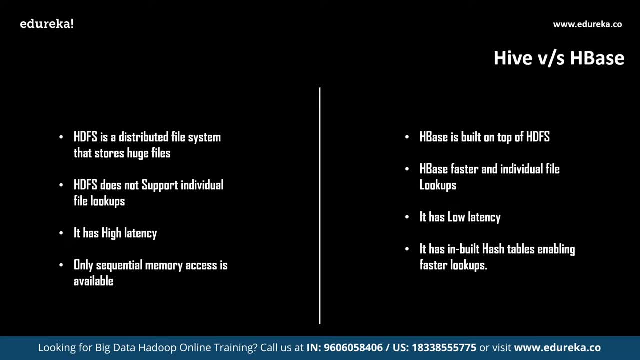 and it does not support fast individual record lookups. followed by the second difference: H base provides low latency to single rows from billions of records. This is because H base is capable to provide us random access to the data, That is, we can randomly read the data from any location. 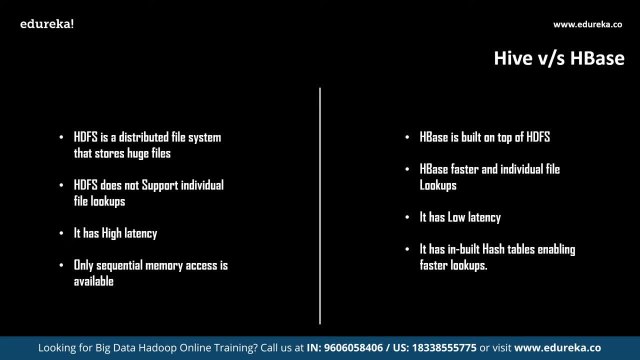 as well as write it. followed by H base. HDFS provides high latency processing and it cannot process random access of data and it is not capable to provide as random access to the data as H base does. followed by the third difference. The fourth difference is H base internally uses hash tables. 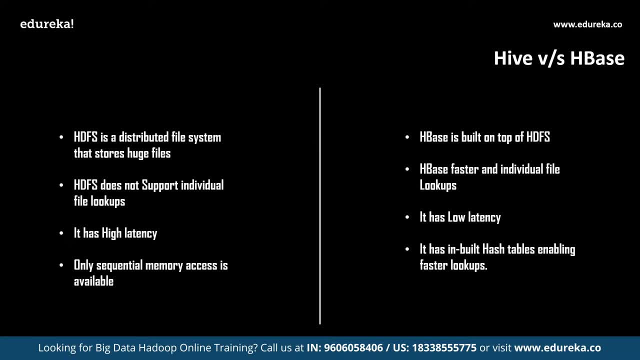 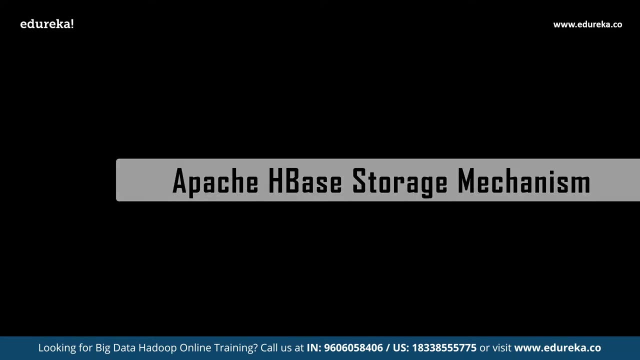 and provides random access, and it stores data in indexed HDFS files for faster lookups, Whereas HDFS provides only sequential access of data. So these are the major differences between HDFS and H base. followed by the differences, We shall move into the storage mechanism in H base: H base. 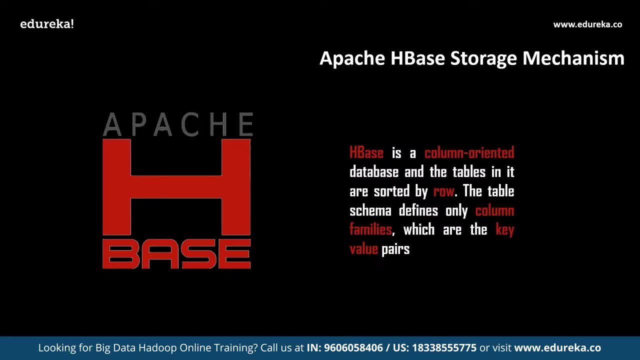 is a column oriented database and the tables in it are sorted by true. the table schema defines Only column families, which are the key value pairs. the table have multiple column families and each column family can have any number of columns. subsequent columns values are stored continuously on the disk. 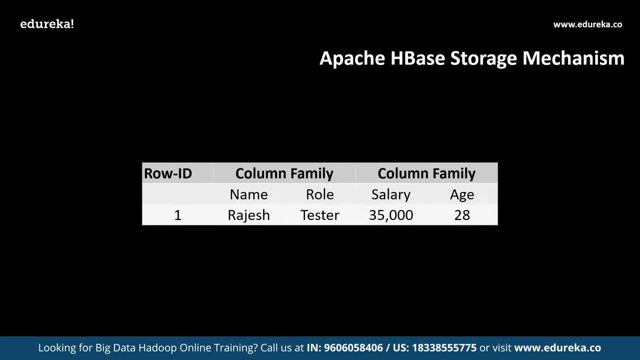 each cell value of the table has a timestamp and, in short, in an edge space, table is a collection of rows. row is a collection of column families. column family is a collection of columns and column is a collection of key value pairs. The following table gives you the brief description. 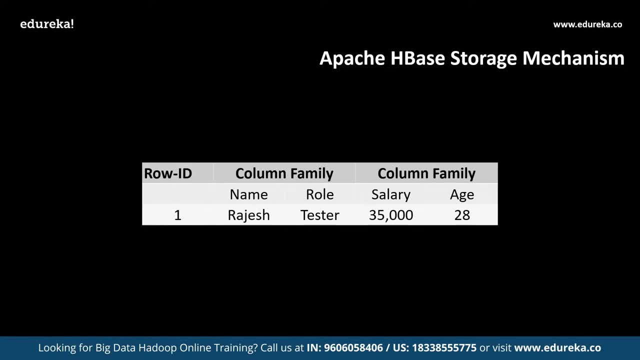 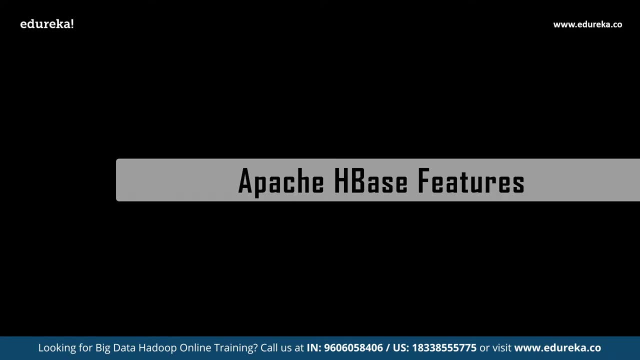 of the storage mechanism, followed in H base, followed by the storage mechanism. Now we shall enter into the next stage, where we will understand the features of H base. The first feature is: H base is linearly scalable because H base is built on top of HDFS. 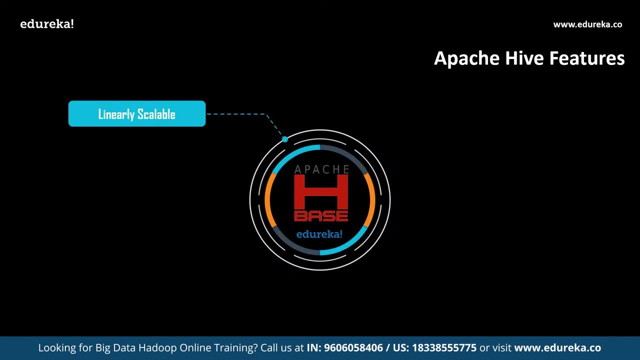 and HDFS provides the horizontal scalability, and this similar feature is also adopted by H base, followed by the first feature. The second important feature is that H base has automatic failure support. this automatic failure support provides as default tolerance feature of HDFS, followed by the second feature. 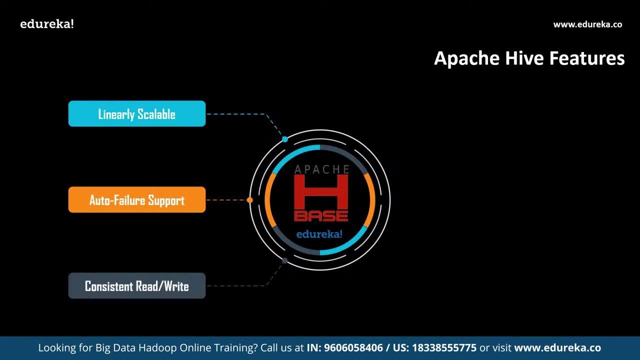 The third feature is HDFS provides consistent read and write. this important feature provides as the random access of reading and writing data. followed by the third feature, We have the fourth feature that says HDFS integrates with Hadoop and both as a source and destination followed. 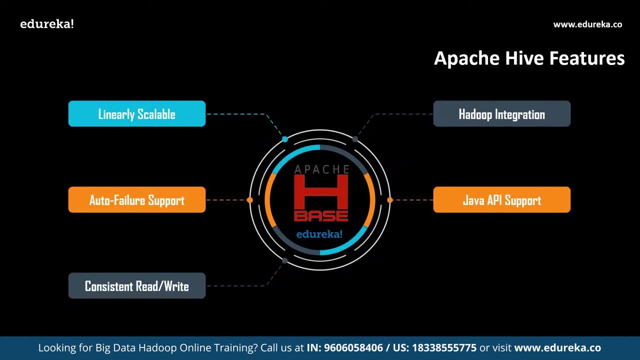 by the fourth feature. The fifth feature is that it is easy for Java API for client. and the last and important feature is that H base provides data replication across all the clusters. So these are the important features of H base, followed by the important features. 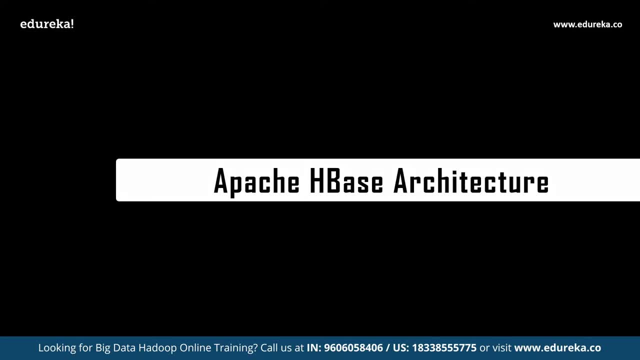 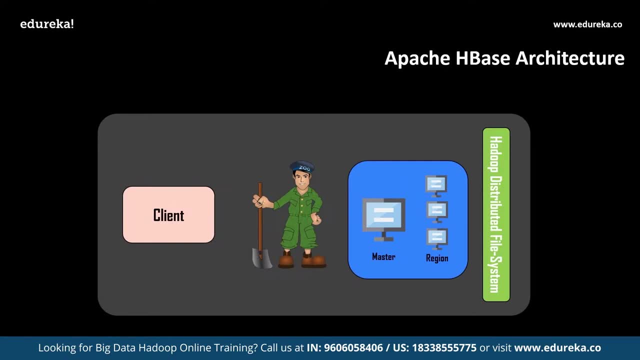 We shall move ahead into the next topic, which is the H base architecture. inside H base, tables are split into regions and are served by region servers. regions are vertically divided by column families into stores, and stores are saved as files in HDFS. The following image describes about the architecture. 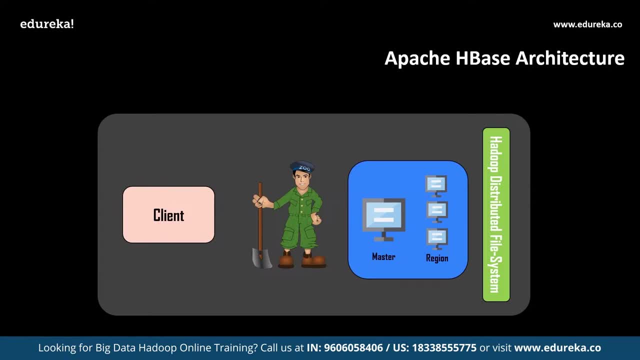 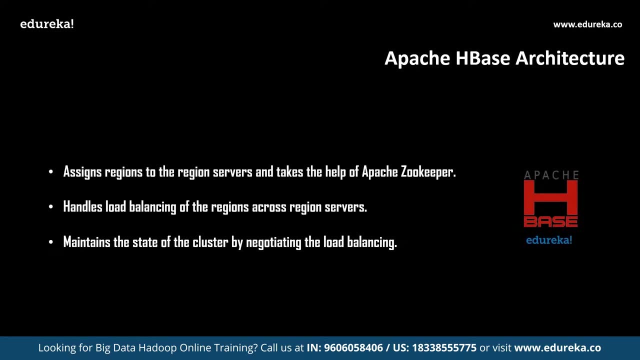 of H base. H base has three major components: The client library, a master server and region servers. which will understand master server first. master server assigns regions to the region servers and takes the help of Apache Zookeeper for this task. master server also handles load balancing of the regions across region servers. master. 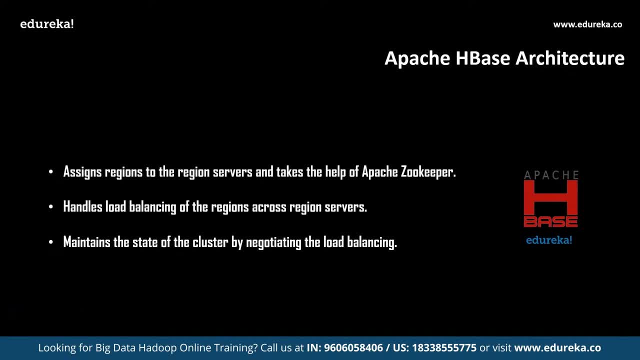 server is also responsible for maintaining state of the cluster by negotiating the load balancing followed by the master server. We shall discuss about the regions. regions are nothing but the tables that are split up and spread across the region servers. The region servers have regions that communicate. 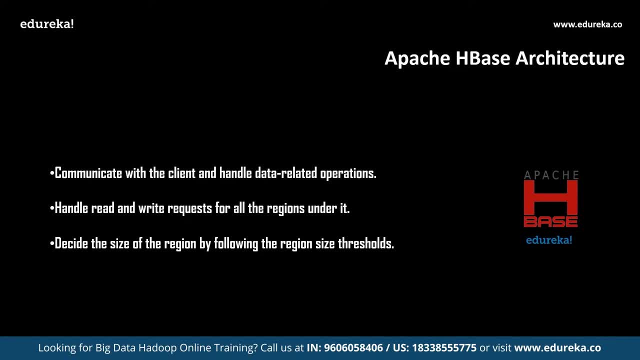 with the client and handle data related operations. They also handle, read and write request for all the regions under it. the region servers get to decide the size of the region by following the region size thresholds. Now we shall move into the next slide, where we will look. 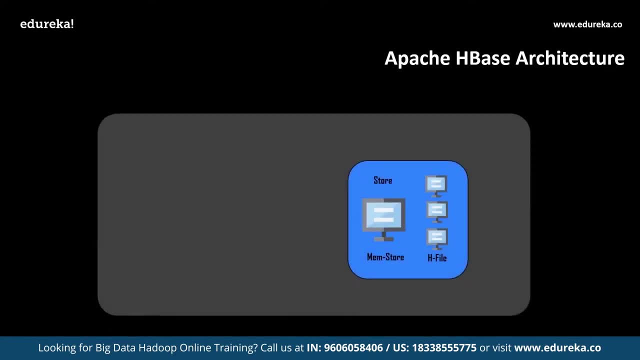 into regions and the following image describes how the region is split up. when we take a deeper look into the region server, It contains regions and stores the data as shown below. the store contains memory store and edge files. mem store is just like cache memory- anything that is entered. 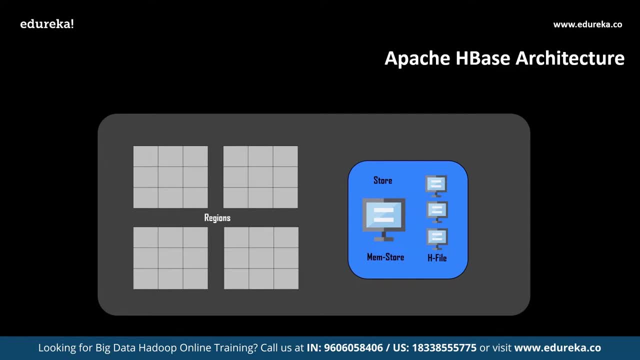 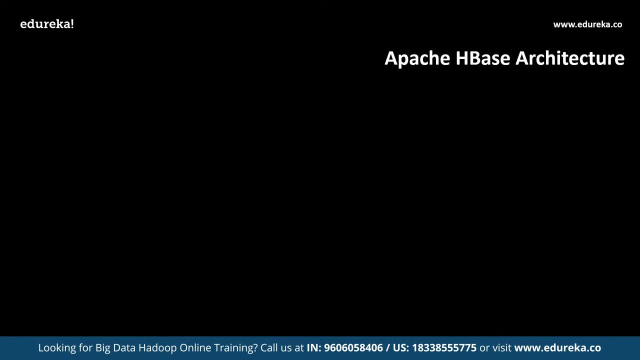 into the edge base is automatically stored initially. later The data is transferred and saved into edge files as blocks and the mem store is erased out, followed by the region server. We shall enter into the next important component, which is Zookeeper. Zookeeper is an open-source project. 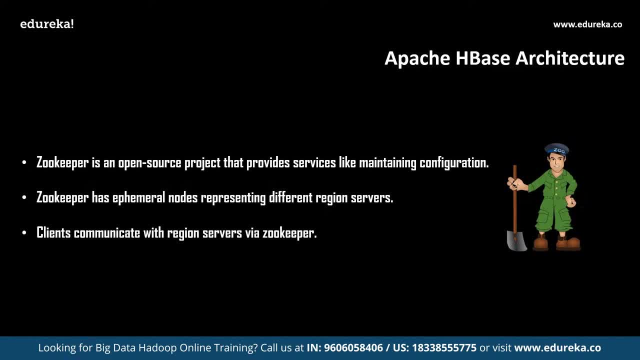 that provides service like maintaining configuration, information, naming, providing distributed synchronization and many more. Zookeeper has Imperial notes representing different region servers master service. use these notes to discover available servers. in addition to availability, the notes are also used to track server failures or network partitions. clients communicate with region servers via Zookeeper and pseudo. 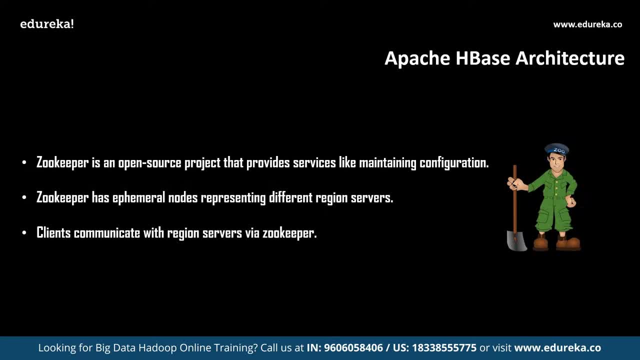 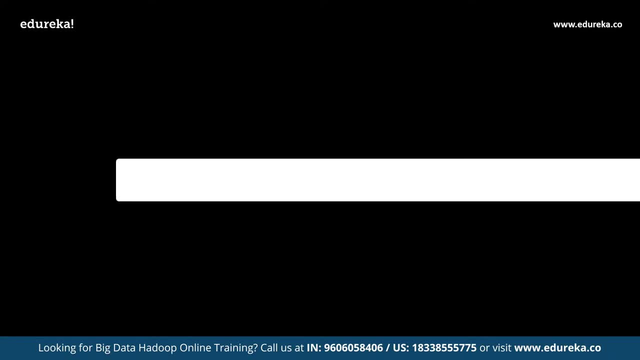 and standalone modes. edgebase itself will take care of Zookeeper. Now, This was the architecture of edge base. Now we shall move ahead into the next important stage of this particular tutorial, which is the edge base demo. So in this particular demo first, 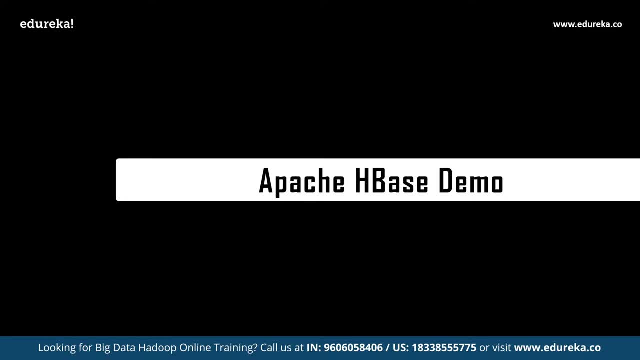 we will deal with installation of edge base into our local system That has Windows operating system. after the installation We shall start edge base in our local host and followed by that, and we shall open a terminal and execute the commands which are possible in edge base now without wasting much time. 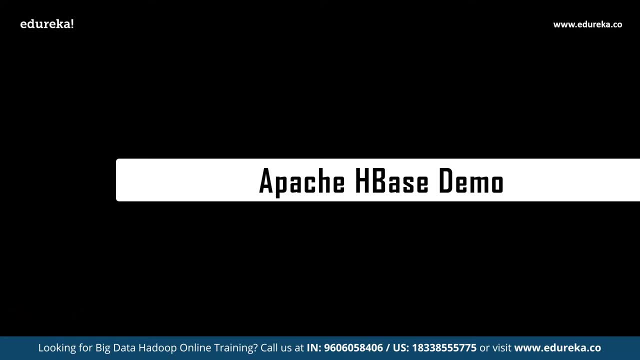 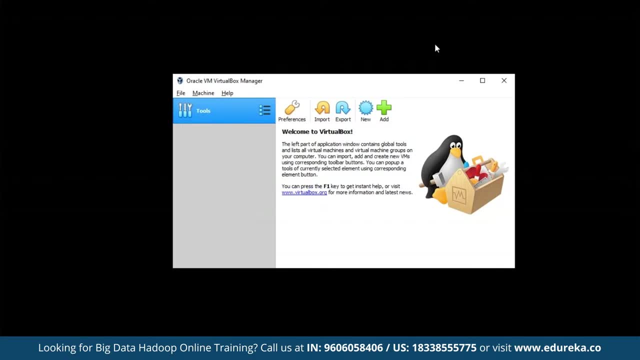 Let's start with the installation process. to install edge base into your local system, The easiest way is to have an Oracle virtual machine, So you have to download Oracle virtual machine and install into your local system once after you have downloaded and installed Oracle virtual machine. 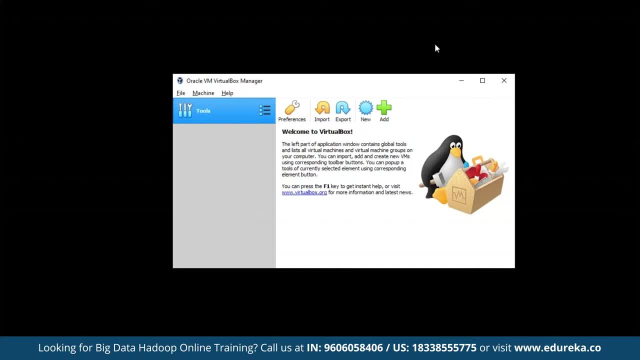 into your local system. The next date would be downloading quick start cloud era VM for your local system. Once after your download your cloud era quick start VM for your local system, you need to just import that using your Oracle virtual box. You have to select import. 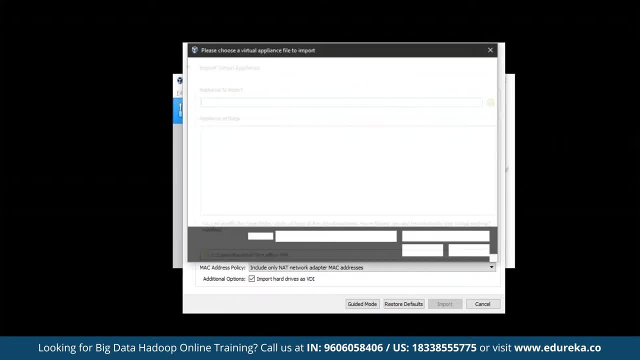 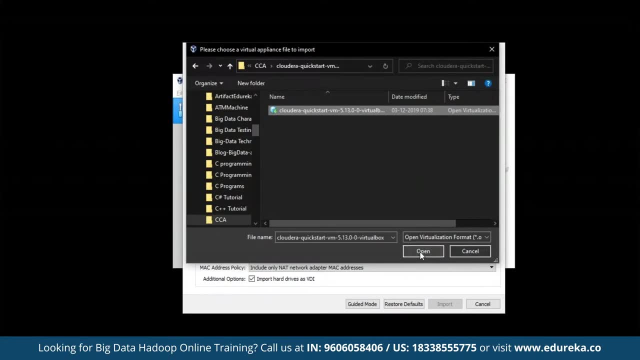 and you will be provided with a new dialog box where you have to provide the location of your cloud era quick start VM. So this is the location of my cloud era quick start VM in my local system, and then you have to select open and there you go. 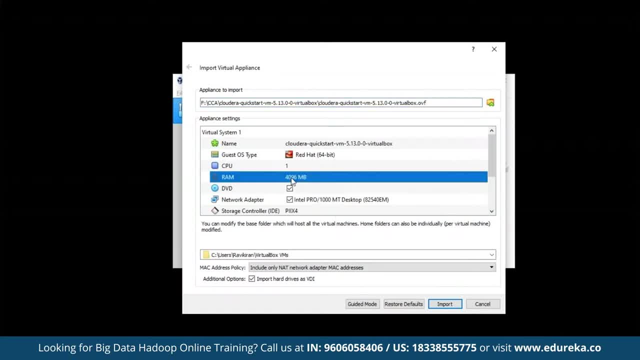 You can see that you have got a new dialog box here and remember to increase the RAM size to at least 8 GB for smooth functionality of cloud era. I have provided a random size of 9000 MB, which is just about 8 GB. 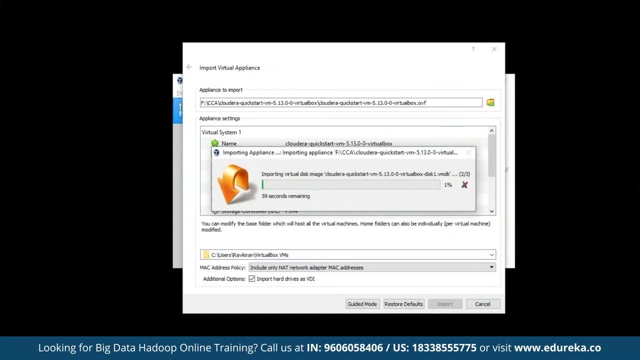 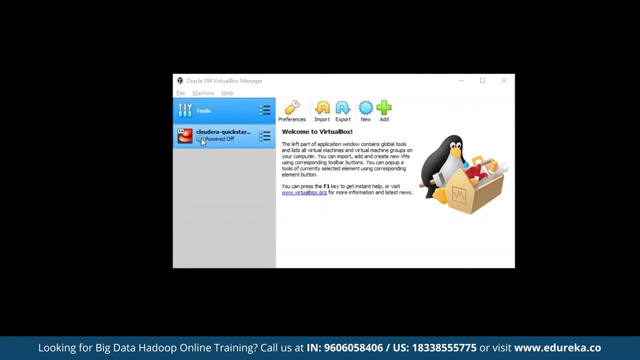 Now let's click import. and there you go- It is starting to import your cloud era quick start VM into Oracle virtual box. This might take a little time. There you go. The process has been successfully finished and you can see the cloud era quick start VM icon. 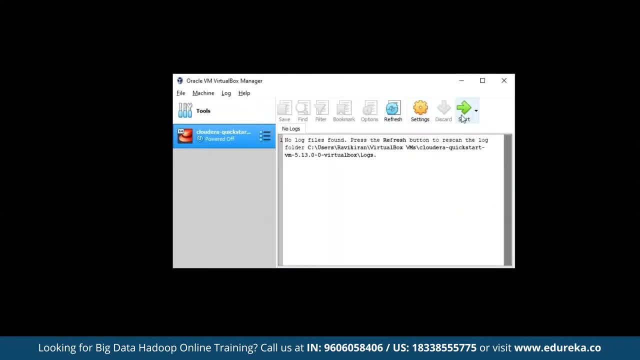 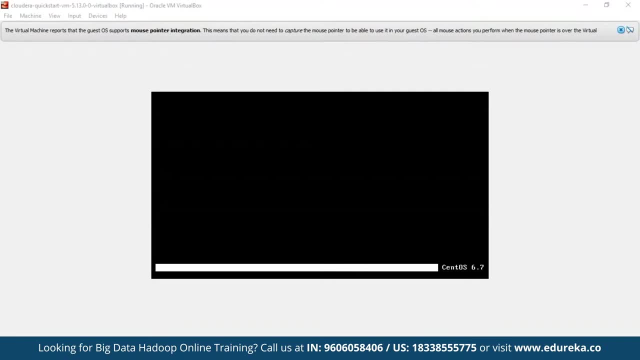 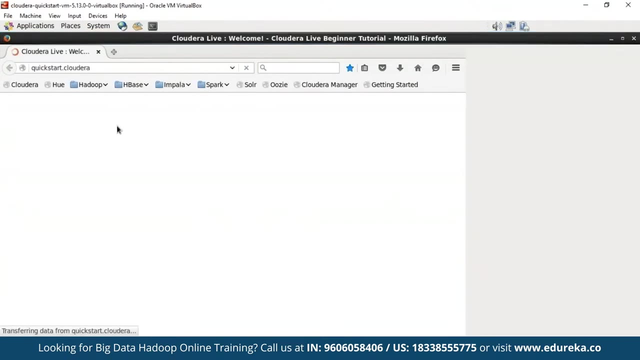 on your virtual box. All you need to do here Is to just click it and select start to start it. You can see a new window just got popped up. Now you can see the cloud arise been successfully started. Now let's open the browser and start a local host. 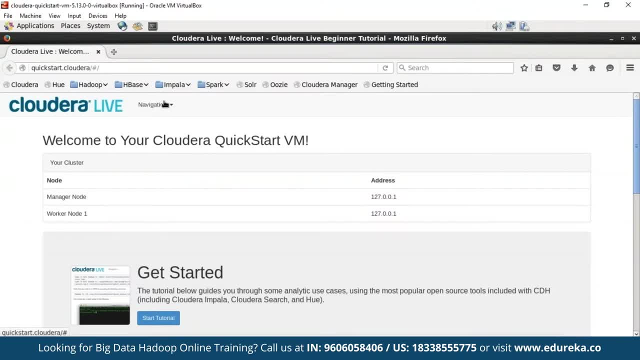 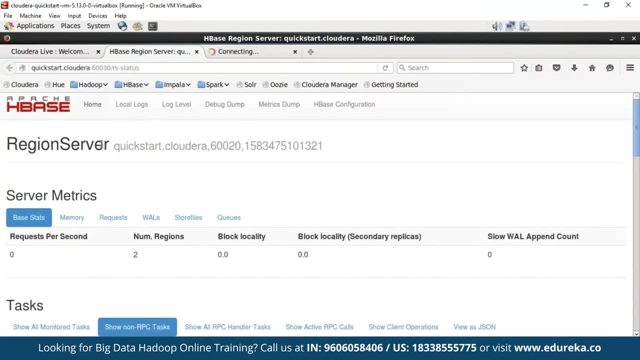 So you can see that cloud era is live now and the local host is also live. So this is our edge base. click on it and just open all tabs And there you go. You have the edge base region server here and edge base master service and everything is online. 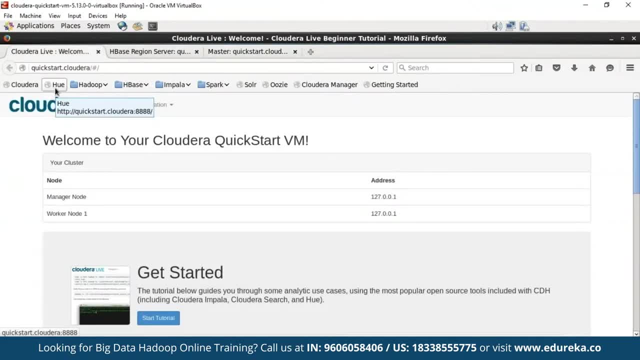 And remember one thing: in cloud era the username and password is cloud era by default. For example, if you want to start up hive or if you want to start up the hue, you will be redirected into a new web page where cloud era will ask you the username. 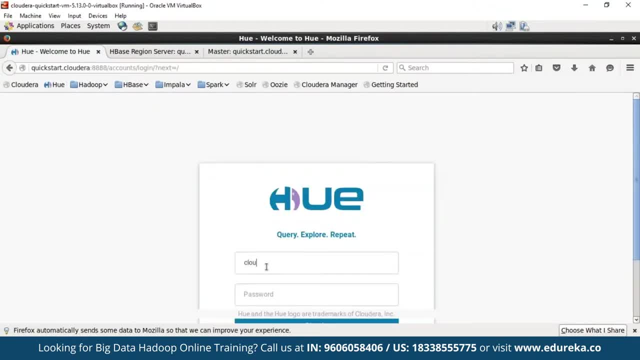 and password, which looks something like this: You just need to type in cloud era as the username and password as cloud era, And there you go, can just simply click on sign in and you will be logged in. So this is how it works now that we have started our edge base. 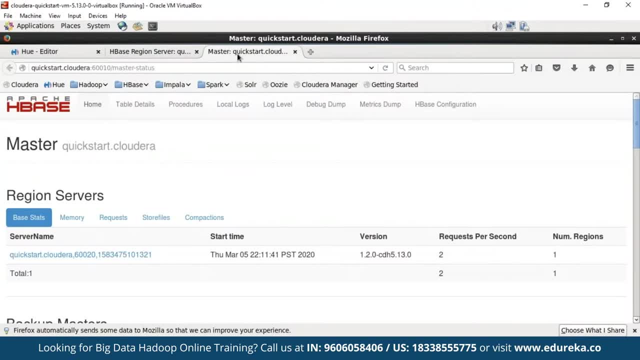 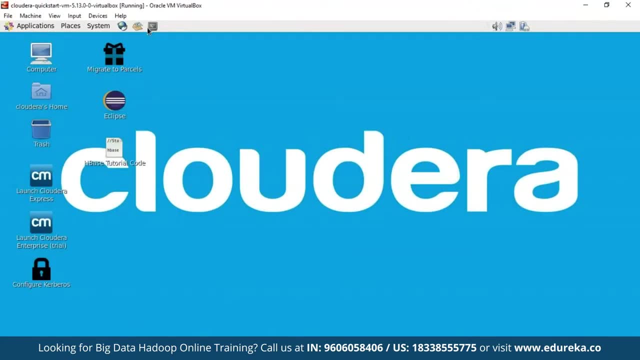 Let's quickly get started with our demo and execute some of the commands which are possible in edge base to have a briefer idea how edge base works. So now that everything is good to go, Let's start our terminal and you can quickly see that the terminal got started. 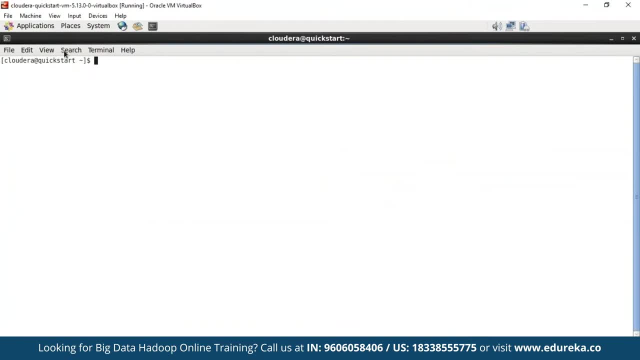 and let's increase the size of the font so that it's visible. Yeah, I think it's pretty good now. So to start edge base in cloud era's terminal, you need to type in edge base- shell and there you go. Yeah, we are successfully logged into edge base. 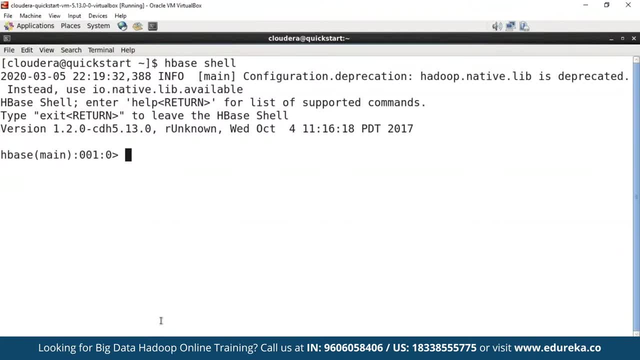 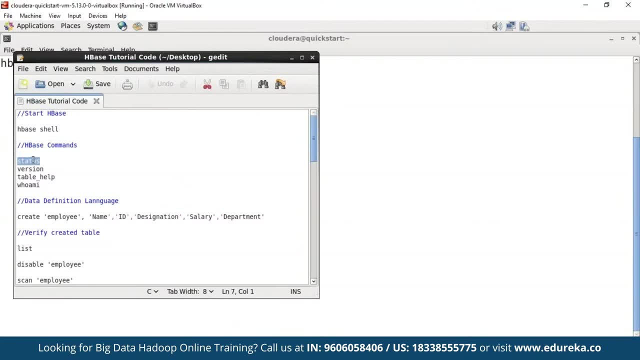 and the edge base got started here. I have created a document of the codes that I will be executing today to just save time. So, firstly, we will try to execute some of the basic commands in edge base, such as status, which will give us some important information about master. 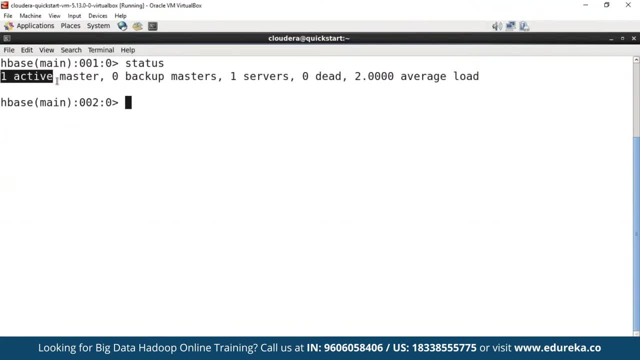 backup masters, region servers and many more. you can see that we have one active master and one server and, since it is a VM, we don't have any backup masters over here. So, followed by status, let's try to execute version command, where we'll come to know the version of edge base. 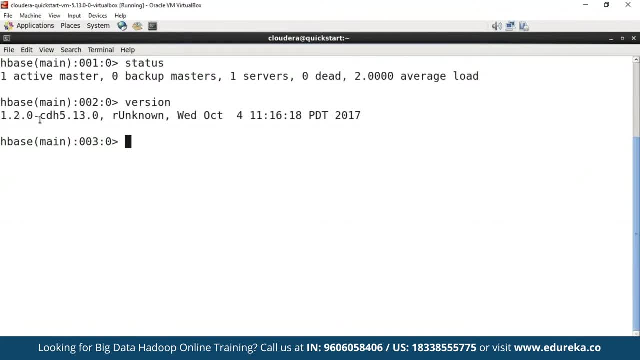 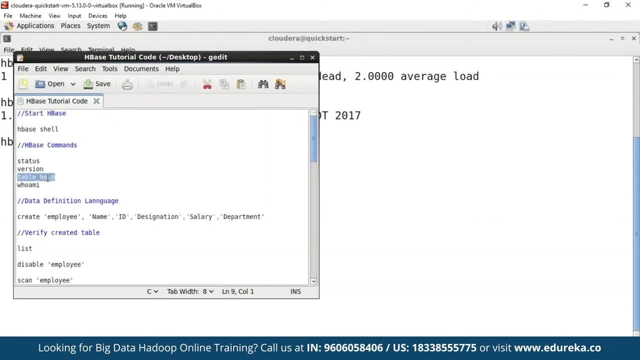 that we are using in our current system. So we are using 1.2.0 and the cloud error version is 5.1. 3.0, followed by the version command. Let's take in another command, which is the table help. 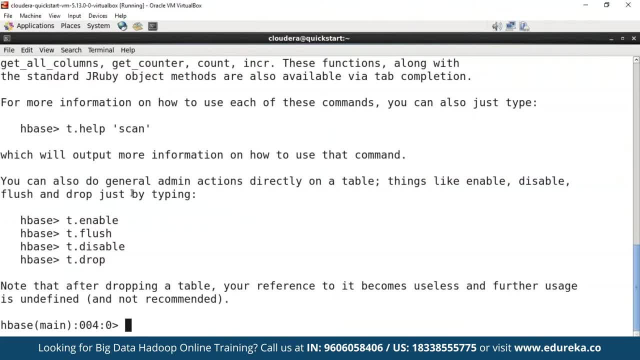 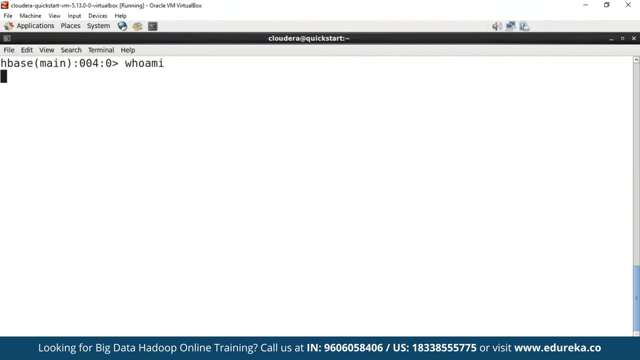 which will show us some various operations that we could perform using that our table enable, table disable and flush the table drop table, which are completely similar to an rdbms. Let's click in a control plus C to clear our screen. Now one last command would be who I am. 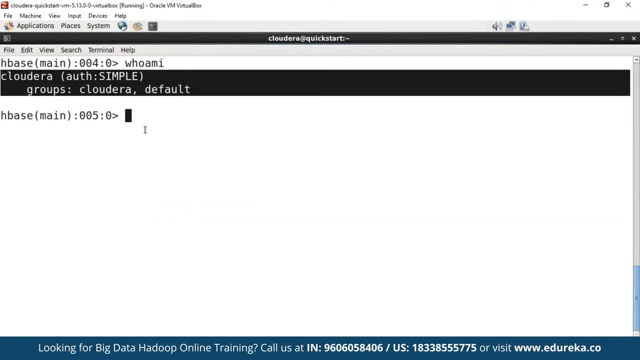 I, which will give you the important information related to your local system that has cloud error groups, cloud error default. There are many other commands in edge base. Now we have executed few of them. You can check out our article and edureka site to get more information related. 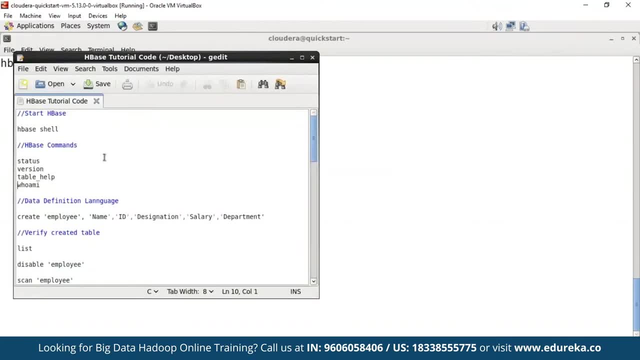 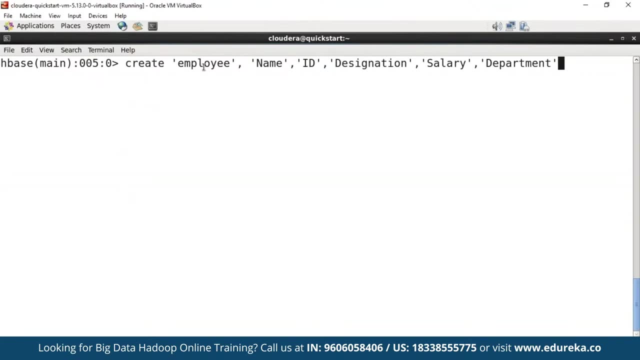 to the commands based on edge base. Now that we have executed some of the basic commands, let's move ahead and create a table. So here I am going to create a table by the name employee, and our table has been successfully created and the columns in my particular table are name. 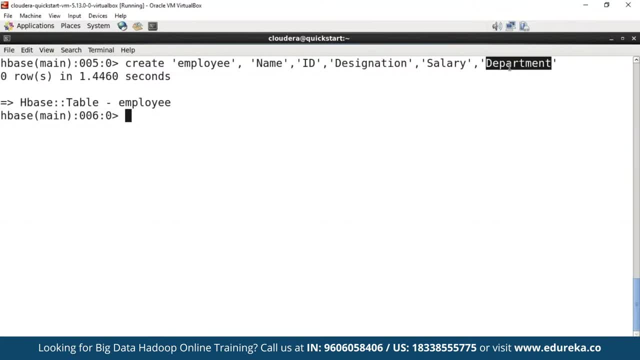 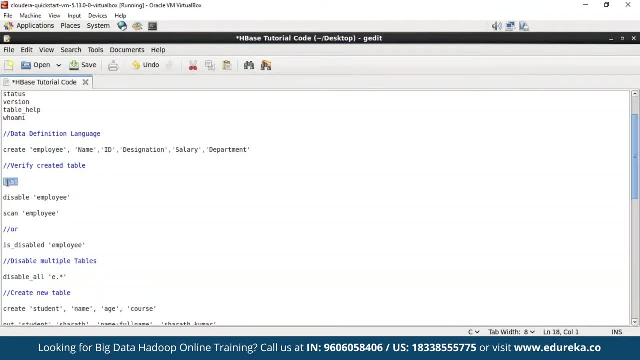 of the employee ID, of the employee, designation, salary and his or her Department, So followed by the creation of table. we shall move ahead and verify our table is created or not. So for that you need to type in list. so when you type in list you will get to know. 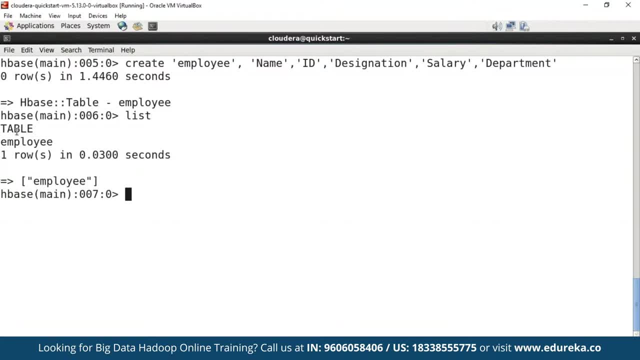 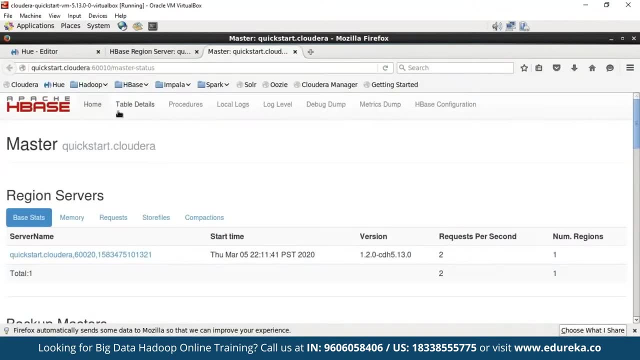 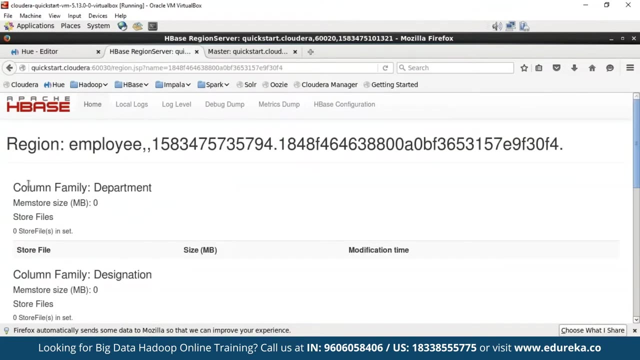 what are the existing tables in your edge base? So we had a table that is default and followed by that, We have employee table. Now let's check our local host and see if the table has been created or not. Yeah, here you can see. the new table has been created successfully. 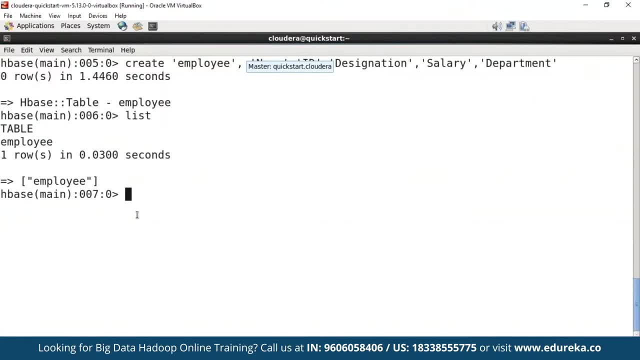 So this is our table now moving ahead. Let's try to perform few more operations on table, such as enabling and disabling them. so to disable a table, You can just write an disable and the name of the table and you can disable it. So there you go. 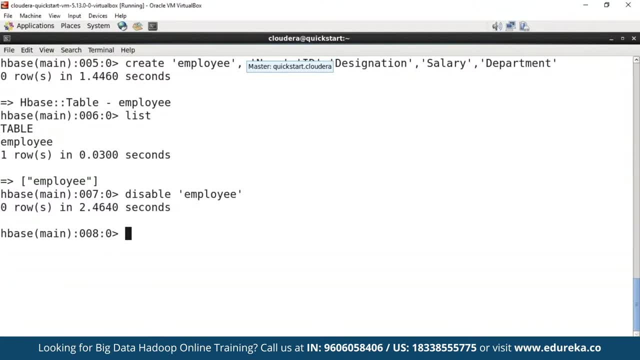 It's been successfully disabled. now you might have a doubt if it's properly disabled or not. So to resolve that issue you can just type in scan employee And if you get the details of the employee table, then the table is not disabled. 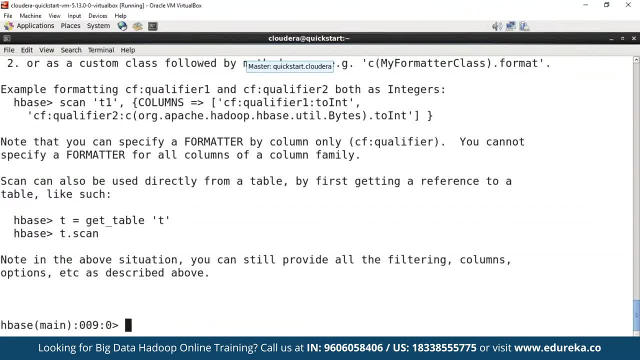 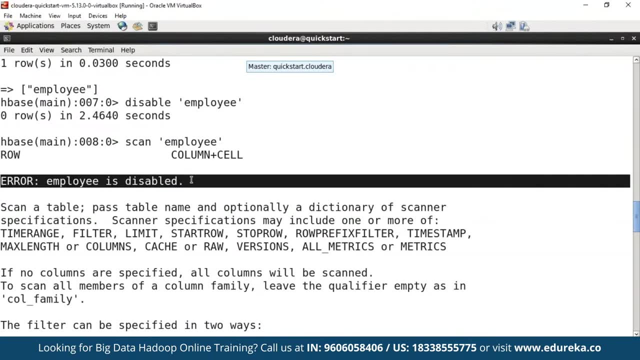 If you don't get the details of the table. instead, if you get something like this which says the employee table is disabled, So you must be sure that the table got disabled now. So this is how it works. Now let's quickly clear our screen. 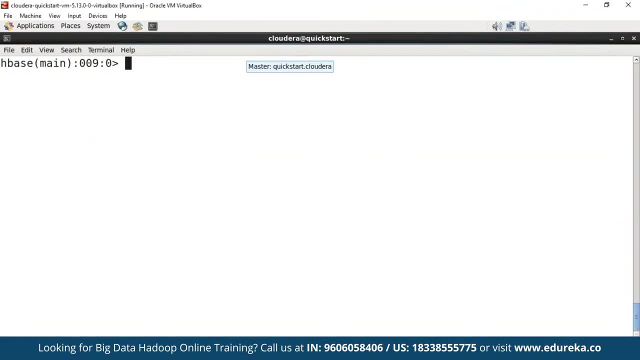 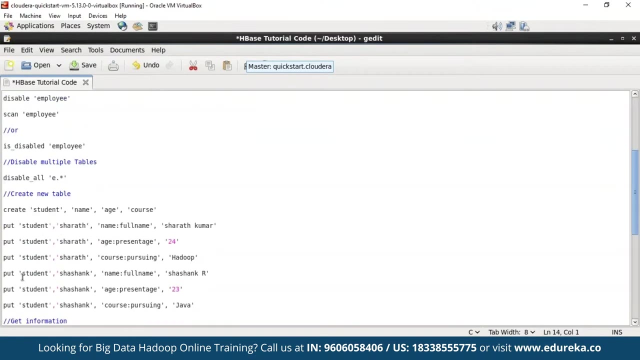 and move ahead with the next type of operations. Now let's try to create another table with different name. This time we will create employee. to now, We have got two tables in our edge space. So if you had to delete multiple tables or if you had to disable multiple tables, 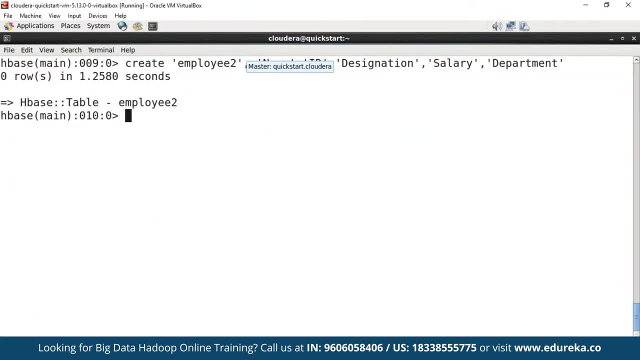 with starting letter e or some, like many other databases have, with same names. for example, if you are in a school, then you have classes and inside classes you might have sections. So for example, if you take class 10, you have section a, section B and section CD. 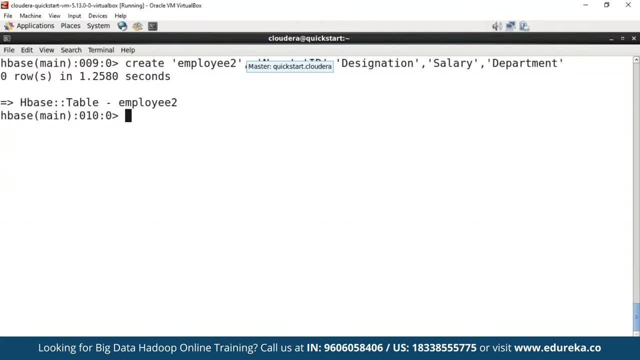 So you might name them as class 10, section a, class 10 section B, class 10- section D. and if you had to delete the all details of all the students of class 10, then you might use this command. So here I'm using disable all e. 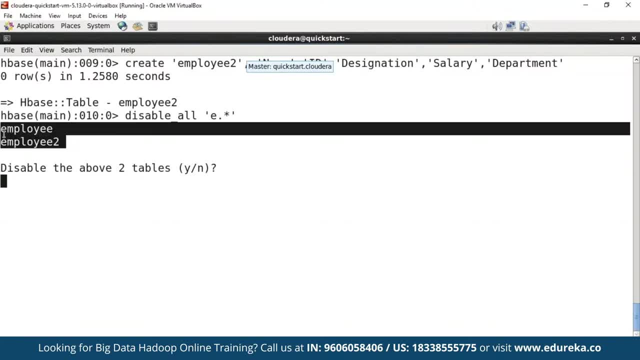 So this command will give me two tables, which are my first table, which are employee and employee 2.. So you can just provide Y for yes and N for no to disable these tables. Now, I don't want to disable my table. 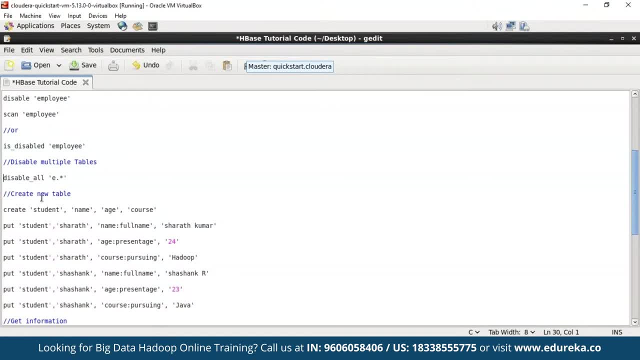 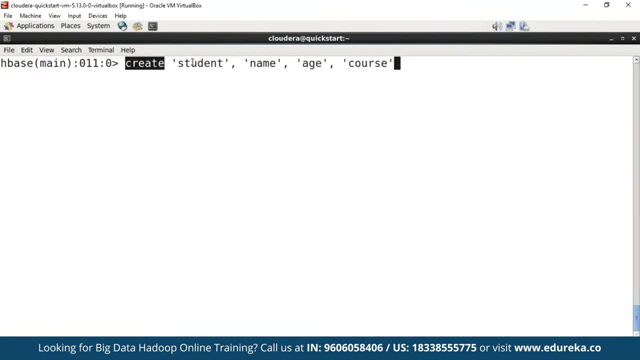 So I'll just give an. so I've closed it now. moving ahead, Now we will create a new table with the name student and apply some operations on it. So create is the keyword and student is the name of my table, and inside that I've columns name, age and course. 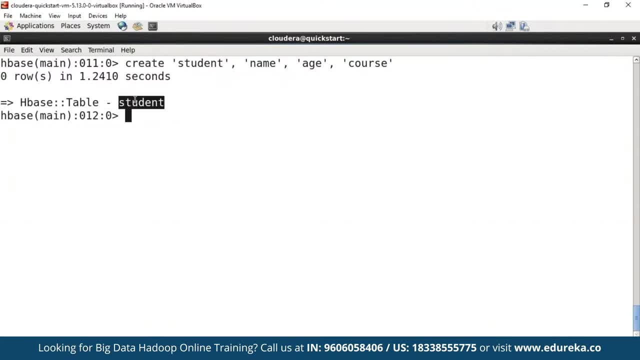 Let's create it. The table has been successfully created with the name student. now, followed by that, We shall try to put in some data into this edge base. So the table name is student and the value will be Sharath and inside the column family name. 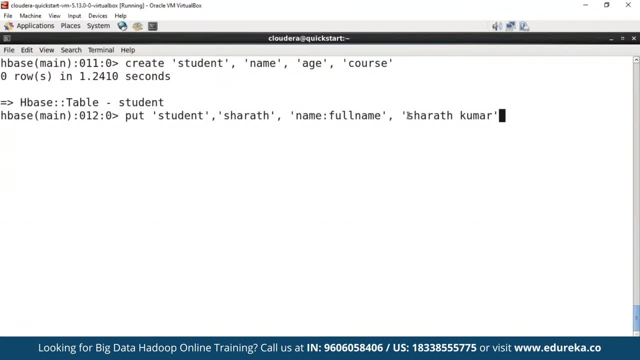 I've got another column which says the full name. So the full name of Sharath is Sharath Kumar. So I'm going to load this data into my student table, fire and enter and the data is in. now Let's add in another data. 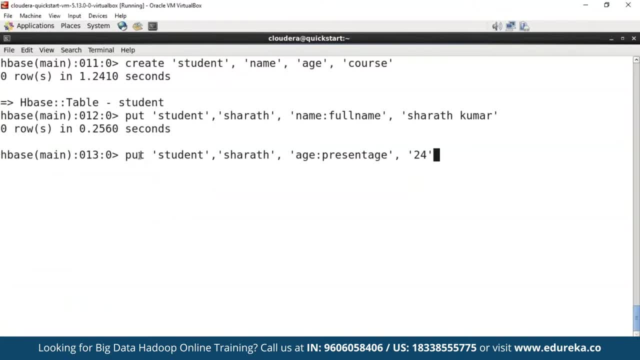 into my table. this time I'll add an age. So here I'm trying to use the keyword put and I'm loading the data into the table: student, and the row is Sharath's row and inside Sharath's row I've got a column family called age. 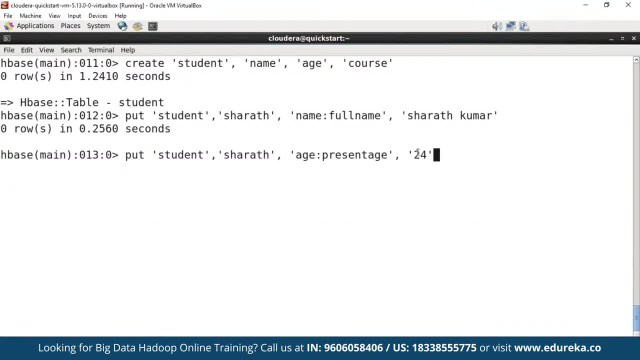 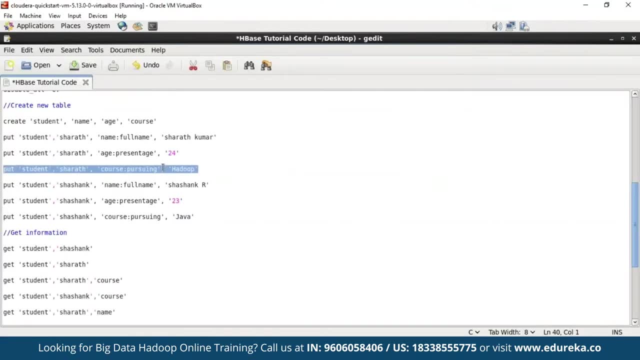 and inside that I've got the column name as present age. So the present age of Sharath is around 24.. So at that, data as well, followed by that, Let's add in the course to Sharath the course which he is studying. 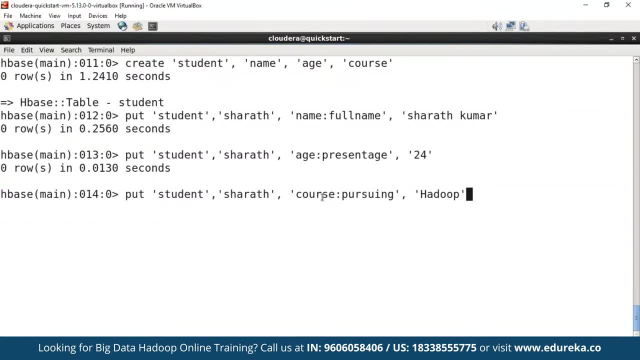 So inside a Sharath's row and student table I've got course family and inside course family I've got pursuing column and his pursuing Hadoop in this particular institution. So now let's fire and enter to load this data. So the data has been successfully loaded. 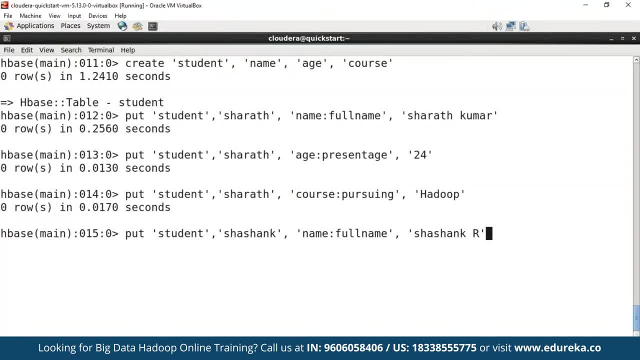 Similarly, let's add the same details for another student, which is Shashank. So we have added Shashank into the table. Now let's add in his age. So Shashank is around 23 years of age, and now we have added that data as well. 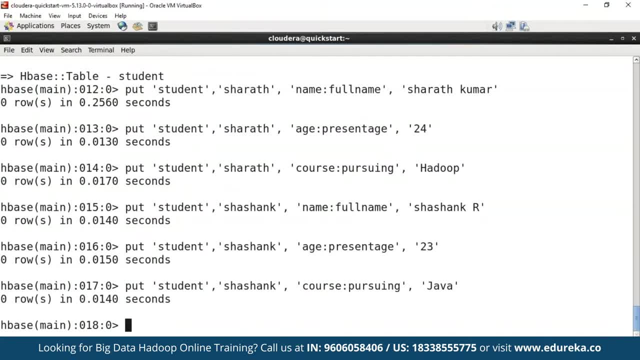 Now let's add: in the course with Shashank is studying, So he's studying Java, which is also loaded now. Now that we have loaded all the data's into the tables, Now let's get the details. So we are here using the keyword get, so we are getting. 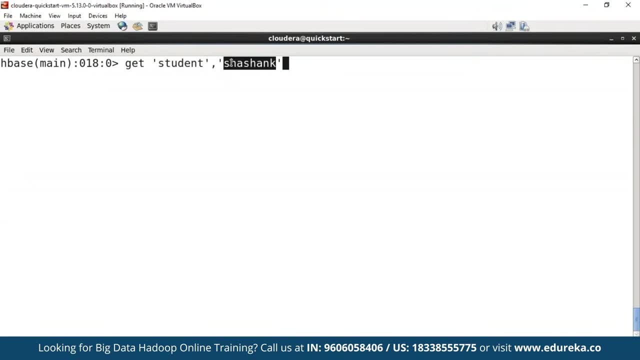 the information from the table. student and the particular student of the information which we require is Shashank. Now let's fire and enter and you get all the information related to Shashank. So the complete name of Shashank is Shashank are. 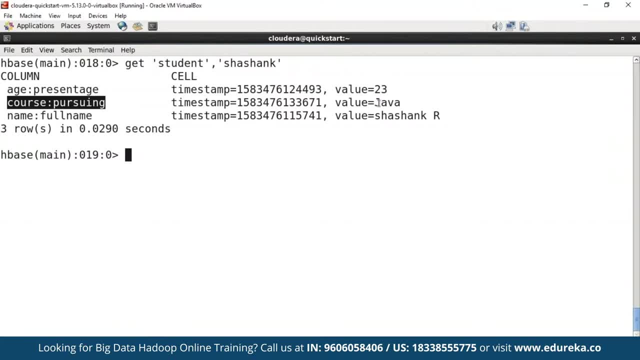 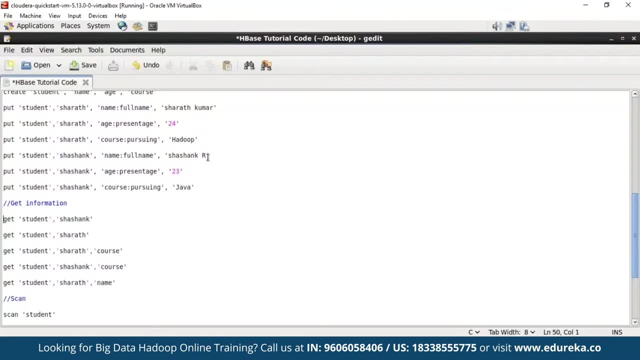 and the course he is studying- That is, course pursuing- is Java and his age- The present age- is 23.. So this is how you get the data. Now we will also get the data of a shutter using the similar way. So there you go. 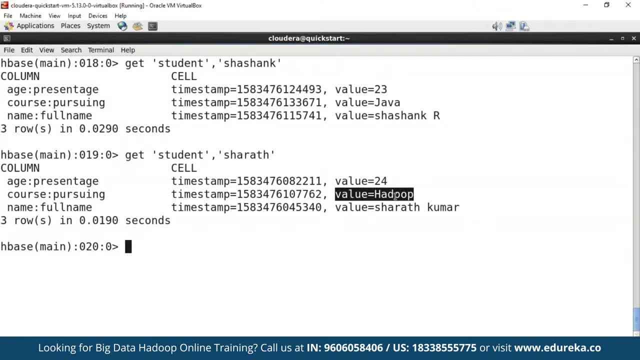 So the present age of Sharath is 24 and the course he is studying is Hadoop and the complete name of Sharath is Sharath Kumar. Now, if you want to get a particular information- like if you don't want his age, if you don't want his full name- 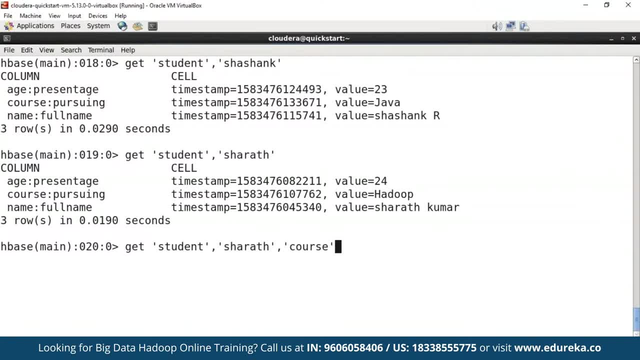 and you just want his course. what is Sharath studying in particular institution? then you can provide the command as get information from the table. student of the student, Sharath, and his course. that is course Now. let's fire and enter and see. you can see. 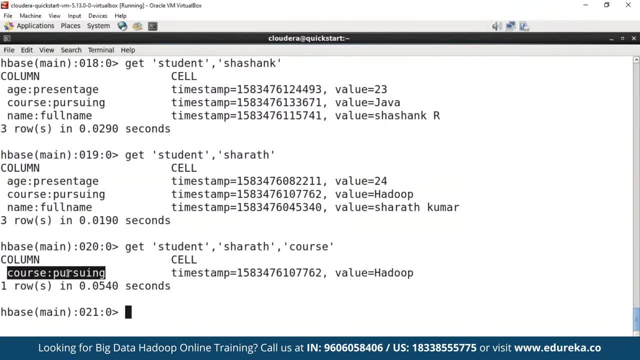 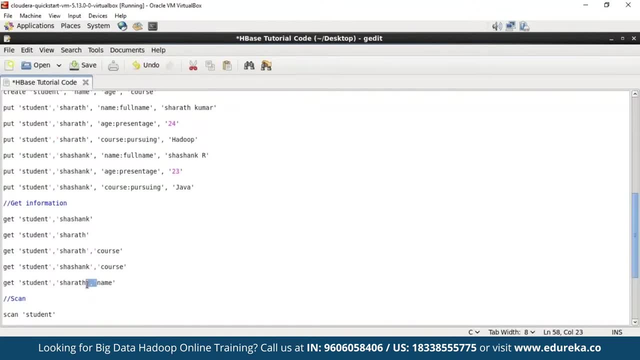 that we have got the course family and inside course family, We have the column pursuing So, which says Sharath is pursuing with the course Hadoop. Similarly, let's try to get the complete name of Sharath. So if you just want the 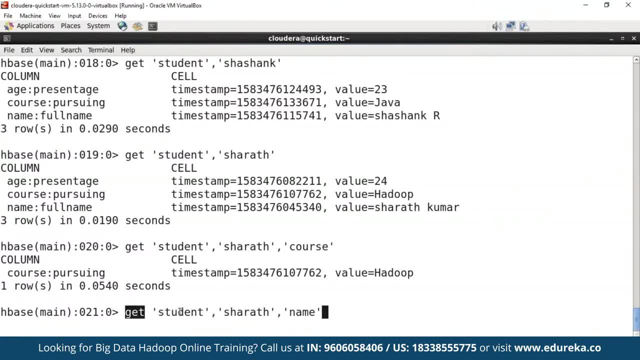 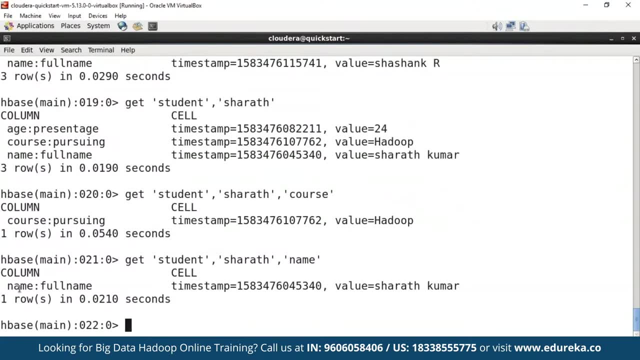 complete name of Sharath. then you can provide the keyword get from the table student from the row: Sharath and his name. So there you go. from the column family name, You have the column full name and his complete name as Sharath Kumar. 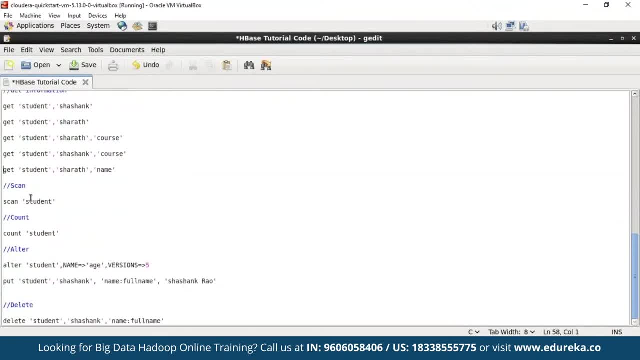 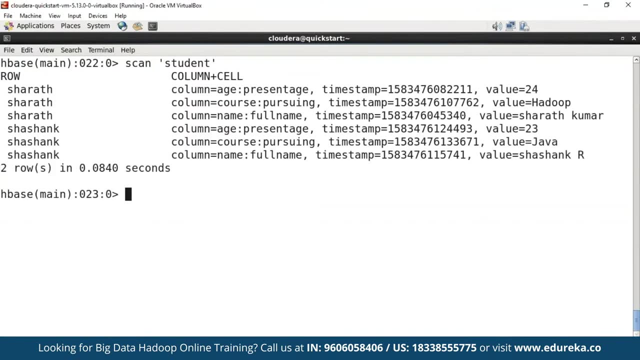 So this is how you get data from a table. Now we shall see the complete details of the table student. So for that you can use the command scan table, which will give you the complete details of all the students present in your particular Institute. 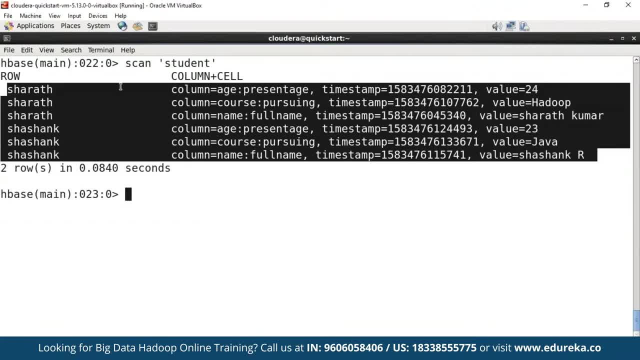 So right now we have two students So, which are Sharath and Shashank. So this particular command gives you the age of Shashank, The course is studying, and his complete name, followed by that you have Shashank, his complete age, the course. 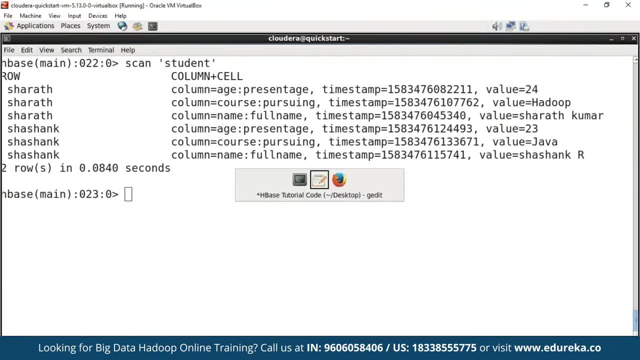 He is studying and his complete name, which is Shashank, are so, followed by this. We shall try to count the number of rows available in this particular table that has student. So we have two rows right now. And yeah, here you go. 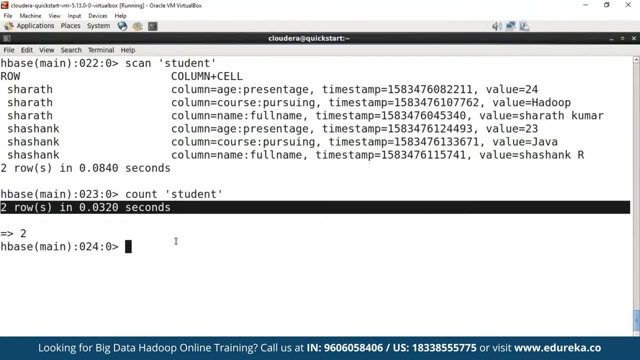 We have two rows which are present in the table student, So this is how you can perform count operation in edge phase, followed by that, You can also alter some informations based on your table. So I'm going to alter the table student and the column. 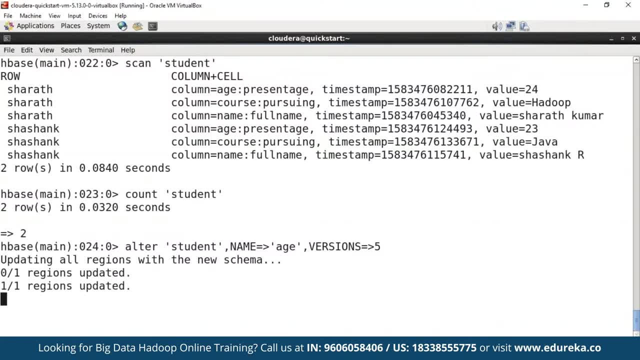 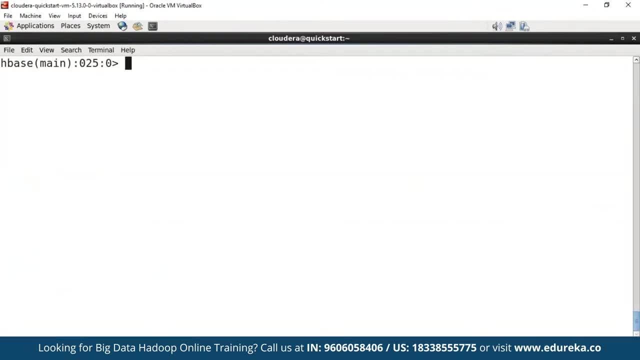 which I'll be altering is age. So you can see that the process is getting done, so you can alter the age. now we shall try to alter the name of a particular student. So for now, I want to alter Shashank name as Shashank Rao. 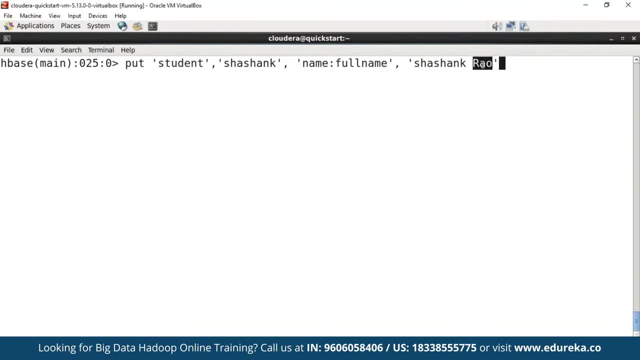 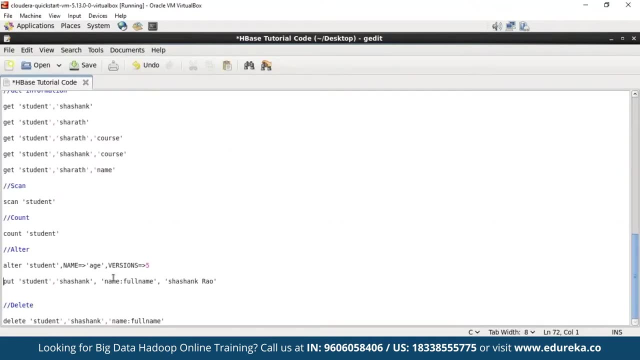 So the R alphabet present in his name is about his full name, which is Rao. Now we will rename Shashank R as Shashank Rao. So the process has been successfully completed. Now let's scan student again and see if his name is changed or not. 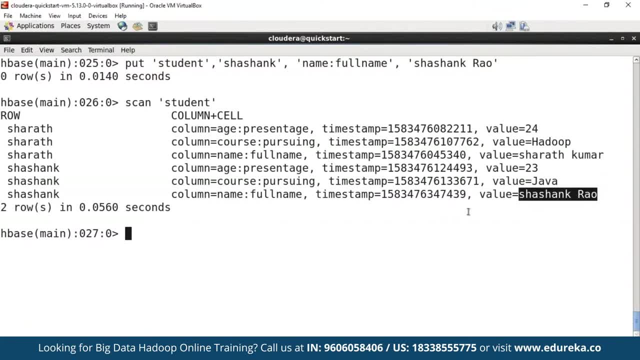 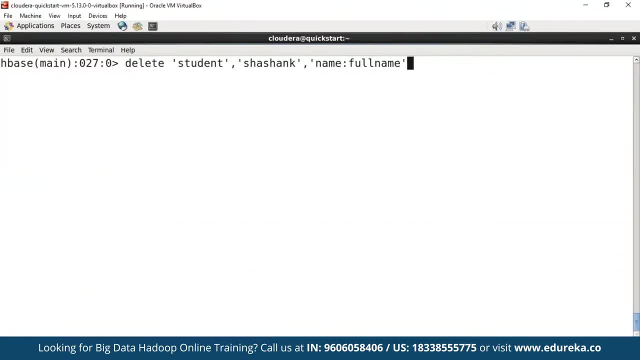 So there you go. earlier We had Shashank R, now it's changed to Shashank Rao. So this is how you can alter some of the rows or data present in your table. Now let's try to delete a one particular column from your table that has the full name. 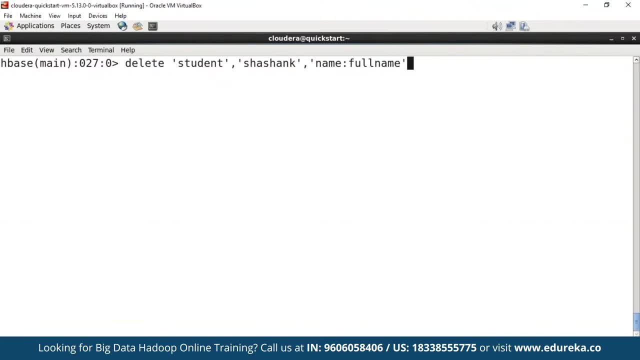 Now we will delete the full name. So Shashank's full name will be deleted and only Shashank will be remaining. So now the process is complete. So this is how you can execute some of the basic commands in HBase, and no worry about this code. 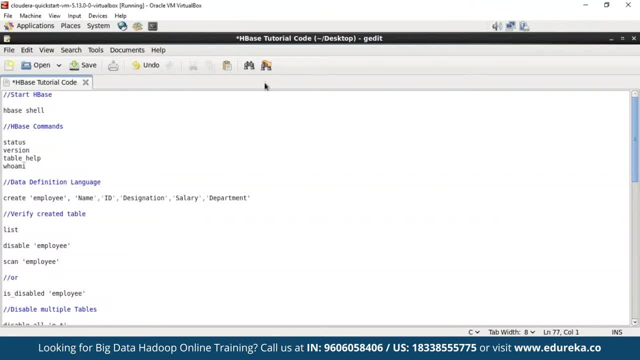 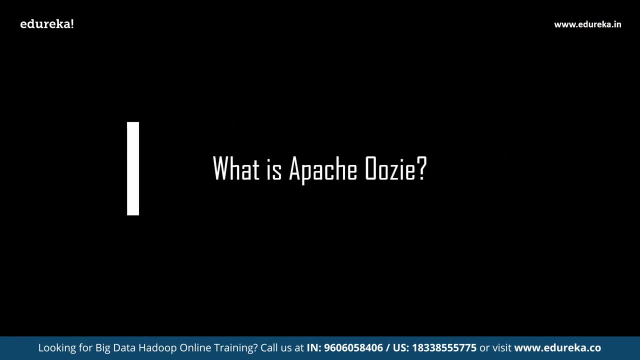 We will drop down this file in the description box below, where you can get access to it and you can execute the same commands in your own personal system, to just have a practice about HBase tutorial. What is Apache Uzi? answer: Well, Apache Uzi can be defined as a job scheduler system design. 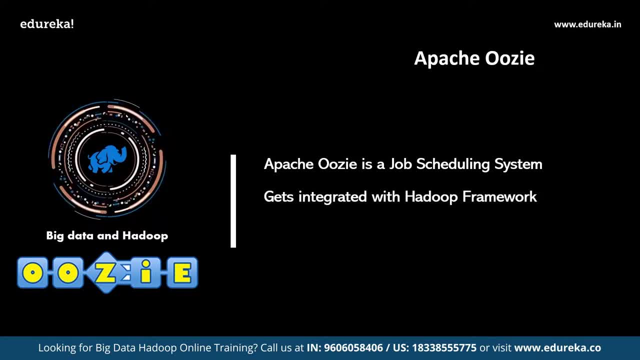 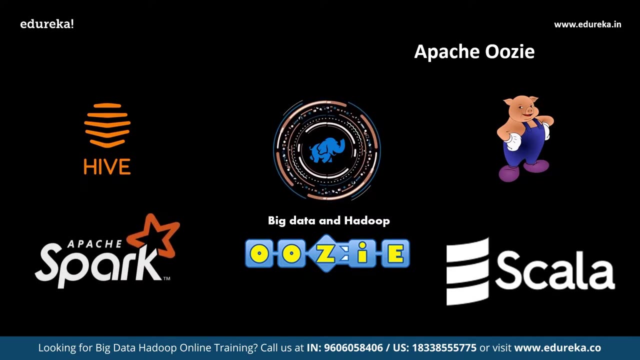 and deployed to manage and run Hadoop jobs in a distributed storage environment. It allows users to combine multiple complex jobs to be run in a sequential order to achieve a higher order job to be finished. the reason behind using Uzi along with Hadoop framework is its capability to strongly bind 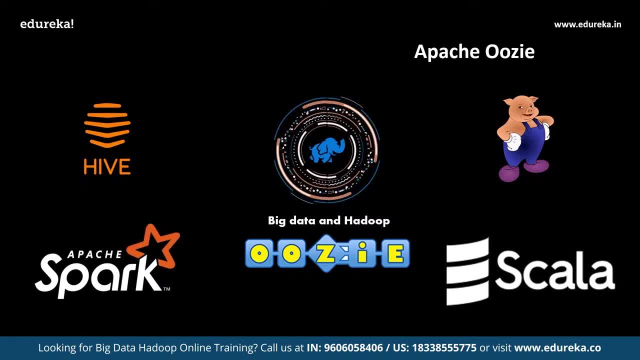 and integrate itself with Hadoop. jobs like hive, Scala, Apache, pig and many more. Uzi is an open-source Java web application available under Apache license 2.0. It is responsible for triggering workflow actions, which in turn uses Hadoop execution engine to actually execute the task. 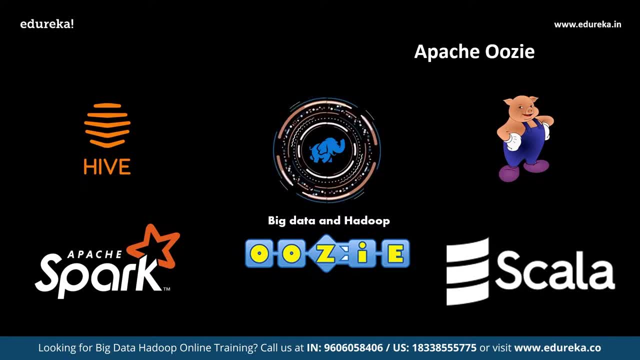 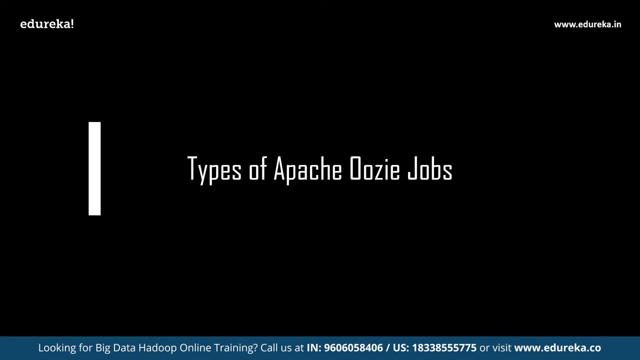 Hence Uzi is able to leverage the existing Hadoop machinery, designed for many tasks, such as load balancing system, system failover and many more. now that we have a brief understanding of Apache Uzi, Let us move ahead and understand the major job types that Apache Uzi can practically perform. Apache Uzi jobs. 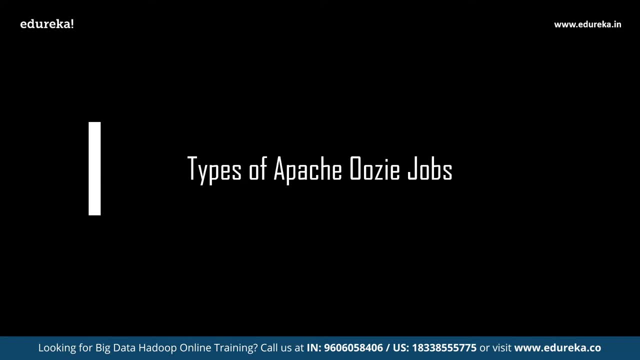 The reason for choosing Apache Uzi for Hadoop jobs is its way of executing its jobs. Apache Uzi is capable to detect the completion of tasks through callback and falling. when Uzi starts a task, It provides a unique callback HTTP URL to task and notifies the URL when the task is completed. 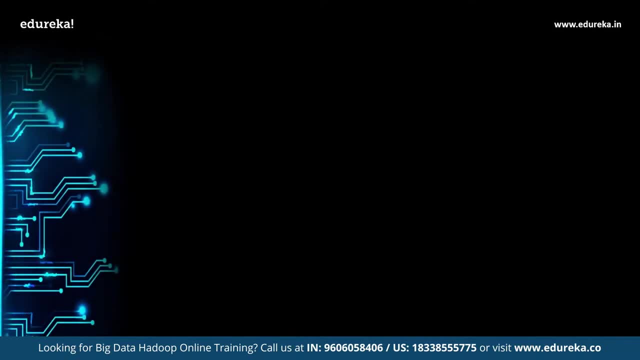 If the task fails to invoke the callback URL, then Uzi can pull the task for completion. There are three main types of jobs in Uzi. They are: Uzi workflow jobs, Uzi coordinator jobs, Uzi bundles. Firstly, Uzi workflow jobs. 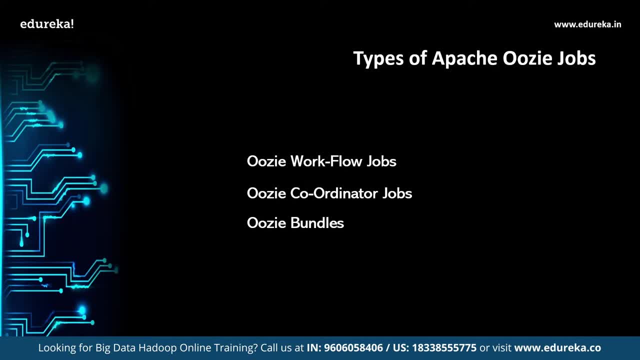 These are directed acyclic graphs or DAGs, which specifies a sequence of actions to be executed. next, Uzi coordinator jobs consist of the workflow jobs triggered by the time and data availability and, lastly, the bundles. These can be referred to as a package of multiple coordinators and workflow jobs. 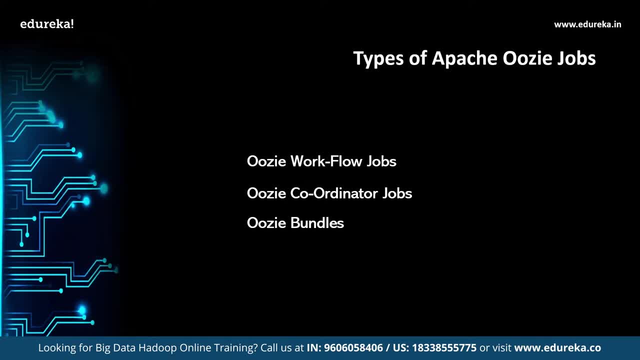 Now let us understand all these jobs in a little detailed way, one by one. firstly, we shall understand Apache Uzi's workflow, a sample workflow with controls. It has start, decision, fork, join and end and actions like Apache Hive shell, Apache pig. will look like the following diagram: Uzi workflow is nothing. 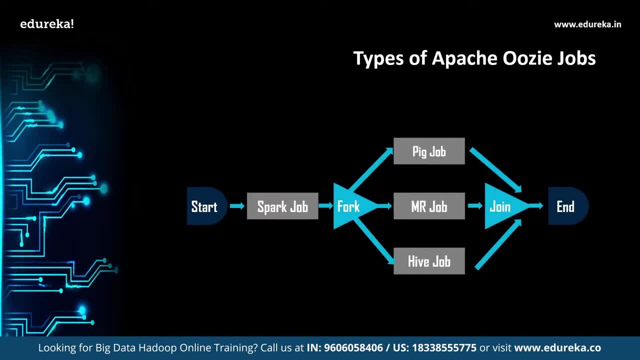 but a sequence of actions that can be carried out and represented in the form of DAGs or directed acyclic graphs. the actions will be carried out in a sequence, which means the output of the previous action will be the input for the present action And the output for the present action will be the input. 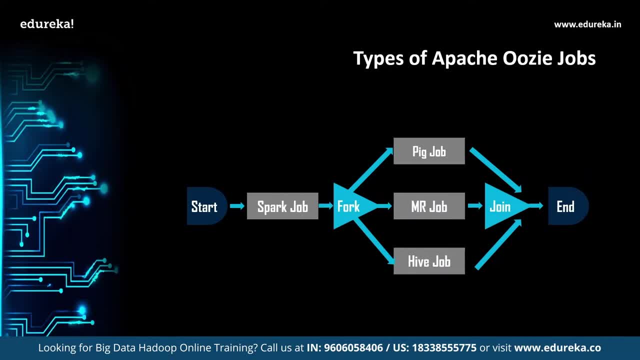 for the next upcoming action. Let us understand this in a bit more detail. in a flow of different sequential tasks, Some tasks can be performed in parallel. to execute some tasks in parallel, We can use the fork option. in Uzi, the join option is used. 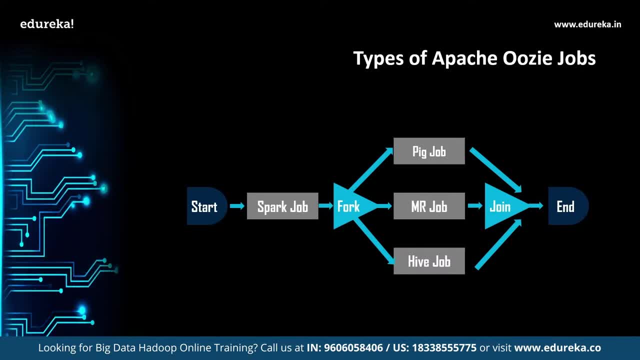 to merge, to pile task into one. Let us discuss with this diagram as shown down below. you can see the starting phase is the start and the last phase is the end, and between we have MapReduce job, big job and fork and join So here out of multiple jobs such as Hive, shell, big MR. 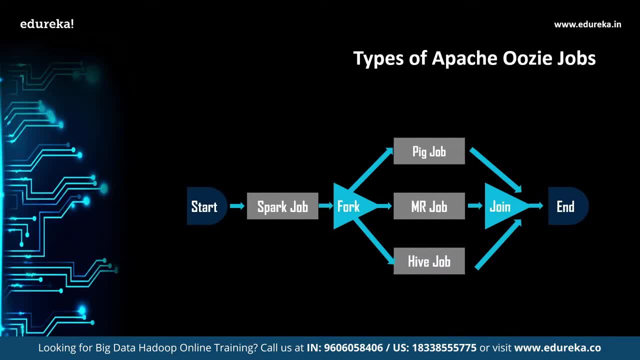 We are using MapReduce job and big job. after starting the job, The workflow will enter the MapReduce job first. after executing the MapReduce job, a result will be generated or an output will be generated which will act as an input For the next upcoming big job and inside the big job. 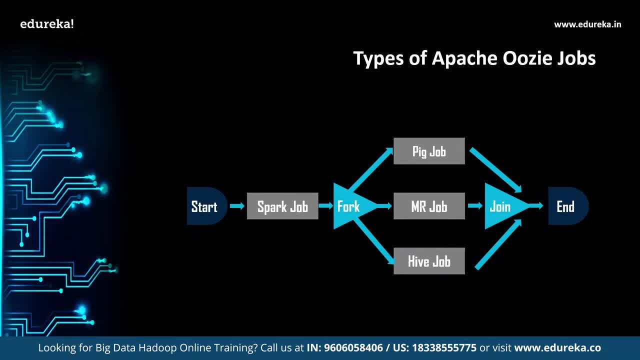 the task get executed and the output will be forwarded to folk. here to other jobs are existing which are MapReduce job and a hive job asset. earlier, folk is used to execute two different tasks in parallel to save time. So here the output from the big job is forwarded. 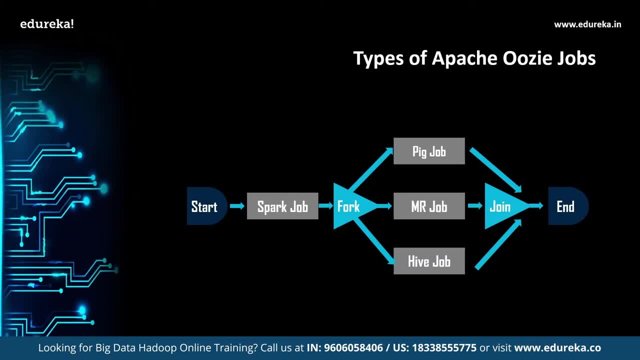 to two different jobs, that is, the MapReduce job and the hive job, using folk, and after that the output will be generated from both the jobs, That is, the MapReduce job and the hive job, and these two outputs will be joined together using the join method and after that, the entire output. 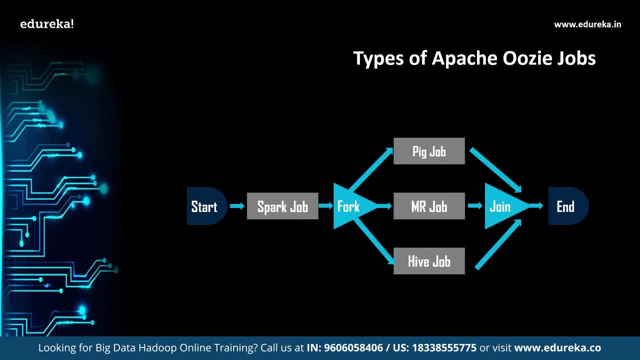 or the final output will be thrown out, and that is the end of the execution of OC workflow. So this is how the Uzi workflow works in real time. So here the different components used in this particular job are: start: MapReduce job, big job, folk join Hive job. 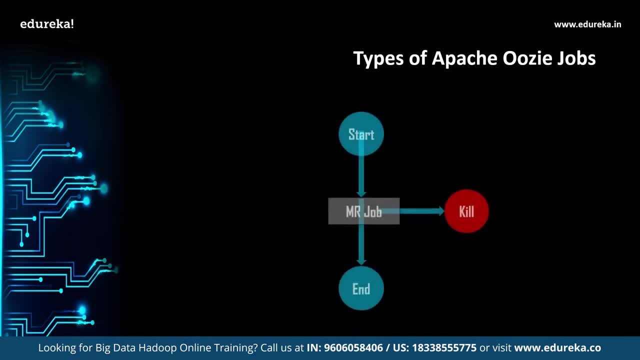 and finally the end. Next are the nodes in the Uzi workflow. There are mainly three control flow nodes in Uzi workflow. They are start, end and kill nodes. as you can see in the above diagram, We have start node in the first and end node. 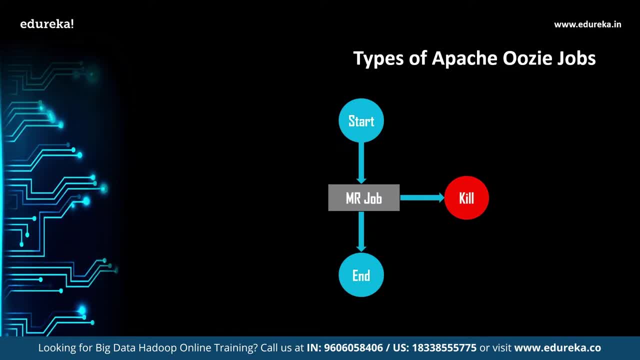 in the last position. in between, we have a MapReduce program which is based on word count. if this particular MapReduce job encounters an error, then the job will be terminated using the kill option or the kill node In case if the MapReduce job is successful. 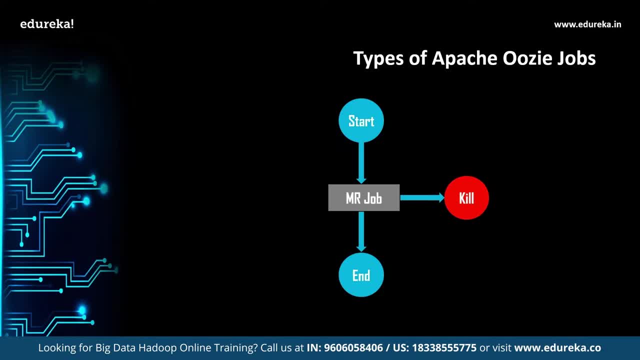 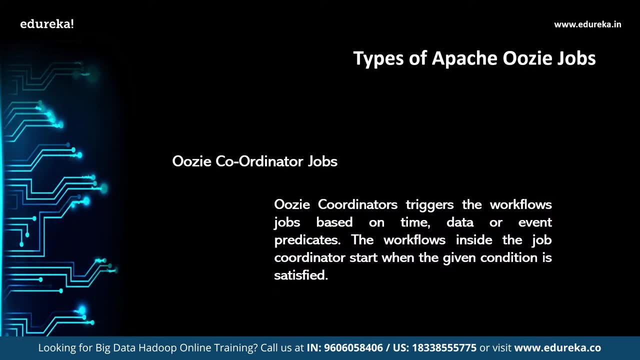 then the control will flow into the next node, which is the end node. next We deal with the coordinators. you can schedule complex workflows as well as workflows that are scheduled regularly using a coordinator. Uzi coordinators trigger the workflow, jobs based on time, data or even predictions. the workflows 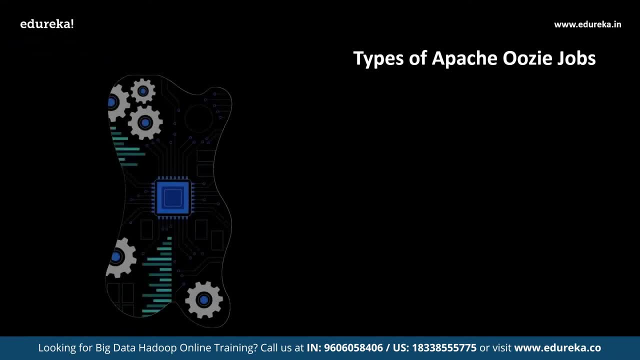 inside the job coordinator start when the given condition is satisfied. definitions required for the coordinator jobs are start and time zone, frequency and some more properties that are available in control flow information. Firstly, the start start says about the date and time which is related to the particular job assigned. next, 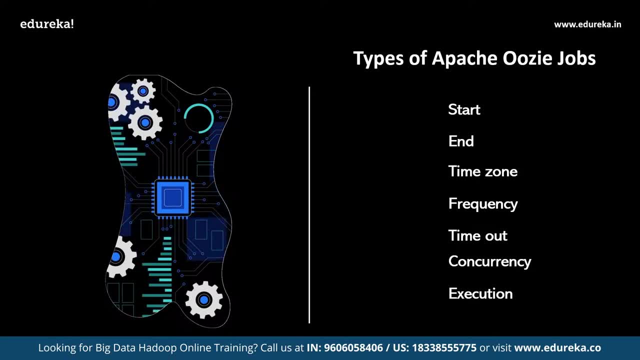 is the end. the end defines the date and time for the particular job assigned. followed by that We have the time zone. times on represents the time zone of a coordinator application based on the particular location where the program is being executed. followed by that we have the frequency. frequency says: 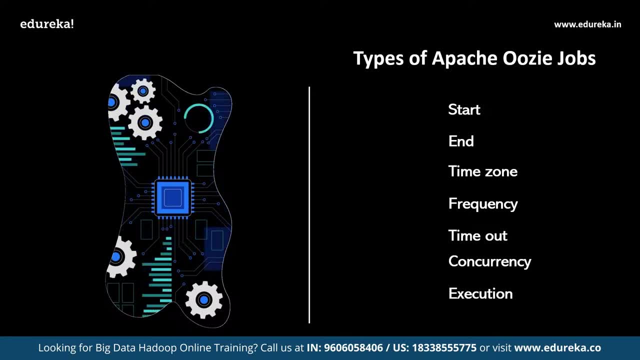 about the information of the number of minutes consumed while executing the job. now, apart from that, we have a few more which I like. time out: the maximum time in minutes for which an action will wait or satisfy the additional conditions before getting discarded. the zero indicates that all the input events are satisfied at the time. 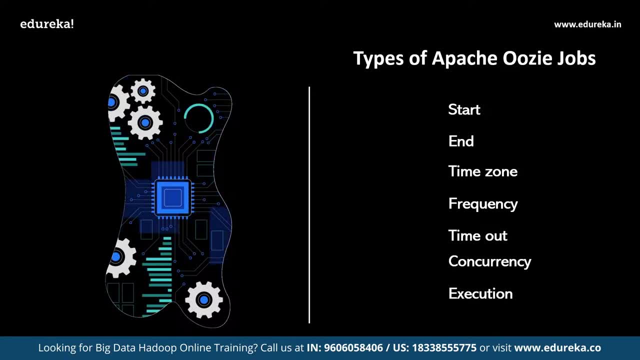 of action: materialization. the action should be timed or immediately. one indicates no timeout, the action will wait forever. The default value will always be one. next is the concurrency: the maximum number of actions for a job that can run pally. the default value is always one followed. 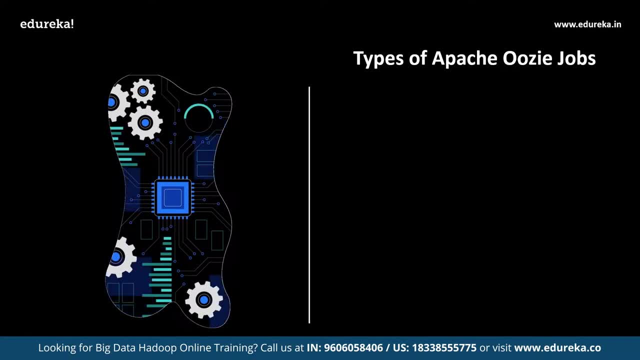 by that we have the execution. the execution specifies the execution order. if multiple instances of the coordinator job have to be satisfied with their execution criteria, that can be FIFO by default, which is first in first out, or leave, for which can be last in first out. finally, 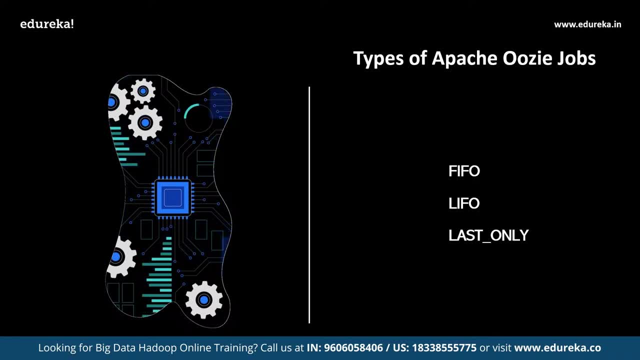 the last, only the command for the coordinator jobs to be executed is shown in the slide below, So followed by the command. if a configuration property used in the definition is not provided with the job configuration while submitting the coordinator job, the job submission will fail. So now, with this, we finish. 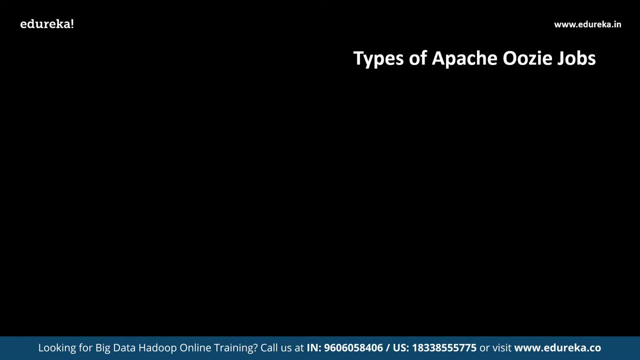 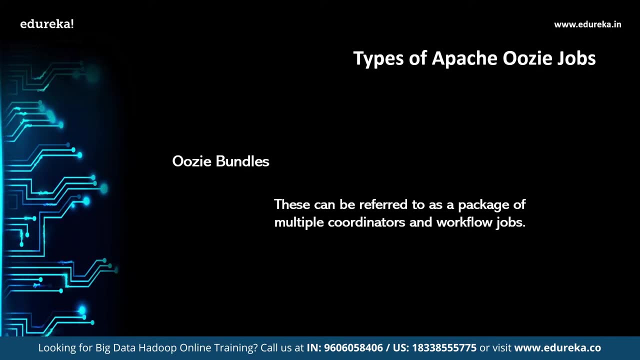 of the coordinator jobs, followed by coordinator jobs. We have the Uzi bundle. Uzi bundle System allows you to define and execute a set of coordinator applications, often called as a data pipeline. in Uzi bundle, There is no explicit dependency among the coordinator applications. 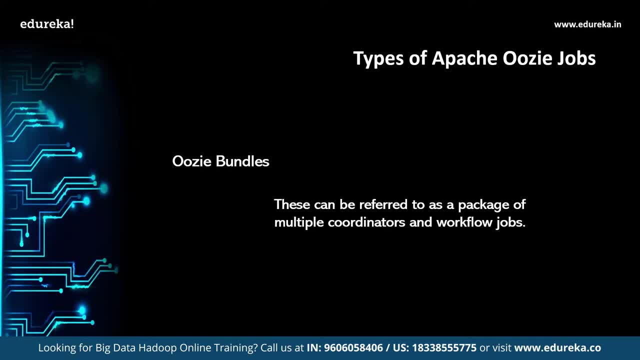 However, you could use the data dependency of coordinator applications to create an implicit data application pipeline. You can start, stop, suspend, resume, rerun the bundle. It gives a better and easy operation control. the most important term We need to understand about Uzi bundle is its kick-off time. 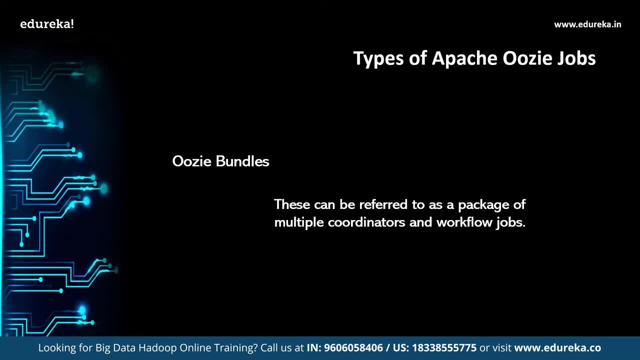 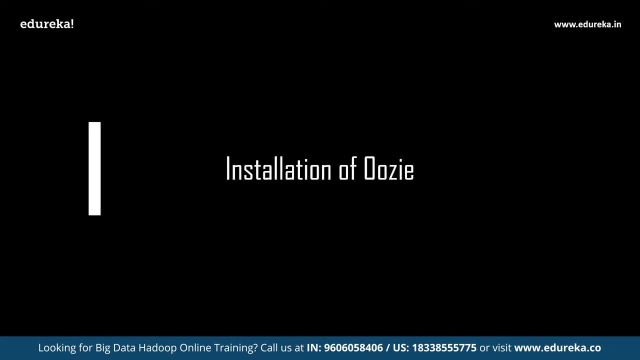 The kick-off time is the time when the bundle should start and submit coordinator applications advancing. in this Apache Uzi tutorial, We shall understand how to install Apache Uzi. Now to install Apache Uzi, There are multiple ways. in centos We need to install cloud era, then download Uzi. download external. 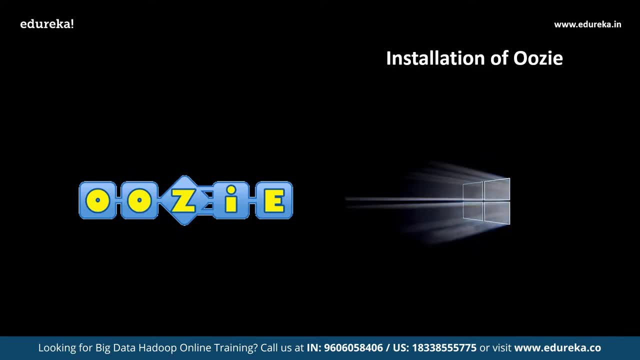 J support for Uzi: download, maven set up and then set up my sequel database, And after that need to configure the setting. and this seems very complex, right? No worries, in this tutorial We shall learn the simplest way of installing Uzi and then later we can try to learn the complex ways. 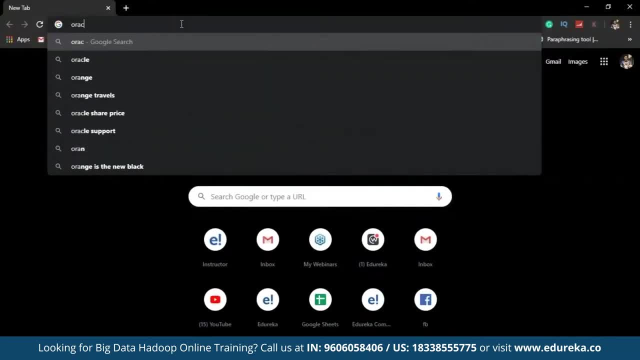 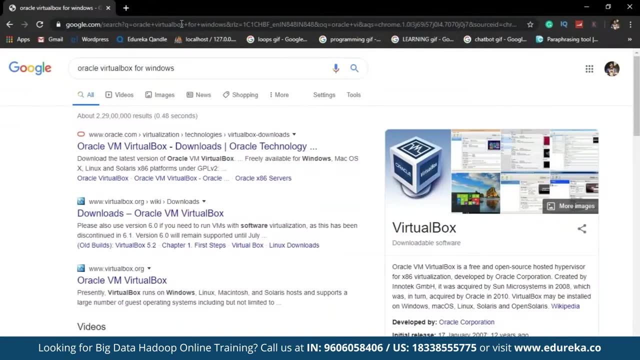 So, firstly, all we need is an Oracle virtual box. So just Google Oracle virtual box for Windows and you will be redirected into a new web page where you can choose Oracle VM virtual box. downloads Oracle technology, which is the first link in the description. You can go ahead and click the latest version of Windows. 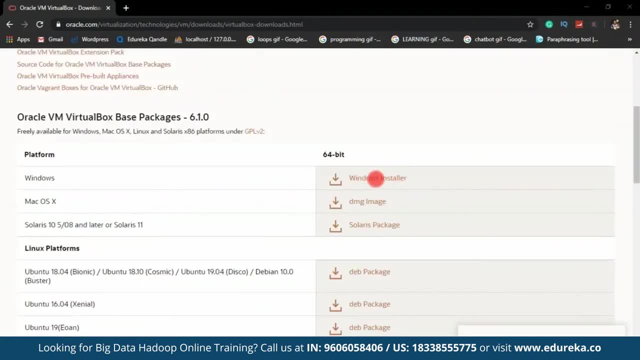 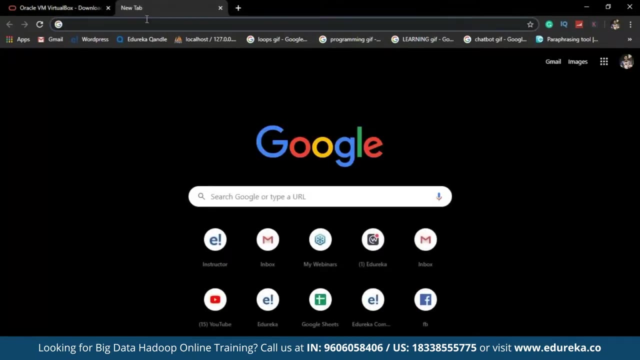 So by clicking on the Windows installer button, you'll get your Oracle virtual box basic packages installed into your local system. You can see the virtual box is getting downloaded, Followed by that open a new tab and Google cloud era. So you can see that we have Googled cloud. 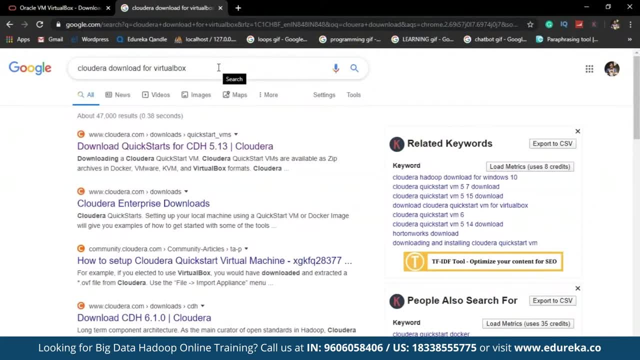 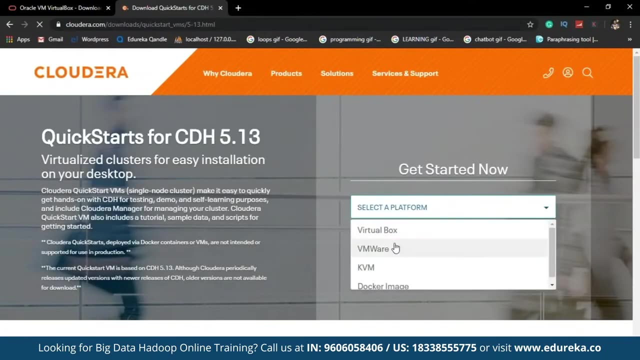 or download for virtual box. So that will redirect you into a new web page and the first link, which is download: quick start for CDH 5.13 cloud error. clicking on this link, You will be redirected into a new web page And in this you need to select a platform. 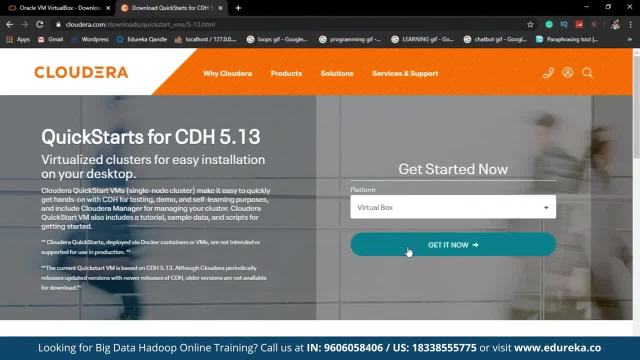 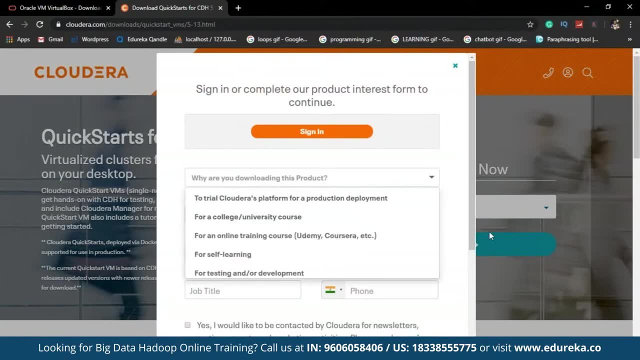 So here we shall select virtual box And now just click on get it now. And here you need to provide your details: Why are you using this product, which is for learning, or anything else? and followed by that you need to provide your name, last name, business, email ID, the company. 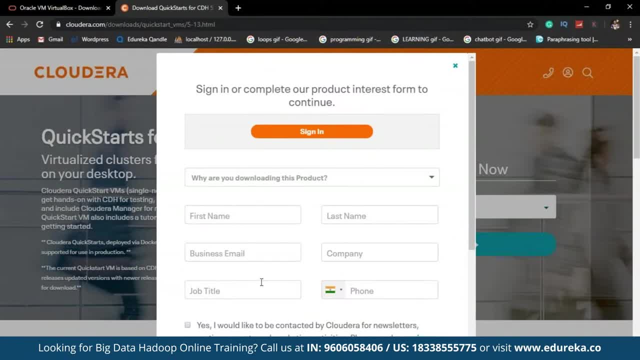 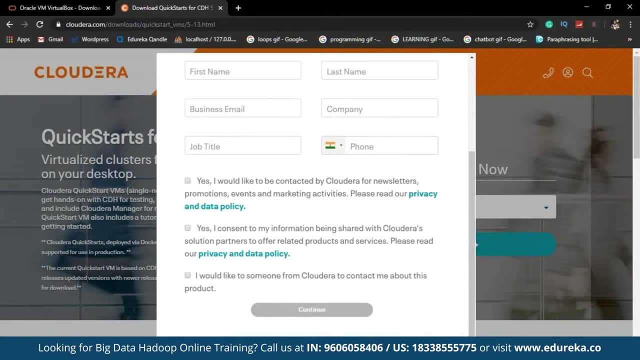 which you're working, or you can ignore if you're a student. after that your job title and you can ignore this. if you're a student and your official phone number, then accept all the above, that private data policies, and if you would like to prefer someone to use cloud era, then press continue. 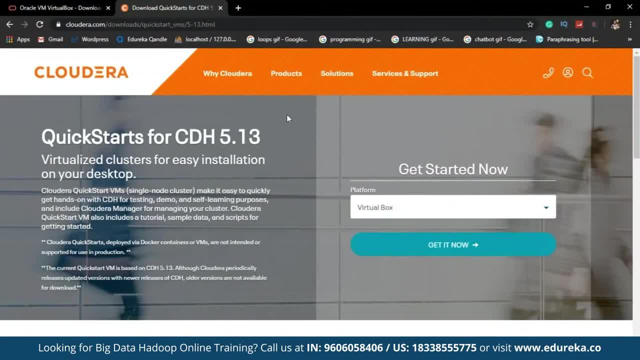 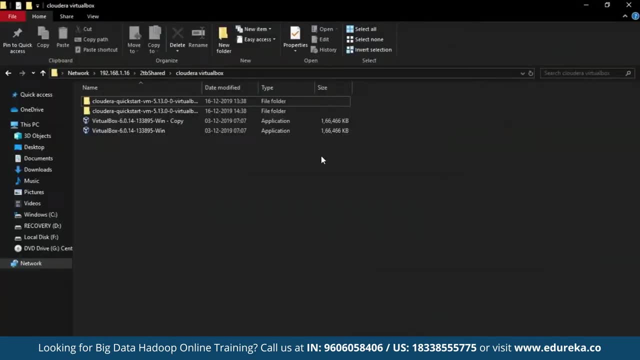 and your virtual box will be downloaded. I have already downloaded a quick start CDH 5.13 in my local system, So I would prefer to ignore this. now that we have successfully downloaded our cloud era CDH and virtual box required, We shall run them and install into a local system. 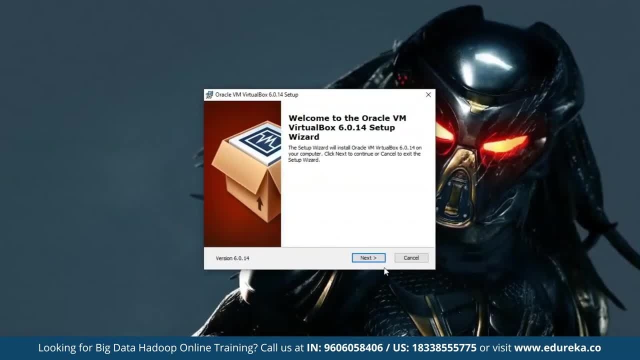 You can see that the Oracle VM virtual box setup is started. Now you can select next, followed by that, just select next again, And here you're provided with different options, whether to create a shortcut menu on your desktop or not. I would prefer not then. you select next, then yes. 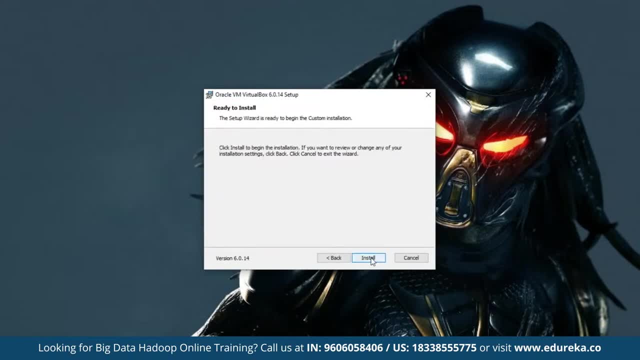 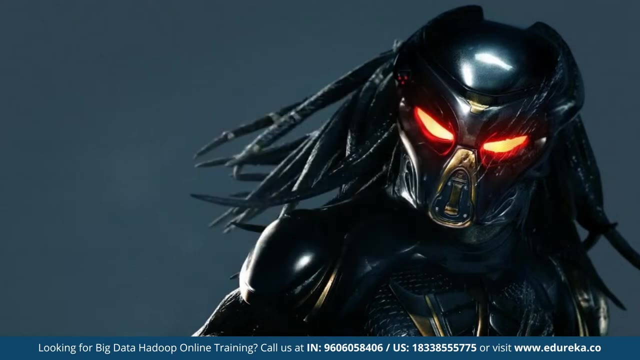 And the last button will be installed. So I have already installed Oracle virtual box 6.4 version into my local system. to save time, We shall cancel this. but you have to select install button to install your virtual box system. So once after the virtual box is installed into your system, 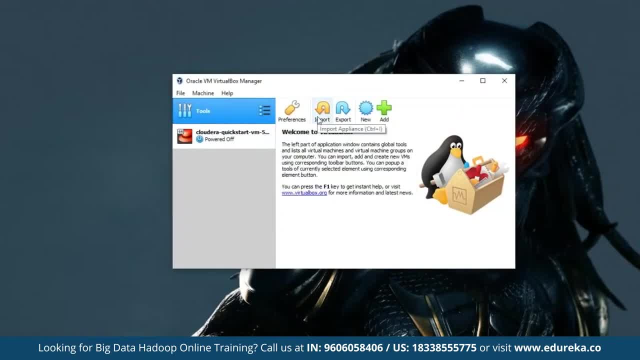 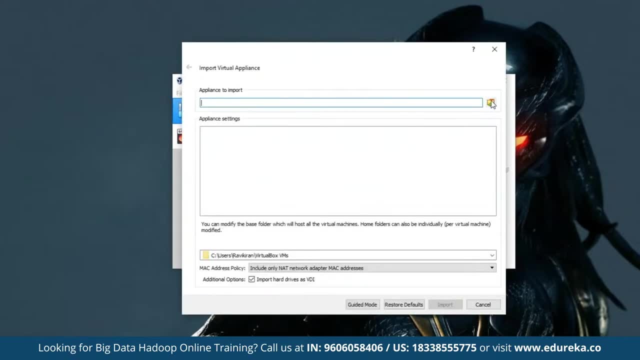 it will be looking something like this: So here you need to select the option import and you will be provided with a new dialog box, and in here you need to select the browse button over here. So once you select the browse button, you will be redirected into a local file system. 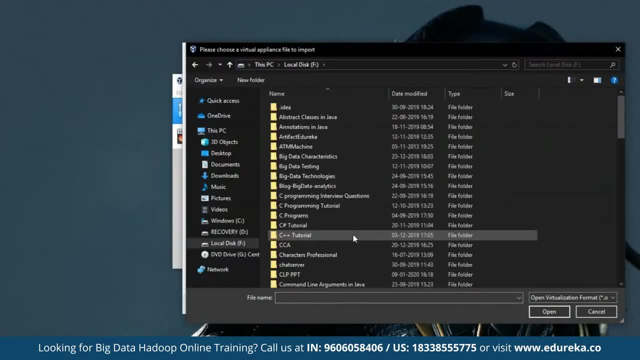 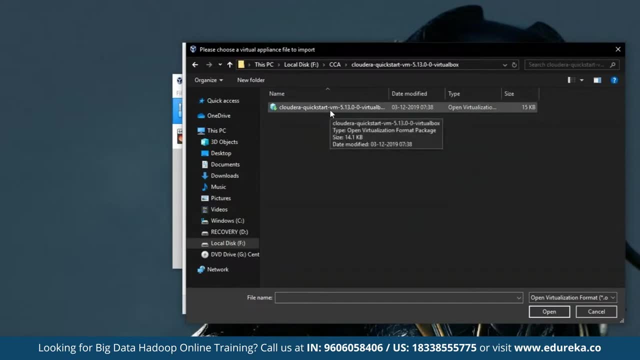 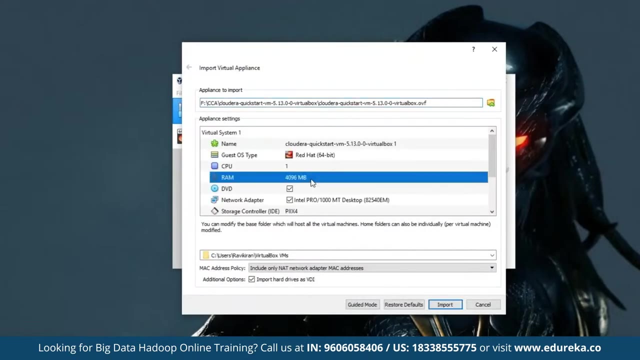 So you have to know the location where your quick start cloud era has been downloaded. So I have saved my quick start cloud era ISO file in this particular file. So I need to select my quick start VM, then just select open and for the safer side in the configuration. 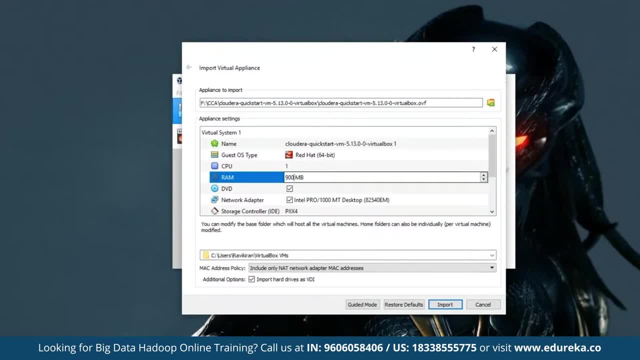 we shall select the RAM size above 8gb. So I'll just specify randomly as 9000 MB, which is just about 8gb. and now just import. You can see the importing appliance has started. So your cloud era will be imported as soon as possible. 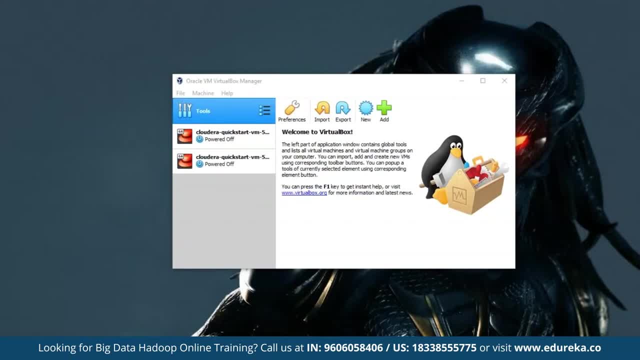 So you can see that the cloud, or a quick start VM has been successfully imported onto the virtual box. Now let's quickly started by double-clicking it, Or also you can just select the start. now you can see that quick start. 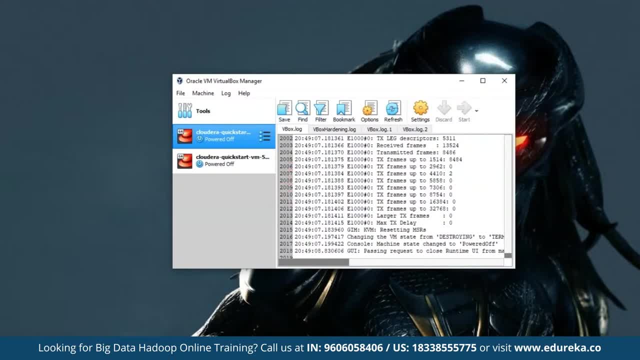 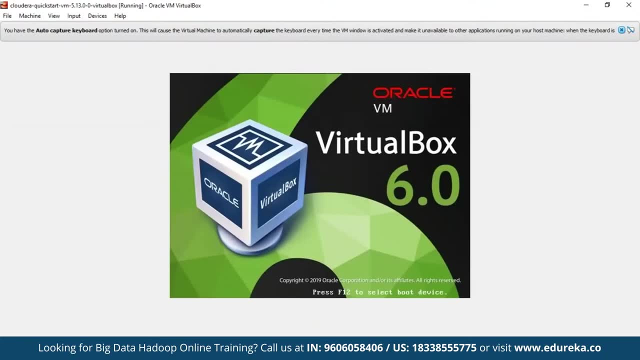 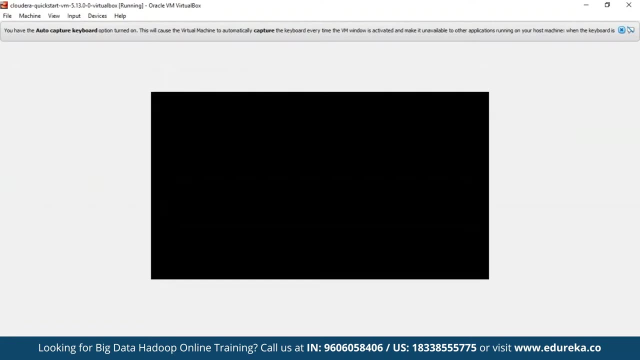 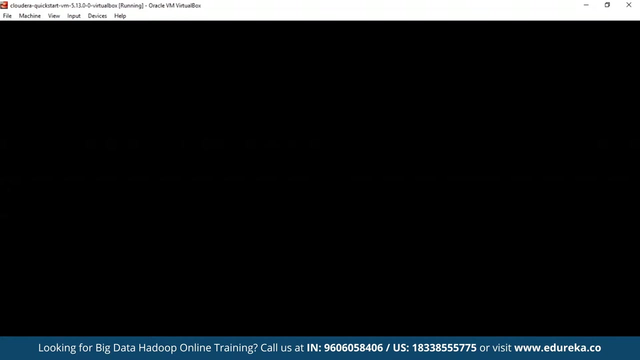 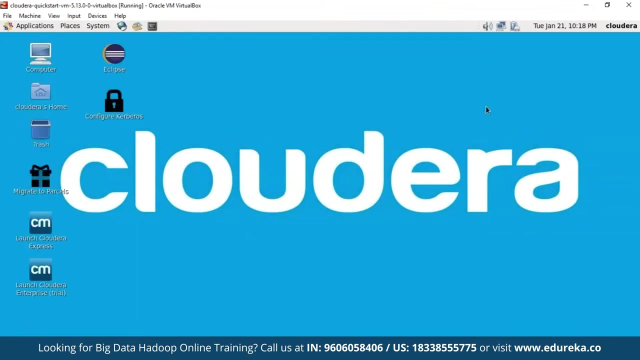 VM has been successfully started and it's loading. You can see the cloud arise getting booted up. So there you go, The quick start. cloud era VM has been successfully imported. put it up Now. the best part about Cloud Array is it's got everything you need. 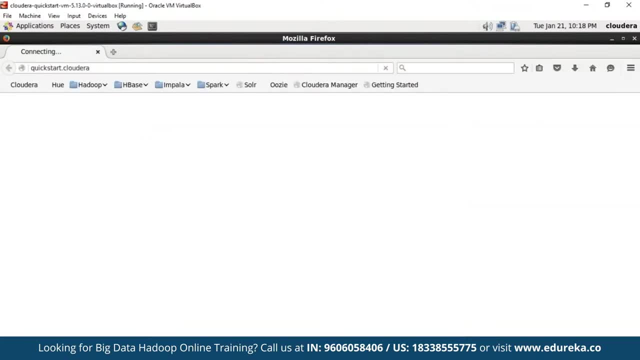 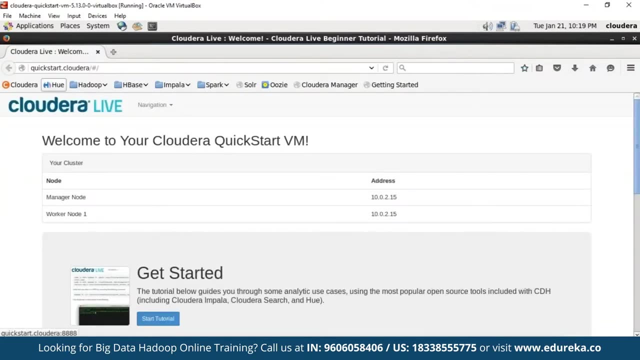 The Uzi Hive, Hue, Spark, HBase, Impala- everything for a beginner to start with. Now what we need is Uzi, So we need to start up our Hue and Uzi first. Let's open Uzi in a new tab. 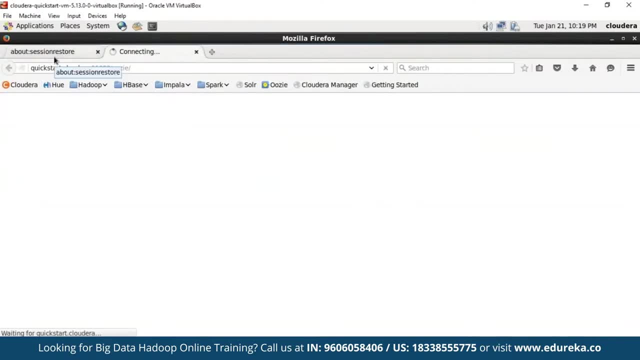 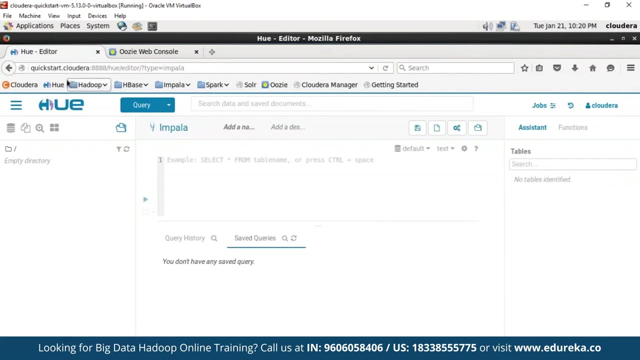 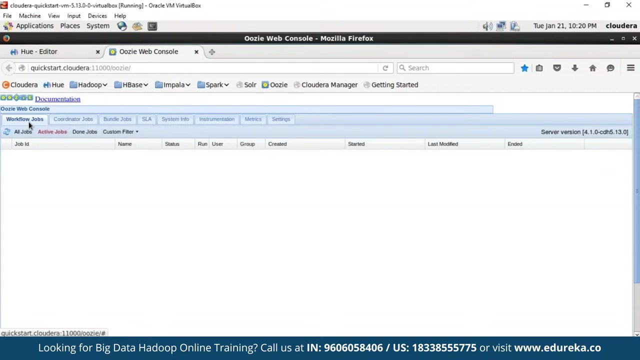 And parallely, let us also start Hue. So this is how the webpage of Hue looks like, or the editor of Hue looks like, And also this is the webpage or web console of Uzi. So here you can have workflow jobs, coordinator jobs. 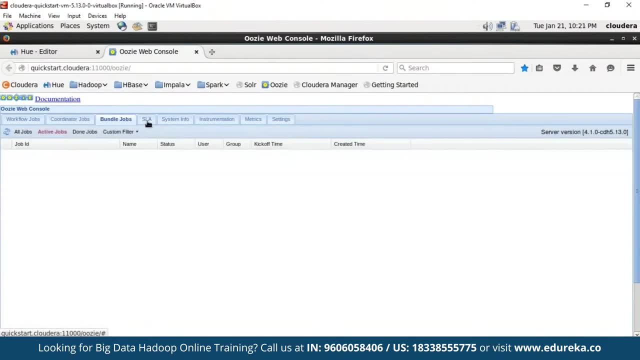 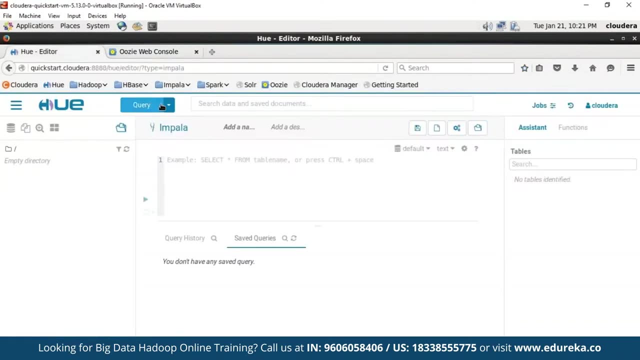 which I mentioned in the previous explanation, and also the bundle jobs, SLA system, info, instrumentation, metrics and all the extra additional settings you require. Now we shall discuss about the editors present in Hue, So to find out the editors in Hue, 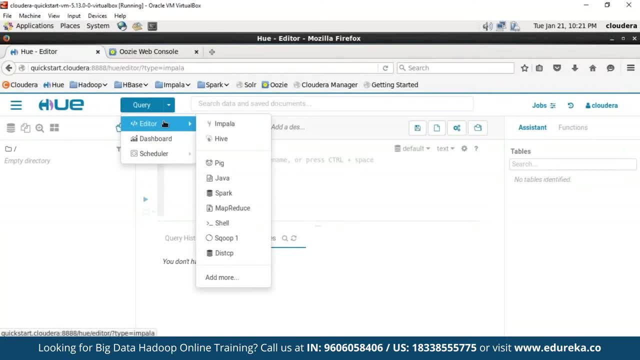 you need to select the button query and inside that you'll be getting a drop down menu and inside the menu select editor and you can see there are various editors present in Hue. that are: Impala, Hive job, Big job, Java code, Spark job. 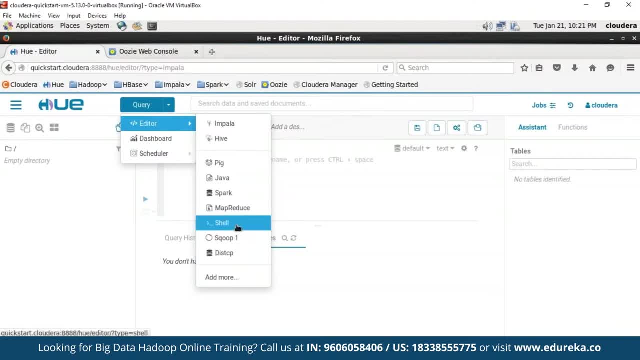 MapReduce, Shell, Scoop and many more. So now that we have understood how to install Uzi into local system and the editors present in Hue and the Uzi web console, we shall advance ahead and understand the advantages of Uzi. 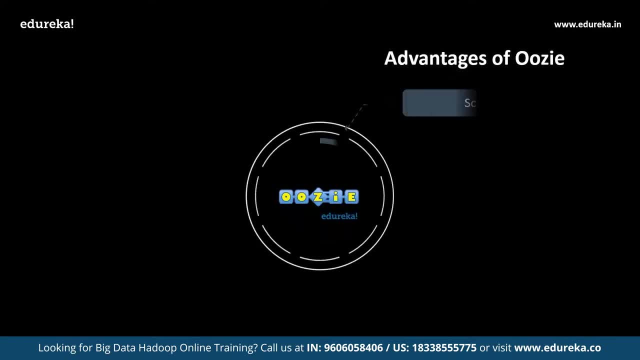 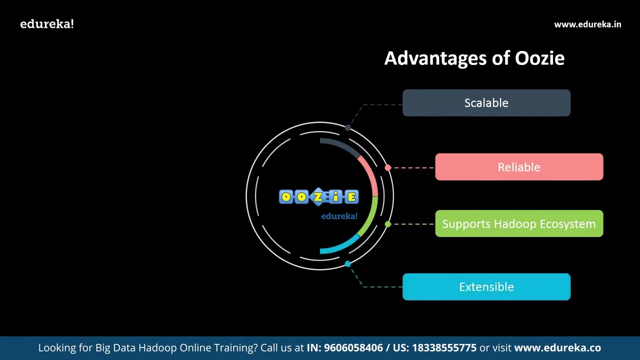 The first among the advantages of Uzi is: Uzi is scalable and reliable to monitor jobs in Hadoop cluster. Uzi supports various jobs in Hadoop ecosystem like MapReduce, Pig, Hive Streaming and also Java based applications. Uzi has an extensible architecture. 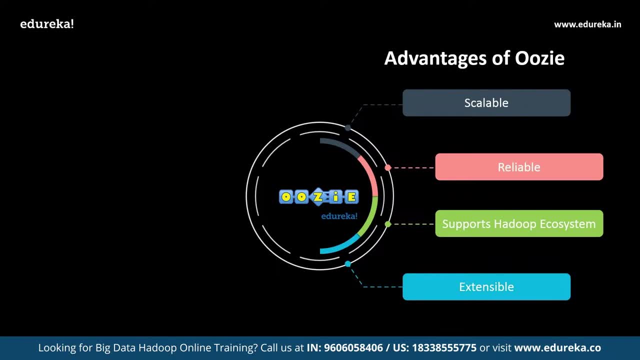 that supports great programming paradigms. The next advantage is complex workflow action and dependencies. Uzi workflow comprises of actions and dependencies, among them, followed by complex workflow action dependencies. We have reduced the time-to-market system. The directed acyclic graph specification enables users 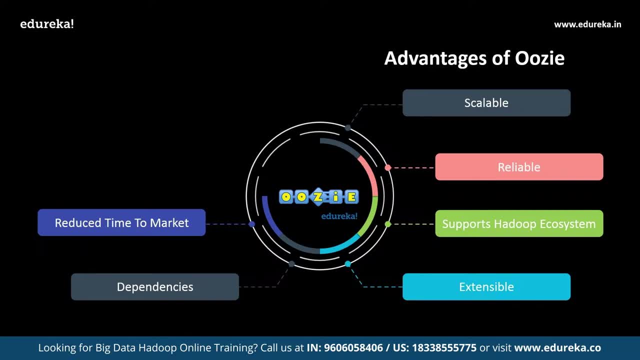 to specify the workflow, So this saves a lot of time to market, followed by TTM. We have frequency execution: Users can specify execution frequency and can wait for data arrival to trigger an action on the workflow, followed by frequency execution. We have native Hadoop stack integration. 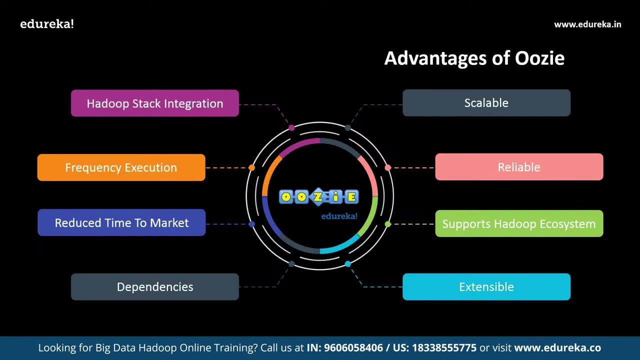 Uzi supports all type of jobs, such as Spark, Hive, Pig and many more. Uzi is validated against Hadoop stack and Uzi is integrated with Yahoo distribution of Hadoop with security and is a primary mechanism to manage a variety of complex data analysis. 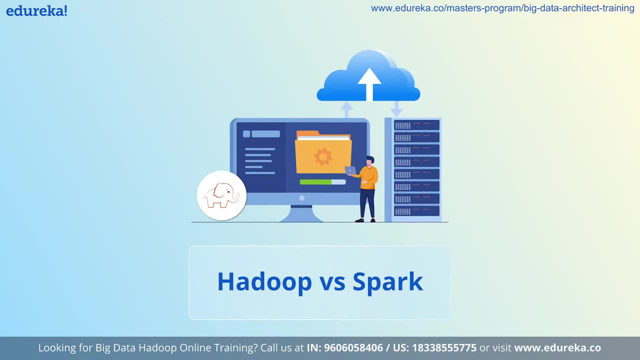 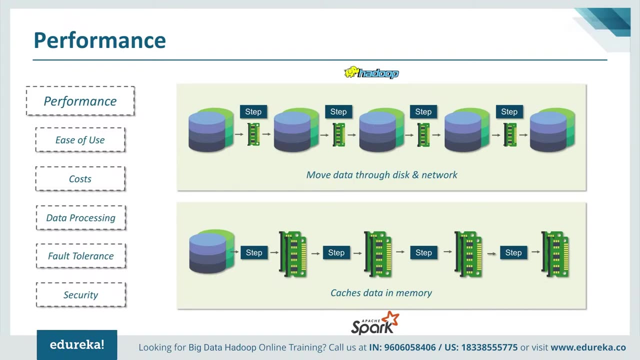 Let's compare Apache Spark with Hadoop on different parameters to understand their strengths. We will be comparing these two frameworks based on these parameters. Let's start with performance first. Spark is fast because it has in-memory processing. It can also use disk for data that doesn't fit into memory. 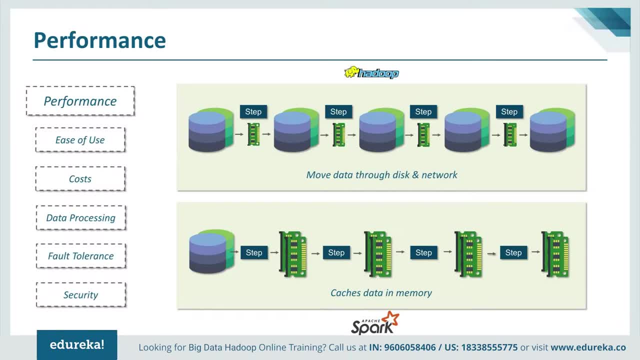 Sparks in-memory processing delivers near real-time analytics, And this makes Spark suitable for credit card processing system, machine learning, security analytics and processing data for IoT sensors. Now let's talk about Hadoop's performance. Now. Hadoop was originally designed to continuously gather data. 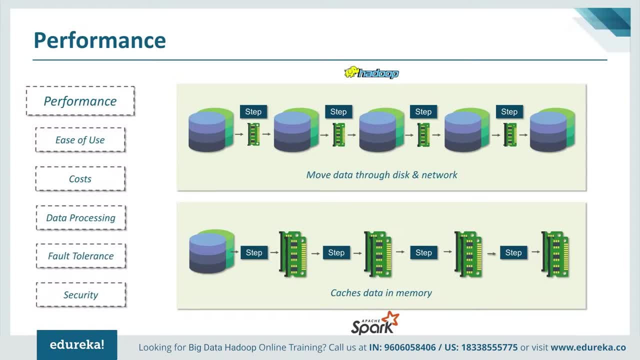 from multiple sources without worrying about the type of data and storing it across distributed environment, And MapReduce uses batch processing. MapReduce was never built for real-time processing. Main idea behind YARN is parallel processing over distributed data set. The problem with comparing the two is that they have different way. 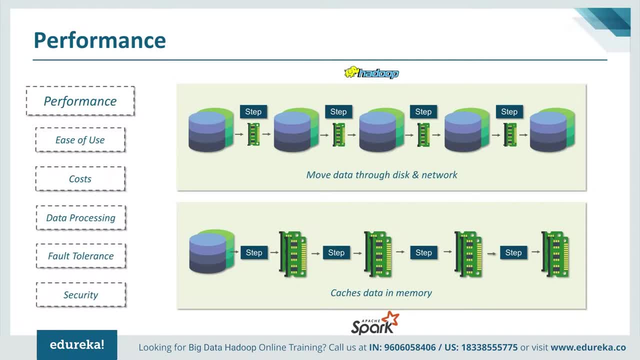 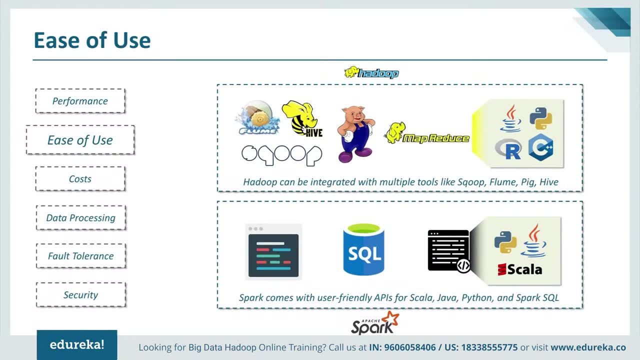 of processing and the idea behind the development is also divergent. Next, ease of use. Spark comes with a user-friendly APIs for Scala, Java, Python and Spark SQL. Spark SQL is very similar to SQL, So it becomes easier for SQL developers to learn it. 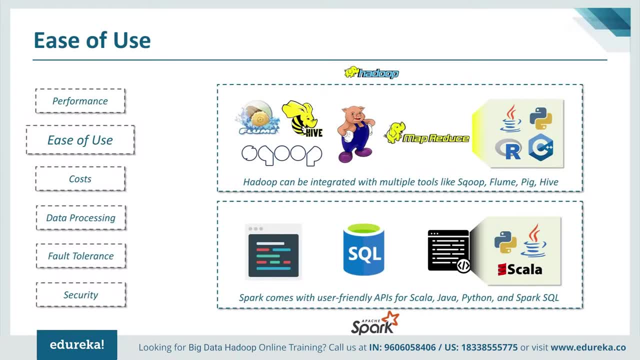 Spark also provides an interactive shell for developers to query and perform other actions and have immediate feedback. Now let's talk about Hadoop. You can ingest data in Hadoop easily, either by using shell or integrating it with multiple tools like Scoop and Flume. 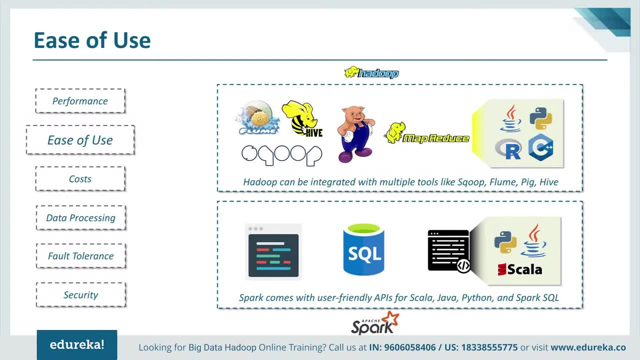 And YARN is just a processing framework that can be integrated with multiple tools like Hive and Pig for analytics. Hive is a data warehousing component which performs reading, writing and managing large data set in a distributed environment using SQL-like interface. To conclude here, both of them have their own ways to make themselves user-friendly. 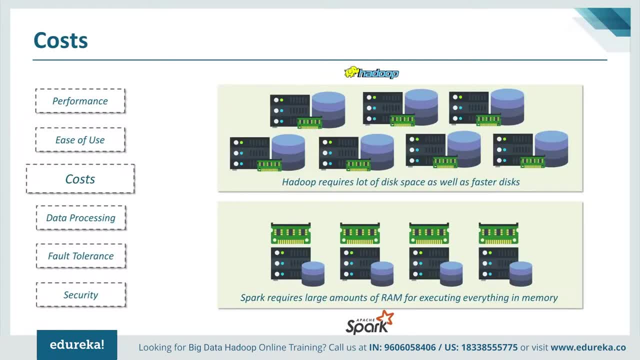 Now let's come to the costs. Hadoop and Spark are both Apache open source projects, So there's no cost for the software. Cost is only associated with the infrastructure. Both the products are designed in such a way that it can run on commodity hardware with low TCO. 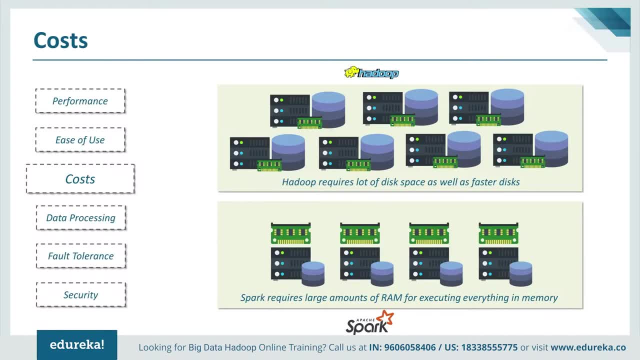 cost of ownership. Well now you might be wondering the ways in which they are different. They're all the same. Storage and processing in Hadoop is disk-based and Hadoop uses standard amounts of memory. So with Hadoop we need a lot of disk space as well as faster transfer speed. 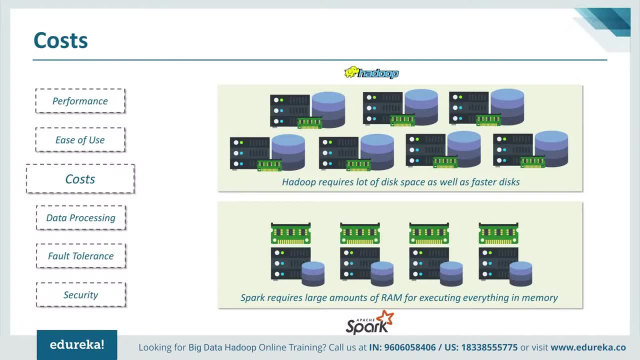 Hadoop also requires multiple systems to distribute the disk input output, But in case of Apache Spark, due to its in-memory processing it requires a lot of memory, But it can deal with a standard speed and amount of disk, As disk space is a relatively inexpensive commodity. 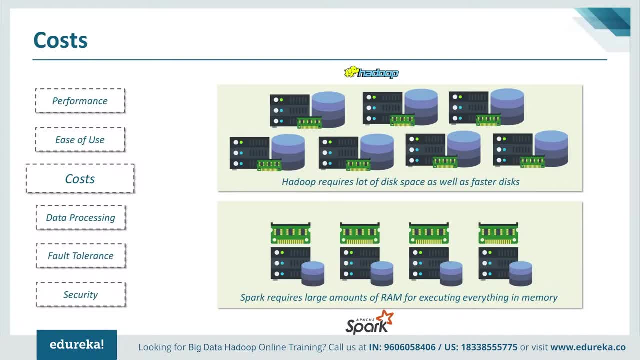 and since Spark does not use disk input output for processing, instead it requires large amounts of RAM for executing everything in memory. So Spark systems incurs more cost. But yes, one important thing to keep in mind is that Spark's technology reduces the number of required systems. 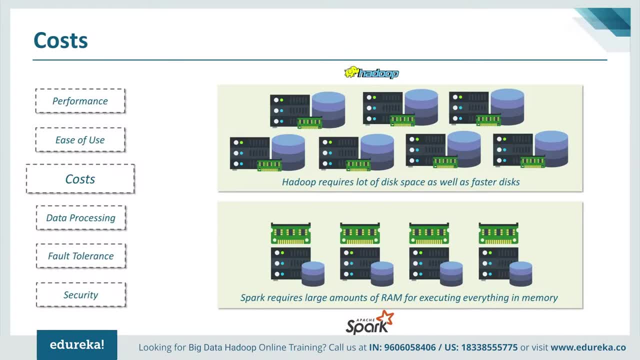 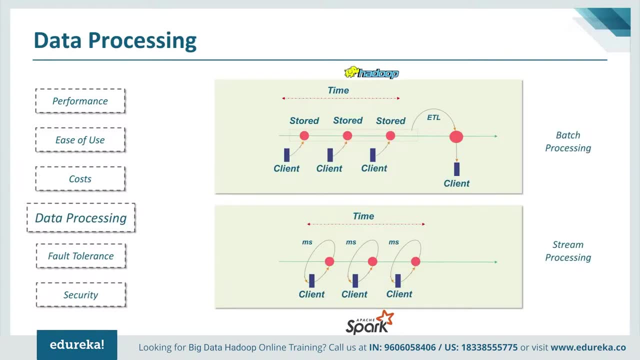 It needs significantly fewer systems that cost more, So there will be a point at which Spark reduces the cost per unit of the computation, even with the additional RAM requirement. There are two types of data processing: batch processing and stream processing. Batch processing has been crucial to the big data world. 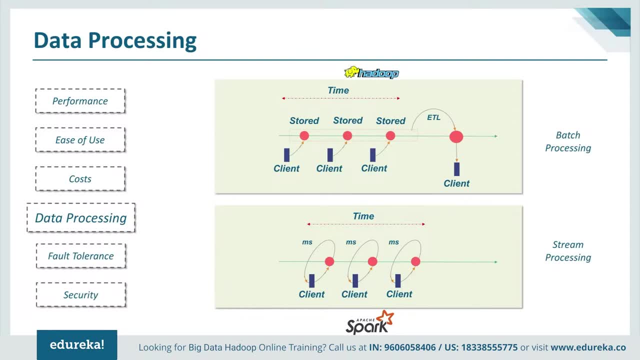 In simplest term, batch processing is working with high data volumes collected over a period. In batch processing, data is first collected, then processed and then the results are produced at a later stage, And batch processing is an efficient way of processing large static data sets. 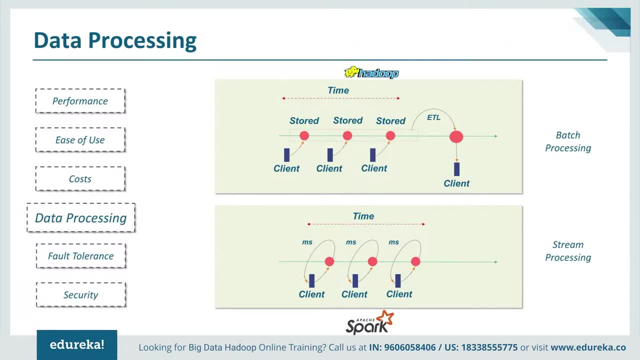 Generally, we perform batch processing for archived data sets, For example, calculating average income of a country or evaluating the change in e-commerce in the last decade. Now stream processing. Stream processing is the current trend in the big data world. Need of the hour is speed and real-time information. 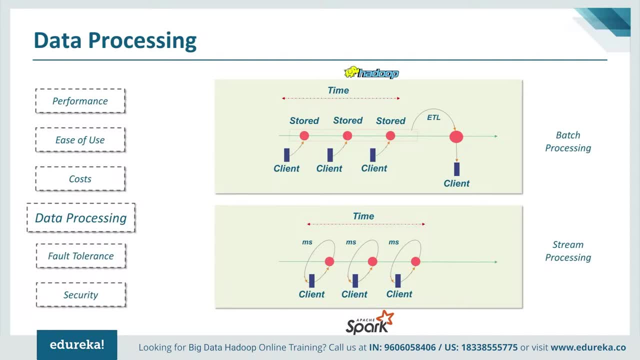 which is what stream processing does. Batch processing does not allow businesses to quickly react to changing business needs in real time. Stream processing has seen a rapid growth in that demand. Now coming back to Apache, Spark versus Hadoop, YARN is basically a batch processing framework. 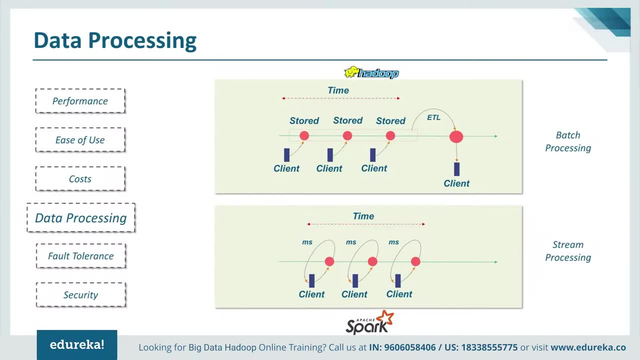 When we submit a job to YARN, it reads data from the cluster, performs operation and write the results back to the cluster. And then it again reads the updated data, performs the next operation and write the results back to the cluster, and so on. 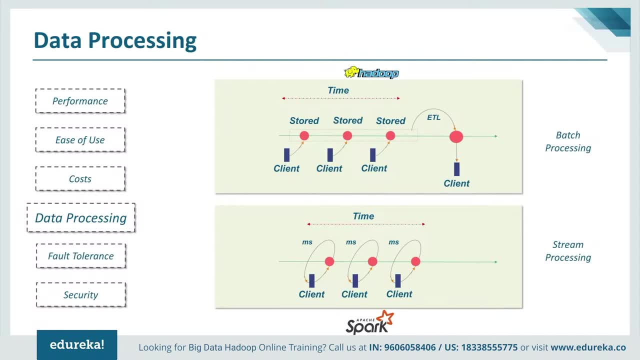 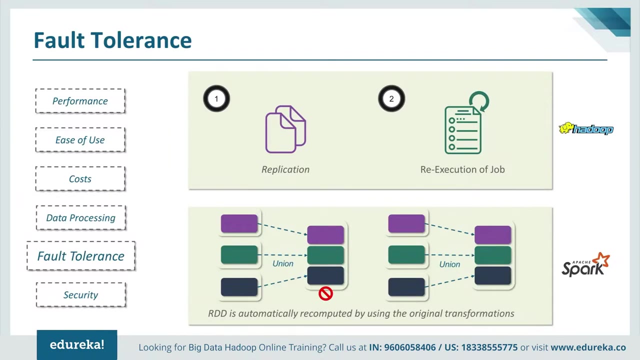 On the other hand, Spark is designed to cover a wide range of workloads, such as batch application, iterative algorithms, interactive queries and streaming as well. Now let's come to fault tolerance. Hadoop and Spark both provides fault tolerance, but have different approaches. 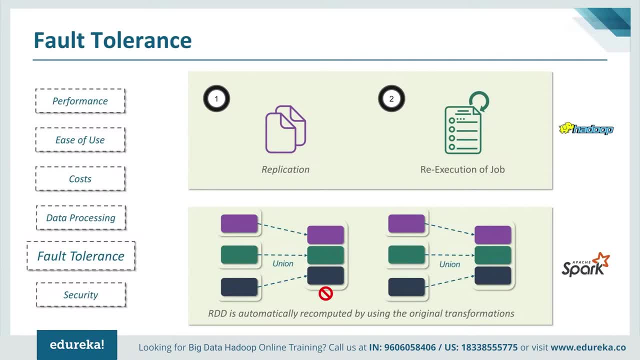 For HDFS and YARN, both master daemons. that is the name node in HDFS and resource manager in YARN checks the heartbeat of the slave daemons. The slave daemons are data nodes and node managers. So if any slave daemon fails, 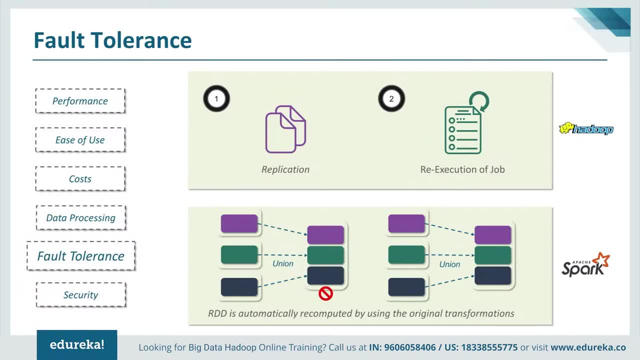 the master daemon reschedules all pending and in-progress operations to another slave. Now this method is effective, but it can significantly increase the completion time for operations with single failure. also, And as Hadoop uses commodity hardware, another way in which HDFS ensures fault tolerance is by replicating data. 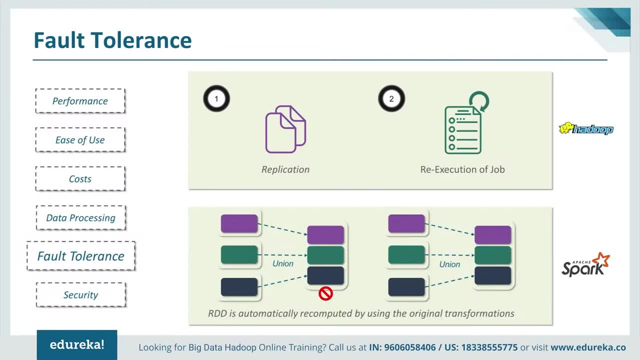 Now let's talk about Spark, As we discussed earlier, RDDs, or Resilient Distributed Datasets, are building blocks of Apache. Spark And RDDs are the ones which provide fault tolerance to Spark. They can refer to any dataset present in an external storage system. 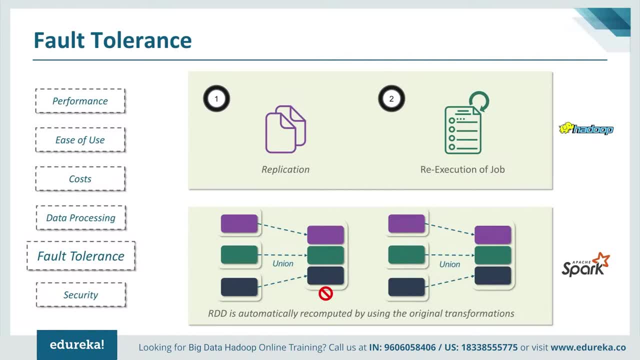 like HDFS, edgebase, shared file system, etc. They can also be operated parallelly. RDDs can persist a dataset in memory across operations, which makes future actions 10 times much faster. If a RDD is lost, it will automatically get recomputed by using the original transformations. 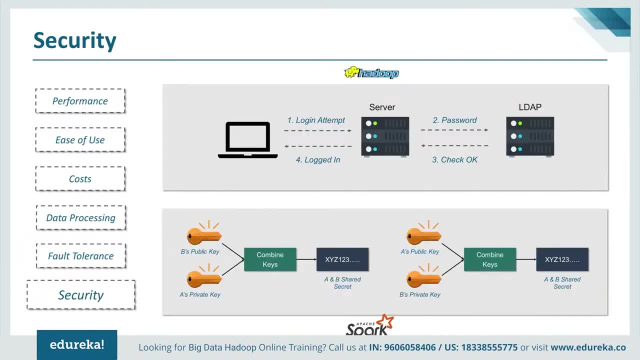 And this is how Spark provides fault tolerance. And at the end, let us talk about security. Well, Hadoop has multiple ways of providing security. Hadoop supports Kerberos for authentication, but it is difficult to handle. Nevertheless, it also supports third-party vendors like LDAP. 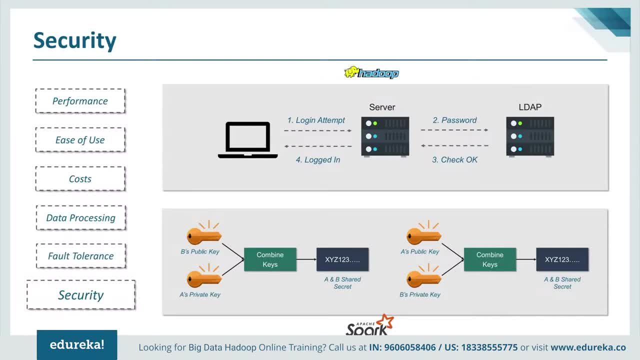 For authentication. they also offer encryption. HDFS supports traditional file permissions as well as access control lists. Hadoop provides service-level authorization, which guarantees that clients have the right permissions for job submission. Spark currently supports authentication via a shared secret. Spark can integrate with HDFS and it can use HDFS ACLs. 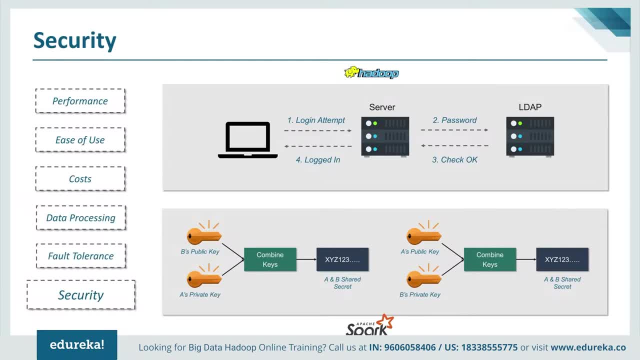 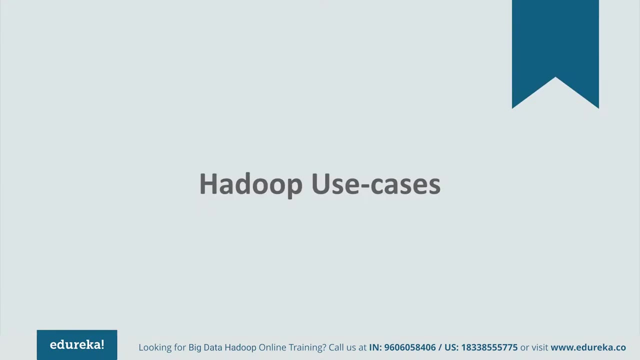 or access control lists and file-level permissions. Spark can also run on YARN, leveraging the capability of Kerberos. Now, this was the comparison of these two frameworks, based on these following parameters. Now let us understand use cases where these technologies fit best. 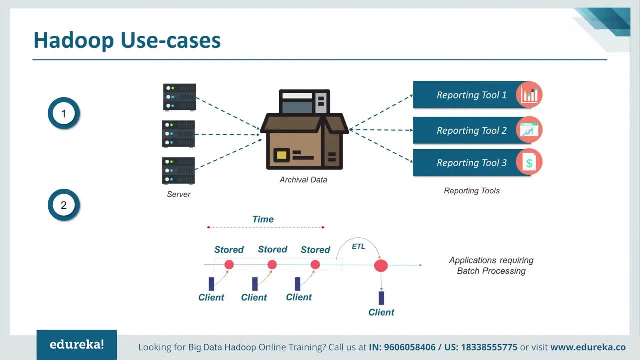 Use cases where Hadoop fits best, For example, when you are analyzing archived data. YARN allows parallel processing over huge amounts of data. Parts of data is processed parallelly and separately on different data nodes and gathers result from each node manager. 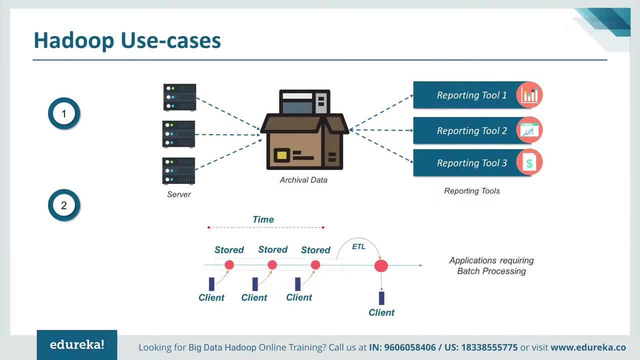 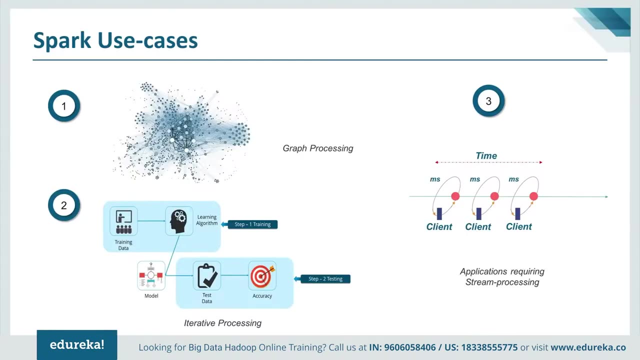 In cases when instant results are not required. Hadoop MapReduce is a good and economical solution for batch processing. However, it is incapable of processing data in real-time Use cases, where Spark fits best In real-time big data analysis. Real-time data analysis means processing data that is getting generated. 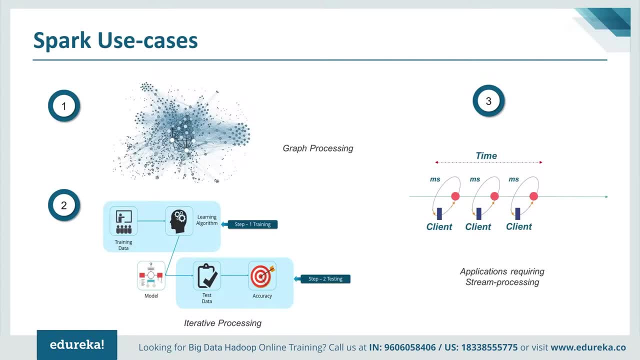 by the real-time event streams coming in at the rate of millions of events per second. The strength of Spark lies in its abilities to support streaming of data, along with distributed processing, And Spark claims to process data 100 times faster than MapReduce, while 10 times faster with the disks. 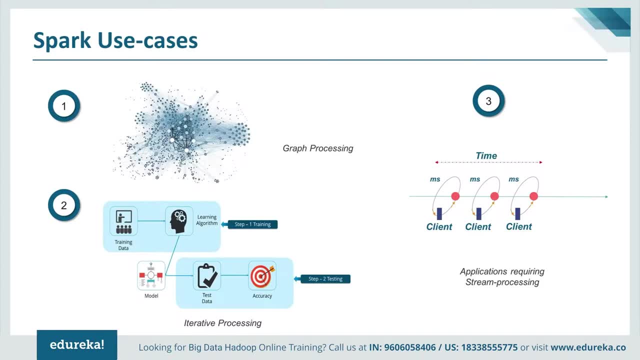 It is used in graph processing. Spark contains a graph computation library called GraphX, which simplifies our life In-memory computation. along with in-built graph support, improves the performance of algorithm by a magnitude of 1 or 2 degrees over traditional MapReduce programs. 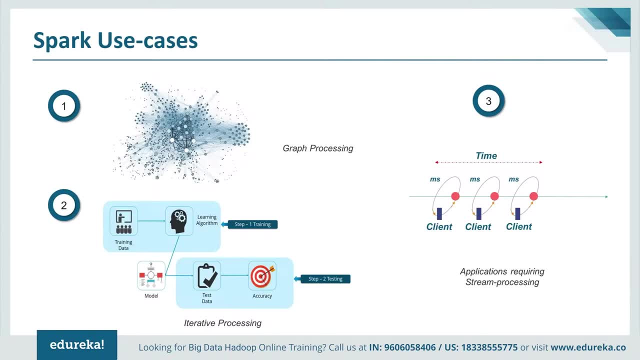 It is also used in iterative machine learning algorithms. Almost all machine learning algorithms work iteratively. As we have seen earlier, iterative algorithms involve input-output bottlenecks in the MapReduce implementations. MapReduce uses coarse-grained tasks that are too heavy for iteration. 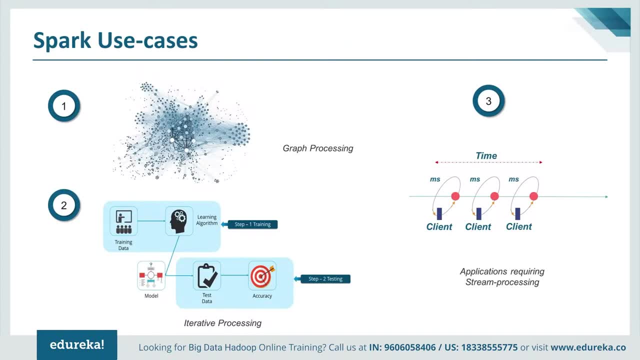 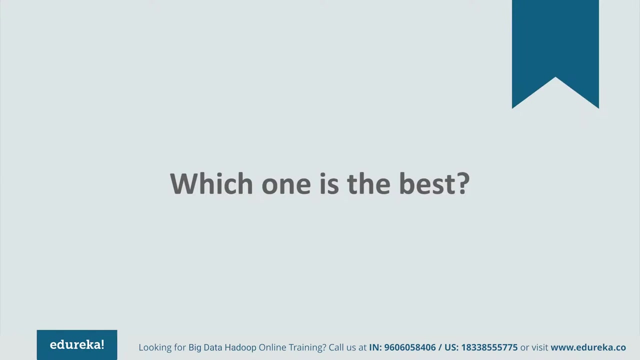 Spark caches the intermediate dataset after each iteration and runs multiple iterations on the cached dataset, which eventually reduces the input-output overhead and executes the algorithm faster in a fault-tolerant manner. So at the end, which one is the best? The answer to this is: Hadoop and Apache Spark are not competing with one another. 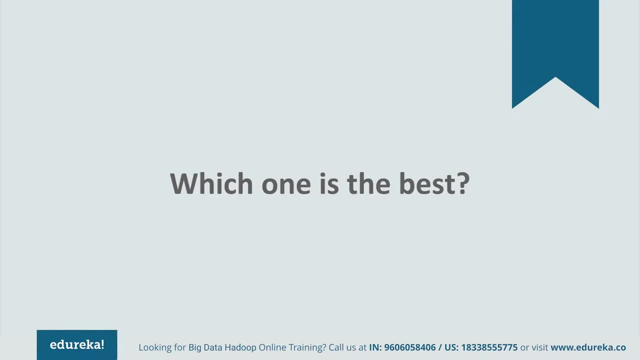 In fact, they complement each other quite well. Hadoop brings huge datasets under control by commodity systems and Spark provides real-time in-memory processing for those datasets. When we combine Apache Spark's ability, that is, the high processing speed and advanced analytics. 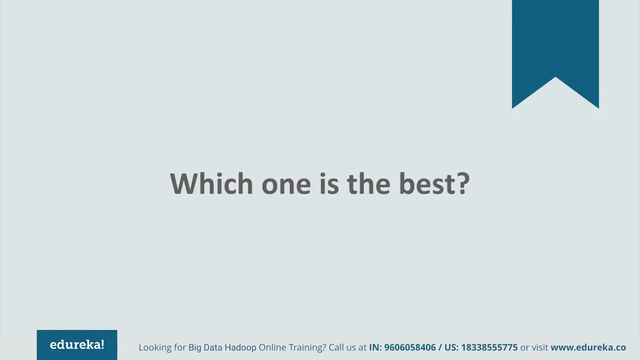 and multiple integration support. with Hadoop's low-cost operation on commodity hardware, it gives the best results. Hadoop complements Apache Spark's capabilities. Spark cannot completely replace Hadoop, but the good news is that the demand of Spark is currently at an all-time high. 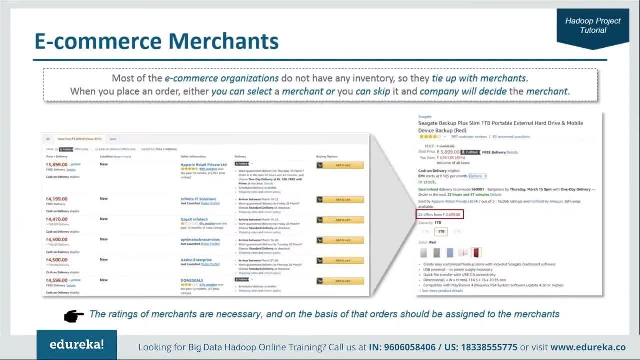 So this project is based on the e-commerce domain, So let me give you an introduction to this project in context of one of the biggest names of e-commerce platforms, none other than Amazon. So if you have ever shopped from Amazon before, which I presume you must have- 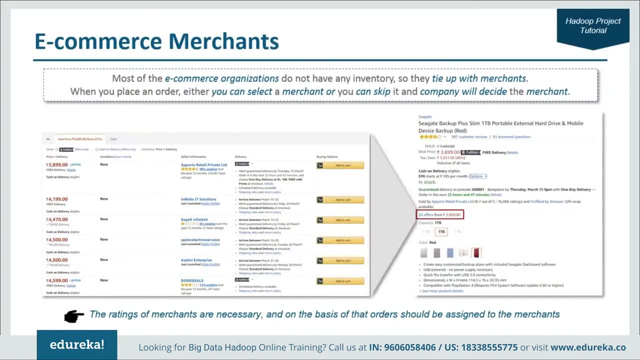 you must have seen something like this when you click on a product So you'll view the details of the product. something like this. And, as you know, most of the e-commerce organizations do not have any inventory, so they tie up with different merchants. 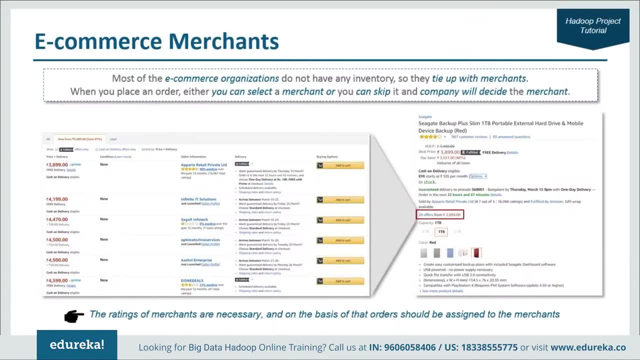 Similar is the case with Amazon. Amazon provides the merchants or the sellers a platform to get connected to the buyers. So when you click on the details of a product, you can see that Amazon gives you something like this, And you also find something like this: 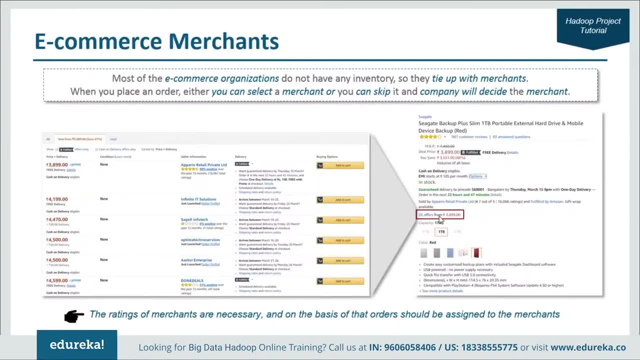 There are 28 offers from this price And if you click on it you can see the name of the different sellers who are selling the same product at different prices, And the prices they're offering are listed like this, But you can see over here that by default. 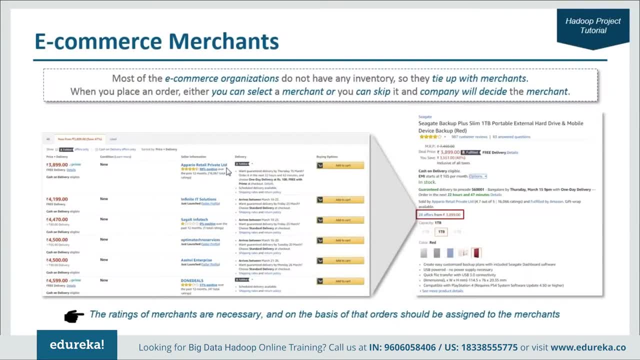 Amazon has selected the Apario Real Estate. It's a retail, private, limited for this particular product. So how does Amazon do that? So it is actually based on a merchant rating system And as a platform, as an e-commerce platform, you have to ensure that you always display the product. 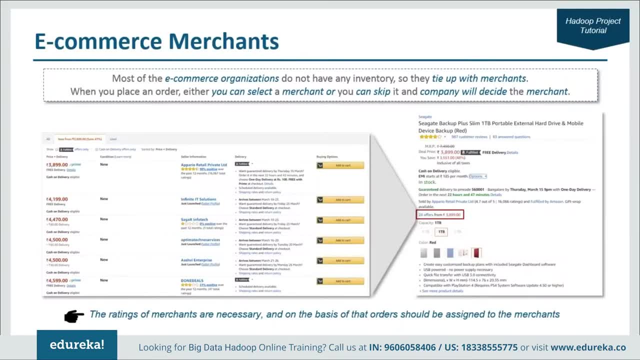 from the best merchant in order to ensure quality, because you don't want angry customers, right? So it is very important that your customers are satisfied with their product. So you have to choose from different merchants for the same product in order to decide which merchant's product needs to get displayed by default. 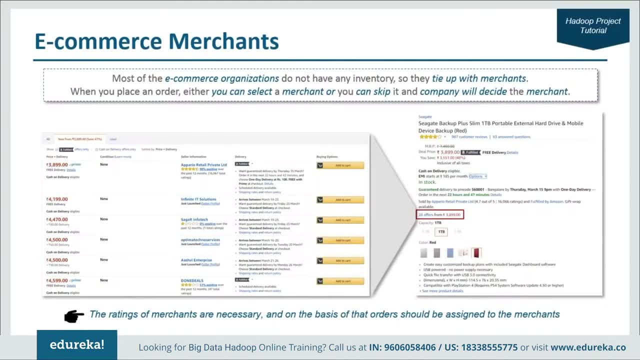 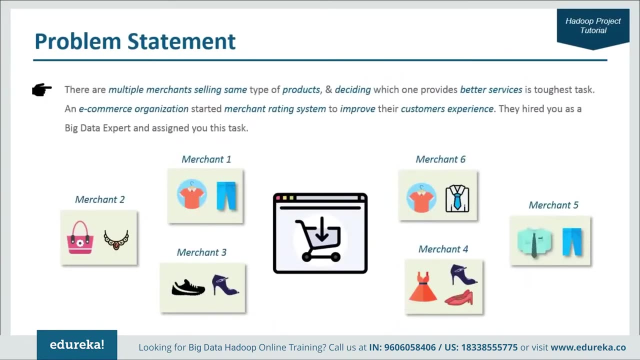 And hence Amazon has a merchant rating system in order to decide that, And this is what exactly we're going to build. All right, So we're going to make a merchant rating system similar to this. So here is the problem statement. So there are multiple merchants selling the same type. 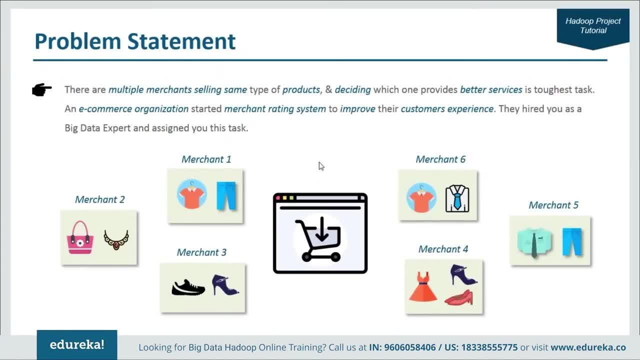 of products, As you can see that merchant one and merchant six are selling the same shirt, Merchant three and four are selling the same shoes And similarly, five and one are selling the same pants, And there are multiple other merchants who are selling the same kind of products. 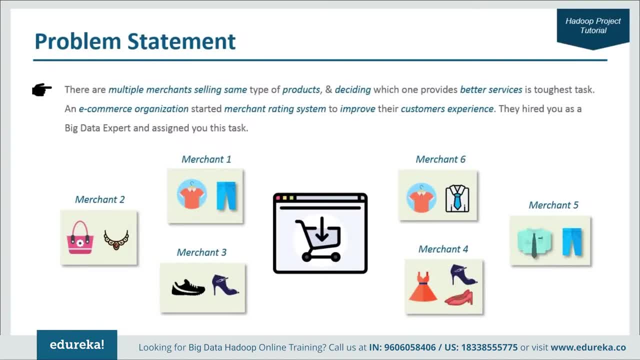 And you have to build a merchant rating system, or the company wants to build a merchant rating system in order to determine which merchant sells the best product, so that their product would be displayed by default. And as a big data expert, let's just assume that you were hired by the company. 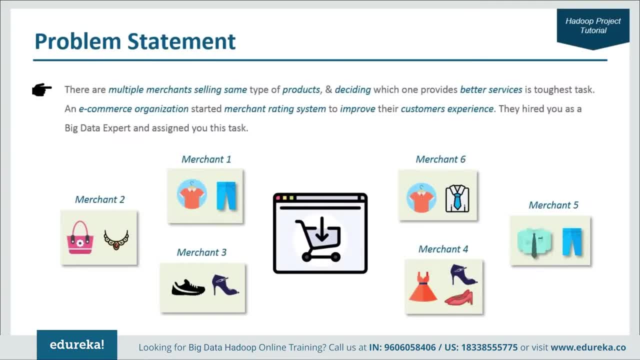 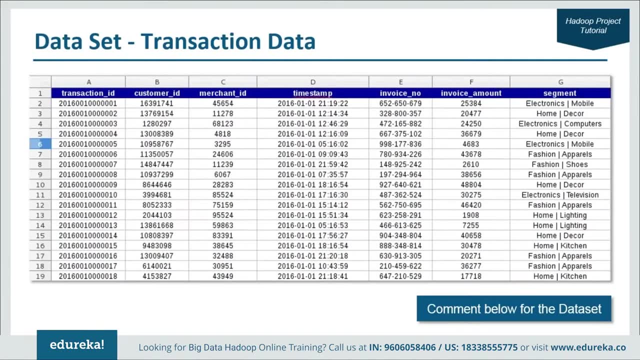 as a big data expert, you are assigned this task, So this is now your problem to solve. So the first thing your organization will give you before you start to do your work is the data set. So this is the data set that you're going to get. 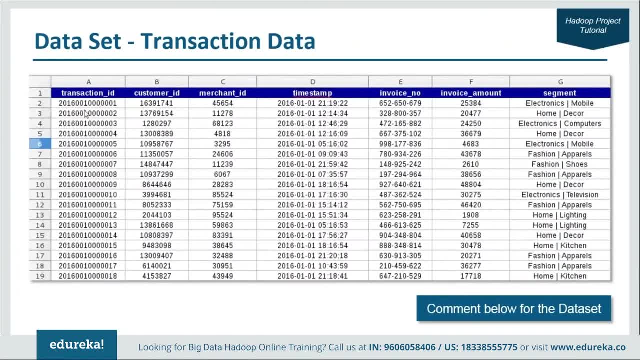 So this is the transaction data set And it has certain fields like transaction ID, customer ID, merchant ID, timestamp when the purchase was made, the invoice number, the amount and the segment of product that was bought. You have another data set. 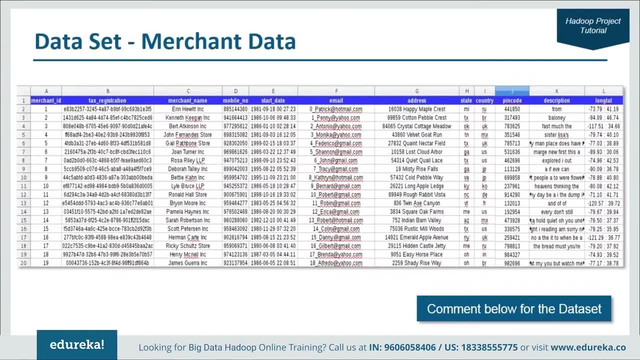 which is the merchant data. So these are the details about the different sellers or the merchants. So you have got your merchant ID, the tax registration number, the merchant name, their mobile number, start date, email address, state, country, pin code, description. 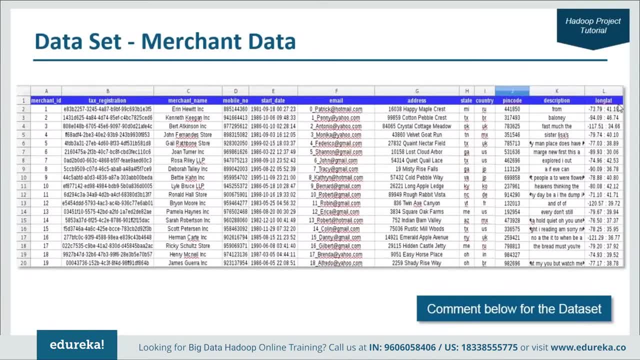 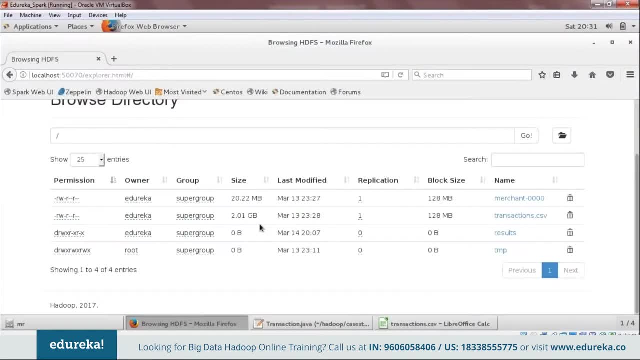 longitude, latitude, the location, basically. So these are all the details about the merchant that you have in your data set. So let me just show you the data set. So this is the data set that is in your HTFS right now. 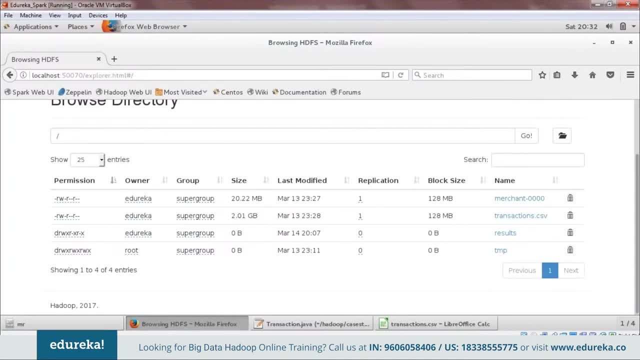 So here is the transaction data. So here is the transaction data, which is a 2GB of file, And the merchant data set, which is 20 MB, Because, as you know, there are many transactions but a limited number of sellers or merchants. 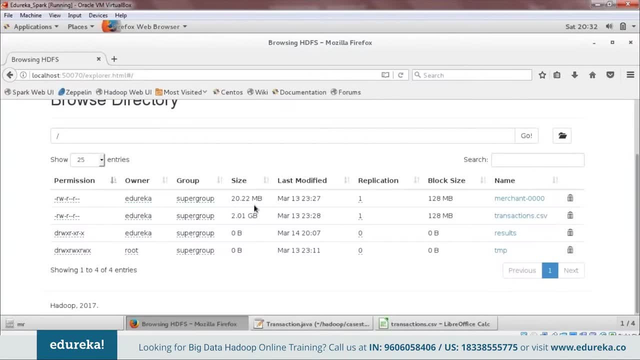 So that is why the size of the data set, the merchant data set, is quite smaller as compared to the transaction one. And, to tell you, we haven't actually used the entire data present in the data set. We have just selected a subset or a sub data set. 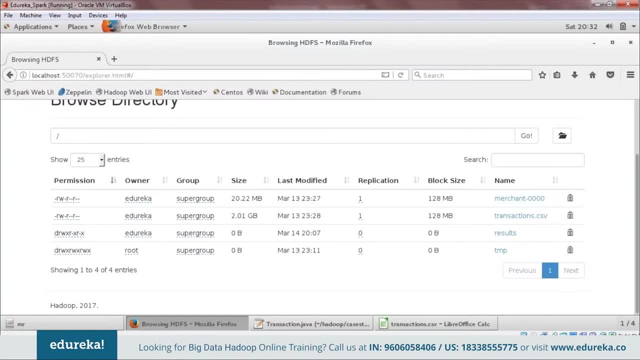 you can say, because the original data set was quite huge And this was a demo project. So, just for your understanding, we have chosen a sub data set. we just took 2GB of data out of it. All right, And this is how it exactly looks like. 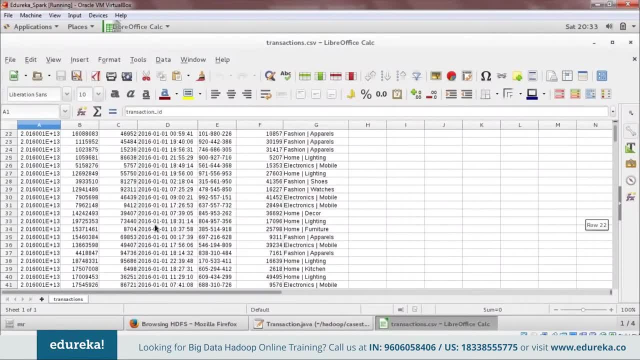 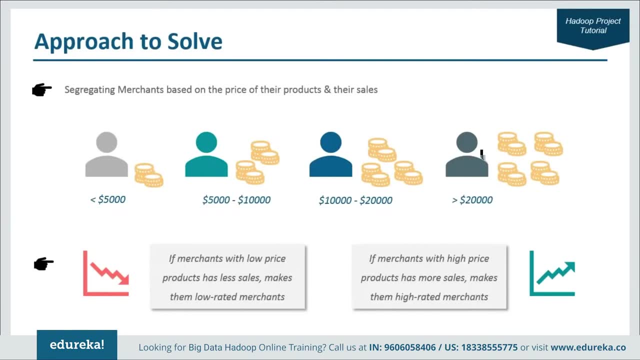 So this is the CSV file of the data set that we have. This is the transactions data. All right, So this is the approach to solve. So the first thing we'll do is that we'll segregate the merchants based on the price of their products. 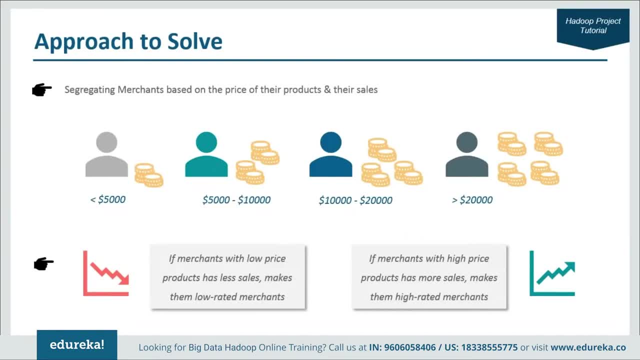 and their sales. So we will be segregating them into four categories. So the categories are the merchants who are selling products that are below $5,000 or less than $5,000.. There is one more category for merchants who sells products between $5,000 to $10,000. 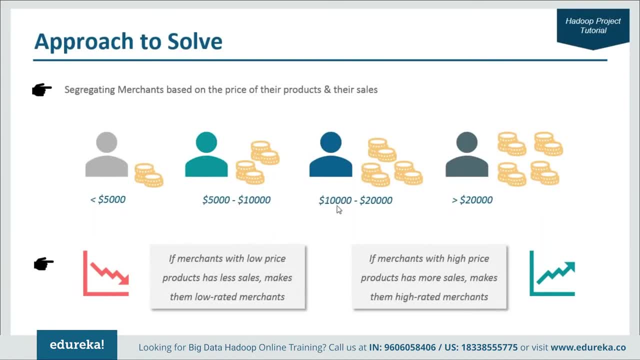 Another category of merchants who sells products between $10,000 to $20,000.. And another category greater than $20,000 or more than $20,000.. We'll be using a simple logic to approach solving this problem. So let's say that 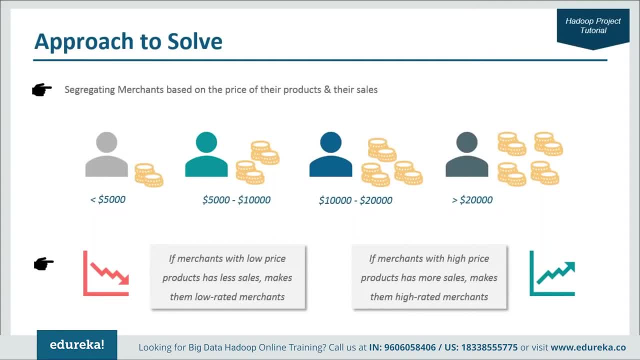 if there is a merchant who's selling their products at quite a low price and you see if he's not making a good number of sales, it means that he is not selling quality products. because if a merchant who's selling the product at quite a less price, 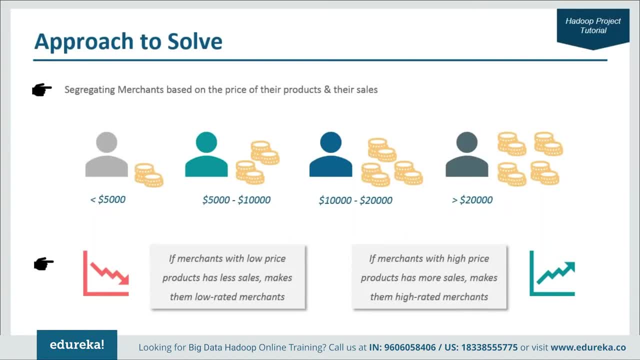 and people aren't still buying from him, it clearly indicates that his products are not up to the mark, So it's a low rating for a merchant. Similarly, on the other hand, if you see a merchant who's selling their product at quite a high price, 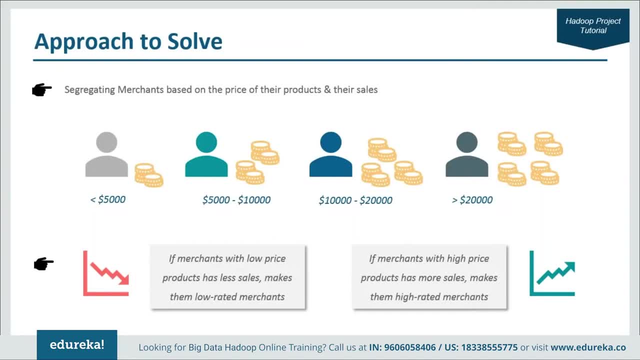 and yet he has a very good number of sales. so it clearly indicates that his products must be very good, because despite of the higher price, people are still buying from him. So in that case, obviously, the rating of the merchant would be also very good. 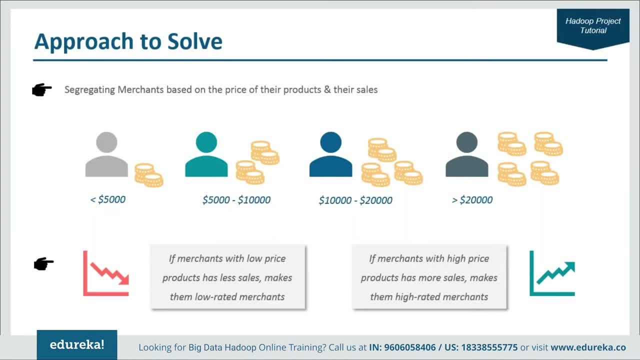 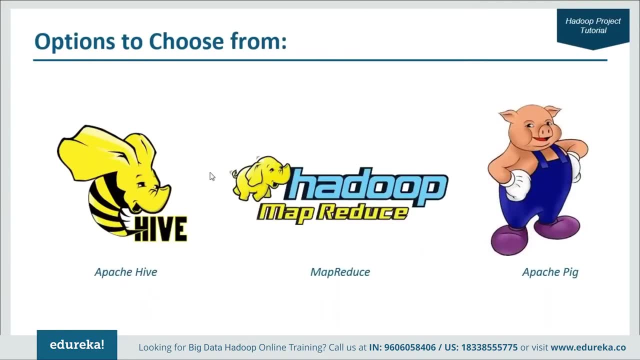 So this is a simple logic that we're going to use in order to rate our merchants or sellers, And you have three options to choose from. So you have got Apache Hive, which is a great analytical tool. We have got Hadoop, MapReduce and Apache Pig. 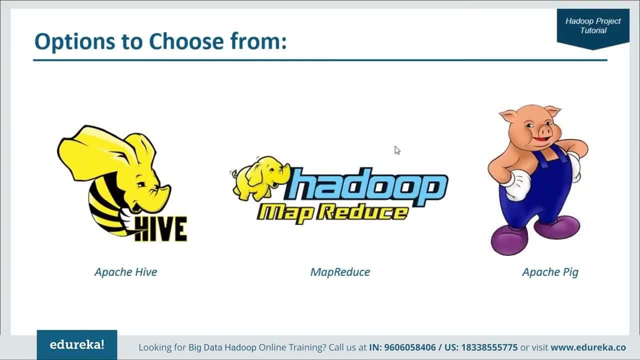 And today we will be choosing Hadoop MapReduce. So MapReduce is the core component of Hadoop that process huge amount of data in parallel by dividing the work into a set of independent tasks. MapReduce is the data processing layer of Hadoop. 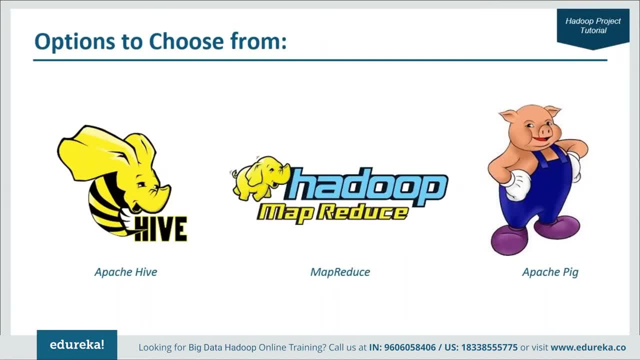 It is a software framework for easily writing applications that processes the vast amount of structured and unstructured data that is stored in your HDFS. HDFS is Hadoop Distributed File System And Hadoop MapReduce works by breaking the data processing into two phases: map phase and the reduce phase. 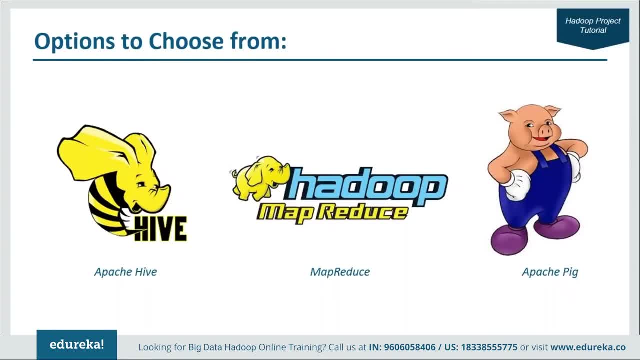 and that is how exactly it gets its name: MapReduce. So the map is the first phase of processing, where we specify all the complex logic, business rules. Reduce is the second phase of processing, where we specify lightweight processing like aggregation or summing up the outputs. 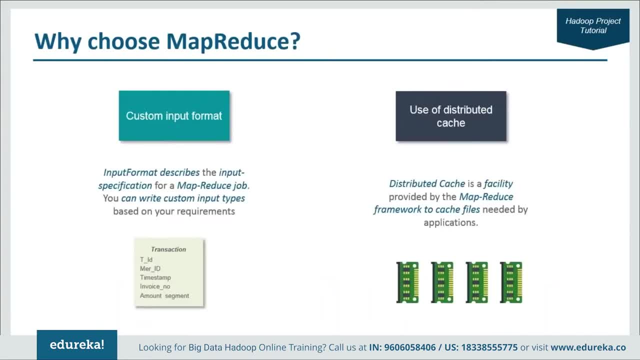 But the question is: why choose MapReduce? Well, I will give you two reasons for it. First is the custom input format. Now, input format is something that defines how your input files are going to be split and read. So in MapReduce, you can create your own custom input format. 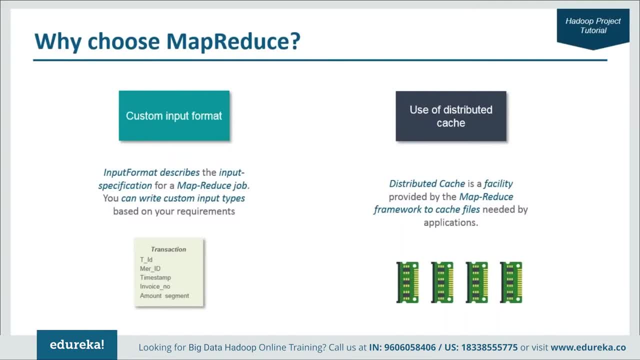 instead of using default input format. This actually makes handling of your data quite easier, because here we can create our custom input format for transactions and pass it as an argument. Then we have the distributed cache. So distributed cache is nothing, but it is a facility. 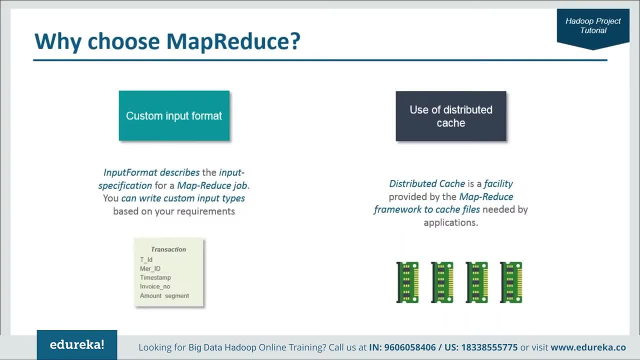 that is provided by MapReduce framework to cache files, Files like your text files, archives, jars, etc. That is needed by your application. Let's understand this with an analogy. Just think about it that there are three students sitting on a table solving chemistry problems. 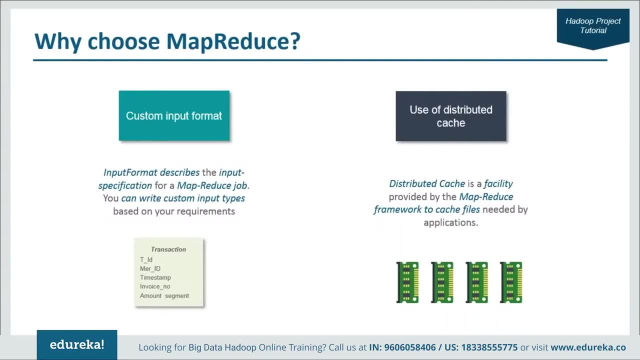 and they have one periodic table. So you keep the periodic table in the middle of the table so all the three students can refer from the periodic table to see the atomic numbers of different elements and solve their problems. So one periodic table, everyone can refer to it. 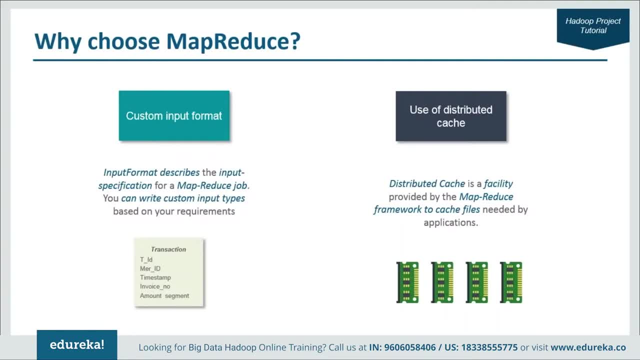 and solve their own problems. So this is what distributed cache is. So with distributed cache, you can put the data that will be used by your different data nodes to refer in order to run MapReduce jobs. So we'll be learning more about how to create your custom input format. 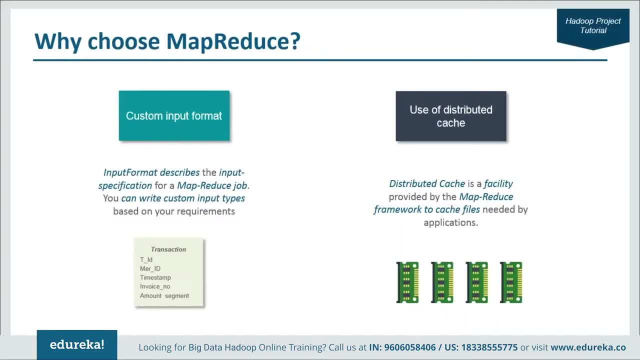 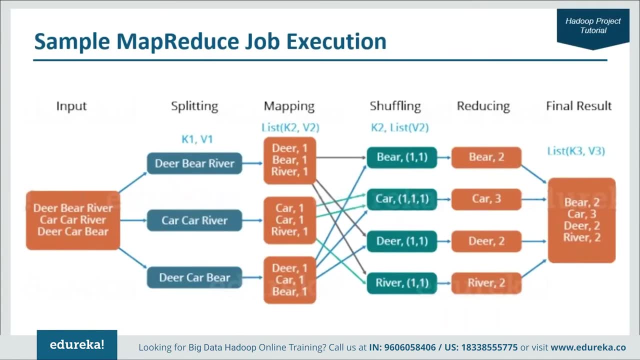 and how to use the distributed cache in the demo part. Alright, So before that, let us just understand how MapReduce exactly works. So this is a sample MapReduce job execution with an example. So this is your input file. This is a text input file. 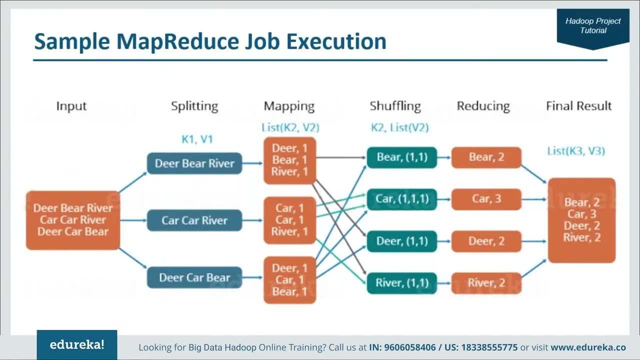 So it contains some words. So first, what will happen is that the input will get divided into three splits. Alright, So I'm taking one sentence at a time, So I have got three splits over here And this will distribute the work among all the different map nodes. 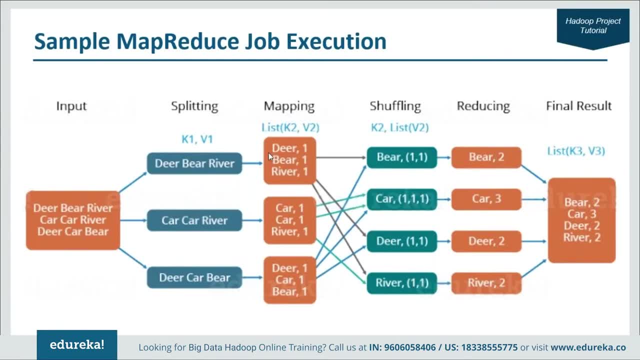 Then we will tokenize the words in each of the mapper and give value one to each of the tokens or words: So dear one bear one, river one. Similarly here: car one, car one, river one. And now a list of key value pair will be created. 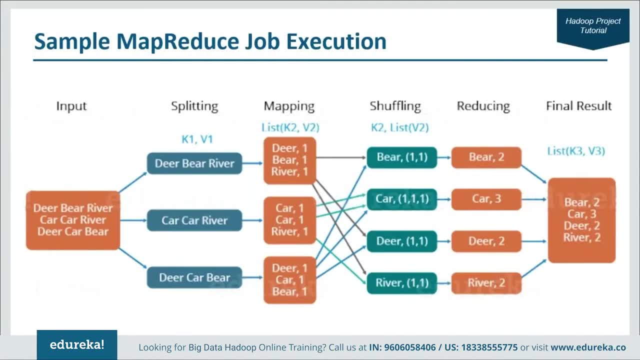 where the key is nothing but the individual word and the value is one. So this is the key and this is the value, And this will happen on all the three nodes. So the mapping process will remain same on all the nodes. So after the mapper phase, 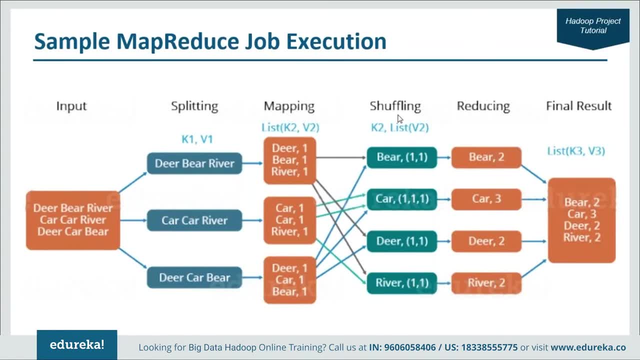 a partition process takes place where the sorting and shuffling happens. Here all the tuples with the same key are sent to the corresponding reducer. So all the bear are together, cars are together, deer and river are together. So after the sorting and shuffling phase, 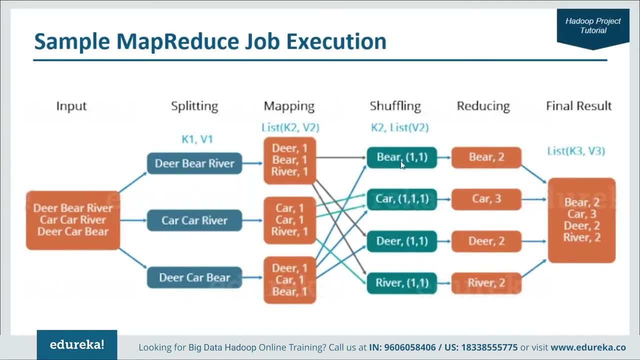 each reducer will have a unique key and a list of corresponding values to that key. For example, bear one, one, car one one and one and so on. Now comes the reducing phase. Now each reducer counts the values which are present in the list of values. 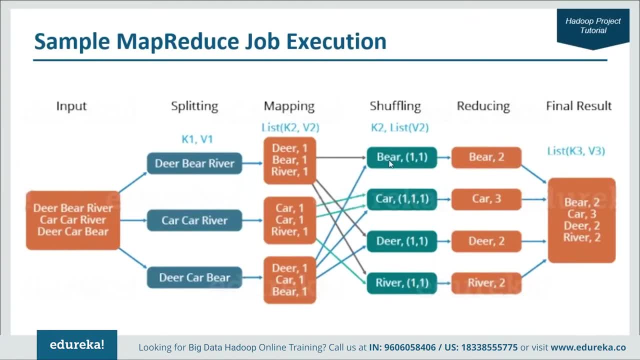 So reducer gets a list of values which is one, one for the key bear, And then it counts the number of ones in the list and gives the final output as bear two. Similarly, for car it's three deer, two river will count two ones, so two. 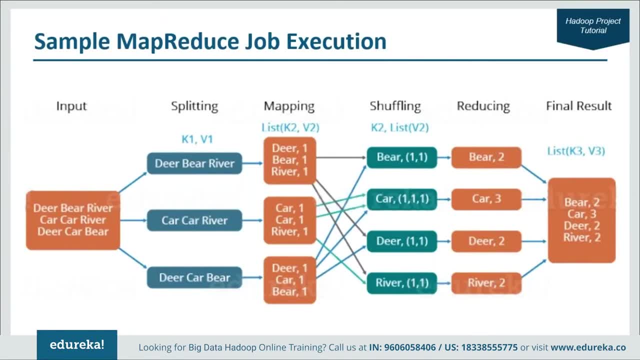 And finally all the output. the key value pairs are then collected and written in the output files. So this is your output file. So it has just combined the result from different reducers And here is your final output. So understood MapReduce with the classic example. 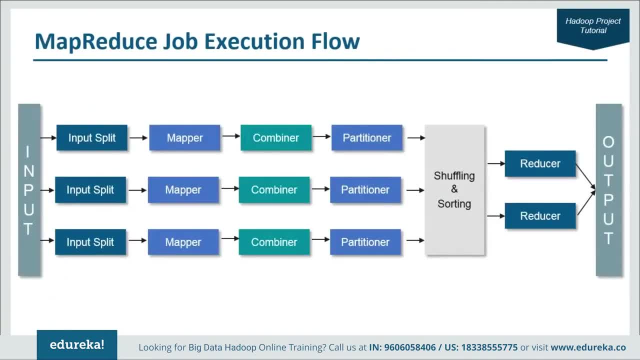 of the word count program. Now, this is the generic execution flow of the MapReduce job. So you have your input file over here. So the data from MapReduce task is stored in input files, and input files typically lives in the HDFS. The format of these files is arbitrary. 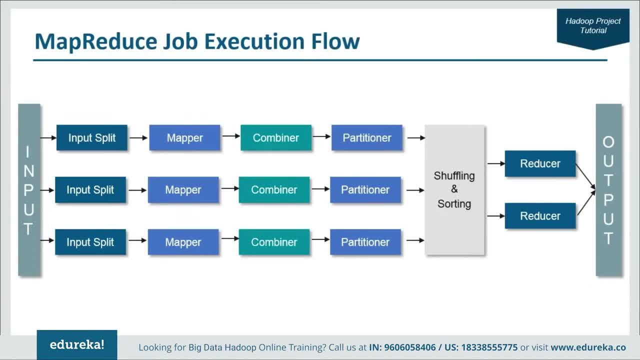 while line-based log files and binary format can also be used And you have an input format. Now, input format defines how these input files are split and read. It selects the files or other objects that are used for input, And input format creates the input split. 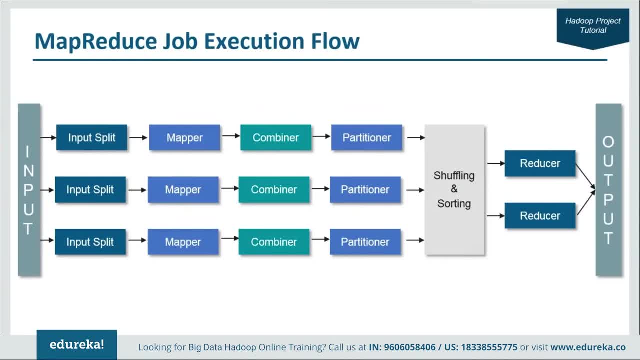 So it logically represents the data which will be processed by an individual mapper. One map task is created for each split, and thus the number of map tasks will be equal to the number of input splits. The splits are then divided into records, and each record will be processed by the mapper. 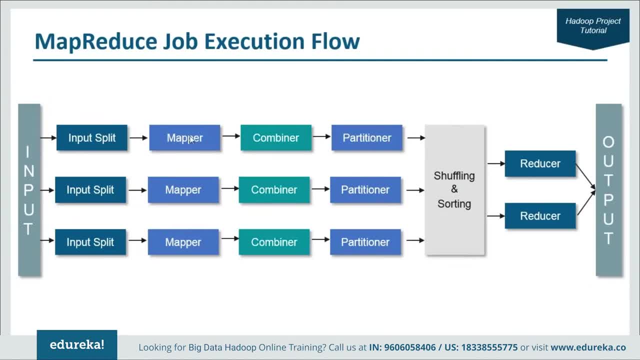 Now let's talk about the mapper. So mapper processes each input record from the record reader and generates a key value pair. And this key value pair is generated by the mapper is completely different from the input pair. The output of the mapper is also known. 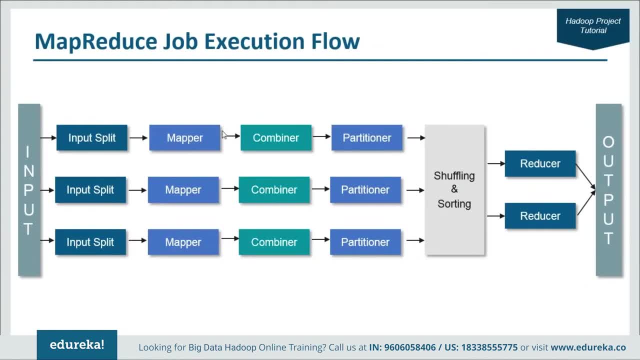 as the intermediate output which is written to the local disk. The output of the mapper is not stored on HDFS, as this is temporary data and writing on HDFS will create unnecessary copies. So then the mapper's output is passed on to the combiner for further process. 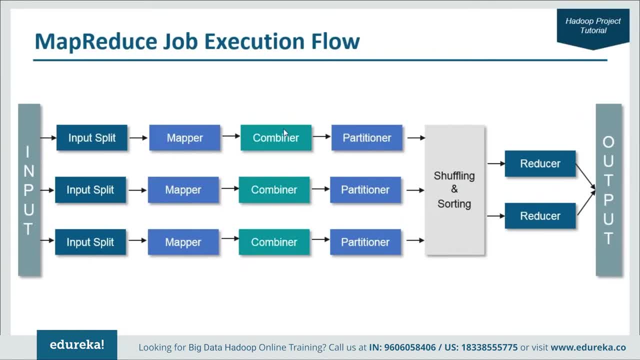 The combiner is also known as the mini reducer. So Hadoop MapReduce combiner performs local aggregation on mapper's output, which helps to minimize the data transfer between mapper and the reducer. Once the combiner functionality is executed, the output is then passed to the partitioner. 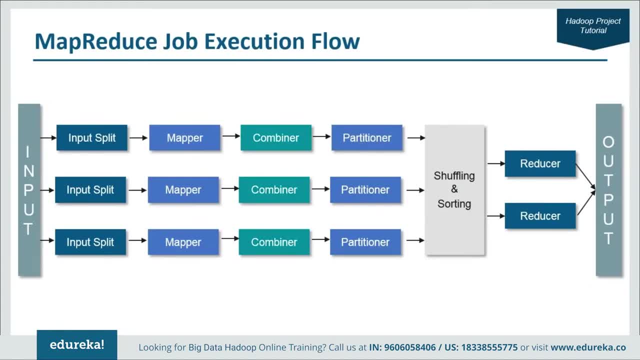 for further work. Now partitioner comes on the picture if you're working on more than one reducer, And here we have two reducers in the example. So if you have one reducer you don't actually need a partitioner, So the partitioner takes the output. 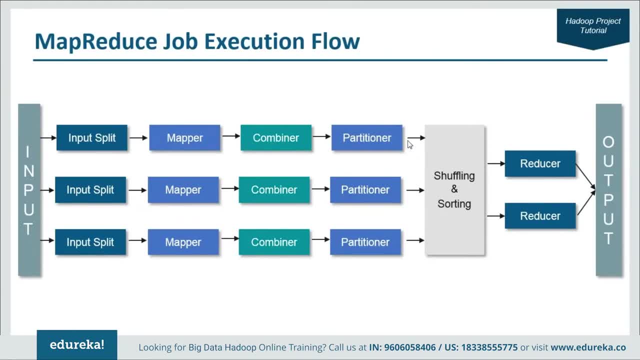 from the combiners and performs partitioning. Partitioning of output takes place on the basis of the key and then sorted So by hash function. a key is used to derive the partition According to the key value. in MapReduce, each combiner output is partitioned. 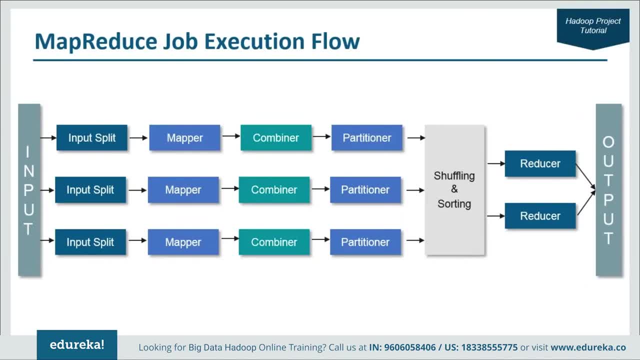 and a record having the same key value goes to the same partition and that each partition is sent to a reducer. So by using partitioner it allows to have an even distribution of the map output over the reducer. So after that comes the shuffling and sorting part. 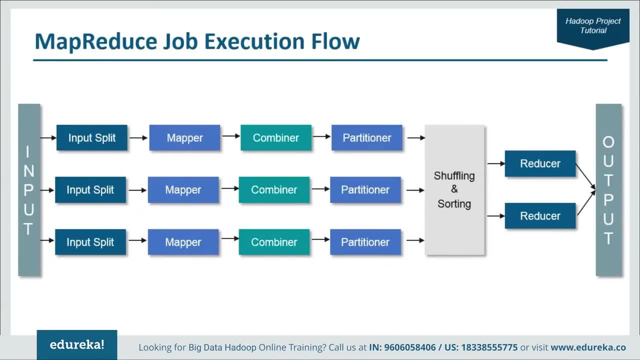 So now the output is shuffled to the reduce node. The shuffling is the physical movement of the data which is done over the network. Once all the mappers are finished and their output is shuffled on the reducer nodes, then this intermediate output is merged and sorted. 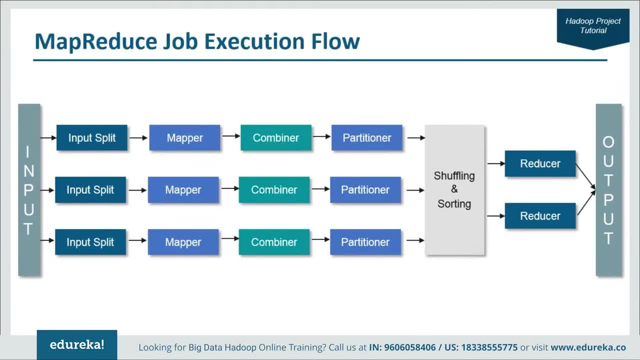 which is then provided as an input to the reduce phase. Now comes the reducer. It takes the set of intermediate key value pairs produced by all the mappers as the input and then runs a reducer function on each of them to generate the output. The output of the reducer is the final output. 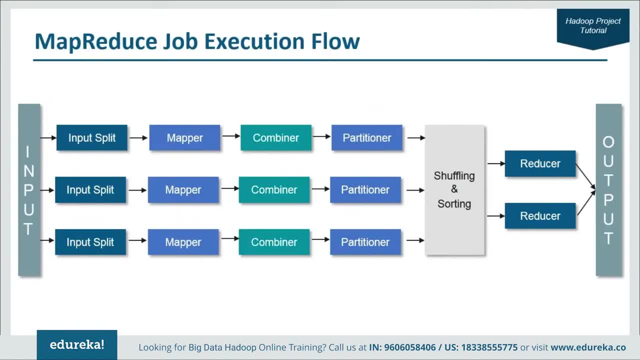 which is stored in HDFS. So if you have multiple reducers, the result from different reducers will combine and that is going to be your final output, which will be written into the HDFS. So this was the map produced job execution flow. So we'll also be using the distributed cache. 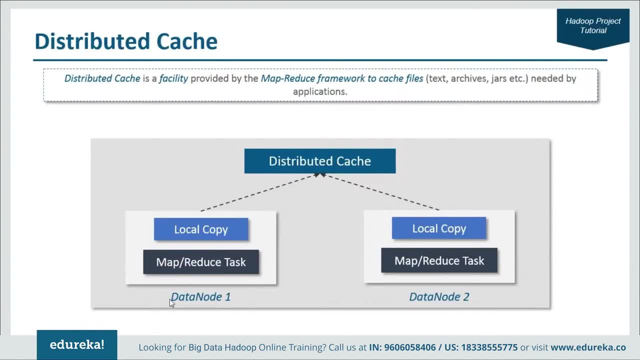 So you'll have different data nodes. Each data node will have their local copy of their data and if each of the data nodes needs to refer something, we will keep that in the distributed cache and in this case we'll be keeping the merchants file, All right. so distributed cache is nothing but. 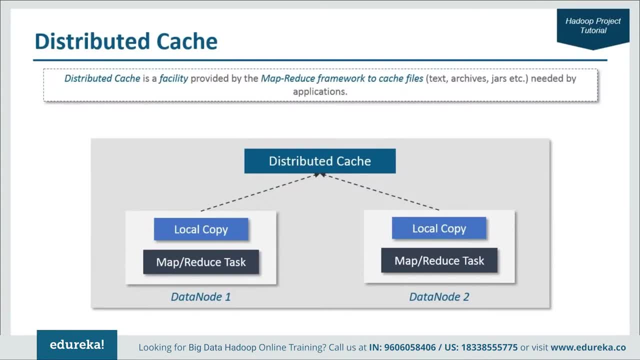 think of it as a share drive, right? So if you have multiple users who wants to have access to one data set, so you can just put it up in the share drive and all of your users can share the data. use the same data right. 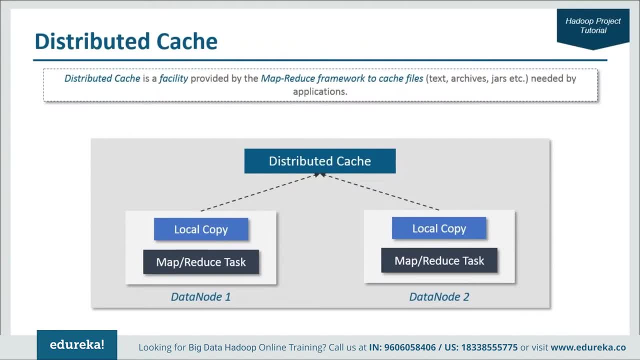 So this is what distributed cache is. So applications specify the files via URLs to cache via the job conf- So I'll be telling you about the job conf later in the demo section. And the distributed cache assumes that the files specified via URLs are already present on the file system. 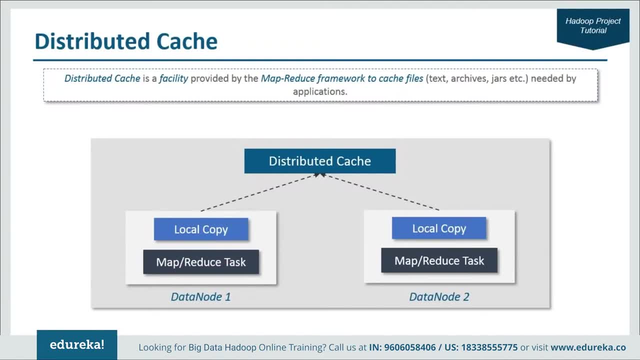 at the path specified by the URL and are accessible by every machine in the cluster. So the framework will copy necessary files to the slave node before any jobs are executed on that node And distributed cache tracks. modification timestamps of the cache files. So clearly the cache files should not be modified. 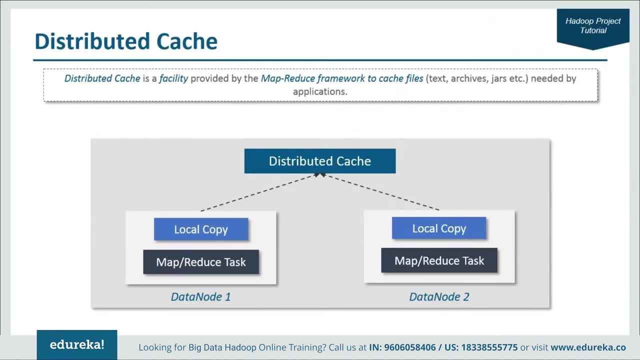 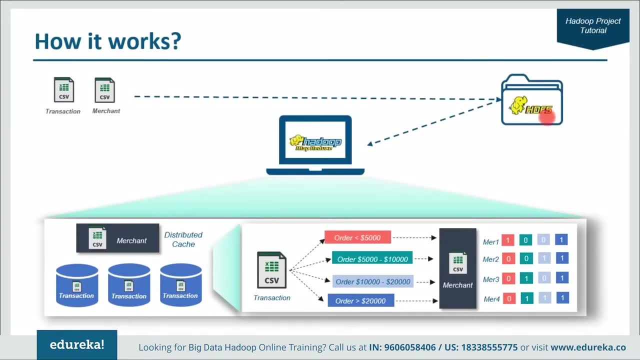 by the applications or externally while the job is executing. So how will it work? So in our case, we'll be storing the data into HDFS and we'll be executing MapReduce program over that file. So we'll store the merchant data in the distributed cache. 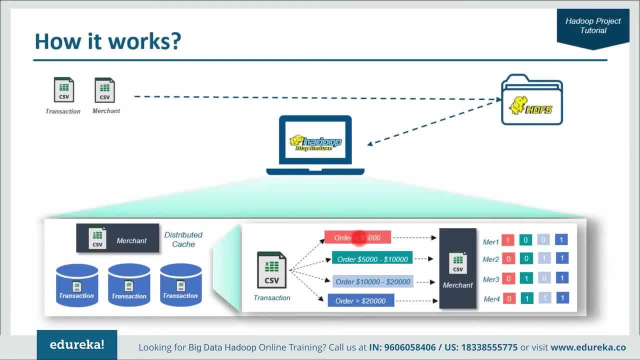 Then we'll segregate the transaction data into categories such as less than $5,000, $5,000 to $10,000, $10,000 to $20,000, and greater than $20,000 with the merchant ID. 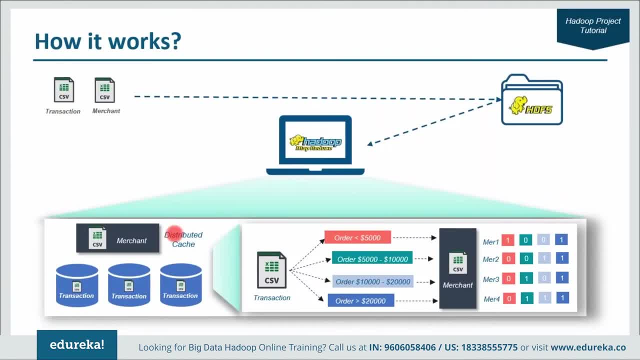 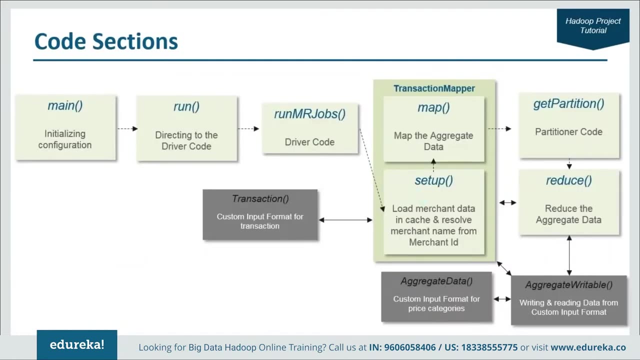 Then we'll use the merchant file from the distributed cache and map the merchant ID with the merchant name And at last we'll receive the output as the merchant name with date indicating the number of sales in different categories. Now let us talk about the code sections. 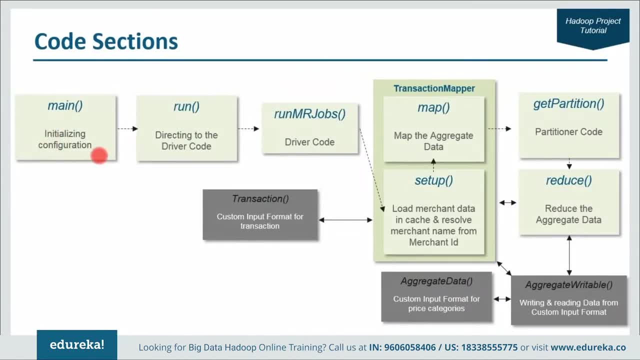 So the execution will start from the main method where we'll use the tool runner So the tool runner can be used to run classes. implementing tool interface. So it pauses the generic Hadoop command line arguments and simplifies the configuration of the tool. Then it will point to the run method. 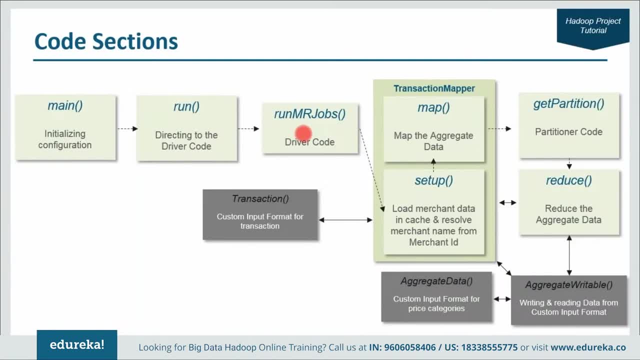 which will point to the run MR jobs. So here we are specifying the driver code. So I'll be telling you about the driver code later on. So next the execution will move to the mapper class, which is the transaction mapper. The framework first calls the setup method. 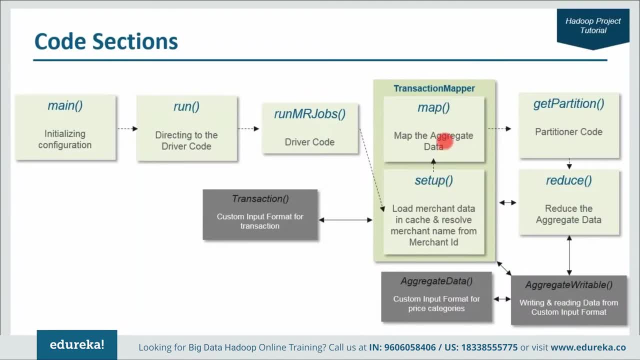 followed by the map method for each key value pair in the input split. So in setup method we are loading the cache file and calling a method where we'll be resolving the merchant name from the merchant ID. Next, in the map method, we are creating the object of transaction. 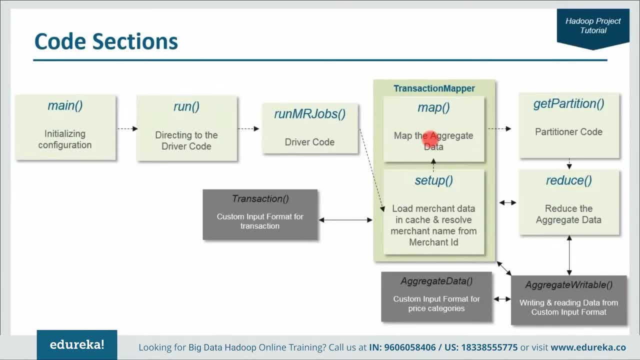 which we will be using to catch all the fields of transaction, first, and then, using the object of aggregate data, we will create the segment of transactions, as we discussed before, The four segments: less than 5,000,, 10,000, 20,000,. 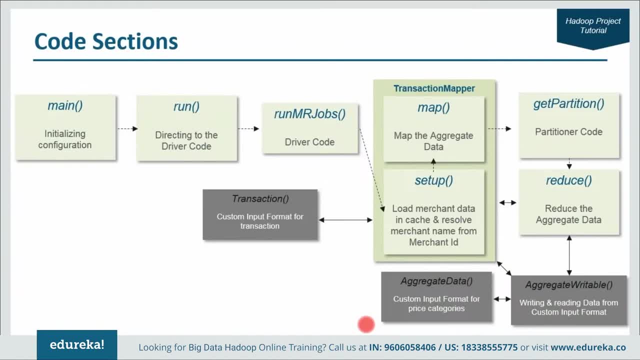 those segments. At last, using the merchant ID name map, we will resolve or find out the merchant name. The output of the map method would be the key, which will be the combination of merchant name and date of sale, while the value would be in the form of number of sales. 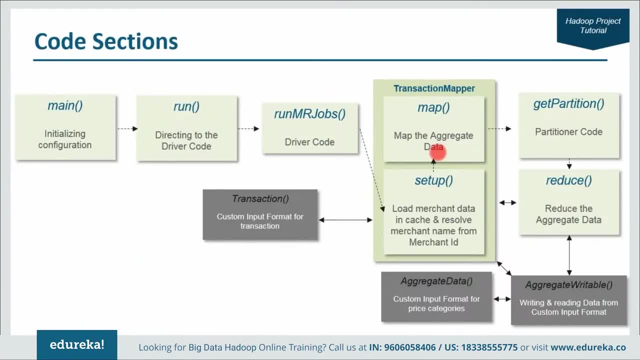 of different categories. Next, the execution will go to the partitioner code, where we'll have the get partition method, which will send the records with the same key to the same reducer And, at last, the reducer code will execute, which will aggregate the data with the same key and provide the output. 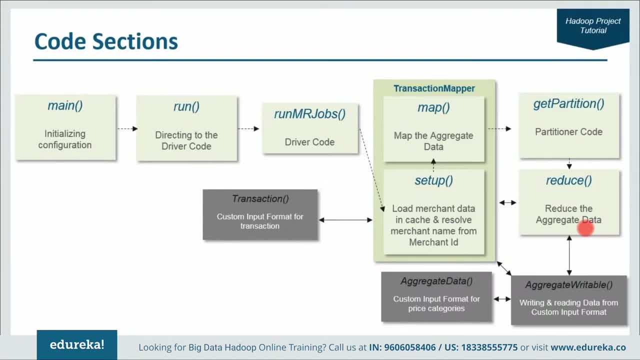 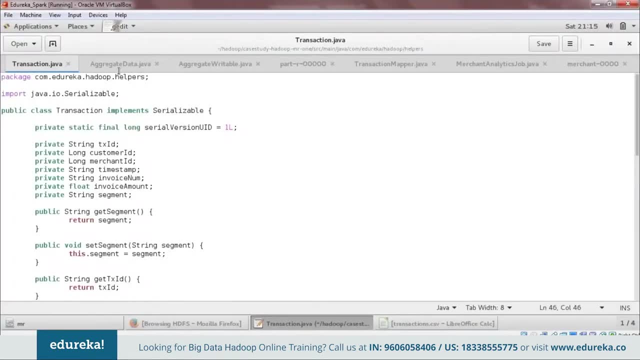 So I'll be showing you and explaining you all the codes involved over here in the demo part. all right, Now let us move ahead. So first let me take you through this transaction class where we are defining all the variables corresponding to the transaction file. 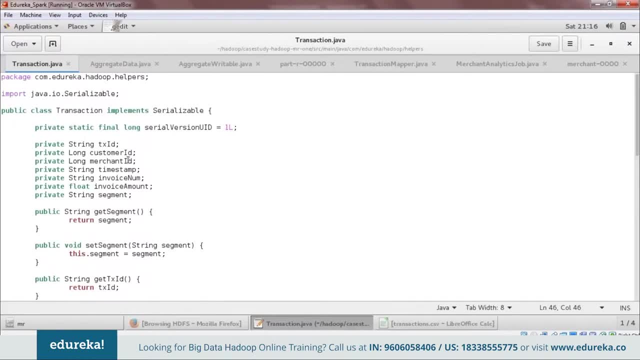 As you can see, we have got the transaction ID, customer ID, merchant ID, timestamp, invoice number, invoice amount and segment here. So these are the fields in the transactions and we have created the variable for the same. So next we are creating the getter and setter methods. 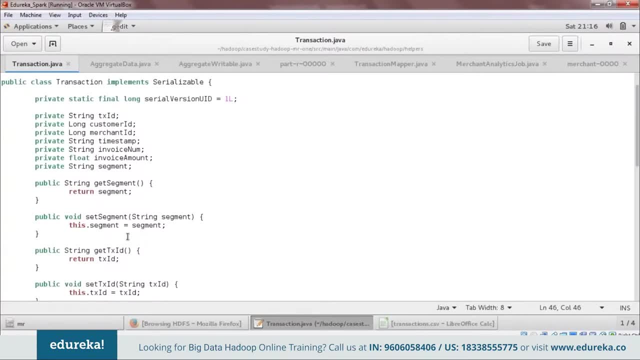 for each of the variables so as to read the value of the field, and we write the value of the field. So, as you can see, here we are defining the method get. So get segment. we have got get segment here, where we are returning the value of the field. 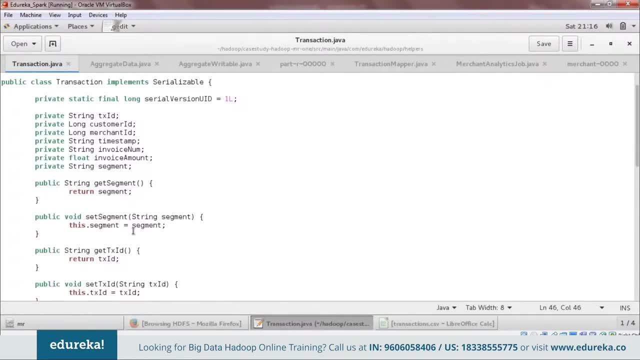 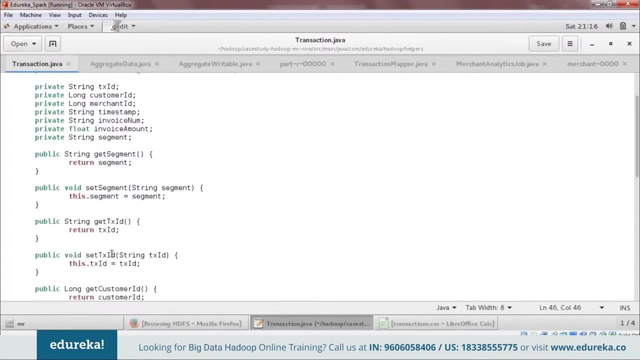 and the set method, here the set segment where we are writing the value of this field. So similarly we are doing it for all the variables, as you can see here. So we have the get and set for customer ID. So we have the get customer ID method. 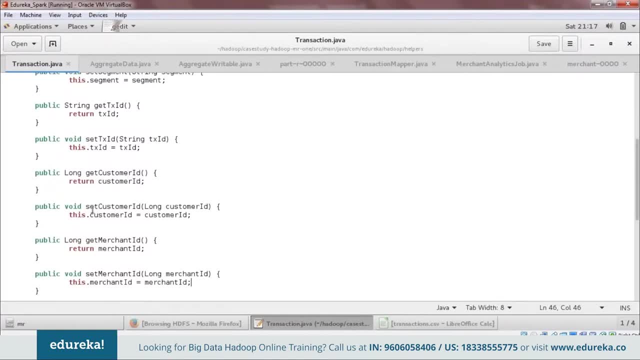 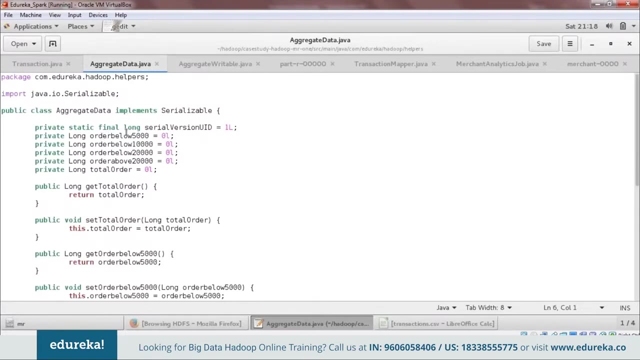 which returns the value of the field, and we have got the set customer ID which writes the value of the field. So this is similar for all the fields in our transaction data. So similarly we can have the aggregate data class which we have used to create the categories. 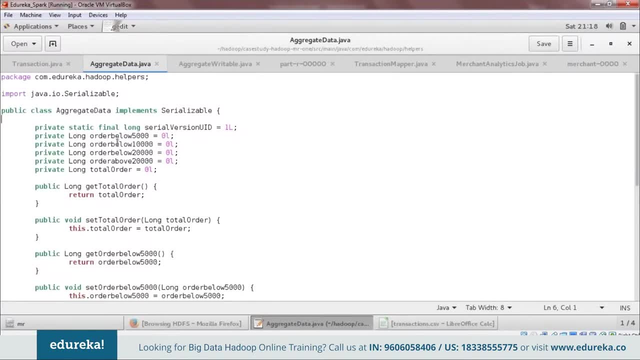 of the product. So here we have fields like order below 5,000,, order below 10,000,, order below 20,000, order above 20,000, which are nothing but the different categories which we have defined earlier And similar to the transaction class. 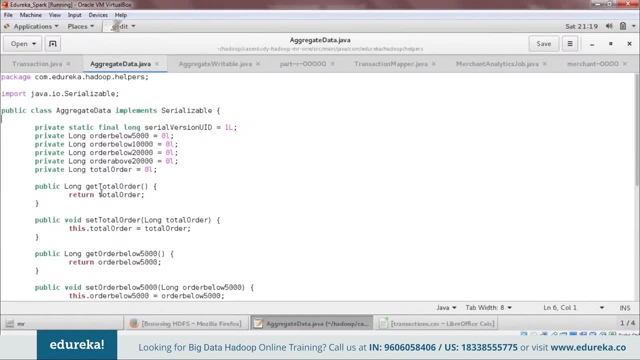 here we are defining the getter and setter methods. So we have got get total order method, which returns the value of total order, and we have set total order method, which is writing the value of this field, total order. So we have the same for all the different variables. 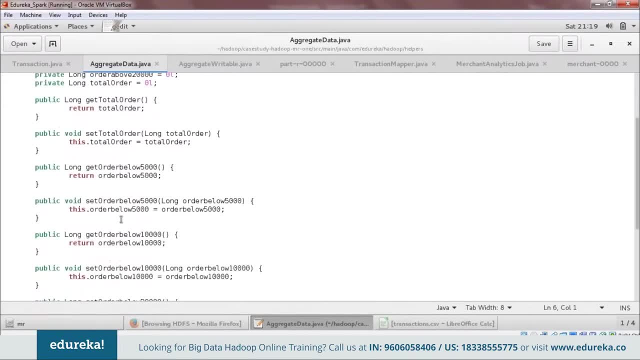 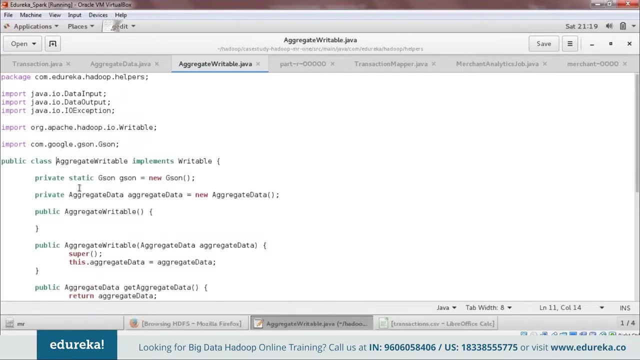 that we have defined in the aggregate data class, the getter and setter methods. Then we have got the aggregate writable class. So first here we are creating an object of JSON class. So JSON is basically used to convert Java objects to JSON format. Next we are initializing the aggregate data object. 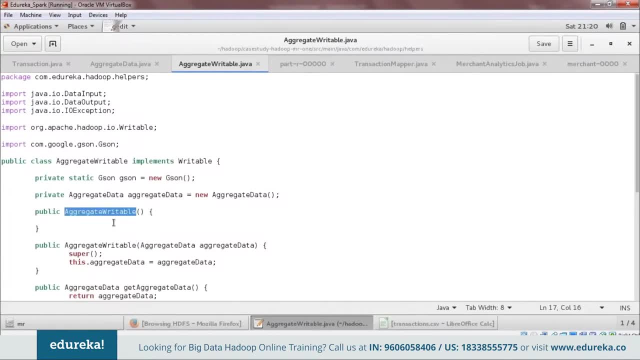 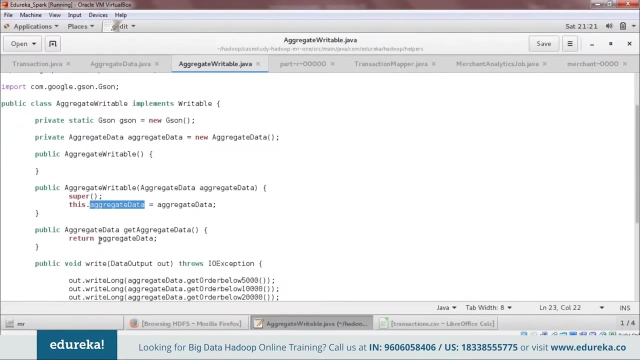 Now we have two constructors. First, one is the basic constructor, which is not taking any argument. The second constructor is taking aggregate data format as an argument and trying to initialize the aggregate data object. Next we have the getter method for the aggregate data, which will return the aggregate data object. 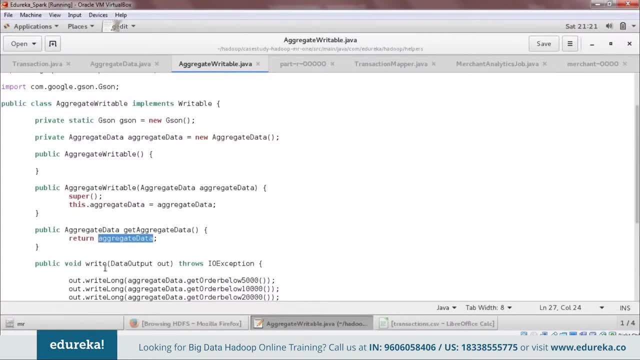 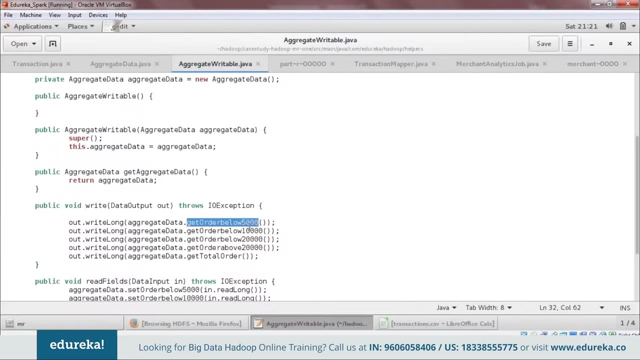 After that we have the write method, which will write the value of corresponding fields using the getter method of the field, Like for order: get order below 5,000,. get order below 10,000,. order below 20,000,. get order above 20,000.. 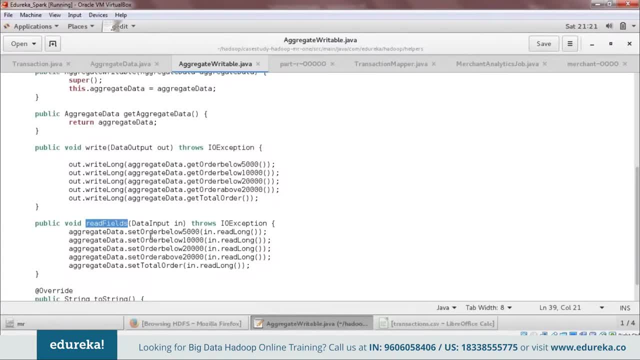 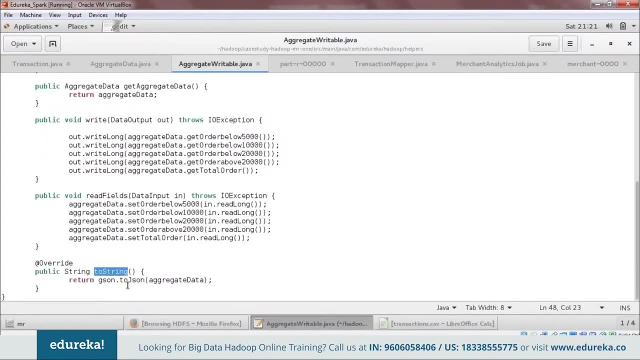 Then you have read fields method, which will be calling the setter method of each field to assign the values to the corresponding field, And at last we are overriding to string method, which will convert the aggregate data object to JSON and then return the JSON. So I hope you guys are clear with the custom input format. 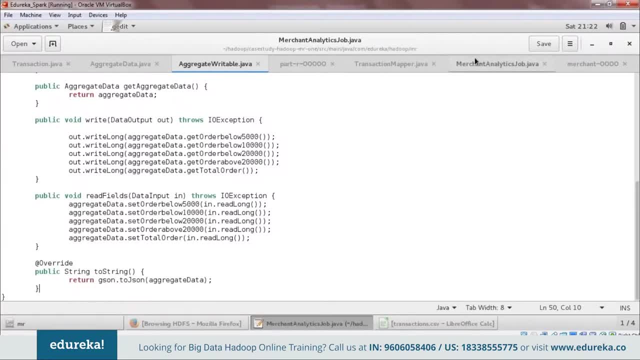 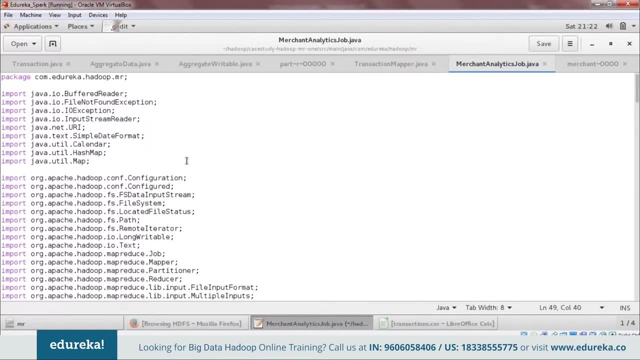 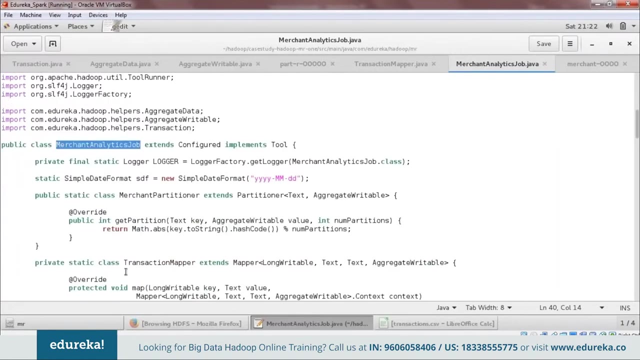 So now let us take a look at the main Java file, which is the merchant analytics jobjava. So the main class is the merchant analytics job class, inside which all the jobs will reside. So the execution will start from the main method. So first let us go to the main method. 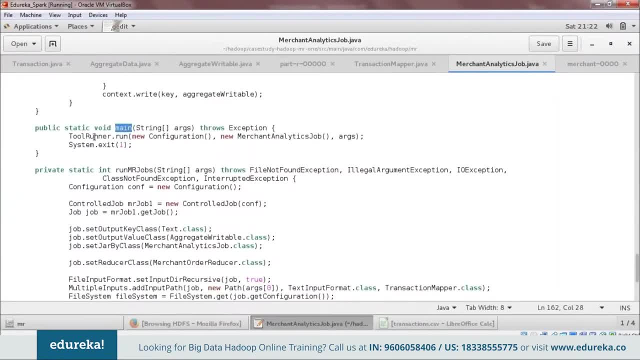 So here we are using tool runner. So tool runner can be used to run classes implementing the tool interface. It passes the generic Hadoop command line arguments and modifies the configuration of the tool. So tool runner dot run method runs the given tool after parsing. 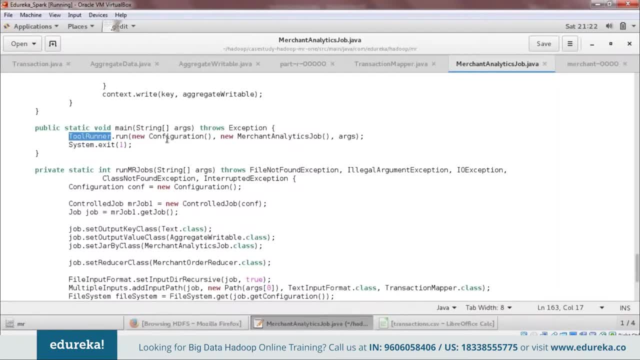 the given generic arguments, It uses the given configuration or builds one. if null, It sets the tool's configuration with the possibly modified version of the conf. Here we are passing the configuration object- merchant analytics job object, which is the main class, and arguments which we will be providing while executing the job. 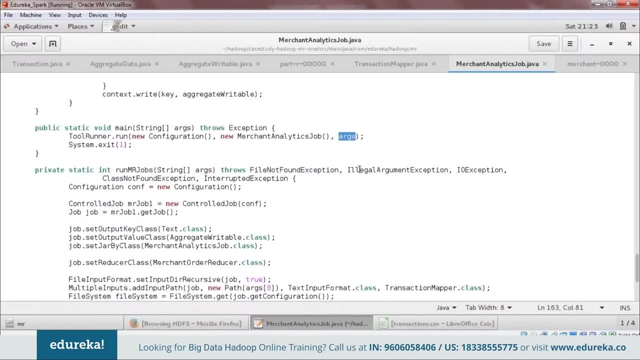 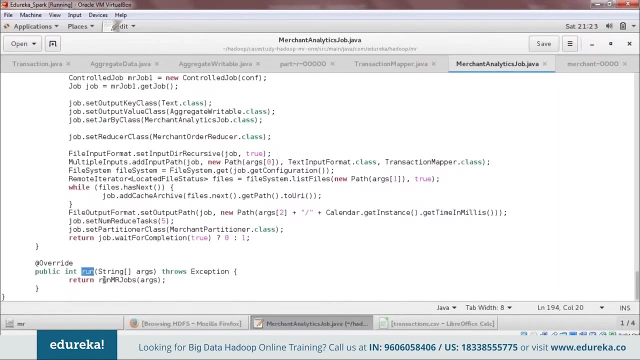 So in our case there are three arguments: First is the path of the transaction file, Second is the path of the merchant file And third is the output directory. Now we will execute the run method, where we are returning the values of the run MR jobs method. 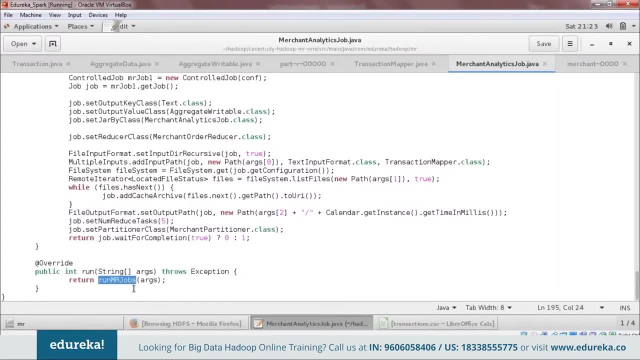 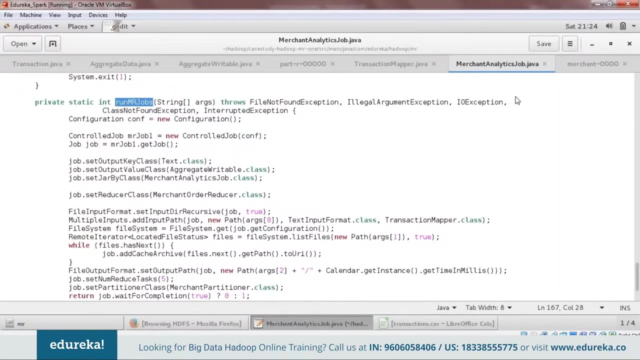 We are also parsing the arguments, that is, all the three paths, that is, the transaction, merchant and output directory, to the run MR jobs method. Now let us see the run MR jobs method. So here we have the driver code. So first we initialize the configuration. 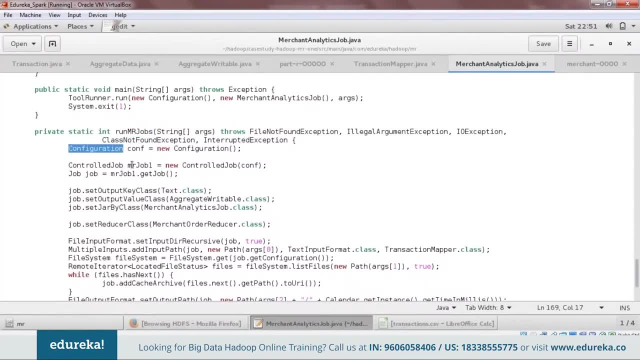 object and then we will initialize the control job object. So control job class encapsulates a MapReduce job and its dependency. It monitors the state of the depending jobs and updates the state of this job. And now we are creating the object of job class. 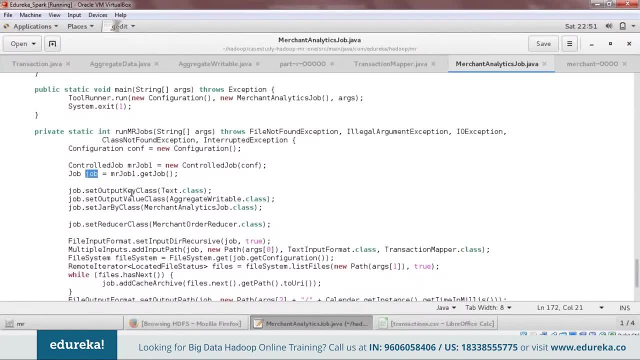 and we will define the properties of the job. So first we have the set output key class property, where we are defining the output format class of the key, which is text class. Similarly, we are defining the set output value class for output format class of the value. 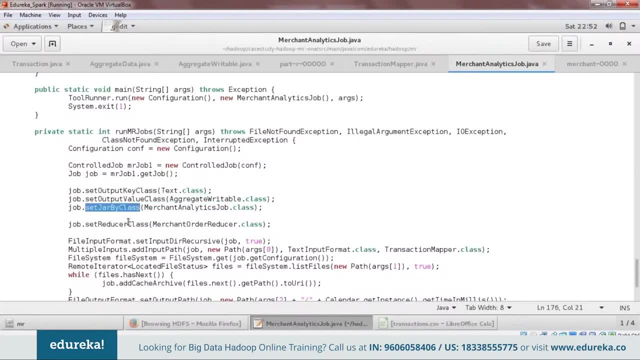 that is the aggregate writable class. Next, we have set jar by class, which tells the class where all the mapper and reducer code resides, which the merchant analytics job in our case. Now we are specifying the reducer class, which is merchant order reducer, And next we are providing the input directory. 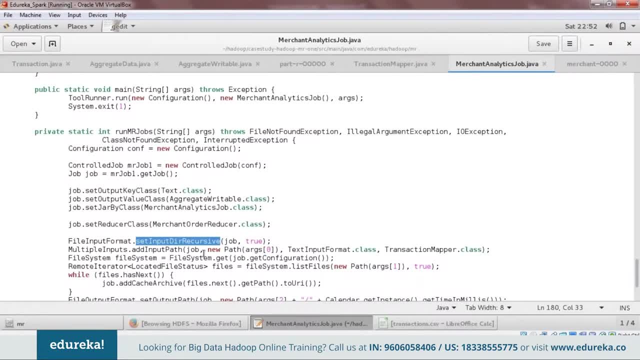 so the set input dir recursive method will read all the files from the directories recursively if we are providing the directory path. So first we are adding the input path of the transaction file which is present in the argument 0, then here we are also specifying the input format of the file. 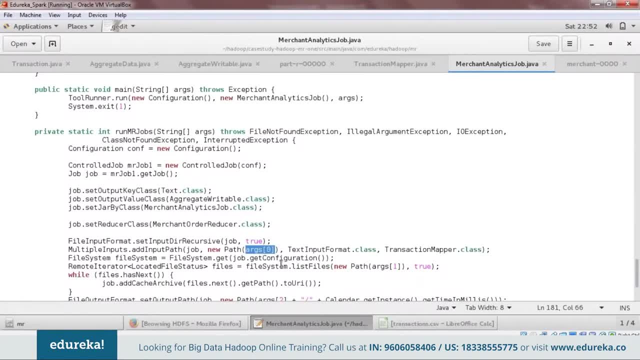 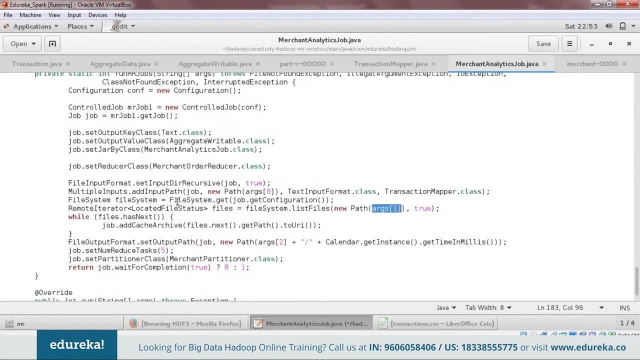 and the mapper class, that is, the transaction mapper. Next, we are talking about all the merchant file from the directory provided in argument 1 and adding this file to the distributed cache using the jobaddCacheArchive method. Moving ahead, we are setting the output directory path. 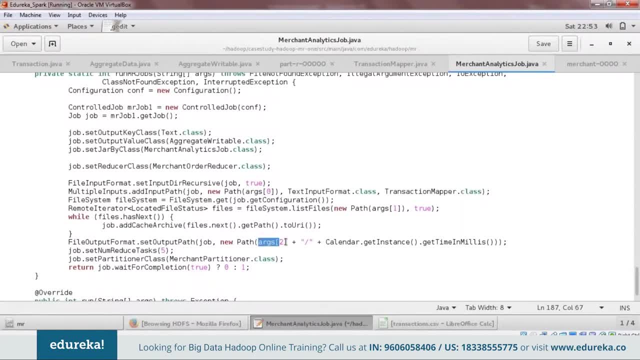 which is provided in argument 2, and we are also adding the timestamp as the subdirectory, And at last we are setting the partitioner class, that is, the merchant partitioner, and then we are returning 0 or 1, depending on whether the job has been executed successfully or not. 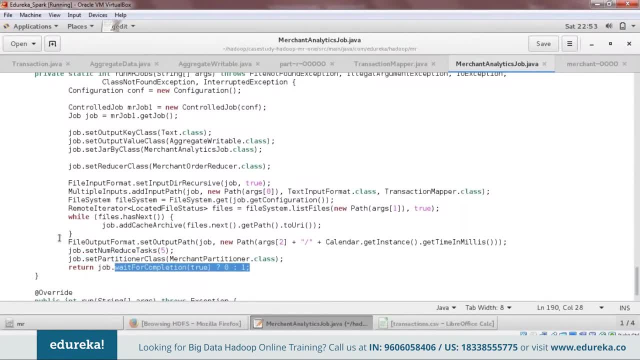 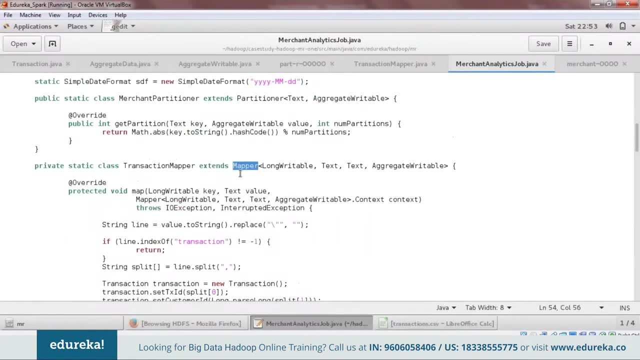 And next we will take a look at the transaction mapper class which implements the mapper interface. so it maps input key value pairs to a set of intermediate key value pairs. So maps are the individual tasks which transform input records into an intermediate record, The transformed intermediate records. 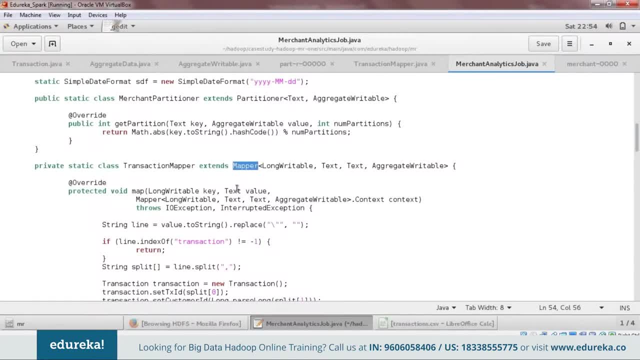 need not to be of the same type as the input records. The Hadoop MapReduce framework spawns one map task for each input split generated by the input format for the job, And mapper implementations can access the job conf for the job via the job configurable. 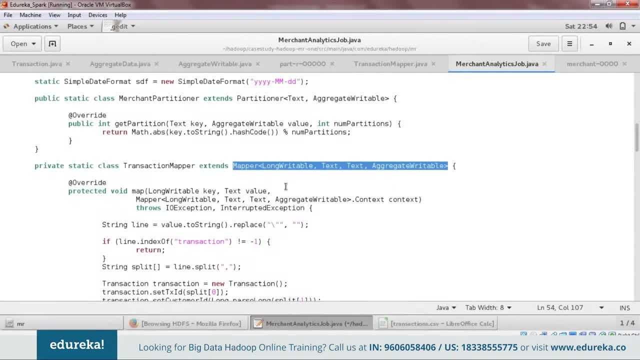 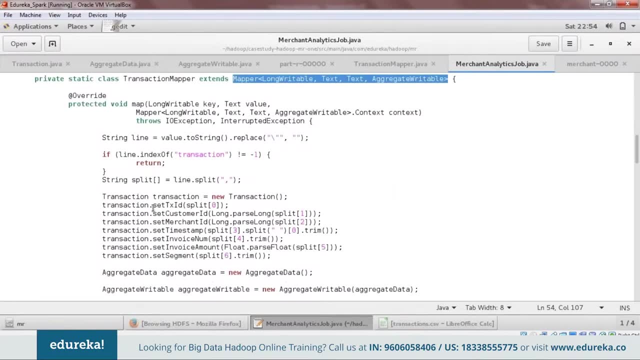 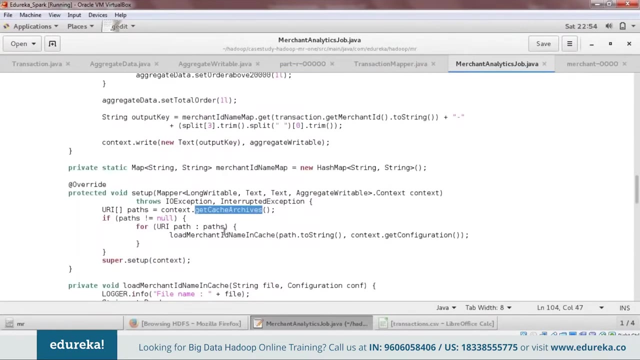 and initialize themselves. The framework first calls the setup method, followed by map method for each key value pair in the input split. So in the setup method we are loading the merchant file from the cache using the getCacheArchives method, Then from each file. 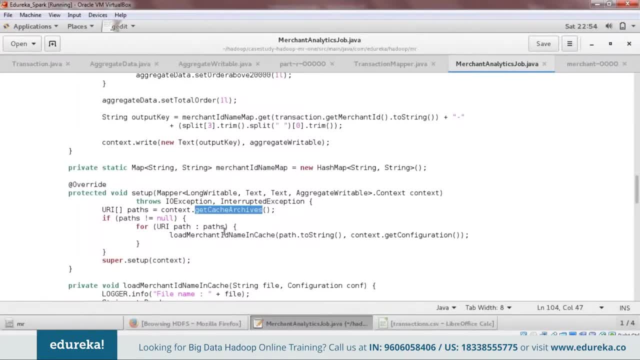 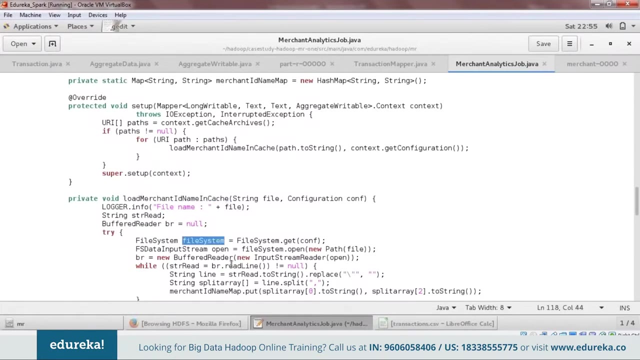 we are calling the load merchant ID name in cache. So we are calling this method and we are passing the path of the cache files and the configuration objects. Now in this load merchant ID name in cache method, we are initializing the object of file system using the conf. 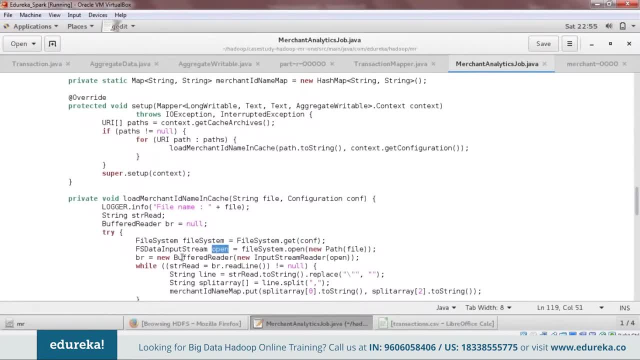 And next we are opening the file and then we are reading the data line by line from the file. Now here, first we are removing the codes from the line, and then we are splitting the line using the comma And at last we are putting the merchant ID. 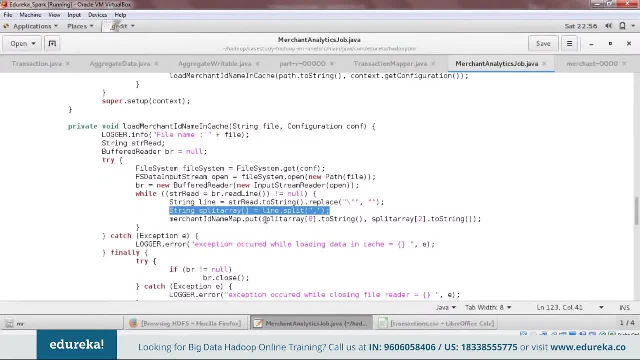 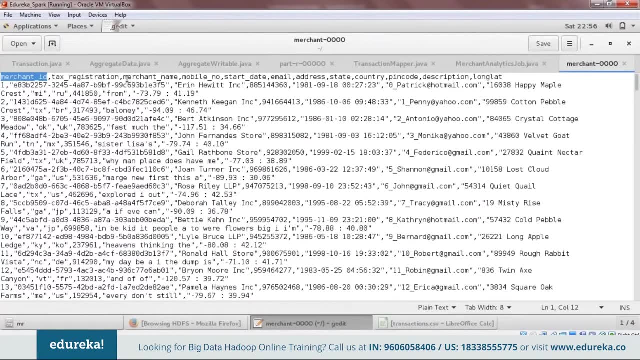 and merchant name in the merchant ID name map variable. So here you can see in the merchant file that we have merchant ID at index 0 and merchant name at index 0. So this merchant ID name map will help us in resolving the merchant name. 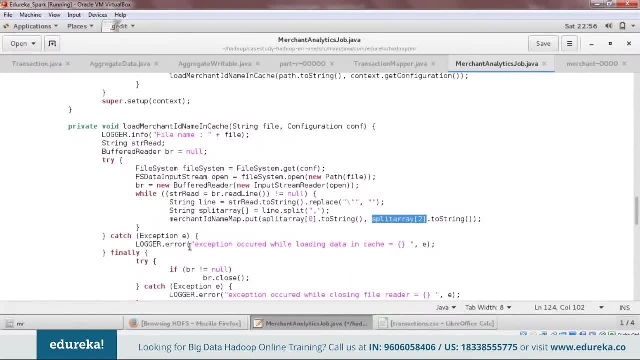 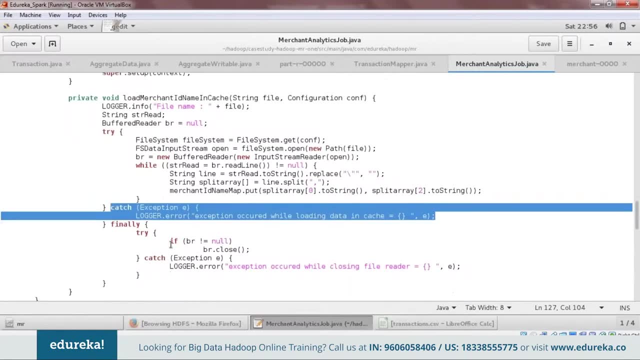 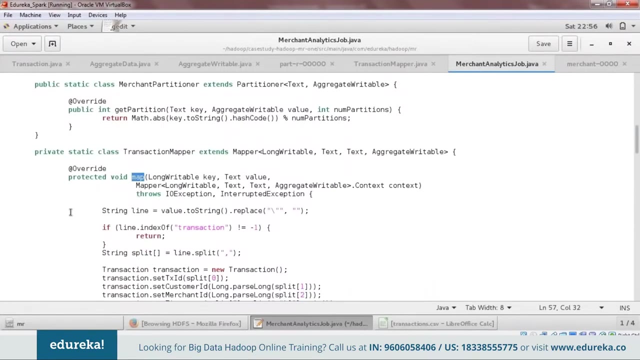 from merchant ID. And next we are defining exception to notify us if the cache file is not read. And at last we are closing the object of the buffered reader. Now let's talk about the map function. So now the map function will be called. 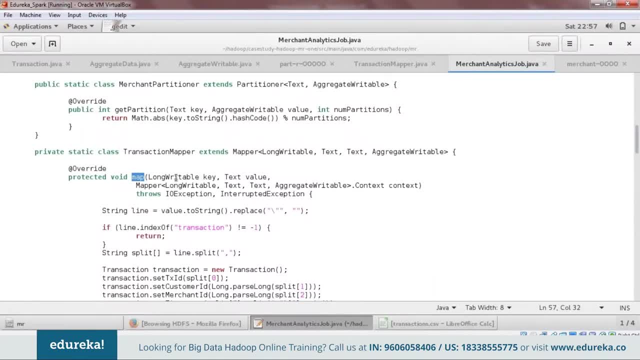 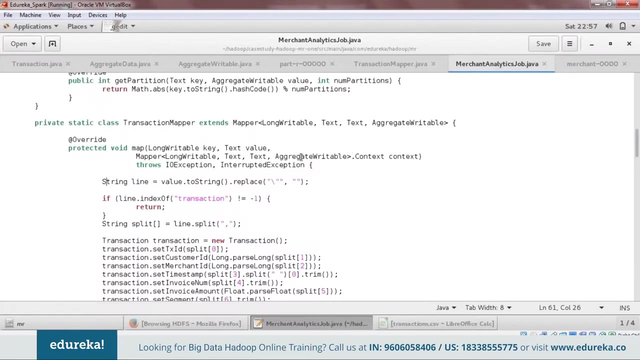 So the input format of key is long writable and the value is text. We are also creating a context of the mapper framework where we will be writing our intermediate output. Now the output format of the key is text and the value is aggregate writable. Again, here we are removing the codes from the line. 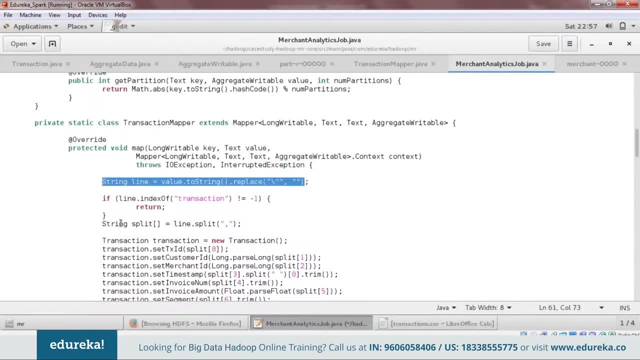 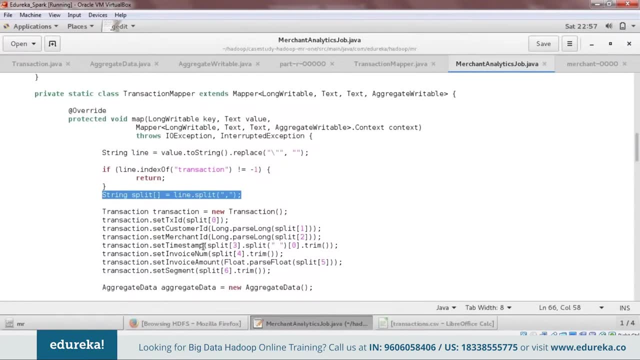 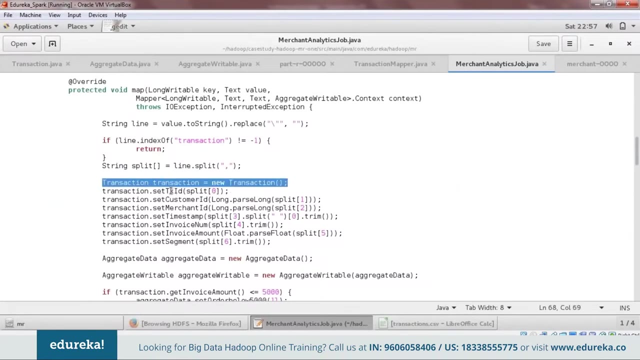 and then we are splitting the line using comma. So in the split area we have all the fields of the transaction data stored in the consecutive indexes. Now we are creating an object of transaction class and setting the values of the field using setter methods, And next we are creating the objects of aggregate data. 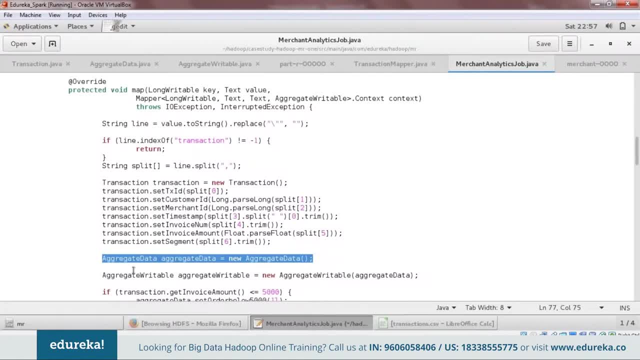 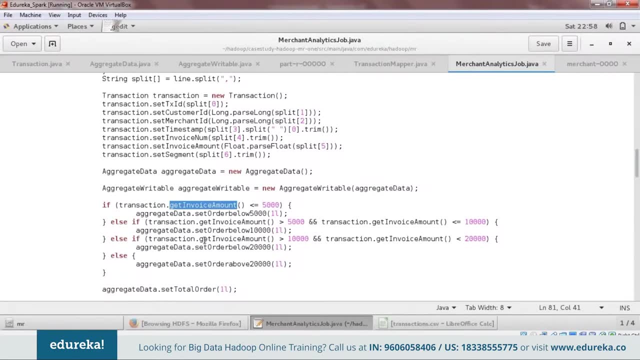 and aggregate writable class. Then, using transactions, get invoice amount field. we are deciding that in which aggregate data field the transaction would lie, We will set the value of corresponding field of the aggregate data object to 1.. And next we have the output key which will contain the merchant name. 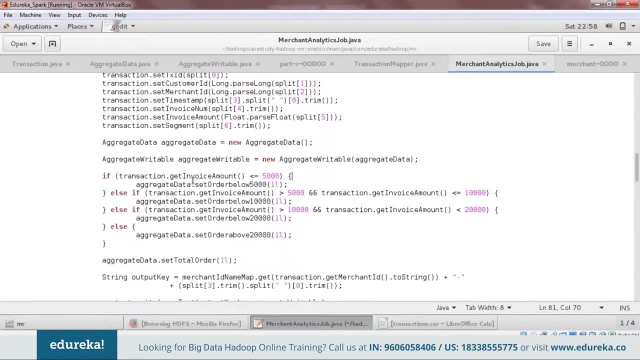 and the date of sale. So merchant ID name map method will return the merchant name from the merchant ID, as we just discussed. So we are passing the values as merchant ID and the date. At last we will pass the intermediate result in the form of key and value to the context. 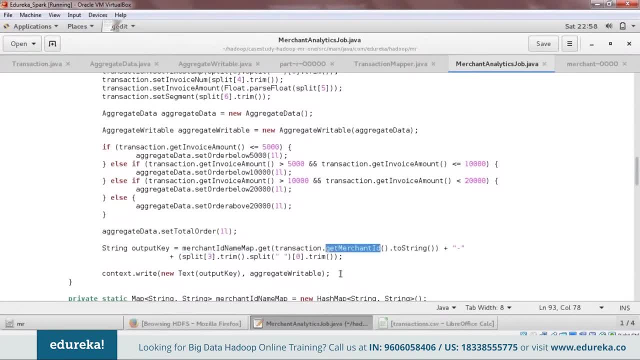 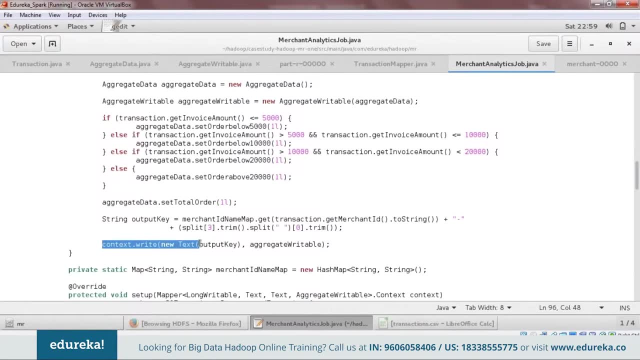 So we are now creating the output key which will contain the merchant name and the date of sale, And next we are creating the output key which will contain the merchant name and the date of sale. So merchant ID name map method which will contain the merchant name. 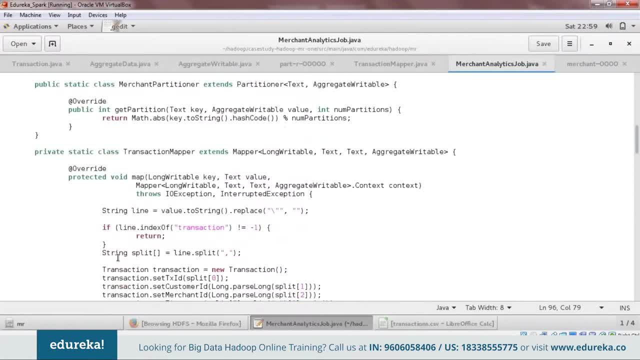 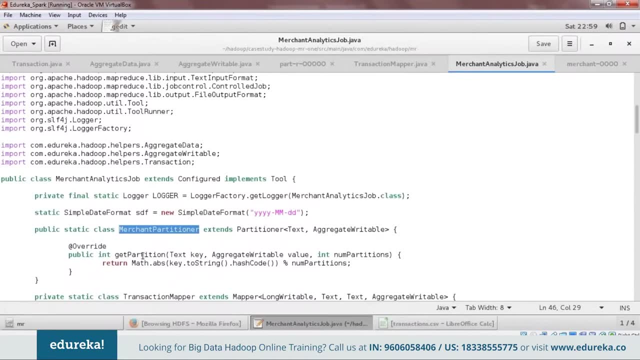 and the date of sale. Next, the result will be sent to the partitioner class, that is, the merchant partitioner. So it's over here. So in this class we are overriding the default get partition method And in this method we are converting the key. 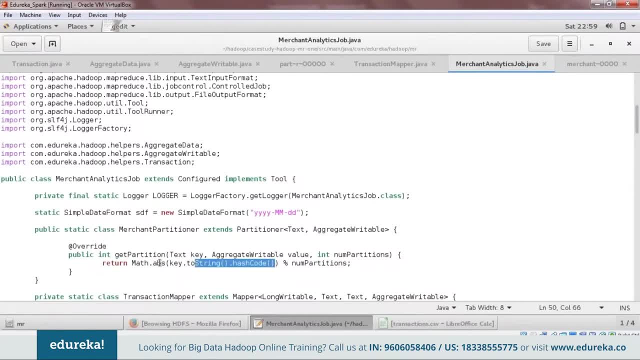 using hash function and using abs method to return the absolute value of a number. And at last we are using the modular function to get the remainder, And now we are dividing it with the number of partitions, So which is nothing but the number of reducers. 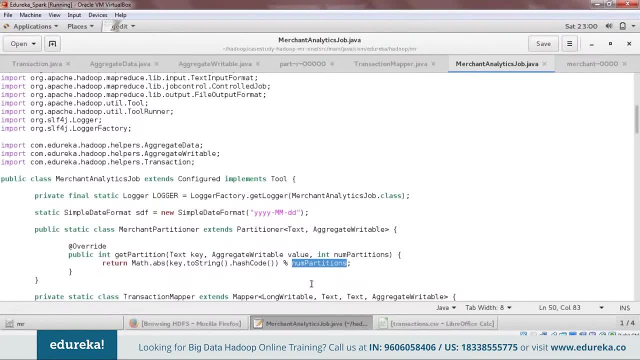 And in our case we have specified 5 reducers, so the module of 5 would return the value between 0 and 4.. And one more thing is: the same key would always have the same hash generated and hence the modular result would be also the same. 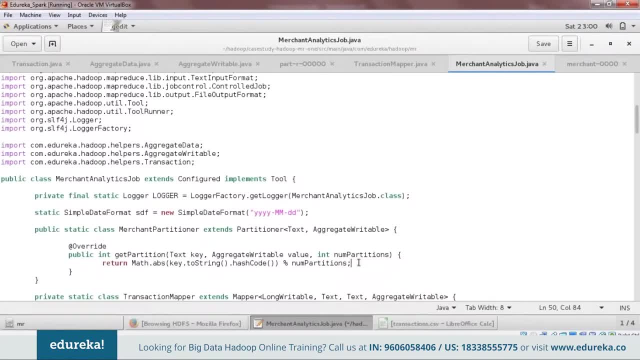 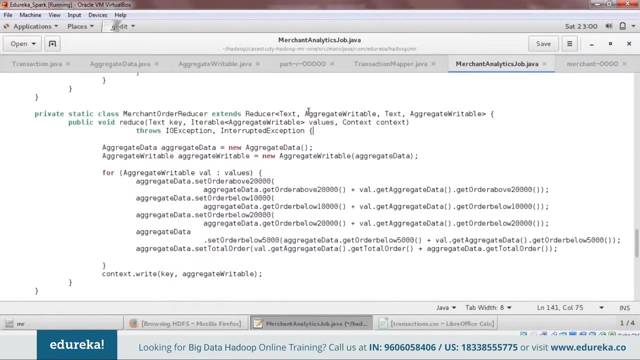 And thus the records with the same key will be sent to the same reducer And, based on this, records are sent to the reducer. So next we have the reducer code And it's over here. So it's the merchant order reducer, The reducer class as defined in the driver code. 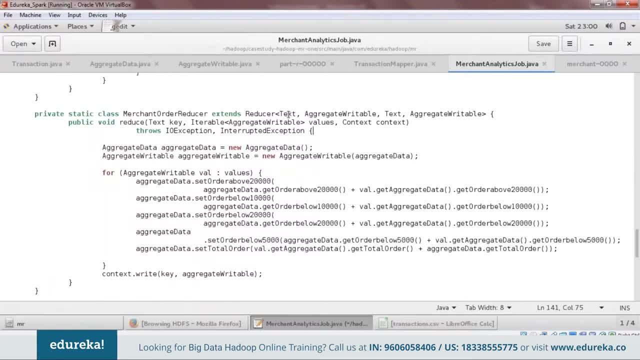 resides in the merchant order reducer class. So here we have the key input as text and value input as aggregate writable, which was written by our mapper class, And the output key format is again text and the output value format is aggregate writable. So here our execution will move to reduce method. 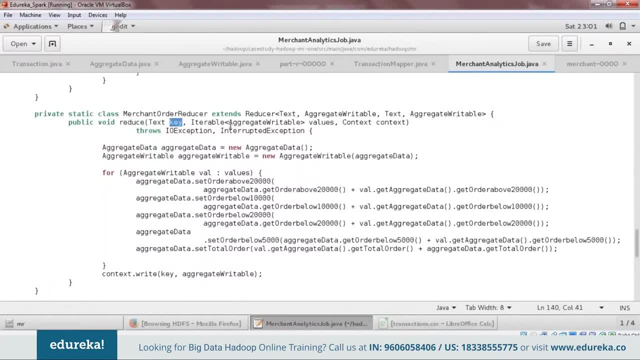 where we are passing the input key value and context as argument. And here we are again creating the objects of aggregate data and aggregate writable class. And next we are taking the input values. Now here we are calling the setter function of each category, getting the earlier value of that category. 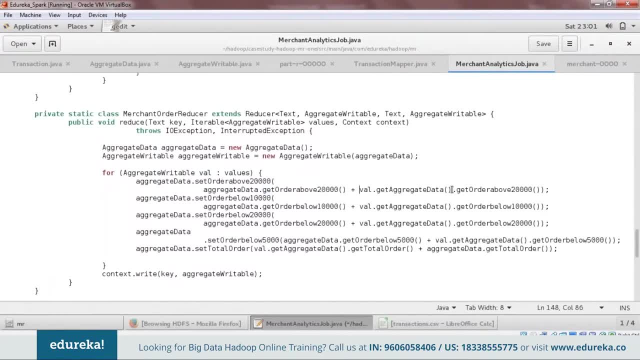 and then adding the new value of the new aggregate data object for that category. So it will add the value to the corresponding fields if there is a record with the same key And at last we are writing the key and value in context dot write method. 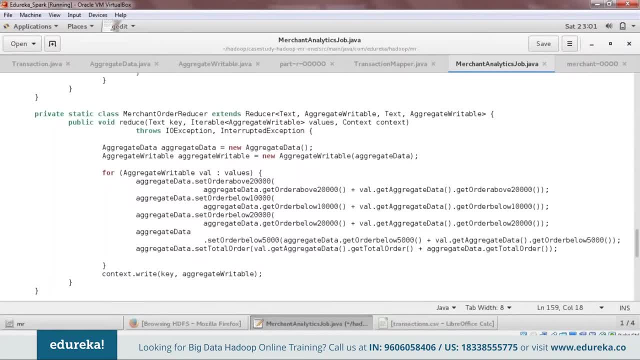 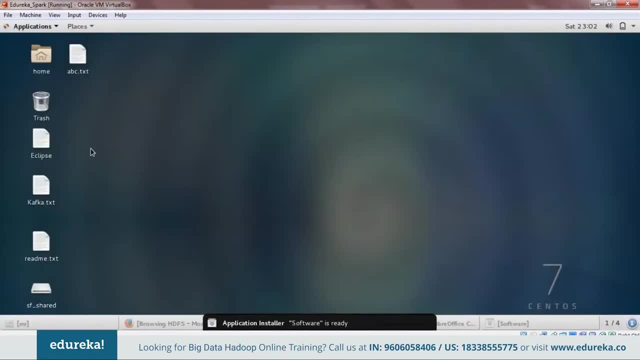 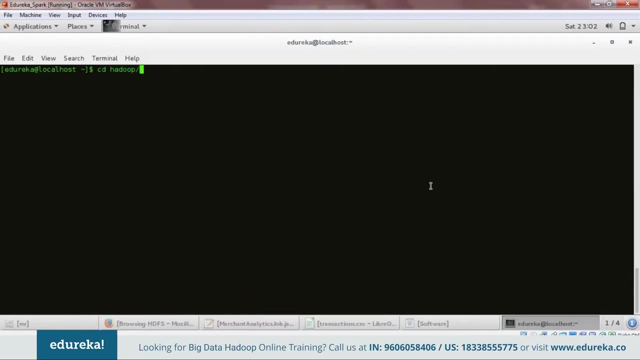 So I have explained you the code, so now let us just go ahead and execute it. So first let us move to the project directory. So we have the palmxml file, which has all the dependencies that we require in order to run our MapReduce job. 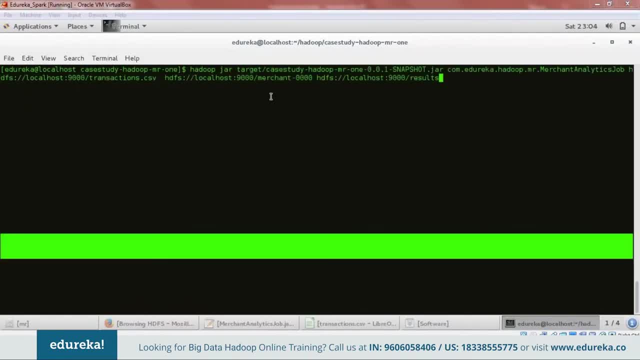 So this is the command. So it has my jar file and the path of my jar file. Then I have got my main class over here, which is merchant analytics job. So this is where my main function is, And then I am passing the three paths. 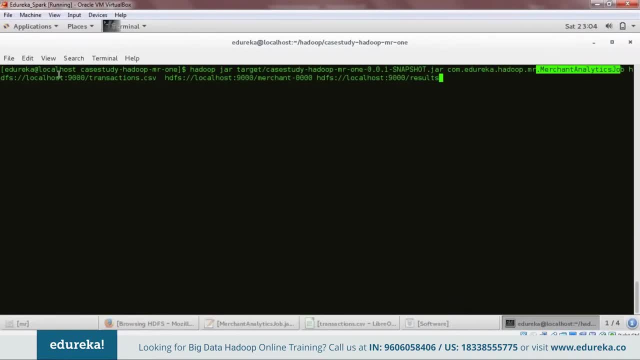 So first is my transactions dot csv. This is my data set. This is my data set. This is the path of my data set. Then my merchant data: This is the path of my merchant data. And finally my output directory, which is the result. 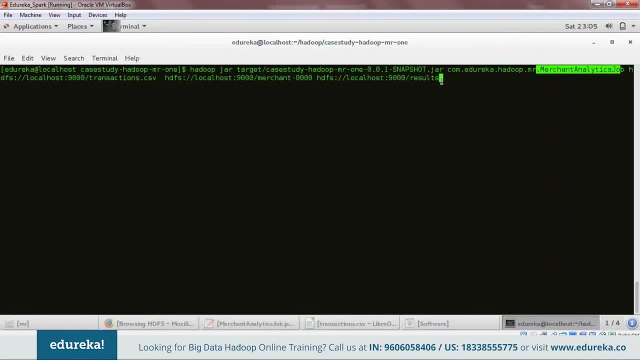 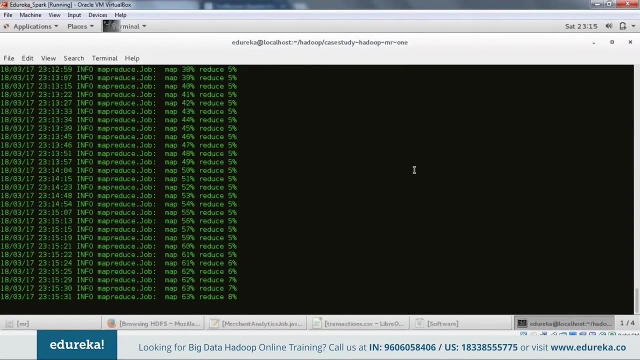 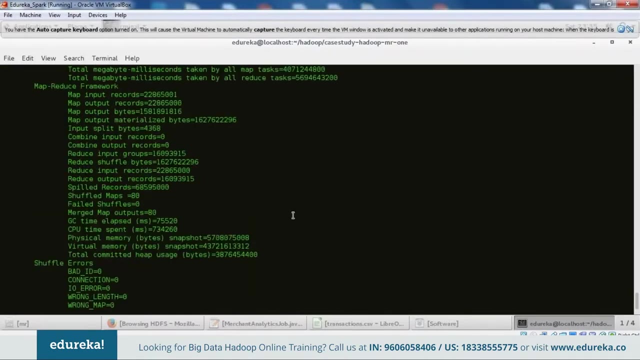 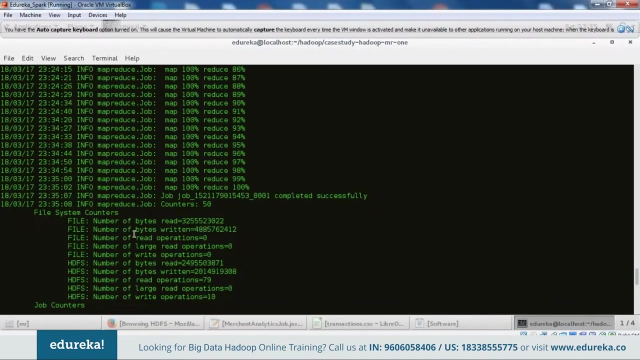 This is the path over here, So let us just go ahead and execute this command. So the code is run. So here are the different parameters on which this MapReduce job was run. So you can see the details over here. So you can see the number of reduced tasks were five. 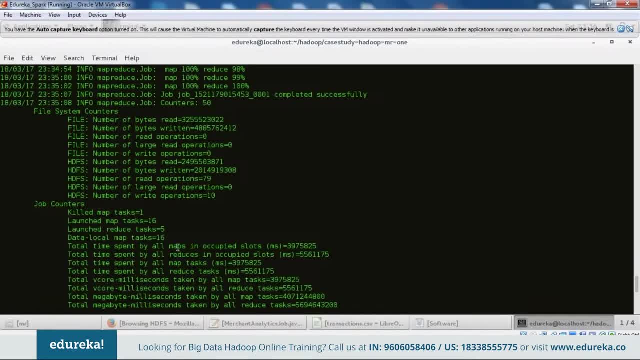 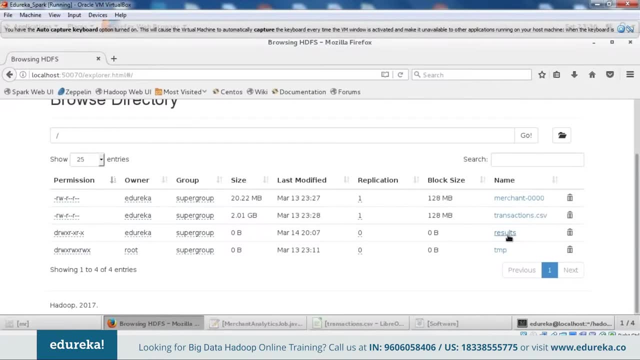 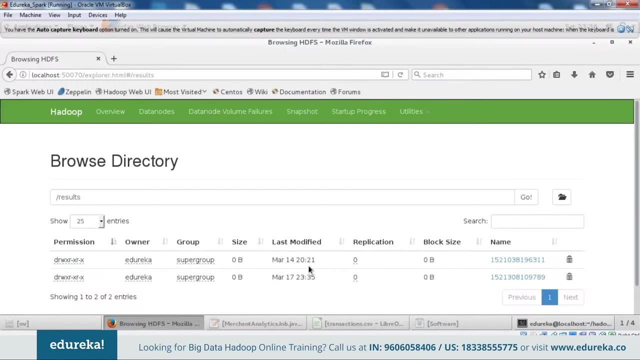 since we had five reducers. So you can see all the details here. Let me just show you the result now. So it is in the results directory. So there are two directories over here, because this was the earlier one, that when I had previously executed it. 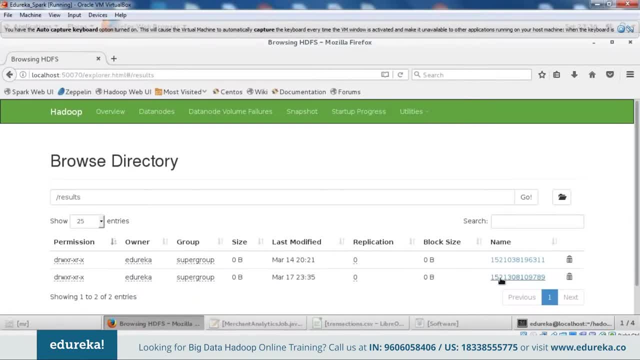 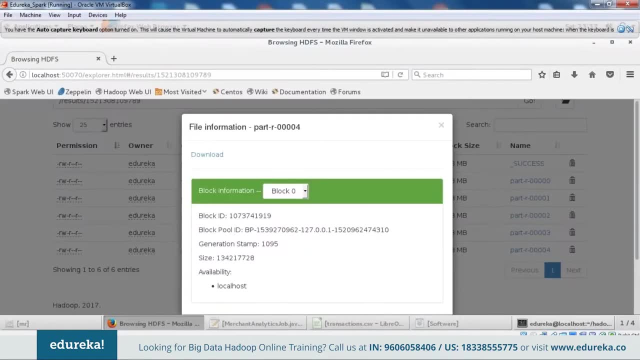 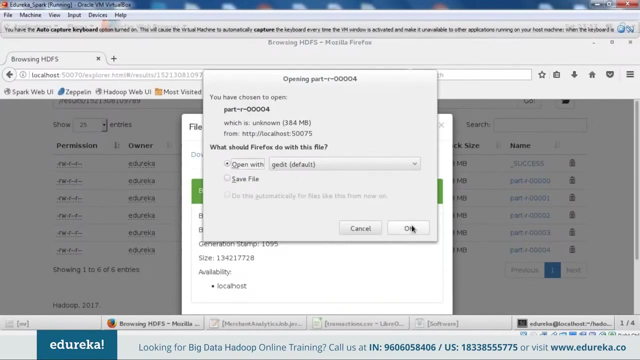 So this is the one that we have got right now, So let me just show it to you. So we have got five part files because there are five reducers. So just clicking on one part and you can just click on download. Let me just open it. 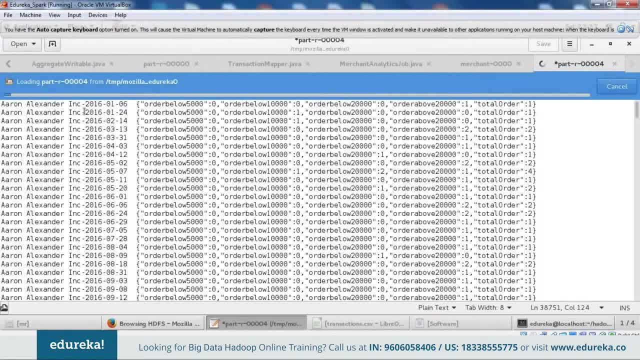 So this is what you get. So you get the merchant name and the timestamp over here and also the category or the segregation that we did based on the cost of the orders, right, So it was order above $20,000 at this timestamp and the total order was one. 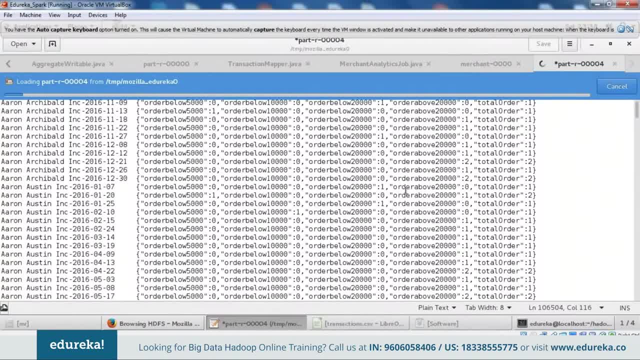 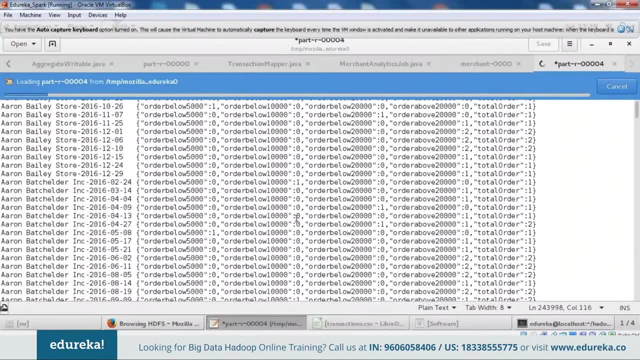 So this is the format of the result. So we have got a lot of rows. So this is the result. So we have just used a few fields or parameters from the merchant file. We have just used the merchant name and the ID over here. 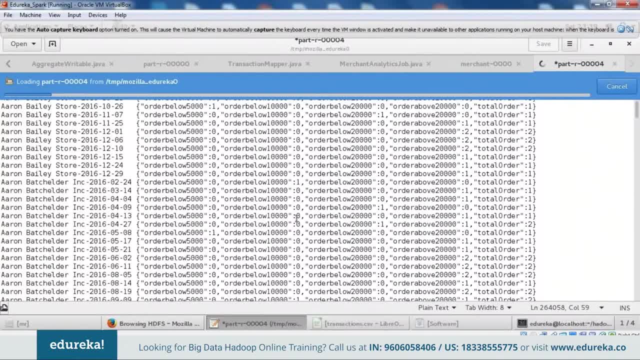 Since this is a sample project, sample demo project, but the scope of this particular project is huge. You can use a lot of other parameters that was mentioned there, like the location. you can analyze it based on locations, based on the time period. 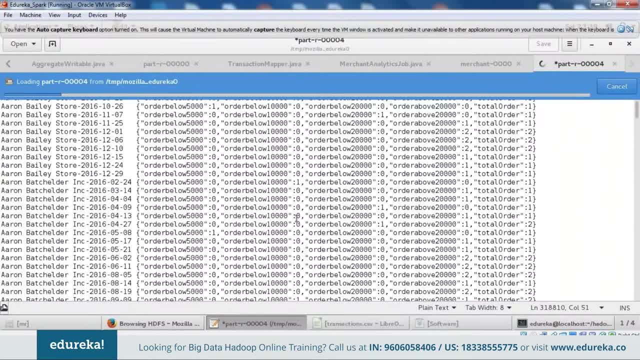 where the order was placed, So you can take in account different fields and improve this or make this analysis even better by yourself. So when you're doing this project as a part of your course curriculum, so you will be exploring the other fields as well. 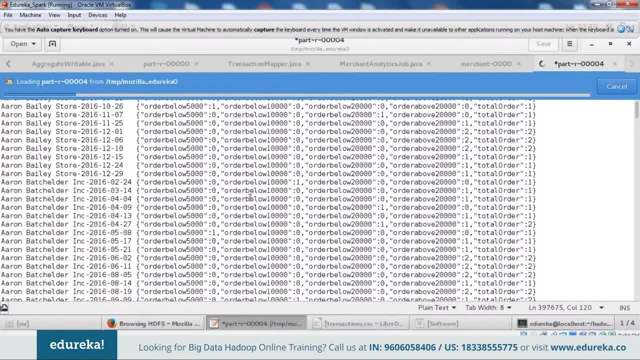 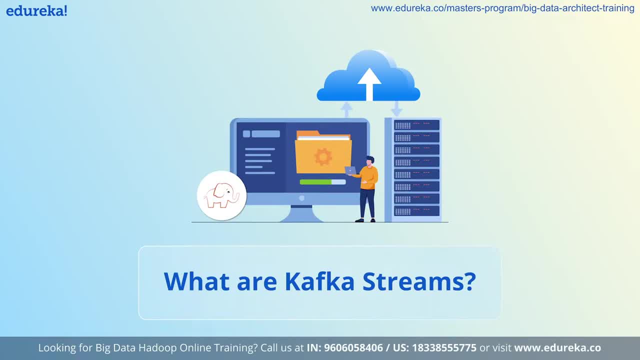 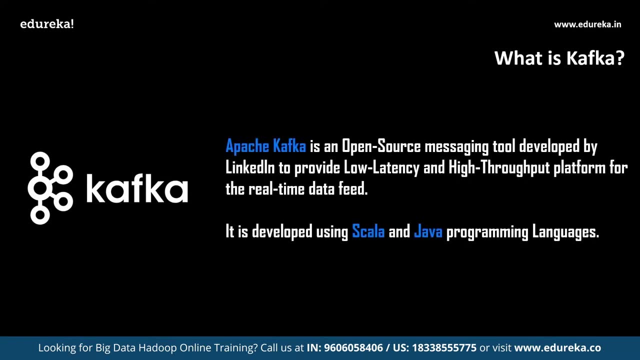 I have just shown you, with just using two fields, the merchant name and the ID, What is Kafka In general? Kafka is a producer to the consumer based messaging system that has a producer that produces the message and the consumer that consumes the message. 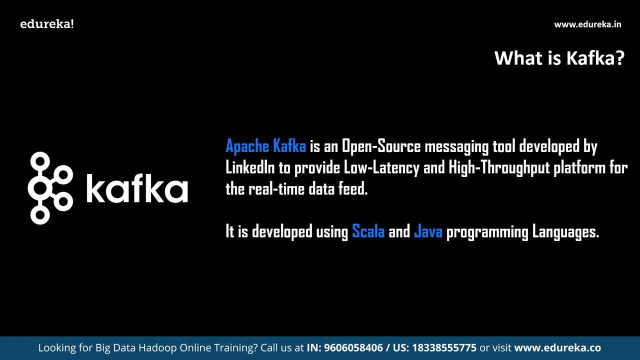 In between the both, we have brokers that distribute the messages to the consumers and data storage unit, which is none other than Apple Apache Zookeeper. to understand more about Apache Zookeeper and Kafka, You can go through the article link in the description box below: Apache Kafka. 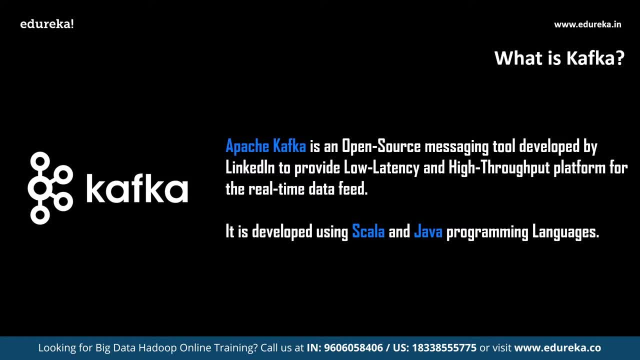 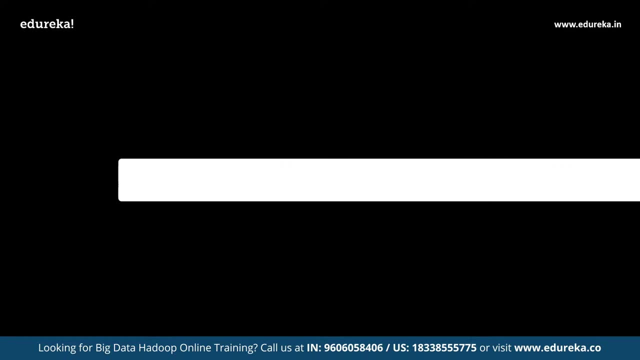 So, basically, Apache Kafka is an open source messaging tool developed by LinkedIn to provide low latency and high throughput platform for the real-time data feed. It is developed using Scala and Java programming languages. So, followed by the definition of Kafka, we shall enter and understand what exactly is a stream. 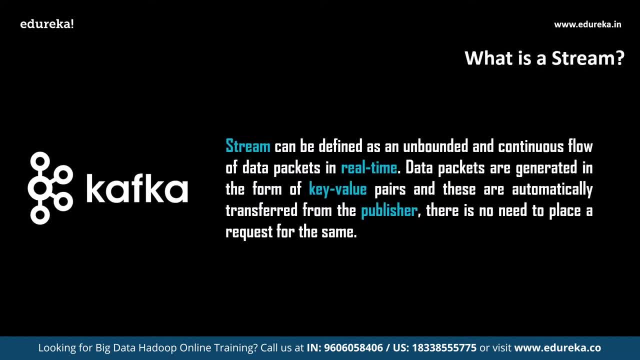 In general, a stream can be defined as an unbounded and continuous flow of data packets. in real time, Data packets are generated in the form of K value pairs, and these are automatically transferred from the publisher. There is no need to place a request for the same. 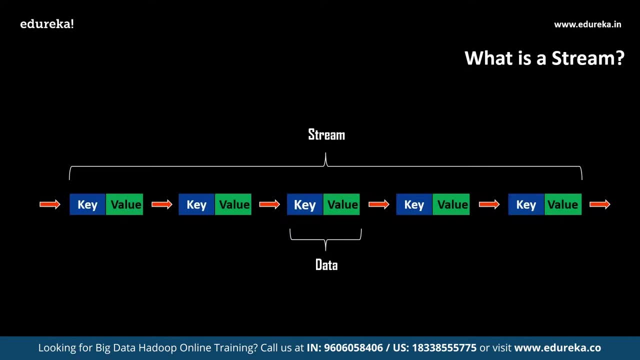 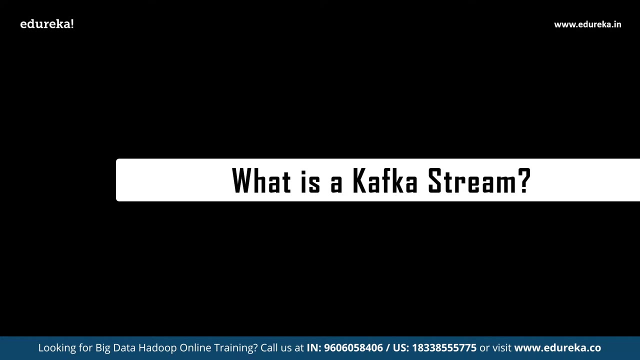 The below image depicts the K value pairs that are involved in data stream. Each and every single K value pair is one single unit of data, or it is also called as one single unit of a record, So, followed by the stream, we shall understand what exactly is a Kafka stream. 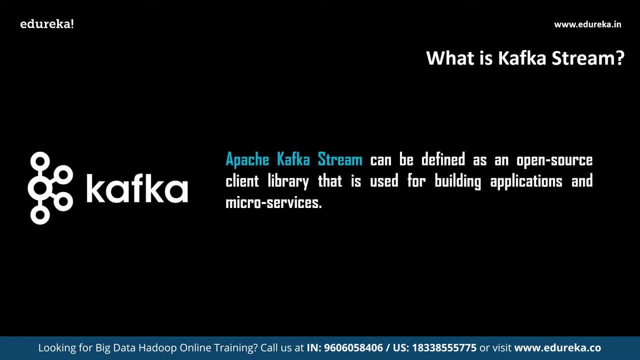 Kafka stream is an API that integrates Kafka cluster to the data processing applications which are either written in Java or Scala. This API leverages the data processing capabilities of Kafka and increases data parallelism. Apache Kafka stream can be defined as an open source client library that is used 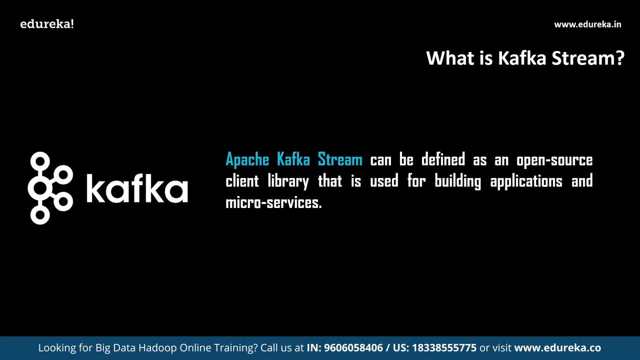 for building applications and microservices. Here the input and the output data is stored in the form of Kafka clusters. It integrates the intelligibility of designing and deploying standard applications using the programming languages such as Scala and Java with the benefits of Kafka server-side cluster technology. 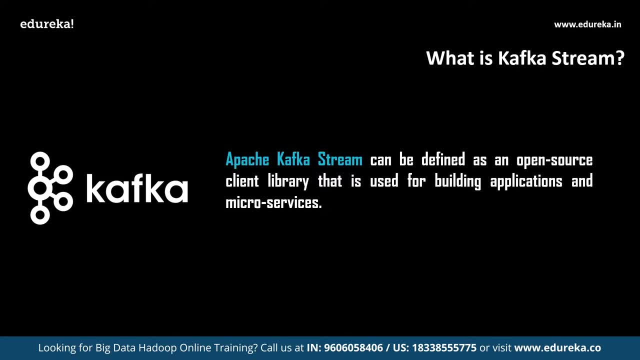 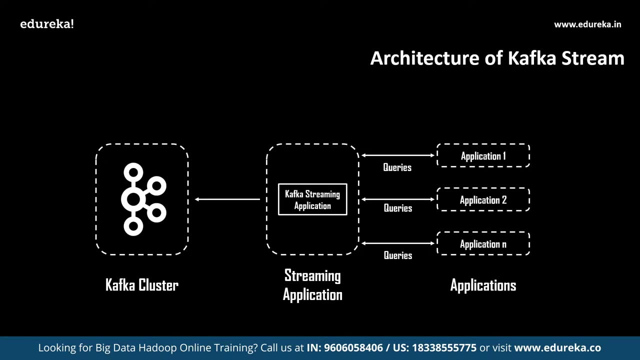 So this was the basic definition of Kafka stream. Now let us understand Kafka stream API in a much better way through its architecture. Apache Kafka streams internally, use the producer and consumer libraries. It is basically coupled with Kafka and the API allows you to leverage the capabilities. 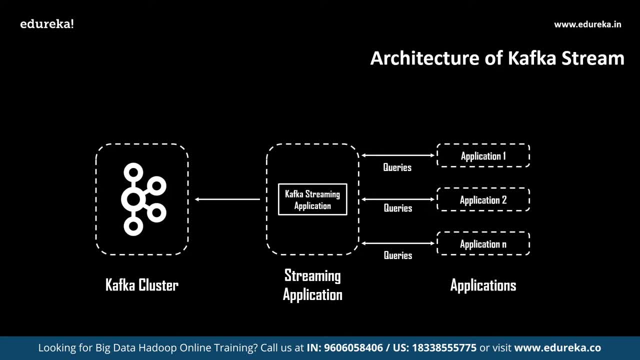 of Kafka by achieving data parallelism, fault tolerance and many other powerful features. The following image depicts the basic architecture of Kafka stream. Here you can see the Kafka cluster, which has the input streams and the output streams together. Followed by that, we have Kafka streaming application. 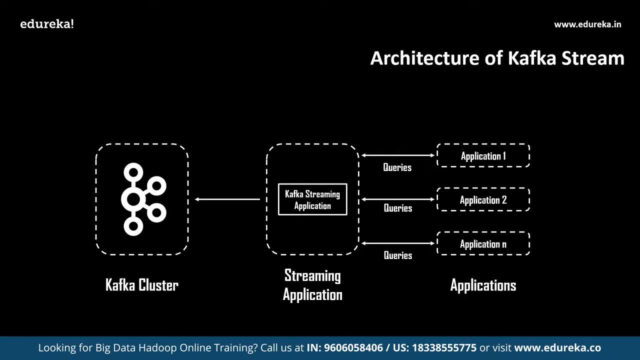 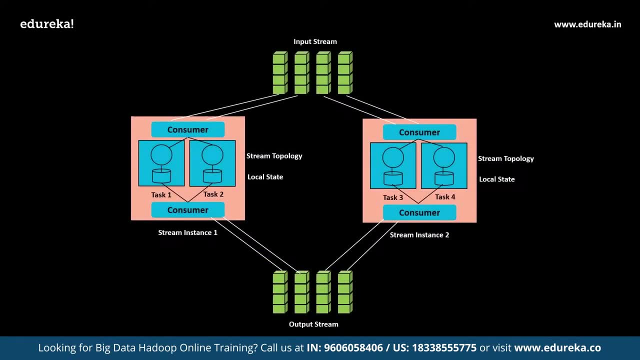 or the API which takes care of the queries which are received from numerous applications which are connected to Kafka streaming application. followed by this, We have numerous components present in Kafka stream architecture, which are as follows. They are input stream, output stream instance. We have two instances here. 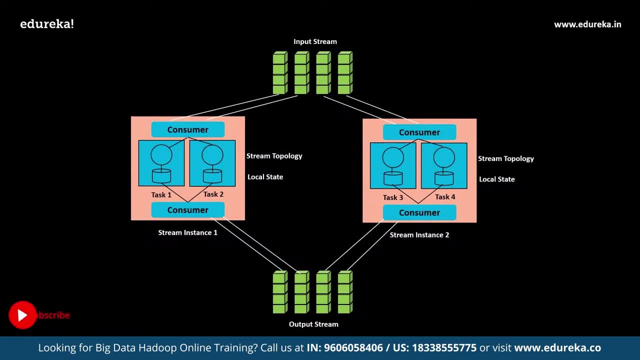 which are stream instance 1 and stream instance 2.. So inside every instance we have consumers as well as local state and stream topology. So in Kafka stream API, input stream and output stream can be one single Kafka cluster. followed by that We have a consumer which provides the input. 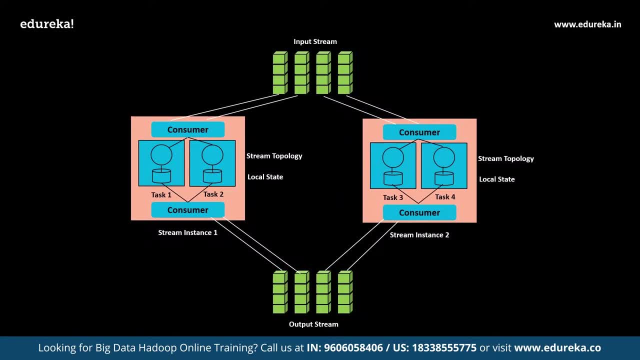 and receives the output, and inside the stream instance We have stream topology and local state, which will understand about stream topology in a much detailed way in the next slide. stream topology is all about the directed acyclic graph, or the steps in which the particular process is executed. 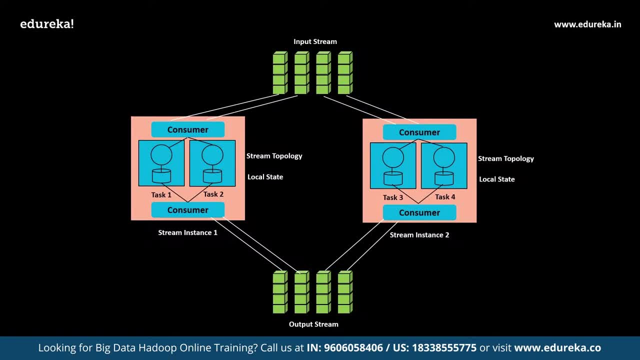 followed by that We have a local state. local state is none other than a memory Location which stores the intermediate data or the result provided by the steam topology. These results are produced after applying various transformations, such as map, flat map, etc. So after the data is processed, the tasks are United together. 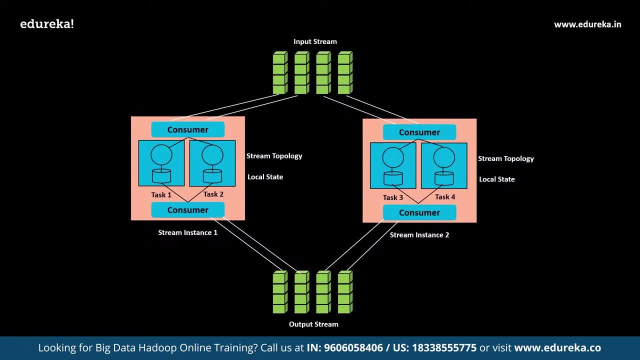 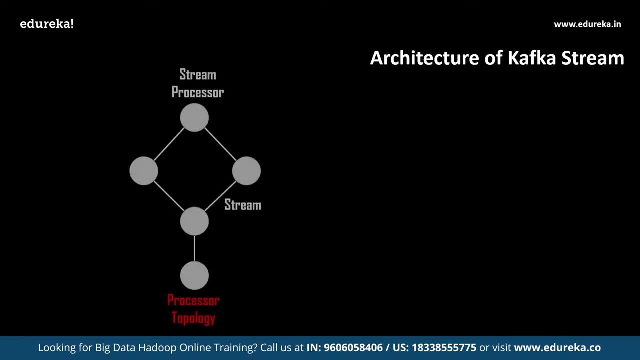 and sent back to output stream. So this is how the architecture of Kafka stream API works. Now let us understand more about stream topology. So this particular diagram explains the stream topology. here You can see the stream process or all the dots which are provided. here are none. 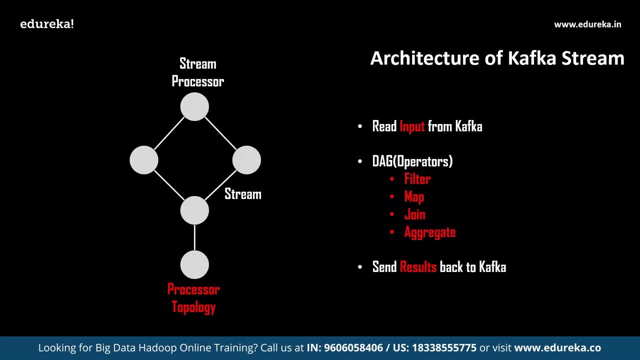 other than stream processors, and the line which is connecting them is the stream. The stream is none other than the key value pairs of the data or records. So, basically, the input is read from Kafka cluster first, followed by that We apply various operators such as filter, map, join, aggregate. 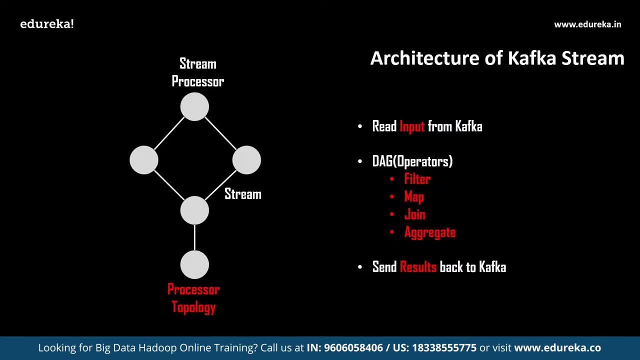 and many more and finally we will receive the results, which will be sent back to the output Kafka cluster. So this is how the stream process works. Topology works. Now Let us discuss the important features of Kafka streams that give it a net over the other similar Technologies. 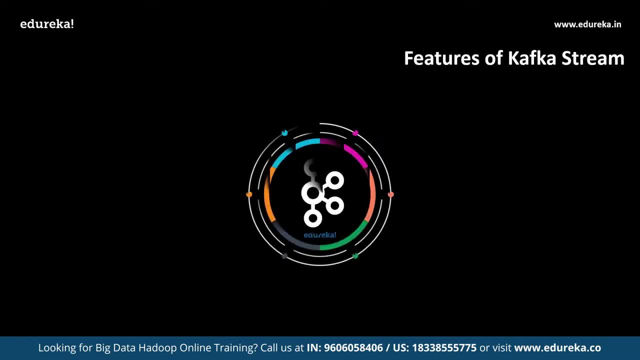 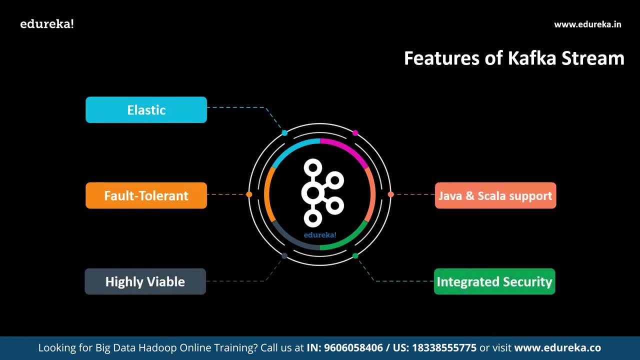 So the various important features of Apache Kafka streams API are elastic, fault-tolerant, highly viable, integrated security, Java and scalar language support. and exactly once, don't worry, We shall discuss each one of them in detail. Firstly, we shall discuss about elastic nature- Apache. 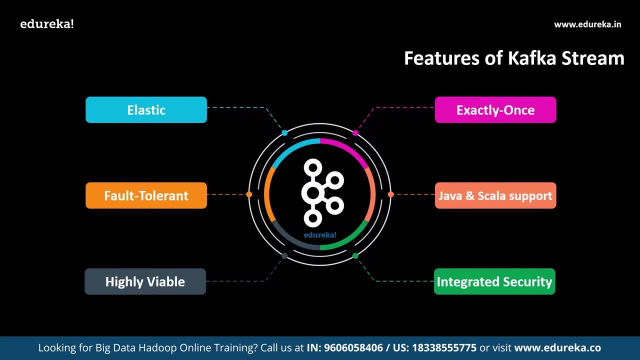 Apache Kafka is an open-source project that was designed to be highly available and horizontally scalable. Hence, with the support of Kafka, Kafka streams, API has achieved its highly elastic nature and can be easily expandable. So this was the first feature, followed by that. 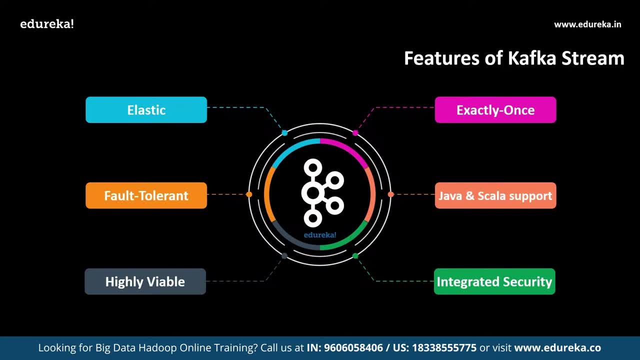 We have the second feature, which is about fault tolerance. The data logs are initially partitioned, and these partitions are shared among all the servers in the cluster that are handling the data and their respective requests. Kafka achieves fault tolerance by duplicating each partition over a number of servers, followed by fault tolerance. 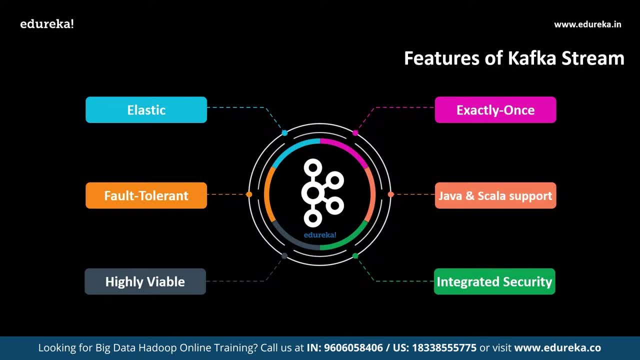 We have the next important feature that is highly viable, since Kafka clusters are highly available. They can be preferred to any sort of use cases, regardless of their size. They are capable of supporting small scale use cases, medium scale use cases Also, the large scale use cases followed. 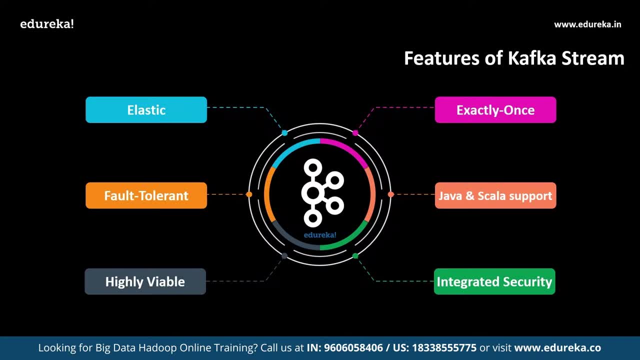 by highly viable feature. We have integrated security. Kafka has three major security components that offer the best-in-class security for the data in its clusters. They are mentioned as follows. They are encryption of data using SSL or TLS, followed by that authentication of SSL or SASL. 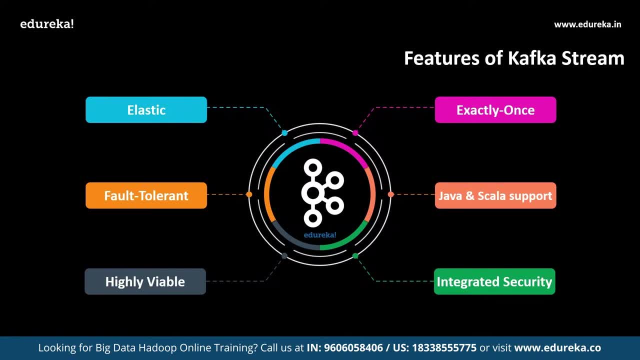 and, finally, the authorization of ACLs. So, followed by the security, we have its support for top and programming language. the best part of Kafka streams API is that it integrates itself with the most dominant programming languages, such as Java and Scala, and makes designing and deploying Kafka server-side applications with ease. 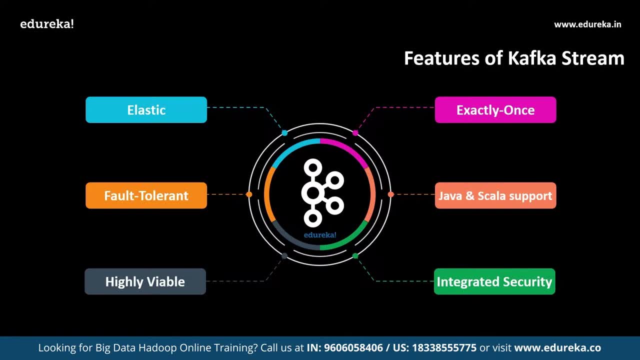 Followed by that, we have exactly once processing semantics. Usually stream processing is a continuous execution of unbounded series of data or events, But in the case of Kafka it is not. Exactly once means that the user defined statement or logic is executed only once and the updates 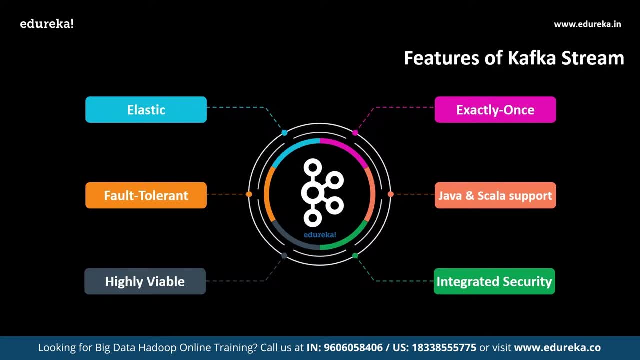 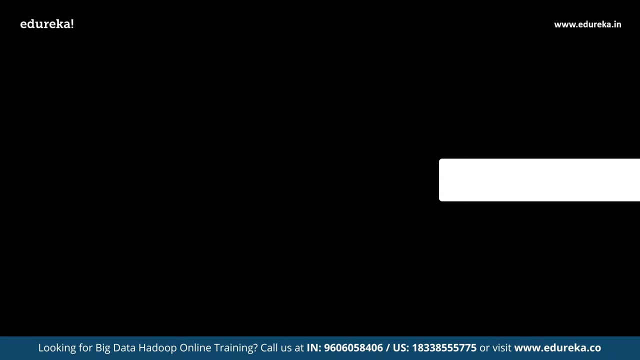 to the state, which are managed by SPE or stream processing element, are committed only once in a durable back in store. So this is how Apache Kafka streaming API is considered to be having exactly once processing semantics. So, followed by the important features, We shall go through a sample program based. 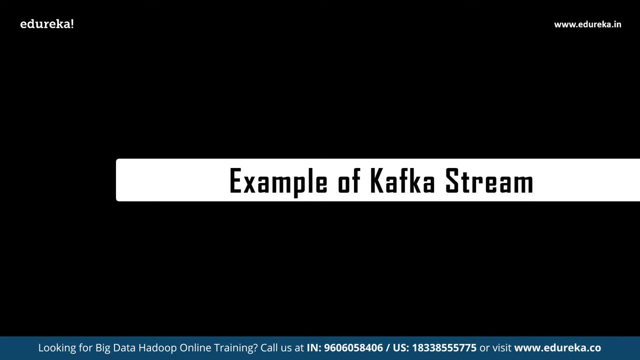 on Kafka streams API. So this is how this particular example can be executed using Java programming language. yet There are few prerequisites on this one. One needs to have Kafka and zookeeper installed in the local system and it should be running in the background. 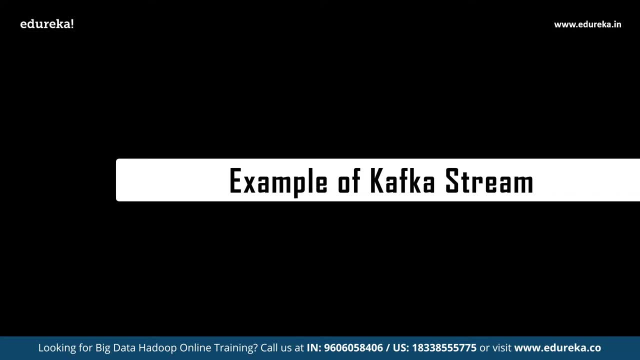 If you have not installed zookeeper and Kafka in your local system, then I have linked the article in the description box below, which will explain you about the detail installation procedure of zookeeper and Kafka in your local system. Once the zookeeper and Kafka are installed into your local system, 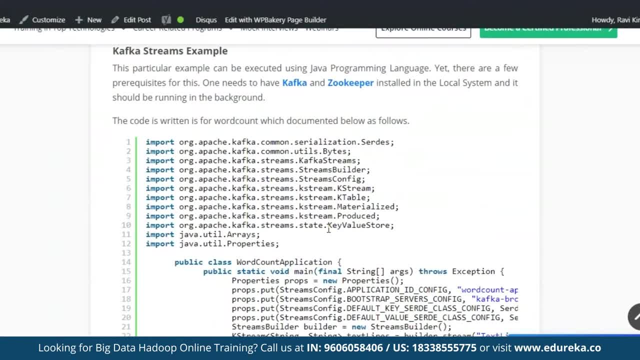 You need to fire them up. once the Kafka and zookeeper are successfully installed into your local system and they are running in the background, You can go to Kafka and define a producer topic and the consumer. once the producer topic and consumer are defined, you can come back to Kafka article. 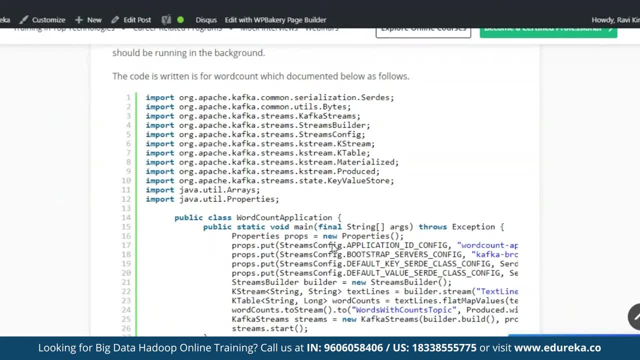 and execute the following code in any of the Java editors. The code will count the number of words that you have provided in your text document and you will receive the output as shown in the article here. Here, the text given to the code was welcome to edureka. 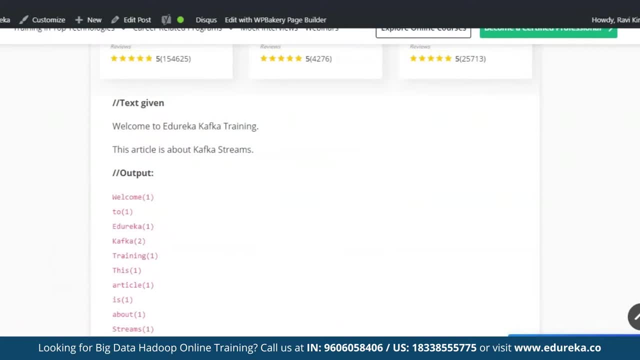 Kafka training and this article is based on Kafka streams. These were the two sentences given to the program and the output is as shown below. here The word welcome is repeated for once, to is repeated for once, edureka once, Kafka is repeated for two times and training is once. this article is about streams. 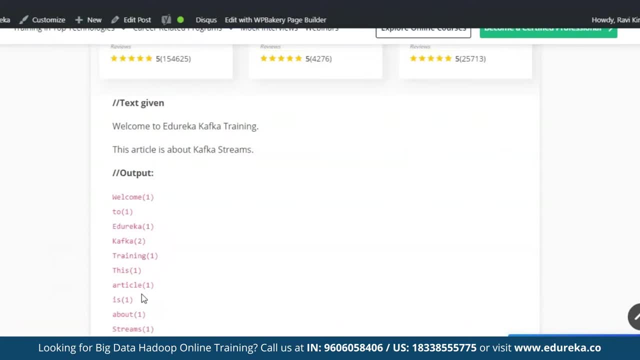 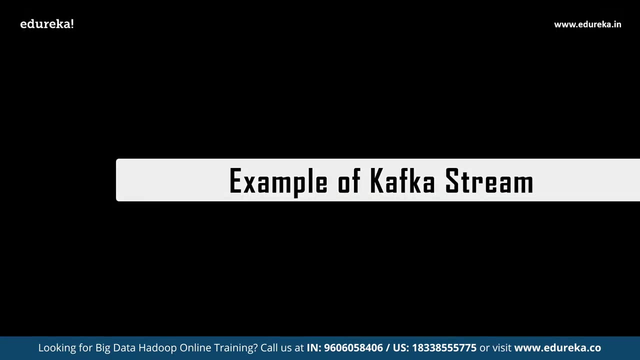 So all these words are repeated for once. So this is how exactly you should be receiving the output once after you execute the following code in your own Java editor: So, followed by the example based on Kafka streams, we can move ahead and understand the important differences. 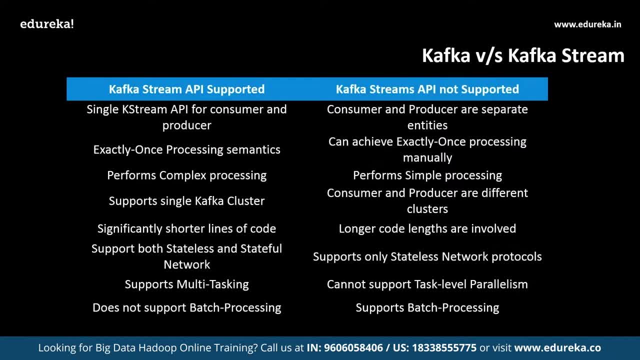 between Kafka and Kafka streams. So now, the first difference is that in Kafka stream API single Kafka cluster can support as both consumer as well as producer, while on the other hand, in Kafka We need separate consumer and producer, and Kafka considers consumer and producer as separate entities. 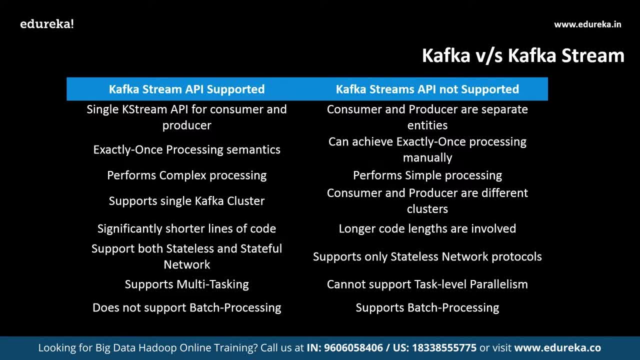 The second difference is that in Kafka API exactly once processing semantics are supported, whereas in Kafka It is not by default, but you can achieve exactly once processing in Kafka manually. The third difference is that Kafka streams API is capable enough to perform complex operations. 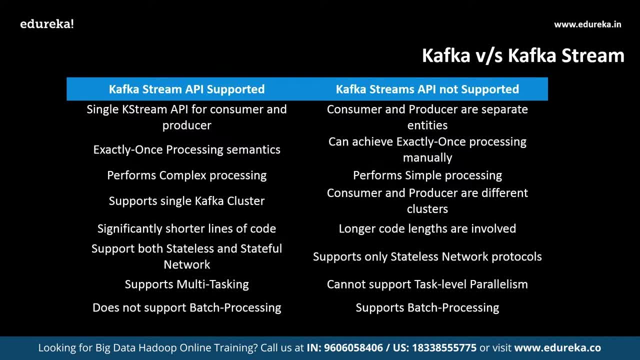 Whereas Kafka is designed to perform only simple operations. The fourth difference is that Kafka API supports single Kafka cluster. on the other hand, in Kafka You need two different clusters for producer and consumer, followed by that. in Kafka API, The code length is significantly shorter when you come into Kafka. 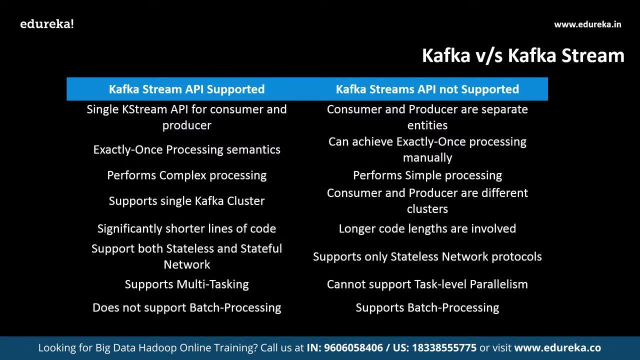 The code length involved is highly lengthy. The next difference between the both is Kafka streams API can support both stateless and stateful networks. What are stateless and stateful networks? in stateless networks, The client provides requests to the server and he gets instantaneous reply from server. 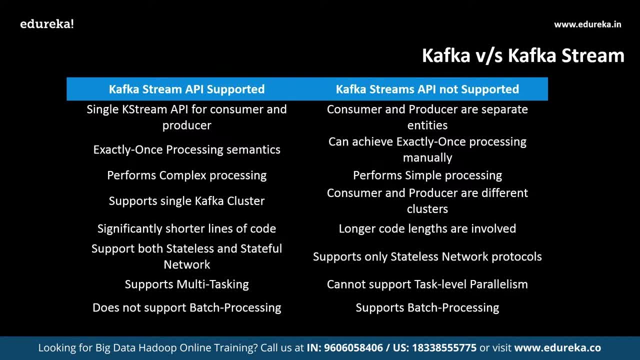 and here the cookies or the request which are sent by the client are not stored, Whereas if you come into stateful network, the client request the server along with some additional data which is required by the server. in this case, the cookies or the request which are provided by the client are recorded. 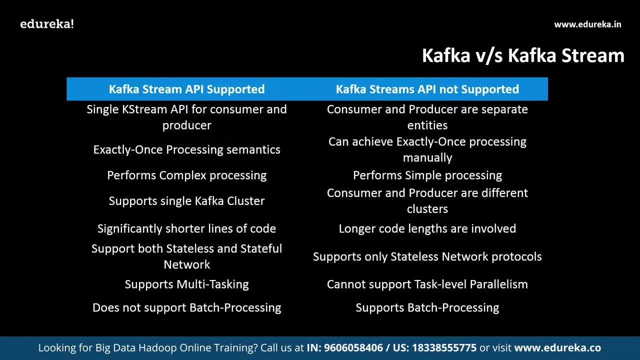 So Kafka stream API is capable to support both stateless and stateful networks, But, on the other hand, Kafka is capable only to support stateless network protocols. followed by that, the Kafka streams API can support multitasking, Whereas Kafka is not capable to support multitasking. 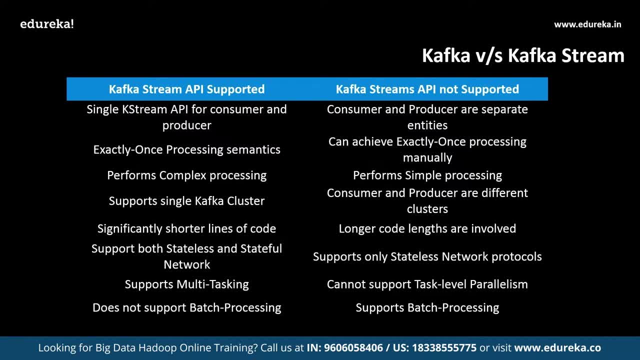 at a single task level, followed by that Kafka stream API does not support batch processing, Whereas Kafka is capable to support batch processing. Kafka stream API is all about real time, So it doesn't have to support batch processing. So these are the few important differences. 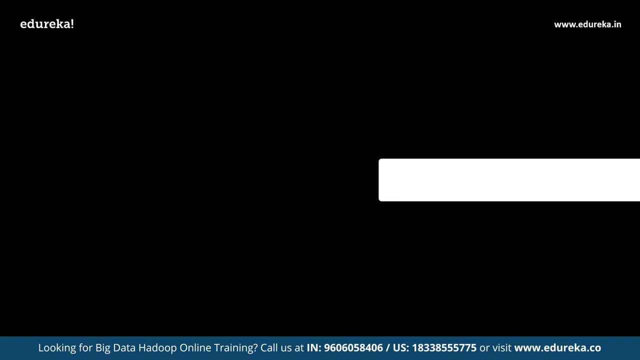 between Kafka streams API and Kafka. Now we shall move ahead and wind up the session with our last topic, which are the important use cases based on Apache Kafka streams API. Apache Kafka streams API is used in multiple use cases. some of the major applications where streams API is being used. 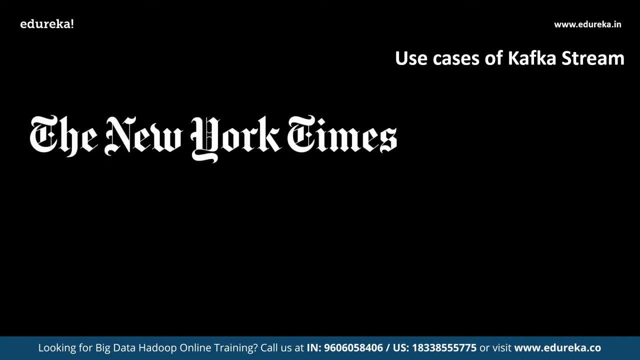 are mentioned as follows. Firstly, the New York Times. the New York Times is one of the powerful media in the United States of America. They use Apache Kafka and Apache Kafka streams API to store and distribute the real-time news through various applications and systems to their readers. followed, 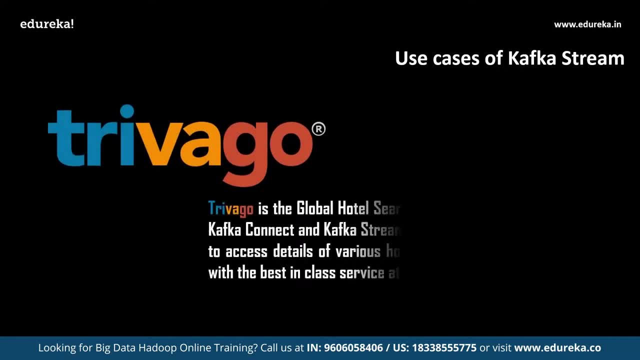 by the New York Times. We have Trivago. Trivago is the global hotel search platform. They use Kafka, Kafka connect and Kafka streams to enable their developers to use to access details of various hotels and provide their users with the best in class service at lowest prices. and finally, 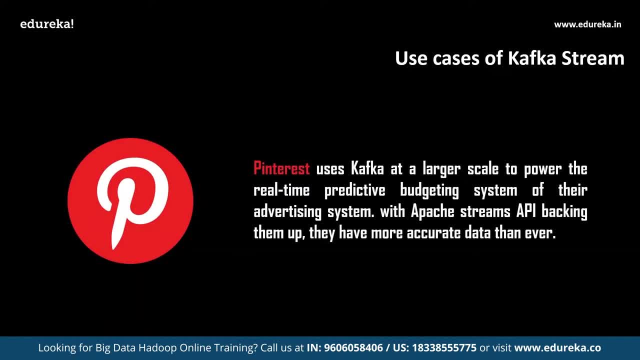 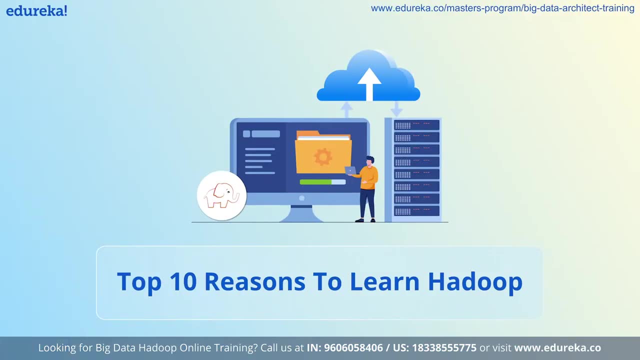 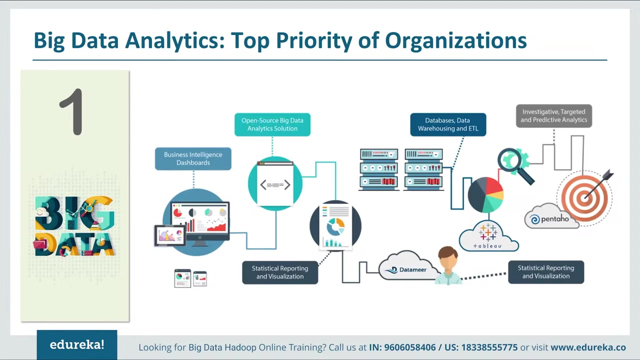 Pinterest. Pinterest uses Kafka at a longer scale to power the real-time predictive budgeting system of their advertising system, with Apache streams API backing them up. They have more accurate data than ever. Reason number one: the top priority of organizations is now big data analytics. 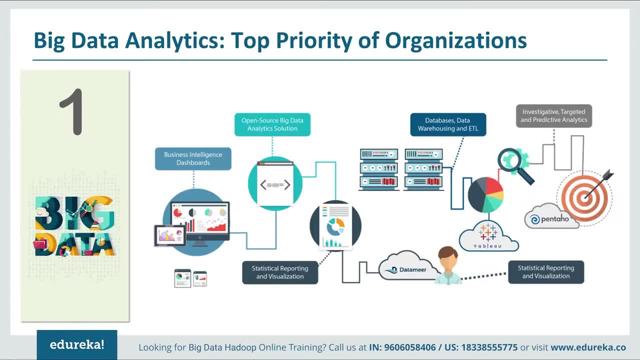 Well, big data has been playing a role of a big game changer in most of the industries over the last few years. In fact, big data has been adopted by vast number of organizations belonging to various domains, and by examining large data sets using big data tools like Hadoop and Spark, they are able to identify hidden patterns. 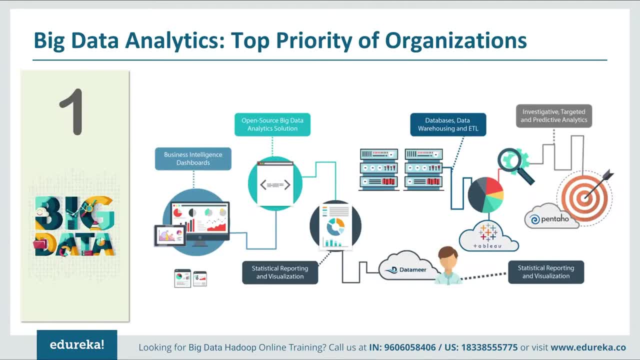 to find unknown correlations, market trends, customer preferences and other useful business information. And let me tell you that in an article in Forbes it was published that big data adoption has reached up to 53% in 2017, from 17% in 2015 with telecom. 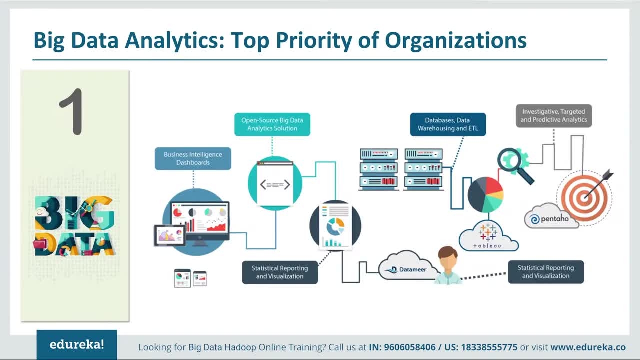 and financial services leading early adopters, and the primary goal of big data analytics is to help companies make better and effective business strategies by analyzing large data volumes. The data sources include web server logs, internet click stream data, social media content and activity reports, text from customer emails, phone call details and machine data. 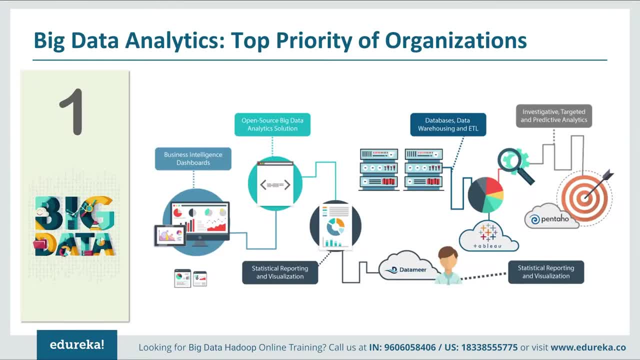 captured by sensors and connected to the internet of things- IOT as we call it. Big data analytics can lead to more effective marketing, new revenue opportunities, better customer services, improved operational efficiency, competitive advantages over rival organizations and other business benefits, and that is why it is so much widely used. 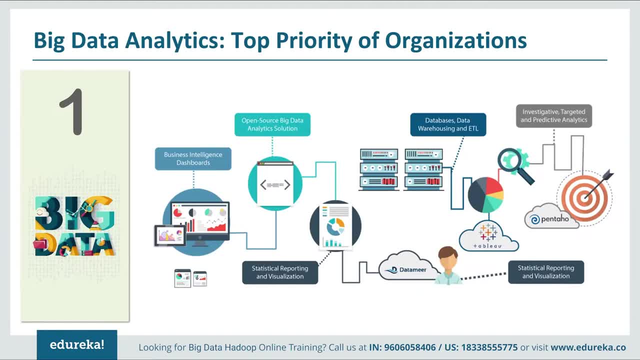 And IDC says that the commercial purchases of big data and business analytics related hardware, software and services are expected to maintain a compound annual growth rate, or CAGR, of 11.9% through 2020, when revenues will be more than 210 billion dollars. 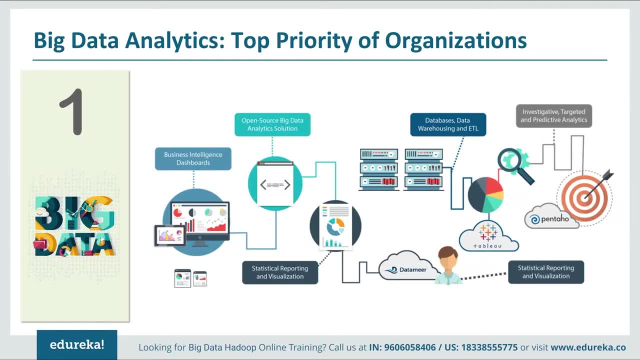 And that is huge. And the image here clearly shows the tremendous increase in unstructured data like images, mails, audio, etc. which can only be analyzed by adopting big data technologies like Hadoop, Spark, Hive and others. This has led to serious amount of skill gap with respect. 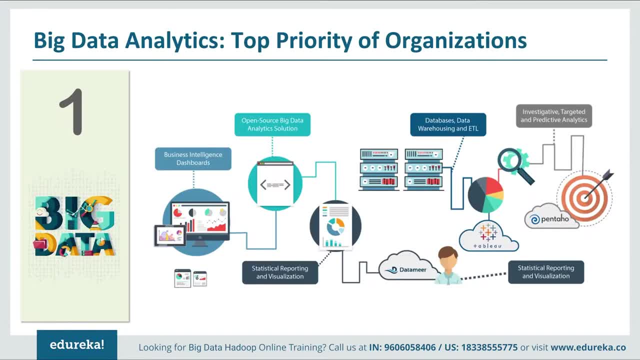 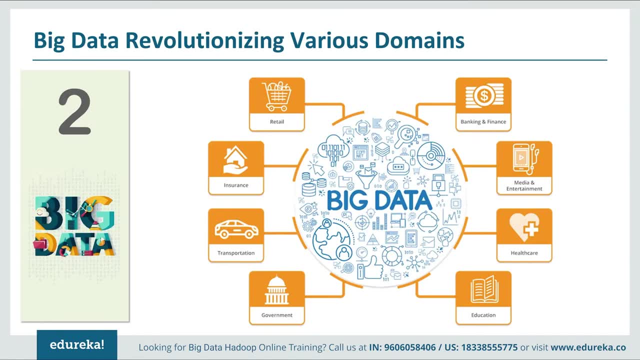 to available big data professionals in the current IT market, and hence it is not at all surprising to see a lot buzz in the market to learn Hadoop. Reason number two: Big data is revolutionizing various domains Now big data is not leaving any stone unturned nowadays. 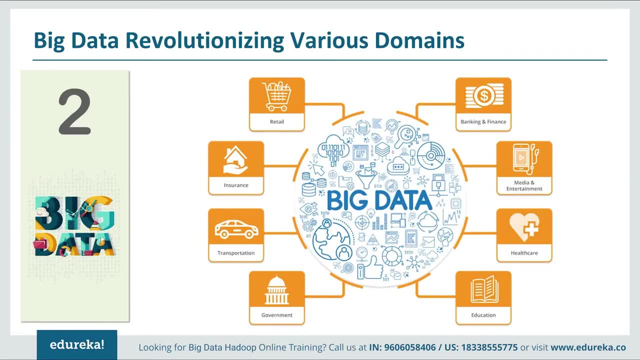 What I mean by this is that big data is present in each and every domain, allowing organizations to leverage its capability for improving their business values. The most common domain which are rigorously using big data and Hadoop are healthcare, retail, government, banking, media. 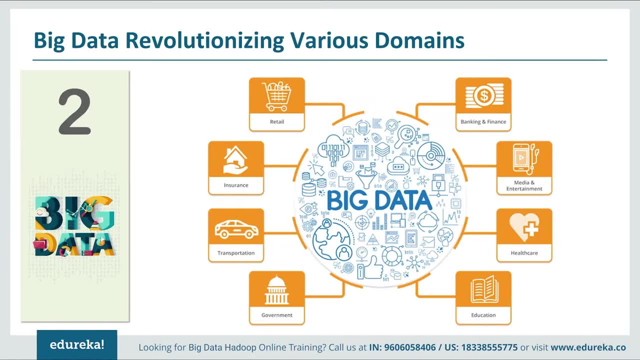 and entertainment, transportation, natural resources and so on, as shown in the image over here. Well, to be honest, it is not only limited up to these domains mentioned here. Big data is spreading even more across different domains. As the technology is evolving, the data is increasing and hence 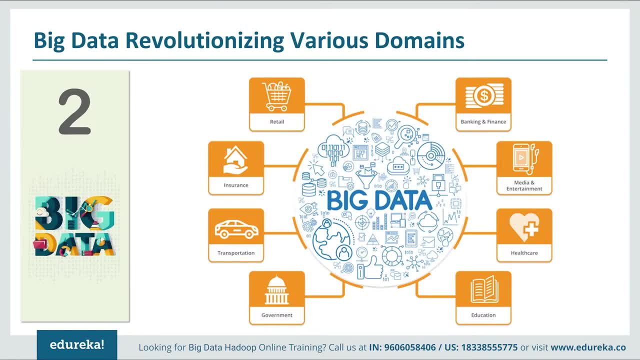 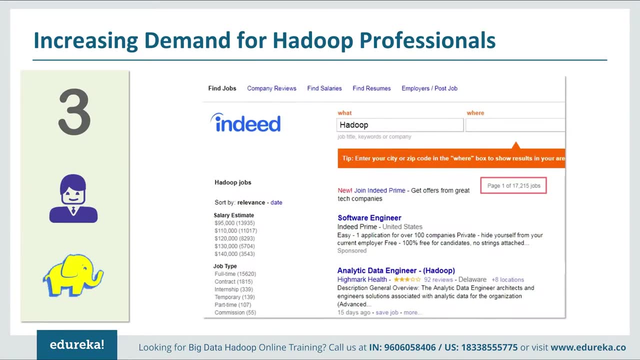 big data is getting adopted across a wide range of domains. Hence you can build your career in any of these domains by learning Hadoop. Reason number three: Increasing demand for Hadoop professionals. The demand of Hadoop can be directly attributed with the fact. 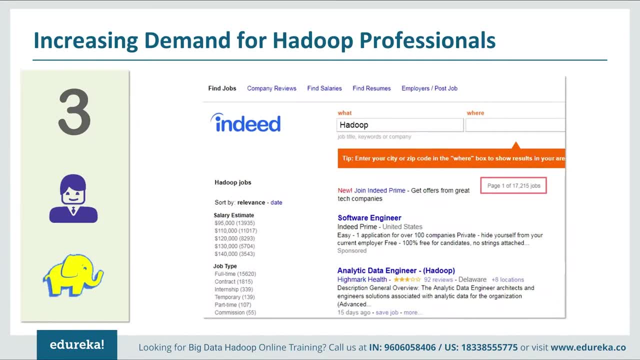 that this is one of the most prominent technology that can handle big data and is quite cost effective and scalable. With the swift increase in big data sources and amount of data, Hadoop has become more of a foundation for other big data technologies evolving around it, such as Spark, Hive, etc. 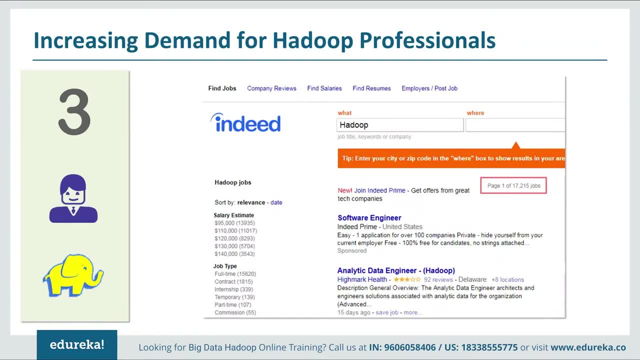 And this is generating a large number of Hadoop jobs at a very steep rate. You can check out different job portals like indeedcom, Knockread Times, Job, etc. and you will see the demand of Hadoop professionals when you browse through the job postings. 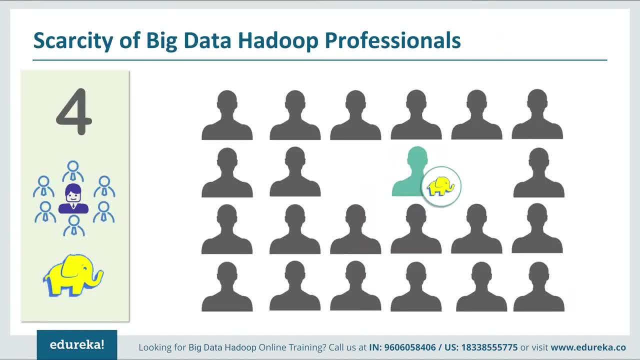 Reason number four: Scarcity of big data Hadoop professionals. Now, the demand must be more, but the supply is quite less And, as we discussed Hadoop, job opportunities are growing at a high pace, But most of these job roles are still vacant due to a huge skill gap. 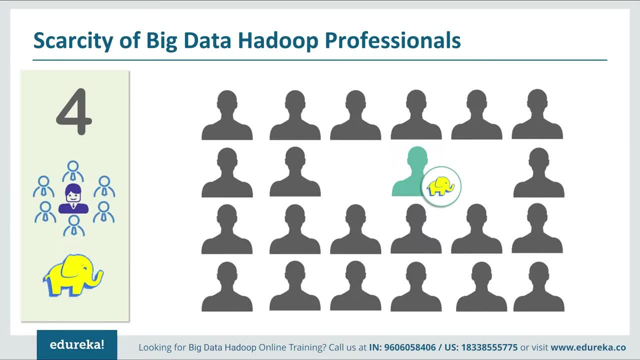 that is still persisting in the market, And such scarcity of proper skill set for big data Hadoop technology has created a vast gap between supply and demand chain, And hence now it is the right time for you to step ahead and start your journey towards building a bright career in big data and Hadoop. 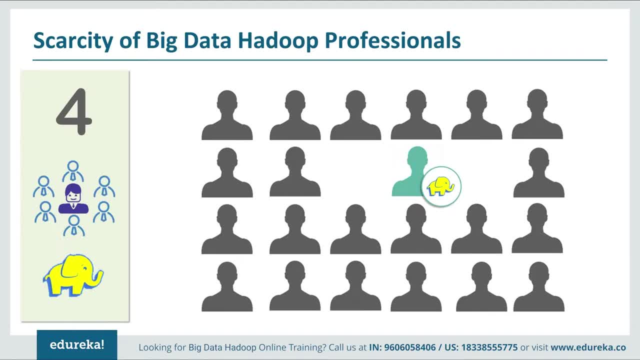 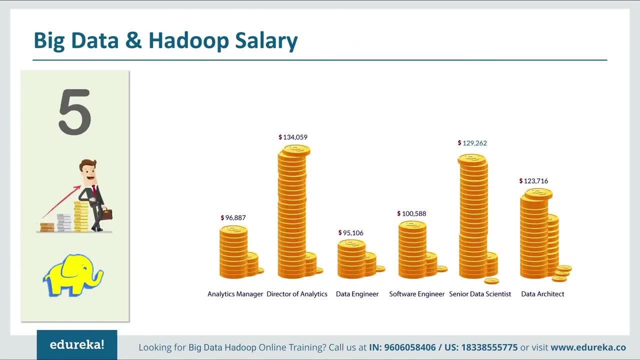 In fact the famous saying now or never. This is an apt description that explains the current opportunities in the big data and Hadoop market. Reason number five: Big data and Hadoop salary. This, in fact, is quite rewarding. One of the captivating reason to learn Hadoop is the fat paycheck. 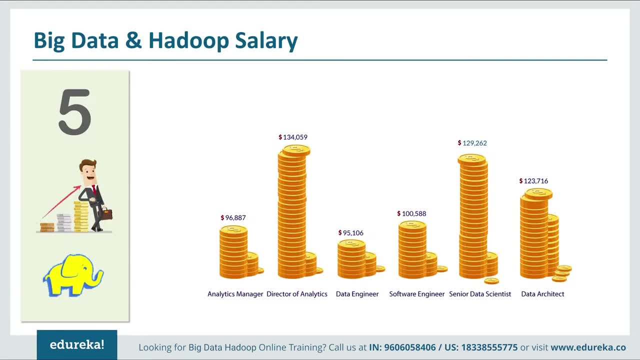 that you are going to get. The scarcity of Hadoop professionals is one of the major reasons behind their high salary And, according to payscalecom, the salary of a Hadoop professional varies from $93,000 to $127,000 a year. 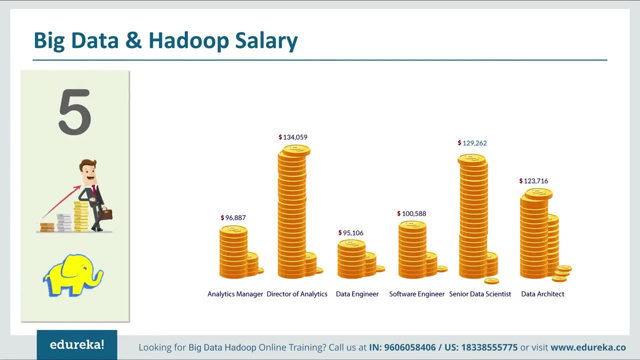 That's $27,000 per annum, based on different job roles. You can see the different job roles and their annual salaries over here, But of course it can vary according to the organization that you're joined in and also with the experience you have. 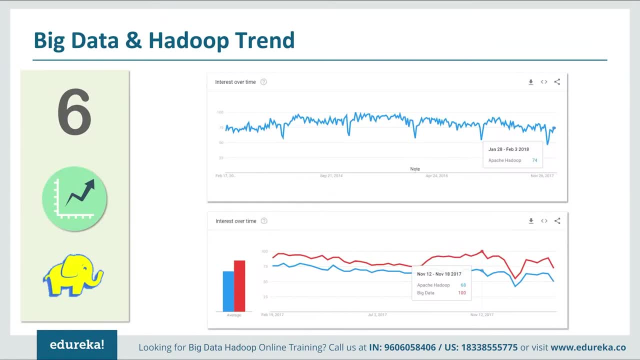 Reason number six: The big data and Hadoop trend. And as per Google trends, Hadoop has a stable graph in the past five years, And one more interesting thing to notice here is that the trend of big data and Hadoop are tightly coupled with each other. 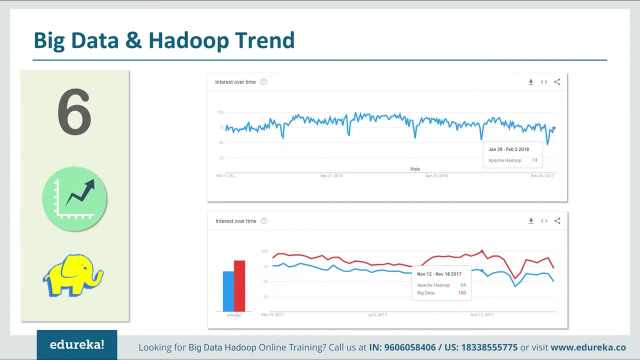 You can see over here that they go hand in hand and have a direct correlation. Big data is something which talks about the problem that is associated with storage, curation, processing and analyzing of the huge amount of data, And hence it is quite evident that all of the companies need to tackle. 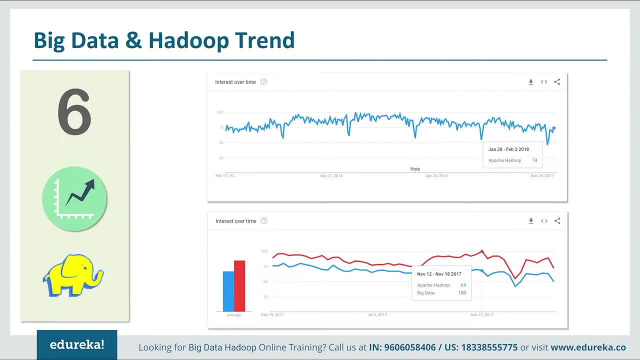 the big data problem one way or another for making better business decisions, and hence one can clearly deduce that big data and Hadoop has a promising future and is not something that is going to vanish into thin air, at least for the next 20 years. 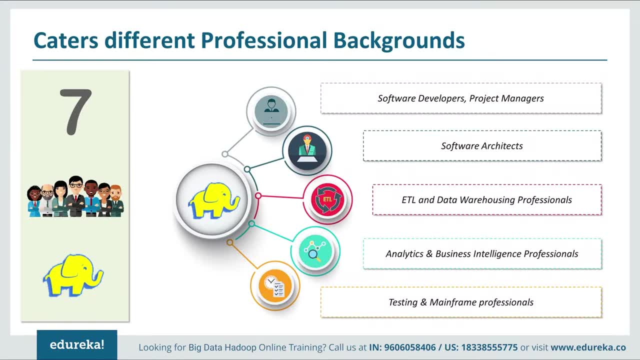 Reason number seven: It caters different professional backgrounds. Hadoop ecosystem has various tools which can be leveraged by professionals from different backgrounds. If you are from programming background, you can write MapReduce codes in different languages like Java, Python, etc. If you are exposed to scripting language, Apache Pig is the best fit for you. 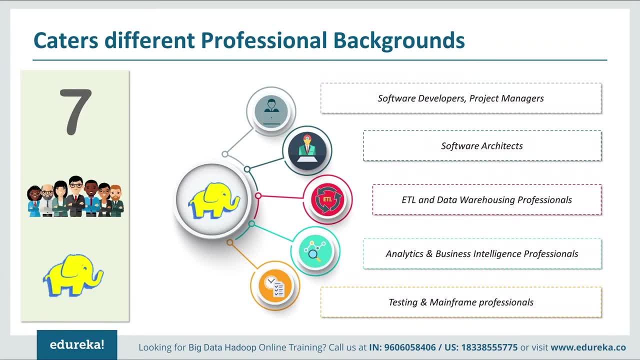 And if you are comfortable with SQL, then you can also go ahead with Apache Hive or Apache Drill. The market of big data analytics is growing across the world and its strong growth pattern translates into great opportunity for IT professionals. It is suited for developers, project managers, software architects. 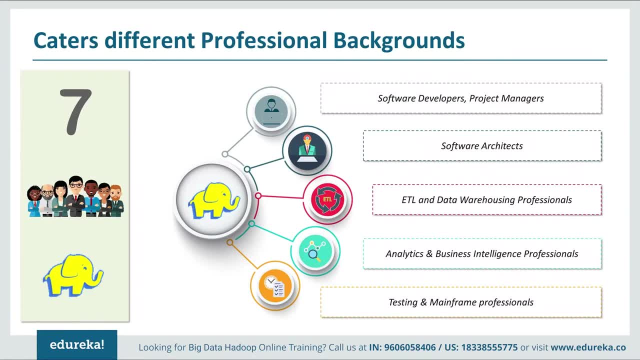 ETL and data warehousing professionals, analytics and business intelligence professionals, and also for testing and mainframe professionals. It is also recommendable for freshers who are going to start a fresh career in the IT world. So if you start with big data, I am very sure that you are going to have 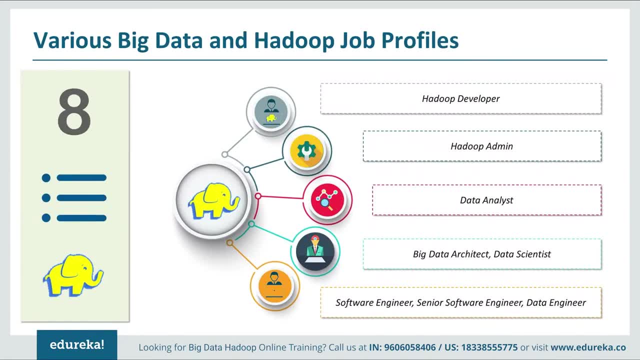 a bright future ahead. Reason number eight: The different big data and Hadoop job profiles. So there are various job profiles in big data and Hadoop Learning. big data and Hadoop doesn't mean that you will be sticking on to just analytics. 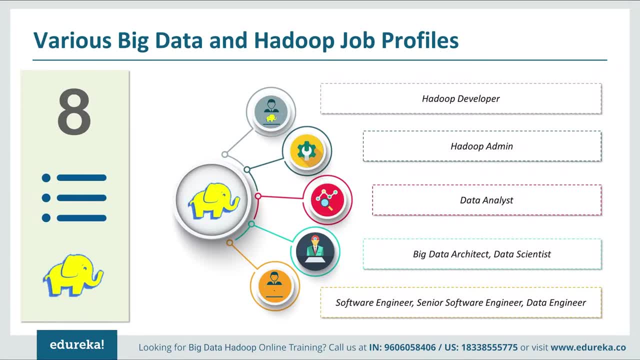 You can pursue any one of these job roles based on your professional backgrounds. You could be a Hadoop developer, a Hadoop admin, a data analyst, a big data architect or a data scientist, software engineer, senior software engineer, data engineer- whatever seems more convenient for you. 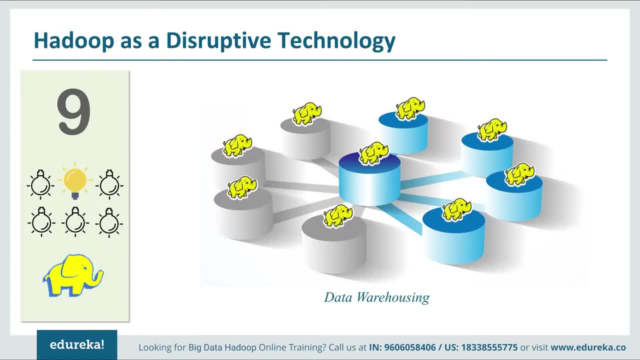 Reason number nine: Hadoop is a disruptive technology. When Hadoop came into the market, it completely disrupted the existing market and created a market of its own. Hadoop has proven itself as a better option than that of traditional data warehousing systems in terms of cost scalability, storage and performance. 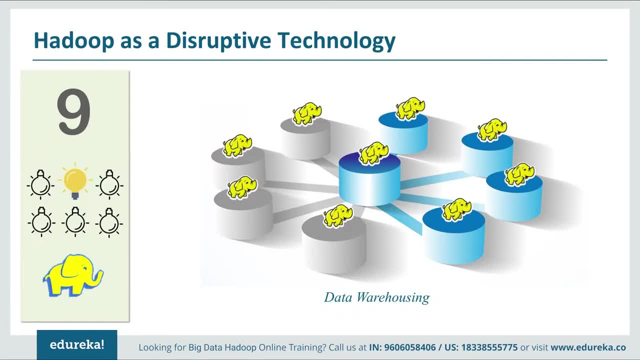 over a variety of data sources. It can handle structured data, unstructured data and semi-structured data. In fact, Hadoop has revolutionized the way data is processed nowadays and has brought a drastic change in the field of data analytics. Besides this Hadoop ecosystem is going through continuous 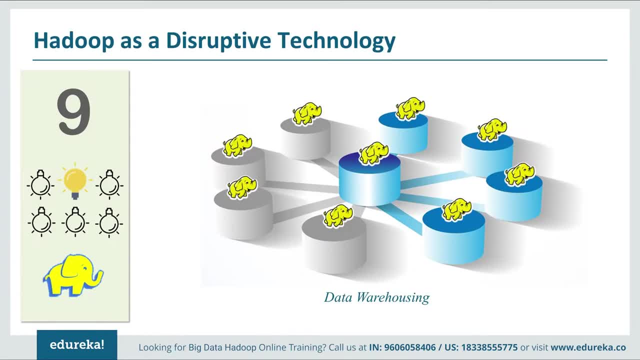 experimentations and enhancements. In a nutshell, I would tell you that big data- Hadoop- is taking out the world by storm And if you don't want to get affected, you have to ride with the tide. Reason number 10, and the most important one: 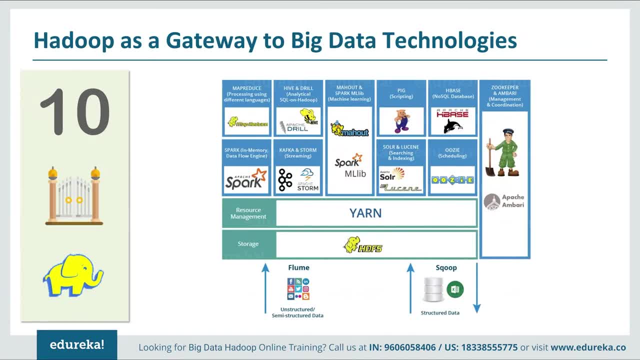 Hadoop is the gateway to all the big data technologies. Hadoop has become a de facto for big data analytics And has been adopted by a large number of companies. Typically, besides Hadoop, a big data solution strategy involves multiple technologies in a tailored manner. 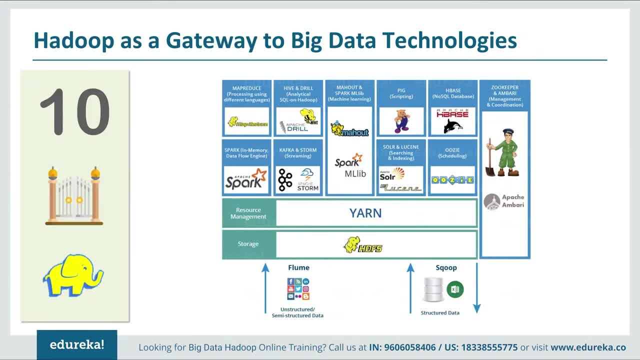 So it is essential for one to not only learn Hadoop, but become expert on other big data technologies falling under the Hadoop ecosystem. This will help you to further boost your big data career and grab elite roles like that of a big data architect, data scientist, etc. 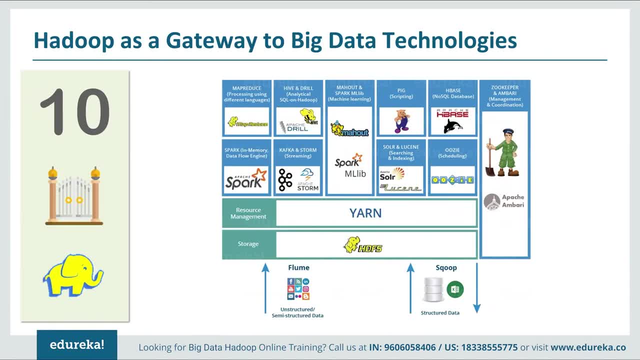 So if you want to become a big data architect or a data scientist, Hadoop is the best option to get started with. Hadoop is the stepping stone for you to move into the big data domain. So here were the top 10 reasons to learn Hadoop. 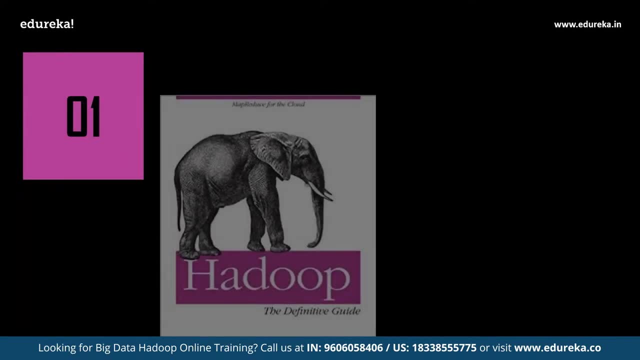 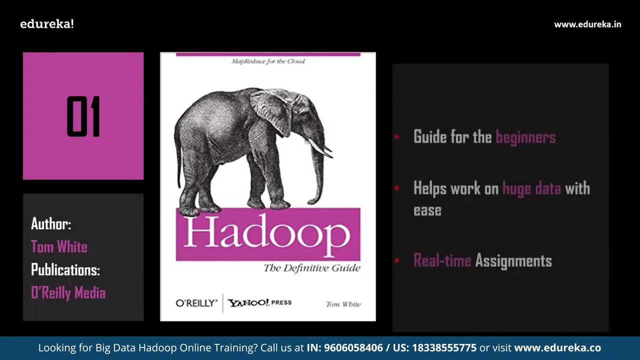 So the first book in the beginner's section is Hadoop Definitive Guide. So this particular book was written by Tom White and the publisher is O'Reilly Media. So let's have a quick overview of this particular book. If you are a complete beginner, 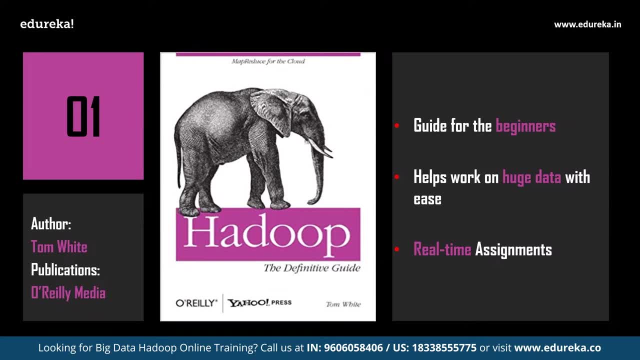 then there is no better book than Hadoop Definitive Guide. This book guides beginners to build a reliable and easily maintainable Hadoop configuration. It helps to work on data sets regardless of sizes and types. It has numerous assignments that help you understand Hadoop real-time. 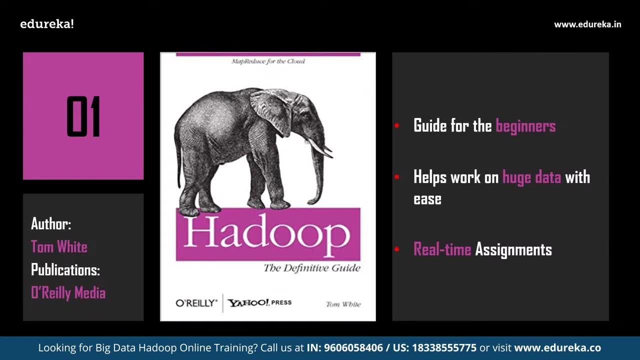 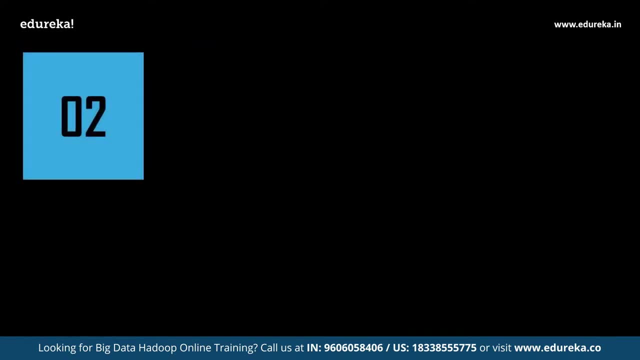 functionality in a much better way. Going through this book will help you to understand even the latest changes very easily, followed by the first book. The second book in the beginners section is Hadoop in 24 hours. So this particular book was written by Jeffrey even. 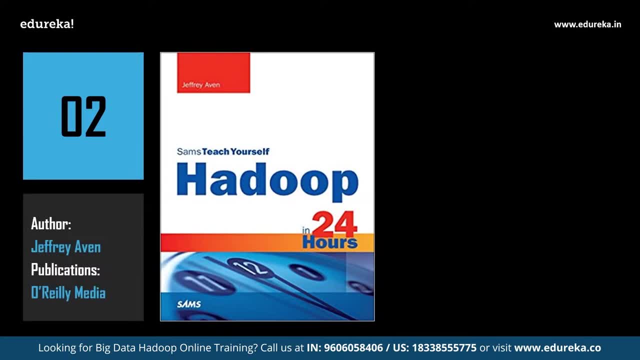 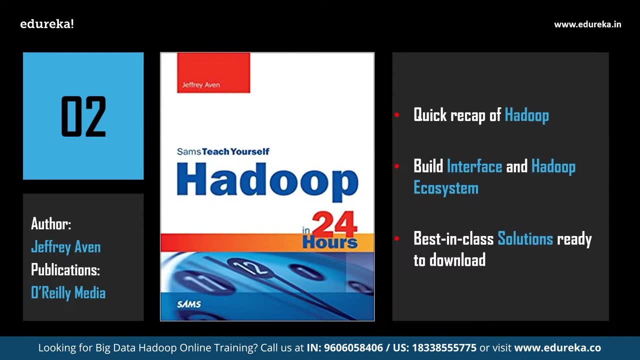 and this book was published by O'Reilly Media. Let's have a quick overview of this book in case. if you already have a brief idea on Hadoop and want to have a quick recap of the technology, Then this book is for you. This particular book gives you a perfect overview. 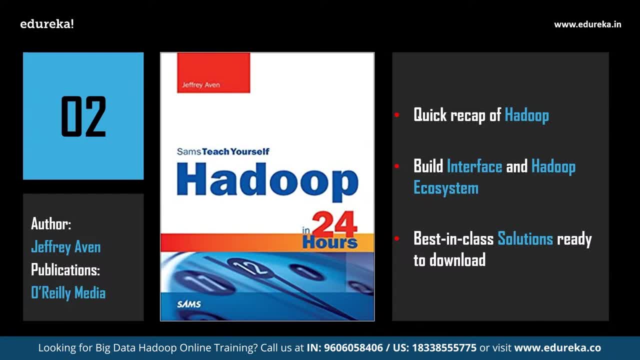 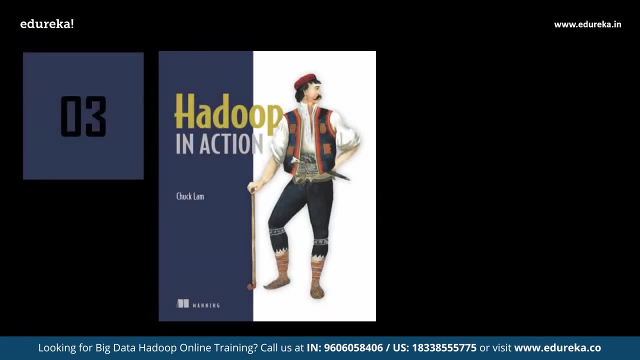 of building a functional Hadoop platform interface, all Hadoop ecosystem components and many more. Also, if you're looking for some real-time examples, then it has the best in class setup solutions ready for download, followed by the second book. The third book in the section is Hadoop in action. 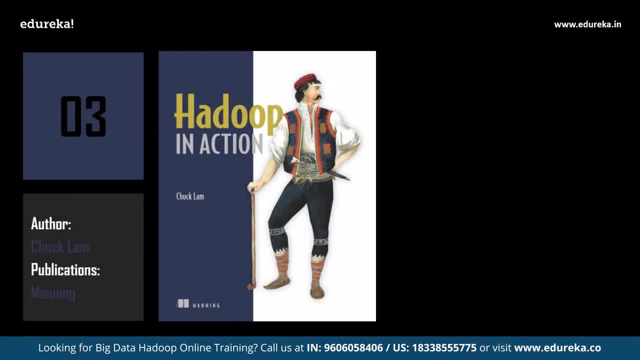 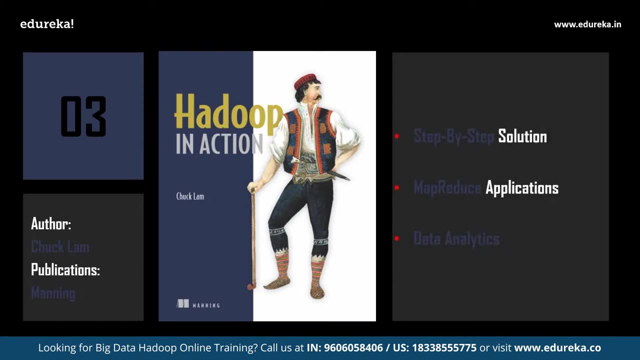 This particular book was written by Chuck lamb and the publisher is Manning publications. Let's have a quick review of this particular book. Hadoop in action is like the one-step solution to learn how to from scratch. This book basically starts from the default Hadoop. 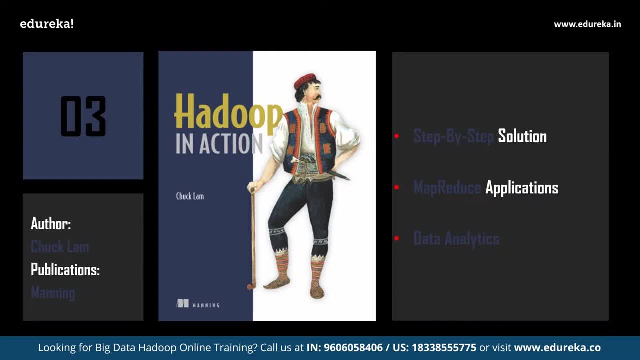 installation procedures followed by the installation. It explains all about the most crucial components of Hadoop, the MapReduce and many more also. the book deals with some real-time applications of Hadoop and MapReduce, including the major big data frameworks which are used in data analytics. 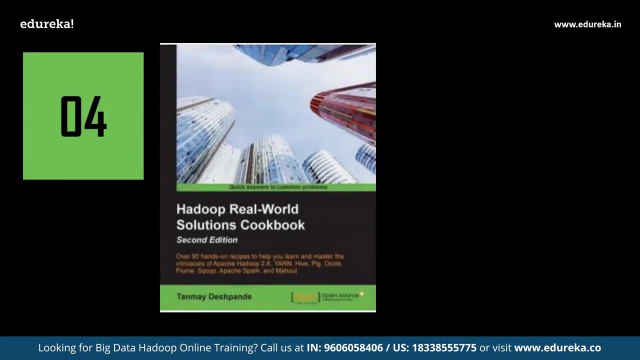 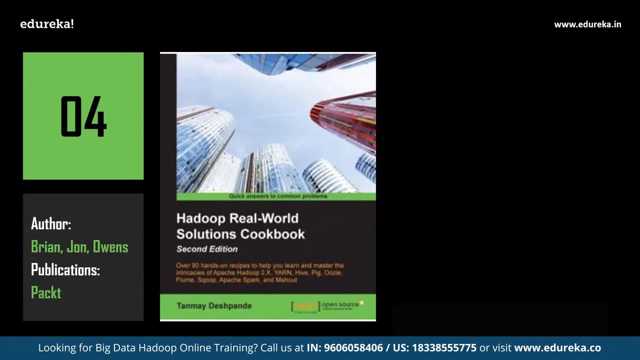 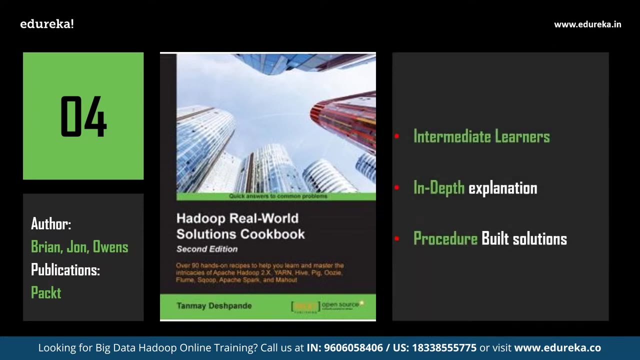 So the last book in the beginner section is Hadoop: real-world solutions. This particular book is written by three authors. They are Brian John and Jonathan Owens, And the publisher of this particular book is packed publishing. and now let's have an overview of this particular book. 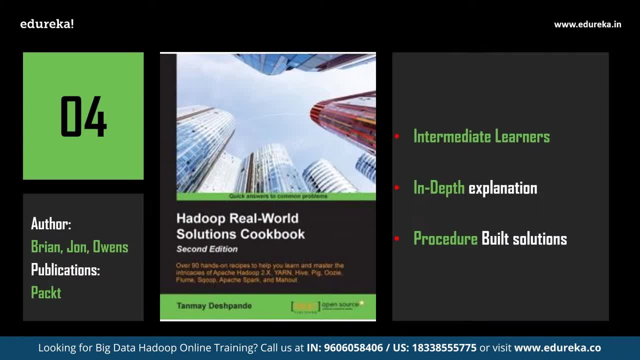 This particular book is for the intermediate learners who are looking to try out multiple approaches to resolve the problems. This book has an in-depth explanation of the concepts, problem statements, technical challenges, steps to be followed and crystal-clear explanation of the code used. You will also understand the procedures to build solutions. 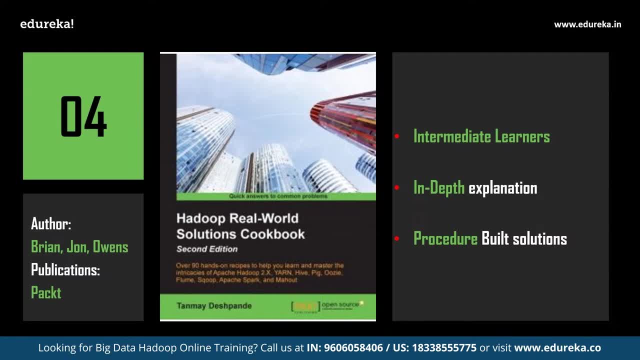 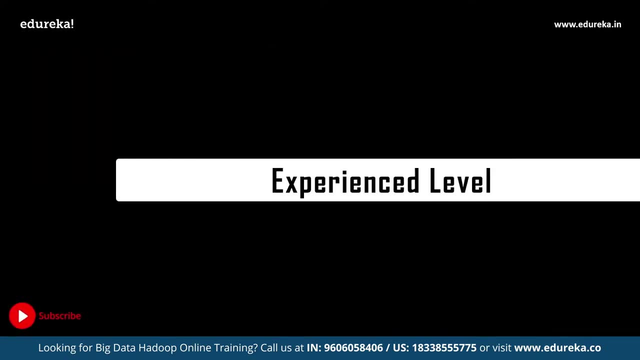 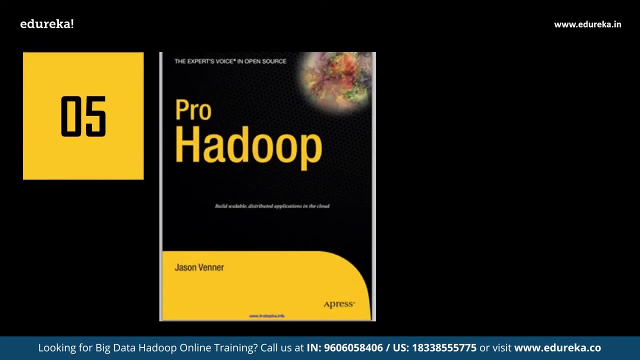 using tools like Apache, Hive, Apache Pig, my house Graph, HDFS and many more crucial components. Now we should learn about some books for the experienced programmers. So the first one amongst the books for the experienced Hadoop developers are pro Hadoop. This particular book was written by Jason Venom. 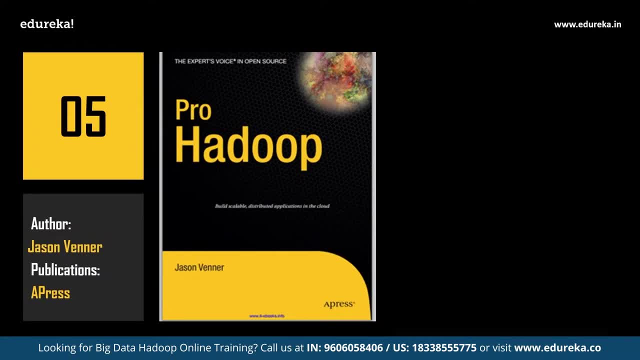 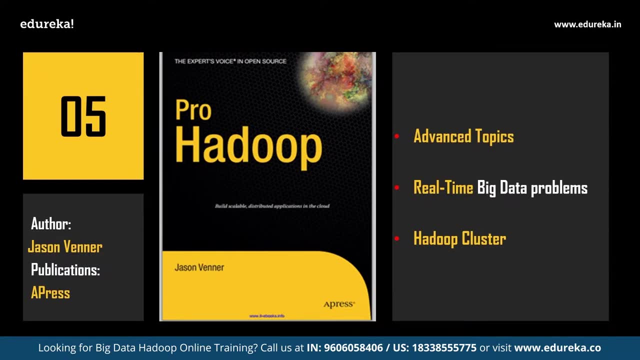 and it was published by a press publications, and the overview goes like this: This particular book against the readers and upgraded stage to play with Hadoop, The Hadoop clusters. this book covers every single detail related to Hadoop clusters, starting from setting up a Hadoop cluster. 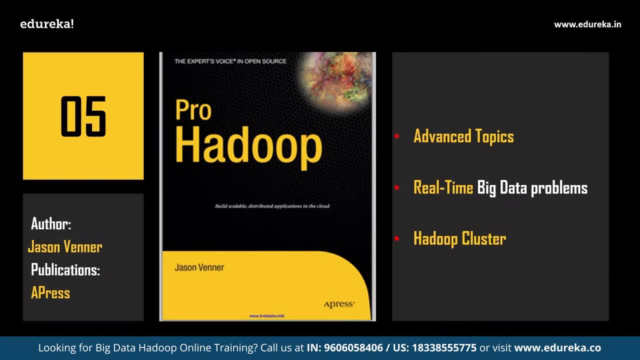 to analyzing and deriving valuable information for improvising the business and scientific research You can understand to solve the real-time big data problems using the MapReduce away by dividing problem into multiple chunks and distributing these chunks across the cluster and solve it parallelly in a short period of time. 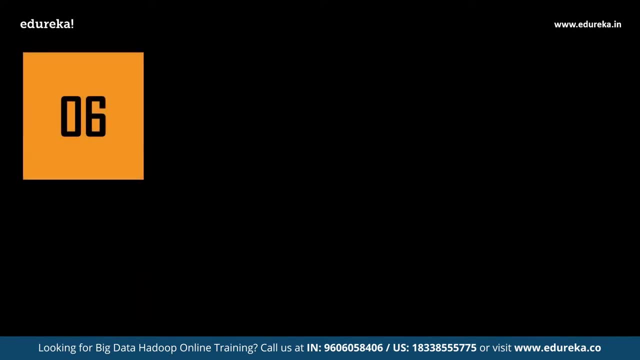 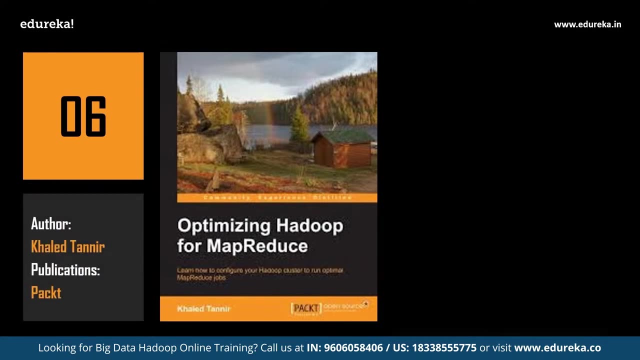 followed by pro Hadoop. We have the second book in the experience section, that is, optimizing Hadoop for MapReduce. This particular book was written by Khalid Taner and the publisher is packed publishing. Let's have an overview of this particular book. 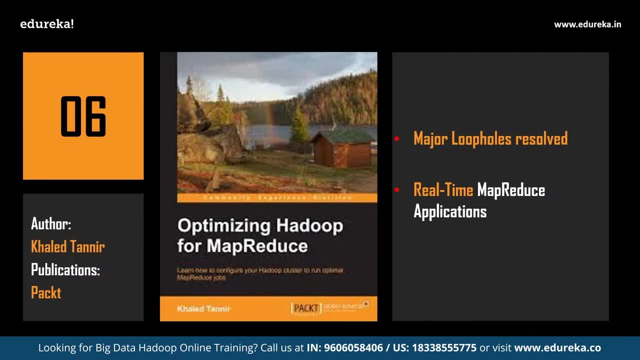 This book is all about solving the major loopholes in real-time applications of Hadoop and MapReduce. This book majorly concentrates on the optimization process of MapReduce jobs. This book basically starts from introduction of MapReduce and then it takes off to the real-time applications. 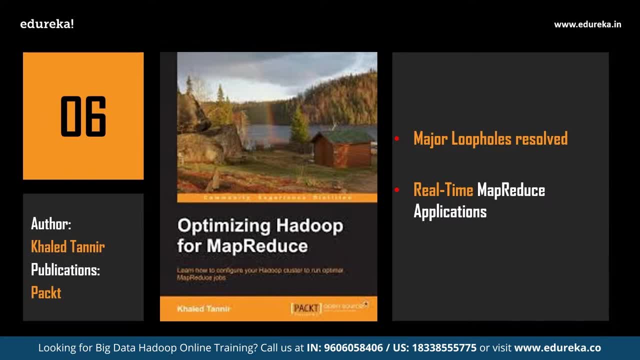 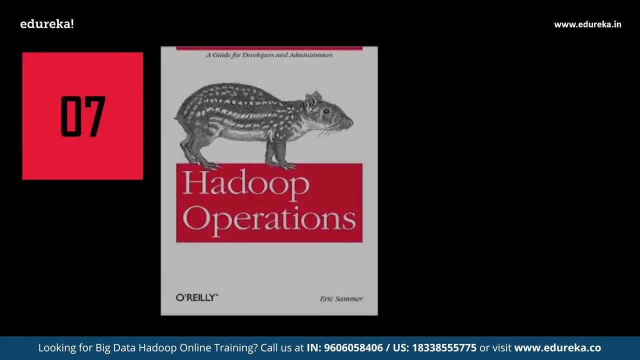 of MapReduce and gives us an in-depth understanding of MapReduce so that we could tune the code to maximum performance, followed by optimizing Hadoop. for MapReduce We have Hadoop operations. This particular book was written by Eric summers and it was published by O'Reilly media. 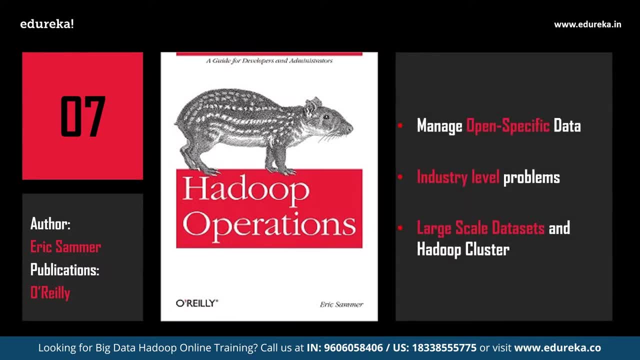 Let's have a quick overview of this particular book. The necessity for managing operation specific data has grown exponentially and Hadoop has become the standard solution for all the big data problems. processing these large scale Industrial level problems require a whole new, different level of approach and Hadoop cluster configuration. 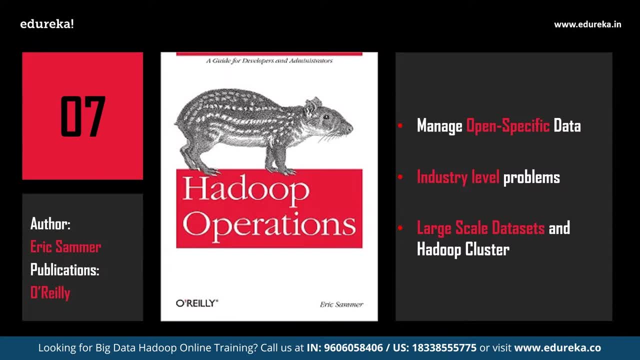 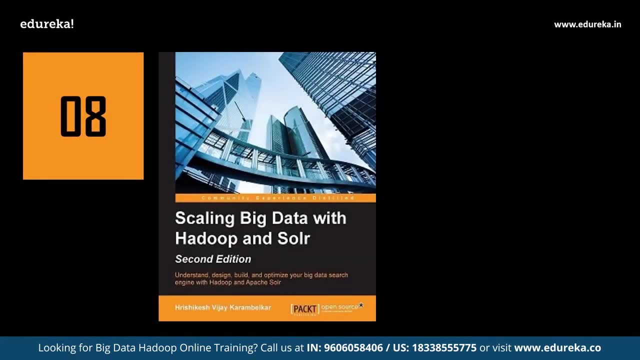 This book exactly explains the same and gives you a brief on managing large scale data sets and Hadoop clusters. So, followed by Hadoop operations, We have scaling big data with Hadoop solar. This particular book was written by Mr Rishi case and it was published by packed publishing. 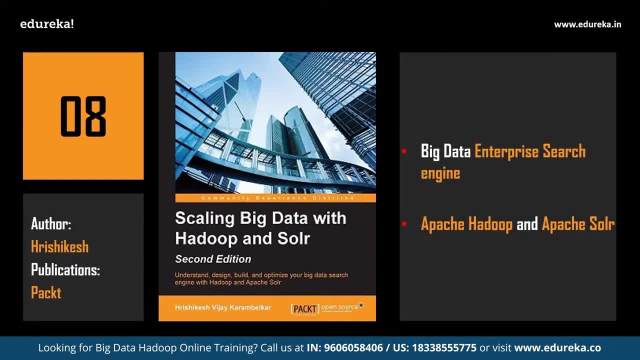 Let's have a quick overview of this particular book. This particular book is all about big data, Enterprise search engine and, with the help of Apache Hadoop and Apache solar. together, Apache Hadoop and Apache solar have come up with an approach to help organizations to deal with their big data and resolve the problem. 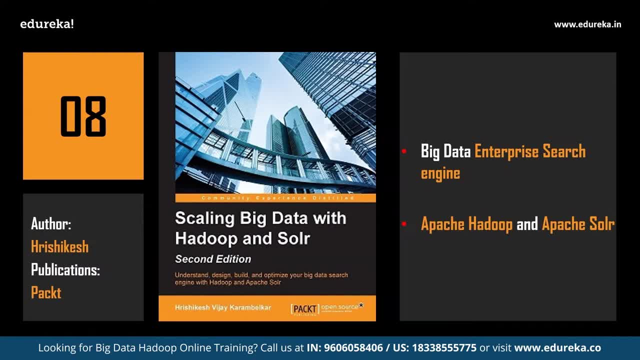 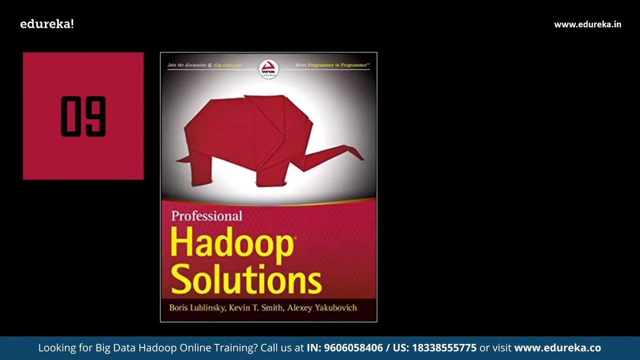 of information extraction through an amazing solution, and it has extraordinary face it search capabilities. This book gives a complete briefing about the scene, followed by scaling big data. with Hadoop solar, We have professional Hadoop solutions. This particular book was written by three authors. 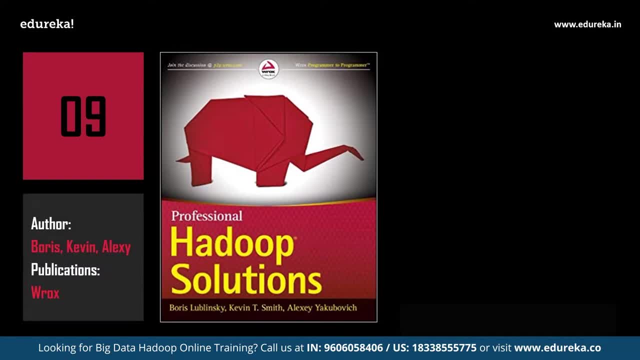 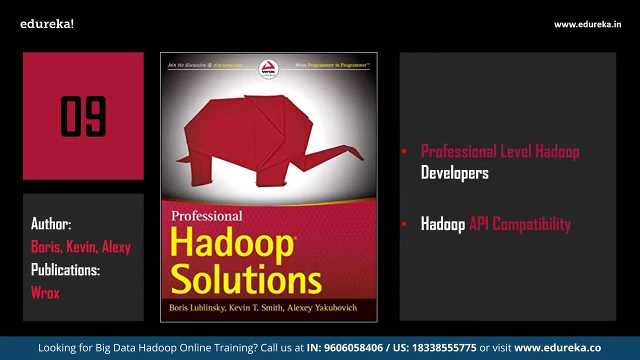 They are Boris, Kevin and Alexi, and it was published by rocks publications. Let's have a quick overview about this book to. this book is for advanced and professional level Hadoop developers. This book deals with one concept: to increase the power and maximize the capability of Hadoop. 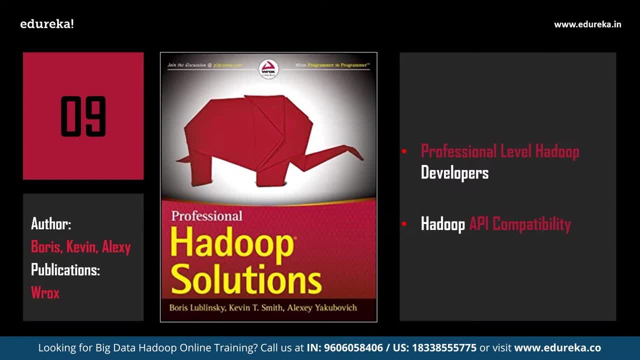 The crucial responsibility of Hadoop developers and Hadoop architects is to understand the compatibility between Hadoop frameworks and Hadoop APIs and how to integrate them to provide optimized performance and to deliver real-time solutions. Now, with this, let us move ahead into the last book. 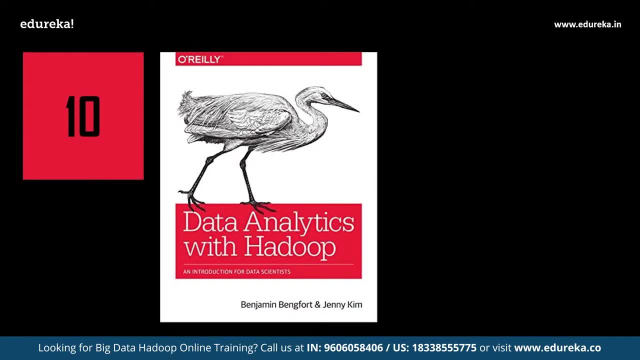 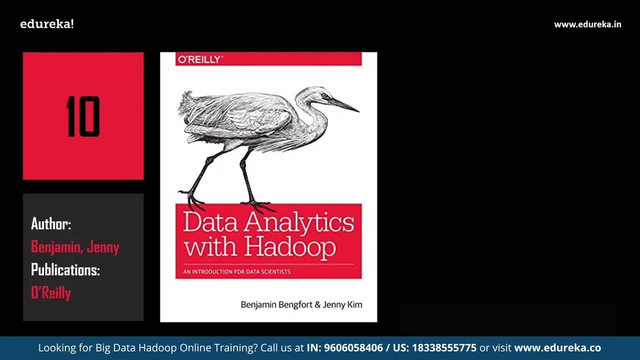 of today's session, that is, the data analytics with Hadoop. So this particular book is written by two authors. They are Benjamin and Jenny Kim. So this particular book was published by O'Reilly media and let's have a quick overview of this book. in recent days, 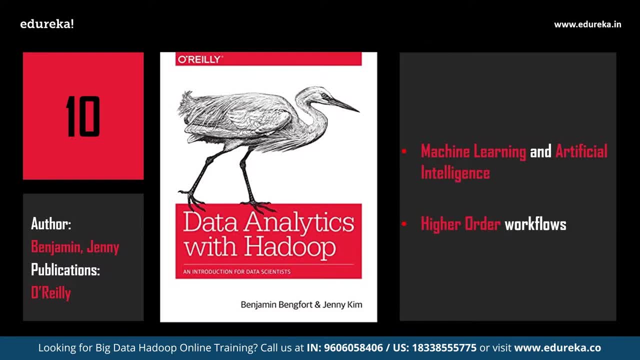 machine learning and artificial intelligence are taking over, and Hadoop is nowhere giving up the race. It is constantly trying to integrate itself with data science, and Hadoop framework has now become the standard for data analytics. This book is a perfect guide to understand data warehousing. 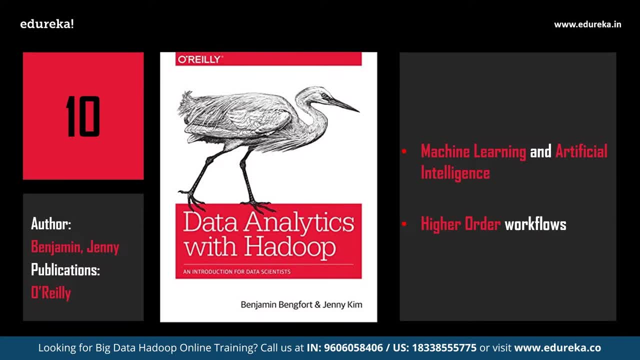 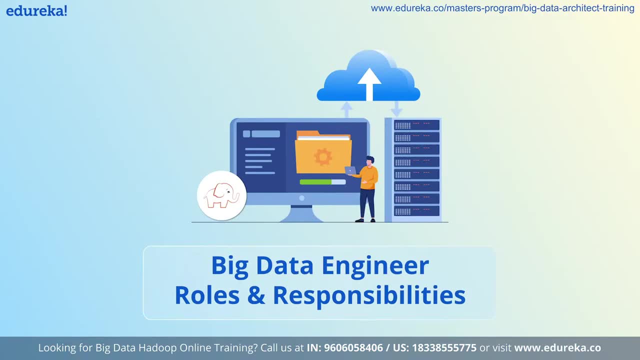 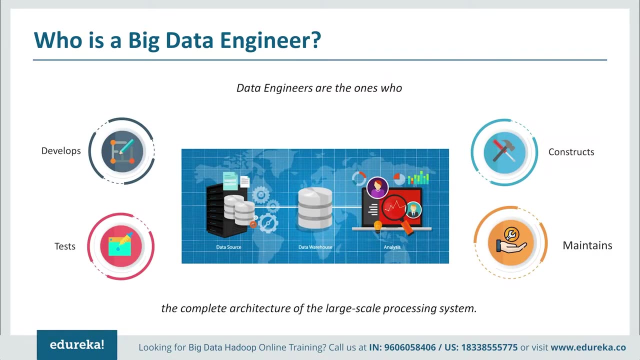 techniques and higher order workflows that Hadoop can perform in the process of data analytics. So these were the top 10 best books for learning Hadoop. Now, who is a big data engineer? a big data engineer is somebody who is responsible for collecting the data. 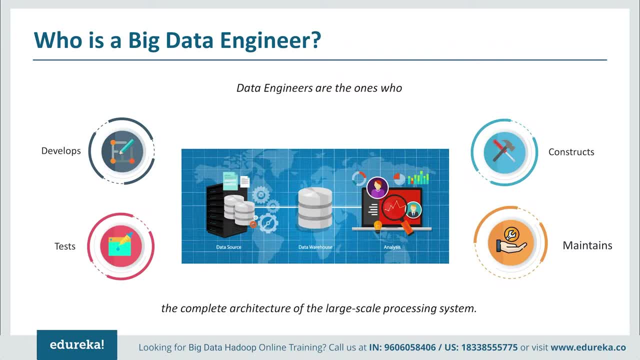 from various sources, transforming it into a usable format and storing it. They basically take raw data and convert it into something that is optimum for stakeholders that access the data. It makes it easier to process and derive business insights from. stakeholders can be data analyst, data scientists. 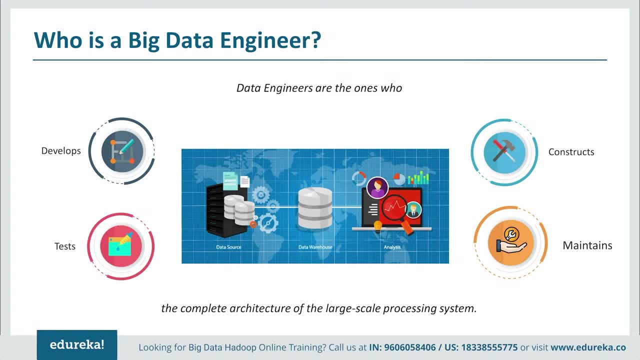 and software developers. in simple words, data engineers transform data into a format which can be easily analyzed. in order to collect and store data, These professionals design, build, test and maintain complete infrastructure. The system provides a foundation for each and every data driven activity and action that is performed in the organization. 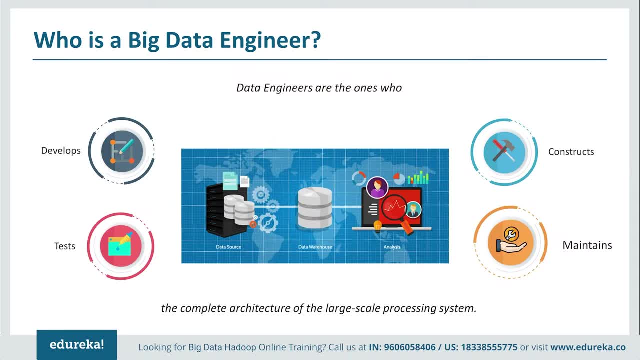 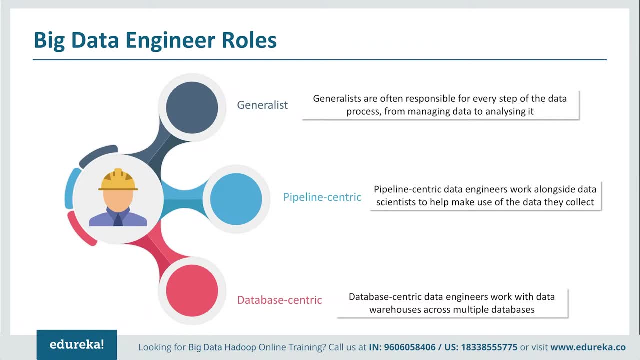 and while doing so, big data engineers always keep the business requirements in mind. Now let's look at the big data engineers roles. Now that typically three kinds of roles that a big data engineer has to assume. First of all, we have the generalist. now, generalists are typically 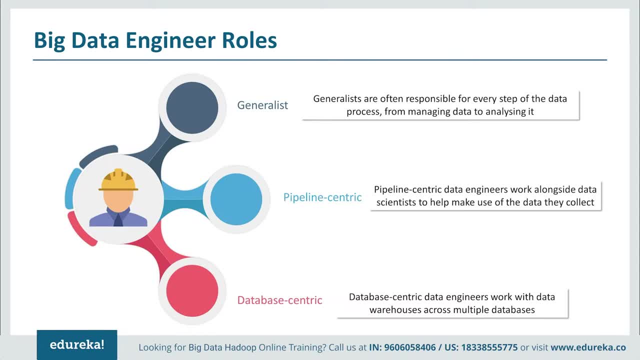 found on small teams or in small companies in this setting data engineers. These engineers wear many hats as of one of the few data focused people in a company. generalists are often responsible for each step of the data process, from managing data to analyze it. Next, we have pipeline centric data engineers, often found in 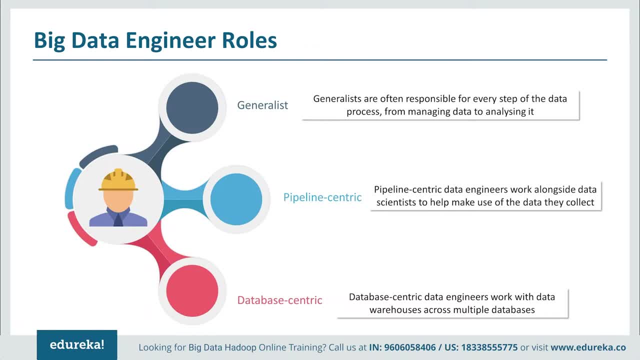 mid-sized companies. These engineers work alongside data scientists to help make use of data that they collect. pipeline centric data engineers need in-depth knowledge of distributed systems and computer science. And finally, we have the database centric profile in larger organizations, where managing the flow of data is a full-time job. 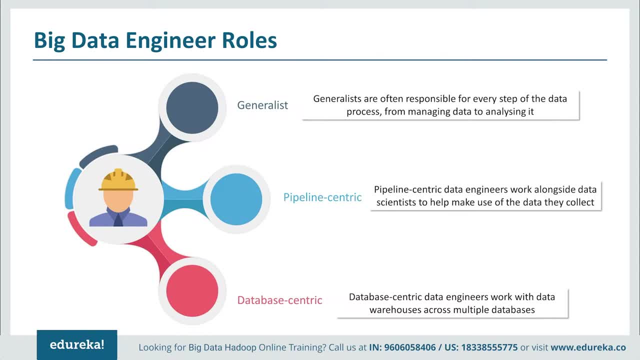 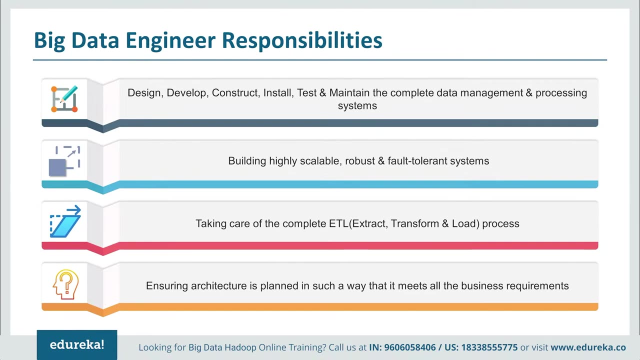 data engineers focus on analytics databases. database centric data engineers work with data warehouses across multiple databases and are responsible for developing table schemas. Now the next logical question will obviously be: what does a big data engineer do? now? big data engineer plays a big role in any 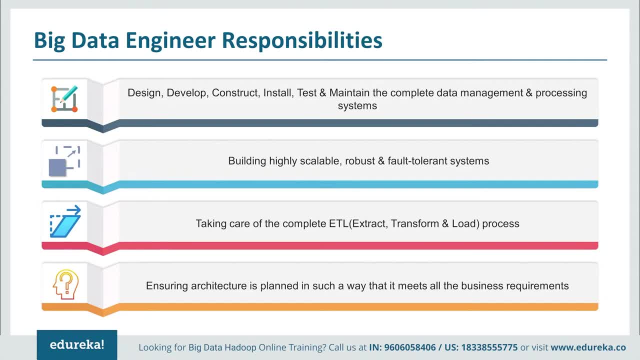 data-driven business, which also means They are responsible for many things, but most importantly, they are responsible for designing, creating, testing and maintaining the complete infrastructure, and for storing and processing data that is gathered from various sources. in order to perform this activity, data engineers need to have a good grasp of fundamental 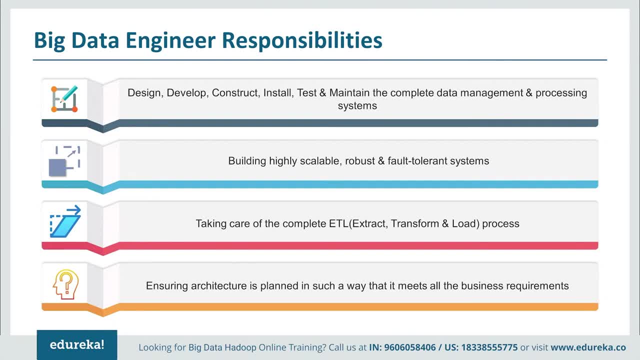 knowledge, such as OS programming knowledge and database management system. Apart from this, the professional has to be an expert in SQL development, Further providing support to data and analytics in database design, data flow and analysis activities. The position of the database engineer also plays a key role in 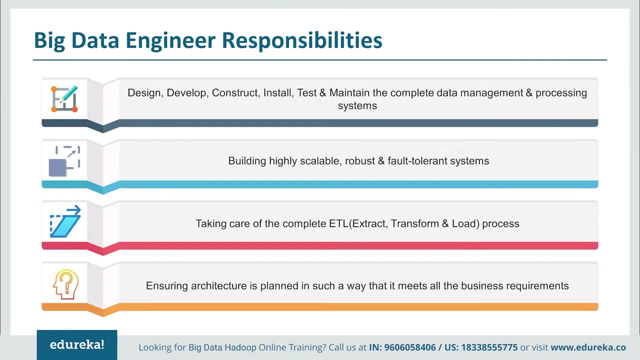 development and deployment of innovative big data platforms and for advanced analytics and data processing. The next thing I want to talk about is building highly scalable, robust and fault-tolerant systems. Now imagine a building. We all know that the deeper it is under the ground, the higher the 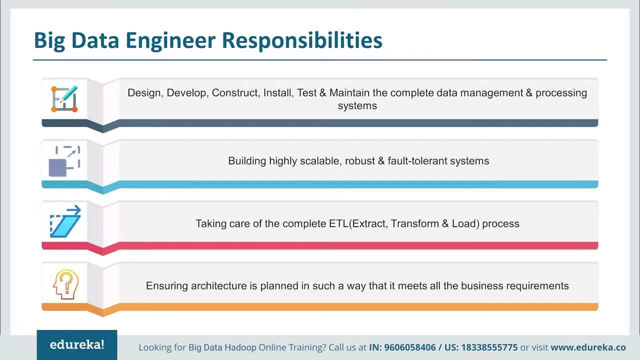 building can be constructed without collapsing. now a big data engineer does something pretty similar with data. Now these data engineers work closely with big data architects in designing a complete architecture. Both of them make sure that the system must be scalable, in terms of either adding new data sources or in handling exponentially. 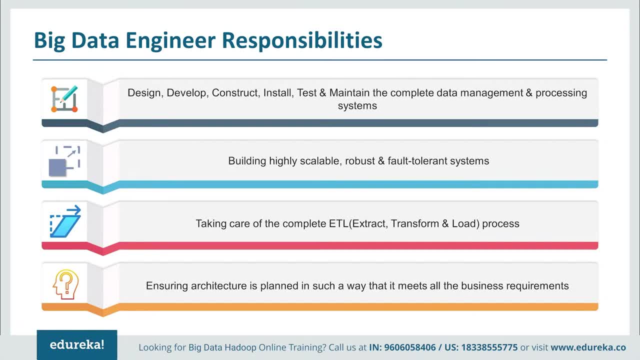 growing huge amounts of data. big data engineers should also have the capability to architect highly scalable distributed data systems using different open-source tools. designing consideration should incorporate that the system must be robust and fault-tolerant, where each component should provide a level of fault tolerance. 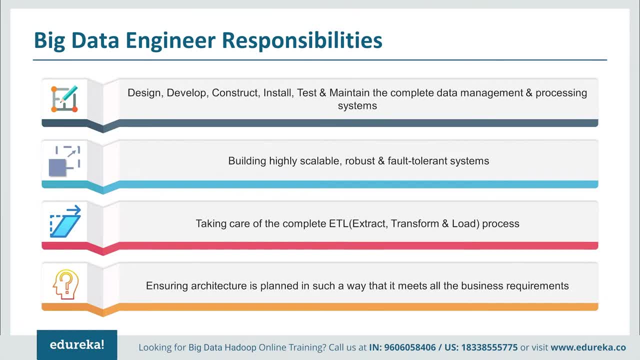 They are also involved in the design of big data solutions because of the experience they have with Hadoop based technologies such as MapReduce, Hive, MongoDB or Cassandra. a big data engineer builds large-scale data processing systems and is an expert on data warehousing solutions and should be able to work with the latest. 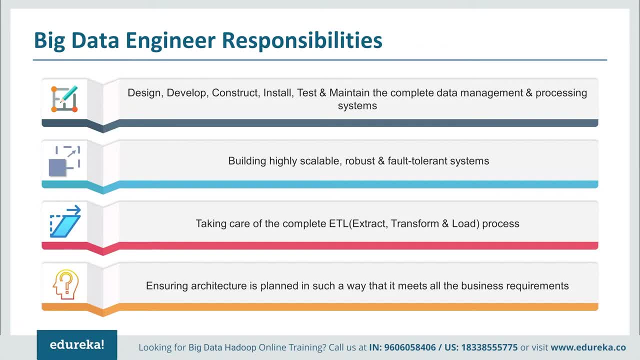 no sequel. database technologies. next, Let's talk about the biggest process in all these responsibilities, which is the ETL, or the extract, transform and load process. mundane as it sounds, This is actually the process which might take the most amount of time in order to store data in such a format that data analysts 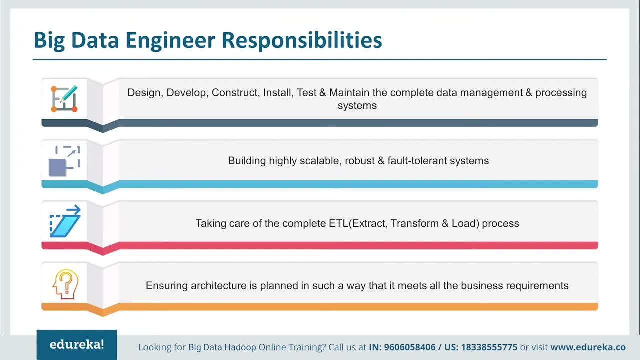 and data scientists can analyze and derive meaningful insights from it. The raw data collected from various sources need to be transformed. data engineers need to have the knowledge of programming language and tools to perform ETL. the ETL process becomes much more complex when big data comes into picture with the advent of huge amounts. 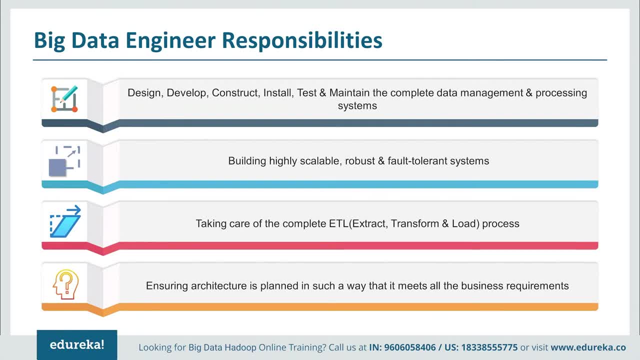 of data which is getting generated at a very high rate, It becomes even more tough to perform ETL. a big data engineer should be somebody who does this with utmost proficiency. Next is the business acumen aspect. Now, data engineers should have a good business acumen so that 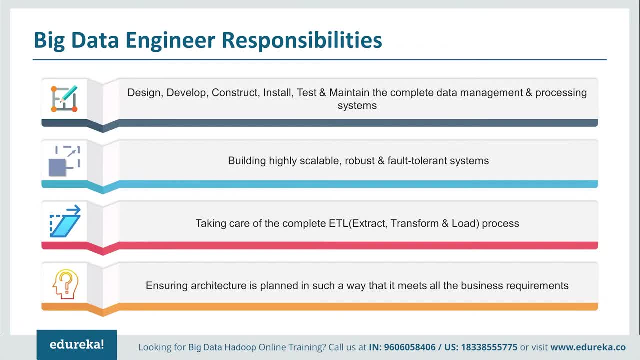 the system that he or she develops or the data that is transformed and stored should be according to business needs. This reduces the cost of deriving insights from data, and a good data engineer performs half the transformation that is required for data analytics. larger organizations often have multiple data. 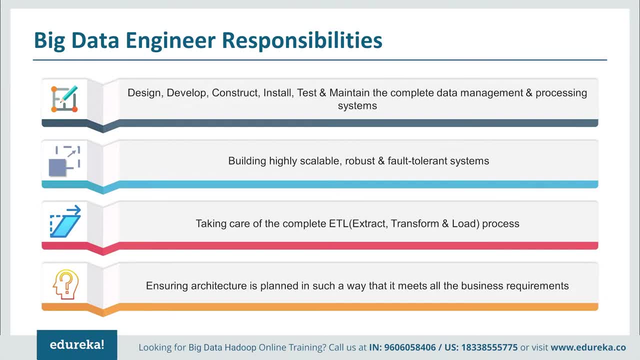 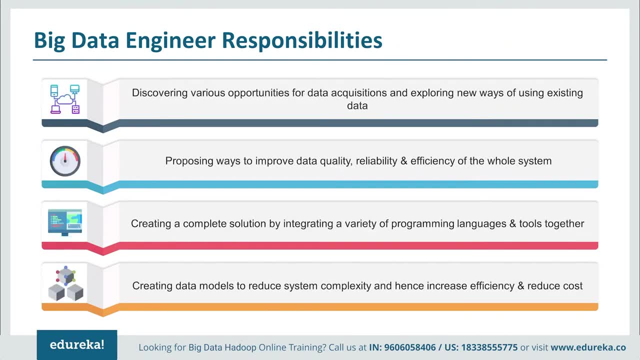 analysts or scientists to help understand data, while smaller companies might rely on a data engineer to do so. Next is data acquisition. Now, data engineer should always look at the bigger picture. He or she must have the idea about gaining data from various sources and how the data helps in gaining insights. 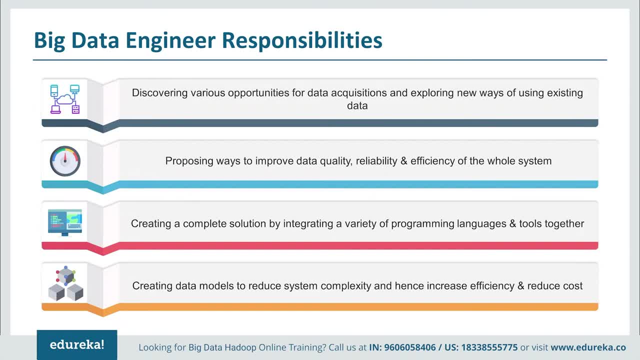 This will help him or her to understand how data is acquired from different sources and can be used in different ways to derive insights from. they can also try finding more data sources that can help getting more accurate predictions And better insights. Next, Let's talk about the programming languages and tools that a data 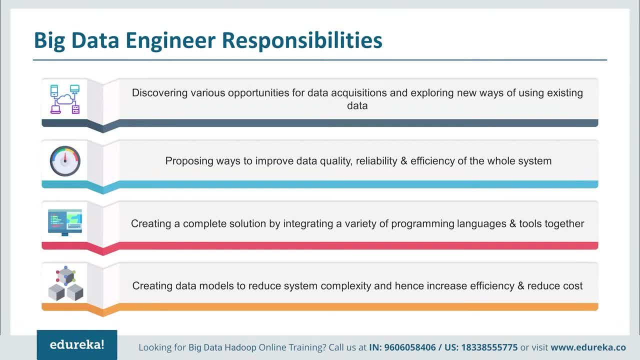 engineer should be proficient in. some of the responsibilities of a data engineer include improving data foundational procedures, integrating new data management technologies and software into existing systems and building data collection pipelines. A big data engineer should embrace the challenge of dealing with petabytes or even exabytes of data on a daily basis. 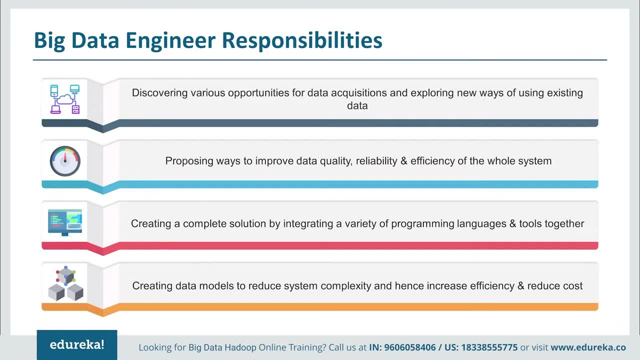 A professional, So understands how to apply technologies to solve big data problems and to develop innovative big data solutions. in order to be able to do this, The big data engineer should have extensive knowledge in different programming or scripting languages like Java, Linux, Ruby, Python or are also expert knowledge should be present regarding different no. 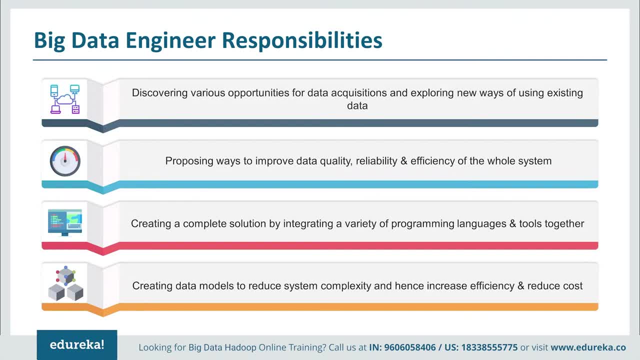 sequel or relational database management systems such as Mongo DB or Redis. building data processing systems with Hadoop and Hive using Java or Python should be common knowledge also to a big data engineer. apart from this, he or she should have a good command over at least one programming language and multiple tools, knowledge of ETL tools and data. 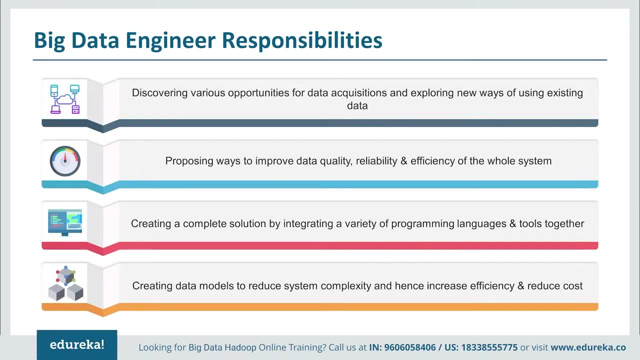 warehousing tools is also required. apart from the knowledge of individual tools, big data engineers should also know how to integrate various tools and create a complete solution based on given requirement. Now, having said all that, one very important thing Which a data engineer should be looking at is performance tuning one. 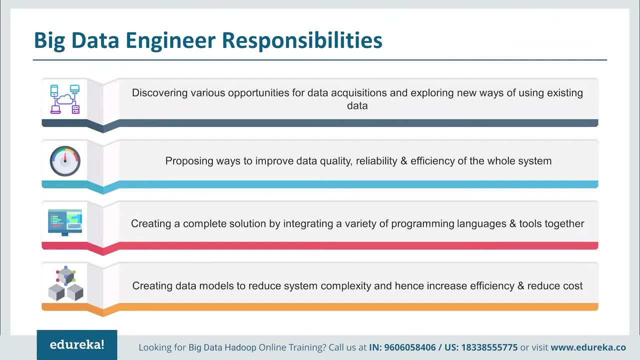 of their responsibilities includes performance tuning and making the whole system more efficient with time. first the performance of an individual component needs to be improved, and then the entire system needs to be optimized. with that, Let's move on to the summary of what we've discussed so far in terms 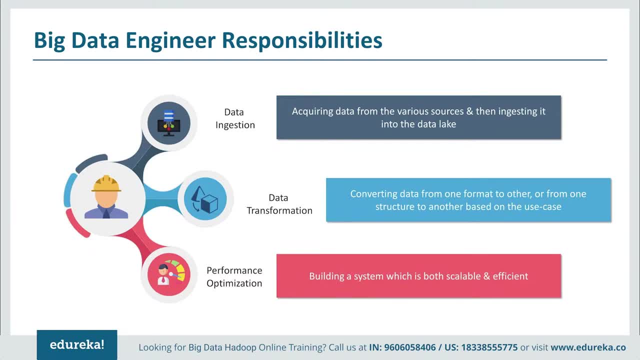 of responsibility. Now, with all that said, the basic responsibilities of a big data engineer. It goes down to these three things. first up, data ingestion. Now, this is associated with the task of getting data out of the source systems and ingesting it into a data Lake. a data engineer should need to. 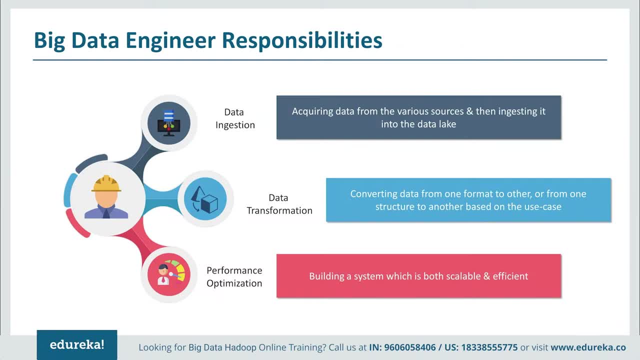 know how to efficiently extract data from a source, including multiple approaches for both batch and real time. apart from these, they would also need to know about how to deal with issues around incremental data loading, fitting within small source windows and parallelization of loading data as well. 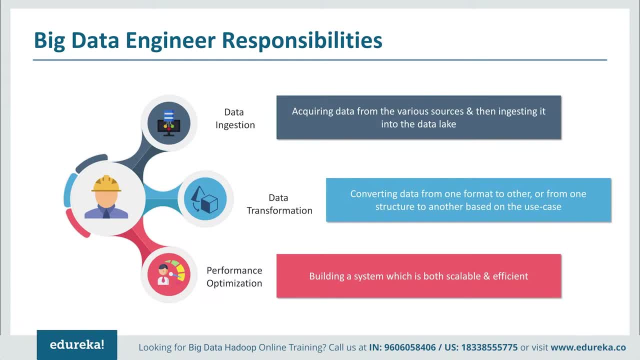 A part of it is also data synchronization, which could be considered. a subtask of data ingestion is data synchronization, but because it is such a big issue in the big data world, since Hadoop and other big data platforms do not support incremental loading of data. 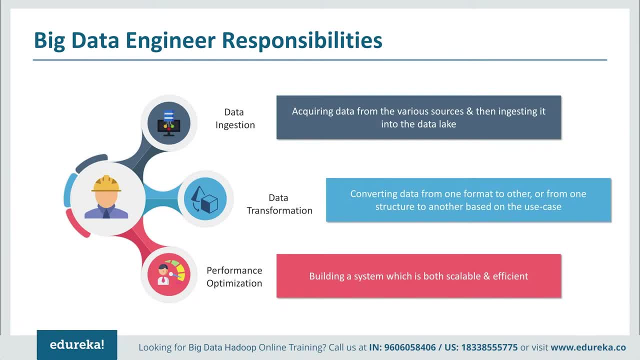 here The data engineer should need to know how to deal with changes in source data. merge and sync, change data from sources into a big data environment. Next, Let's talk about data transformation. This is the tea part in the ETL, which is extract, transform and load. 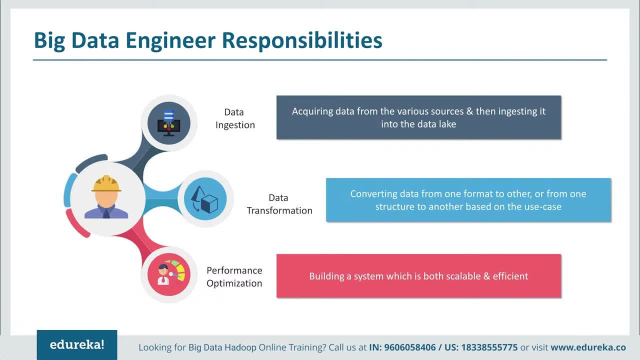 and is mostly focused on integrating and transforming data for a specific use. The major skill set here is knowledge of SQL and, as it turns out, not much has changed in terms of the type of data transformations that people are doing now, as compared to a purely relational environment. 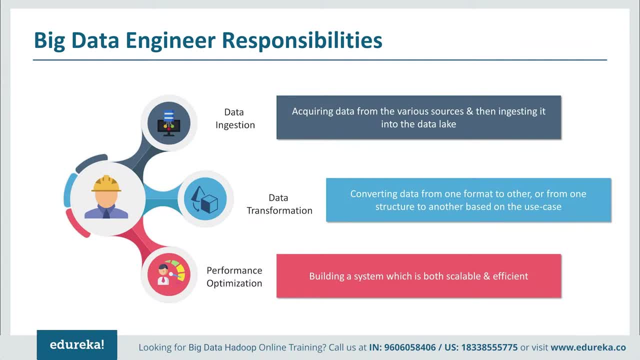 Finally, performance optimization and data models. Now, this is one of the tougher areas: How one can build a slow-performing system. The challenge is to build data pipelines that are both scalable and efficient. So the ability and understanding of how to optimize the performance. 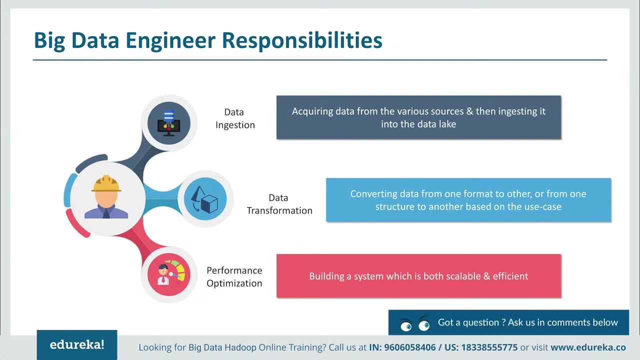 of an individual data pipeline and the overall system are at a higher level of data engineering skill. For example, big data platforms continue to be challenging with regard to query performance and have added complexity to a data engineers job in order to optimize performance of queries and the creation of data. 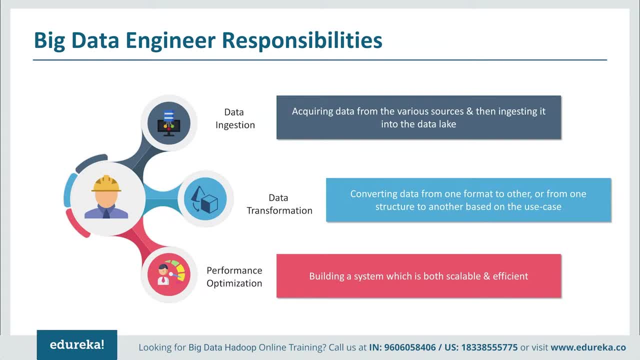 And the creation of reports and interactive dashboards. The data engineer needs to know how to denormalize, partition and index data models, or understand tools and concepts regarding in-memory models and OLAP cubes. Now that we've spoken about the responsibilities of a data engineer, 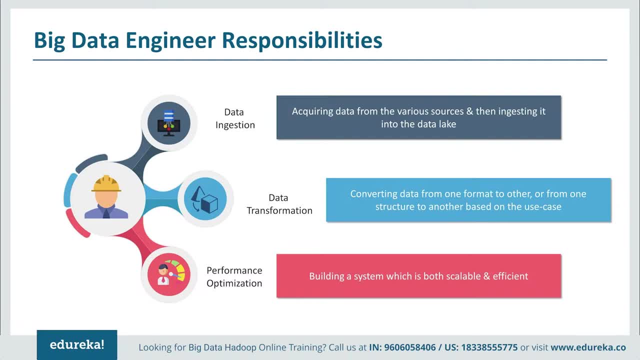 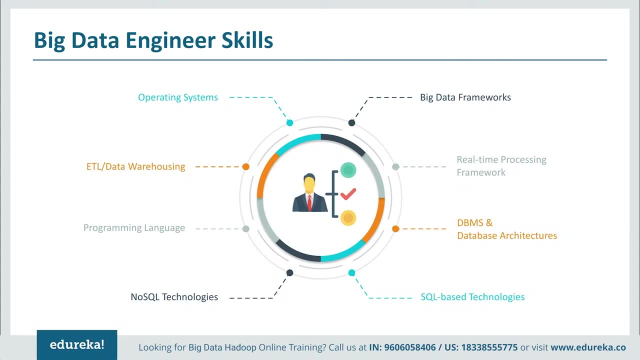 Let's talk about the skills that is required to assume these responsibilities. These are the basic skills that one should have to fulfill the responsibilities of a big data engineer. First of all, let's talk about big data frameworks, or Hadoop based technologies. Now, with the rise of big data in the early 21st century, 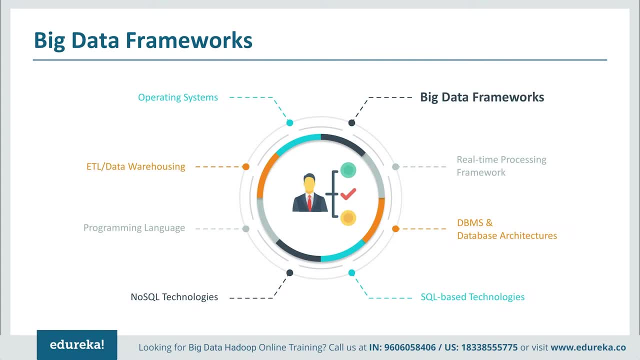 a new framework was born, and that is Hadoop. All thanks to Doug Cutting for introducing a framework which not only stores big data in a distributed manner, but also processes the data parallelly. There's several tools in the Hadoop ecosystem which caters to different. 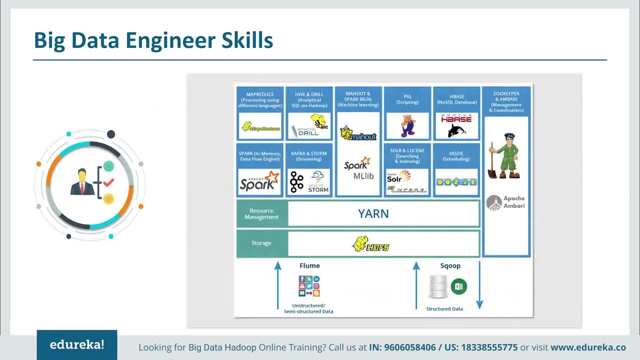 purposes and professionals belonging to different backgrounds. But some of the tools will be used to master Hadoop, But some of the tools which are must to master are HDFS or Hadoop- distributed file system which, as the name suggests, is the storage part of Hadoop. 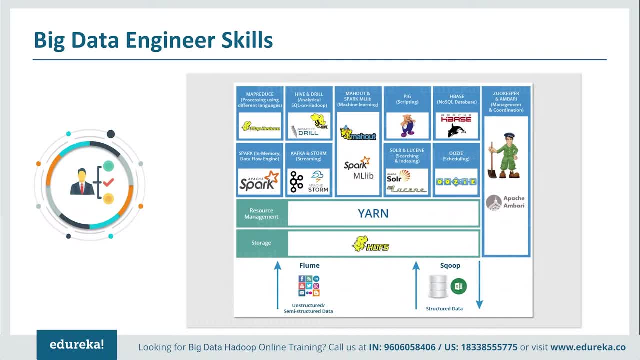 which stores data in a distributed cluster. Being the foundation of Hadoop, knowledge of HDFS is a must to start working with this framework. Next, we have YARN, which is introduced originally in Hadoop 2.x in order to make Hadoop more flexible. 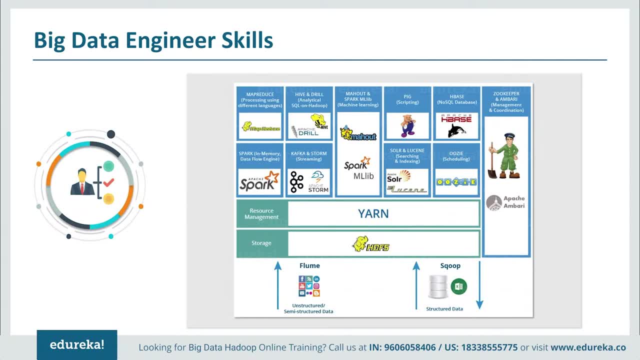 efficient and scalable. YARN performs resource management by allocating resources to the different applications and scheduling jobs. Next we have MapReduce, which is a parallel processing paradigm allowing data to be processed parallelly on top of distributed Hadoop storage. Next we have Pig and Hive. 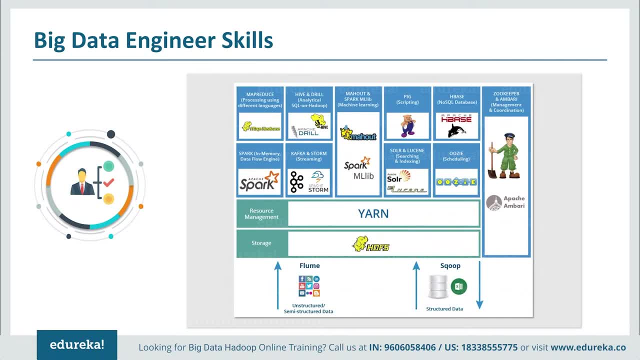 which look at the data warehousing perspective of big data to perform analytics and scripting. Next we have Flume and Scoop, which are popular tools for importing and exporting data to HDFS. Next we have ZooKeeper, which acts as a coordinator. 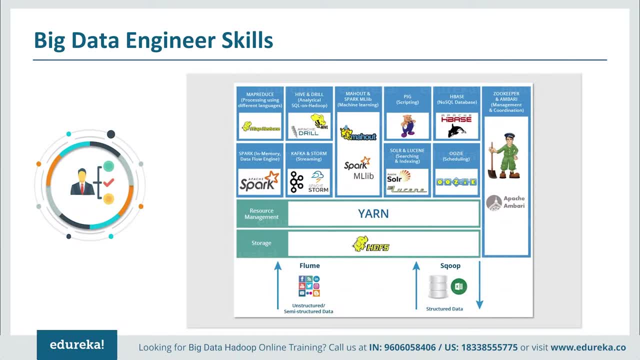 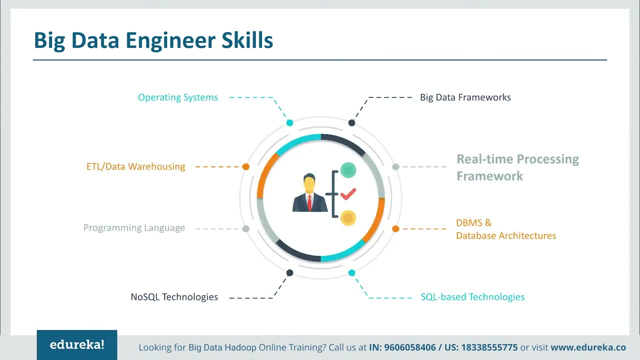 amongst the distributed services running in the Hadoop environment. It also helps in configuration management and synchronizing services. And finally, we have Uzi, which is a scheduler, binding multiple logical jobs together and helping in accomplishing a complete task. The next skill I'm going to talk about is real-time processing framework. 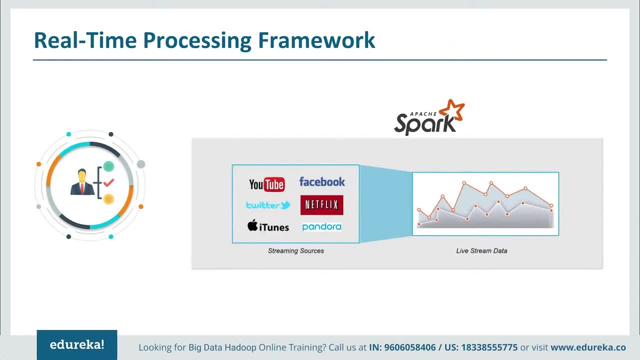 Now, real-time processing with quick actions is the need of R, Either it is to detect fraudulent transactions in a credit card system or a recommendation system. Each and every one of them needs real-time processing, and it is a very important skill for a data engineer to have. 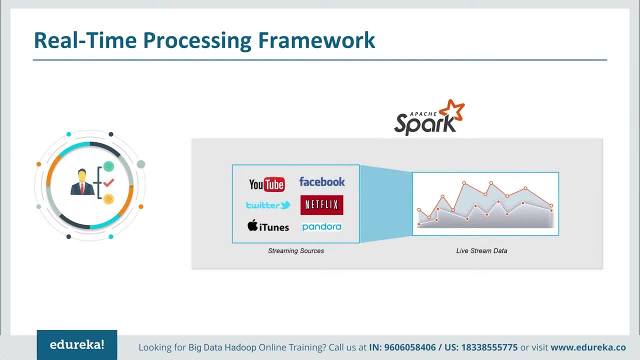 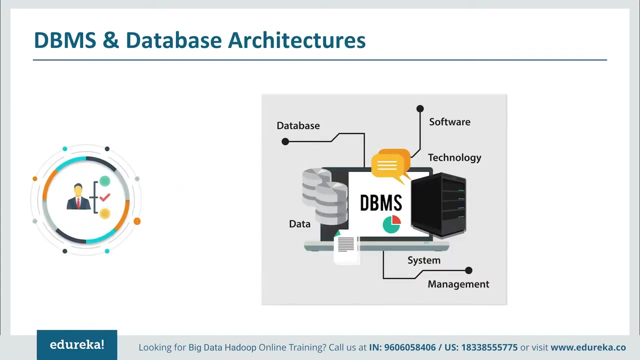 Now Apache Spark is one such distributed real-time processing framework which is used in the industry rigorously, and it can be easily integrated with Hadoop, leveraging HDFS. Next, database management systems and architecture. A database management system is something that stores, organizes and manages a large amount of information. 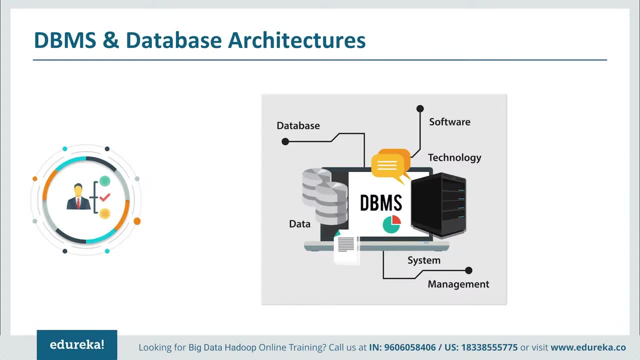 within a single software application. Data engineers need to understand DBMS to manage data efficiently and allow users to perform multiple tasks with these. This will help the data engineer in improved data sharing, data security, access integration and minimize data inconsistencies. These are fundamentals that said professional should know. 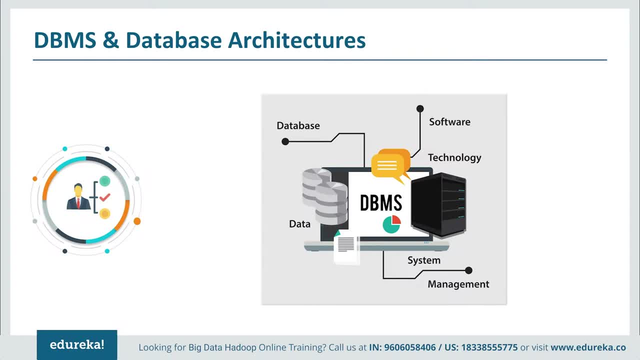 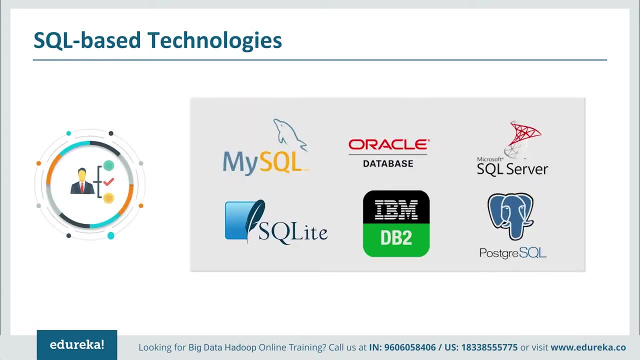 to build a scalable, robust and fault-tolerant system. Next, we have SQL based technologies. Now there are various relational databases that are used In the industry, such as Oracle DB, MySQL, Microsoft SQL Server, SQLite, etc. Now data engineers must have at least the knowledge of one such database. 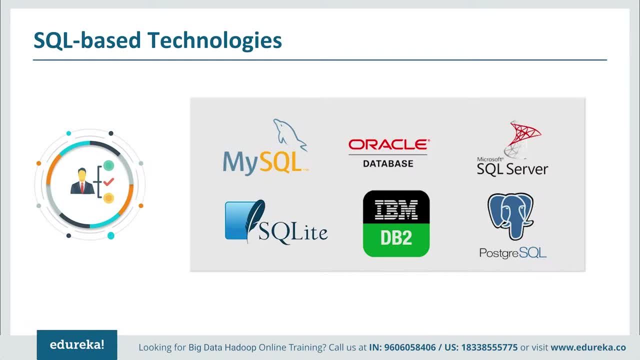 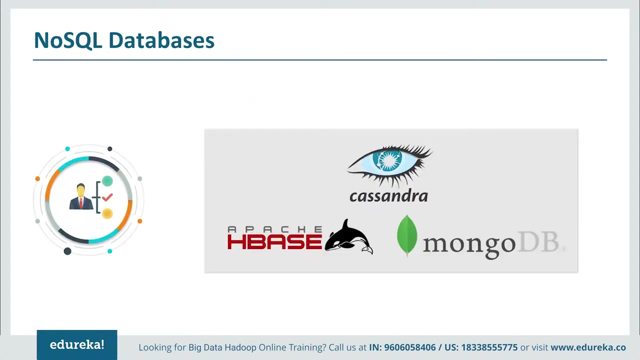 Knowledge of SQL is also a must. Structured query languages is used to structure, manipulate and manage data stored in relational basis. As data engineers work closely with relational databases, they need to have a strong command on SQL. Next we have NoSQL technologies. 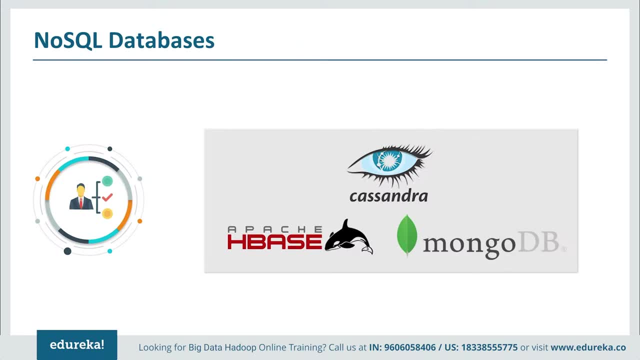 As the requirements of organizations had grown beyond structured data, NoSQL databases were introduced. It could store large volumes of structured, semi-structured and unstructured data, with quick iteration and agile structure as per application requirements. Some of the most prominently used databases are HBase. 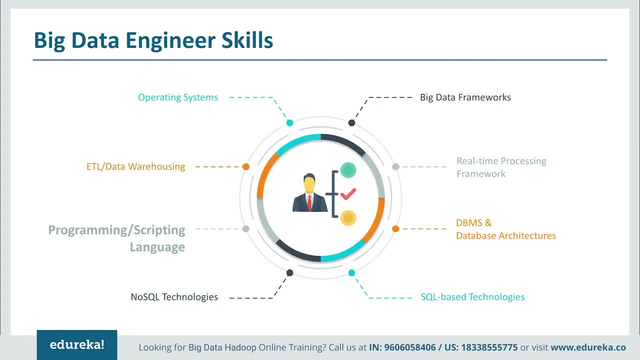 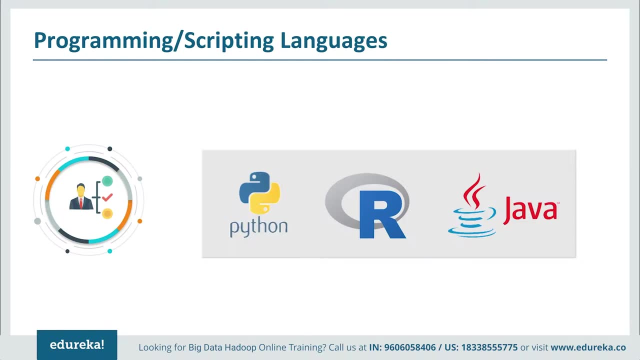 Cassandra and MongoDB. Next, we have programming languages. Now various programming languages can serve the same purpose. The knowledge of just one programming language is enough, As the flavor changes, but the logic remains the same. If you're a beginner, you can go ahead with Python, as it is easy to learn. 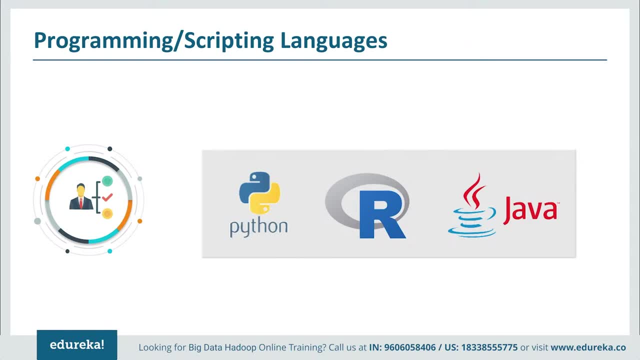 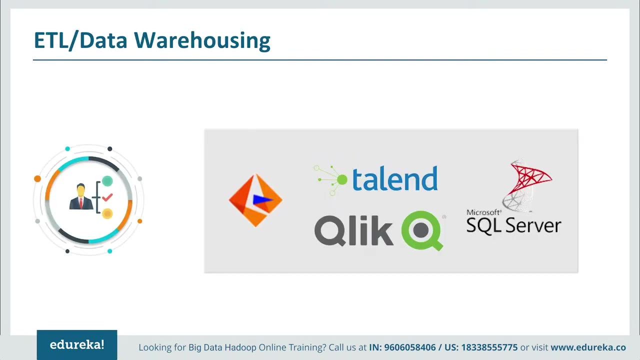 due to its easy syntax and good community support. Whereas R has a steep learning curve, which is developed by statisticians, Now R is mostly used by analysts and data scientists. Next, we have ETL, or data warehousing solutions. Data warehousing, which is very important. 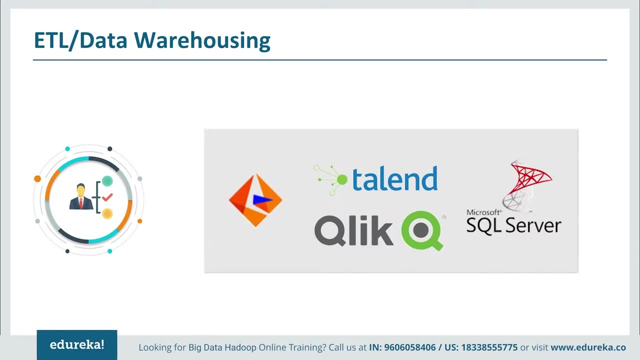 when it comes to managing a huge amount of data coming in from heterogeneous sources, where you need to apply ETL. Now, data warehouse is used for data analytics and reporting and is a very crucial part of business intelligence. It is important for a big data engineer. 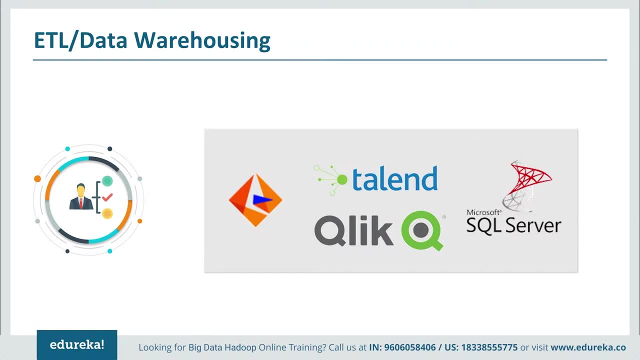 to master one data warehousing or ETL tool and after mastering one, it becomes easy to learn new tools, as the fundamentals remain the same. Informatica, ClickView and Talent are very well-known tools used in the industry. I would recommend you start with Talent. 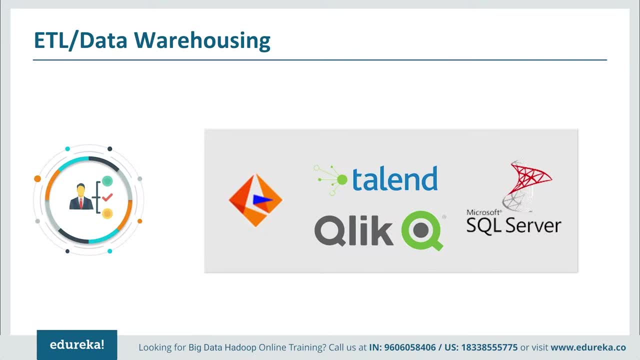 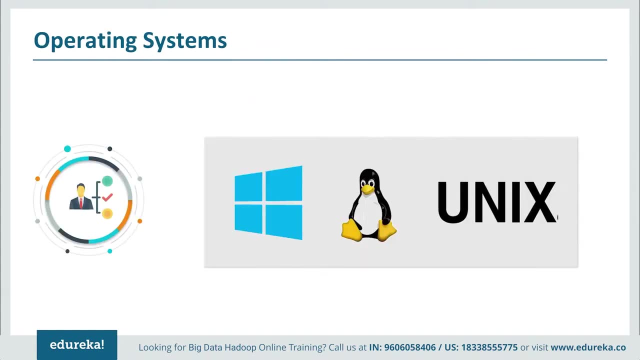 because, after this learning, any data warehousing tool will become a piece of cake for you. And finally, we have operating systems. Apart from all these skills, intimate knowledge of Unix, Linux and Solaris is very helpful, as many math tools are going to be based on these systems. 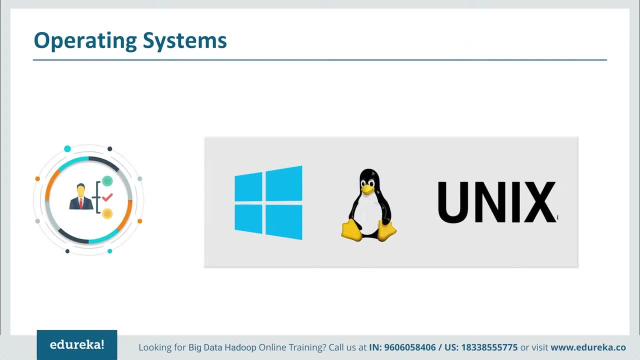 due to their unique demands for root access to hardware and OS functionality above and beyond that of Microsoft's Windows or Mac OS. That was all about the skills. We have spoken more about this segment in a previous installment to this video. You can go and look at it. 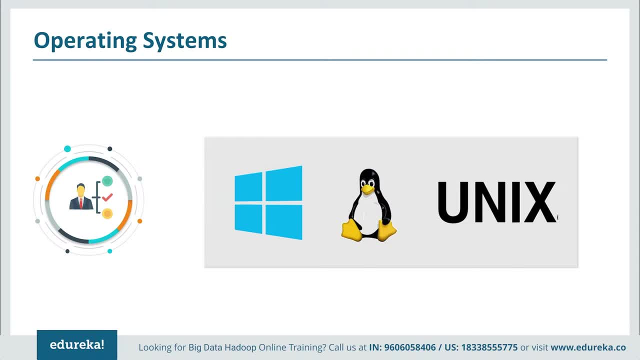 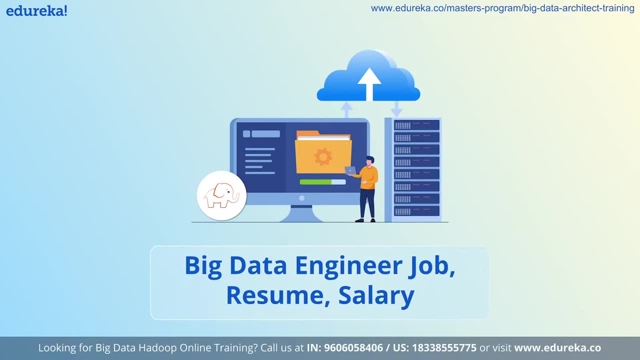 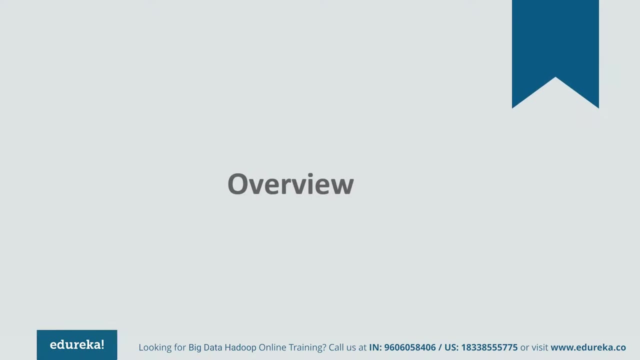 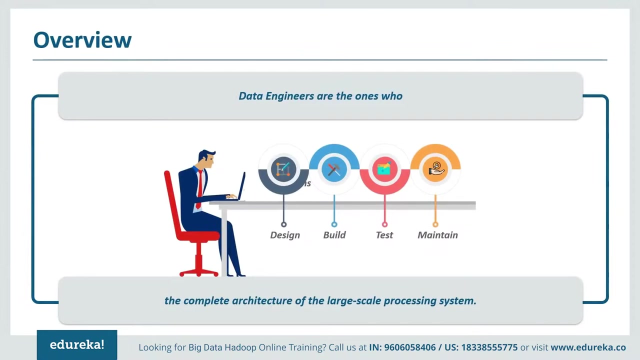 to understand the skills you will be requiring as a big data engineer in detail In this era. each and every organization is acquiring data from all possible sources, analyzing it and making thought-out data-driven decisions. Now, data engineers are the ones who design, build, test and maintain. 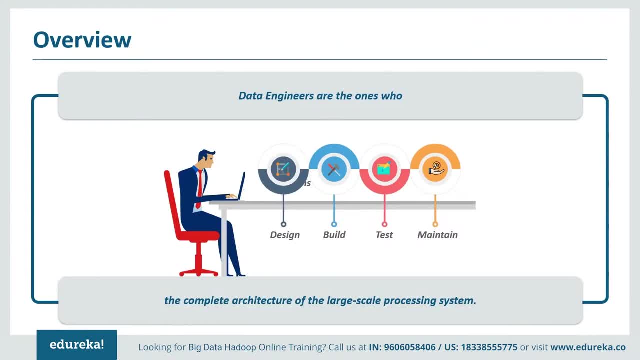 the complete architecture of this large-scale processing system. With the increasing data sources and accelerating data growth, various challenges have emerged in storing, processing and handling data, and that is called big data. Fun fact, according to an Accenture study, 79% of enterprise executives agree. 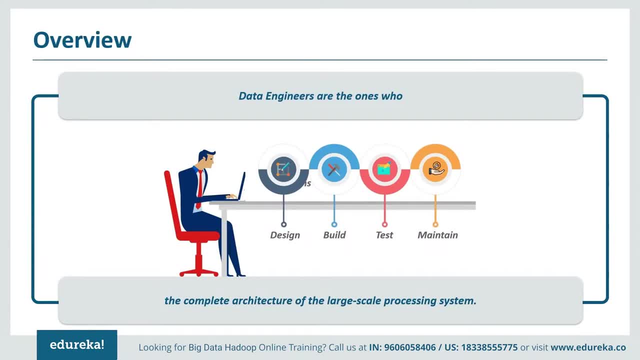 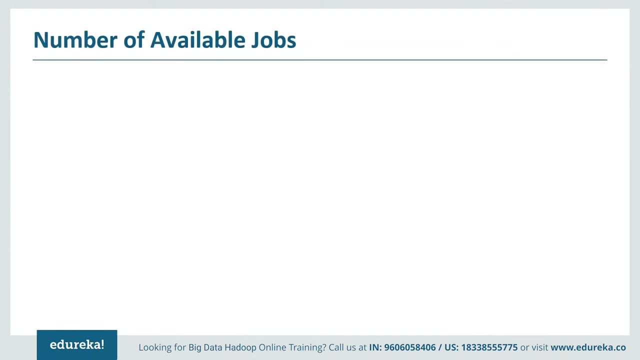 that companies that do not embrace big data will lose their competitive position and would eventually face extinction, as quoted by the Forbes magazine. Next, let's look at the market trends and projections. Now, the best way to analyze a big data engineer's job trend is by analyzing the jobs available. 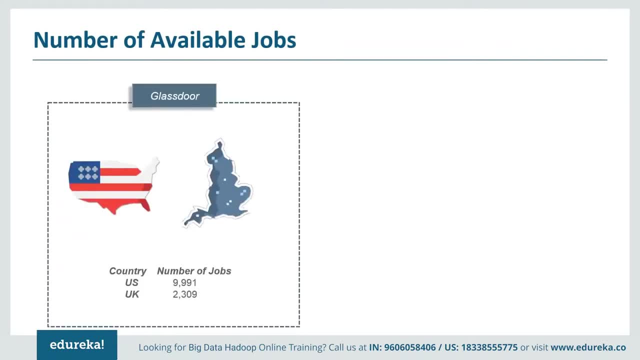 on various job portals. According to Glassdoor, the number of jobs for a big data engineer is way over 9,000, and in UK it is way more than 2,000.. But Indeed begs to differ. According to Indeed, the number of jobs for a big data engineer 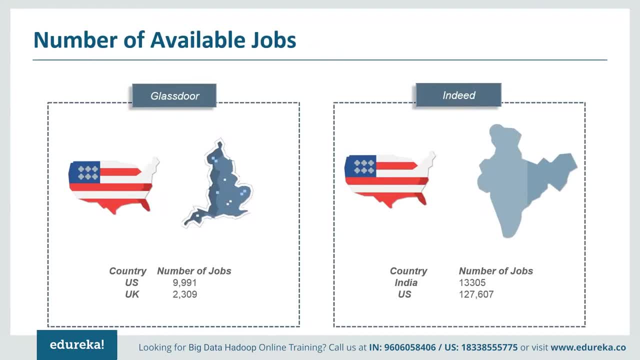 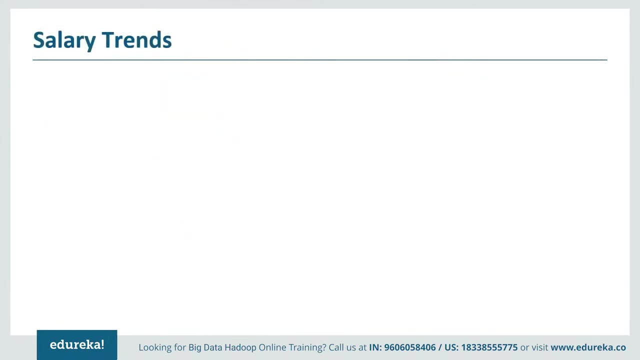 in India are way above 13,000 and in the US is way above 127,000.. In spite of considering big data as a challenge, organizations are turning it into an opportunity to find insights from the data and gain competitive advantage over the rivals. 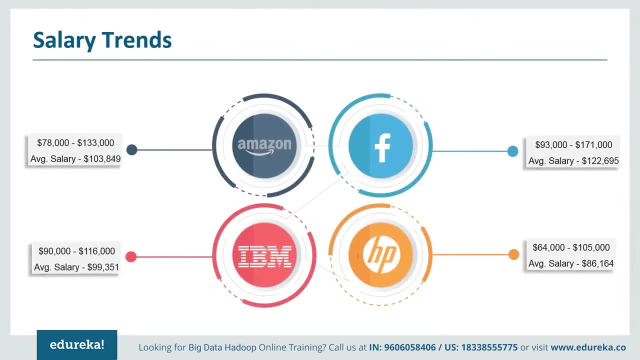 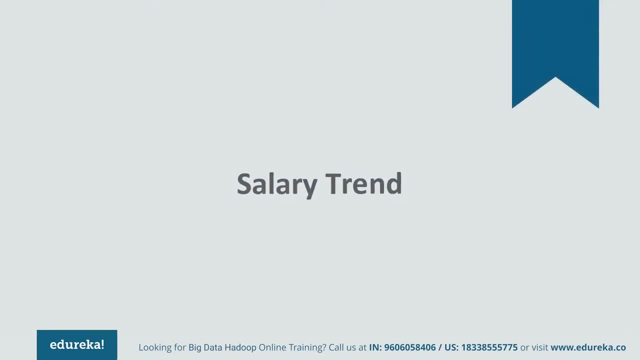 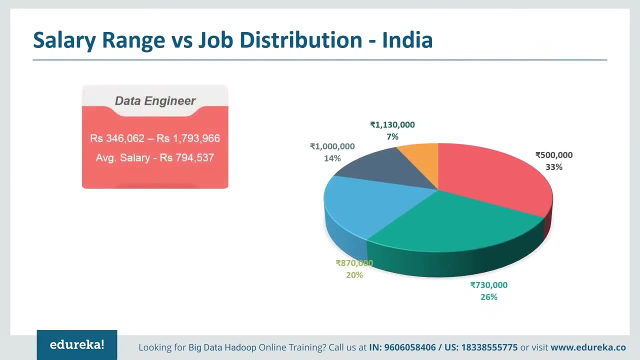 To achieve that, they hire big data engineers who are paid handsomely, no matter how fresh they are in the field. Here you can see the job distribution per salary range in India for a data engineer, As we can see people who get paid more than 5 lakhs in annum. 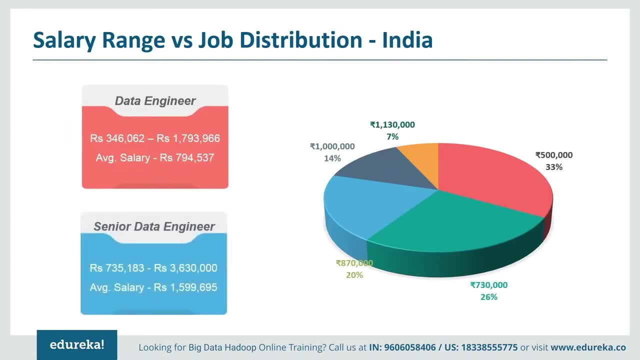 are about 33%. 730 per annum are 26%, 8,70,000, about 20%, which are very high salary brackets. Apart from that, the average salary for a data engineer is almost 8 lakhs in annum and for a senior data engineer. 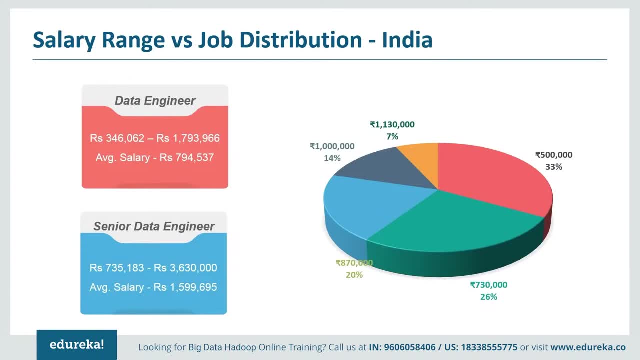 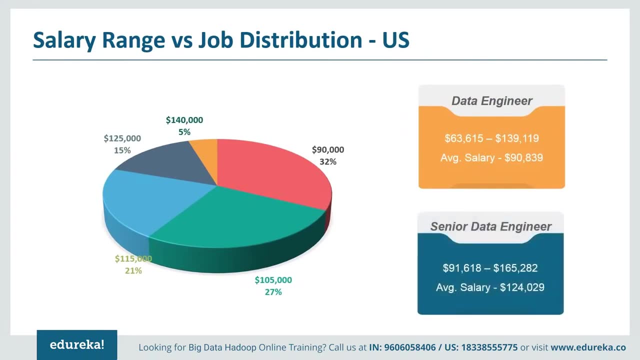 is almost 16 lakhs in annum. If we look at the same numbers in the US, there are 32% of professionals who make more than $90,000 a year and 27% professionals who make $105,000 a year. 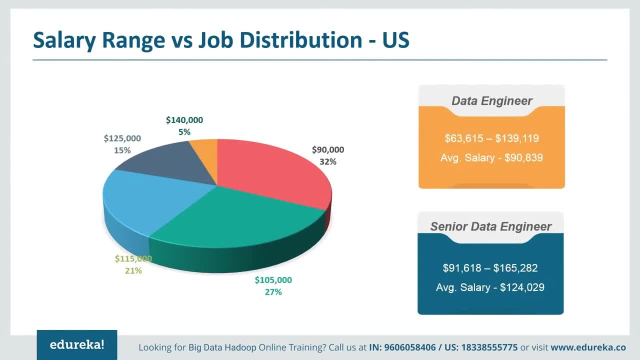 The average salary in the US for a data engineer is way more than $90,000, and for a senior data engineer it is $124,000 per annum. Now, as we have discussed the salary of a big data engineer, let's look at a few factors. 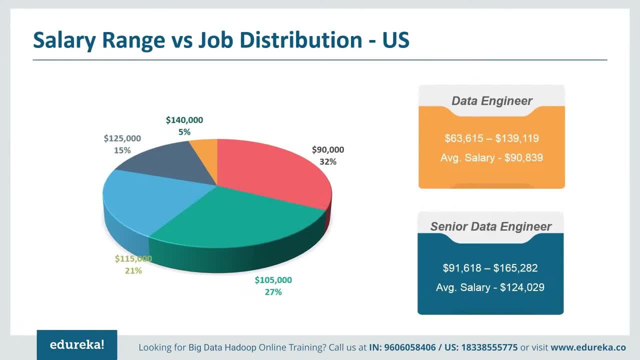 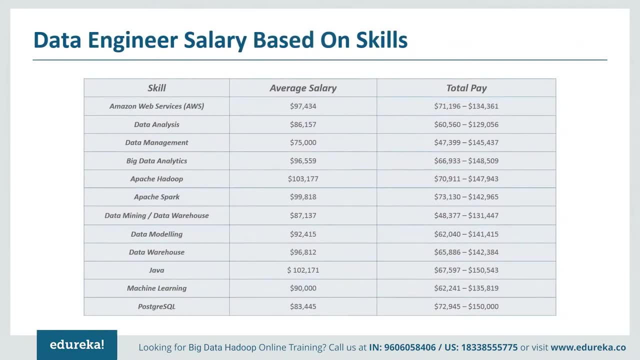 in the form of skills and technology that they know, on which their salary depends. Here we've carefully curated a table which lists out the skills and the average salary which can be encashed through them. You can see services such as AWS data analysis. 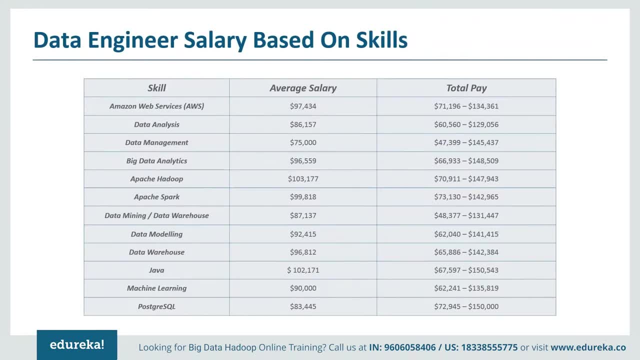 data mining, warehousing, machine learning and even programming languages like Java and R. Apart from that, you can see BI tools and statistical tools like Tableau, database architecture, ETL and structured query languages. Now, another influence on the salary is experience. 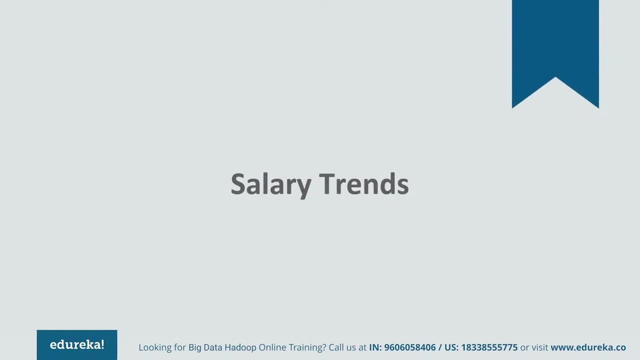 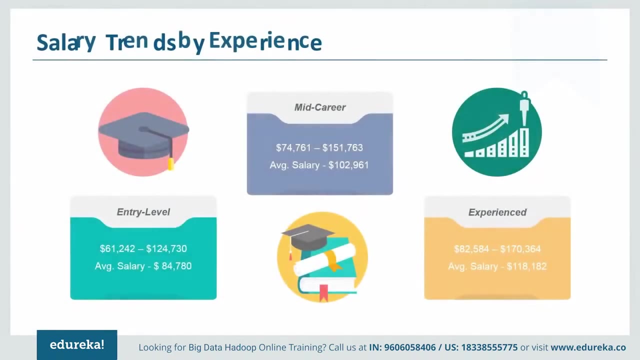 because experience is also a very important factor in deciding the big data engineer's salary. The distribution of salary is like: so: An entry-level data engineer makes about $85,000 a year. People who have 5 to 8 years of work experience. 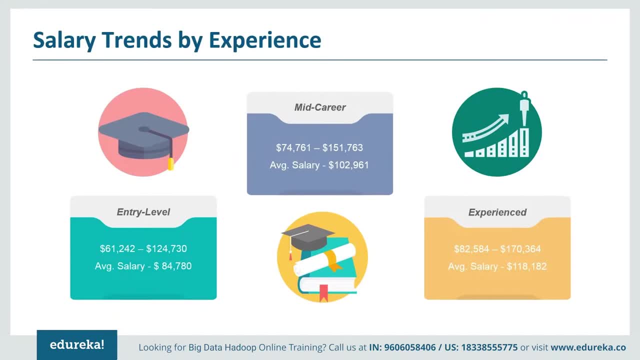 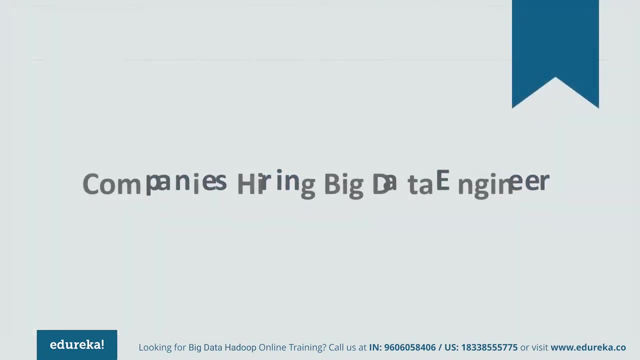 bag nearly $103,000 a year, and people who are experienced- I'm talking like 10 years of industry experience- get over $118,000 a year. Now this salary must be coming from somewhere presenting to you the companies that hire. 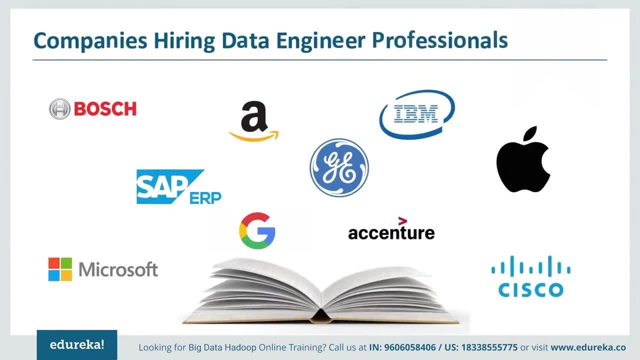 in this job role. As you can see, there are some very big names like Amazon, Google, Bosch, Microsoft and IBM who hire big data engineers. Now, companies that hire big data professionals are companies that are invested in the future And the worldwide. 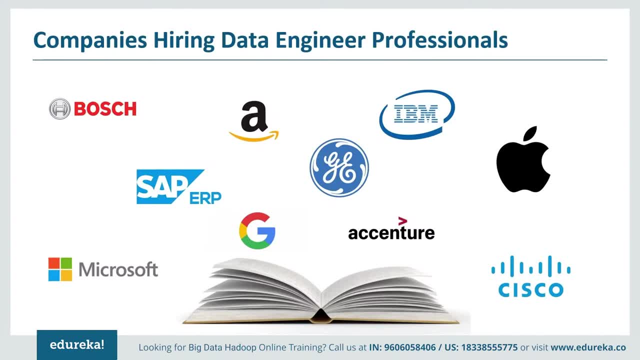 big data. market revenues for software and services are projected to increase from $42 billion in 2018 to $103 billion in 2027, attaining a compound annual growth rate of about 10.5%. That sort of a growth needs some kind of work. 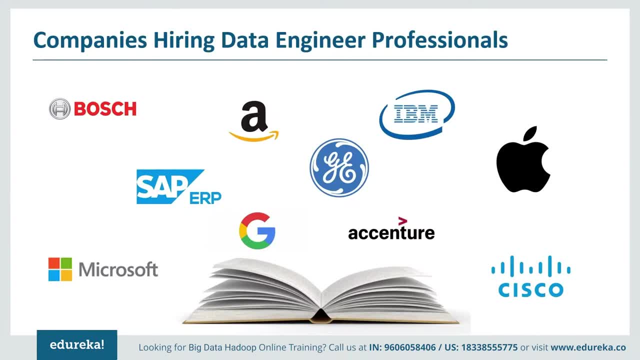 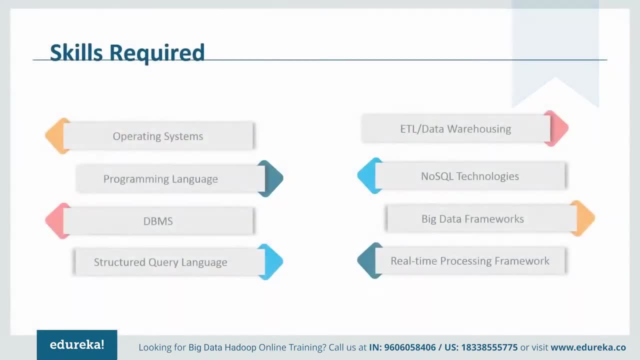 After going through multiple job descriptions, we found that the big data engineer's salary has many variables. Here are the skills that you require to be a big data engineer. A big data engineer must know his operating system, and Linux is one of the most widely used OSs in the industry. 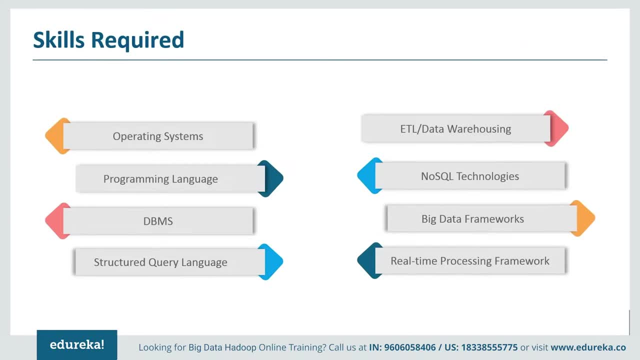 Apart from that, they must be proficient in at least one programming language, say R or Python, for instance. Database management system is also a very crucial skill required for big data. Apart from that, they must know how to work with structured query languages and NoSQL technologies. 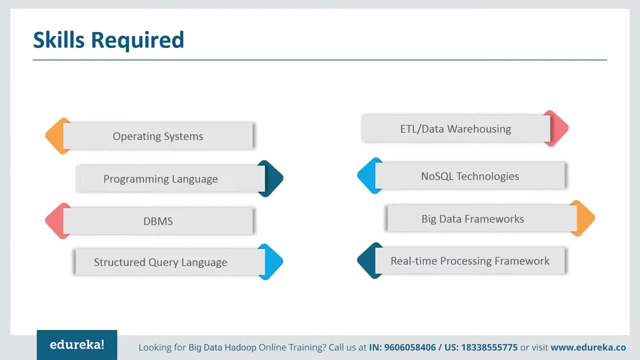 Data models and data schema are amongst the key skills that a data engineer should possess. Hence, data warehousing is something that they should be acquainted in doing. Apart from that, what is a big data engineer who does not know big data frameworks, HDFS? 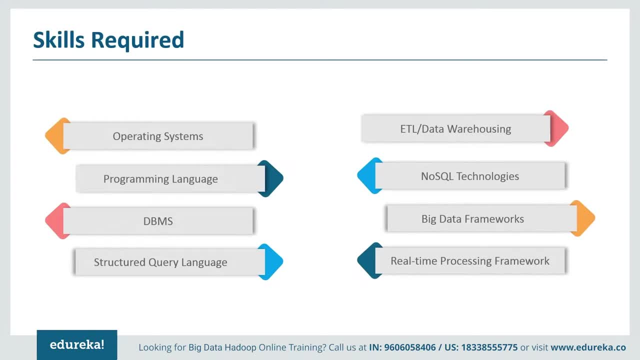 YARN, MapReduce, Pig & Hive should be on the fingertips of the big data engineer. And finally, real-time processing with quick actions is the need of the hour, Either it is a credit card fraudulent detection system or a recommender system. 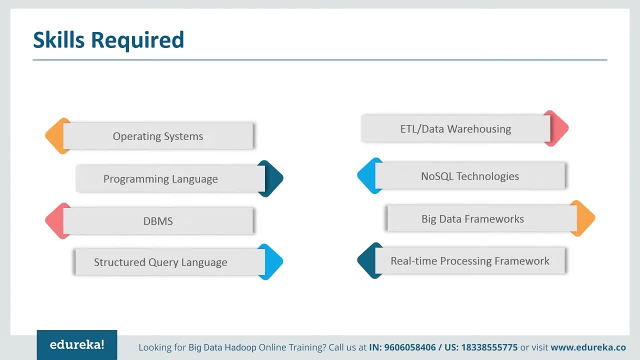 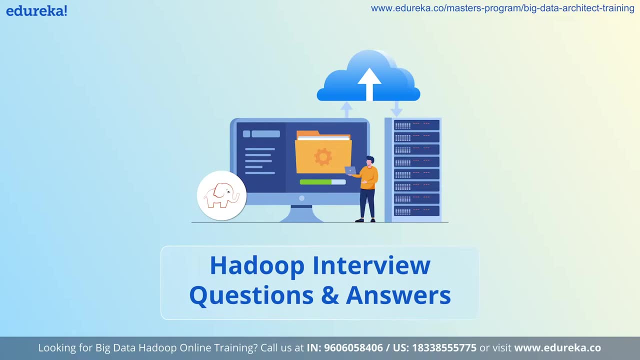 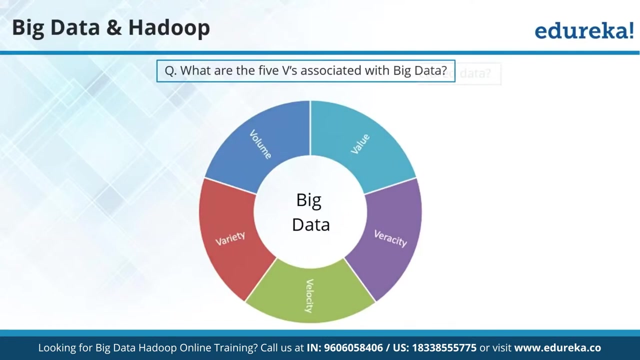 Each and every one of them needs real-time processing. It is very important for a data engineer to have this knowledge. Now, when we talk about big data, right, the very basic question a lot of times pops up: What are five B's? 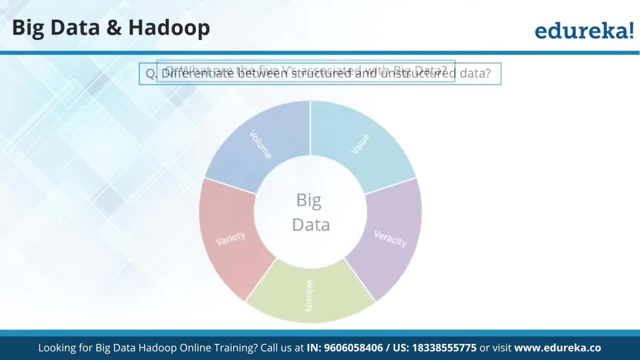 available in big data. Can anybody answer that? Okay, so Ravi wants to answer this. Okay, let me unmute Ravi. Ravi over to you First is volume. Volume and size of data: how much is growing day by day? 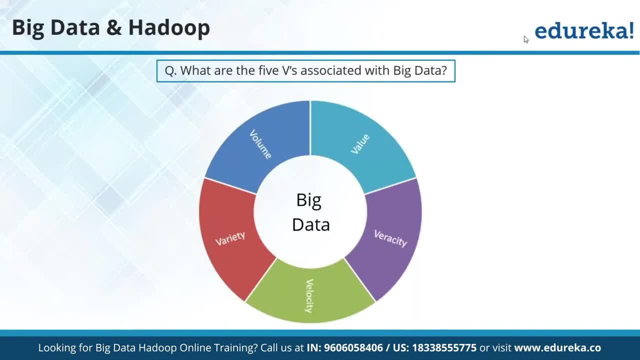 And next is variety. Variety is we have various types of data: actually structured, unstructured and semi-structured data. Structured data is nothing but relational database, all those things. Unstructured data is audio, images, files, all this data Semi-structured. 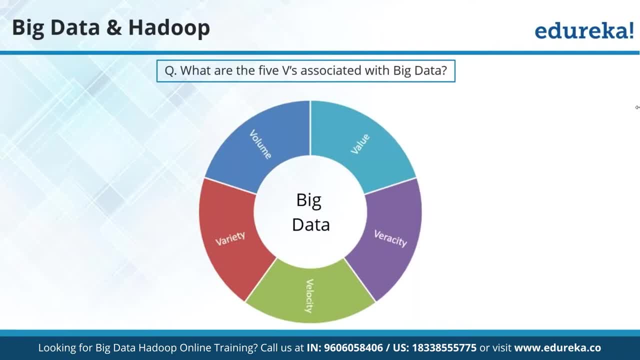 is XML file. Velocity is how much fast is growing? Okay, very, very much a good answer. When big data started, IBM gave a definition with just three B's. So three B's were volume size, volume variety, velocity. 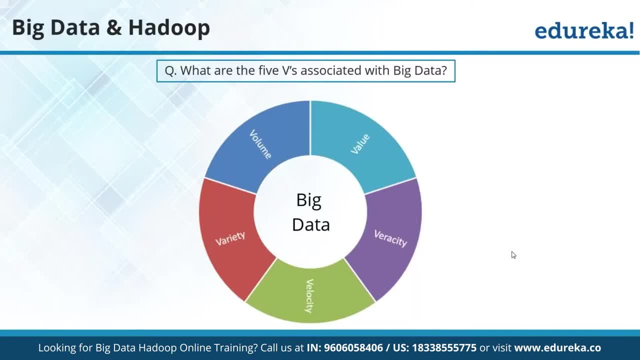 So what was in volume? Volume was, when we talk about, like, in terms of amount of data, what we are dealing with. right, For example, today's Facebook is dealing with very huge amount of data. right? When we talk about variety, now is it only Facebook? 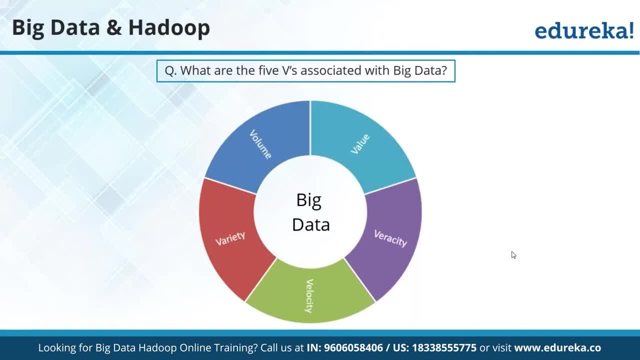 which is generating data? No, right, Even Twitter is generating data. Okay, we are talking about just social media sites? No, we can. a lot of big data is getting generated. so that's a different variety of data. We have structured data. 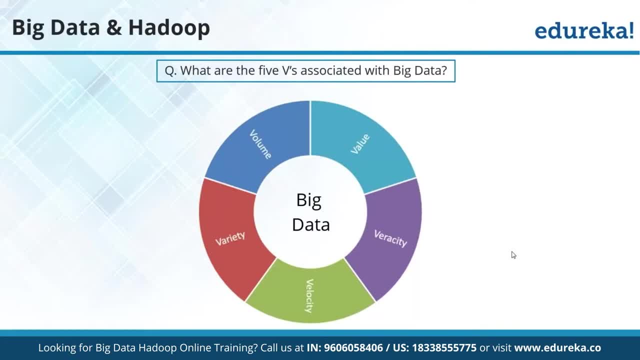 unstructured data, like we can have videos, audio, right. This is basically going to be called as a variety. Third component is velocity. Like I said to you, Facebook is just a 10 to 12 year old company and imagine the growth. 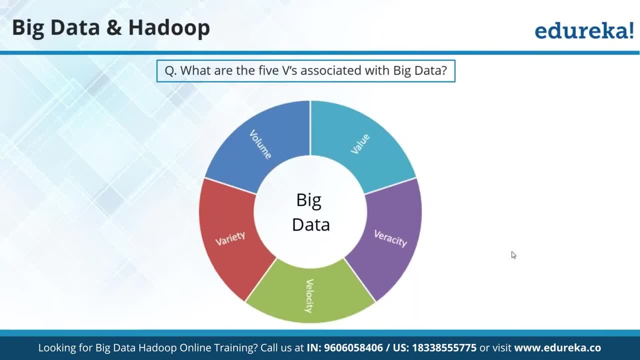 they have made it in just 10 to 12 years. Imagine each user is also doing this activity: posting video, audio, all kind of chats, right? Is that how much data they are dealing with? So that is, you will be calling that velocity. 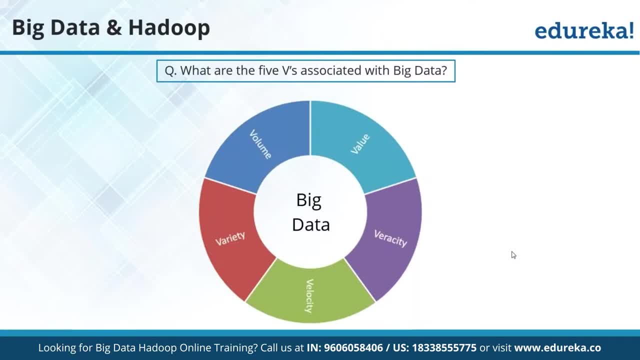 With the pace they have grown up from scratch to this level, with the speed they have grown up to this level is called velocity. Now, these were the three components which were actually going in the market for long. Actually, if you ask me, these three were: 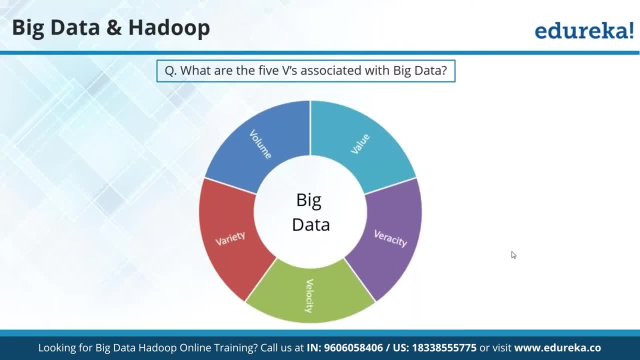 the major components even go today, but slowly they started realizing there should be a fourth category of data, which is velocity, and what basically happens is that the data, what we receive to us, right, The problem with that data is we cannot expect that the data is going to be. 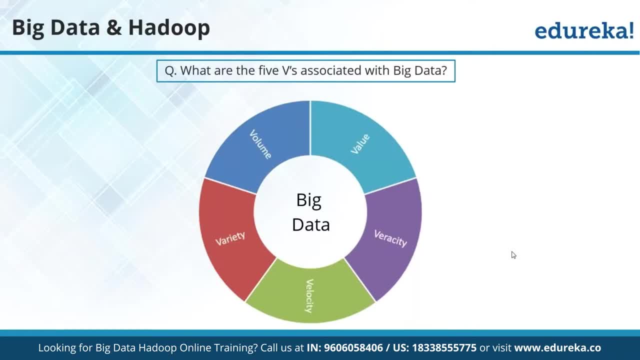 always a clean data. There can be a missing data, there can be a corrupted data, and it is how to deal with this scenario, How to deal basically with those scenarios, because that is a component of now that big data, right? So basically, that corrupted 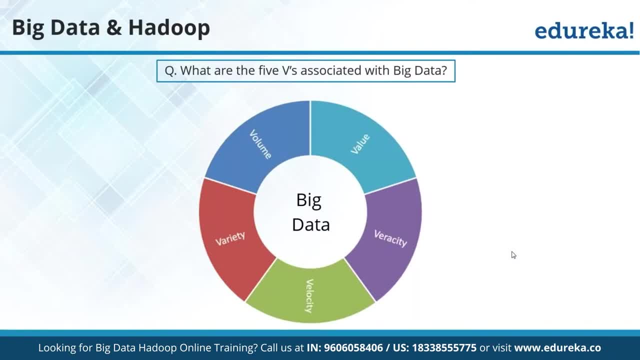 or the bad data is going to be added to velocity. Now people started calling that, okay, these four are the major component, but they are not yet done. Now they started adding few more components. They started saying that, no, we are not going. 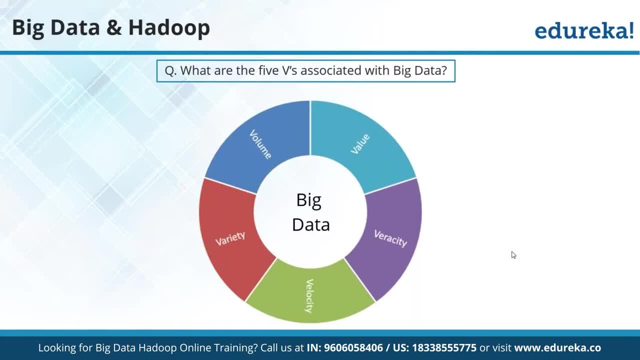 to stop with four, when you are saying that velocity can be added, why not value? Because the data what I am getting. I want to know what is the value of data, how much important that data is. Now I want to see the vocabulary of the data. 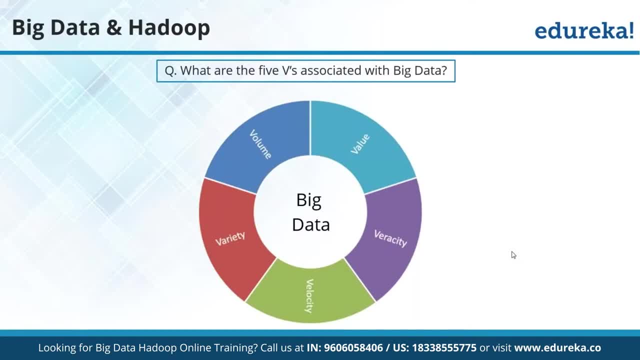 or the validity of the data. Now they started people adding their V's but majorly, if you talk about there are four V's which carry some good value, Okay, And usually in any interview they will not expect you to know all the V's. 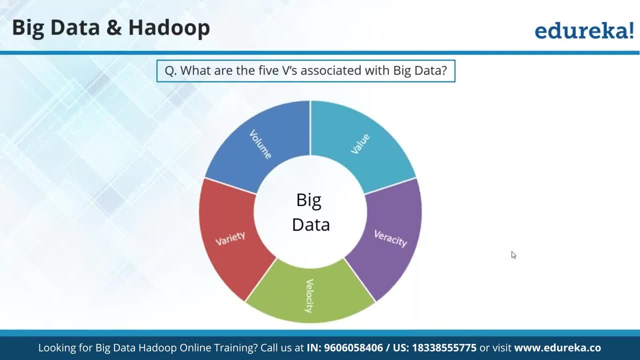 basically, If you know, it's all good, but they will be just expecting you to kind of understand that. okay, do you know that? how good you are in terms of thinking like I generally do that. So when I generally ask questions, I generally see. 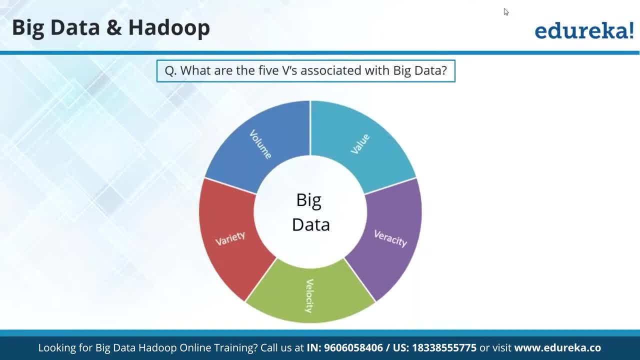 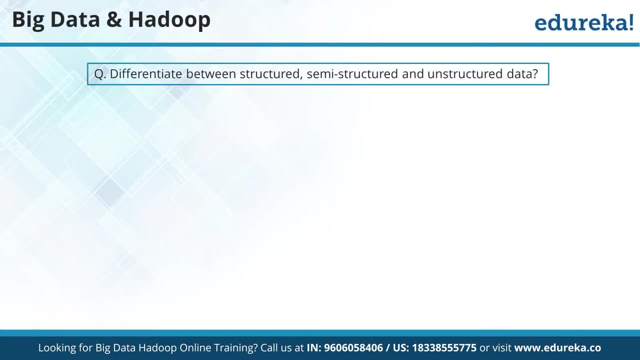 that, okay, that guy must be doing four V's. let me ask five V's. let me see that he is able to think little beyond what he knows already. Moving further, We just talked about something called structured and unstructured data, Right, Can anybody? 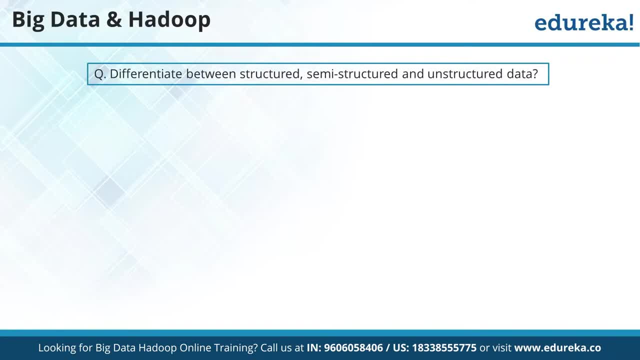 explain me the difference between structured and unstructured data? That third category of data, let me add it Now. can anybody explain this, plus give me the difference between them as well? Can anybody give me an answer? So unstructured, not easy to save. 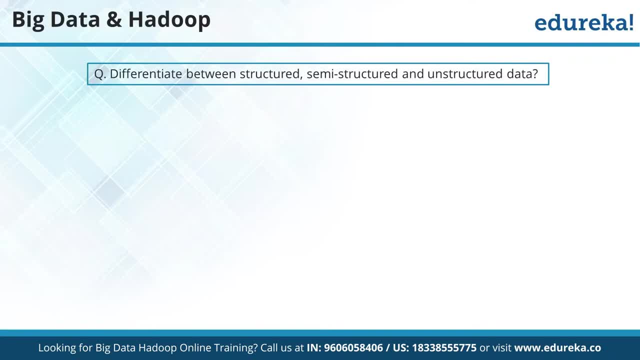 the data into RDBMS? that's the question answer from Nabish. Structured data is basically in row and column. unstructured is like log audio video. semi-structured is like XML JSON. Yes, So lot of people are giving the right answer here. 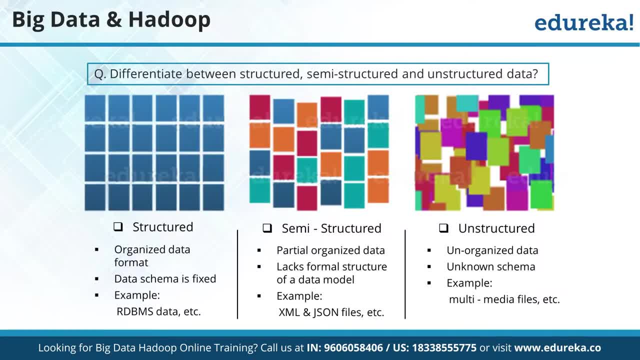 If we talk about basically structured data, If you go with basically 1980s, when this Oracle and IBM and all those companies came up into the market, So if we talk about 1970s, 1980s, you will be surprised to hear. 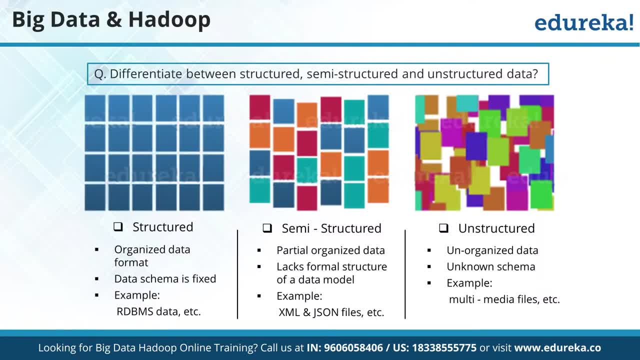 at that moment, it was still a challenge to deal with that data, Though it was having some sort of pattern. it used to have some sort of pattern and it's a small data Now. people used to think that, how to use it, how to 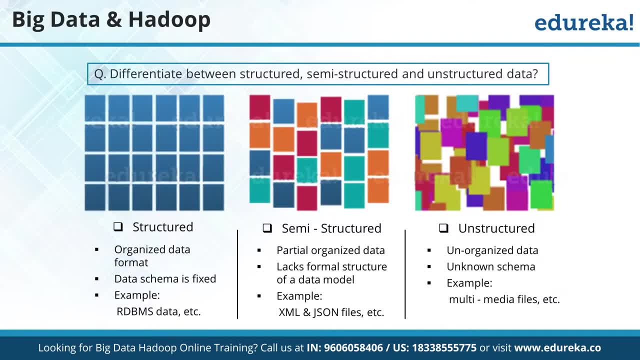 that you can now store the data, you can now process that data. what sounding like having some pattern and you will be all good. And today, I need not tell you that today, where these companies are like Oracle, Microsoft In fact, everybody must be willing. 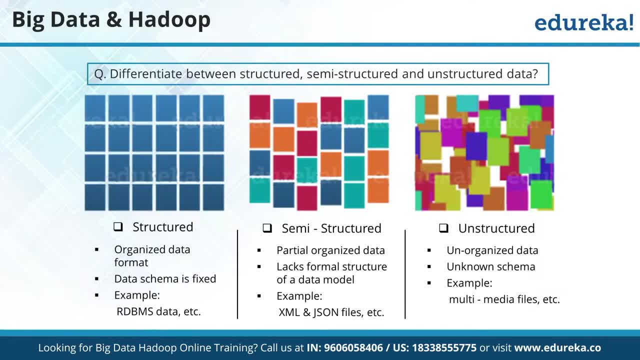 to work for them if given a chance. So the data, what they were dealing with, was structured kind of data, But with today's world, like Facebook came up in few years back now, as soon as Facebook came up into market. I'm just 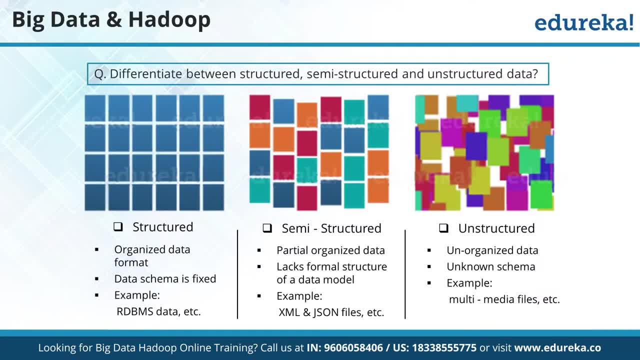 giving an example now: what you do in Facebook. on Facebook, you either upload video, upload audio pictures, so you started dealing with structured data. Now we cannot call this data as structured data, because this kind of data do not even have any sort. 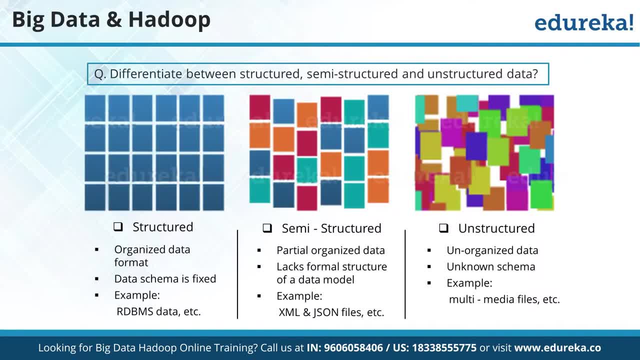 of pattern, and that is where we started calling it as unstructured data. Any sort of data which do not have pattern kind of thing, like your audio videos- we started calling it as structured data. There are some sort of files, for example. 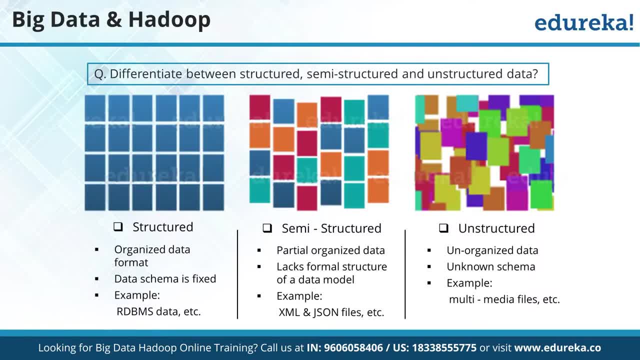 let's talk about XML data. So as soon as you see XML, what is it sounding like? Does it have pattern or not? Does it have pattern or not? XML files: do they have pattern? Yes, it has pattern. So 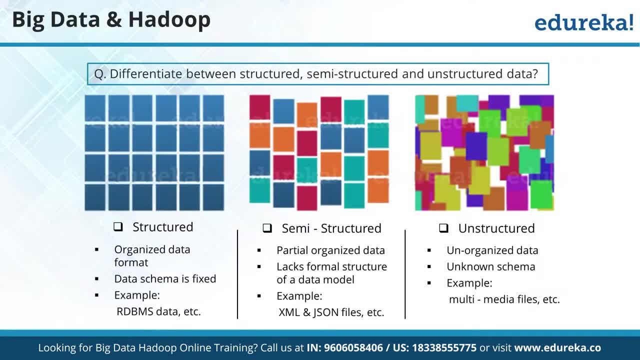 it is structured data. Now, as soon as you tell me that it's a structured data, my question for you is: in that case, can you do all the activities, what you can do in RDBMS to XML data? I know you can. 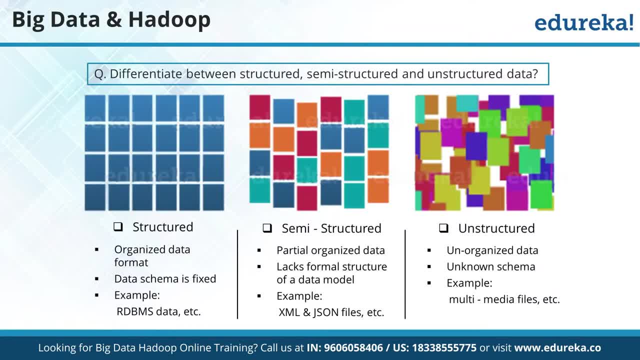 do today. even you can deal with unstructured data. Now I am confused whether it's a structured data or unstructured data. That's where they created a third category called semistructured, so that they can keep it in the middle. 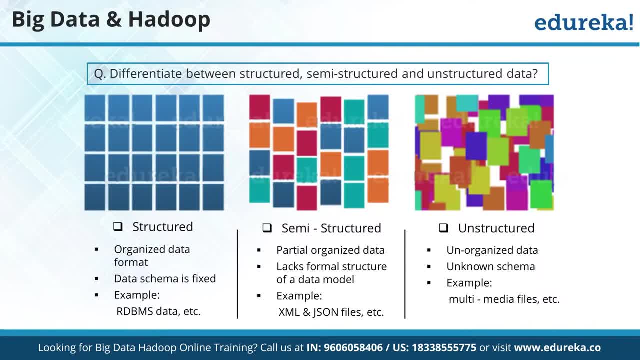 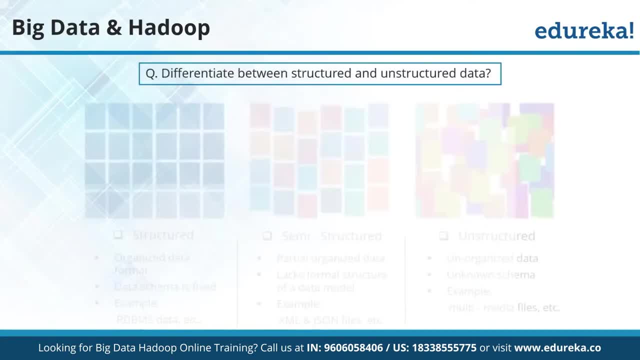 The data, which is sounding something of the structured type or as an unstructured type, so that they can keep it in the middle. Now I have another question for you: How Hadoop differs from your traditional processing system using RDBMS. Can I? 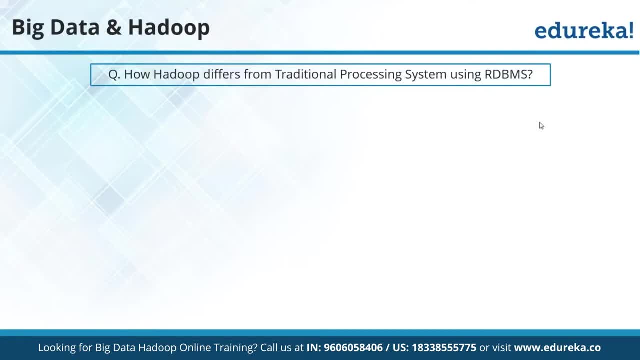 get an answer? What would you answer this part? So these are like warm-up kind of questions. Usually in interviews we refer from traditional processing system using RDBMS And friends. I have a request. Rather than raising your hand, please type it. 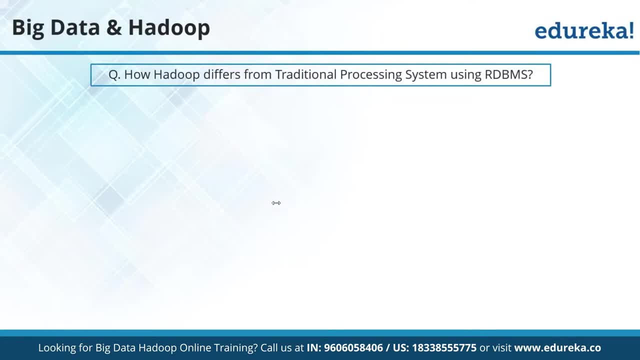 on chat window, because this chat window I want to make it more interactive. I don't know why your name is showing up, but let's take it. Processing only relational data. Okay, I can take this answer. comment. Distributed storage and processing. 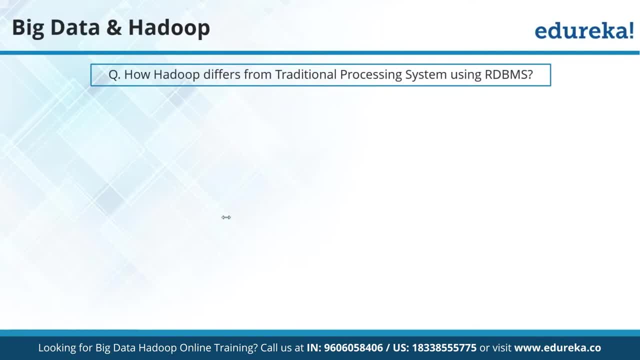 Okay, Good answer. word: Parallel processing- large data distributed. So few people have just started answering. what is Hadoop? Don't answer me that. I want difference. Read the question properly. The questions they give me are the same as the questions they ask. 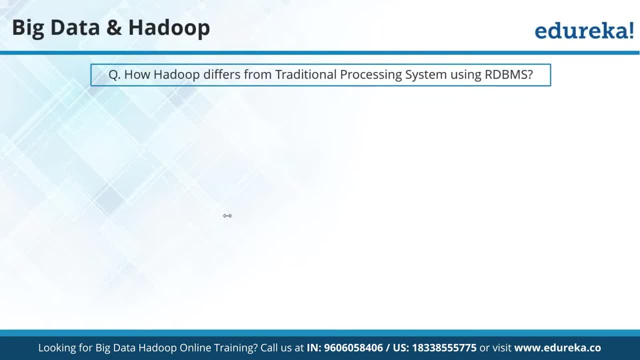 me. I can ask you another way as well. Can Hadoop replace RDB system in future, or maybe is it really replacing right now? Okay, This question can be asked in this way as well. Now, can you answer me this question? Both are. 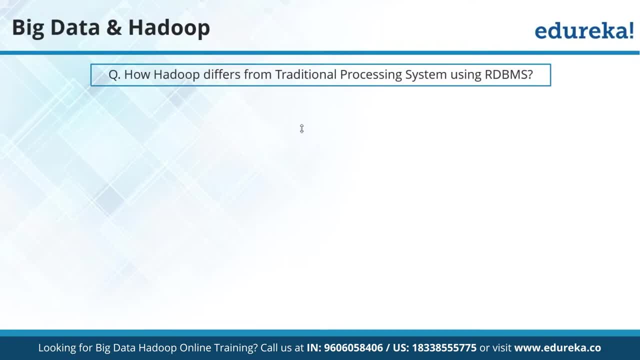 complementary to each other. Okay, Good, Anyone who want to come on here want to answer it. This will give you good confidence also When you will be speaking in interview. it cannot replace RDBMS, but I want. reason is not supported. create, delete. 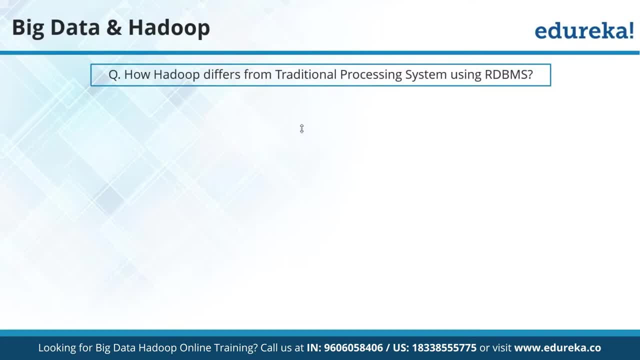 update. can I do that at pro level? No, Right. So that's the major reason. you cannot go with Hadoop systems, like you cannot replace them. Also, when the data is small, okay, If the data is small, you cannot replace it. So 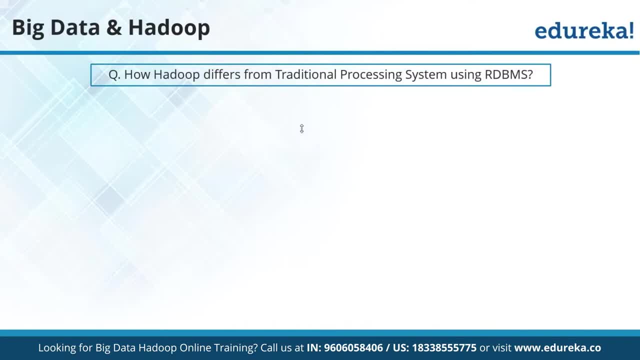 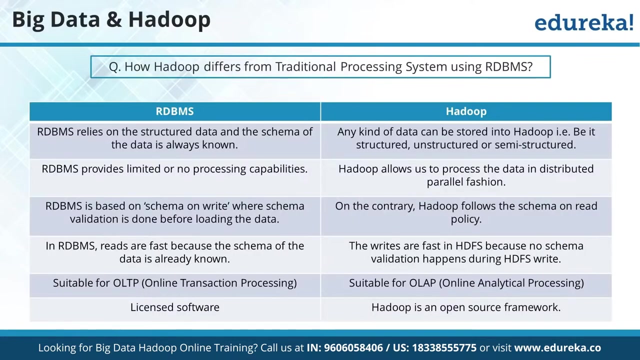 let's look at Hadoop 3.X, which is yet to come in the market properly. So hold on till the time it come up, because it has no restriction, It has no right, no lot. once read multiple times. Okay, So and one more. 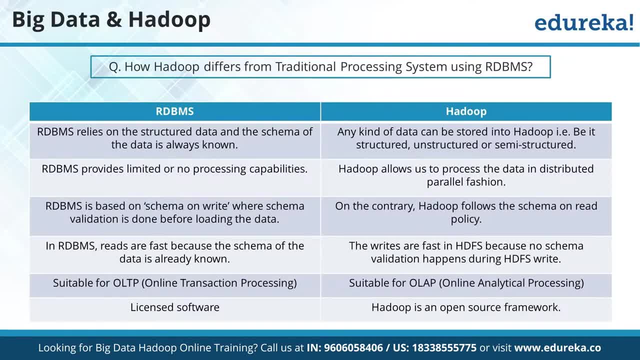 important difference: RDBMS is free of cost. Is RDBMS free of cost? No, Right. So basically, it's a license software. You need to pay for it, Right. But when it comes to RDBMS, if you get stuck, 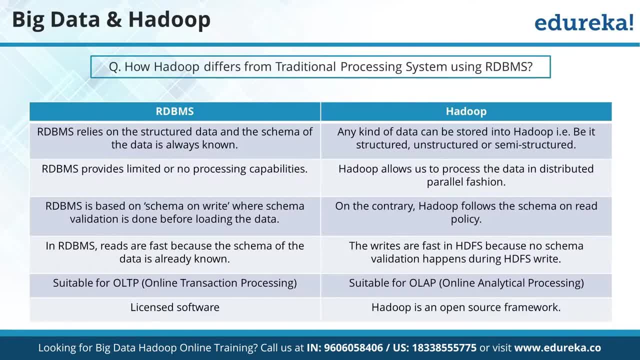 where you will get the support. There is nowhere you can get the support If you get stuck in RDBMS system. there are companies to support you, But what about Hadoop system? If you get, let's say, some bug, who will fix it for? 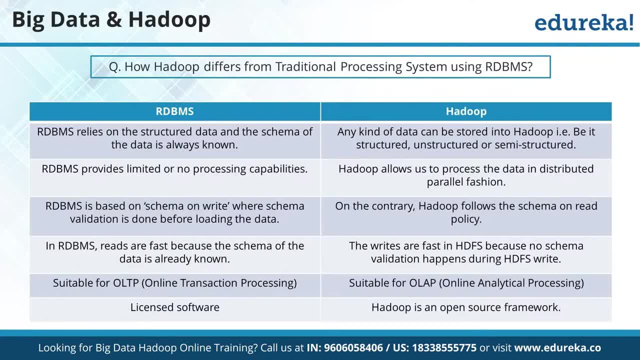 you Right? So RDBMS can only deal with structured data, Right? Basically, when we talk about RDBMS, we are talking about RDBMS and we are talking about RDBMS and we are talking about RDBMS and we are. 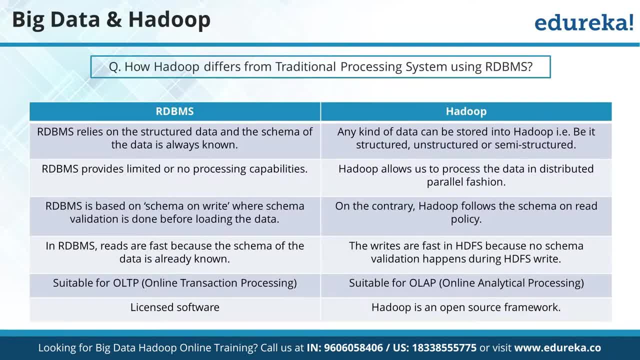 dealing with un structured kind of data. Or you can deal with it. everybody just argues with me, you know, trying to support even, But it has a lot of distribution, it's not efficient at the moment till the time it doesn't come out of. and DLOB, right where what they say that you can now store unstructured data and can work on it. 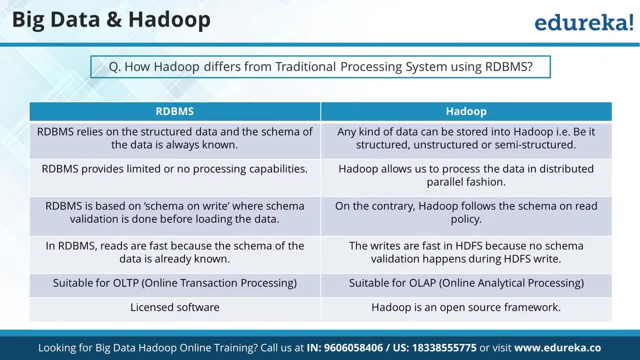 but are they efficient? answer is no right. so, similarly, like most of the data, what you deal with RDMMS is going to be structured data, but when it comes to your Hadoop system, it can be unstructured, semi-structured as well as structured data. right, because if we take an example of high 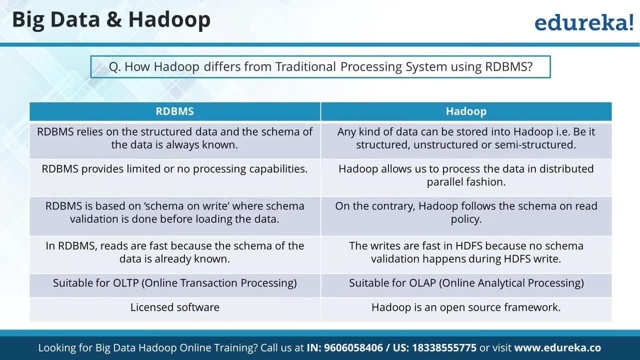 you know they deal with structured data, right? so that is one thing. which is there: RDMMS- you work just on a single machine, right? so let's say, you work on a single laptop where you have RDMMS installed and working, but when it comes to Hadoop, you are working in a distributed fashion, right? 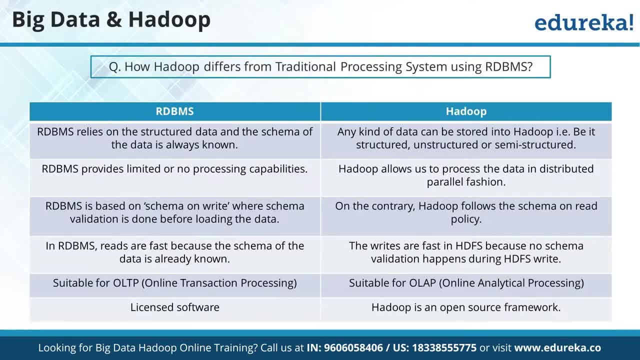 there will be multiple machines which can be involved. in this case, right and as I said in RDMMS, mostly when the data is small, your speed will be very fast. your computation is going to be very quick. at the same time, with Hadoop, your computation speed. 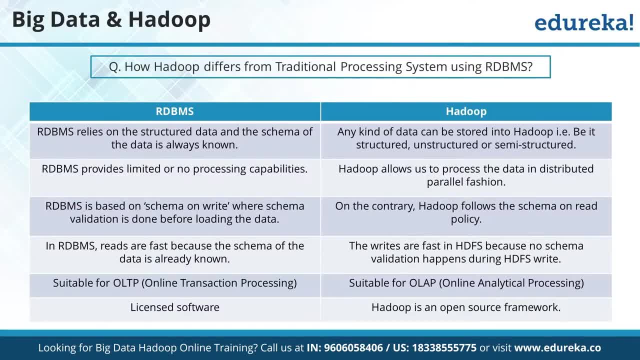 is not going to be that great. okay, with the small data. it's not going to be that great with the purchase path switching into the market. that's a different story. now they are actually picking up, basically because if your memory is good, then you can actually make up a good speed. 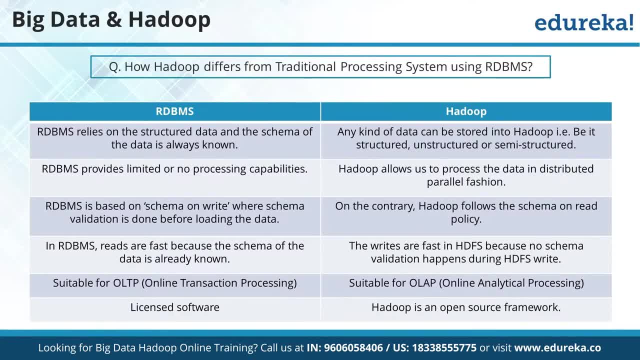 but with traditional Hadoop, when we talk about map reduce, the speed are slower. you, I believe if you have already done the classes of map reduce, you might have already noticed this, right, when you were doing that word count example, right, I hope everybody must have done word count. 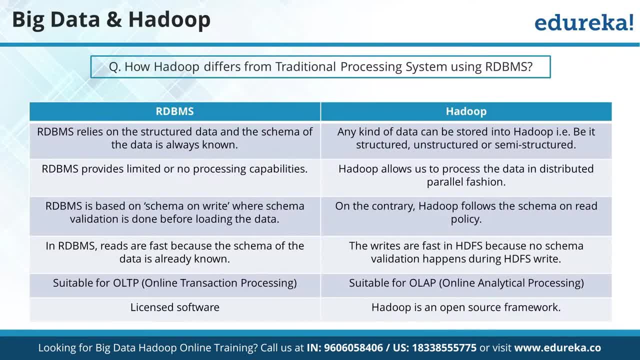 example in map reduce right, if you have taken the session right. so in that case you might have seen the speed of word count example that it is not that fast. so that is one thing. with Hadoop system, especially the data is smaller. your speed is not comparatively with RDBMS. it's going to be. 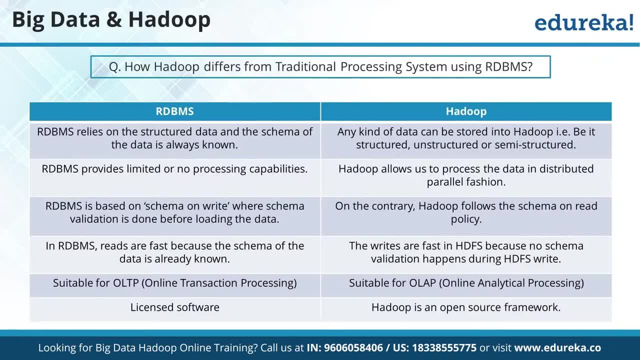 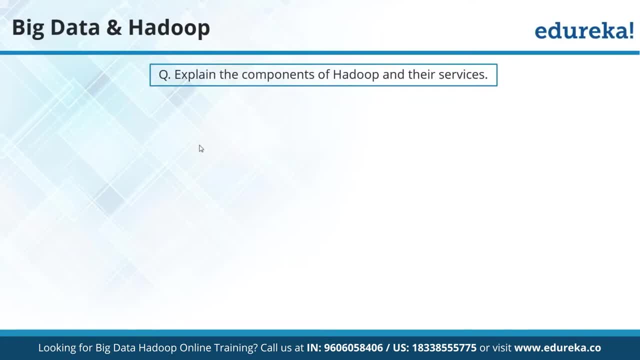 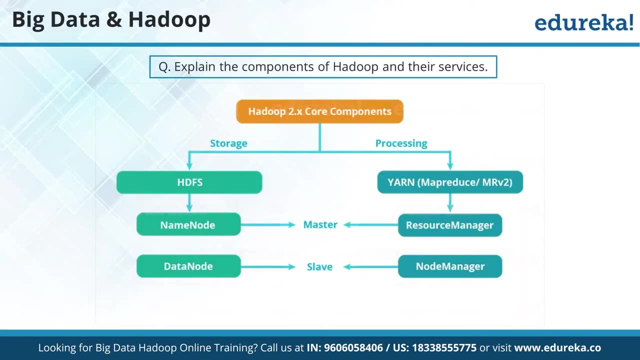 slower now, which brings me to another question. can anybody tell me the components of Hadoop and their services? in fact, i'm showing you all the components. can you explain these components? what are the components available of Hadoop and what are the services, what they provide, can I get an answer very good? so basically, when we talk about 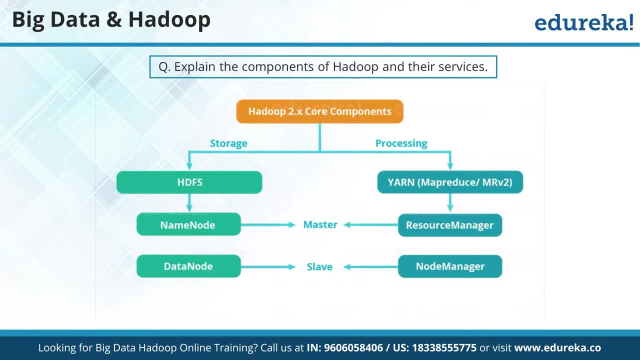 HDFS: right, it is for your storage side. okay, very good, connect. can I get more answers? I believe everybody must be knowing this part. nursing is saying storage. HDFS is for storage, yarn is for processing cluster. very good, so you can say: yarn is a cluster resource manager. right, there are few more thing. can I get? 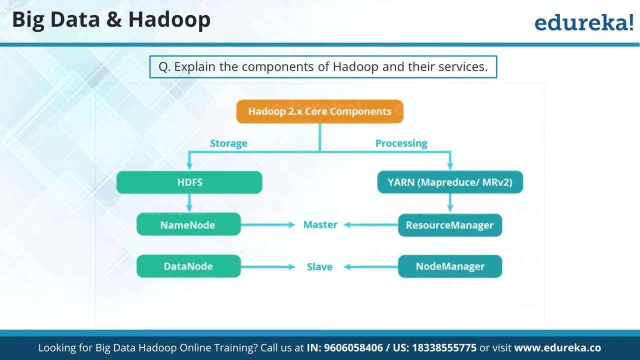 more answers. name node manages the cluster. data nodes stores the data. okay, I can take this answer, but partially. debut: name node manages the cluster. can you be little more explicit in this part? yarn for模 after its allocation: very good a envy saying yarn to run map reduce. okay, 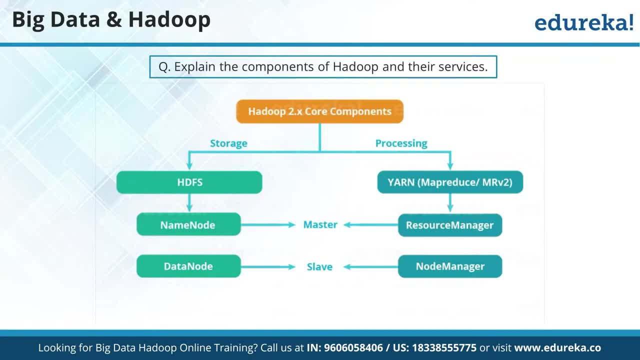 or you can say to share dual movies. that would be better anyway, right? rather than think to run the produce, understand and prime. but in case you are an ingenious kid, that would be better, right? rather than saying: two, run, map, reduce that willigator, anyone, right? rather than think to run, map, reduce again. I think. 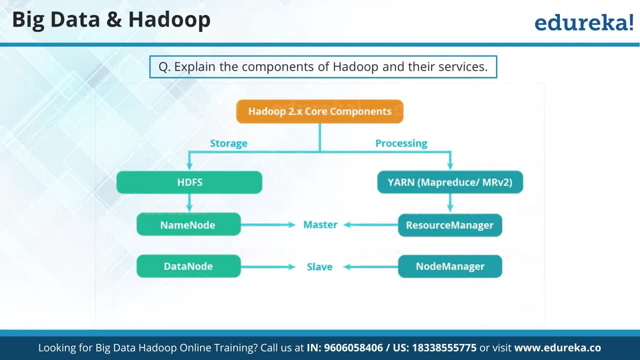 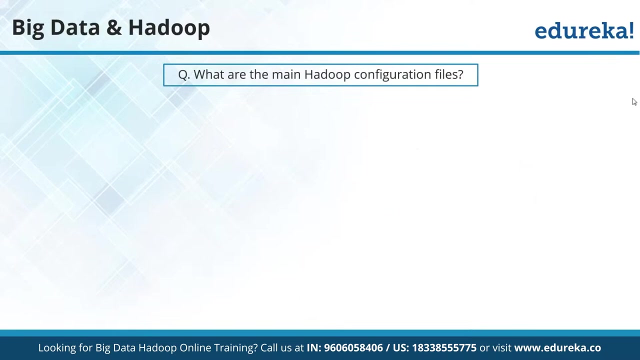 schedule map: reduce, right, that would be a more appropriate answer here, but a good attempt. name node has meta data. very good, right, name node has meta data. you can take it of something of this sort. so, uh, in your real-time scenario- right, let me go back. you can simply relate it with this: 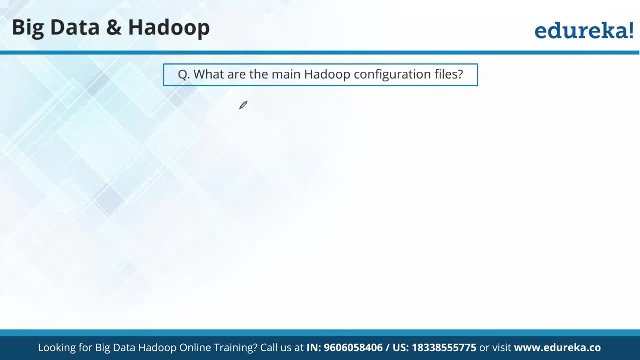 your real-time flight watcher right. let's say in real-time scenario what happens. let's say you have a boss. okay, how many people have a kind of a smiling boss- good boss, smiling boss, but a cunning boss, very cunning. he plays with your emotions. when i say emotions, i basically mean that basically. 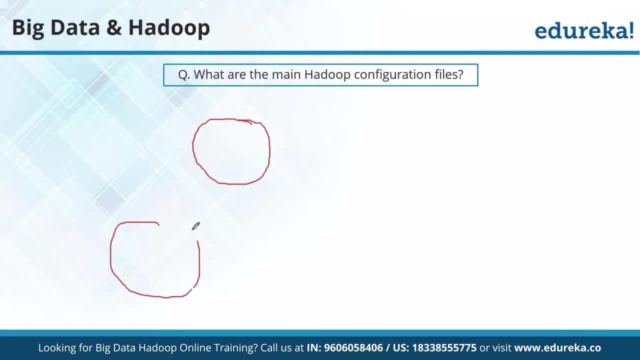 he kind of is a very clever boss. anybody who have it okay a ribbon, have it narration boss is very interesting. okay, so let's say this boss, okay, let me draw a smiling boss. okay, so, smiling. now, usually every boss is smiling, right, they just keep on smiling. 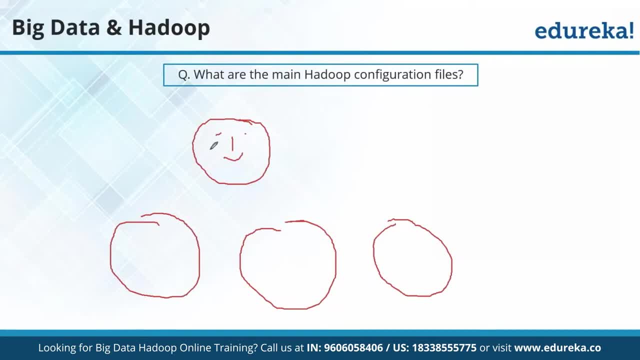 but the the point to work here is that smile is cunning smile, or what kind of smile now? what next? now, these are people who are working right, like uh, like she said that he reports to such kind of boss, right. so basically, vivic say: please report to such kind of boss, who is a very clever boss, right now. let's say um, 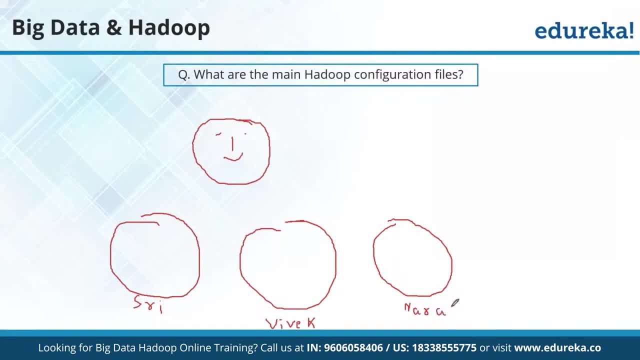 narasimha is saying that, okay, fine, his boss is also kind of a very innocent boss, but you know, behind that, he knows there might be a lot of cleverness, i think, right behind us. so let's say these three people are reporting to this clever boss. what happens, boss? get products right, boss. 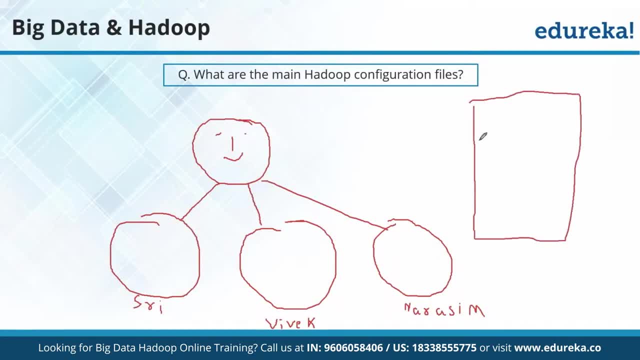 get product, let's give the product. now what happens? boss will report to such kind of boss. getting a project, these three people are reporting to this, uh, to this boss, right? so what they will do. so boss usually will distribute the project selected. the project was p, he distributed into. 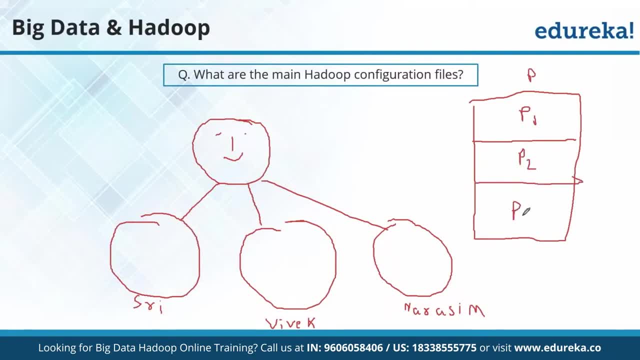 three parts: p1, p2 and the third component. he made it p3. what he is going to do. so he is going to keep this p1. uh, he gonna come to shree and say that work on p1 project. he will come to vivek and say: 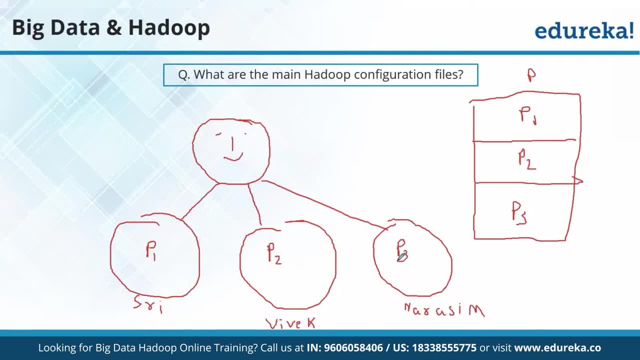 that work on p2 project. he will come to nursing and say that work on p3 project, right. he will say that, uh, all the three people are working properly. given the project on timeline, boss is going to be happy. now imagine a scenario that vivek ditch is not basically ditch, but maybe he said that. okay, fine. 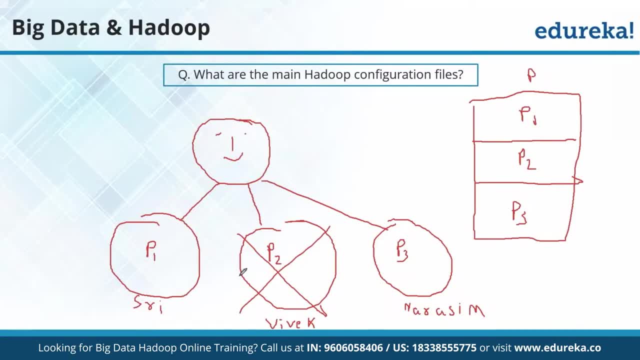 my boss was innocent, so let me take an advantage of him telling him that you know, i have a family emergency. i can't work, i want, i have to take leave. something of family emergency cannot be now. boss is in presence. right, because boss needs to work on these two products, right? 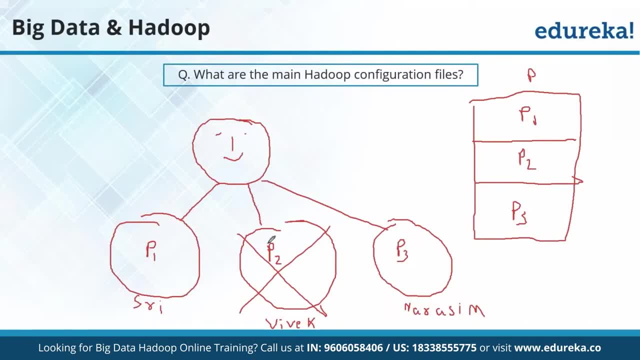 one and p p who will deliver p2 product. so that is the problem. so, boss, what they do? they come up basically between earlier uh kind of backups, and boss is clever, remember right? so boss is going to call shree in his uh cabin and say to shree: shree, you know, you are doing very, very good job. 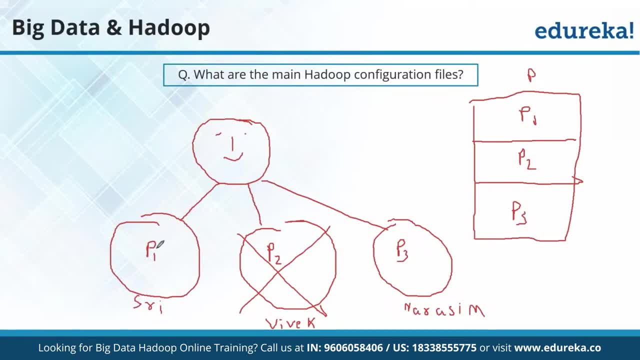 right, so you are doing very good job. i am thinking to promote you. if you keep on working like that, you will get promoted very quickly in the market for sure and um, so you should take up some senior responsibilities from now. right, so as soon as shree will. she will not hear anything, she will. 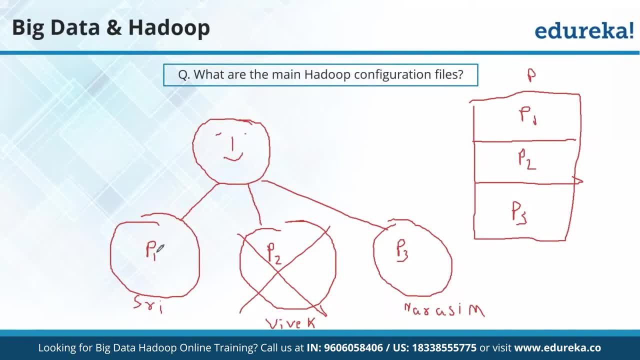 just hear that you know boss is telling me promotion word. okay, he will just be a promotion word and he will be very happy in his mindset. suddenly his boss will throw a time bomb because boss is clever. so boss usually what he will say: uh, actually, we just discussed right that. 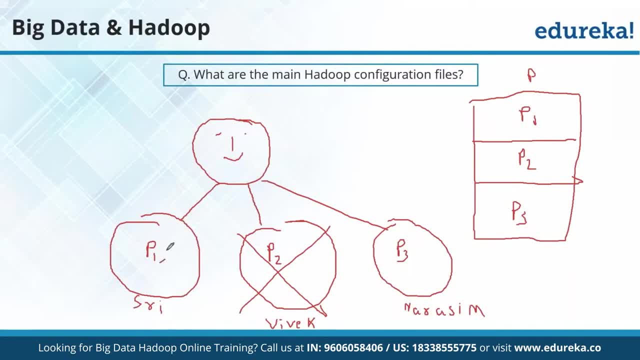 you are going to take up some senior responsibilities, so can you do one thing now? can you basically take the backup of today's project now what happened in this case? immediately, as he said that, can you take the backup of basically vivek project now shree came back. 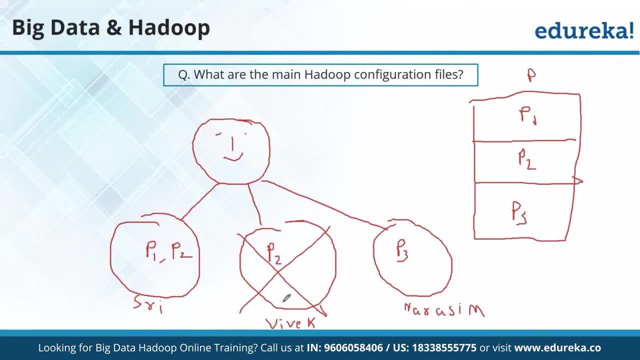 to centers and started arguing. you know i'm already busy, but he said that you have to just take backup. i'm not asking you to work, right, just take backup of his work. if you did me, then only you have to work anyway. you are a senior candidate anyway. boss will work. shree will not be able to. 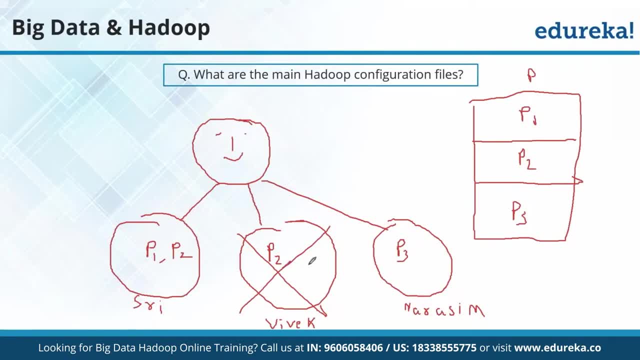 say no, right, you have to work for him. similarly, he will go to vivek. he will do the same stuff, right, because managers usually tell this: right, everything is confidential. so same thing he will do with shree: to not speak about it outside. same way we call vivek, tell the same story and he will ask now to. 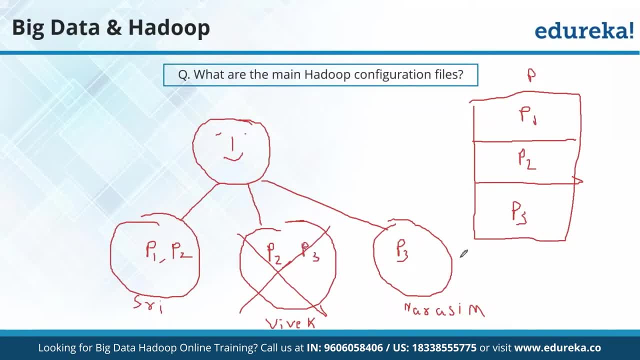 take the backup of nursing project right. so he is backing up this project, similarly nursing. if you note that nursing have to backup shree project, he did the same thing with nursing also and basically now nursing have to back up this, basically the shree project. now, if you note, in this situation, 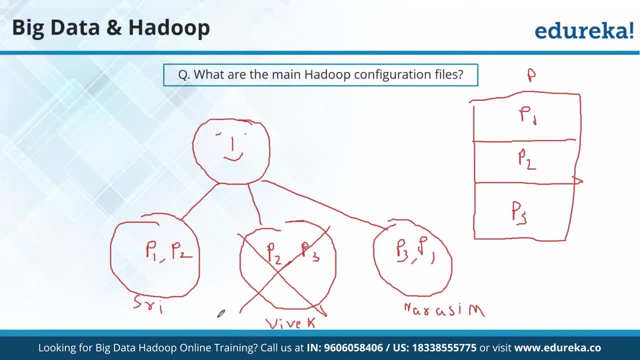 if vivek took half emergency leave now, boss will not face any trouble right now. boss will not face trouble because the work, who has to do the extra work? in fact, who will be sacked in this scenario? definitely, boss is not going to be sacked, but who is going to be sacked in this scenario? 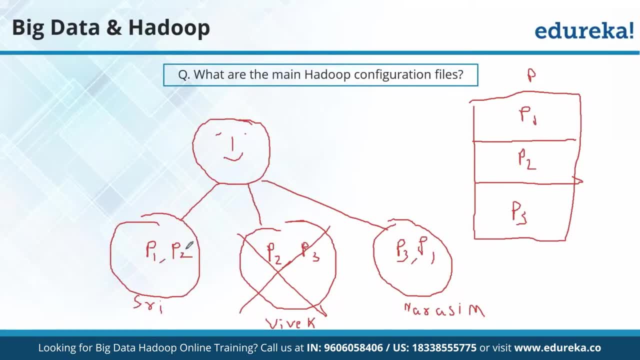 definitely she is going to be sacked, right, but definitely she is going to face the heat of doing the extra work now. similarly, why i am telling you all this? because all the components you can relate here. so basically, the in when we talk about hadoop, hadoop is not much different than this. 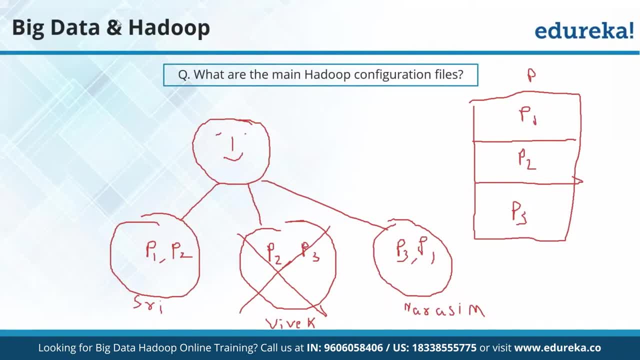 what hadoop do is. and boss is also keeping one more information, right. so boss is also keeping information of, let's say, what all projects he have, who is working on what project. let's say, shree is working on project p1 and we have also a backup of p2. so all these details, what boss is keeping. 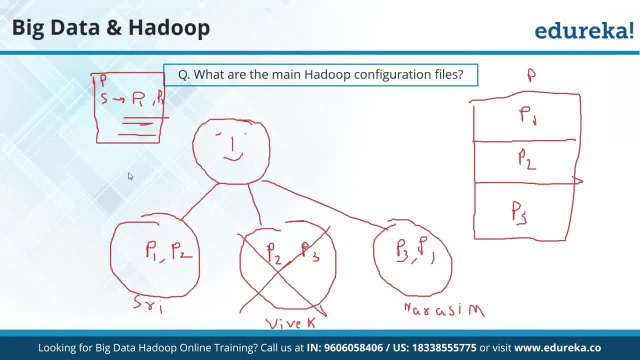 when we talk about hadoop. hadoop is kind of doing that, exactly the same kind of stuff. when we talk about boss, the first thing is now in hadoop, what every human is going to be replaced by machine. now, the first thing is what is going to be replaced by machine. so what is going to be? 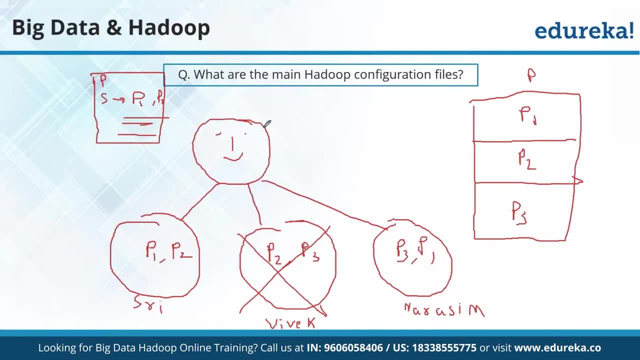 replaced by machine. so what is going to be replaced by machine? so what is going to be replaced by machine? first component: what we were talking about, right? so if we talk about the first component, it was name. the boss is representing name, no. second component was data node: these employees who were 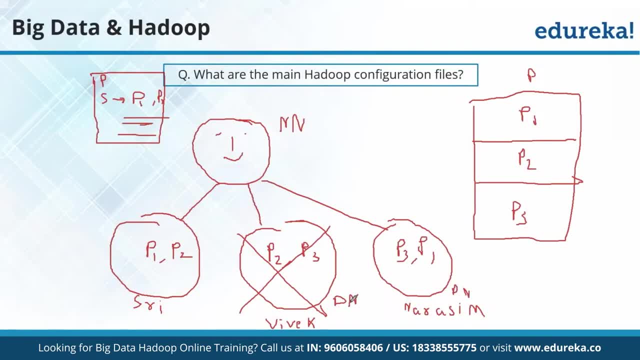 working basically for that boss. you can represent them as data node, the node where you are doing all the processing, because employee do the work right. employee do the work, boss only, instructor managed right. same story here, so these are your data nodes right. same story here, so these are your data nodes. third property: what is this? metadata right, even name. 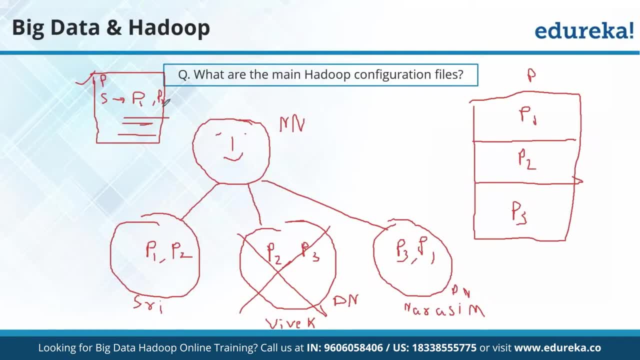 node is going to keep all the data about data that is called your metadata. now, what is this? you, this basically secondary name node and all those stuff. so basically, we require some like: this is the backup for the data part right for this data file: p1, p2, p3, but what about this boss man? so basically, 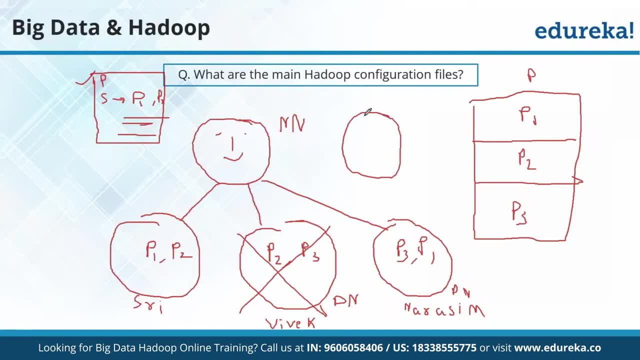 we want to create some backups for that. so that's the reason we keep like passing name node and all those stuff here. okay, so basically that is the back end. so basically this is the back end. we- but that's one of the components. now that that is means like, let's say, in your company they have 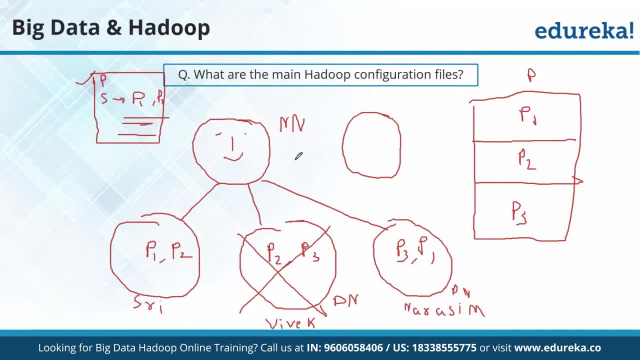 also backed up a boss like, if in case, if this boss needs, then i should have all the details. that's, that's what the backup media. now there is one more component called as load manager, resource manager. what are these things? now? what basically a boss is doing, right? what is boss doing? boss is. 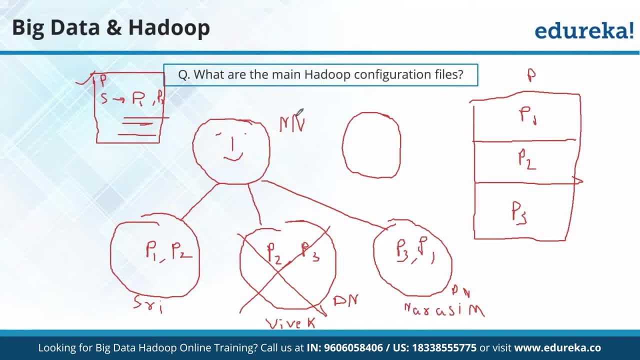 having the skill set to schedule the job right. he only decided where to send what- all those details- right, so that you can call it as a part of your resource manager kind of scheduling the work. who is helping you to schedule the work? you can call it as a resource manager. right, boss, have that. 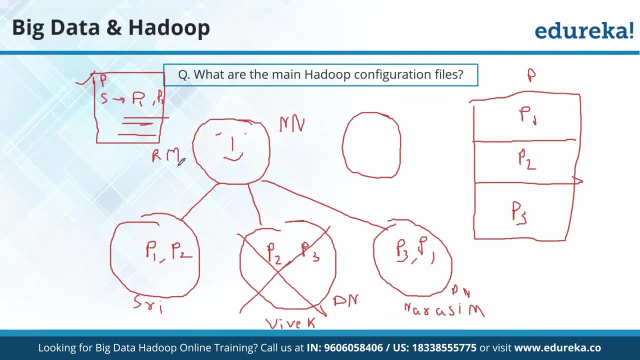 skill set, similarly, in your hadoop, what your resource manager is going to schedule everything up now, the last part, right node manager. now do you think you will be able to work on this project without any skill set? no, right, you require some skill set to work on that project, right? 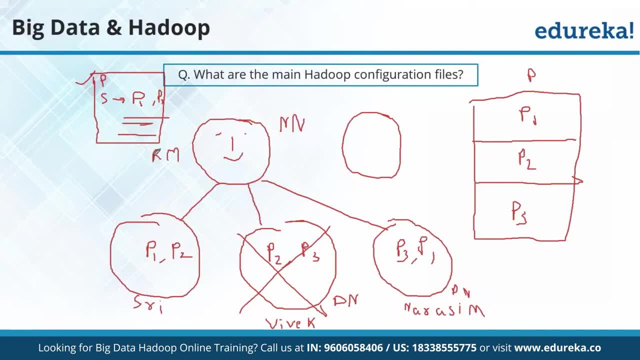 so that skill set you can relate it like your load manager, which is managing your own load, means you can delete it like your skill set which is helping you to solve the project right. so same way, this load manager, you can say that it is managing the whole work. it is kind of helping the node to execute the task. 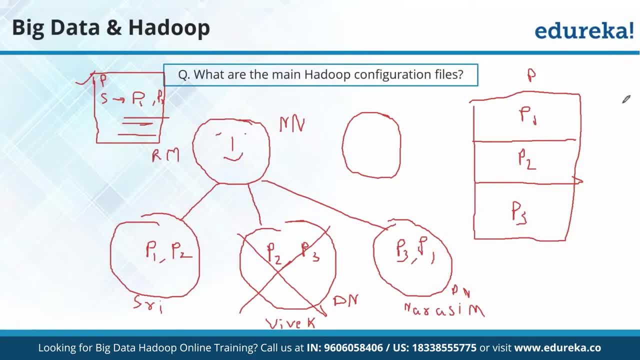 that you can call it as node manager. so this is how you can relate everything. i hope, with this example now, it will make your life easy to remember all these components, because this is a very important question and basically in interview questions they generally ask this question: what are the? 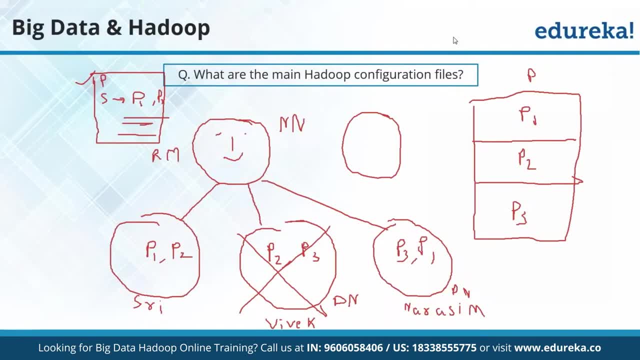 configuration files, what? what basically are the main components? so you should be aware of this and that's the reason i have explained you with this analogy, so that you get some idea and you can relate to it, that if you have to explain in interview you need not remember all this stuff. 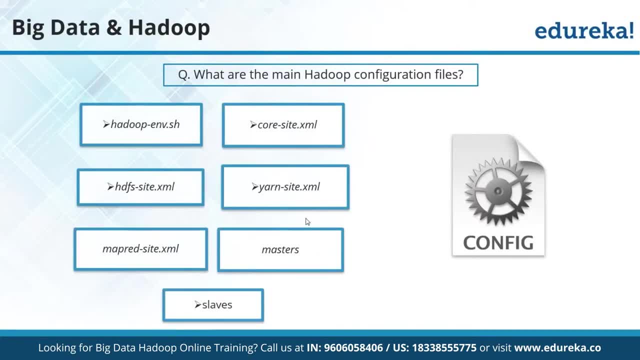 okay, let's move further now. so can i ask this question now: what are the main hadoop configuration files, right? so basically, now we are talking about configuration file. this is related to mostly hadoop administration into this. now, when you talk about hadoop administrator, right? so? 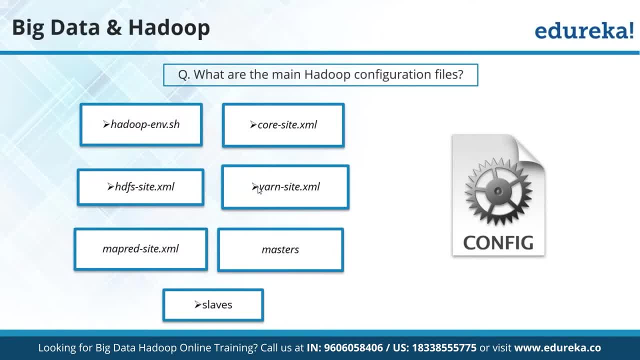 there will be few files which you need to configure. so i hope there are people in this batch, in this session also, where people must have done some hadoop. administrator first, right, so i'm assuming that you two people know that. people who do not know that, let's, let's not worry about this, that's. 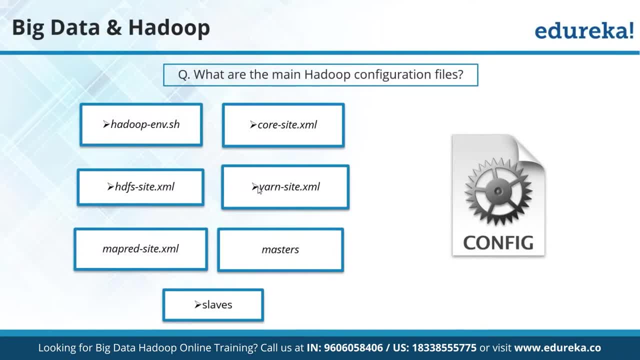 the reason i'm answering this directly. so there are few important files here. one is hadoop environment dot sx. this is where you kind of mention all your environmental variables. for example, where is your java home, where is the hadoop form, all those things you define in hadoop, emd dot sx, port site dot xml. so these, this file, typically you define. 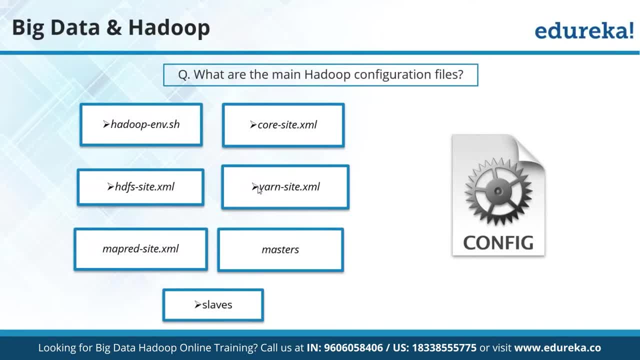 where your lecture name node is going to run, right. so you need to tell the address of your name node where you want to run that maybe you want to run a some machine at 9000 port, so you will be telling all that in your port site xml. when we talk about hdss site xml, here we talk about what? 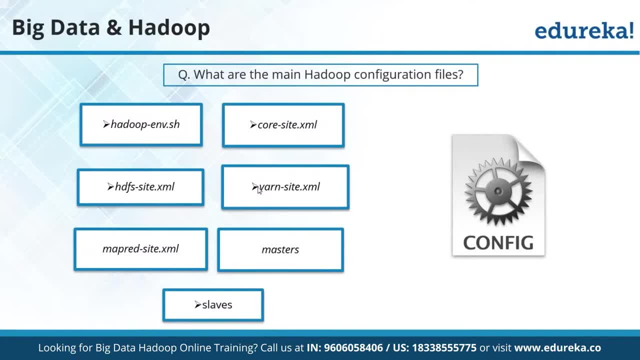 is the replication factor. where should, physically, my data nodes should be present? where, physically, my name node should be present? all those things to define in hdss site, dot xml, yarn site and matrix site basically defines the map jobs. right, what kind of cluster you are going to use, are you? 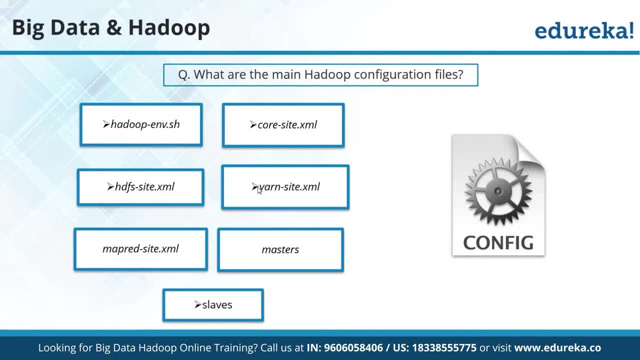 going to use let's end the source, or you are going to use yarn, or you are going to run a local distributed mod- all those things you will be defining here. also, you will be defining where your resource manager should be running. it should be running on this machine, or nine, nine thousand. 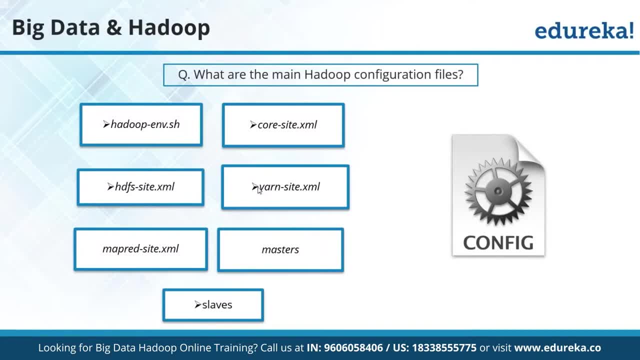 one port or whatever port you want to define, right? so those information you will be defining in yarn site or mac red site, dot xml. now, last two files are master and slaves file. in masters file we usually mention where my secondary name node was. when i say secondary name it's like a backup, not 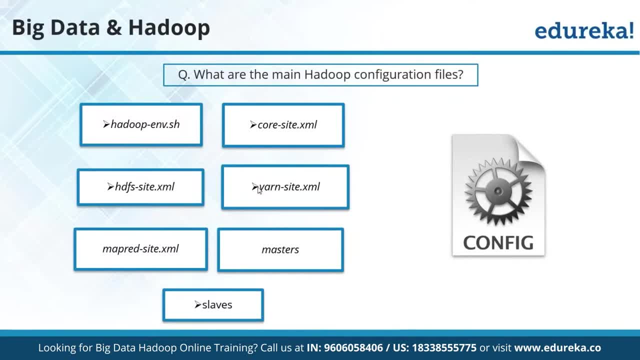 i should call it as a backup, but i should call it as a snapshot of the name node. it's something like this: like somebody is just copying the metadata, that's it. it's not going to become active as soon as the main node is done. it is copying the data so that if name node is down, 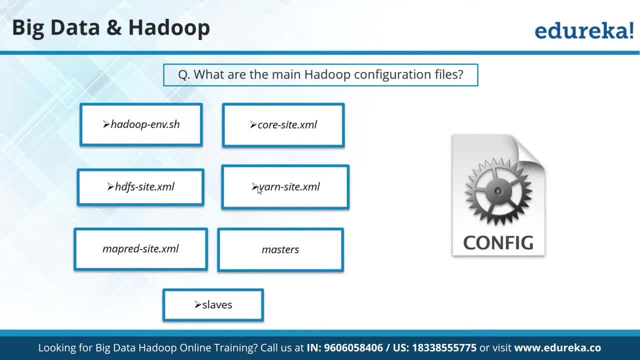 at least i should have a backup. that's it: slaves, very clear with the name. where are all my data nodes, what all machines are going to be my data that can be defined in my slaves machine. so, people who have done this, hadoop administrator, you must have basically played with this file. these are the 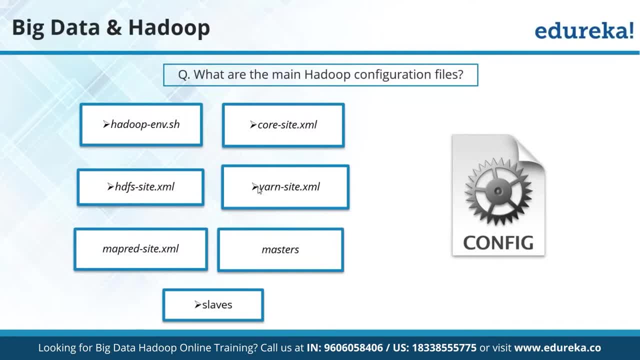 major hadoop configuration files. there are other cells right like hype site xml. there are others like hbs site xml. now, these are very much kind of uh tool specific. so that's the reason they will not be called as the main hadoop configuration file when somebody says main hadoop configuration. 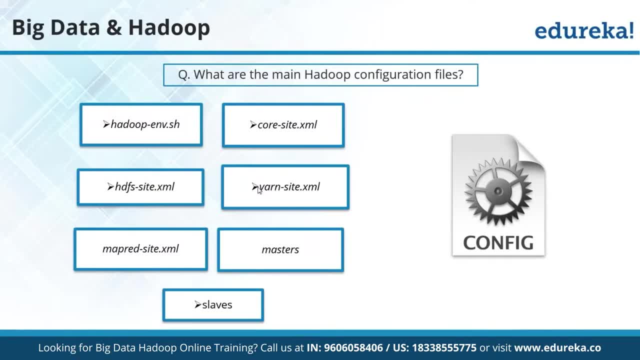 file. your answer would be these seven, five. you need to remember these seven files. basically, these seven files are the one which is the main hadoop configuration file you will mention if you are going for hadoop administrator interview. expect good number of questions in this. okay, they will ask you to explain each and every file how basically you will. 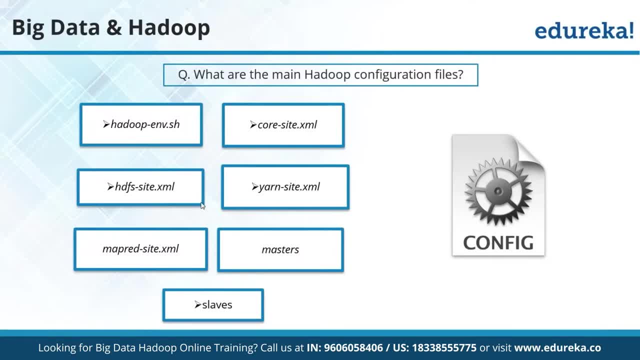 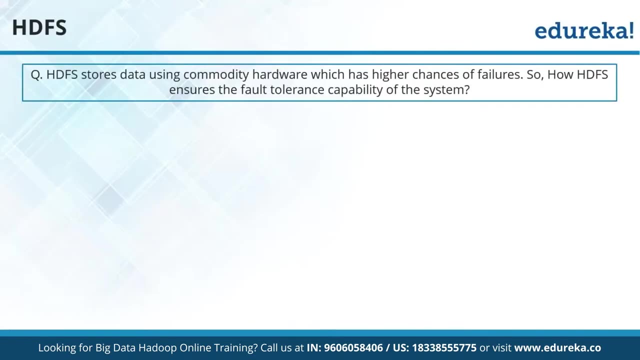 be what you do in which file, which i make a note of that and that is definitely one of the favorite questions of the interviewer when you go for hadoop administrator kind of group. moving further now, let's talk about some hdfs questions. in terms of hdfs now, my question is: hdfs stores data using commodity hardware which has higher chance of? 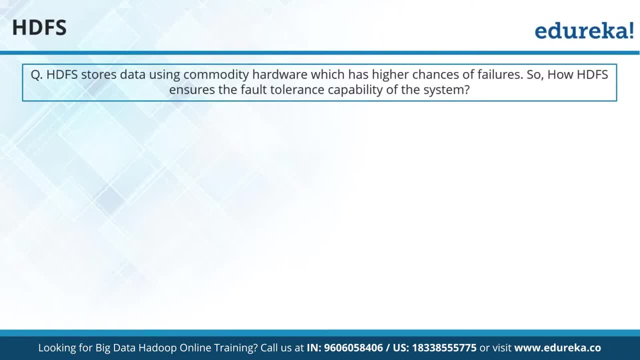 failure, which is obvious. right, because my laptop can be one of the data. no, right now, definitely. my data can fail at any moment now. so how hdfs ensures the fault tolerance capability of the system? can anybody answer this? very good work. can i get more answers? i just answered it beforehand itself. remember that, boss, and 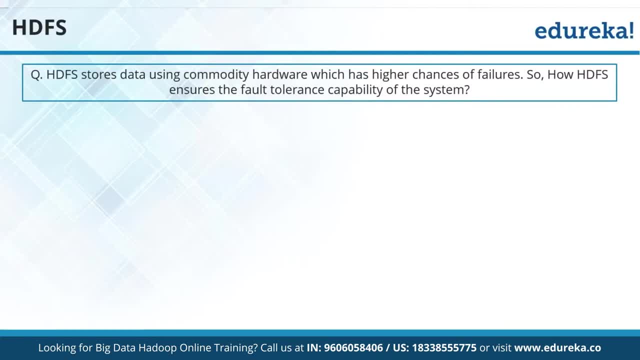 employer relationship. what that boss was doing. boss was keeping backup right. boss was creating backup. similarly, hadoop also create backup right. that backup in hadoop word is called replication right. so basically, if you have, let's say, one block p1, you are creating one backup or two backups of. 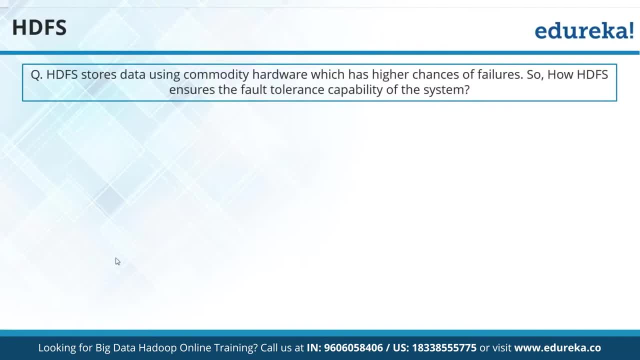 basically that block p1 and that is called replication. this is how hadoop is ensuring that in case of any failure also there should be no mistake. okay, we should not be using data because in case it's very much, one machine fails also, it's okay, it will all work fine for me. so 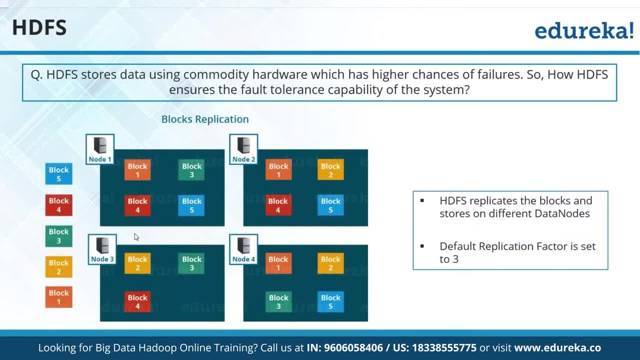 that is what going to happen. so, very good, lot of people have given me the right answer in this case. so block replication is the answer in this case. as you can see in this example also, like block one is replicated three times, if you notice here, right? so block one is replicated three times. 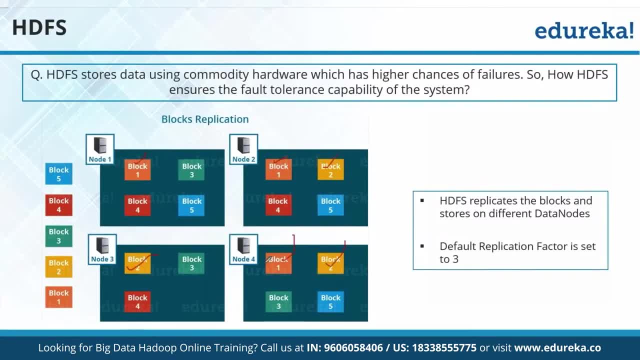 similarly, if you notice, block two is also replicated three times. so these are four different machines and i have replicated block one, block two, block three, block four, block five. okay, so this is what is happening: edit log and fs image is used to recreate the image. fs image and edit log are two different things. these, these basically, are two different things. 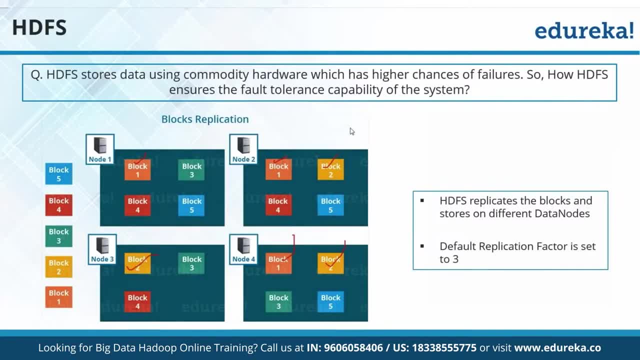 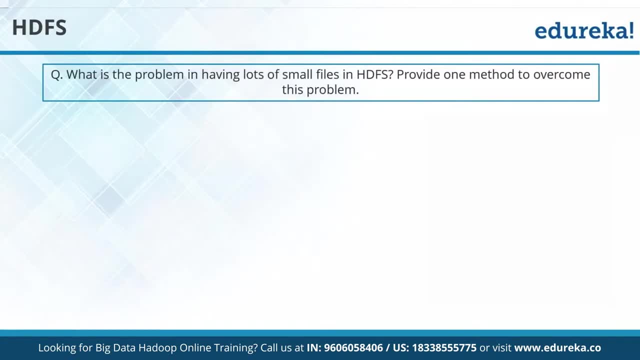 you cannot relate with replication. if you want to know about that, let me just answer you here. so what happens? what is physically this fs image and edit log is now what happens. basically, you have a name node, right, you have a name node where you keep the data in name node. anybody have answered? 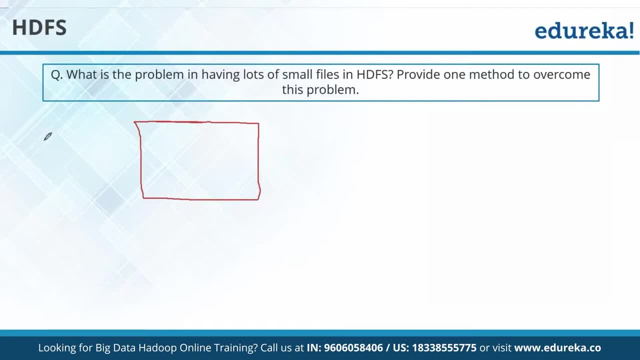 where you keep the data in name node? no, not fs image file initially. where you keep the data in, not fs image? i'm asking in name node. this can also be an interview question. very good, anand, we keep it in memory. why? let me answer this part. let's say there is one client came up. this is one client. 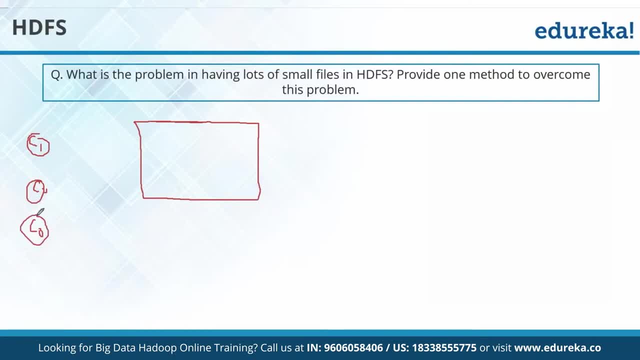 this is clients. into this client, let's say there are multiple clients. okay, now what is happening in this case is, let's say, uh, if this was my name node and let's say my data in name node is my metadata is, let's say, setting in this, what would be the problem? 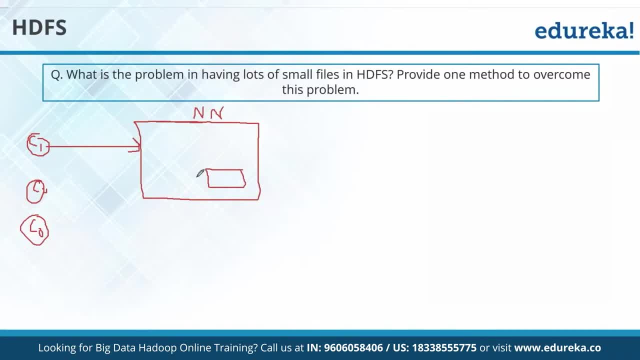 here. let's say, client 1 came and want to access some data. what is going to happen? this data will be moved because any processing which need to happen, right that happens in memory only right now. this data will come to the memory. once this memory walk will be over, then what will happen? 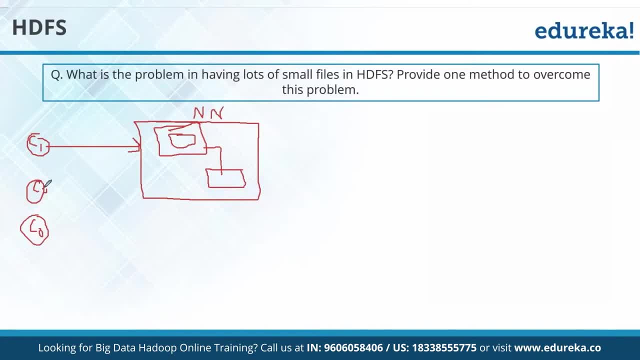 then, basically again, it will come back to this right, it will remove it from memory. now, don't you think there is a input output operation happening, and input output operation is always expensive right now. imagine if there are multiple clients asking at the same time to the name node, don't you think? 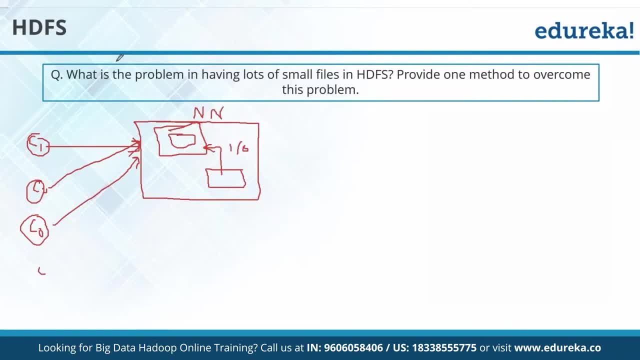 there will be too many input output operation. every time, you need to basically bring the block to the memory and then basically do the stuff and give the output. now, this is something which we want to avoid, in order to avoid what they came up with. the idea is that, whatever you are going, 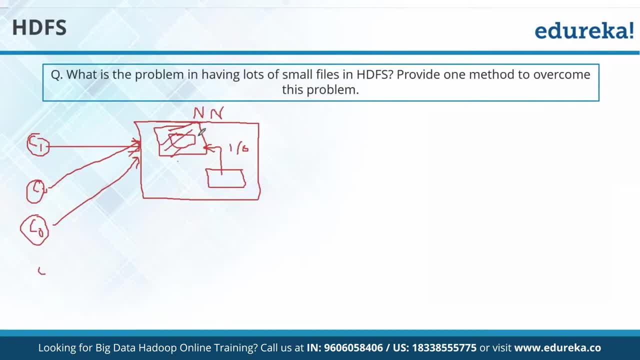 whatever metadata you are going to create should directly be created and kept in memory. okay, that is what the idea they came up. they are not going to keep any data in the disk right now- should be directly kept in the memory. which brings another question for you, in fact, a severe question. 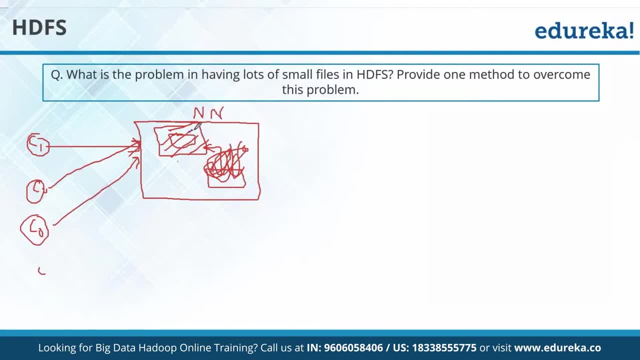 for you now, as since you are telling that the data, what you can keep in memory, but my ram is volatile. when i say volatile, i will lose. i can lose the data at any moment. right, that's very obvious. i can lose the data at any moment because my ram is always going to be volatile right now. 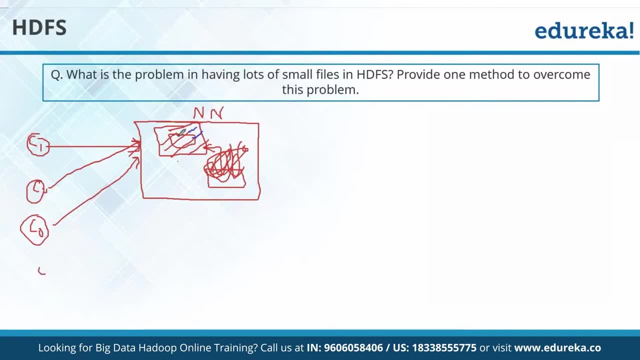 i restart my system when ram data is gone, right, so i will lose all the metadata. in that case, how i will ensure that i should not lose my metadata now? what they started doing is okay. fine, i will create everything in name node memory only. but what i am going to do is, whenever any uh like. 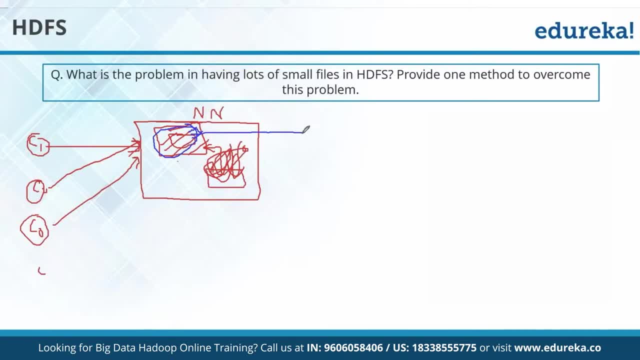 what i am going to do at some interval of time. at some interval of time i will keep on taking a backup of that metadata data in disk. okay, in this i will keep on taking the backup of that data, and whatever backup you are taking in the disk from memory is called your fs image. now, don't you think this fs image is going? 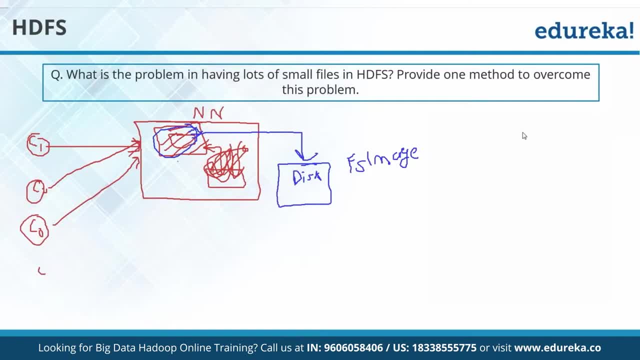 to be big. right, this fs image is going to be big. now, what usually happens is usually, let's say, today my fs image is version fs1. now usually the backup, what they take is every 24 hours if any pop-up kind of thing comes up. it actually stopped my. 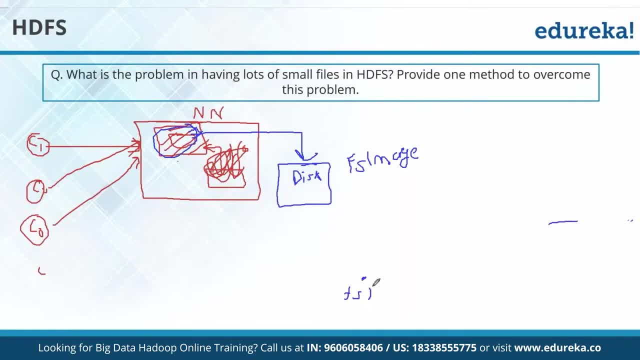 uh, system now, anyway. now what basically is going to happen? so what happens is: every 24 hours we can usually do this backup, okay. so basically, today we did some backup, tomorrow again this metadata is going to do backup now, which brings another problem. the problem now again would be, let's say, 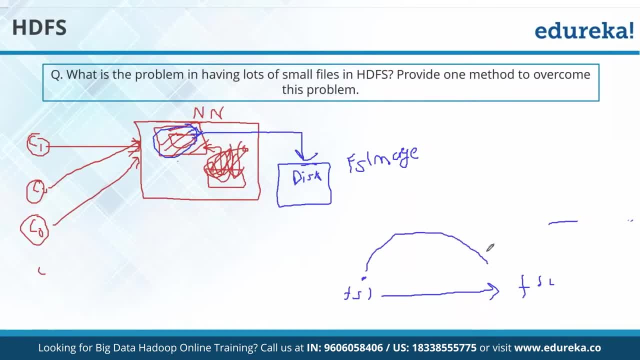 about in 18th hour or maybe in 23rd hour. my machine takes or my rank takes. In that case, I am going to do the 23 hour data, which is again not good. What should I do for that? Now, for that, what they came. 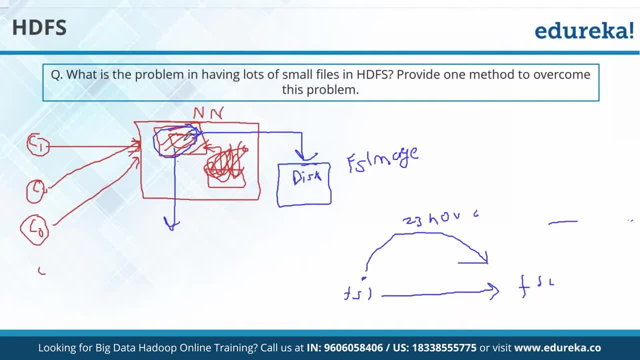 up is that let's create whatever activity is happening here. I will keep on writing in a small file that will be created for, let's say, 24 hours And that file is called as edit log. Then what going to happen for 24 hours, whatever activity? 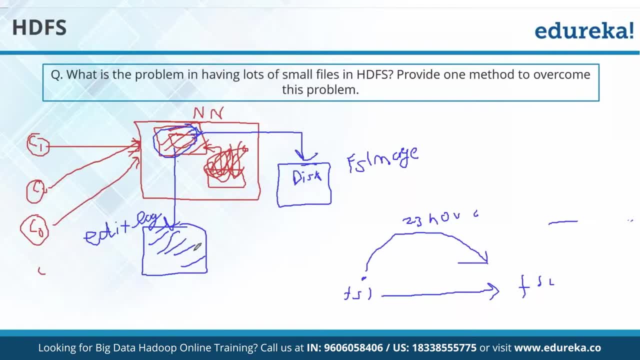 you are doing will be getting stored as a edit log. Now, what going to happen? after every 24 hours, SS1 plus edit log is going to be added up and SS2 will be created Now, in this scenario, even if I use the data in 23rd hour, 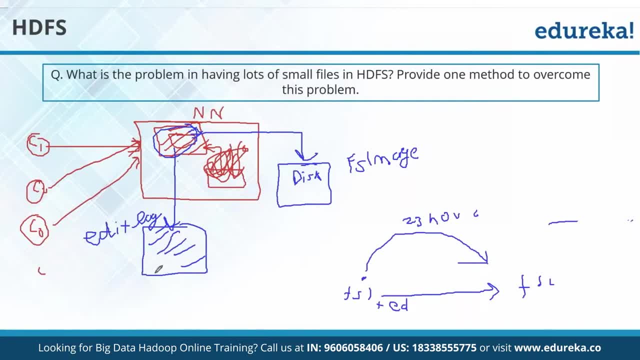 my edit log will be having the data and that's how I am ensuring that I am not losing any data. Now, are you clear about this edit log and fsimage question? I usually see that people are very confused with this logic that what is fsimage? They just kind of 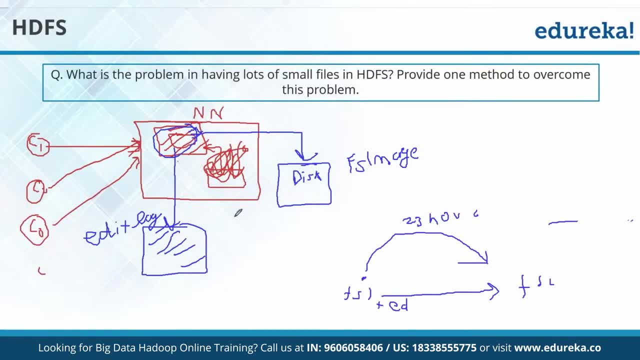 bug up and come back and tell that you know, I know fsimage and edit log, but what exactly are they? I have seen people actually kind of confused with it, So I hope you should be very clear now on this. In this file, can this backup time interval be? 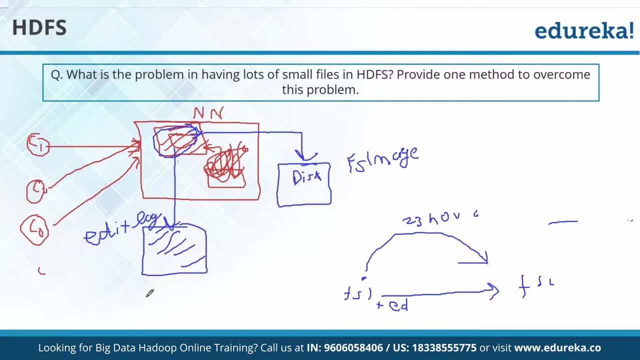 configured. So basically wherever the physical location of name node you have configured and where you configured- I just told you what- in hd, fs, sitexml, right, So wherever you have configured that, so there will be a name directory in it. in that name directory there is another. 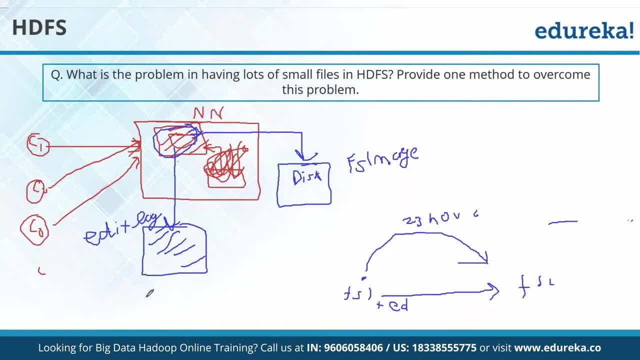 subdirectory called as current directory. in that current directory there is another directory called as snl directory, which is secondary name node directory. there we keep this fs image and edit log Clear about this part. So this is where we basically keep that. So can you please summarize the answer? 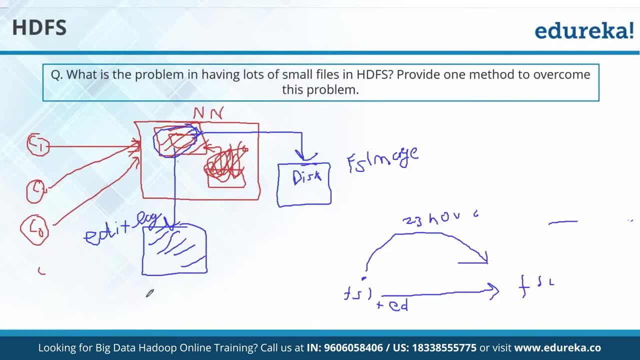 once You have the same answer of fsimage and edit log, but correct, correct, not exactly two files, one file will be kind of very big file. so that's the reason we are creating a smaller version of that file called edit log, so that every 24 hours 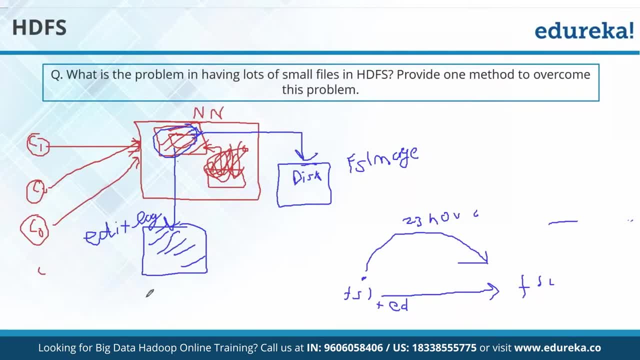 activity we can backup. Edit logs are stored in the disk element, yes, in the name node, So it's kind of act like a backup. that's it. It's a very good interview question. that's the reason. as soon as this question came up, I thought to answer it up, though it's not a part. 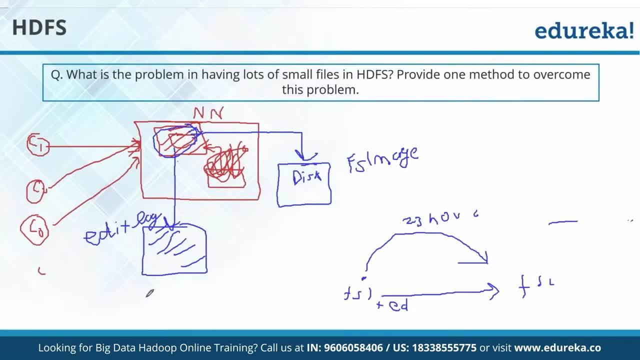 of this slide, but this is a very famous interview question, that: can you explain this fsimage and edit log? and I can tell you that most of the people fail to explain this Here. memory is ranked correct, correct, So it's just metadata which is stored. correct, correct, It is. 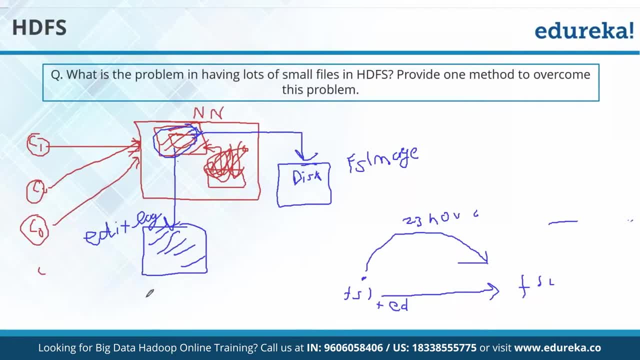 just creating a backup of that metadata for the 24 hours activity That means edit log is getting erased and getting and get new data. yes, yes, every 24 hours it just keep on working and kind of erase the data. That's what keep on happening, Or it creates a 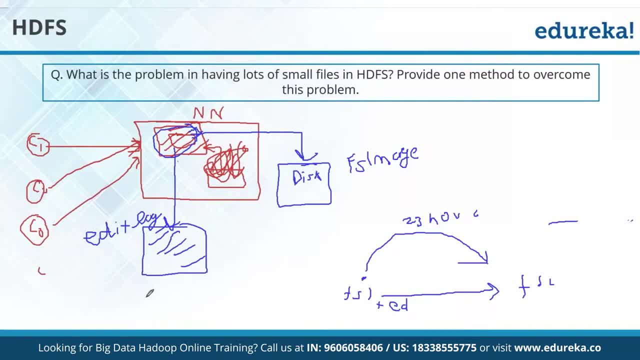 new version. It depends how your admin have configured that. What is the block? data goes more than the memory. Now, in that case, there is something called as fill. Usually it's not, it do not go like that- but there is some concept called as fill. 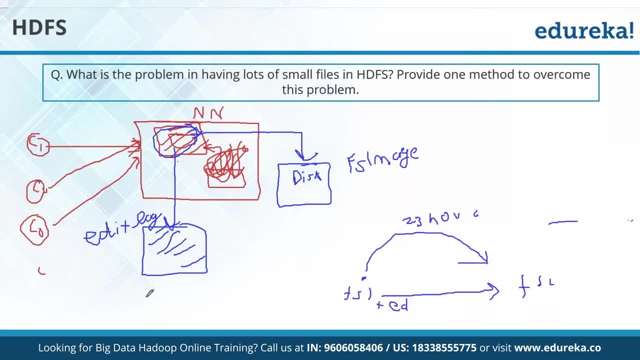 So in that case there will be some input output operation happening. You have to deal with that. So then you are making your name nodes work. So you have to make sure if you should have a good configuration. but if you do not have it, then in that case you have to do input. 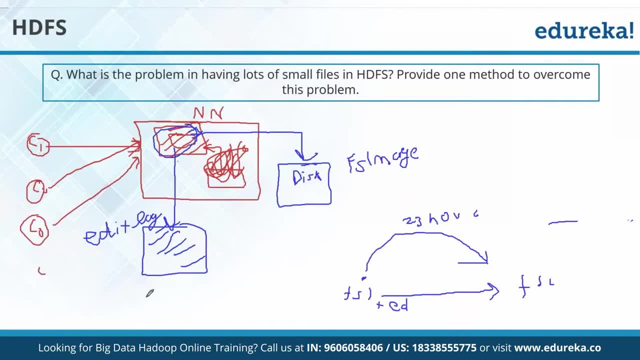 output operation, No other option. Then you have to keep in the disk and then the data will be having input output. The window is of 24. backup can be changed. Yes, it can be changed. To summarize this, what we just talked about: 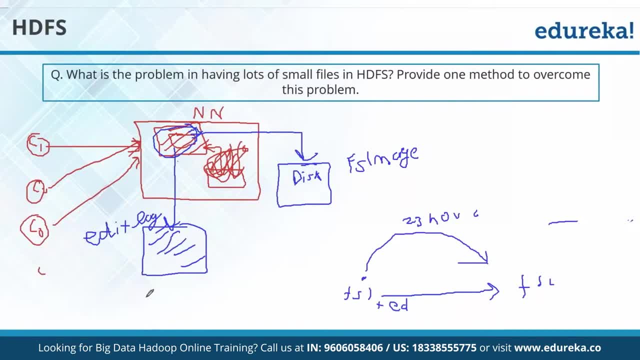 So in name node, in name node, basically, you will be storing all the data, But the problem is my RAM is going to be volatile Now because of that, I want to- definitely want to have a backup. Now. we keep a backup in the disk and that whatever. 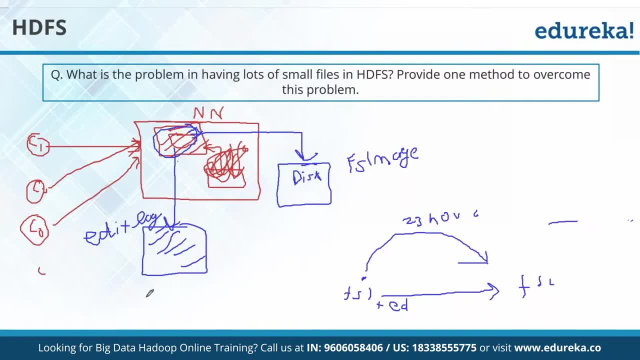 backup we are keeping. we call it as fs image. Now, fs image backup is always taken in 24 hours slot. Now the another problem started with this: What happened if I lose the data in 23rd hour? In that case, I should again create a. 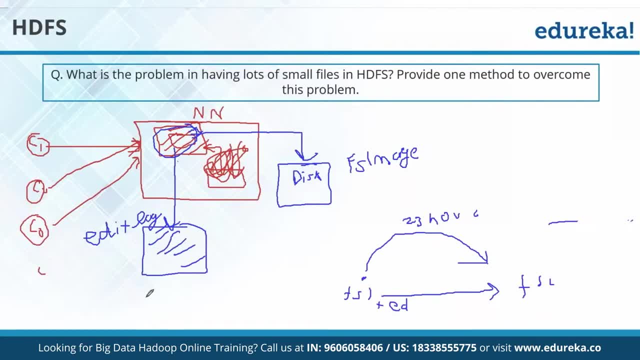 smaller version of the file called as edit log. Okay, That will also be a problem. Now these things will be added and will be basically given What can be the RAM size. The bigger the better. So definitely there is no right answer for it Now, definitely. 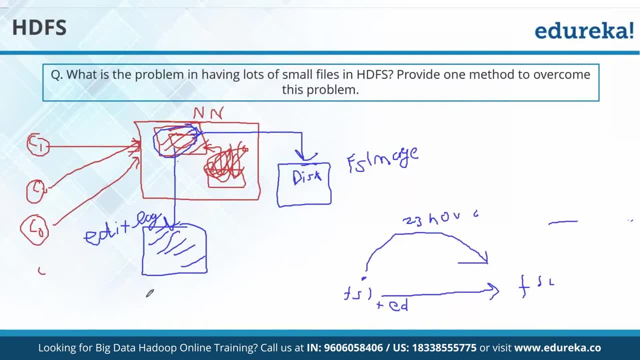 if you say that 32 GB is good, I will say: how about 128 GB? If you say 128 GB is good, I will say how about 256 GB? because that will be better. What if more better data? So we can keep on. 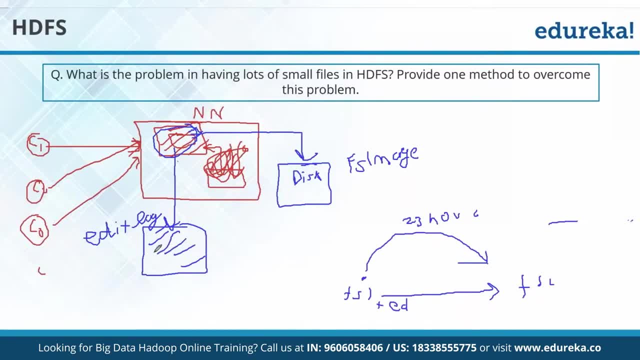 arguing and keep on improving. Right, So the more the RAM, better it is for you, Correct, Correct: With every change in sdl, that's a way of yes, Correct. That's that's what basically happened. Now let's move further. 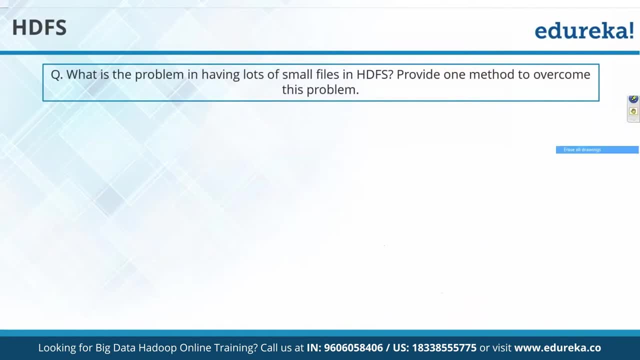 So I hope now everybody should be clear with this question, Though it's a separate question, but actually it's good that you brought it up because that's one of the very famous interview questions, So I thought to cover it up. Now another question: what is the problem in having lot of small files? 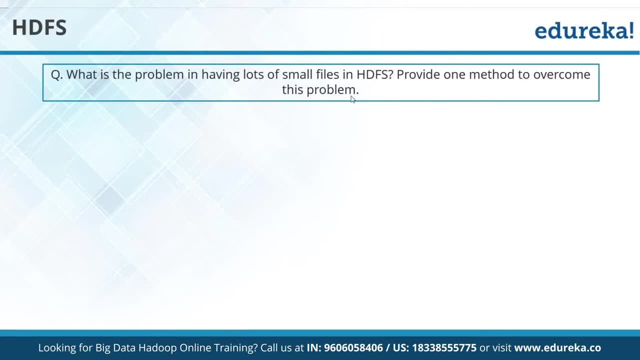 in your database. Please provide one method to overcome this problem. Can I get this answer? Can I get this answer? So what are the problems? that you will have small files in your database And also, can you give me a basically a method to overcome this problem? Change block size, If you. 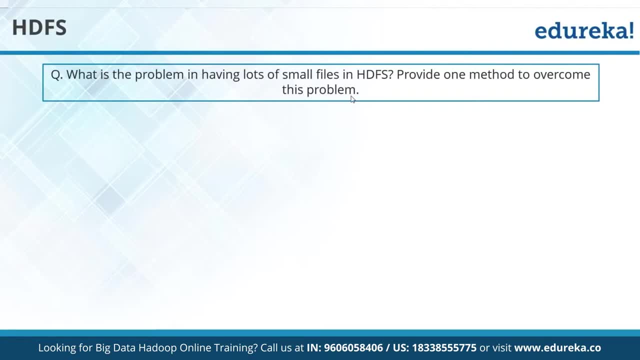 change the block size. I want a better answer. I want a better name. note: memory will be overload. good, good, now you are coming to write track right. ram will run off. yeah, because if you will have small data right, if you will have small files definitely. 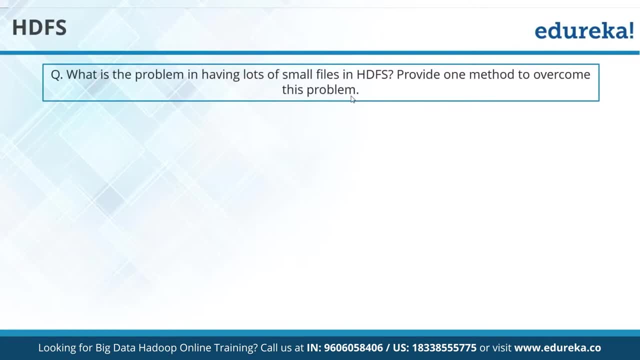 your metadata is going to be kind of too much. right, your metadata entry will be too many and that's how you will be kind of filling up your ram right of your- basically- name note. we just learned that every metadata is stored in the ram of the name note. now, what are the solution for it? 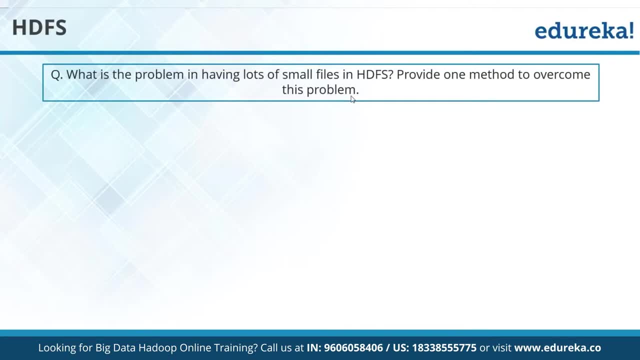 so this is the problem. what is the solution for it? having larger data plot size so that name note will have reasonable metadata to handle? i can take this answer, but i'm expecting a better answer. more map jobs will be used. yes, that's also one of the problem. merge them and tape them. very 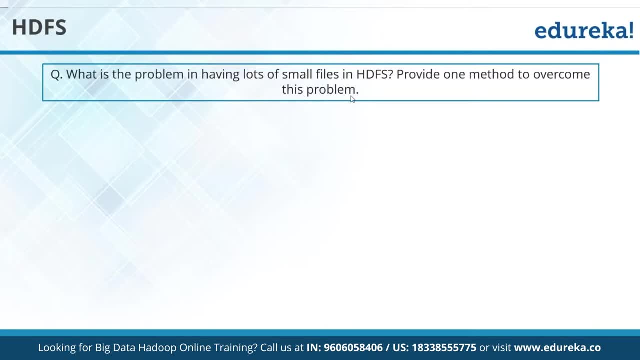 good job, okay. uh, what's your name? basically jo chala jo chala you. i hope that that should not be a real name. i don't know why it's showing me jo chala jo chala. oh, is this your real name? because it's telling me twice: jo chala jo chala. okay, so it should be. 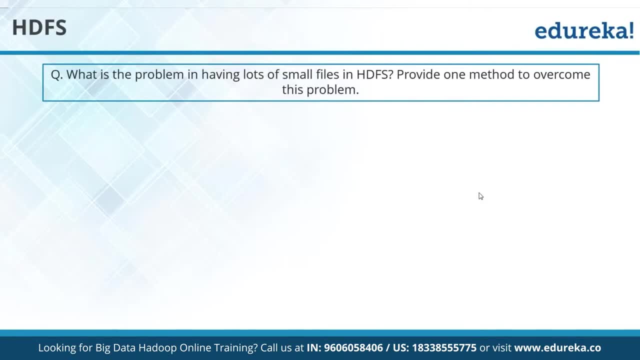 once. right, it should be once. i should call it okay then. fine now, so i don't know. this is offering two times, so that's why i'm filling it here. so increasing block size and lgfs merging the file with same and it's easier to read and write the data. somebody just answered. can you combine? 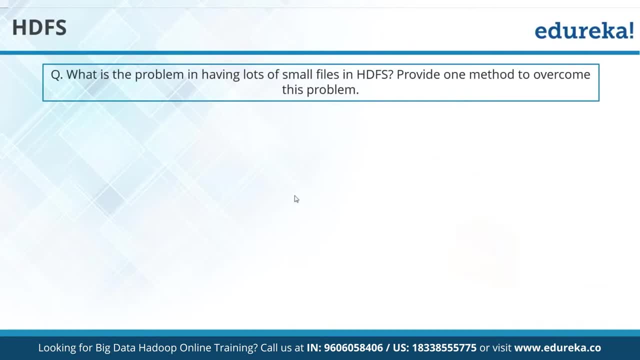 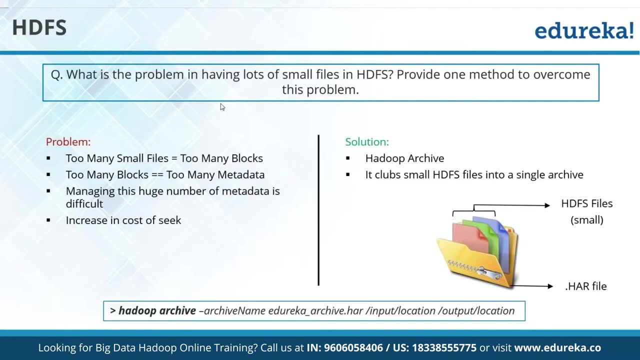 everything. that is the right answer. we can create dot h a r file in your windows. what you do? you create a zip file right for a rar file. similarly, in hadoop also you can do that. you can create a dot h a r file, which is called a hadoop archive, so you can bring all the small files into. 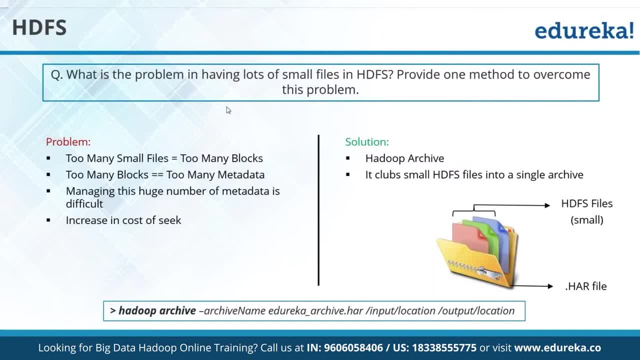 one folder together, kind of zipping it together. now, basically, with that, what's going to happen? it's gonna just keep only one metadata for it. if the metadata entry is going to be reduced, how to do that, this is the command i do: archive now hyphen, archive, name, whatever. 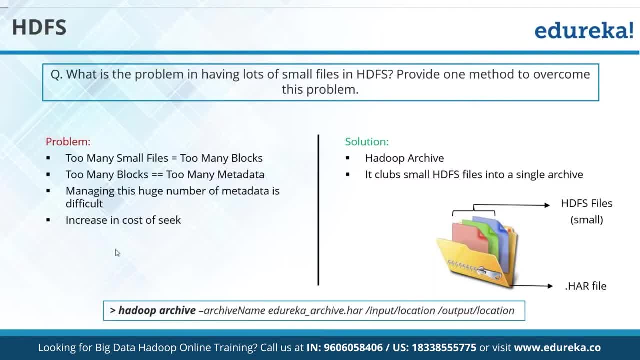 alternative name. you want to give it your input location and output. okay, so basically, this is how you can be with the smaller files as well. better to create a zip file. this is what you do in the real time also. right, when you have multiple files of the same type, you zip them. 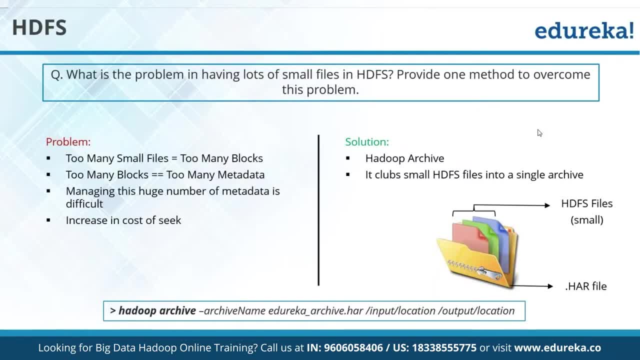 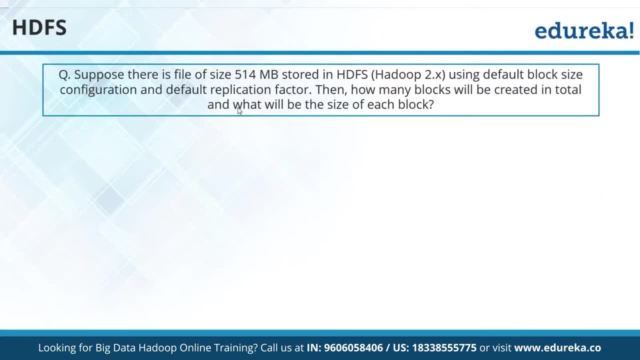 right, just to keep them together. so the same thing you will be doing in hadoop as well. moving further now, another question. this is also a very interesting question and an easy question also. suppose there is a file of size 514 mb stored in hdfs 2.x using default block size configuration. 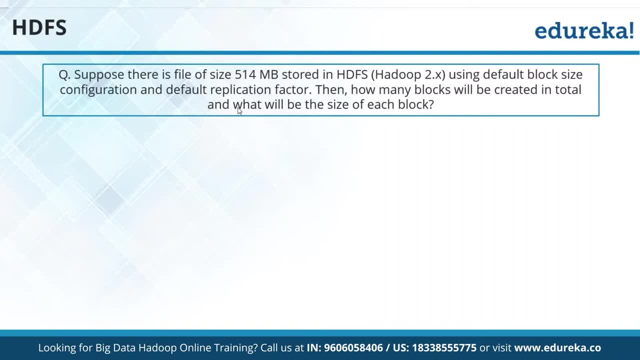 and default replication factor. we did an assignment with image files. i'm on linkedin, okay. okay, now i so using a default block size configuration and default replication factor, then how many blocks will be created in total and what would be the size of this block? okay, before you answer this, 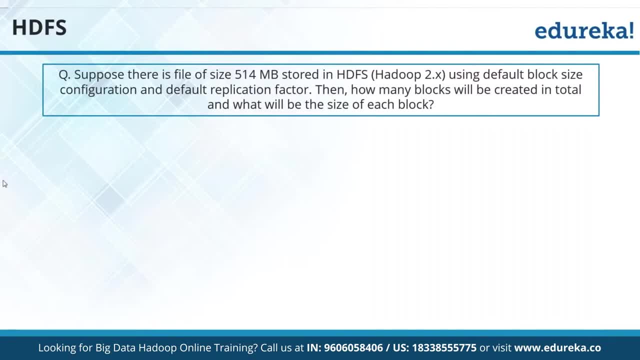 can i get an answer? what is the default replication factor and what is the default block size? if i am talking about hadoop, 2.x, very good, so replication, as everybody said, 3 mb. what is the size? very good, 128 mb. now, it's very easy to answer, can everybody? 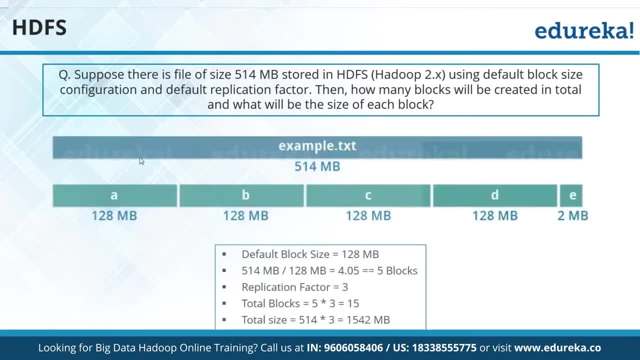 answer how to split this 514 mb of file. how to split this 514 mb of file. it's in front of you. you can do the calculation and give me the answer as well. can i get this answer? very good, 15 block. lot of people have given me basically less. they said five blocks, but don't you think there will? 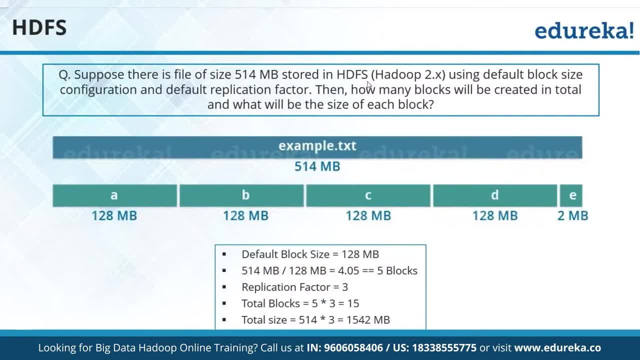 be a replication also of all the blocks. so a lot of people who are giving me this answer of four block is completely wrong. right, because there will be a block of two mb as well. right, if you notice what's gonna happen. this is 128 into four is basically 512. 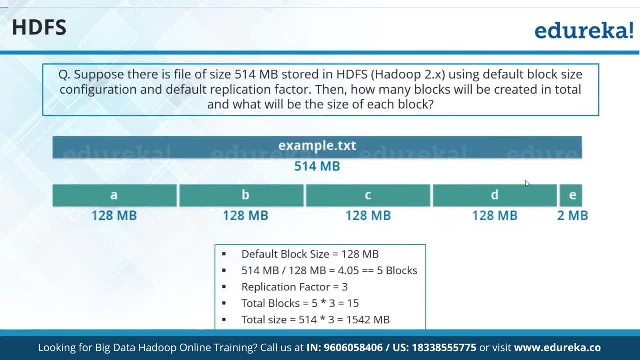 right, there will be two mb blocks. they are going to be five block because the replication is five. now, sorry, replication factor is three, so it's gonna be five into three block. okay, this is how basically we will be calculating. this is very famous interview version. moving further, how to: 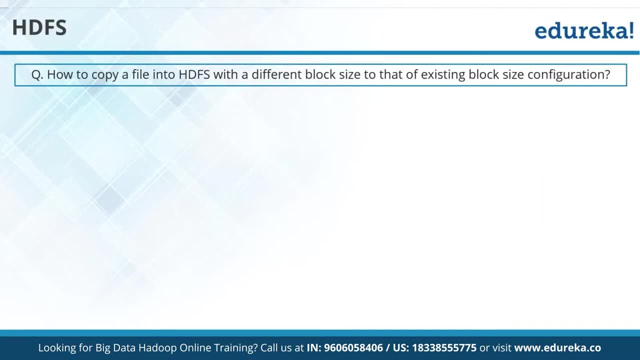 copy a file into hdfs a different block size to that of existing block size configuration. can i get an answer? what basically i'm asking is: let's say you have a block size of 128 mb by default, but when you are copying that data right, when you are doing, let's say, sbfs hyphen. 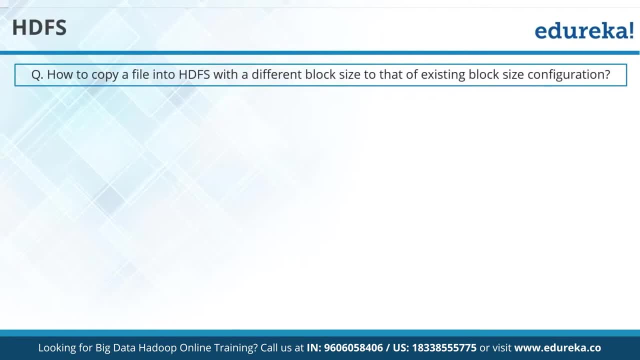 code: sbfs hyphen code. maybe you want to now use the block size of 32 bit, not the default of 128 bit. then what you will do to achieve that? yes, and so i will tell you how to do it right there for you in sbfs better. 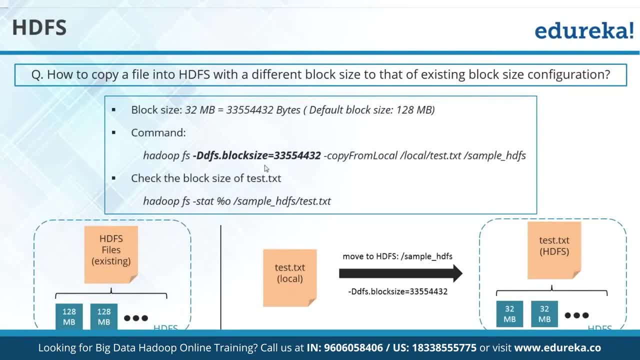 command�Arraydfsblock-size inteiro parameterwhat is that parameter? block size? um, no, can you see this itation? okay, so what you need to do, you need to just define the, basically the bytes, what you want to mention. so 32 bytes is equivalent to this number. okay, 32 byte is equivalent to this number. 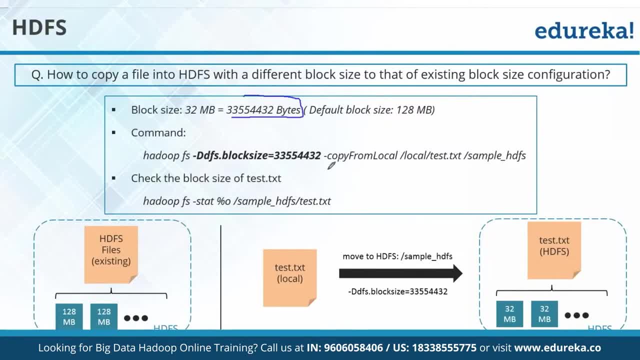 bar doing any command. let's say hyphen put or maybe hyphen copy from local. there you can mention this dfs dot block site and whatever number of bytes you want to mention. so you can mention that. okay, if you want to check the block size, you have another command called a stat. I do fs hyphen stat and you can see all the. 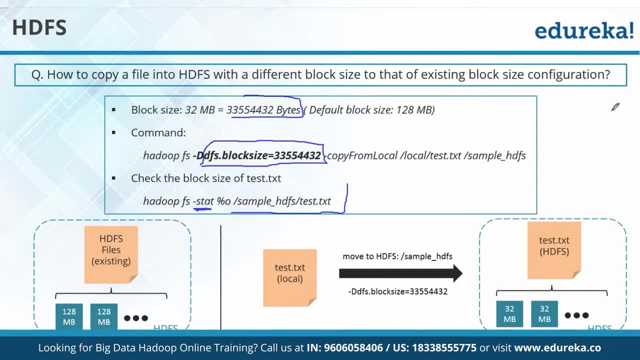 statistics related to it, so it will tell you how many bytes it is basically distributed and everything up. you can basically directly use this fat thing and you will get that output. okay, there's are some times useful in projects and that's a reason. it's a very good intro to question answer, because a 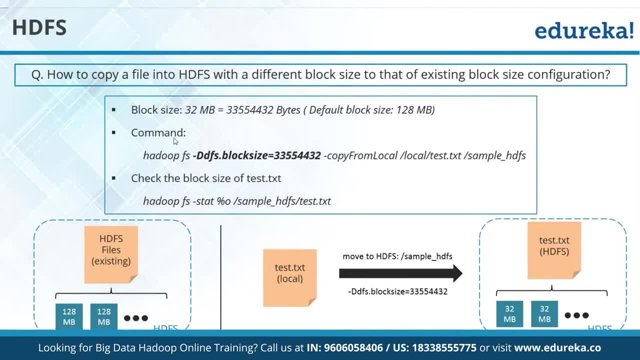 lot of time in the projects you want to. you don't want to use the default size, you want to change some other to some other number. so in that case we will be moving this, because one way is: either you could change everything from the configuration facts, which is part of good idea to do so. better thing is: 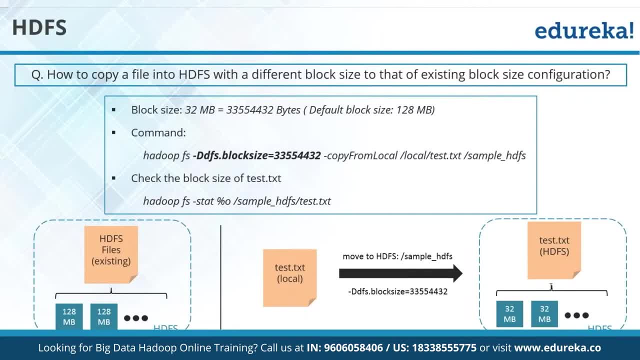 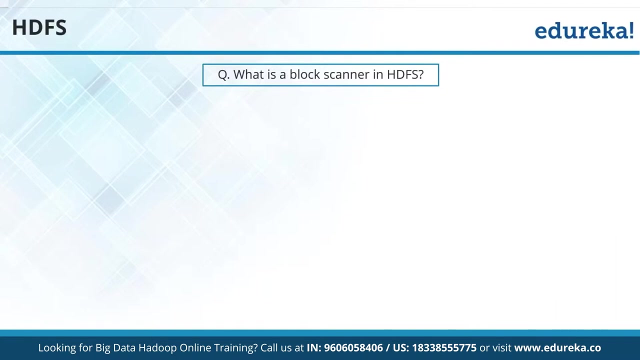 programmatically deal with it, and here you can change it by the usage of dfs dot block size. okay, so it's not block underscore size. i hope you got your answer. what's the mistake you are doing? it should be block size, but you are close now. what is a block scanner in hdfs? can i get this answer? this is a, usually a. 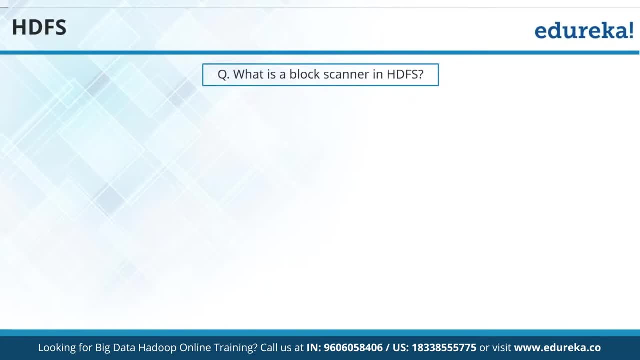 question in your hadoop administration. this: this is basically what your hadoop administrators do, so people who have who have done this hadoop administration classes, can you answer this? i'm expecting this answer basically from you. even others can answer. what is a block scanner in hdfs? 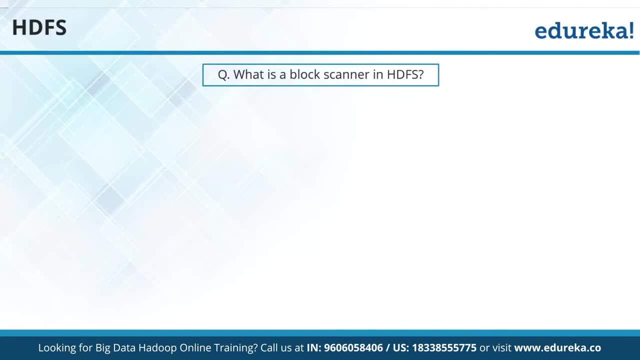 what is a block scanner in hdfs? can i get answer? nobody is answering this. who all have done? administration code or no? administrator hadoop administration. can i get answer? who all have done? i'm not asking you to answer me this part, just to answer me who all have. 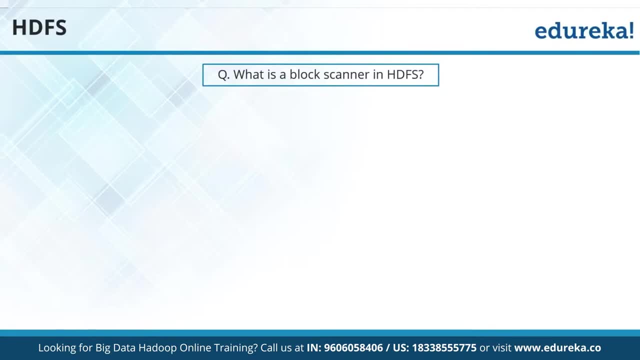 done this hadoop administrator course. initially few people mentioned it that we i have done this administrator course. you must have read about block scanner. okay, let me answer this part. usually in a block scanner, okay. word is answering now, so check if the block has any empty space left. 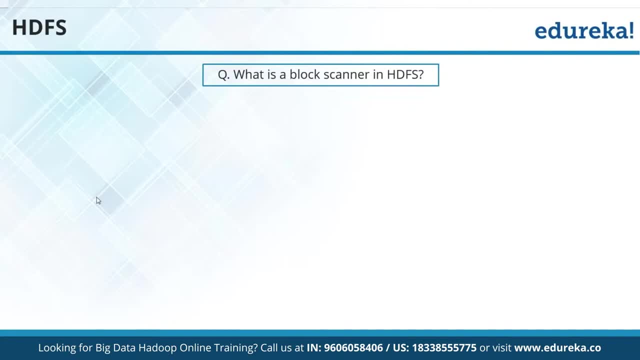 in that block. uh, okay, one of the answer, one of the answer i can take, but not exactly exact answer. it's not very good. uh, scan the block and report the remaining spaces, okay, okay, again, i can take partially this answer, not just the claiming space, but in fact it ensure the integrity. 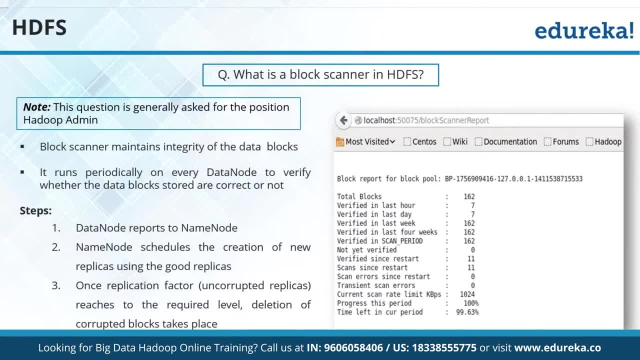 of your data blocks. okay, it basically keep on recruiting every your data node, will keep on reporting to the nameboard and it will keep on checking the integrity of the data block. let's say data block or got kind of corrected right, or maybe the replication replica value become low. 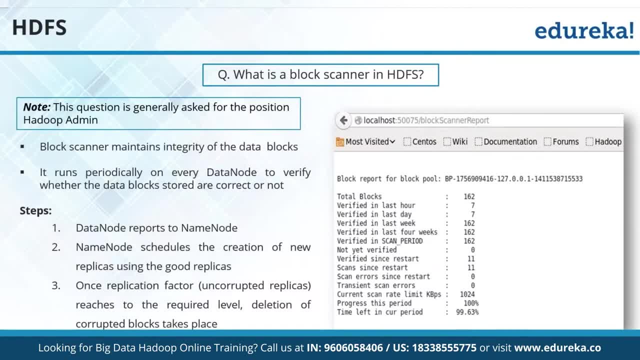 right all those things. it keeps on monitoring and trying to rectify it. okay, so i can basically keep informing the name. but that's the reason this has been usually done by administrators, because they keep on monitoring the health of the data nodes- data block, name node- they're also responsible. 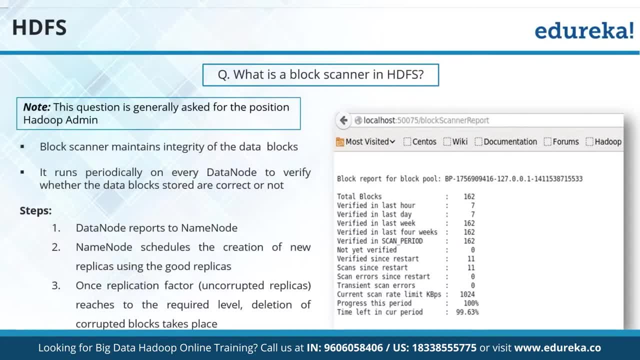 for this work, right? so this is what they keep on doing in order to make sure that they use blocks scanner, basically to do that. okay, there is one more way to check the replication factor. anybody know what is that? there is one more way to check the replication factor. 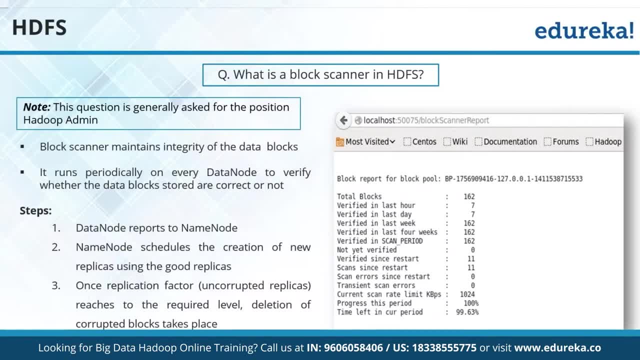 so this is about block scanner. but there is one more way to check the replication factor: environmental file. no heartbeat. no heartbeat will just tell that data node is good or not data node right. i'm talking about, let's say, some file got under replicated. in that case, how? who will kind of 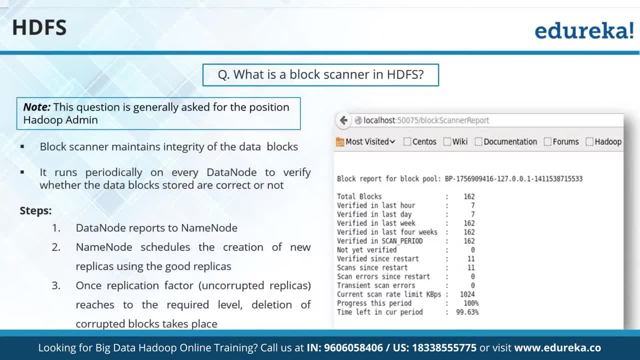 work. let's say, blocks scanner is not there. there is something called as hadoop load balancer. i'm not sure if you have read about that. i do load balancer. that basically ensures that if- uh, if- your data blocks are not up right, if they are under replicated enough, that basically informs that okay. 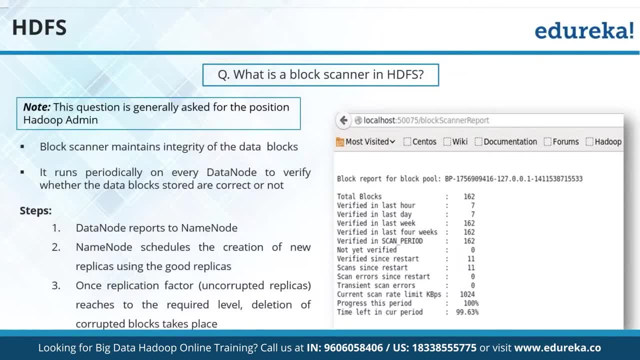 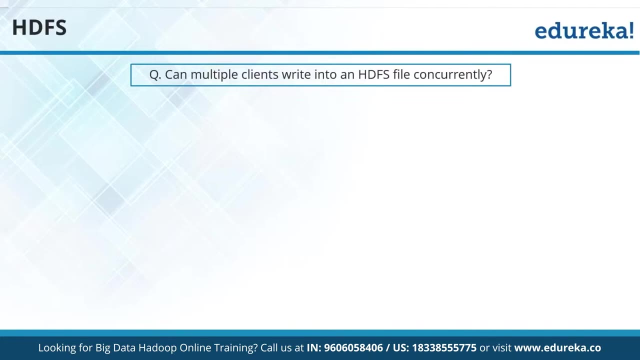 this is under replicated. let me take that out. okay, so this is basically, uh, the way also to check the replication factor of the data node. for the same reason- i'm talking about over replicated or replicated or over replicated crops- can multiple clients write into an hdfs file concurrently? 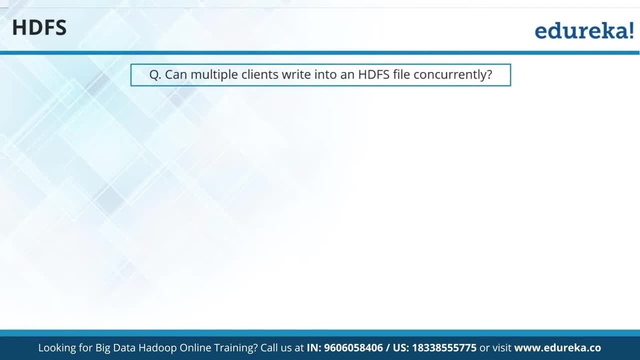 can i get this answer? if somebody asked you this question, can multiple clients write into an hdfs file concurrently interesting? i'm getting one yes, one no, now, two years, one no, could it true? no, two years, god us. yes, okay, multiple write. i am not saying reading, i am saying writing. notice this part. 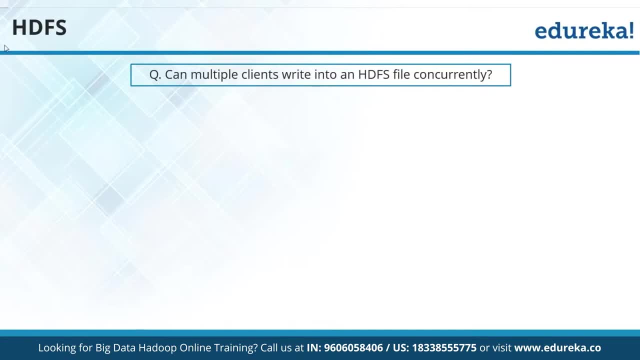 now can you answer? don't you think it will? it will make my file inconsistent. yes, single file i am talking about. don't you think it will make my file inconsistent? if i do that right, it will make my file inconsistent. so it is not allowed. basically, it allowed only one writing and multiple. 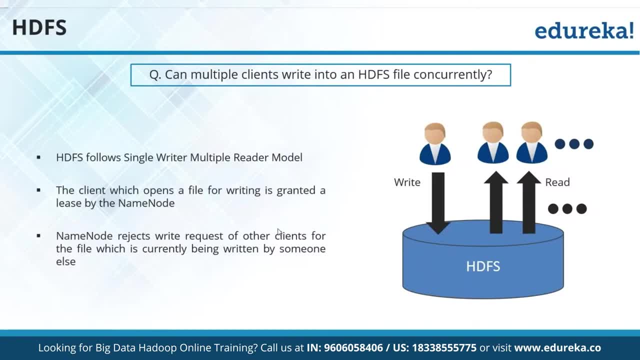 reading stuff. so that's the reason: single file: it will not allow you to basically keep on writing by at the same time by multiple clients. it will not allow you to basically do that for multiple clients at the same time. once one client is writing, it will be kind of file will be kind of. 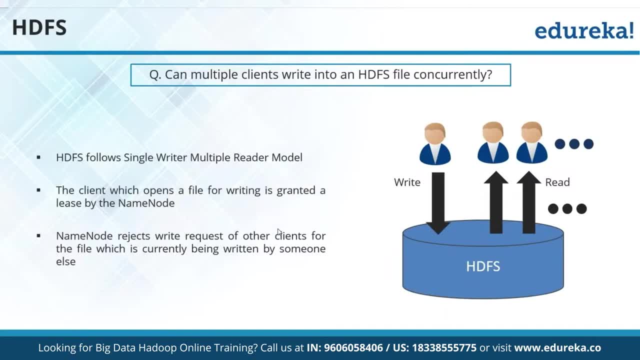 locked for other clients once the client have written. after that only the other clients can write, but everybody can read concurrently. that is one thing which is very important in hadoop. so writing at the same time is not possible concurrently, but reading is possible. that's how hdfs is basically. 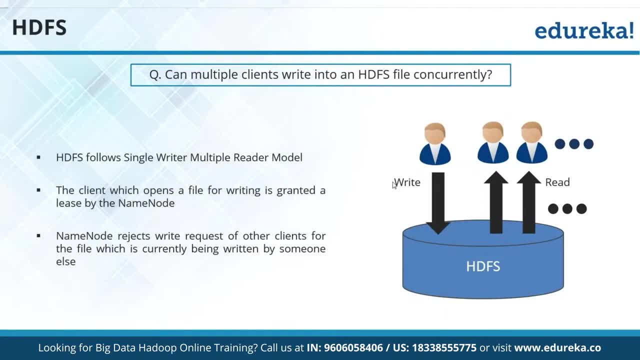 created why they have not allowed multiple rights together if at the same time, because if they do, it can make the file inconsistent. that will be a big trouble and that's the reason they do not allow you to do concurrent right, because this is distributed system. if multiple clients will. 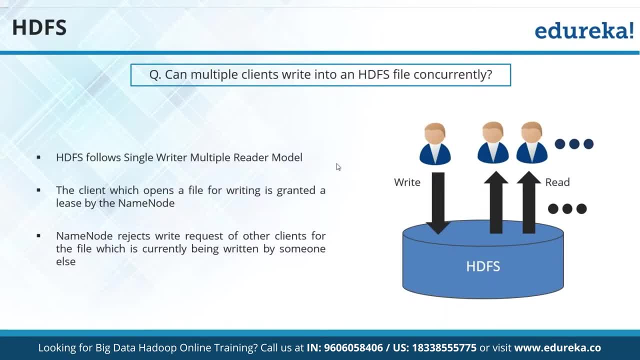 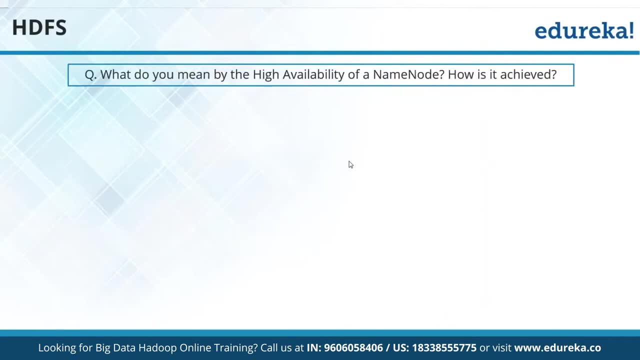 write on the same file now maybe somebody can overwrite my change right. so that's the reason they will not allow you to do. okay, this is by architecture. another question: what do you mean by high availability of name node and how it is achieved? can i get this answer: how this is achieved and what do you understand by high availability of? 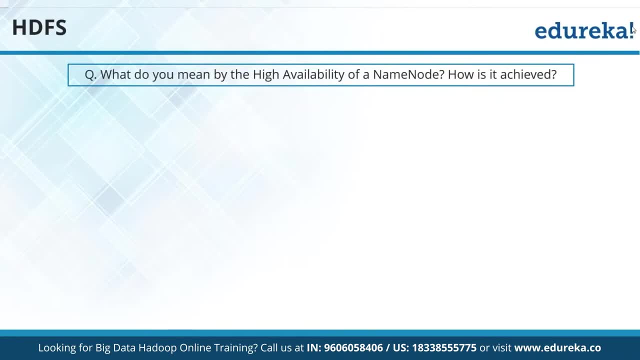 the name node. in fact, i already answered this in boss example. you can answer me this, but not replication: a rack, awareness, name node, fields of passions. they will be stand there. so, okay, two people are giving right answer now: active and passive number. what basically happens in this case is: so, let's say, if there are two, internet may show you the slide itself we have. 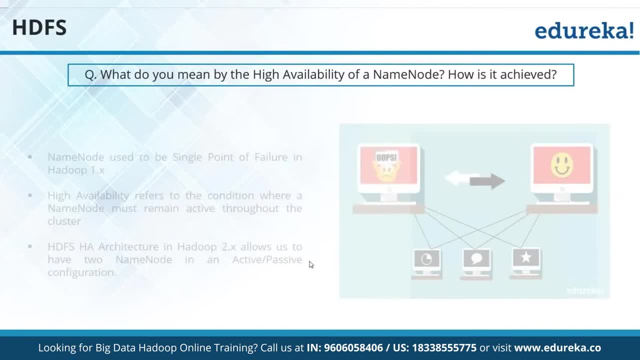 drawn it properly. see the file. there will be two name nodes: one will be active name node and one will be passive member. so what happens is, let's say, this is my uh active name node, which is running okay, and what these data nodes are there at uh, who are reporting to the active member now? 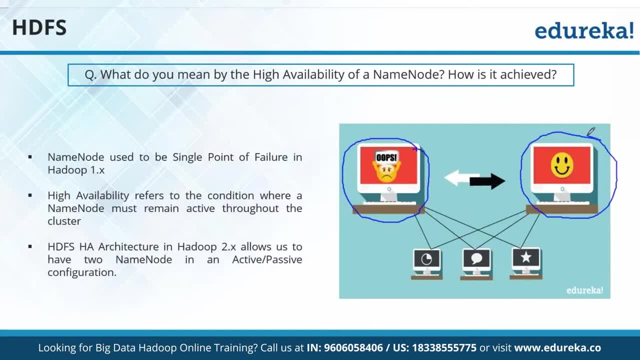 we also create a passive member. now, this passive name node also, these data nodes will be reporting. this passive name node will not be doing anything, but it will just keep on collecting the data from your data nodes. okay, that is what the role of passive name node would be now, as soon as this. 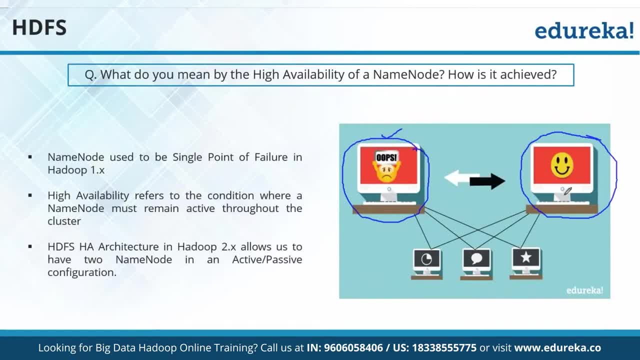 because this now is reading right. so it knows the status of data node. it knows that where the blocks are being written, everything it has the information. now, suddenly, if this machine is down, in that case my passive name node will ensure it will immediately start acting like a backup. 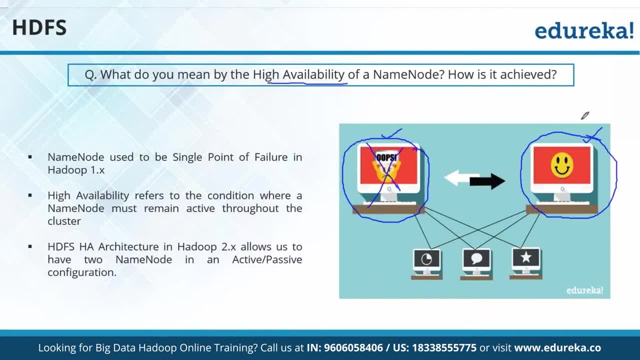 and that is how it is ensuring high availability. you are not going to lose your cluster time, so basically, the downtime will not be there. immediately, your passive name node will start acting like an active member. okay, so this is how, basically, the hadoop is ensuring high availability. 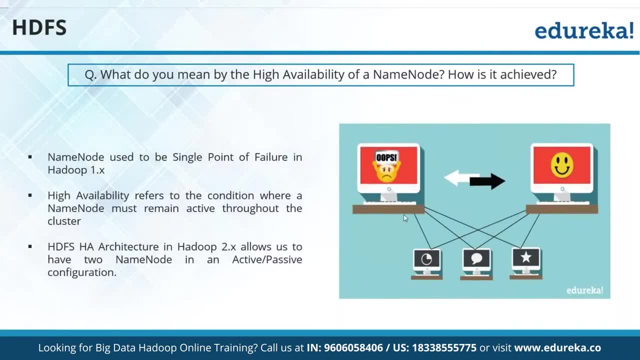 this is a very famous interview question: passive and secondary name. good question: difference between passing name, node and secondary number. secondary name- what we used to use in hadoop 1.x, now secondary name- what used to happen was secondary number. you can say it's just like a snapshot of 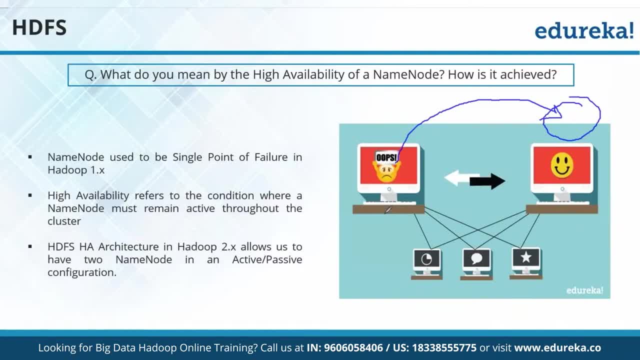 this machine means you're just copying the data, copying the data to other machine. but if my active name node is down, if my main name node is down, in that case my secondary name node will not start acting like a backup. it will only keep the data, but it will not start acting. 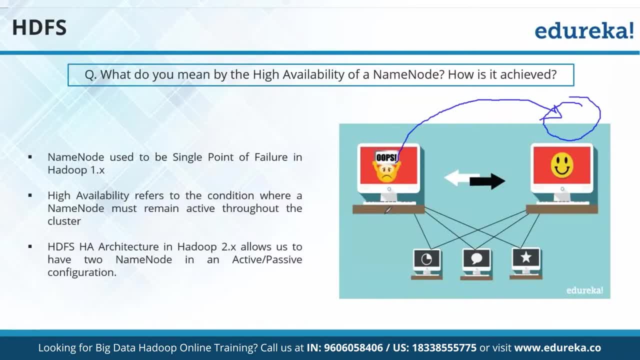 immediately like a name node. it will just keep the data. you have to physically, manually, uh kind of, bring the name node up, copy the data from the secondary name to primary name node and then start working on it. but in passive name node, yes, so it's kind of a queue or human intervention, right? 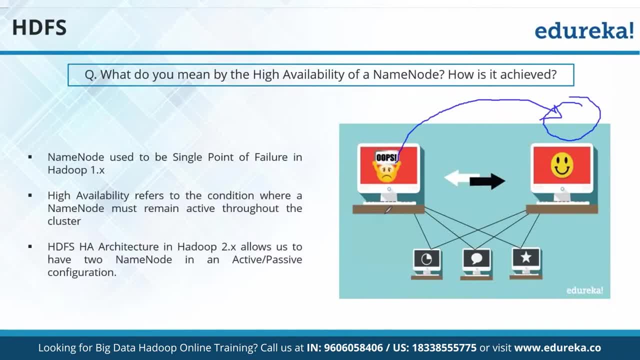 manual intervention is required here and there will be a downtime. there will be a downtime here, but when it comes to the active and passive member, passive name node is going to ensure that it is not only collecting the data metadata but it, as soon as active name node is down, passing name. 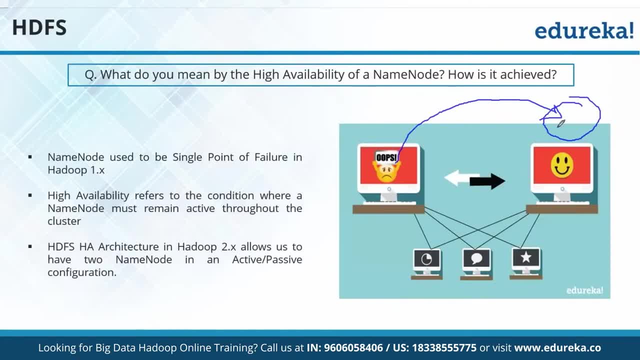 node start acting like a active name node, clear on this difference. but now no one you have at this question right, clear about this question answer and the difference should be very clear to you wait, so let's move further. okay, so we have few more questions now. uh, so this is for map reduce side. so let's do one thing. 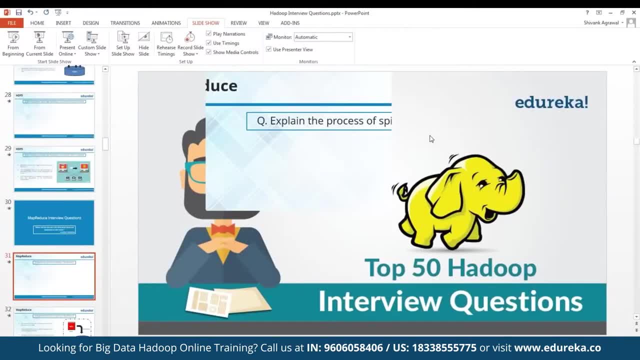 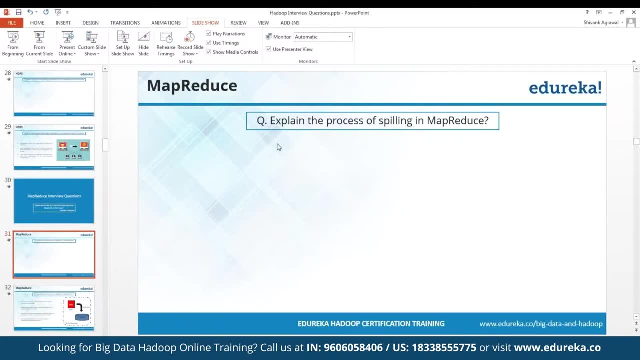 friends, let's take a five minute break. let's take a five minute break and we will start with map produce questions, okay. uh, i'm not sure, maybe somebody will answer. you just need a, uh sip of water or so. so just give me five minutes. they will take a. okay, you want 10 minutes? 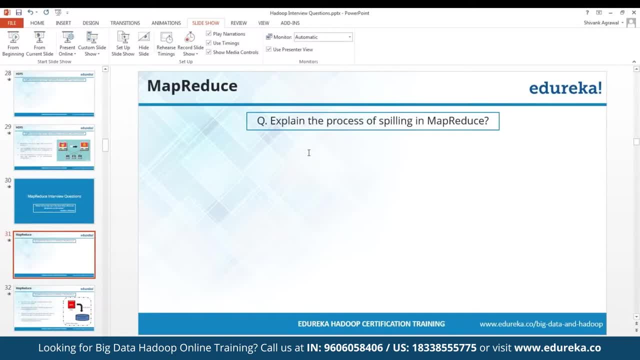 uhthis is just basically a two to three hour session, so we don't want to make it too much. let's make it a seven week. seven to eight minutes. with that work. let's come up with our embedded kind of solutions. so let's come back by, maybe by 10: 3. okay, we will start. we have a water break. also, we will come back. 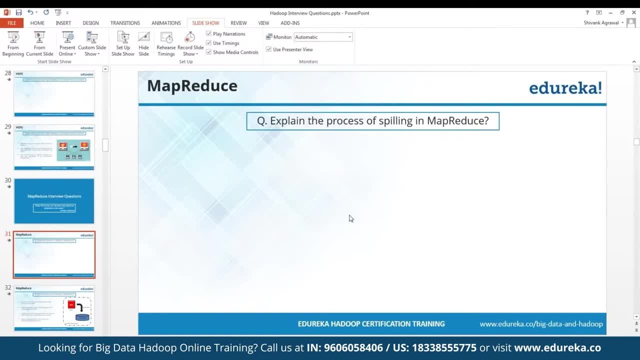 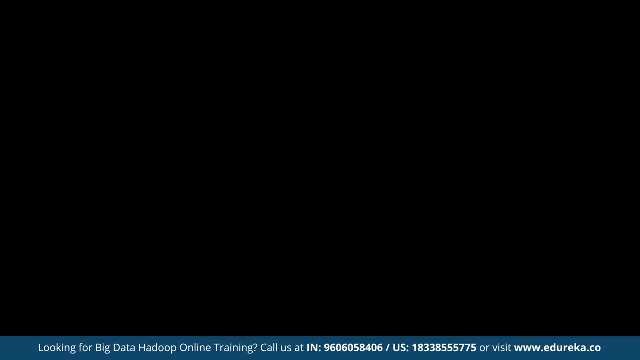 to back produce. then we have five, we have school for that, so let's come everybody. please be back by 10-3. exactly, I'm going to start by 10-3, okay. so, guys, everybody is back now. everybody back. Namin, you should be able to hear me now. okay, looks like he is being starting, okay. 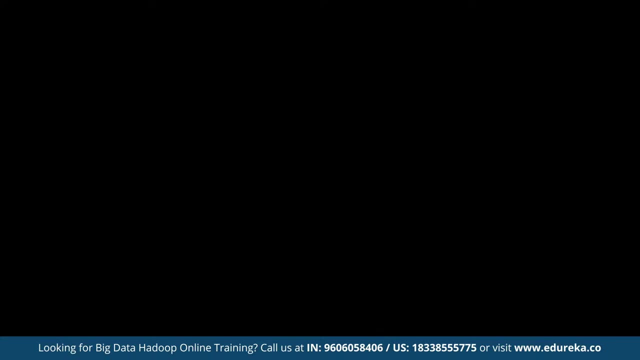 fine, so now we are going to start. so, basically, now we are going to start with back produce topic. okay, now in the- yeah, I'm not sure, I'm not sure. I'm just going to share that. just give me a second. it takes almost two seconds to basically. 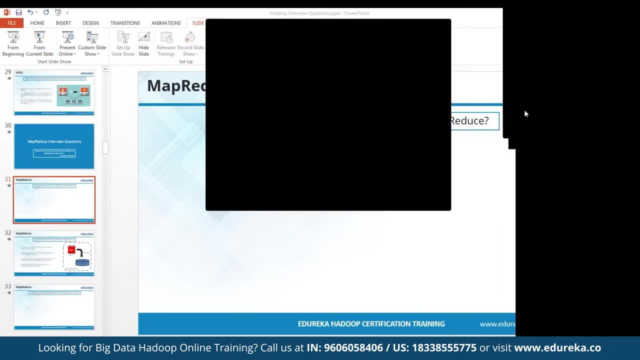 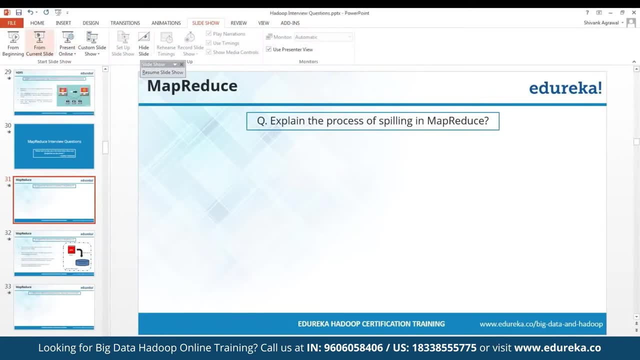 come to this now. I hope it should be showing to you, okay? meanwhile, I have talked with the Edureka team and they have informed me that you all will be receiving this video recording in a day or two. okay, since there that was a question from lot of people, will we be getting all this? 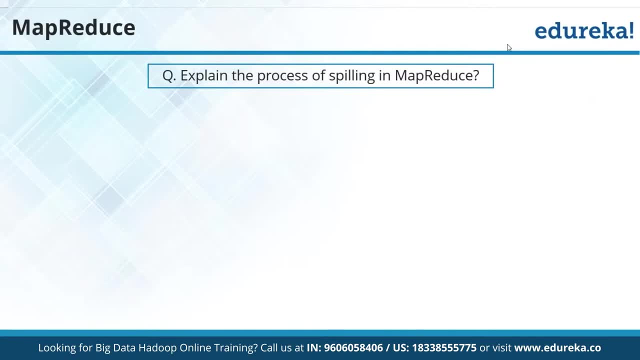 video recording. so now. so you will be getting this video recording on your email ID in a day or two, so all these things will be there with you. so I think that will be a quick review for you, if you want to take a look at any moment. 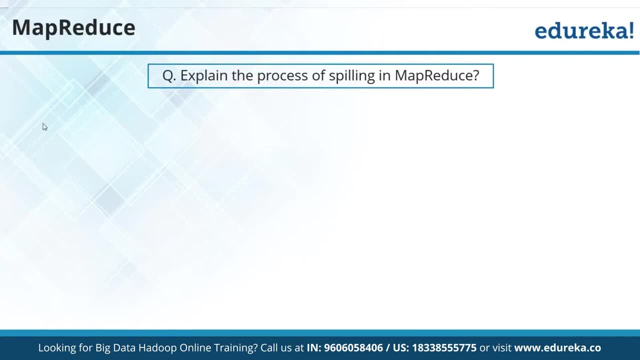 now question for you: can you explain me the process of spilling in mass produce? this is an interesting question in fact. think from a perspective of where mapper keeps the output and from that you can basically make out what is this filling. I give you a bigger thin possibility, so 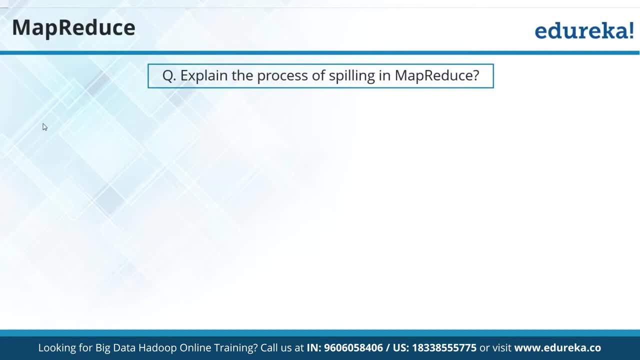 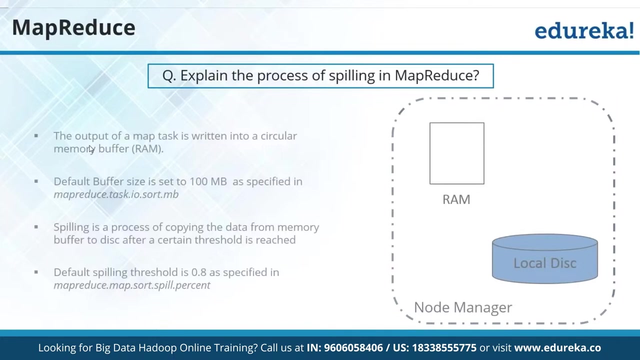 can you give me this answer? can you explain the process of spilling in mass produce spills to temp folder LFS, of when it spills and from where it spills? can I get this answer? mapper, if very good. what usually happens is the output of your mapper task. it goes to your wrap. now what basically gonna happen? they have kept. 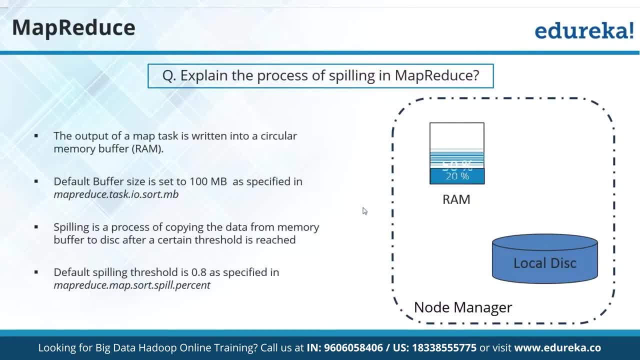 or specific size of that thing. so let's say they keep. let's say just hundred and b, now hundred MB of data will be kept. let's say in that, but they have, they will be keeping a threshold so it slowly keep on filling up, slowly keep on filling a. 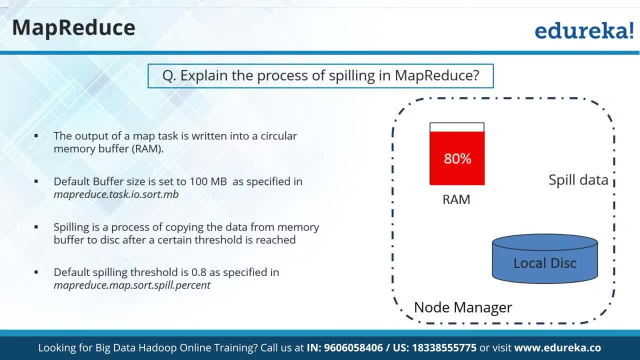 data will be kept, but they will be keeping a threshold. so if you slowly keep on filling up, slowly keep on filling up, then what will happen? as soon as it will reach a threshold, let's say 80 percent of that ram of 100 mb split, it will start filling that output to the local disk. notice here i am not saying hdss. 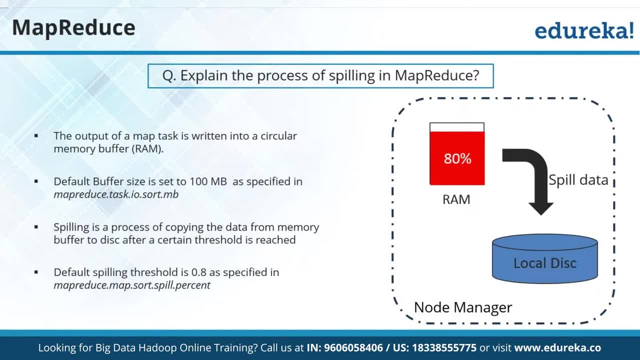 i am saying local disk okay, to local disk only. we will be keeping this data. local disk means your c drive, d drive, wherever you want to keep up. so this is how they have designed it. so as soon as the mapper output in the memory reached to a threshold limit, it starts filling that. 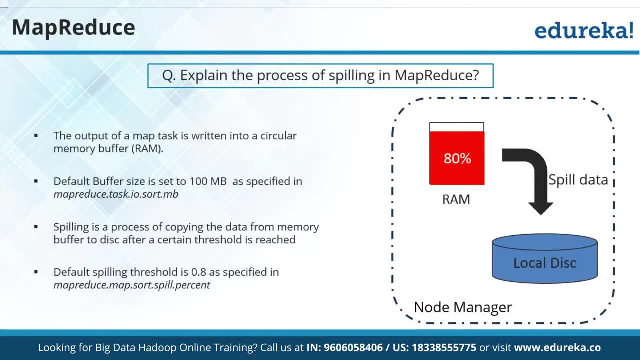 mapper data to your local disk and this phase is called as filling phase in map. okay, so this question is also asked and this shows basically the internal working of your map. okay, so basically this is how, internally, your map produce work. so this is how it is filling the data. once it's filling, it will again come down and you can keep. 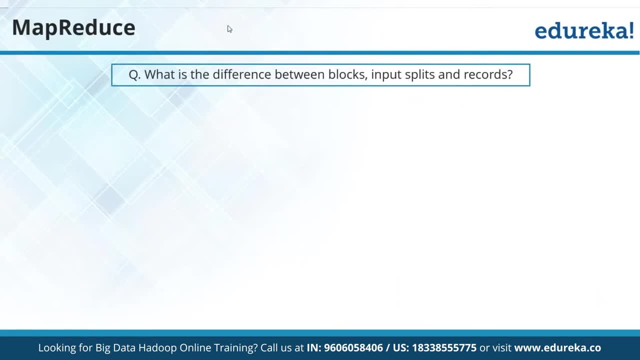 more and more data in it, which links me to another question. can you explain me the difference between block, input splits and record? this is a very famous interview question. can anybody answer me quickly? what is the difference between blocks, input split and records? what is the difference between b3. 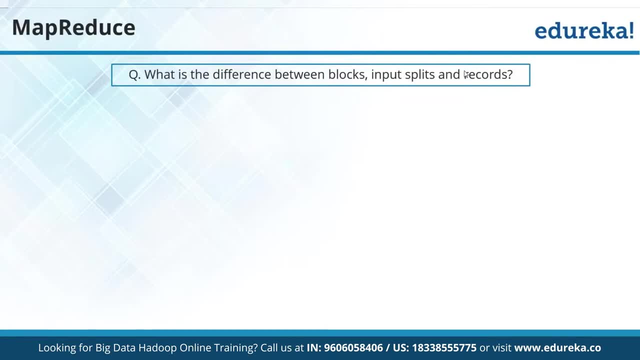 thanks. this is a very important question. if you have done this map reduce part, then you must be knowing this part. difference between blocks, input split and records. very good, jyoti. so jyoti is answering: record is a single line of data, right, very good. kanal is saying: block is hard, cut of data, just 128 mb. very good. 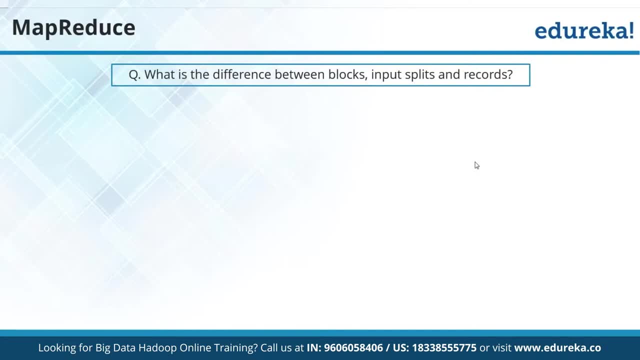 block is equal to 128 mb. if record is 130 mb, input split will happen. very good, block is based on block size, input split: make sure that the line is not broken. so it makes sense: record is single line. block is set by sdfs. input plate is logically split. very good, very good. so what usually happens? 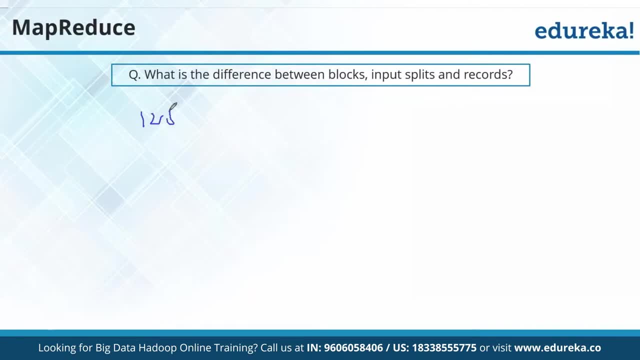 right. so let's say: when we talk about block, so let's say you have default spaces 128 mb, so that will be called as a physical block. so let's say you have default spaces 128 mb, so that will be called as a physical block. okay, when we talk about input split- right, so let's say, if your data 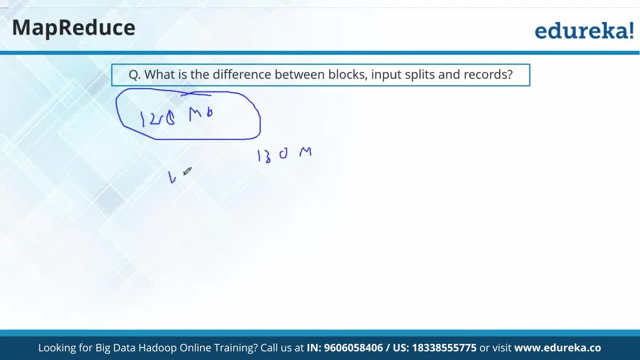 is of 135 now. in that case don't you think it makes us to have a logical split of 130 mb here? so that will be your input. and record is, when you do map, reduce programming right. when you do map with this programming, how your mapper take the data. it takes line by line, right? 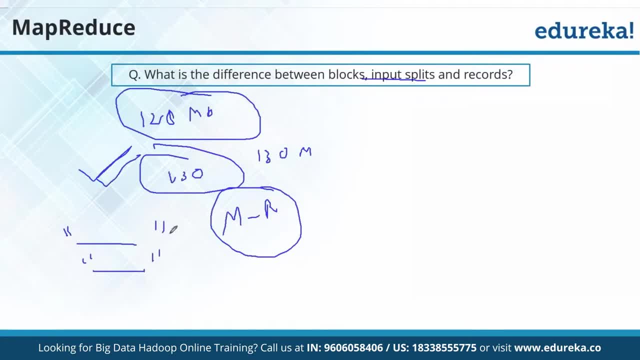 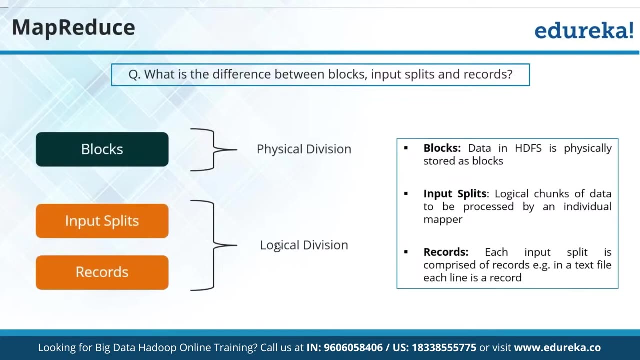 it takes line by line, that line is called record. so one line of data which it picks up in the mapper phase is called your record. okay, very, very famous question on this part. so you can say: block is a physical division by logical division are called your input splits and records. okay, because the logical division is what your mac produce program do. 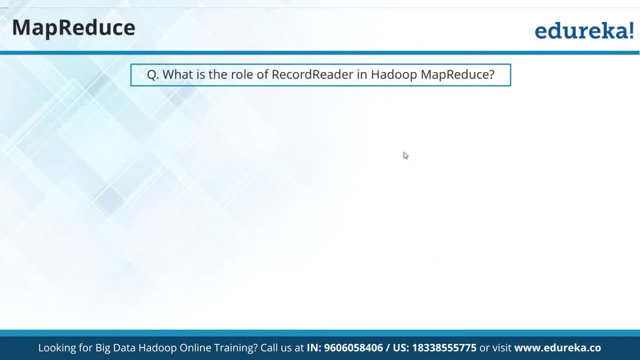 which brings me to another question again relate to map reduce. what is the role of record reader in adobe map reduce? what is the role of record reader in adobe map reduce? make sure to read the complete record. no, no, how. that is how mapper reads a record. 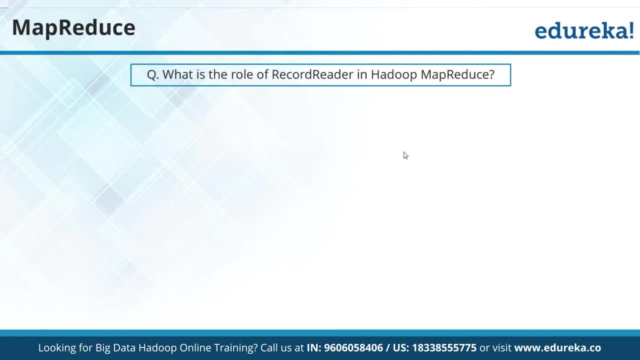 good, but digambar, can you give be a little more explicit? you are coming close to the answer. can i get more answer? also, digambar, can you just be a little more explicit? that is how mapper reader and record. you're coming close. what about others? what is record? 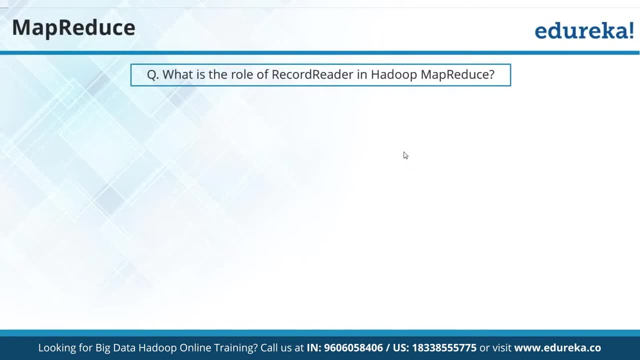 record is single line. we have read, just understood it. so what should be record reader parsing that single line? very good one, right? so don't you think that single write what you are reading and how mapper convert your data? it converts into key value pair, right, so it initially takes an input. 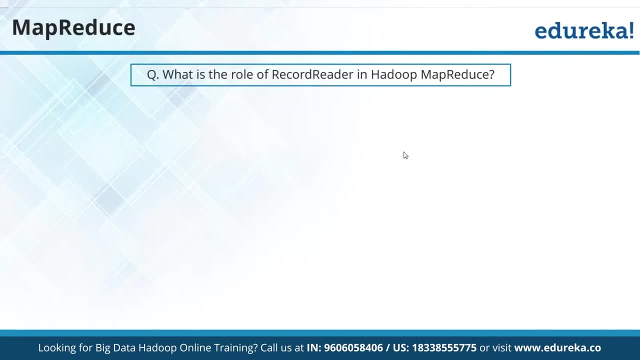 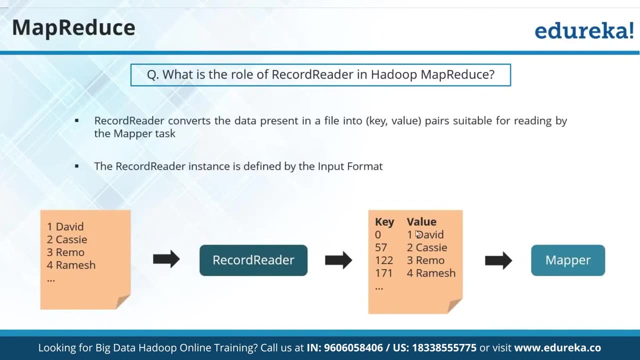 as a key value pair. so when that conversion is happening, that is done basically by record reader. look at this, see. let's say this is the data. it will be getting converted to key value pair where key is called your offset and value is first line right, or second line or third line, right. so this is done by record reader, okay. 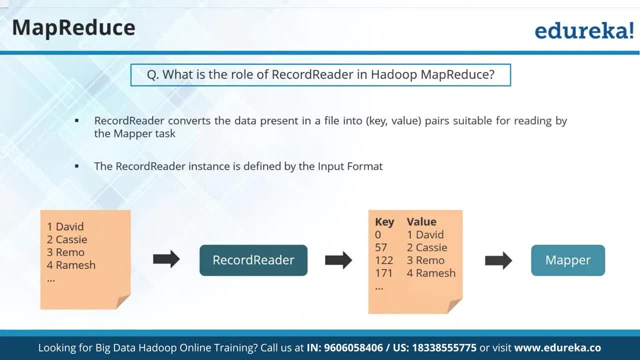 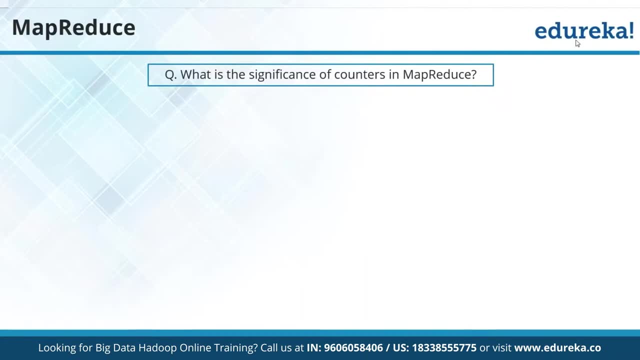 but this is what record reader do. now what is the significance of counters in map? reduce mapper is significance of counters in mappers? give statistics of data. counters will be done in name node. okay, counters to validate the data. read to calculate that because good, not just bad record people, it can do even other things right. 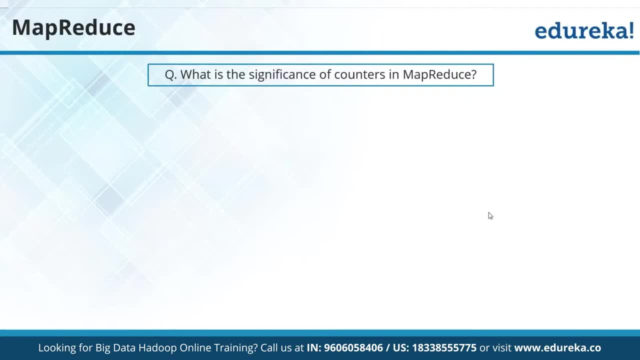 if this bad record is just one example, right, it just is one example you can do. so what it do is it just give one example. it will do a bad record, so what? what it do is it gives one example. so what it is. it helps you to identify the statistics right now. basically, it gives you the statistics about 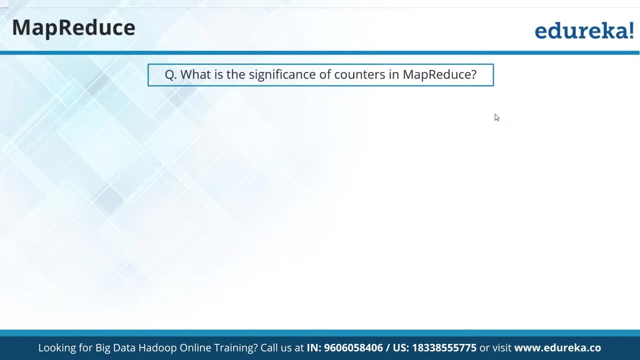 some operation, what you want to do, you can print it in the console also. i i believe that if you have done this hadoop course, you must have seen one code for your counters, right where you must be doing some sort of operations, and you might be printing it on your console window. now how you 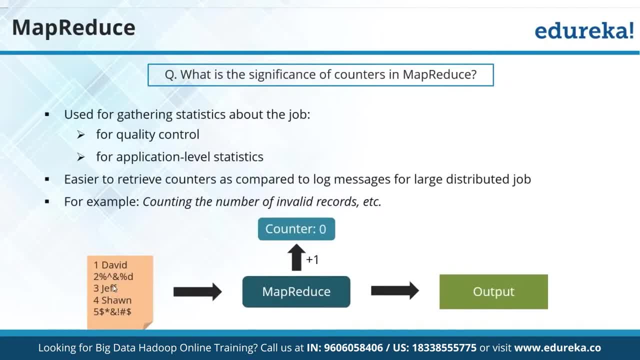 will be doing all that. so what you will do? let's say we are applying counters on this example and in this example, as i think somebody just mentioned, for the kind of reading the bad data. this example actually bring up the same thing, but it can do even other things. i will tell you what are the 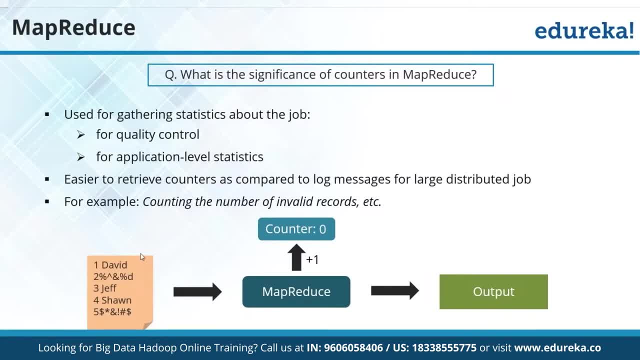 things now. but let's take this example. let's say we want to find out what all bad data i have in this. so let's say it is reading. it is reading david, all good, no problem. counter will remain as zero. then what it did? it basically just gave the value as zero. it reads to the second line. now this: 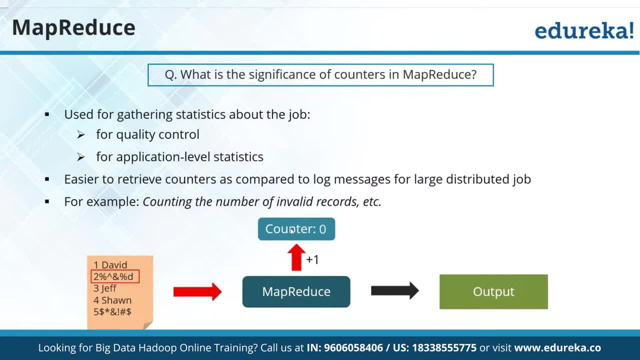 value move up now. basically, this was a bad data. i read it, i passed the statistics. now counter value became one. it reads to: jeff if the value stays as one because this is a good data. now sean again. the value remains the same. now, as soon as it reads the last line of bad data, it will again increase this. 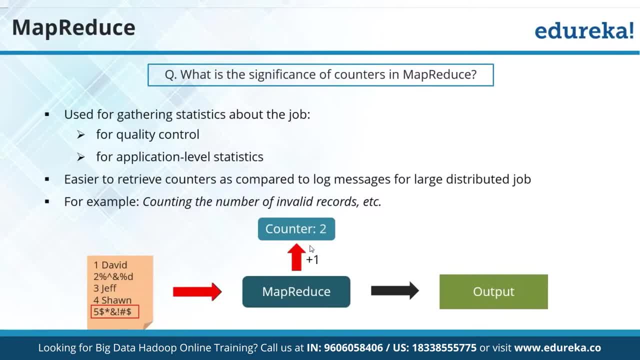 counter and will return that i have two bad line of code. but does that mean we can only do this operation on this? no, maybe i I can have an example where, let's say, I have data of which is, let's say, of timestamp, timestamp, subject: okay, I want to print in this time, so timestamp I can convert to date type, right. 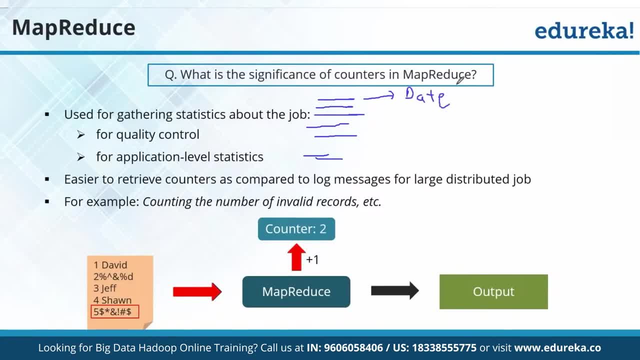 in my program I can convert it to date type. now, when I convert to date type maybe I have months being defined right, because in in date I have months. now maybe I want to find out or want to calculate the statistics that in among this timestamp how many times January is occurring. 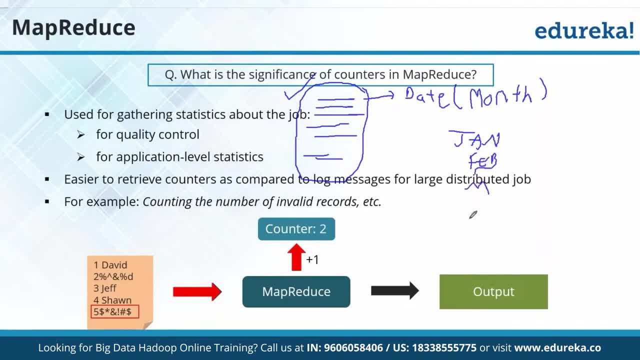 how many times February is occurring, how many times March, April, and all are occurring. let's say, I want to identify all the statistics. I can do that with the help of counters very easily. okay, so this is the process of your counters now moving further. why the output of? 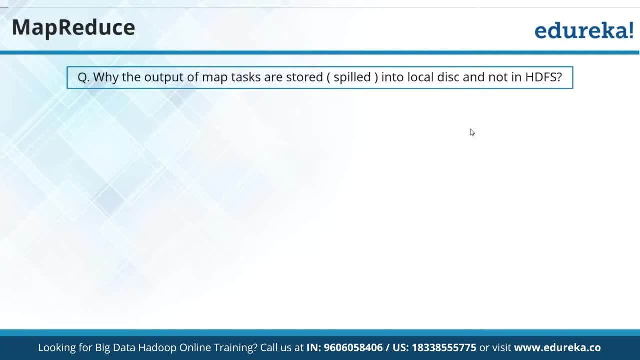 maths is not good math. pass for spilt into the local disk and not in HADSS. good question now. can you answer me this? remember we talked about? we talked about. yes, we have just discussed that question, right, so we have just seen spilling. we have seen spilling. now how can we assess counters there? 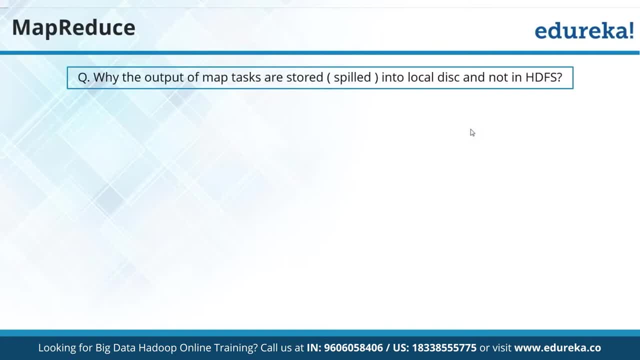 are basically libraries available for that. there are classes available. get counters, that is the member function to get that. this is how basically we'll be assessing it. so counter is the class in which we have member functions, predefined functions. using that, you can assess that because it's an intermediate output. okay, intermediate output, that's fine, but why we? 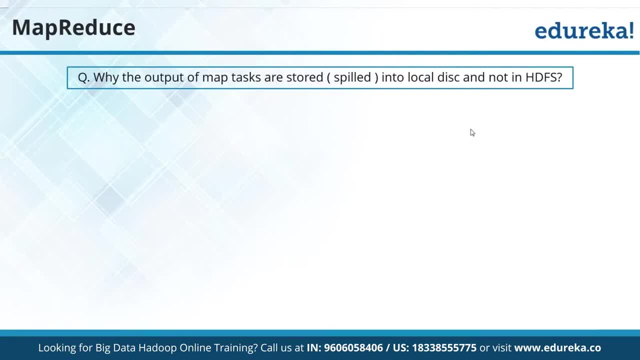 are not keeping an HDFS. that that's my question. when I can keep intermediate output in HDFS, very good, very good Ramya, very good Narasimha. so basically, if you notice what happens if you keep in HDFS, right, remember there is a replication of the function. so if you keep in HDFS, then you can. 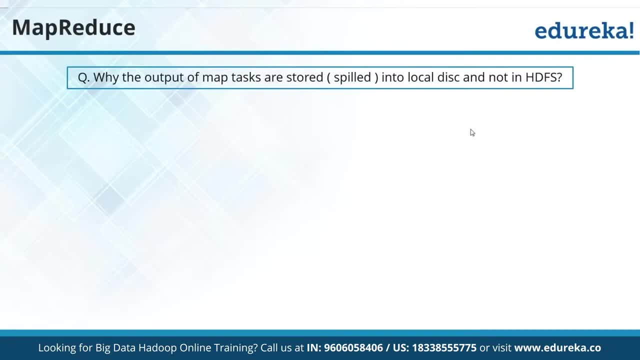 keep in HADSS, right. so, basically, if you notice what happens if you keep in HDFS, right, remember there is a replication factor, right? that replication factor will do what: it will increase the number of output blocks. do you think it makes sense to increase the replication for your mapper output? definitely, 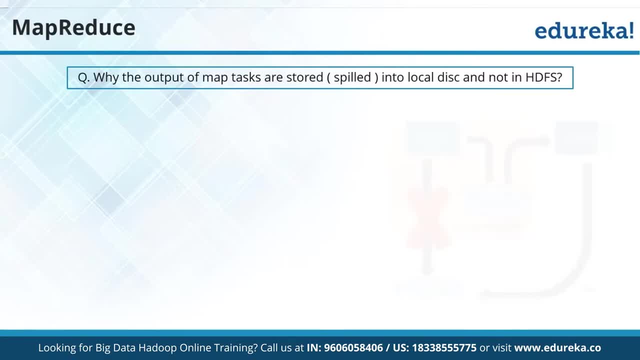 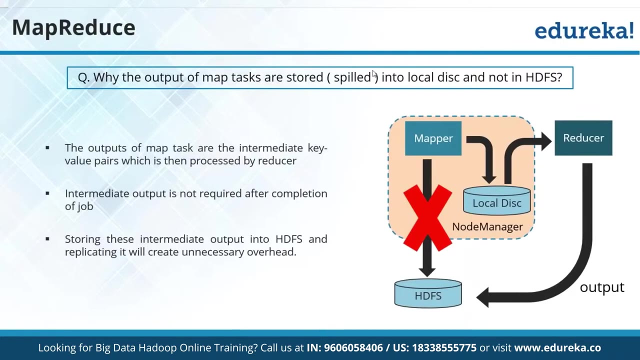 a big no right. so that's the reason we will be keeping in your local file system. we will not keep in HDFS. otherwise HDFS will replicate even mapper output, which we don't want to happen to do. so that's the reason we will stop that. so we will be keeping in the local disk, not in HDFS. 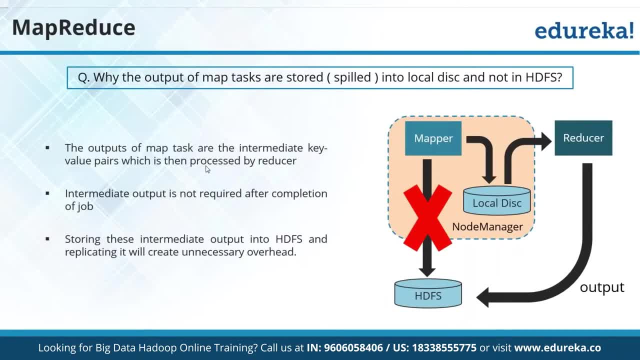 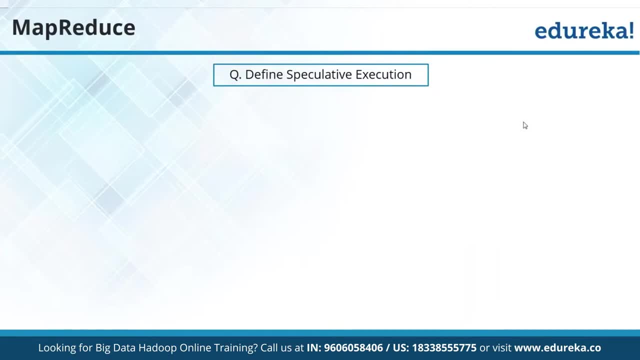 in order to avoid basically the replication, which brings me to another question: can you define this speculative execution? can you define this speculative execution? can I get this answer? can we define speculative execution? it prioritize only some tasks coming close, but not exactly right, Namashree, if a job in a node is taking much time, very good, very good, very good. so this is. 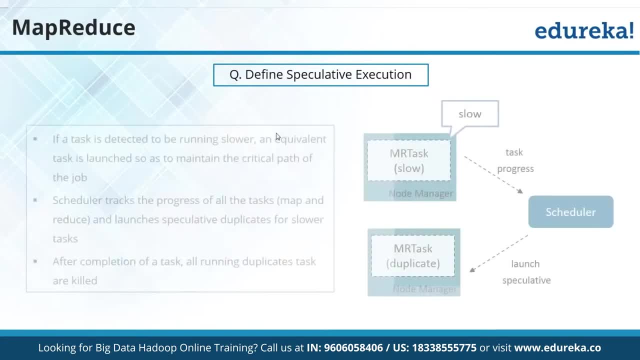 what happens in speculative execution. let's say, if any of your task is running very slow, in that case your speculator- there will be a scheduler which will basically start a duplicate task of it. it will start running a duplicated task for it to ensure that, basically, that duplicate task runs faster and once it will finish, it will kill all the. 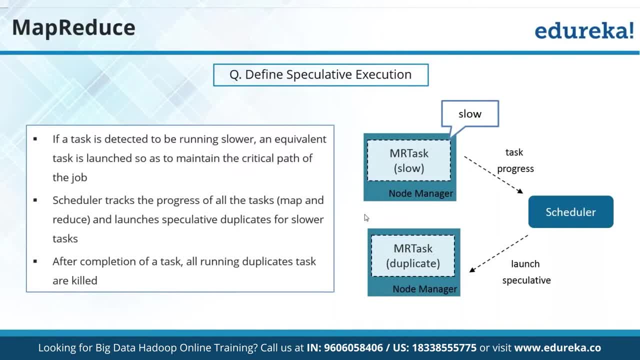 duplicate tasks. so it is just kind of making sure that, because it can happen, right, maybe your task is waiting due to some resource, it got blocked due to any reason, so in that case it will start immediately a duplicate task and making sure that your job finished quickly. okay, so this is the part of your speculative. 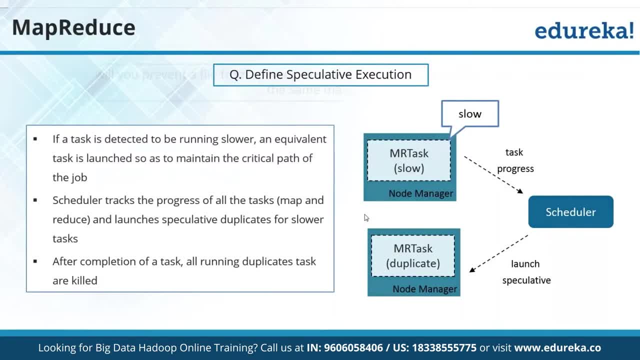 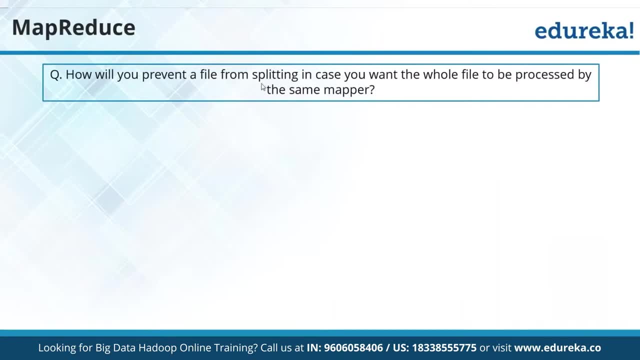 execution, which brings me another question. question is: how will you prevent yarn? very good, very good. how will you prevent a file from splitting, in case you want the whole file to be processed by same mapper? how you will prevent a file from splitting, in case you want the whole file to be processed by? 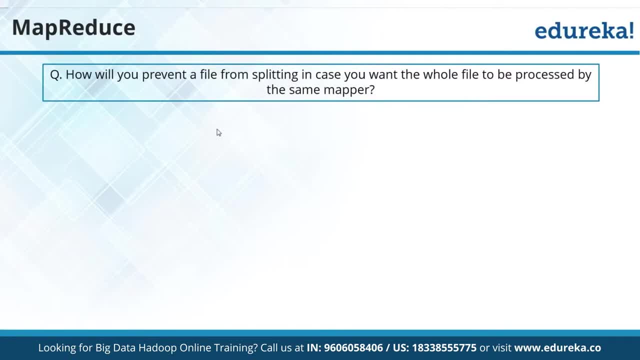 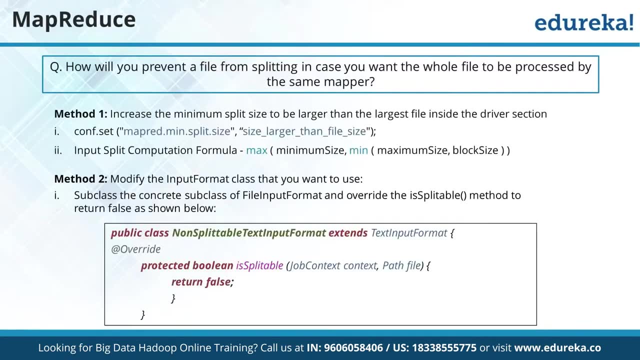 same mapper. I want my file to be now basically to be used by the same mapper, not combined. not combined with the number. can I get some more answers? it's easy. can you see this part? so what we can do here is, first of all, we can increase the minimum. 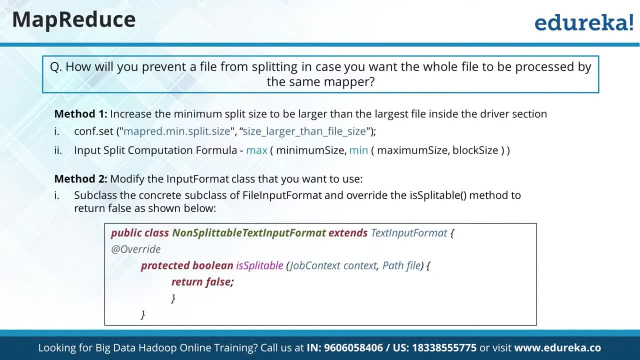 number of split size, which should now make it larger than your last aspect. this operation is itself good enough to make this case true. right, because if we increase the size itself, it will be all good. but there is one more thing which you can do after that is: this is method two. basically, in method one, you can just 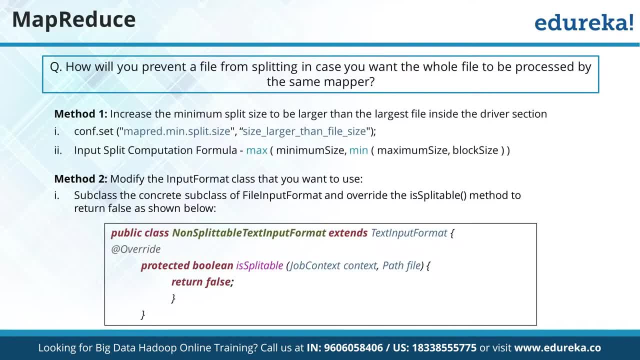 basically increase the size itself. it will be all good, or what you can do. you can go to your input format class and in that you can just update this property. you can make this it splatable to be returned in first. usually people prefer method 1 because that's the easiest method, right, and you need 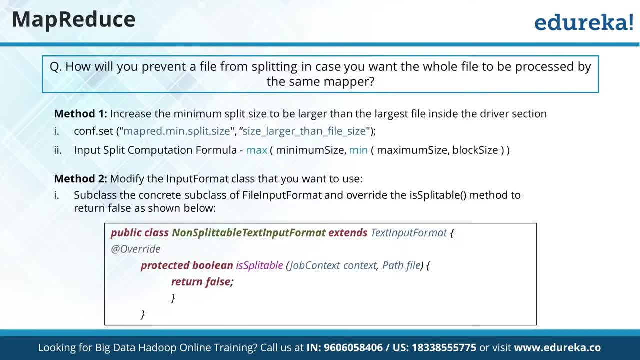 or update the Java code, basically to achieve all this. So what we will do for this. can you please tell us where file splitting is not needed? It all depends, right? So let's say, if I know, that I have only one data node. 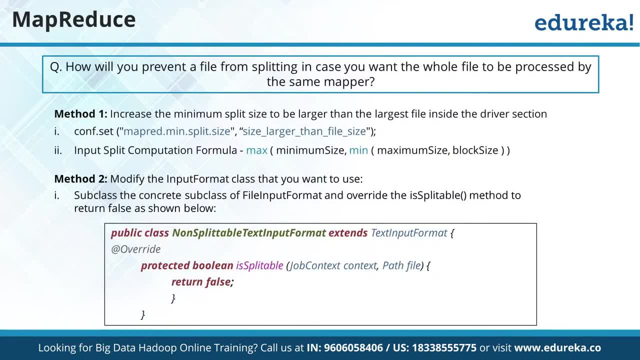 Let's say I have only one data node. Now, in that one data node, do you think it makes sense to divide a file? multiply together. I have only one data node, right? Do you think it makes sense? Because again, it's in the same machine, right? 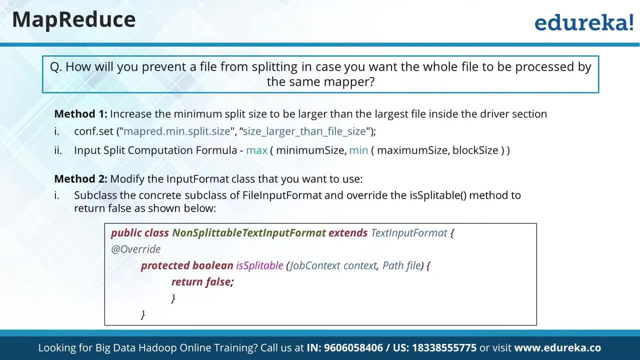 So that's the reason there: you want to basically keep one block itself so that I can execute it. So this is: these can be two situations where you can decide not to split the file and, in that case, how you will be doing it. 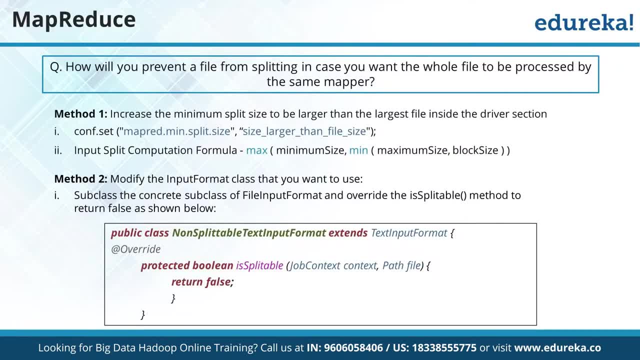 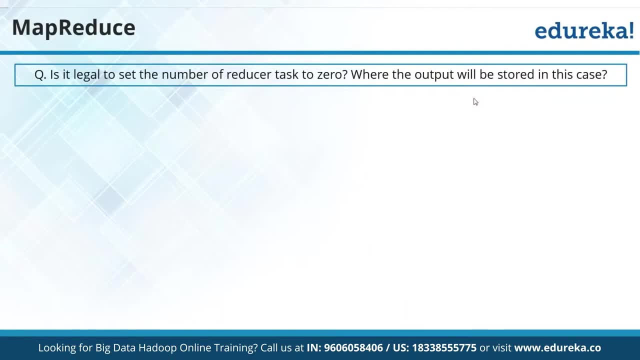 These are the two methods to achieve. okay, Moving further, Is it legal to set the number of reducer tasks to zero? That's question number one, Where the output will be stored. in this case, Is it legal to set the number of reducer tasks to zero? 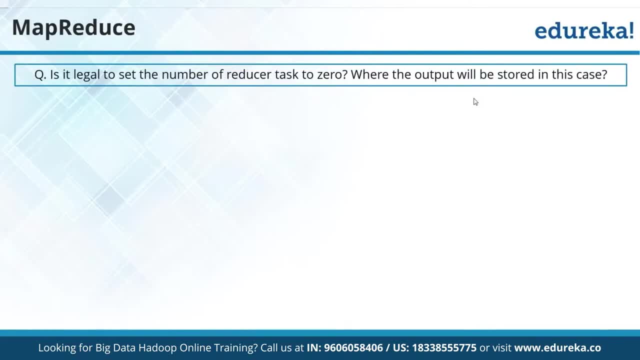 Is it legal? Definitely legal right. Everybody have used Scoop In Scoop. was there any reducer? Was there any reducer in Scoop? No Scoop only. use mapper. no reducer right. That's itself a tool, right. 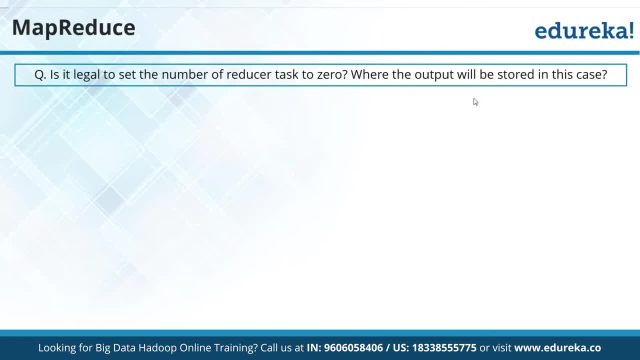 When a tool is not even creating any reducer? definitely I will not be using that right. So what is going to happen here is: let's say so: what was the purpose of reducer? Purpose of reducer is when you want to do some sort of aggregation right. 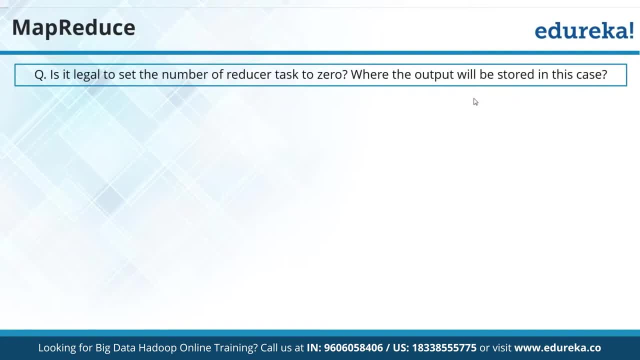 Maybe you want to sum it in the end and all those kind of thing, But it's not mandatory that all the problem statement in the world require aggregation, right? So those problems where you do not require aggregation, like I said, Scoop, because in Scoop what happens? 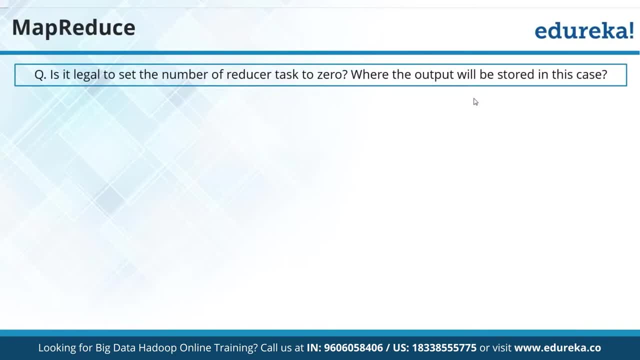 You copy the data from RDBMS to your HDBFS or vice versa. Now are you doing any sort of aggregation? No right, You're just copying the file from RDBMS to your HDBFS system, no aggregation required. 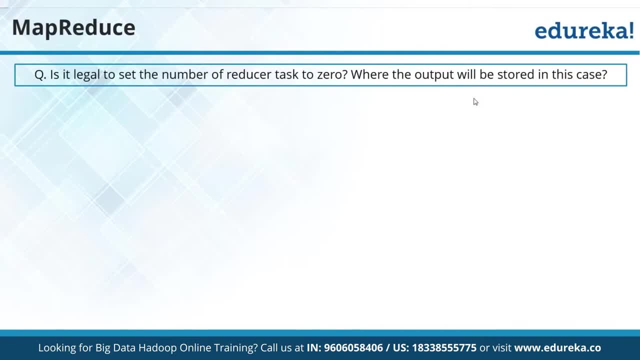 So in those cases you will be having reducer as low Output where to store. Definitely, whatever mapper output is coming wherever you are telling, it will be stored in that HDBFS location, right? So that's how you will be using it. 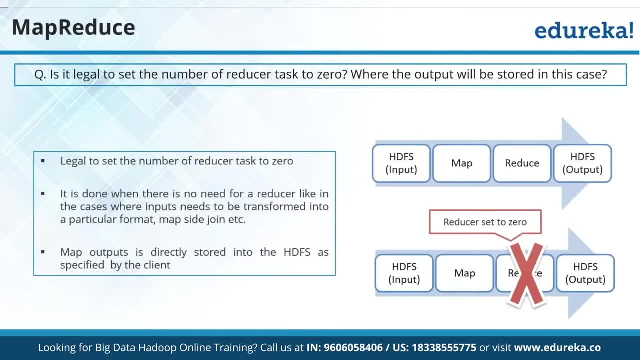 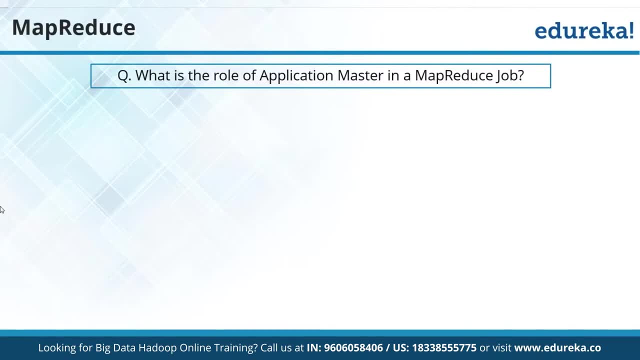 So definitely, the answer is yes And basically, wherever the mapper output you are keeping there, it will be getting stored. What is the role of application master in MapReduce job? Can I get this answer? This is a very famous interview question. What is the role of application master in MapReduce job? 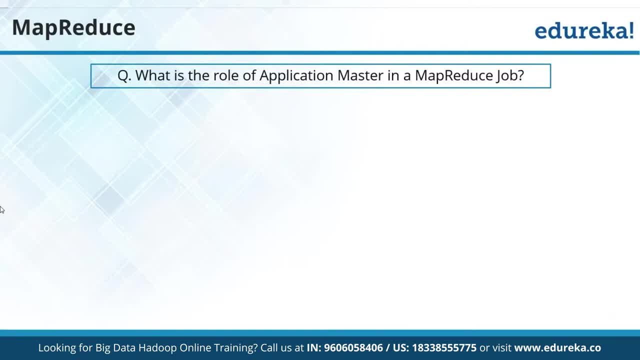 To assign the task: okay, that's it Only to assign the task. Sets the input split: okay, It manages the application prior than keep track of subprocess. that's it, Before nothing else, To get the resources needed for the task. 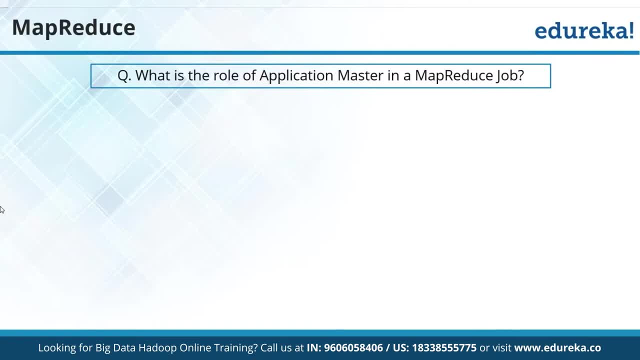 very good one here. Now you are coming here, you are coming close To create task until and until it runs. yes, What basically application master do? First thing is: application master is kind of just finding that how many resources it needs. okay. 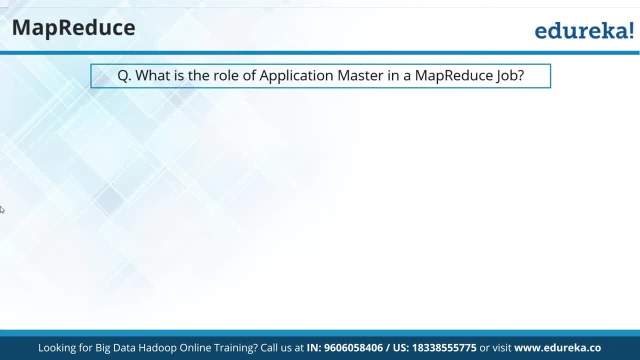 And it can basically now inform resource manager that I require this many resources And give me this many resources to execute that. Then, after that, resource manager, give back the container. If you might have gone through a yarn architecture right There, you might have understood all this portion right. 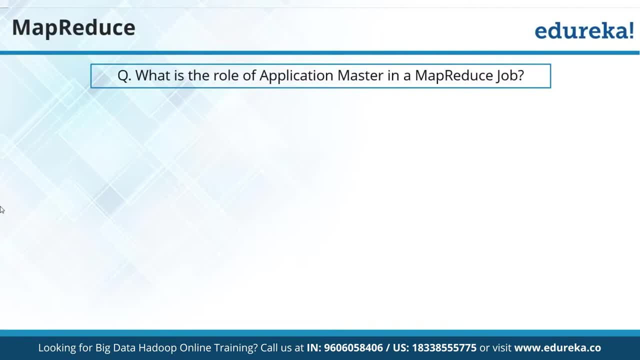 So basically, what happens is first, basically find out how many resources are required. Secondly, what it want to do is it basically want to find out once it happens. when it gets all the container. it kind of basically get them working together, It collect the output back and return it to basically. 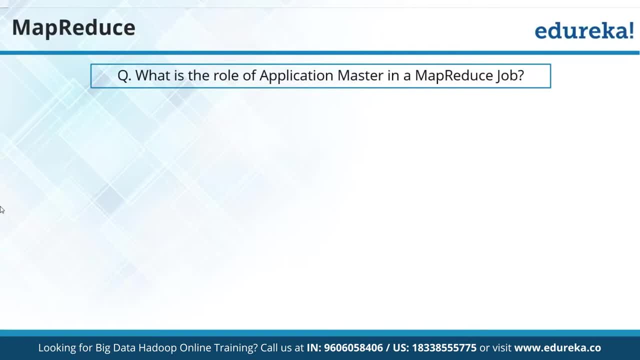 the master node. So it is doing multiple things in MapReduce It's not. it's basically not doing just one task. It is also checking, which is a very important role of it. It is checking that how many resources I require and kind of helping the resource manager. 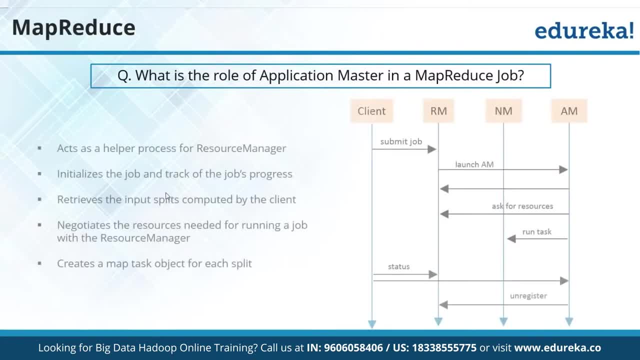 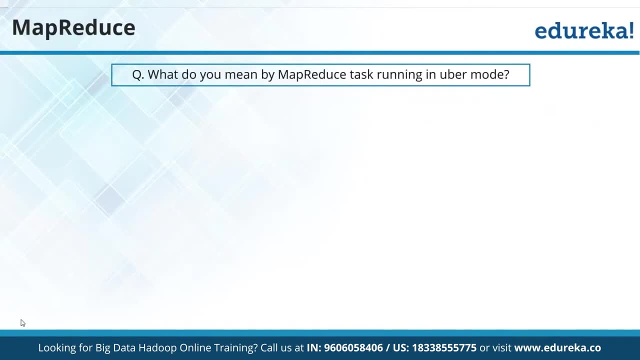 to take that, okay. So this is what, the same thing being explained here: The role of your application master, Which brings me to another question. What do you mean by Uber mode? So when your MapReduce job run? I don't. 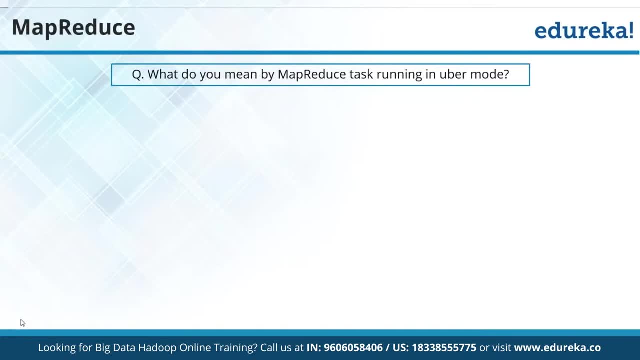 I'm not sure whether you have noticed that or not. There is something called as Uber mode. It's something comes in your console, If you have noticed that. So can you tell me what is that Uber mode? Is there any advantage of switching on the Uber mode? 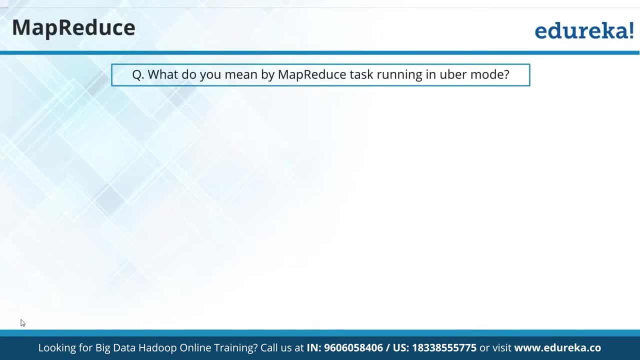 What basically Uber mode is going to do. Runs on applications. Can you give me some more insights on this? Can I get some more answers? Yes, So let's say: if you have a small job, right, If you have a small job. 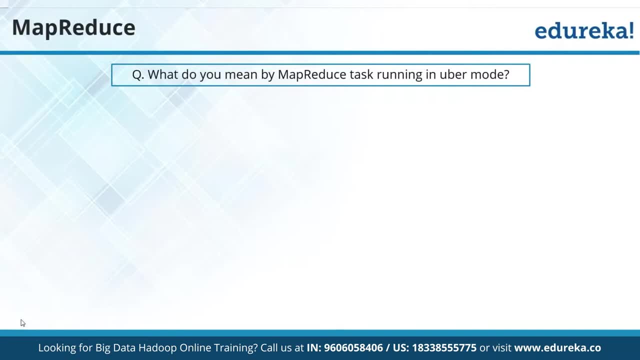 In that case you are basically again: application master needs to be anywhere Now application master will request and then it will allocate container. So container sending and all basically creating container, all those things are time consuming, So that is a good thing. 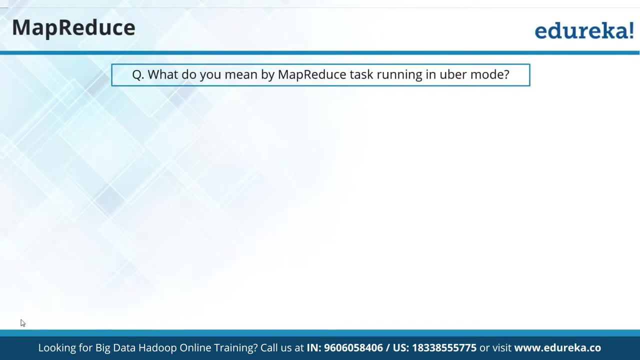 Okay, If the jobs are small, what your application master can do. Application master can start a JVM in itself. So basically, application master can decide to complete your job. Because the job is small, it may decide to complete the job on its own. 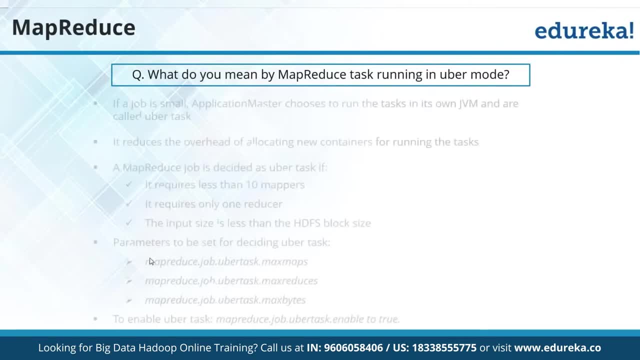 In that case we call it as over mode. So over mode basically requires less when you will be using, let's say, less number of mapper, let's say only 10 mapper. You have only one producer to work on. So in those cases we use over mode. 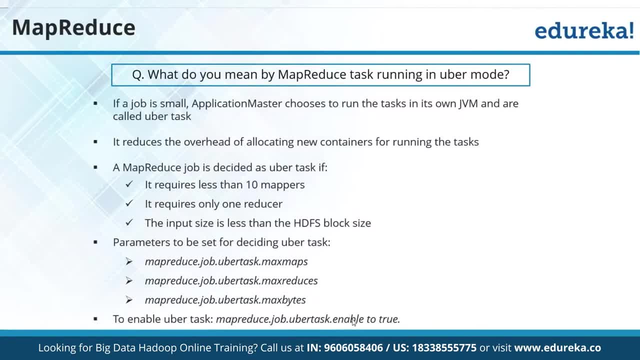 Now how to enable all that. So, basically, there is a property which you can set to true and it will basically enable your over mode, In which, what's gonna happen- Your application master will start acting like a JVM and will finish the job. So that's it. 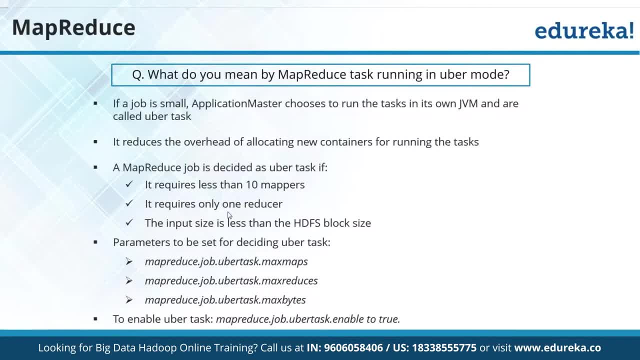 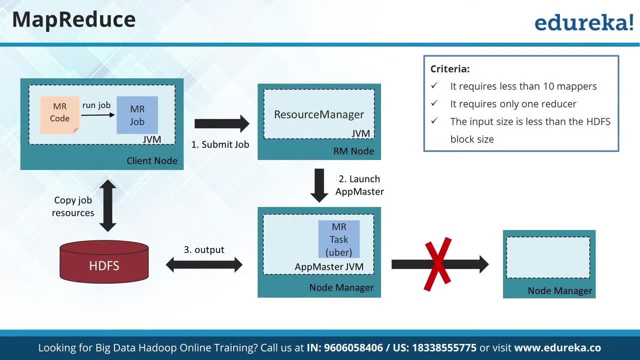 It will save you by creating container, making your performance better. So usually what people do is whenever they will be having some sort of, whenever they will be having small jobs right, And they want to improve the performance, they usually kind of enable the over mode. 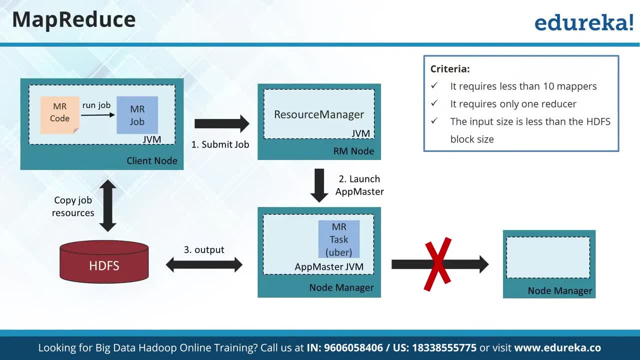 So now the application master. it will start executing the task and that way they improve the performance. But when you have a bigger job, it will not work. In that case we need to keep the over mode as first, Otherwise you will degrade your performance. 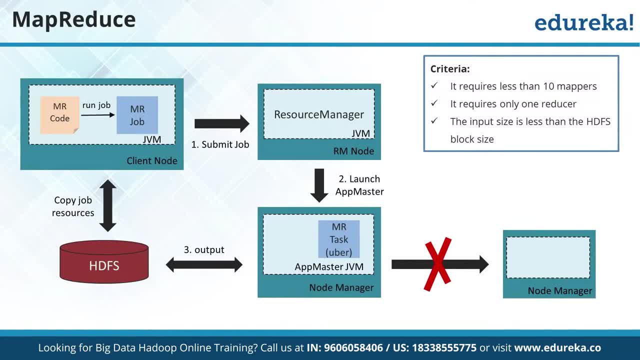 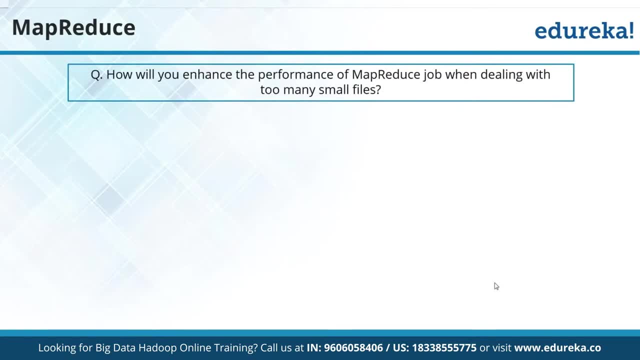 It will not even work. Okay, So this is basically your over mode. Another question: How you will enhance the performance of mapper-based jobs when dealing with too many small files. If you have, let's say, many, many small files, in that case, very good effort. 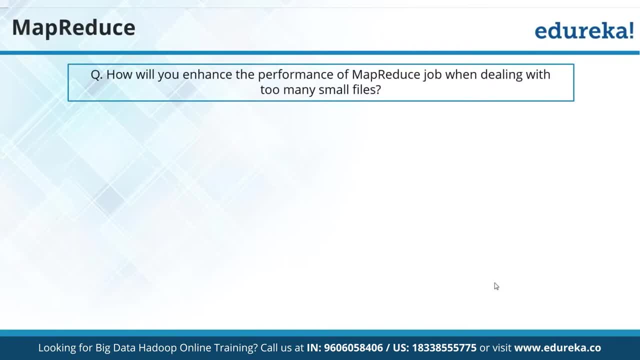 Yeah, that's also one thing. If you have, let's say, many, many small files, how you can improve the performance, How you can improve the performance of your mapper-based job Combiner. No, Coming close, but not the right answer. 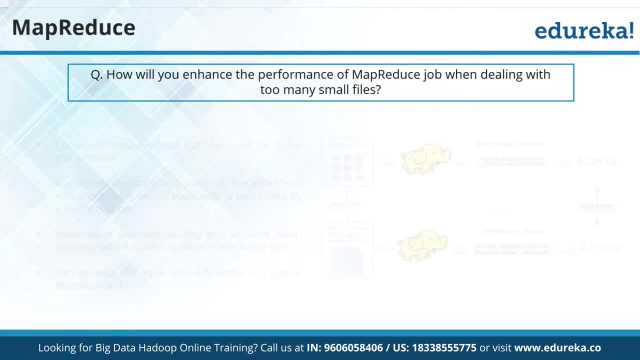 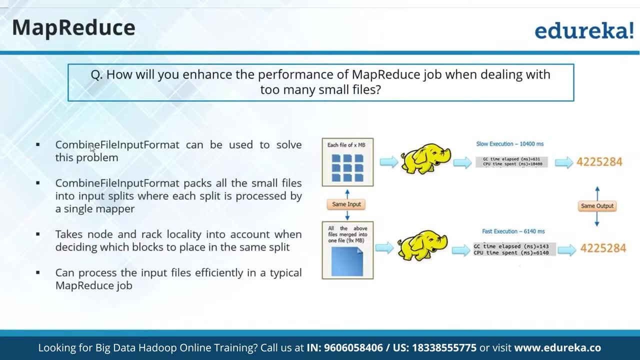 Too many small files are there? Then now what you will do. Basically, there is something called as- because none of you give the very right answer- There is something called as combined file input format. That's the reason I told you what You are: coming close, but not exactly coming right right. 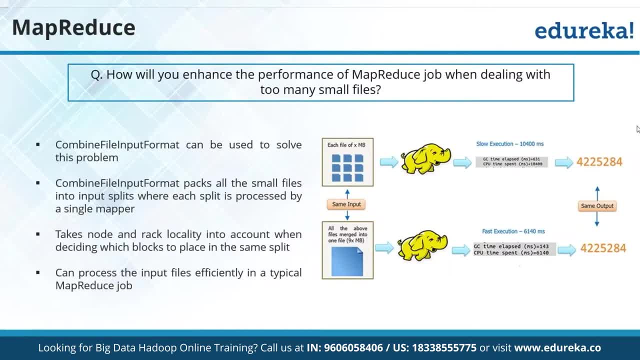 What this do is it kind of package all the small files together. See this diagram, See this part. Like these are some small files. It basically now combined all the files together. Now, because these small files got combined together now, my execution time will be faster. 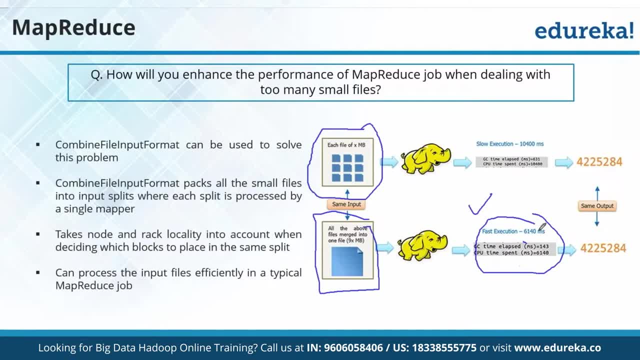 This is basically one practical thing which is being represented. This performance. can you see Like the small files was taking this much of time and basically with this, when you combine this, it actually started taking less time. So that's improving the performance of your system. 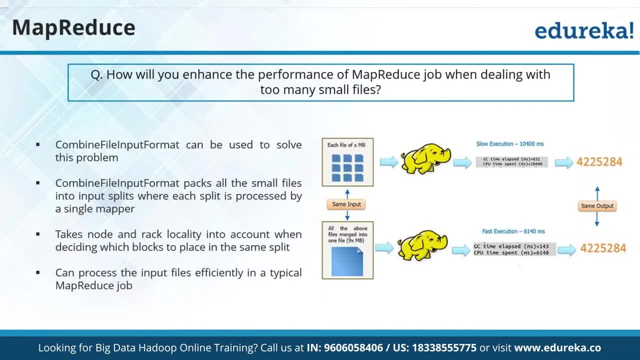 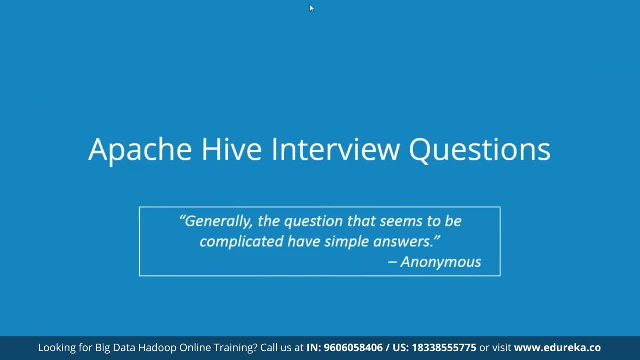 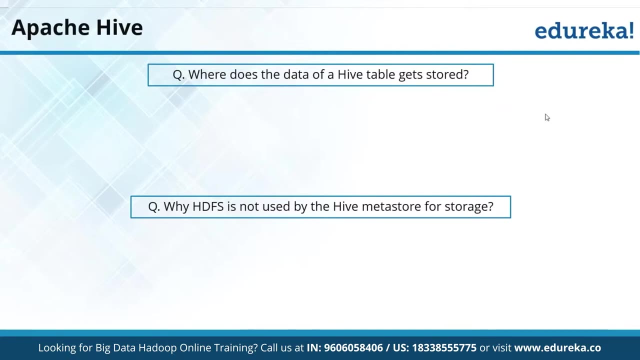 So this is what, this is how basically you can improve the performance if you have multiple small files. Now let's move to Hive. Hive is very important topic. Now question for you Where the data of Hive table get stored. Yeah, I know that you are going to be in SGFS, but where is the location of that? 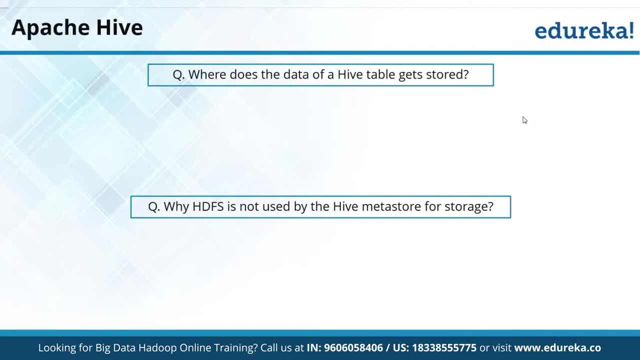 Where is the location for that? But what is the default folder? Next version. Very good, Now you are coming close, So by default you keep it in slash user, slash hive, slash warehouse. So this is the location where, by default, all your hive table get stored. 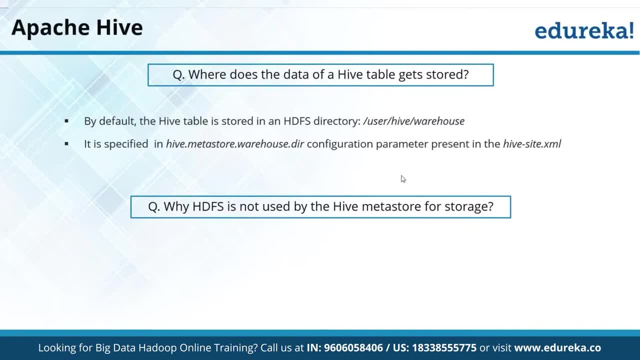 If you want to change this, you can go to your hivesitexml And can update this setting as well. Another question: Why HDFS is not used by hive meta store for storage. What I mean is, you might have read in your course that you keep your hive, basically your meta store, in your RDPMS. 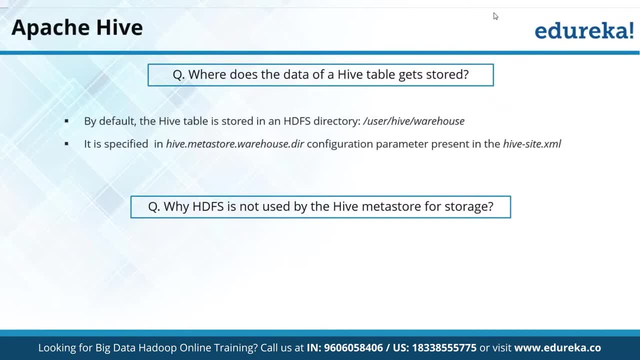 Right, Not in HDFS. What is the reason behind that? Why we not keep all these things in my HDFS. Why your meta store is created in your RDPMS. Why you are configuring your meta store in RDPMS for hive. 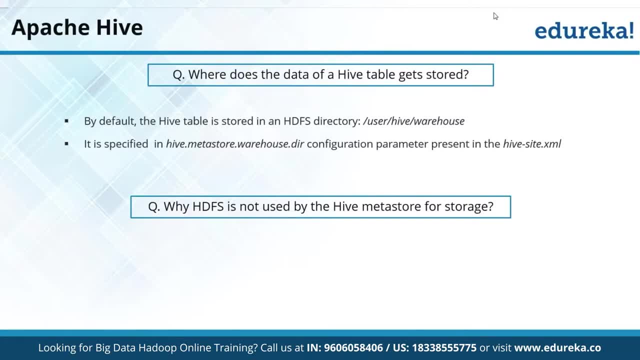 Why not in HDFS? Can I get this answer? Why you are keeping your meta store in your RDPMS system and not in your HDFS? I can tell you This is the most important question of hive. In any interview of hive you will go expect this question. 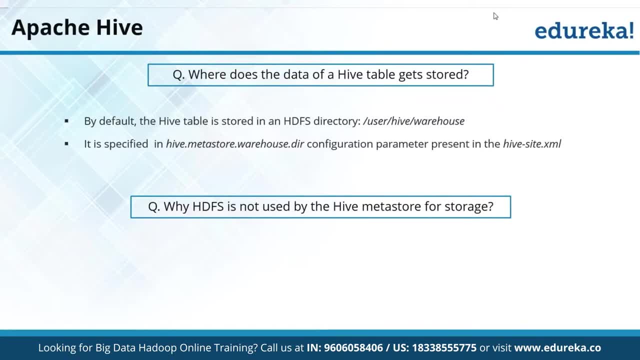 This. usually everyone ask For random access, but that you can do in HDFS also. Ramya, if we need DB catalog, what is that catalog? Because if need to use JDBC connection, no, no, that's not the answer. 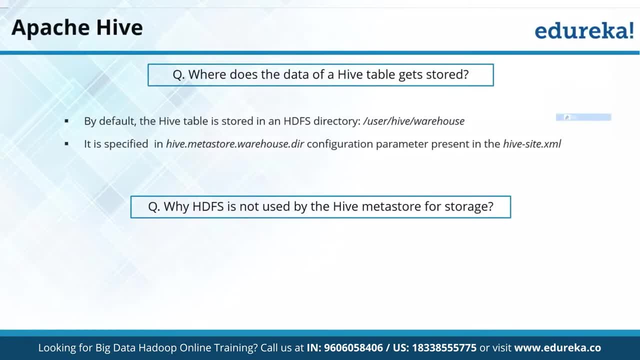 Okay, Let me ask you this question. Okay, What is the main reason for it? So let's say, if what you do is, when you create a table in hive, what happens? It creates an entry for that table in meta store table. 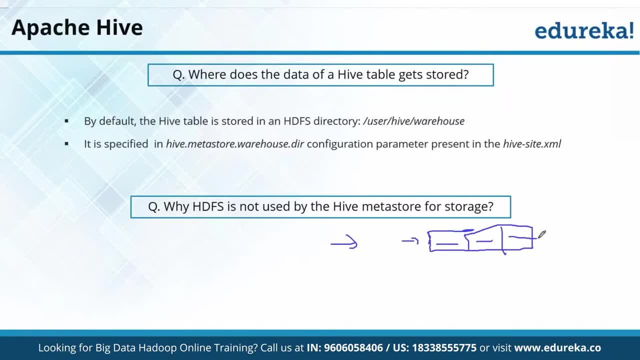 Right. What it's doing, It's inserting the row level. Right At a row level, it is inserted. You created another table in hive. Again, you are basically inserting some values here Right Now. let's say you deleted some table in hive. 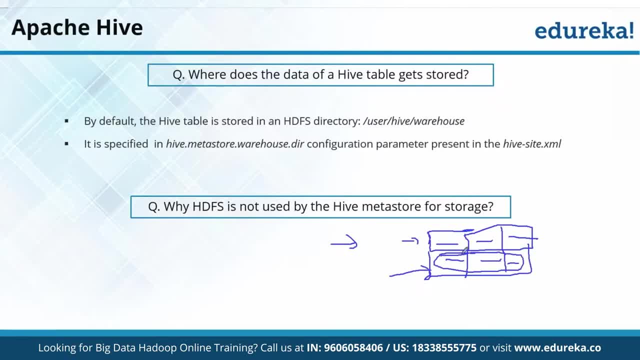 What happens? It did a row level delete. Can you do this- row level delete, row level insertion, and all in your HDFS? Okay, You are saying referring to the same thing, Arishkari. then you are good. Can you do this, basically this, in your HDFS? 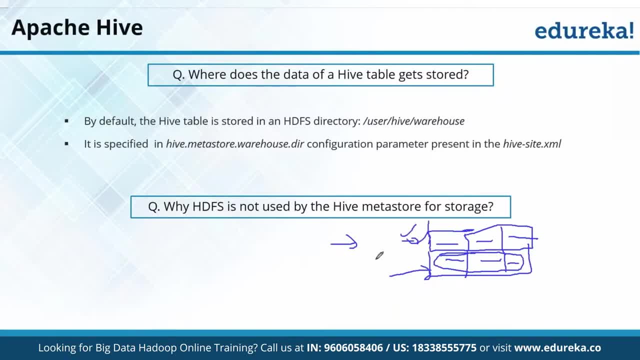 No, Right. This itself is a good answer to explain this, Right. So, and second thing is definitely in RDBMS the syncing time is going to be faster and all Those are the other factors. But first thing is basically your CRUD operation cannot be done in HDFS. 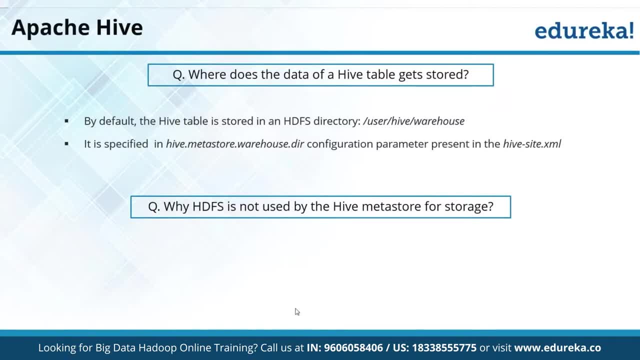 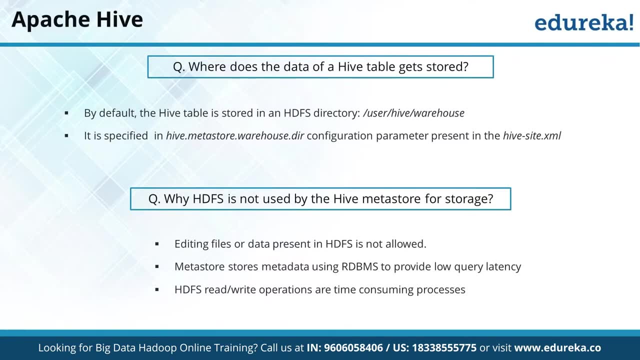 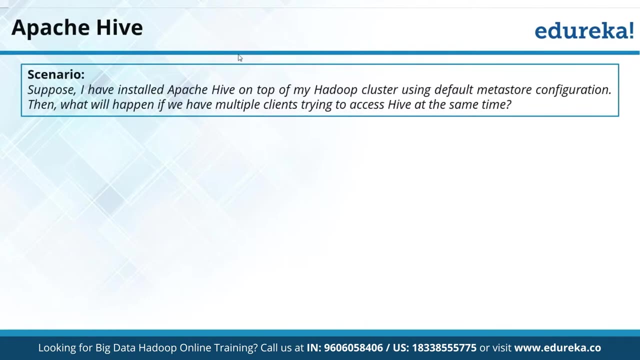 That's the reason we will not be able to keep in HDFS. Forget about other factors. Right, They do not make any sense, in fact, because my first property itself is failing of basically CRUD operation. Now let's see some scenario question. Usually in hive you will find some scenario questions coming up. 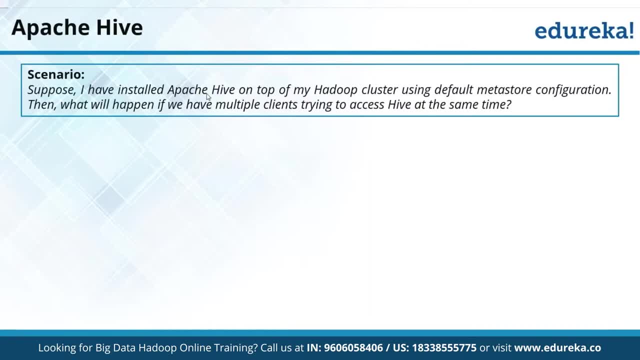 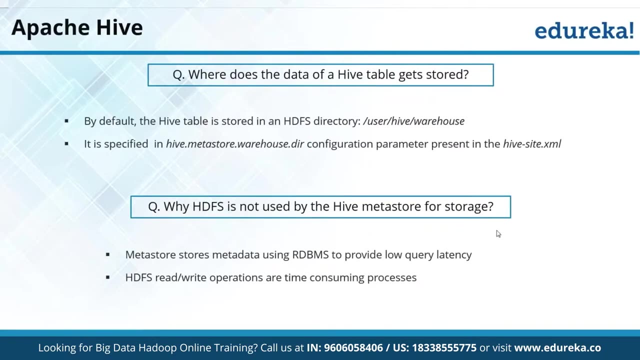 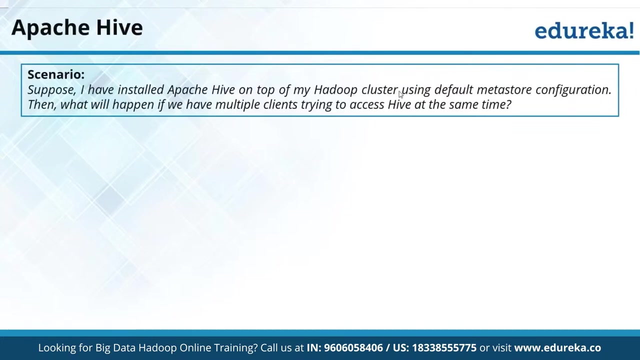 Now scenario question is: suppose I have installed Apache hive on top of my Hadoop cluster. Can you please show the last answer? Sure, Why not? Can you see this question now? Suppose I have installed Apache hive on top of my Hadoop cluster using default metastore. 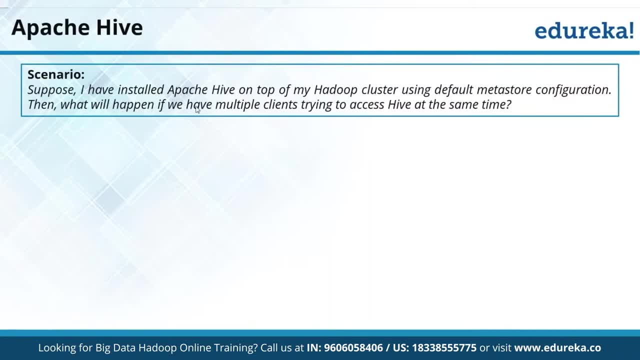 configuration, Then what will happen if we have multiple clients trying to access hive at the same time? Right Suppose I have installed Apache hive on top of my Hadoop cluster by using default metastore configuration, Then what will happen if we have multiple clients trying to access hive at the same? 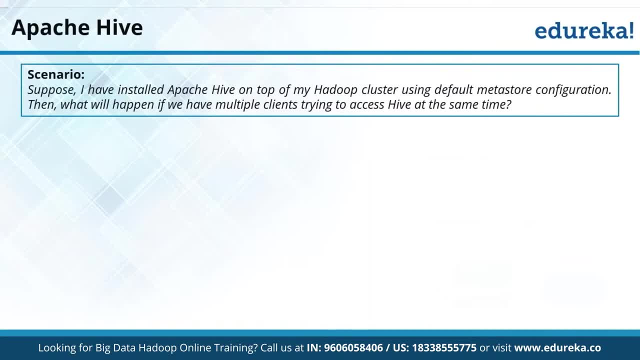 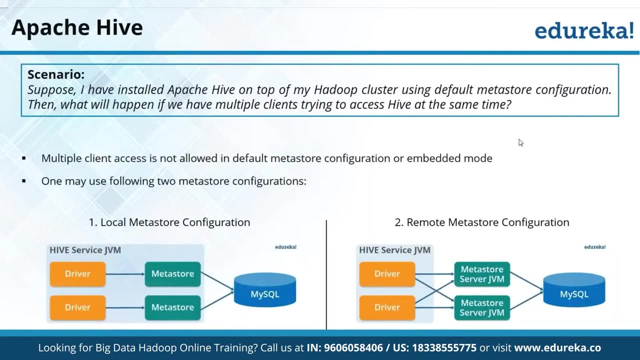 time. Very good. Usually in hive you can only basically access one by one client, So multiple client access itself is not possible, So multiple client access is not allowed. Right, Very good, collectively They have given the right answer. So usually these are the scenario, what it follows. 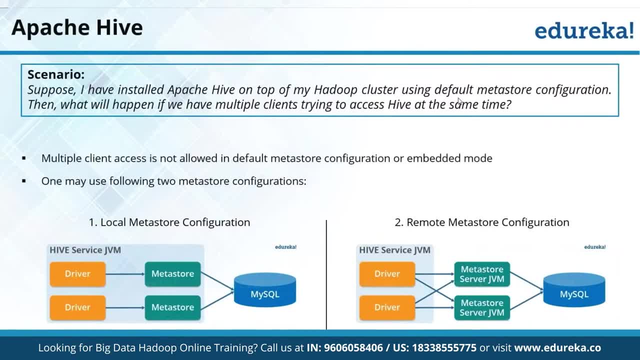 So what is your main thing is your multiple client access in hive is not allowed. This is my architecture, Right, Because you should maintain the read consistency. Very good, So that's the reason this itself is not going to work out. So, basically, that is what you need to understand. 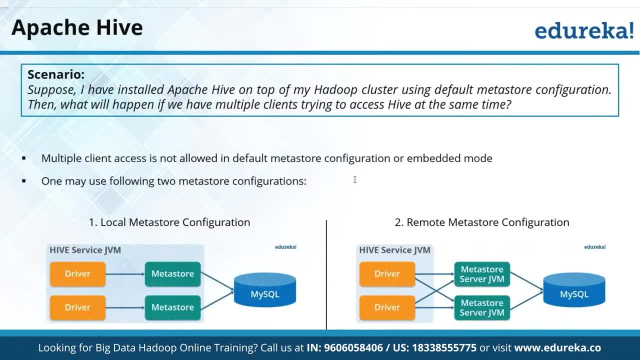 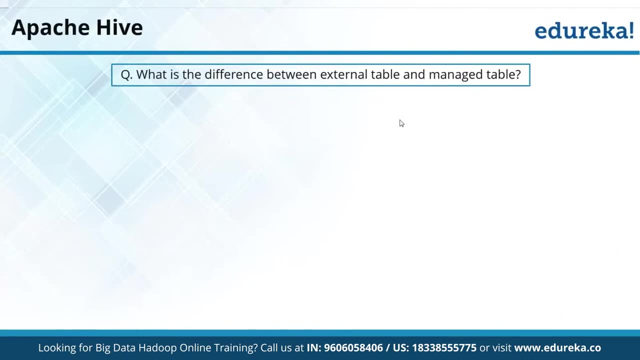 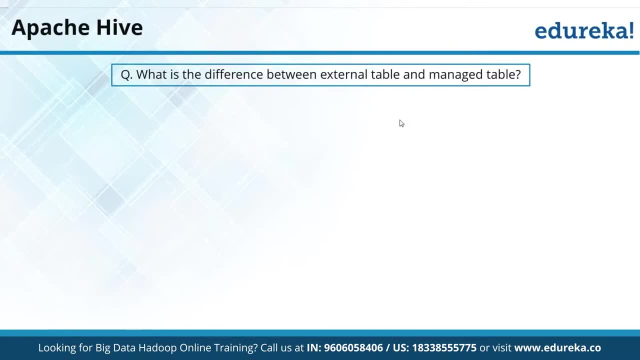 can I get an answer? what is the difference between external table and managed table? can I get this answer? external table can be a file, okay. but I want a difference, proper difference. external table, where the HDFS file won't be deleted. if we delete the table and you say HDFS file, okay, okay, I can accept. 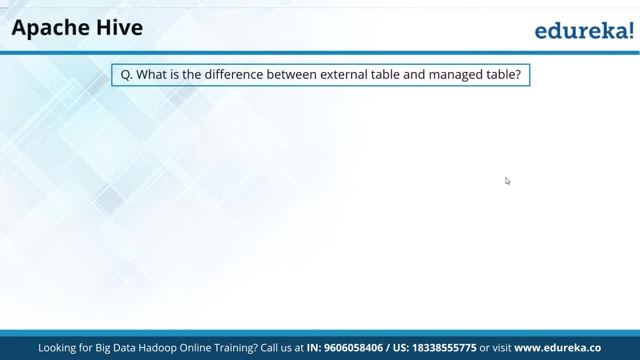 your answer, Angela. external table is stored in separate location of our thread. but even in internal table I can store it at some other location by defining the location keyword, and the external table keeps data when it get deleted. very good, that is the major factor where the data is stored. that is the major factor when the data is stored. 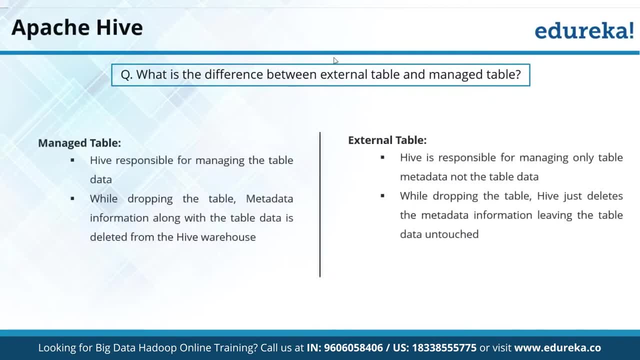 When you talk about managed table, what happens is, if you have deleted any of the data table, what is going to happen? It will delete the entry in your meta store. At the same time, it is also going to delete the data file. 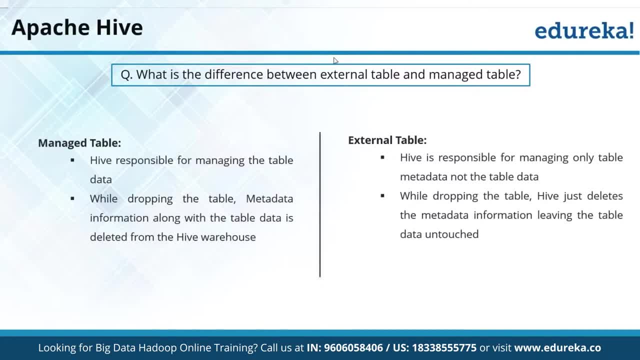 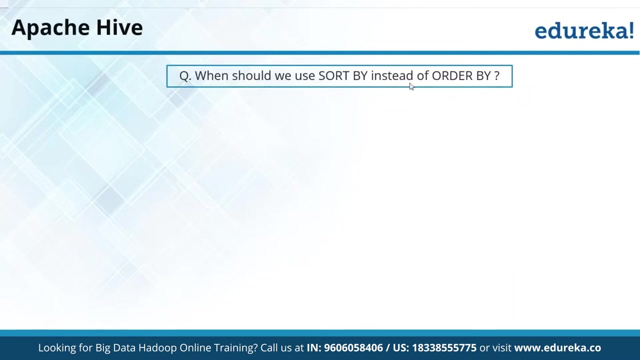 But in external table. if you delete a table, it is going to only delete the entry in your meta store, not from your main data. okay, So that is the major difference, basically in the managed table and external table. Another question: when should we use sort by? 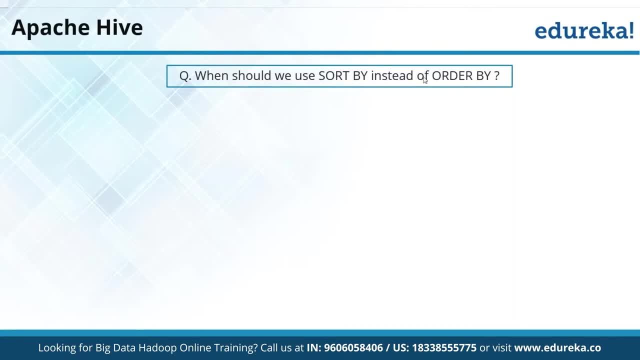 instead of order by. If you notice, these two APIs belongs to file and these two basically going to do exactly same thing. So when should I use sort by and not order by order by Operation? When should I use sort by and not order by operation? 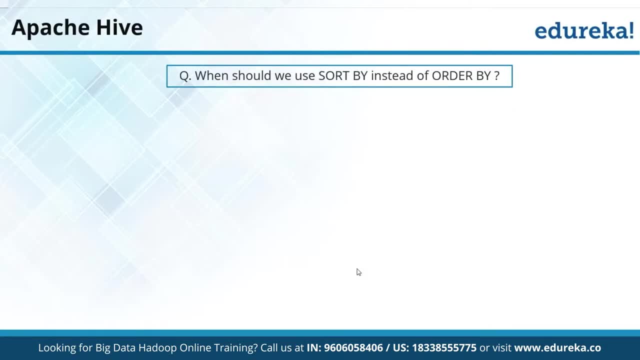 So, basically, to answer this, not able to catch things, I did not get this, Ravi, When we should have only one mapper. Okay, Ravi, I think you are in fifth module, right? So that's the reason. yeah, I can understand. 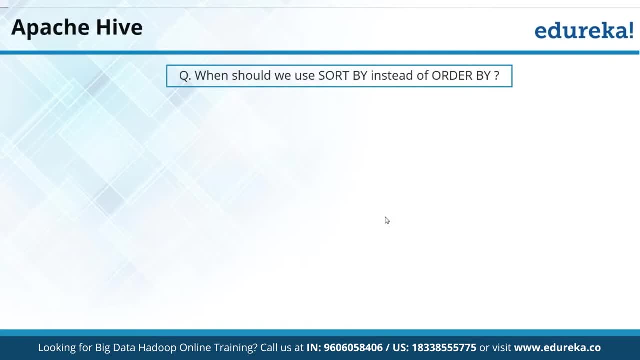 You have told me in the starting itself right that you are still going through this course, So if you are not getting it, it is completely fine. just listen to this, okay. Just listen to this conversation Once you will go over these course topics. 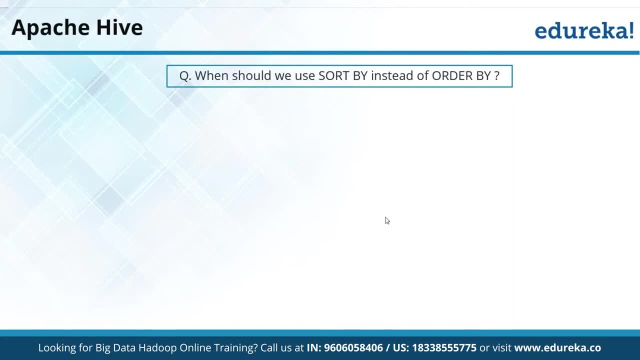 in basically from wherever you are doing. you will be all compatible with it. okay, Basically, now I can understand if you will not get anything because these modules is not being taught to you yet. So these are basically the new modules which will be taught later. 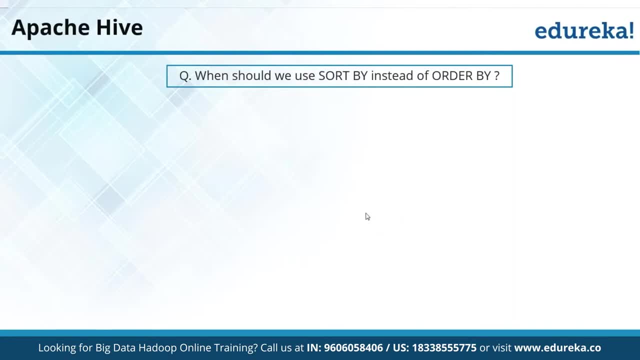 Now can I get this answer? In case of numericals? no, no, that you can use also order by One of it. use reducer, other use mappers. okay. Okay when you use group by operation: no, no, that's not the way. 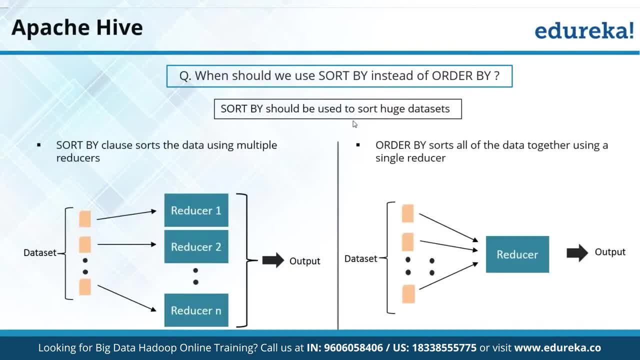 Actually what happens is if you have huge data set, in that case you should use basically the sort by option. If you will do this sorting on multiple reducer while order by do it on one, That is basically the major difference. So when you have huge data set, 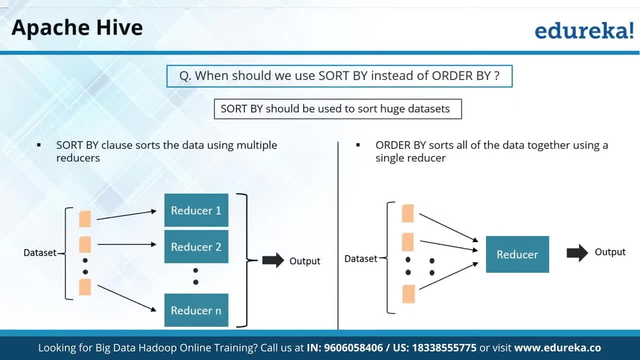 use sort by instead of order by. okay, Lot of people remain confused with this. That's why this is a very tricky question: What people are usually? if you ask anyone, right, If you do not know the answer, you will tell you both do the same thing. 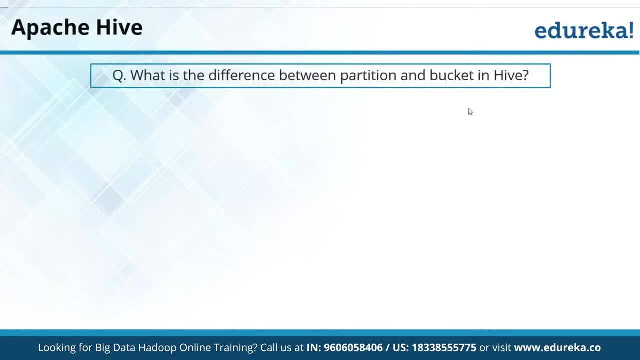 But actually that's not the fact. there is a difference. Now another question: what's the distance between partition and bucket in Hive? I think the most easiest question to answer. Can everybody answer this, Whoever has done on Hive topic: What's the difference between partition and bucket? 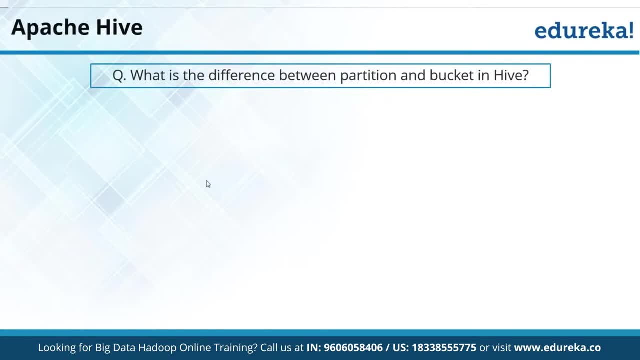 This is the most easiest answer. Can I get this answer? Difference between partition and bucket: simple, right. Partition is basically at the first level right. When you split the data into different directly, bucket is like a sub-partition of that right. 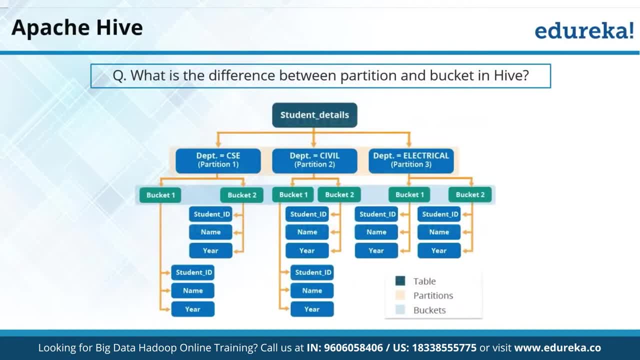 So even for that partition it's when you create another sub-partitions, you can call them as bucket, Like in this case. can you see, the first partition is TLC department, civil department, electrical department, But after that we have also created 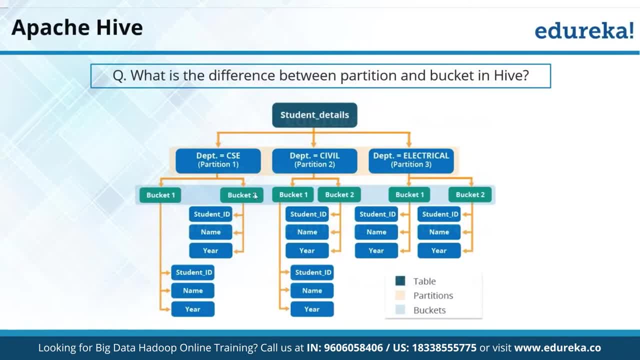 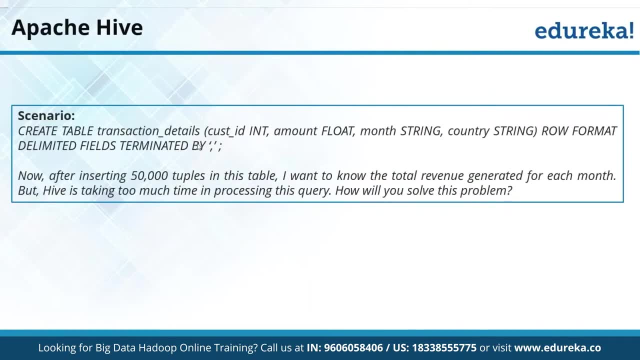 some sub-partitions of it And that is your bucket. That's basically the difference there. Another question: let's say this is the scenario: You are creating a transition table. Now this is the table. what we have like a transition table is the table. 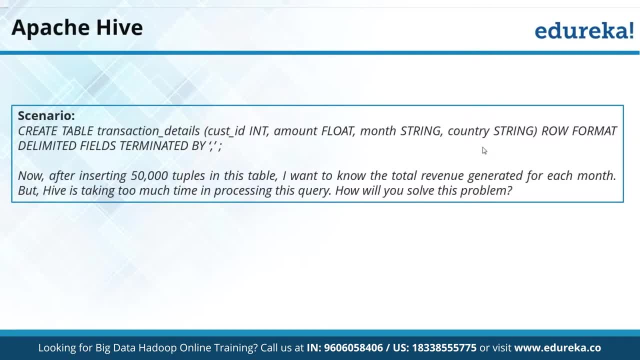 You have this many columns Delimited field by comma. Now let's say you have inserted 50,000 tuples in this table. Now I want to know the total revenue generated for each month, but Hive is taking too much time in processing this query. 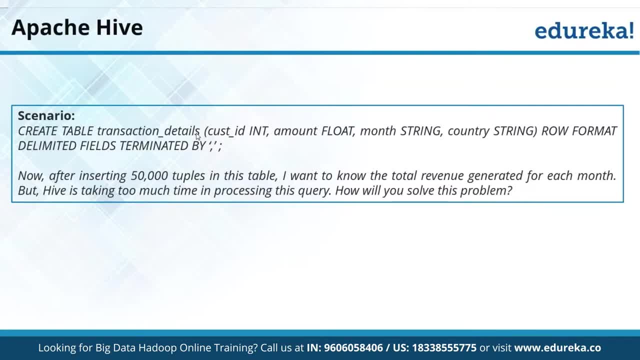 Can you tell me what the solution you are going to provide? This scenario is actually a very good interview scenario. Very good, Narsima. Can I get more answers? Very good, very good, Vipul. Can I get more answers? 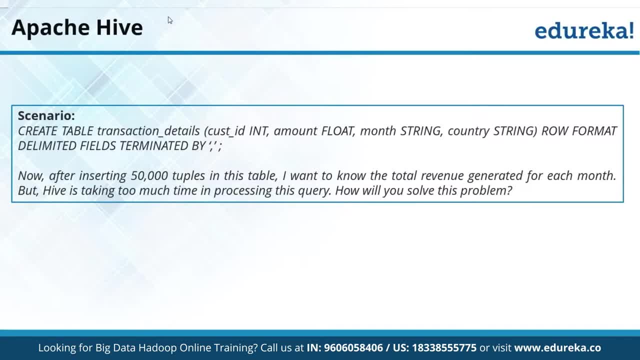 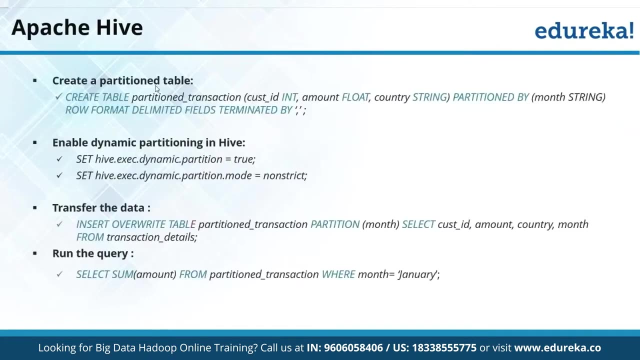 You will be partitioning this table, How you will be partitioning. You will be partitioning your table with month, right? So basically, if you partition your table, you will improve your performance. So these are the simple steps. You can create a table partition by month. 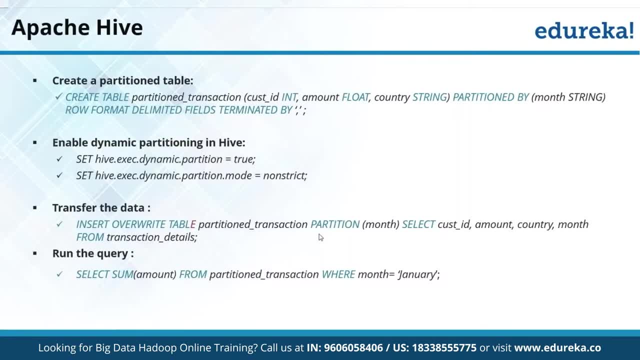 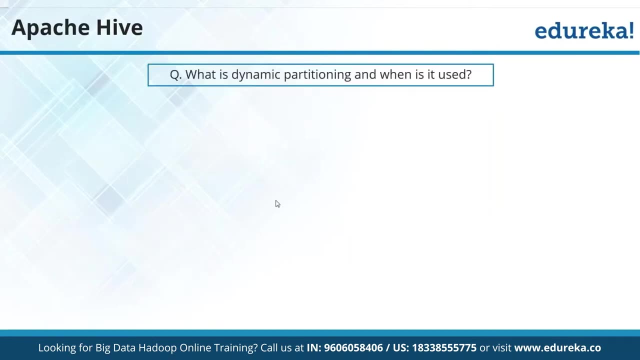 set these properties So that you can enable your partition, insert the data and then you can retrieve the data where your month is going to January. So while partition, after partitioning the table, you can improve the performance. Second one: Can I get an answer of this? 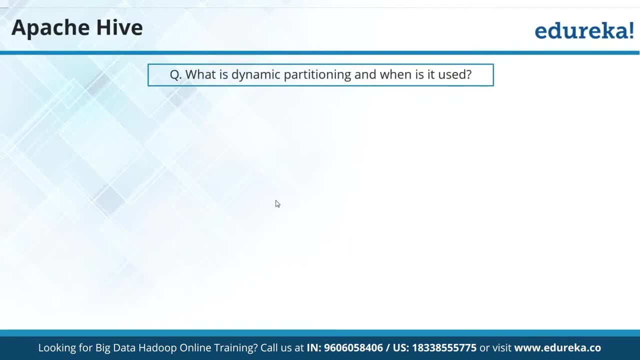 What is dynamic partitioning and when is it used? Can I get this answer? What is dynamic partitioning and when is it used? That can be static partitioning also in the right, So I want to know what is dynamic partitioning. 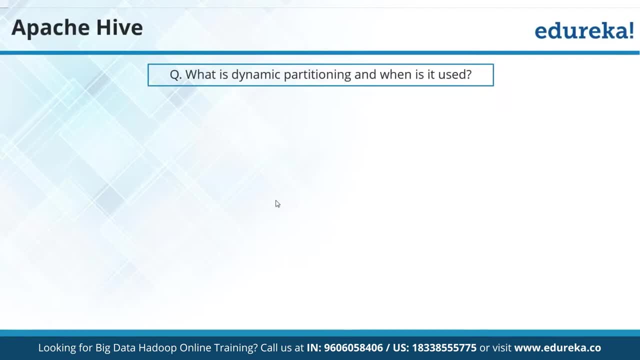 Very good. Partition happens when loading the data into table. Right now I don't know that if I do a dynamic partitioning where it is how many partitions also it is going to play. So the value of your partition columns will be known. 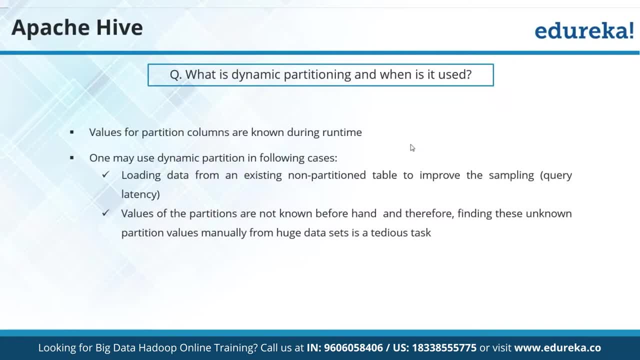 only during your run time when you will be creating the partitions. So the value of your partition columns will be known only during your run time when you will be creating the partitioning. So the value of your partition columns will be known only during your run time when you will be creating the partitions. 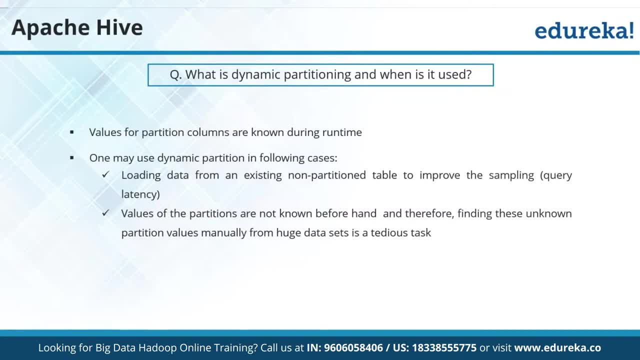 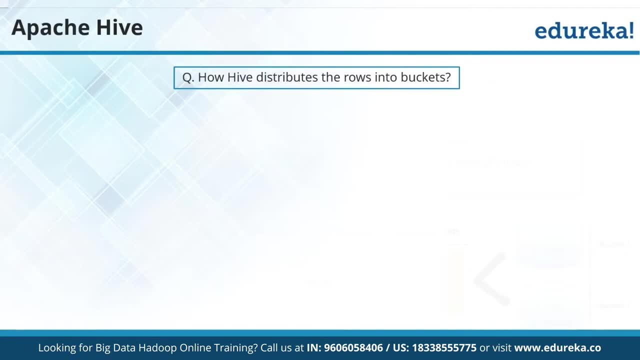 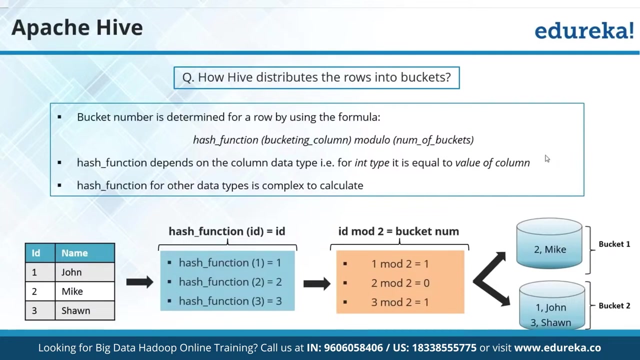 That is called your dynamic partitioning. How Hive distribute the rows into buckets. Can I get this answer? How Hive distributes the rows into bucket? Very good Hash algorithm. It uses the hash algorithm to understand this part. If you look, what we are doing here is: 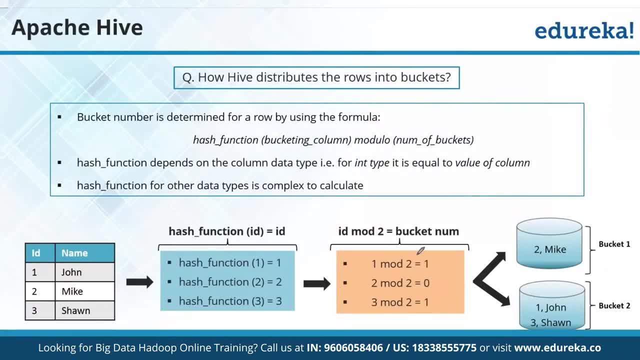 Now, no, You will be using hash algorithm. right, be using clustered by, but basically are in the how internally. this is it that? basically how it is it? let's say, you want to put into two bucket in that place it is going to do modulo of 2. okay, so let's say modulo of 2. this output came. 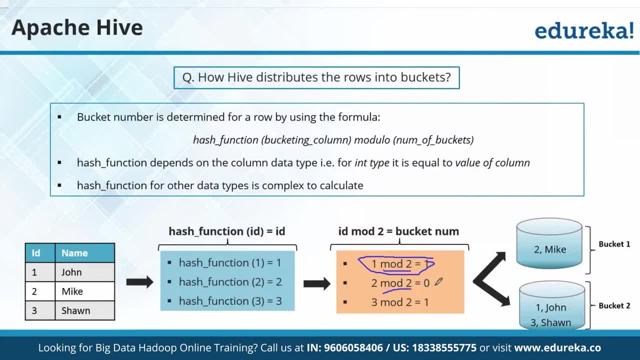 out to be 1, so it will decide to put in bucket 1 modulo 2. it is going to become 0. it is going to keep in this second bucket. so this is how it will be decided. okay, it will be using basically a hash computation of this. so, basically, 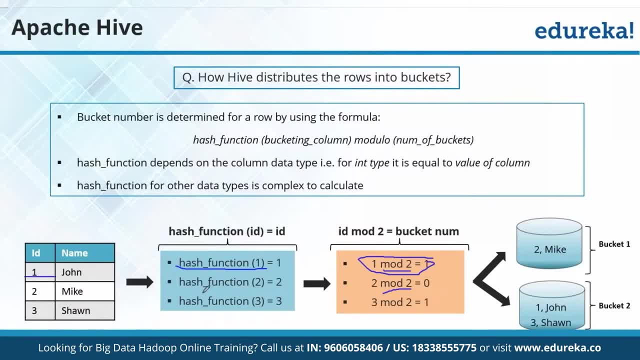 it will be using hash function of this. so let's say, hash value of this value came out to be 1. hash function of this value came out to be 2. hash function values: this came out to be 3. then, basically, it is doing this modulo. 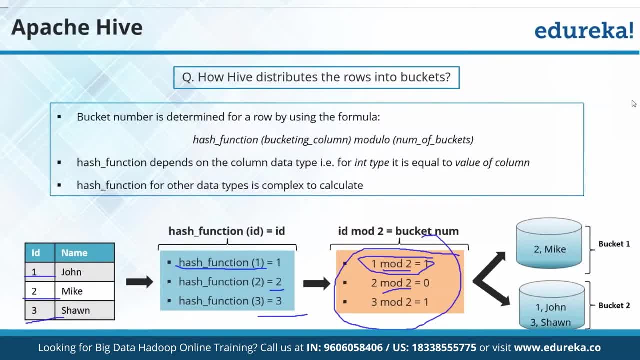 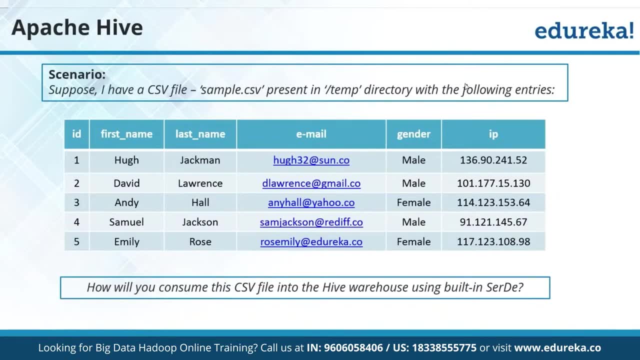 operation and giving the output, and that's how it distribute the bucketing data. now, which brings another question. suppose I have a CSV file which is named as sample dot CSV, present in pfx and directory, with the following: increase in that case, how you will consume this CSV file into where hide warehouse using big insert them. 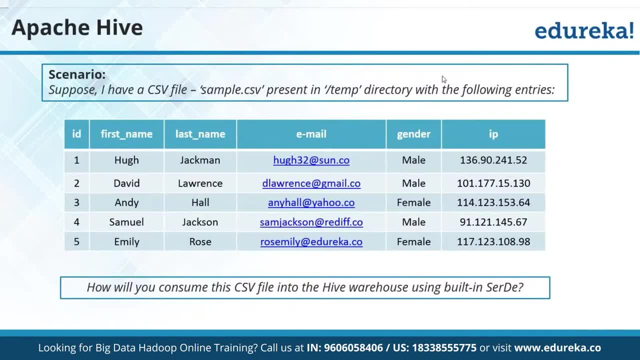 sudden with serialization surdus. these are the stat to the free serialization be serializes hon. when you convert your data into kind of work, kind of bytes, can I get this under row format delimited by comma? underlying code: so it is a byte and it is a data set. it is not an animation in. 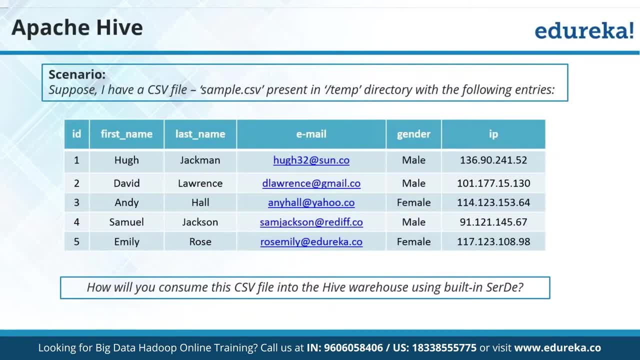 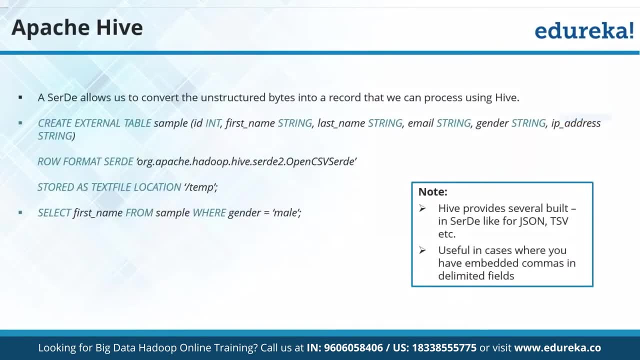 Not exactly. I'm looking for something else. Absolutely, it requires some APN. So let me show you this part. See this answer. In this case you will say raw format: Serde orgapachehiveserde2.opencspserde. 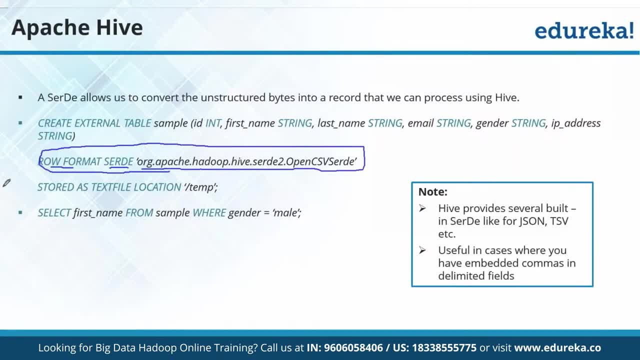 This is what you need to add. okay, Now you got it. what's the mistake you are doing? So, basically, this is what you need to add. Otherwise, everything is the same. You can save it in the tmp folder, and all that. 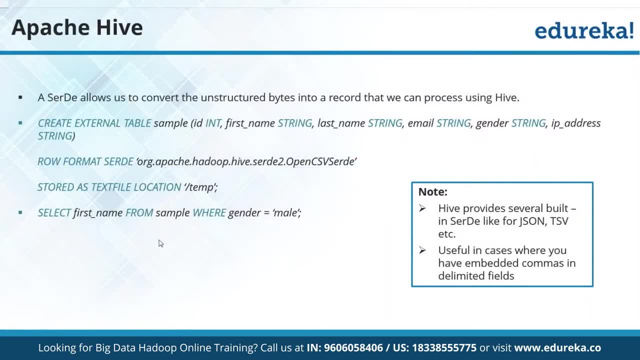 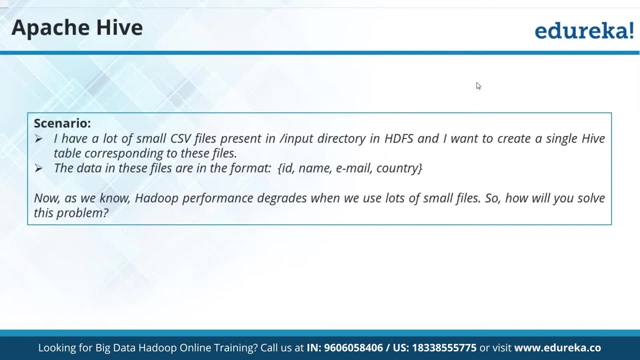 Just that the only difference will come in raw format. Serde. Another question: I have lot of small CSV file present in input direct training papers And I want to create a single table, high table, corresponding to these files. The data in these files are in this format: 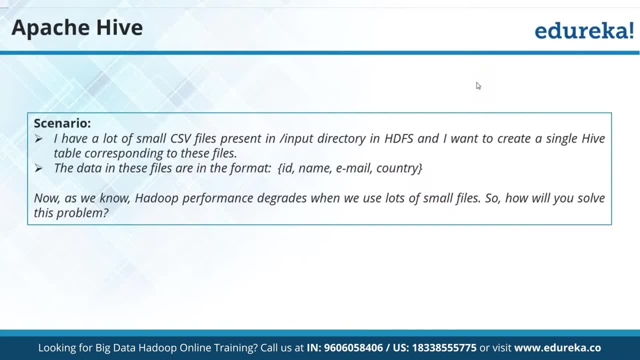 Now, as we know, Hadoop performance degrades when we use lot of files. So how you will solve this problem? Can anybody give me a simple answer of this? This should be easy. You have multiple small files Now. in that case, what should be the solution? 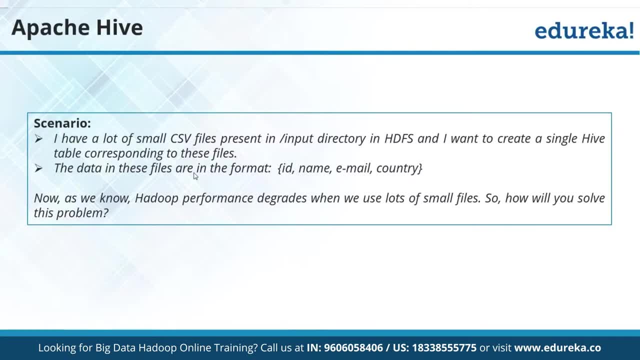 Because definitely my performance is going to degrade. What should I do On catenate solve file? but can there be another answer? Don't you think you can use sequence file here? Sequence file, right. If you have one solution, that is for my HDFS level itself. 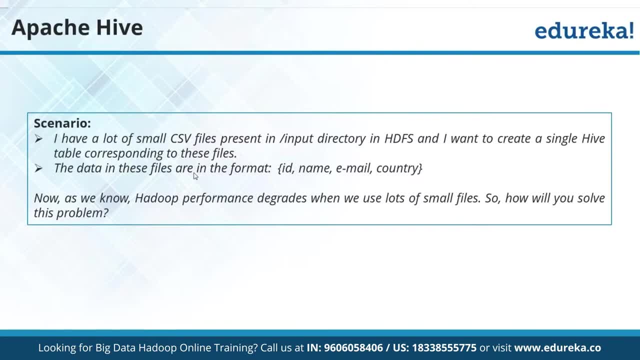 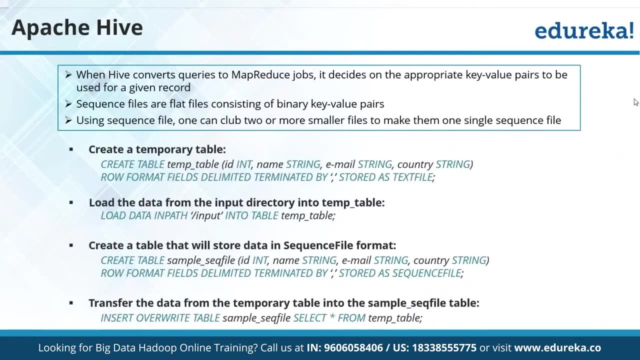 Great, right, I'm talking from this. This is basically high perspective, right? Don't you think I can convert in a sequence file? Sequence file will convert everything like zero one, zero one kind of thing. So that's what make it better, right? 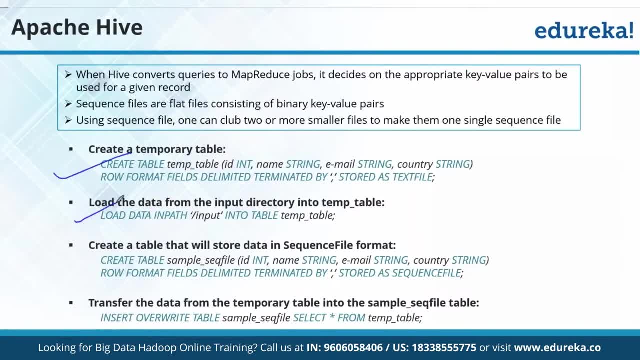 Will improve my performance. So first create a table, load the data- After that what you do- store it as sequence file And then basically load this data from this file, whatever inserted to this file. This will ensure now that your speed will be good. 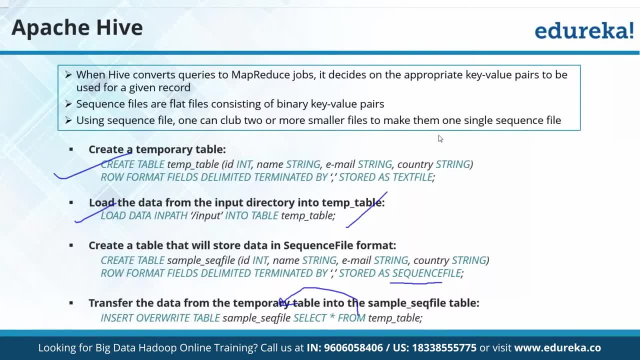 Why do we need to do in service? Why do we? okay? So basically, when you do service right, The advantage what you get is: so let's say, first thing is compression, because you are serializing the data. When you serialize the data, it makes that transfer. 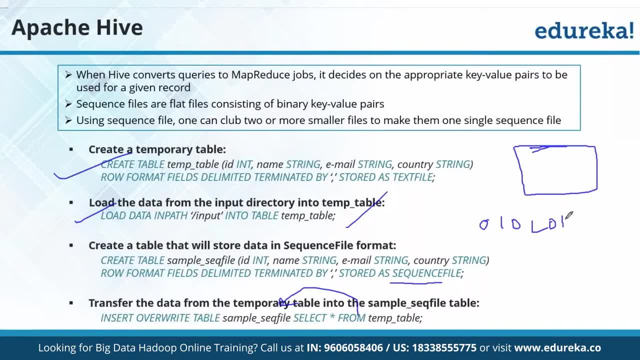 also very easy because we have converted like zero one, zero one, zero one kind of thing, right. So first thing is, when you convert to service, you compress the data. Second thing, since you convert to this zero one format, now the transfer over the network. 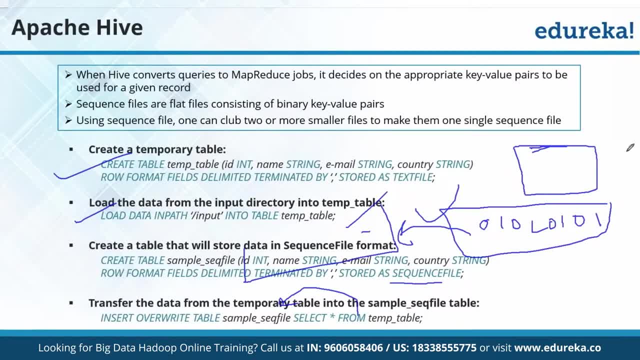 it becomes a lot more uniform. Here they come up. That's the reason we basically use service in this demo. So, but remember, there is no free lunch, right? There is nothing called as free lunch. Don't you think this will also have a disadvantage? 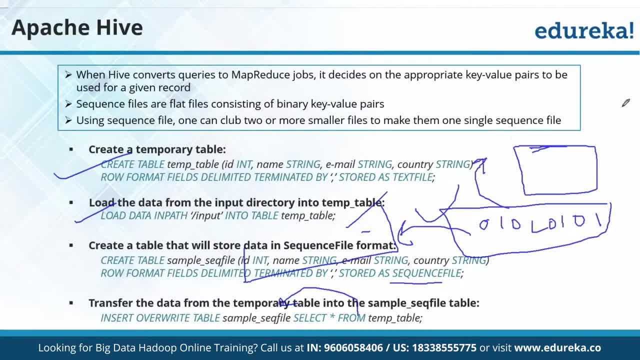 When you do a de-serialization again, you need to convert it back, Don't you think it will impact the performance a bit, right? So remember, there is no free lunch. Though it is helping you in this, that, but at the same time it will demand your performance. 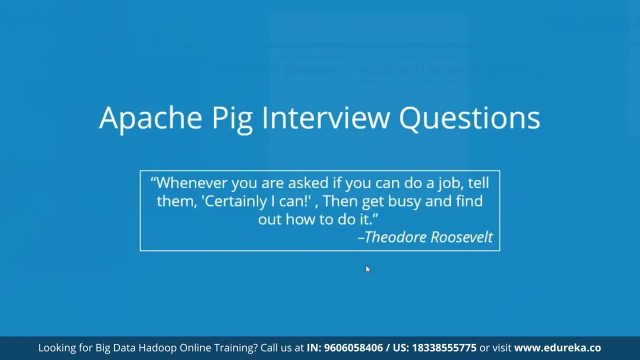 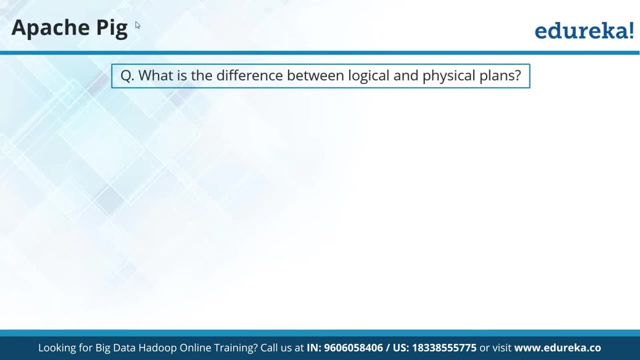 It will lead to some of your performance. Now some quick questions. Can you give me this answer? Difference between logical and physical plan. Can you do something? Difference between logical and physical plan. I know, guys, that you got a little tired because this is a big session. 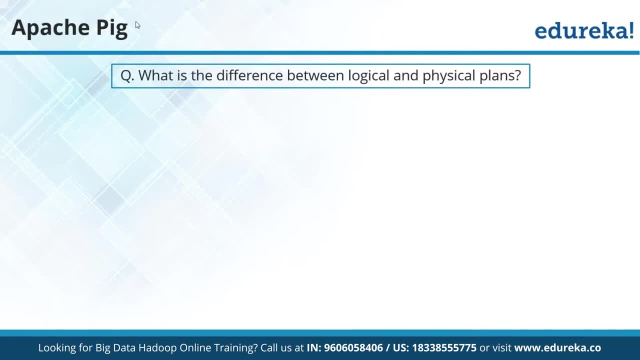 but don't worry, we are almost getting there. So I want everybody attention to be back now. Can you tell me the difference between logical and physical plan? This must be the first thing, what you must have learned in your Hadoop course when you went to pick topic. 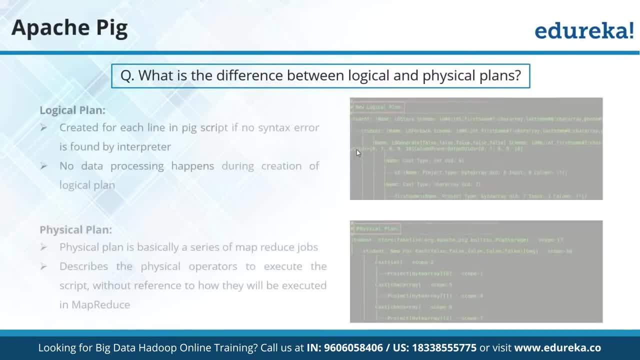 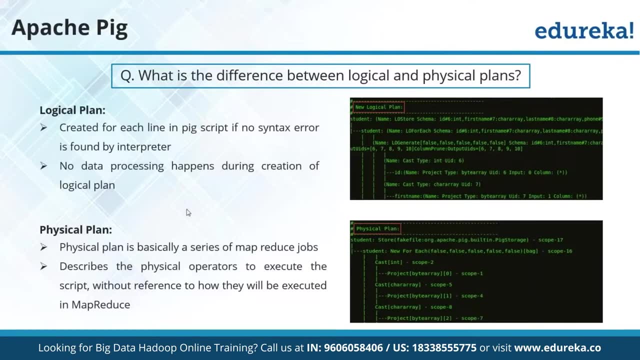 Whenever you are executing statement by statement, okay, It is just executing the statement, nothing In that case? first, it creates a logical plan. Means, let's say, if there is no error, right, In that case, it is just creating a logical plan. 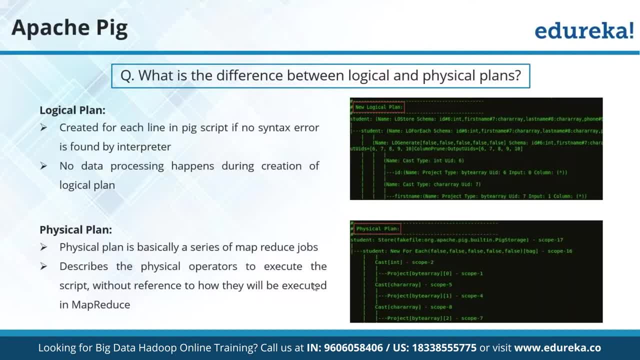 But when you do dump, right, When you do dump, then only the execution start right Because of lazy evaluation. Then your logical plan right. Then your logical plan right, Then only the execution start right Because of lazy evaluation. 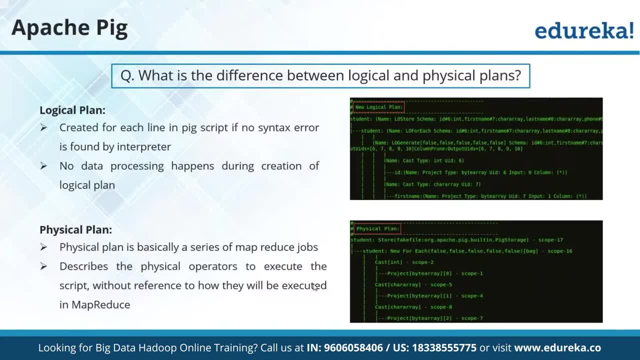 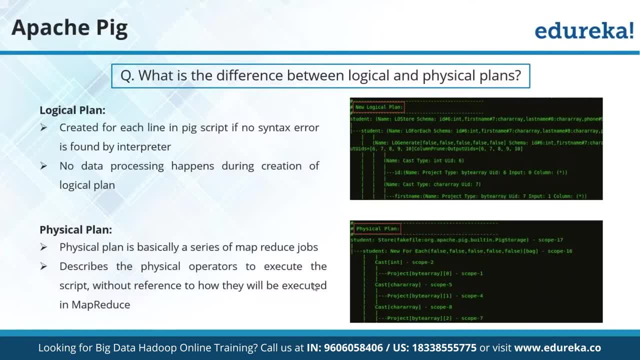 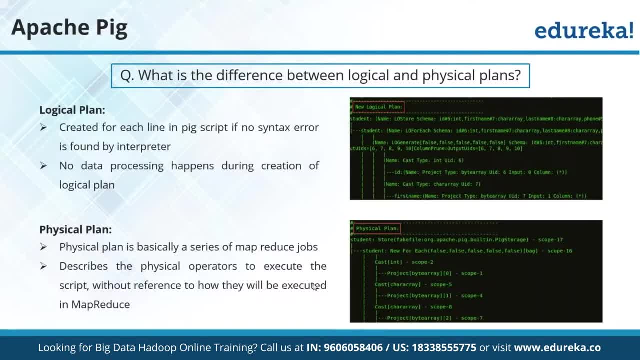 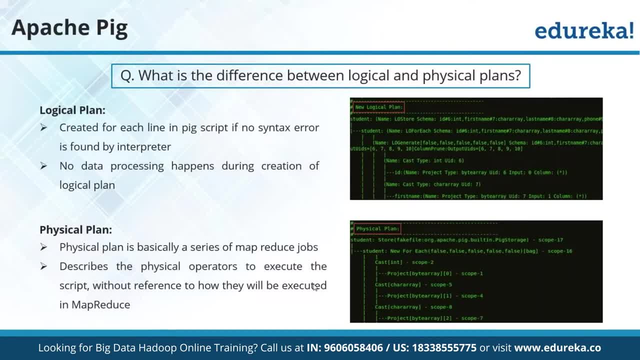 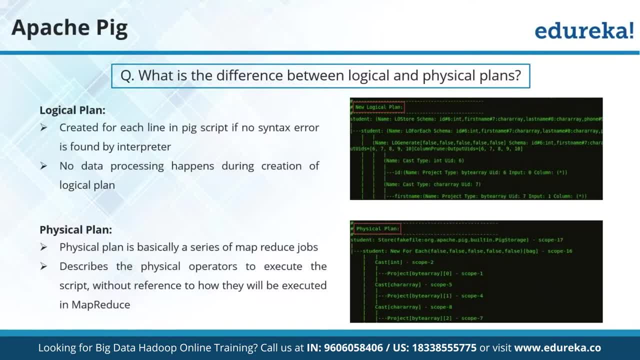 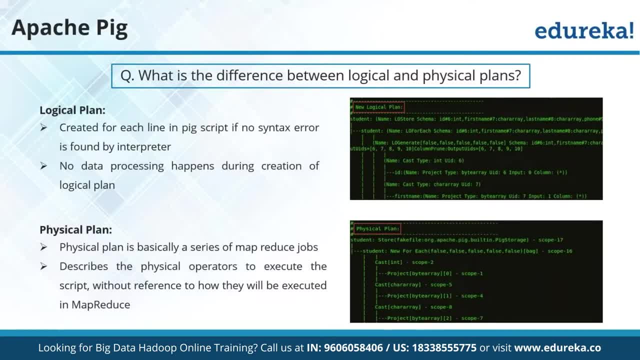 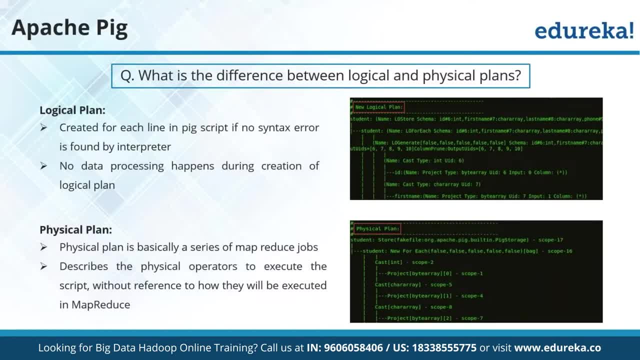 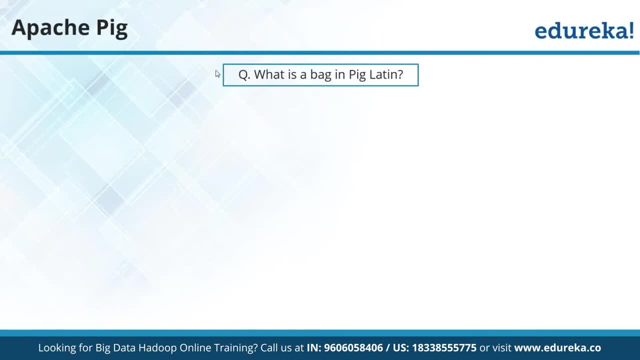 getting converted to map producer and by logical plan is at the initial level. okay, so that is what happened. can you tell me what is bad? what is bad? collection of tuples, very good, right. so basically, when you say a whole data file itself right, collection of tuples. if you notice. so let's say this is the data. 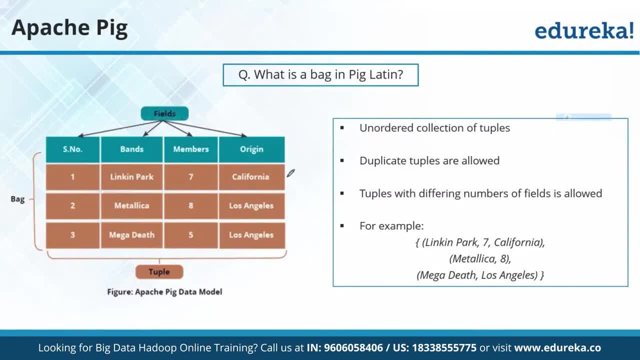 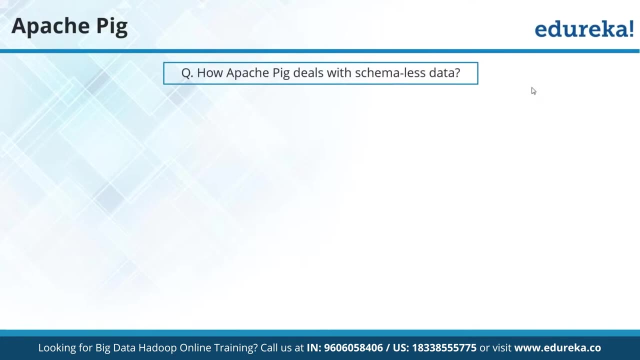 right, if this is the data. now, if you see, this is one tuple, this is second tuple, this is third tuple. so collection of all these things will be called as back. okay, collection of all these things will be called as back. now, how hive is only working with. like hive is able to deal with only structured data, but pig is. 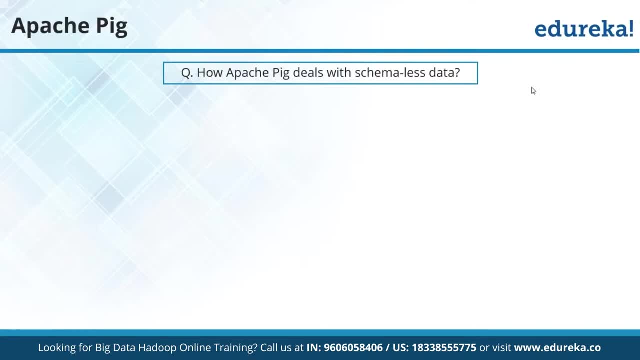 able to deal with unstructured data figures? how pig is able to deal with unstructured data? can I get this answer? how pig is able to deal with unstructured data? it is actually happening because of schema less part, right schema less part. basically, if you do not have schema, if you do not have. 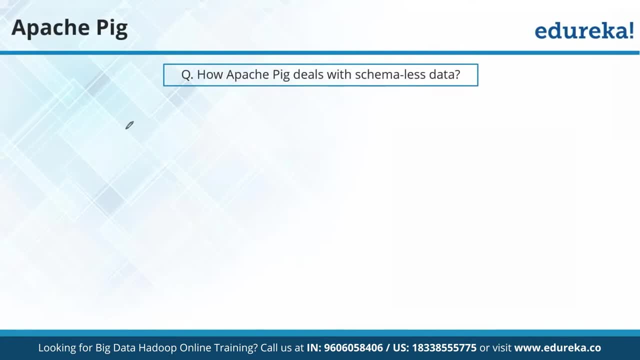 schema defined, then also pig can work what pig do is. let's say: you, you do not know, like in hive, you have column names, right. let's say: column name is age integer, all that right. so you need to define the column names. in pig there is nothing like that. let's say, if you do not know the column, 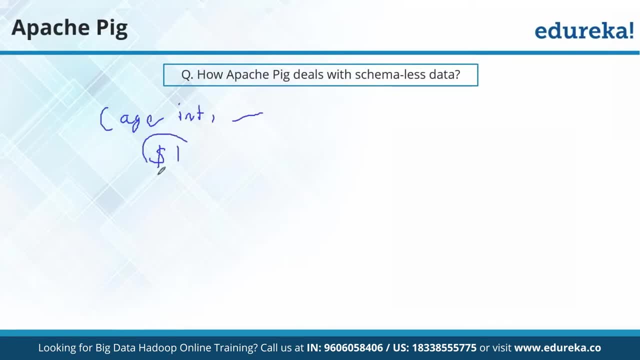 there is no schema being defined. you can define it like this: first column you can define the dollar one. second column, you can define with dollar two. so that's how you can also define. so basically, pig, you can define even your schema, less thing, okay. so you don't have anything. it will treat it like null. it will start treating. 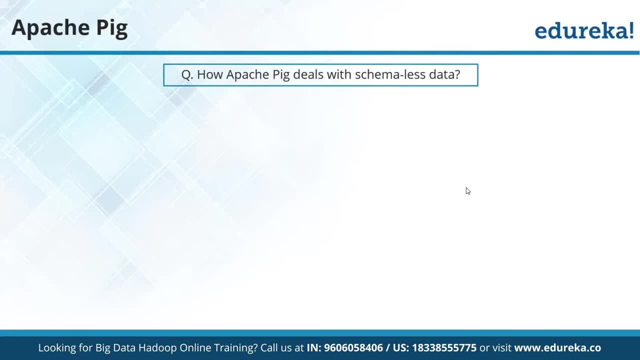 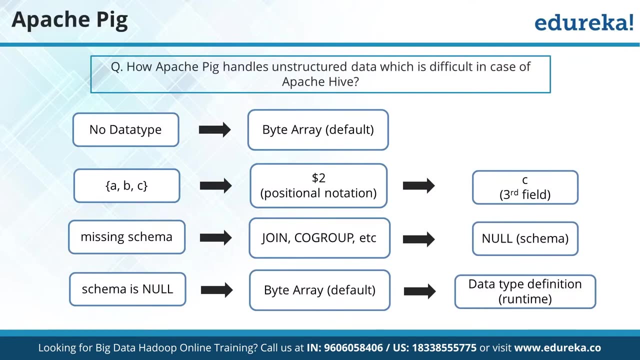 if you do not define data type, it will start taking get a buy. so basically pig kind of converts your values to a better way. so basically that's a reason you can physically go with pig with unstructured data. this is one of the major reason that pig can be even. 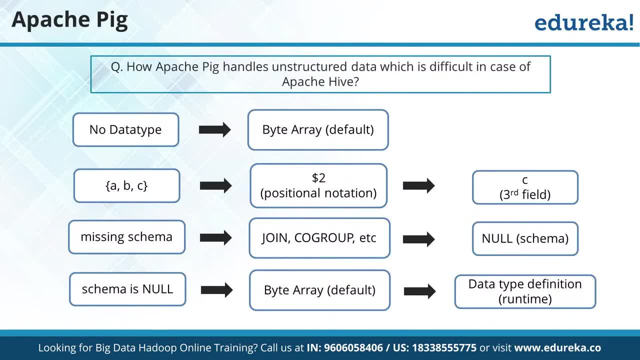 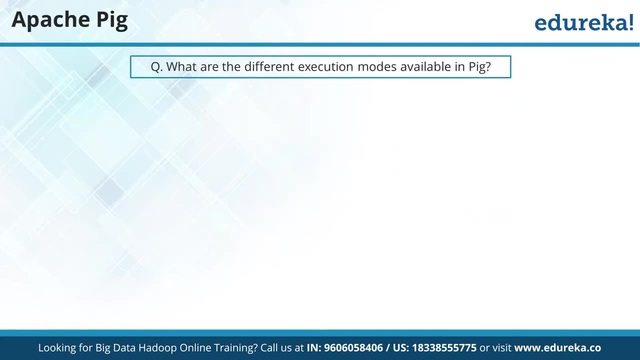 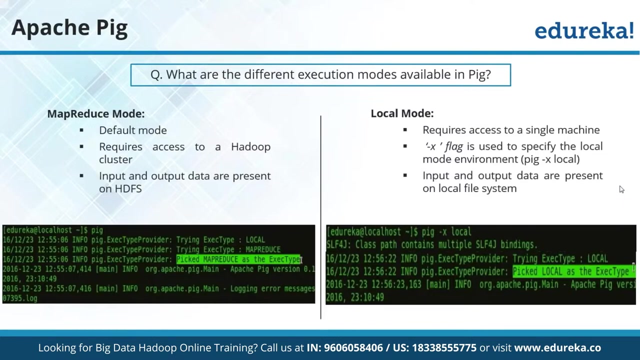 unstructured data while hive cannot do, because pig kind of converts the data or treat that data in this indifference way, right, like if you don't have column name, you can define this as dollar two, dollar one, all those things as well. what are the different execution mode available in pig? so there are two modes, right. one is: 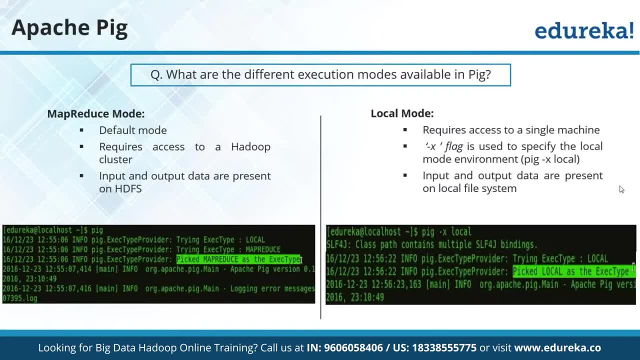 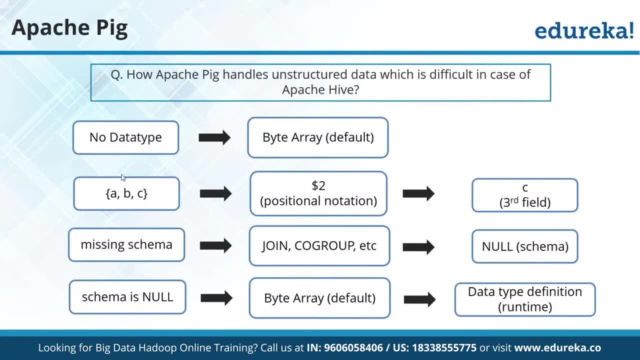 local mode. one is map reduce mode. yeah, sure, I mean into that. this is the same thing. I mean like: if you have no data, I treat it like byte array. if you don't have column, it start treating a dollar one, dollar two, right one before. okay, this. 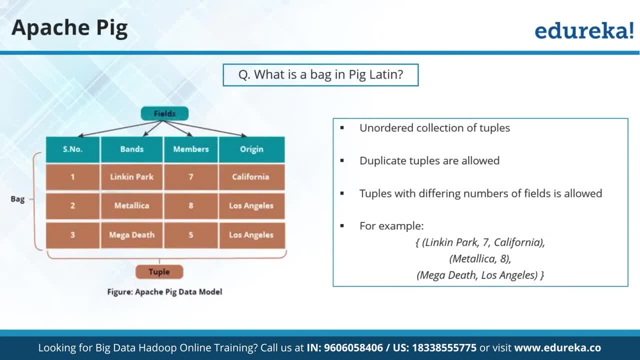 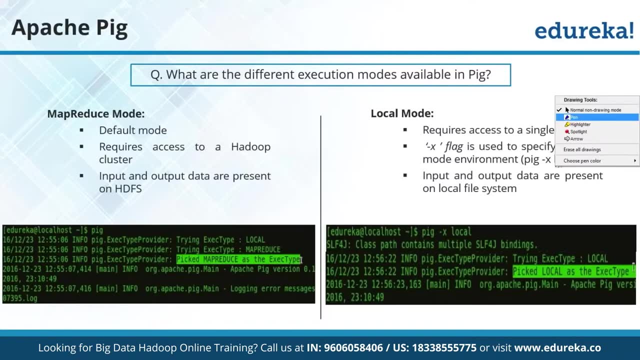 one back, got it now. wait, let's move further now. so there are two modes available. one is map reduce mode, one is local mode. so when you go with pig in map reduce mode, so when you just type pig right, it takes you to the grudges by default, it takes you to the map reduce mode, which 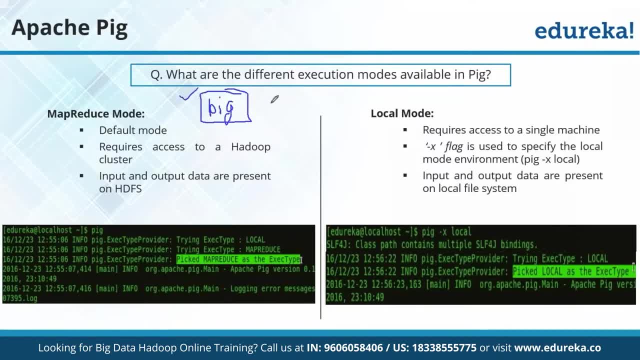 basically also states that that, basically, if we are going with map reduce mode, you are assisting your HDFS, while if you are using local mode, what you need to do you need to go like this: hyphen X- local. it will now take you as in the local mode. when you say local mode, 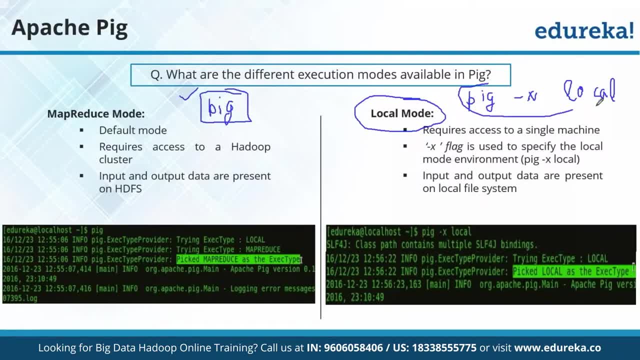 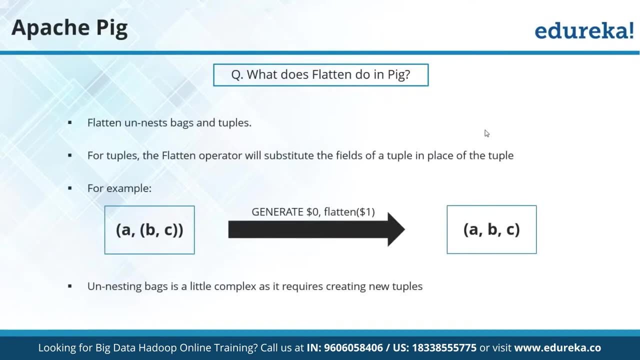 what basically happens here. it basically now start assessing the file from your local file system. now it is no more assessing HDFS, but it is directly assessing the data from your local file system. these are the two execution modes: flattening- this is very simple, right? so basically, flatten is the keyword available if you have this kind of data. 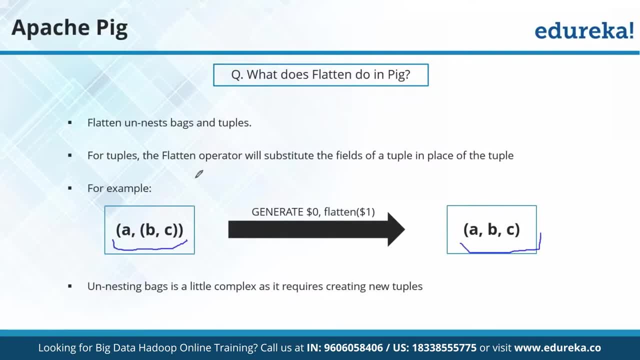 you can flatten in top like everything will come together in the land. so flatten is just an API. right, you can see this flatten. so basically it is this: basically converting this form of data to this form of data. okay, so this is basically meant by flatten. these are simple questions now. can anybody explain? 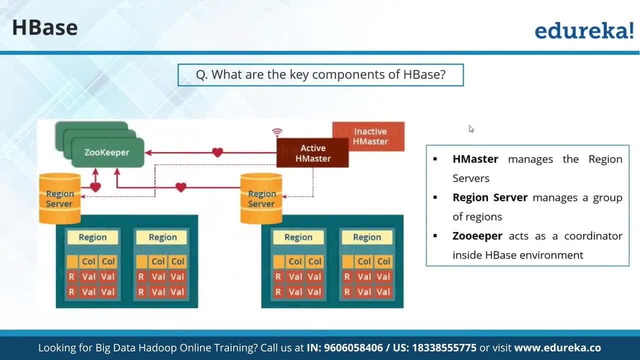 me this: X based components and anybody explain me these X based components, components, anyone who want to talk about it, HBase components- it's in front of you. can anybody explain me these components of HBase? you can start by one by one. this is the last topic. so, friends, I want everybody to be attentive here. so HBase keeps the data in a distributed 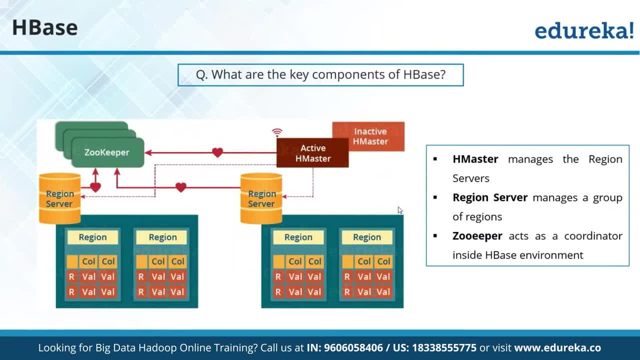 mode: right. so distributed mode where it keeps the data. it defines a region where it keeps the data, so, like, this will be your first region. this will be like region where you are keeping, let's say this: column value, row value: right, this is your one region, not together, just like how you. 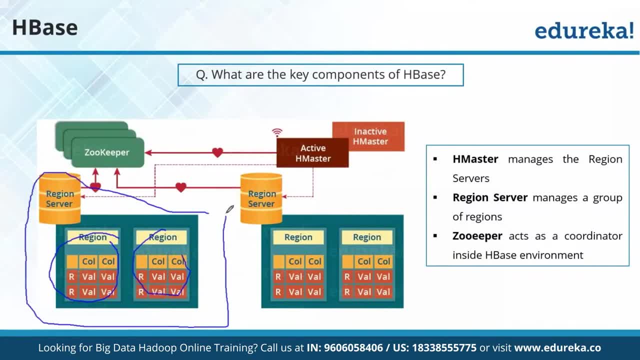 define rack right. you can define region service right where you are defining basically different different regions together. so this is one region server. this is one region server right now. what happens? the master will keep. basically your will be called as x master, like active master, just like your name. node works right. 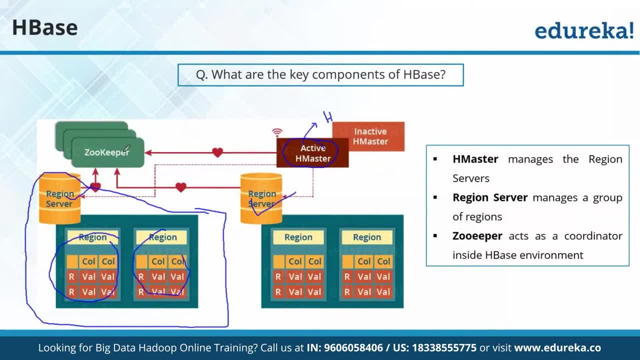 similarly, HBase uses this x master. what is this zookeeper doing here? zookeeper is kind of helping you to execute everything, so, like in zoo, what happens in zoo? basically, they keep animals. right, they keep animals. they manage multiple different category of animals. similarly, zookeeper like big. 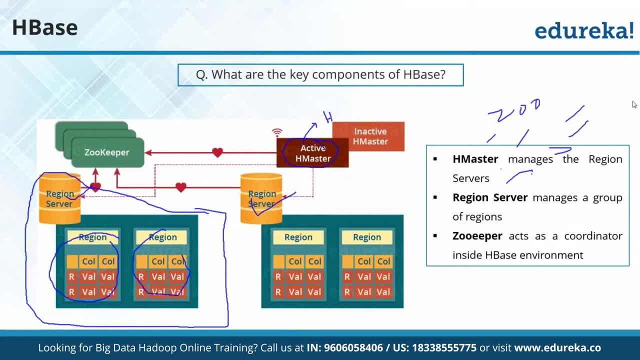 data also got so many tools available for you know, and basically it helps you to manage everything up. so zookeeper maintains lot of things for HBase. it kind of helps you to basically kind of see that consistency is maintained, like in HBase, right when you work basically in your big data. 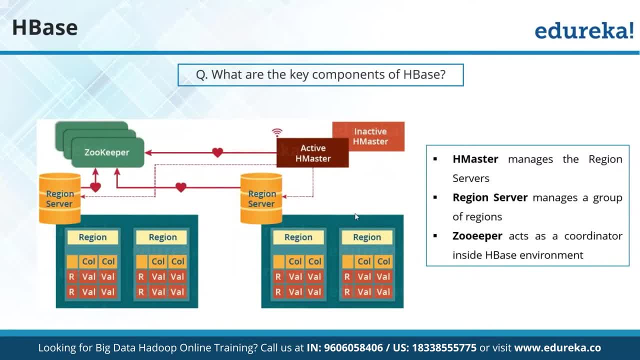 when you are working in hadoop now, you have name node, data node, all those things available. but when you are working with HBase you don't have all those things right. so in HBase you don't have concepts of name node, you are keeping data and all. so for that, to do this part like zookeeper. 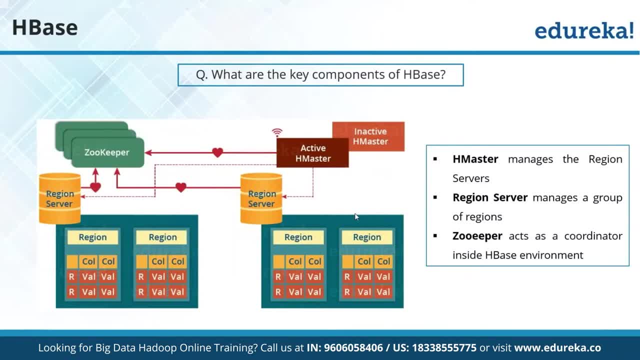 play a major role here. so zookeeper is kind of going to act like a coordinator in your HBase environment. okay, it will help you to coordinate all the things, because here we don't have name node, data nodes, you know so and there is no yarn, basically, so you can treat it like. 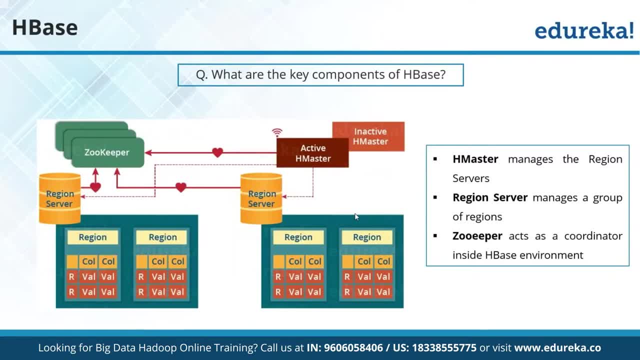 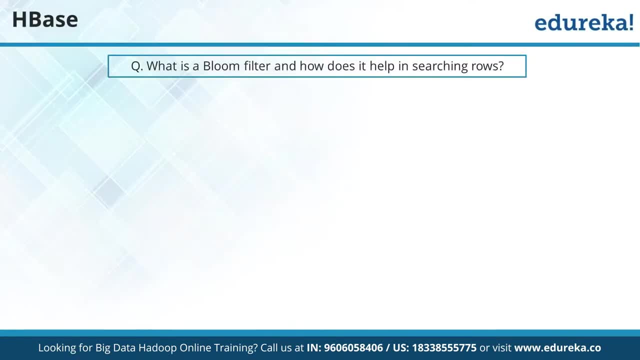 basically just like how yarn was handling things. it is going to help you as a coordinator. it also maintains the directory structure, you know. can anybody tell me what is bloom filter? bloom filter- anyone know what is bloom filter in HBase? can i get this answer? what is bloom filter? 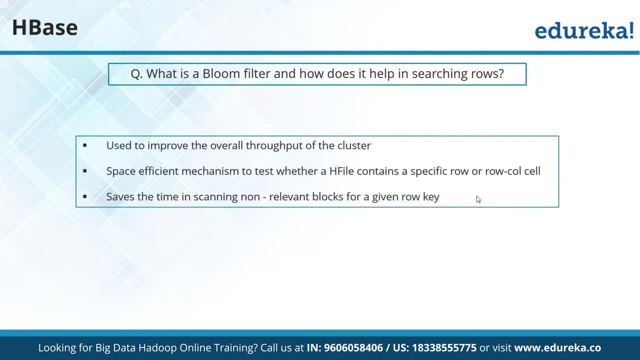 basically, it helps to improve the overall throughput of your cluster. it helps you to basically improve the performance. okay now, if you want to search any specific row column cells, it also helps you to do that. so it makes your system very fast. so that's, that's what you need. 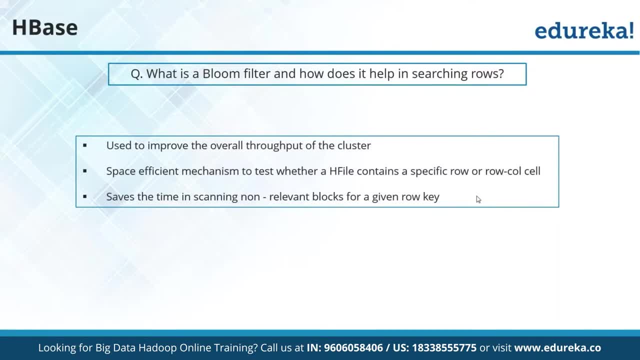 to just enable this and if it is enabled it it kind of improves the throughput of your cluster. this is the role of your cluster. so it is very good. simply, it suits you. but you can also. you can even invert, like, say, if you want to do a circuit, you want to use a microgrid or you want to use a grid, you can. 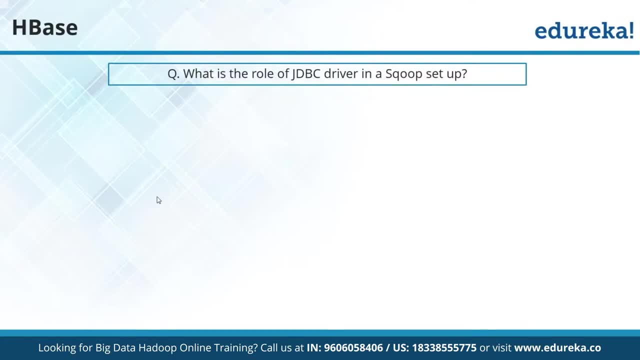 either do this, so so do that and use the blue filter in HBase. coming to the next question: what is the role of jdvc driver in a scoop setup? simple, can i get this answer? this is basically scoop R important topic in interview HBase. I would still say that 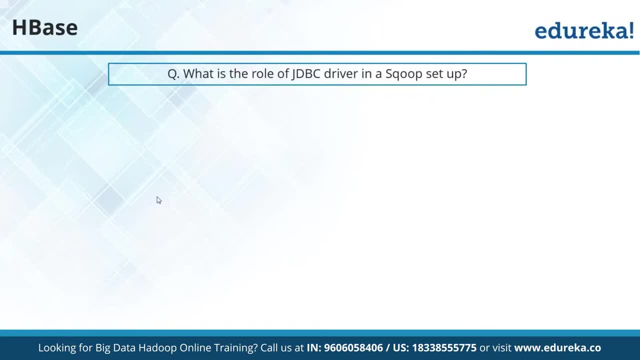 they are not very important. these. this people do not ask questions on NBase, but definitely the scoop topic is very important. very good, are you going to answer me? HBase, i would still database I want to connect now. basically, RDBMS can be of any type it can be. 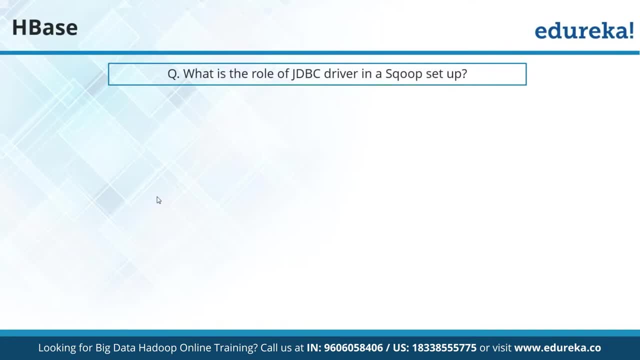 MySQL, it can be. it can be MySQL. it can also be your Oracle DB. it can be DB2, right? so JDBC driver will be common and can be used for any of your things. so this will basically help you to create a connection with any sort of RDBMS system. this is a very famous question. what's the difference between? 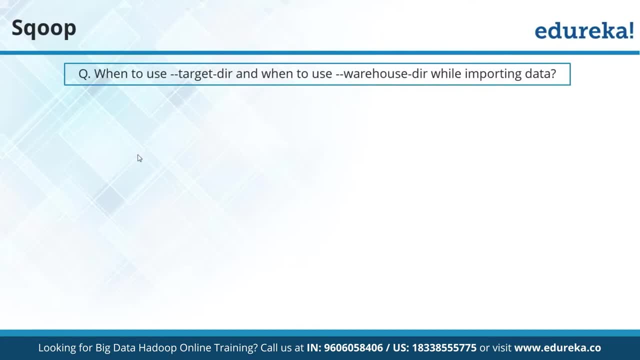 hyphen hyphen target DIR and the difference with warehouse hyphen DIR. hyphen hyphen target DIR with warehouse DIR. this is a very famous interview question for school because both will basically help you to put the data in as some HDFA specific location. then what's the difference between them? 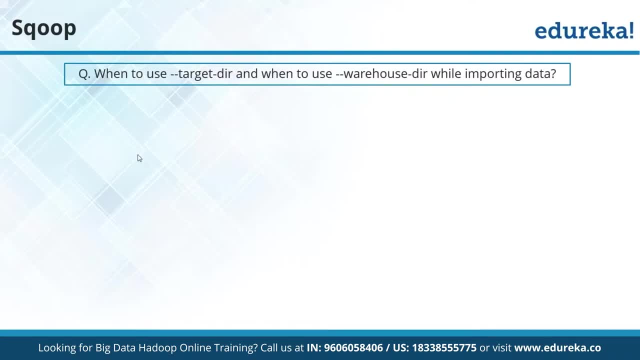 very good, not so porting all table, and alls fine that you are giving me a use case customer. I want basically a proper solution, means what's the difference between them? is defined. No, Rajesh, what happens in target DIR is in target you DIR, if your defining target DIR. 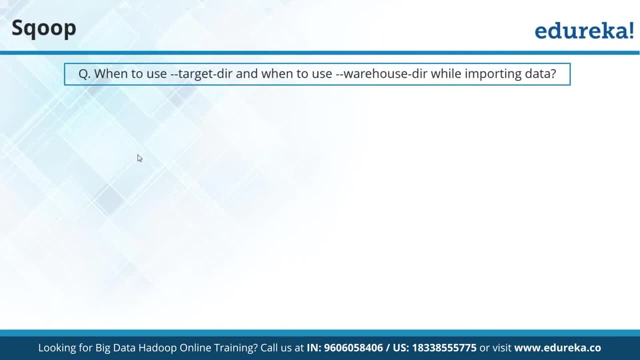 you need to give the directory path name. okay, so you need to give the directory path name- name where you will be keeping data. so it is possible. let's say in your MySQL or in RDBMS. let's say you have table called as accounts, but now you 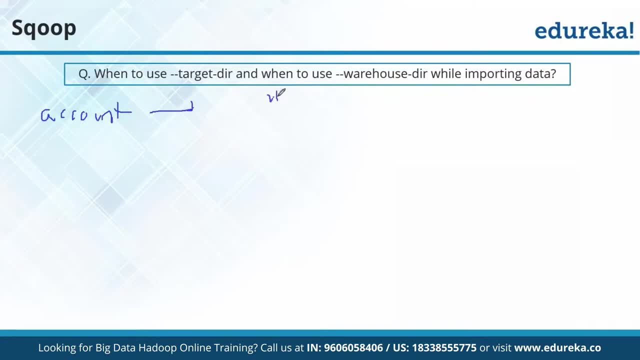 want to import this table to your HDFS using the school now by. if you give target dir, you need to tell the name of the HDFS directly where you will be keeping this. so now you can change this name of HDFS from accounts. so let's say: 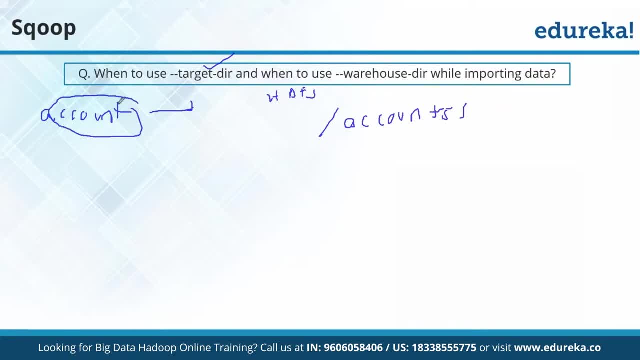 accounts one. you can do all that. if you are using target dir, you can change the name of this account to accounts one in HDFS. but if you are using warehouse dir, in that case whatever the name will be there in your RDBMS, same name will be. 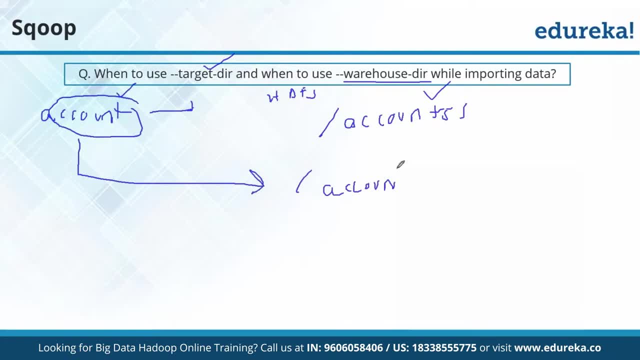 created in your HDFS, same name will be created in your HDFS. no change with that. okay, so that is one of the major difference between them. so warehouse dir will maintain the same name, while with target dir you can keep the same name or different name as well. so you have force to basically give the name of the HDFS folder where. 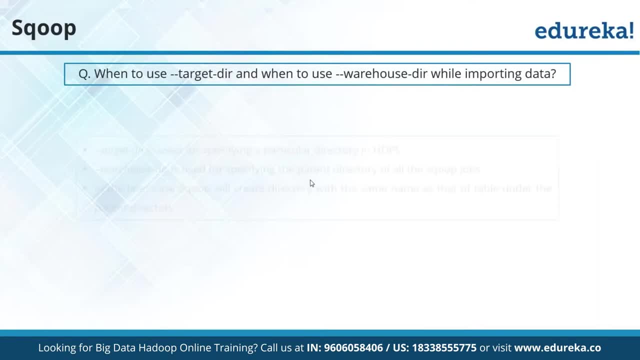 you want to import, while in warehouse dir, that's a different thing. now, can you tell me what this query is doing here? read this query and tell me what this query is doing here. incremental data: no, no, you can update that data, so what you can do is that you can write the data. 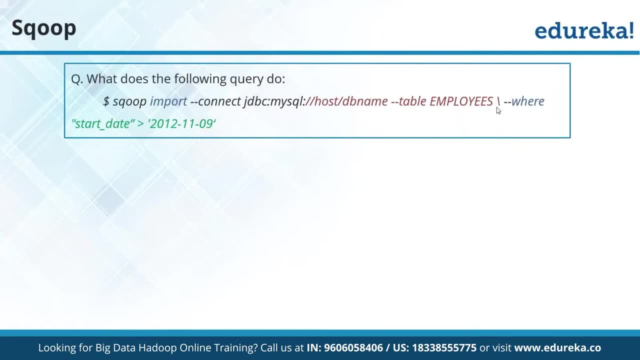 data into this table and you can upload it into port mode, like this, and you have the data in the port mode, and that's what you are doing. you want to do is you want to send it to the set up position, and that's what you want to do. and then 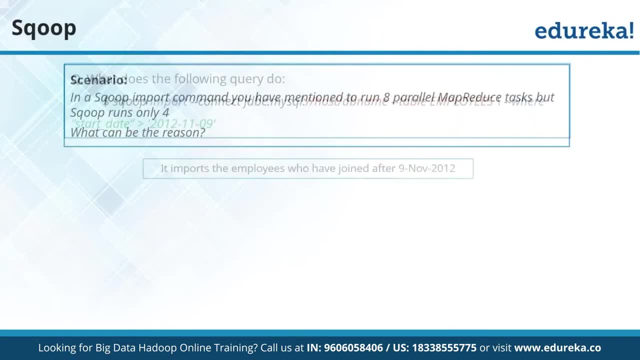 when that data is not created. you want to put it in this state, where it will have a space, where it will be ready, because you want to put data in this place. okay, okay, produced task, but scope is only running code. what can be the reason? what can be? 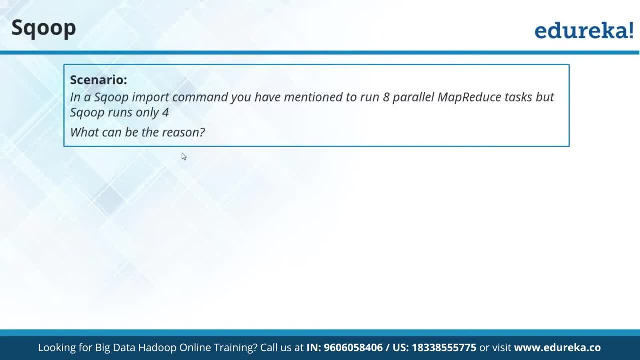 the reason. very good, very good, Ansiba. yes, because maybe your number of codes are not allowing you to run 8 tile less than produced, right? maybe you have less number of codes itself. in that case, scope will not be able to take you up to 8 tile less than produced. 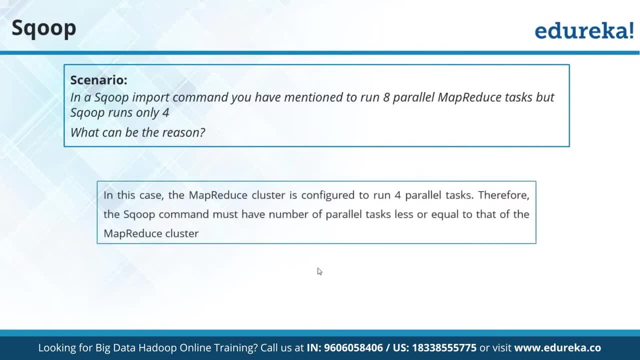 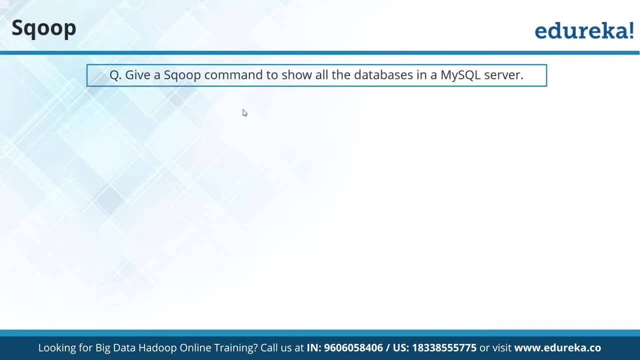 task right. it will only use less number of code. so basically, if your codes are less, in that case this is bound to happen. give us scope command to show all the databases in the MySQL server and you give us scope command to show all the databases in MySQL server. it should be simple. 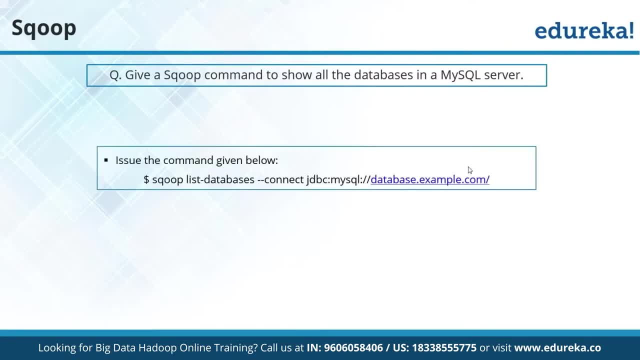 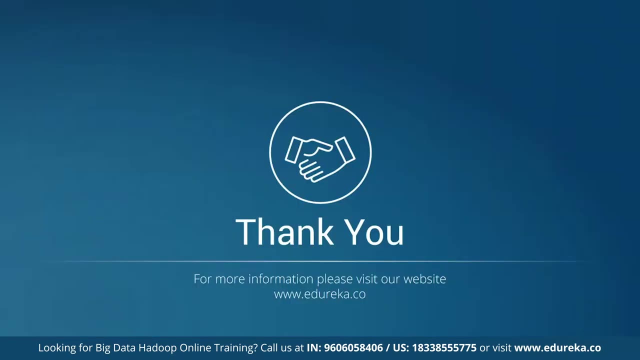 see this: scope: list databases, not show databases. list databases become okay. hyfind, hyfind, connect, give the connections. that's it will list all the databases. that's it. this will list all the the databases. okay, so those sessions will be very useful for all of you. thank you everyone for. 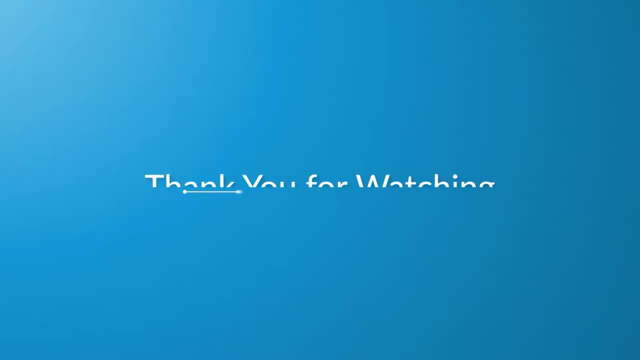 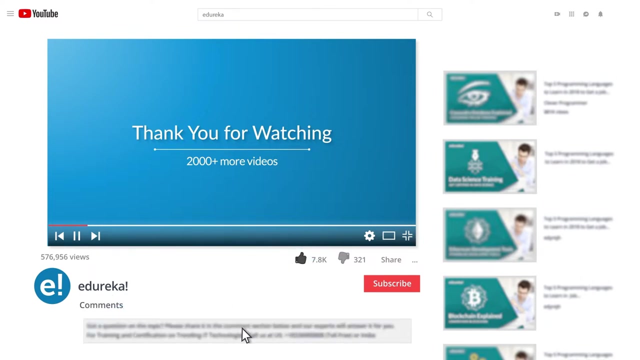 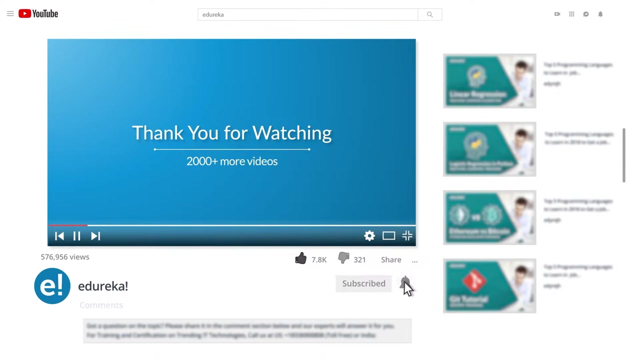 making it interactive in a nice session. i hope you have enjoyed listening to this video. please be kind enough to like it and you can comment any of your doubts and queries and we will reply them at the earliest. do look out for more videos in our playlist and subscribe to edureka channel to learn. more happy learning.